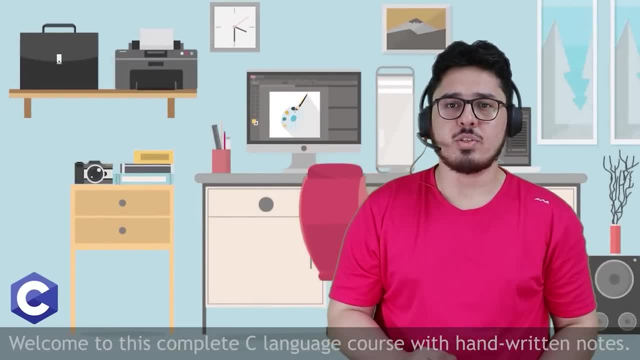 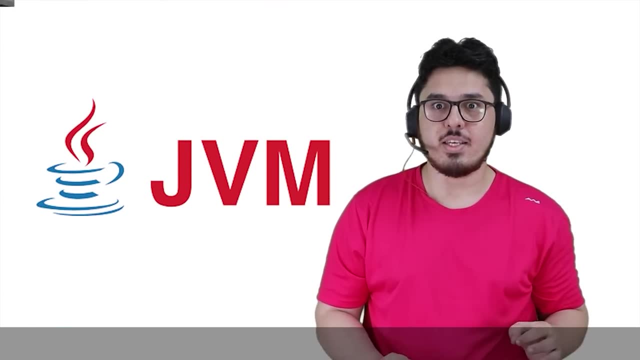 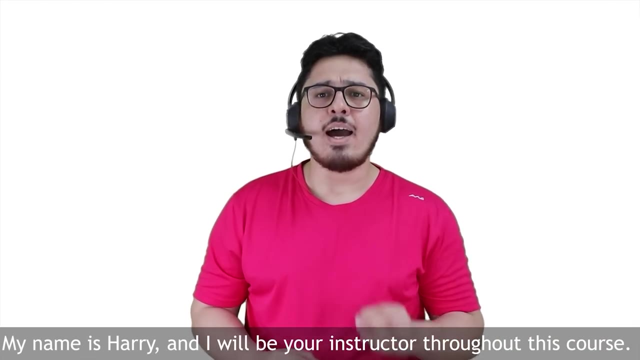 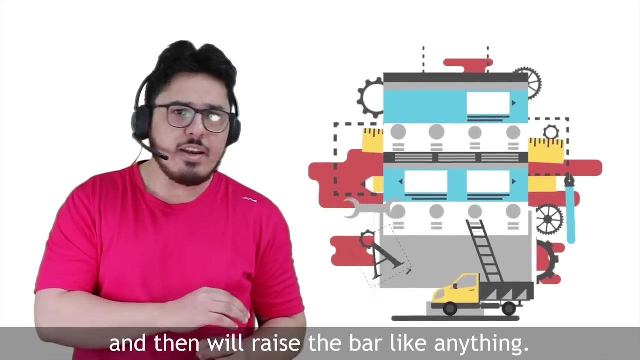 Welcome to this complete C language course with handwritten notes. C is known as the mother of all programming languages. In fact, a lot of compilers and JVMs are written in C. Whenever it comes to programming, C language is considered as the best to learn for beginners. My name is Harry and I will be your instructor throughout this course. We'll start from the basics of C, In fact, from the basics of programming, and then we'll raise the bar, like anything. We'll learn about pointers, We'll learn about functions, We'll learn about dynamic. 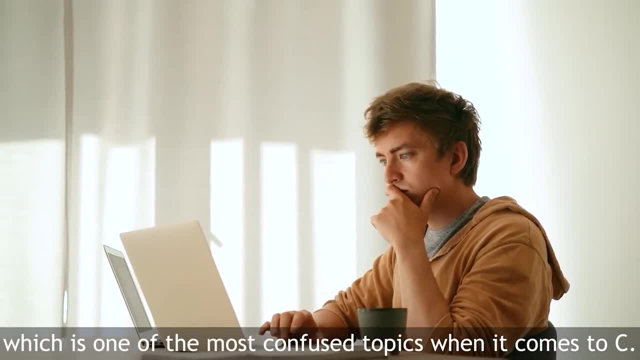 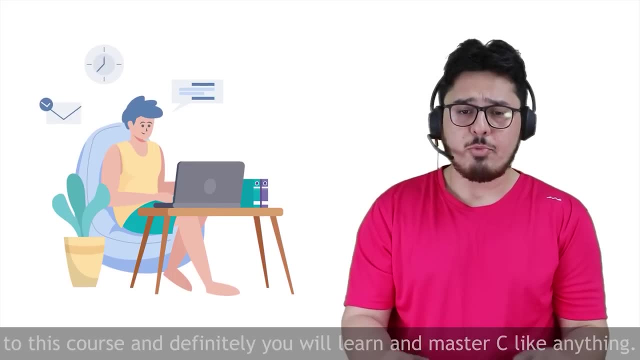 memory allocation, which is one of the most confused topics when it comes to C. The only prerequisite of this course is your time. I just want you to come here, devote some of your time to this course and definitely you will learn and master C like anything, If you want to support. 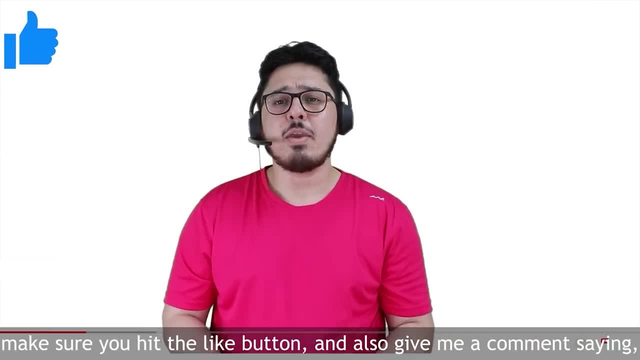 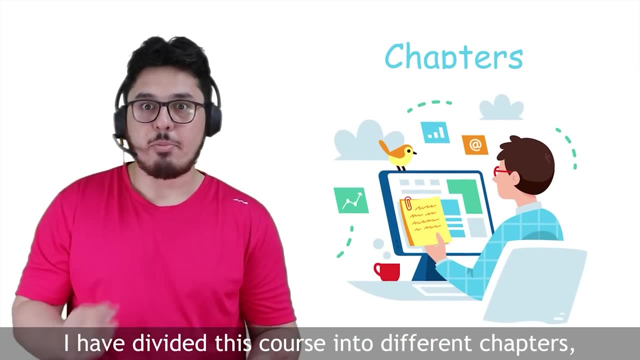 this initiative. make sure you hit the like button and also give me a comment saying this C language course is helpful. That would mean a lot to me. I have divided this course into different chapters. Each chapter has its own practice set, which makes it easy for you. 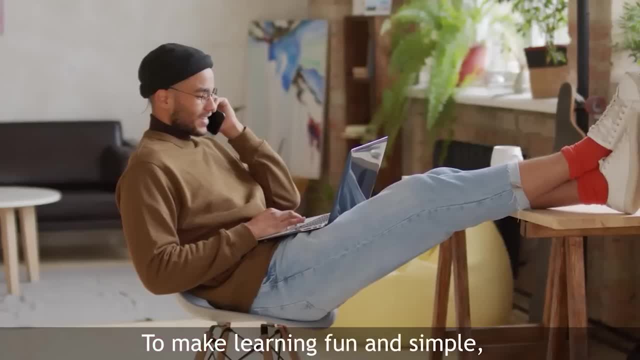 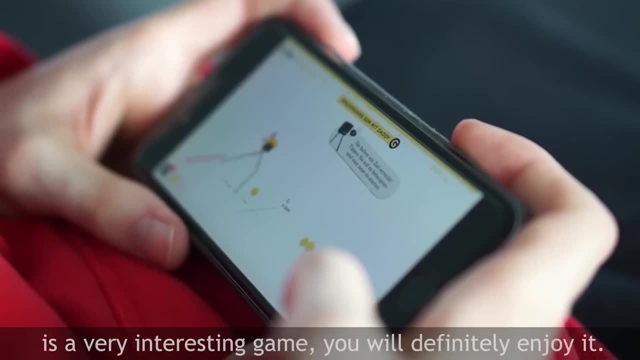 to practice about the topic discussed in that chapter. To make learning fun and simple, I have also included some projects for you, And one of the projects we are going to do in this course is a very interesting game and you'll definitely enjoy it. When I started, 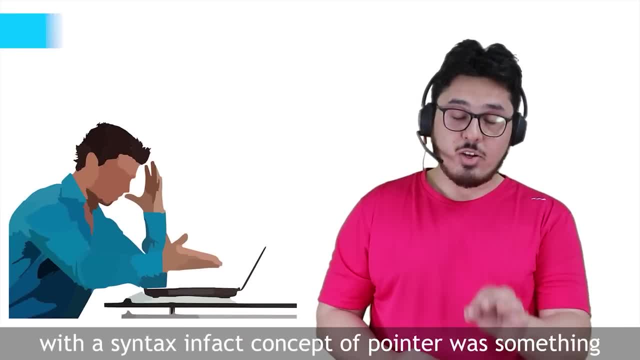 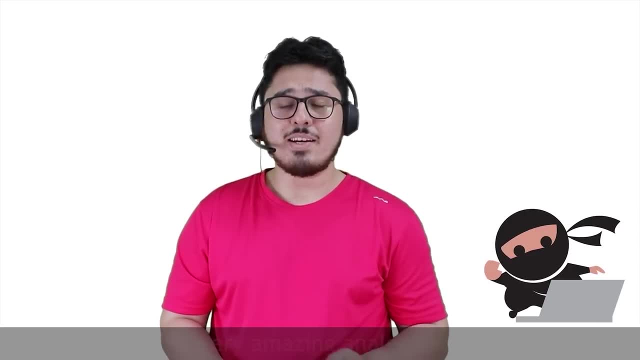 learning C, I was really very confused with the syntax. In fact, the concept of pointer was something I was not able to wrap around my head. But there were some of the tips and tricks that I used and some of the very amazing analogies which helped me learn C in a very 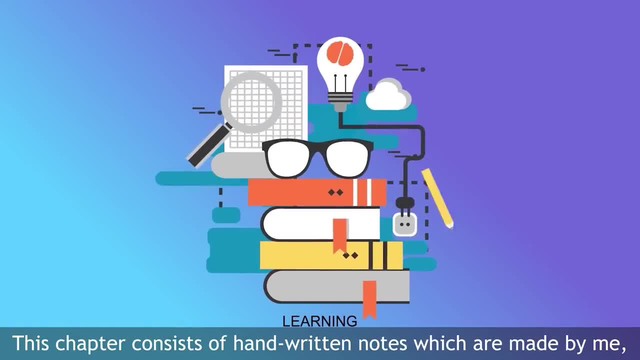 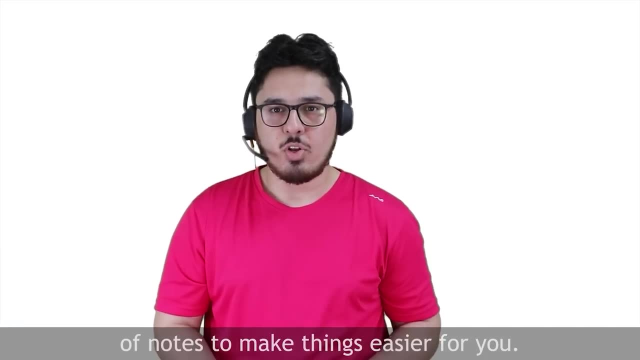 very beautiful way. This chapter consists of handwritten notes which are made by me. I have used different colors in the notes. I have written each and every chapter in the practice set of the note to make things easier for you. Not only that, I have also included a cheat sheet with this. 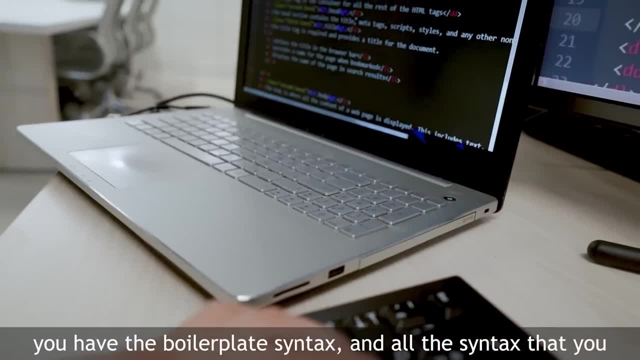 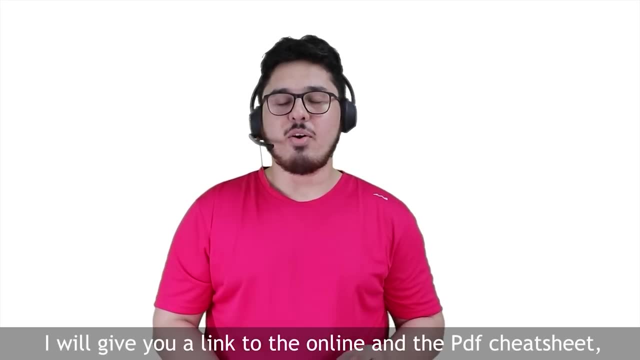 course, so that after you are done with the course, you have the boilerplate syntax and all the syntax that you want to use in your C programs is single. I'll give you a link to the online and the PDF cheat sheet Along with the cheat sheet. 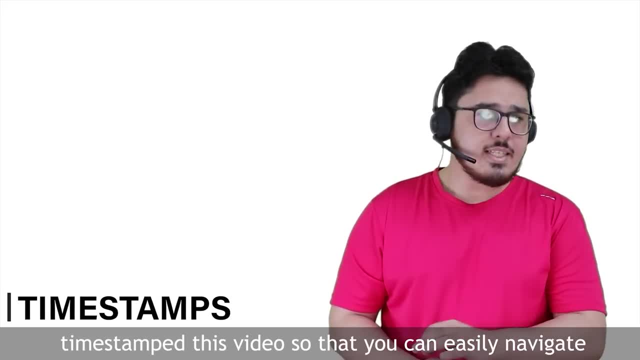 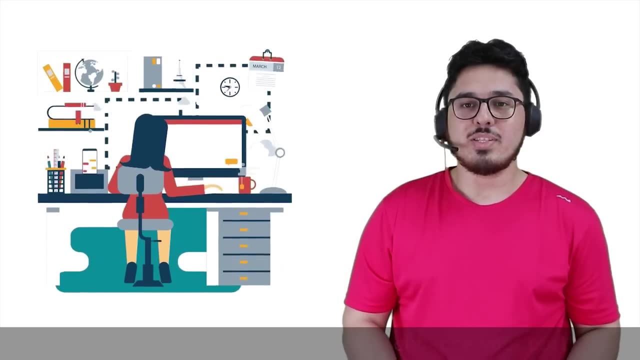 and notes. I have also timestamped this video so that you can easily navigate to the different chapters and you can easily learn C programming language. The projects that we are going to do in this course can be added to your GitHub profile to enhance your portfolio. Do not 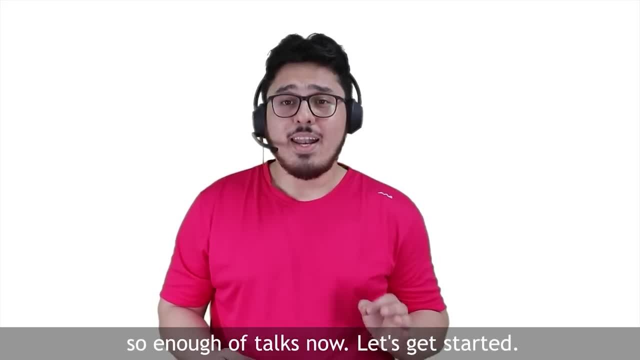 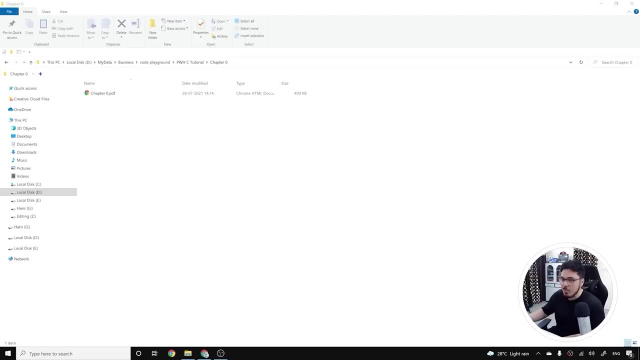 forget to add them to your GitHub profile. So enough of talks, now let's get started. So I am inside my computer screen. Let me be very honest with you guys. This course is very, very beautifully structured. I have created notes for all the chapters and we have around 11. 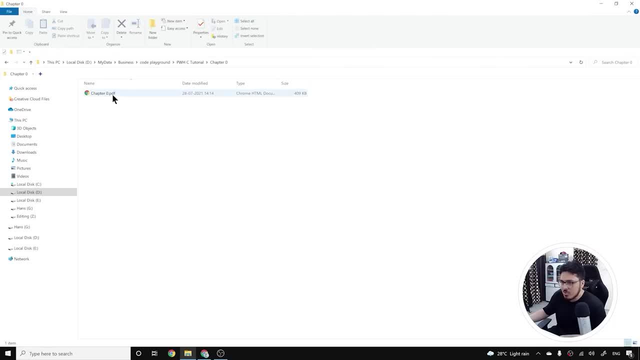 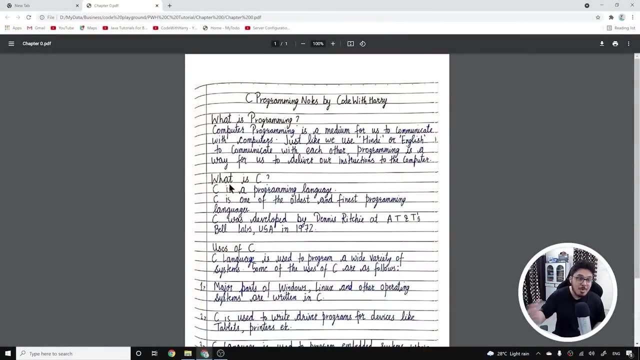 chapters and two projects, And this is going to be fun. So let's open chapter number zero, where I'm going to give you introduction on what exactly C programming is and what exactly programming in general is, Because if this is your first language and you have not seen programming, or maybe you 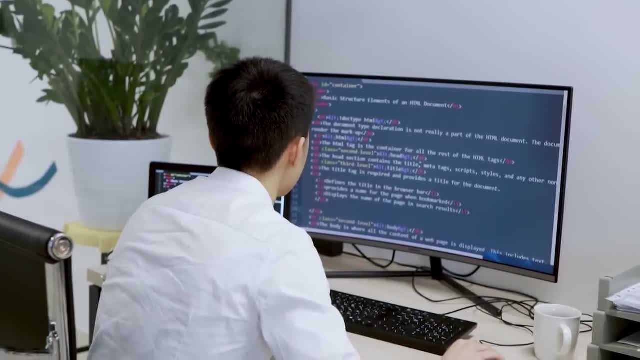 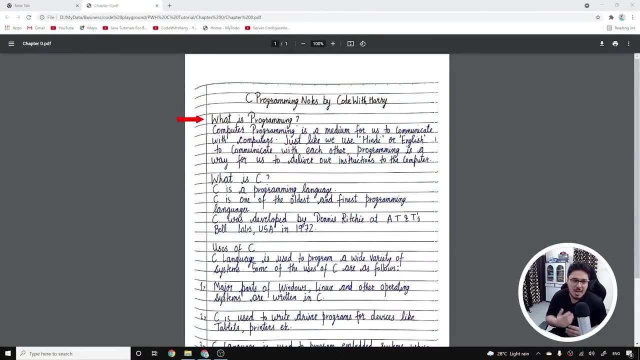 haven't written any program in the past. this course is going to be the starting point. So what is programming? It's a medium for us to communicate with computers. So, just like me and you are communicating, we are communicating with the help of a language which is English. I'm using English language to 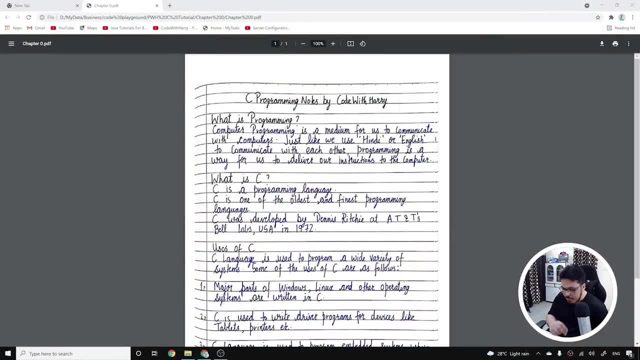 express my feelings to you. I'm using some English words which you can understand and take actions on. For example, if I say please come here, you can come here. If I say please go to the market, you will go to the market and all those things. So we have a computer and computer can be a. 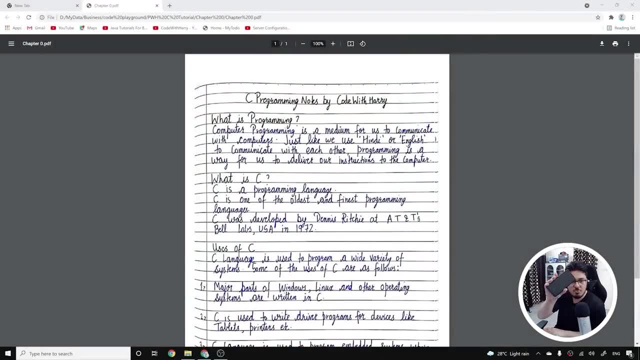 desktop computer, a laptop computer, This phone as a computer. This is also a mini computer, So we can give instructions to the computer. It can be of any form. It can be a chip of this size or a phone of this size or a laptop of this size. 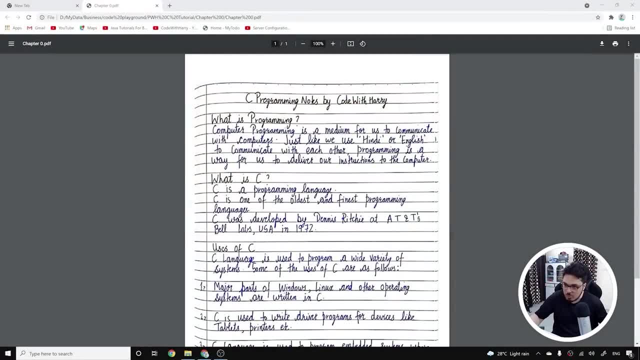 Irrespective of what your computer is, you need a medium to talk to the hardware, and that medium is programming. So programming can be seen as a medium for us to communicate with computers, just like we use in your English to communicate with each other. Programming is a way for us to deliver. 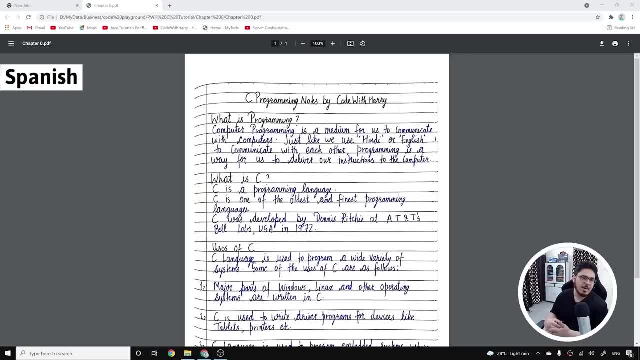 instructions To the computer. you might use Spanish, You might use touch, You might do some other language. Irrespective of what language you are using, you are simply using it as a medium to communicate with the other person, Just like that. we use C programming language to communicate with our computers. So what is C? C is a programming language. It is one of the oldest programming languages. It is called mother of all programming languages for a reason. A lot of JVMs and compilers are written in C. operating systems are written in C. 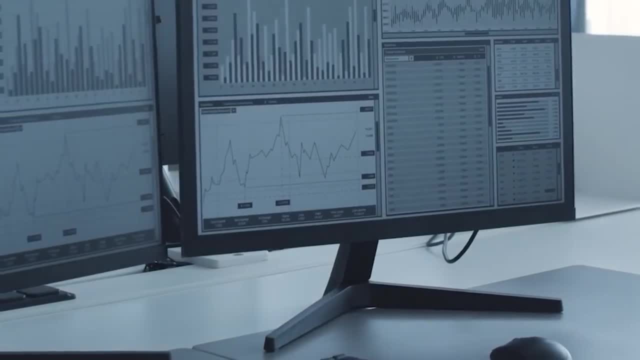 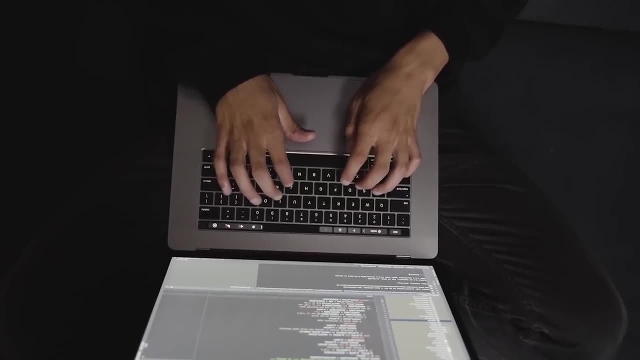 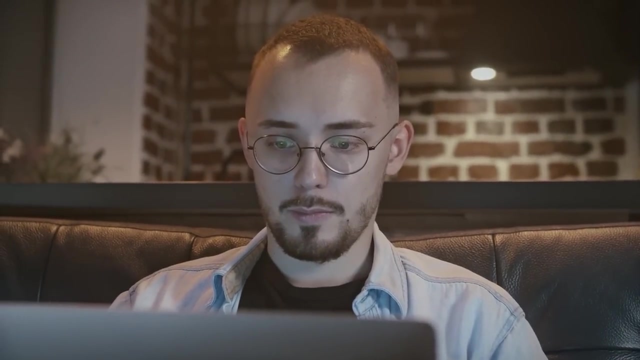 operating systems are written in C. a lot of low level stuff is written in c, so c is one of the most important programming languages and this is said to be a programming language which all the computer enthusiasts and computer software engineers must learn. so c is one of the oldest and finest programming languages. he was. developed by dennis richie at at&t's bell laboratories in 1972. you don't have to remember this. i remember this just because i've seen or read this statement a lot of times. but you don't have to remember this, but remember the name of dennis richie. he indeed brought a revolution to 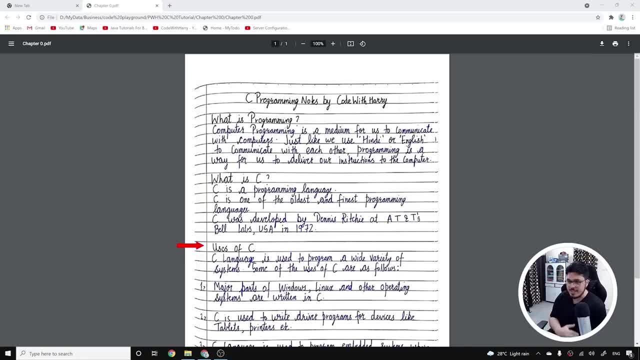 the world of programming. now let us talk about the uses of c. what exactly are the uses of c? where would you want to use c programming language? so c language is used to program a wide variety of systems. some of the use cases are major operating systems, linux, and there are a lot of other linux. 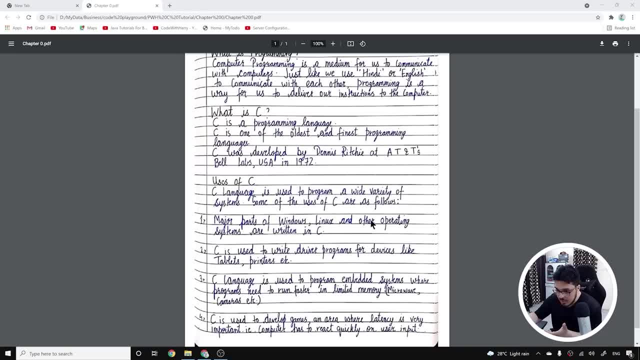 distributions which are written in c. so we use c to write an operating system which controls all the hardware of our machine. so c is a very important language. now let's talk about driver programs. c is also used to write driver programs. let us say: i have a device, it's a camera. it can be a printer, it can be. 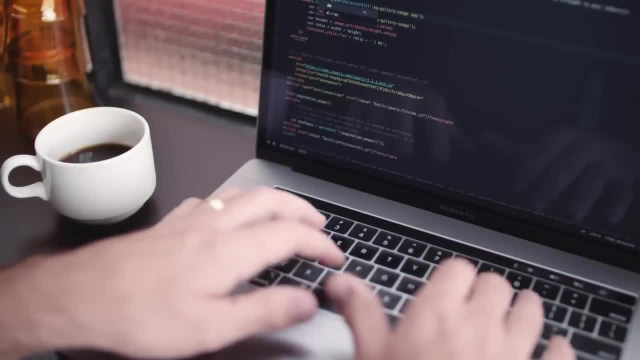 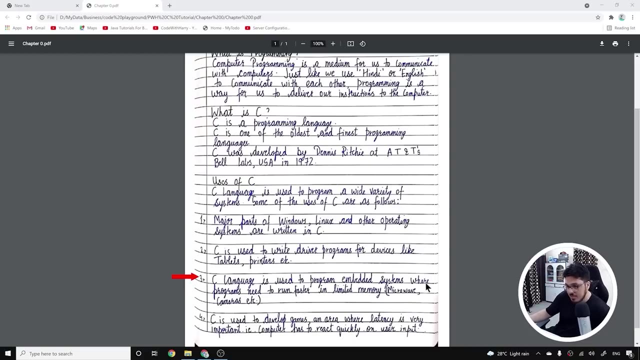 uh, it can be a chip. i can write device driver software using c programming language. now c programming language is also used to program embedded systems where programs need to run faster in limited memory. see, there are a lot of programming languages in the market. we have python. all these programming languages are good for one task or the other. c is good and c is famous to run. 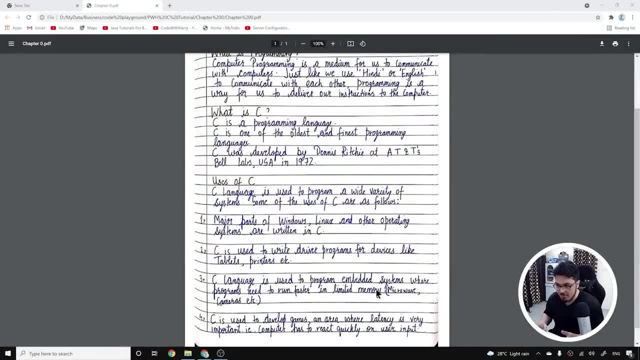 faster in limited memory and wherever we have limited memory, wherever we have embedded systems, a microwave, a very small chip, something that needs to run in milliseconds, is written in c. now, c is something that is very, very close to the hardware and it is one of the most loved language. 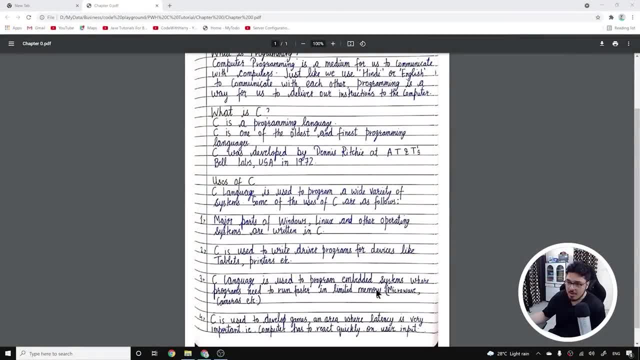 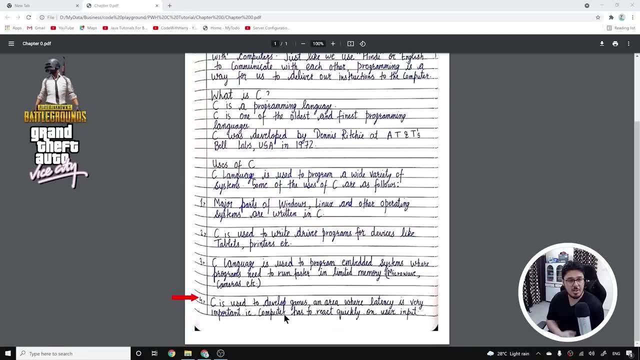 by those people who want to have a lot of controls in hand. now c is also used to develop games, an area where latency is very, very important. if you have played pubg or gta vice city, gta san andreas, gta 5, cyberpunk, we all play games. 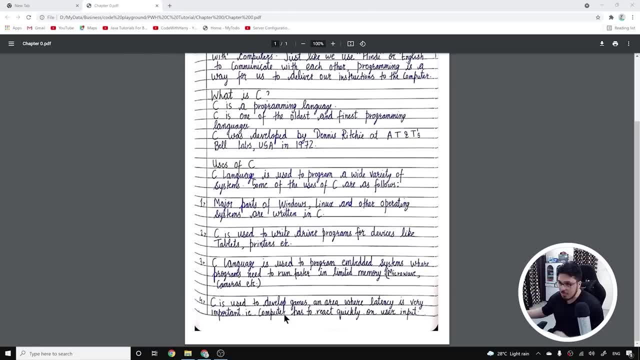 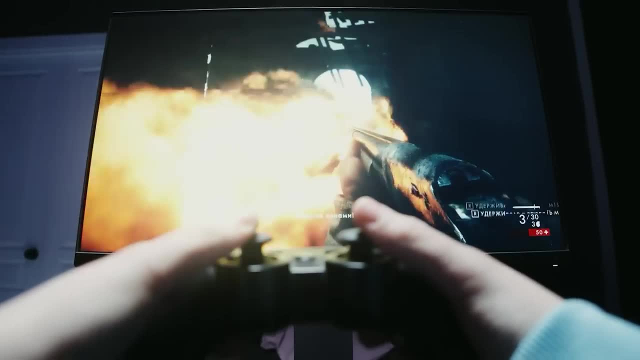 right, we all play one or the other game in our phones. sometimes the latency is really very important, especially in the case when we have limited hardware and memory. when we have limited hardware, limited amount of memory, latency is really very important. can you imagine you are pushing a button and that button is kicking? 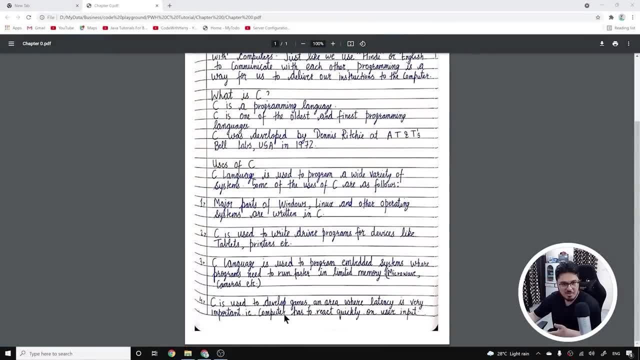 somebody in your game and that kicks actually takes place seconds after you press the button. you'll not play that game, you'll not enjoy that game. so latency is really very important in such games and c language is used to develop such games. it really reduces the latency and c is an amazing. 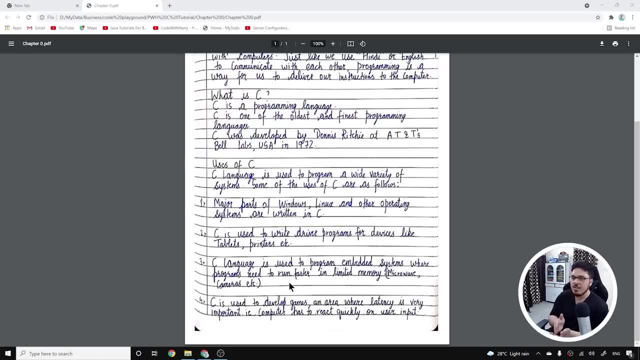 language. so we will start writing our first program. in the next chapter we'll see the building blocks of a c program. we'll see how c program is structured and how it looks and why we need to follow some of the best practices. we'll see all those things in the next chapter. let's move on to 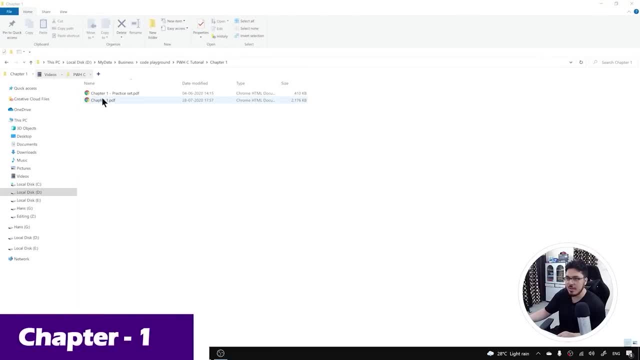 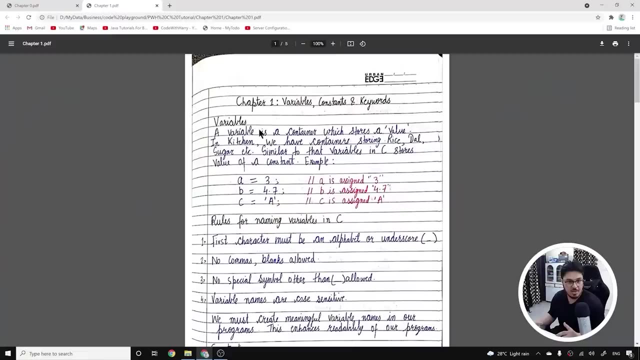 chapter one. now let's start with the first chapter and let's open this pdf. i have written this pdf with a lot of hard work, so please listen to whatever i'm telling you in this video very, very carefully and definitely you will become a champion of c within no time. let's now install a. 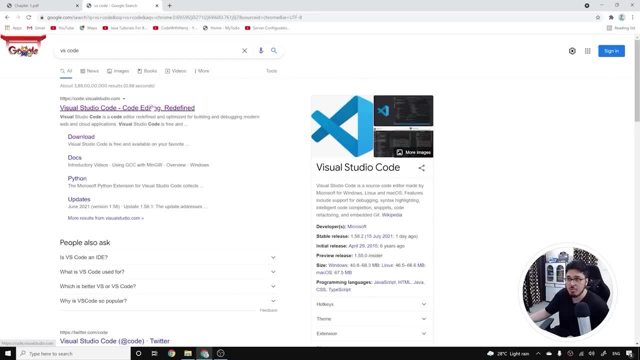 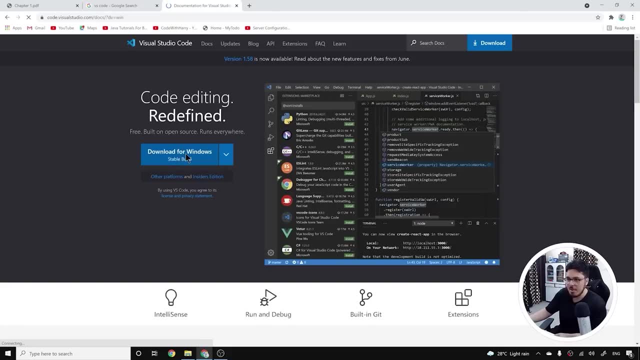 software called vs code. you must be wondering what vs code is if you are a beginner. but just follow along and see how i am downloading and installing visual studio code. you just have to download it. i'm downloading it for windows because i'm using windows. if you're using mac, linux or some other operating system, it should be available for your. 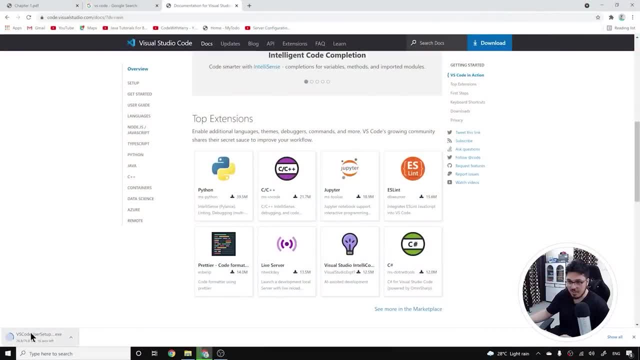 operating system. it's very famous and it is really very good and fast. so i'll simply install this vs code by clicking on this. it is going to take 10 more seconds. in my machine visual studio code has been installed, so i'll run it. i'll simply click next. but i'll not be able to click next until i. 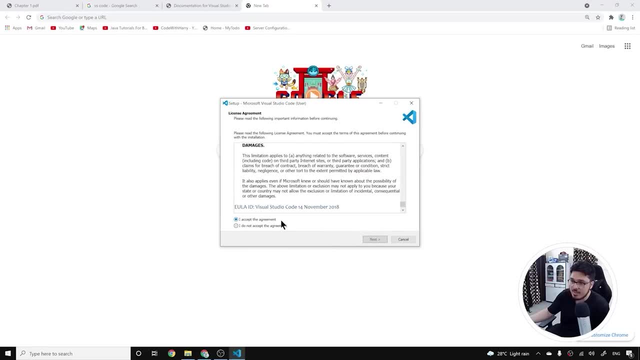 read this license agreement. i've read the license agreement. i'll click on. i accept the license agreement. i'll click on the license agreement. i'll click on the license agreement. i'll click on the license agreement. i'll go to next and make sure that these check boxes are checked. this is very 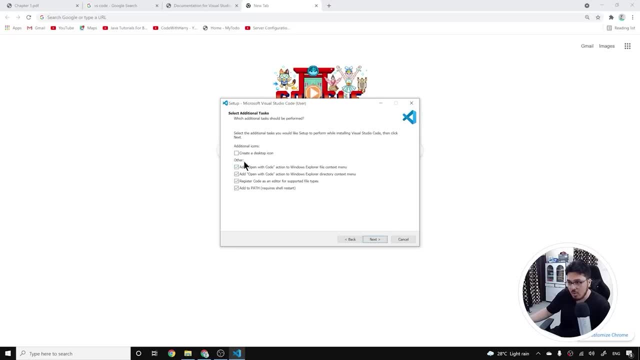 important, and i'll tell you why later. but make sure that all these check boxes are checked. you might want to create a desktop icon. if you want to create, you can check it, otherwise not. but these other check boxes must be checked. i'll tell you why. after some time, let's click on next. let's 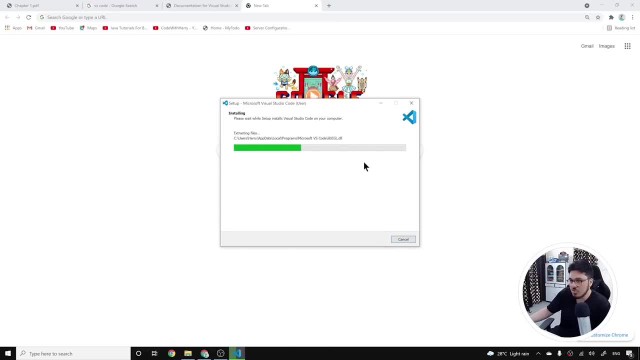 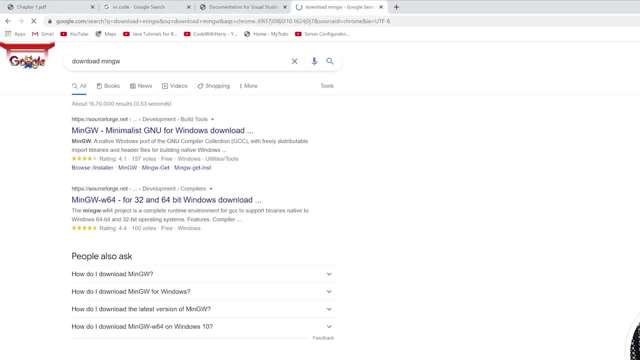 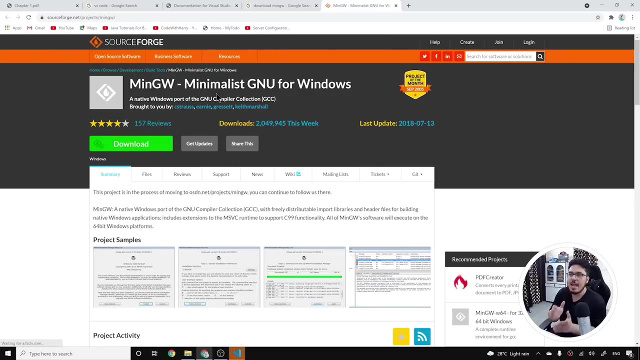 click on install and this is going to install visual studio code on my machine. so i'll wait for it to install and in the meantime, what i'll do is i'll say: download mint gw. now, what is this gw? it's a compiler that we are going to use, and this is something that will help us. 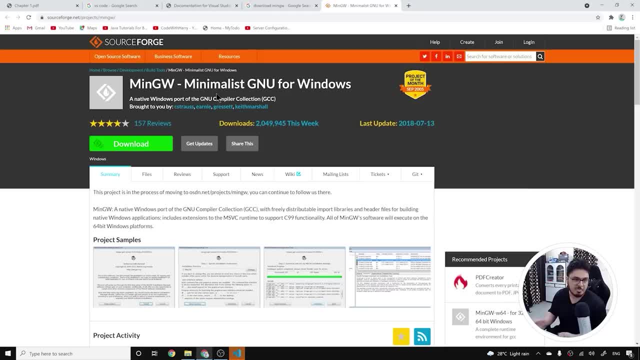 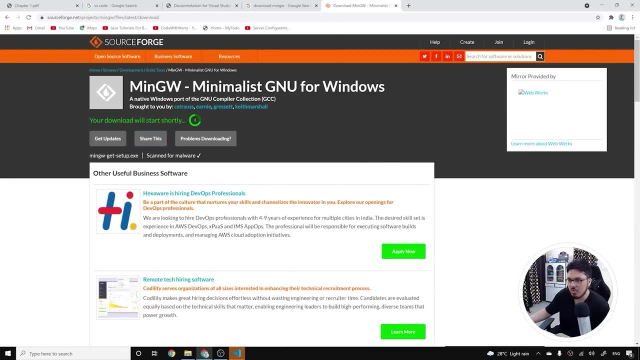 run our c programs. i'll tell you how and why later, but let's download it and let's set up min gw in our machine. so all you have to do is simply click on this download button and your download will start shortly. i'm waiting for it to download. this is simply gnu for windows. it's gcc. 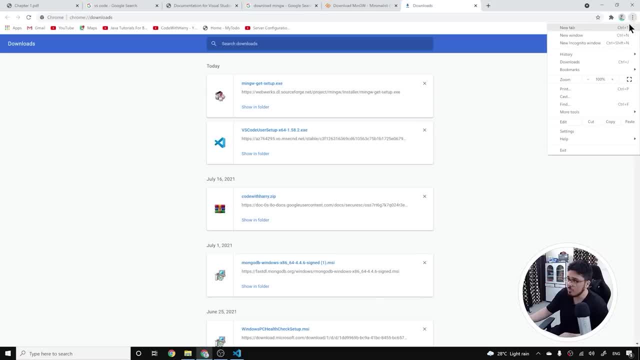 which is used to compile c programs. you can see your chrome downloads by clicking here and clicking on install, and after you do that, you will see that mean gw get setupexe. this has been downloaded, so i'll run it. i'll simply click on install. this is the directory where i want my min gw to get. 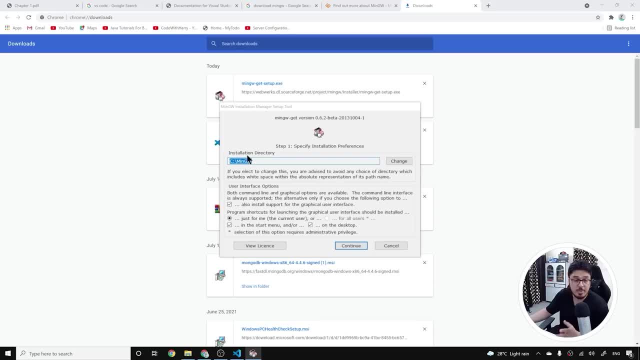 installed. if you don't want to get it installed here, you can install it in program files or something. but i'll not touch it, i'll simply go to continue. and this is downloading the installation manager. this takes some time. let me be very honest with you. i'm using quite fast. 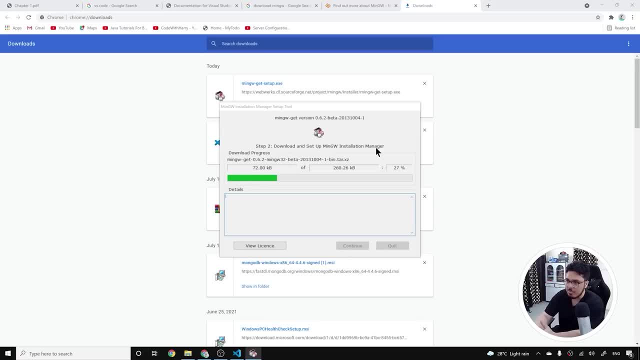 internet connection. still, it takes some time. so give it its time. can go grab a cup of coffee, or maybe you can go for lunch or dinner and come back and this will be downloaded. but yeah, it is downloading quite fast. it depends upon the source for servers to 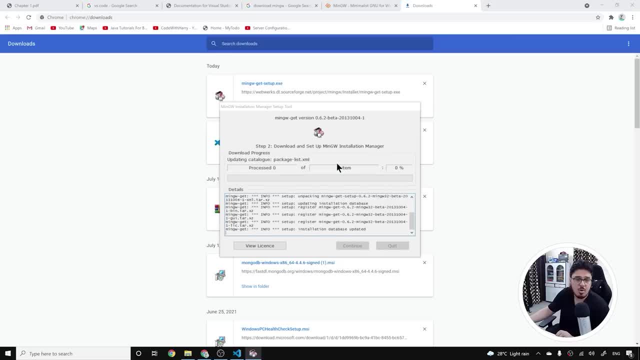 be very honest. sometimes it's fast, sometimes it's slow, but again, irrespective of whatever the case is, you can grab a cup of coffee. so i'll give it its time and in the meantime, i'll look into visual studio code. but i'll not launch visual studio code from here, and i'll tell you why. i'll simply. 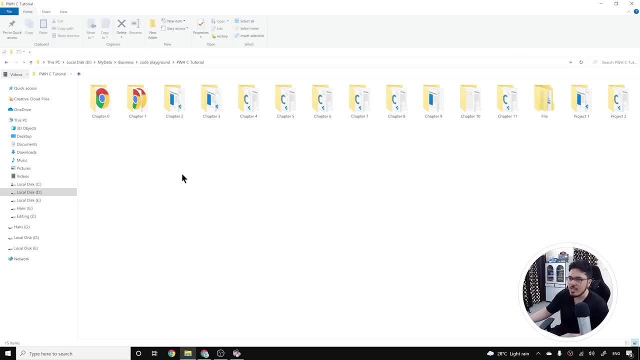 uncheck this check box and i'll click on finish and what i'll do is i'll come back to this folder where i've created all the nodes for you. i'll come back to this chapter one folder, and what i'll do is i'll right click and i'll see this option open with code in a very 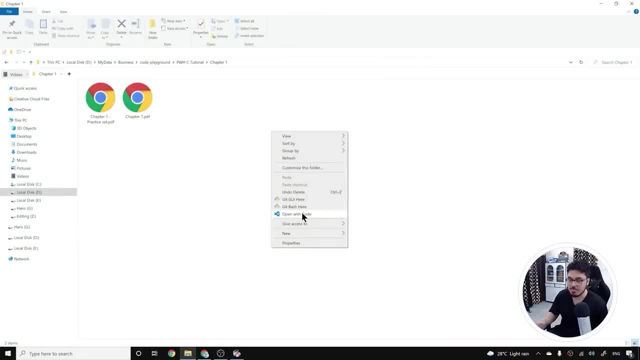 very rare case. if you do not see these options after following the steps that i mentioned, you can restart your computer, but in most of the cases you should, and you will definitely see this option open with code. simply click on open with code and once you do that, this folder. 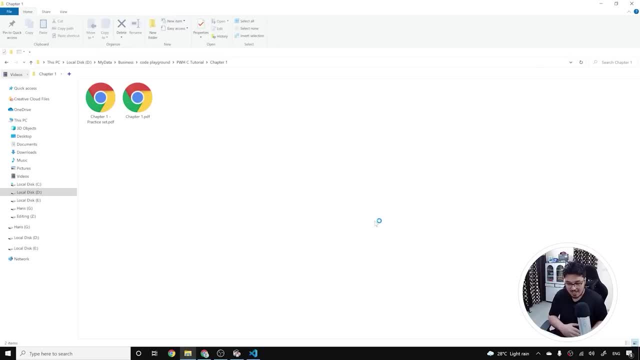 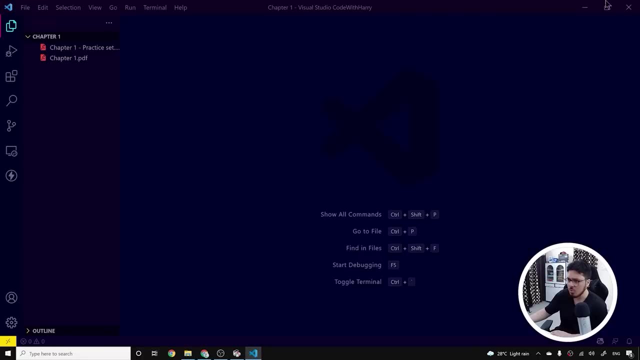 will be opened in visual studio code. now, what does this mean? when i say that this folder will be opened in visual studio code, this simply means that i have this visual studio code source code editor and all the files that i'll create here will reflect here and vice versa. so if i 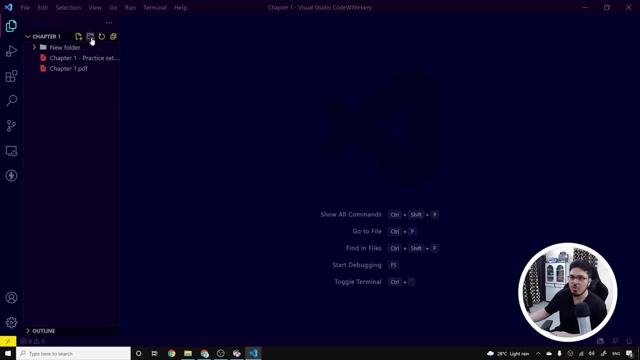 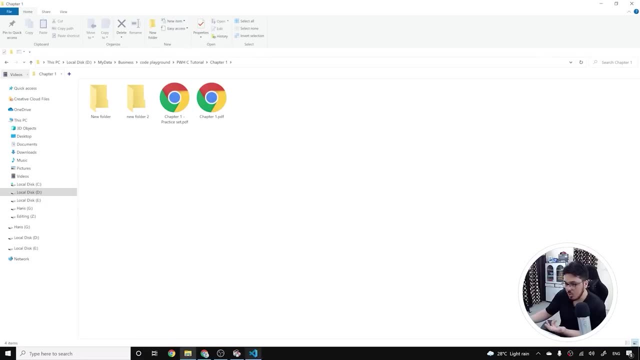 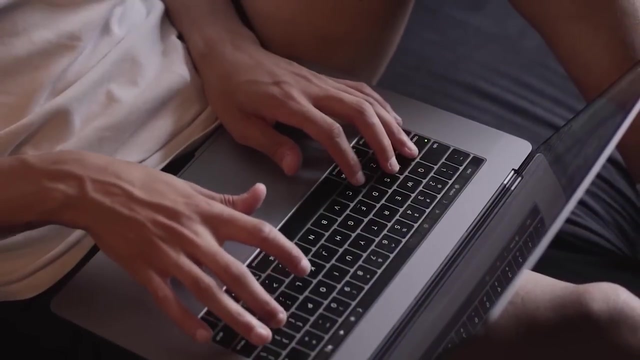 create a new folder here, i'll see it here. and if i create a new folder by clicking here, let me call it new folder 2, i'll see it here as well, so i can look into all the files, delete, read, write all the files from here itself. so this is one of the biggest advantages of visual studio. 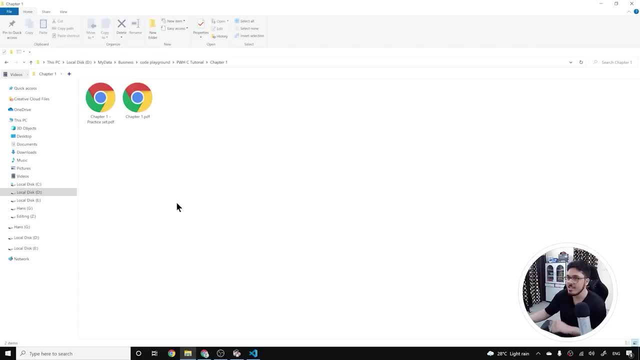 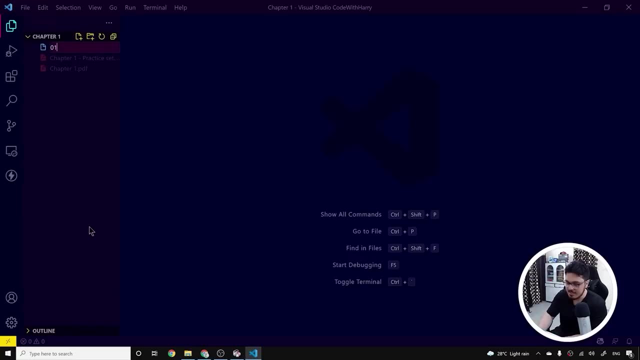 i simply selected it and pressed delete on my keyboard, and this actually deleted all those folders that i didn't need it. now what i'll do is i'll simply click on this plus icon and i'll say zero, one underscore, basic dot c, and this will actually create a file. now, what is this dot c? 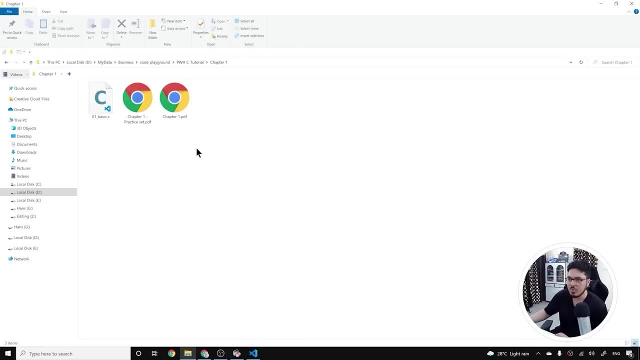 and what does this program name mean? and let me tell you so. when i say zero, one underscore basic dot c, it actually creates a c file, a dot c source code file. just like we save our pdfs with an extension of dot pdf, just like we save our text files with an extension of dot txt. just like we. 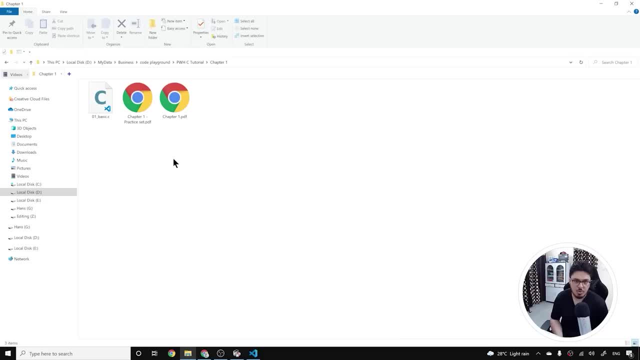 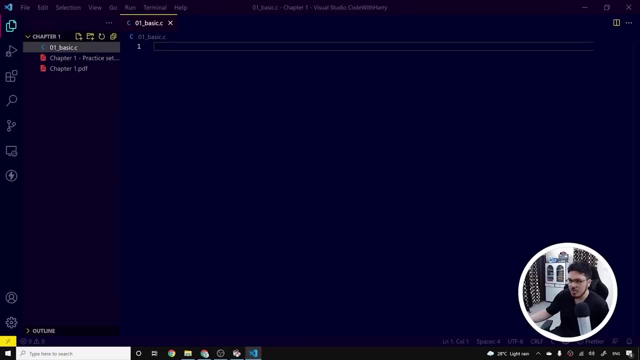 save our movie files with an extension of dot mp4. we save our c source code files using dot c. now what i'll do is i'll come back to visual studio code and this will look very, very haunting to you. if you are opening it for the first time, you might get confused what these buttons are about you. 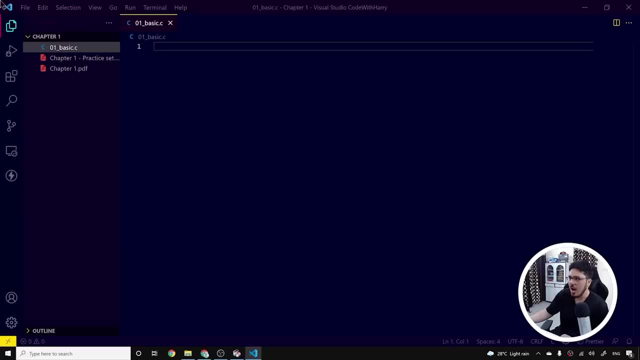 might get confused what the setting is about, and let me tell you how this visual studio code has been optimized for my case. now you will see some other color in your visual studio code and that might bother some of the students, so let me tell you that you can actually install a jellyfish. 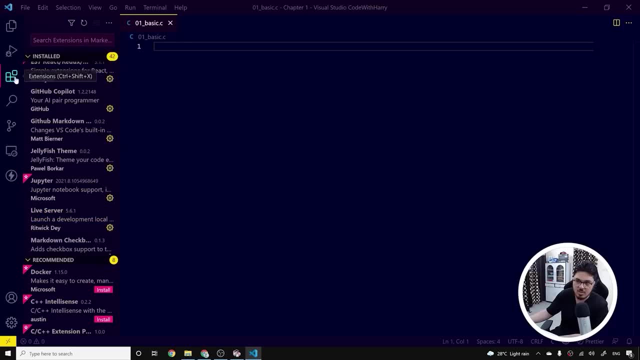 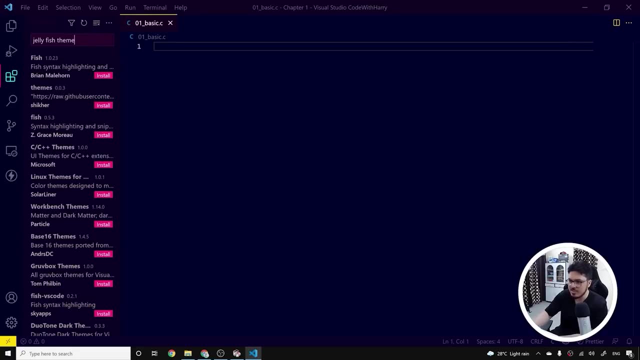 theme extension. simply type jellyfish themes after clicking on this extensions button. so i'll say jellyfish theme or other themes, if i'm not wrong, i think it's theme jellyfish theme and i already have jellyfish theme installed. uh, maybe i'm not spelling it correctly. let me find it out. 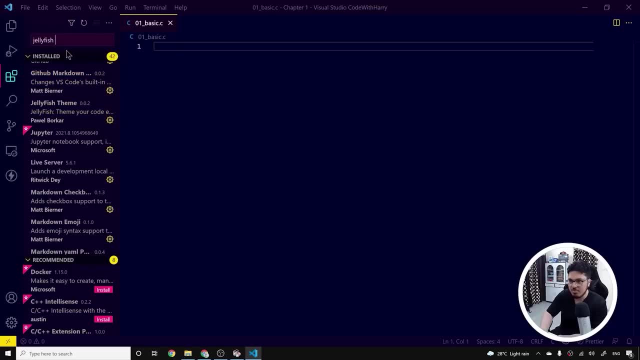 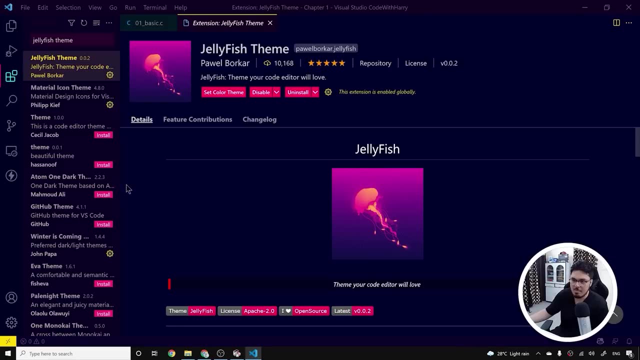 jellyfish- jellyfish theme. yeah, so it's jellyfish theme. it's here, so simply search for this jellyfish theme install and you should also see this color theme. another thing that i'm using is c, c plus, plus intellisense, so you can click on install. you will see this install button. for my case, it has already. 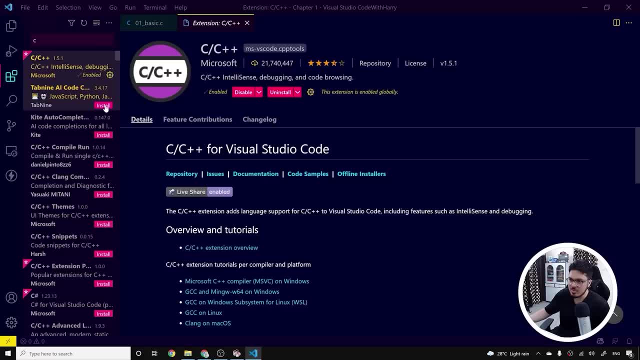 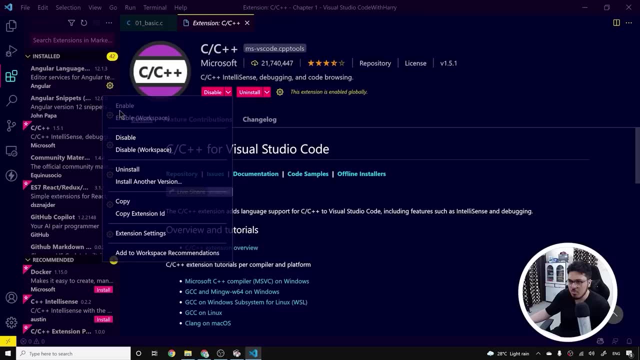 been installed, so i am not going to reinstall it. you can click on this install button and this will be installed. so for the time being, we'll use these two extensions. i have some other extensions too. i have uh enabled for other projects, but i'll disable them immediately, so let me disable all. 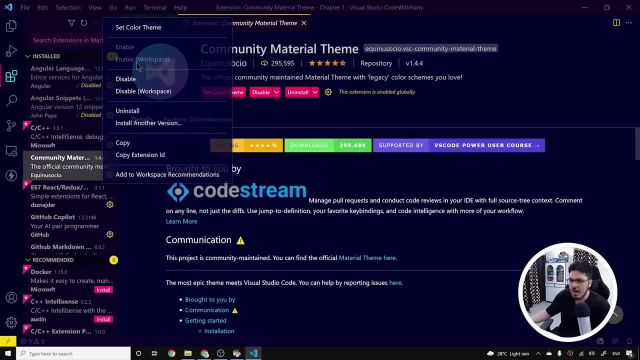 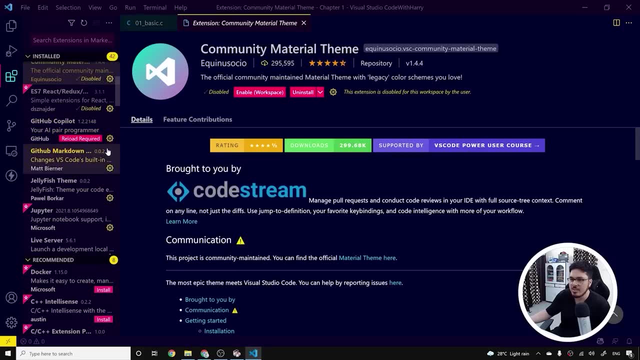 these, uh, community material themes. so i usually work with a lot of extensions, with a lot of other languages, so what i'll do is i'll simply disable all these extensions. so i have disabled github markdown, so let me disable all these things which we do not need here and which might confuse you. 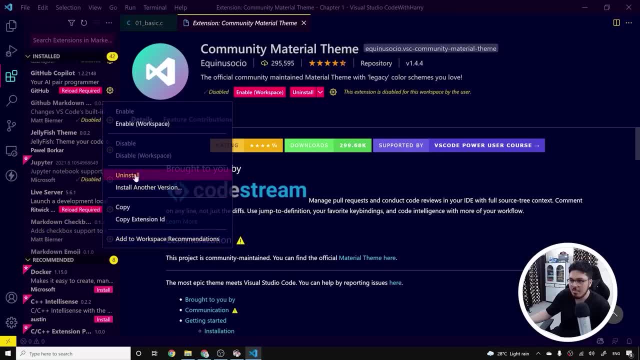 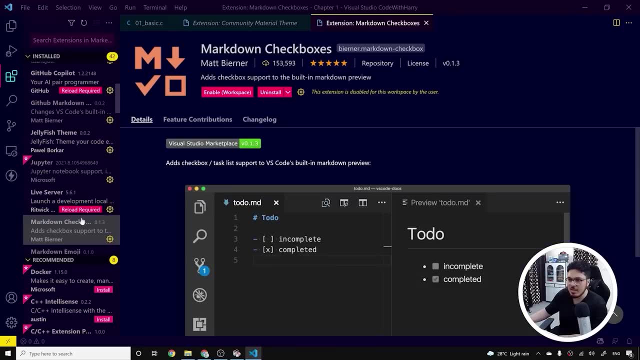 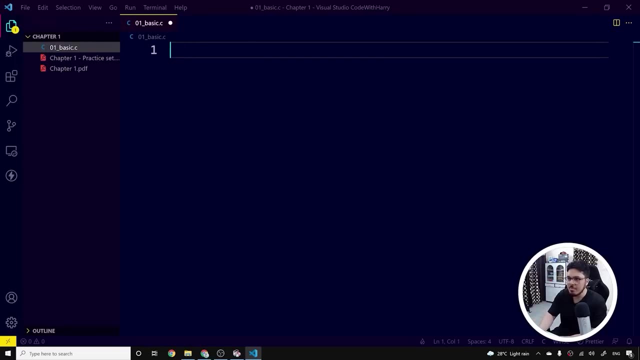 you don't have to install and disable all these extensions. let me tell you, i'm disabling it because i don't want them to disturb me while i'm coding in c with you. so let me reload my vs code. i'll simply click on reload and that should do. now what i'll do is i'll simply create a boilerplate c code. 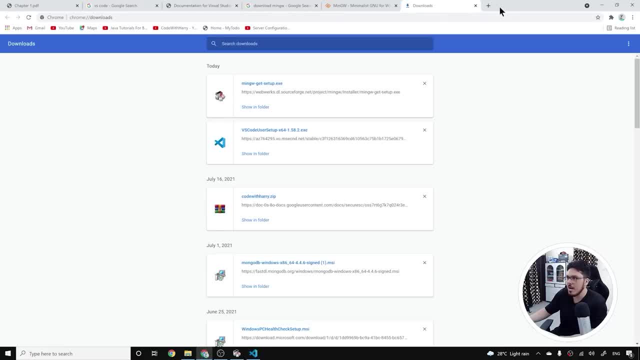 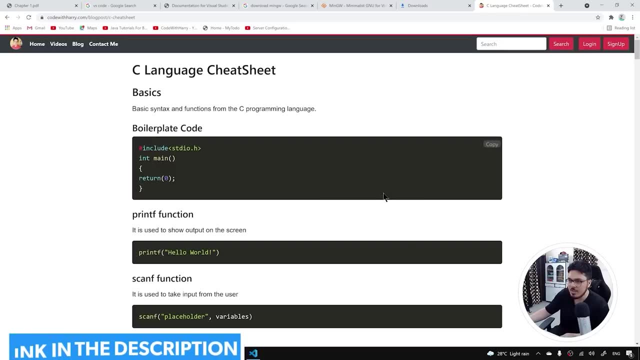 and for that, what i'll do is i'll open my c cheat sheet and i'll give you the link of my c cheat sheet from the description. so let me open the c language cheat sheet, i'll copy this code, i'll paste this code and save, and what i'll do is i'll just type in my c cheat sheet and i'll just type in. 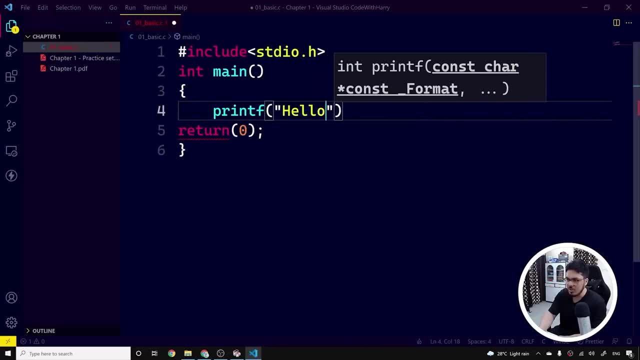 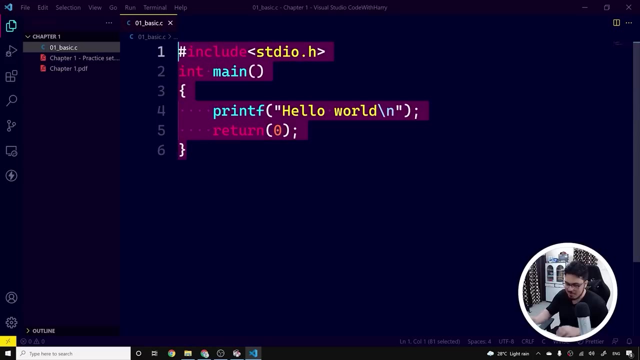 my c code and paste it in the description and i'll just say hello world and i'll say print f. i'll simply say print f and i'll say hello world. now you must be thinking: what have i written here? i haven't explained anything here and i have written all these things without even explaining. 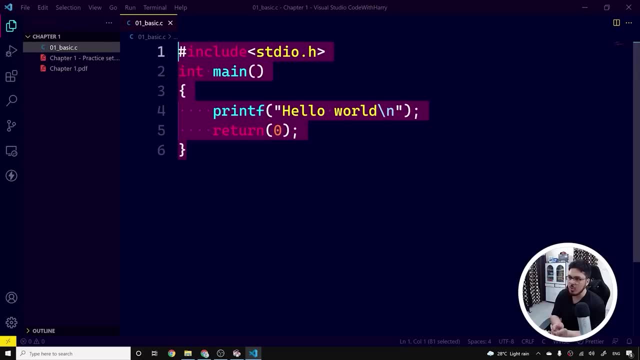 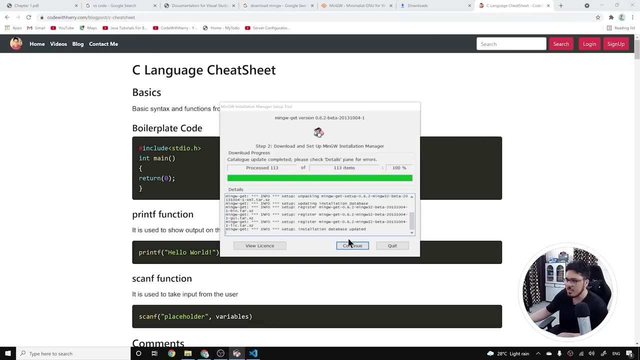 this is unfair, but again, you just have to type this without understanding- yes, without understanding- what it means, because we are going to look and dissect into all these things in the rest of this video. i'll give you the link of this cheat sheet as well, and also what i'll do is: i'll see if this 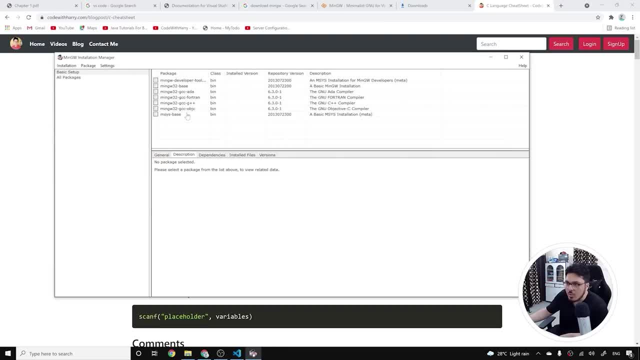 has been completed. so i'll click on continue and all you need to do is you need to click on this min gw32 gcc g plus plus and i'll mark this for installation. just click and click on mark for installation and this is a c plus plus compiler and c plus plus compiler, as well as a c compiler. 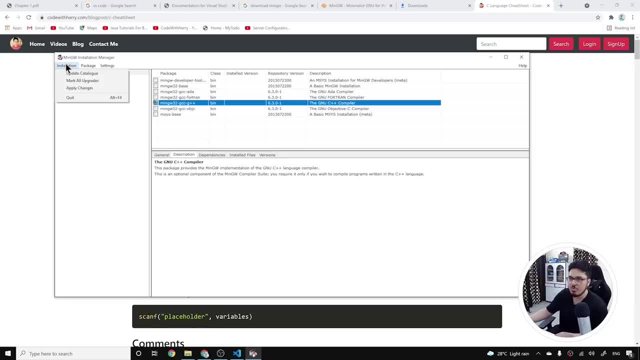 because we have gcc g plus, plus, so just install it. i'll go for installation and i'll say apply changes and i'll say apply and this will actually download this and install it. it sometimes gets very, very annoying when the server is slow and it takes a lot of time. so let me warn you beforehand. 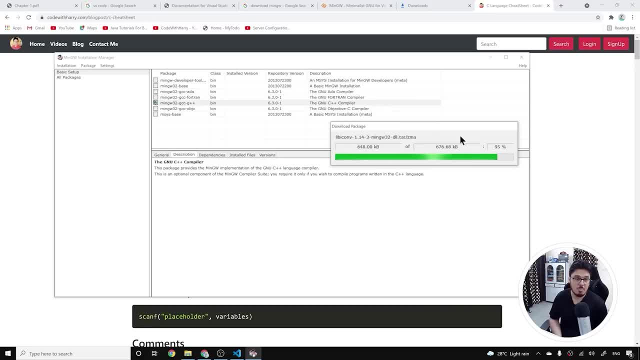 do not cancel it. it sometimes takes a very long amount of time and, yes, it is annoying, but again it's worth it. just go for a cup of coffee or go for lunch or dinner, and you'll definitely love it when you come back and see everything you know getting installed and set up for you. so i'll also 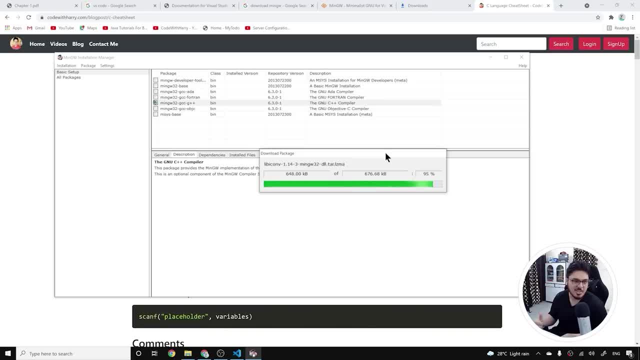 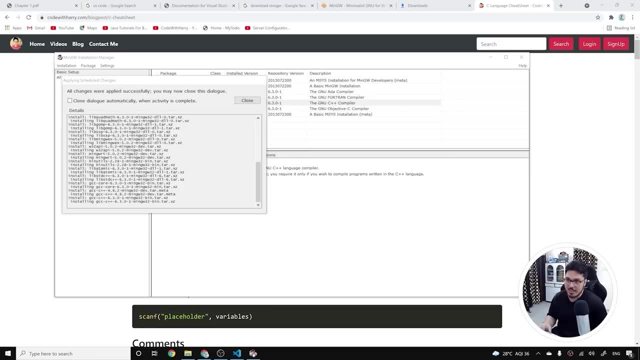 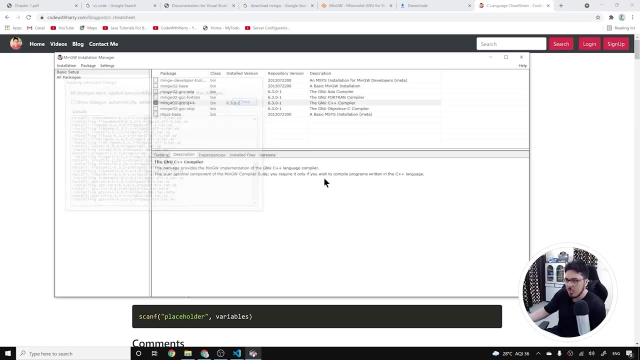 do the same. you go and grab a glass of water, and i'll come back after i have all this installed and set up on my machine. so, finally, this has been completed and let me tell you, guys, this took a lot of time, lot of time, and my computer is fast and internet is fast. so let me close this dialog box and we 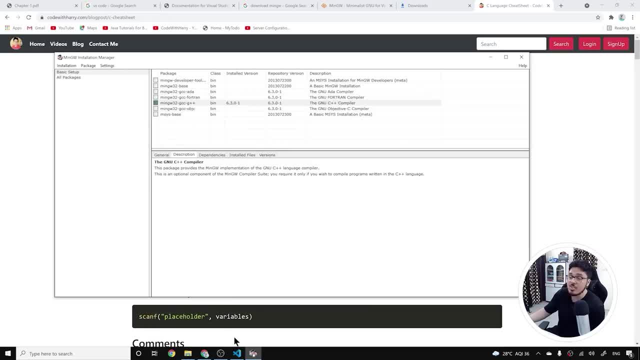 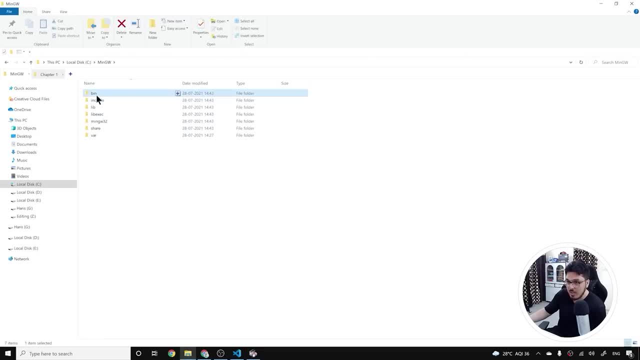 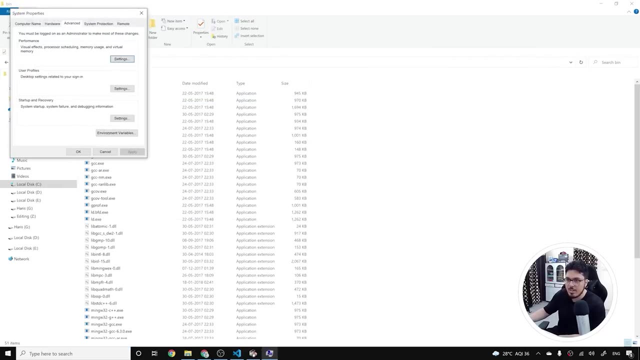 have installed min gw gcc g plus. let's now see how we can use it. so what i'll do is i'll go to my local disk c and i'll go to the folder where this min gw has been installed. i'll go to bin and i'll simply copy this path. now what i'll do is i'll type env and i'll be able to edit my system. 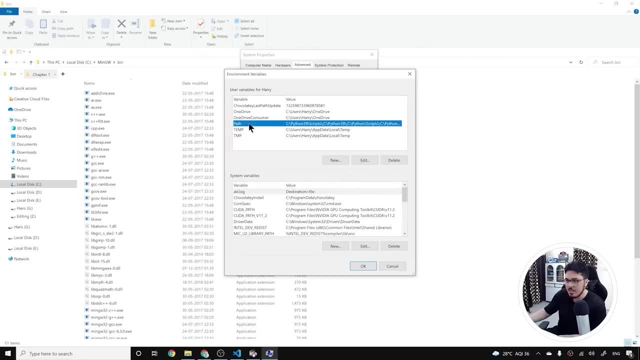 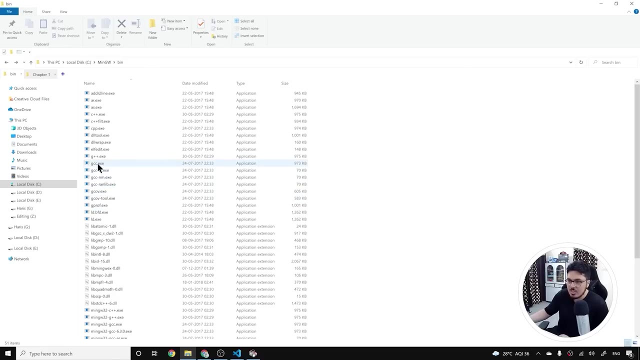 environment variables and i'll click on environment variables, then i'll click on path, then i'll edit the path, i'll add a new path, i'll paste this path and i'll click ok. and then i'll simply click ok once again and once again, and that will actually add gcc, gccexe, this thing, to path. so basically, 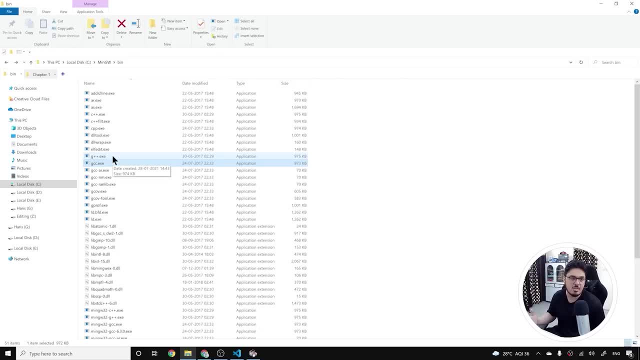 what i want to do is i want to use this gccexe to compile my c programs and, because of that, what i've done is i've added this folder, this particular folder, to path. what happens when you add a location to path? basically, you will be able to use all the exe executables without having to navigate to. 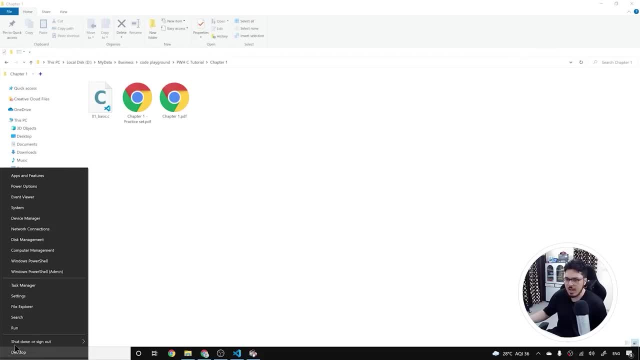 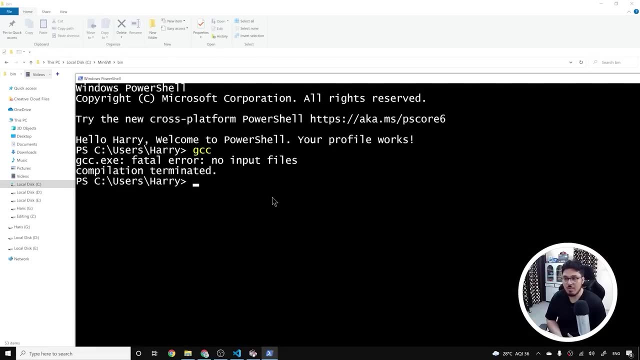 this path. so let me show you. i'll close this and what i'll do is i'll open my windows portion and i'll simply say gcc. now, the moment i enter, you can see that no input files message is going to be provided to me. it is basically telling me that you have not given me any source file to compile. 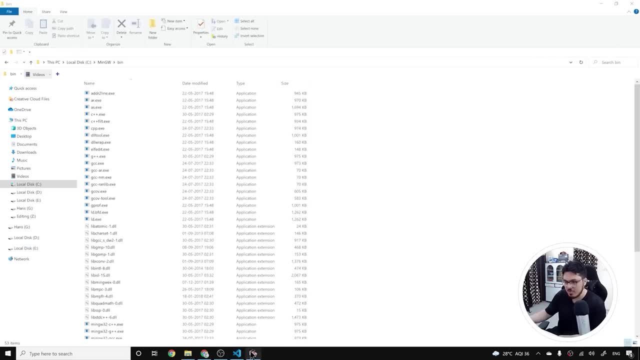 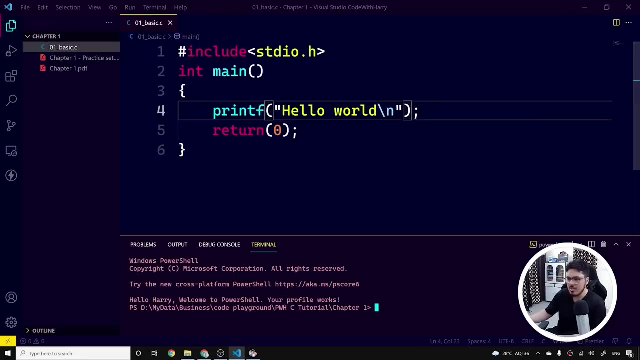 so let's come to visual studio code and see how we can compile our source files. so i'll close this terminal and you can open the terminal by clicking here: terminal- new terminal. this actually opens a new terminal and you can say gcc01 underscore basicc. so once you type this, you are basically. 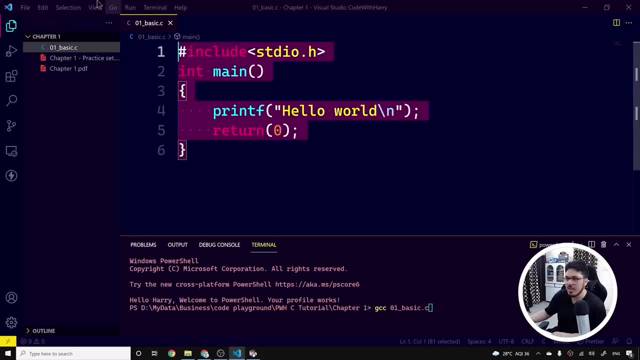 saying: compile this program which is written inside this source file, gcc01 underscore basicc. so you want to compile this file to a file which can be executed by this machine. this machine is a windows machine, so it will compile it to a exe file. let's see the moment. 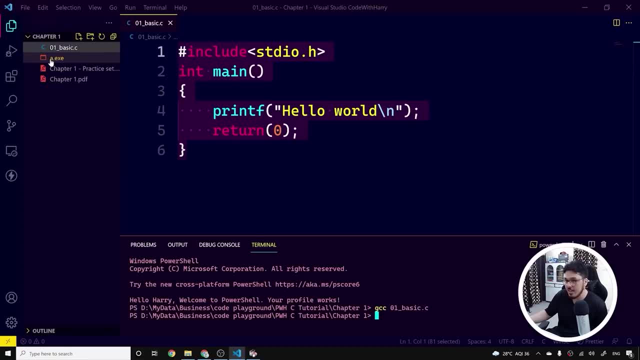 i press enter, you will see an aexe file created here. now i can run this aexe file. i'll simply say a and press tab. this actually auto completes the moment you say a. so anything that starts with a will get auto completed. so i'll simply say a and then i'll press tab, or i can even type this: 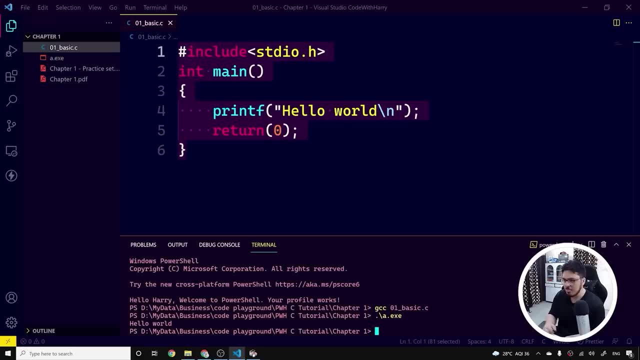 particular thing: dot backslash aexe. the moment i press enter, i'm seeing this hello word. so this program basically prints hello word. i can even say hello, harry, let me show you. and backslash, n is nothing but a new line character. so it actually prints a new line character, because of which we 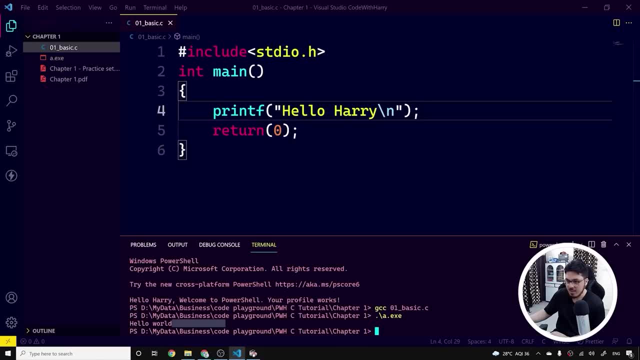 are seeing this psd, this thing here instead of here. so if i, if i skip this backslash n, what happened is, let me compile it once again, and then, once again, i'll say dot slash aexe. the moment i say hello, harry, this will actually not print a new line. so let me show you a practical example. 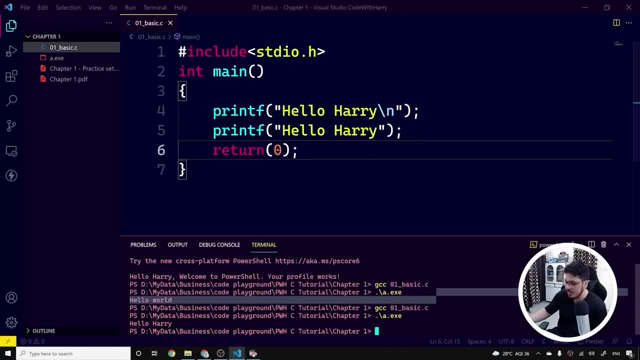 of what this backslash n is doing. so the moment i run this program once again, you'll see that hello harry, a new line, and then hello harry. but if i skip this backslash n and once again i'll compile this and i'll run this, you'll see that there is no new new line after. 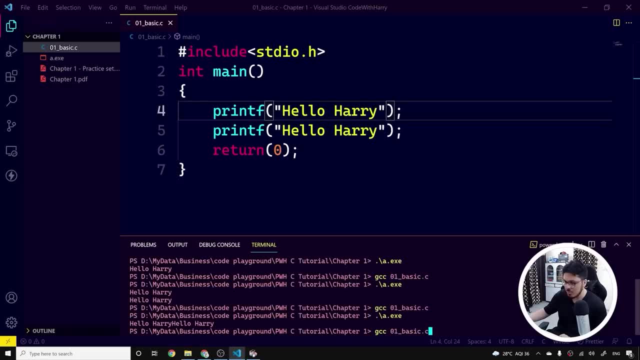 harry. so what i'm doing is i'm using my arrow keys to compile my program once again and execute my program once again, so you'll have to compile every time you make a change to your program. this is something that you need to remember. i hope that i'm clear. i hope that all these things are clear. 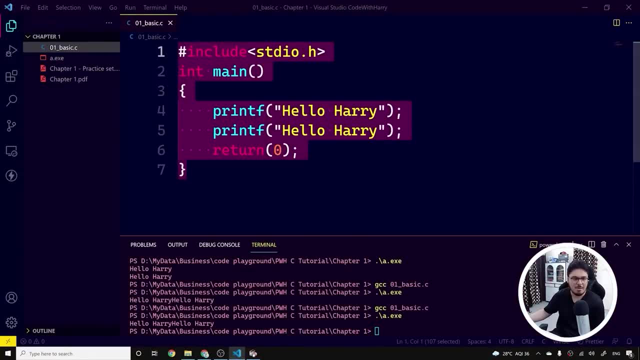 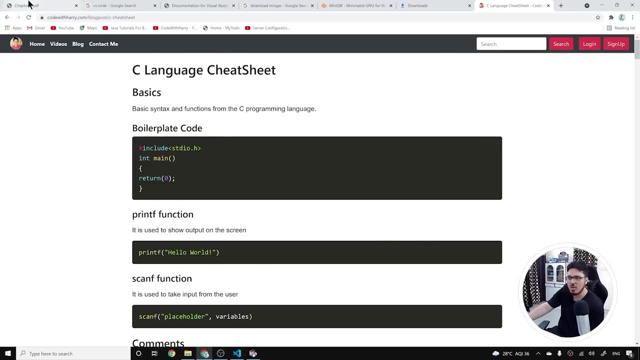 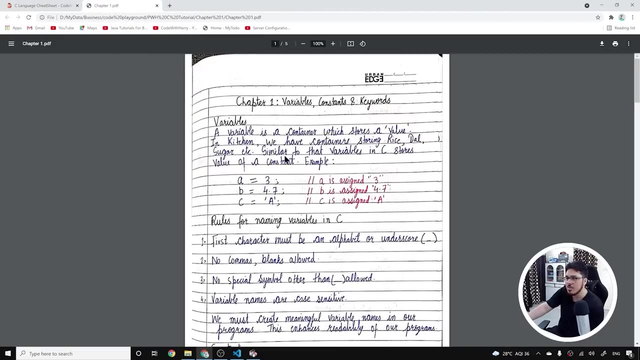 in fact, this is not clear so far, but i'll make it clear to you very, very, very soon. so let's come back to our pdf cheat sheet, or rather pdf notes, not cheat sheet. let me close, or i'll simply keep this cheat sheet open as well. i'll close other tabs and let's talk about variables constants. 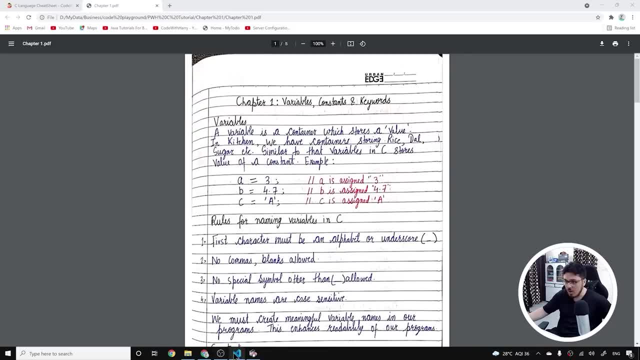 and keywords. so for now, just forget about how all this works and let's focus on the concept of variables, constants and keywords. what are these three things and why do we need these three things? so let's talk about a variable. it's a container which stores a value. so if you have a kitchen, 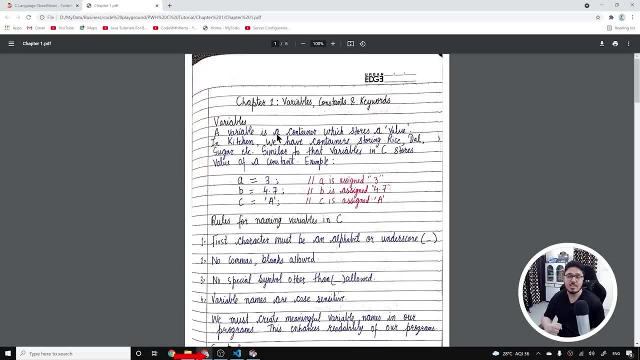 and you cook some food in your kitchen, there is a high chance that you'll have some containers which will contain some rice, maybe some dal, maybe some- what do you call it- some tea leaves. maybe you will have some vinegar in some container. you will have some water in some container. you will definitely have some. 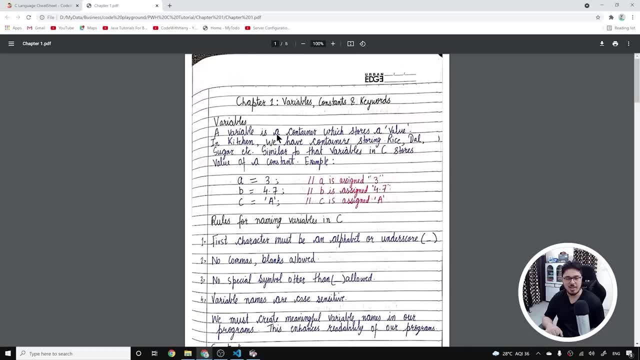 soya sauce or tomato sauce, all those things in a container. in a very similar way, just like a container is used to store a particular thing, we use small container for dal and for rice and we use a big container to store, say, flour. or we use bottles to store vinegar. and also we use 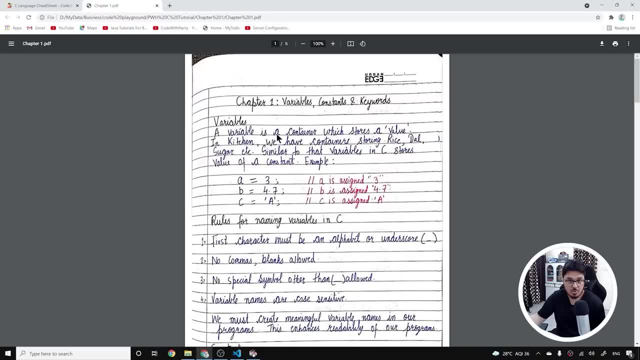 one or two liter bottles to store water. okay, so different containers for different things. in a very similar way, c programming language has a concept of container and container is nothing but a variable. it is called variable in c programming language. in fact, in any programming language it is called a variable and it simply stores a value. so in kitchen we have container. 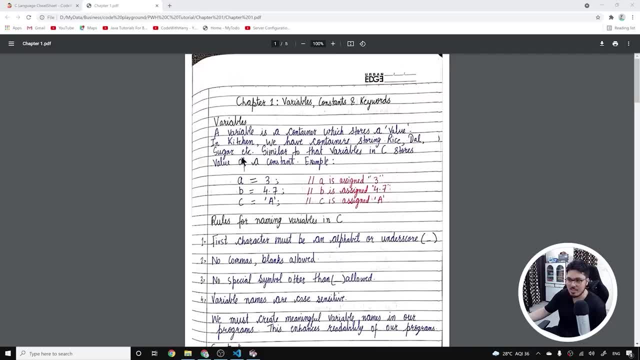 storing rice, dal, sugar, etc. similar to that. variables in c stores value of a constant. for example, a is equal to 3. now a contains a constant which is 3, b is equal to 4.7, b is assigned 4.7. c is equal to a. 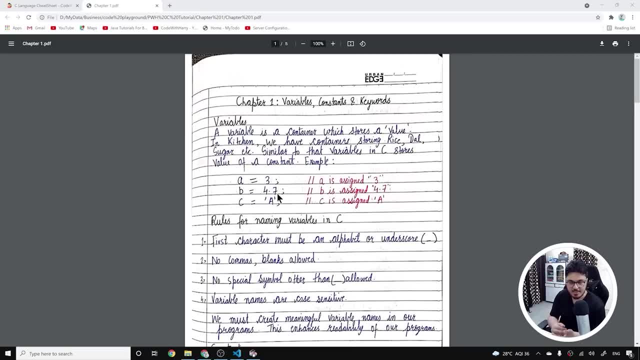 c is assigned a character, which is a. we'll talk about what characters are, what floating point numbers are and what integers are, but for now we need to get a hang of how these things are working. so let's talk about few rules for naming variables in c. can i name my variable as: 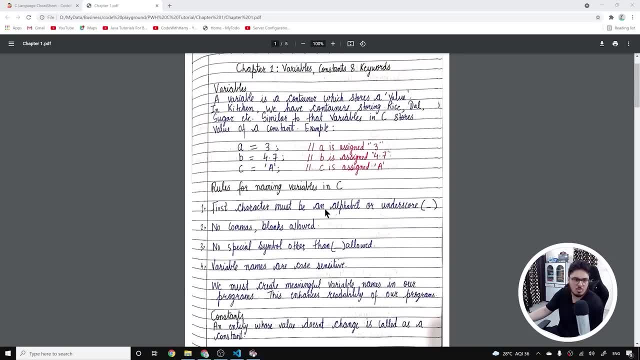 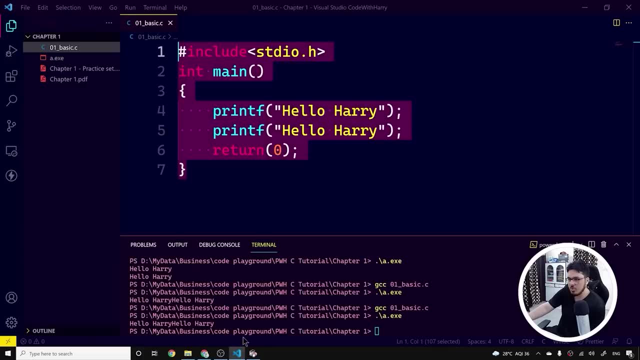 0, 0, 1, harry, double 2. no, i cannot do that and we'll see why we cannot do that. so first character must be an alphabet or an underscore, so you can use an alphabet or an underscore. so let's try. so i'll say int, underscore a and semicolon, and i'll say seven. now just forget about what this int is. 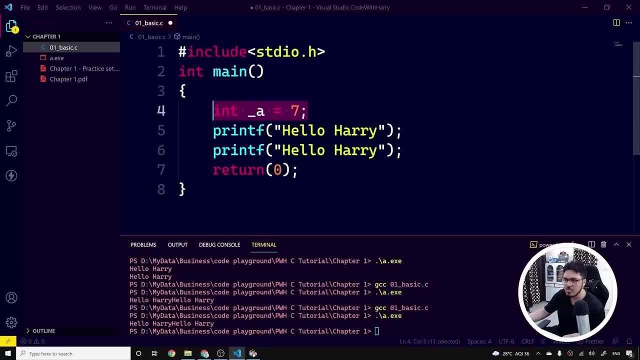 what this equal to is how these things are working. just focus on the concept of variable. see, i'm not getting any error. i'm not getting any error. i'm not getting any error. so let's try to do this. not seeing any error from my vs code when i type underscore a, but the moment i say zero underscore. 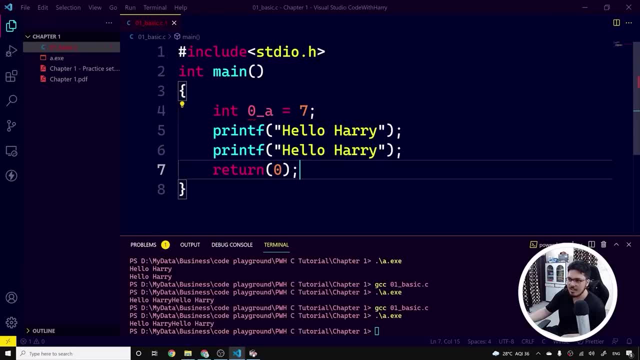 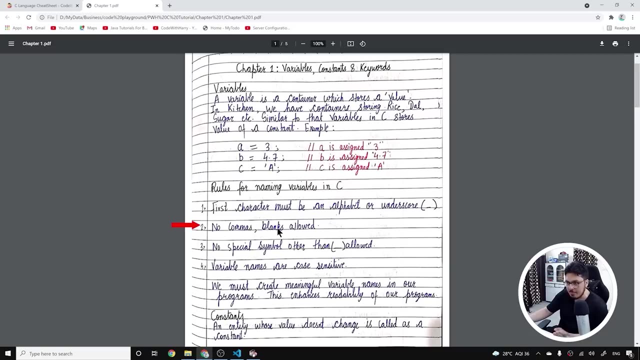 a and i save it, you'll see that a red line is actually beneath this zero, which is basically telling me that, hey, you cannot name this variable starting with zero. so i'm actually violating this particular rule, because of which i'm seeing that error now. commas and blanks are not allowed in. 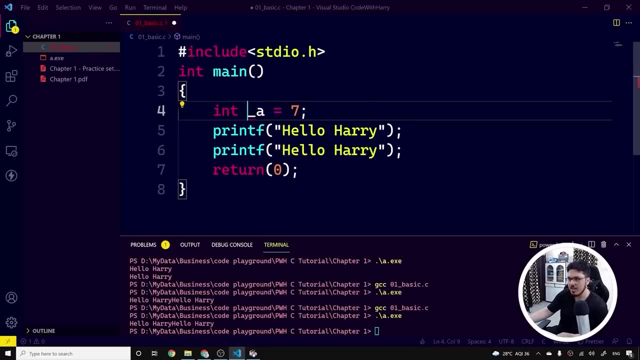 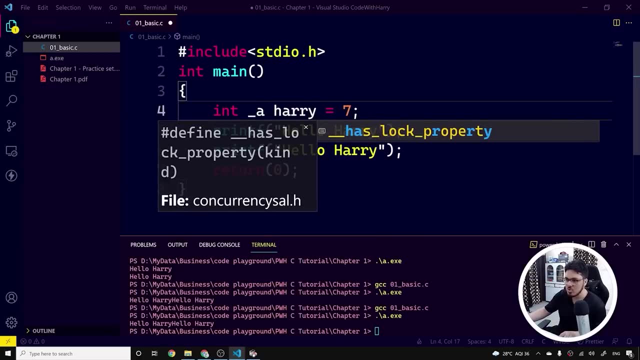 variable names. so even if i have it as underscore a and let me save it. so even if i have an underscore a and i give a space and say, harry, no, this is not allowed the moment i save it. this will give me an error. but if i join it with an underscore and save it, this is actually allowed, because spaces are not. 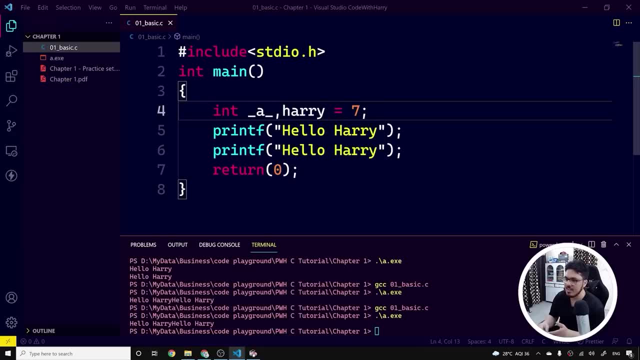 allowed. commas are also not allowed, so if i put a comma and save it, this is actually not allowed as well, and this will also create problems. a variable with this name will not be created. okay, so this is something that you need to know, and let's move. 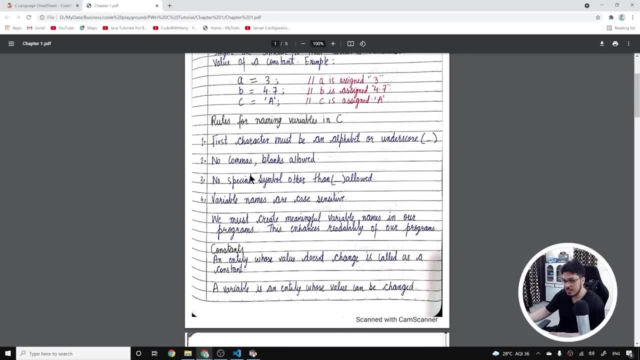 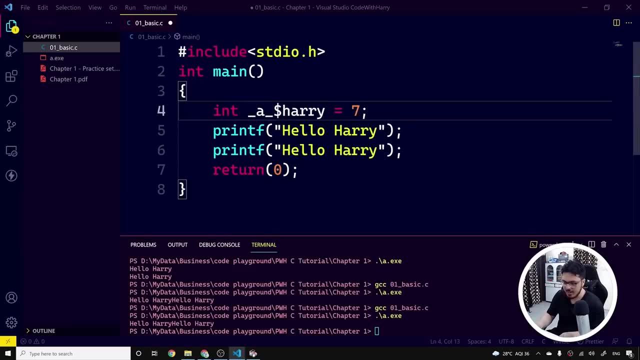 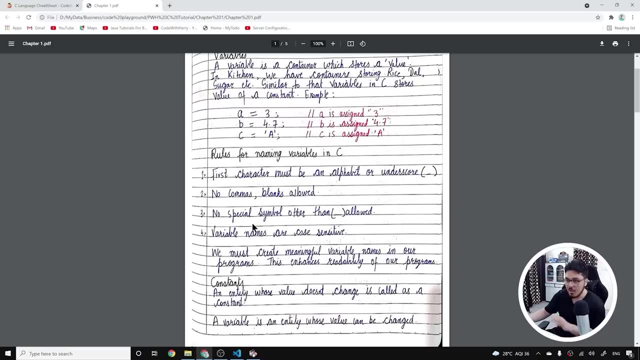 on to the next rule for naming variables. in c, no special symbol other than underscore is allowed. so let me show this to you. let me put a dollar here and save it. no, this is not allowed. the moment you try to compile this file, you'll not get the desired output. now, no special symbol other. 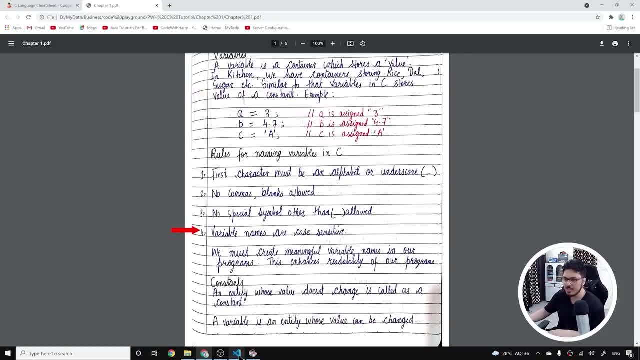 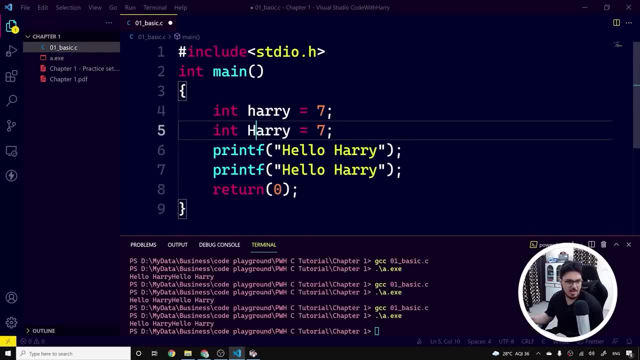 than an underscore is allowed. also, variable names are case sensitive, which means that if i have a variable called harry and i have another variable which is capital h, harry, these both are different variables and will store all these numbers differently in different separate containers. these are not exactly the same thing, so this is allowed. so you can say in small harry and 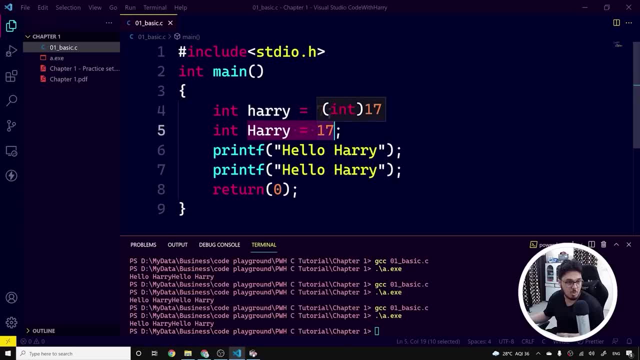 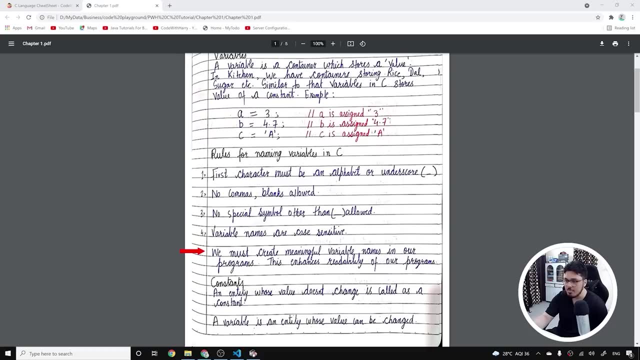 in capital harry and this will not create any problems in your program. now we must create meaningful variable names in our programs. this enhances readability of our programs and actually makes it easy for other programs to create meaningful variable names in our programs, to read our code. so this is something that you need to follow: always use meaningful variable names. 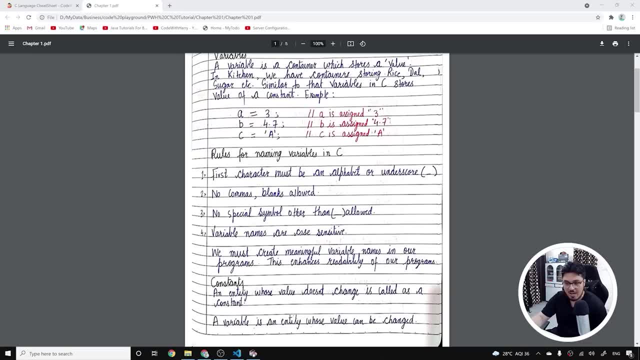 if you want to create a variable for storing, say, value of a url, simply call it url or value of url. do not call it abcd or something else or your neighbors or your crush's name. do not do that, just type the thing that it is. for example, if i want to create a variable for storing the amount, 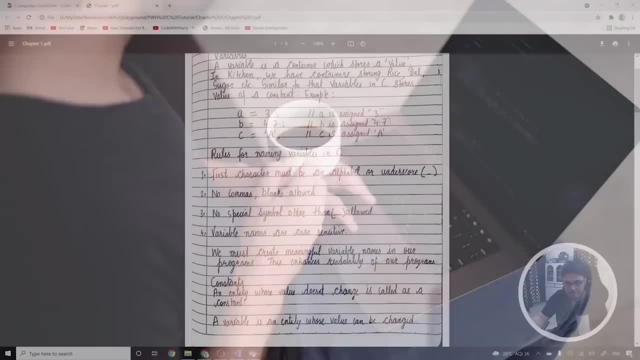 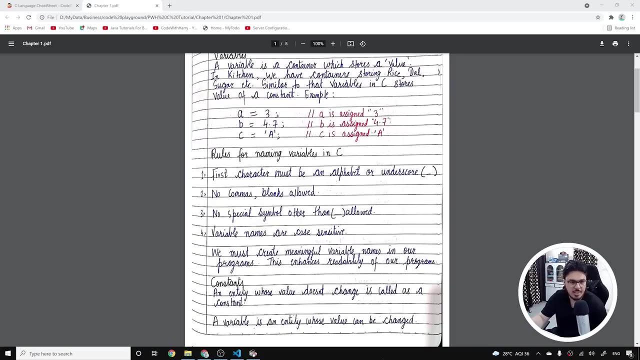 of coffee that i'm taking per day. i should type the value of the coffee that i'm taking per day. i should actually name it: amount of coffee, cups of coffee or something like that. i should not call it puja, reena, tina or monica, for that matter. so let's talk about constants for now. an entity whose 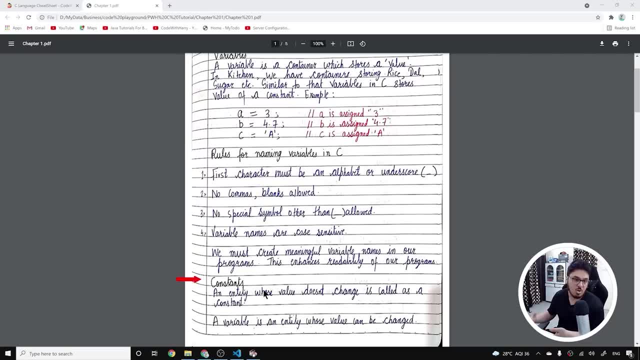 value doesn't change is called as a constant. what is a constant? it doesn't change. three, it doesn't change. four is four. it will never change. four will never ever become five, or ten for that matter. so four is a constant, three is a constant. something which is not going to change is a constant. but if 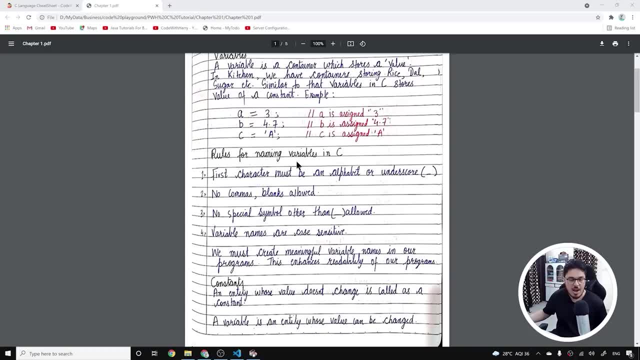 a is equal to three, i can always say a is equal to four and i can actually put four inside that container which was previously holding three. so i can change this container to hold four now. so this is a variable, we can change its value. its value is three at this point, but later it can become four. 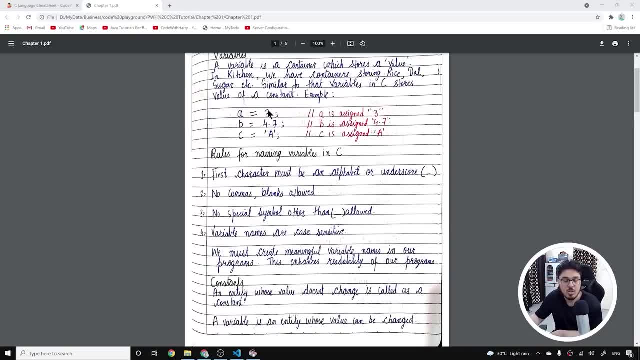 also, it can become 40 in some time in the future. so you never know. but a constant is not going to change. four is not going to change. four is going to be four in the future, so i can change this lifetime and even when we have kids of our kids, they will also call it four and it's going to 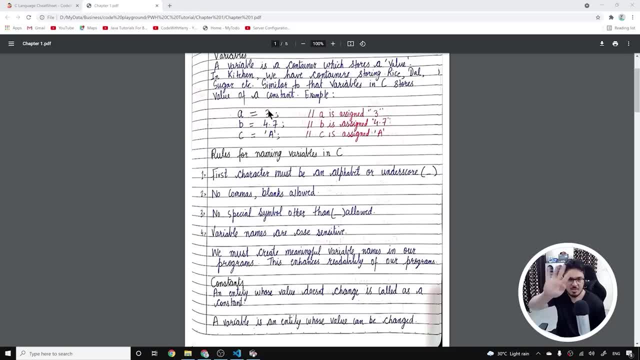 carry the same value, which is four. so four fingers are going to be this now, 40 years ago, and even 2000 years later it is going to be four, so it's not going to change ever so. this entity is called constant variable is an entity whose value can be changed now it doesn't mean that it will always. 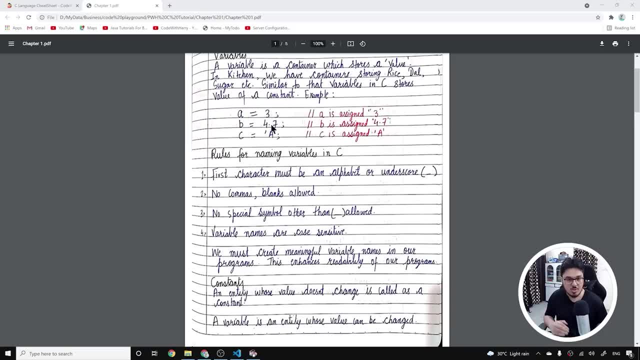 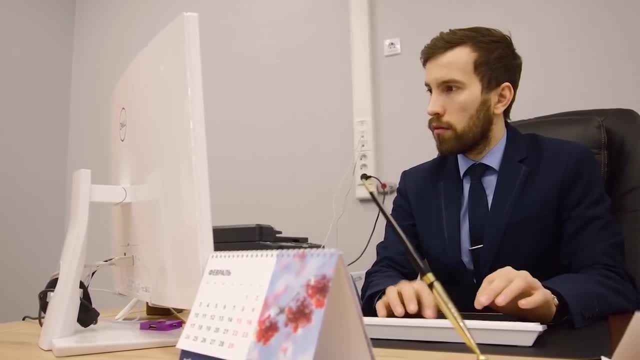 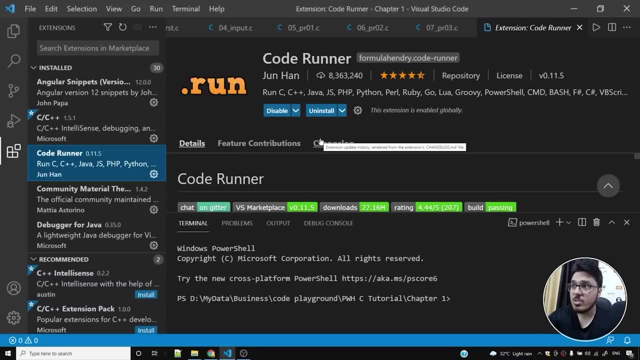 change, but it can be changed. so a is equal to 3 can be changed, b is equal to 4.7 can always hold 8 in the future, so it can change. this is something that we need to hold in our mind before we start with this chapter, before we start writing programs and see, i want you to ensure that you have this. 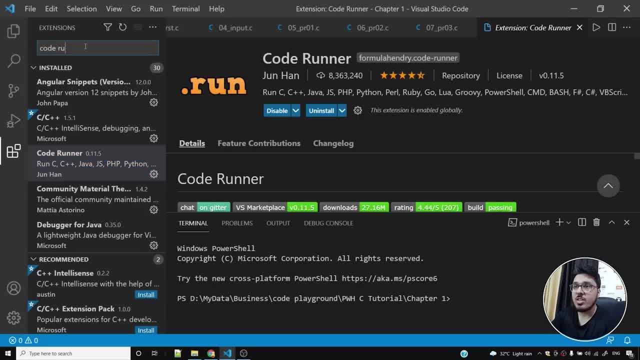 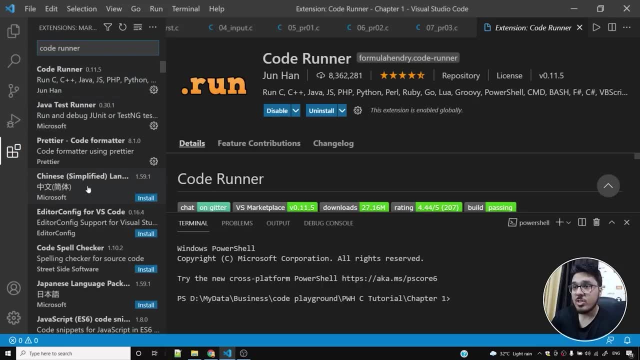 code runner extension. if you don't have this extension, simply type code runner and simply install it. you will see an install button here, just like i'm seeing for chinese and for editor config. you simply have to click on that install button and your code runner will be installed. 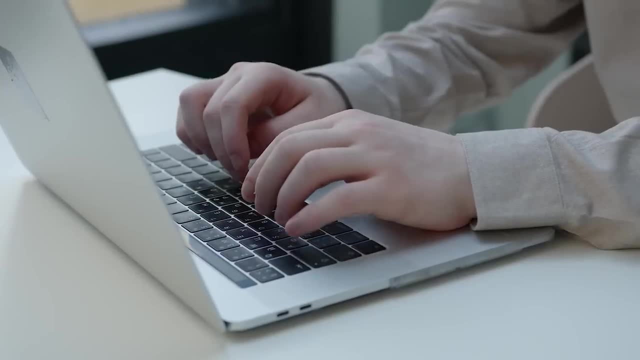 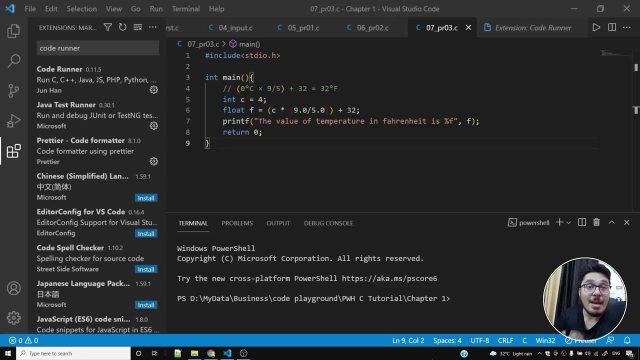 and this will give you this run button here. so whenever you are in a c program, you will see this run button. so make sure that you get this run button as soon as possible. it will help you execute and run your c programs comfortably. now we'll move ahead and talk about the types of 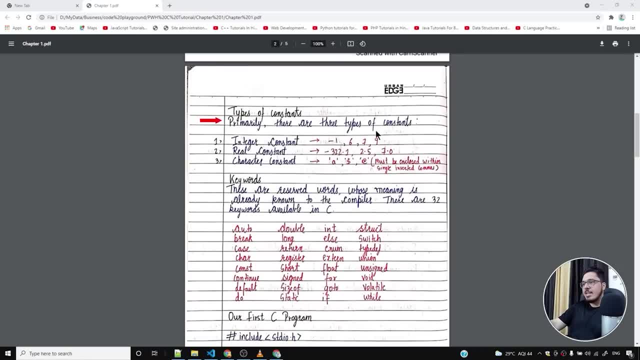 constants. we have various types of constants. primarily, there are three types of constants. we have an integer constant. we have a real constant. also, we have a character constant. so we are going to see how we can write these three types of constants in our program. so let's start. 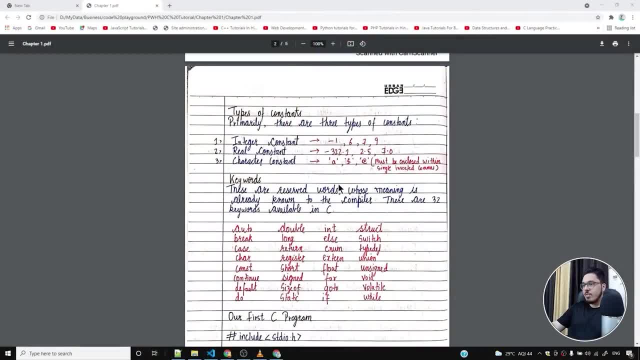 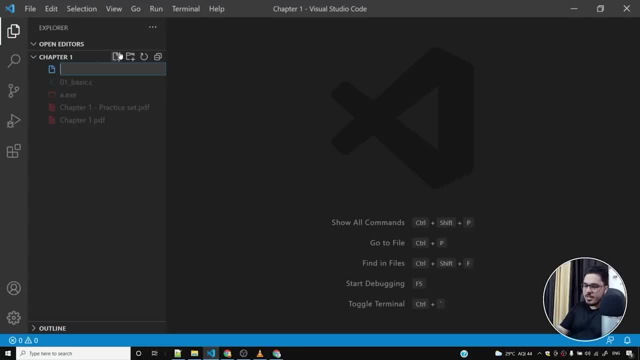 in c. also, we are going to see few examples of us assigning these constants to a variable. so what i'll do is i'll open vs code. you can see that i already have this program written. i'll do one simple thing. i'll say 0, 2 underscore. i'll simply say constants, dot, c, and the moment i say constant. 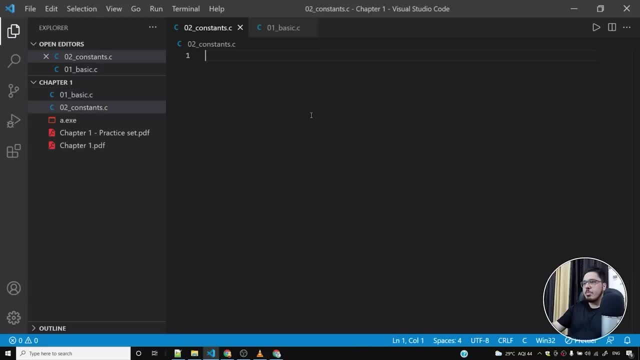 dot c, and let me also copy the boilerplate code. i'll simply save this. what i can do is i can say: harry 2 is equal to c. notice that i am using single quotes for a character. you have to make sure that whenever you are assigning some variable to a character, you need to use single quotes. now. 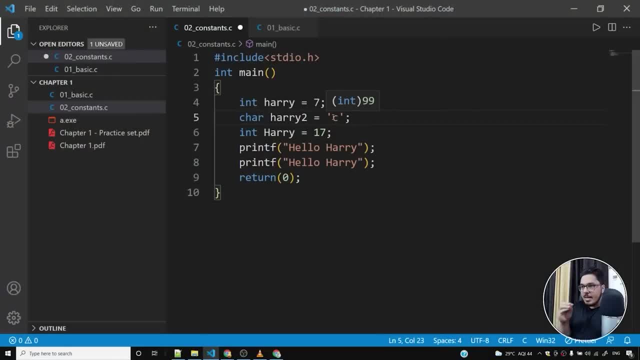 this might sound very, very confusing to some beginners, but let me tell you something as we move ahead in this course, you are going to find all these things very simple and easy, so please bear with me for some time and definitely you are going to grasp all these things and you are going to 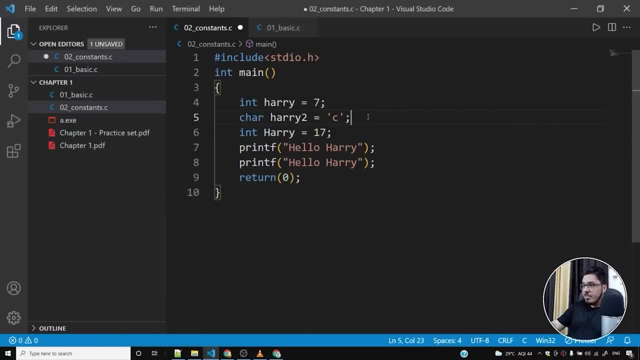 these concepts very, very easily. similarly, we use a float keyword. now, these keywords might sound very, very strange to you if you are a programming beginner, or c beginner for that matter, but let me simply show you how we can assign some values, different types of constants, to a variable. so 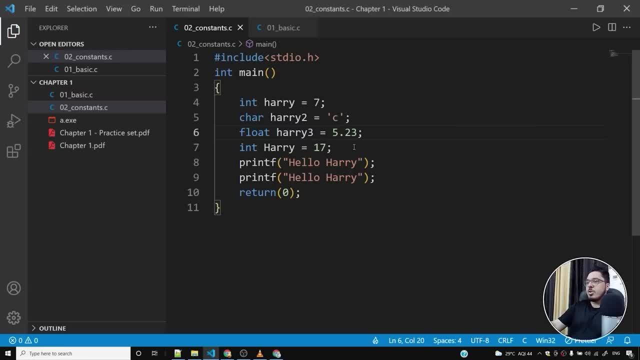 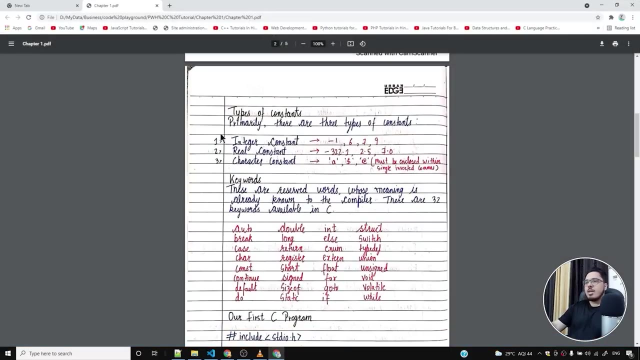 i wrote 5.23. i could have written 5.23, i just removed minus sign. and similarly, i can use minus 7 when i'm assigning an integer to this harry variable. now let's come back to the notes and let's build some understanding around this, and then what we'll do is we'll come back to vs code. 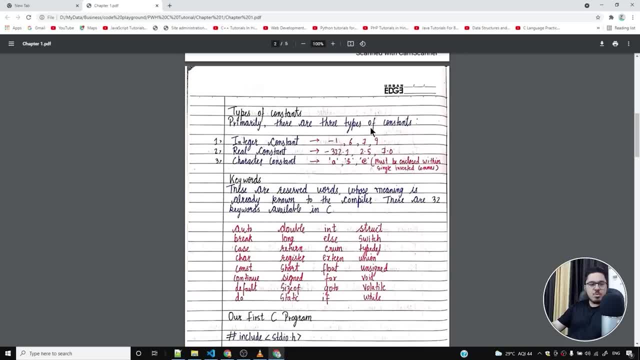 and write some sensible programs. so, primarily, there are three types of constants. we already saw that: integer constant, real constant and character constant. so this is very, very important. these three types of constants are something that you really need to remember. and let's now talk about keywords: what? 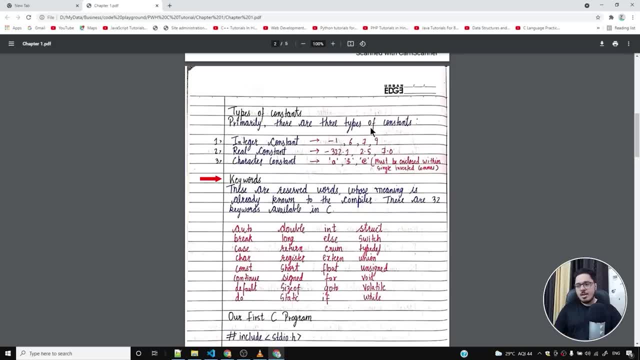 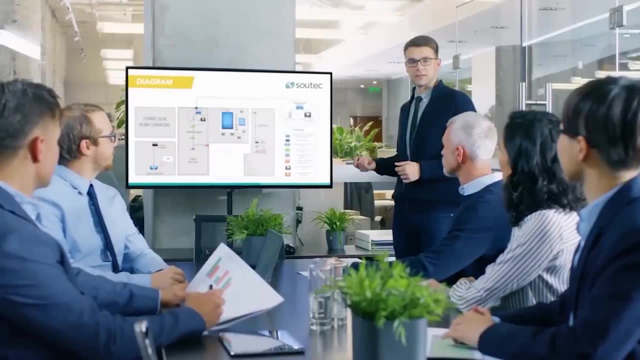 are keywords. so whenever we are writing a program, there is some part of the program that we have written it's coming from our mind, it's coming from our head, and there is some part of the program which is not coming from our head. it is something that has already been reserved by the c programming. 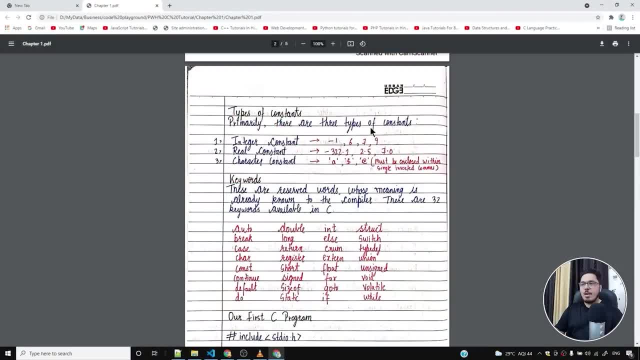 language community. somebody who built this programming language reserved these keywords, or rather declared these keywords as reserved. so these are reserved words whose meaning is already known to the compiler. so meaning of all these keywords is already known to the compiler. now there are 32 keywords available in c. let's see what those 32 keywords are. but before we see these, 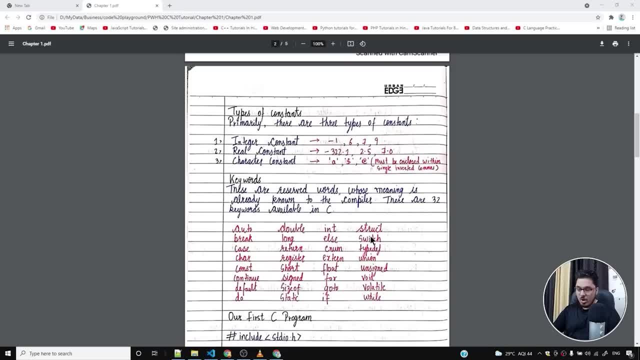 32 keywords. let me tell you, you don't have to remember these keywords. a lot of people try to remember these keywords, and that doesn't sound good. you don't have to do this. please do not try to remember these keywords. this is something that we should avoid. you will eventually start. 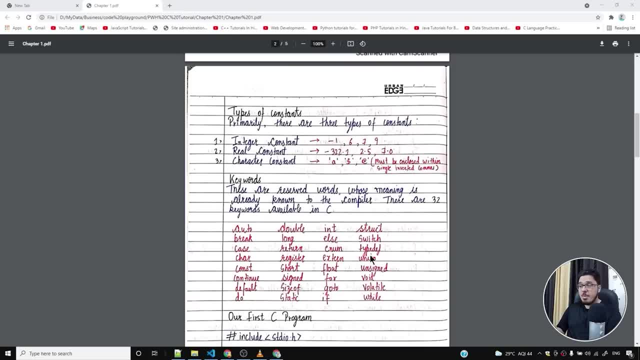 remembering all these keywords, when, once you start remembering all these keywords, you'll be able to start writing some meaningful programs, and once you start building few projects in c language, these keywords, or rather some of these keywords, will definitely sit in your head. now, auto double instruct: break long else. i have jotted all these keywords down just for your understanding, because 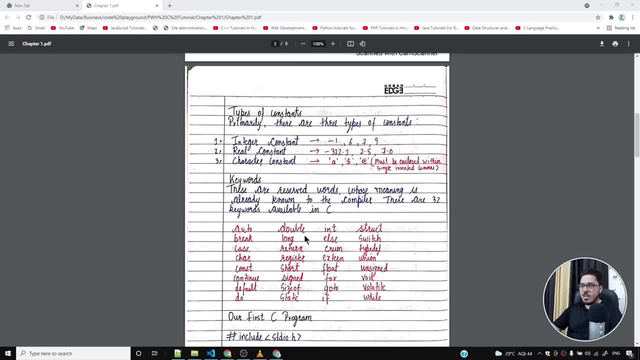 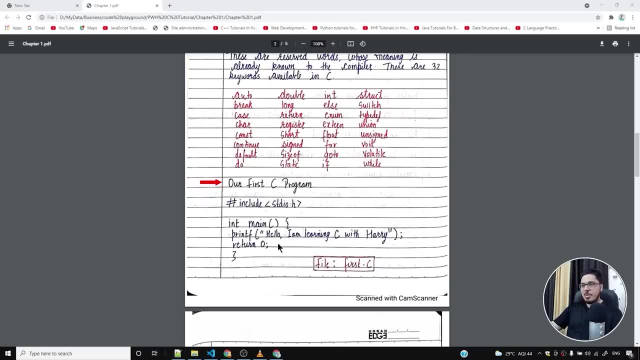 i wanted you guys to have a comprehensive list of all these keywords at your disposal. so let's write a first c program. we have already written a first c program, but i want you to write this program as your first c program. type each and everything. do not use any shortcuts or copy paste. 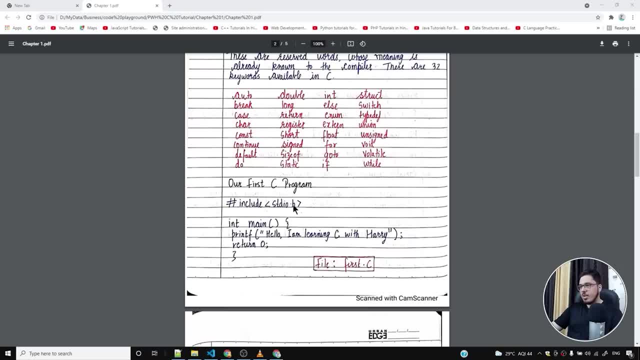 simply type this out. simply type this hash include stdioh now. simply say int main and simply type it out. do not think about what hash include is what stdioh is, do not think about what int main is, what printf is, what return zero is, just type it out. 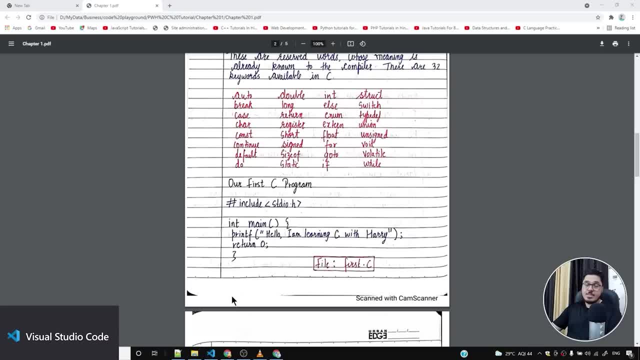 you and execute it in your vs code, or if you're using some other ide or source code editor, which i do not recommend. if you are a beginner, please follow along. if you are a beginner, but if you are an advanced user just trying to hone your c skills, you can simply come to this. 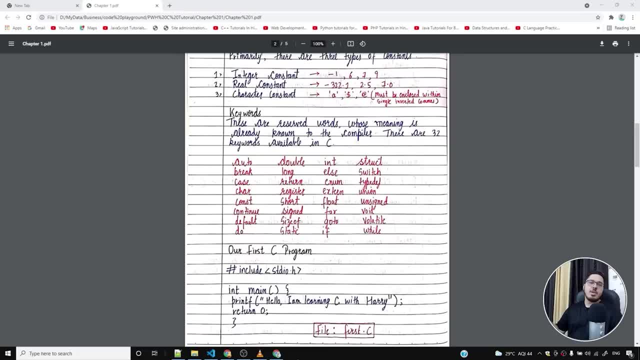 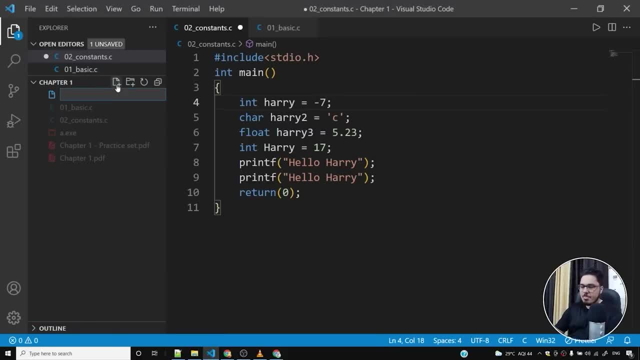 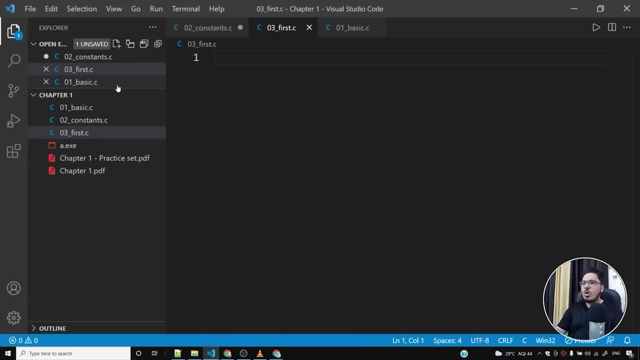 tutorial and use the ide or source code editor of your choice. so once you start typing this program out, let me write the first program as well. so i'll say zero, three underscore, first dot c. so i've typed this program out and also what i'll do is i'll simply copy this. 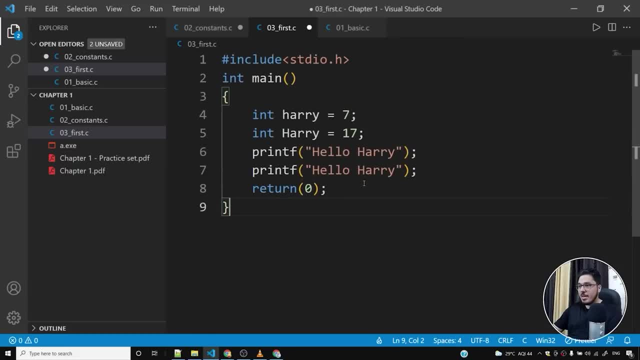 uh, i, i told you that you have to type, but i'm copying. i'm copying because i don't want to waste your time, to be honest, but i want you guys to type it out, because when you type it out, when you type something out, you actually remember things. but if you copy paste and you know start. 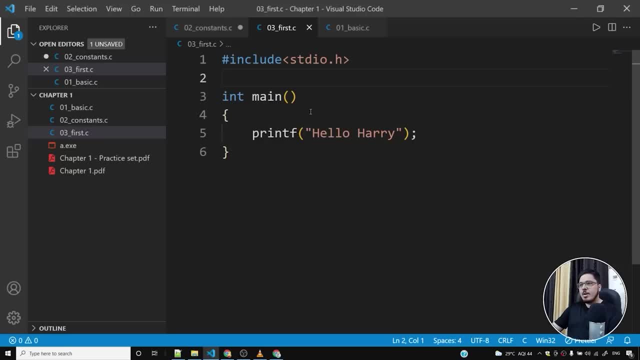 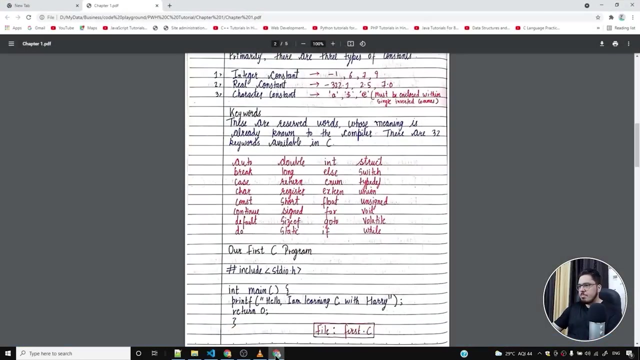 running or simply read from the notes. you might not remember it that well, so let me see if i can see if it is the exact same program which i've written. uh, hello, i am learning c with harry. let me write it down. hello, i am learning c with harry and backslash n is something that you might want. 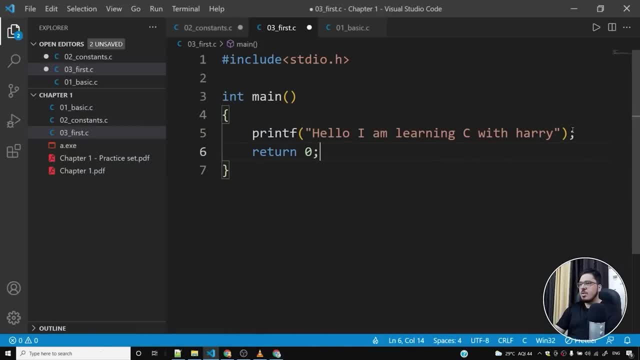 to write, but let's write return zero and let's run this program also. i'll save this program. so what i'll do is simply run this program and once i run this program, you can see: hello, i am learning c with harry has been printed on the screen. 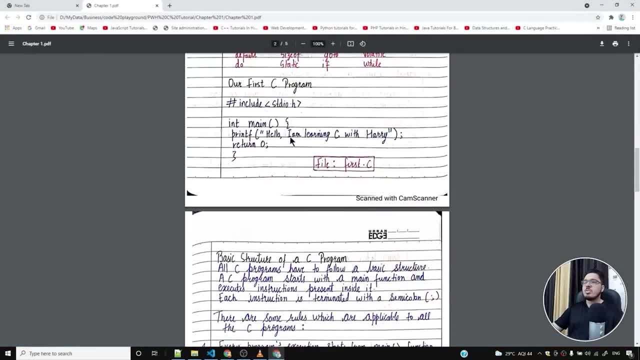 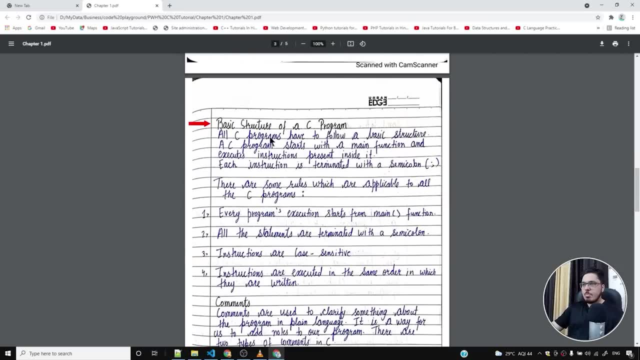 now let's talk about what this structure means. what is this basic structure of a c program, how all this works together. this is really very important, so let's talk about this. let's talk about the basic structure of a c program. so all c programs have to follow a basic structure. 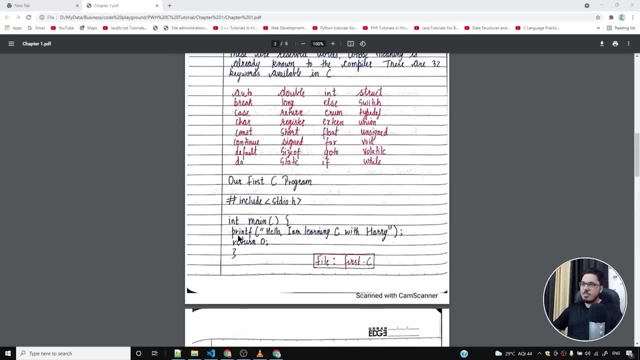 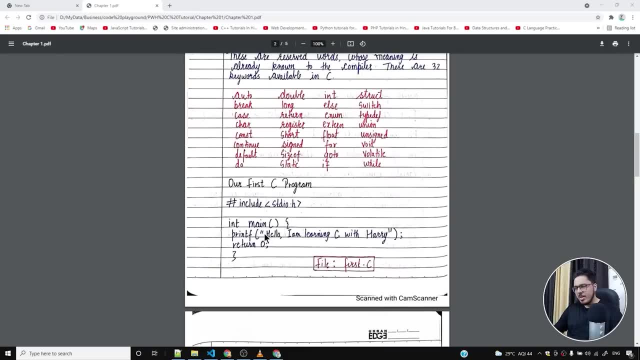 a c program starts with a main function. you can see that we have a main function and executes instructions present inside it. so main is a function. now you might think what? what is this terminology about? what is this function? i've never heard of a function, but bear with me. function is. 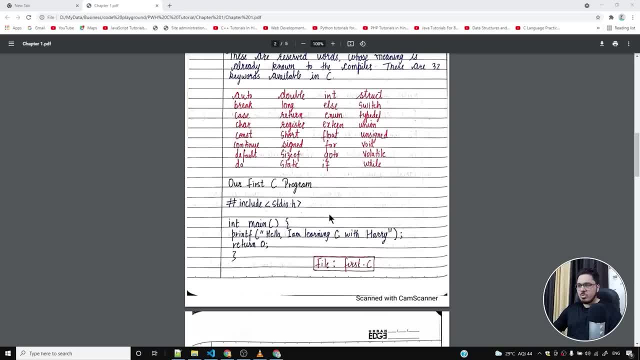 something, uh, you can even look at function as an entirety, enclosed in this curly braces. name of this function is main. int is something that it returns, but we'll come back to functions in the later chapter. let's focus on, uh, this particular function, and let's let's think of function as: 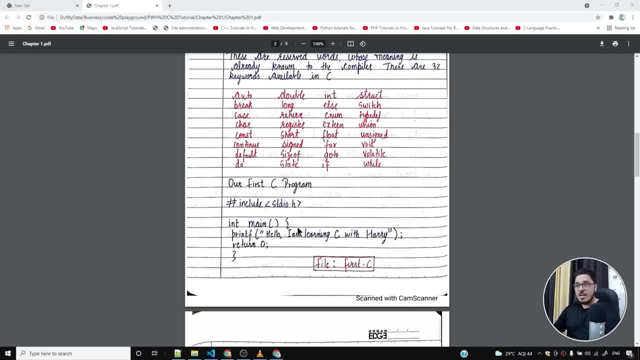 uh, let us say a box containing instructions. let's, let's see function in a very, very uh layman terms of uh box containing structure instructions. so build dev- hello, i am learning c with harry- is instruction. return zero is instruction. but for now, what we will do is we'll ignore this return. 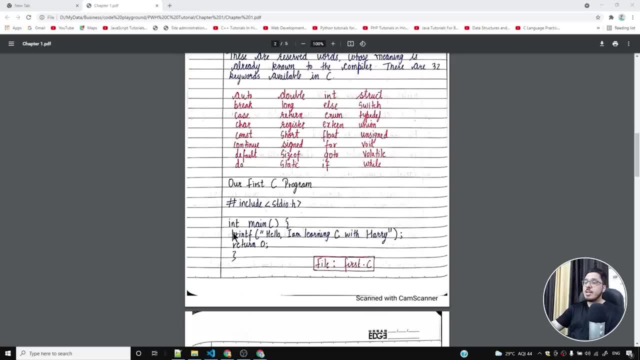 zero instruction. definitely it's doing something, but let's ignore this part of the program in main and return zero. let's look at this piece of the program as something that we will have to write to execute the program and, believe me, we'll come back to this and we are going to 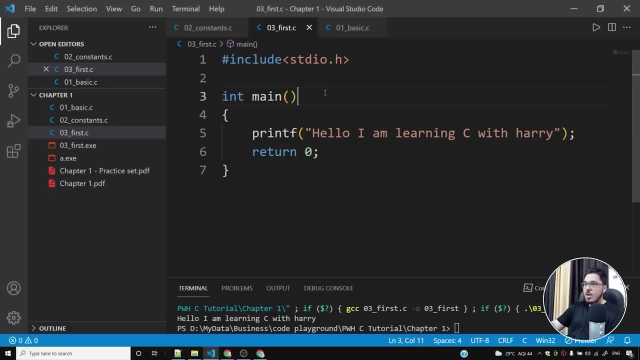 understand all these things in a real great detail. also, this is a header file and we are going to talk about it as well, so let's ignore. line number three and four and line number six and seven and whatever is between this and this, which is a single line, will be executed by the. 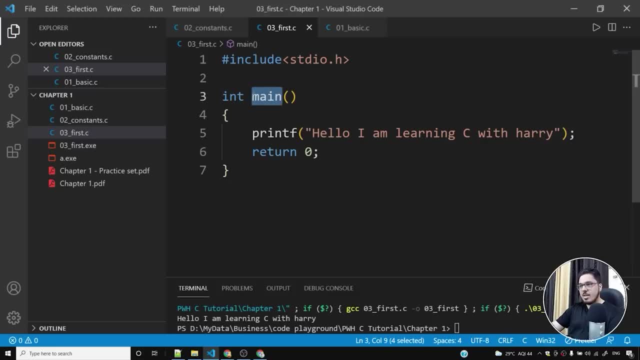 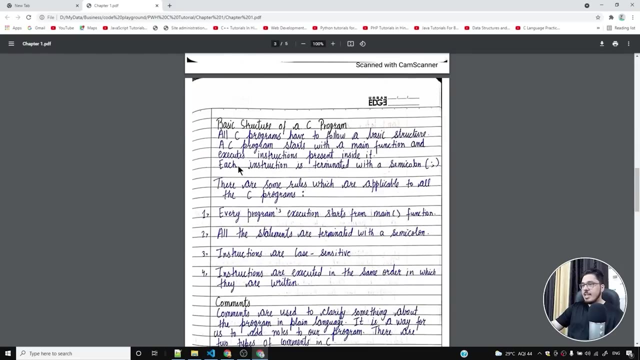 program. let's look at this and let's also remember that we cannot change the name of this function. it has to be main, because main is the function which gets executed whenever your program runs. okay, so i hope i explained this program to you pretty well. let's move ahead and let's see each structure is terminated with the. 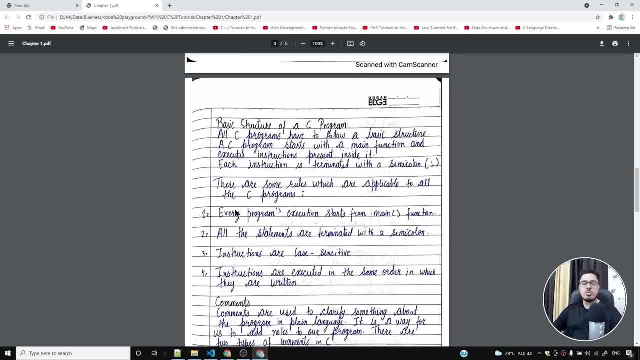 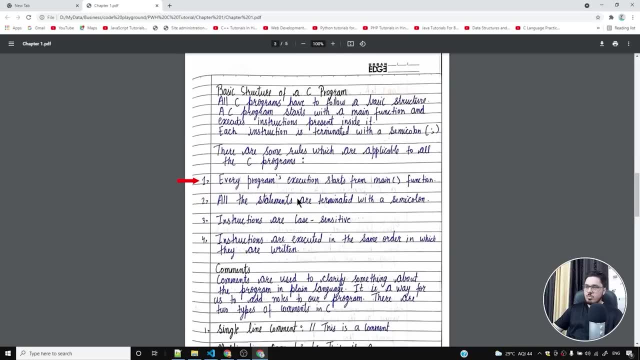 semicolon. there are some rules which are applicable to all c programs and we're going to see all these rules now. so the rule number one is: every program's execution starts from the main function. so whenever we are executing a program, the execution starts from the main function. 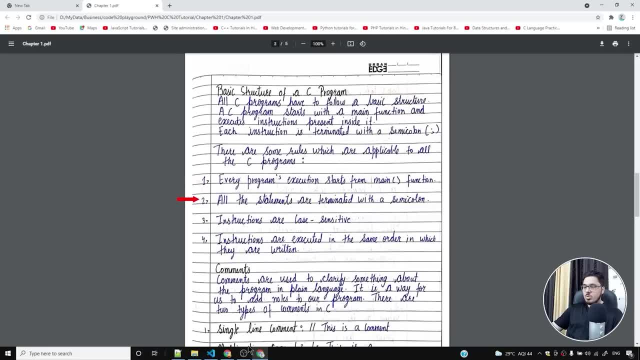 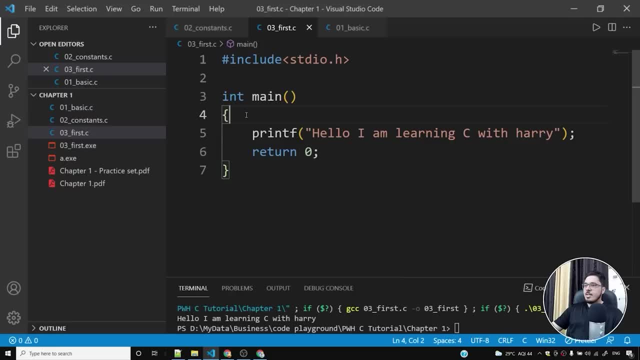 all these statements are terminated with the semicolon. so this is instruction. it is terminated with the semicolon. this is instruction. it is terminated with the semicolon, with a semicolon. this is actually part of this function, so this is not terminated with a semicolon. also, this is a part of the function. this is function definition, so this is not terminated. 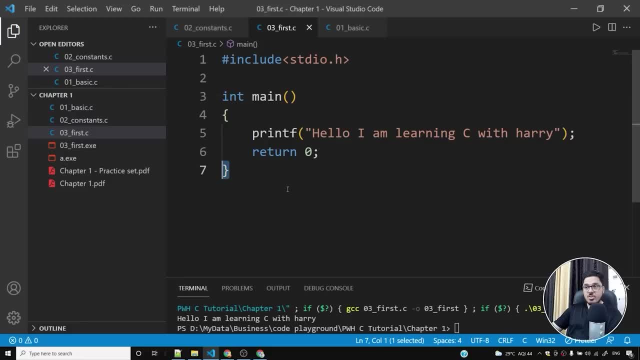 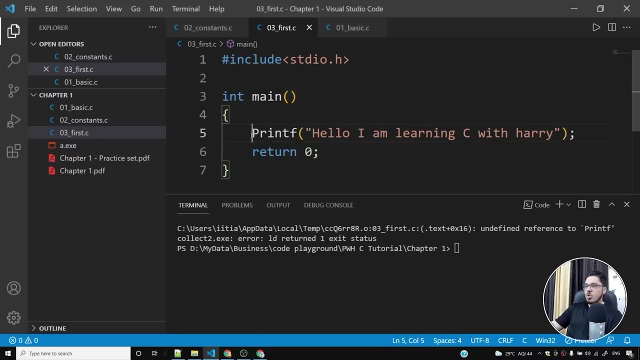 by a semicolon. we are going to come back to functions and function definitions, so please bear with me until that time. now, instructions are case sensitive. if you type something in capital p, if i say capital print def, this is going to show me some issues, because capital print def is not. 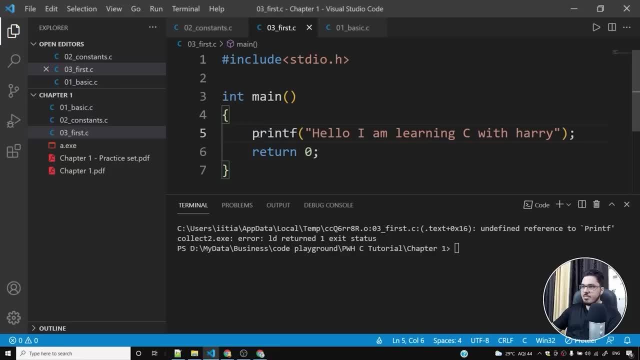 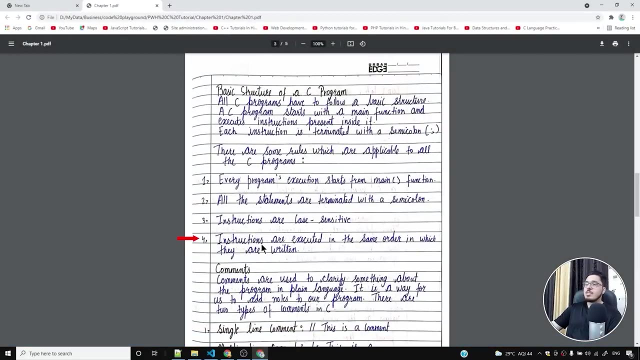 a function to print it's small printf, so it is case sensitive. do not change the case of the function names or the keywords, or the function names for that matter. i hope you are enjoying and understanding what i'm trying to tell you. instructions are executed in the same order in. 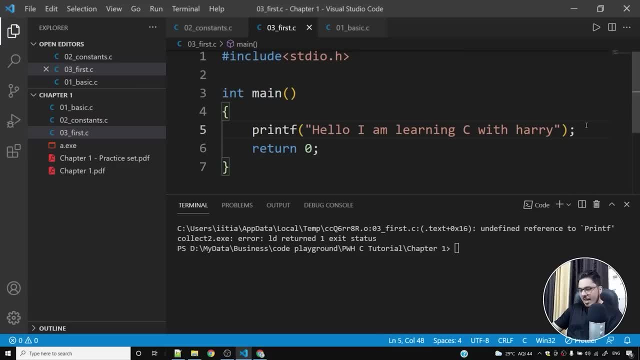 which they are written. so if i have written hello, i am learning c with harry first, and let us say i write another hello after that. this is going to print first and this is going to follow you, the first print statement let me show you. so what i'll do is i'll save this program and run this. 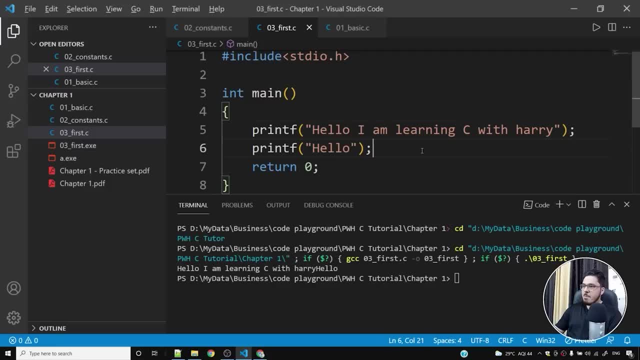 you can see hello- i'm learning c with harry and hello has been printed. but if i shift this line above this line, then hello will be printed first and then hello i am learning c with harry will be printed. let me show you so. i accidentally selected it and ran it. you don't have to select. 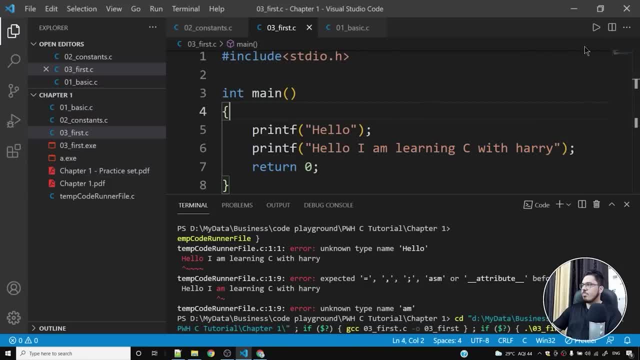 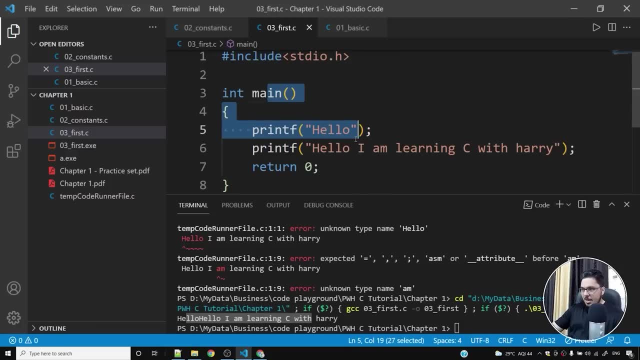 it and run it. so i'll click somewhere and once again i'll try to run it and you can see: hello, hello, i'm learning c with harry- has been printed on the screen. so never, never, select a part of program and run it if you don't know what you are doing, because whenever 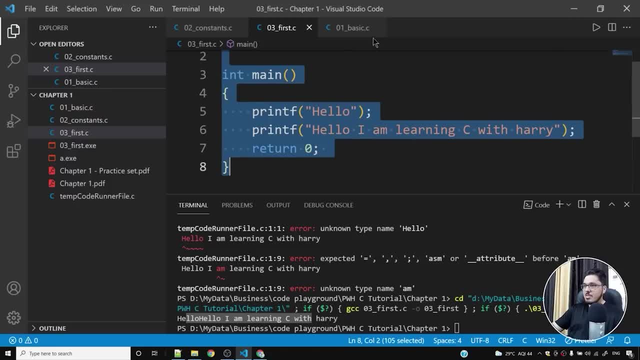 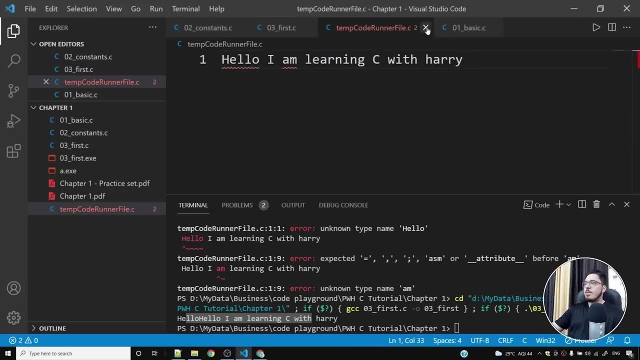 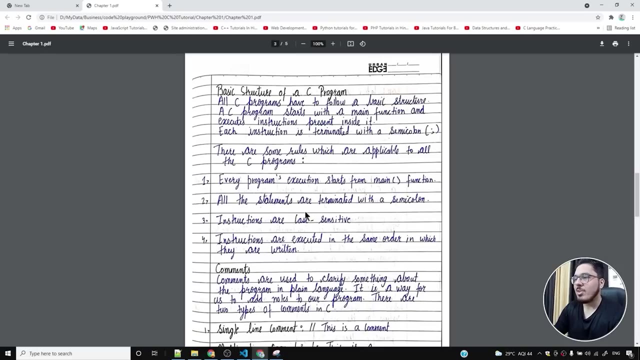 you select a part of program and try to execute it, what happens is it is copied to a file called temp code runner, filec, and you are going to be in trouble. okay, so always make sure that whenever you are running your programs you're not selecting a part of it, okay. so coming back to nodes we have, 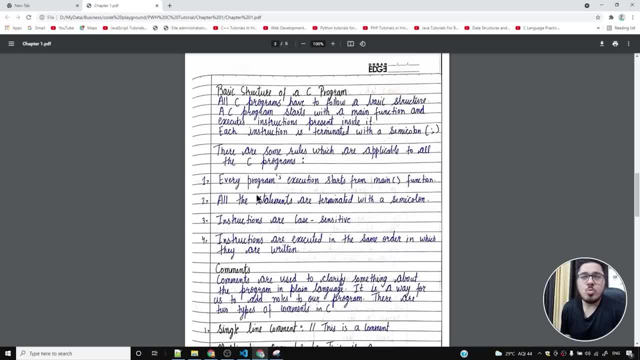 understood what the basic structure of c program looks like. you might also have some ambiguity in your mind. you might have some ambiguity in your mind. you might have some ambiguity in your mind. you might be thinking: what is this main? what is this end? what is this curly bracket? but i want you. 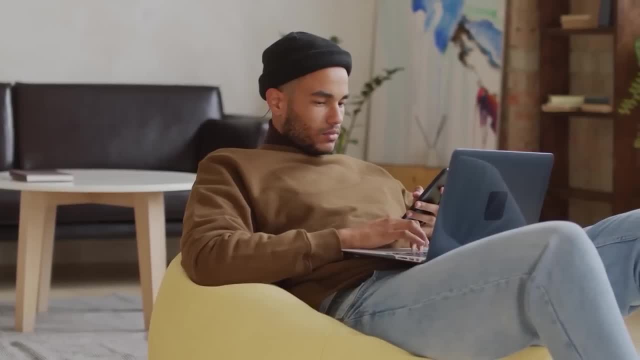 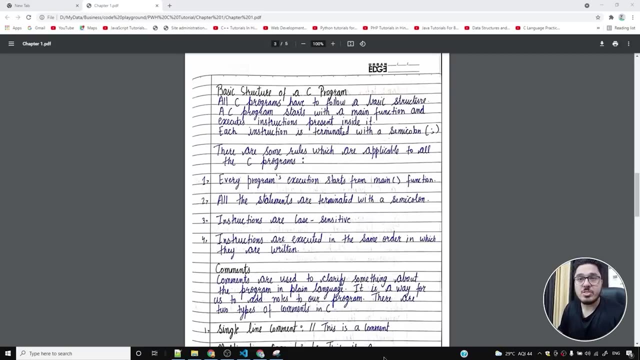 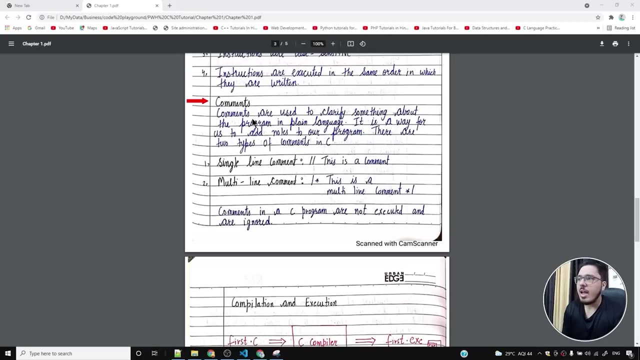 to please sit back, relax and just listen to me for some time, and as we move ahead in this course, you are going to clear a lot of your concepts, i promise you. so let's now understand the concept of comments. what exactly is comment? so comments are something that is used to clarify something about the program. 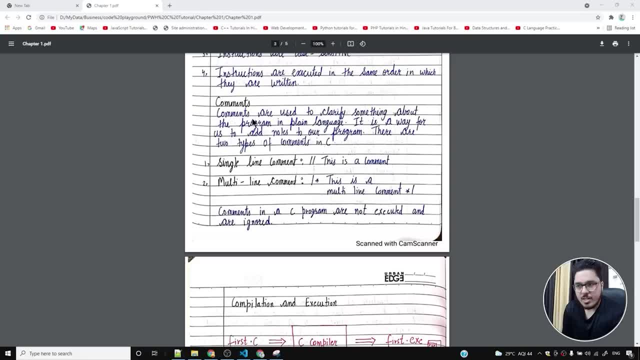 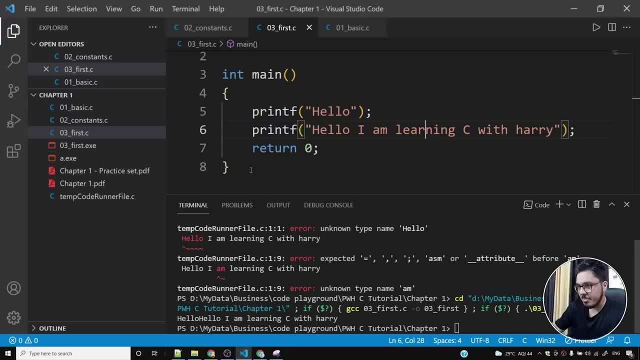 in plain and simple language. let us say me and you are working on a c program. what do i want to tell you? that please do not, uh, touch this function. i'm going to write it. if i write something like this, if i say that i want to write code to read the user mic, if i, if i write it in plain text, what is going to happen? 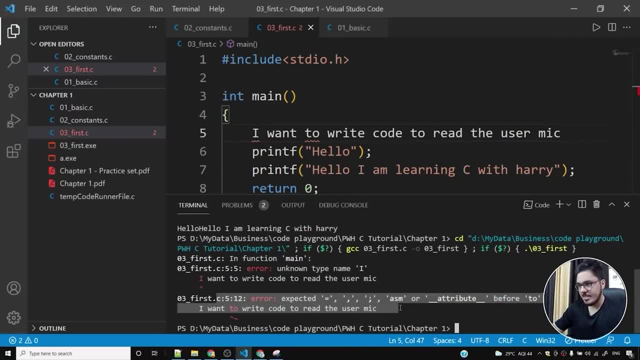 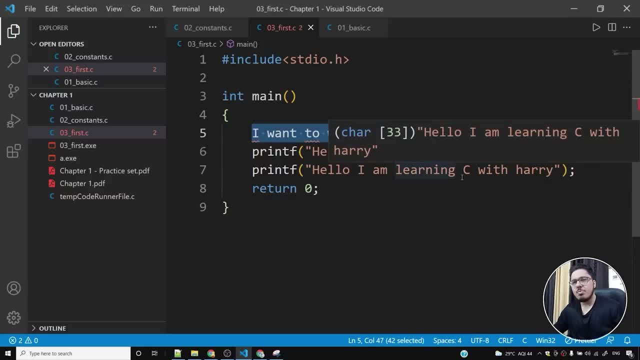 if i run this program i'm going to see some errors. you can see that c language compiler is telling me that this is not a valid c code. please do not write it here. another option for me can be creating another text file with the same name as that of program and putting all these 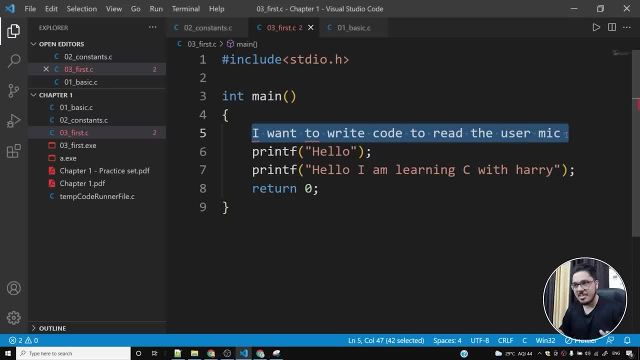 comments with line numbers, but that will be really very tedious. so c provides the mechanism of comments. you can add comments to your c program. all you have to do is simply use these double forward slashes. this is a single line comment in c, and what it tells your c compiler is that do not. 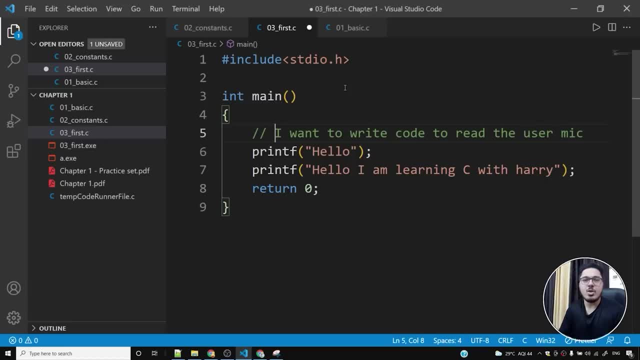 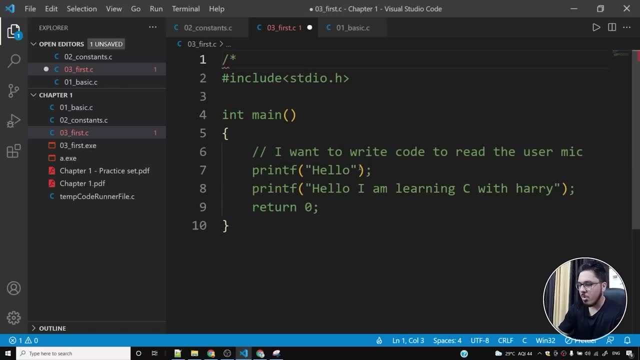 execute this line as an instruction. completely ignore this line. this is written for me, so i can also add some other details to my program using comments. there is another format of comment, which is multi-line comment. whatever you write between these two is a multi-line command. so if i say author: harry place india, i can write all these. 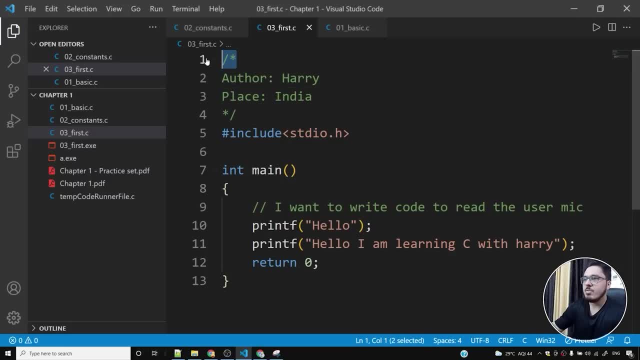 comments inside my this forward slash star and star forward slash and this is going to really make my life a lot, a lot easy, because i don't know if you guys know, but if you know, don't touch this easy, because i don't have to create a separate text file. also, it will be very easy and 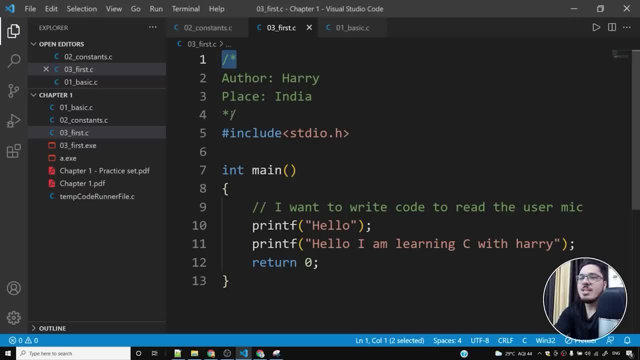 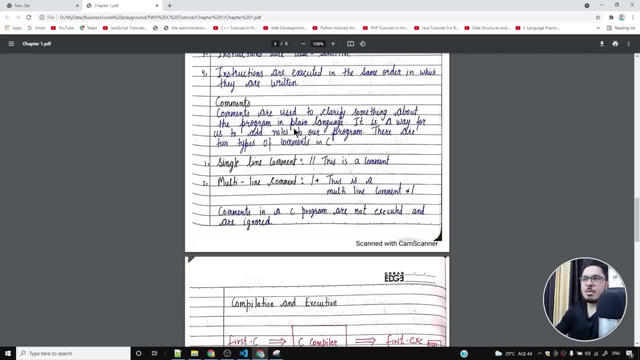 straightforward for me to mark few places in the program with some text. so this is all what comments do. coming back to the notes, comments are used to clarify something about the program in plain language. it can also be a specific place in the program, a specific line number, so it is a way. 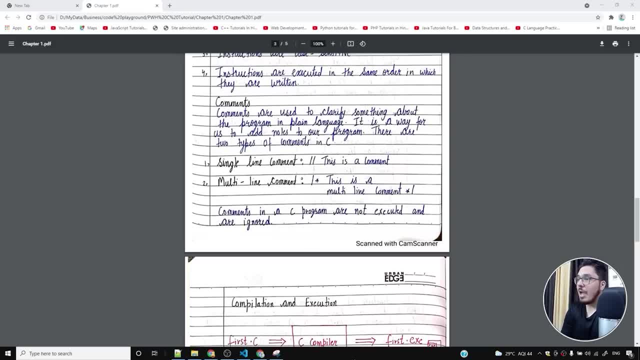 for us to add notes to a program. there are two types of comments in c. a single line comment is one. multi-line comment is another one single line comment is written like this: this is a comment. forward slash, forward slash. this is a comment. so this is a comment. forward slash, star. this is a. 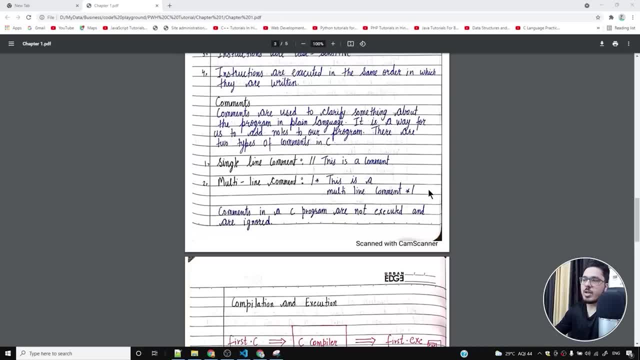 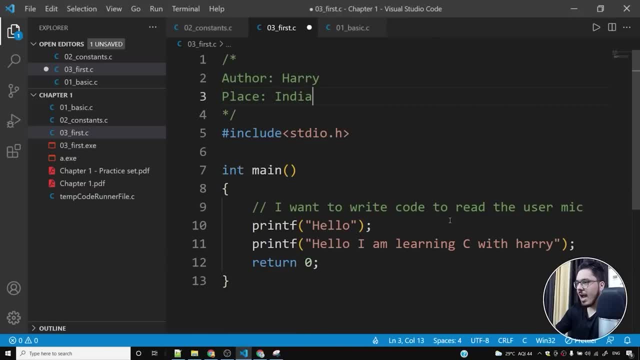 multi-line comment: star forward slash. this is a multi-line comment, so you can actually press enter and write as many new lines as you want, but here you cannot add new lines, because the moment you add new line, this particular line is treated as a separate instruction, and this might. 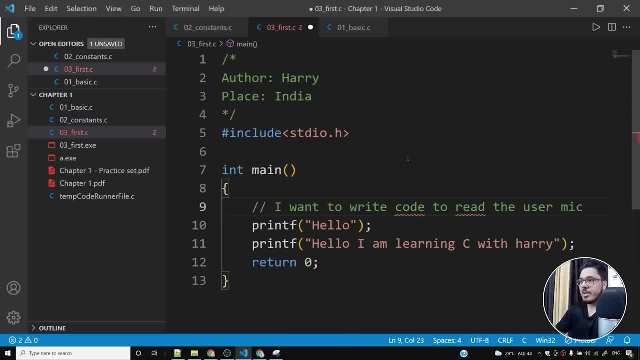 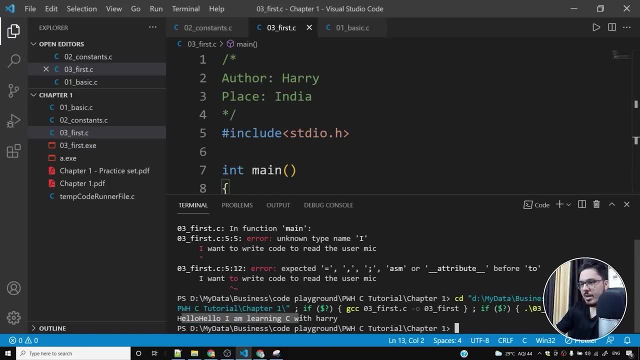 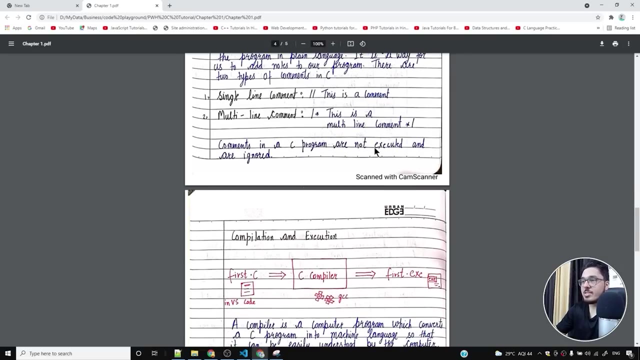 uh, cause some errors in the program. we don't want that, so i'll press ctrl z, i'll simply save and we can see that our program looks clean. if i run this program, you can see hello. hello, i'm learning c with harry has been printed. coming back to the notes, comments in c program are not executed and 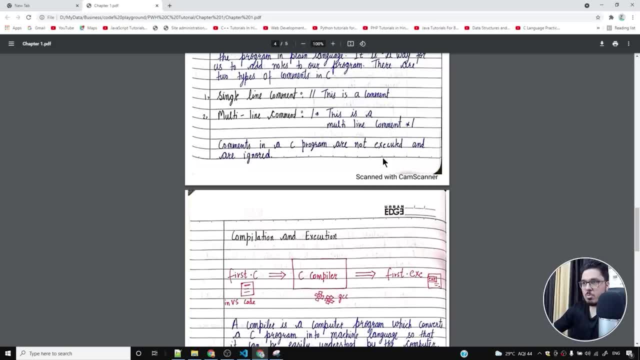 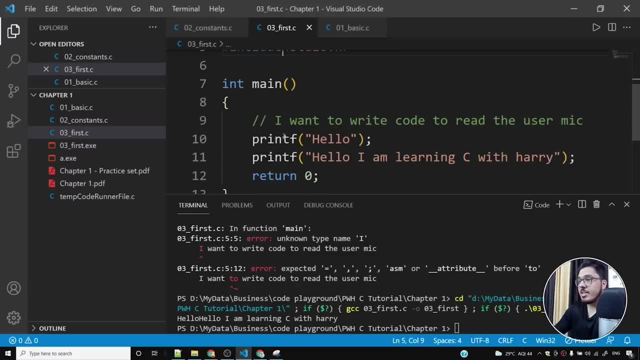 are ignored. so comments are ignored by the compiler. compiler will not execute your comments as instruction, even if it is some code. for example, if i comment this particular line out, i can use a keyboard shortcut which is ctrl forward slash to write single line comments. so the moment i 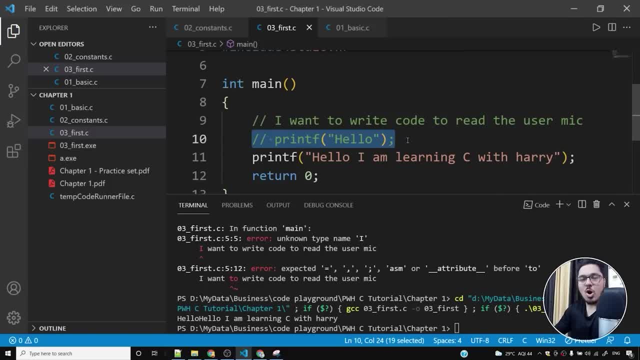 comment this particular line out. this print of hello will not be executed. so the moment i run this, you can see hello i am learning c with harry has been printed. so this is how this particular program works, and hello i am learning c with harry has been printed also. what i want to do is 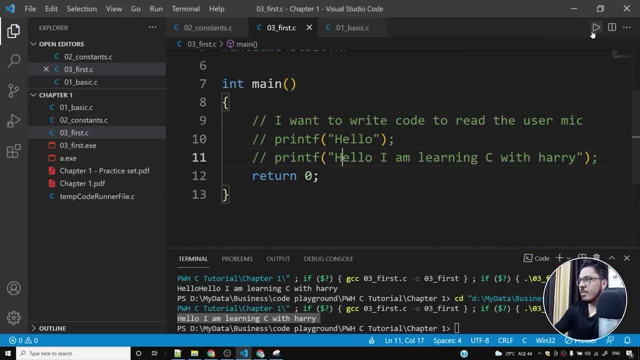 if i comment this line out, i can see: hello, i am learning c with harry has been printed, so i can. the same thing, we can add it right here, so we're gonnaorkan have a program as well. check out, интересно terribleover normalmente type c into anıl items space, and also we has purport to called it loading. 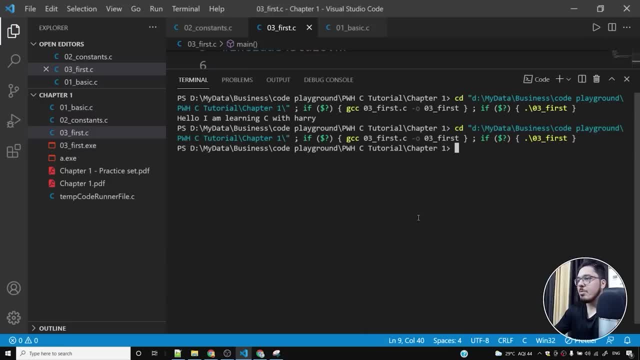 outcome as well. so let's just say that i can tell mu sons eram will going to log in by just that at any true account. no, nothing happens. a program has no instructions, so it simply executes the same Programm. need to cascade: all programs will automatically execute main files. we don't. 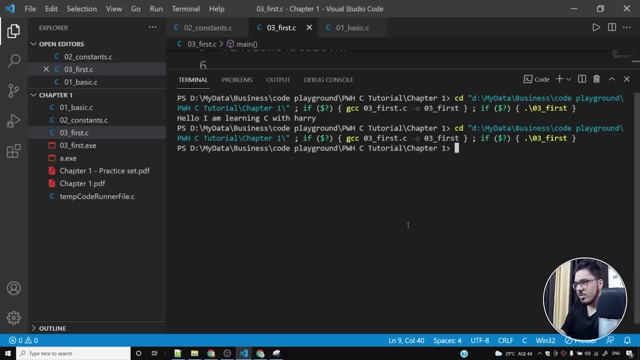 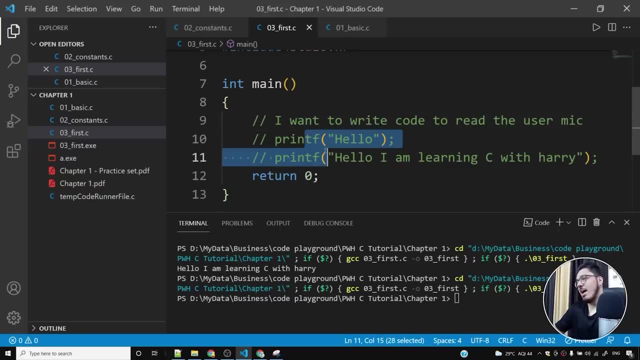 executes and exits. let it go because there are no instructions to execute inside the main. cą l, but ideally otherwise. i am observing no. mais ac captured cute analytic issues in the look. it should pop. we'll not have this kind of scenario. we will have some instructions. 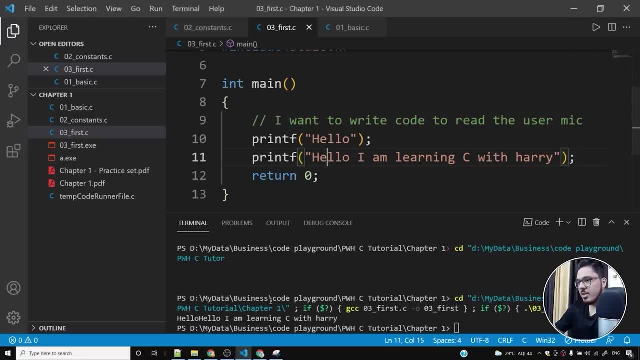 no main happens. we'll have some instructions that we want to execute and you see that the come about using the same shortcut of control: forward slash. we can see that i am now able to. you can see that i am now able to see hello and hello. i'm learning c with harry printed on the. 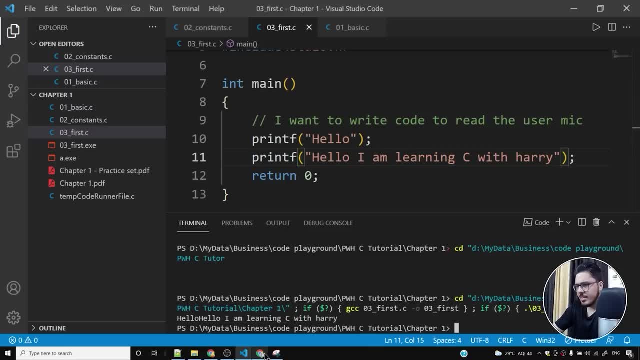 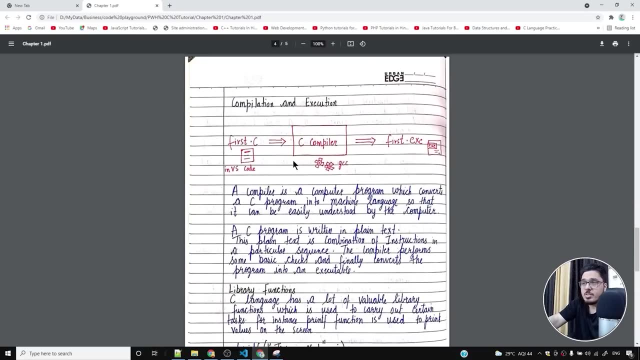 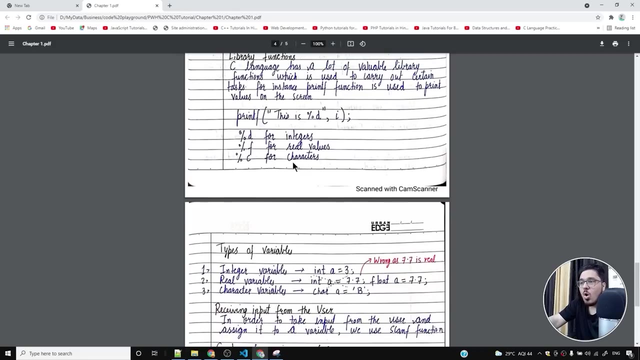 console. so i hope you understood all these things. i hope this was easy for you. now we are going to learn about, i would say, the most important concept in c programming language, which is a concept of compilation and execution. and do not get haunted with this concept, because i'm going to explain. 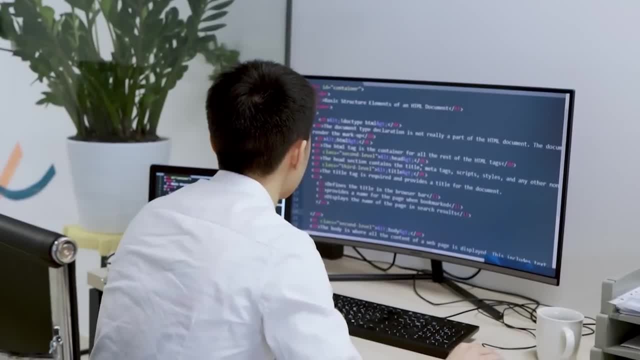 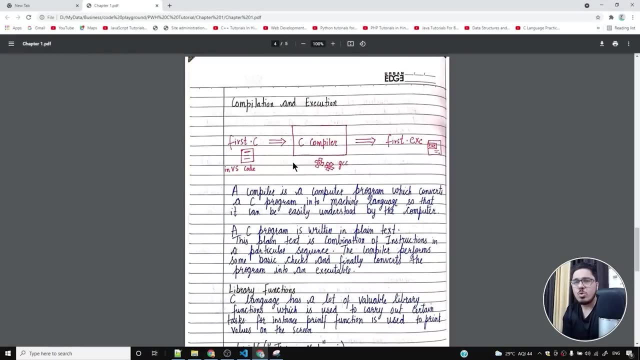 you in a very simple way and you don't have to understand how compiler works. if you are a programming beginner, yes, if you are in the field of compilers, if you are a compiler expert, maybe you, you might want to look into those topics. but for the sake of this tutorial, for the sake of 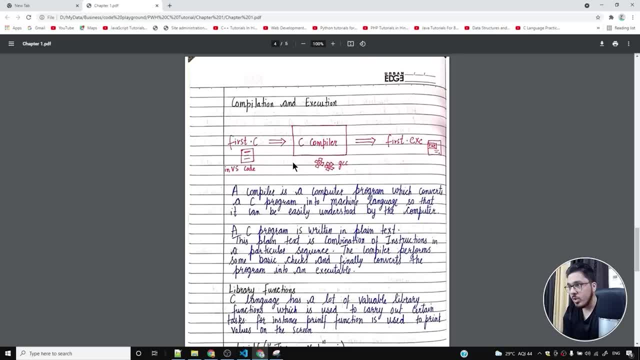 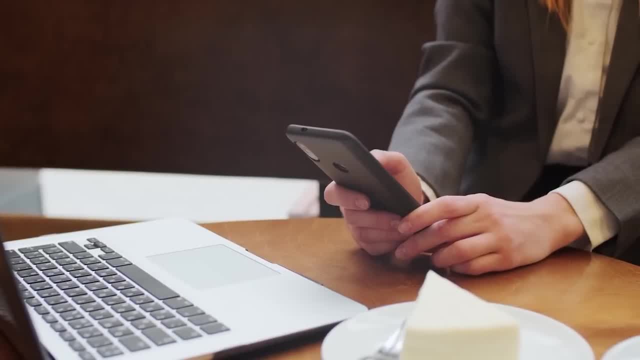 learning c programming language. i do not recommend looking into ins and outs of working of a compiler. you should know how to use a compiler, just like you know how to use your cell phone. you know how to use your laptop, but there's a high chance that you do not know. 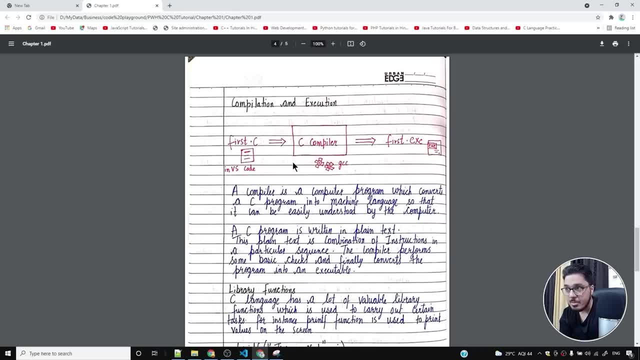 what is happening inside the chips of your laptop. in a very similar way, we are going to use the compiler and maybe in the future, if you are, you know, choosing that field as your major, you might want to look into what a compiler is. but for the sake of this tutorial, let's understand how compiler 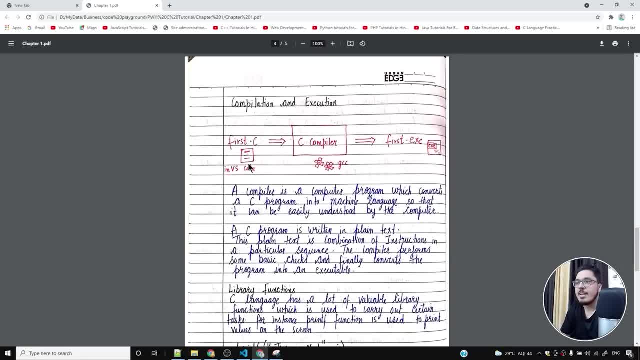 works. so firstc in vs code is the file that i created. it is no different than some file that we create using notepad or using microsoft word or some other text file for that matter. microsoft word is not a plain and simple text file. it is a plain and simple text file. it is a plain and simple. 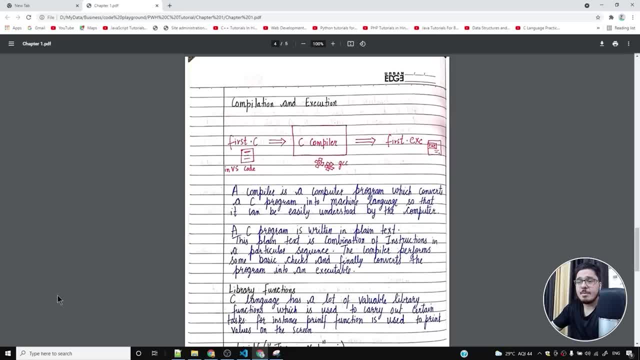 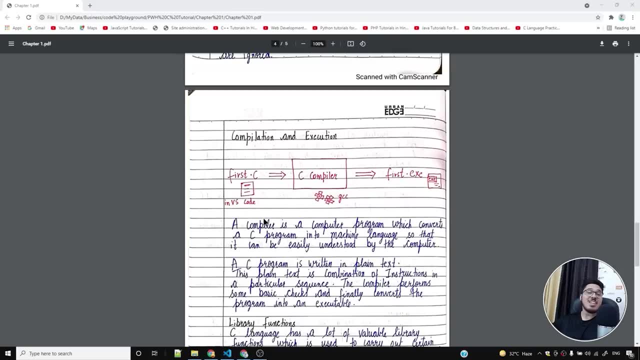 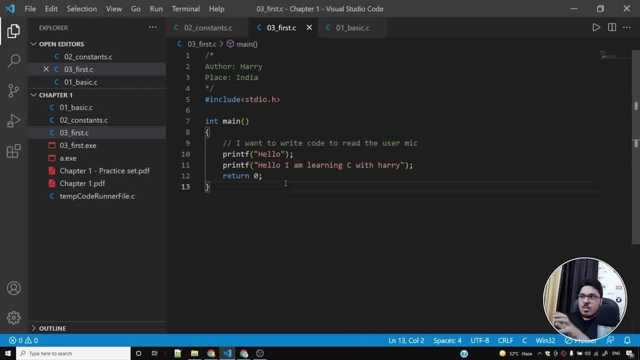 file. it might be a binary, because it is created using ms word. so what basically happens is that we have this source code file. we have some characters written inside this file, just like we have characters in the notepad. so if i show you this file, it looks something like this. now this file: 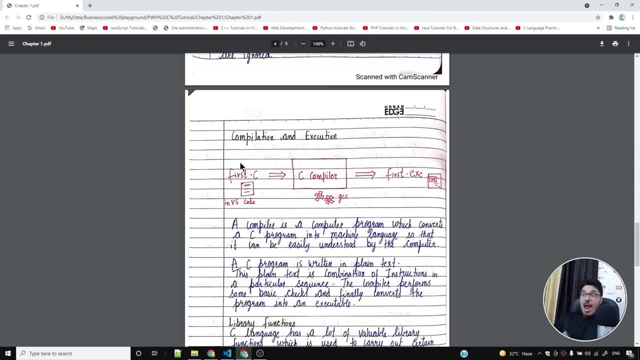 will be taken as input by the c compiler, and what c compiler, which is gcc. what it will do is it will convert it to a code which is understood by my operating system. so what it will do is it will convert it to my operating system, which is understood by the machine i am on in this case. 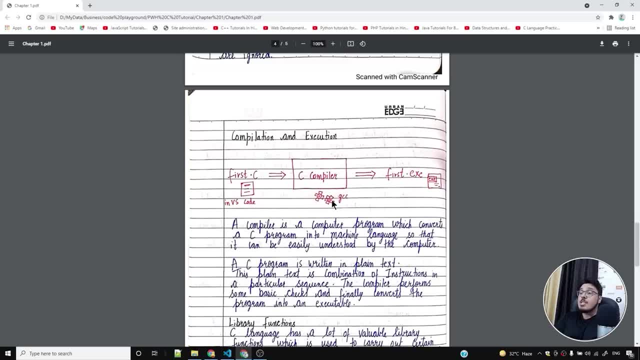 windows machine. so for the windows operating system this particular source code will be compiled, and for windows it is compiled to a firstexe file. soexe is the file extension to which it is compiled in windows. so let me show you this thing. i'll come back to my vs code. i'll 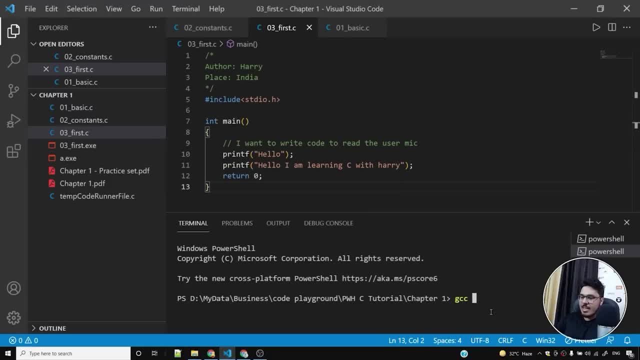 open the terminal, i'll say gcc, i'll say zero three, obviously, after a space i'll say zero three, underscore first dot c, and the moment i press enter i'll get a, a dot exe. so a dot exe is the file which is generated. but in case i want to get a file with a desired output name, i'll say: 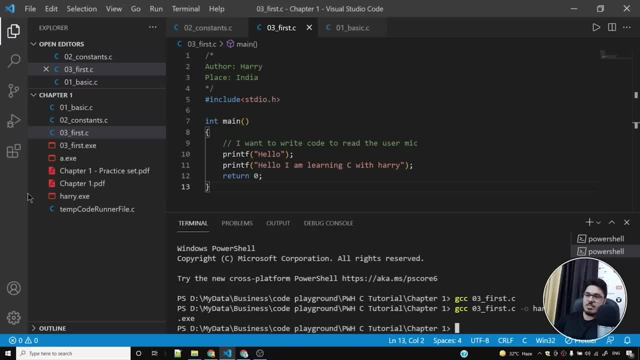 harryexe. so a harryexe will be created. now, if i type harryexe- uh oops, i need to type something like this- it's telling me that you need to type this instead of harryexe. so i'll obey the instructions and the 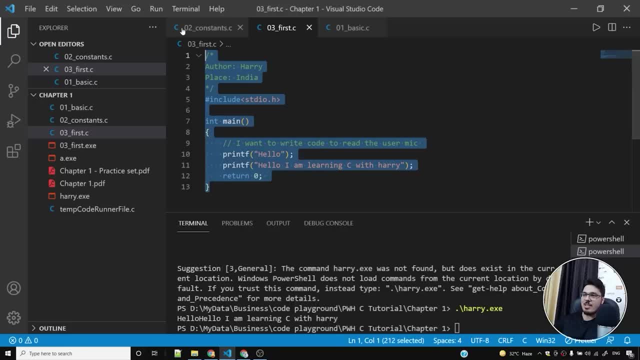 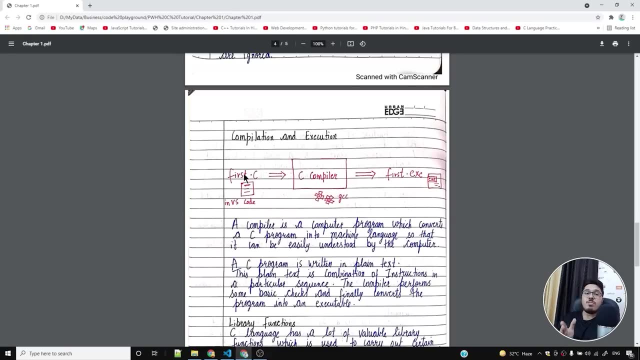 moment i do this and press enter, you can see that this program is being executed. so how is it working? let me explain it to you once again. so firstexe is a universal code file which can be circulated around to any operating system. but once you are into an operating system, what is an? 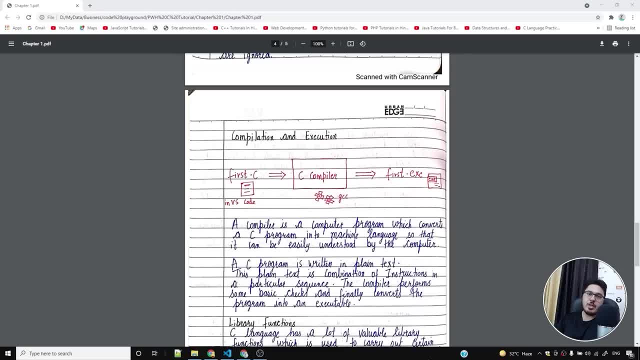 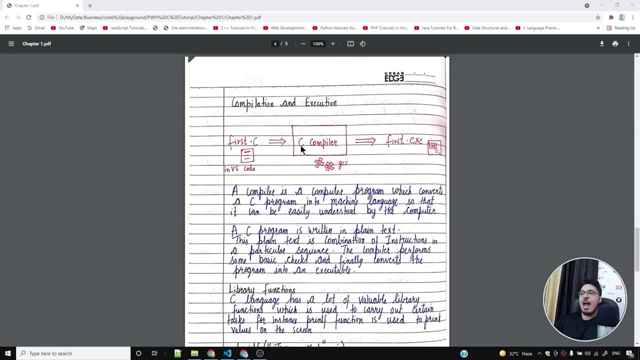 operating system. linux is an operating system, mac is an example of operating system, windows is an example of operating system and there can be a number of operating systems, but at this point what we are worried about is we need a compiler for our operating system. i have installed a c compiler for windows and the moment i use that. 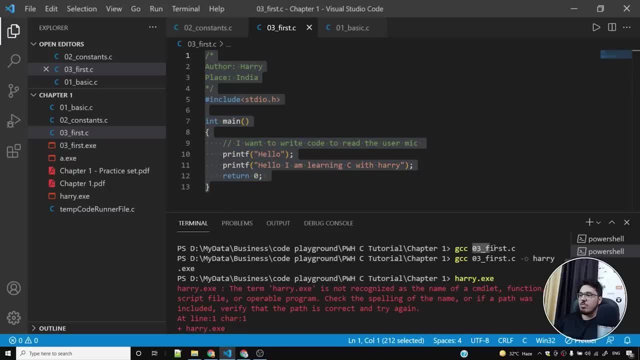 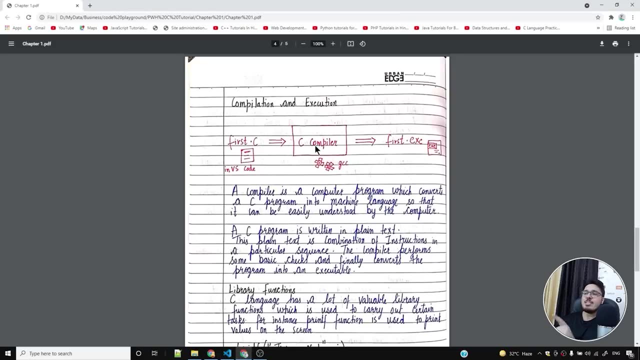 compiler using gcc 03 underscore: first dot c minus o: harry dot exe. what i'm telling this compiler is i'm saying: hey compiler, hey c compiler, i have this first dot c file. please take this file as an input and spit out a file which is compatible with my operating system. so first dot exe is generated. 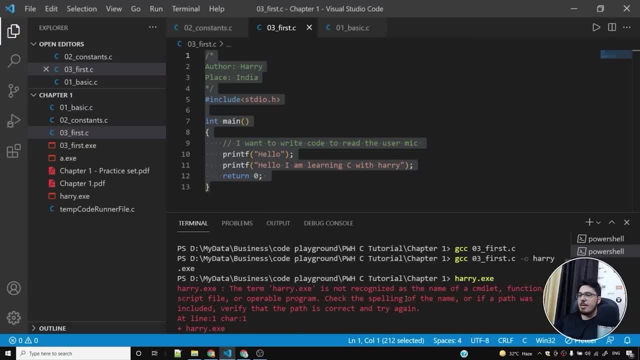 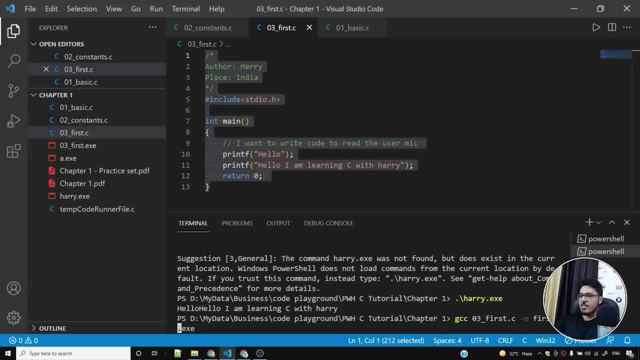 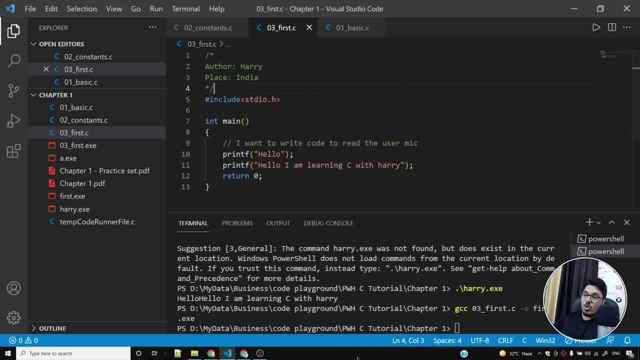 since i've written harryexe. harryexe is generated. but let me do one thing: let me make it firstexe. so what happens is firstexe. this file will be generated after compilation of this source code file. now i cannot distribute, or rather take this file to some other operating system. this is a 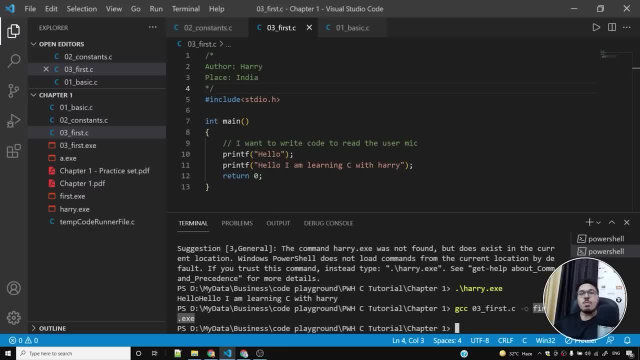 binary for window. this is an exe file for window. this will only work in windows. i cannot take it to mac and run directly. directly it's not possible to run. maybe you can use some virtual machine. there are a number of ways to run it in mac. but again, we are talking about straightforward, direct. 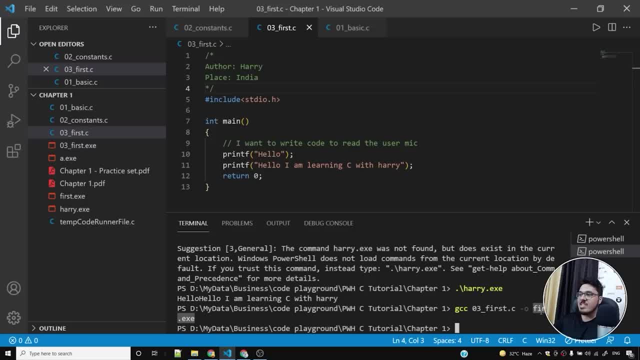 running from the terminal. you cannot do that. you cannot take an exe file and run it in mac or in linux directly. you will have to use this source code file and once again compile the source code file for your operating system, and then only you'll be able to use that binary. i hope i'm clear. 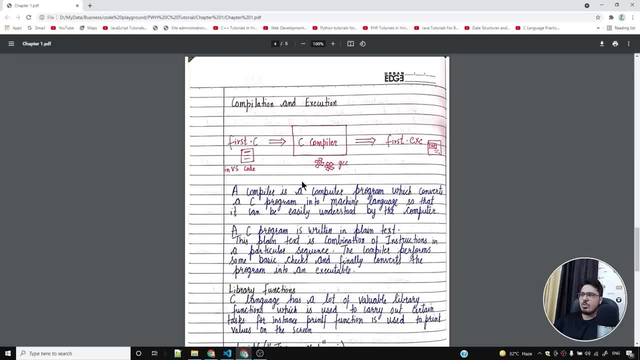 i made these things easy for you. so, coming back to the nodes, a compiler is a computer program. what is a compiler now? compiler is also a computer program and it might sound strange to you. if compiler is a computer program, who compiled the compiler? please do not think all these things. 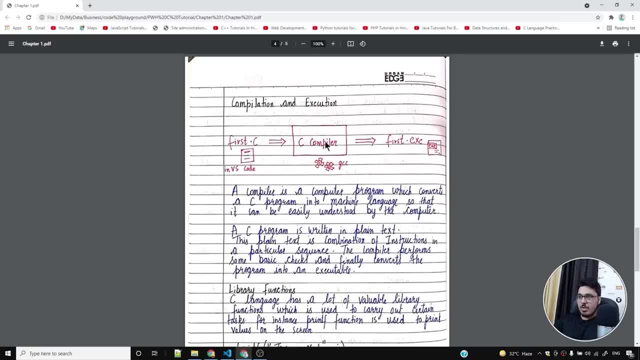 just focus on how this compiler is working. this is a computer program, which is gccexe. i've shown you. we have seen this gccexe file. what it is doing is it is taking firstc as the input and it is fitting out an exe file for my operating system. this exe file is supported by. 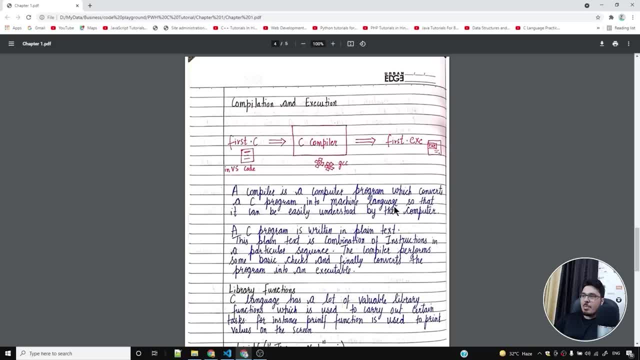 my operating system. it converts a c program into machine language so that it can be easily understood by the computer, and that machine language is not uniform across operating systems. it is specific for a windows operating system, for a mac machine or for a linux machine for that matter. but you will have to compile it for your machine and the source code file can be distributed. 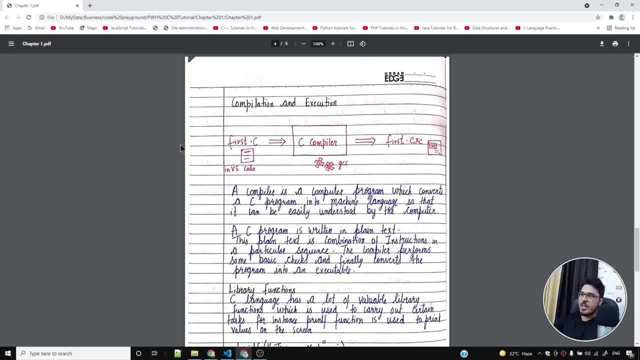 across operating systems. you go to the source code file and you compile it for your machine. go to some other operating system, take the source code file, compile it for your operating system and you are good to go. a c program is written in plain text. the plain text is combination of: 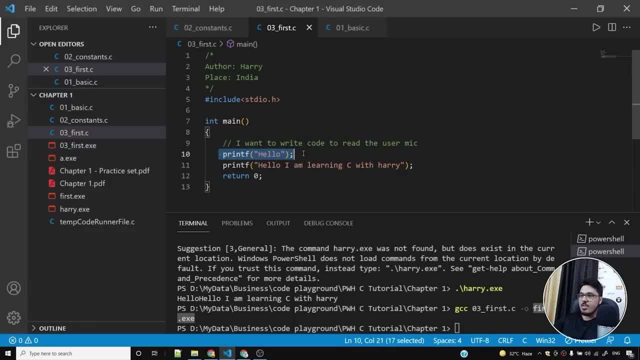 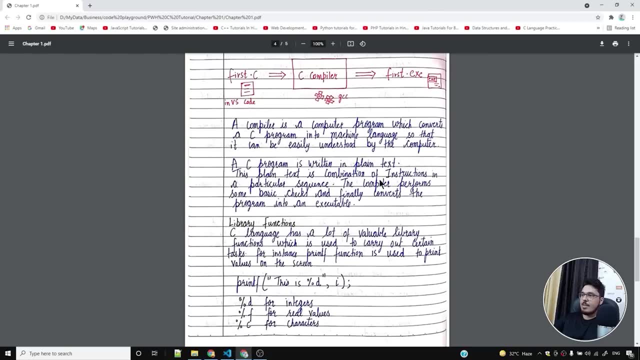 instructions in a particular sequence, just like we saw here. this is an instruction, this is an instruction and this program is a set of instructions. we have already seen that now the compiler performs some basic checks and finally converts the program into an executable. so this is a program. this program will be converted to an executable, which is: 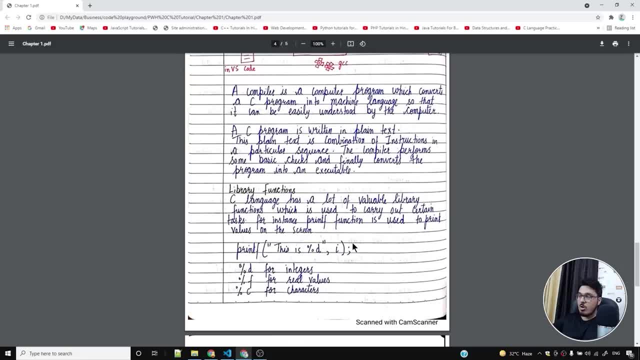 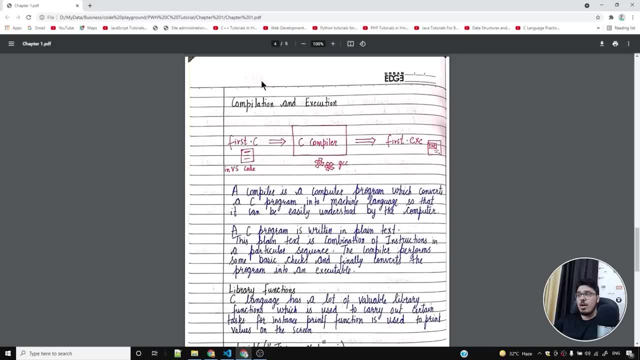 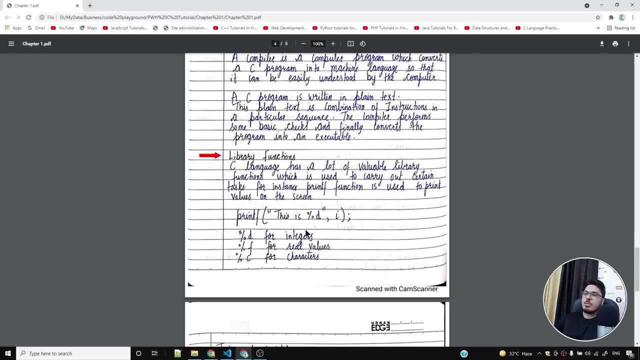 an exe file by my c compiler. so the c compiler will take the task of converting this particular piece of text, i would say, to a piece of binary which is executable or understood by the machine. i hope that is clear. now let's talk about some library functions. now, what are library functions? 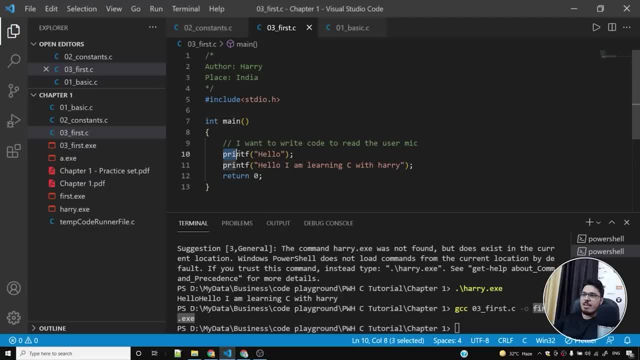 in c. remember we are using this printf, but we never defined it. where is this printf coming from? how are we able to use this printf and how does this work? let's talk about this. printf is nothing but a library function, so c language has a lot of. 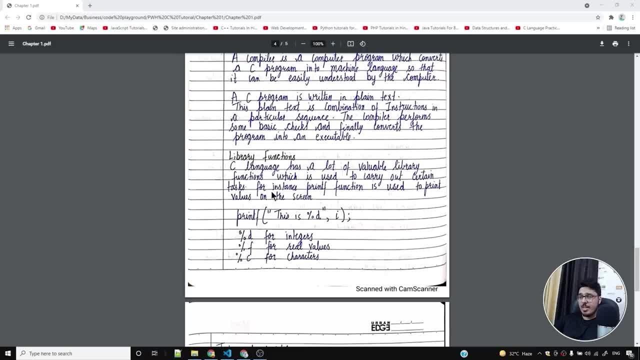 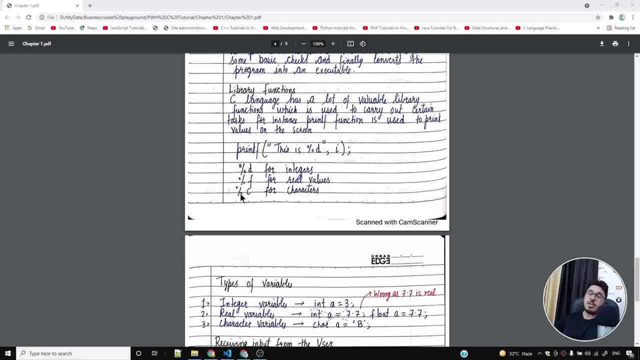 valuable library functions which is used to carry out certain tasks. for instance, printf function is used to print values on the screen. you can print values using printf, just like we are doing this. and percentage d is for integers, percentage f is for real values and percentage c is for. 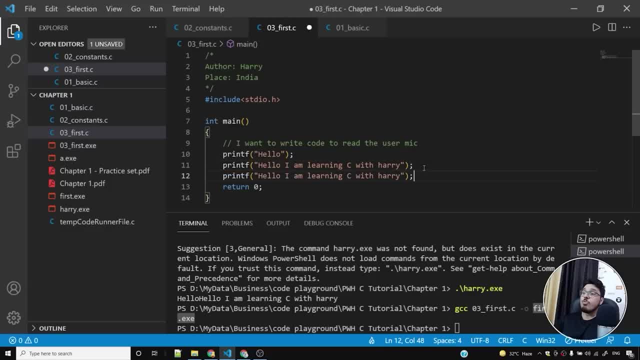 characters. we'll look into these once again, but if we want to print a number, i'll say this is an integer and i'll simply say percentage f- sorry, percentage d- percentage d is for integers- and i'll simply say a. i can say: int is equal to 3, it's an integer, int is equal to 3 and this: 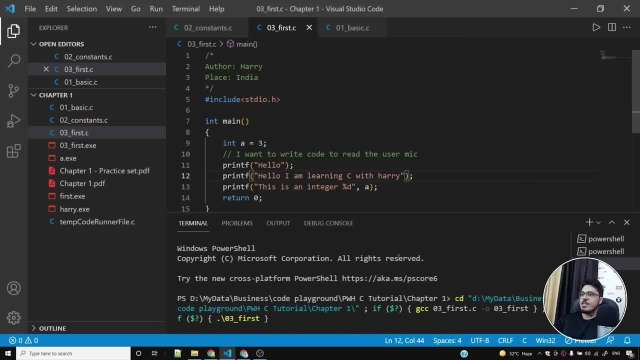 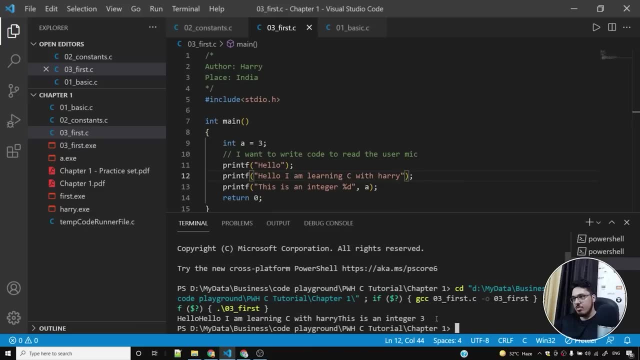 particular thing will print nothing, but this is an integer 3. so you can see this is an integer 3 has been printed. so this is how this- this is an integer 3- is printed on the screen. i hope you got the point. i hope you understood how all these things are working and i hope you also understood 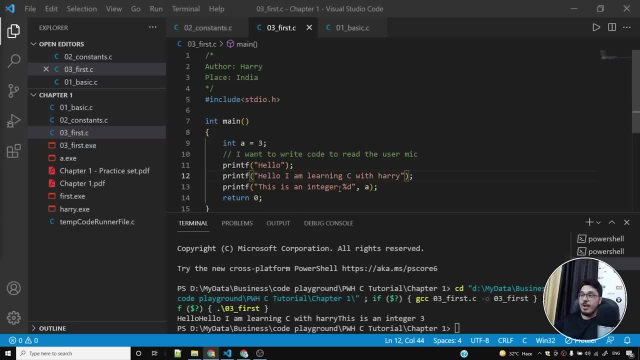 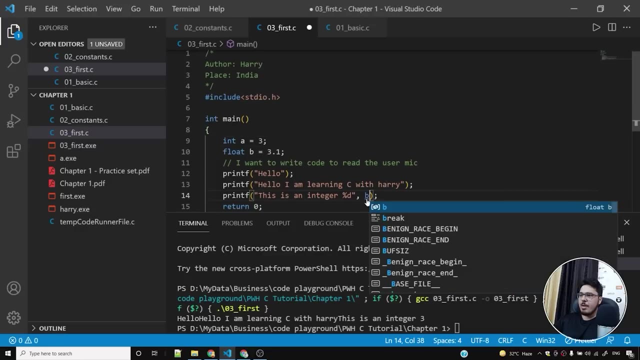 how i'm using this particular thing to print this particular integer. but what if we want to print a double? can i say: int b is equal to three, point. uh, sorry, float. i want to print a float, so i'll say: float b is equal to 3.1. can i print b? let's see what happens when i try to print b. this garbage. 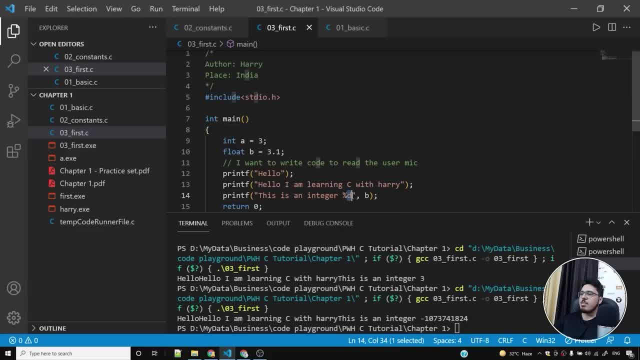 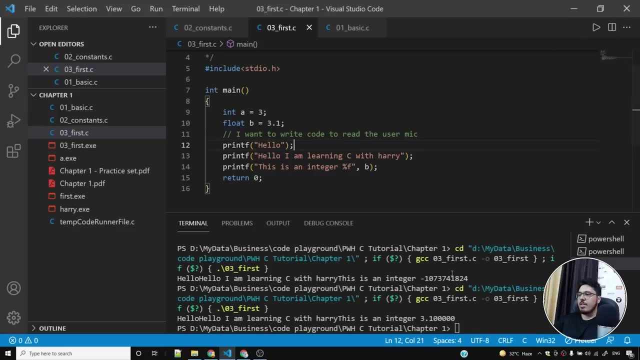 value is being printed. why is it so this is happening? because if i want to print a floating point number, which is a number with a decimal, i need to use percentage f. so now, if i run this program, you can see 3.1 is being printed. 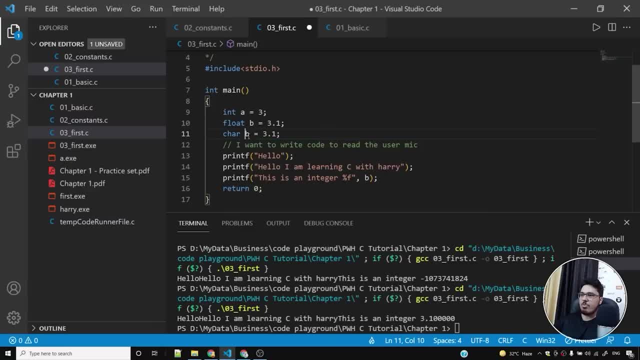 and this will work for character as well. so i'll have to say: char c is equal to, and whenever we talk about characters, we need a single quote. so single quote, and inside single quotes will be a character which will be printed on the screen. so what, what will i do? i'll say: this is a character. 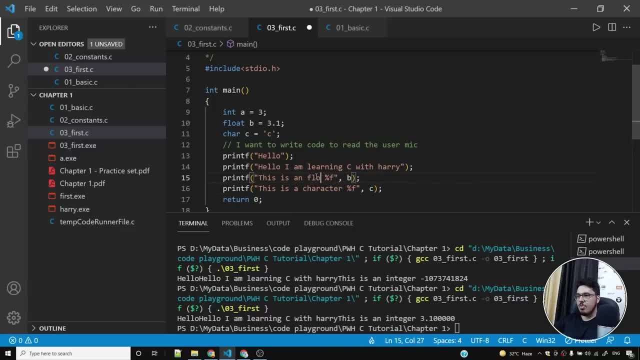 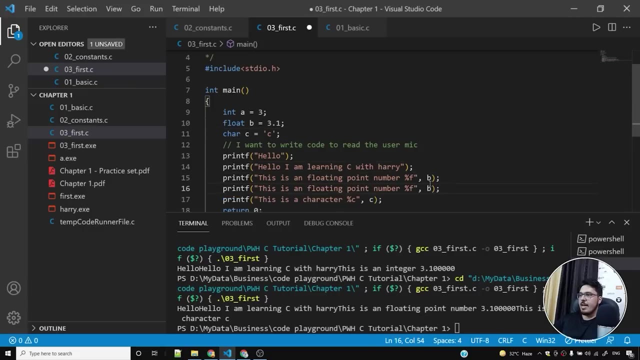 i'll say c and this is a floating point number, and i'll have to use percentage c for character. if i run this, you'll see this is a character c. this is a floating point number 3.1, and let me write this for a as well. this is an integer and i'll say this is a floating point number. let me 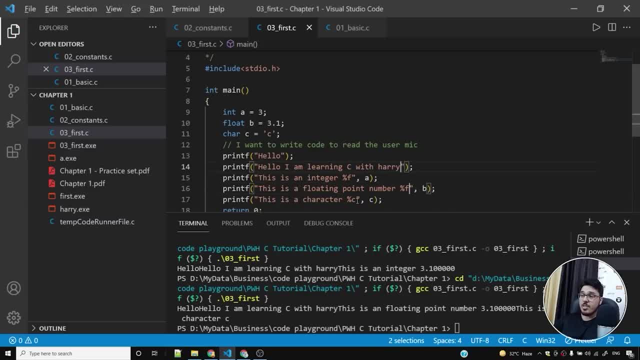 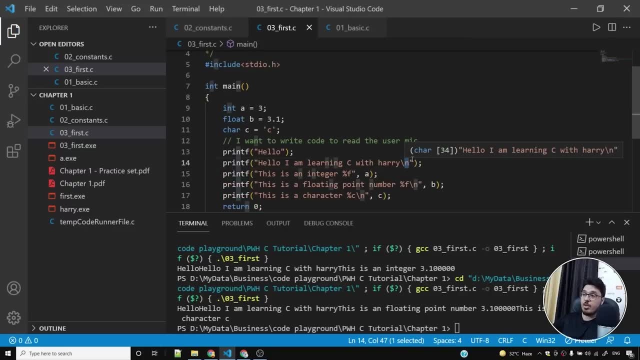 also add a percentage n. sorry, not percentage n backslash n. i'm sorry about that. backslash n is the new line character. it simply adds a new line at the end of your print statement, and i'll have to do the same thing here as well. so after every line i'm writing a new line character, just to ensure that whatever i'm writing. 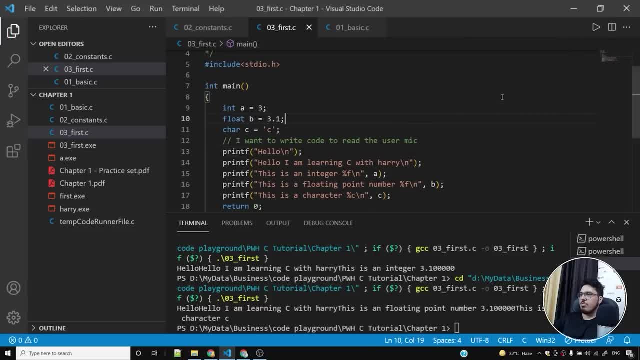 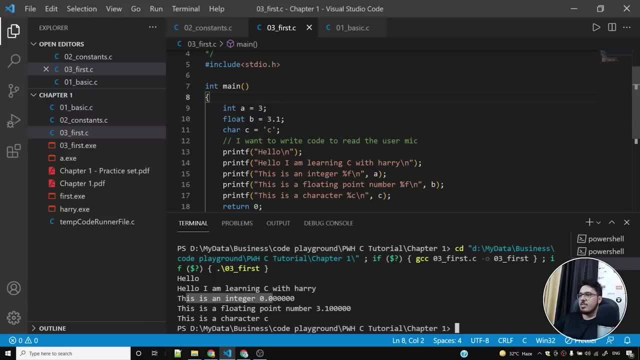 contains a new line at the end of it. so if i try to run this, you'll see hello, hello, i'm learning c with harry. this is an integer. why is it showing me 0? okay, i need to use percentage d for integers. let me run it once again. yeah, this is an integer. 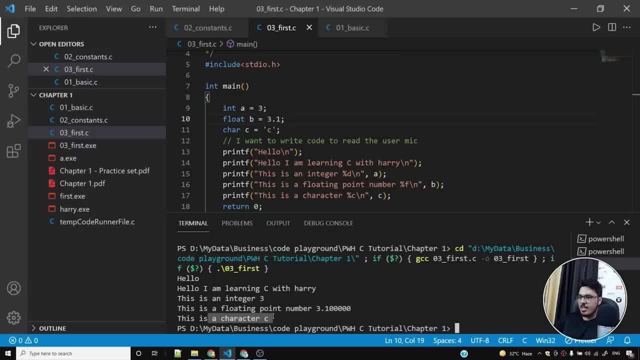 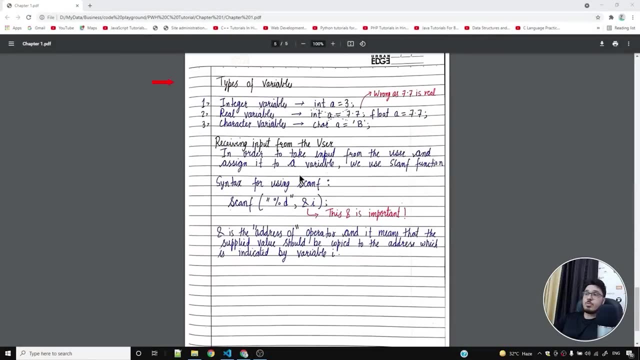 3: this is a floating point. number 3.1: this is a character c, and i hope you got the point. i hope you understood everything that i taught you so far. okay, let's now talk about the types of variables. how many types of variables do we have? we have integer variables, just like we saw recently. i 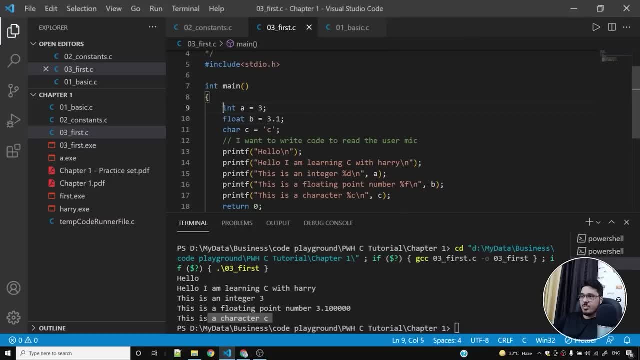 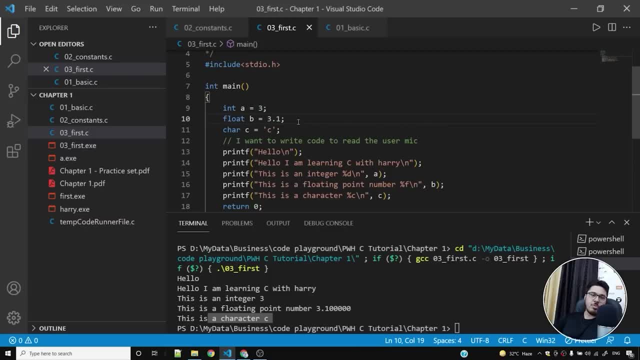 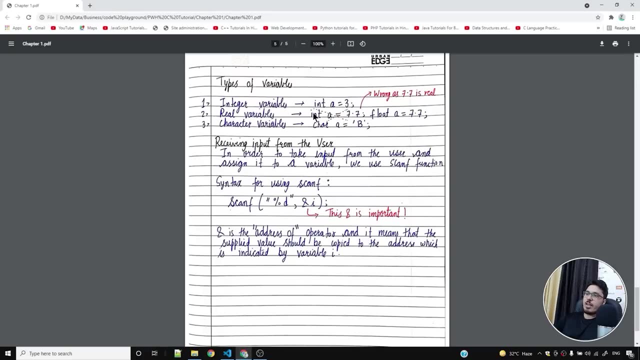 decimal number. we use floats. so we say float b is equal to 3.1 for floating point numbers. now what i'll do is i'll talk about real variables, and we have two types of real variables. we cannot do. int a is equal to 7.7. this is wrong. 7.7 is not an integer, it's a real number. it contains a. 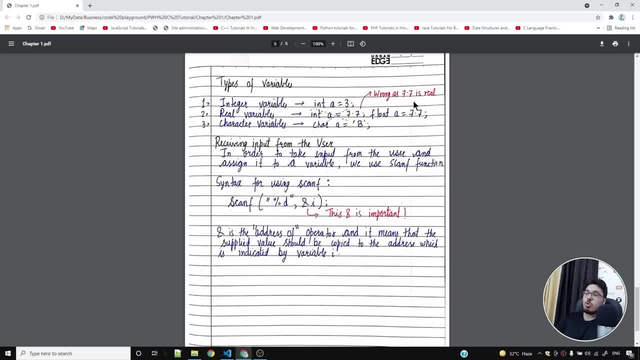 decimal and a number after it. so we'll have to use something called float. so we say float a is equal to 7.7, and this will store this number accurately and correctly. so character variables: similarly, we have character variables which are nothing but character containers. they simply store characters. 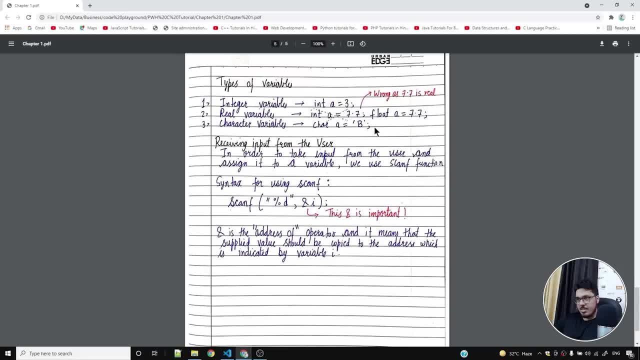 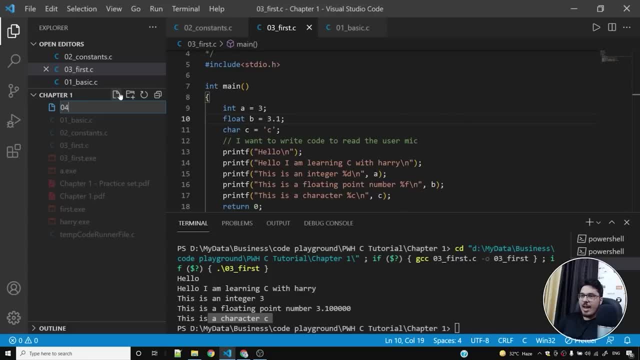 and you can store a single character inside these character variables. they take one byte in memory and let's not over receiving input from the user. so what i'll do is i'll create a file lc04, underscore, input dot c, and what this input dot c will do is 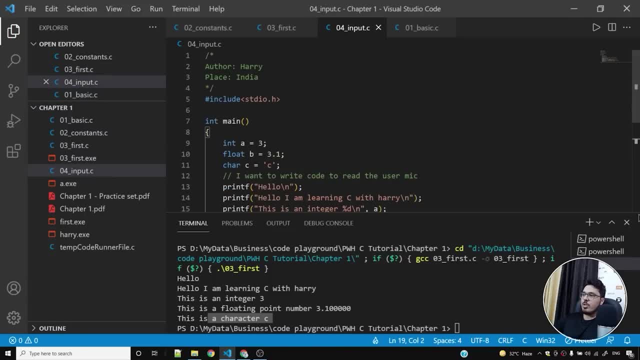 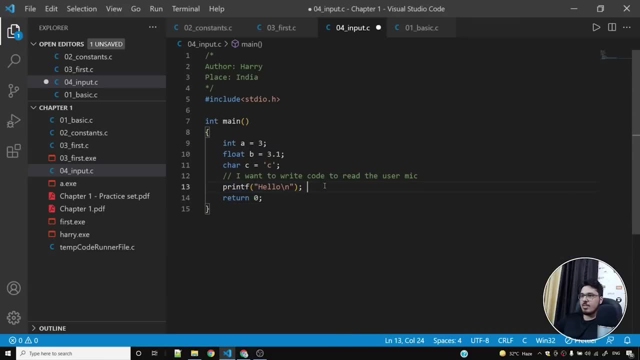 it will prompt a user to take an input. so let me show this to you. let me delete all these terminals. i've opened a lot of terminals. i don't want that. i'll remove these variables as well. now what i'll do is i'll say printf- enter your number, okay, and i'll simply say int a to declare. 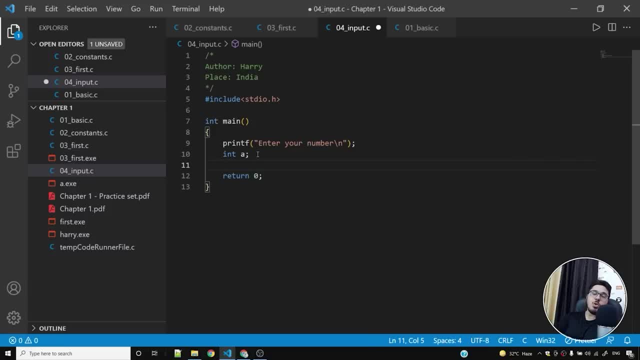 an integer. so basically, what i'm doing is just like if you want to have an empty container ready to store something in your house, you go to the market and you come back from the market and keep that container safely so that whenever you have something to store, you can simply put it inside that container in a very 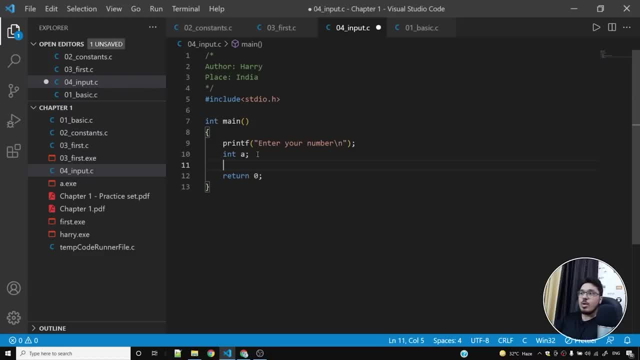 similar way. what i'm doing is i'm declaring an integer. so in case i have an integer to store in my program, i can use this container or variable and i can say: a is equal to 8 and it will be stored inside a. so i have simply declared a variable. now what i'll do is i'll use a function. 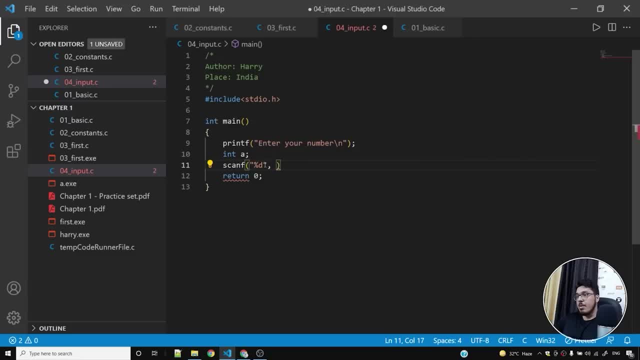 %d, because i want to take a number as an input and i'll simply say i'm %a. and let me explain this thing to you because this might sound very scary, and also let me show you something before we discuss about this. i'll say: printf: your number is %d and i'll simply say a and definitely i'll. 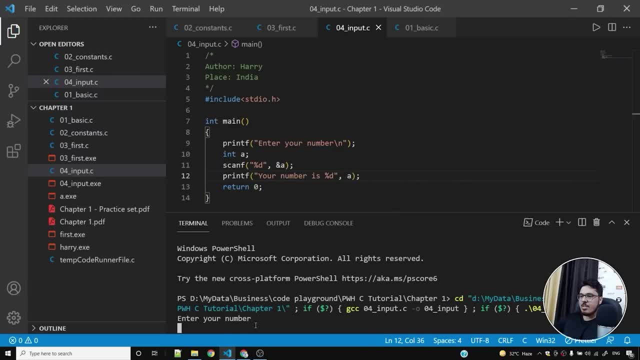 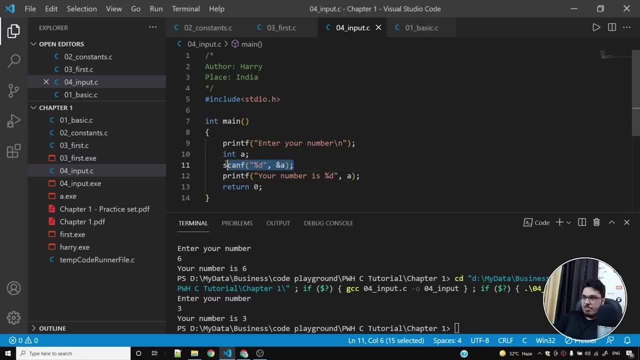 put a semicolon. let me run this program and see what happens. enter your number six. your number is: let's try this program once again and see if it works for variable inputs. yes, it does. your number is three. how is this thing working? so scanf is basically a function, it's a library function. 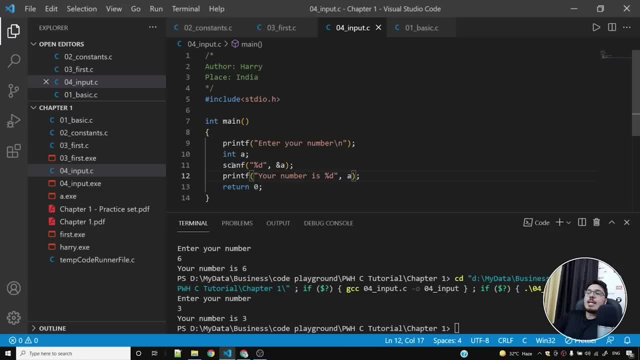 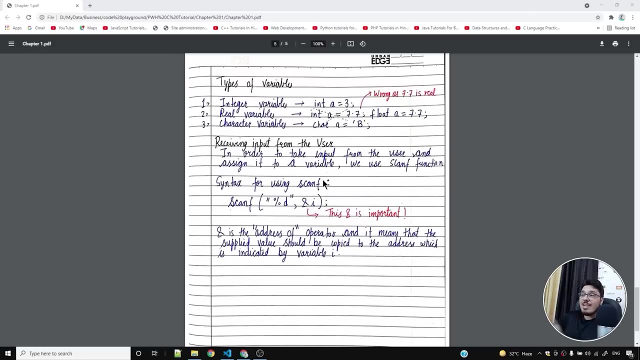 and you can use scanf to take input from the user. so what you are doing is you are saying to the compiler that i am going to enter an integer from the keyboard. kindly store that integer at this location. simply look at the syntax and you are good to go. so if you look at the syntax, scanf, %d and the memory location where, 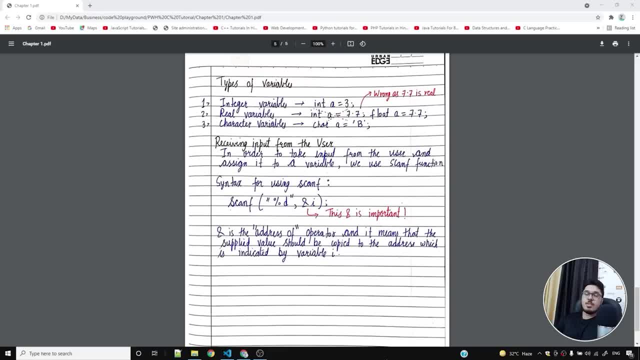 you want to put that number which you are going to enter. this is all you need to know about scanf at this point in the course. i'm going to explain you more about scanf and functions in the future, but let's look at this amp% operator. this is very important. i've even written this. 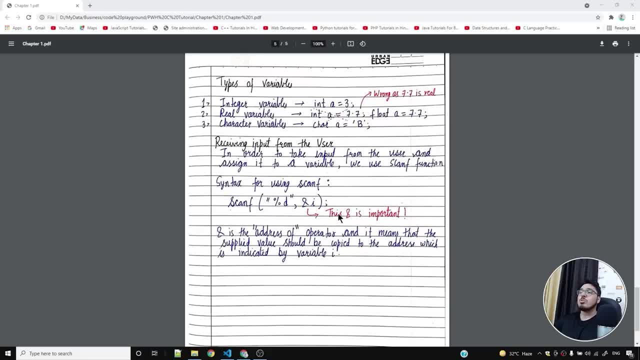 red color in the nodes. this amp% is important. amp% is the address of operator and it means that the supplied value should be copied to the address which is indicated by variable i. so when i say amp% i, i'm saying the memory location of i in the 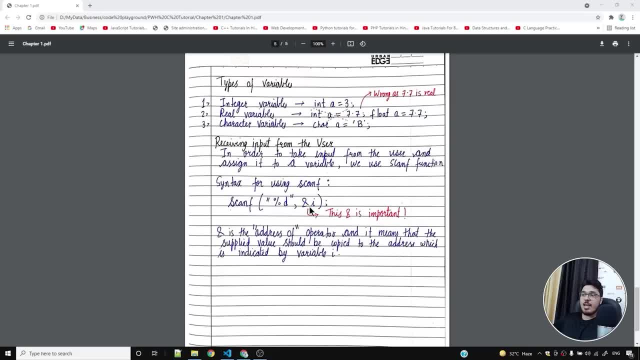 memory. the location of i in the memory is amp% i, and what is i is the value at that memory location. i don't want to know which location, i just want to know the value. let us say i'm talking about you, i named sham. if i say sham is a good boy, i'm commenting on sham. if i say amp% sham is a good, 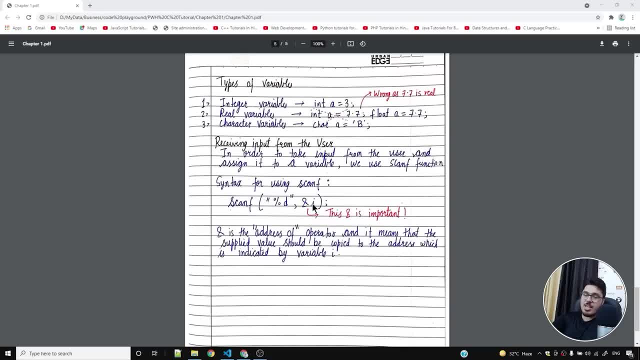 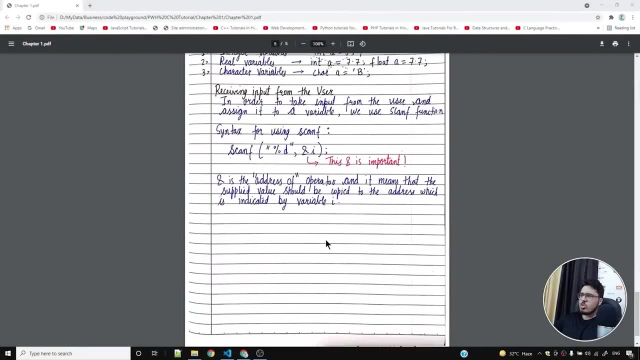 place. i'm simply saying the place where sham resides is very good. i'm not commenting on sham. sham can be a good boy or sham can be a bad guy as well. i'm not commenting on it. i'm simply commenting on the place where sham is living. i hope this address of operator is clear to you. so that was. 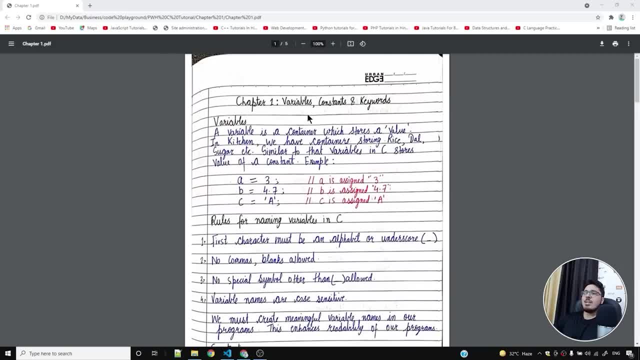 about chapter number one. i hope you liked chapter number one and you enjoyed the concept of variable constants and keywords, but this is not it. we are going to practice chapter number one and the concepts in chapter number one using a practice set. we are going to move to chapter one. 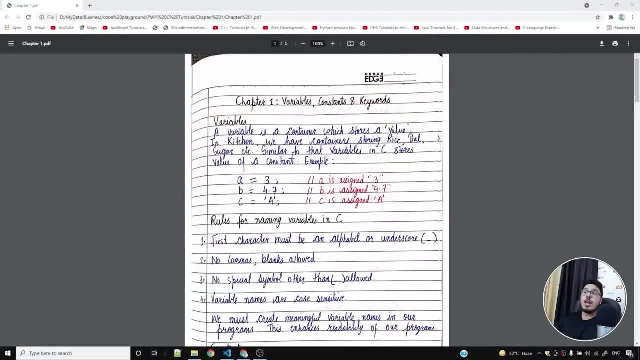 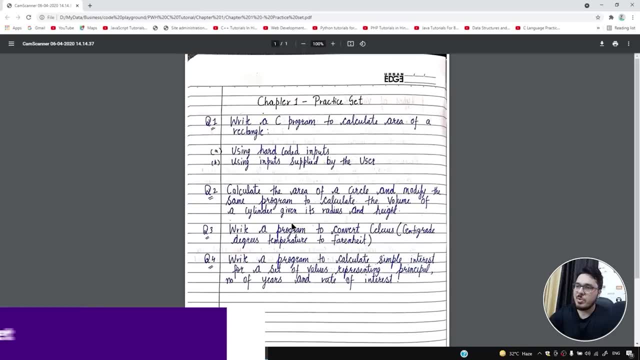 practice set where we are going to solve few questions. so let's move on to chapter one practice set and solve some problems. now that we have learned so much about c, we are going to look into this practice set so that we can practice the concepts that we have learned so far. so the 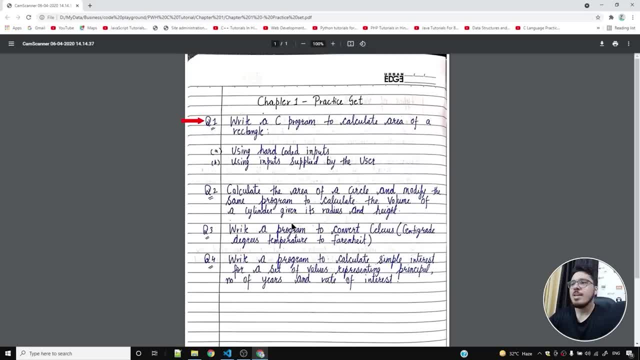 question number one says: write a c program to calculate area of a rectangle, and it is going to be very simple because we are going to use hard-coded inputs. also, we'll use scanner function to supply input from the user end. let's start coding this problem. so what i'm going to do now. 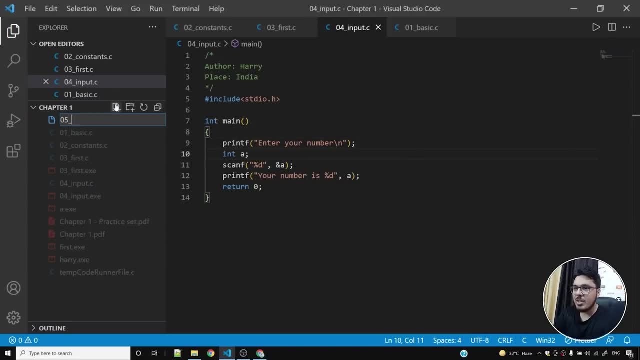 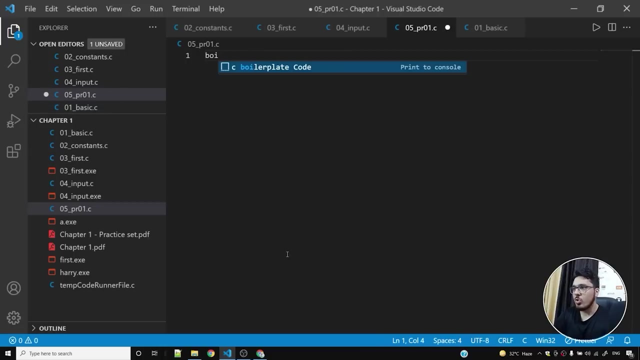 is: i'm simply going to create a new file, which is program number five, and i'll simply say pr01.c, which basically means that i am going to, i'm going to write the first problem solution of my practice set. so what i'll show you is: 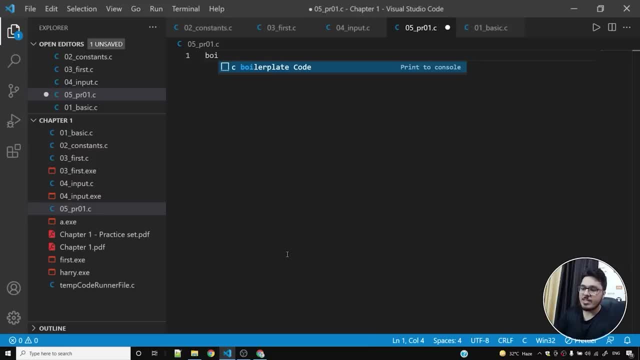 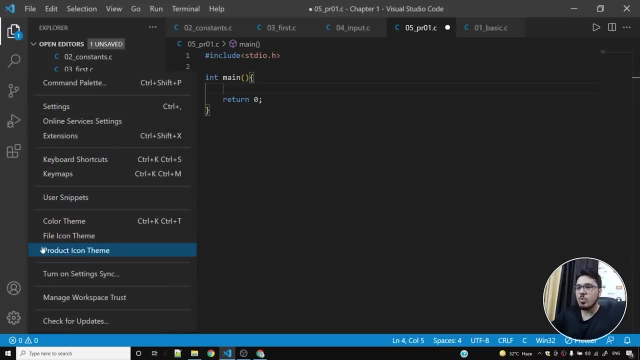 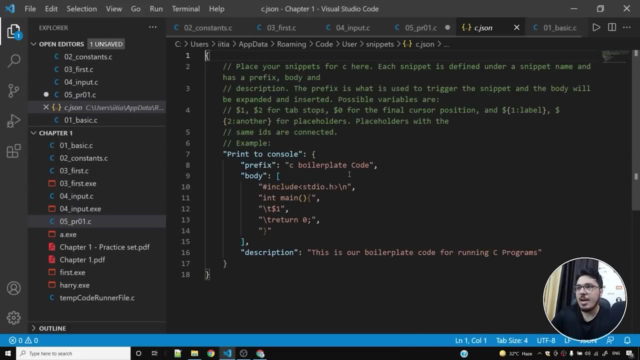 the moment i see boilerplate code, so i simply said boi and press enter. you'll see that something happened. how did i do this? i want to show you. so if you click on your settings in visual studio code and you go to snippets- user snippets- and you go to cjson, you can add something like this: 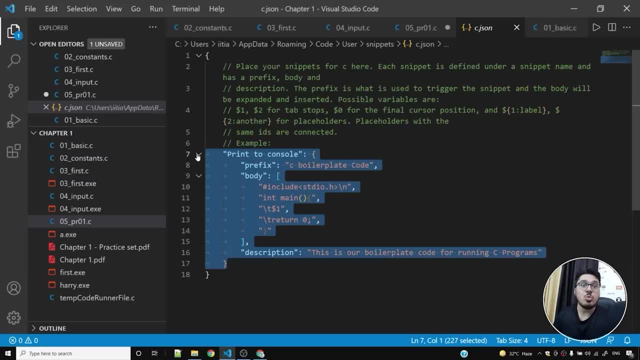 and this will basically be the shortcut to type a very long boilerplate code repeatedly. let me show you what i'm doing. so what i'm doing is i'm adding to this json a key value pair, which is an object. so if you don't know what json is, simply copy this. you can look into this stuff and directly. 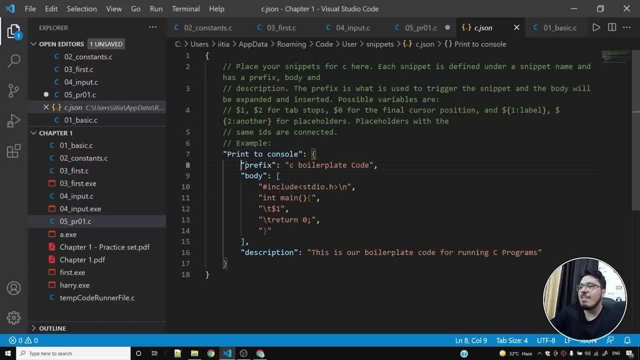 make your cjson look something like this. so we have a prefix, we have a body, we have a description. prefix is something you will use whenever you want this body to be added to your program. make sure that you use backslash n for new lines and also backslash t for tabs. if you look into my 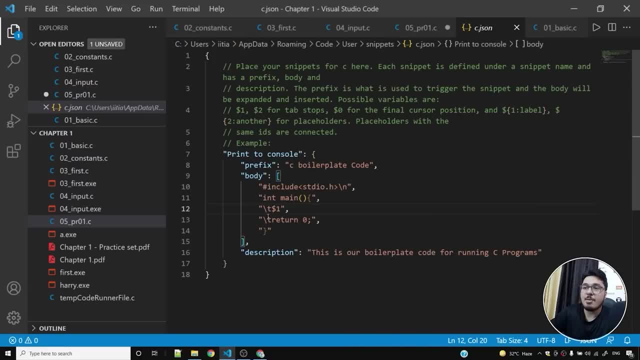 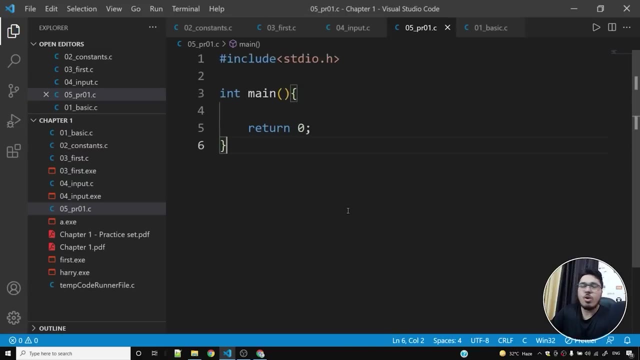 you can see that i have a tab here, a tab here just because i had backslash t here. so make sure that you type this and then you can add description of your choice and we can have as many snippets as we want in this particular cjson. if you're not able to add snippet for any reason, maybe you are. 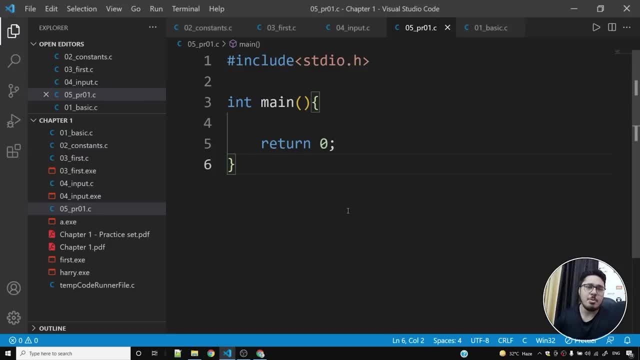 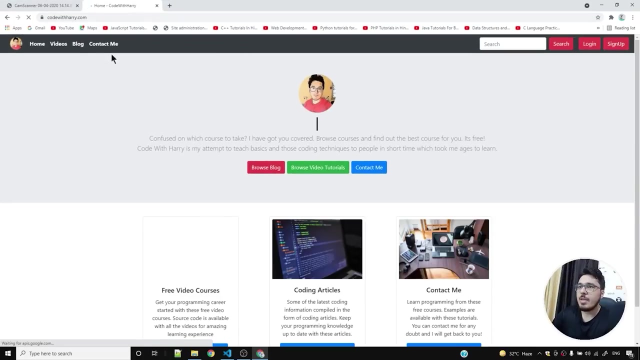 in some different source code editor or something. do not bother about that, because you know what. you will simply have to type these many lines. that's about it. you don't have to worry, and if you have the cheat sheet, that i've lied to you. so let me show you the cheat sheet. i'll simply go to my website and the blog and 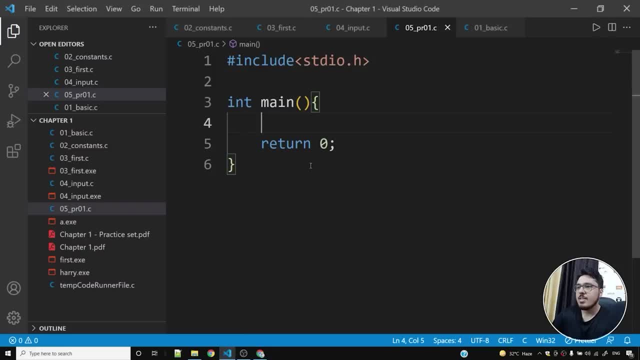 we'll open the c language cheat sheet. you simply copy this and you can paste it in, and that's about it. you have this boilerplate code, okay, so you can add your code here, and you know what. you can simply either use the boilerplate or use the cheat sheet. it doesn't matter, you should know how to use. 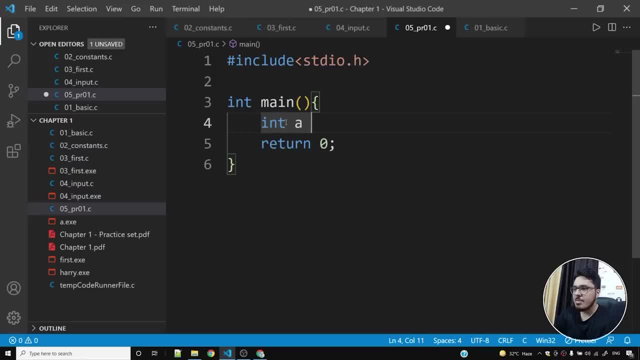 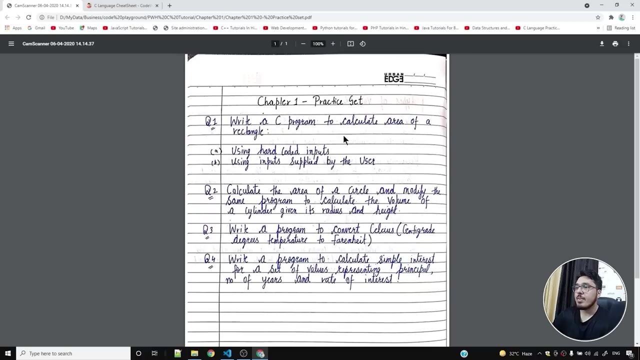 both of these things. let's come back to the problem. i'll simply say int a is equal to 4 and i'll say int b is equal to 7. what is a and b? a and b is nothing but the height and width of of my rectangle, so i have to simply calculate area of the rectangle. 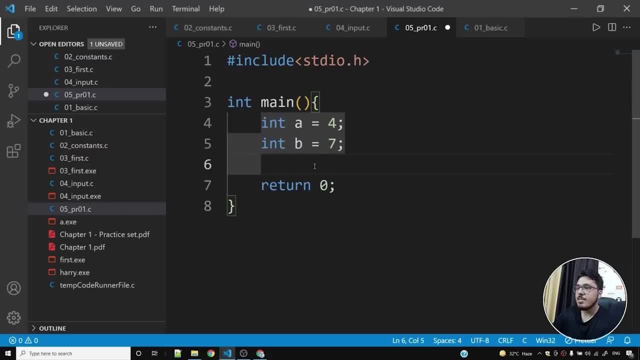 so using hardcoded input. so what is the area of rectangle? i'll simply use printf. i'll say the area of rectangle is. i'll simply multiply a by b and say percentage d and i'll perform a calculation. i'll say a star b and that should do. that should do the trick. so percentage d is, for integer, my. 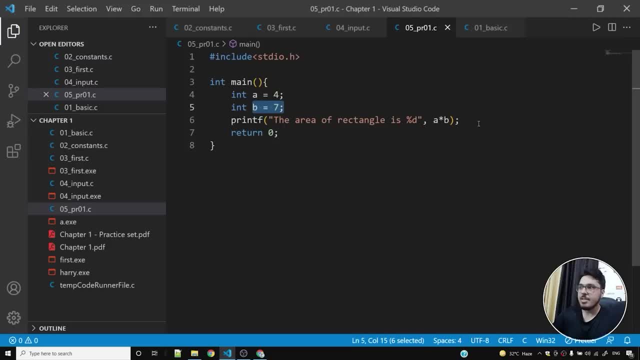 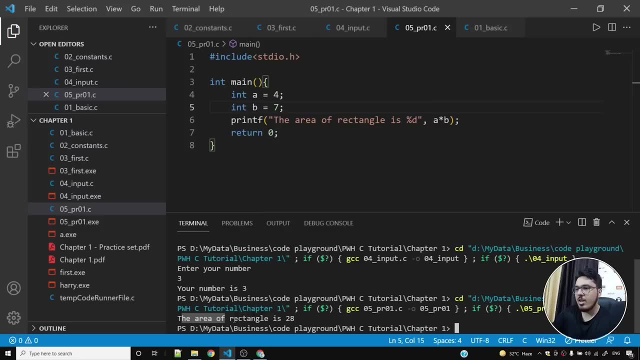 a is an integer, b is an integer is the width, b is the height and a multiplied by b will give me the area of the rectangle. let me run this program for you and show you that the area of the rectangle is 28, because seven multiplied by four is 28, and this program works. what if i want to use this? 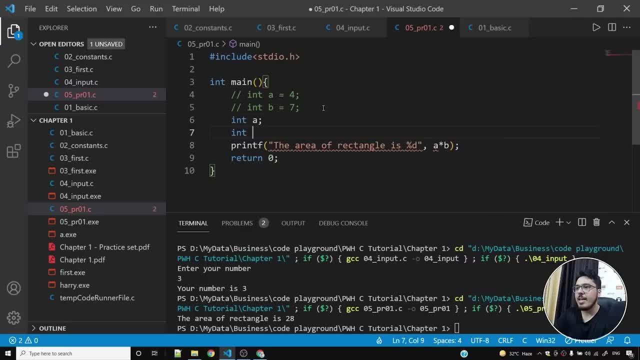 the user supplied input. In that case, I'll simply declare A and B and then I'll simply say scanf %d and I'll want my user to enter A and I'll do the same for B. But before I make my user enter something, I'll simply put a message for him. I'll say: enter the. 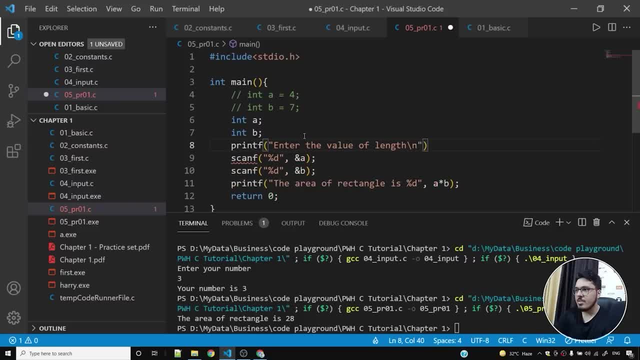 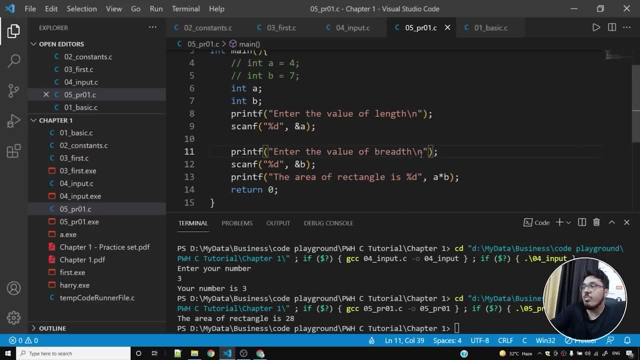 value of length backslash n, and then I'll say: enter the value of breadth, bth. and if I enter the value of the breadth it'll be stored in B because I've written B here. Let's run this program and the value of length, 8, and the value of breadth, let me say 3, and 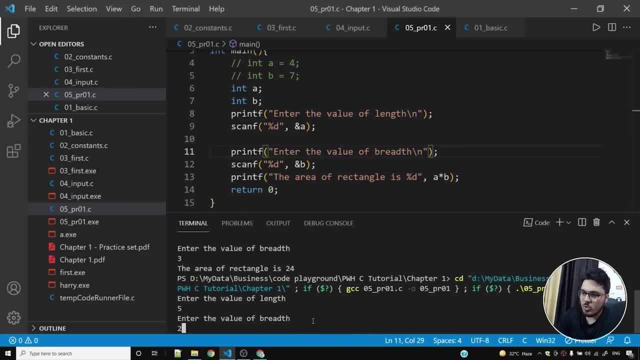 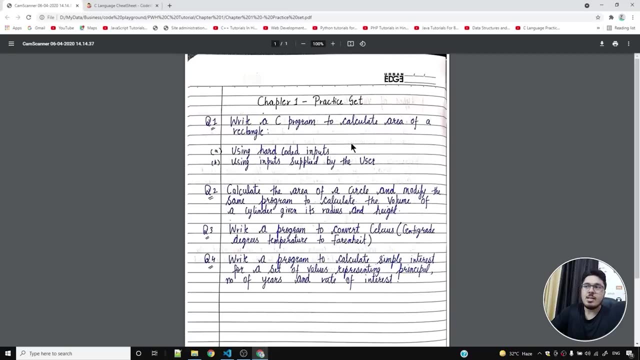 you can see 24.. What if I go for 5 and 2, it should be 10 and yes, it is. So the area of the rectangle been calculated using the hard-coded inputs and using the inputs applied by the user. now what we? 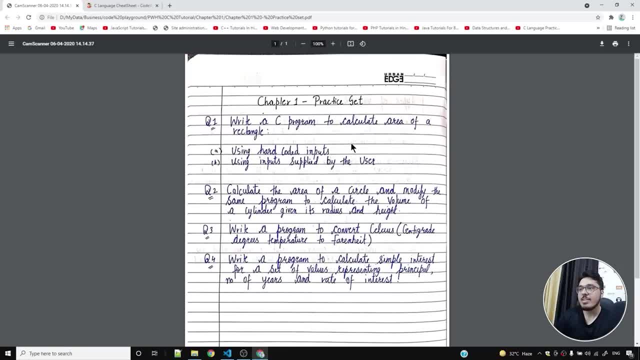 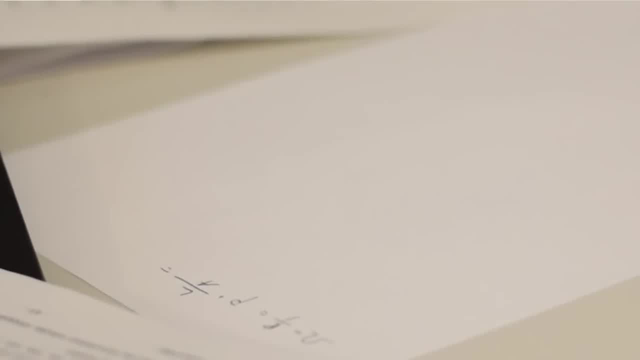 are going to do is we are going to calculate the area of a circle and modify the same program to calculate the volume of a cylinder, given its radius and height. now, if you don't know mensuration or you are not into a lot of mathematics, bear with me, i'm going to explain everything to you. so this 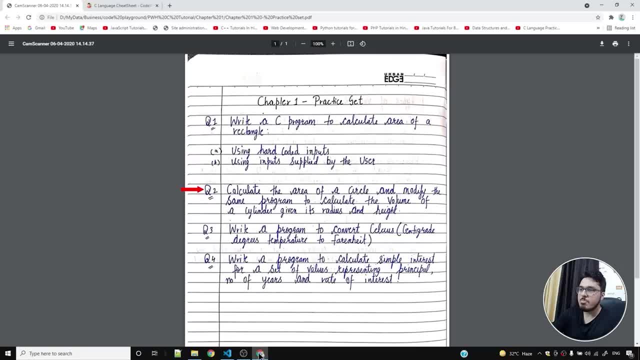 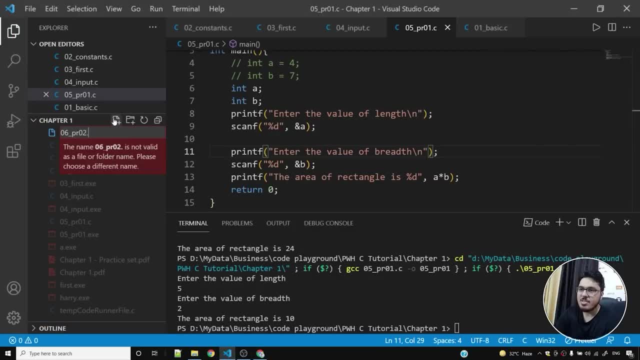 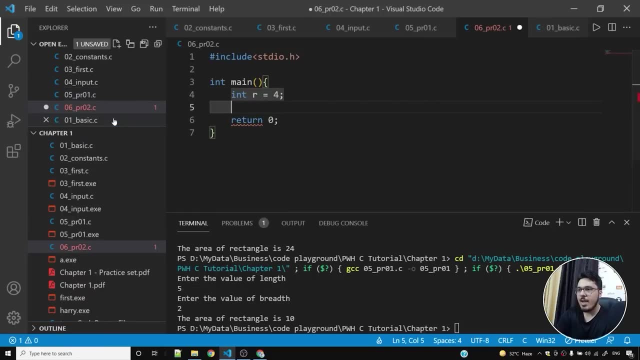 question says: calculate the area of a circle which is pi r square. so let's prepare for calculating the area of a circle in a program called 06 underscore, pr02, dot c. let me add the boilerplate code and i'll say: int r is equal to 4. and now what i'll do is i'll say printf: the area of circle. 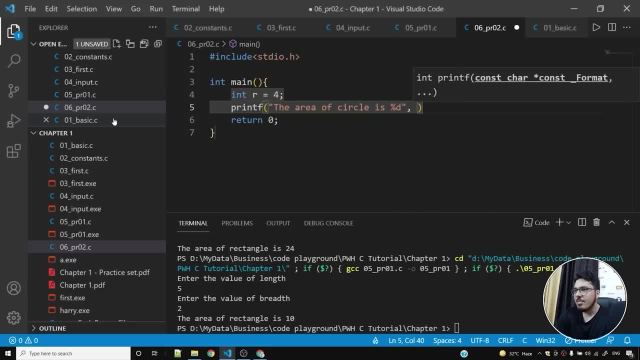 is percentage d, and what i'll do is i'll put down the value of pi and then i'll say, please say r, and then, once again, i'll say r. so pi multiplied by r, multiplied by r, is the area of the circle pi r square. let's run this program. 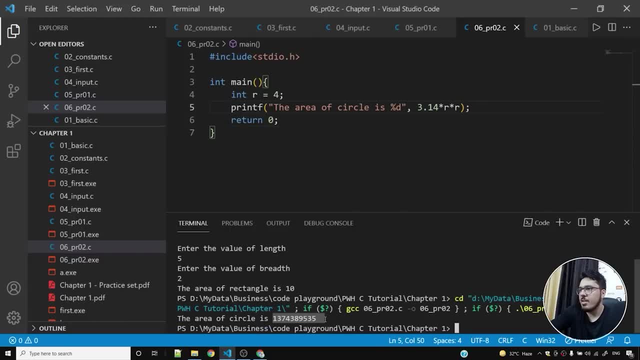 and see the area of the circle is this thing which is a bit problematic, because i have used percentage d. i should have used percentage f, because this is going to evaluate to a floating point number. so this is something that you need to remember. now, if i run, you'll see 50.24, 4 multiplied by 4. 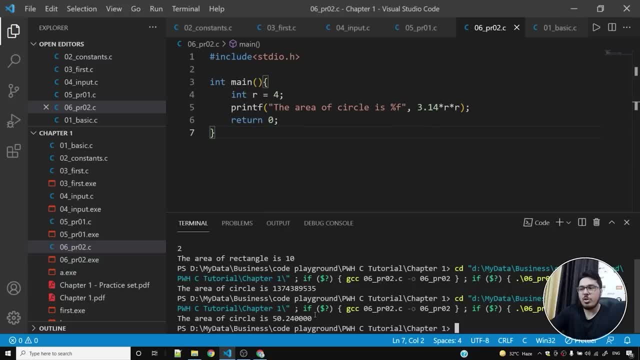 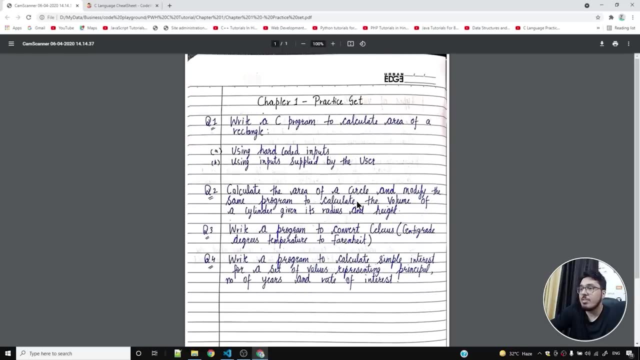 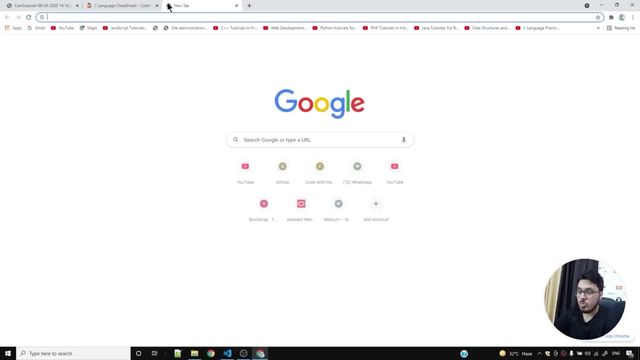 3.14 will be approximately around 50.24, which makes sense. okay, i hope you understood this. now i have to modify the same program to calculate the volume of a cylinder, which is pi r square multiplied by h, where h is the height of the cylinder. let me show you these formulas: area: 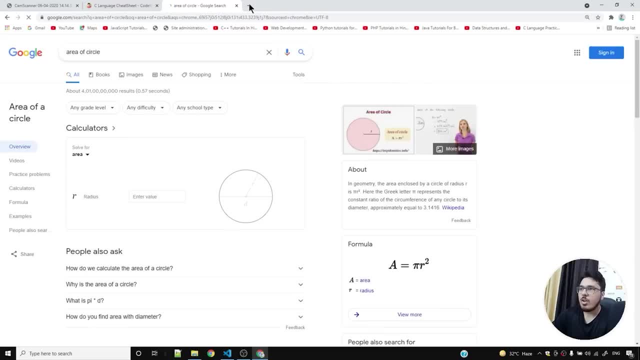 of circle and also i want to show you volume of a cylinder. so area of the circle is pi? r square. i'll enter the value of r and it'll show me the area. so when the area is 4- sorry, the radius is 4- the area is around 50.26. they are using 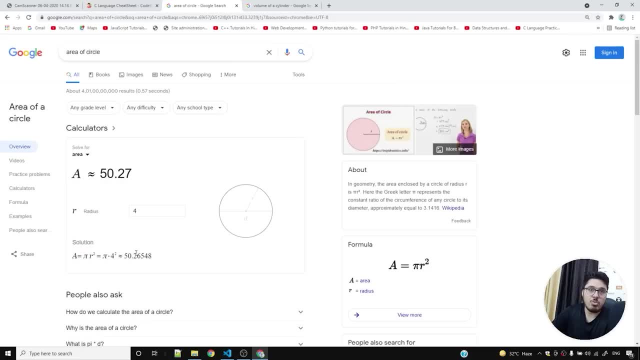 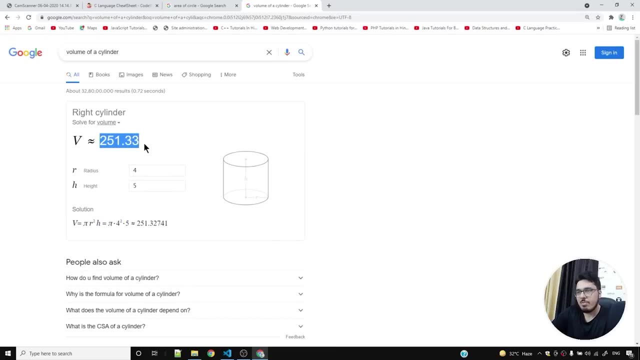 the exact value of pi. i'm using 3.14, which is approximate, so maybe there are some differences now. similarly, if i enter 4 and 5, the value is 251. let's see if we are able to achieve that. and let me area the volume of the cylinder. 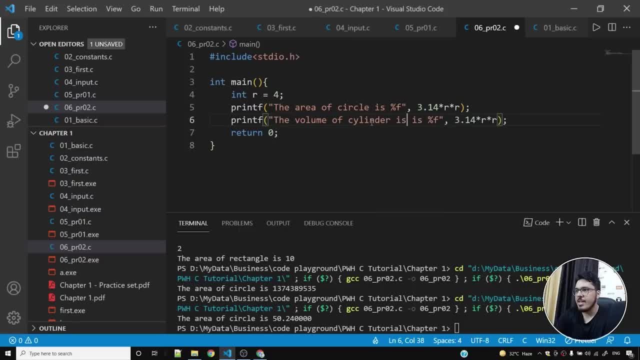 volume of cylinder is, and let me say int h is equal to 5, and i will say: multiply by h, 4 and 5, 4 and 5, let's see what we get. we got 251.2 and, yes, we got something very close. once again, i'm using an approximate. 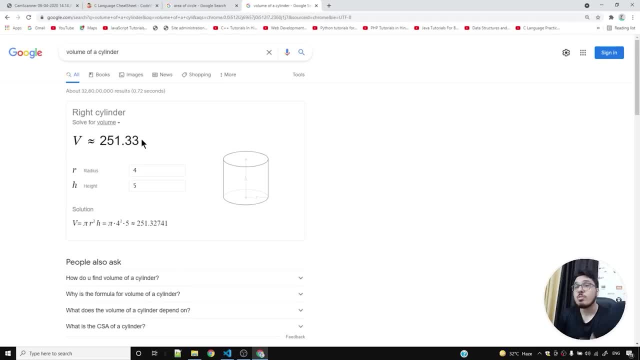 value of pi. 2 point sorry. 3.14 is an approximate value of pi, so make sure you understand that pi you are using might be a bit different from what is being used in the online formulas, because of which our results are going to be a bit different. so they got 251.33 and i got 251.2. 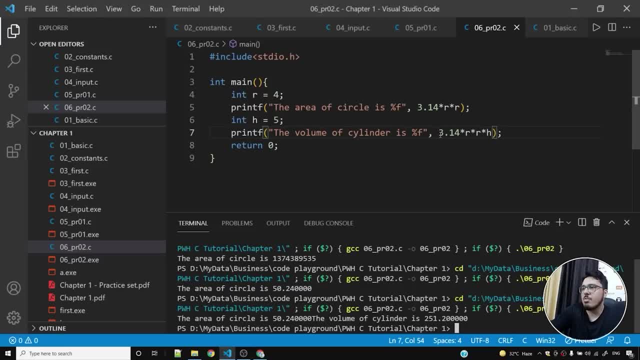 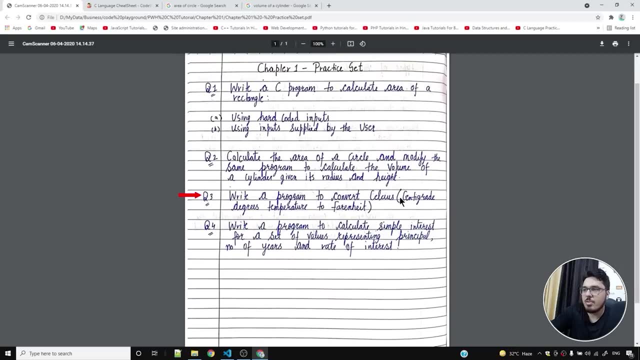 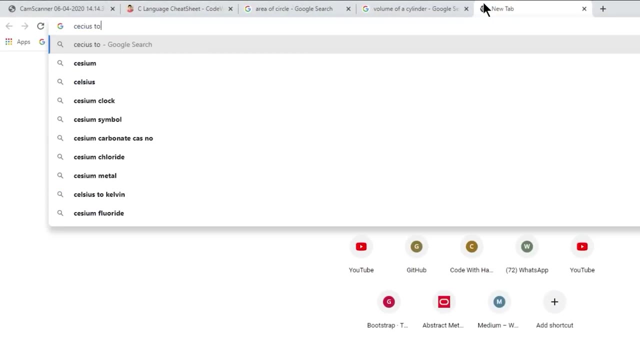 which is pretty close, but again not exact, just because of the value of pi. but congratulations, we have solved this problem. moving on to the next question, write a program to convert celsius degrees temperature to fahrenheit. so what i'll do is i'll say celsius to fahrenheit, and here is the formula: 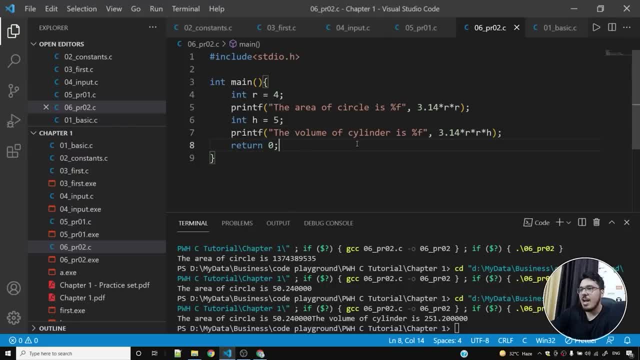 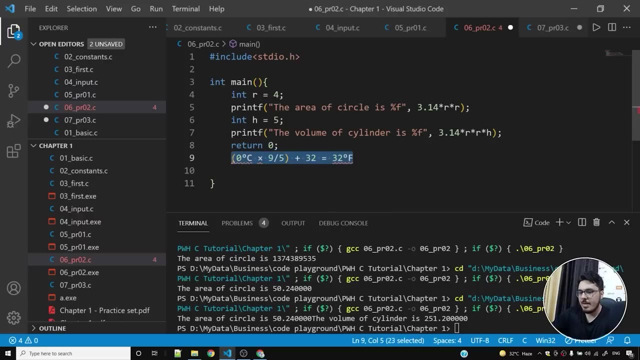 i'm going to copy this formula as is, and before that, what i'm going to do is i'm going to write a new program, name 07, underscore pr03, and this is a c program, so i'll say boilerplate code. i'll simply cut this. 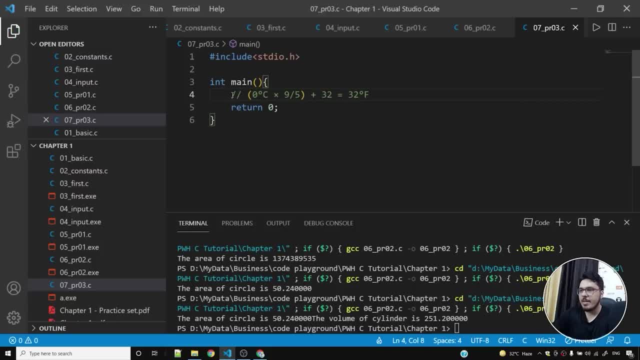 and i'll simply write a comment here. i'll simply refer to this formula. i'm not going to use it exactly. i'll say nc is equal to 5 and i'll use printf and i'll say: the value of temperature in fahrenheit is percentage f. and i'm going to use this formula, but it will be easy for me. 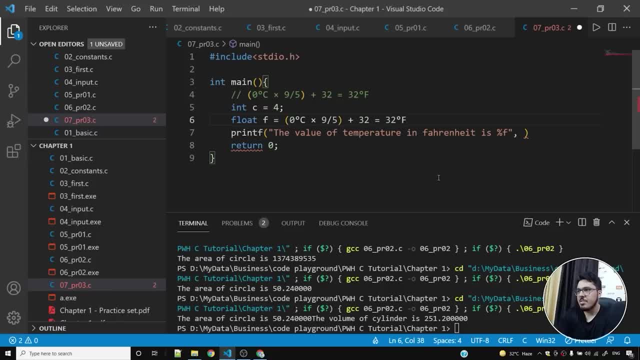 to do it. so i i'll just let me use this formula: um, let me going to tonin cuenta beca, to fantasy, because let's see if i use something like this, let me paste this formula, let me fix this formula and replace x with star, because in c, star is the multiplication operator. 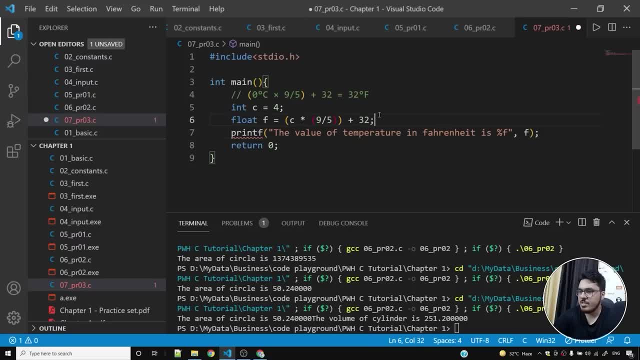 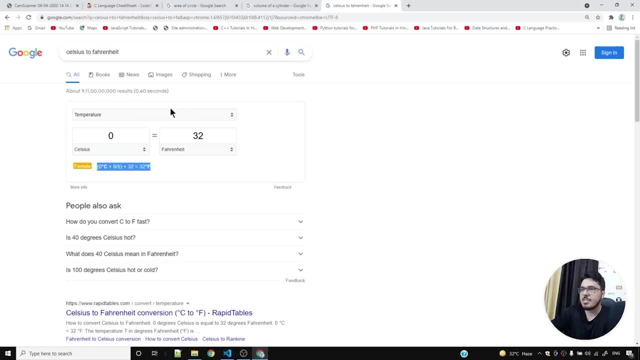 not, not x. okay, so i'll simply say c, this expression, and this should do the trick. So if I say C is equal to four, I should get 36.. Let me punch in four, I got 39.. Looks like there is some problem with my formula. 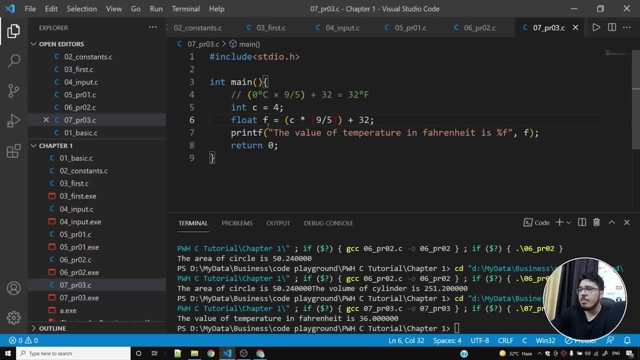 So let me see what the problem with my formula is. I think I've replaced the value of C wrongly, So this should be C multiplied by nine, by five, and yeah, I got the problem. So the problem is that the value of C is an integer. 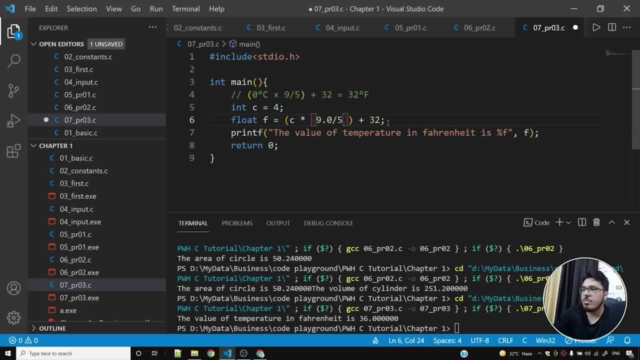 nine is an integer. five is an integer. simply say 9.0 divided by 5.0, and I'm going to explain to you why this is the case, why you need to use 0.0.. So let me run this and we get the correct answer. 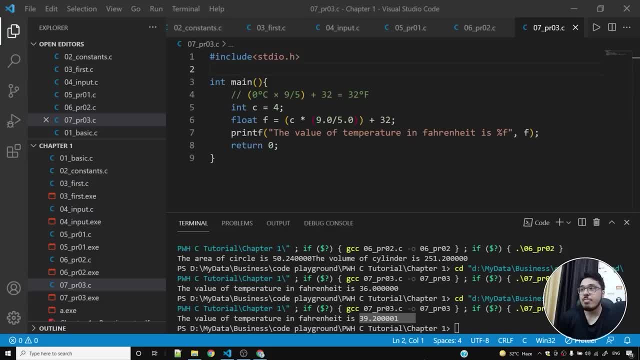 But allow me to quickly answer you this question that why did nine by five not work and why is this 9.0 by 5.0 is working. So whenever there is an operation between integer and integer in C, the resultant is also an integer. 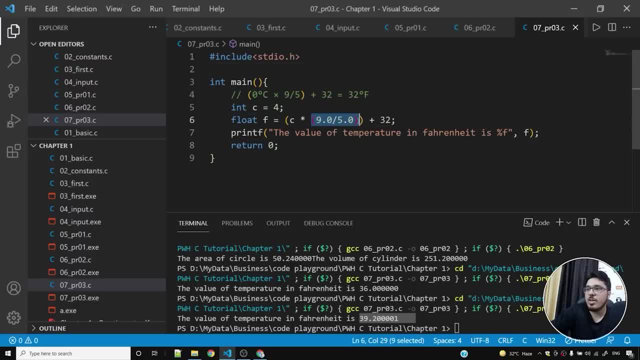 So nine by five will be rounded off to the nearest integer and this will be the value, and then it is multiplied by C and then 32 is added to it, which creates a lot of error. When we say 9.0 by 5.0, we get the exact value in decimal. 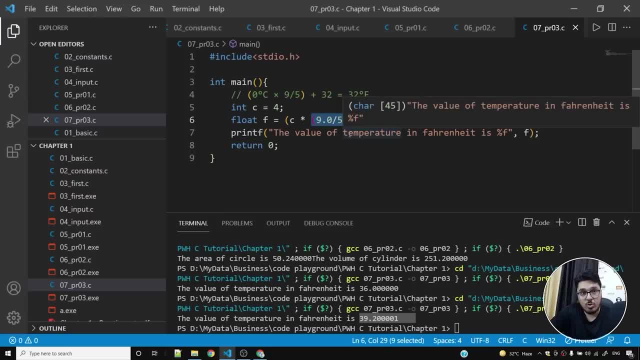 because this is evaluating to a float. Float by float is a float, int by int is an int, So this value will be a float. Multiply by an integer is a float. and then we add: an integer is a float. So this is why we are getting the correct value. 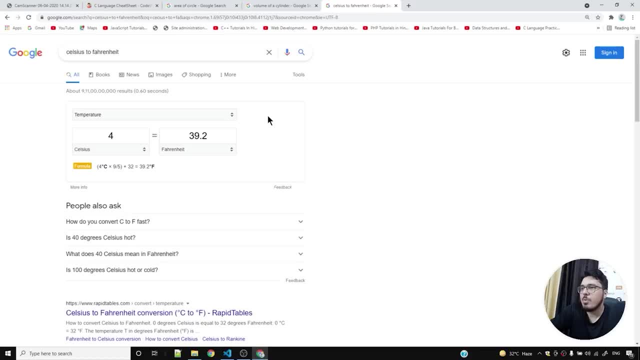 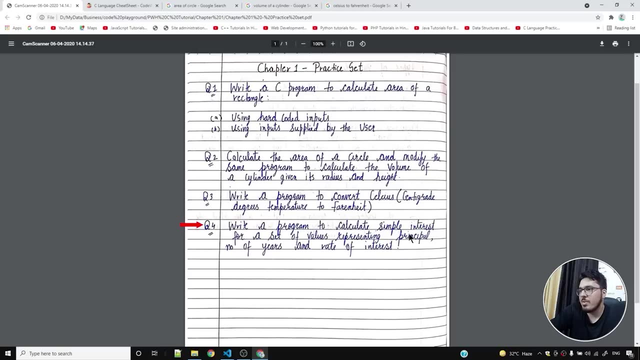 using this formula. I hope you understood it. I hope you got the point. Now coming back to the next question, which is write a program to calculate simple interest for a set of values representing principle number of years and rate of interest. 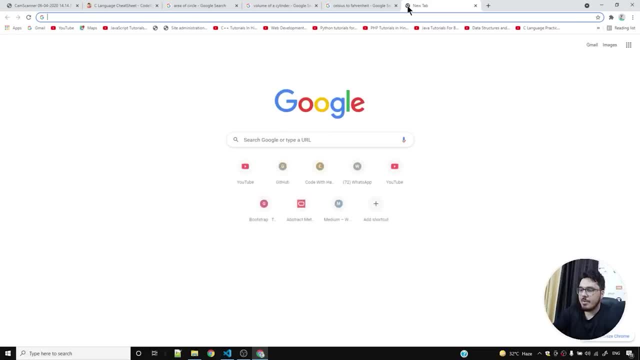 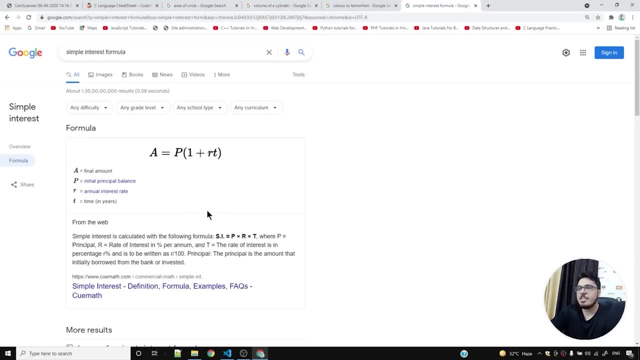 And this is very straightforward. I'll show you something simple, Simple interest formula. And simple interest formula is really very simple. It's PRT divided by 100.. So if you want to calculate the interest, this is PRT by 100.. 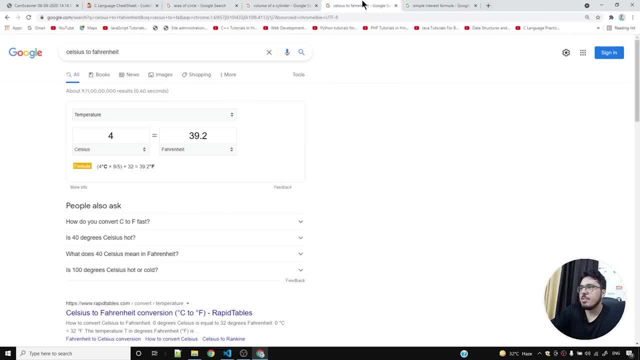 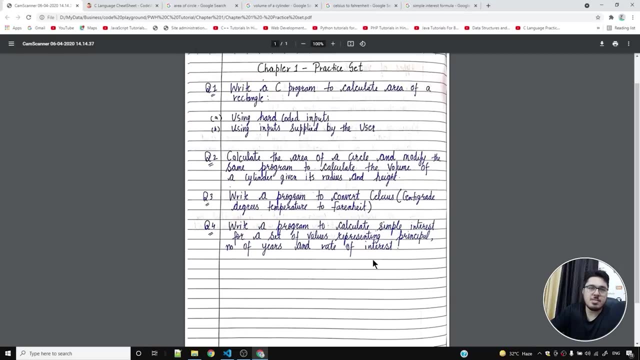 But A is the final amount, So you need to use PRT divided by 100.. So why divided by 100? Because we have the rate of interest in percentage. If the rate of interest is not in percent, then you can simply use the decimal rate. 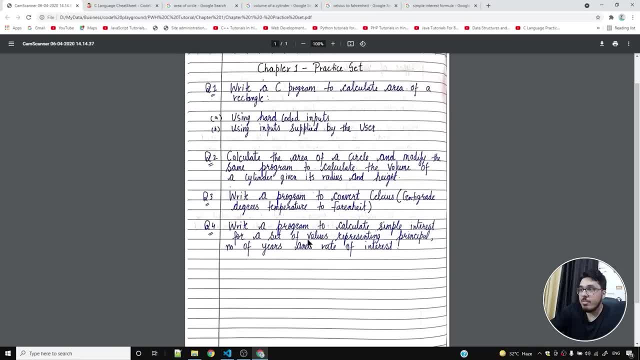 And then you don't need divided by 100. But if you have the rate of interest in percentage, then you need to do divided by 100. So if you have 4% rate of interest, 9% rate of interest, then you definitely will have to do divided by 100. 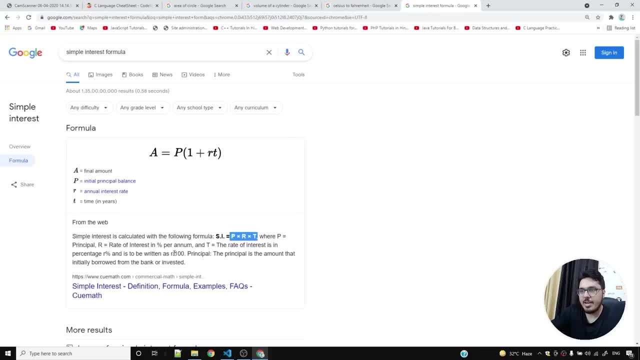 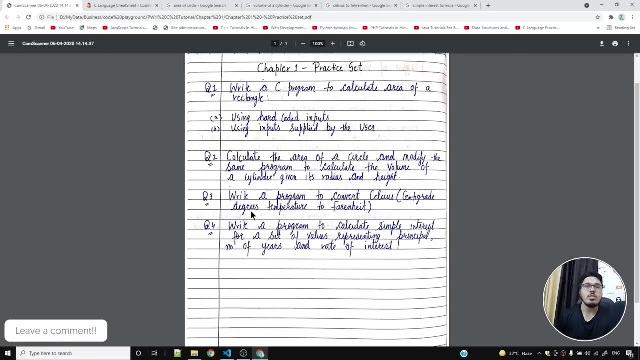 So simply apply this calculation: use PRT divided by 100. And that's about it. You'll get the answer. I want you guys to comment below If you have solved this problem. I want each and every one of you to comment and say that we have solved questions. 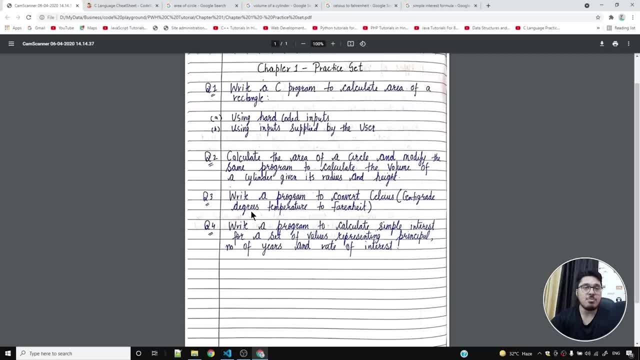 So if you have any questions, please feel free to comment below Question number four. I have solved question number four. Take accountability of yourself and tell me what is the answer for the simple interest, If the value of principle is 100, number of years are four and rate of interest is six. 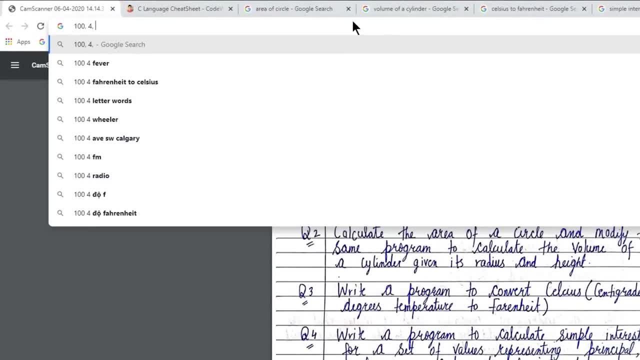 Let me repeat it: 100, 4 and 6.. Rate of interest is 6% for the four years. Principle amount is 100.. How much will be the final amount? How much will be the simple interest? You need to calculate the simple interest. 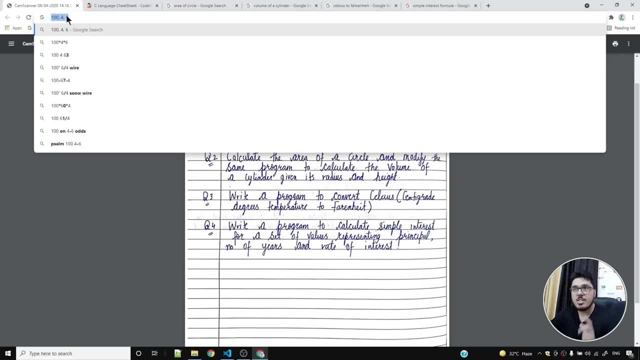 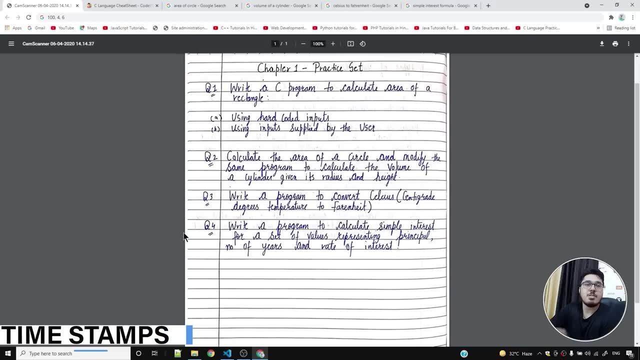 So tell me the simple interest. Tell me what will be the simple interest for these values. I am waiting for your comments. I hope everybody posted the comment and also don't mention to put the timestamp when you are commenting so that I'll know where or which part of the video you are at when you 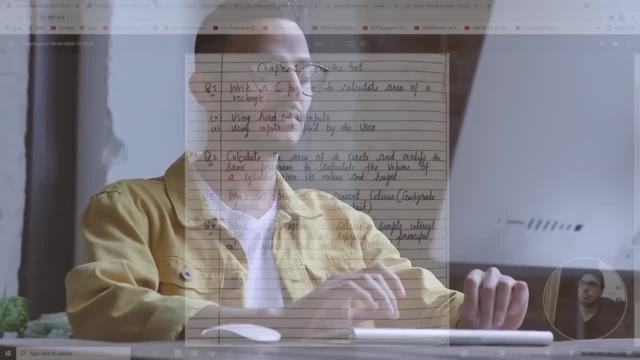 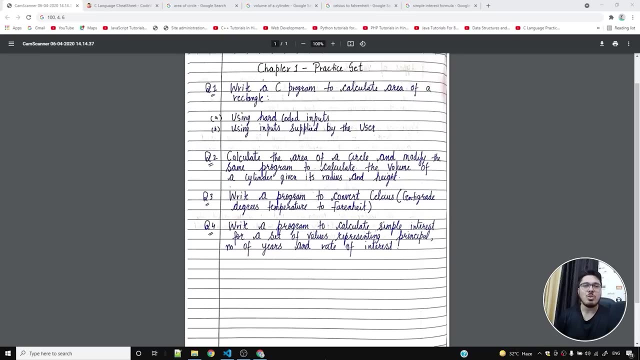 are commenting. I hope you enjoyed practicing all these questions from chapter one: practice set. Now we'll move on to chapter two and we'll explore more concepts of C. Let's move on to chapter two now. So what I'll do now is I'll open this chapter two PDF. 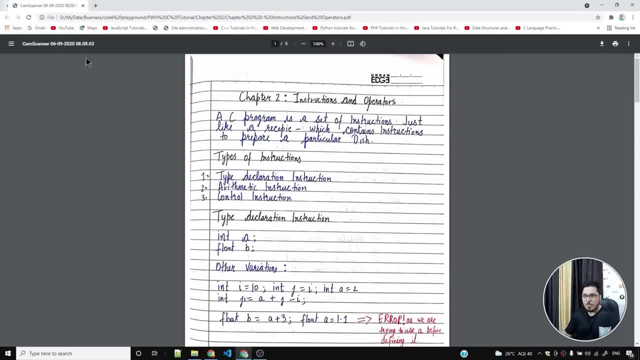 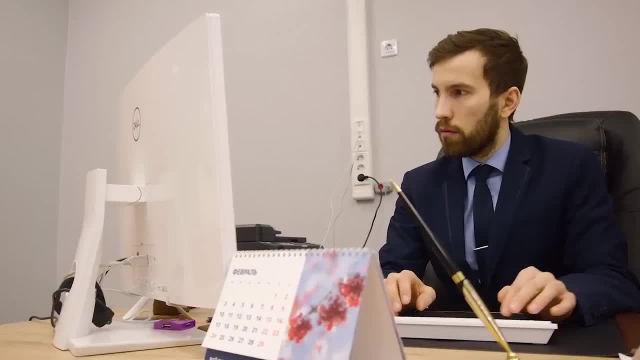 So let me open it in my Chrome browser And in my opinion, Chrome browser is the best PDF viewer- In my opinion, I mean. there are a lot of other PDF viewers- and it doesn't even matter if you have a very powerful computer. 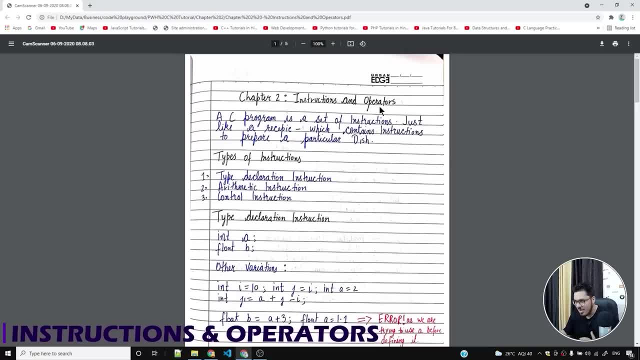 Coming back to the C topic, chapter two, instructions and operators. What are instructions? Instruction is something you tell computer to do, just like you give instruction to your younger brother to bring something, or your dad to bring something from the market while he's in the market. 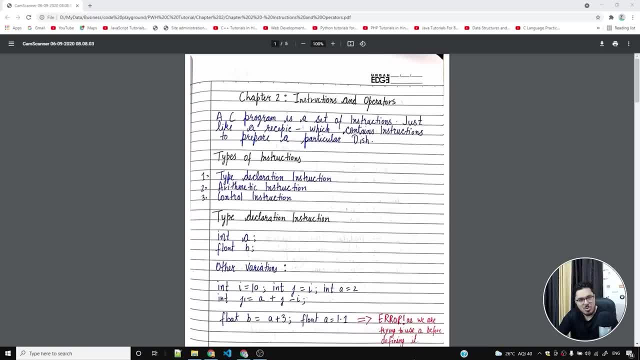 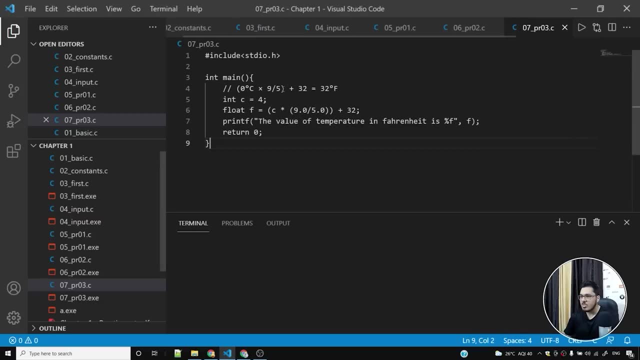 Or whatever your mom might give you instruction to get some groceries. in a very similar way, we use c program to give instructions to the computer. so a c program is a set of instructions, it is a collection of instructions indeed. so if i show you my vs code, you can see that this particular c program 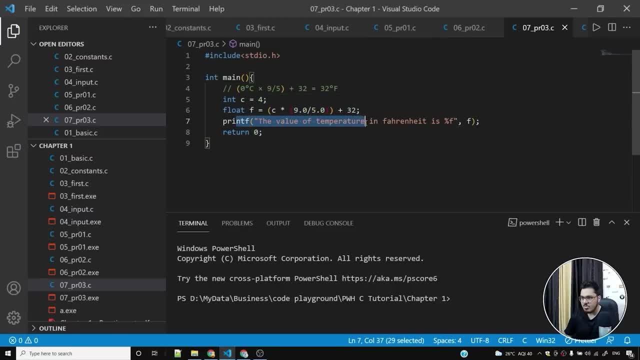 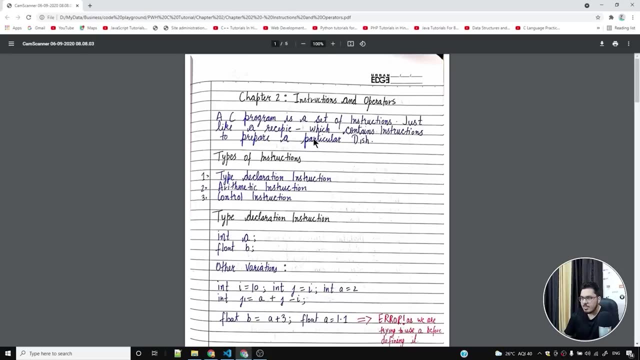 is set of this instruction, this instruction, this instruction and this instruction. so, coming back to the notes, instructions are nothing but instructions are nothing but commands for computer to do something. just like, if you want to prepare a particular dish, you will have certain set of instructions: add salt, add pepper. maybe you will have some instructions of marinating. 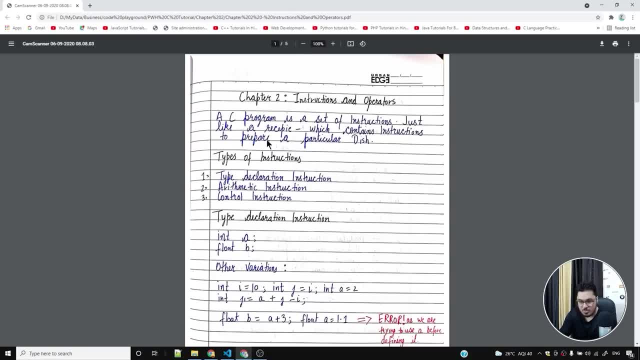 something for some time. these are all instructions for preparing a particular dish. you might want to- uh, you know- cook some vegetable, you might want to cook some oatmeal, and there is a way to get there, basically using some set of instructions. in a very similar way, we write programs and they are. 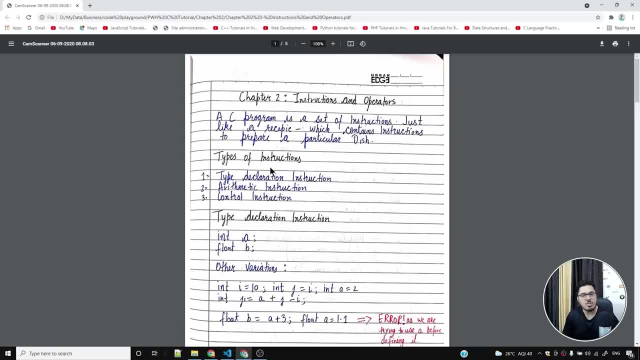 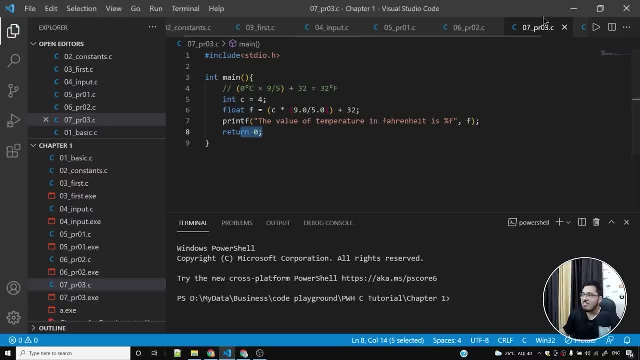 collection of instructions. now let's talk about types of instructions. what are the types of instructions we can give to our computer using c program? so if i show you my vs code, you can see. this particular type of instruction and this particular type of instruction are a bit different. 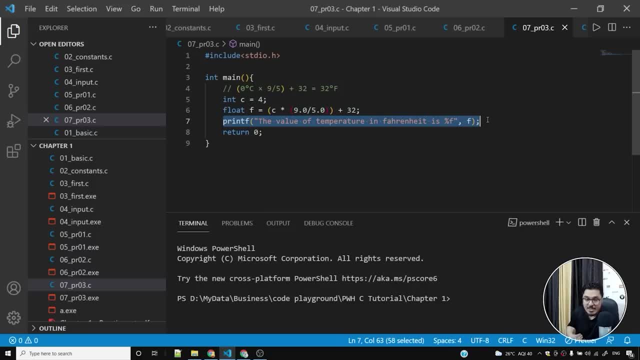 they are not exactly the same. so if i show you my vs code you can see this particular type of instruction. they are not exactly telling the computer to store something in the memory. this particular instruction is saying that store four inside this variable c at some place in computer's. 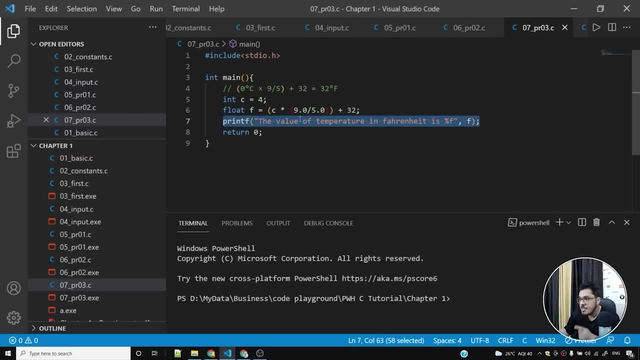 memory. and this particular instruction is saying: print this particular thing in the console, fetch the value of f and format it this way. print it in a way that it looks beautiful, just like this. so this is an instruction and this is an instruction, but these two are different types of instructions. so, coming back to the nodes, there are three types. 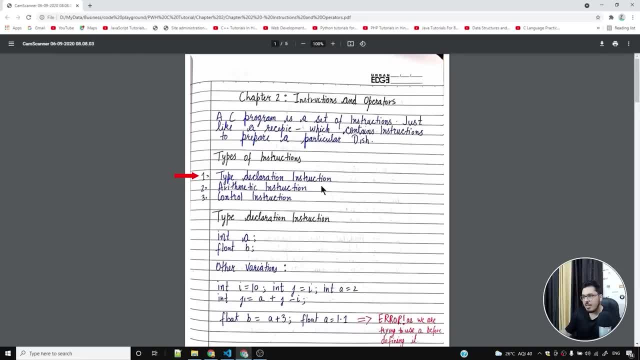 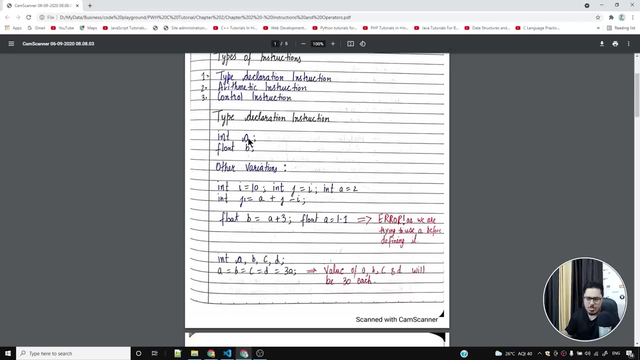 of instructions primarily. first one is type declaration instruction. second one is arithmetic instruction. third one is control instruction. so let's talk about type declaration instruction. remember we talked about int a, float b, char c. we can have even more data types and we can use those data types to declare a variable. so when we say int a, we are basically saying: 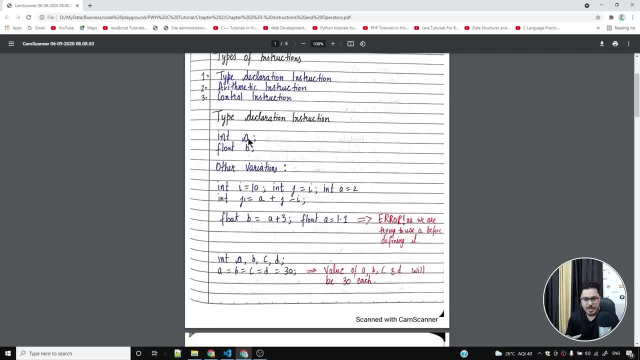 reserve four bytes in memory, which is taken by int. so an integer in c language takes four bytes. what i'm telling my computer is: hey, computer, please reserve four bytes in memory. i want four bytes to be reserved in the memory. so int a means reserve four bytes in the memory. float b means 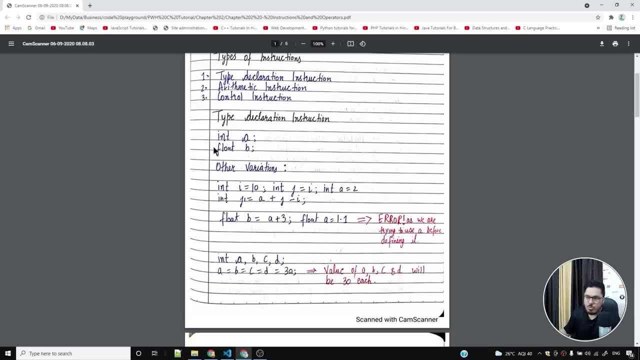 reserve four bytes in the memory for a floating point number. then there are some other variations of this type declaration instruction: int i is equal to 10, j is equal to i, int a is equal to 2. so basically, here i'm saying: give i the value of 10, so 10 is a constant and it will be stored inside i when i say j is equal to i. 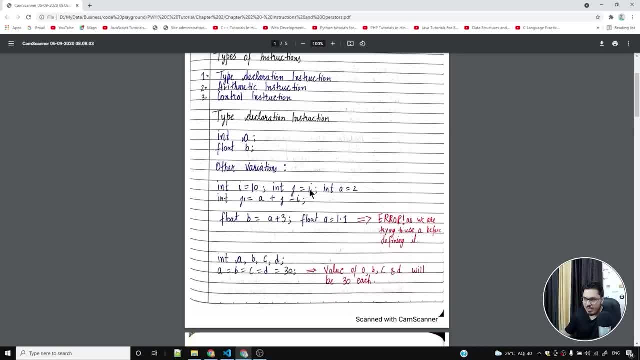 what i'm telling my computer is. i'm saying: fetch the value of i and put it inside j. then when i say int a is equal to 2, i am assigning a bit 2. and in a very similar manner we can have such kinds of variations of type declaration instruction. so let's talk about type declaration instruction. 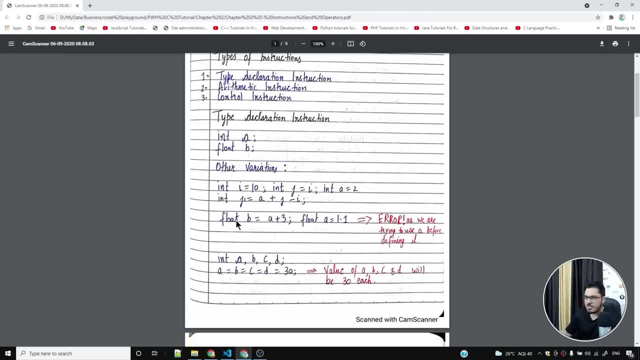 so let's talk about type declaration function. but if i do something like this, float b is equal to a plus 3, float a is equal to 1.1. this is going to throw an error, as we are trying to use a before defining it, so you need to define the thing first. remember, in c language, instructions are executed. 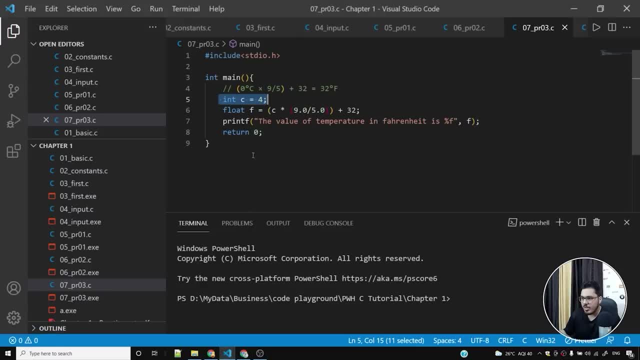 from top to bottom, so they are executed one after the other. so this will be executed first, this instruction will be executed after that, this will be executed after that, and this after that, and so on. so here, if i say int c is equal to 4, i can actually use c. 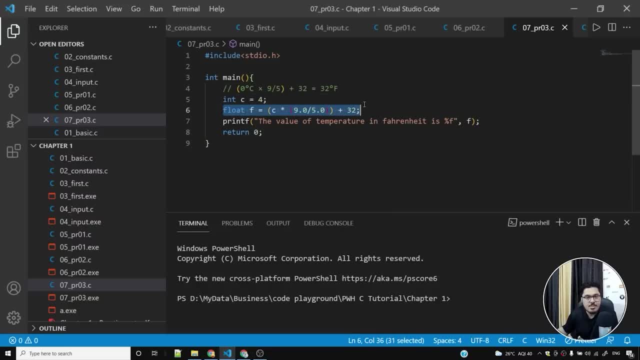 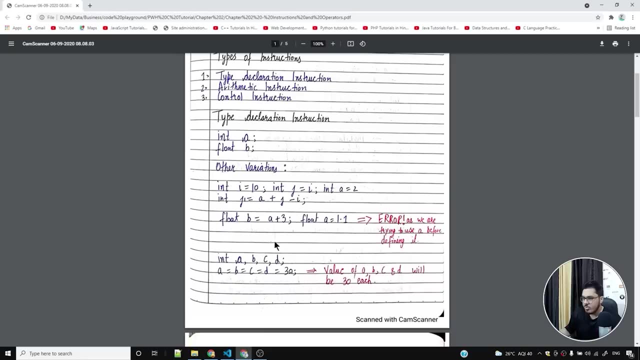 in this particular instruction. but if i try to use c in some instruction and then i define c, that is going to get me into big trouble. okay, so i hope that you understood this. i hope this concept is clear to you now. int abcd is a shortcut to tell. please. 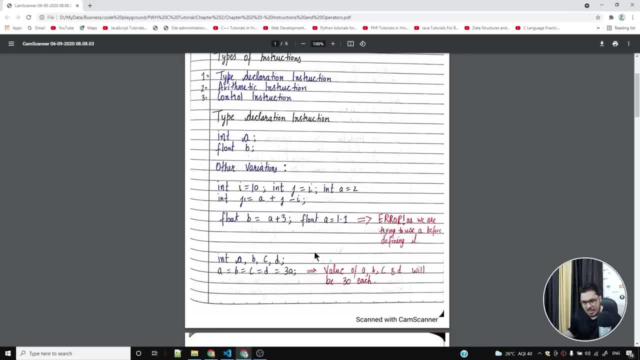 reserve four bytes for a, b, c and d. so this is a shortcut. so in of writing int a, int b, int c, int d in four different lines, we have a shortcut. We are writing all these things at once, int a, b, c, d. And if we say a is equal to b, is equal to c is, 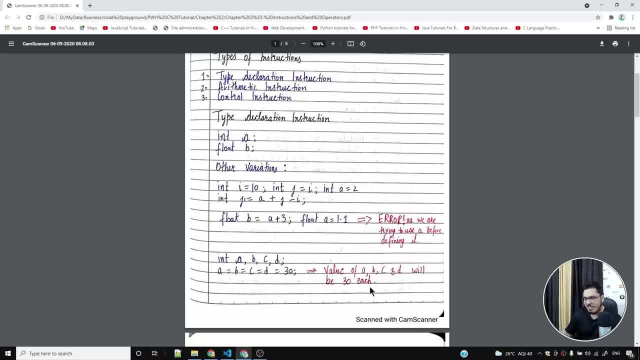 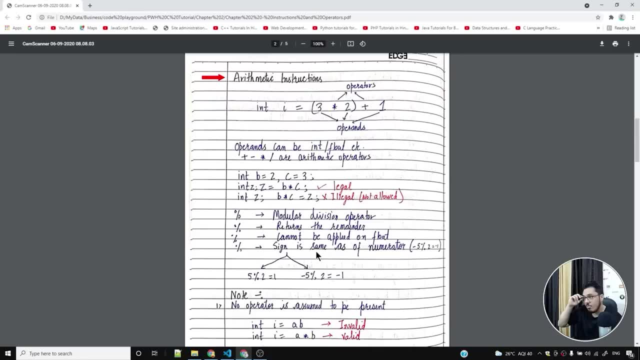 equal to d is equal to 30, value of a, b, c and d will be 30 each. I hope this thing is clear to you. Now let's talk about arithmetic instructions. Int i is equal to 3 multiplied by 2 plus 1.. 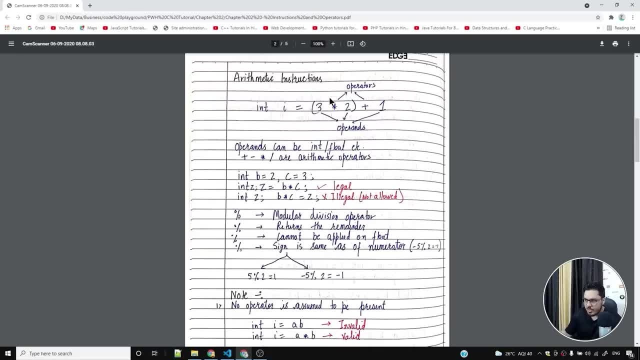 When we do something like this, what we are telling our computer is perform these calculations. We are telling our computer perform 3 multiplied by 2 and then add 1 to it. So basic mathematics. But let's see some terminology. When I say int, i is equal to 3 multiplied by 2 plus 1, here star and 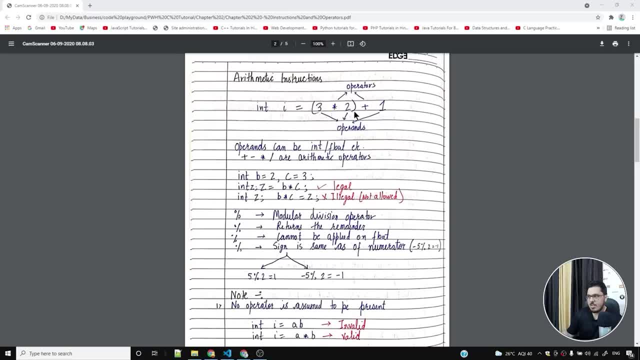 plus are operators and these numbers are operands. So basically we have these operands which are operated upon by the operators. So operator can actually operate on these operands and then produce a result And that result can be stored inside i. So when I say int, i is equal to 3 star, 2 plus 1,. 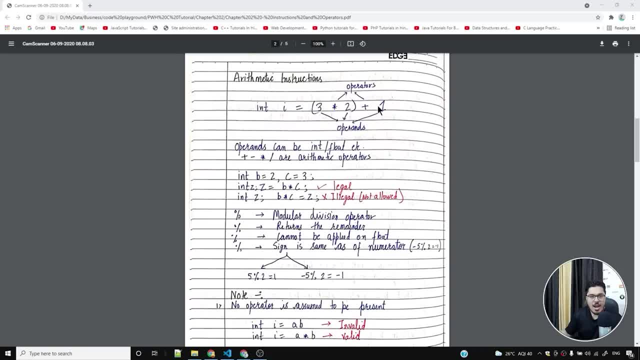 basically, 6 will be the result of 3 star 2.. And when I say 3 star 2 plus 1,, then it will be 6 plus 1, which will be 7.. Operands can be int, float, etc. It can be anything And plus, minus times. 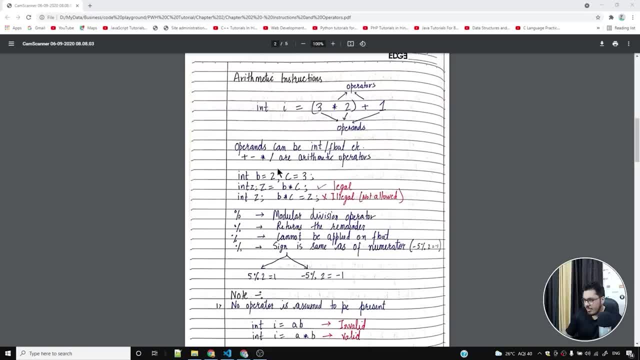 divide are arithmetic operators. Okay, There are some other arithmetic operators as well, but these are the most basic ones. And if we say int b is equal to 2, comma c is equal to 3, it means please assign b with 2 and c with 3.. 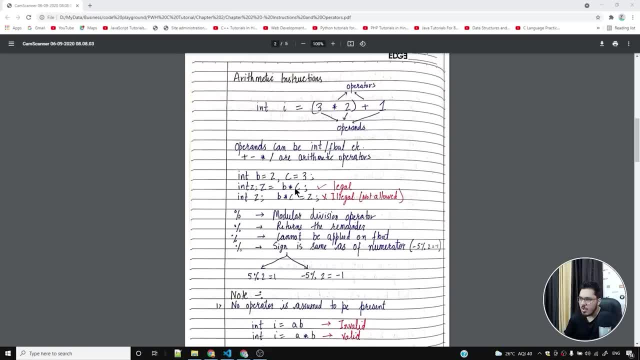 And when I say int z is equal to b multiplied by c, or rather, if I say int z and then after semicolon I say z is equal to b multiplied by c, this is legal. But if I say int z and I say b multiplied by c is equal to z, this is illegal. This is not allowed, Because when 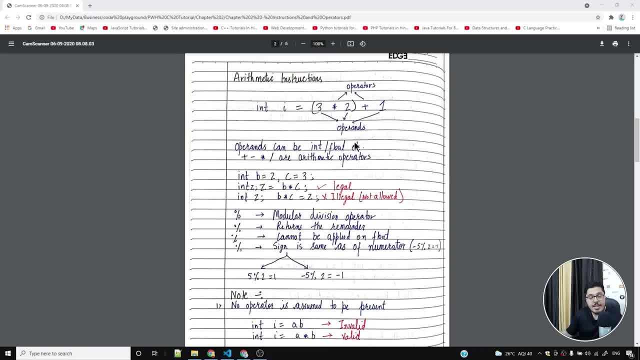 I say z is equal to b multiplied by c, the right-hand side will be evaluated first. In case, when i say b multiplied by c is equal to z, the right hand side doesn't have any value. this is illegal. you cannot do that. so whenever you want to assign something to a variable, 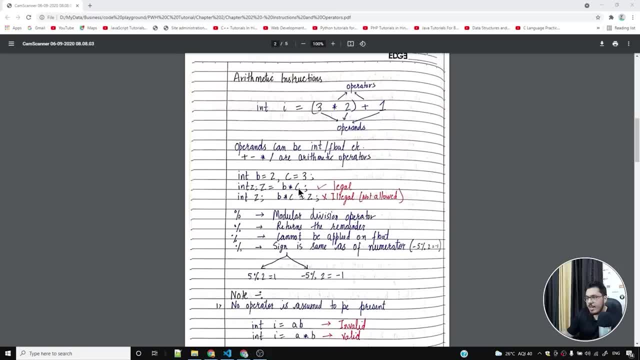 this needs to be clear answer. this should have a clear value. b multiplied by c here has a clear value of two and three, because b is clear, it's the value two, c is value three and b multiplied by c will be value six. so we are all clear on what b is, what c is, and hence we are clear on. 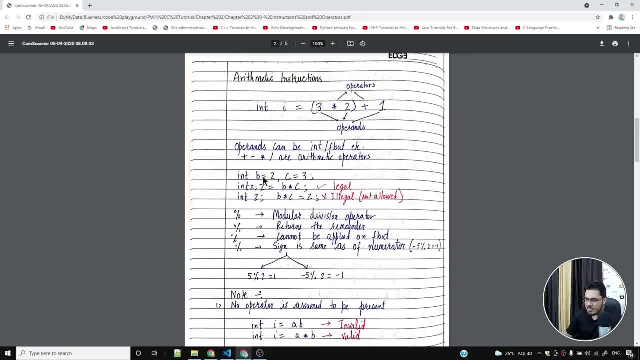 what b multiplied by c is. but had we not had this, b is equal to two, c is equal to three. instead of this, if there was just in b comma c, this would have created an error. so i hope you understood this and we'll practice and we'll see how these things are working so you don't have to worry on. 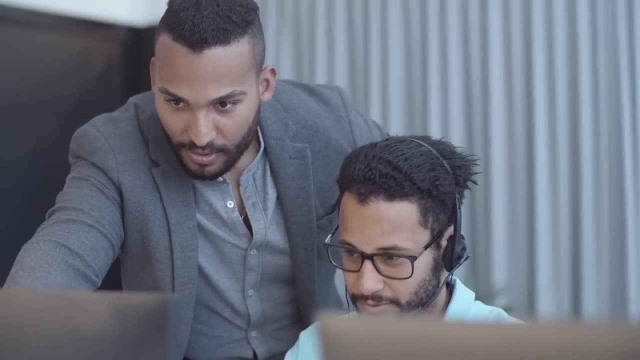 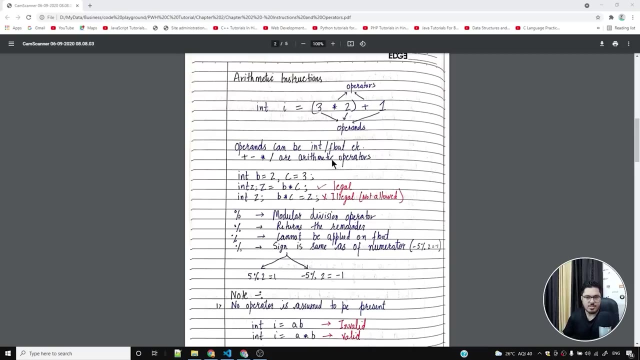 anything, because i'm going to hold your hands and walk you through all these concepts, both in the notes and in code as well. so practical is very important. this is something that i totally understand and we are going to do the practical as well. now. percent is modular division operator. it returns the remainder and it cannot be applied on. 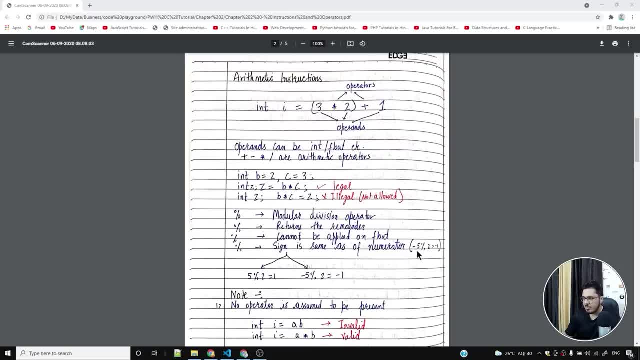 floating point number. percent sine is same as numerator. so basically, when you do something like this, if you say five percent two, what is the remainder? when five is divided by two, it's one, so it returns one. but if i do minus five percent two, i'll get minus one. so sine is same as that of 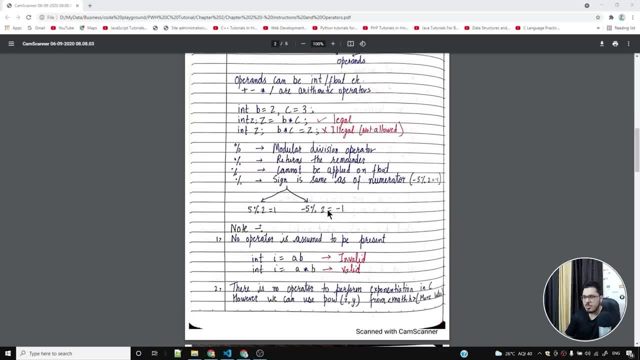 numerator. we rarely use minus five percent two. you know modulo with negative numbers is something that you will very rarely see, but again, if you were to see, this is the rule: if there is minus sign before this five, it will be transferred here. so minus five percent two is equal to minus. 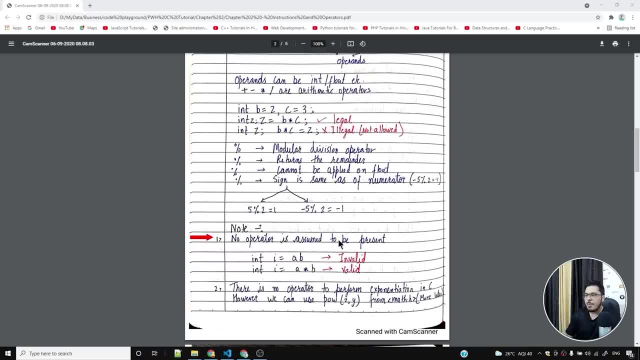 one. now you need to note some things. no operator is assumed to be present. you cannot say i is equal to a, b, just like you do in basic mathematics. and a- b means say multiply by b. no, it doesn't hold true. in c language there is a, no presumption on any operator being present. if you say in time, C is. also because a and b are thumbnails, so there is nothing, for a and b is not a gagnator sometimes, because it doesn't matter why any operator is present. so you can get 5 percent in other categories at the top, which is three. that's good enough, but it J got two. it has one element in it, so you 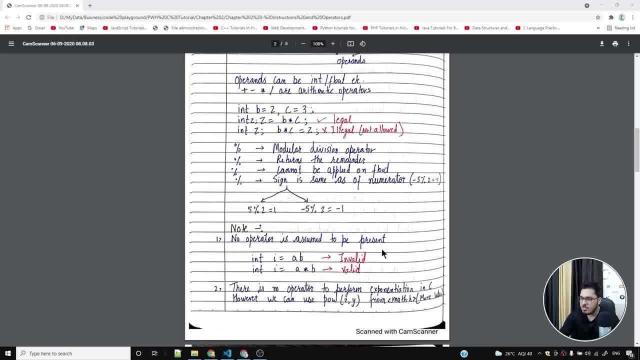 tell this in the deep study time. I still have to have someierz strength to knock it down. product value: same. if you say int i is equal to a star b, yes, star is present between a and b, so we can multiply a and b and the value of i will be a multiplied by b. but if such kind of operator is not present, if you say: 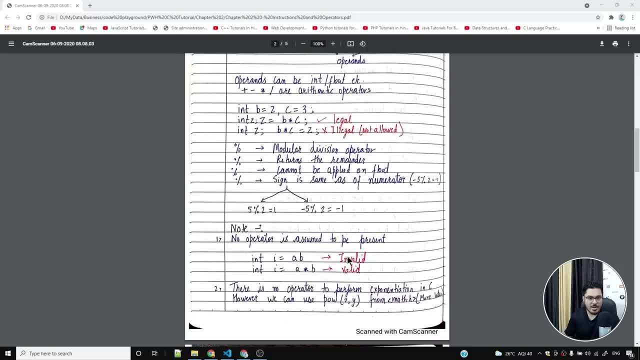 i is equal to a, b. this is invalid. this is invalid and this is going to throw an error. there is no operator to perform exponentiation in c. however, we can use pow, x, comma, y from math more later. so there is no direct operator in c to perform exponentiation. if you want to create. 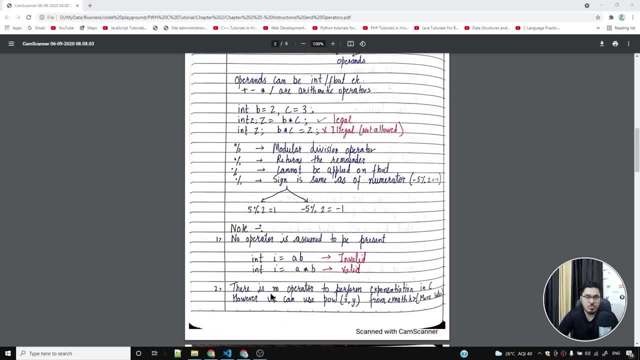 a square, you can do a star a. if you want to find out cube, you can do something like a star, a star a. but if you want to do a to the power 39, there's no other way directly than to write a 39 times manually. but there is a function called pow where you can do x comma y and it will evaluate to x to. 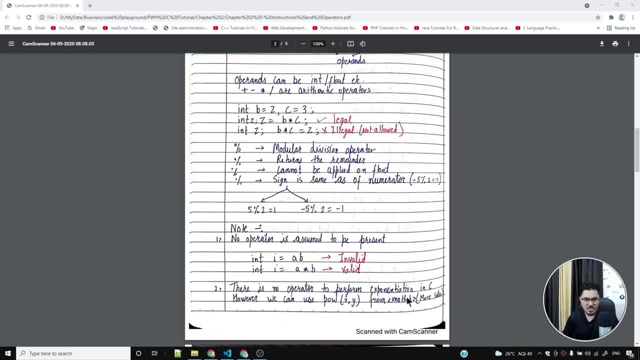 the power of y and it is from the library mat dot h. we are going to look into the library very soon later in this course, but again, this is something that you need to keep in your mind: that, yes, we have a function, we have a handy function. it's not like you cannot do it in c, you can. 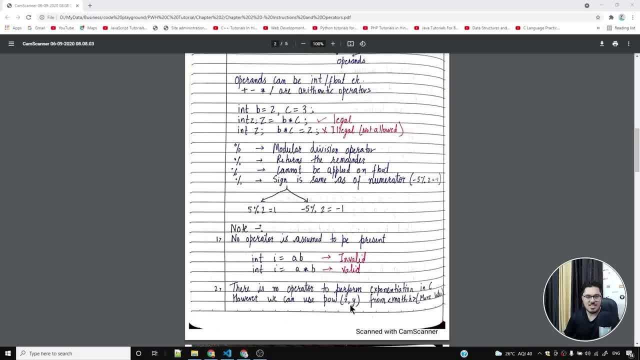 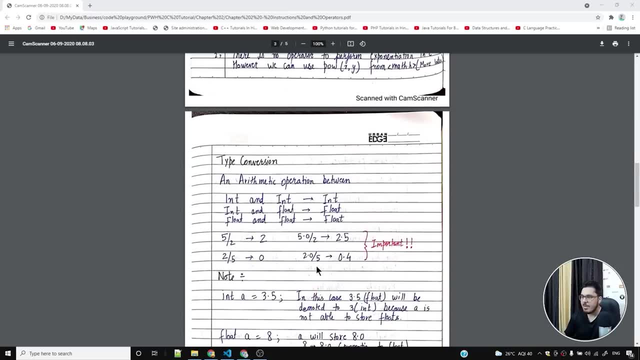 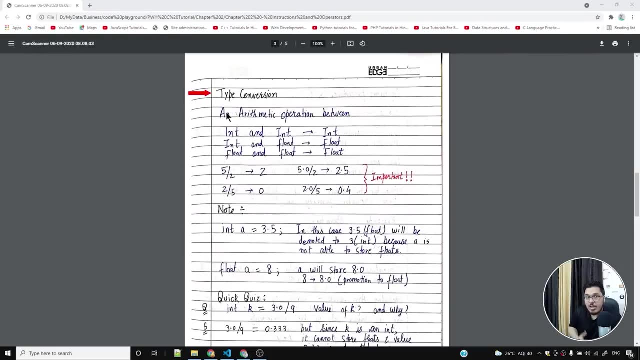 definitely perform exponentiation very, very easily in c. so we'll have to use something called power, and we are going to learn mat dot h later, so let's skip it and move ahead. type conversion: what is this type conversion? so there is a rule that an arithmetic operation between int and int will. 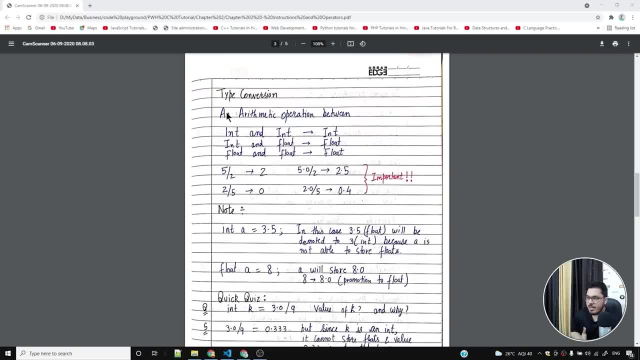 result to an int. an arithmetic operation between int and a float will result in a float. an arithmetic operation between float and float will result in a float. so at a very high level, roughly i can say that int and int, or rather any data type and other data type, the result will be promoted. 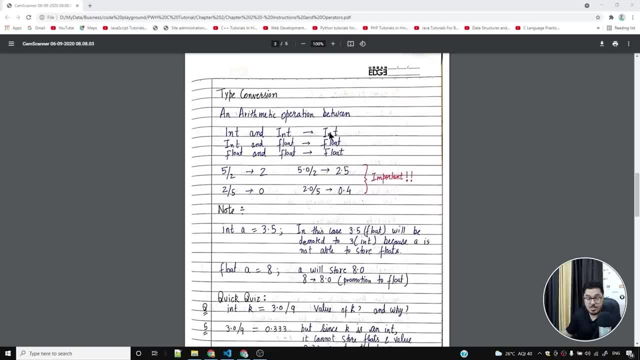 to the higher data type. so int and int will return an int, int and float will return a float. float and float will return a float. so 5 by 2 is 2, not 2.5 in c. and a lot of people they face a lot of. 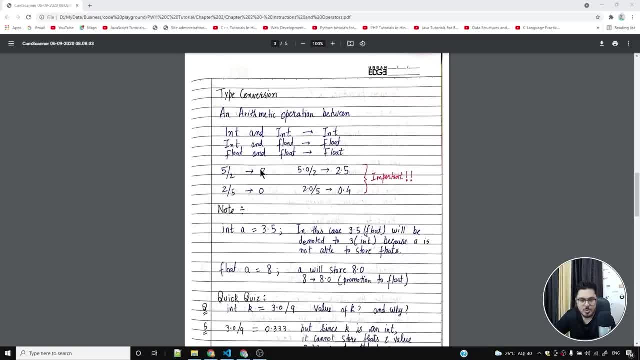 trouble because of this. so what you have to do is 5.0 by 2.0 if you want to get the accurate answer. but if you do 5.0 by 2, then also you can get the accurate answer. if you do 2 by 5, it will be 0. 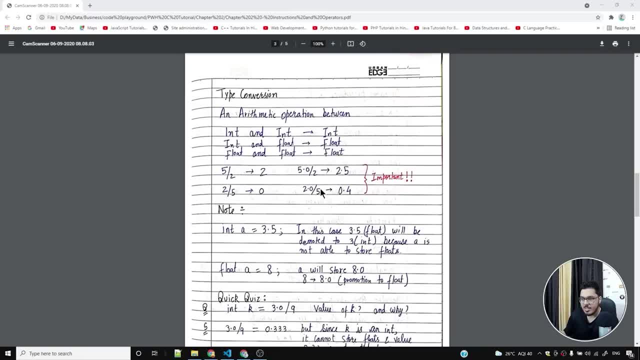 but if you do 2.2 by 5 it will be 0.4. reason being: it will be a calculation between a float and int and it will be a float. but here it will be a calculation between int and int and it is going. 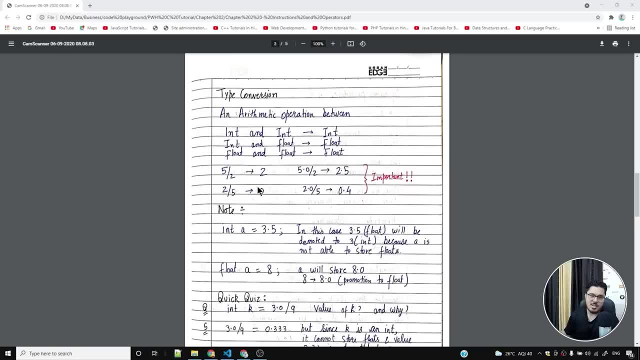 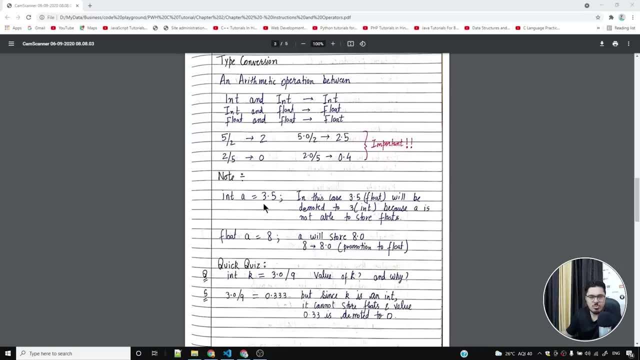 to be an int which is 0, and hence it will be wrong mathematically. now let's talk about some nodes. so when you say int a is equal to 3.5, in this case 3.5, which is a float, will be demoted to 3, because when you say int a, 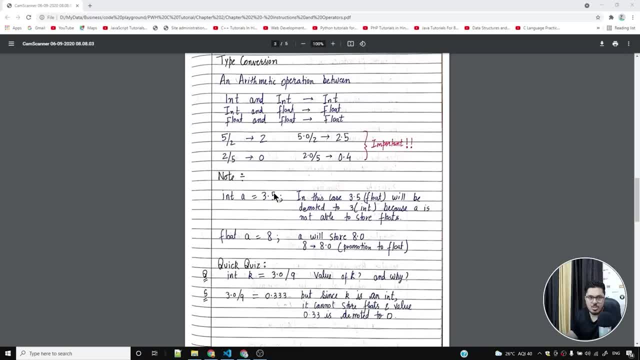 is equal to 3.5. a cannot store 3.5 because it's an integer. you cannot store a floating point number inside an integer variable, so what will happen is it will be demoted to 3 because a is not able to store floats. this is something that you need to keep in your mind. then, if you 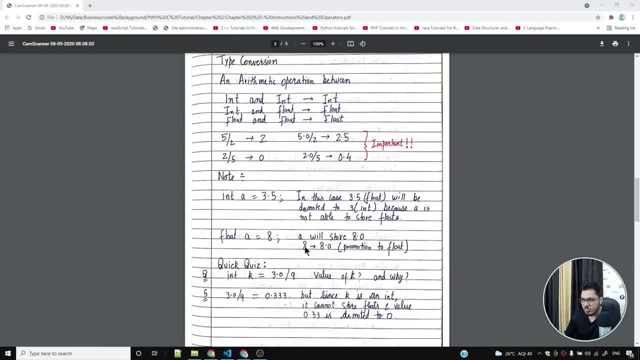 say float a is equal to 8, a will store 8.0, so 8 will be converted to 8.0 and it will be a promotion to float. so when you say float a is equal to 8, a will not directly store it because a is a floating. 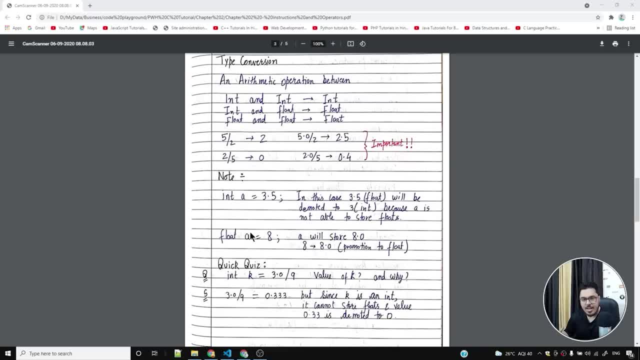 point number and since a is a floating point number, it will definitely have decimal. so float a is equal to 8.0 and float a is equal to 8 will be the same. when you say a is equal to 8, in floats it will be 8.0 by default. now here's a quick quiz for you. what will happen when you say float a is? 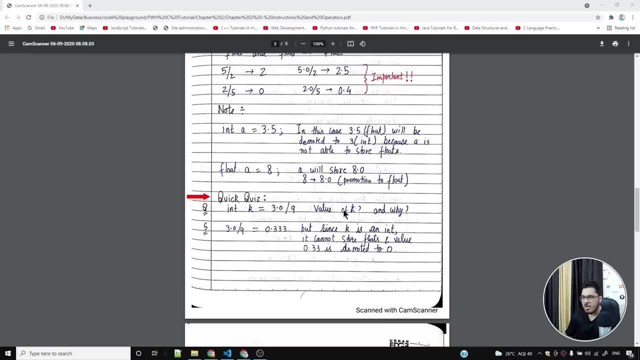 equal to 3.0 divided by 9, what will be the value of k and y? so if i do something like 3.0 divided by 9, this particular thing will be evaluated to 3 by 9, some 0.33 something, and since this is an 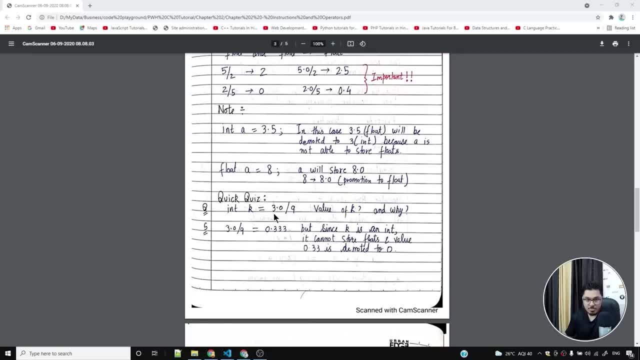 integer k will be 0 because k cannot hold floating point numbers. now, if i do something like 3.0 divided by 9, it will be 0.333, but since k is in it, it cannot store floats and value. this is equal to 0. and yes, we can see this. we can definitely see this in action. let me open this. 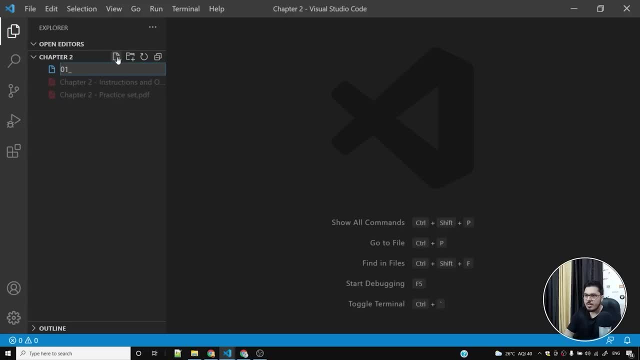 in vs code and we are going to create a first program. uh, let me call it demotingc, or rather, let me call it calculationc. i'll put the boilerplate code. i'll say: int a is equal to 3.0 divided by 9, if i'm not wrong. yes, and now what i'll do is i will simply say printf and yes, i. 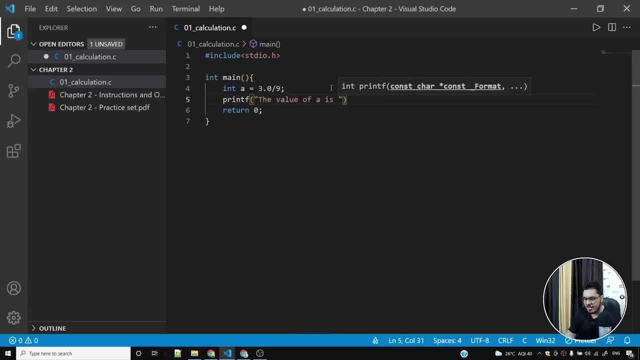 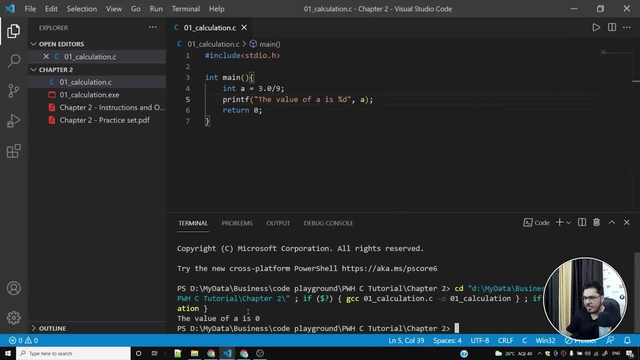 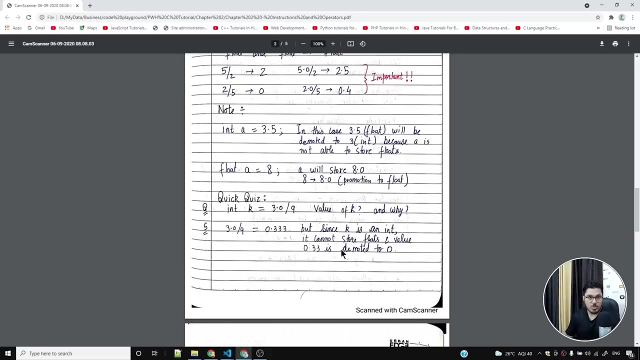 want to do printf. the value of a is, let me say, percentage d, and if i try to print the value of a, it is going to be zero. so hence it is demoted to zero. it was three point. sorry, 0.33, but it will be demoted to zero. 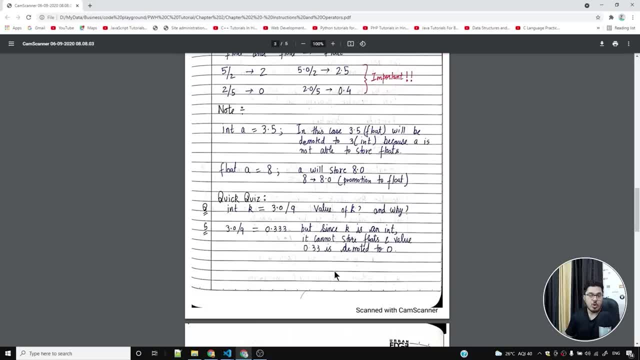 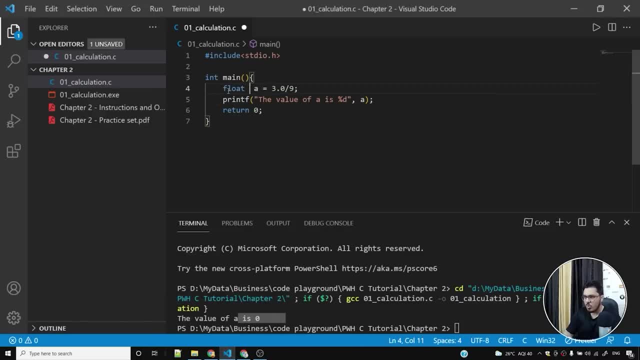 because a cannot store floating point numbers. what will happen? let me close this one. what will happen if i make it float and if i make this percentage f? will it be 0.33? yes, it will be 0.3333. so this is something that you need to keep. 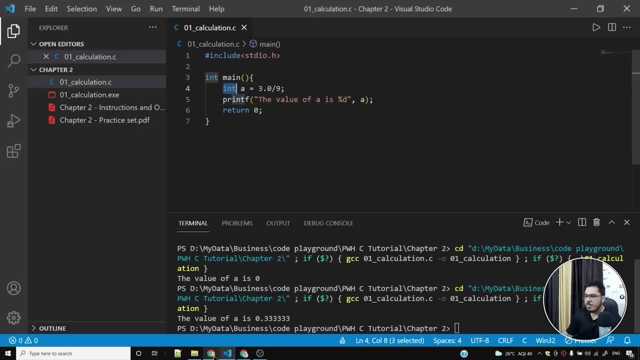 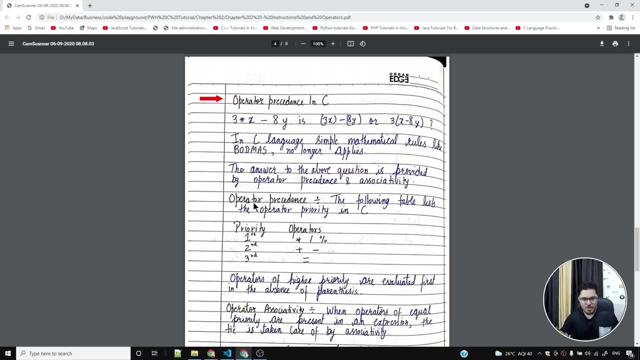 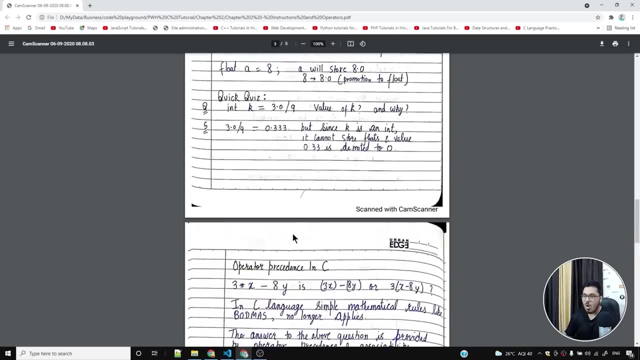 in mind. i'll make it int because you might refer to the notes and you will see that program for sure. now let's talk about operator precedence. so before i talk about operator precedence and associativity, let me also tell you that this is one of the most confused topics when it comes. 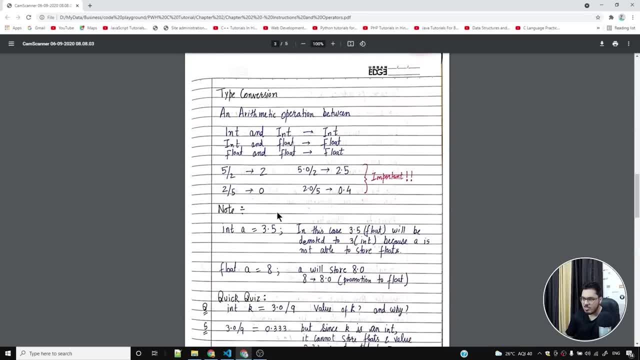 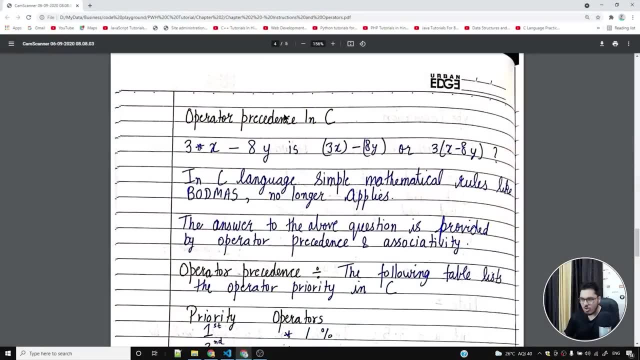 to c language and i'm going to demystify all these things for you because in my opinion, this is really very simple and these are unnecessarily complicated by people. so let's talk about operator precedence. what if i do 3 star x minus 8 star y, it is 3x minus 8y or 3x minus 8y. what will this be? 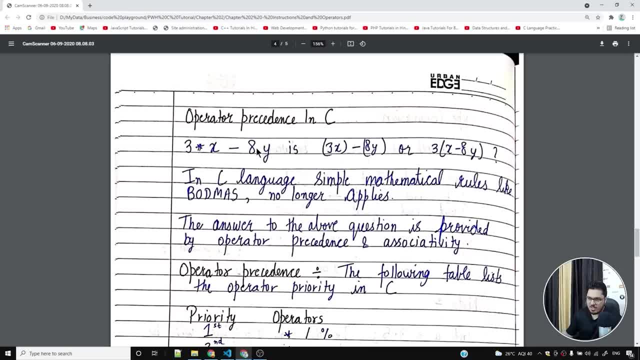 evaluated to. if i do something like this and see there should be a star here, i want to put a star here: 8 star y. so is it this expression or is it this expression? because these two expressions are different. they are not the same. this is something that you need to keep in your mind in c language. 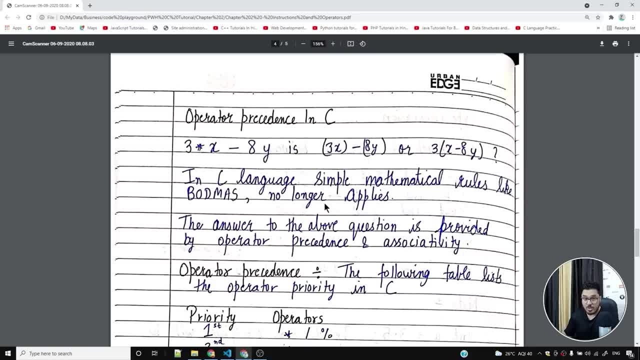 so let's talk about operator precedence. so in c language you can apply simple mathematical rules like board mass no longer applies. you cannot directly apply board mass from mathematics to c you. you cannot do that. the answer to the above question is provided by operator precedence and associativity, and operator precedence and associativity are one of the most important. 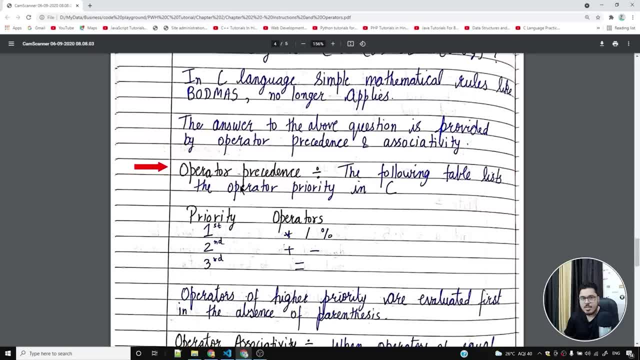 concepts of c. let's see what these concepts are. let's talk about operator precedence. the following table lists the operator. priority in c is given to plus and minus and third, most parity is given to equals to. now you can google the priority chart and you will definitely find priority of other operators, but these are the. 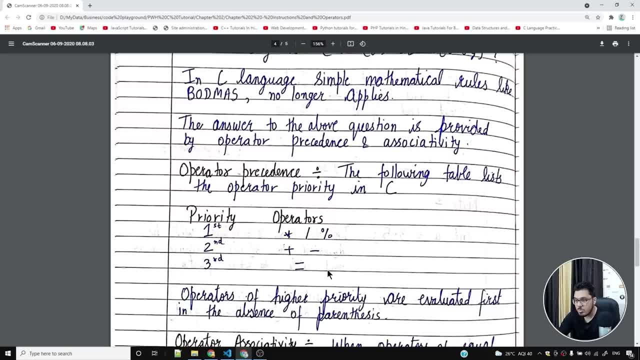 most used operators, and these are the operators whose parity you would want to learn. yes, remember all these. this is not difficult to remember. let me tell you. the first row contains star slash and percent. second one contains plus and minus. and third row contains star slash and percent, and. 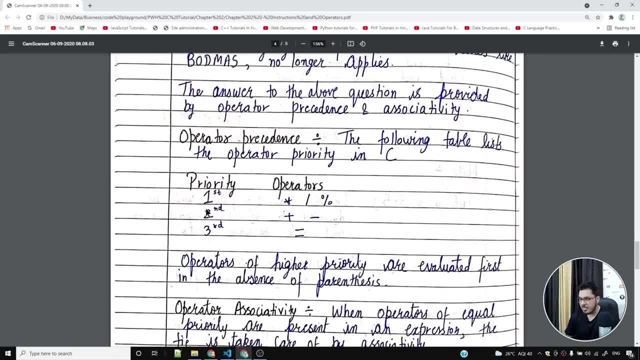 third, one contains equals to. so this is something that you need to remember: operators of higher priority are evaluated first in absence of parenthesis. so yes, parenthesis will definitely evaluate first, because the meaning of parenthesis is that you want something to be evaluated first, but in the absence of parenthesis, what happens is that priority of the operators is checked and then 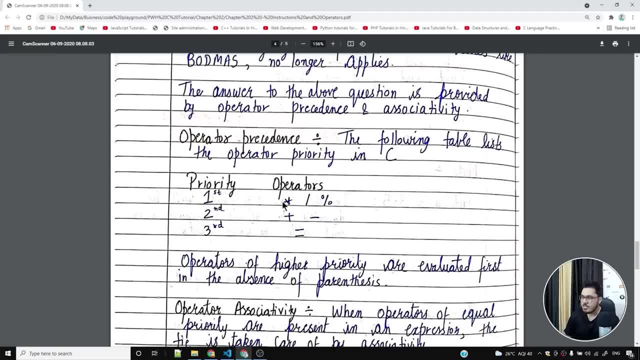 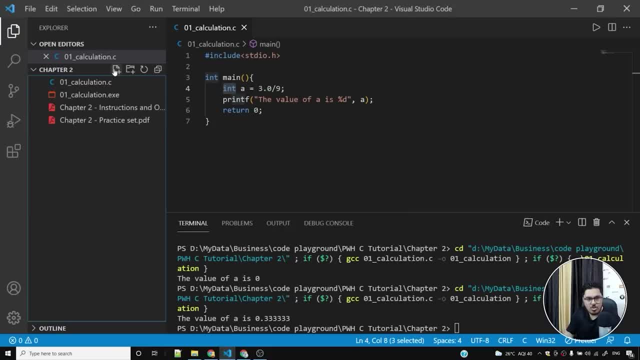 these operators are applied to the operands. so let's, let's see this in action. i want to show you here some examples of the order. don't forget to show the order in this example. sorry, this, the order is doctrinal. here's my an interval visible onto rules, like we usually call in scripting. but this one here means that 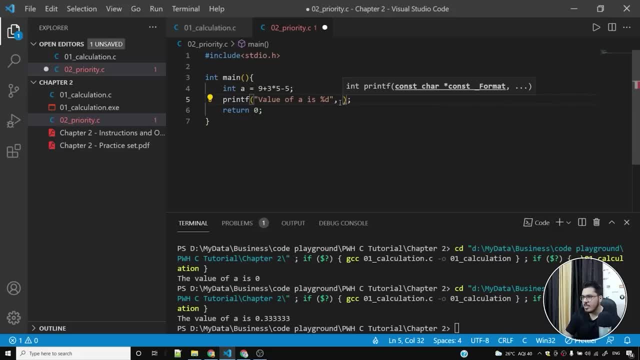 to what we call. you know the list of subordinates. thus, i will simply create a program called priorityc, boilerplate code int. a is equal to three multiplied by five minus five, and let me also do nine plus three multiplied by five minus five, and I'll simply do printf: %d. I'll say a value of A is %t, and what i'll do is: I'll write: A is gonna say so, the ni, her and also lam Mercy is the i in which we are interested in all the attributes of them. so we are假ini, our mi is, and so all 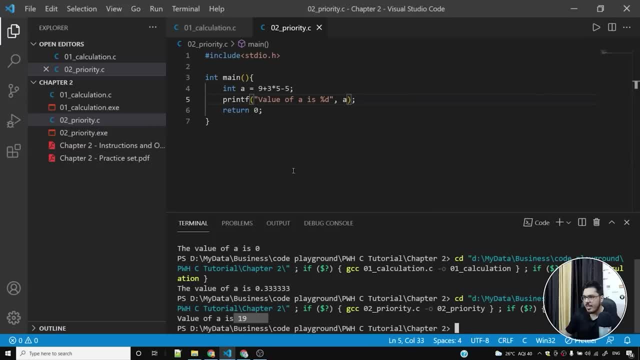 I'll write A here. let me run this program. The value of A is 19,. let's see if we are able to use this priority table and find the value of A. So five multiplied by three, this will be evaluated first. 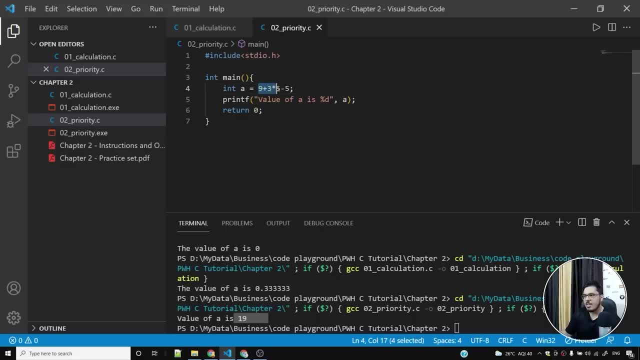 which is 15,. then 15 plus nine is nothing but 24, minus five is nothing but 19, and hence the result 19.. I hope you got this point Now. do not apply board mass here. Some people might argue that board mass 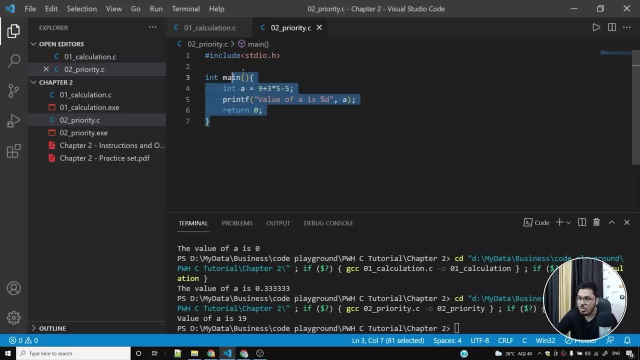 is directly being applied here. No, do not apply board mass. You have to go with operator precedence and associativity, because sometimes, in a very rare case maybe- board mass might not work because these expressions are not evaluated using board mass or some other mathematical rule. 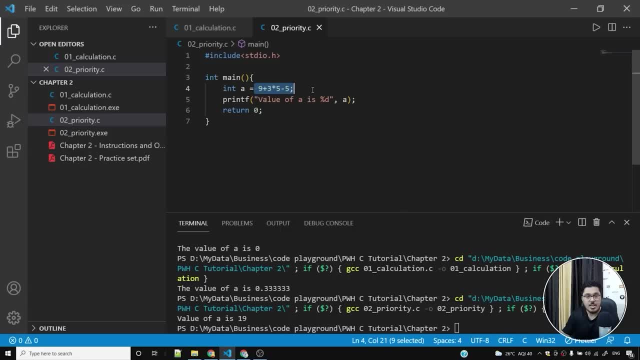 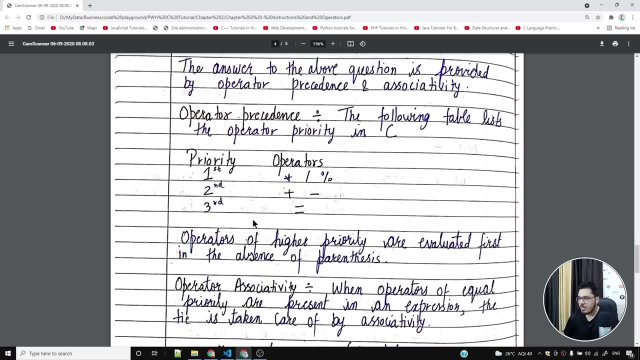 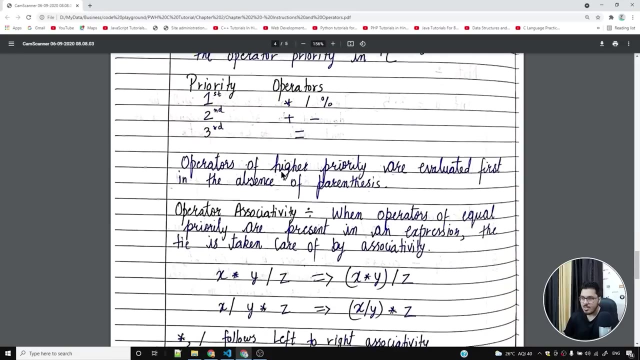 for that matter. These are evaluated using operator precedence and associativity, so you need to keep this in your mind. Now coming to operators of higher priority evaluated first. Now let's talk about associativity. so we talked about precedence. What is associativity? 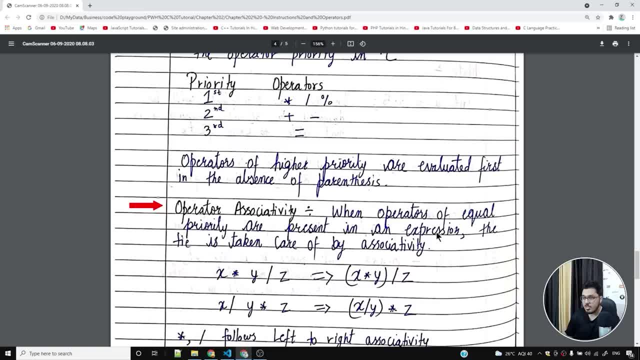 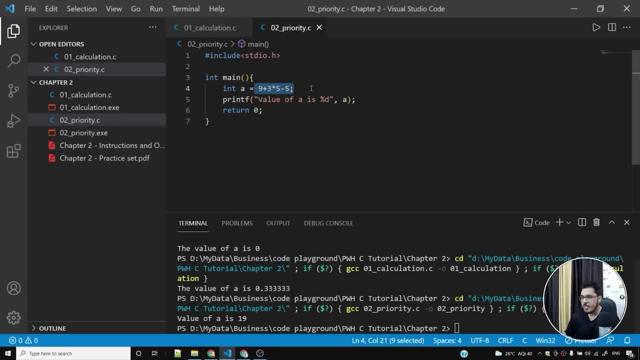 When operators of equal priority are present in an expression, the tie is taken care of by associativity. So what if you have a star and divide What will be performed first? So let me show you an example of this. What if, instead of this, I had this: 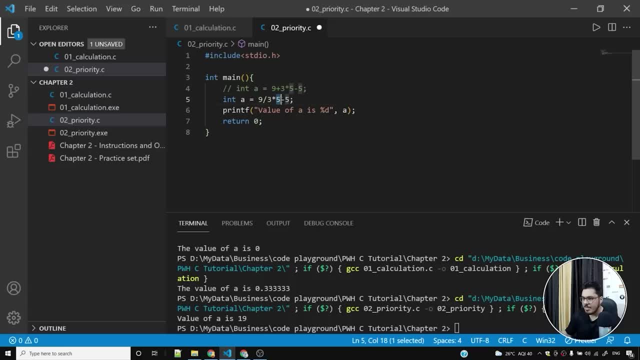 nine divided by three, multiply by say 27, minus five. Now, if you perform this thing first, then yes, answer will be different. If you perform this thing first, answer is going to be different. What is the rule that C follows? 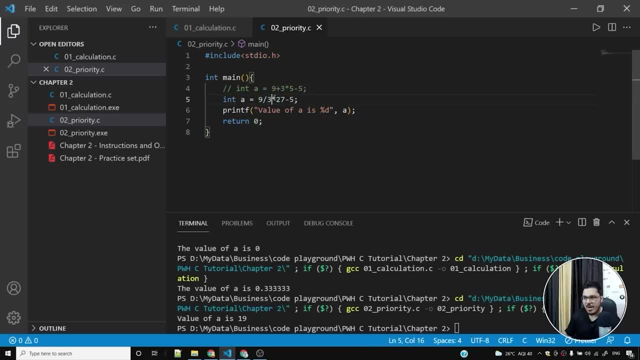 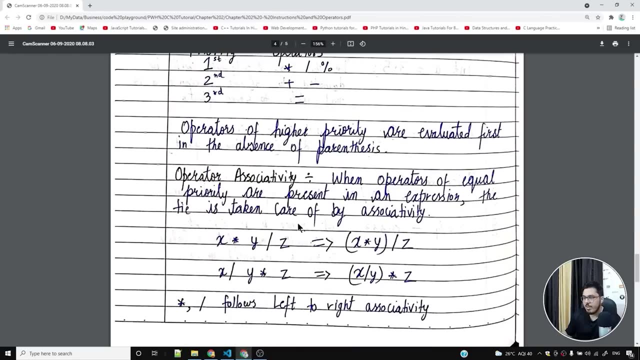 So, firstly, what we do is we know that either slash, which is divide, or star is going to be executed first, But which one out of these? And let's see what the associativity rule says. So, when the operators of equal priority are present in an expression, 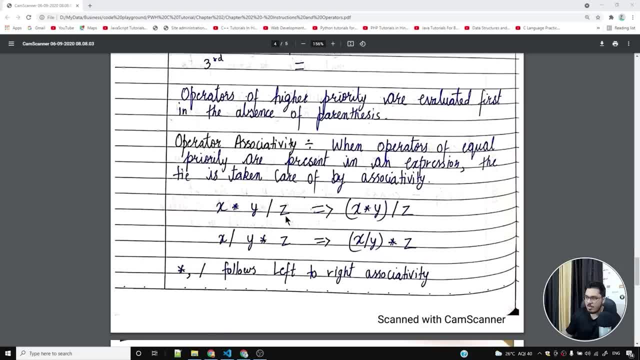 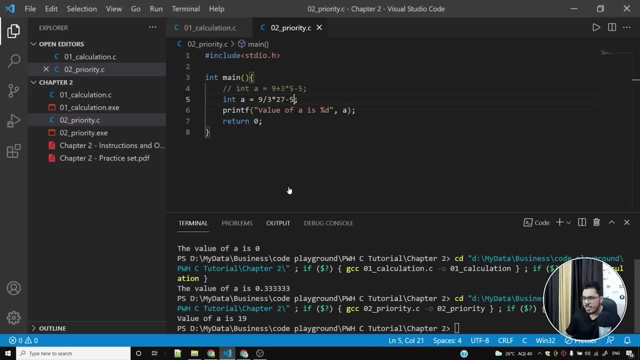 the tie is taken care of by associativity. So x star y by z is evaluated to x, star y divided by z, x by y, star z is evaluated to x by y star z, And star slash follows left to right associativity. So what is left to right associativity? 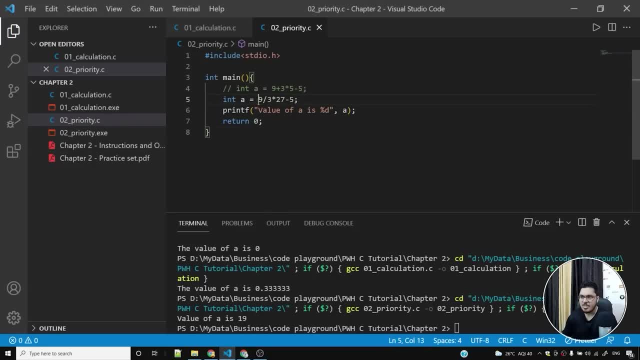 Left to right associativity simply means that you need to evaluate the left expression first, then the right. So nine by three will be three. Let me write a comment for you. So it will be three multiplied by 27, minus five, which will be 27 multiplied by three minus five. 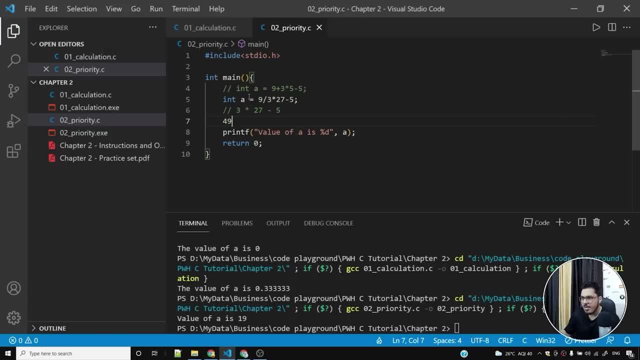 which is 49, okay. So let's see if we get 49.. So this is nothing but three multiplied by three, multiplied by nine, which is nine, multiplied by nine, which is 81, minus five, which is nothing but 76, okay. 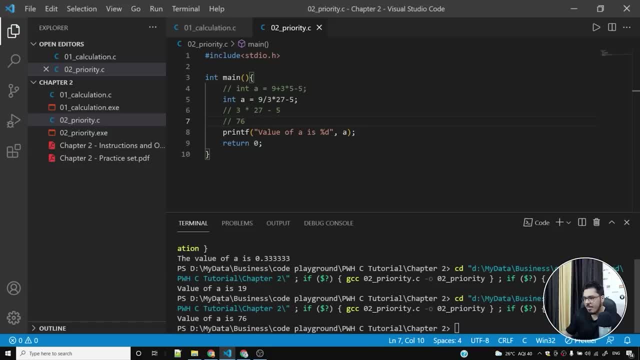 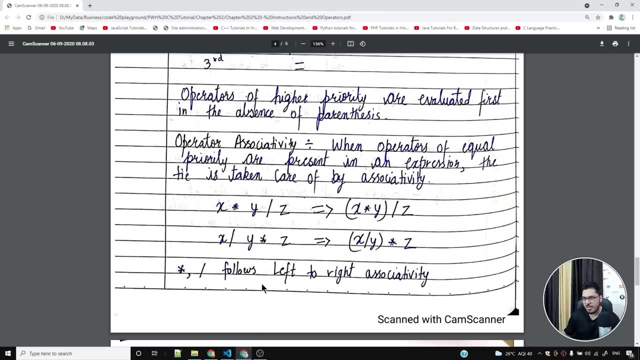 So let's see if we get 76. And if I run this program, the value of a is 76. Yes, this works So star and slash follows left to right associativity And we need to evaluate them from left to right. 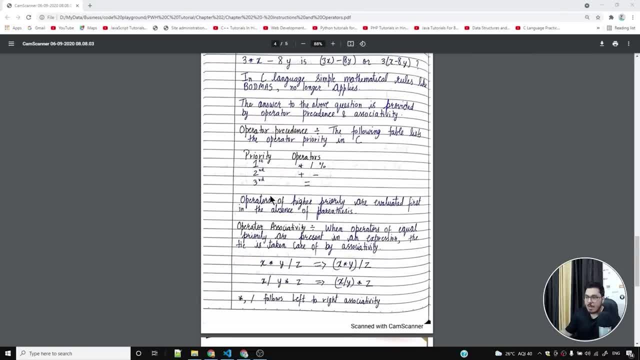 Always remember. okay, When it comes to remembering the priority end: associativity. let me tell you something. This is all you need to remember and you'll be able to solve most of the questions- 99% of the questions, But in some of the rare cases, 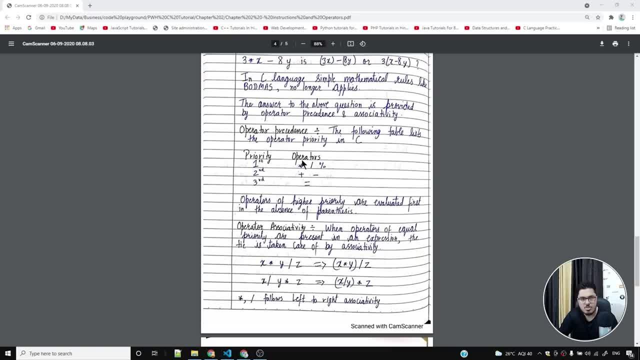 you might want to Google the priority of some of the miscellaneous operators. So the rule will be applied just like this: First find the priority. Once you have the priority, you need to evaluate the operators which have the higher priority. Which one will be evaluated first? 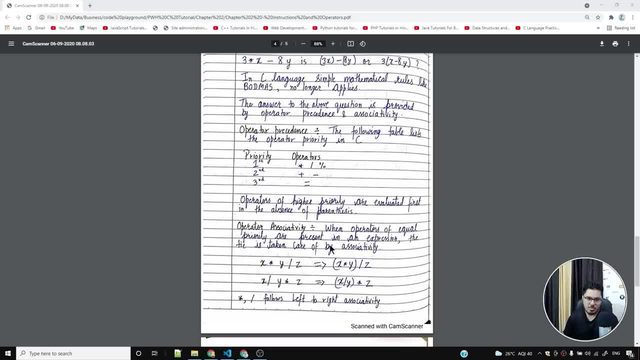 You need to find the associativity. If it is left to right, then yes, you will use the left to right associativity to evaluate those operators. Go from left towards the right and keep on solving the operators. I hope you've got the point. 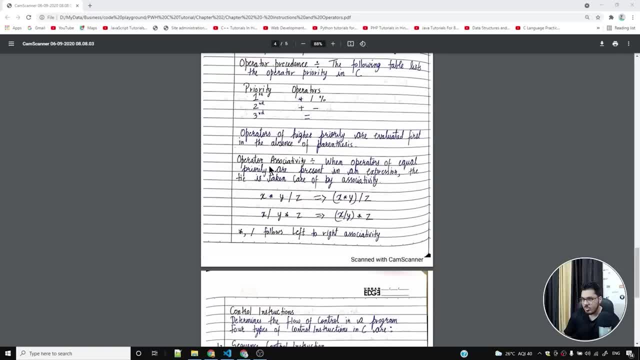 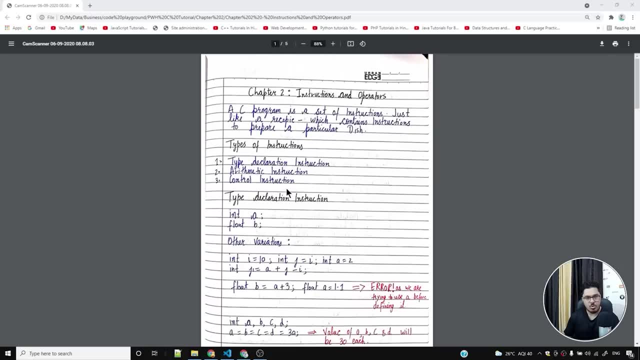 I hope this is clear. Let's talk about control instructions. Remember we were talking about instructions. We had type declaration instruction, arithmetic instruction. Then the third one was control instruction, The type declaration function. look like this: sorry instruction. look like this: 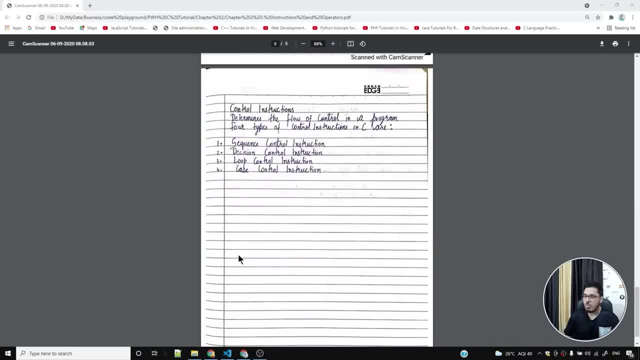 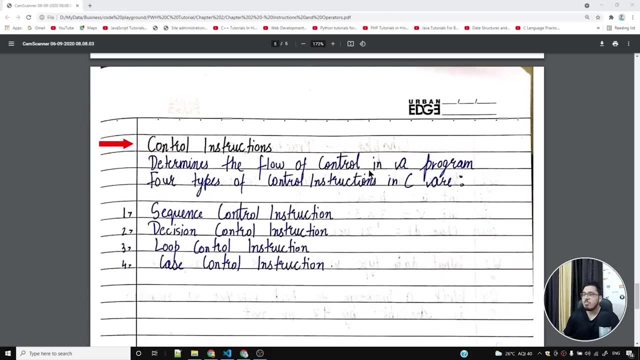 Then arithmetic instruction. look like this: Now let's talk about control instructions. Now let's talk about control instructions. Now there are four types of control instructions. in C. it determines the flow of control in a program. What is a control instruction? 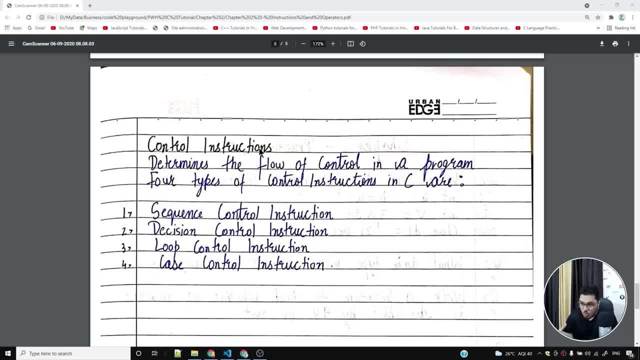 It determines the flow of control in a program: where to go, when, what will be executed first. So there is a sequence control instruction, there is a decision control instruction, there is a loop control instruction and there is a case control instruction. 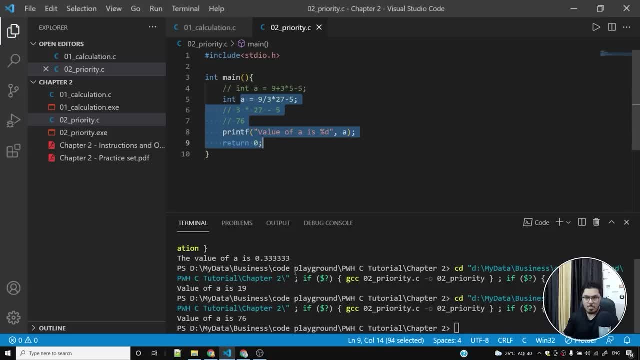 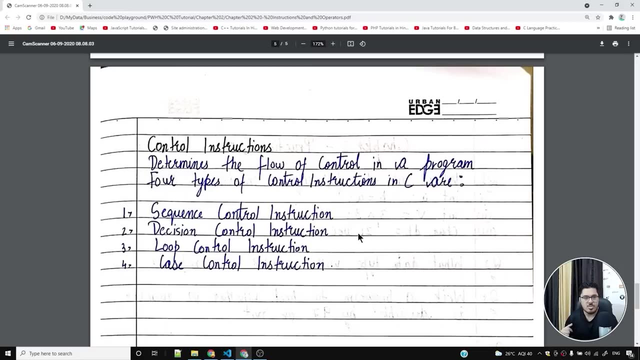 Sequence control instruction is nothing but what we already saw. Then there is something called decision control instruction. we will look into, if else, in the later chapters and you will come to know what decision control instruction is. Then we have loop control instruction, which is nothing but some of the loops while loops. 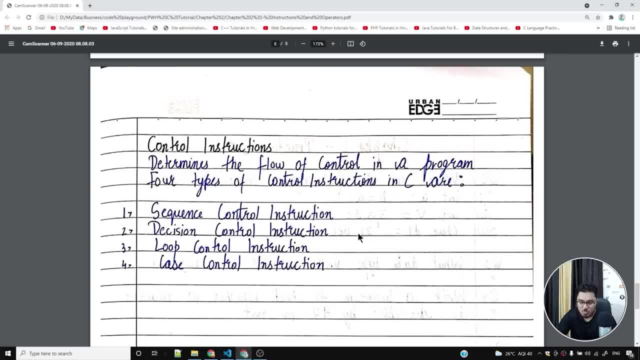 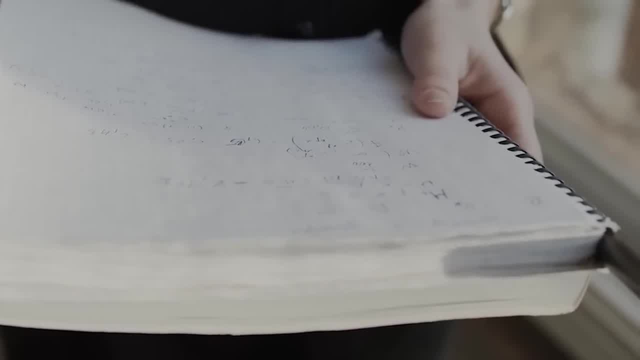 for loops do while loops. we will look into loops. do not worry about loops, But this is one of the control instructions, is something that you need to remember. You might want to come back to this page from the notes when we look into loops and if else. 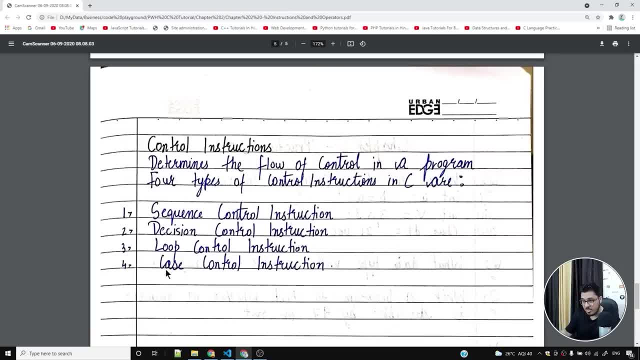 statements and switch case statements. So case control instruction is something that we will look into later as well. So these are the four instructions. we are going to look into the later chapters and let's now do something which can strengthen our concepts of instructions and operators. 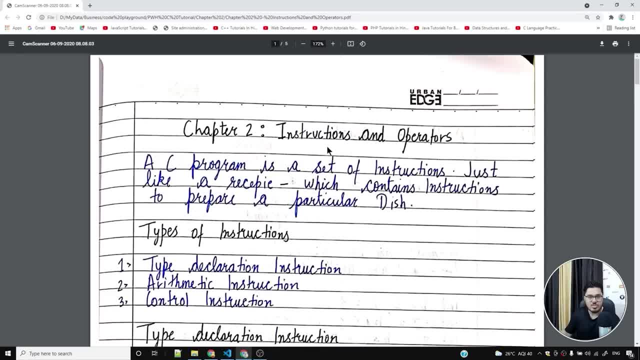 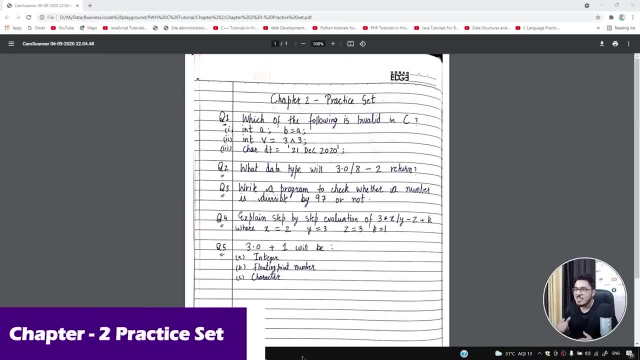 Let's go to chapter two practice set and solve for some of the questions on instructions and operators. Let's move to chapter two practice set now. Now, before we look into the C chapter two practice set, I want to discuss a few things, and these things are going to be really important. 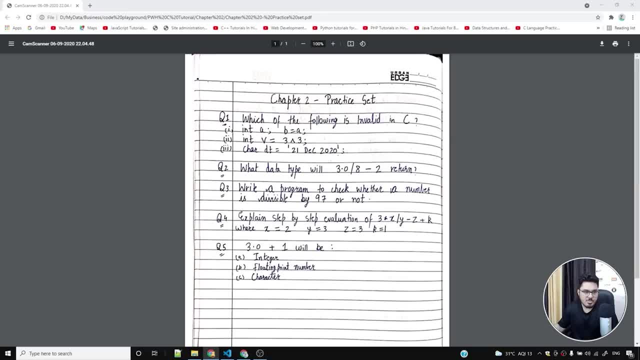 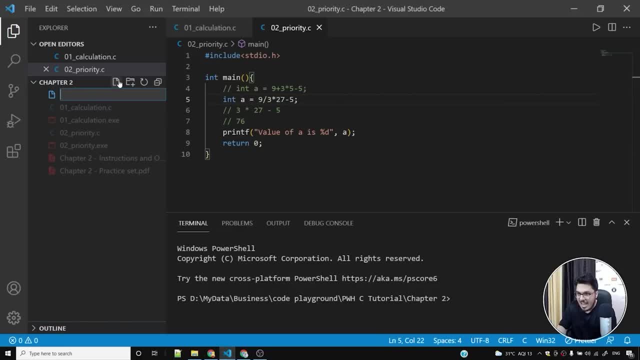 So listen to me very, very carefully. We'll look into the data types in C, So we'll learn about the four major data types in C which are CAS. So let me mark it as question number one. So program number three, question number one from the practice set and dot C is the extension. 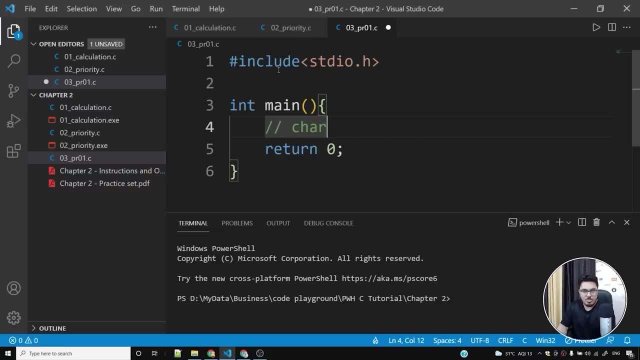 Let me write down the boilerplate code and let me write down the first character. So let me type it down. There are four major data types, So let me write down the first character. So let me type it down: There are four major data types in C. What is the first one? 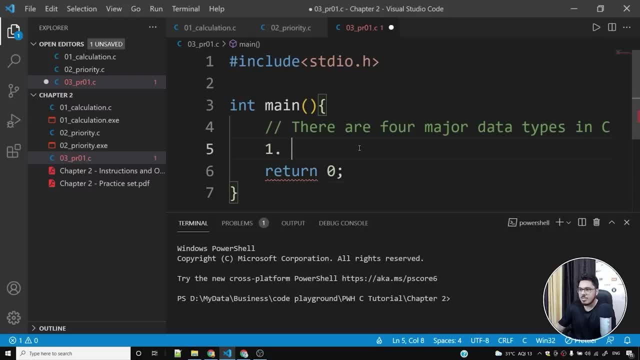 In C we'll talk about the first one. and the first one is- let me also put something like this: It's int, then we have float for floating point numbers, Then we have char, and char is for characters, and then we have double, and double is for. 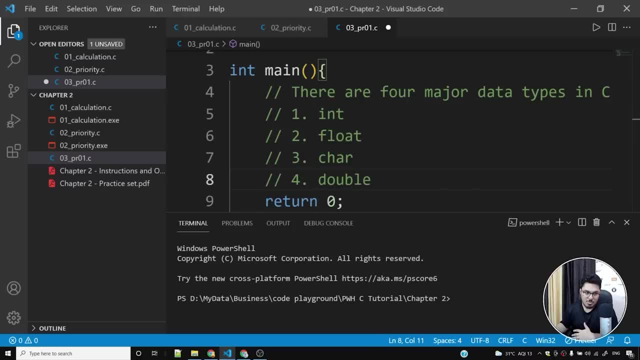 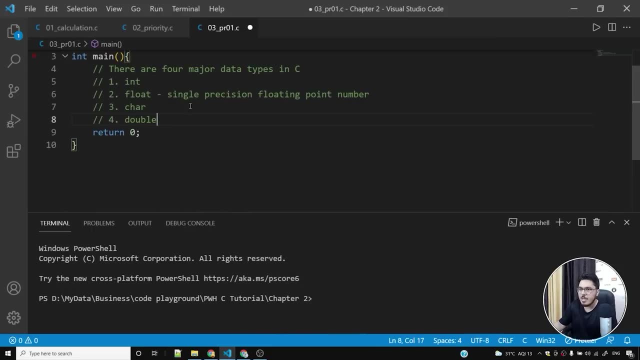 it's for decimal. It's for decimal numbers, but with double precision than the floating point numbers. Okay, So this is single precision floating point number, And let me also close this, and what I'll do is I'll now write a double precision floating. 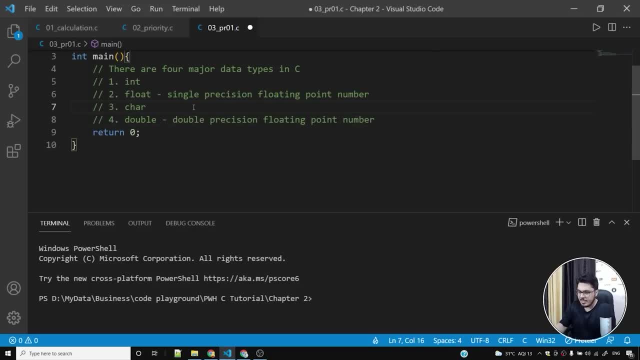 point number. So let me type double here and then character is for storing characters enclosed in single code. So this is something that is important: You need to enclose a character in single code, So you cannot do something like this to store characters. 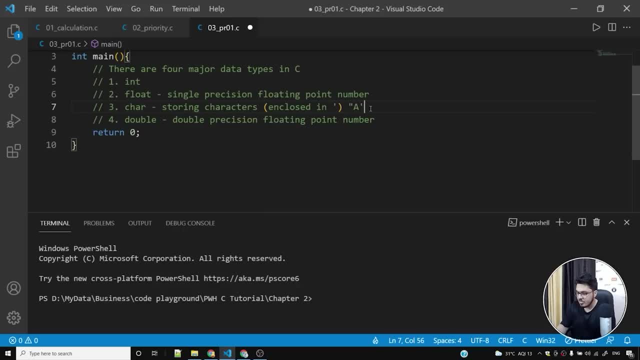 So this is something that is important. You cannot store a character. You'll have to do something like this, So let me type it down: This is valid. Okay, So this is important. And then this is for storing integers: Okay. 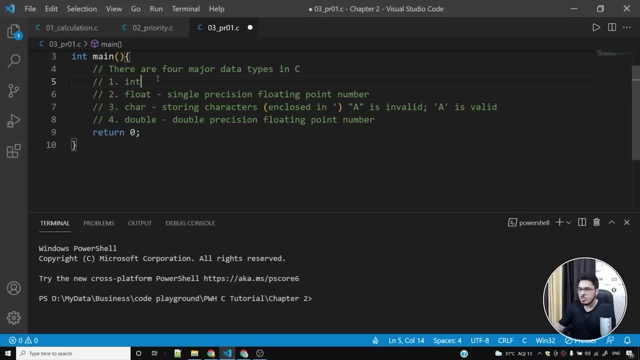 So this is something that you need to keep in your mind. Now let's solve the question number one. So, coming to the question number one, which of the following is invalid in C? First one is valid, Second one: maybe Let's check it. 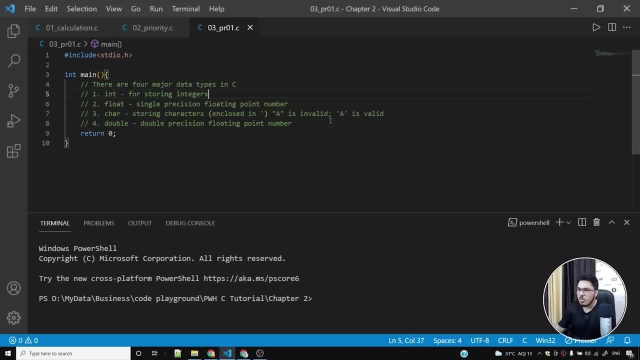 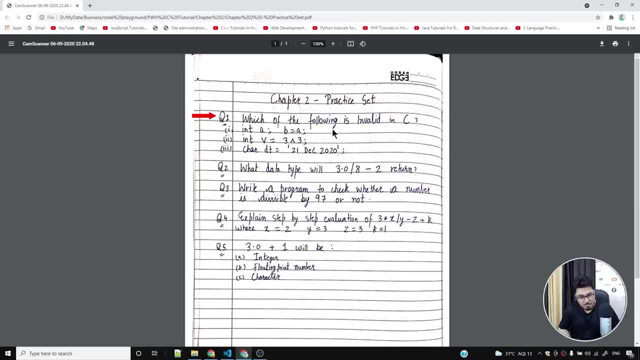 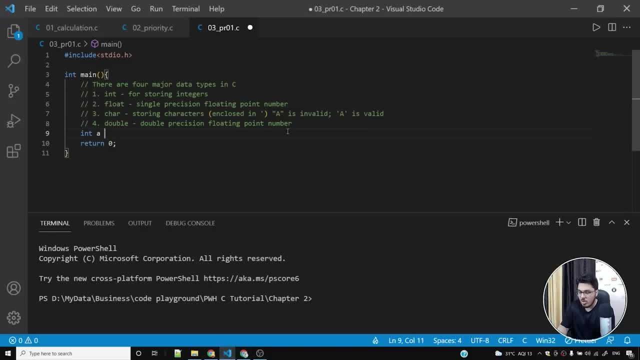 So let's see. So let's see, So let's see, Maybe let's check it. It's invalid, by the way, But in case you want to check whether it's valid or not, you can simply use this. So if you have done some sort of mathematics and you want to use this character to raise, 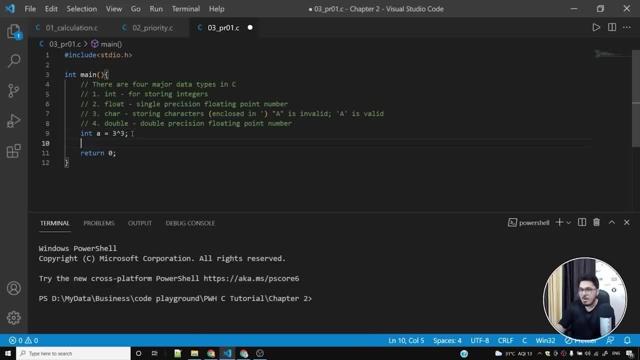 the power of three to three, it is going to be invalid. But if you want to see whether this actually runs or not, this is going to run because this is a bitwise character in C, So we are not willing to look into bitwise characters in this video. 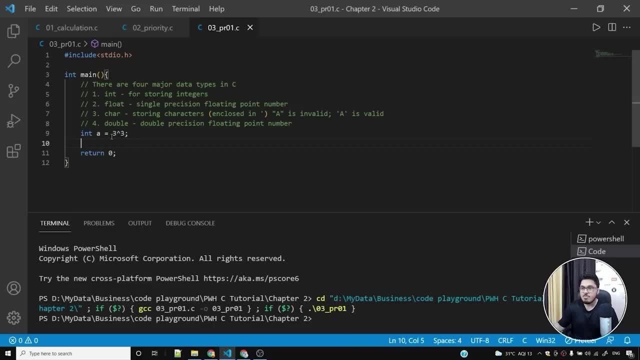 but this is actually valid. this is valid in c. this will. this is not valid to calculate the power of three to the power three. so this is valid. so you need to make sure that this is a valid character in c, even if you don't know about a character that might be a valid character. 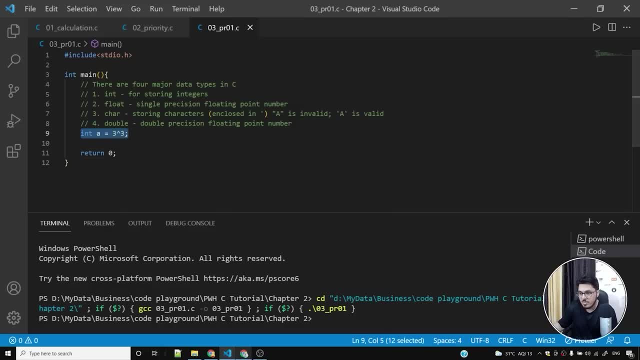 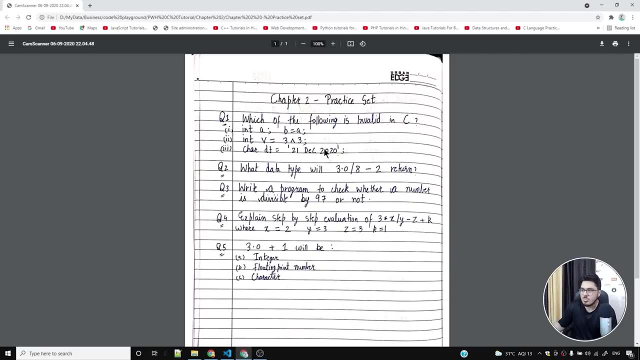 in c. so this is the takeaway of this question, basically. and what about the third one is definitely invalid because you need to store a single character in a char variable. you cannot store a date, you can't do this, so this is something which is invalid, so you need to. 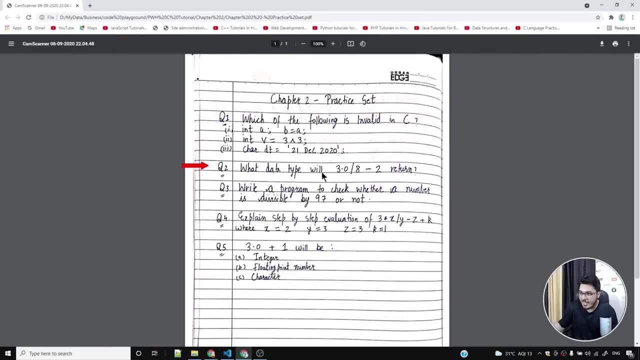 make sure that this, this is valid. what data type will 3.0 divided by 8 minus 2 return? and this is clearly very simple. this particular thing will return a float and the entire thing will return a float, right or wrong, wrong? let me show you why. so, um, i know, i know you are. you might be thinking. 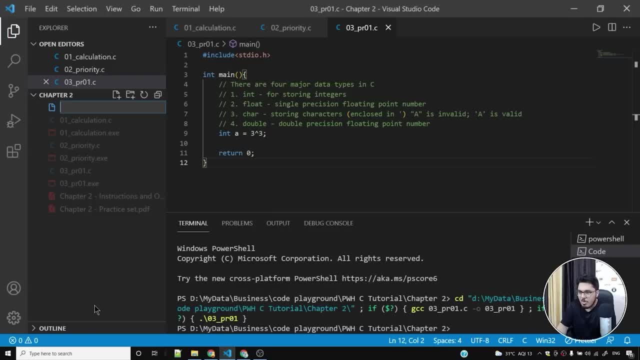 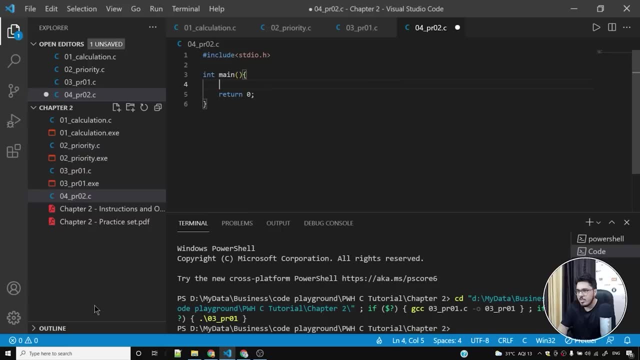 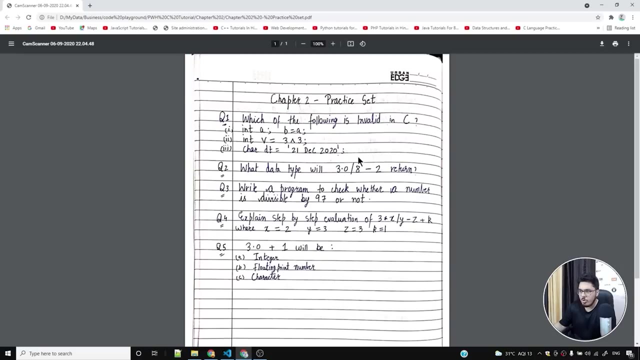 that: uh, why is it wrong? what? what's wrong about this? so let me tell you. so this is problem number 2.c. let me put the boilerplate code and let me show you. so what i'll do is i'll simply say, uh, 3.0, divided. 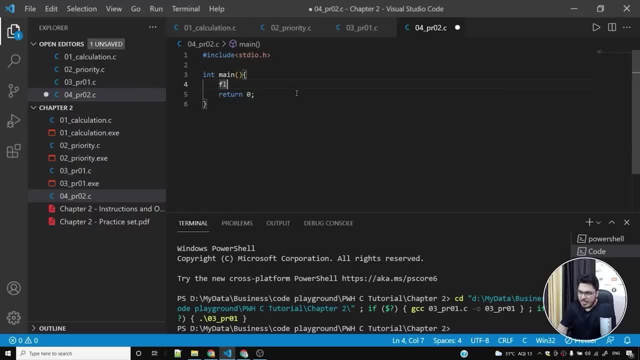 by 8 minus 2. so if i do something like this, i'll say 3.6666. what is this? is it a double? is it a float? it's by default a double, so whenever you write a decimal number in c, by default it is double, but sometimes it might. 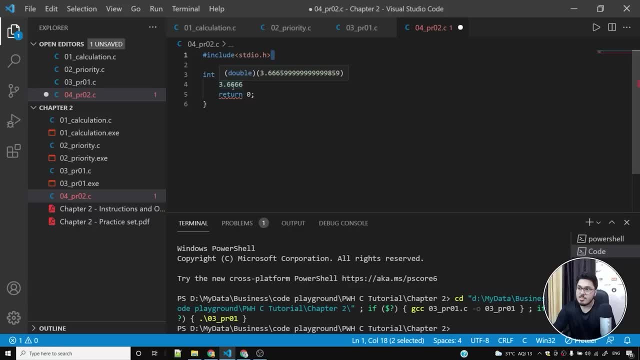 depend upon the compiler, but in most of the cases it is double by default. so since this is double, so the entire thing is going to be double. so let me save this program for you and let me also show you why this entire thing will return double. double divided by. 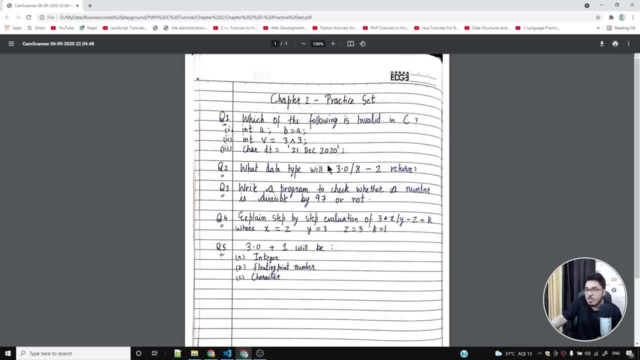 integer will be a double. double minus integer will be a double, so this will return a double data type. i hope that this is clear and you are able to grasp the concept of this problem concept: i want to teach you write a program to check whether a number is divisible by. 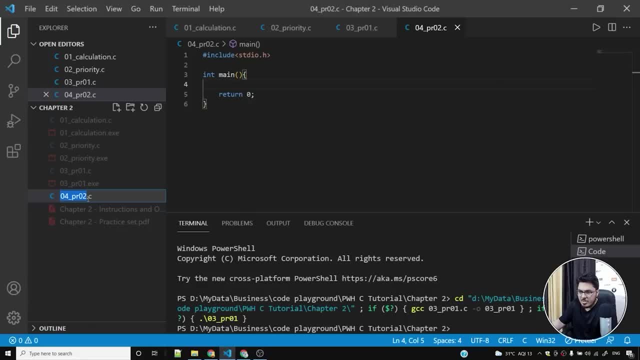 97 or not, and this is going to be simple. let me change this to pr03. pr02 was very simple, so i just want to check whether a number is divisible by 97 or not. so i'll say int a is equal to. let us say, i have a number which is 194 and i want to check whether this is. 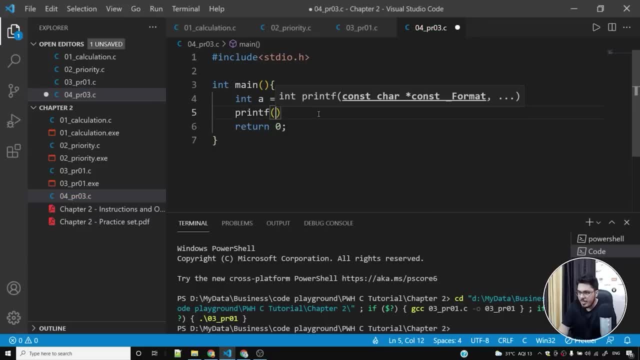 divisible by 97 or not. so what i'll do is i'll do printf and i'll do percentage d and let me see if i get a remainder. so i'll say a percent 97 and let's see whether this is divisible by 97 or not. so i run this program. i get zero. 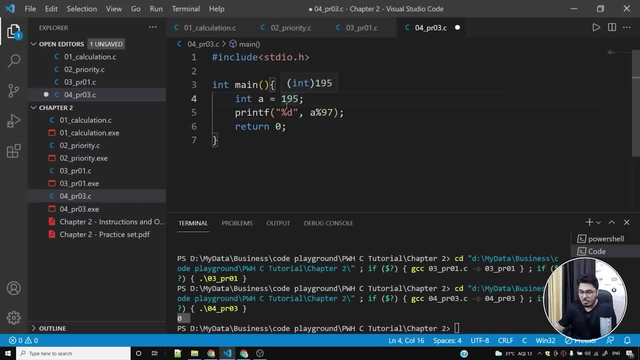 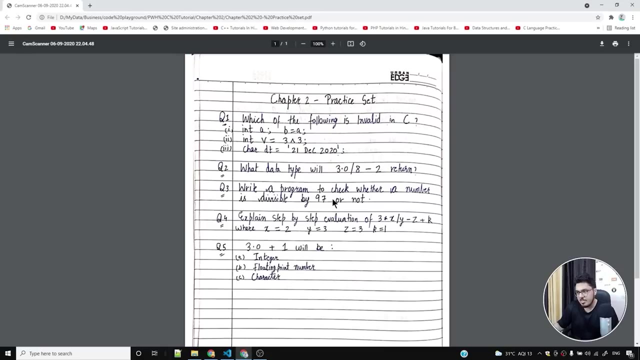 so the remainder is zero, which means it is divisible. what about 195? uh, it's one, remainder is one, so this is not divisible by 195. a 97 doesn't divide 195, so 195 is not divisible by 90.. seven- okay, i hope you got this point. and this is a program to check whether a number 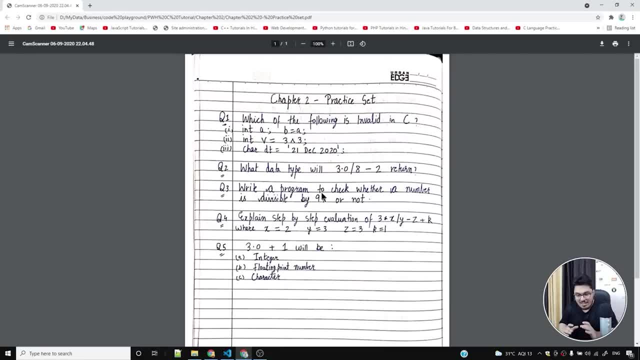 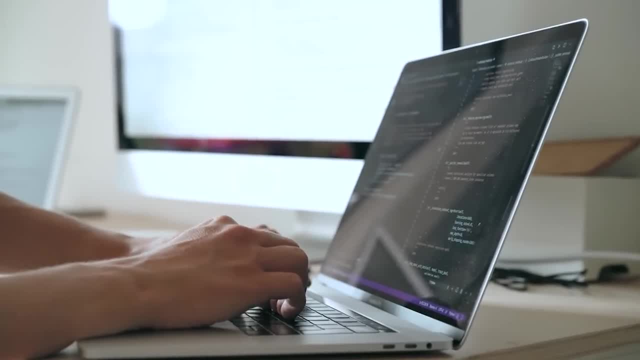 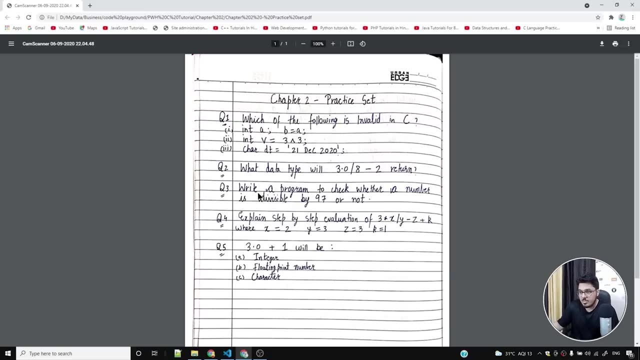 is divisible by 97 or not. now i want you to refactor this program and convert it to a program which takes an input from the user. i want you to write a program which takes an input from the user. yes, you heard that right now. this is it for this question, i hope. 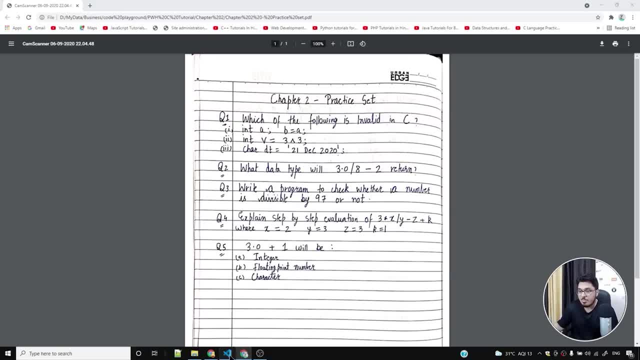 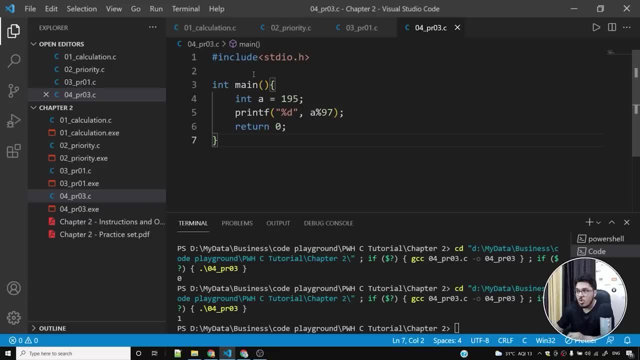 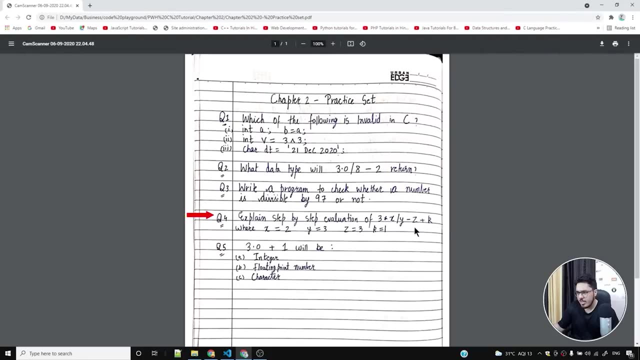 you will accept the challenge and show me the program wherein you are accepting input from the user. i want all of you to comment that program in the comment section below and comment it if there are any questions. you have any questions, etc. pd try writing in the comment section. make sure to write the timestamp so that i can see which question. 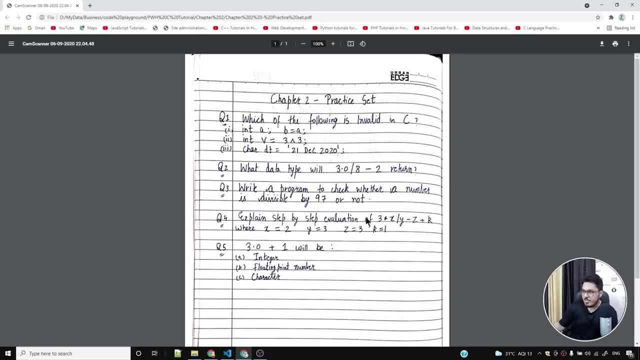 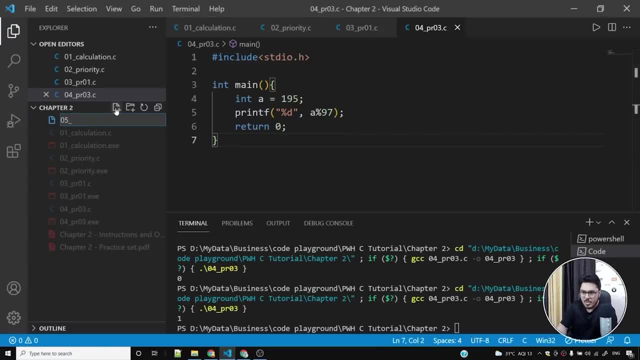 you have solved. okay. coming back to the practice set, question number four says: explain step by step evaluation of this thing. where x is equal to 2, y is equal to 3 and z is equal to 3 and k is equal to 1, and this is important, this is very important. so it's 3x divided. 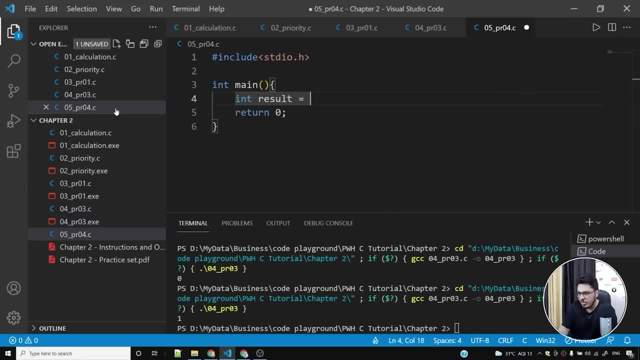 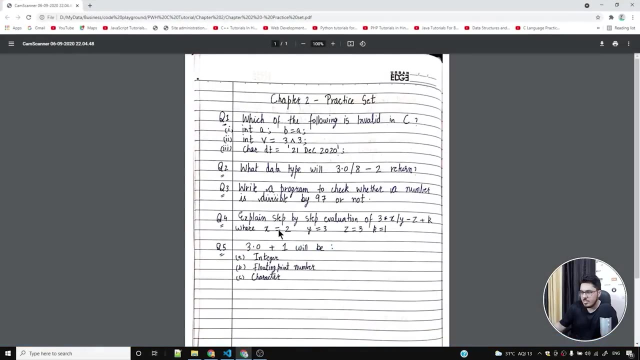 by y minus z plus k. let me write it down. let me create a new file and then write it down. result is equal to- and let me write it down: 3x by y minus z, 3x by y minus z plus k. but we still have to write down all these, um, all these variables. x is 2, y is 3, z is 3. 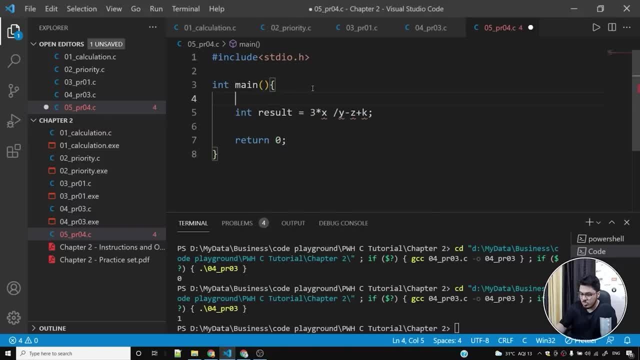 and k is 1. okay. so x is 2, y is 3, z is 3 and k is 1. okay. so let's try to find out what this particular thing will return. and yes, you can always say int result is equal to expression. this will put the value of the expression into result variable. also, what i'll do is i'll use 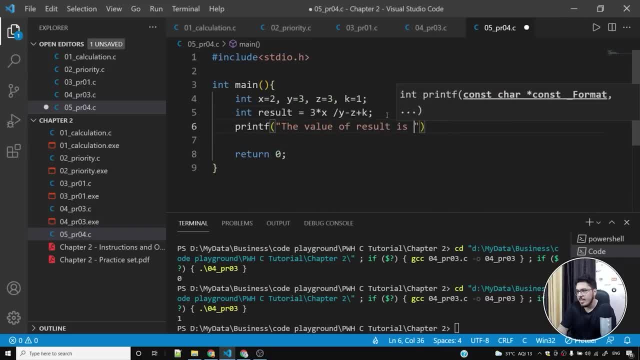 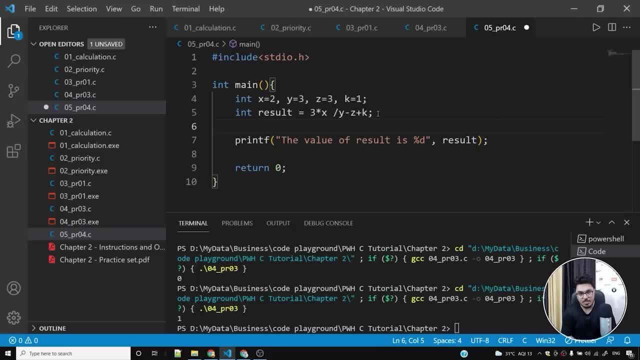 we are going to see is the priority, or rather precedence. what is the precedence? which? which one is the operator with highest precedence? star and divide are the operators with highest precedence. what is the associativity? because we have two such operators: one is star and one is divide. it is left to right. so 3 multiplied by x will be evaluated first, which is going to be 6. 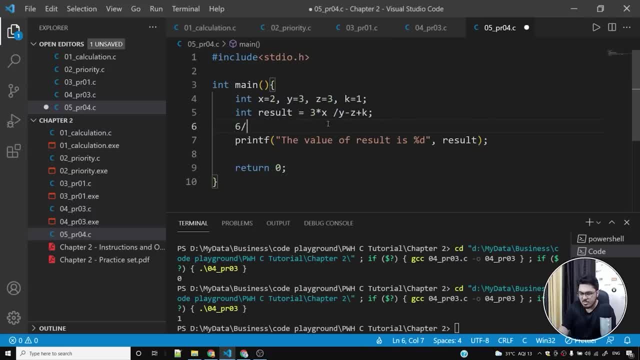 so let me write it down: 6 divided by- and the rest of the numbers will be written as is 6 divided by 3 minus 3 plus 1. okay, so this is going to be the resulting expression. now, what i'll do is i'll simply evaluate 6 by 3 to 2. why? because this is going to be the operator with highest precedence. 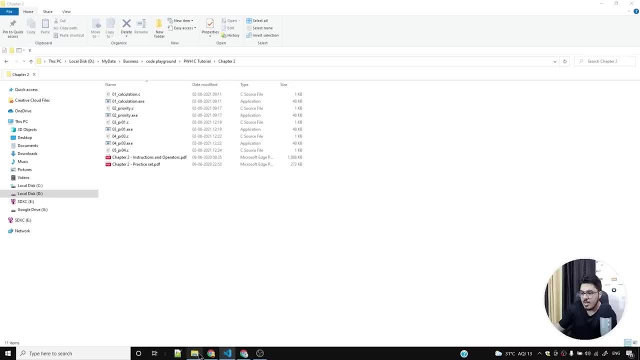 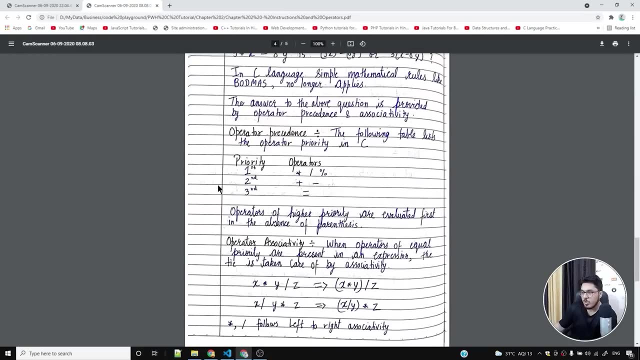 star and divide are the operators with highest precedence. let me show this to you if you have not seen it previously. i've written it down in the notes for you. so if you look at the priority of these operators, you will see the first priority is given to these operators. second is to these: 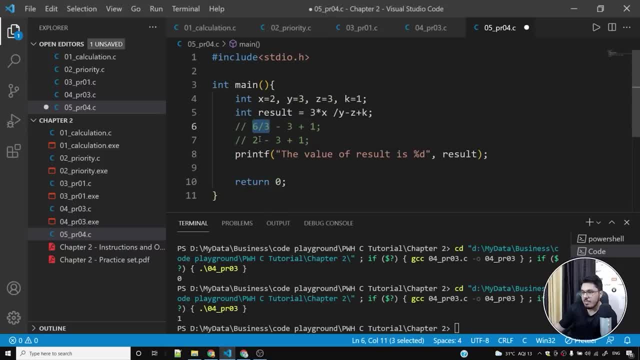 operators. now we, since we have operator with the topmost priority, we will have to evaluate it to the integer. now, 2 minus 3 plus 1 is going to be 0, so the answer should be 0, and let's see if this is the case. and yes, this is the case. 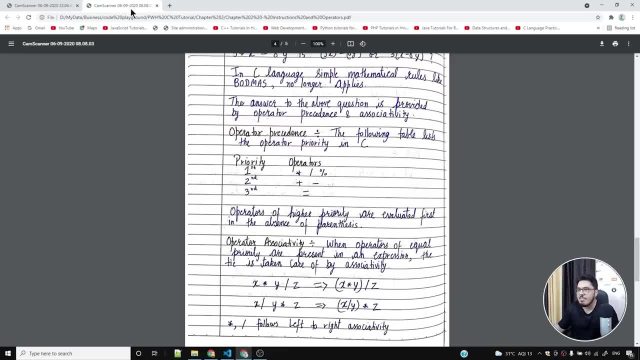 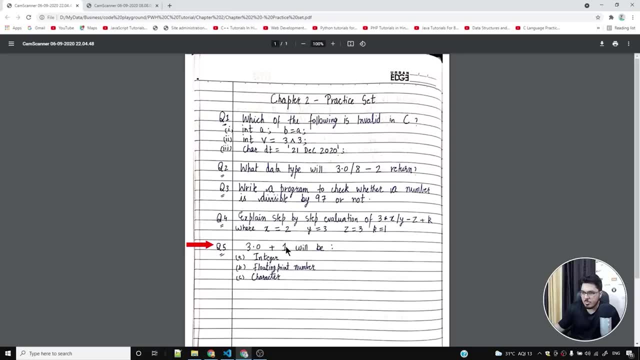 answer is 0, so this is how we can evaluate this particular thing, step by step. now, this is a. this is an important question. what is this? is it a 3.0? is 3.0 plus 1, an integer character floating point number? it is going to be a floating point number, for sure, but not float. it is going to be. 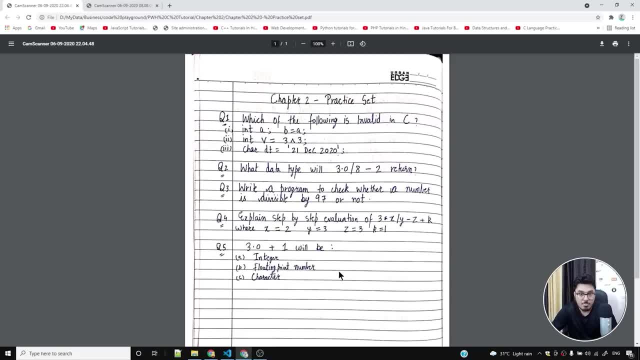 double and it might depend on the compiler as well. your compiler might store the default floating point number as floats. you never know. you can always design a compiler which stores a number as a float, but in my case, the compiler i am using it is a double, but it's always a 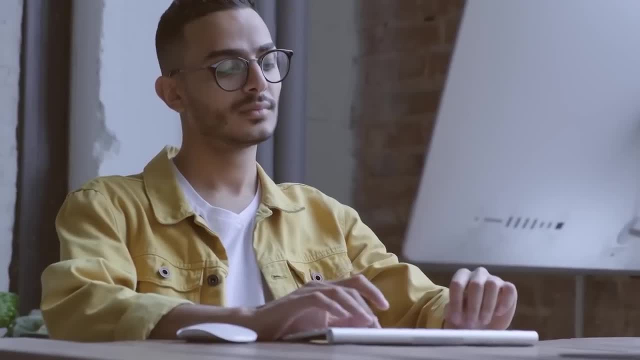 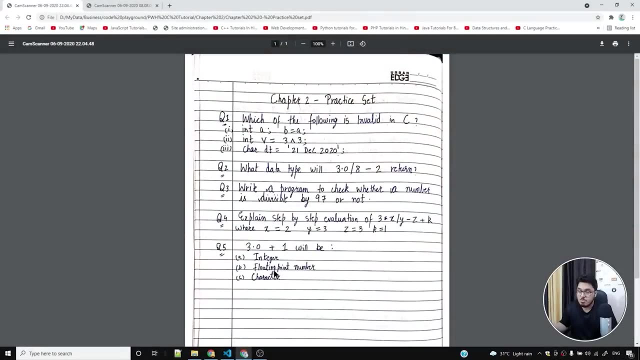 floating point number, so b is the correct answer. i hope you were able to understand all the concepts pretty well, and the moment we, you know, start exploring more and more concepts in this particular course, the basic things are going to be clear, for example: uh, we can, we can do something like: 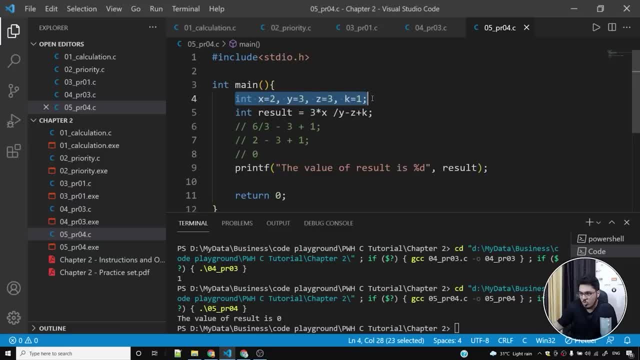 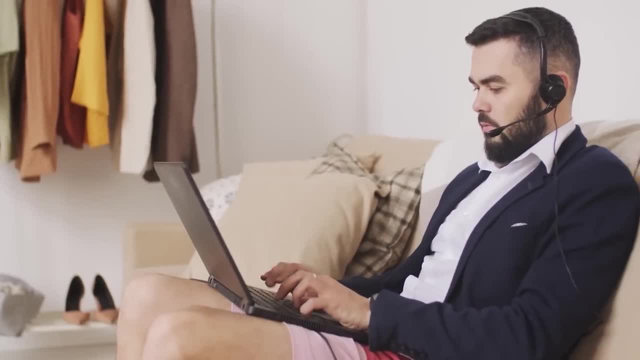 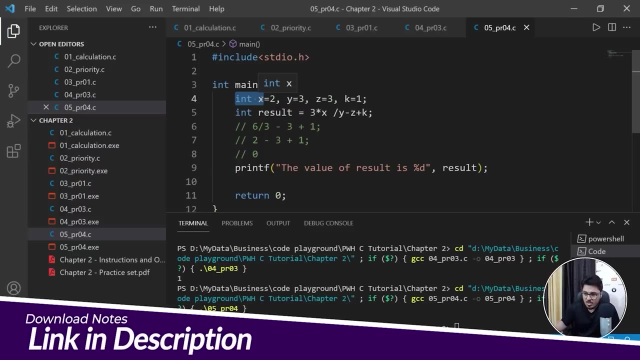 this is something which you know now. we can do something like this is something you know now. you always knew that we can do int x semicolon right, so i am going to do something like this. you know, try things that you know. you can make something like this. but if it is simple then it will take some time, but it is going. 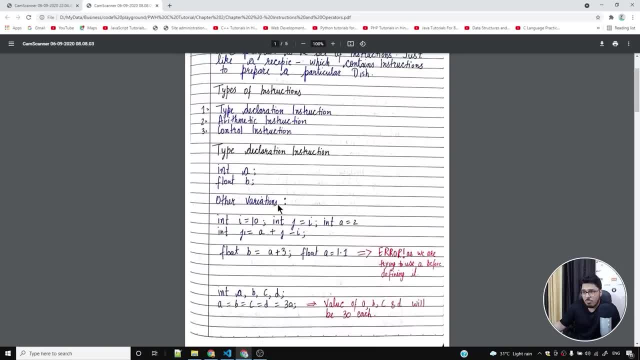 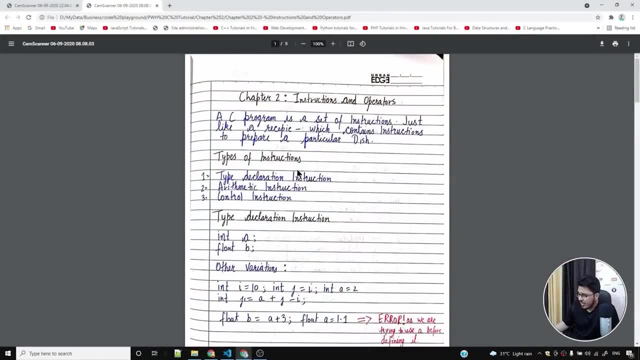 to be easy, so make sure you understand all these things and you. so. all these things are going to make your life easy. all these programs that i'm going to make for you are going to make your life easy when it comes to the revision, so make sure you download the notes, you, you. 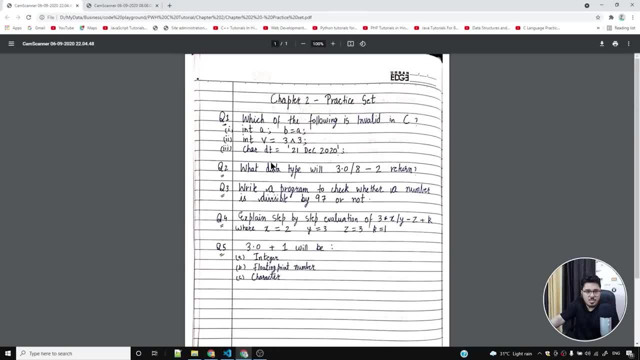 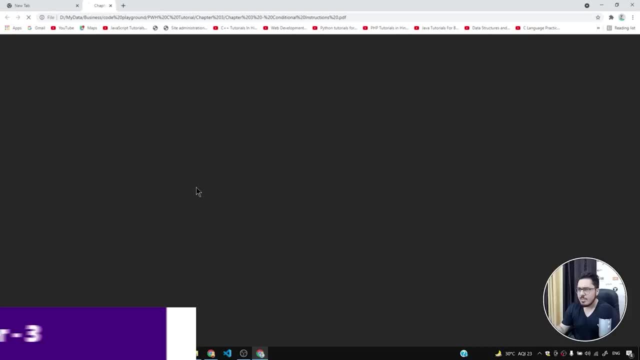 don't know how much hard work i have put into you know, bring these notes for free for all of you. i would appreciate if you download it and we have some good idea of the c programming language. let's move towards chapter number three. i'm going to open this pdf that i've created for you and let's see what this pdf has to say. so i 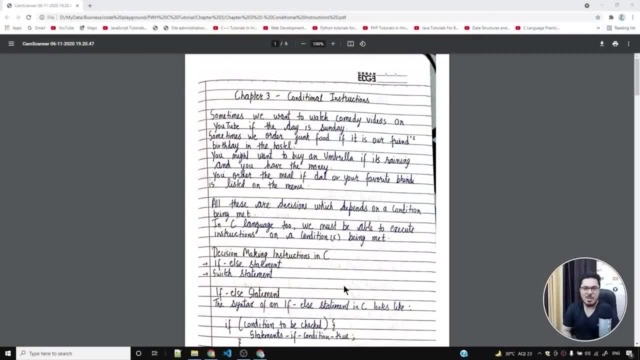 have written some of the lines which will sound a bit fun and it will make things easier to understand for you. for example, conditional instruction is something that might sound boring, but i have tried to make things interesting. so this chapter is about conditional instructions. what exactly are conditional instructions? most of the computer programs use conditional 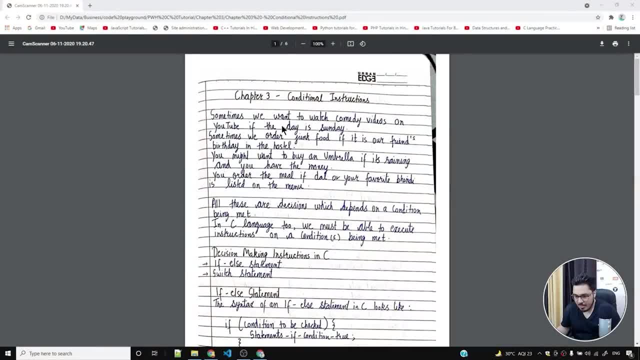 expressions. and what does this mean? they simply mean that whenever you are writing a program, you might want to do something and you would want to execute an instruction only when a certain condition is true. so i've written this. sometimes you want to watch comedy videos on youtube if the 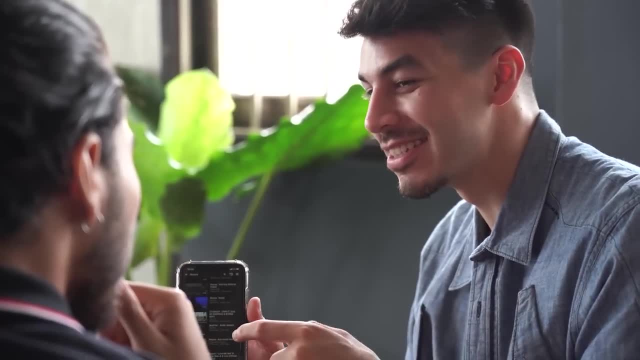 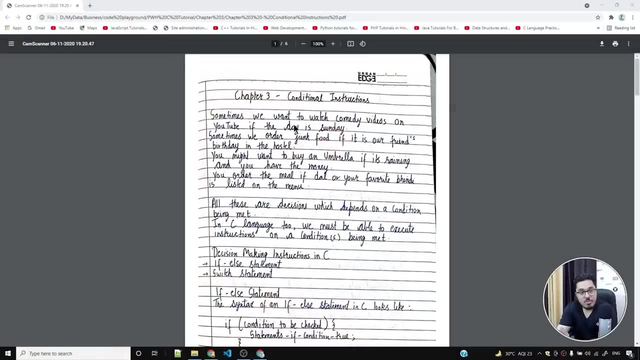 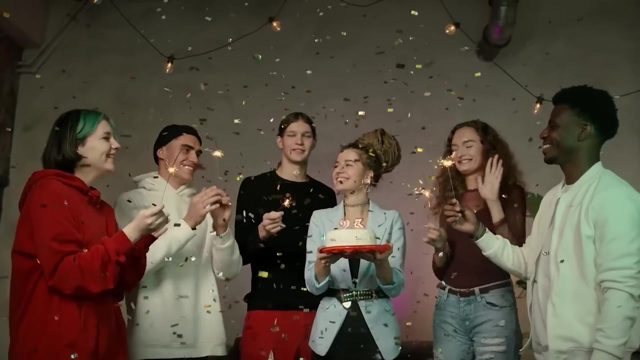 day is sunday. so if the day is sunday, you might want to watch a comedy video on youtube. otherwise, you might want to watch some study videos on youtube. sometimes we order junk food. if it is a friend's birthday, in the hostel you might be dieting year round, but when it's your friend's birthday, or your birthday or some, 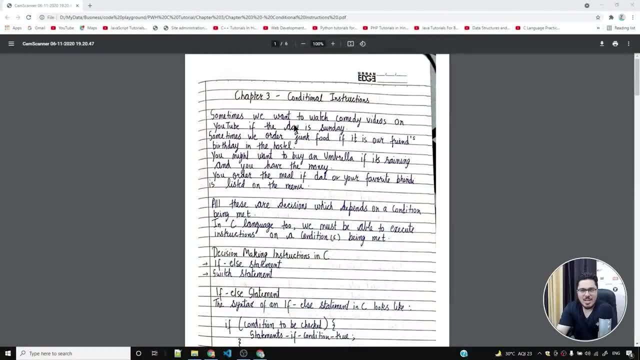 other friend's birthday, you might, you know, ease on your dieting and you might go out and eat some junk food, or maybe order it from outside. so, in all these scenarios, what happens is based off a certain condition. you are doing something based off some condition. you are doing something, you're. 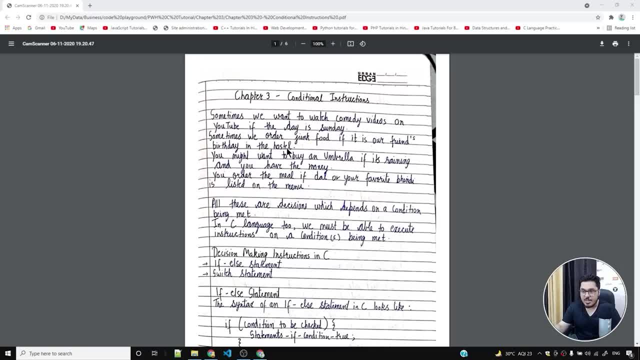 watching comedy video. when the day is sunday, you are eating junk food. when it's your friend's birthday, in the hostel, you might want to buy an umbrella, if it's raining and you have the money. so there are two conditions here: if it's raining and if you have the money. if you have the money. 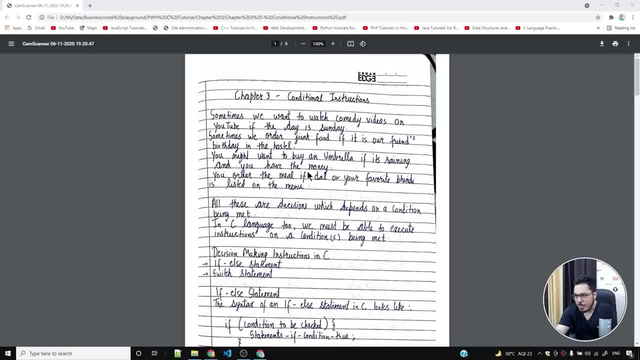 then only you will go and buy the umbrella, otherwise you would not want to buy the umbrella. you order the meal if dal or your favorite bhindi is listed on the menu. so if your favorite food item is listed on the menu, then only you will go and order the meal. okay, so these are some of the 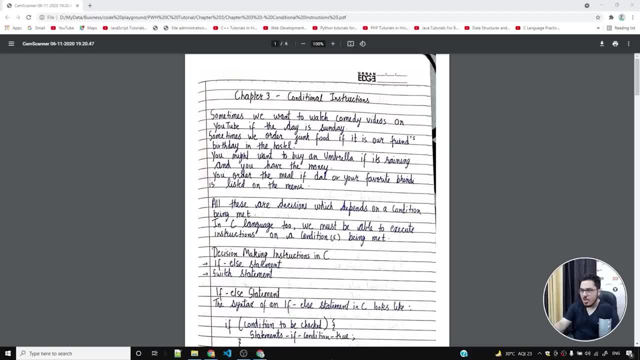 conditions based on which you are performing certain actions. all these are decisions which depend on a certain condition being met. in c, language 2, we must be able to execute instructions on a condition or more than one condition being met. so this is decision making, instruction in c. 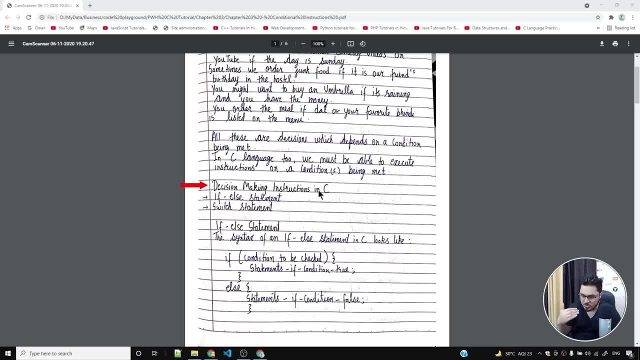 so we have two types of decision making instructions in c. we can use an if else ladder, we can use just an if and also we can use switch statement. so we'll look at if else statements and switch statements one by one. so let's get started by opening this folder in vs code. so let me open this folder in. 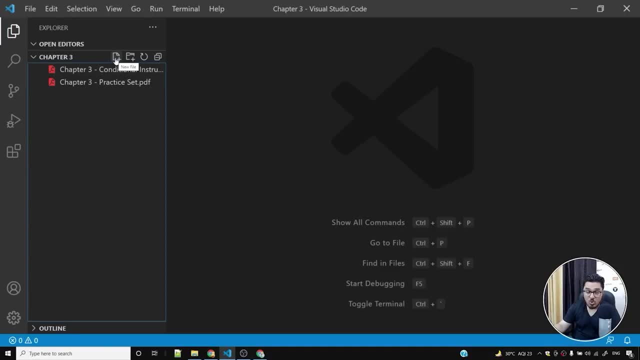 so i'll simply right click and click on open vs code, open in code, and let me write the very first program for you. so i'll simply say, if else, dot c, i'll put the boiler code, boilerplate code, down here and i'll show you something. let us say i have a variable and i'm assigning three inside a. 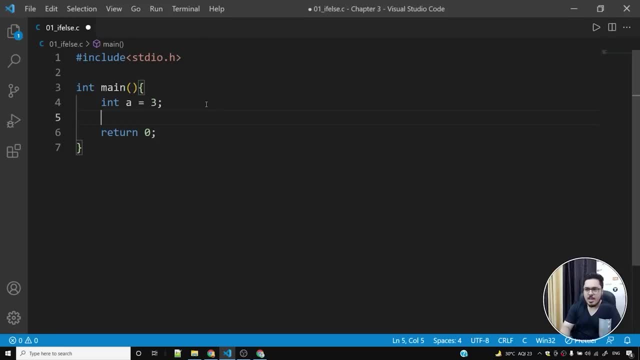 variable, which is an integer, and the name of the variable is a. now what i want to do is i want to check if a is greater than three or other four. it can be either three or four. i want to print: a is greater than four. okay, otherwise what i'll do? i'll do nothing, i'll not print anything, or if i 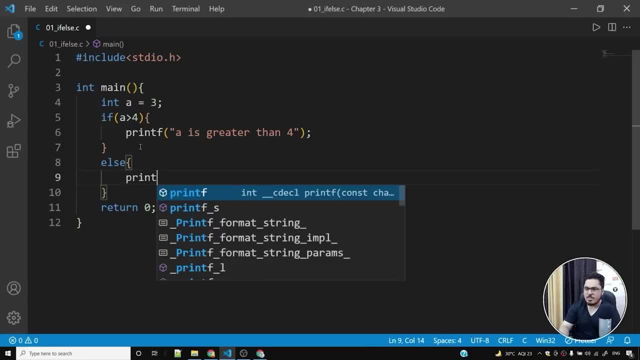 want to print something, when a is not greater than four, i'll simply say: print f, print f and i'll say: a is greater than is not greater than four. okay, so i'll simply do this and i'll press a semicolon, and now what i'll do is run this program and you will see that this program is executed and 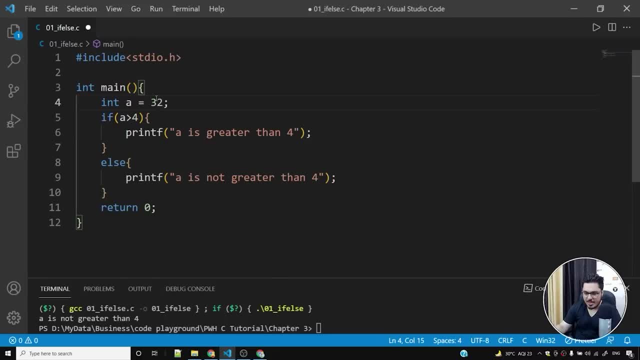 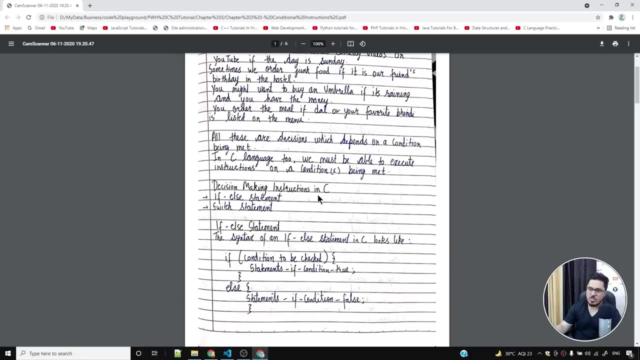 a is not greater than four because a is three. now what if i make a as 32 and if i run it, you'll see a is greater than four. so this is an example of if else, conditional statement. coming back to the nodes, we have another type of conditional or other decision making instruction in c, which is switch. 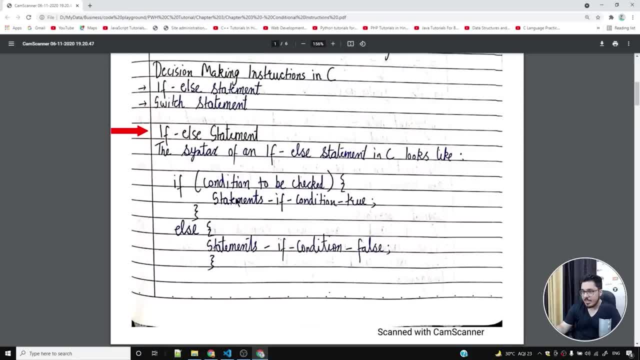 case statement. so we just saw the syntax of if else statement. we simply write condition to be checked inside, if and if that condition turns out to be true, then what we do is we simply write some statements or we write some instructions which we want to get executed. 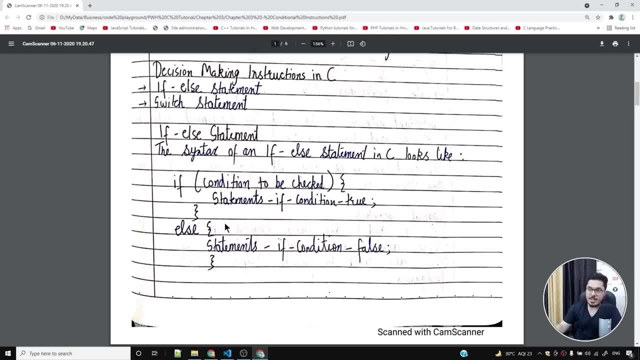 and if that condition is not true, then else is executed. so it's kind of simple, plain and simple english when we write this if else statement: if this happens, do this, else do this. so this is just to make things easier for the programmer. at a very low level these instructions are compiled into 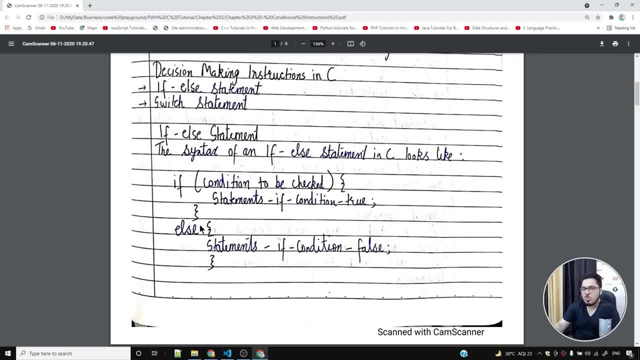 some other instructions which your cpu can understand, but we are not going to go into those details. what we want to do here is we are going to write some statements or we write some instructions. here is we simply want to be able to write fl statements. we want to write some conditions. 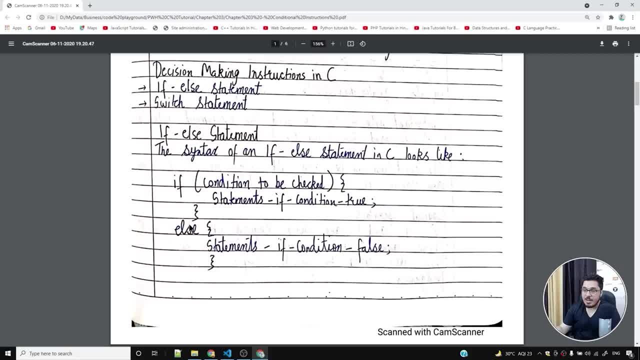 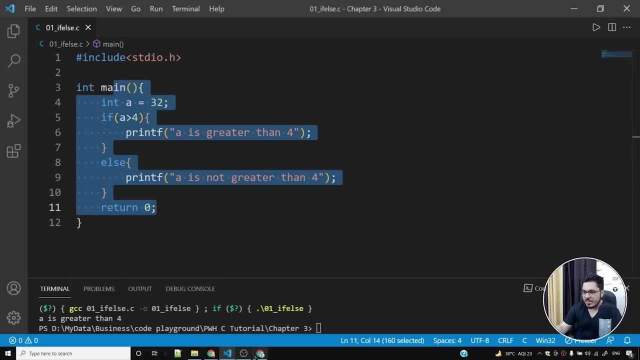 inside c, inside if and whenever those conditions are true, we want some statements to be executed, and if those conditions are not true, then we want something else to be executed. so let's see a code example. just like i show you this example, here we have another example where we have an integer. 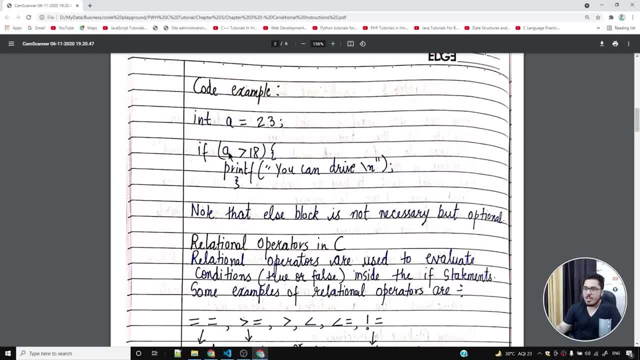 variable a. the value inside this integer variable is 23. if a is greater than 18, we are simply saying, yes, you can drive, otherwise you cannot drive. i don't have any else here and that's totally fine. you can simply have an f without an else. and if that condition is true, then only these statements. 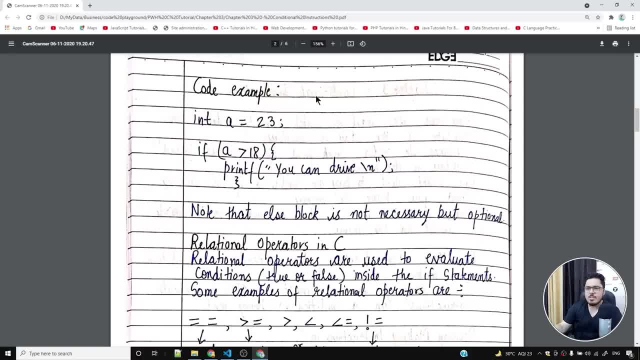 will be executed. otherwise these statements will not be executed. so when i say int a is equal to 23, i can simply say printf: you can drive if a is greater than 18. now note that else block is not necessary but optional. else block is optional. so you can either have else or you can simply have an. 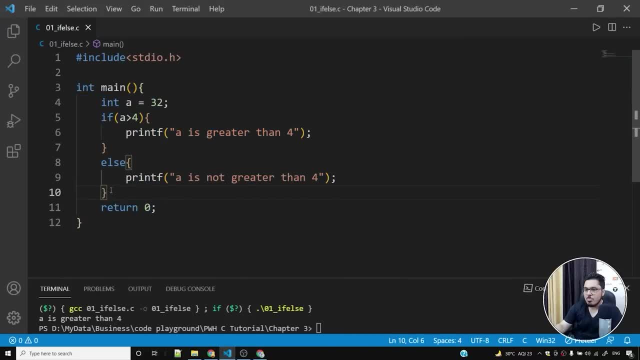 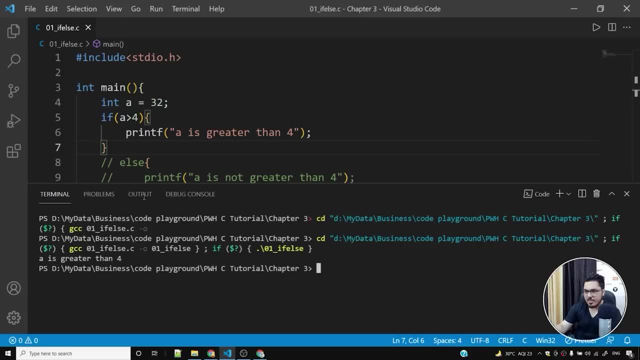 else, and that's totally fine, even from our program. here, if i comment out my else statement, let me show you this program works perfectly. so let me show you the terminal. so a is greater than four and if i make it two, if i save the program and run it once again, nothing happens because i don't have an else. 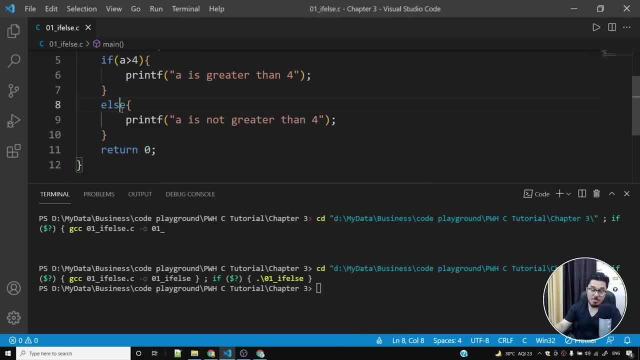 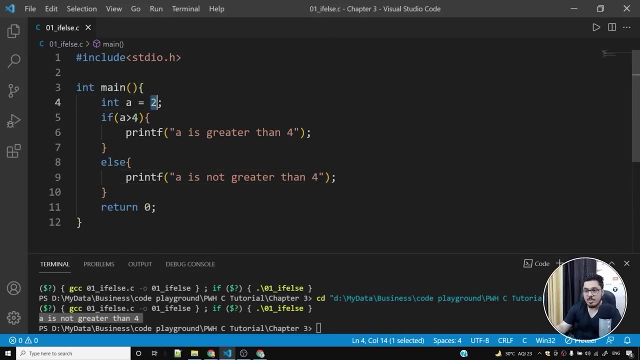 statement here. but the moment i comment uncommented and run the program, a is not greater than four is printed, which means that now a is not greater than four. so i'm actually going to run the program and actually able to check whether the value of a is greater or lesser than a constant which is four. so 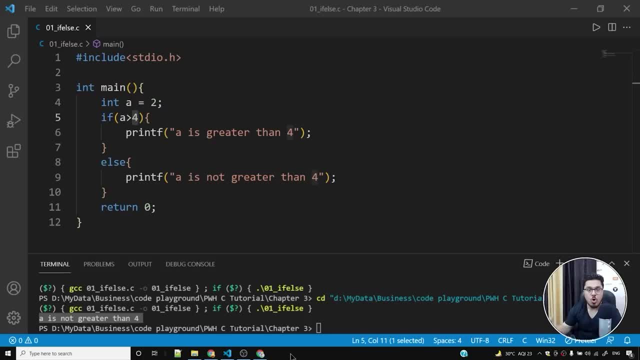 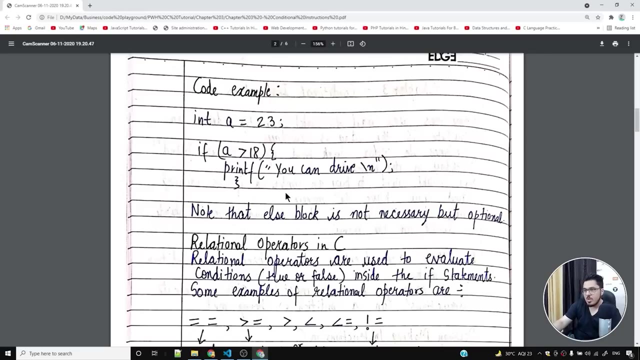 now in c language. i'm able to write some logical things. i'm able to perform some logical operations. i can check whether certain condition is true or not. i can compare a variable with a constant. i can compare two values, which is pretty cool, and we are going to look more into this, so note that. else, 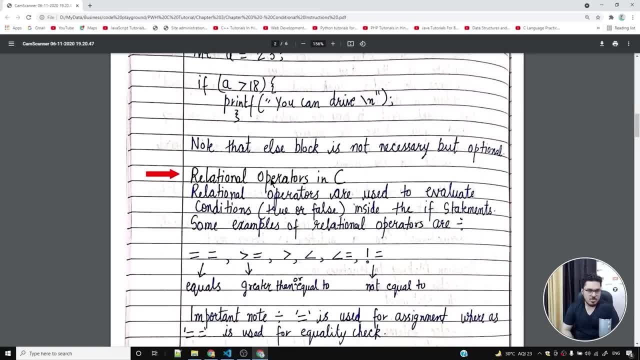 states are mostly simple, but what you can do is go in and tell it to the same logic. i'm going to run this and let's see what happens. so let's see what happens. so let's talk about relational operators in c. what are relational operators in c? so don't get scared by the names of these. 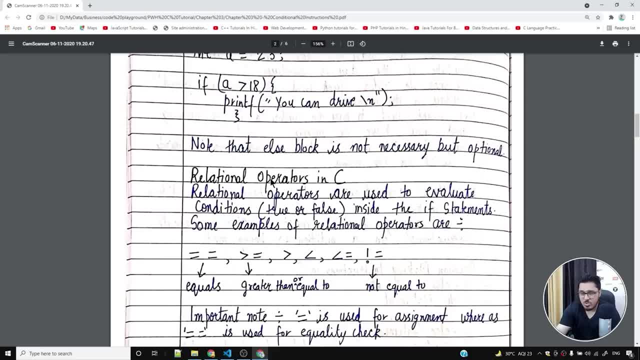 relational operators, logical operators. these are really very simple. let me tell you. just understand the concept behind it. you don't even have to remember down the line which one is relational, which one is logical, because you are going to automatically remember all these things in programming. whenever a beginner comes to learn all these things, what they think is that they will not be able to learn so many terminologies in programming. but believe me, in the alphabets have really good 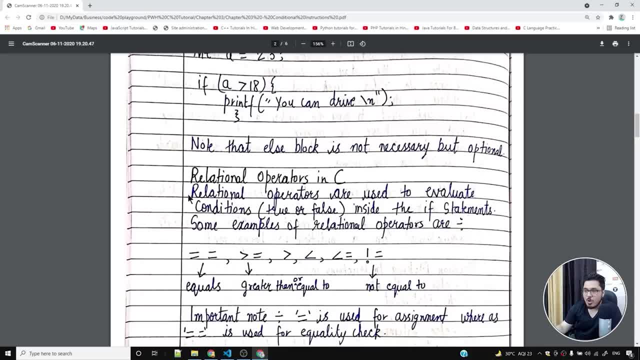 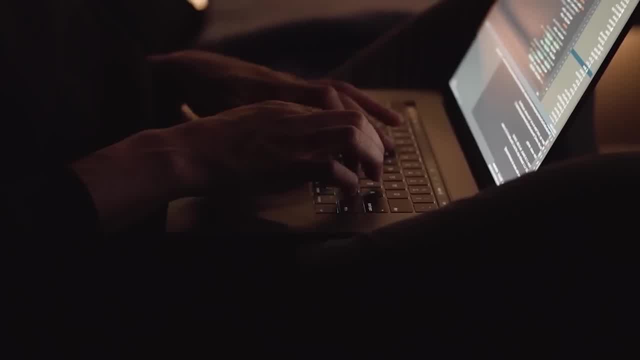 you're going to remember everything by yourself, and at this point, do not focus on remembering what relational operator is, how many types of relational operators are there, but rather practice and write more and more programs. that will get you the programming success that you want. so let's. 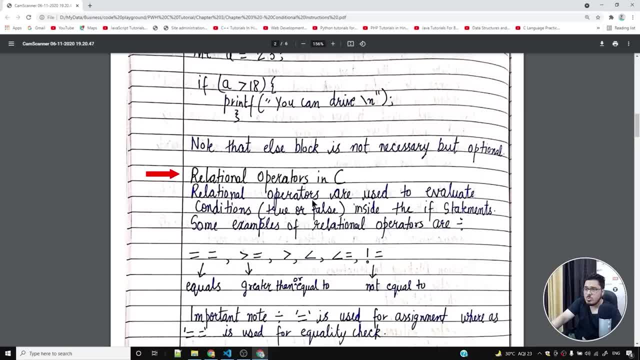 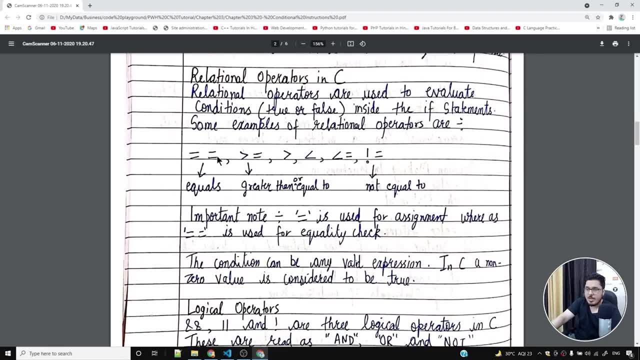 talk about relational operator and see relational operators are used to evaluate conditions true or false- inside the if statements. some examples of relational operators are double equals. to note that this is double equals, it's not single equals. single equals to in c is assignment operator and you don't have to confuse equals to with double equals to. double equals to is a comparison. 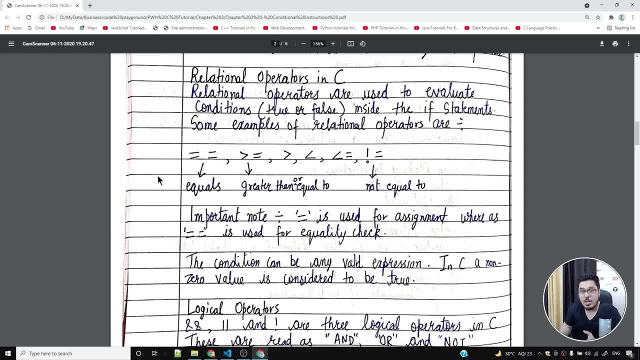 operator which will tell whether two values are equal or not. now, this greater than equal to will tell you whether a value is greater than or equal to some other value or not. similarly, we have just greater than and less than than, less than equal to. not equal to is exclamation mark, and then 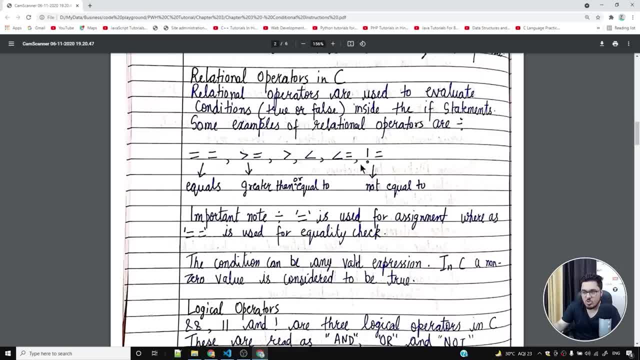 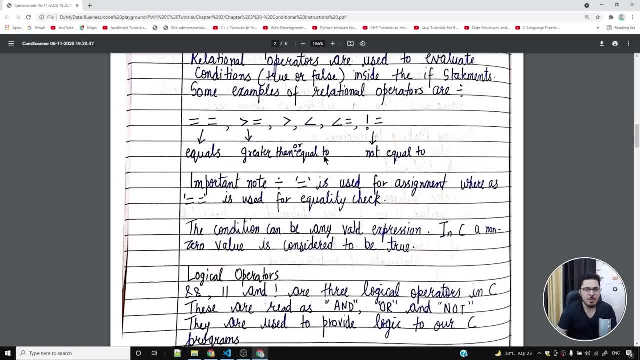 equal to, not equal to is exclamation mark, and then equal to, not equal to is exclamation mark to. so this is not equal to, and this is also something that we are going to use a lot in this course. so you need to remember a bit all of these operators initially, and you don't have to. 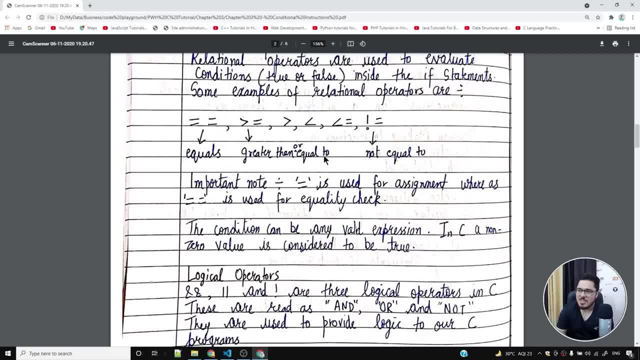 mugify all these things. what i want you to do is just reference these notes and you know, look, look up all these things and once you write few programs, everything is going to sound very, very simple to you. so i have an important note here. equals to is used for assignment where 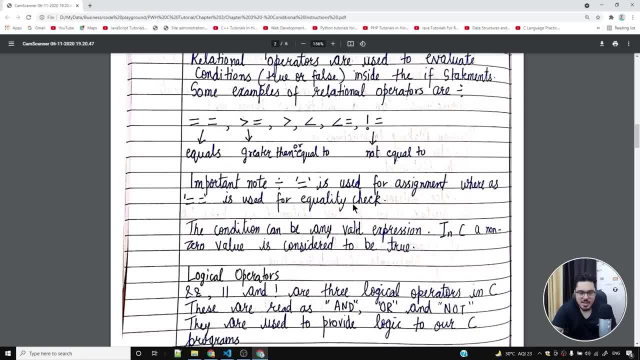 as double equal to is used for equality check. i just told you this that beginners will confuse this double equals to with single equal to, and you don't have to do that. equal to is assignment operator and we have already used equal to here. we, in fact, we just used it in this program into. 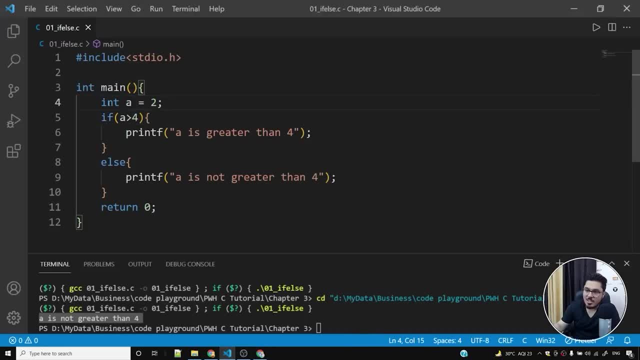 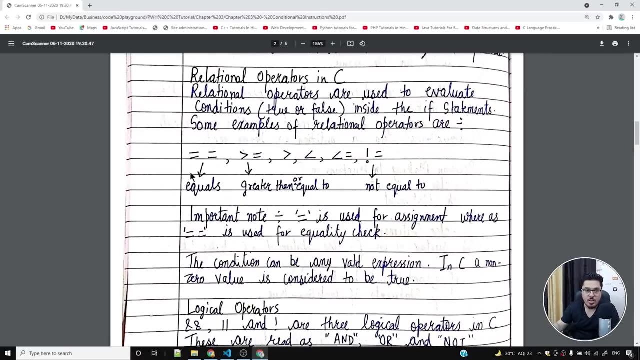 a is equal to 2. here we are not comparing a with 2, but rather what we are doing is we are assigning the value to inside of this variable, a. so you need to understand this. coming back to the notes: double equal to is comparison operator, which will actually tell whether two values are equal to each other or not. now the condition can: 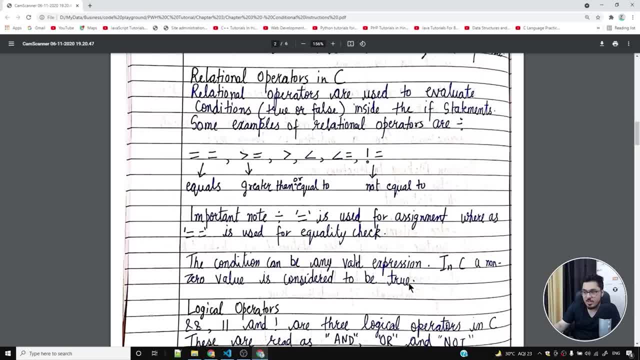 can be any valid expression and see: a non-zero value is considered to be true. this is super important and let me shout here so that you know i can emphasize that this is super, duper important and i'm shouting like this so that i can emphasize enough on this. any non-zero value is considered to. 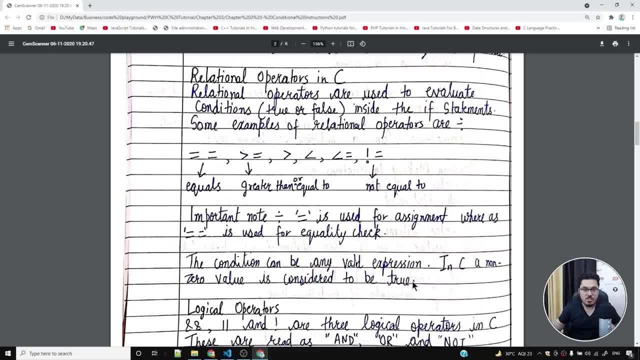 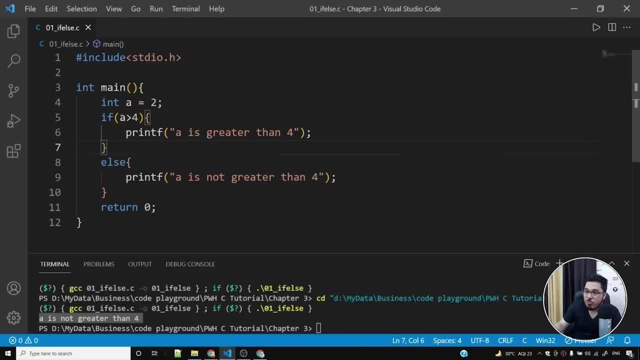 be true in c and you must be thinking why i'm so excited all of a sudden. i want to emphasize on this- you can see that the non-zero value is considered to be true. so even if i put if 1, this is true. even if i put if 10, if 10 is considered as true, whatever is there inside the if block will get. 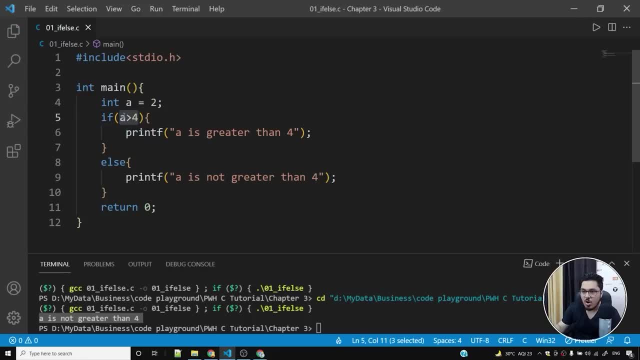 executed. you don't have to have a greater than 4 or, you know, a less than 5 or a double equal to 10. no, you don't have to have to do that, even if you have a non-zero value. if it is a non-zero value. 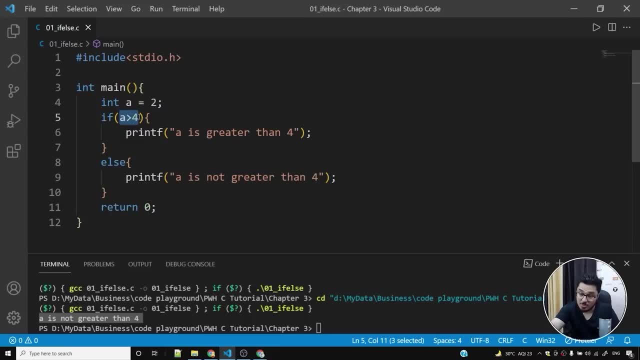 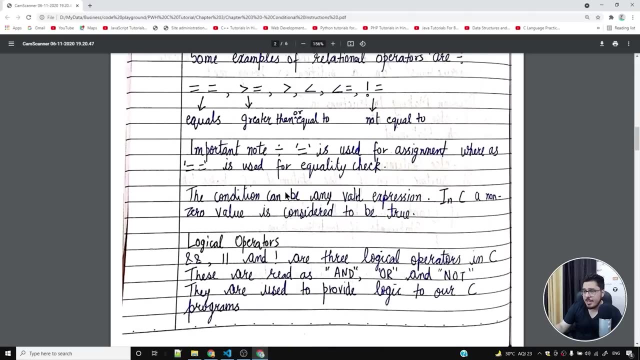 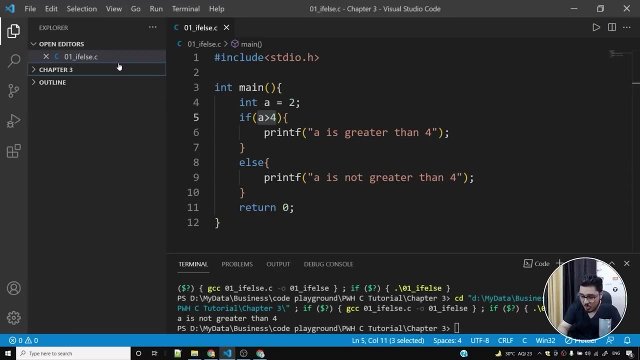 your if block is going to execute for sure. this is something that you need to remember here. now what i'll do is i'll simply come back to the notes and the condition can be any valid expression and see: non-zero value is considered to be true. let me emphasize a bit more, and i know that you'll- 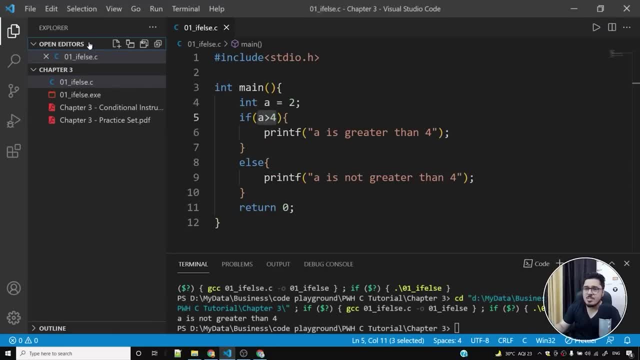 think that why am i emphasizing so much? but this is important and i can't emphasize more on this. let me write a program for you- non-zeroc- and what i want to tell in this program is that if you have a non-zero value and if you write something like this, you can write a non-zero value and you can. 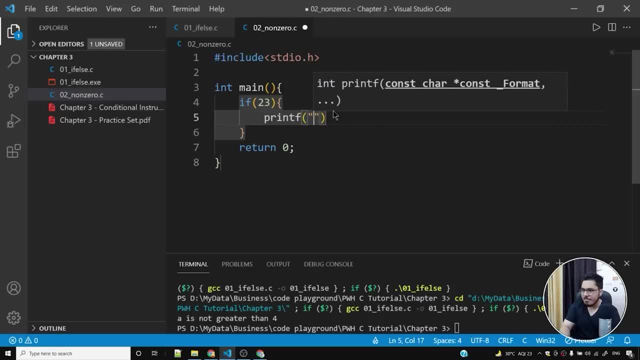 write this printf. by the way, uh, i write programs in python as well, which is why, you know, whenever i type, i just type print. but that's fine, even if you're coding in multiple programming language. evaluated to true, or rather, let me tell, any non-zero value is evaluated to true semicolon. 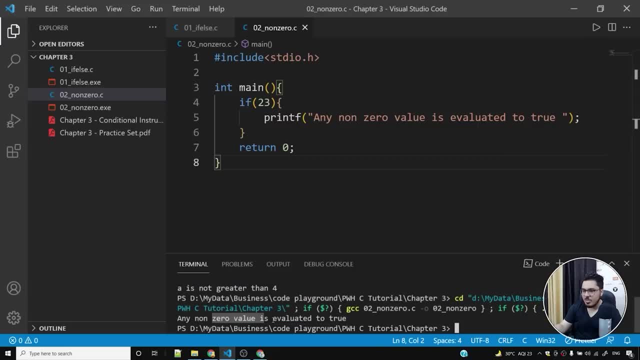 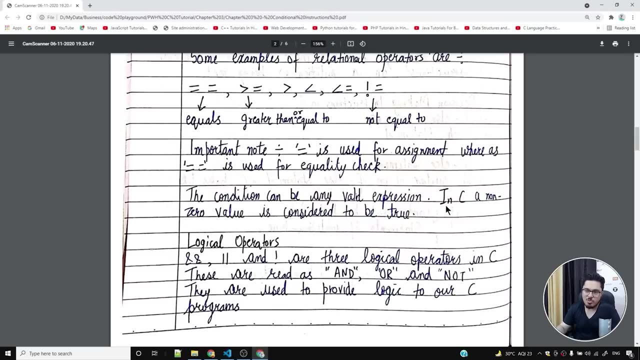 save and if i run this, any non-zero value is evaluated. true, this is something that you need to know, and a lot of people will tell me: why are you emphasizing so much? you have written it in the notes, you have told it several times, but this concept is very important, which is why i have 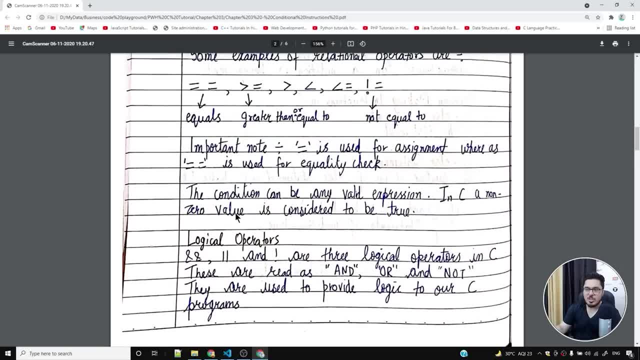 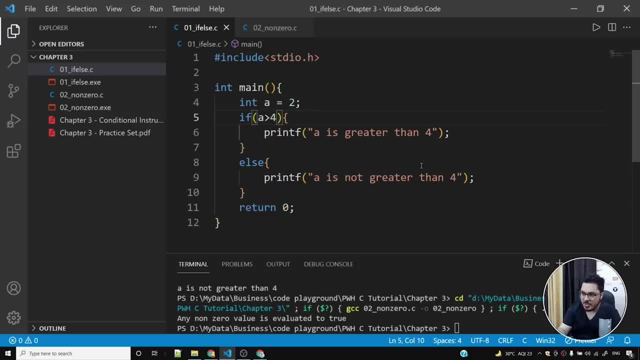 to emphasize it this way, let's talk about logical operators now. we just talked about relational operators and i hope that you will understand, uh, what relational operators are. just try out these operators: greater than equal to, less than less than equal to. i think this is pretty straightforward and you don't have to, you know, rather, i don't have to show you each and every. 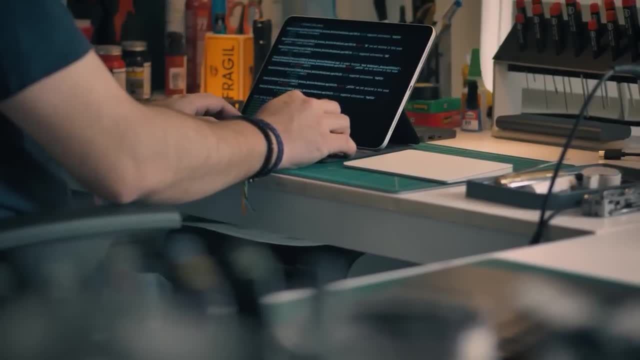 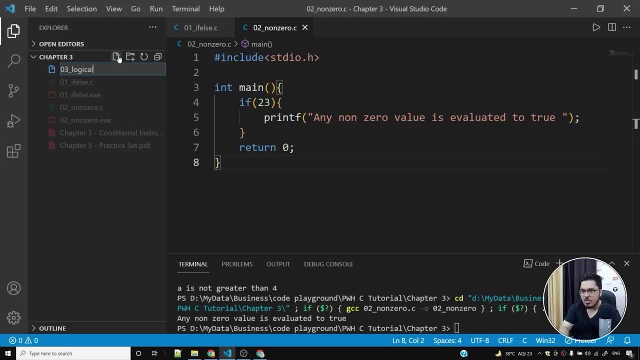 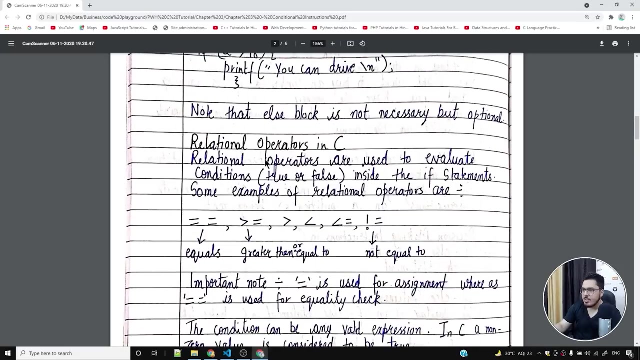 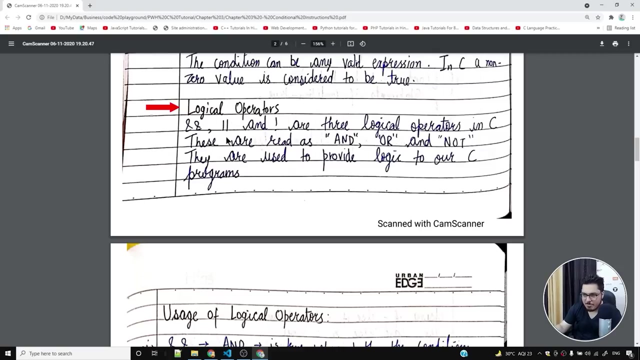 operator inside of if statement. i hope that you will practice all these operators yourself. now let's write another program and we are going to talk about logical operators in this program. so let me write a boilerplate code and let's talk about logical operators. double n, all and exclamation mark. this is actually a pipe sign. double pipe- this is double. 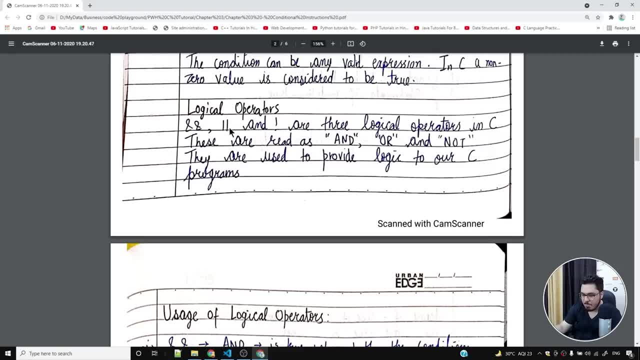 end. this is double pipe, in case you are wondering where is pipe in your kitchen, so let's do that. where is pipe in your keyboard? let me show it to you. can you see this key, this key, this one? this is the pipe. okay, i know that it sounds really crazy me holding the keyboard, and you know. 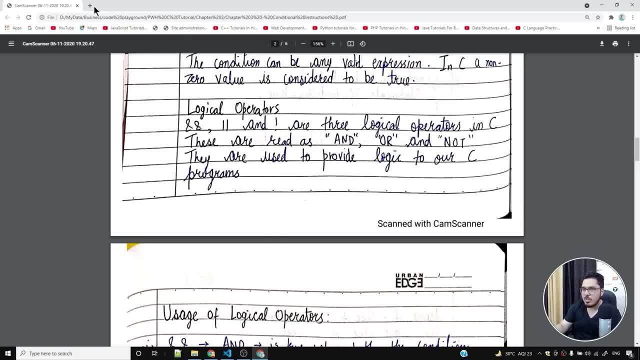 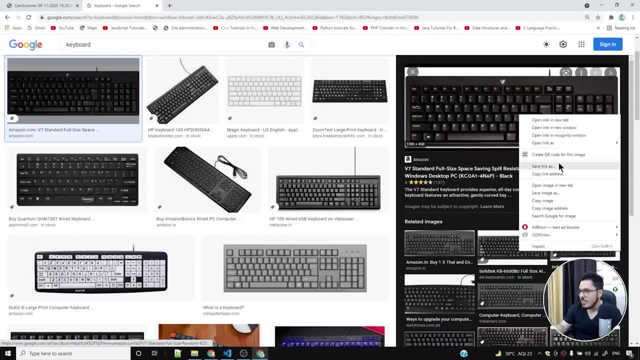 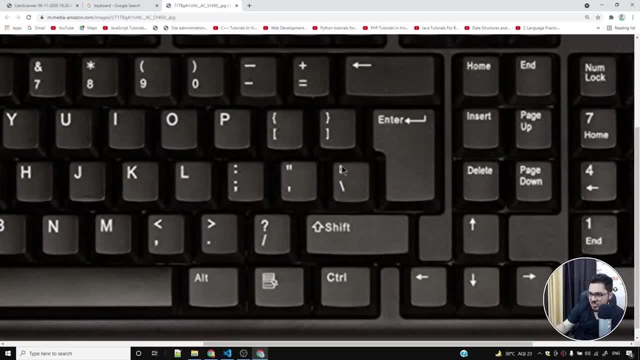 holding it in front of the webcam. but i hope that you understood. let me google keyboard and i think this is a better way of showing the pipe key. so if i open this image, this is the pipe key, this one. oops, let me scroll this one, so you'll have to press shift and then you'll have 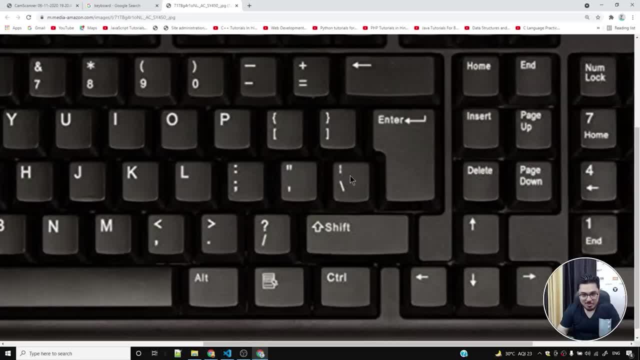 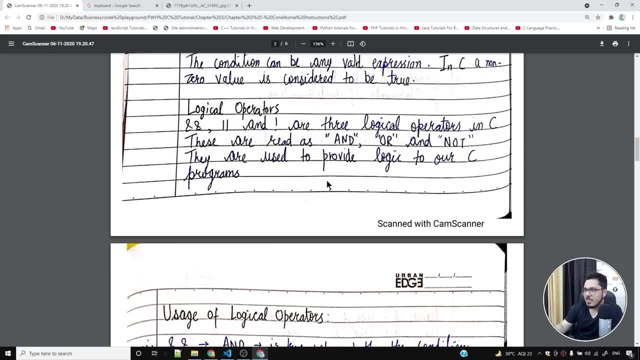 to press this key and this will give you a pipe. this is something that you might not have used a lot while you are typing, or maybe surfing the web or doing anything in the computer, but when you're programming, you will use this a lot. so let's talk about these logical operators at a very high level. 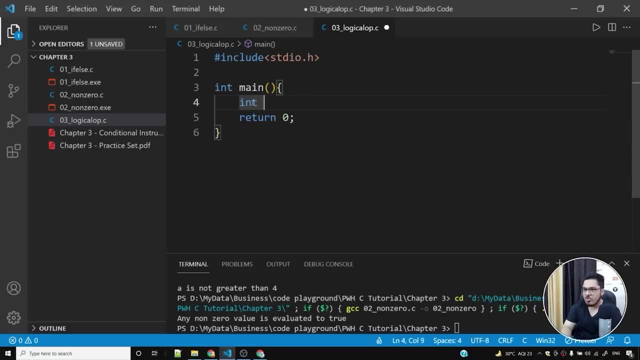 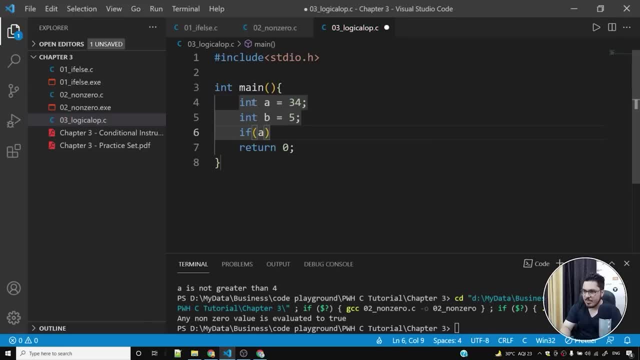 equal to 5. what if i say: if a is greater than 7 and b is less than 4, let me show you how this works. i'll simply say yes. okay, so if this happens, i'll simply say yes. otherwise, i don't want to say no. 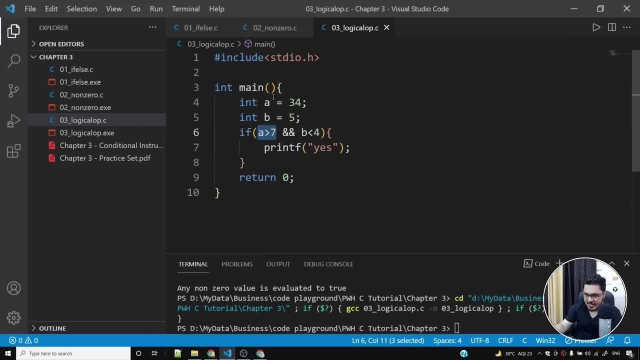 i'll simply say yes. so if a is greater than 7, is a is greater than 7? no, a is not greater than 7. is b less than 4? no, b is not less than 4. it's actually greater than 4, which is 5. so both these conditions are false. this is false. 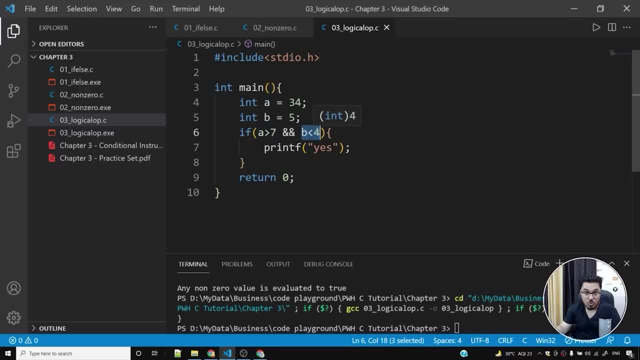 this is false. false and false is false. okay, now let's make things a bit interesting here. let me make this two so. one of these conditions is true. a greater than 7 is false. b less than 4 is true. false and true will evaluate to false. okay, so a is greater than 7 is true actually. uh, my bad, a is greater than 7 is true. 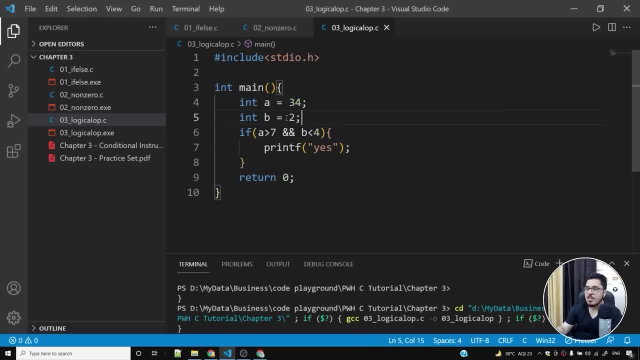 and b is less than 4 is also true now. so b is also less than 4, 2 is less than 4 and 34 is greater than 7. so both of these conditions are true now. so true and true will evaluate to true. but if i make one of these conditions as false, it will not return yes, but if i make it 2, it will return yes and uh, i know that this is a bit confusing at this point, so let me explain this to you in greater detail, and that's why i've written these notes for you. okay, so we have three operations to write, so let me write the. 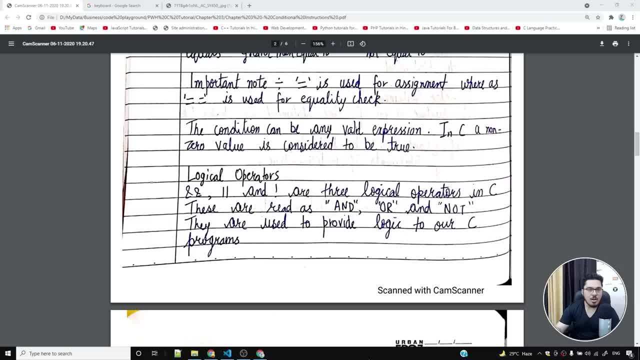 operators and or and not. these are the three most used logical operators: and or and not. now, what we'll do is we'll simply use it in our programs. these operators are read as and or and not. they are used to provide logic to our c programs. okay, so that's why they are called. 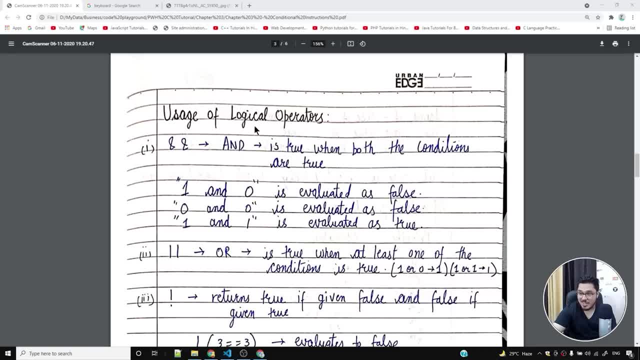 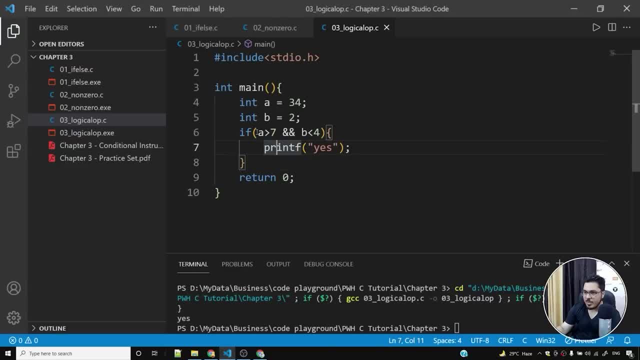 logical operators and i have put them down in the notes really very well, and let me tell you what i mean when i say that. so this is the and operator. we have used this end operators on two conditionals. okay, so these are two values which will evaluate to either true or false. 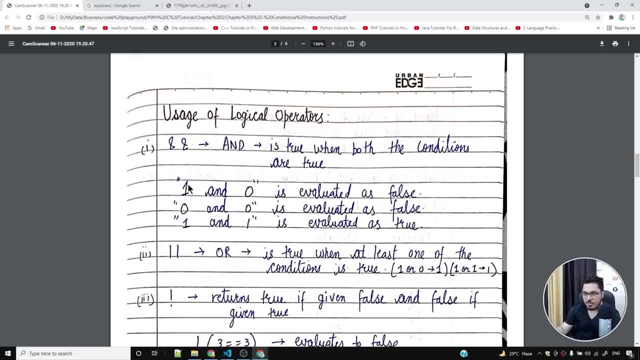 now, what we are doing is we are operating on one and zero, so let's talk about end operator. it is true when both the conditions are true. so if you say true and true, it will be true. otherwise, it is going to be false. if you have true and false, it will be false if you have. 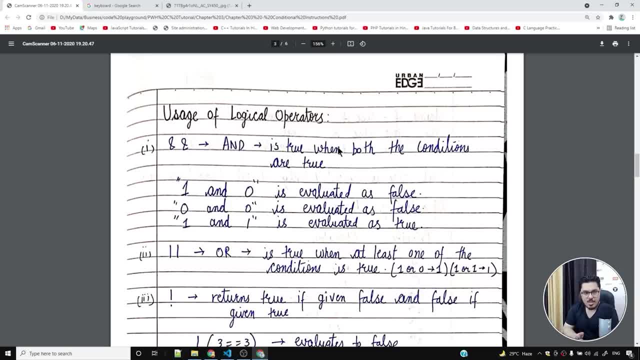 false and false? definitely it will be false. if you have false and true, it will be false. so one and zero is evaluated to false. by the way, one is true in c- any non-zero value is true in c and zero is false in c. zero and zero is evaluated. 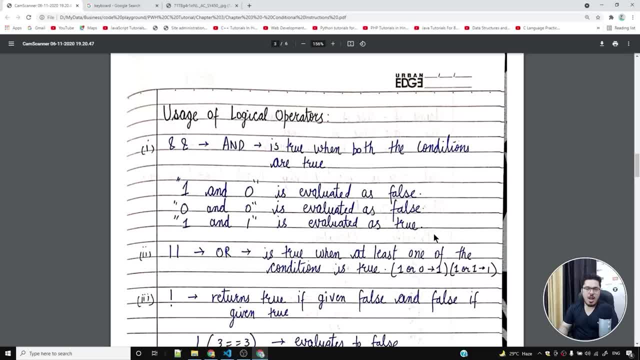 to false. one and one is evaluated to true. and even if you think about it from the language, the english language perspective, just think about it. when you say i want this and this, it means that you want both the things, doesn't mean that you want one of these things. so whenever, 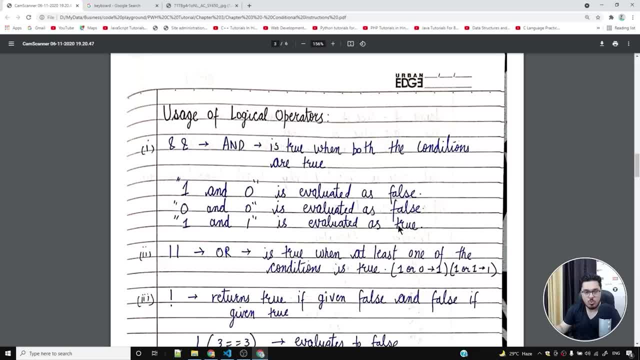 you have one and one, then only that condition will be evaluated to true. if i say that you are a good boy and you live in new york, so you will have to be a good boy and you will have to live in new york for this entire statement. 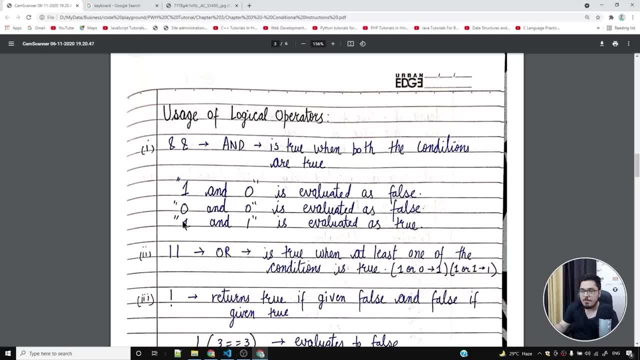 to be true. so both of this, both of the operands, should be true. when i operate these two operands with end, both of these operands should be true. both of these conditions should be true: you should be a good boy, you should live in new york. then only this entire statement is going to. 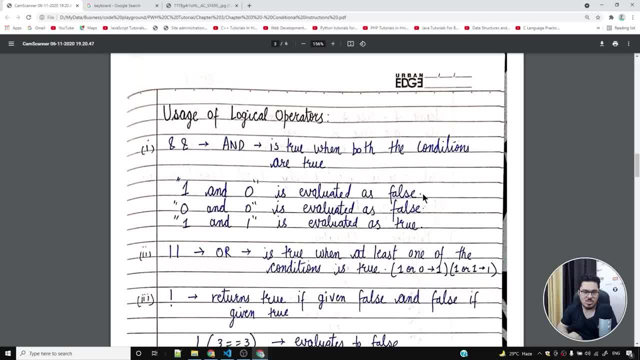 be true. if you are a good boy and you don't live in new york, then only this entire statement is false. if you, if you don't live in new york, if you live in chamoli and let us say, then i say that you are a good boy and you live in new york. no, you don't live in new york, you live in chamoli. 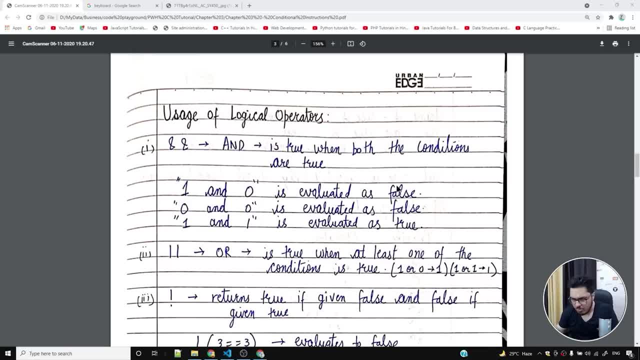 so the thing is that this entire statement is going to be false. so one and zero is evaluated to false. zero and zero is evaluated to false. one and one is evaluated to false. now that we have spent so much time on and operator or operator is going to be super clear to you. or means choice. 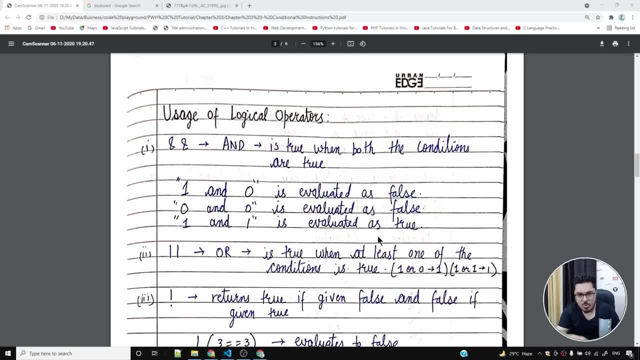 what would you like to have? we have two options. either you can have chapati or you can have rice. you can have these two things. what do you want to have? so you can have either chapati or rice. you can't have both of these. so if you're going to a mess- and they are- they tell you that, uh, you can either have chapati or 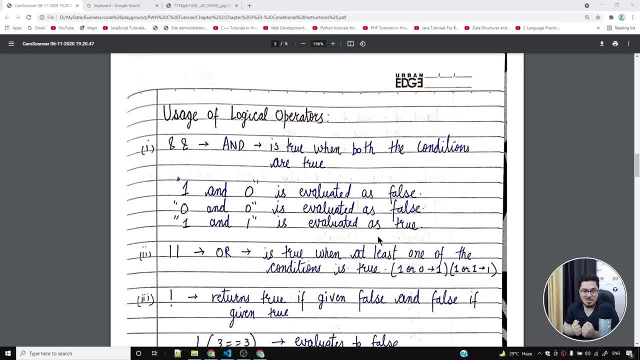 you can have rice. what do you want? so you cannot say that i want both of these things. no, they're not going to give that. either they'll give you chapati or they are going to offer you rice, based on your choice. in a very similar way, if you say true or false, 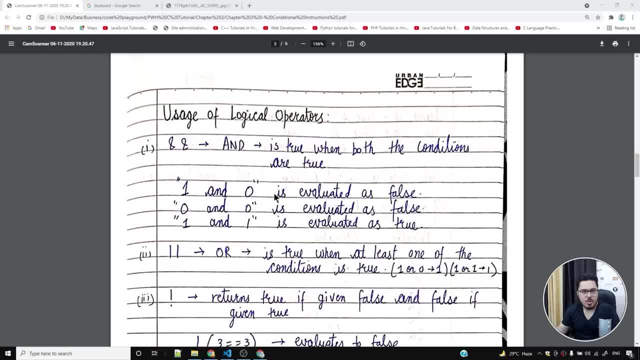 one of these conditions is true, so it will evaluate to true, false or true. one of these conditions is true, so entire statement will be evaluated to true. but if you say false and false, that will be false, okay, so or operator will evaluate to true when it is operated on one. 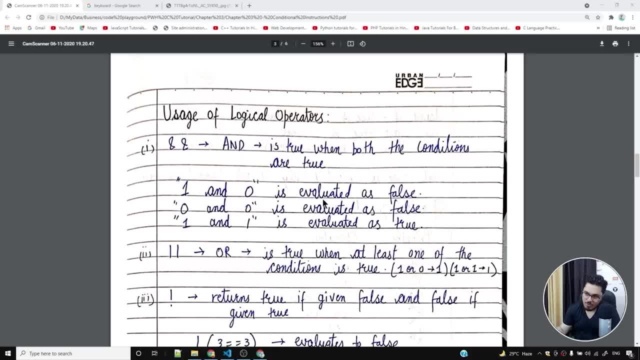 or zero, one or one, one, zero or one, but if we have zero or zero, it will be evaluated to false. rest of the things will be true. so zero or zero is false, rest is true. okay, i hope that i'm able to explain this pretty well. now let's talk about not operator, and not operator is important because it will simply. 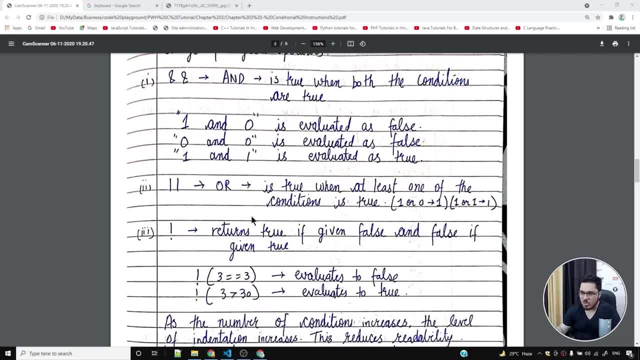 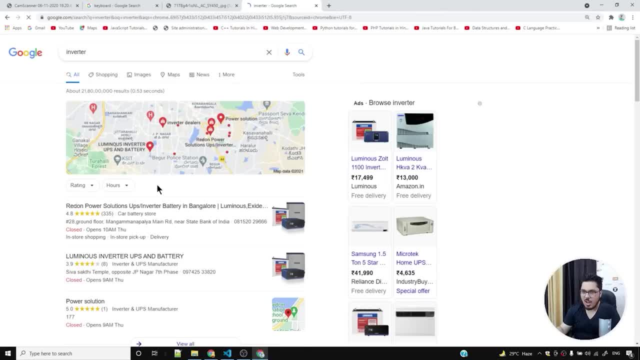 invert true to false and false to true, so this is also called an inverter. this, not operator- is called an inverter. and no, i'm not talking about this inverter. no, this i'm not talking about this inverter. no, don't, don't confuse it with this inverter i am talking about. 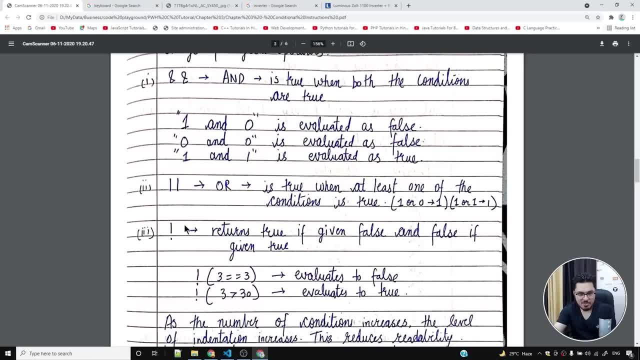 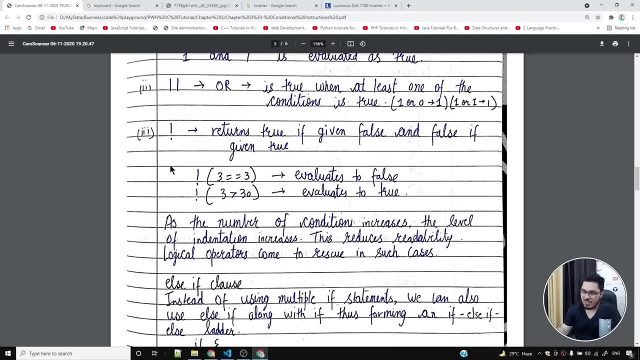 inverter. inverter means something which can invert, which can make true as false, and false is true. okay, so this is going to return true if it is supplied false and if you supply true to it, it will return false. as simple as that. i hope that, uh, this makes sense now if i say not of 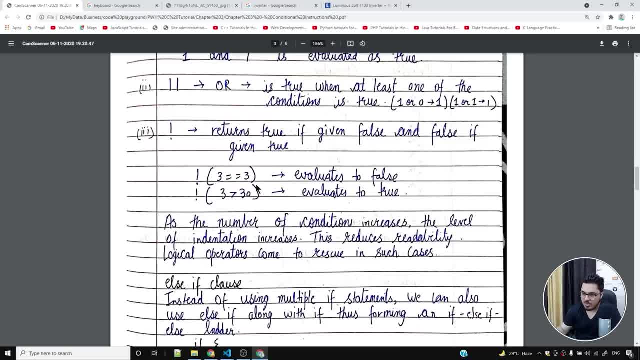 three double equals to three. so you'll have to evaluate this first. three double equals to three is actually true, because three is equal to three, and when i'm saying double equal to, i mean three equal to three or not. yes, it is so. this is true, but not of true is going to false. uh, is going. 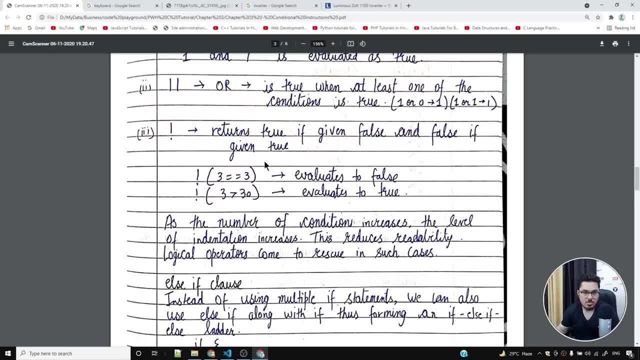 to be false because not operator is an inverter, so this entire thing will evaluate it to false. now, if i say three greater than 30 and i put a not outside of it, three is not greater than 30 so this thing is false. but since we have a not operator outside of it, this is going to evaluate. 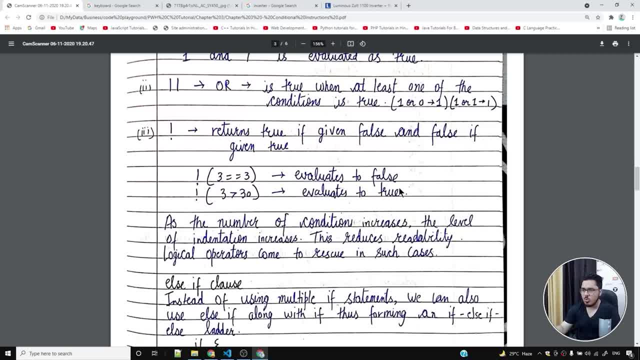 to true. i hope that this makes sense to all of you. as the number of conditions increases, the level of indentation increases. this rate is going to be true. so this is going to be true. diagnosis reduces readability. logical operators come to esq in such cases. and let me tell you what. 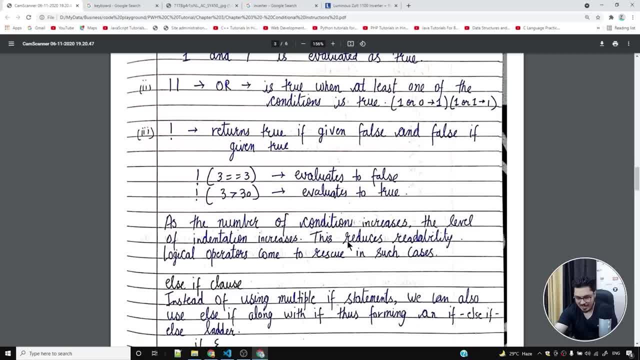 i mean by this statement. so let us say, you have a, you have an if statement, now you have another if statement inside that if statement and then again you have another if statement inside that if statement and you keep on going. so what happens is your program will start from here and you will. 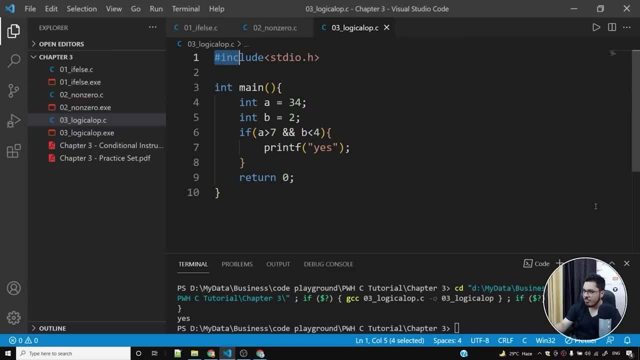 find your program going here, because you will have if, if, if, if, if, if, and you will, you know, keep on indenting, keep on intending until your program starts from here. you know the j para type, not your error number. so let's first look at the log number and then your fleet. so what we have here, which is: 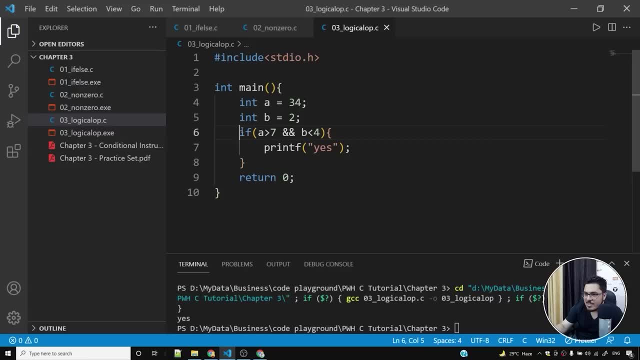 program looks ugly. so what you will do is you will want to write something like this, and that will actually give a better logic to your program, and we are going to use these logical operators in the practice set. so, in case you are not able to understand this, you will have to just wait for. 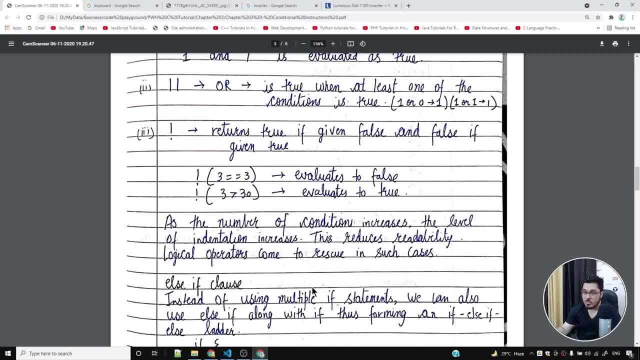 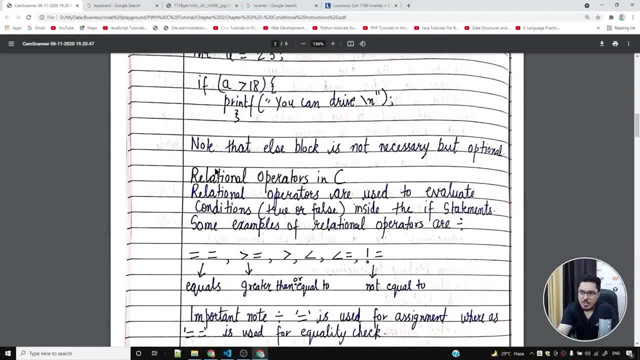 the practice set and listen to these concepts, download these notes, read about all these operators. i know if you are a beginner it might be little bit difficult to wrap all these concepts around your head. but again, i can assure you that by the end of this course you are going to 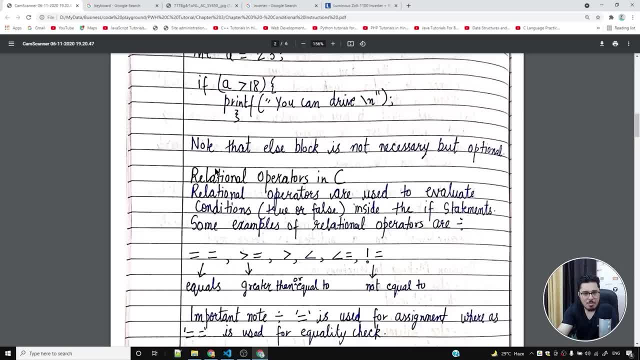 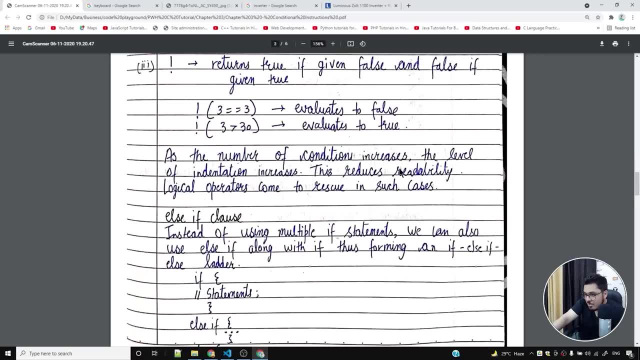 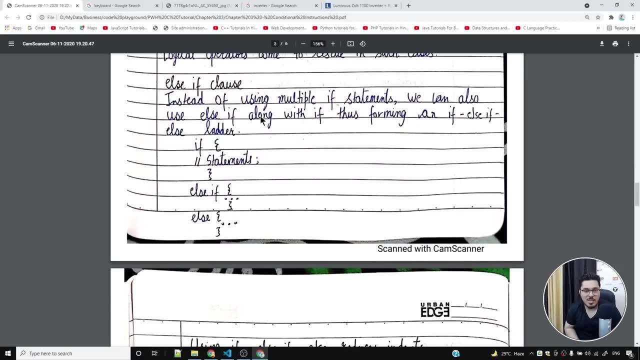 have each and everything, including pointers, dynamic memory allocation, crystal clear in your mind. this is the guarantee. so let's move ahead with this guarantee and, as the number of condition increases the level of intention we just talked about this, let's talk about else: if clause, something that we have not yet talked about, else, if, what is this else if we talked about, if we? 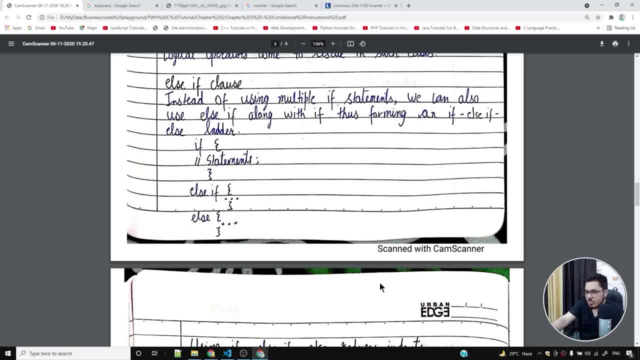 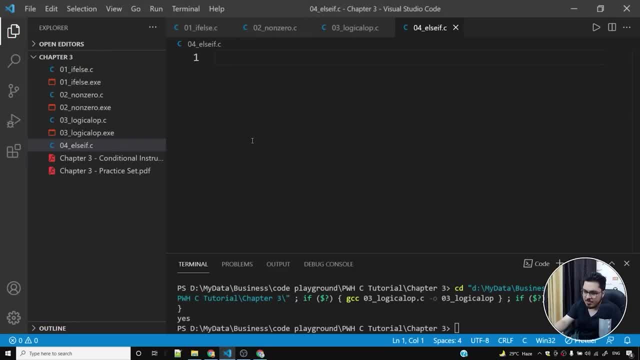 talked about else, we didn't talk about else, if okay, so let's, let me show you a scenario. let me create a program for you. i'll call it else, if dot c, i'll put the boilerplate code. what if i say: if a is greater than five, let me, let me, let me say: in age is equal. 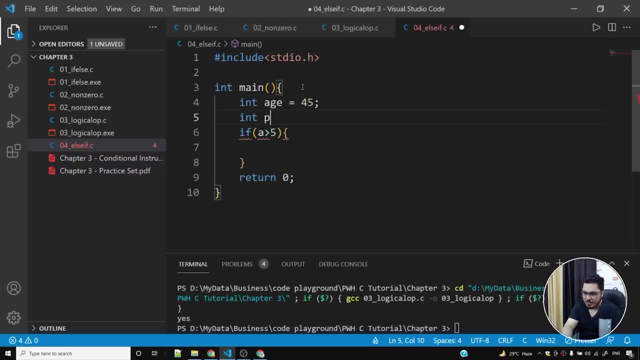 to 45, and let me say int place code is equal to 12. let us say we have 12 places and a person can have a place code where he has got his passport. okay, now what i want is i want to say if a is greater than five, if a is um, or rather if a is greater than 18, if a is greater than 18, then what? 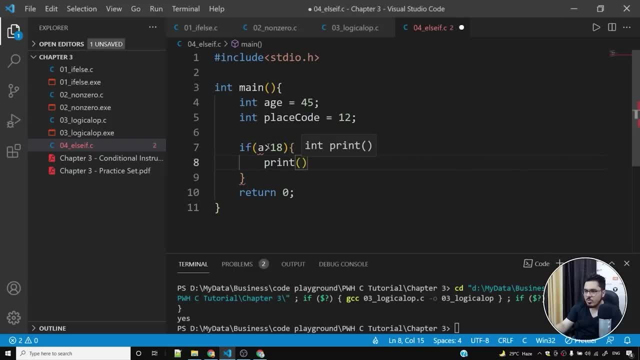 you do. is you simply print? sorry, i should write age. if h is greater than 18, you simply print: you are eligible to drive. okay, you are eligible to drive, else if age is not greater than 18, so i'll say else. if so, i'll have something inside here. 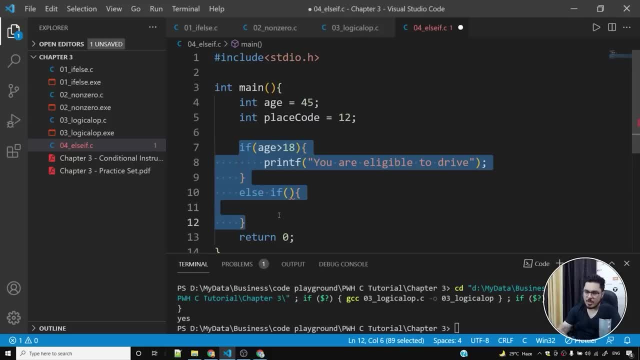 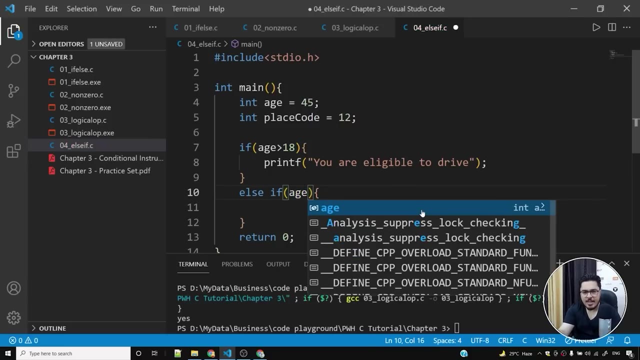 and let me explain you how this is different from a normal. if else, okay, so let me write it down first and then i'll explain it to you. so if age is greater than 18, then you do this. else, if age is, if age is not greater than 18, then definitely age is less than 18. 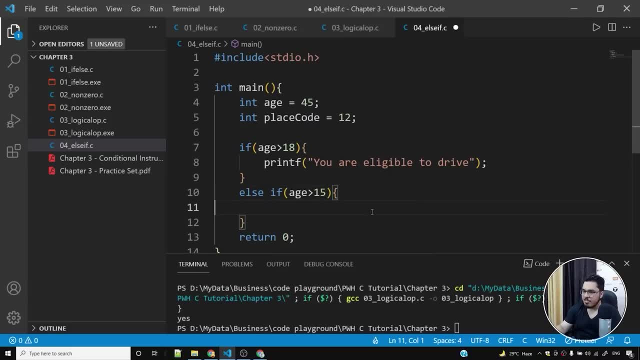 we'll check if age is greater than 15.. we'll simply say: you are eligible. you are not eligible to drive. you are not eligible to drive, but we will check for a toy vehicle for you. okay, we can do something like this. so let us say we have, uh, 12 places and inside all these 12 places we have some toy vehicles on rent. 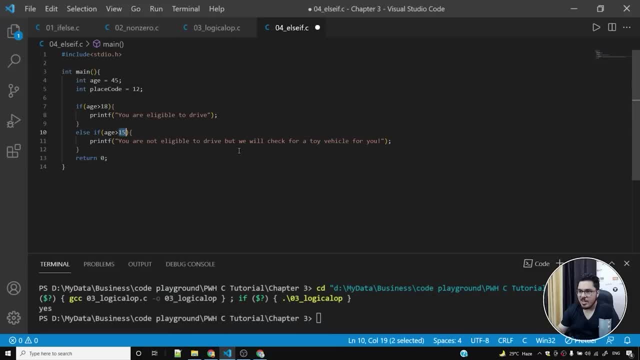 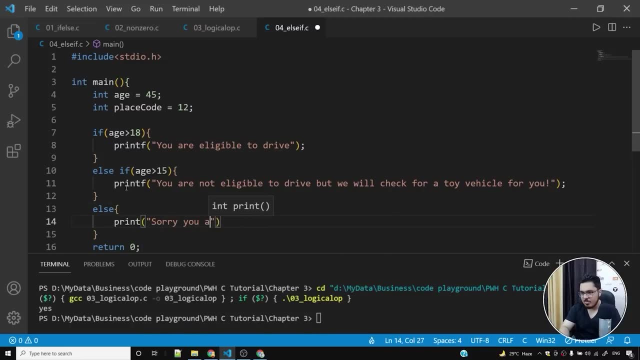 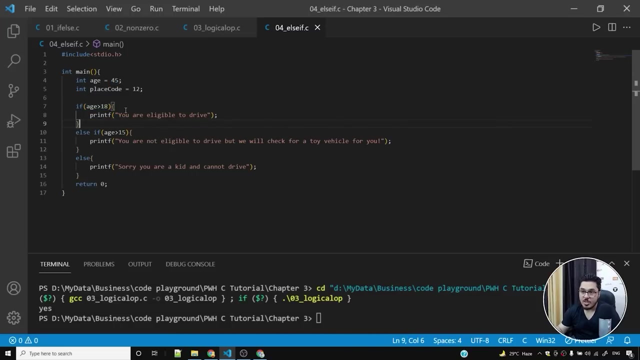 which people with age greater than 15 can drive. okay. now what i can do is i can simply say else: sorry, you are a kid and cannot drive, okay. so now if i run this program, so the age is 45, so what will happen is this thing will get executed first and this condition will be checked for. that, so is age. 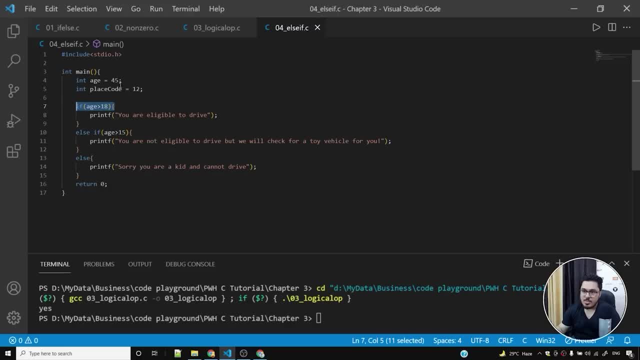 greater than 18 or not, the answer is true. since the answer is true, this will get executed. and since this is executed, this will not get executed. this will not get executed. so what i mean to say by this is that this entire thing is one single entity. this is one single entity, and what does it mean? it simply means that either this or this or 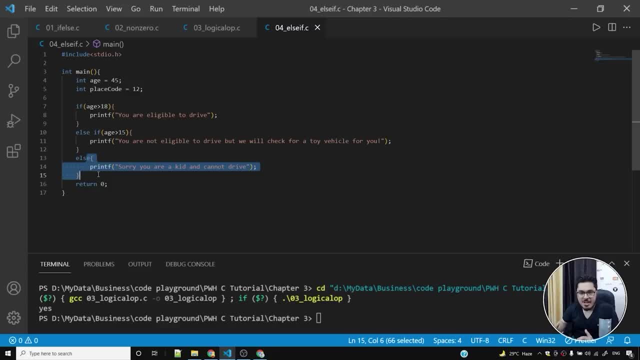 this will be executed. but if we have- only if- statements, all those conditions will be checked. so let me create two scenarios for you. so this is scenario one, and let me also create another scenario for you, and we'll compare these two scenarios. so what i'll do is i'll simply comment. 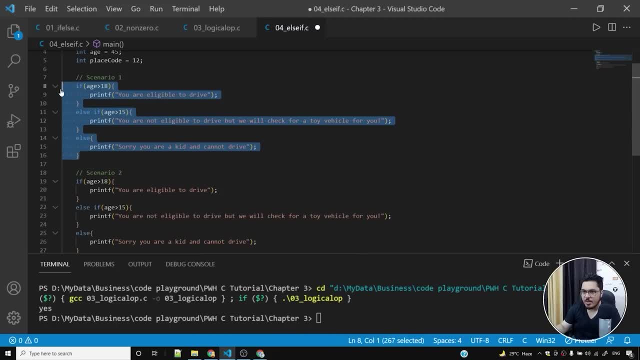 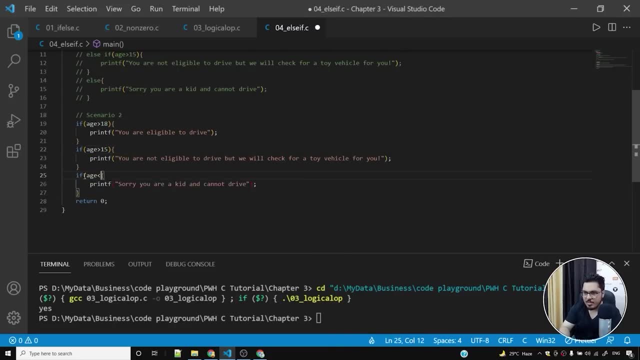 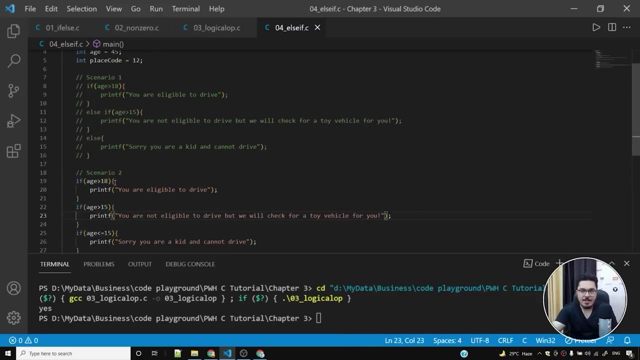 out scenario number one, okay, and let me create a scenario number two for you. and inside the scenario number two, what i'll do is i'll simply say: if age is less than 15, okay, less than equal to 15, maybe. so what i'm doing is, in scenario two, i'm checking three different conditions. so how will c compiler? 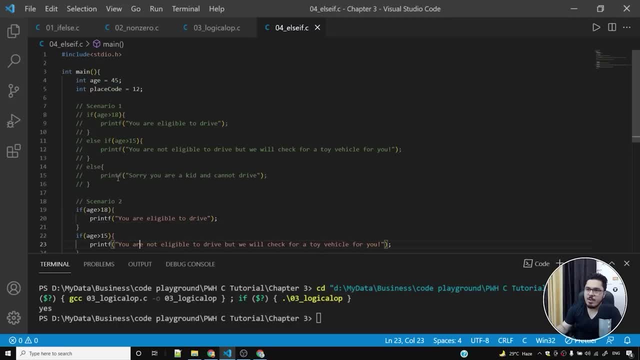 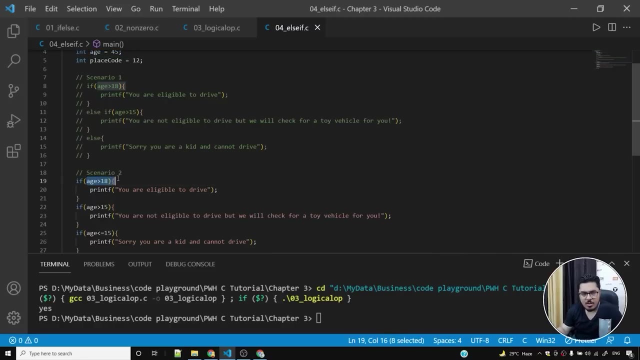 decode the scenario to. what it will do is it will see the value of ages 45. so the value of age is 45. now what it will do is, since the value of age is 45, what it will do is it will check whether this 45 is greater than 18 or not. is it greater than 18? yes, it is greater than 18. it will print. you are eligible to print. 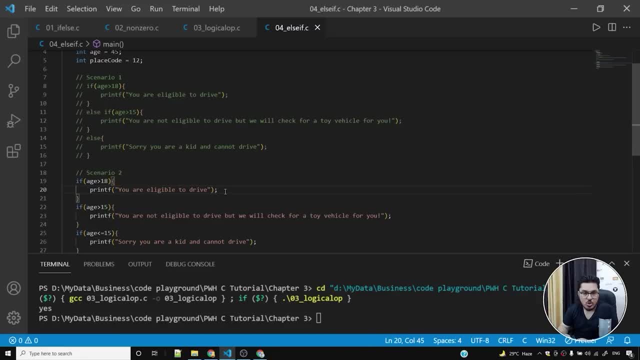 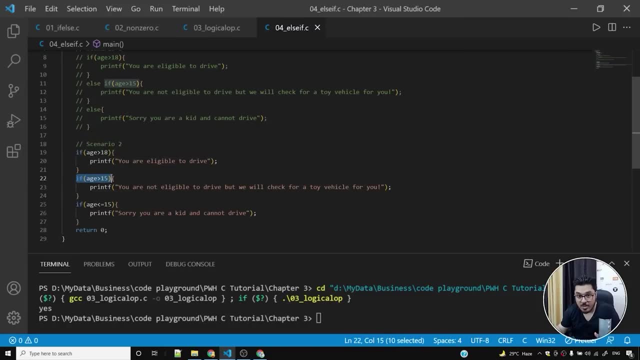 drive. but instead of stopping it, skipping the other conditions, what it will do is it will once again check for this condition: 45 greater than 15. 45 is greater than 15. yes, what it will do is it will print this once again and again, it will check whether 45 is less than or equal to 15. 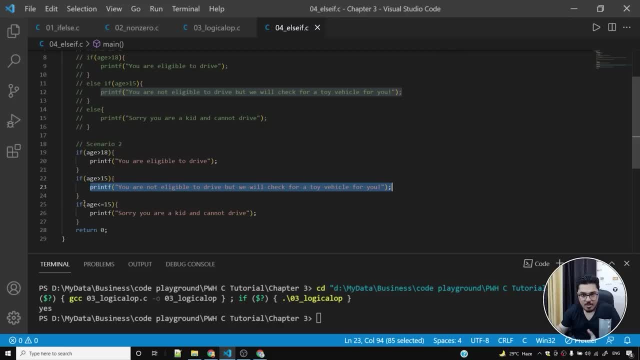 is 45 less than or equal to 15? yes, it is. uh, no, it is not. i was just kidding. i was just checking whether you are attentive or not. 45 is not less than equal to 15. okay, so this is not going to get printed. now you are eligible to drive: will be printed. you are not eligible to drive: will be. 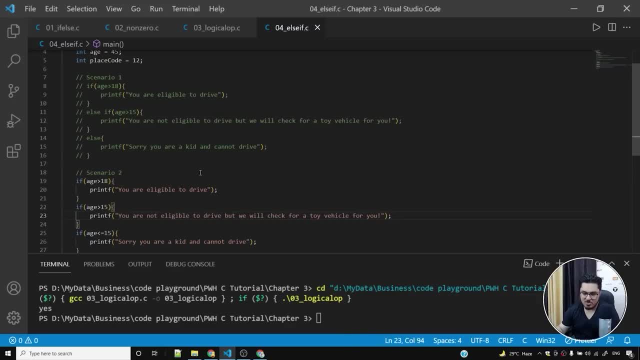 printed. so this will. this will get a bit confusing, so let me show you. so this, this is, this is printed. let me add a backslash n after all these statements so that you know we have some pretty output. so i'll simply say backslash n, so. 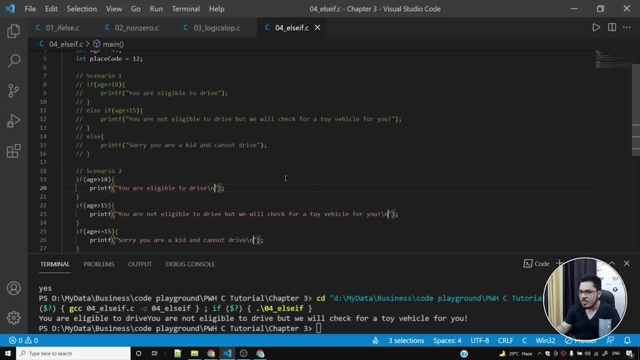 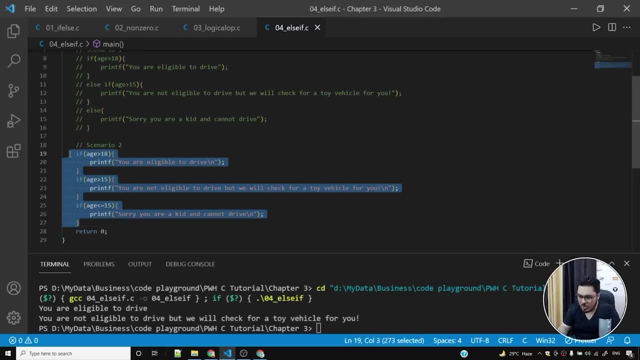 i'll say backslash n and um: yeah, i'll run this program. so you are eligible to drive. you are not eligible to drive, but we'll check for a toy vehicle for you. so both of these conditions are executed. let me comment this scenario out. do not try to. you know. map the. 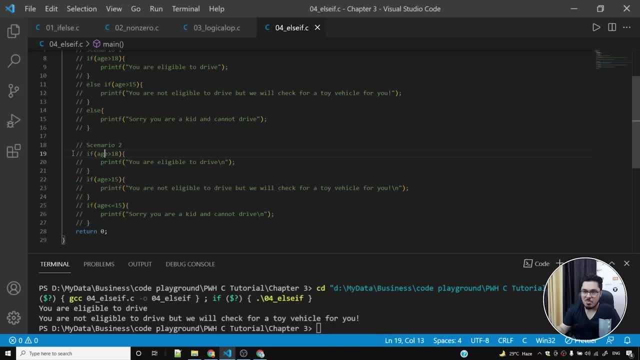 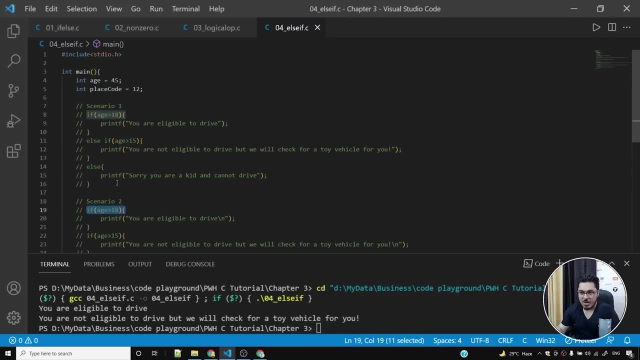 logic of whether you can drive or not. i'm just showing you some if statements you don't have to think about. why are these two things are printed? this is because we use these if statement. now let me show you how c c compiler is going to run through these statements. what c compiler will do is it will. 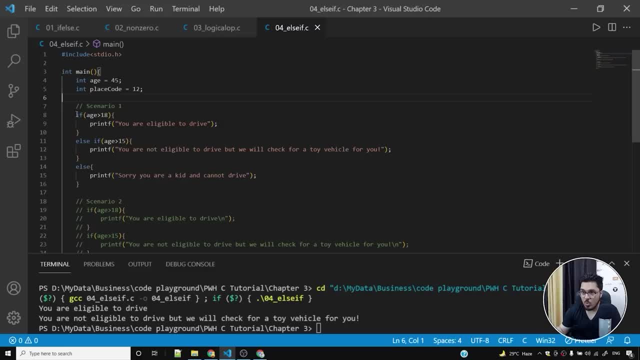 go and check the value of age, which is 45. what it will do is it will see whether age is greater than 18 or not. is it greater than 18? yes, it is now that we have else. if it will ignore, it else will be ignored because we have already matched one condition. so what it does is that. 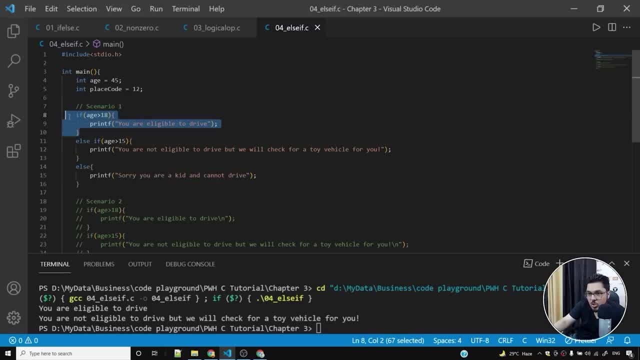 it will check for if. if. if this condition is not true, it will go ahead and start checking for else. if is, is it met? is this condition true? if not, it will go out. if there is another else, if, let us say, we have another else, if we can have more than one else, if inside our if else render this is if else. 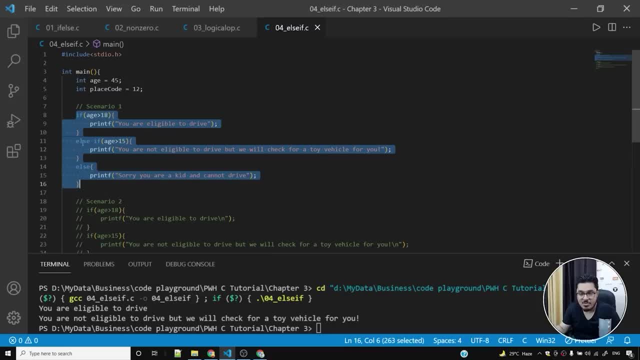 if else, ladder, this, this entire thing is called one ladder and this is one single entity and only one out of these. if else, if else, if and else will be executed. only one out of these will be executed and the moment it finds one which will get executed, which actually 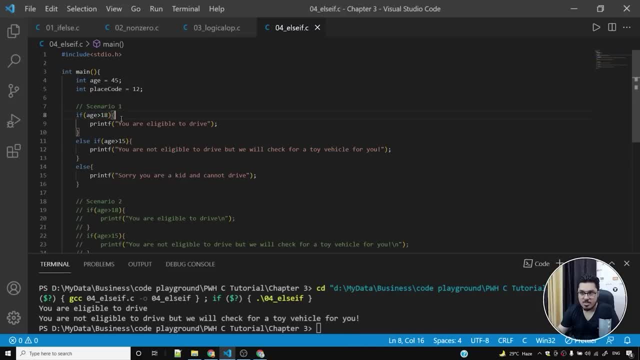 the condition, in this case, age greater than 18 will meet this condition. this condition is true, so this is executed, and then this c compiler will directly jump out of this ladder because we have already matched one condition. one condition is true. it will directly come out of this and will. 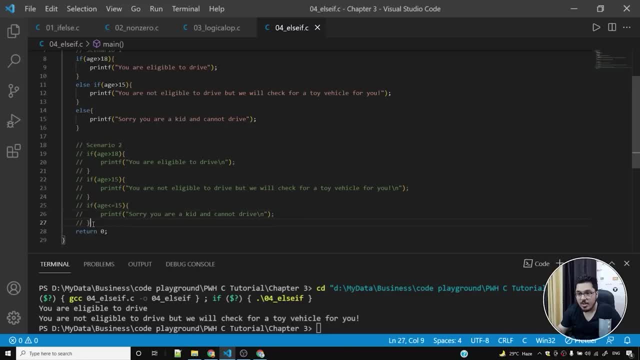 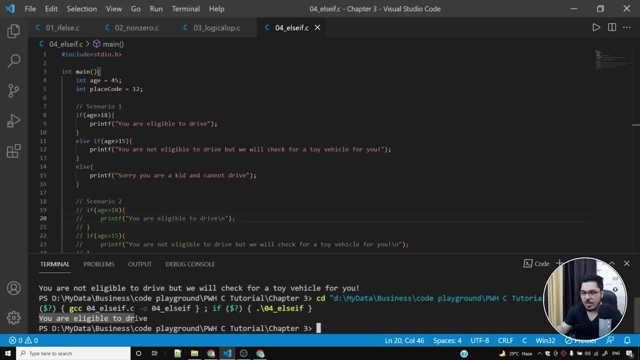 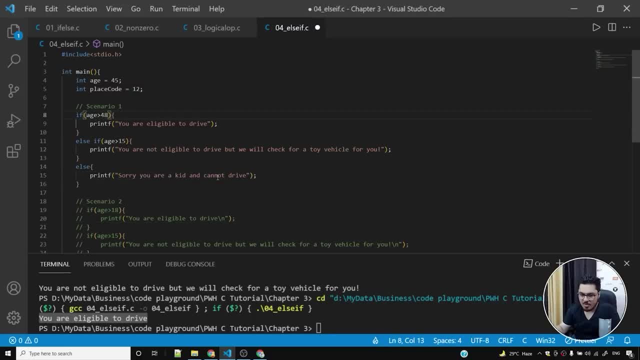 false. what if i say if age is greater than 48? it will check whether age is greater than 15 or not. and yes, it will be greater than 15, so this will be printed and then it will stop. so i'll show you. uh, oops, i selected and ran. you don't have to commit this mistake, so you are not eligible to. 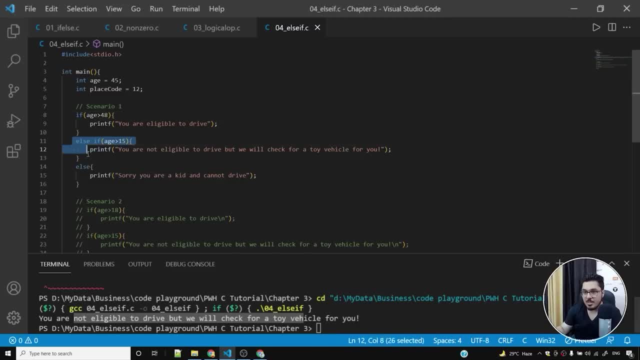 drive, but we will check for a toy vehicle for use, printed because this condition is matched. and once a condition is matched, it will forget about the entire ladder and it will go out and again it will start executing the statement. okay, so we are all here. we have taken out all our statements which are written outside this ladder. 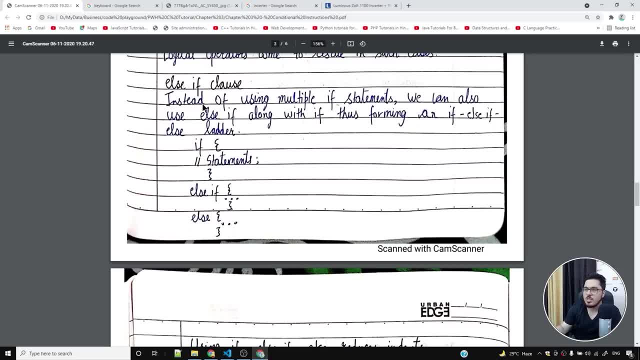 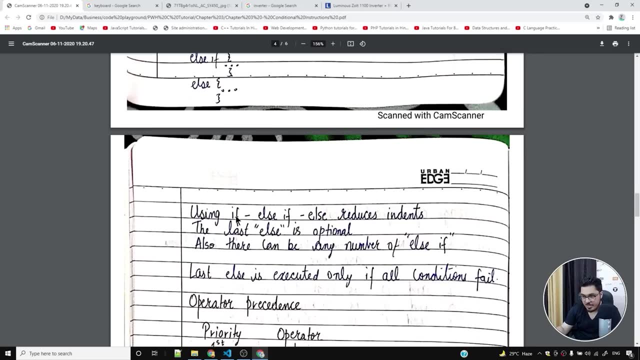 okay, coming back to notes, and this will really clear all the confusion- uh, because i've written it and put it in the notes in a very beautiful way. instead of using multiple if statements, we can also use else, if along with if, thus forming an if, else, if else ladder. so this is a ladder and only 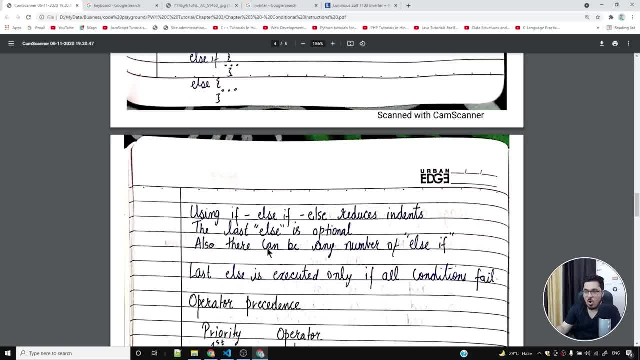 one out of these statements will be executed using: if else. if else reduces the nints. the last else is if. so this is something that i've made clear in the notes. you can have any number of else if you can have only one else, and you can also omit that else if you want. okay, so i hope that you understood. 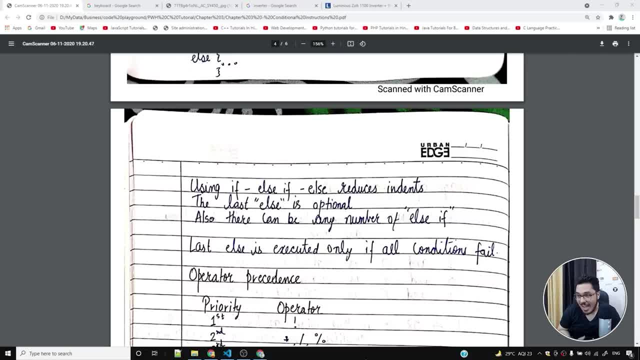 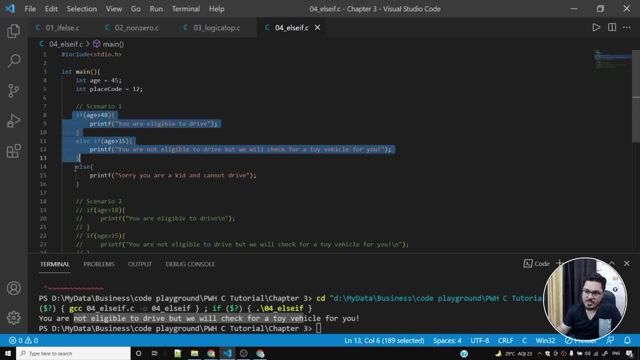 all these things. now i've written something very important here: that last else is executed only if all the conditions fail. so if all of these conditions will fail, then only this else will be executed. so this is something that you need to keep in your mind once again. so now we'll talk. 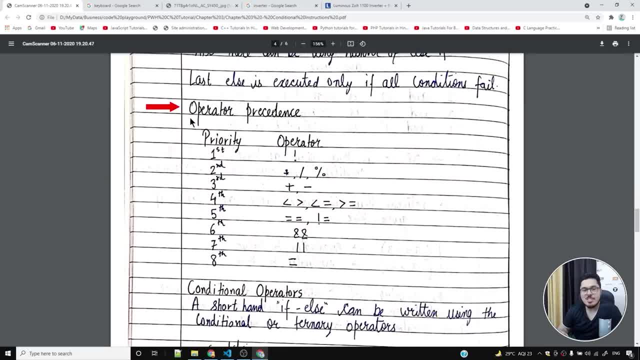 about operator precedence once again. in the previous chapter i talked about operator precedence and i thought that you know i need to jot down some more operators for their priority, because you might want to use this priority table and you should have some good amount of operators for your reference, which is why i created this list for you, and i've added this here because 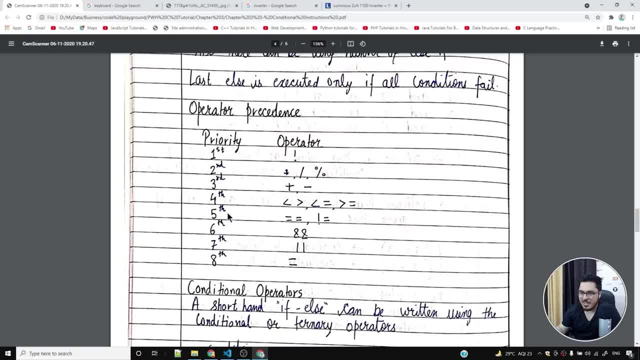 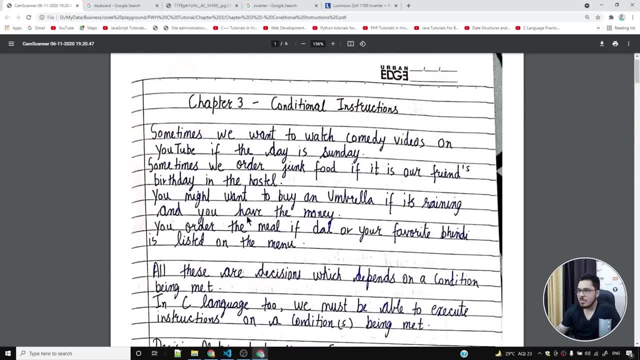 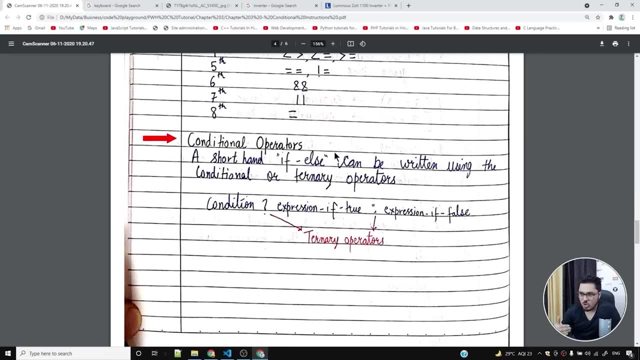 i haven't added it in the previous chapter, so i simply added it here. okay, so remember that we have a priority table of some more operators in chapter number three. okay, so now we'll talk about further concepts. which is a conditional operator, so we have a shorthand. if else, which? which is also called ternary operator. okay, it is written using a. 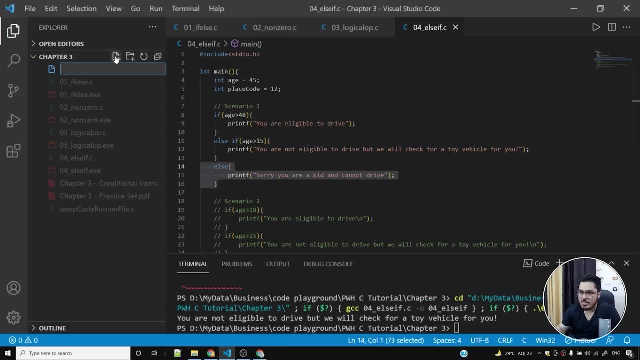 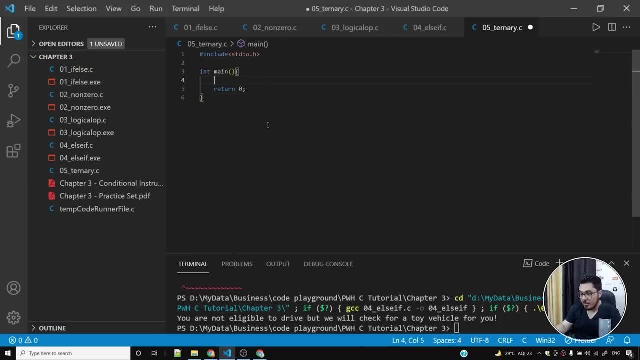 conditional. let me show you how we use it. so i'll simply say 0, 5 underscore ternary dot c. i will add a boilerplate code and i'll show you. so what i'll do is i'll say: int a equals 2, and what i can do is: 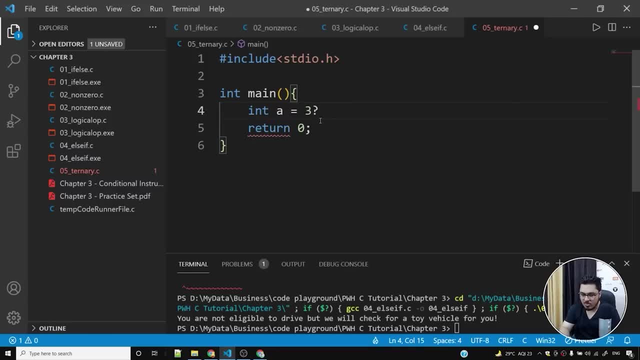 i'll say 3. if 5 or other uh say c equals 2, equals to b, else it is going to be 7. okay, now, if i say print, the value of a is percentage d, a, and yes, let me finish this program because i have not. 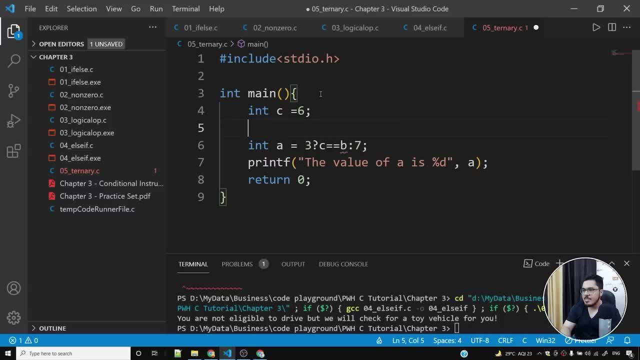 defined c, i'll say c and then i'll say, in, b equals to 8. okay, so c is 6, b is 8, and we have this thing which is called ternary operator. so how this works is if you say int, a equals to 3. 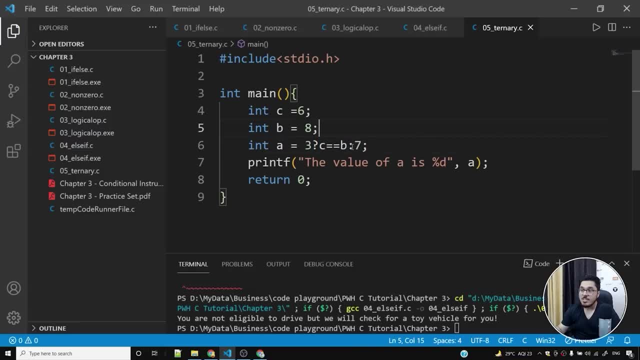 question marks a condition and then colon 7. so if this condition is true, then 3 will be assigned inside a, otherwise 7 will be assigned. so let me run this for you and you can see: the value of a is 0.. okay, so i've made a mistake here. this condition will come here and this value will come here. so 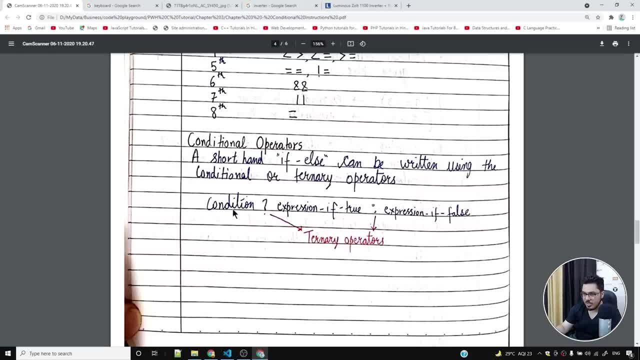 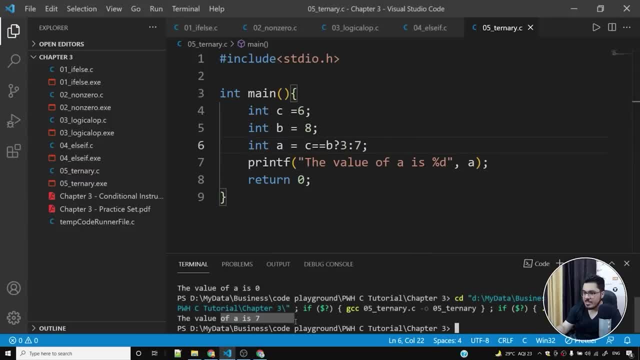 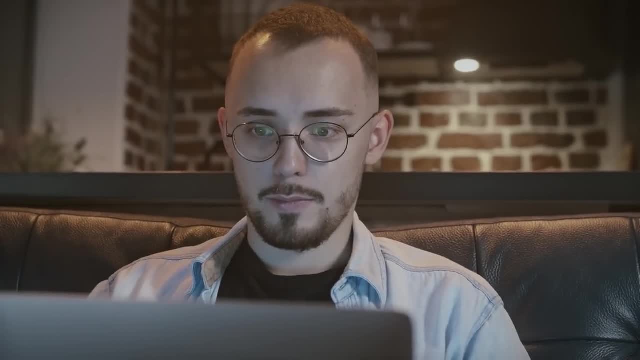 i have written this very clearly in the notes: that condition, then ternary operators, expression if true, expression if false. so let me run this once again and you will see the value of a 7. why is it 7? because this condition, or let me you know, add parenthesis so that you can easily understand. 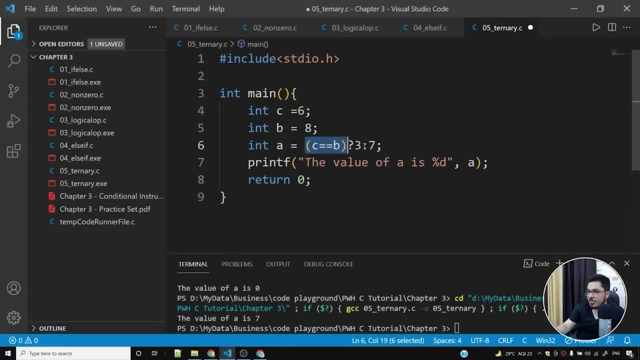 this is the condition. if this condition is true, then the value of a will be 3, otherwise it will be 7. okay, so this is how it works. if i make it 6, then c double equals to b will be true, because c will be equal to b. and if c is equal to b, what is the value of a? 3? 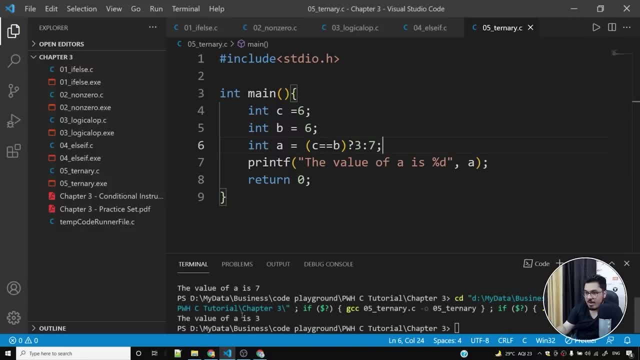 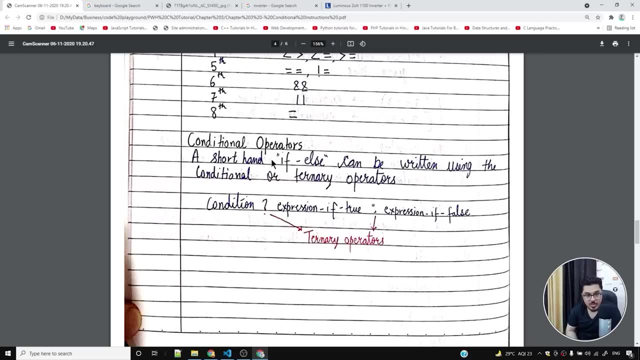 let me show you. the value of a is 3, so this is how ternary operators work. this is also called shorthand. if l statement, it can be written using the conditional or ternary operators like this. so you have a condition here. question mark: value, if true, value, if false. 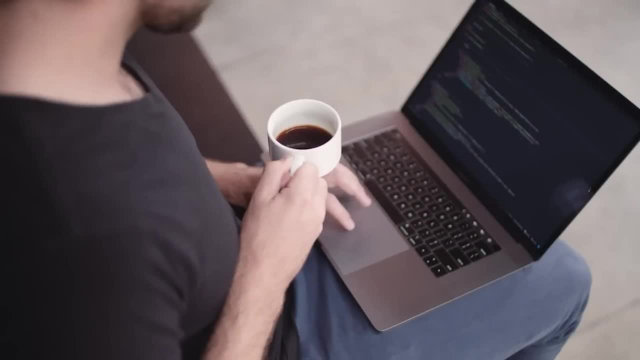 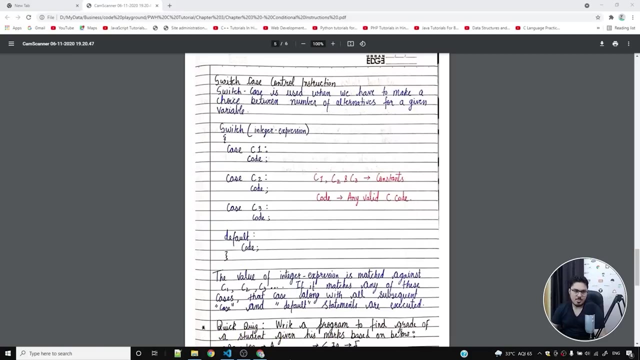 so as simple as that, so i hope that you understood all these things. now we are going to move towards switch case control statements. what are these types of statements and why do we need these switch case statements? so switch case is used when we have to make a choice between the alternatives. 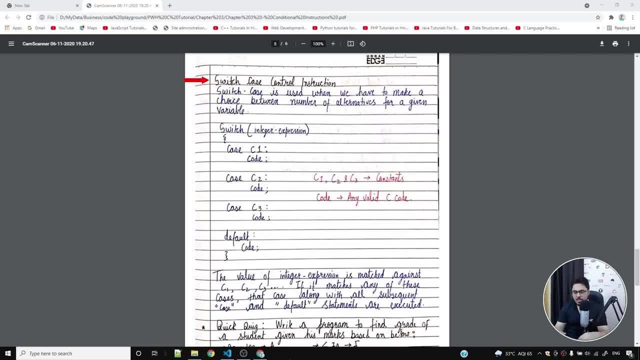 for a given variable. so let us say we have few alternatives and we want to make a choice. for example, let us say we have, we are saying that press 1 for this, 2 for this, 3 for this, 4 for this, 5 for this, and we have a lot of options for this. so let us say we have a choice for this, 4 for this. 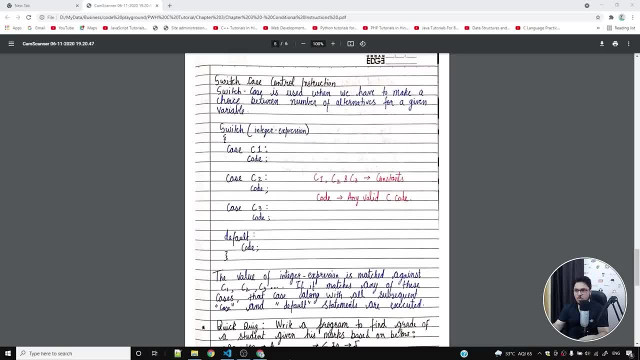 now you can either press 1, you can either press 2, 3 or 4. so what i would want is: i would want the user to press a key and, based on what keys pressed on the keyboard, i would want to do something. so i hope you understood the essence of switch case statements. now what i'll do is 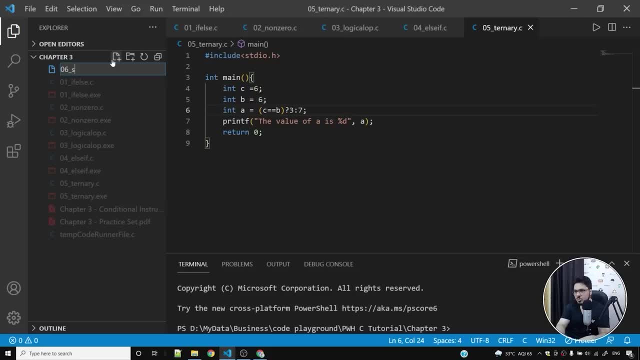 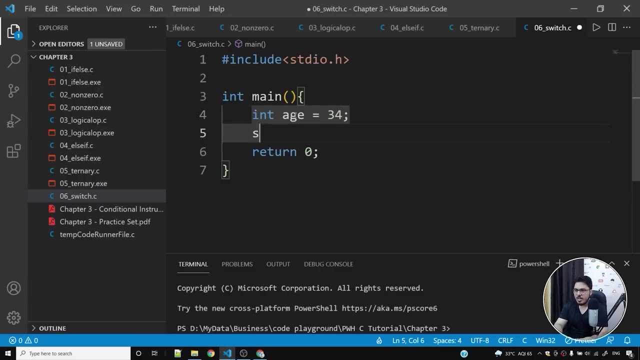 i'll simply create a program and i'll name it 06, underscore switch, dot c. and this is going to be very, very easy for you because you have already looked into afl statements. so what i'll do is i'll say: int age is equal to say 34. now what i'll do is i'll simply write switch. 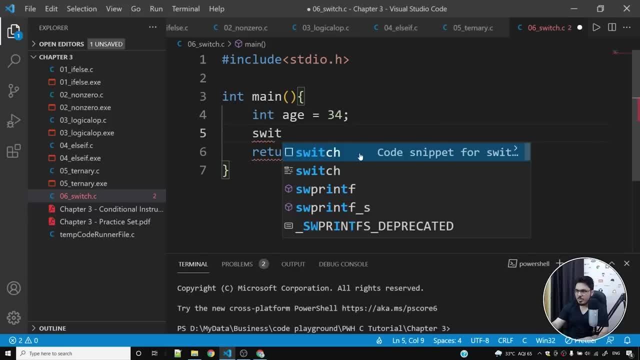 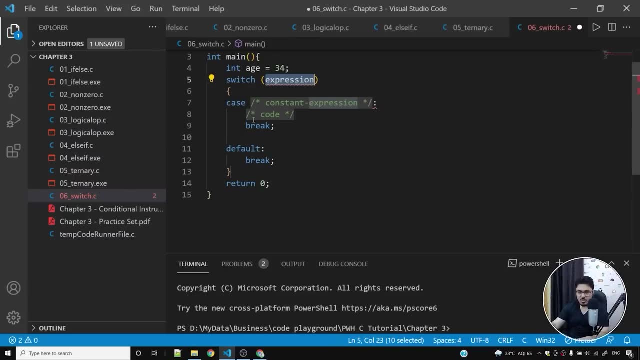 swidch and the moment i do that, there is a code snippet for switch and these code snippets are provided by the cc plus, uh plus plus extension. if you don't have these snippets, do not worry, you can type all these things on your own. you don't have to use snippets. but again, i'm using 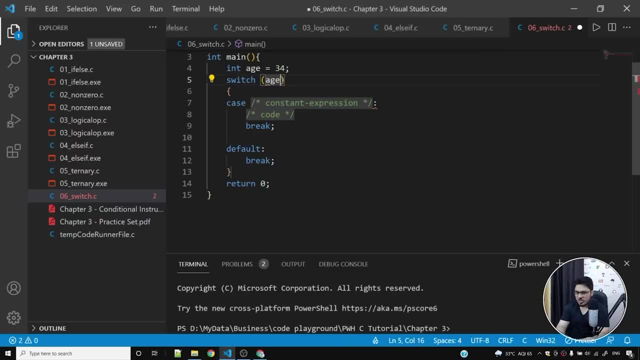 snippets, just to save time if i say: if age switch age, okay. so i want to check whether age is 06 underscore switch dot c and i'll say 06 underscore switch dot c and i'll say 06 underscore a particular number or not. if it is 24, i want to say i'll remove this code. i'll say 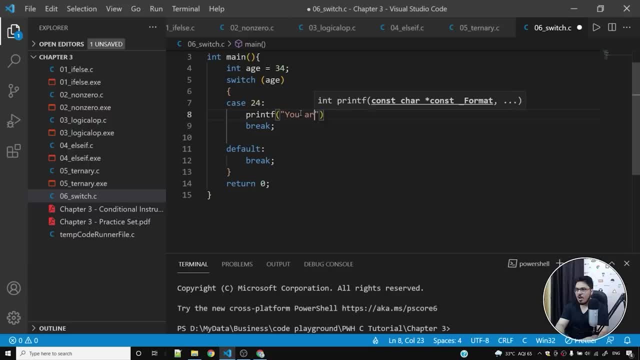 printf: you are 24. okay, now, after this, what i'll do is i'll put a semicolon for sure. so let me put a semicolon here. i'll write another case, let me. let me say 25. i'll say you are 25, i'll do the same for 26, i'll do the same for 27 and also i'll do the same for 28. so let me. 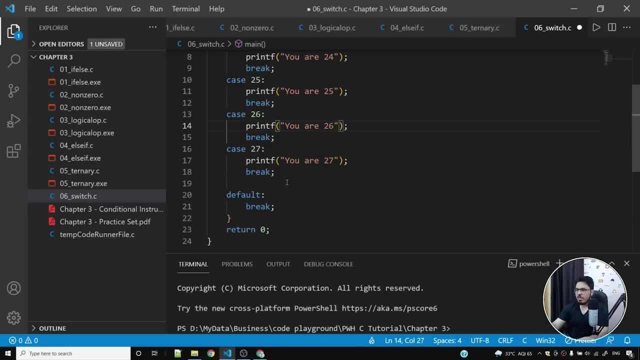 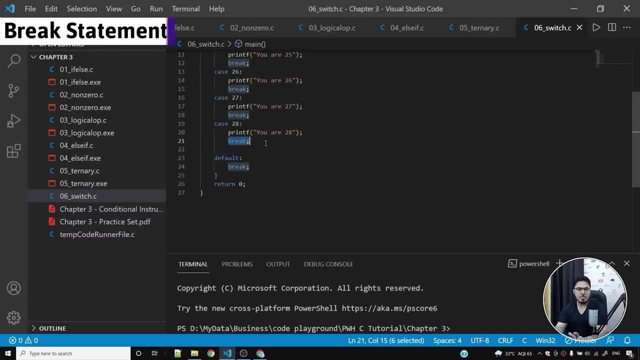 say 27 here, let me say 26 here. 25 is already there, so we have case 28 and let me save this. so case 24: you are 24, you're 25, 26, 7, 8 and just ignore this break statement at. 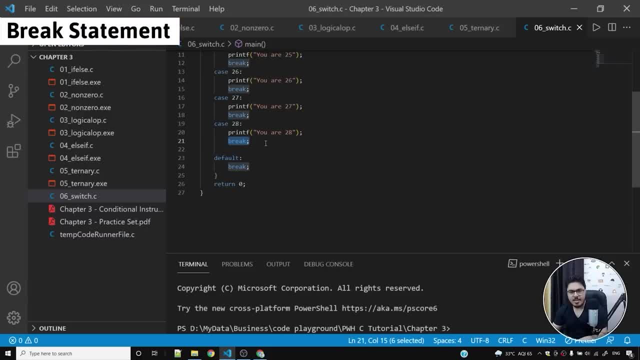 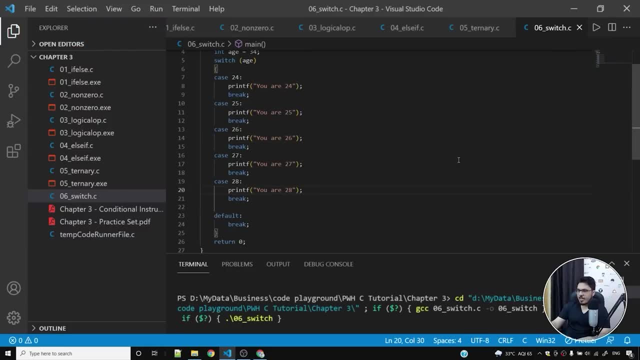 this point because i'm going to talk about this break statement in a very great detail. you, for now, just forget about this break statement. okay, let's run this program and see what happens. so, the moment i run this program, nothing happens because, uh, because, i don't have 34 as the case. 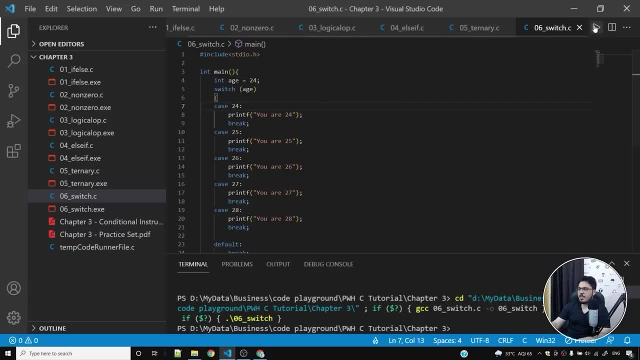 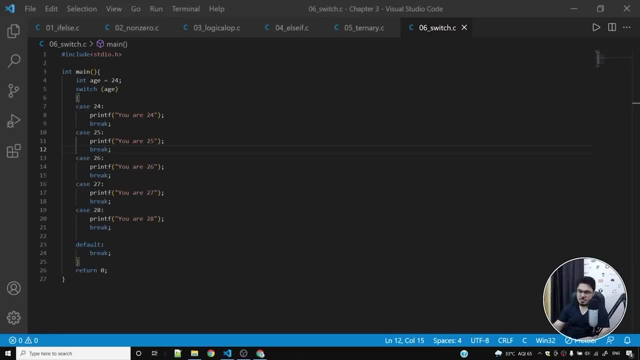 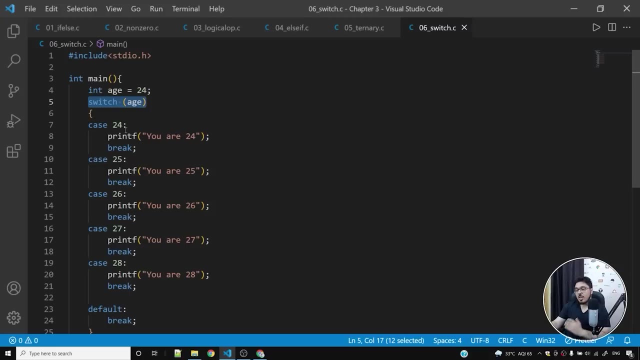 so let me punch in 24 here and let me run this so you'll see that you are 24 is being printed on the screen. why is this? you are 24 being printed on the screen. let me explain you how this thing works. what happens is, the moment you start a switch statement, it starts checking for the cases. 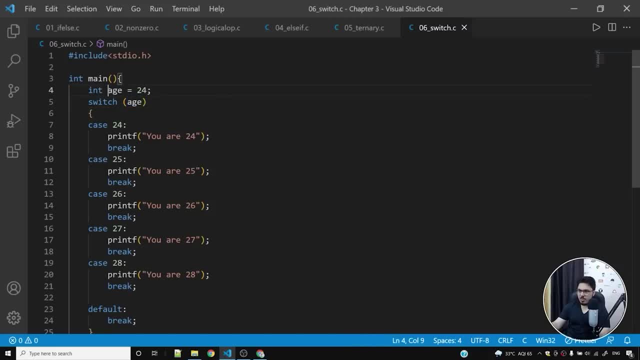 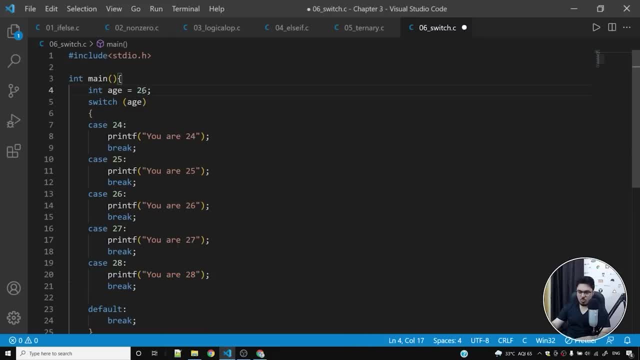 let me give you another example. what if age is 26? if age is 26, what happens is, since we are doing switch on age, it will take the age variable. it will, one by one, start comparing with this: is this 26? no, it's not, it's 24. is this 26? no, it is 26. so let's run this program and see what happens. 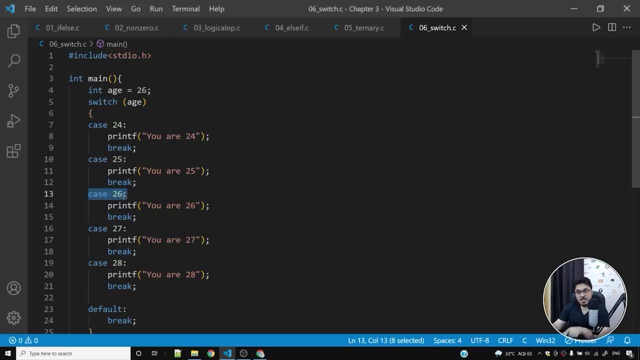 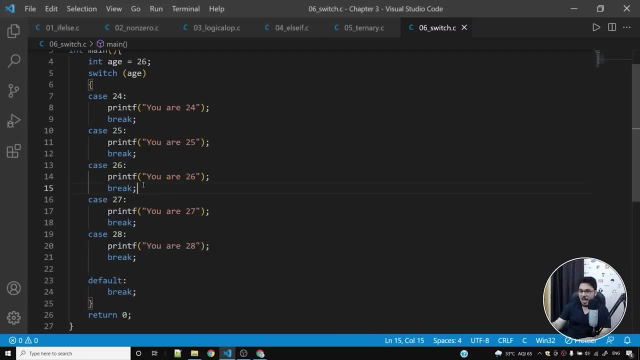 not. is this 26? yes, it is 26 and since it is 26, what it will do is it will start executing all the cases from here onwards. but wait, what happens is the moment it goes into the switch case of 26 value. so the moment we have case 26, what happens is it will print your 26 and it will encounter a 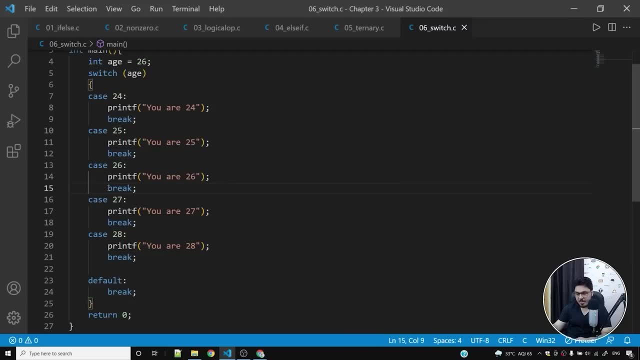 break statement. now, in order to explain what this break statement will do, let me comment all these break statements off, so i'll comment them and you'll see what they were doing. so the moment i run this program now you will see: you are 26, you're 27, 28, everything is being printed. 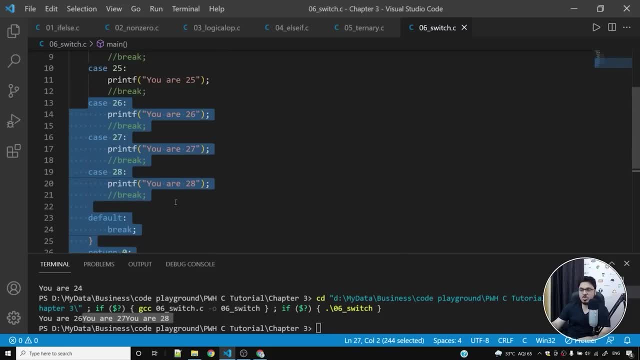 so all the cases from here onwards are being printed, so this code is executed. it will not even check the condition, because we have already matched the condition. so all the cases starting from case 26 will get executed. so you are saying case 27, you are seeing case 28, everything is being 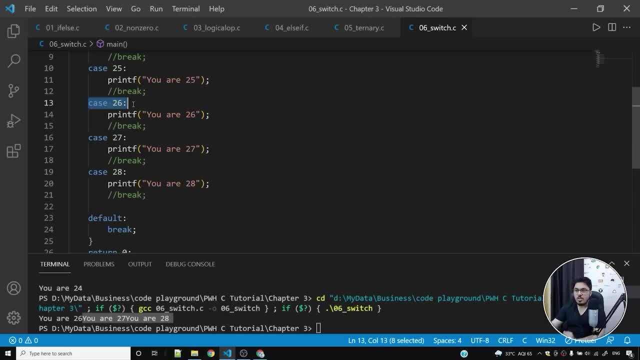 executed, but i want to stop on case 26,. I want to execute just this code, the code which is inside case 26.. How do I achieve that? And how do I achieve that? All I need to do to achieve this is I simply write a break statement. 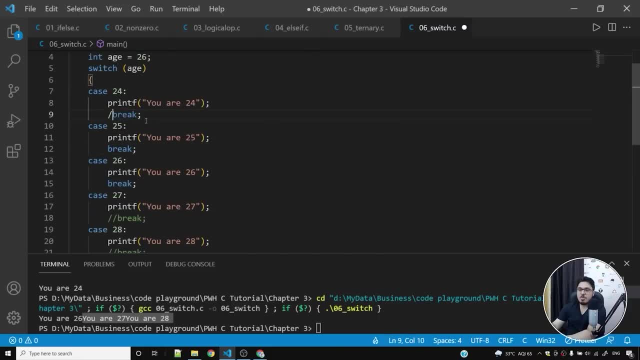 So I'll uncomment these break statements. So these break statements will ensure that the moment I encounter any case, further cases will not be executed. Only the case which is matched will be executed. In this case, only case 26 will be executed. 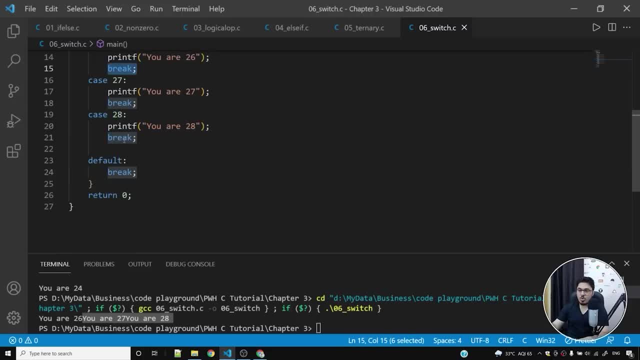 Because what this break statement will do is it will throw the control out of the switch case statement. So break, simply control, throws the control out of this particular statement, which is switch case statement. So we'll talk about break and another keyword, which is continue, in later chapter. 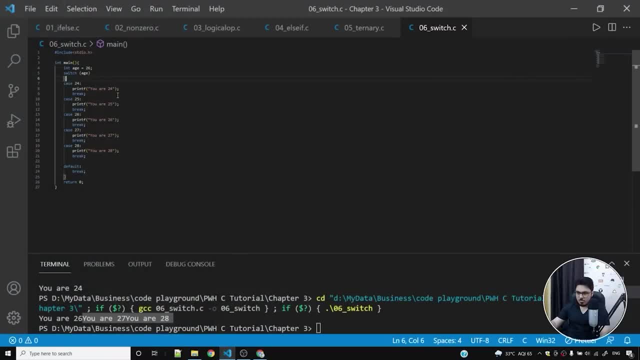 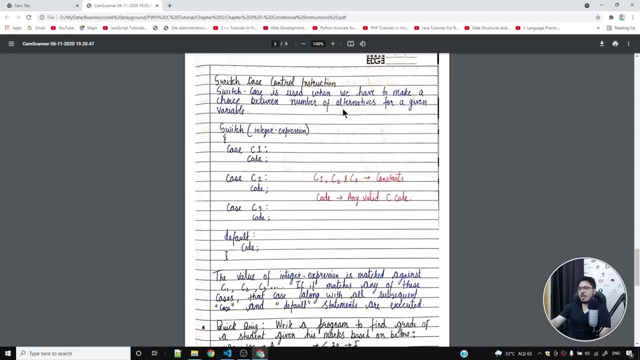 And there you will understand even more. on break and continue, but for now let's keep it this way. Okay, so coming back to the nodes, switch case is used when we have to make a choice between number of alternatives for a given variable. 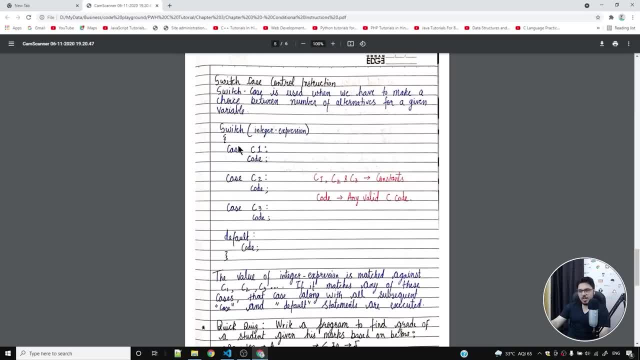 We simply say switch and we have an integer expression and we can start our cases and the moment a case is matched, all the code below the case is executed. And I have written all these things in the nodes as well. The value of integer expression is matched. 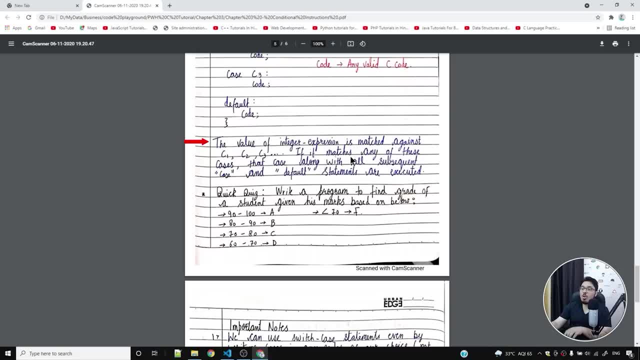 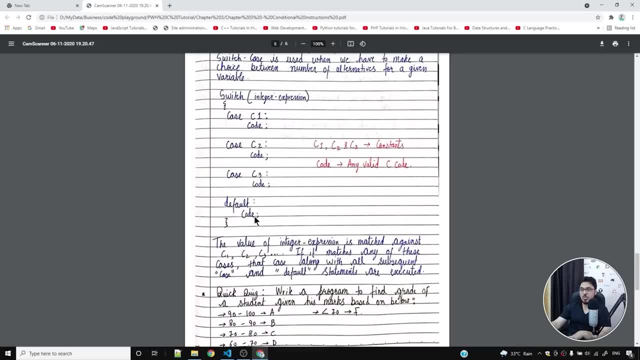 against these values. If it matches any of these cases, that case, along with all the subsequent case and default statements, are executed. Even the default statements are executed. The statement is executed. okay, This is something that you need to keep in your mind. 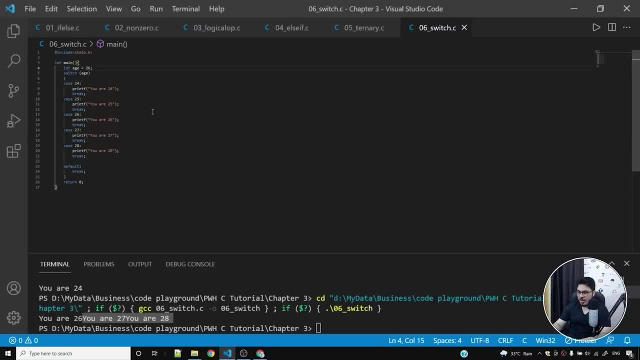 So what happens is, let us say the age is 36, okay, Let me add a printf statement after default and show you. I'll say no case matched. okay, And the moment I run this program now because age is 36 and it is not going to match any of the cases. 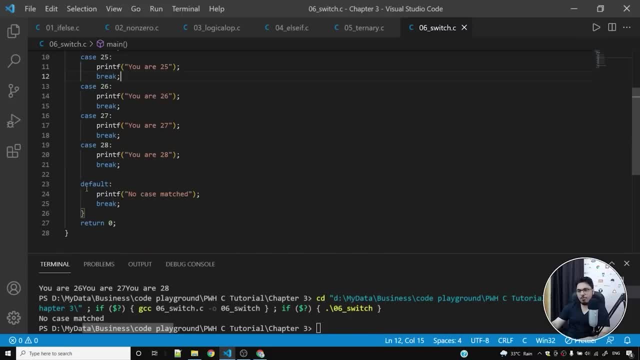 what will happen is it will simply run the default statement. So none of the cases matched. So it has no other option than to run the default statement. So the default statement simply gets executed when none of the cases match. But if any one of the cases are matching, 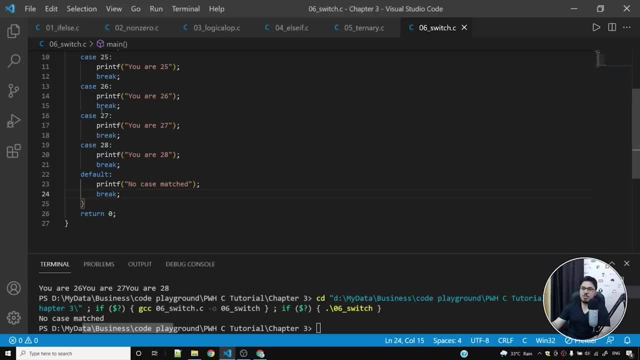 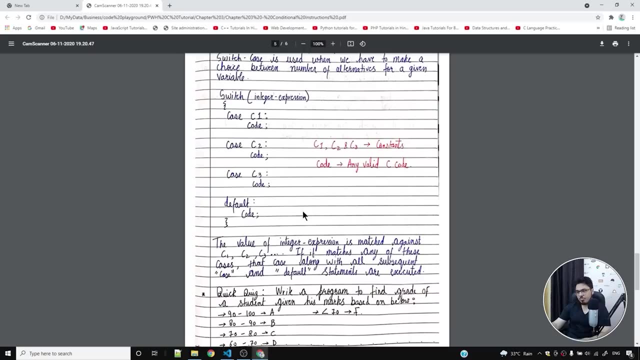 what happens is all the subsequent cases will run, But since here we are using a break statement, break statement will throw the control out of the switch case statement. okay, I hope this is clear for you. The value of integer expression is matched against this. 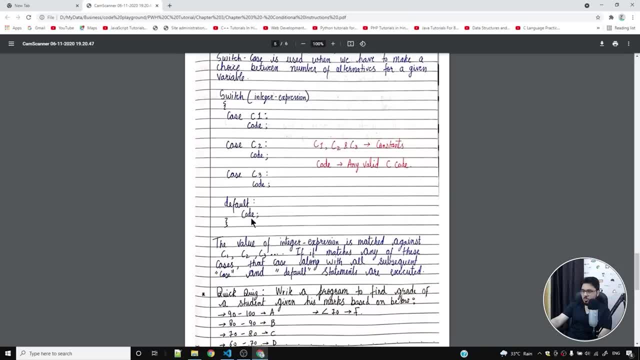 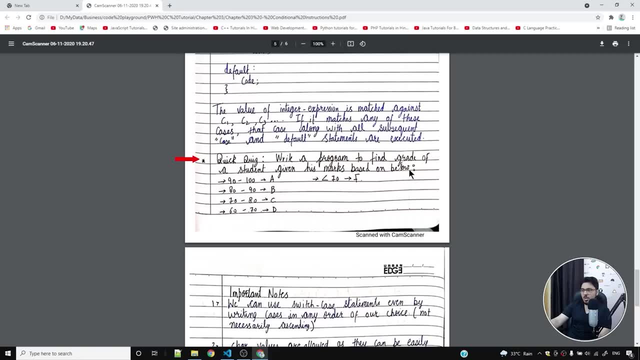 and we already talked about this- that all the subsequent cases match. All the subsequent case and default statements are executed. A quick quiz for you. Write a program to find grade of a student given his marks, based on below criteria. So we have this criteria. 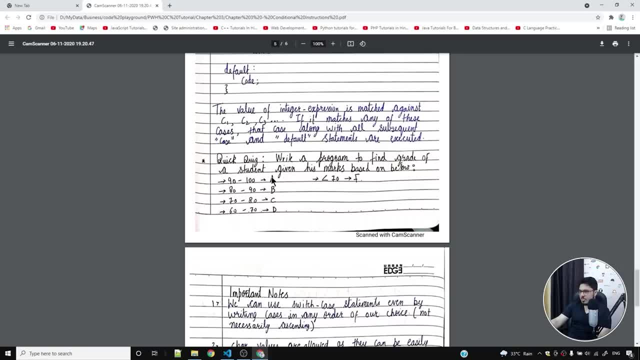 If the marks lies between 90 to 100, you need to tell that the grade is A. If they lie between 80 to 90, you need to say the grade is B, otherwise C, otherwise D. So make sure that you solve this problem. 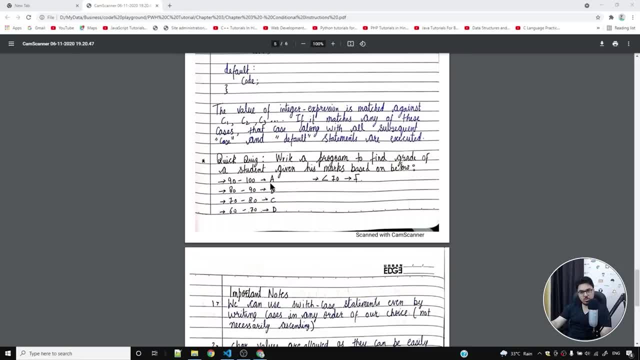 And you can use if-else statements to solve this problem. Okay, so this is going to be a very simple problem for you. Okay, so this is going to be a very simple problem for you, If you have listened to me very carefully on if-else statements. 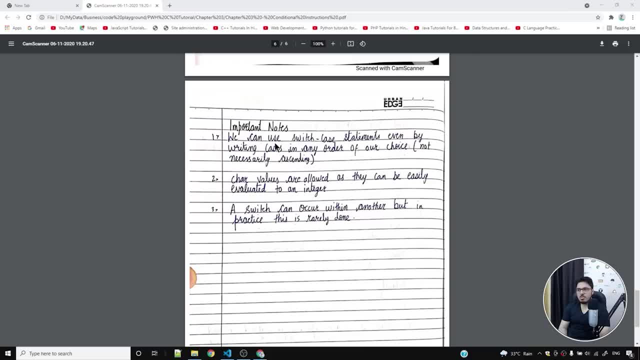 Now some important notes on if-else statements and switch case statements. We can use switch case statements even by writing cases in any order of a choice, So it is not necessary that you have to write your cases in increasing order. 24 will come before 25.. 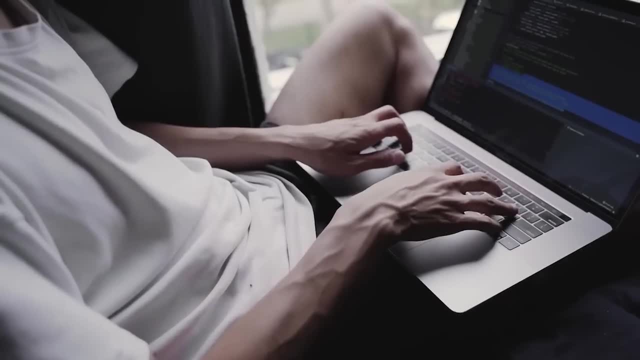 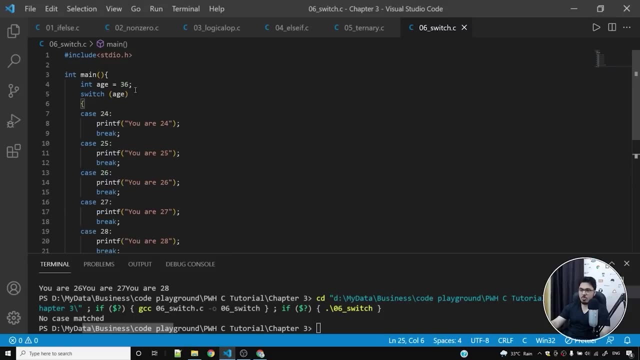 No, you can write cases in any order And whenever you write cases, they will simply get matched with the number you are running switch on. In this case, that particular variable was age, So whatever the value of age is will be matched with all these cases. 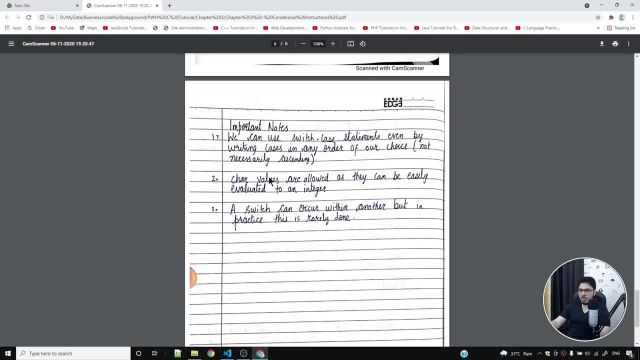 Okay, so I hope that you understood this. Next important note is that character values are allowed as they can be easily evaluated to an integer. Character values can be easily evaluated to an integer. Character values are nothing but integer expressions, because every character has a value associated with it. 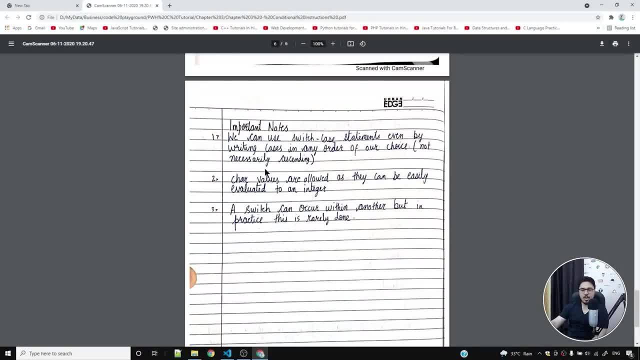 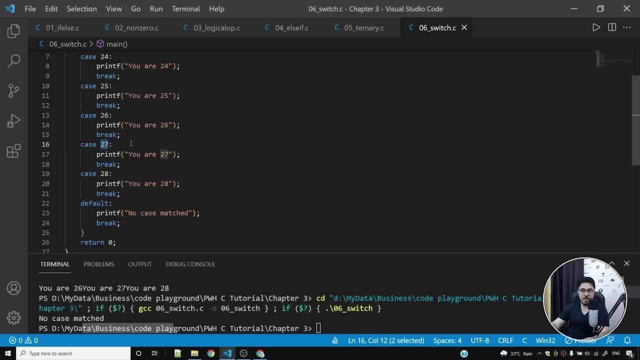 And do not get confused with this statement- but character values are allowed, which means you can always do something like this: If you want to match characters, you can do something like this, and that's absolutely fine. We'll see some questions later on how we can use characters inside switch case. 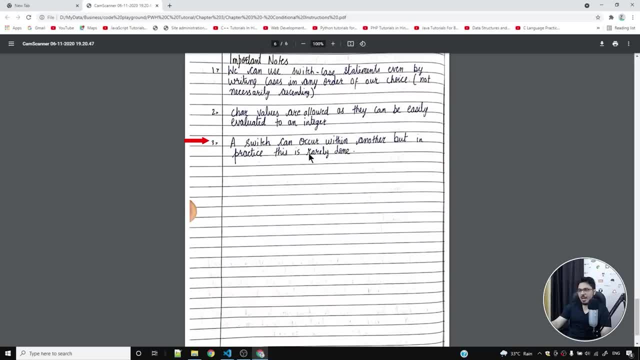 Now a switch can occur within another, but in practice this is really done, So you can have a switch inside of switch. Whenever you have a switch case and you have some code inside a case that is simply a C code, You can either have if-else statements inside that case. 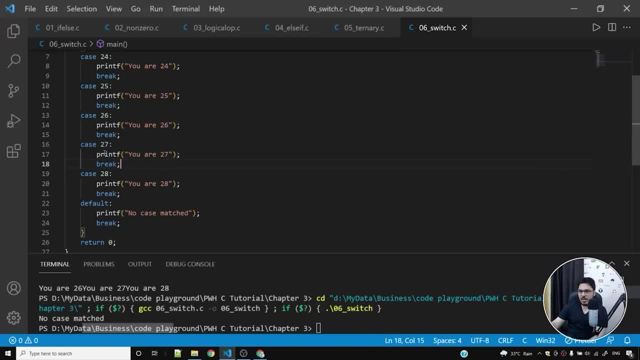 So let me give you an example. Let us say we have case 27.. Now that you are executing this particular line, can you write another switch here? yes, you can. you can start in the switch statement here, but in practice this is readily done. you can even have fl statements inside a. 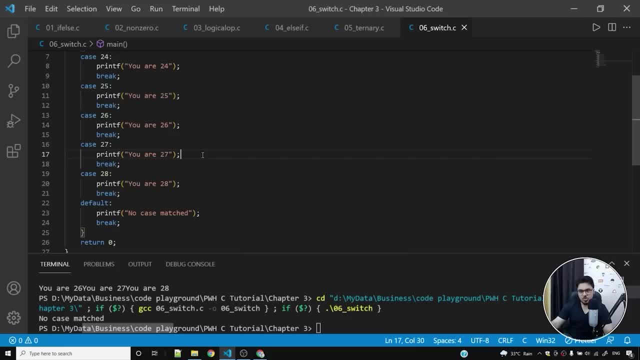 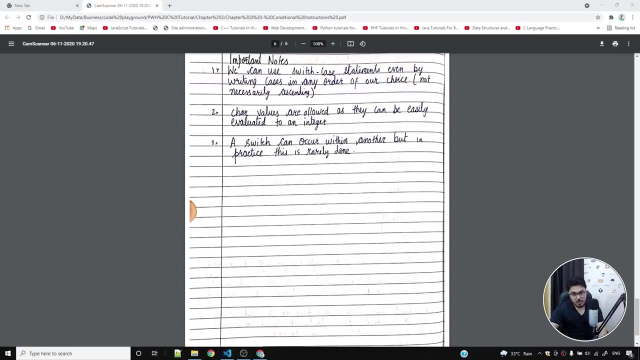 case, but again, that is also readily done. so i hope you understood all these things and you were able to find out how you can actually use switch case statements and conditional expressions in general. so we now move on to chapter number three, practice, where we are going to look into some questions on. 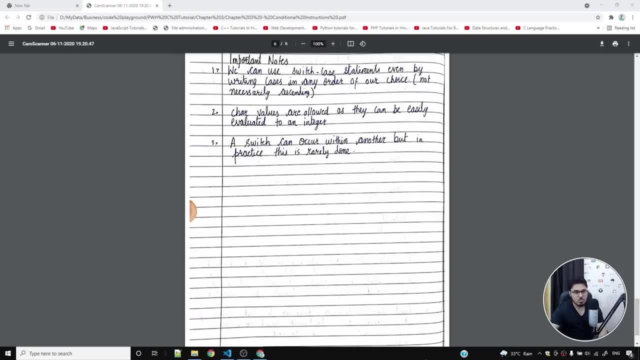 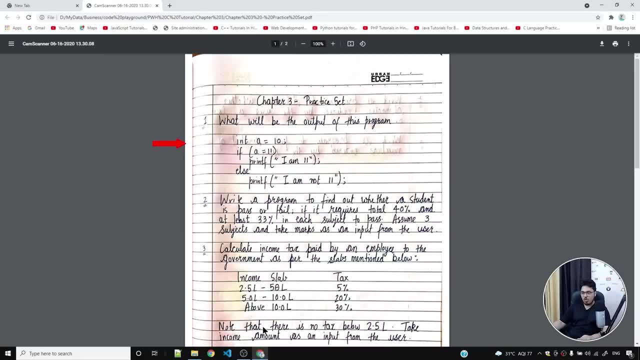 switch case statements and then we'll start moving towards some other lectures on c. let's move on to chapter three, practice set now. so here is a chapter number three, practice set, which i've created for all of you, and let's now start coding some of the problems so that we have some solid understanding. 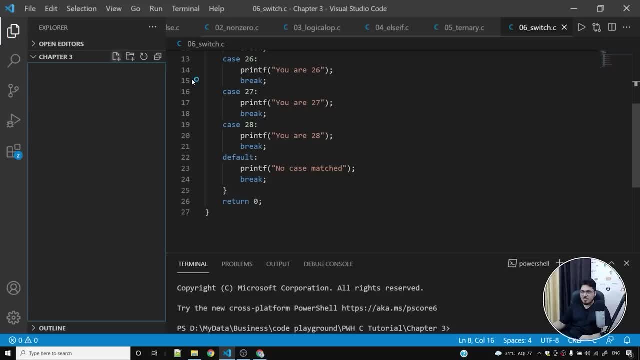 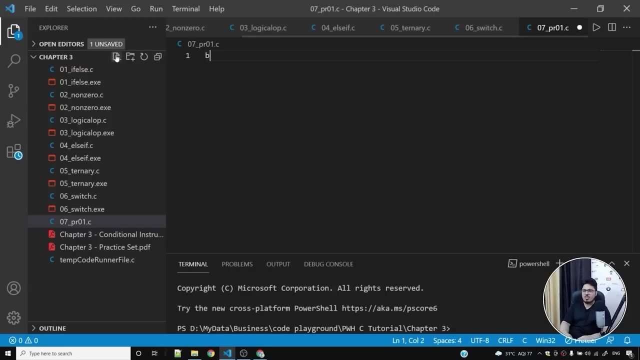 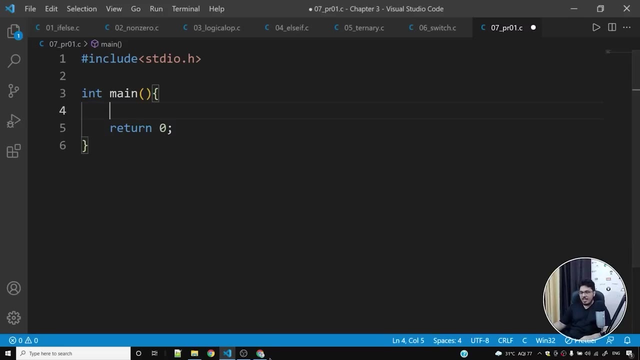 of the conditional expressions. how do we start solving these problems? i'll show you all the techniques. let's start with the problem number one. i'll simply name it pr01.c. i'll include the boilerplate code. i'll, you know, close this terminal just to get some space. and let's read the question. it says what? 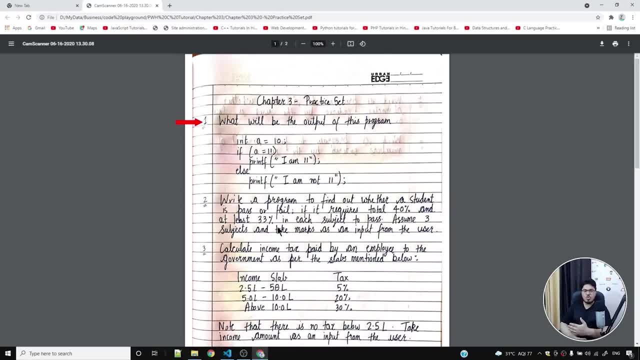 will be the output of this program. so we have: a is equal to 10, the value of a is 10. then we have a is equal to 11. if a is equal to 11, printf, i am 11, else i am not 11, if you do not look at this. 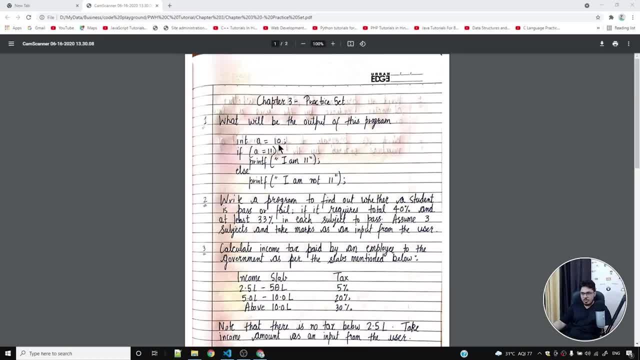 question carefully. what you will end up doing is you will say: a is equal to 10, it's not equal to 11, so this is false. if a is equal to 11, i am 11, but a is 10, so i am not 11. 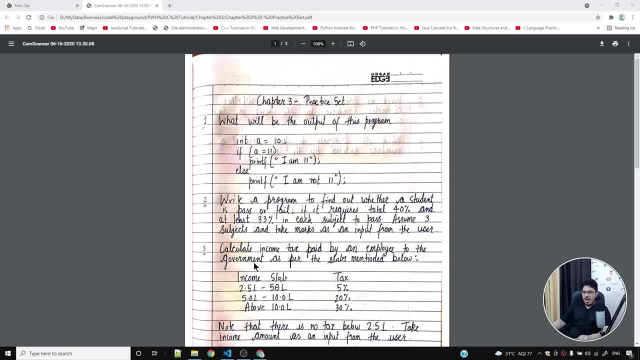 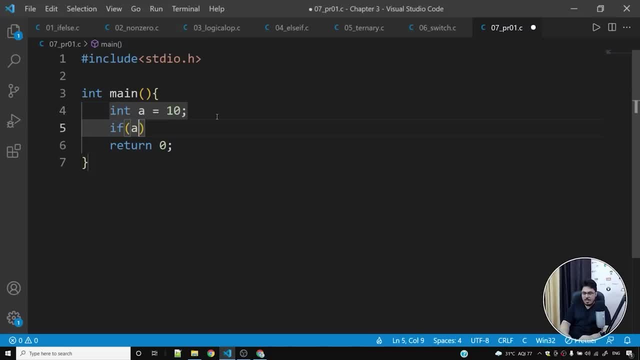 so if a is instead of 11, then i'mqueue box f will give a number and that's the way to solve the problem. so remember, from here we are going to write: problem is a is equal to 10, then it won't work this time, cell by cell, by cell. 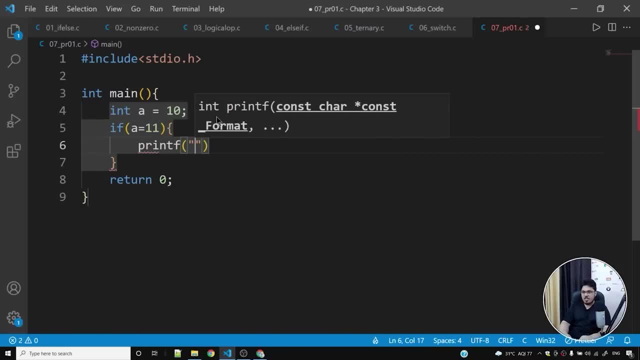 we can write this form right here and perform this layer crunchy. you should start to observe this figure, your Sir. we want to say: I want to see if you have c teaches you to specify the number of cells. is вел vamos, darble is 10, so let me replicate it and i'll change it to else, and once i do else, i'll say a is 10. 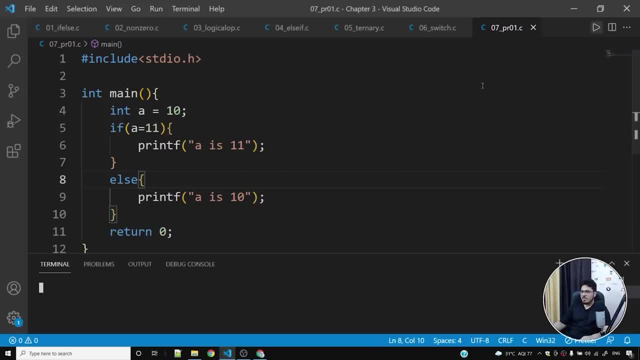 but if i run this program, i'll show you what guess what it prints: a is 11, but a is 10. why is it printing? a is 11 and i told you initially that the answer is wrong. why? why is it wrong? so i'll wait for some of you to comment down below why this answer is wrong, and i want your comments. 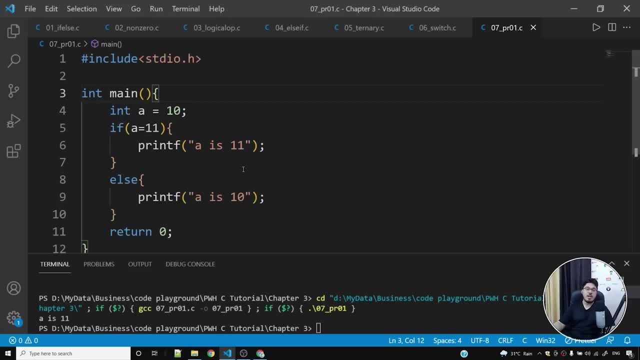 guys just put the timestamp and drop a comment, and i want you to tell me why this answer, or rather why this program is behaving in this manner. all right, i hope few people commented. and if you told me that a equals to 11 in a equals to 11 equals to is an assignment operator and this 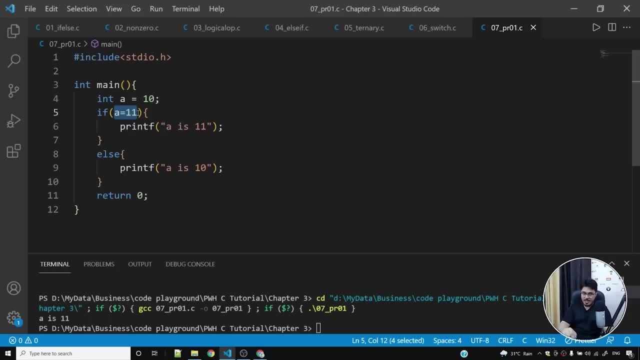 entire thing will return a non-zero value. you were right: this entire thing is going to return a non-zero value. when you assign something to something, then this is not a boolean expression, this is a non-zero value. and since this is a non-zero value, this is true in the eyes of c. 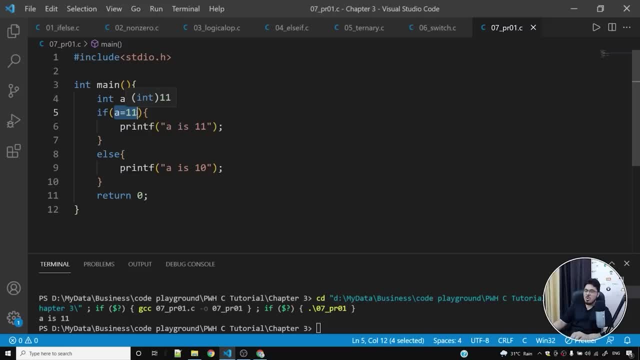 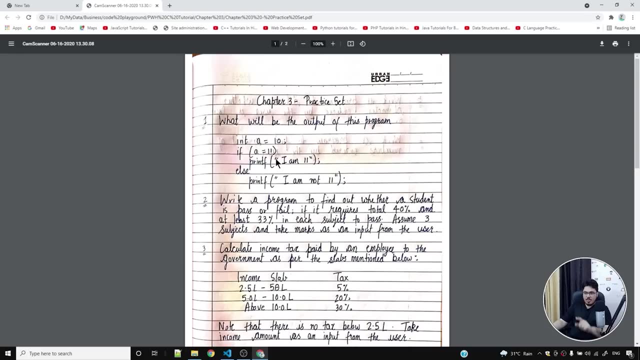 programming, or rather in the eyes of c compiler. so this is the reason why this is printed. so i hope you understood this problem number one. let's now move towards problem number two. write a program to find out whether a student is pass or fail if it requires total 40 and at least 30 in each subject to pass. so at least 33 is required and 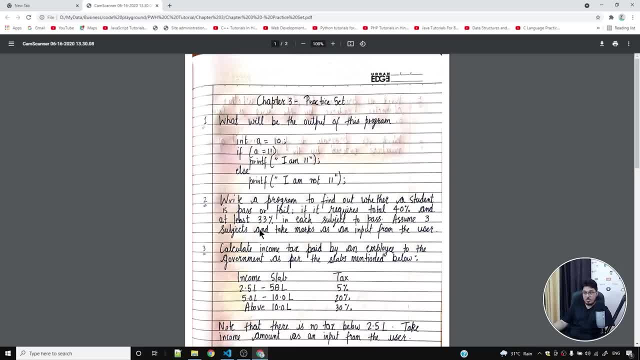 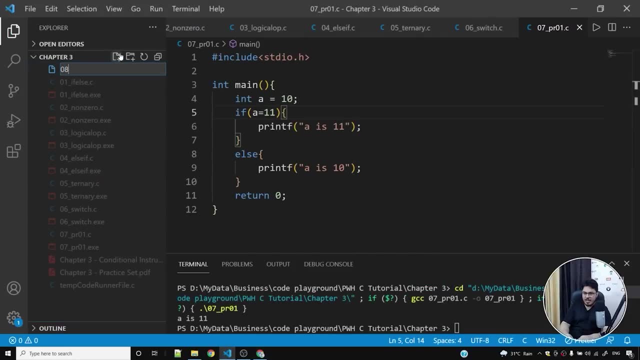 a total of 40 is required in each subject to pass. assume three subjects and take marks as an input from the user. so you have to take marks as an input from the user. okay, so let's write this program and what we'll do is simply write a file. this is 0- 8, which is the eighth program of this. 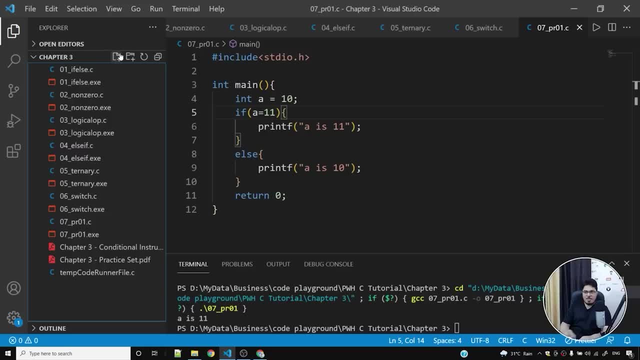 course, and itsÓ. instead of syllables we have the other五. this is the abjective person model which, of course, we are going to use. if you want to save space, say that number two is not available either. you can have it as a null set, so we will just call it to write. 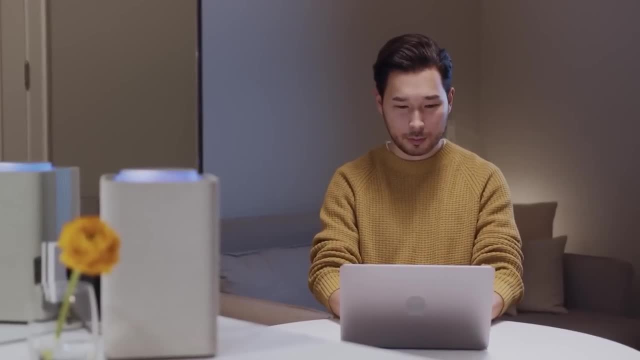 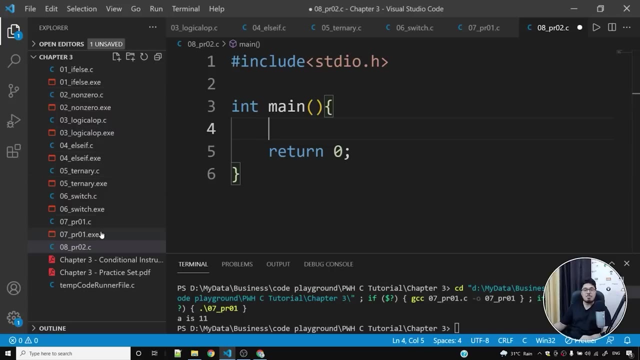 another 하면, and to get rid of them you have to give value in that name. that editor set means that that's our tail. the courier access field. this is theastic product. JS is what you are going to be using for this. you are going to use it to create some in the next few rows. that is the same point. the함 is behaving the same way. so it'll, because when we create that, the dot thelam, we start with if c dot and when we create it will give values in this course. so we are going to come back to the same string and change it as c dotail and this g if t0 on the. 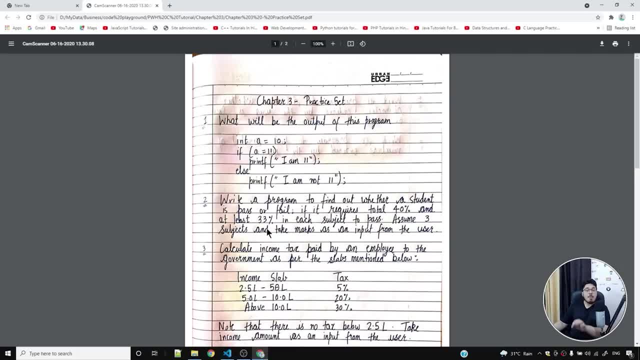 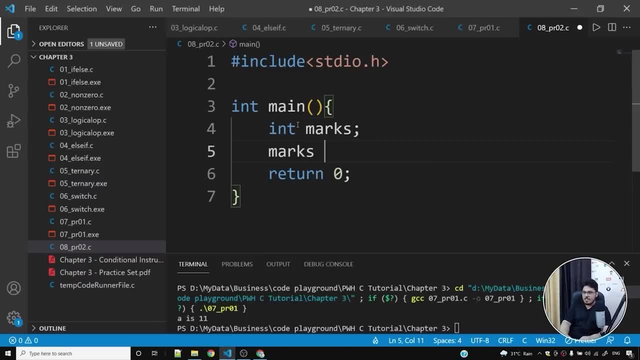 okay, coming back to the question, i have to take marks as an input from the user. so what i'll do is i'll say int marks and i'll say marks equals to scanf. what is it? it's, it's an integer, so percentage d and ampersand marks. okay, and i don't have to do. 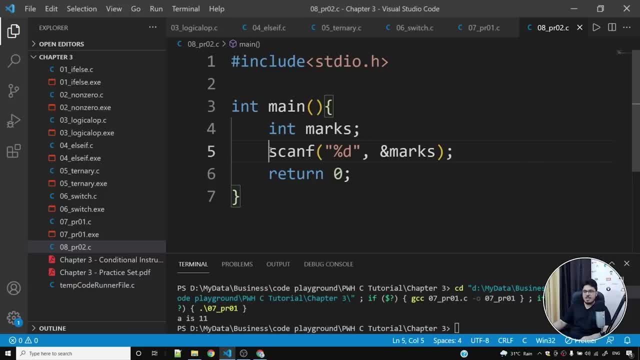 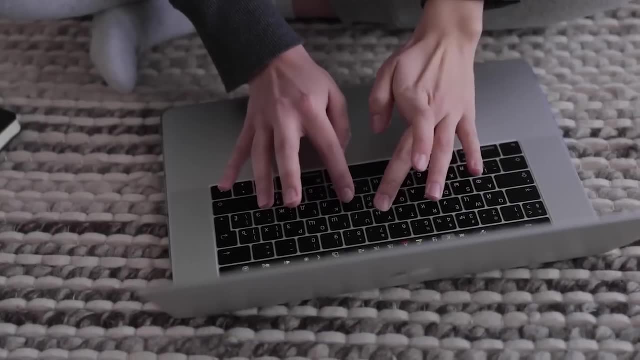 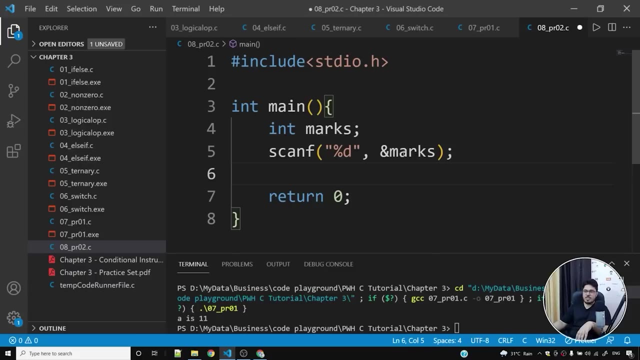 something like this just plain and simple scanf function will take care of everything. so we have this scanf, which will take marks as an input from the user and, after the marks are taken as an input from the user, marks will be stored inside this integer variable. because i 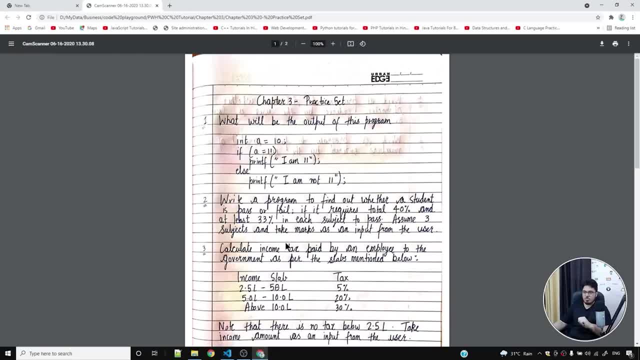 have mentioned percentage d here. okay, i hope it's clear so far. so we have a marks variable which is integer. now i have to check whether a student is part of it or not. so it requires total 40 percent and at least 33 percent in each subject. so we have to assume 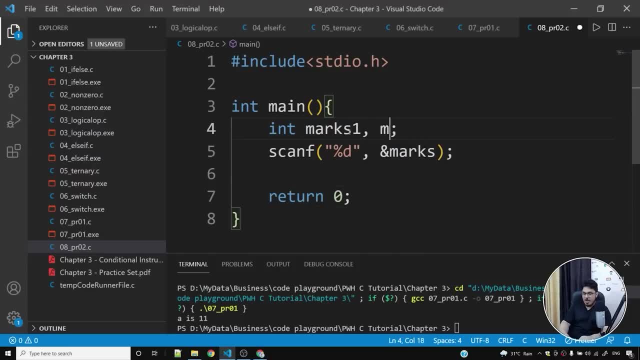 you. so what i'll do is i'll simply say marks one, marks two and marks three. so these are three subjects. you can even say physics, chemistry, mathematics, or you can say commerce, economics, accounts. just assume your subjects, guys, and do the same thing. so just to facilitate the 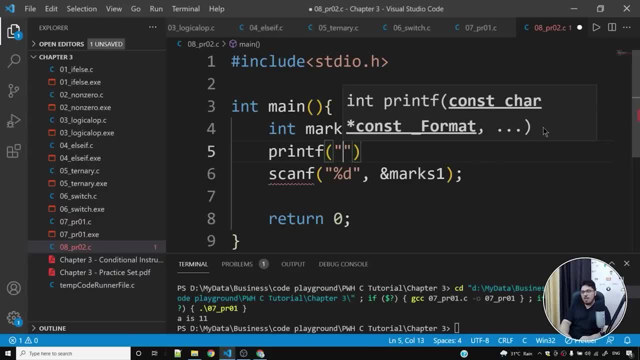 input taking from the user. what i'll do is i'll say printf: enter marks one, okay, and enter your marks in the first subject, and i'm going to use backslash n just to you know, just to make sure that these things are very nicely organized. and i'll repeat it for marks. 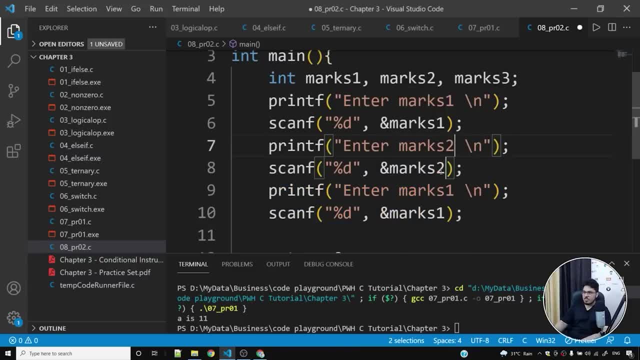 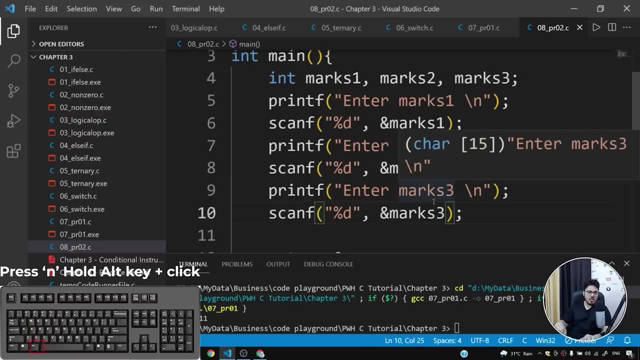 two, i'll use alt and click to use multiple cursors of vs code. i'll simply use alt and click here again. so when i hold alt and start clicking, i keep on getting the cursors, and this is how you use multi-cursor functionality of cursors. so this is how you use multi-cursor functionality of cursors. 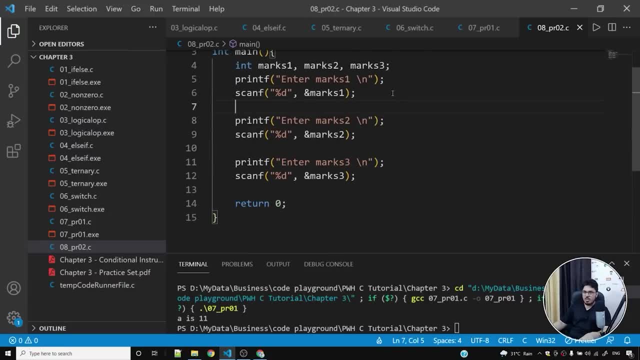 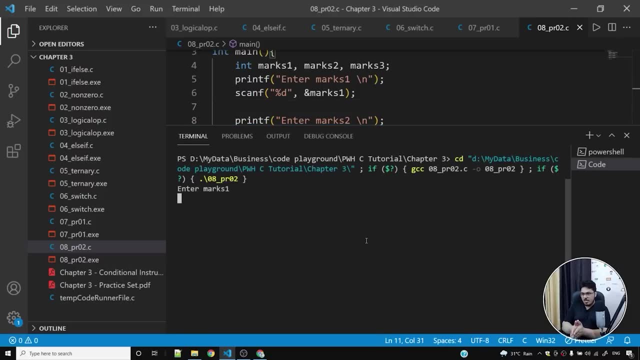 in vs code. so this is a great feature in vs code and i love this feature. to be honest now, if i run this program- and i have a habit of checking my program at different milestones just to be sure that i'm writing correct code- so 34, 34, 54, the program works nice so far. let's move ahead and 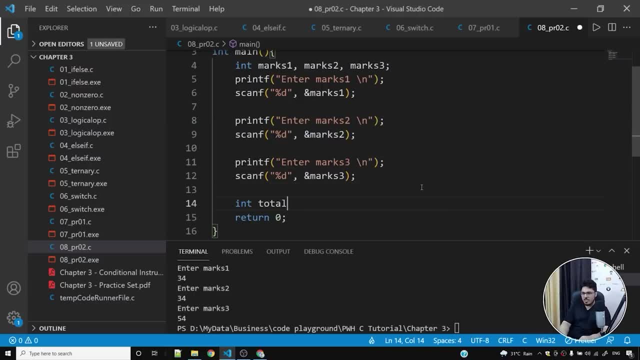 start writing the logic. so what i'll do is i'll simply say: in total is equal to, so the total marks will be marks one plus marks two plus marks three. just see how i'm writing: m3 and i'm getting marks three. so it's speaking m from here and three from here. even if i say mks, it will pick up all the. 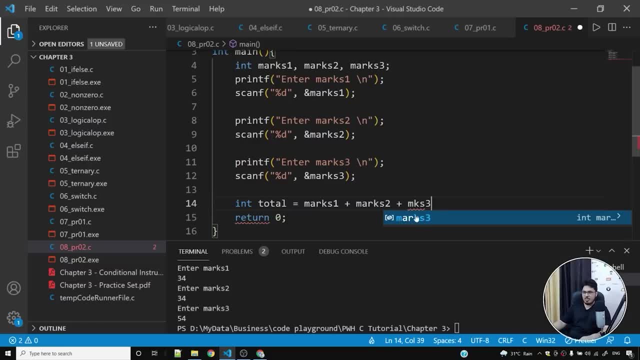 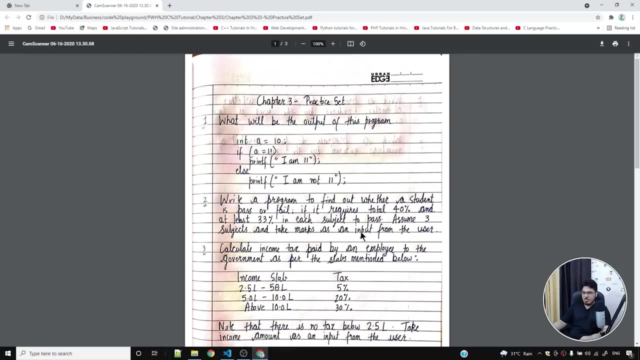 variables which contain this mk and s. and if i, if i type three, then this is the only variable which has mks and three. so you can use this type of technique to you know, write your code faster. so we have this total. so assume three subjects and take marks as an input from the user. but here's the catch we need at least. 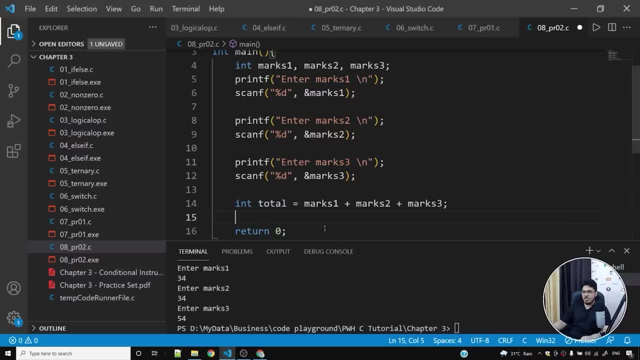 33 in each subject and total of 40. so let's check the total and since this is percentage, i'm going to use float. why am i using float? because i'm going to divide this by three. i'm going to take average of these three marks and if i use integer i might lose precision. i don't want that, okay. 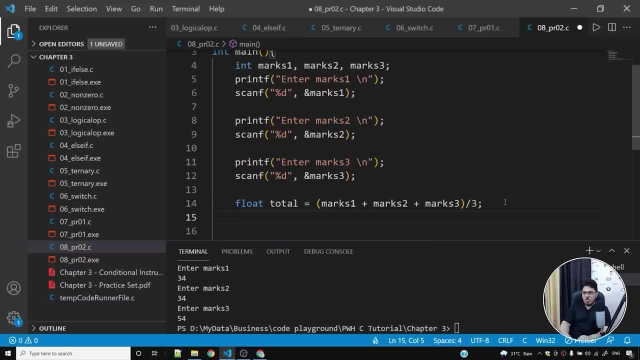 oops, i need to write three, because these are three values and also what i'll do is i'll check this, i'll save to and i'll keep the element sprinkle between them. you can take all of these three. finally, once again note that if our specific class is 0% of 40 of our total value, if we are passing, 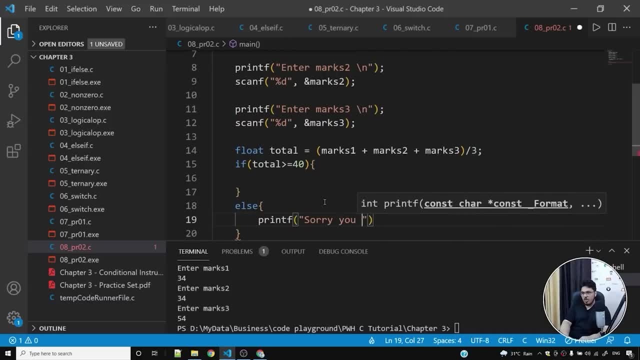 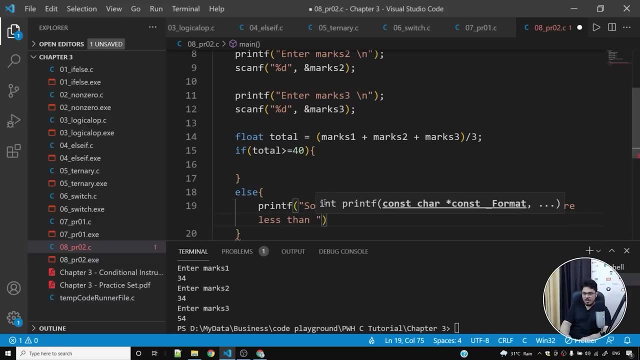 that 10% of total is greater than or equal to 40, you are passed okay. but if it's not greater than or equal to 40, what i'll do is i'll say printf- sorry, your individual marks. so what I'll do is, if marks 1 is less than 33 or or so, I'll use this pipe. 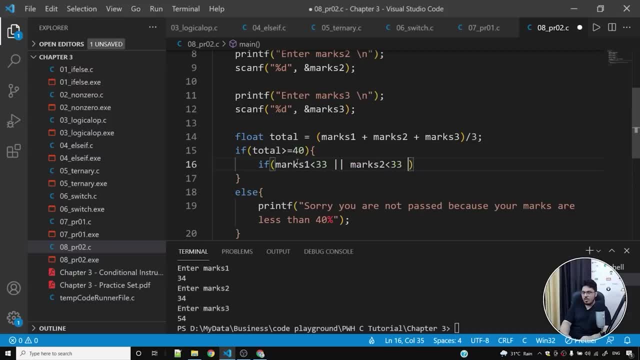 marks 2 is less than 33, or I'll once again use the pipe. so what I'll do is I'll say: marks 3 is less than 33. if this happens, what I'll do is I'll simply say printf: you are not pass. you are not pass because your marks in one of these subjects is less than 33. okay, so this is. 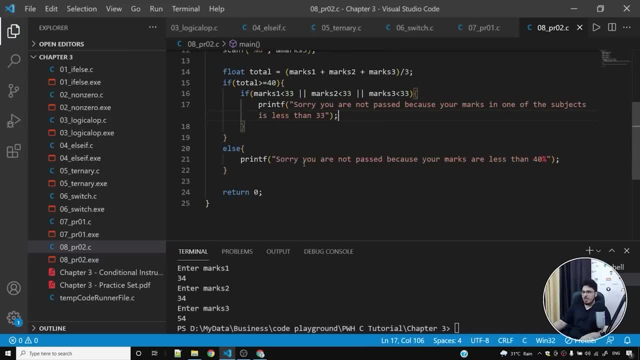 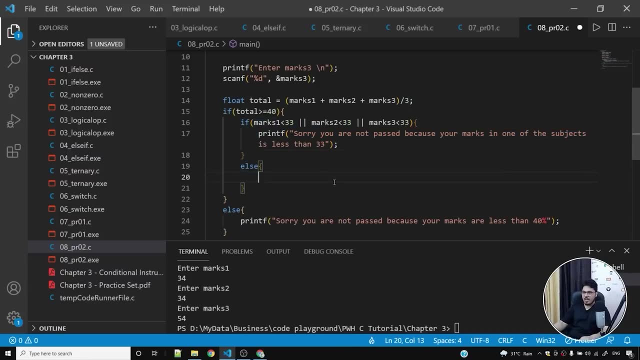 something that you can write and yes, that's fine. okay, now what I'll do is: if this is not the case, I'll simply say else. if this is not the case, simply say: congratulations, you are. you have passed the exam. you are. you are not pass because your marks in one of these subjects is less than 33. 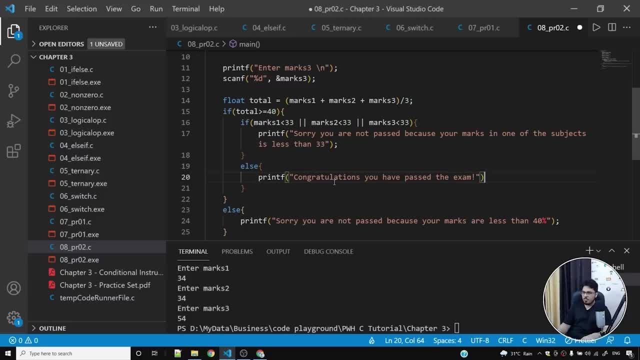 okay. so once I do this, I can run this program once again and let me, you know, award myself 23 marks in one of the subjects and 55 in the other, 88 in the other, and I have not passed because my marks in one of the subjects is less than 33. okay, so this is how this program works. I'll once. 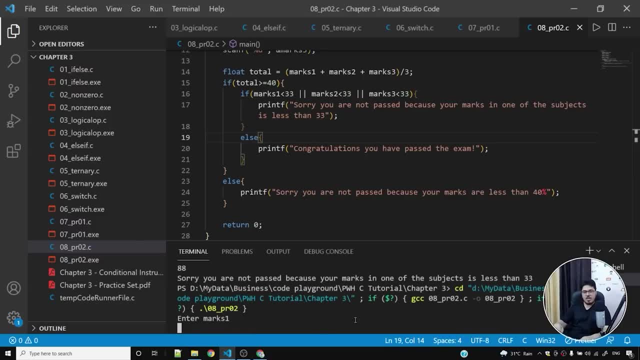 again, use arrow keys and press enter, and in fact I use the up arrow key and you can do that. you know, click on the arrow key and you can do that. so I'll just say once again: I'll run this program on the terminal. use up arrow key, press enter and your program will fire up once again. okay, so marks. 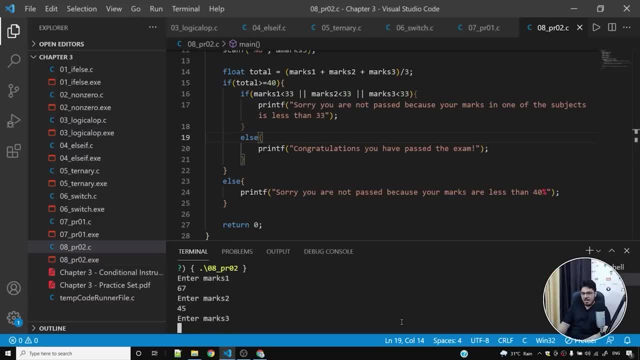 one is 67 marks, 245, and let me say 35. so yes, I have passed the exam, because my marks in all three subjects are greater than 33 and the total aggregate is also greater than 40. okay, now let's run it once again. so what I'll do is I'll simply award myself 34 marks, 34, 34. 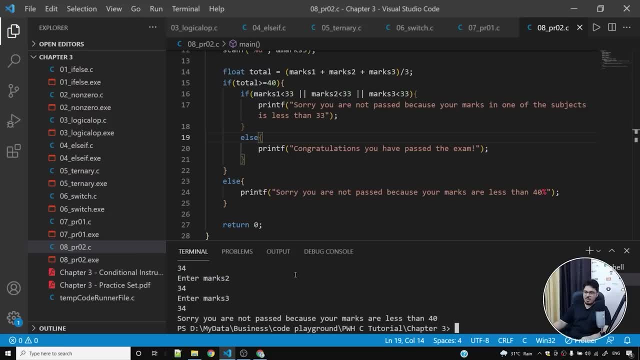 and 34, so what this will do is this will end up awarding me 34 marks in total, which is 34 percent in total, and since this is less than 40, I'm going to fail. okay, so you are not passed because your marks are less than 40 percent. okay, did you notice one thing? that we typed this percent? 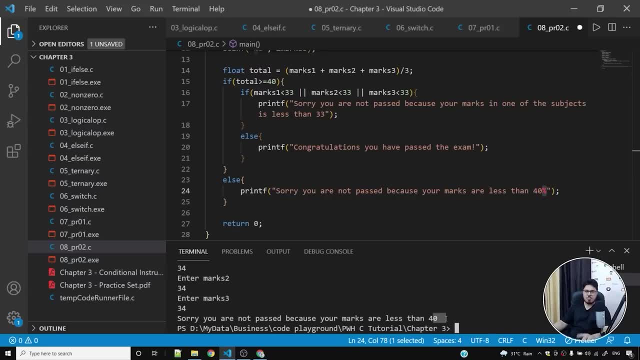 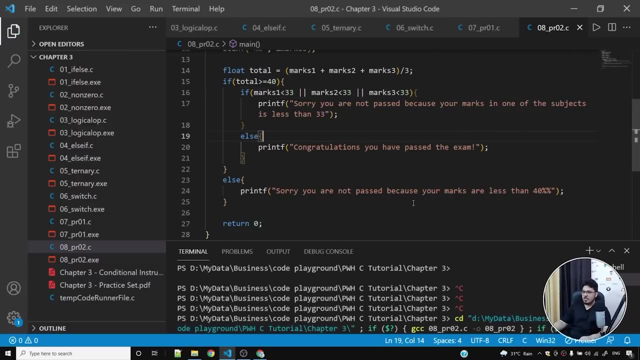 and we were not able to see this person inside the console. why was that so? what I'll do is I'll type double percentage, and when you say double percentage, it is actually printed as a single. let me show you: I'll save this program, this program, and I'll simply run this program once. 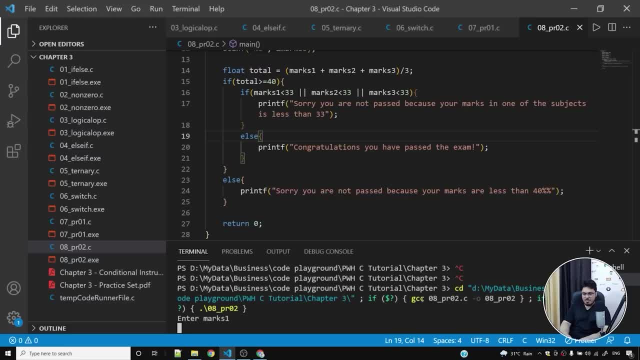 again now. what I'll do is I'll simply award myself 35 marks in all these three subjects and you can see that this percentage has been printed. so when you say percentage, it will assume that you are going to type something like percentage d, percentage f or percentage ld, or 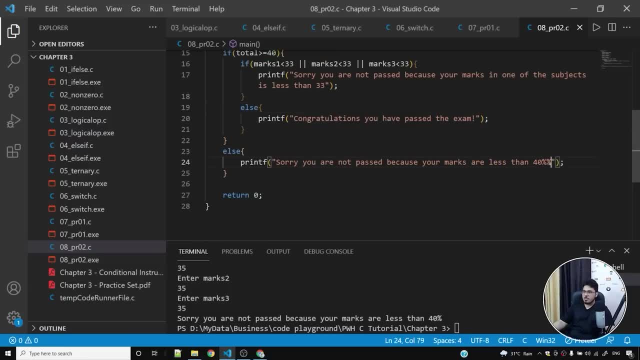 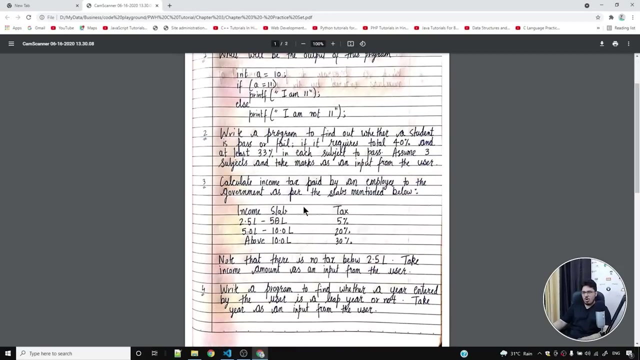 something, but but if you type percentage, percentage printf will get the signal that you are going to type or you want percent literally to be displayed here, like this. so if you want to have percentage displayed literally on the screen, simply type percentage percentage and that will solve the problem. okay, that will do the trick for you. so we solved question. 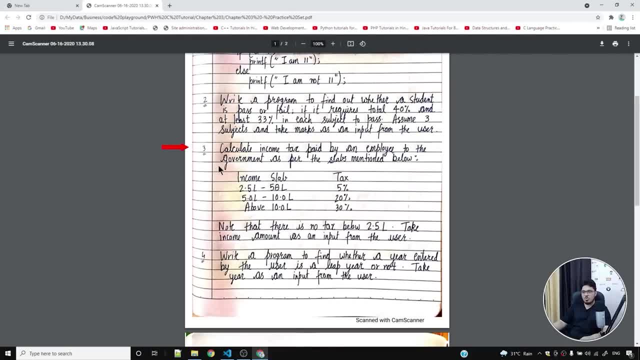 number two. we solved question number one. let's move on to question number three now. and it says: calculate income tax paid by an employee to the government as for the slips mentioned below. so income slab rates are these and tax is this. note that there is no text below 2.5. 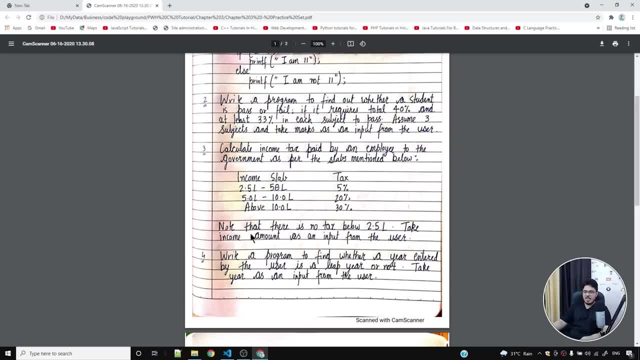 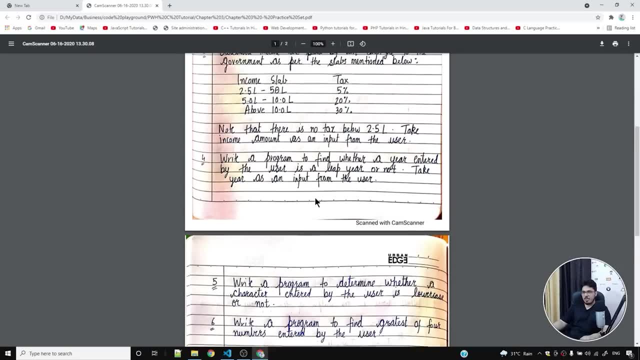 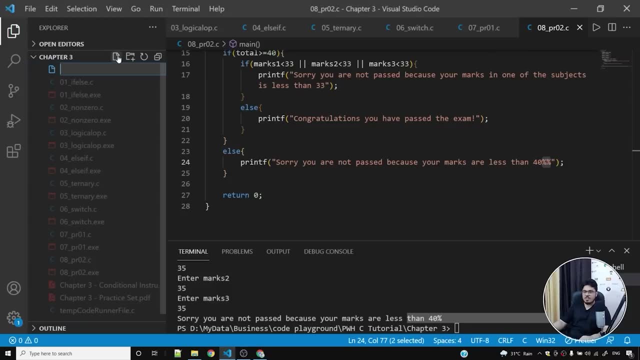 lakhs. take income amount as an input from the user. simply take the income amount from the user and you can write some logic to calculate the text. so let's, let's solve this problem. this is an interesting problem, so what we will do is simply create a new file. 09 underscore. 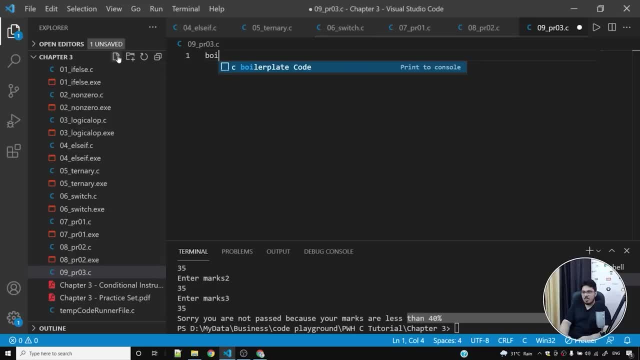 pr03.c, and we'll simply add some boilerplate code. we'll simply say: and you know what i'm going to do, i'm going to copy the printf and scanf from here and i'm going to create a variable tax and income. okay, so let's assume that the income is. 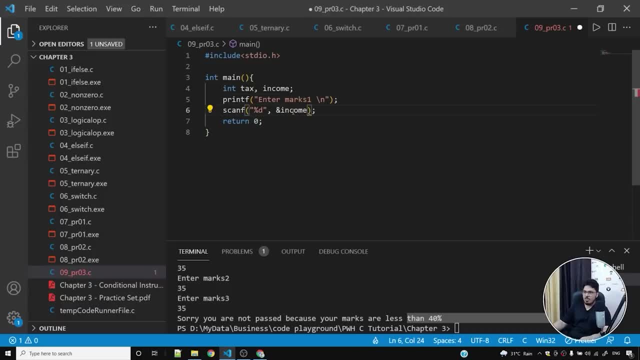 an integer and, uh, we'll see. if you want to make tax as float, so let's make tax equal to protections. so i'm going to blocked income away and i'm going to- Are you going tohalate this income as split, what you want to do? so i'm going to write share or transaction low of cut to. 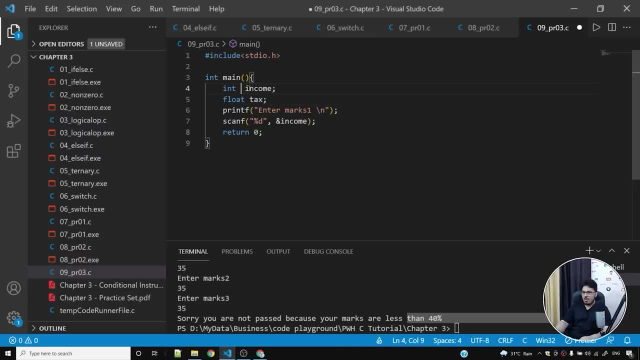 tax as float and let's keep on adding to text if the income is, um, you know, greater than 2.5. so if the income is, please enter um, enter your income, okay. so so the user will enter the income if income is less than 2.5 lakhs, or rather 2.5. 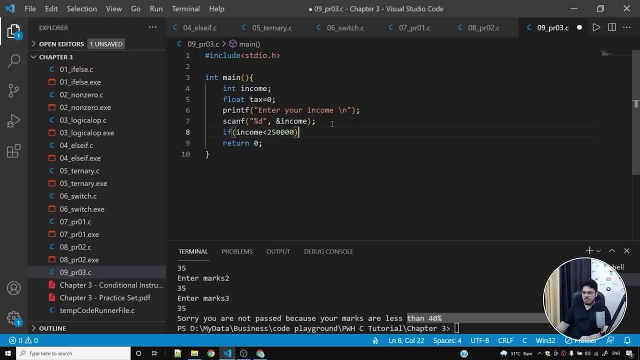 this is 2.5 lakhs. if this is the case, your income is less than, or equal to, or- let's keep it- less than 2.5 lakhs. so no text for you, okay? so, uh, since the tax from 2.5 lakhs to 5 lakhs. 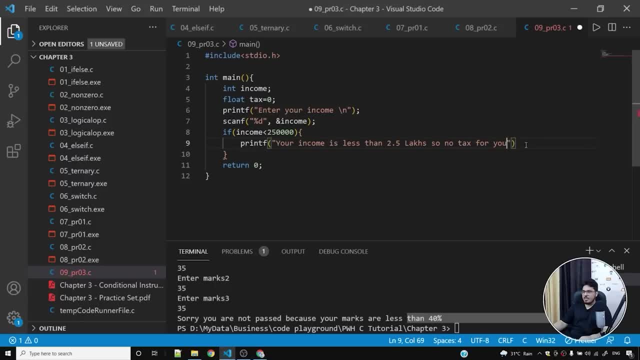 is five percent, what we'll do is, uh, we'll simply add zero to the text. if this is the case now, what we'll do is, if the income lies between 2.5 and 5, what we'll do is: we'll add that particular amount. 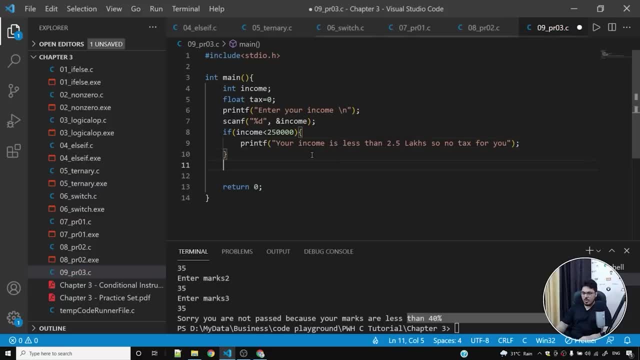 of tax to the user's income. okay, so what i'll do is i'll now type else if, and inside the if what i'll write is i'll say if income is less than 7.5 lakh, and it's greater than 2.5 lakhs. 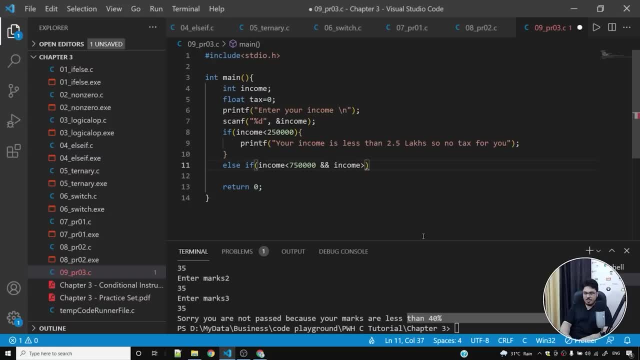 so i'll just type that. so i'll say: if income is greater than income is greater than 2.5 lakhs. now what will happen if i do this? so i hope i have put down the zeros correctly. yes, i have 4 plus 1. 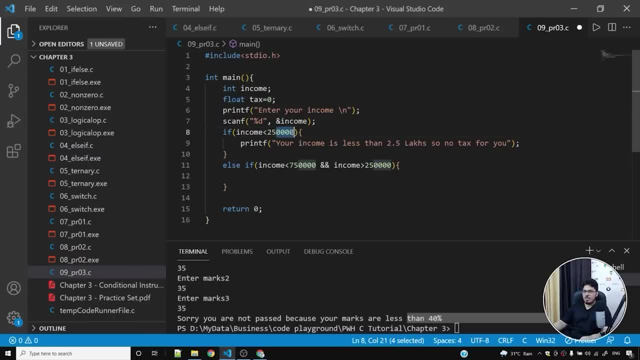 5, 4 plus 1, 5. yes, just make sure that you are typing the number of zeros correctly, okay? so what i'll do now is i will simply say your income is. your income is between 2.5 lakhs and 7.5 lakhs, so 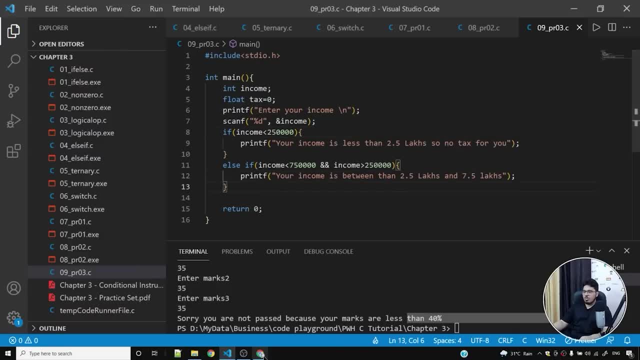 that's it. we are not going to see no text for you now. what we'll do is: we'll see: uh, or rather it was 5 lakhs. my bad, so i'll have to say 5 here, 5 lakhs and also 5 here. 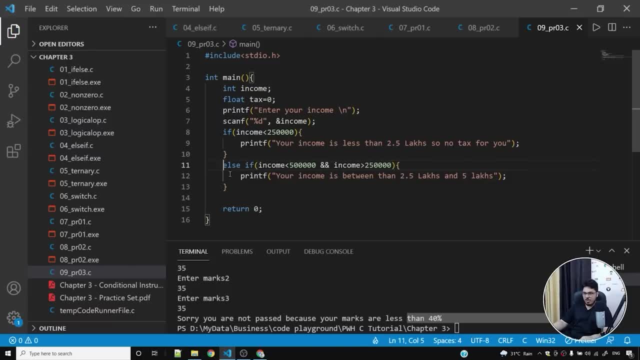 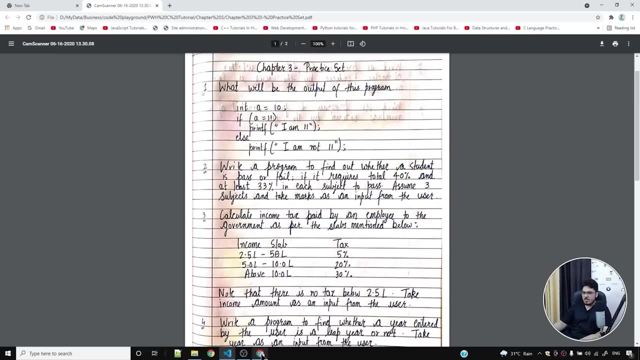 here, okay. so if this is the case, we'll do something. okay. now, if this is the case, where the user income is, uh, greater than five and it is less than, uh, say, 10 lakhs, okay. so if it's less than 10 lakhs, uh three plus one four. 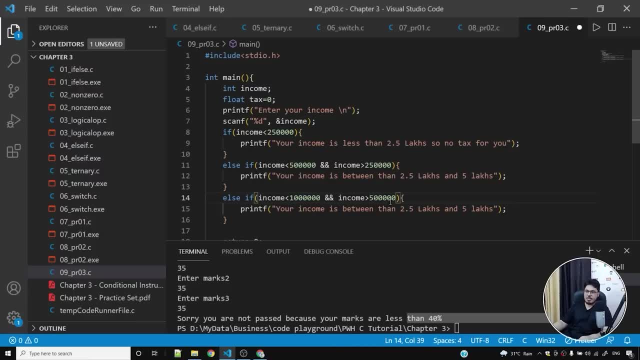 plus one five, three plus one, four plus one, five. so if it lies between five lakhs and 10 lakhs, what we'll do is we'll charge 20 of the ticks, okay- on this income. otherwise, what we'll do is, if the income is greater than 10 lakhs, what we'll do is: 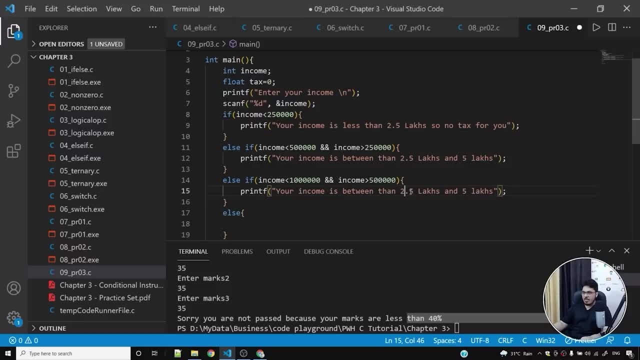 we'll charge the base amount and then we'll add 30 percent of tax to the remaining of the income. okay, so if this sounds confusing, simply take a piece of pen and paper and start writing whatever i'm saying, start calculating, use a calculator and things will start making. 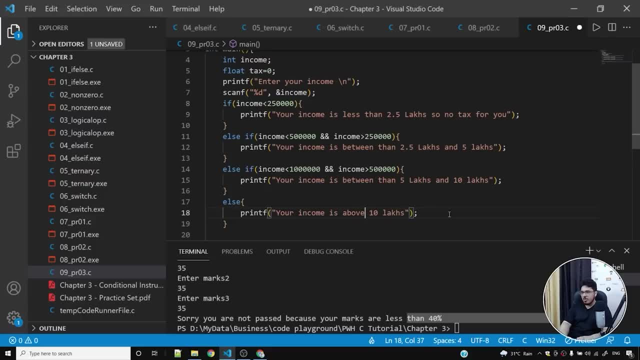 sense to you. so i'll simply say: your income is above 10 lakhs here. now let's add to the text. so when the income is between 5 lakhs plus 2.5 lakhs, what we'll do is we'll simply add something to the tax, so we'll say: tax equals to tax plus will add a value to the text and 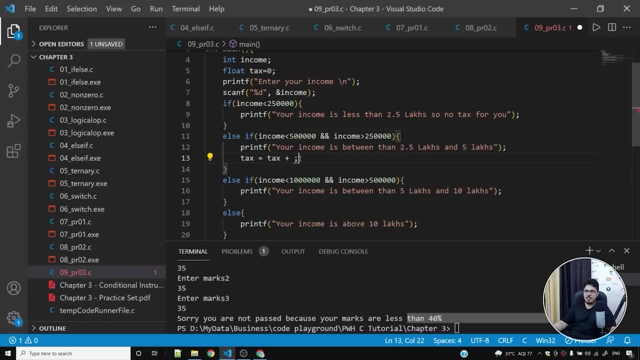 this is how you add value to a variable. so let us say the text was zero and i add five to it. so i'll simply say: tax is equal to text plus five and text will now become five because i have added five to the text. but how much will i add to the text? i'll simply add um. 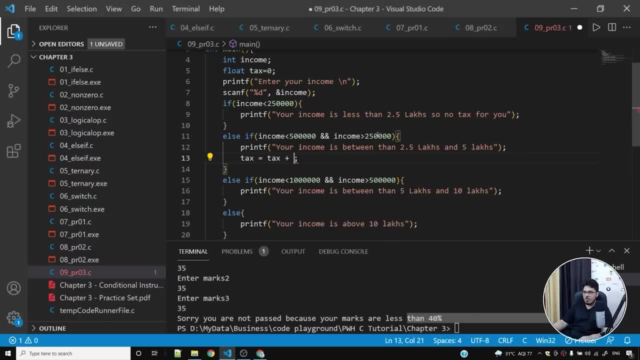 20 percent all the way to 5 lakhs, and i'll add 5 to거 ta Kevin Santat. i put 5 lakhs, I'll 20%, or rather 5% of the tax. So since the income is between 2.5 and 5,, 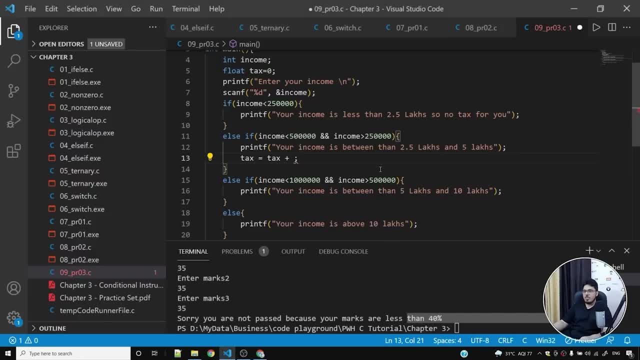 I'll simply add 5% of the tax. So what I'll do is I'll simply say 0.05 multiply by what is the income Income between 5 lakhs and 2.5 lakhs. I'll simply say income minus 2.5 lakhs. 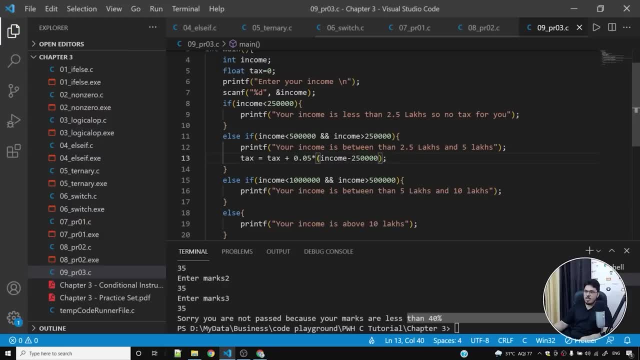 Why did I do that? Because I want to charge tax only on the income which is above 2.5 lakhs. So if you're earning 3 lakhs, I'll charge income tax on 50,000, because till 2.5 lakhs there is no tax. 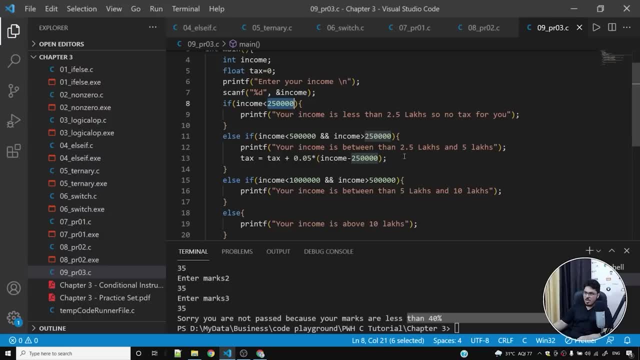 And after 2.5 lakhs, we have 5% of tax. okay, So this is how we calculate tax. Now, if the income is between 5 lakhs and 10 lakhs, what will happen is: I'll simply use how much. 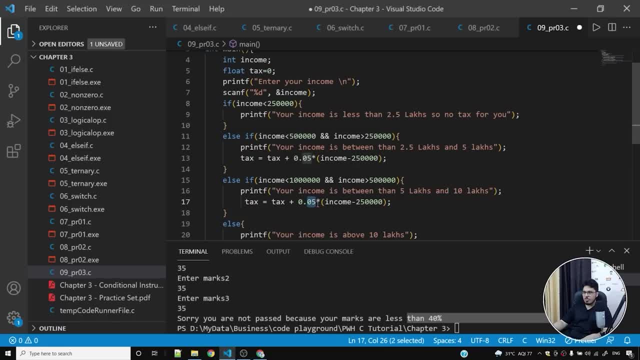 10%. Yes, no, 20%. So I'll simply say 0.02 this time. So I'll say 0.02.. Which is 20%, and I'll multiply this by income minus 5 lakhs. So, whatever you are earning above 5 lakhs. 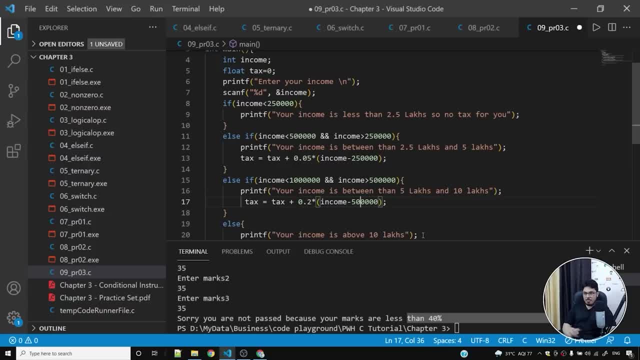 I'm going to charge you income tax on that, okay, But I also need to charge you income tax on- you know, your income- between 2.5 and 5 lakhs, So I'll add another tax for you, Let me. let me do it this way. 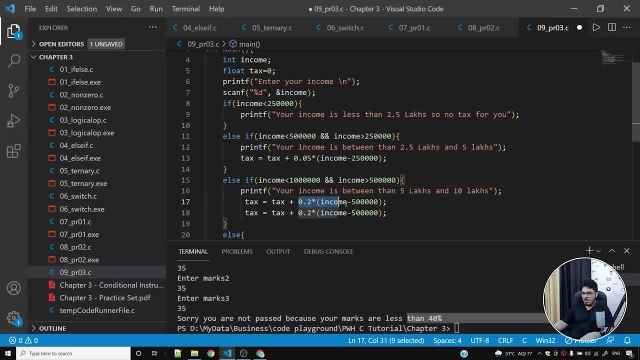 So I'll charge this much as well. So, on your income, between 5 and 2.5, I'm going to charge you 0.05, okay, So between 2.5 and 5 lakhs, whatever you are earning. 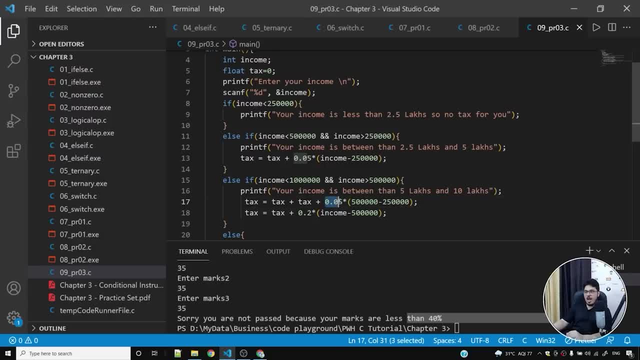 I'm going to charge 5% And between 5 lakhs to whatever you are earning. because your income is between 5 lakhs to 10 lakhs, I'm going to charge 20% on that And when you are earning above 10 lakhs. 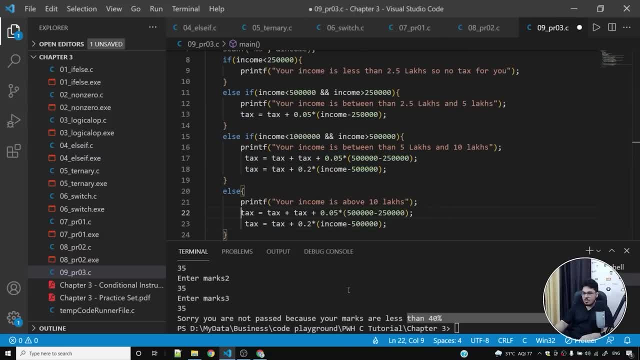 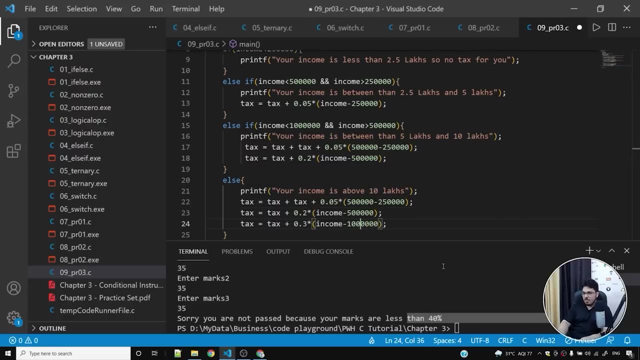 what I'll do is I'll simply- I'll simply say 0.05 on this, 0.2 on this and 0.3 on remaining of the income between 10 lakhs and above, And what I'll need to do is: 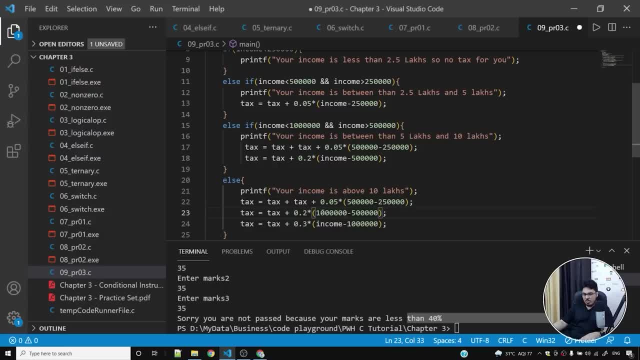 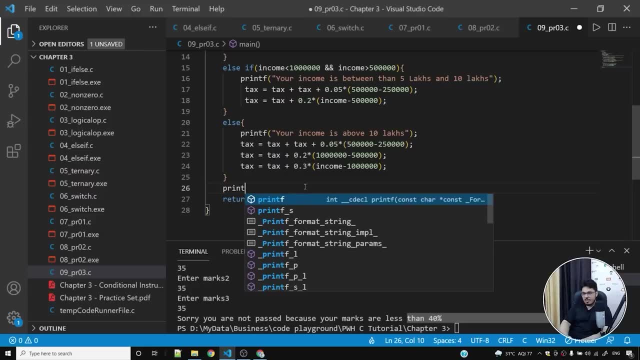 between your income between 10 lakhs, sorry, between 5 lakhs and 10 lakhs, I need to charge 20%. So this is going to be the total tax. Let's see what is the total tax. So I'll simply say: 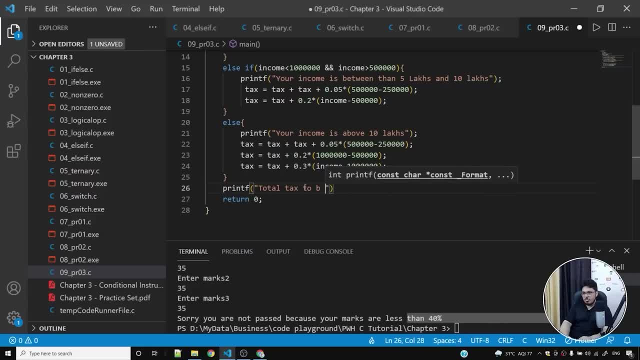 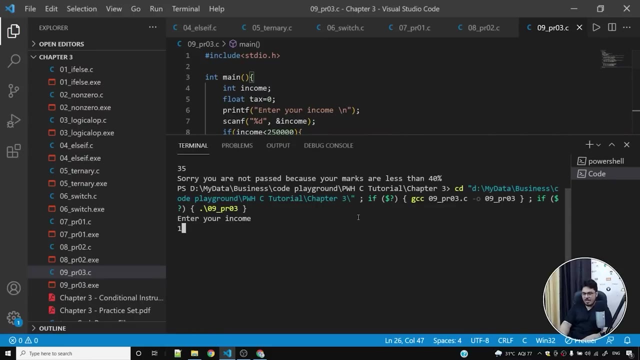 so I'll simply say total tax to be paid is percentage F And I'll simply say tax and I'll press. I'll simply press the semicolon. Enter your income: 10 lakhs, or rather 11 lakhs. 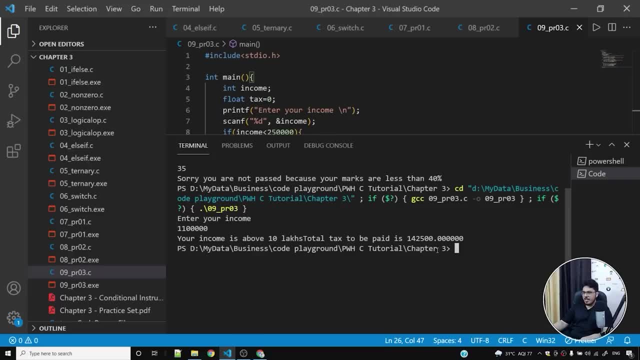 If I enter 11 lakhs, you need to pay this much in tax, so 3 to 5, so you need to pay 1 lakh 42,000 in taxes. okay, Now if your income is 23,000 rupees, 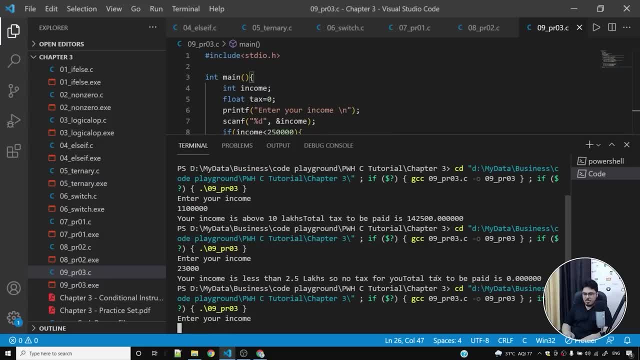 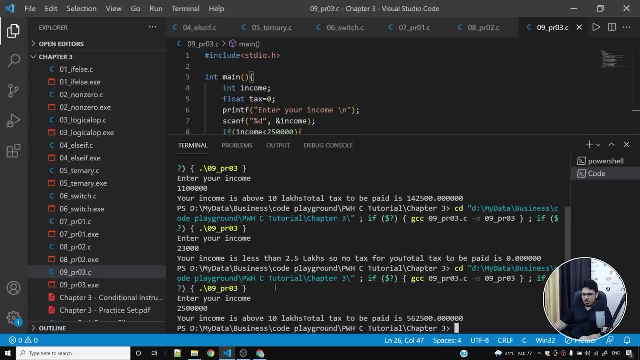 you need to pay zero tax. okay. Now, if your income is 2 lakh 50,000, you need to pay some tax. Your income is above okay, so I actually used an additional zero 3 plus 2, 5, I actually entered 25 lakhs. 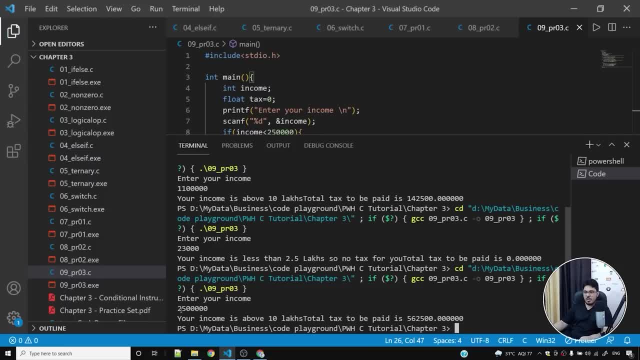 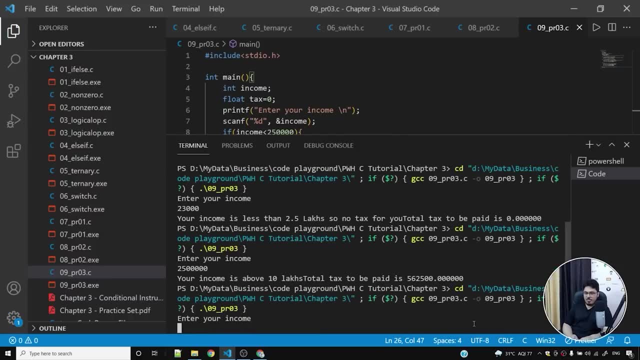 I should have entered one zero less. But again, if your income is 25 lakhs, this is the amount of tax you need to pay. You need to pay around 6 lakhs in taxes, okay. So if I enter my income as 2 lakhs, 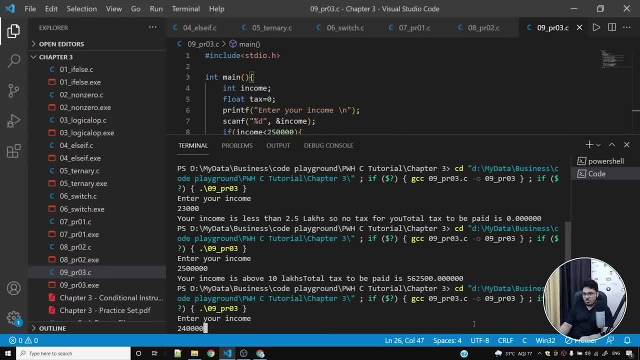 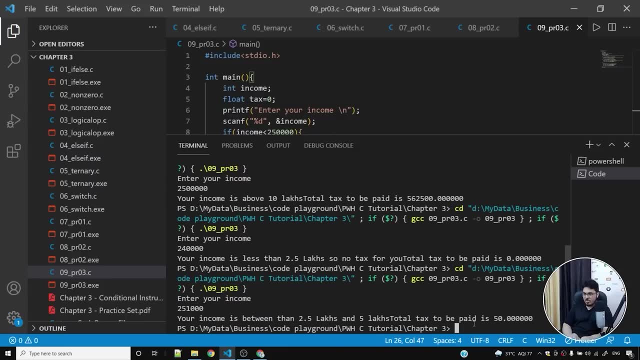 my income as 2 lakh 40 thousands. this is my income tax. And if my income tax is 2 lakh 51 thousand, you can see that the tax to be paid is 50 rupees, which is 5% of 100 rupees. 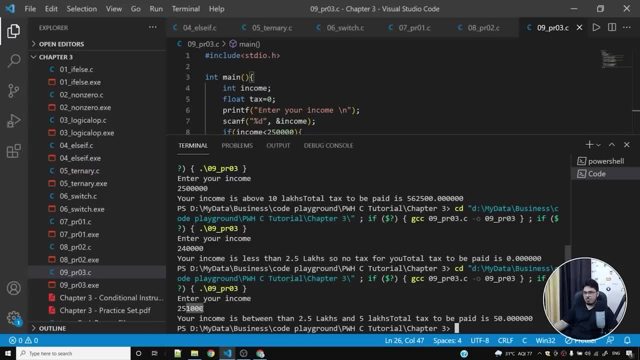 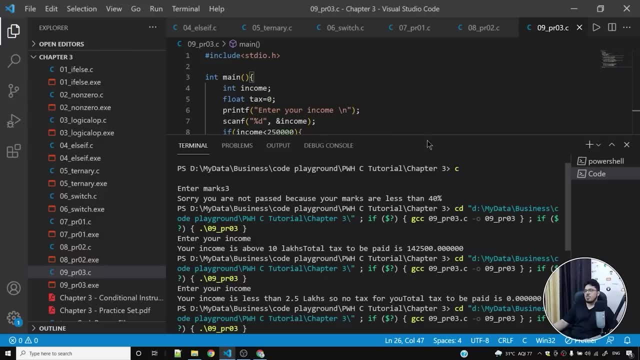 Sorry, not 100 rupees, 1000 rupees. 5% of 1000 rupees is 50 rupees. Yes, that's right. okay, So I hope you understood and I hope that this problem solved a lot of your existence. 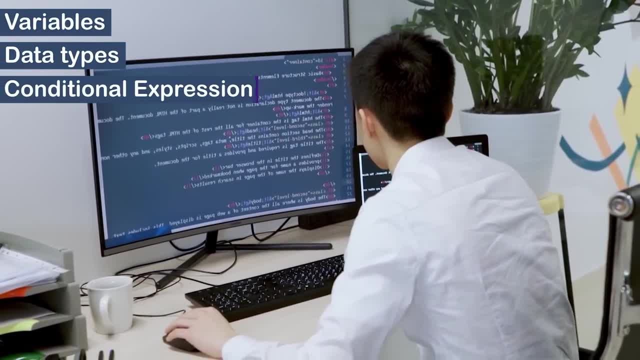 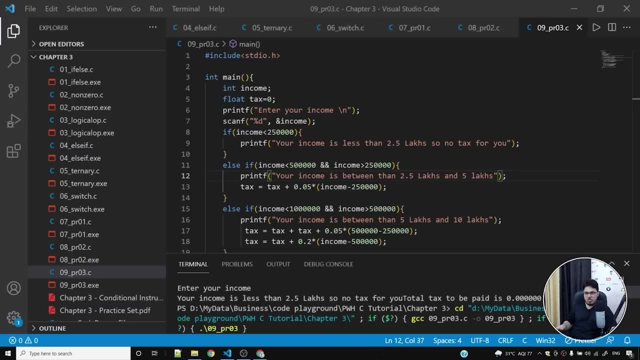 So I hope you understood that there are no existing doubts on variables, on data types, on conditional expressions. And if this program sounds haunting to you, watch the video once again, You know? just skip to where we started this question and start practicing this program yourself. okay. 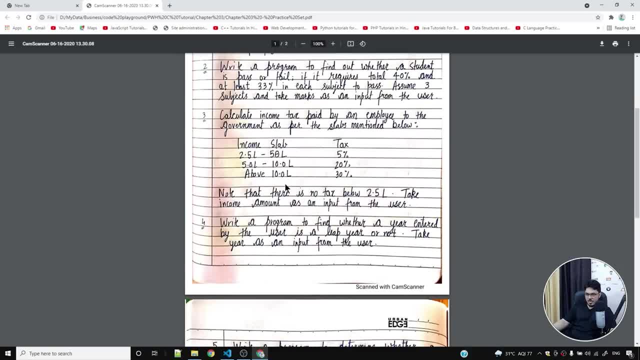 And things will start making sense to you. So this is how you calculate income tax. Once again, do not take this as you know, the accurate information, This is assumed information. I'm giving you a disclaimer: Google for the tax rates in your country. 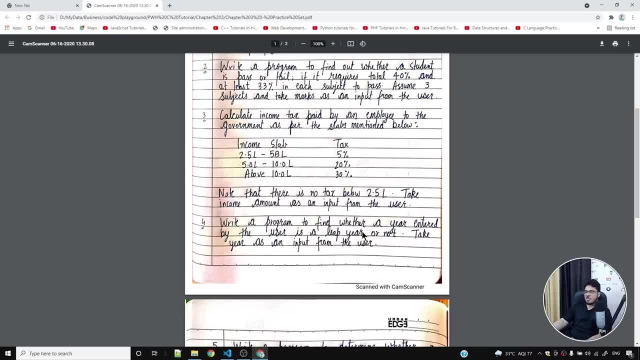 and you know, do not use this to calculate your tax. I know nobody will do that, but again, it's my duty to give the disclaimer. Now write a program to find whether a year entered by the user is a leap year or not. 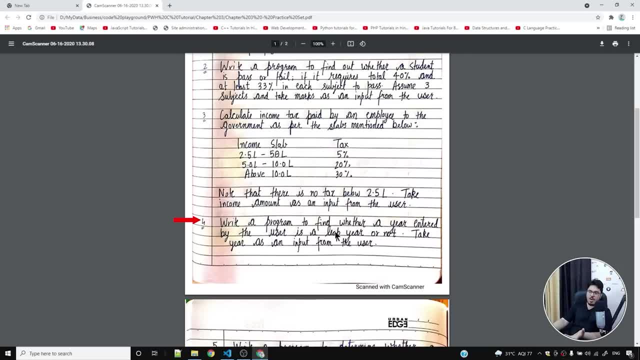 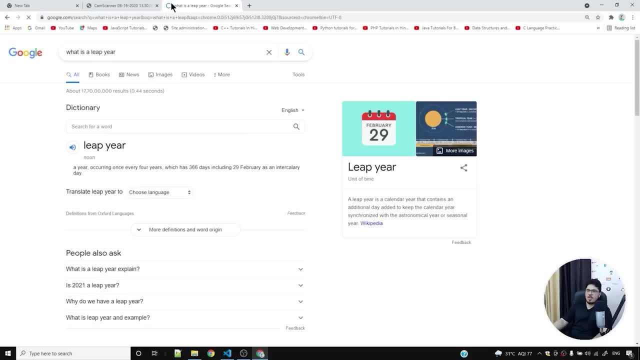 Take year as an input from the user. So in order to find out whether a given year is leap year or not, you simply go to Google and simply say what is a leap year, okay, And you'll get the conditions. A year occurring once every four years. 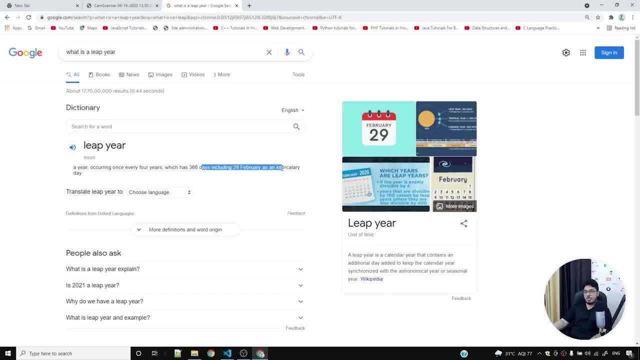 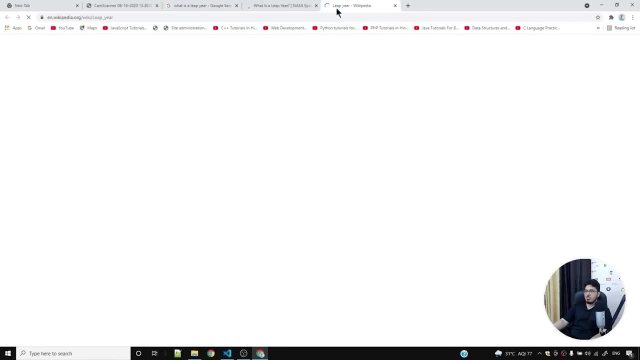 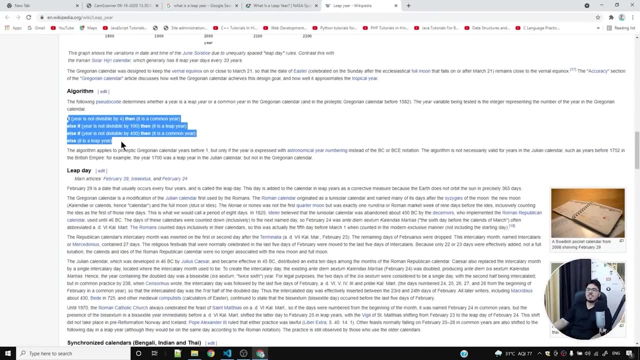 which has 366 days, including 29th February as an intercalary day. So if you go into detail and if you go to Wikipedia of leap year, there are some of the you know they have in fact written the algorithm okay. 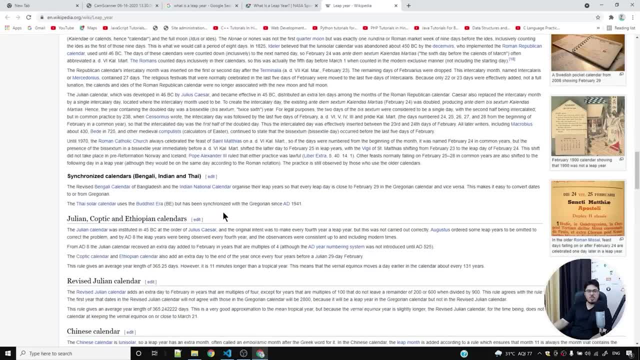 So I'm not going to you know, look into this algorithm. I want you to build the algorithm yourself, okay, And you can always look into the algorithm and if you type that, you are going to write the program accurately. But what I want you to do is: 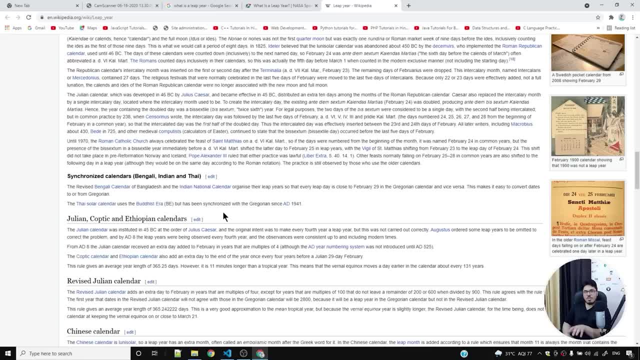 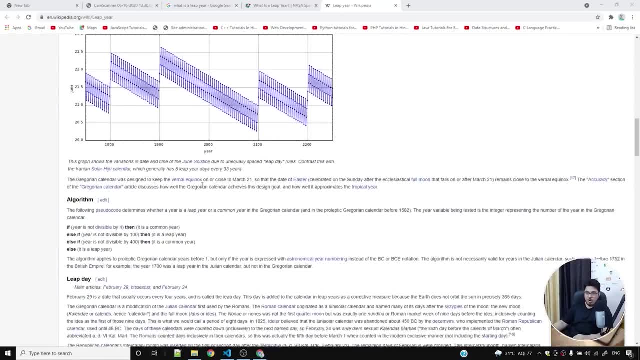 just think about what a leap year is and then, once you have an idea of what a leap year is, then start coding, and then you'll feel very confident after you write the program. Having said that, what I'll do is I'll simply copy this algorithm. 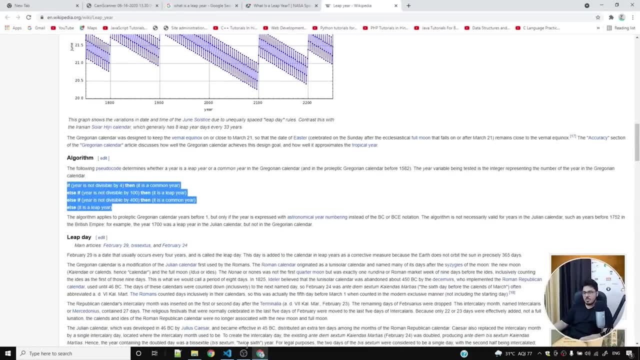 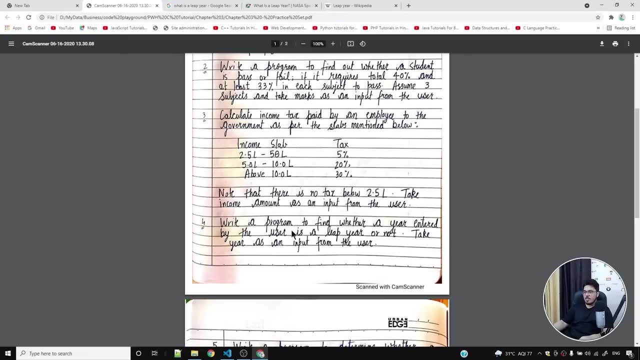 I just told you that you need to understand the algorithm, understand the process behind the algorithm, and then start writing the logic. But just for the sake of saving some time, what I'll do is I'll simply copy this logic and I'll start coding. problem number 4,. 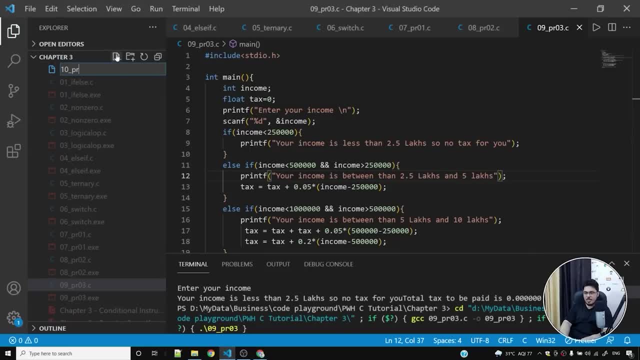 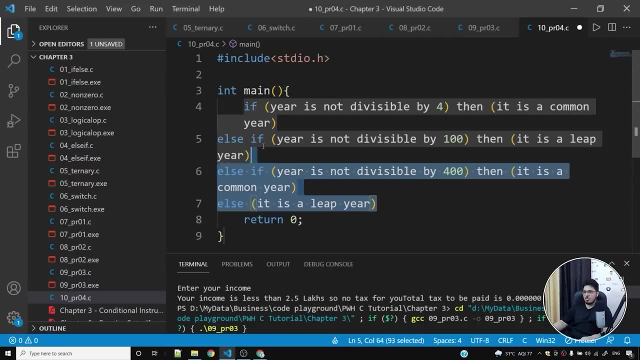 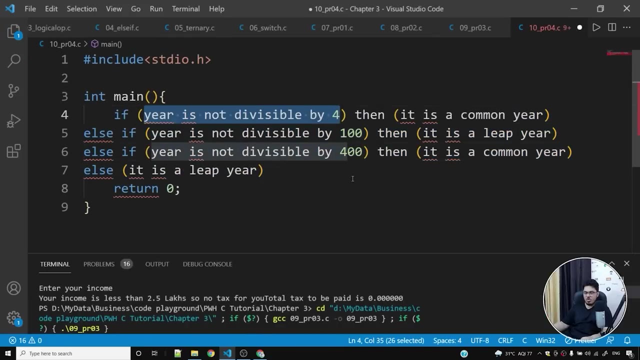 which is program number 10, pr04.c. and when you do something like this and you, you know, paste it, you're going to get a lot of errors. We need to fix these errors. It says year is not divisible by 4.. 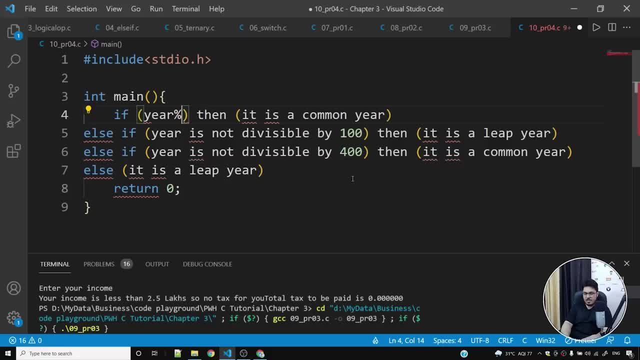 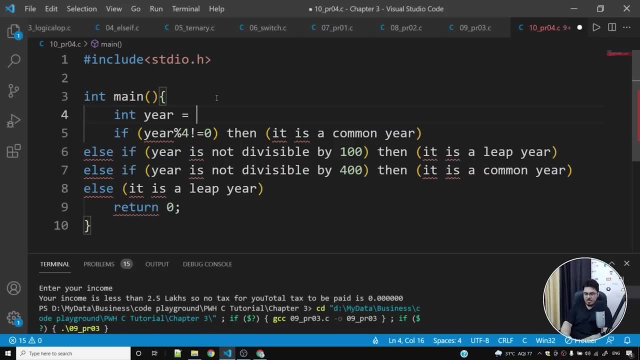 How do you say this? in C? You simply say year. percent 4 is not equals to 0.. It's not equals to 0. You can always say this. Let me say int year is equal to 3444 and I'll simply printf: 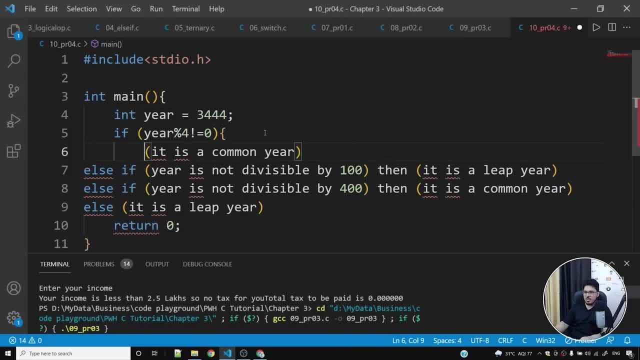 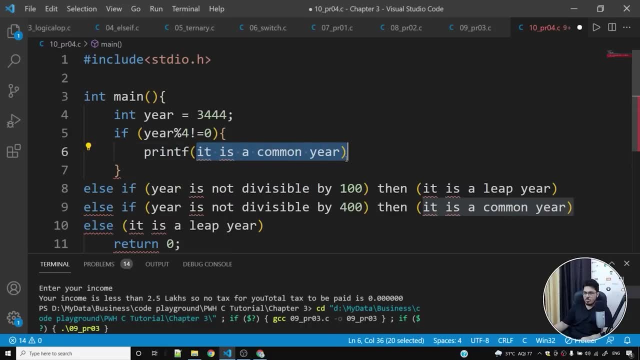 and say it is a common year. In place of then, what I'll do is I'll add these parenthesis and I'll simply say printf, and I'll add double quotes. I'll select this, add the double quote, and I'll do the same for these as well. 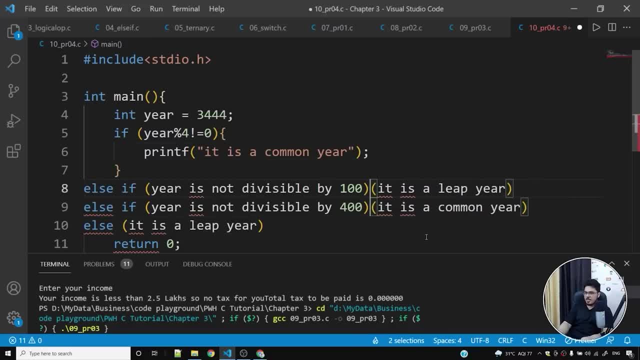 So let me do one thing. Let me start using multi-cursor functionality of VS Code. I'll simply say printf and I'll simply shift this. I'll add this. I'll press end on the keyboard. I'll use arrow keys Once again. I'll close this. 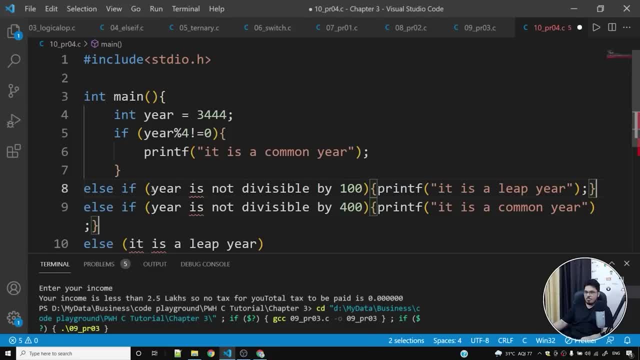 I'll add the semicolon, I'll close it like this. Now I'll do the same thing for this. I'll simply say: if year percent 100 is not equals to 0.. If year is not divisible by 100.. Year is not divisible. 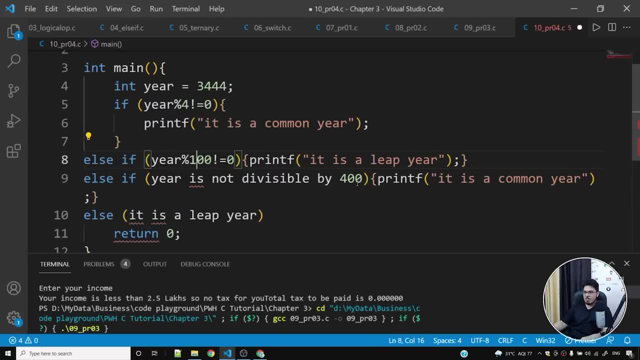 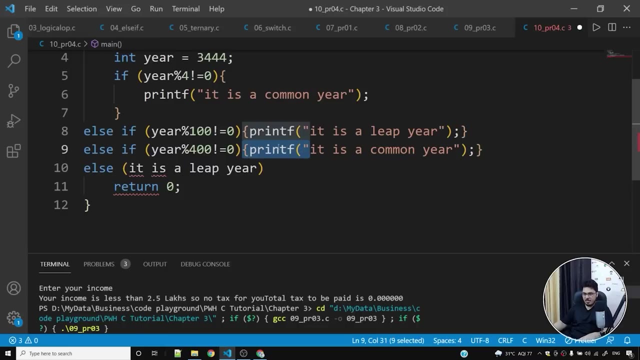 by 100. And if year is not divisible by 400. I'll do the same thing Divisible by 400. And once again, what I'll do is I'll say it is a leap year, so I'll simply copy this thing again. 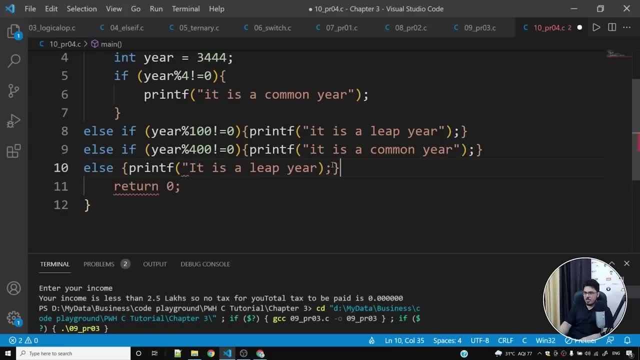 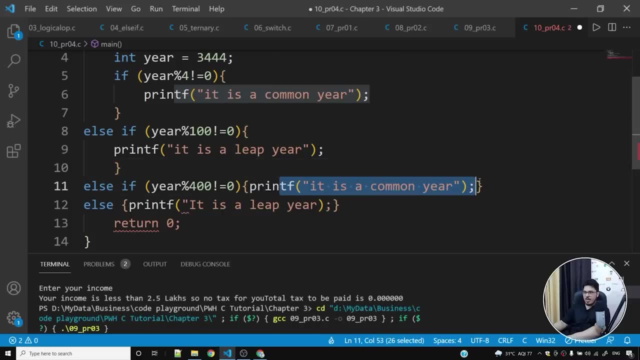 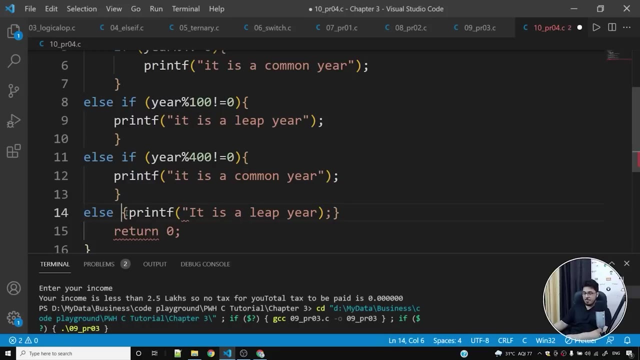 And it is a leap year. semicolon curly braces closed. You don't have to do like this. You can keep it this way and this program will work just fine. But again, it's a good practice to make your program look good with the indents. 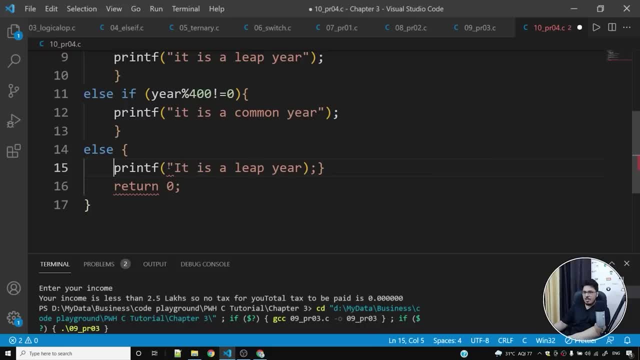 Let me add these indents to the program Printf: missing closing code. Am I making? Okay, I'm making this mistake. I'm not adding the closing code. I think everything is fine now And let me cross check the logic. The logic: 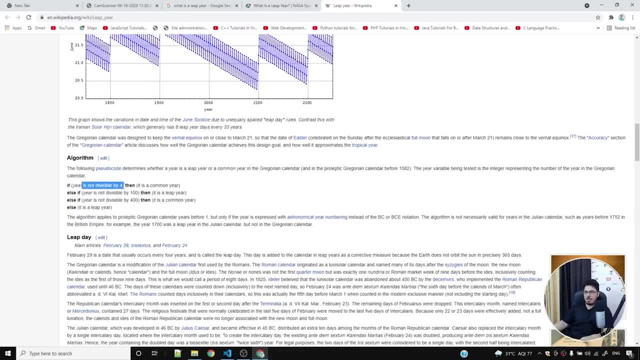 says that if year is not divisible by 4. Not divisible by 100. Not divisible by 400. Then finally, it will be leap year. Okay, So if it is not divisible by 100. And it is divisible by 4. It will be a leap year. So this is the. 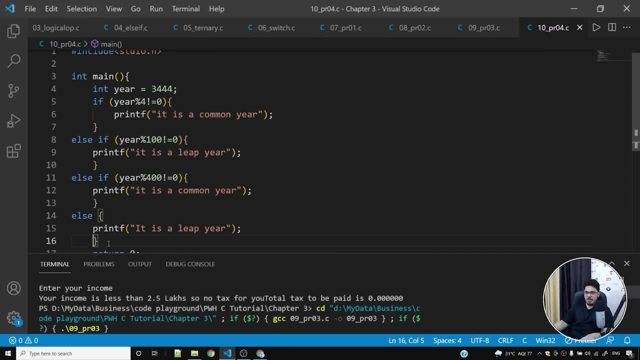 logic. So how this works, Let me explain it to you, And what I'll do is I'll add another indent, just you know, so that this looks good. You can always say: format document. It will format it in a good way for you. So 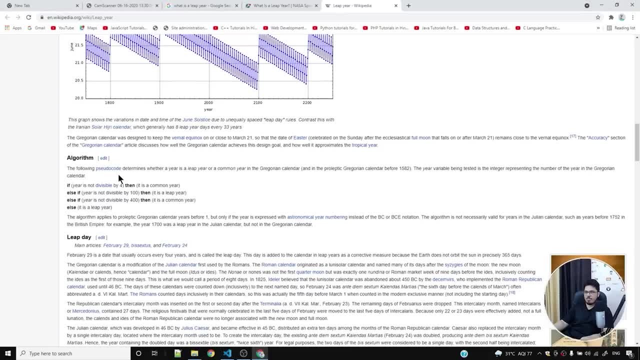 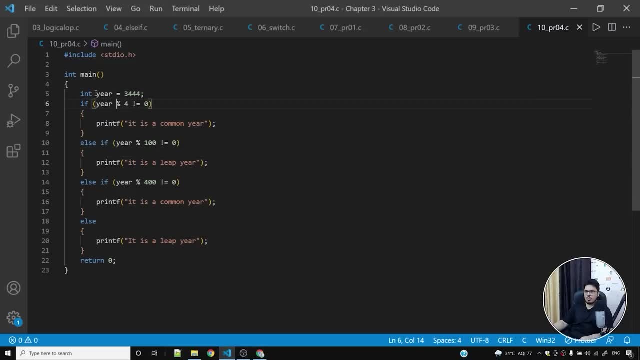 how is this logic working? So we have divisible, sorry, not divisible, Not divisible, Not divisible- And let me call it not equals to 0.. Okay, yeah, cool, So it is a common year. I've written the logic correctly. If the year 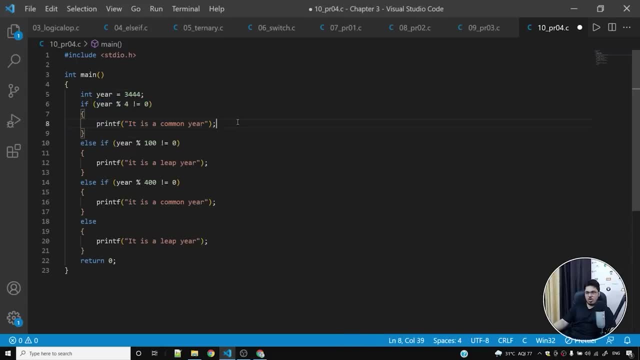 is 3, 4, 4.. It will check whether it is divisible by 4 or not. If not, it is a common year. It has to be divisible by 4 to be a leap year. But there are some other conditions which 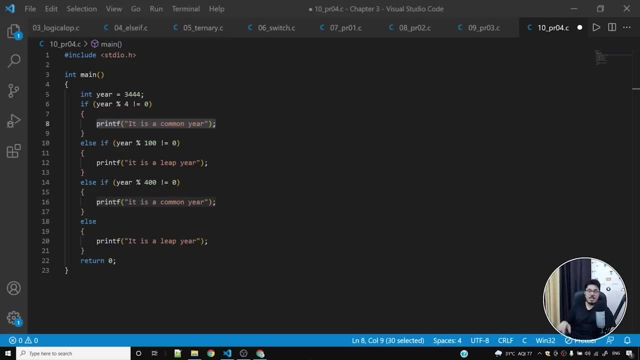 should be met for this year to be a leap year. So what we'll do is we'll check for all those conditions. We'll say: is it divisible by 100 or not? If it is not divisible by 100. Yes, it is a leap year. 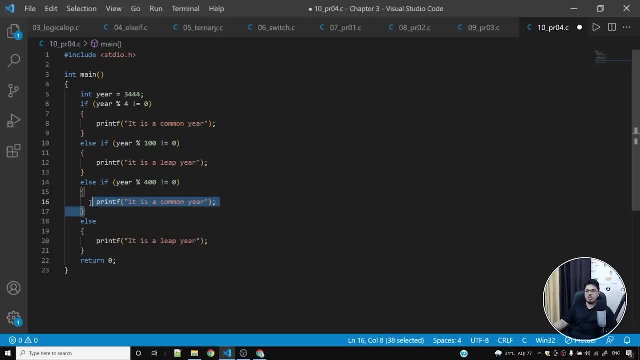 Is it divisible by 400 or not? If it is not divisible by 400, then it is a common year, But if none of these conditions are actually getting true, then it is a leap year. Okay, so what happens is if it is divisible by 4, which means this is false. 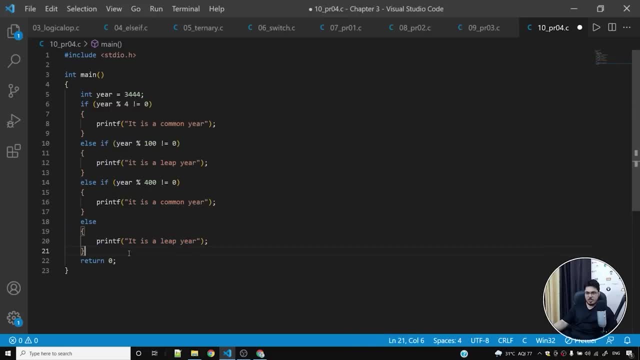 This is false. This is false and finally, it will be a leap year. Okay, just think about it and start relating your program with the actual logic of things. So you should have the logic of leap year ready. and then, once you have the logic of leap year ready, 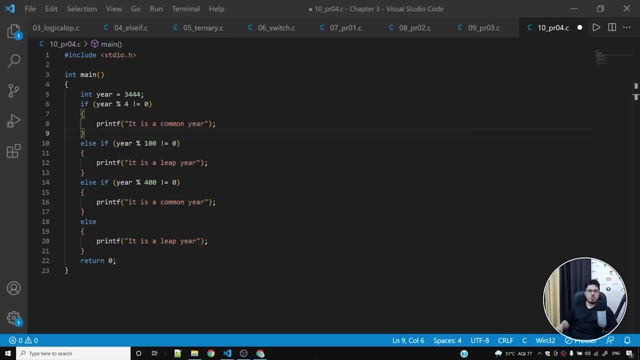 you write the program and then it will start making sense to you. So one of these if else, if else, if else will be executed. Just look at this program in this way and it will be super simple, Moving on towards the next problem, And the next problem is really very 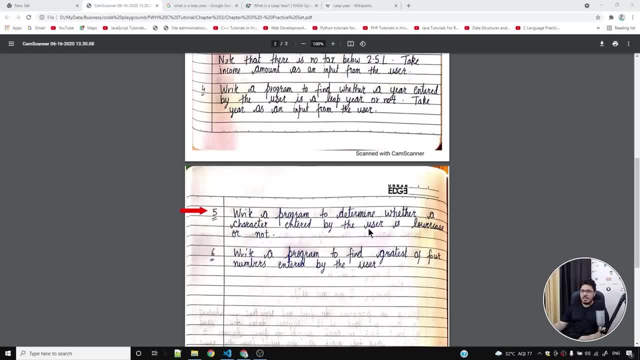 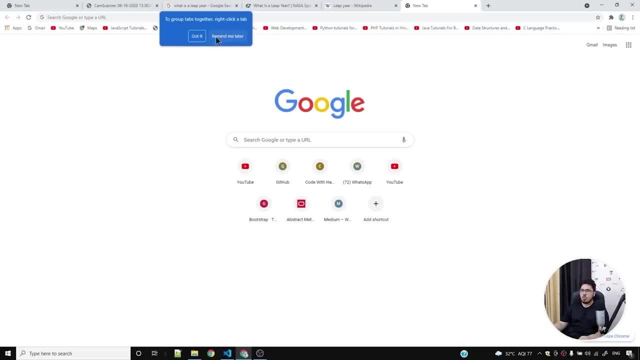 simple and straight forward. It says: write a program to determine whether a character entered by the user is lower case or not. So let me tell you something: Whenever you write a character in C language, Let me show you something. I'll simply type. 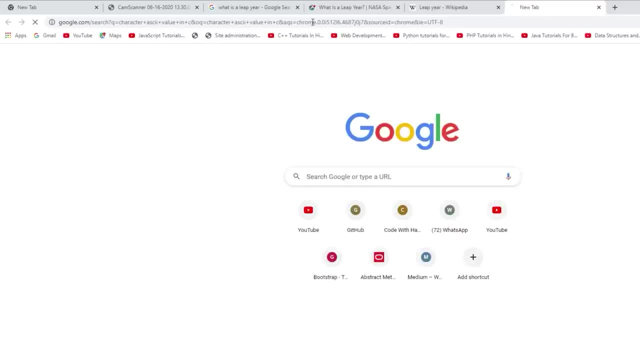 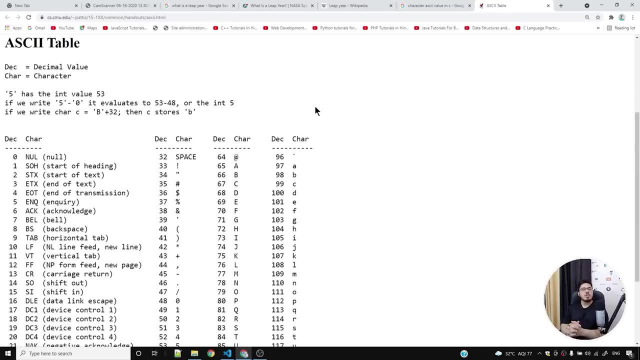 character s key value in C. Okay, what I'll do is I'll say: simply use this s key table and what this s key table is. let's try to understand this first, and then we'll solve the question. So s key table is nothing but some. 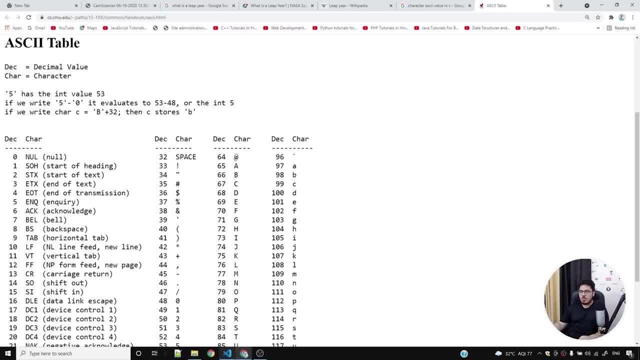 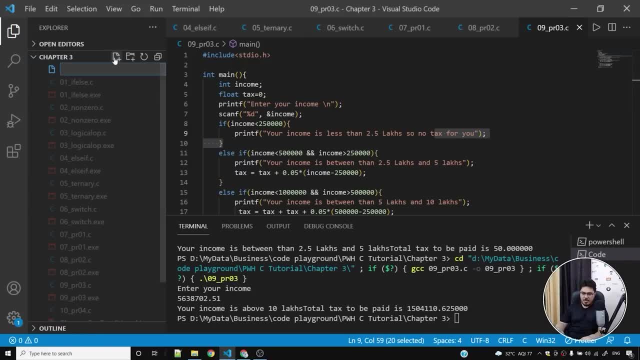 values which are mapped to the characters. So let me show you something, Okay, and once you have, you know, a good understanding of that, then you'll be able to solve this question. So let me create 11th program, and it's pr 0, 5, dot c. 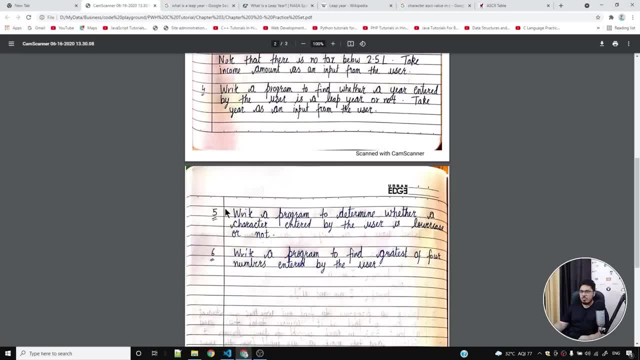 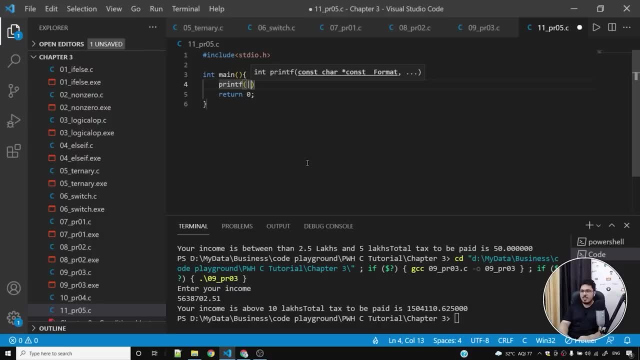 if I'm not wrong, It's problem number 5, if I'm not wrong. Yes, So let me show you something. Let me put this boilerplate code and let me show you something. What if I say something like this? I'll say: 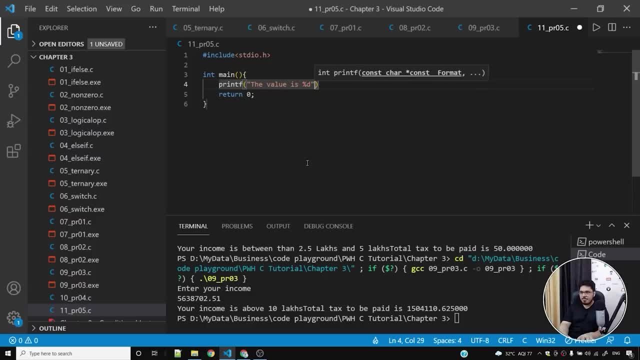 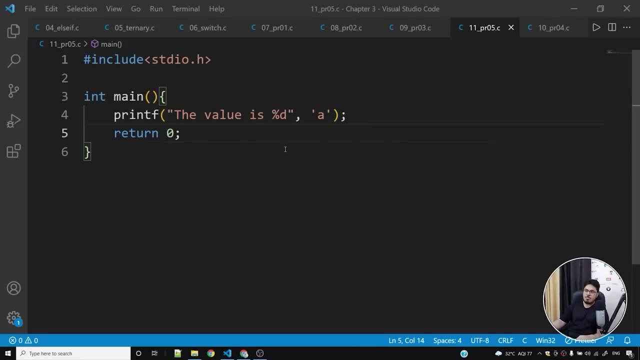 the value is, I'll say percentage d and I'll simply say a character, a, which is a. Now listen to me very carefully. If I run this program. This is not an integer, by the way. Let me tell you this is a character, but if I hover over it, you'll see. 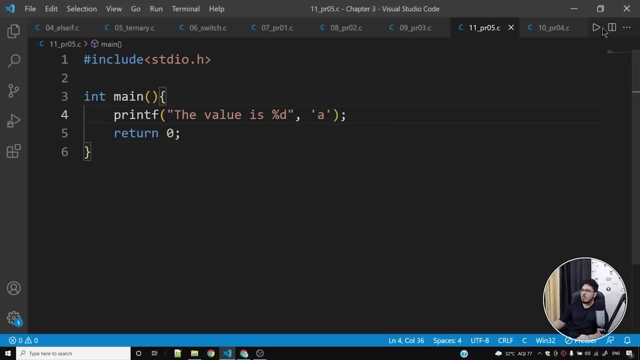 that it is an int with a value 97. Let me run this program for you and show you that it indeed prints 97. So a character is stored as an integer in c in the form of sky value, and if I say percentage c, then I'll be able to see a. 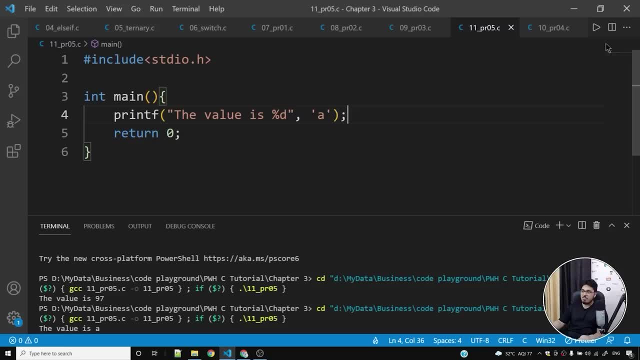 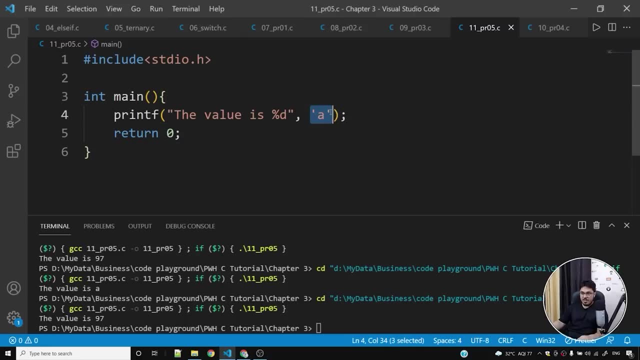 But if I do percentage d, then the s key value of this particular thing is 97, which is being printed. So whenever you are writing this literal, whenever you write this character literally, what it means is it means that it is an integer with the sky value. So you can. 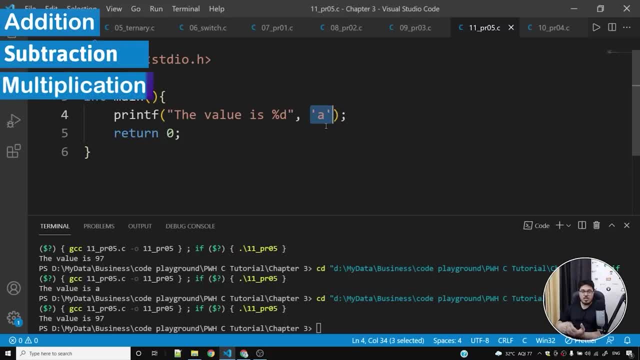 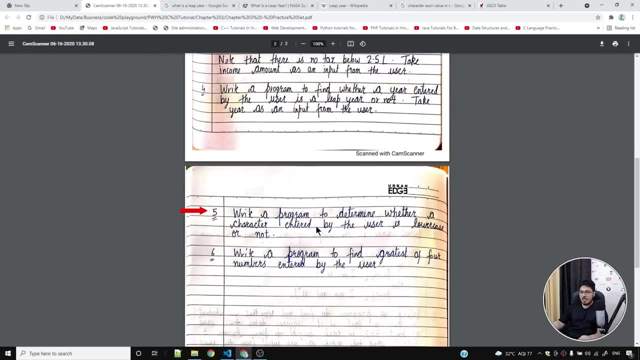 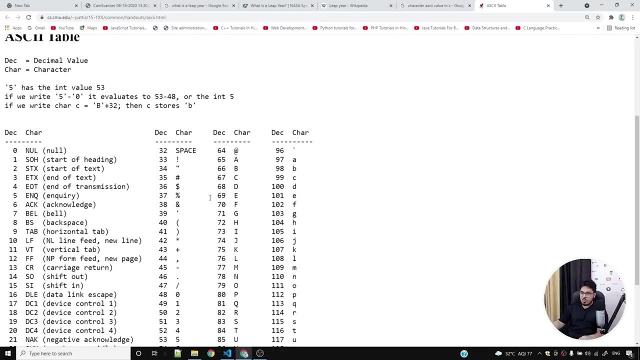 perform addition, subtraction, multiplication and division with all these values. Okay, let me show you how. So now we have a program to determine whether a character entered by the user is lowercase or not as the question. So this is the question. We have to solve this question. So let's look at the 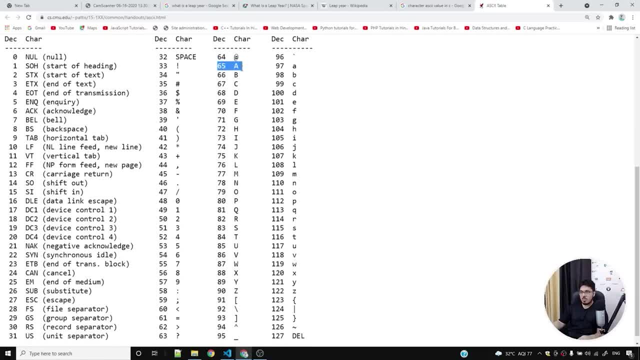 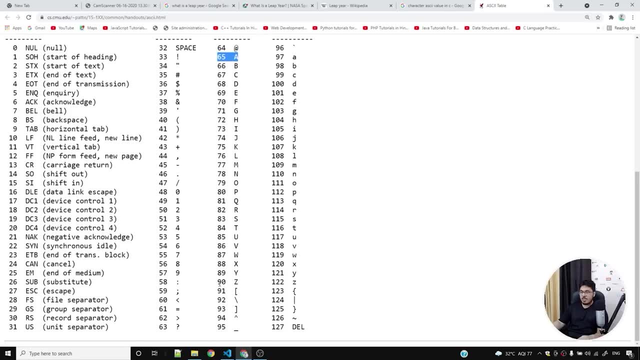 s key table, and let's see where abcd is, you know, being started from. It's being started from 65 and it's going all the way till 90, or rather 90. Okay, not even 96. So if a character is lowercase, 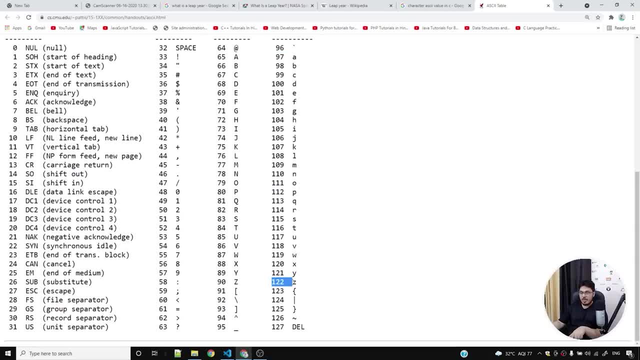 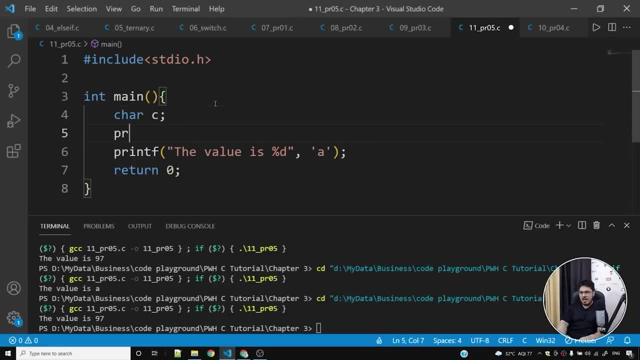 it has to lie between 97 to 122.. So that's all. That's a check. I'll say: enter your character. So let me say char c. I'll say printf: enter your character and definitely backslash n. Okay, and once I 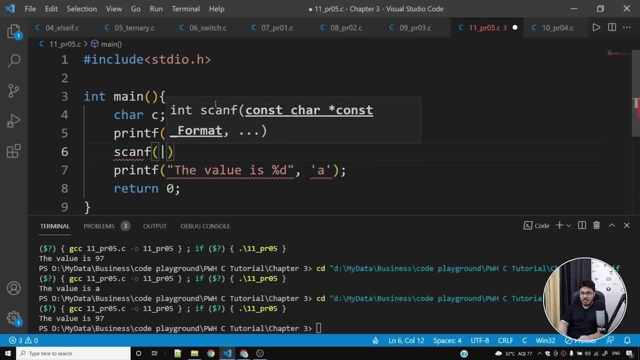 do that. I'll use scanf and I'll say percentage c. note that it's not percentage d. you need percentage c and am percent of c, Where c is the character. Let me change it to char so that you don't character. Let me change it to character so that you have a good. 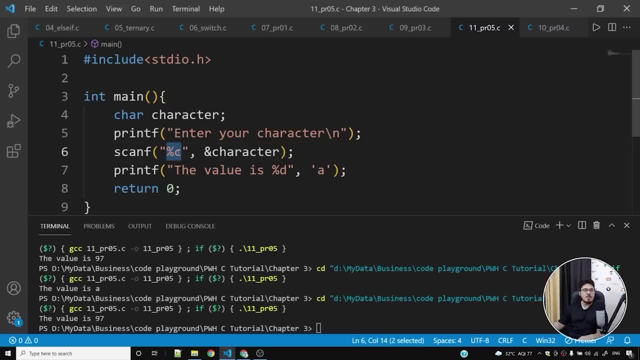 idea of which one is variable and which one is format specifier. So we have this as a print statement and we are taking character as the input from the user and the moment we do that, what will happen is we are going to check whether this particular character 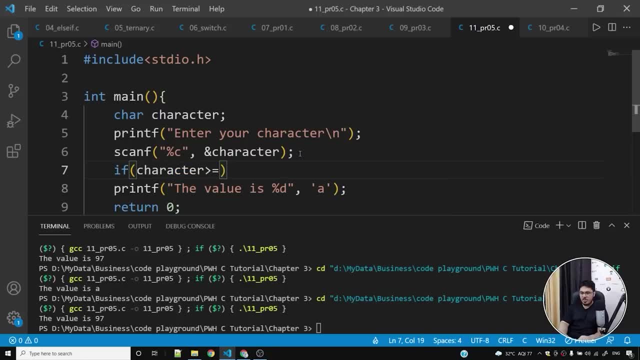 is greater than or equal to, what is greater than or equal to 97, and also we need to check if this character is less than or equal to what: 128, if I'm not wrong, 122. yes, I'm wrong 122.. You don't have to. 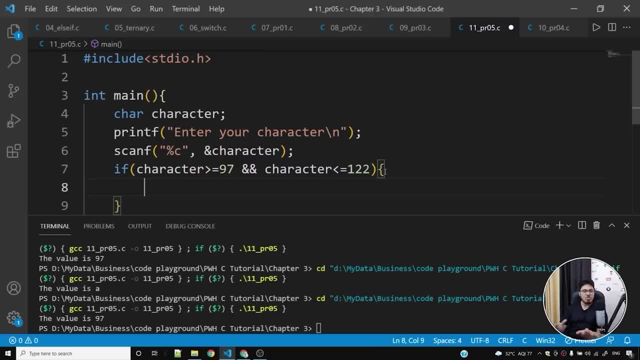 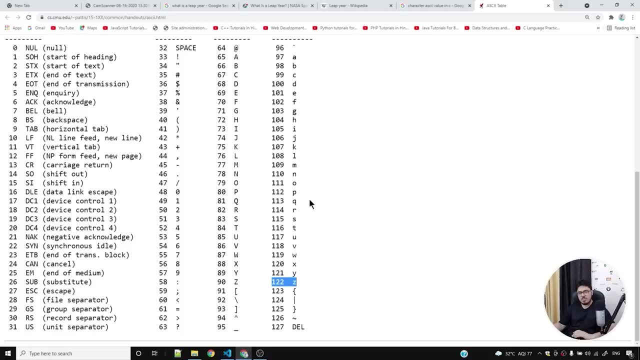 remember this. You might think that I don't even remember a sky table. I don't have to remember a sky table and you also don't even have to remember a sky table. Some people prefer to remember, and even some schools and colleges. they say that you know, remember the. 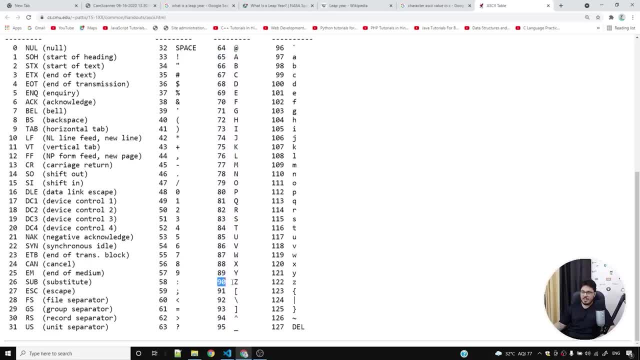 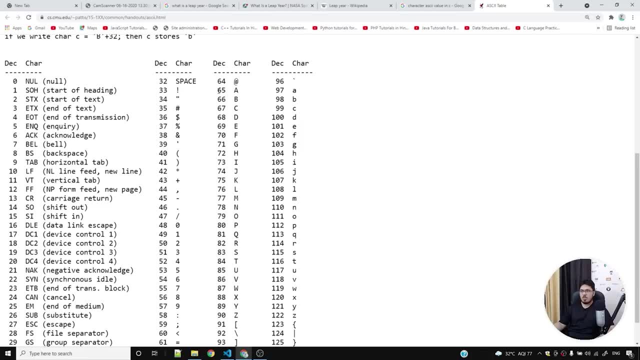 ASCII value of 65 and the value 90 and you know you add 32 and you get this particular value and this particular value respectively. So if you add 32- you know- to 65, you will get this. So whenever you have to convert a character from uppercase to lowercase, 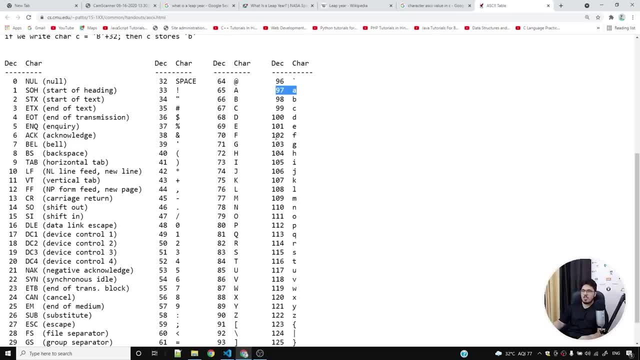 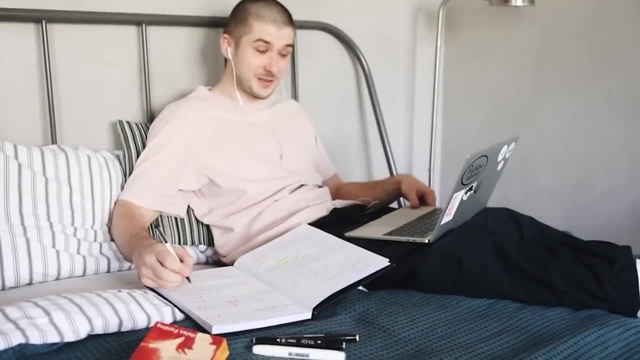 you simply add 32 to the value and you know you get the character which is lowercase version of the uppercase character. So you can do all those things, but I don't. I don't think that you have to remember anything. if you remember 65, well and good for you. You can. 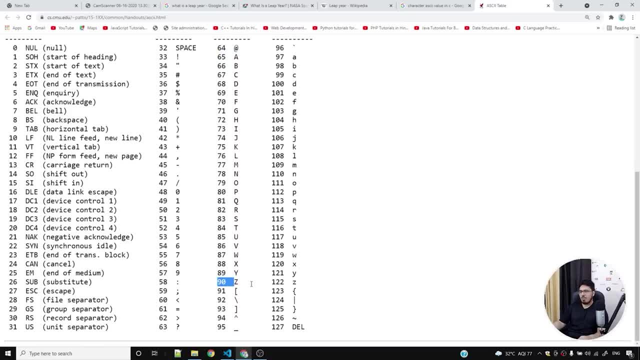 easily come to 90 if you have 65 and also you can easily come to this thing- 98 and you can easily- sorry, 97 and you can easily come to 122 by counting from A to Z. so if you remember 65 and 32, 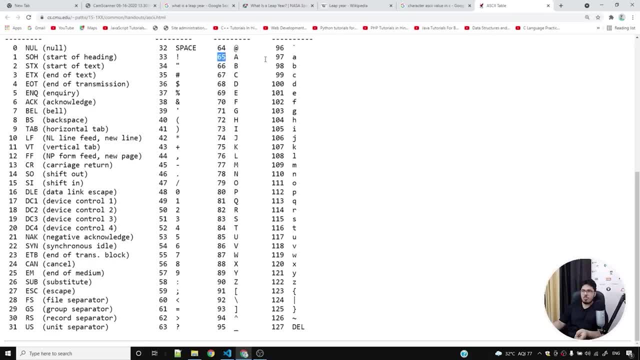 just remember these two numbers: if you add 32 to 65, you will get this, and if you add, you know. if you start counting from A, B, C, D, all the way till Z, you can come here and similarly, you can come to this value if you start counting. 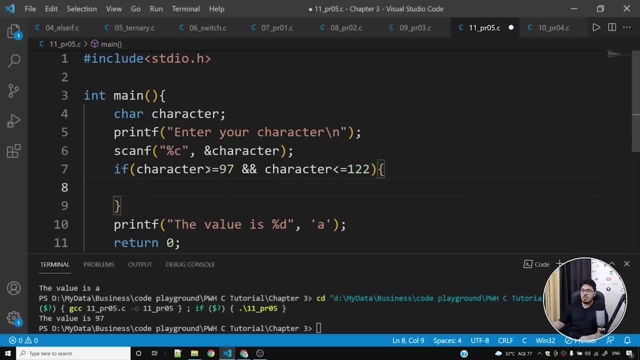 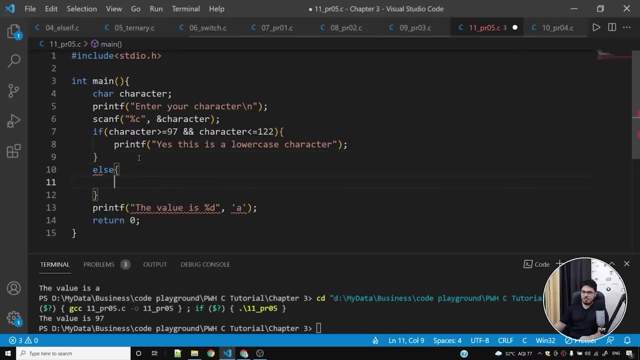 from 97. okay, but coming back to the question, we have to check whether a character is greater than or equal to 97 and less than or equal to 122. I will say: printf: yes, this is a lowercase character. and otherwise, what will I do? I will say: 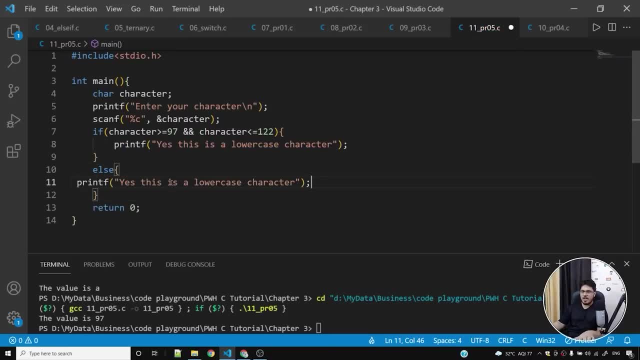 I will remove this. I will say no, this is not a lowercase character. so let me do something like this: I will say no, this is not a lowercase character. and let me run this for you and your character 5: no, this is not a lowercase character. capital A: no, this is not a lowercase character. 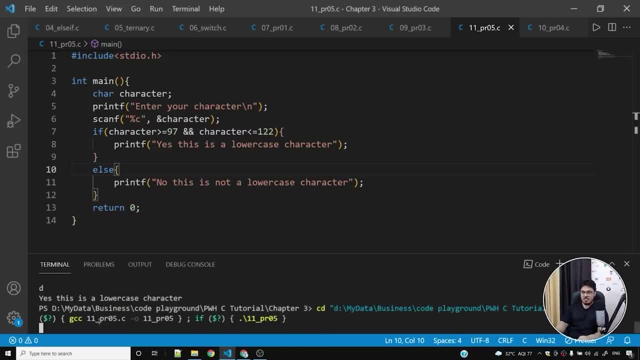 small a: yes, this is a lowercase character. small d: yes, it's a lowercase character, capital D- no, this is not a lowercase character. V- lowercase character, capital V, not a lowercase character, and so on. you can, you know, I can keep on going for 3-4 hours, but I will not. 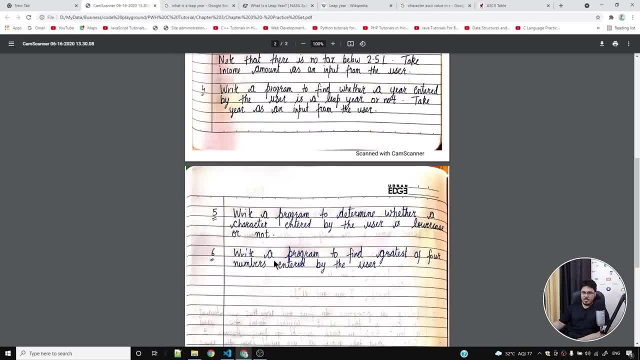 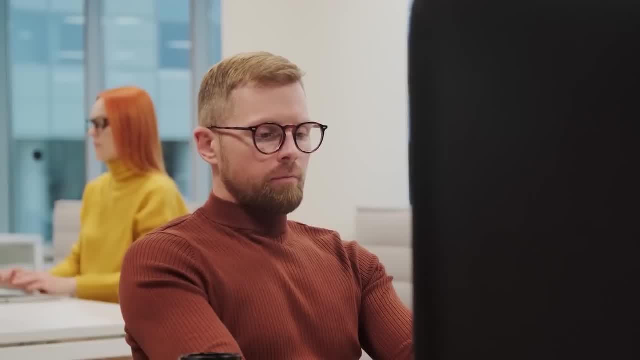 coming back to the question, coming back to the practice set, question number 6: write a program to find greatest of 4 numbers entered by the user. and I think this is the easiest problem of the practice set, because if you have a little bit of, you know. 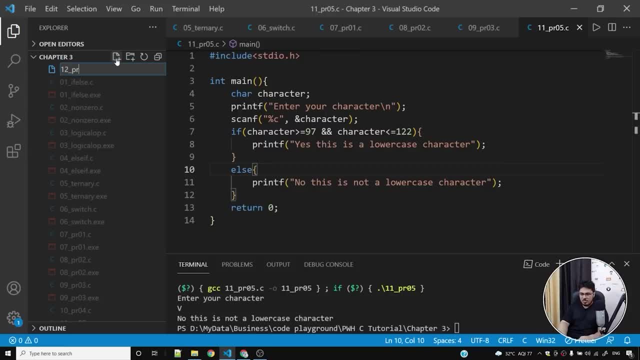 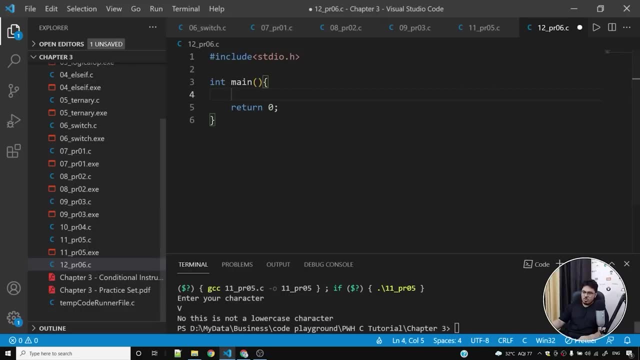 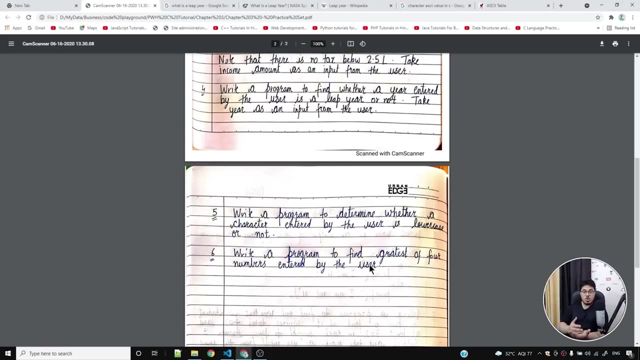 logical mind, you can definitely do this. this is problem number 6, pr06.c and the boilerplate code. so let me tell you how you can solve this problem, how you can find greatest of 4 numbers entered by the user. let us say you have 4 numbers. let us say you have. 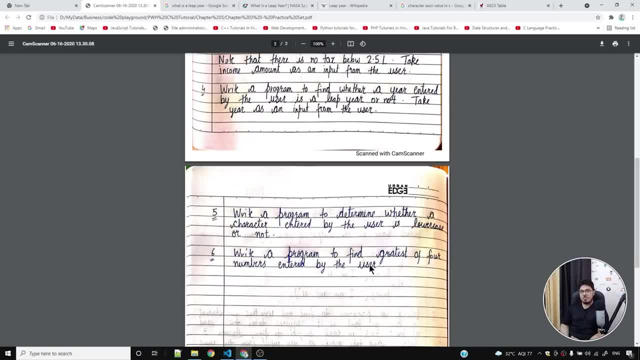 4 fighters. you have 4 of your friends and they say that I am the strongest person in the room. so what you do is you make 2 people fight and then you make 2 people fight again. they both will fight and the winner of this 2 and the winner of this 2. 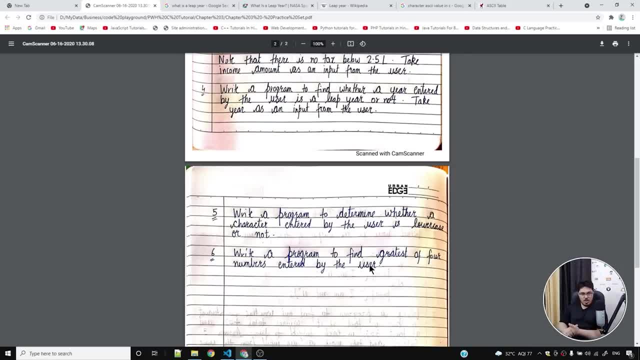 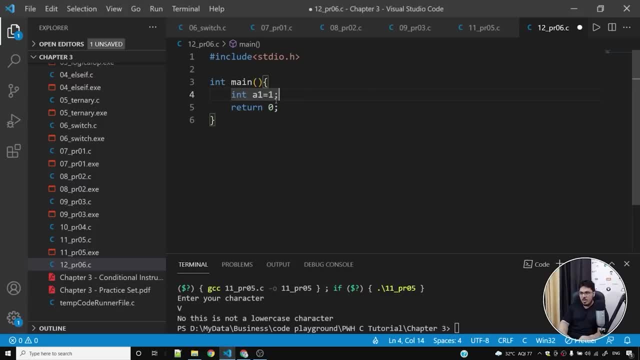 will fight with each other and they will find out who is the strongest of all. so we will do the similar thing here. we will take 4 numbers. so let me say in a1 is equal to 1, and let me do the same thing for a2, a3. 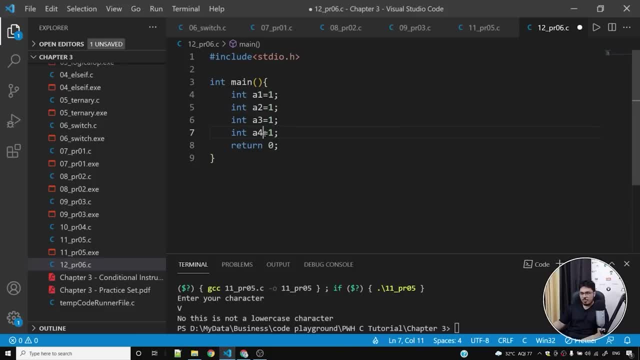 a4 and a4. let me, you know, assign some random values to these variables. now, what I will do is I will say: if a1 is greater than a2, ok, and if a1 is greater than a2 and a1 is greater than a3. 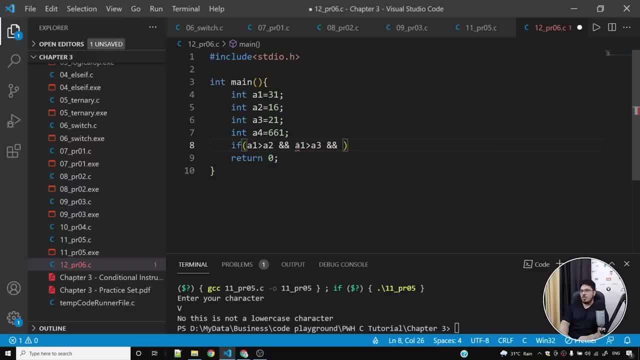 and also a1 is greater than a4, who will be the winner? a1 will be the winner. I will say a1 is the greatest and a4 will be the winner. ok, and you can do the same thing for all the values. so let me show you. 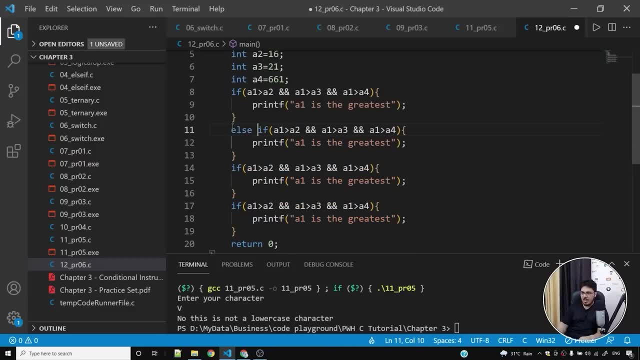 how you can do, how you can have you know, if else, if else, if else, if ok. now, if a1 is greater than a2 and a1 is greater than a3, then a1 is the winner, and if I do the same thing with a2, 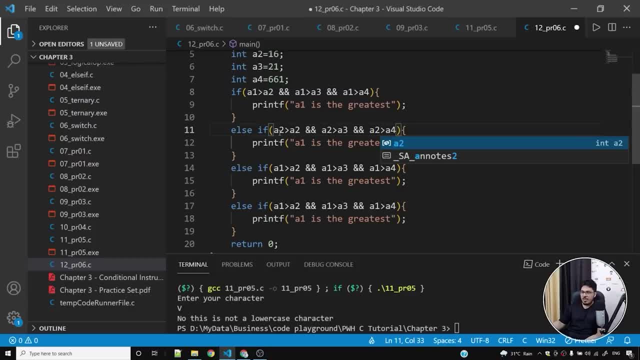 a2, a2 and we need to compare a2 with a1, a3 and a4. similarly, we need to compare a3 with a1, a2 and a3 with a2, a1 and a4, and then a4 with a4, a4. 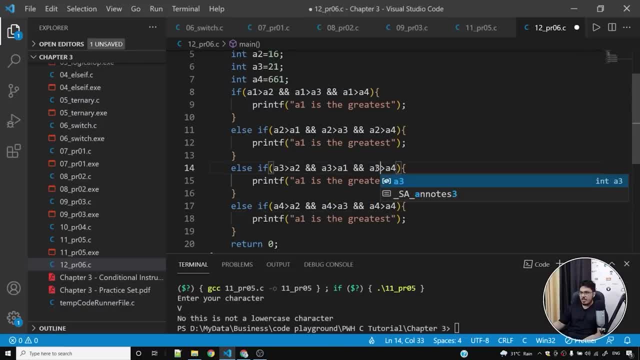 and here also I need to make it a3. a3- here I am checking if a1 is the winner, here I am checking if a2 is the winner, here I am checking if a3 is the winner, and here I am checking if a4 is the winner. 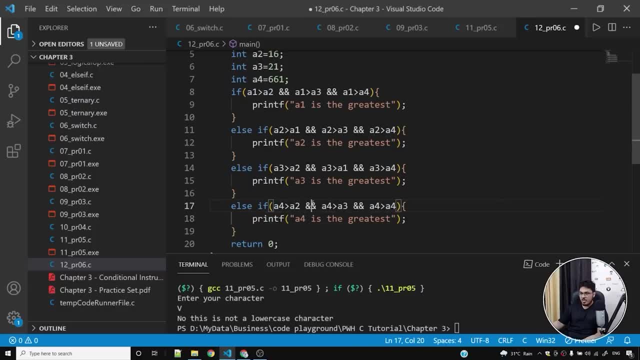 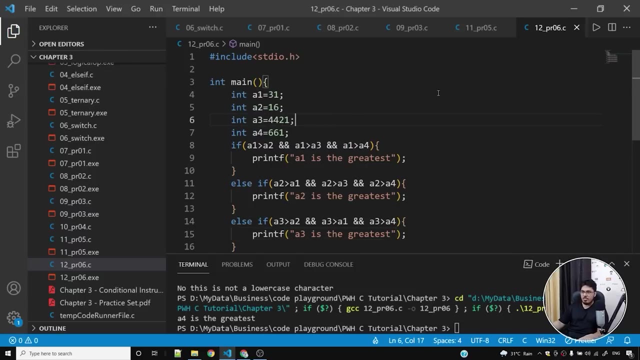 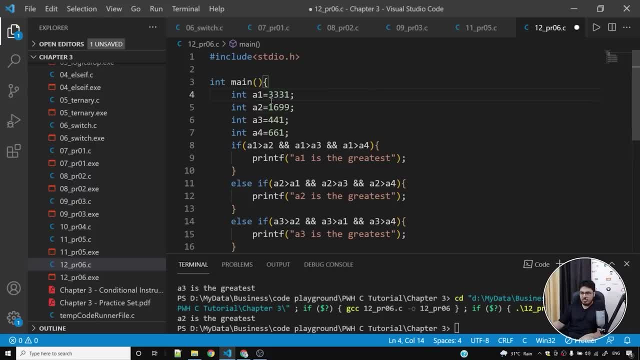 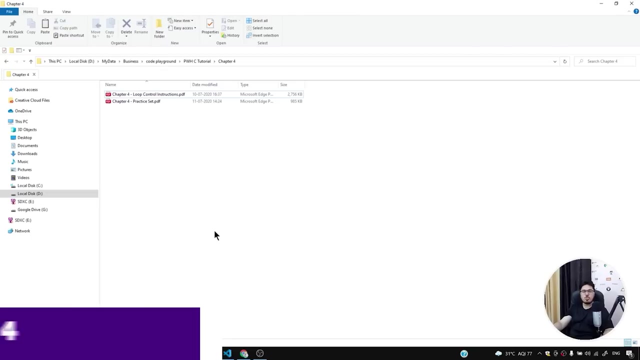 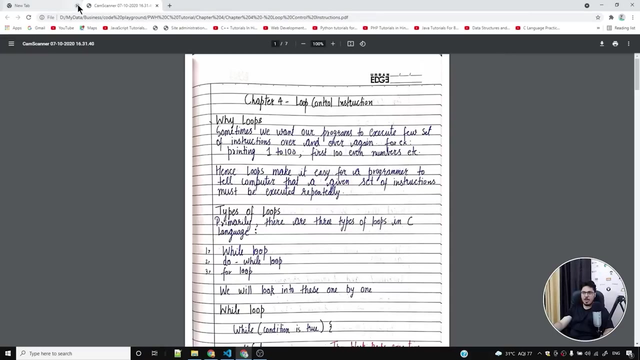 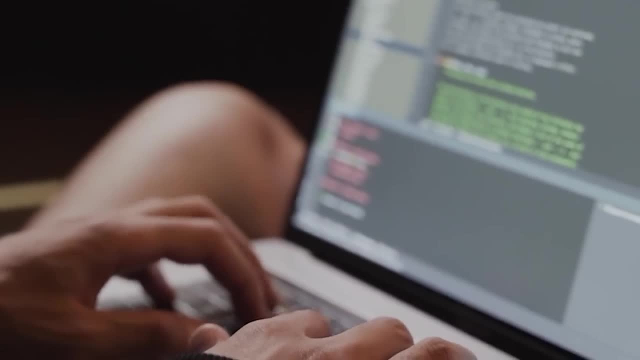 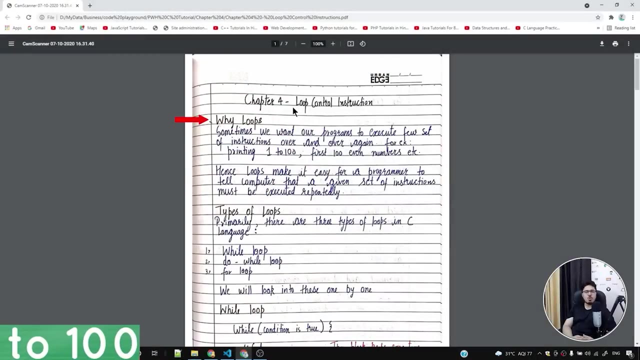 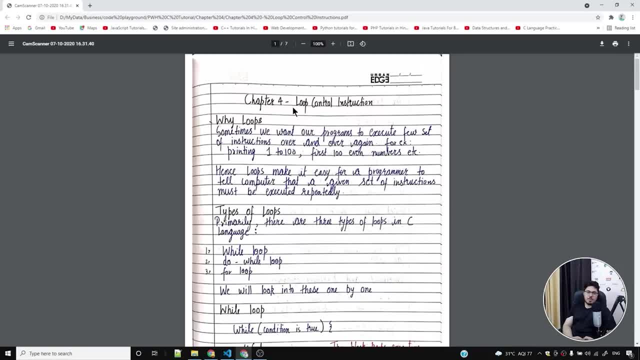 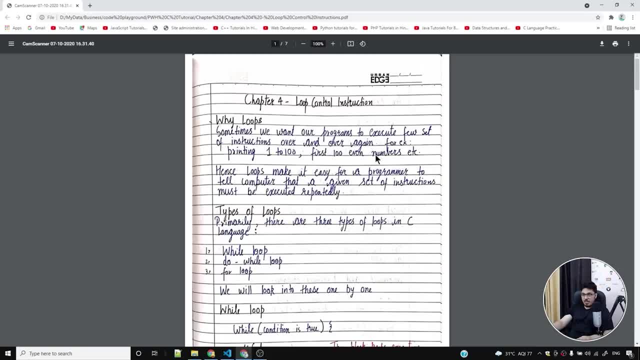 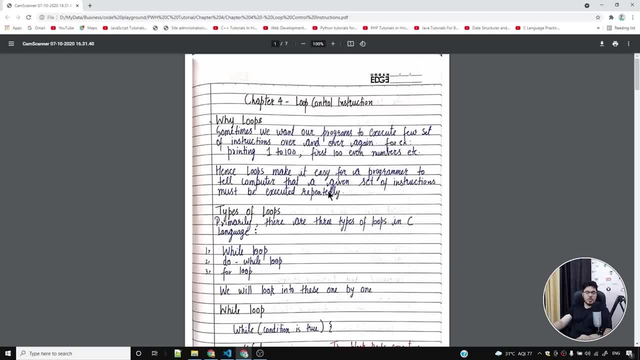 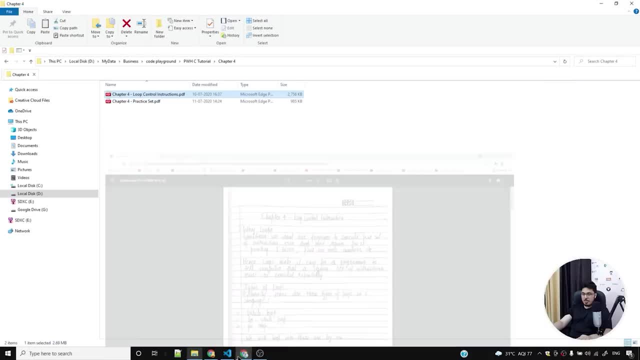 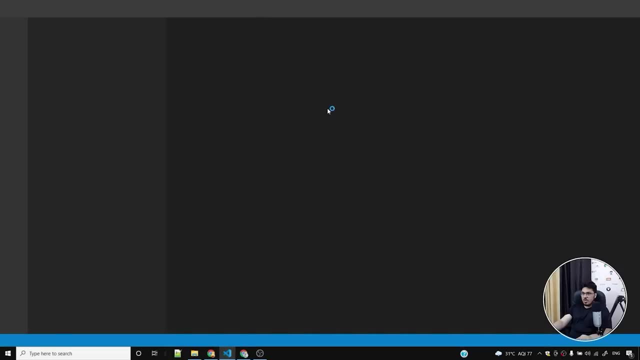 all the way till 10 times. but if i ask you to do it 100 times, it will be tedious for you. but using loops you can do it in fewer lines. let's see how. so what i'll do is i'll simply close this particular thing from my vs code and i'll open this folder in vs code. let me open this folder in vs code and. 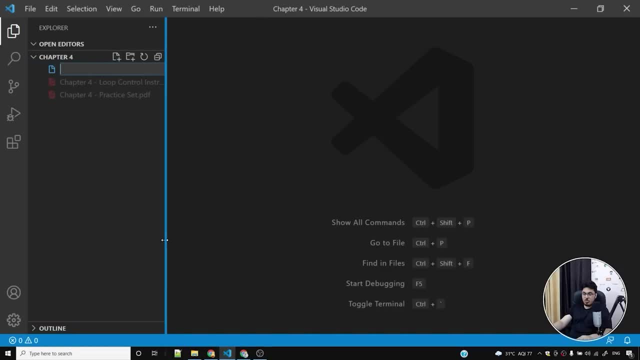 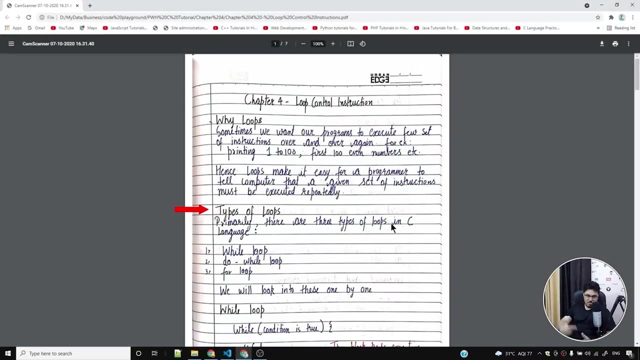 the moment i do that. what i'll do is simply create a new file and i'll simply say 01 underscore loop dot c. let me put the boilerplate code and let's learn about what loops are primarily. there are three types of loops in C language. we have a while. 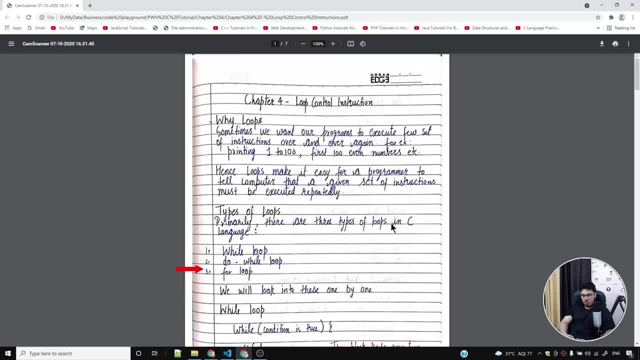 loop. we have a do while loop and we have a for loop. let me tell you something from my experience: we are going to use while loops and for loops a lot more than we are going to use do while loops. now, this is. this is just something I'm telling you from my experience, but again, there might be. 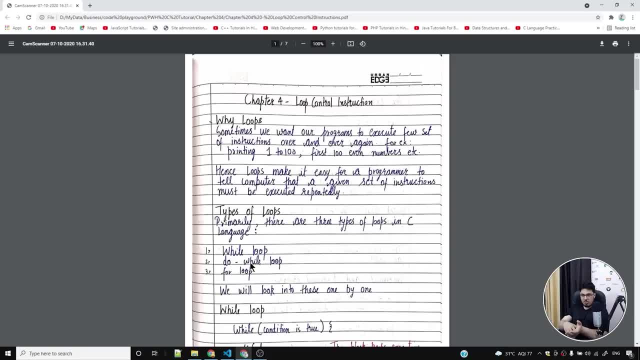 scenarios where you will use do while loops more than while and for loops. but in general- and I can say this for programming in general- we use a lot of for loops, then we use pure while loops and then again we very rarely use do while loops again. this is going to change. that depends upon what you are. 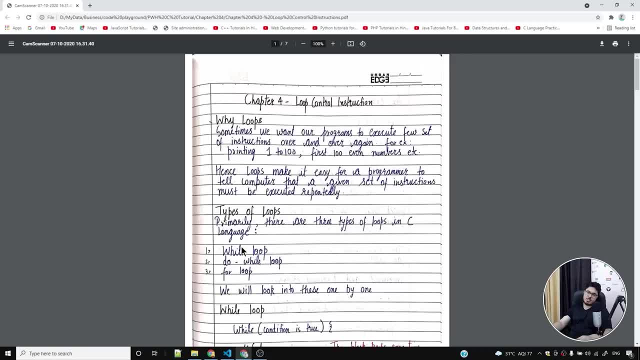 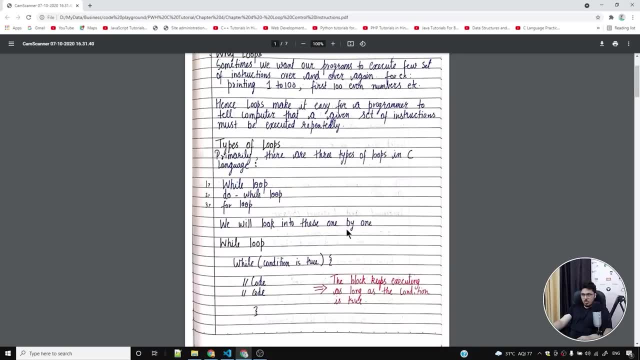 doing, but in most of the scenarios, for loop is the mostly used, while loop is second mostly used and do while loop is something that you are going to use sometimes. okay, now let's look into these one by one. let's look into while loop first. what is a while loop and how? syntax of a while loop. 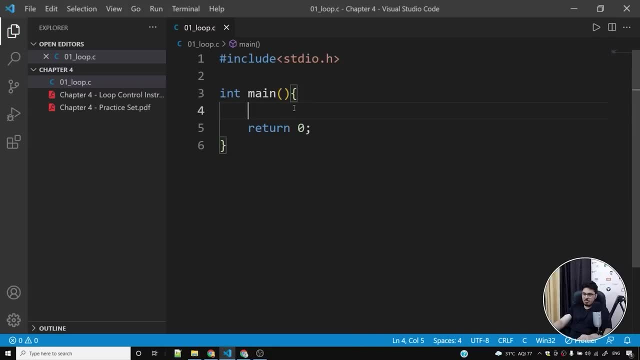 looks like. so what we usually do is we create a variable, we simply say int i is equal to 0 and we start counting from 0 because of arrays in arrays, the index starts from 0. if you don't know what arrays are, you don't have to worry, because I'm going to talk about arrays in the later chapters. 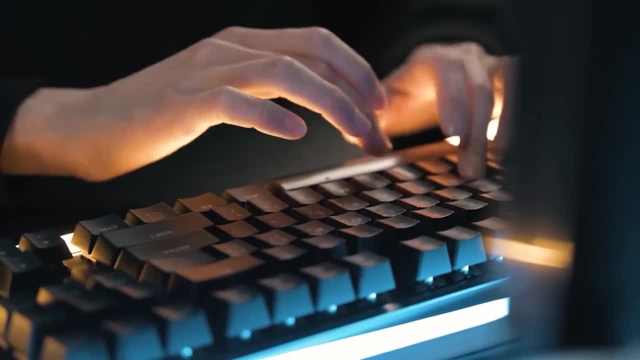 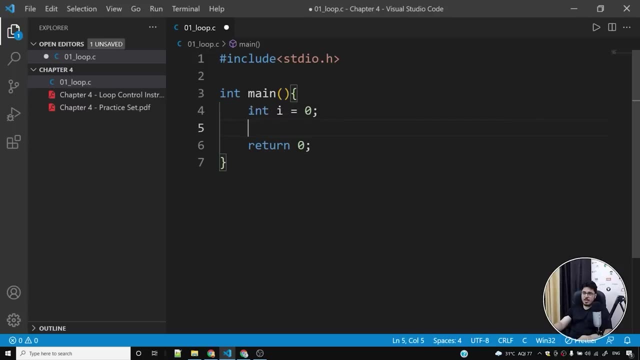 but for now, keep in mind that whenever you are doing programming, start counting from 0 instead of counting from 1, because it is going to make things easier for you. so let's make int i is equal to 0 and let me write y, and the moment I do that, you can see that I got a snippet. what I'll do is I'll say if i is less than. 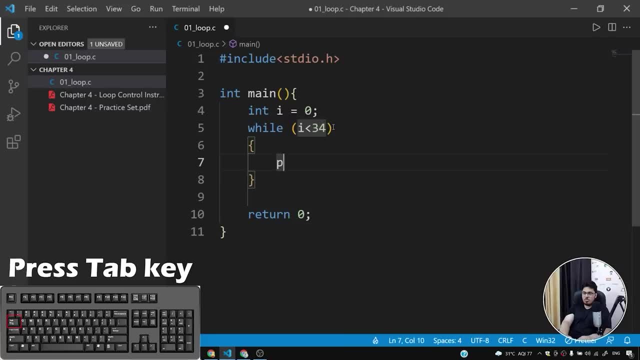 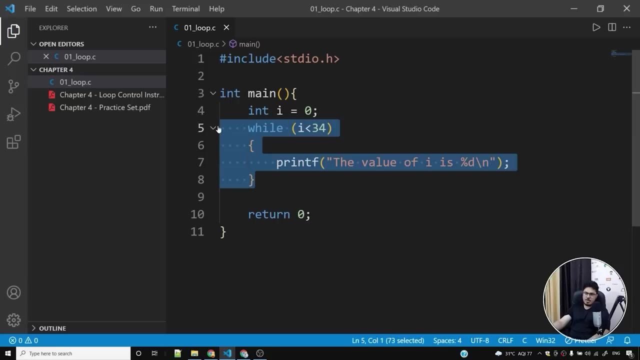 34, I'll press tab key on the keyboard and I'll simply say printf: the value of i is percentage d, and let me also write a backslash n here, so that I can see a new line. now, this is something that you can type as well. I mean, I didn't do any magic. you can very easily type this thing and typing is: 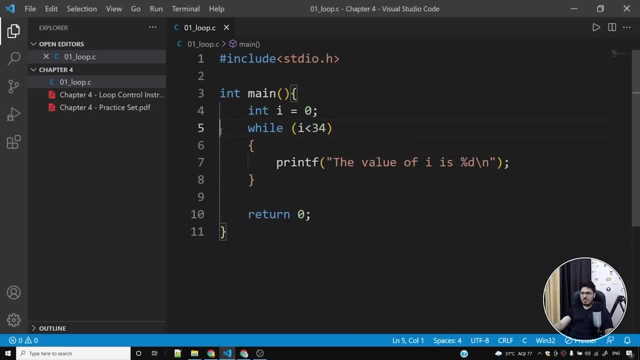 going to be a lot more easier. if you are not having snippets or some other extension. if you are coding in some source code editor which doesn't support these kind of snippets, you can simply type this out, and it is really very easy to type this thing out. then typing the value of i is 0, 1, 2, 3, 4, 34 times. let's see. 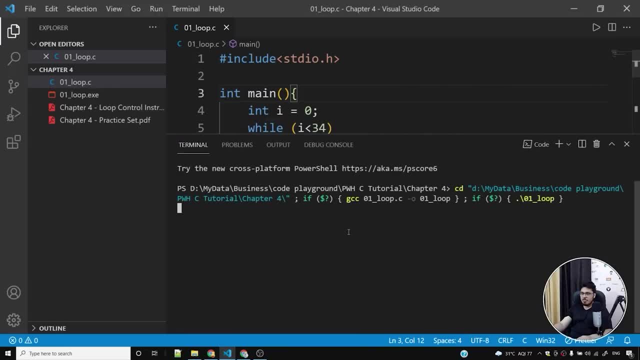 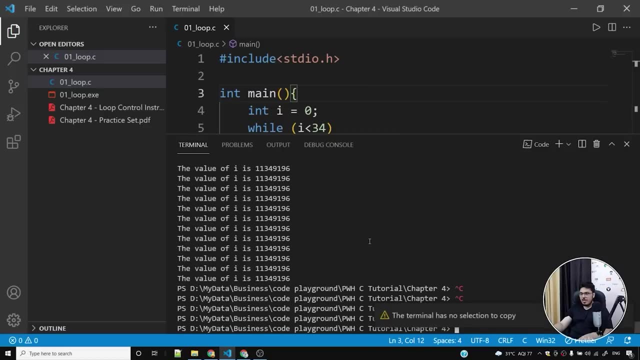 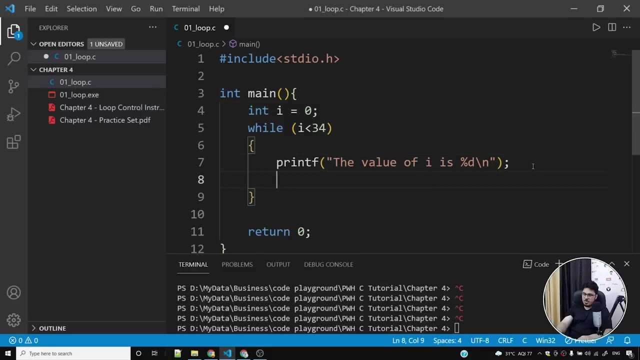 what this program returns. so the moment I run this program, you'll see something like this. so what happens is it keeps on printing, keeps on printing, and I'm in trouble. let me tell you why. why am I in trouble? so I had to cancel this and it went on infinitely. so what I forgot was I forgot to. 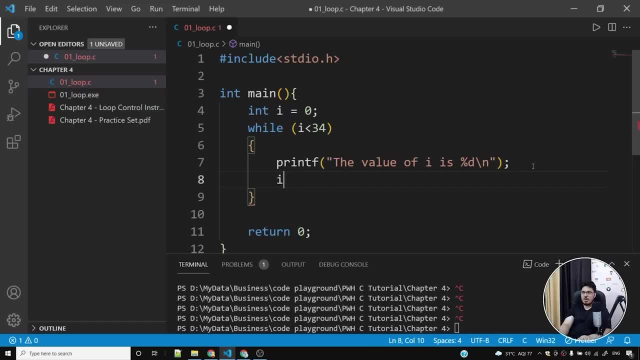 increment the value of i. so there are two ways you can use to increment the value of i. either you can do something like i plus plus, or you can do something like i plus c equals to one. you can also say: i is equal to i plus one, and this is going to have almost the same effect. okay, so you can use. 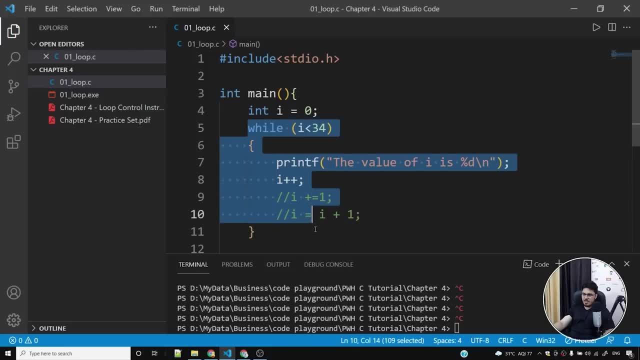 either of these. basically, what I'm doing is I'm simply running this while loop and I'm going to update the variable. so there will come a time when the value of i will simply be nothing but more than 34, or it will become 34 at some point, and whenever that happens, this condition will 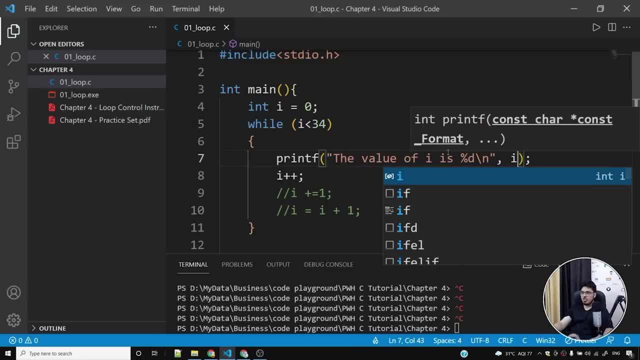 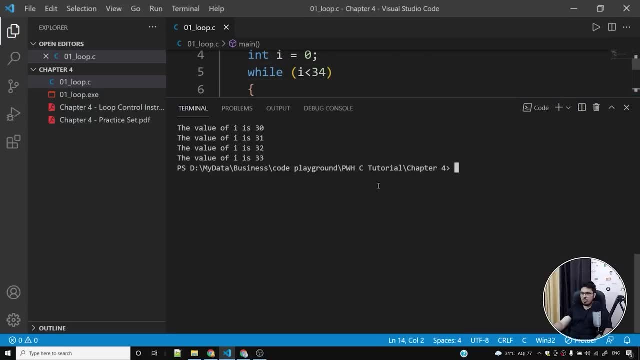 turn out to be false. I also forgot to write i here. so now we have a program which will definitely work and it will start printing from 0 to 33. so you can see. the value of i is 0 to 1, 2, 3, 4, all the. 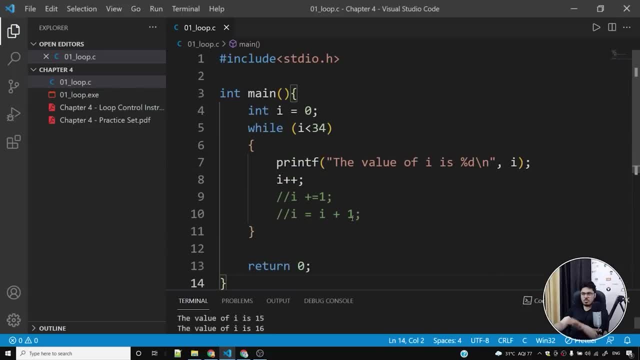 way till 33.. How does it work? let's now try to understand how this syntax is actually giving the result that I am getting. so what happens is, whereas int i is equal to 0, i is initialized to an initial value of 0. now, when I say while i is less than 34, I'm saying this is a block and you have to keep on. 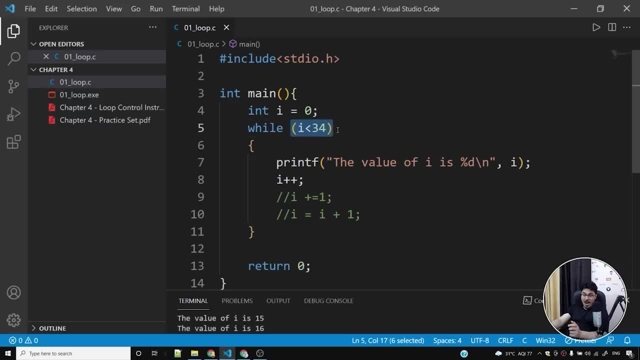 executing this block until this condition is true and inside this block something can happen which can make this condition return false. So something can happen inside this block which will make this condition false eventually, and if that doesn't happen, this is going to be an infinite while loop. we don't want that. okay, in ideal. 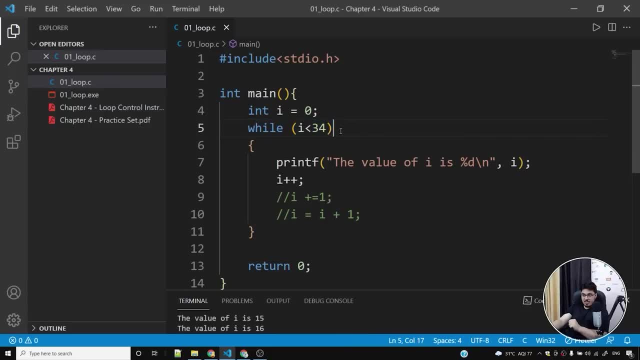 scenarios. we don't want that. now, when I say: while i is less than 34, this is a condition and as long as this condition is true, this block will keep on repeating. it will keep on repeating. so what happens is: is i less than 34? yes, it is, because 0 is less than 34.. 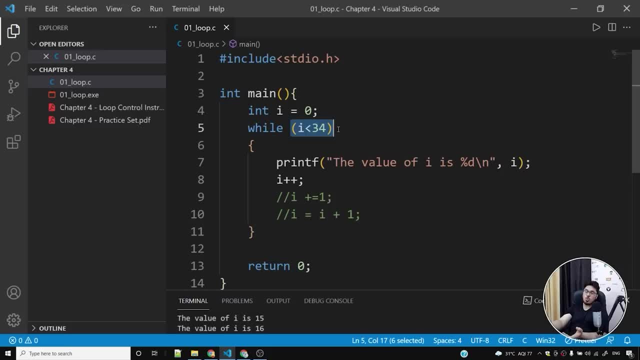 So i'm going to be change it back to 5, 2, 2, 1, and if I see that this particular expression is evaluated to true, what happens is these two lines of instructions are executed, so this will get printed. the value of i is 0, so the value of i, 0, is printed. and then the second piece of instruction. 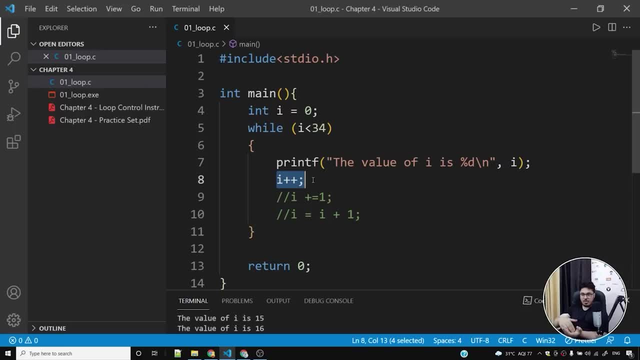 says that you have to increment the value of i by 1. so if i is 0, it will become 1, if i is 1, it will become 2, if i is 2, it will become 3, and if i is 3 it is going to become 4, and so on. okay, so this is. 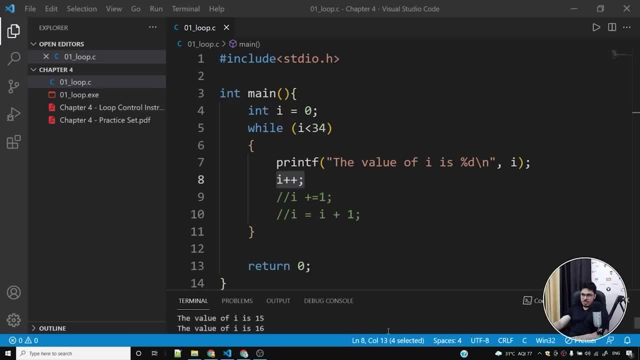 how to make an infinite block, how entire thing is going to work, printfs and i++, and eventually the value of i is going to be 33, and when it is 33, this condition is going to be true again. so the value of i is 33 will be printed. 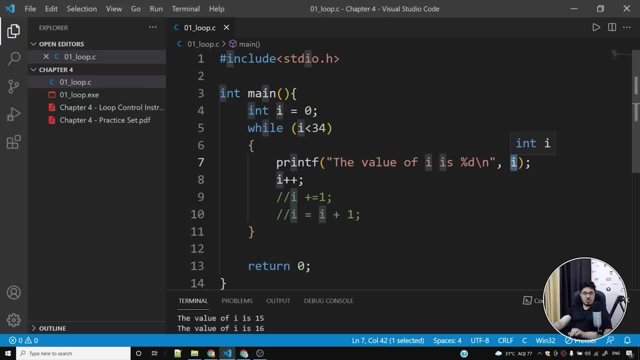 but during this iteration, something special will happen. the value of i is going to be 34 and this condition no longer evaluates to true now, which is why this while loop will cease to execute. that's it for this while loop. that's it because the condition is now evaluating to false. 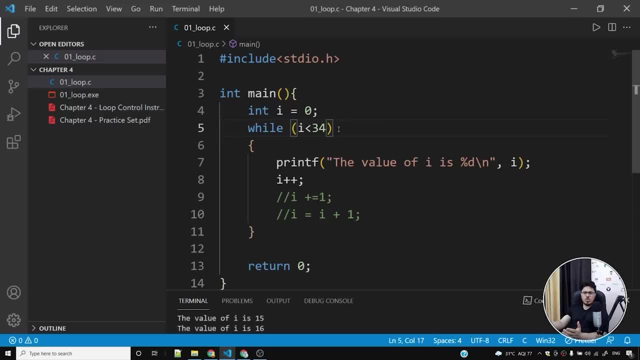 as long as the condition is evaluated to true, the while loop was running, but the moment we see that the condition is being evaluated to false, this loop will no longer continue to execute. okay, which is why this program will end, because we have a return zero here, and hence the result. 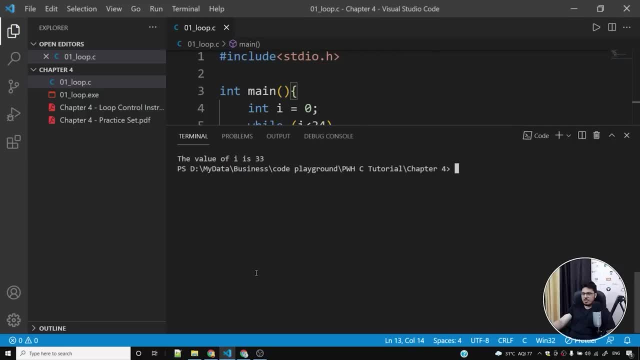 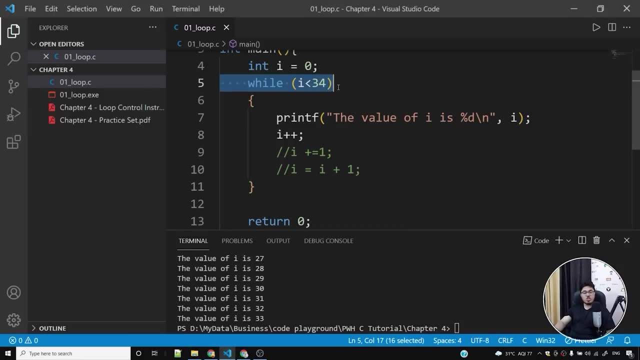 hence we are getting this: the value of i is 0, 1, 2, 3, 4, 5, 6. eventually you become 34, which makes this while loop to stop, because now the value of i is 34 and the condition inside this while loop is going to be false. okay, so i hope that you understood all these things. 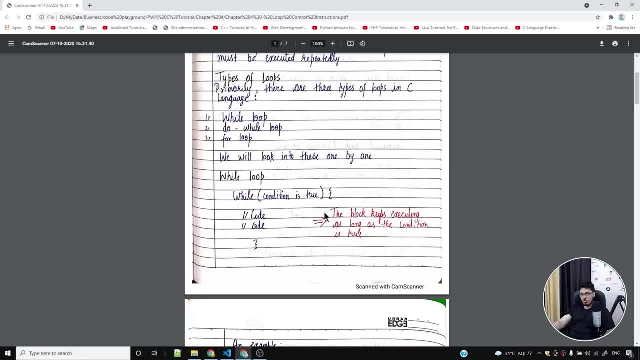 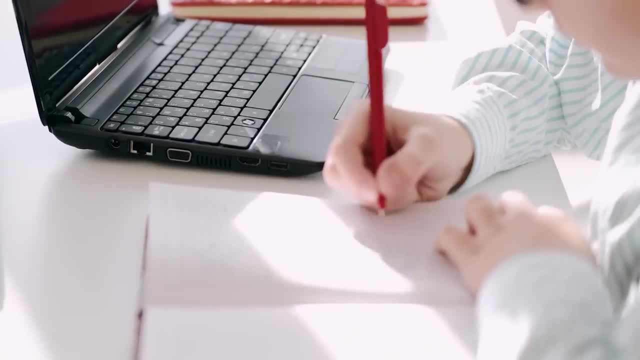 and now what i'm going to do is i'm going to move ahead and show you the syntax which i've written in the notes. and why do we have these notes at the first place? because i want you to come back to these notes after six months and you're going to have everything back in your mind. 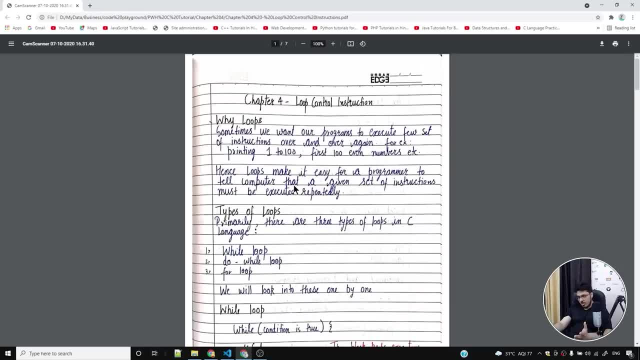 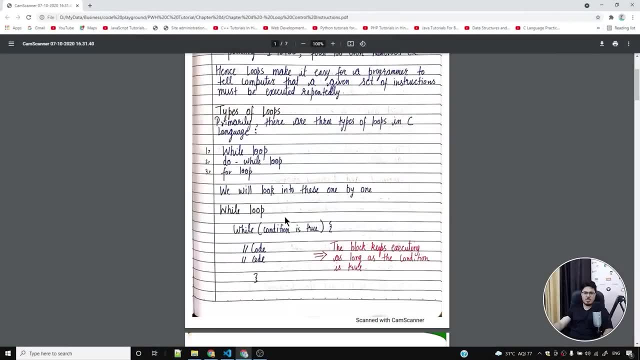 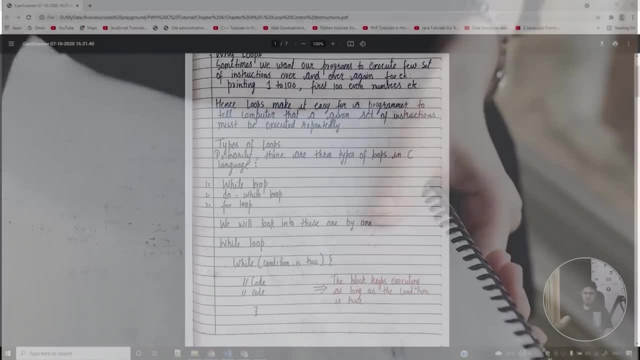 because you have refreshed all the concepts which you were already aware of. now you have these notes and you can simply come back to these notes and start revising whatever topics you like. okay, so make sure that you download these notes and make sure that you have a printed copy of these notes, and no, i don't have any tie-ups. 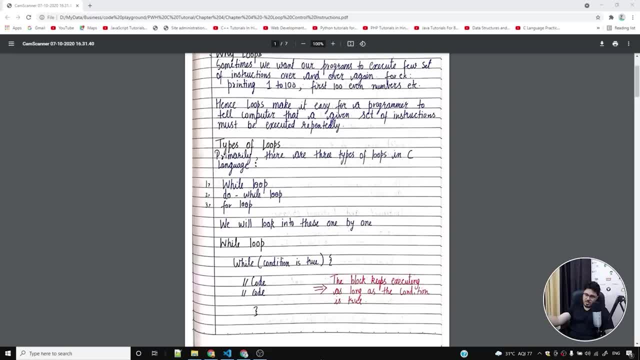 from the xerox shop in your country. okay, you can go to your nearest xerox shop and, you know, get these documents printed and it is going to be really very useful. but if you are a kindle guy or you are an ipad guy or you know some kind of a xerox guy, or you know some kind of a xerox guy. 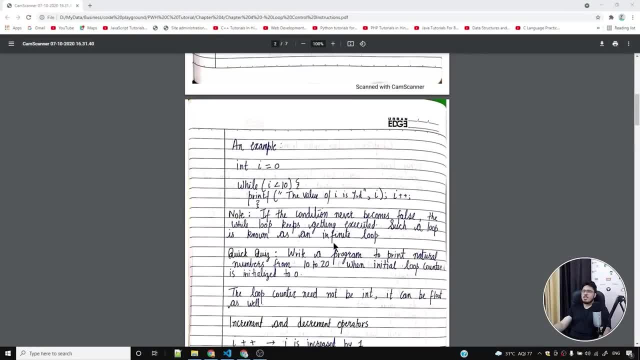 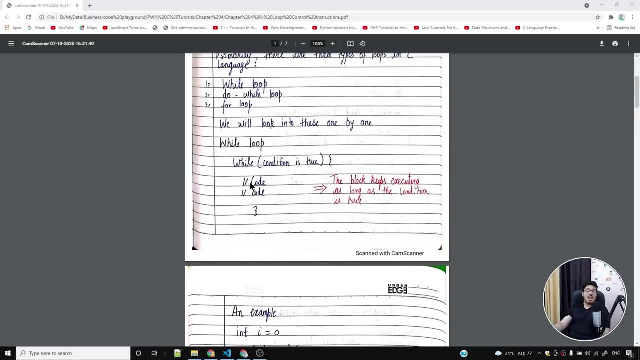 some tab guy, you might even use a pdf. okay, let's see what i've written in the notes. i've written the basics index, which is while, and the condition, and then you can: you have multiple lines of codes inside the block and all these lines will keep on executing until this condition is true. so the 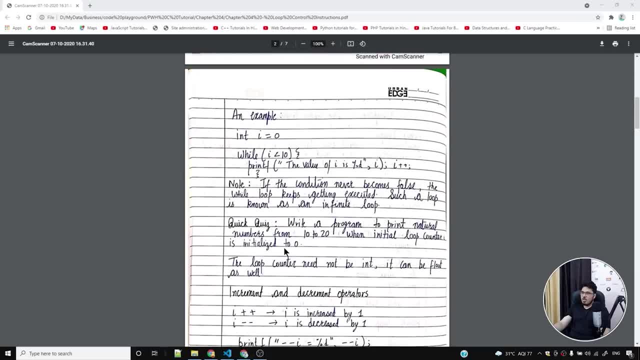 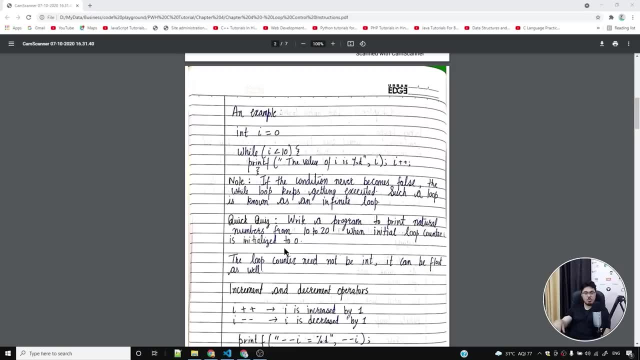 block keeps executing as long as the condition is true. eventually the condition should become false for this while loop to halt, or else you should have a continue or break statement inside the block and then you will see how continue and break works. but again, an example of while loop has. 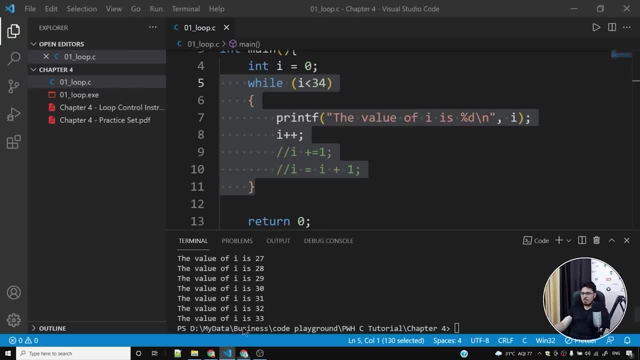 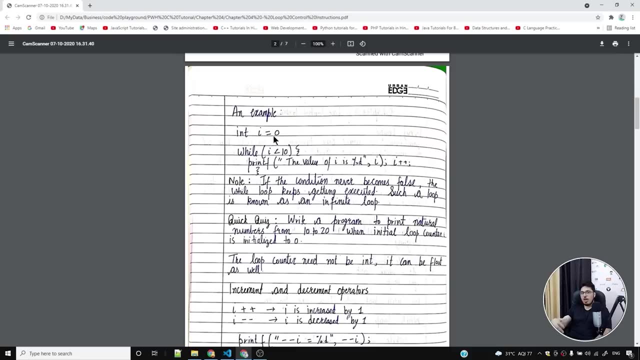 been written here. the value of i is- i've shown you this example and this is the same example that i've shown you, so you can play around with this code and you know, start changing the numbers, start changing the initial value of i, start changing the condition. you can make this 10 instead of 34. 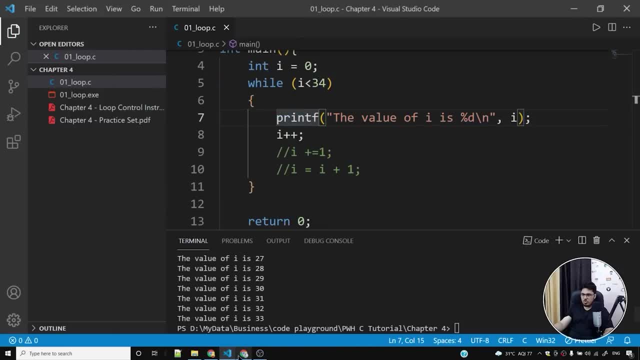 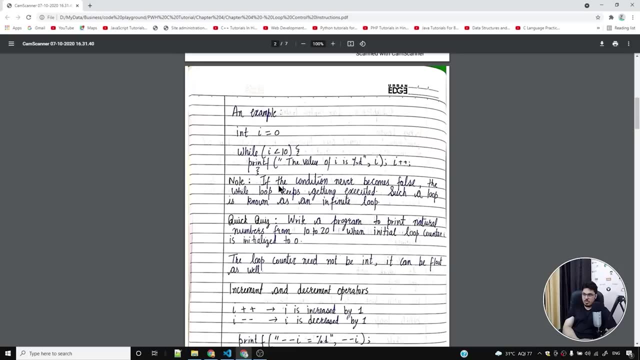 you have this code. i'm going to zip all this and i'm going to send it to you, so you don't have to worry about that. i've written a node here. if the condition never becomes false, the while loop keeps getting executed. such a loop is known as an infinite loop, so i haven't shown you the infinite. 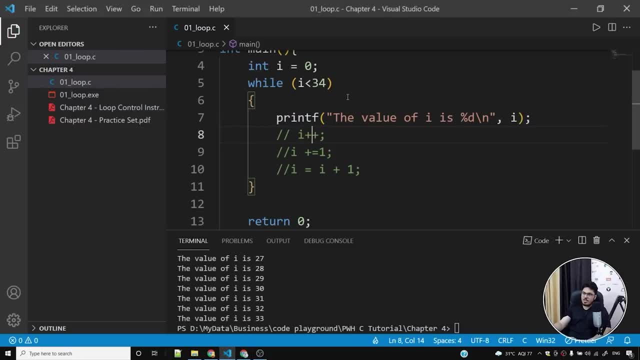 loop. yet if i don't have this condition, the value of i is going to be 0 always and this thing is going to be printed on the console always. let me show you so: if i run this program, the value of i is 0, will keep on printing. will keep on printing until i press ctrl c to halt this program. so i'll. 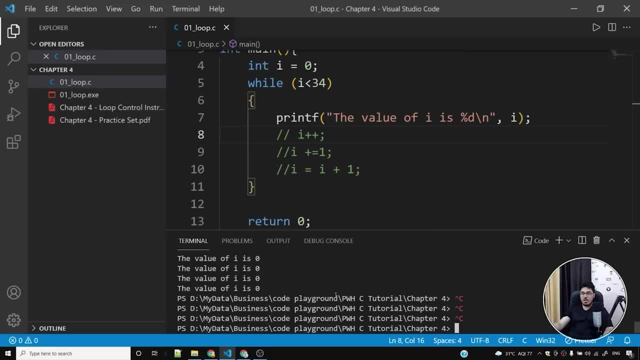 have to manually halt this program or halt vs code or this terminal to stop this program. okay, i can either click here or i can even close the vs code on my computer altogether, which will, you know, stop this program. but again, we want our program to stop eventually because we want. 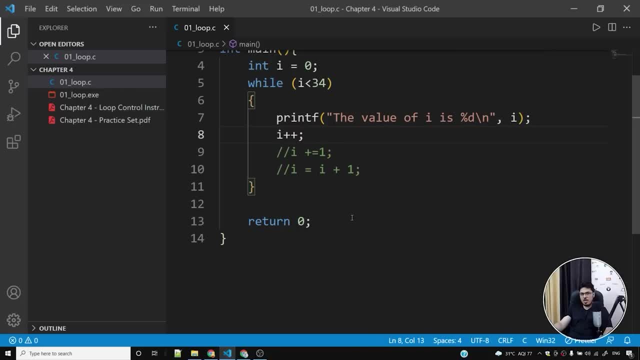 to accomplish something from our program in ideal scenarios. there are some cases where we use intentional infinite while loops. what are those scenarios? let me tell you about few scenarios. there are few scenarios where we want our program to keep running and you know, keep checking in regular intervals. so if you want that, you can have a wild one and inside that you can keep on. 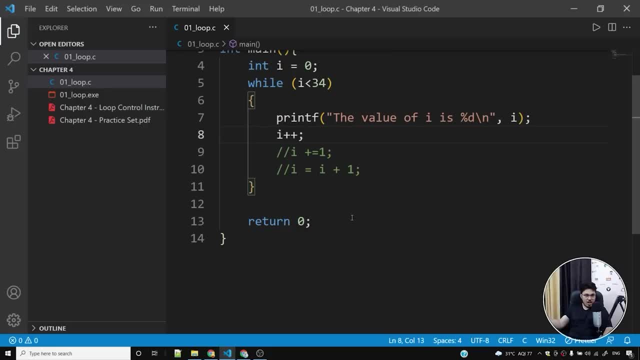 checking something for some time. you know you can wait for half an hour and check something. then again wait for half an hour and check something. one of the example is whether a stock price has hit a value or not. let us say you are tracking the index of your stock market and you want to see. 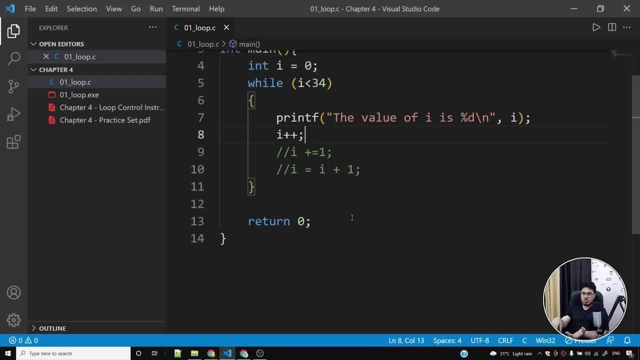 if your index is down by 10 or not. so you might want to keep checking that every half an hour. you can either while one loop which keeps on checking for the time and the moment. time becomes a multiple of, rather, the minutes becomes the multiple of 30. so every half an hour you are. 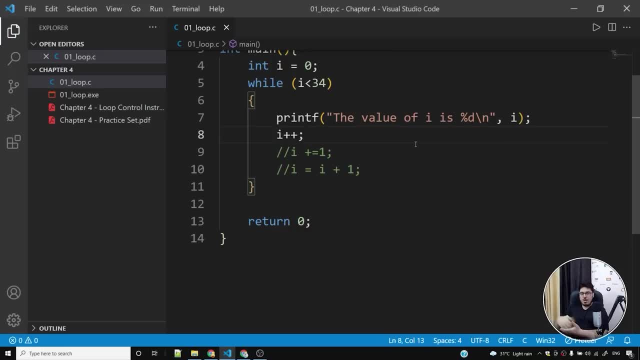 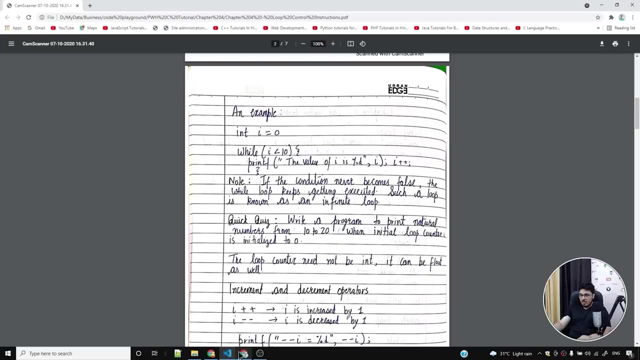 checking whether your index has hit a particular value or not. but in most of the cases we want to avoid infinite loops and in most of the cases, for beginners, infinite loops are a result of mistake in the coding logic. okay, we don't want that. let us come to the quick quiz which i have. 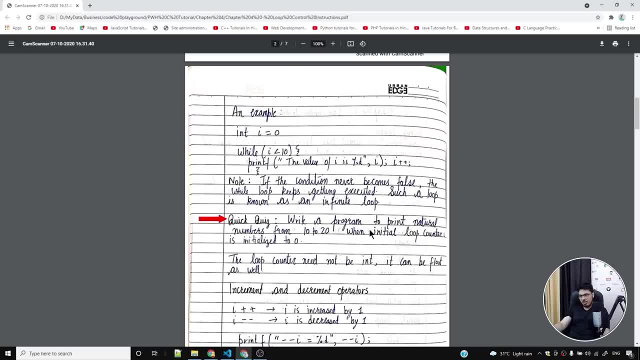 written for you. it says: write a program to print natural numbers from 10 to 20 when initial loop counter is initialized to zero. now the initial loop counter is initialized to zero, which means i will have to keep this. i is equal to zero. if that was not the case, i would have simply changed. 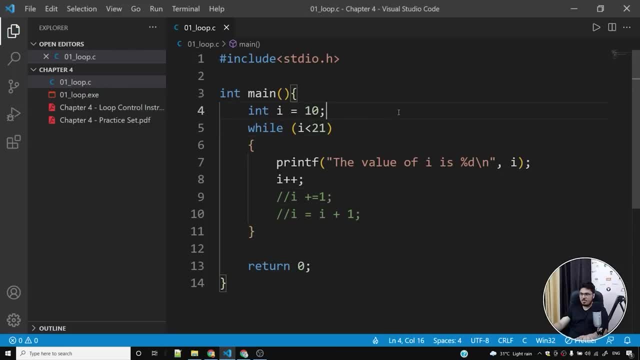 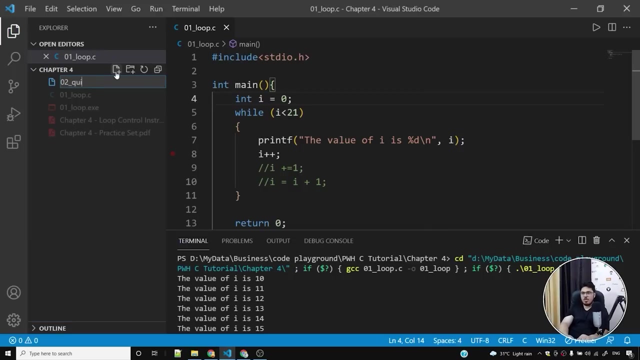 this value as 10 and this value is 21, and that should have done the trick. but no, the initial value has to be zero. how do i solve this problem now? so let me write another piece of code for you. i'll simply say: quick underscore quiz. 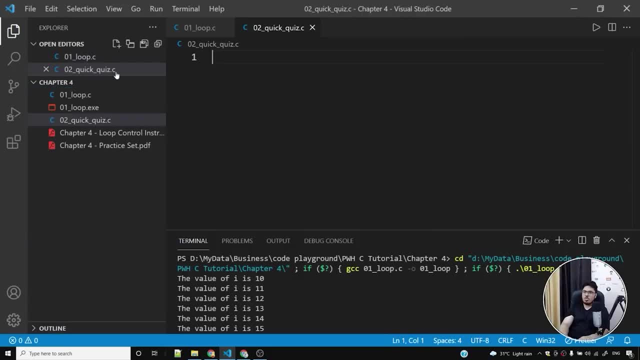 dot c. okay, so let me paste this and also let me keep this 34. i'm going to play around with this, so the value of i is zero, and what i'll do is i'll keep on going till 20, from 0 to 20, but i'll have a if. 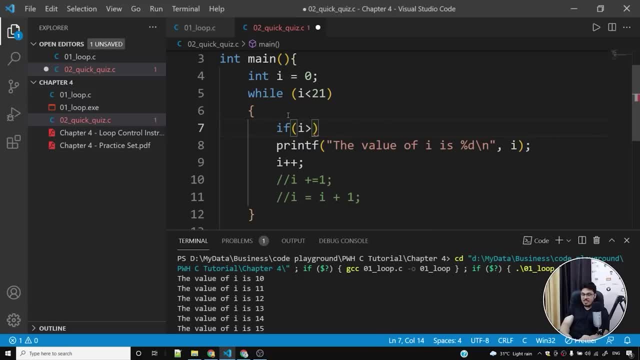 statement here and inside the if statement, i'll simply say: if i is greater than or equal to 10, then only you are doing that, then only you are printing this, otherwise you are not printing this. okay, so if i do that, for i is equal to 0, this line will not be executed, for i is equal to 1. this 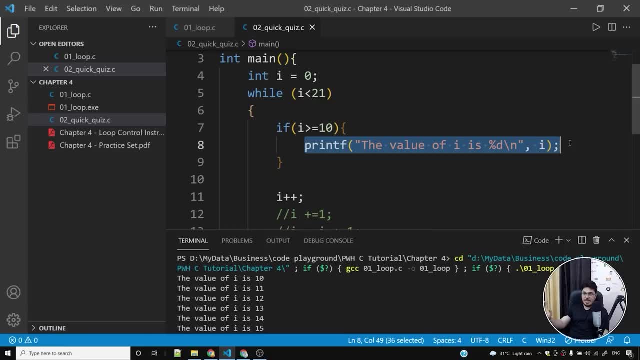 line will not be executed for 2, 3, 4, 5, 6, 7, 8, 9. this will not be executed. in the moment i have the value of i as 10. this will be executed, so i'll get the value of i is 10 all the way till 20. let me. 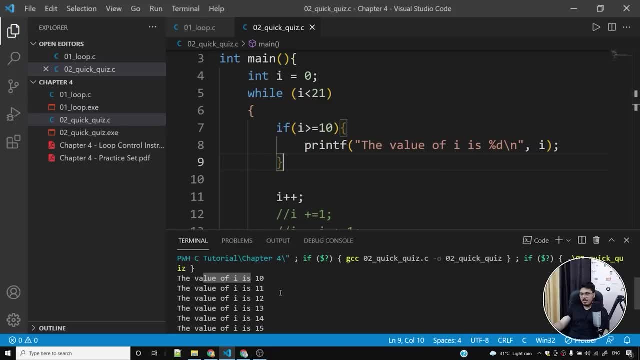 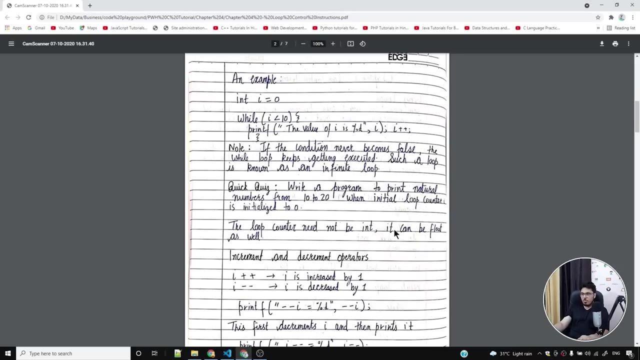 show you. so we're on this program. you can see the value of i is 10, 11, 12, 13, 14, 15, all the way till 20.. so this is how this uh y loop works. okay, coming back to the notes, uh, we have solved the quick quiz. the loop counter need not be in. it can be a float as well. 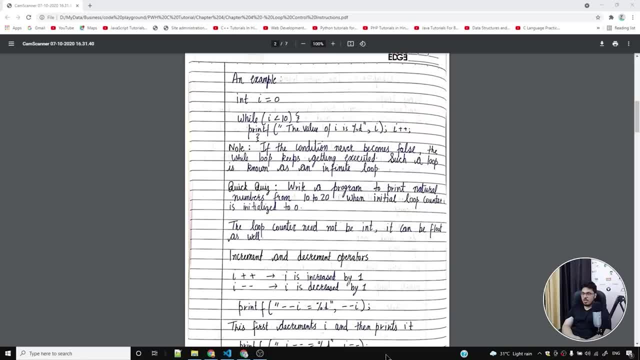 so this is something that you need to keep in your mind: loop counter can be a float, it can be a double, it can be anything. okay, you, you don't have to keep it as an integer, but in most of the cases we keep it as an integer so that we can count conveniently. okay, now let's talk about 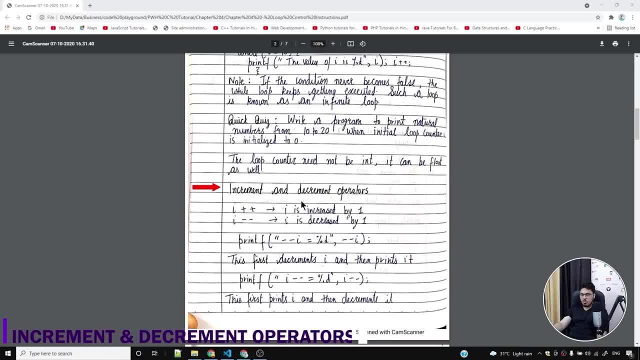 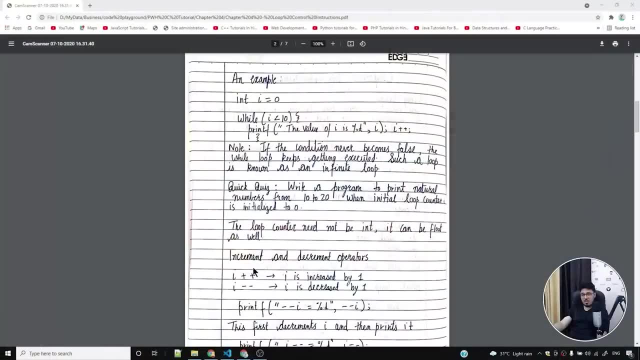 increment and decrement operators. what are these operators and why do we need to use these? and this is something which is asked a lot in c programming interviews, and even if you are studying c programming language at school or in your college, this is going to be asked for sure. 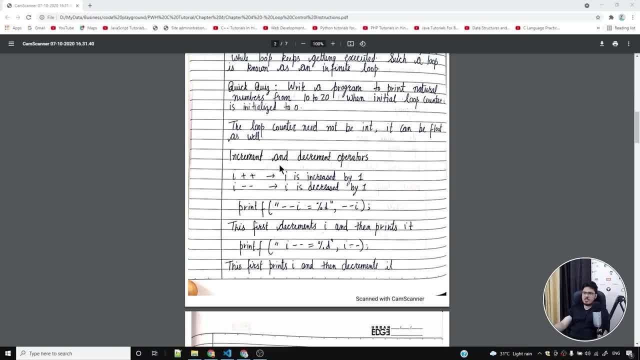 okay, i plus plus. what does it mean? it simply means that increase the value of i by one. so if i was four, make it five. if i was nine, make it ten. if i was 22, make it 23. i minus minus. yes, you guessed it right: i minus minus means that decrease the value of i by one. so if i was 54, make it 53. 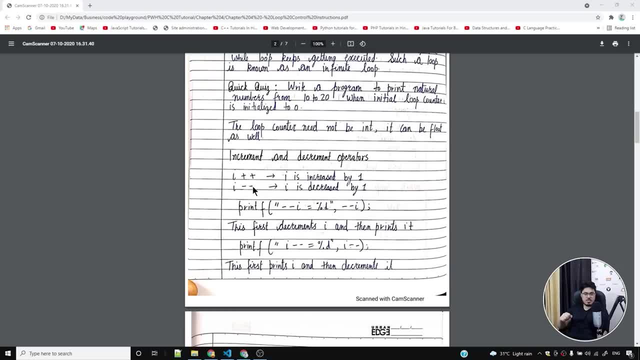 if it was 128, make it 127, and so on. but we have another decrement operator which we use like this: minus minus i. instead of doing i minus minus, we do minus minus i. and and how does it work? it basically decrements the value of i first, and then it prints the value of 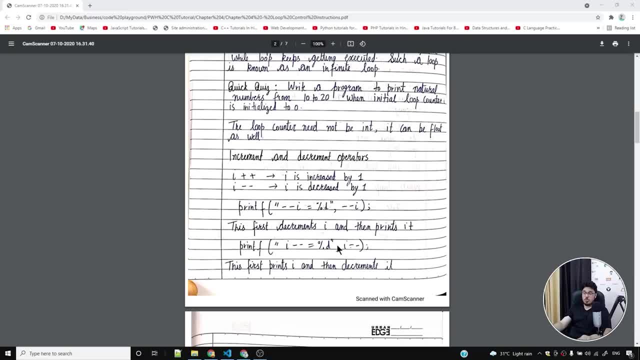 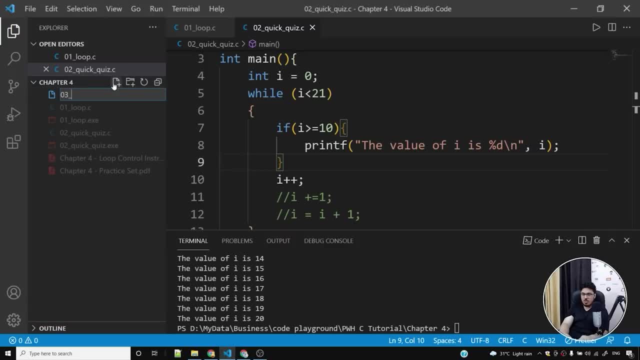 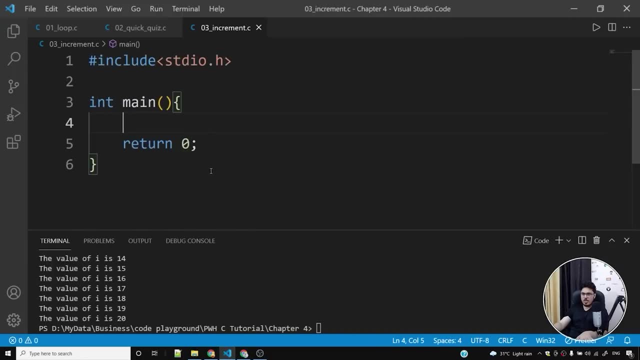 i when kept inside printf. so let me explain this to you how this works. so, in order to explain this, let me come to my vs code. i'll write a program three and let me call it incrementc. i'm going to say boilerplate code, so that i can put the c language boilerplate code here. i'll simply say: 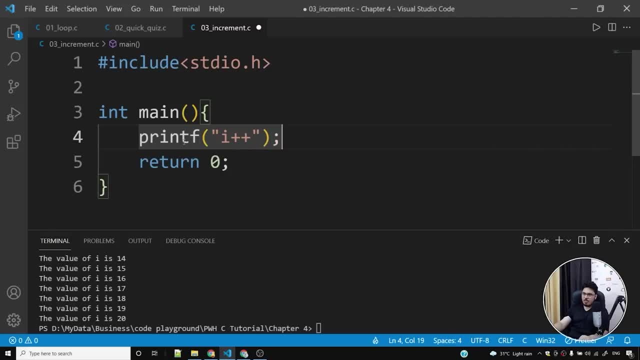 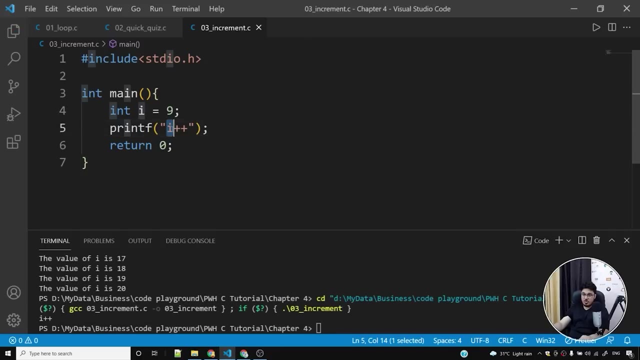 printf and then i'll say: i plus plus. okay, let me show you what it prints. if the initial value of i is, say, nine, okay, if the value of i is nine, and if i do, i plus plus, what i'm going to get is i'm going to get: uh, oops, i need to. 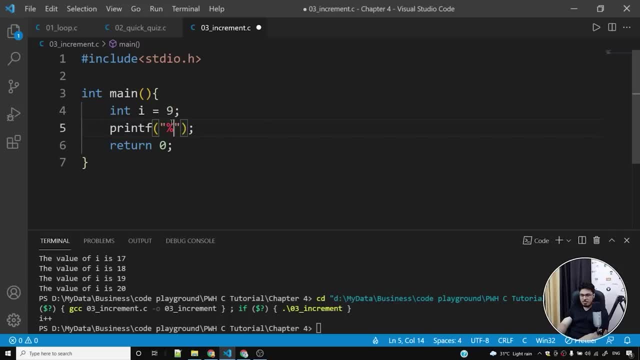 i made a mistake. i need to say percentage d, i plus plus, instead of literally printing i plus plus. my bad. let me run it again and you'll see that the value of i is nine. so even if i do i plus plus y, i'm going to get i plus plus, and i'm going to get i plus plus, and i'm going to get i plus plus. 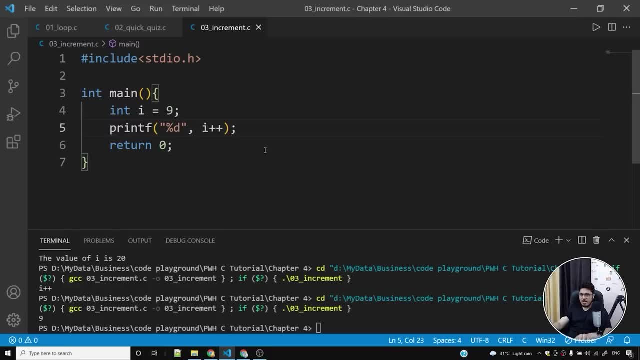 why am i getting nine? why? why don't i get ten? let me try this once again. let me try to print the value of i. after i do this, i plus plus, the value is nine one zero. what is going on? why is it nine one zero? it's in fact not nine one zero. uh, i'm not using backslash n. let me use backslash and. 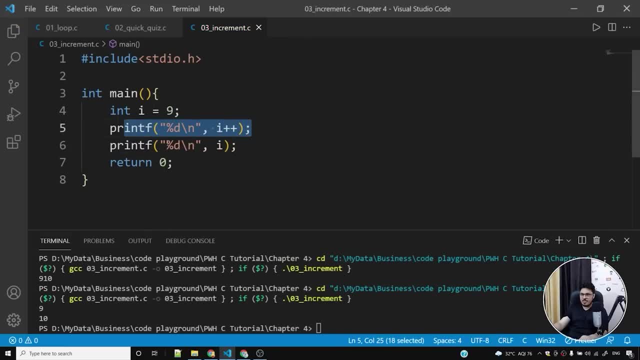 then you are going to understand what is happening. so this line prints nine, this line prints ten. so how does this work? how does this increment operator works? if i have a value of i which is nine, and i say i plus, plus, and i have a printf wrapped around it, what will happen is: 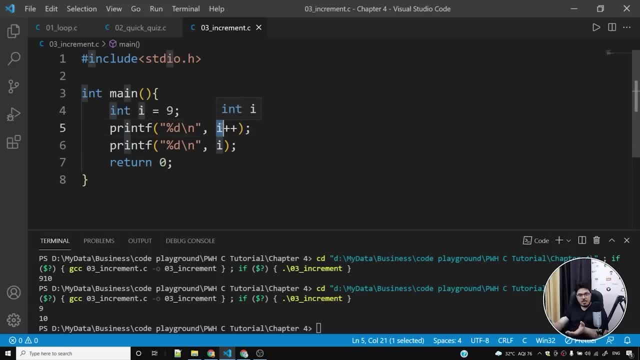 the value will be printed first and then it will get incremented. so nine is printed, but post printing of nine, what happens is that the value of i now becomes ten because we have a i plus plus here. so what happens is, after this is executed, the value of i is ten. so if i say 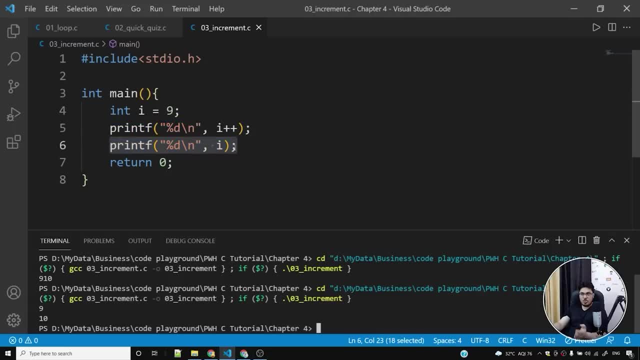 i printf i, i'm going to get ten. so i plus plus means first print the value of i. what is the value of i nine? so first print nine and then increment the value of i. and what does plus plus i do? let me change this to plus plus i now, plus plus i means first increment the value of i and after 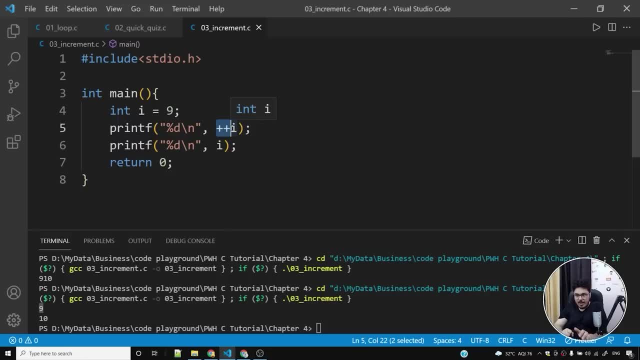 you have done, incrementing the value of i, you print the value of i, so what will get printed? ten will get printed. and what will get printed for this statement? ten will get printed because value of i is nine. we first incremented it and then we printed it, so this will print. 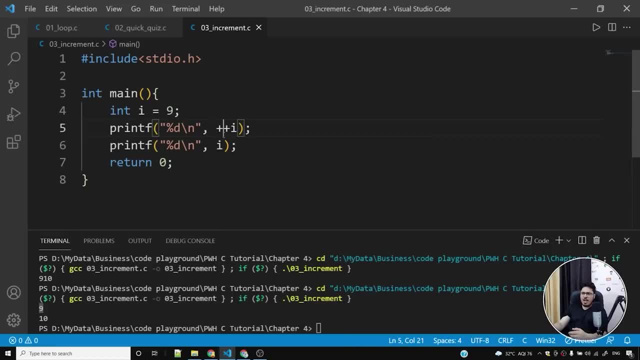 ten as the value of i, because the value of i is ten, because i have incremented it from nine to ten. so first incrementation takes place, which makes the value of i as ten. then printing takes place. so this is how it works. so let's see if it prints ten and ten. oh yes, 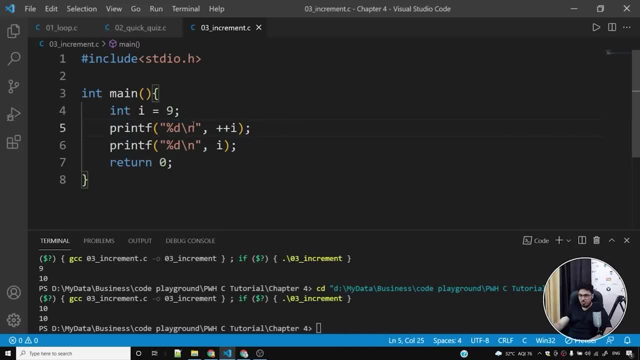 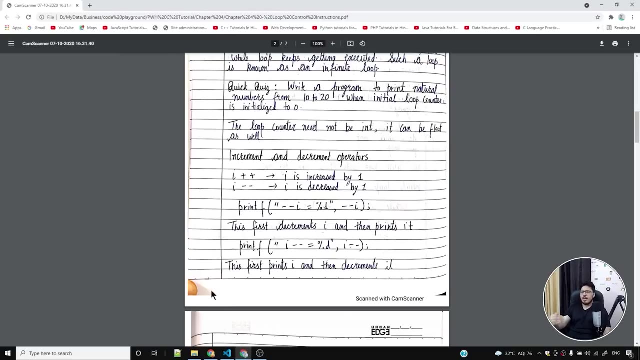 it does prints ten and ten. so this prints ten because i am first incrementing the value of i and then i'm printing the value of i, which is ten, and this also prints ten because i'm printing the value of i, which is ten. i hope you understood how this works. so, coming back to the nodes, increment and 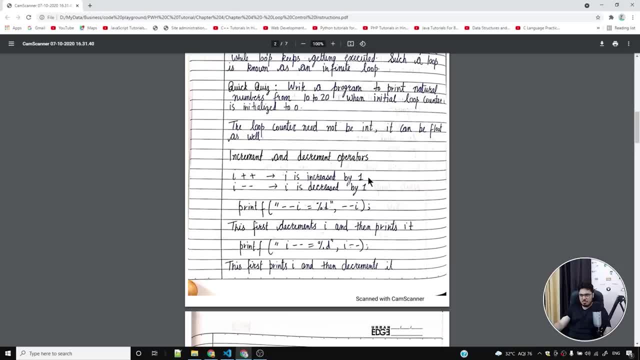 decrement operators: i plus plus means i is increased by one. i minus minus means i is decreased by one. when i do something like printf minus minus i and then percentage t, what will be printed? first i will be decremented, then i will be printed. now first this first. 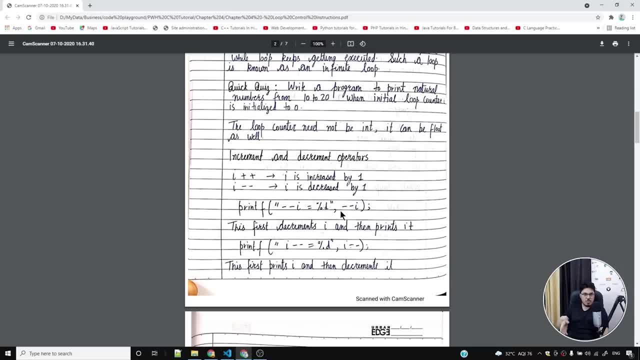 decrements i and then prints it. so minus minus i means first decrement the value of i, then print it. i minus minus means first print the value of i and then decrement it. i hope you understood this. try to run as many programs as possible to understand this concept. initialize: 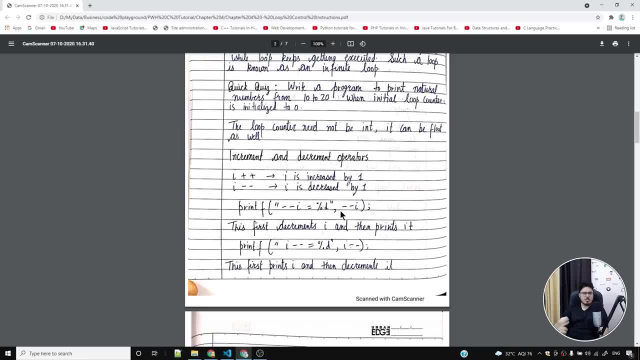 i with a value. try to print i plus plus. try to print plus plus i. this will not cost you anything. you have your laptop. just write the program a plus plus or a minus plus i and program open vs code and start writing code. now this first decrements i and then prints it and 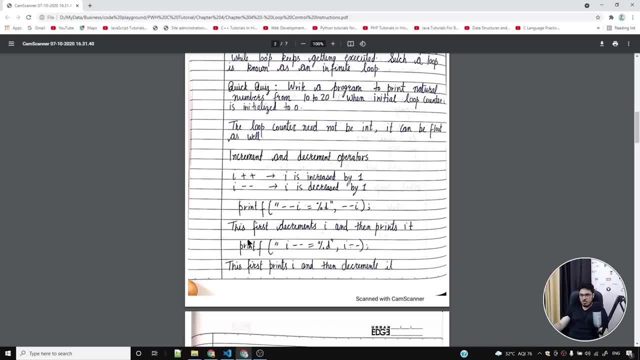 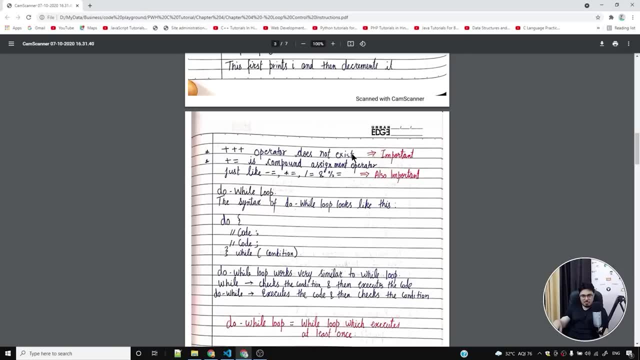 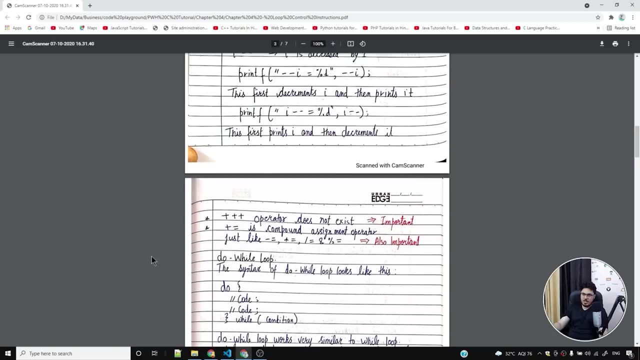 this prints i and then it decrements it. so i've written this very clearly: triple plus operator does not exist. make sure that you are not using i plus, plus, plus, plus, plus, plus and you expect it to increment i four, five, six times. no, that doesn't happen. we just have this plus plus operator now. 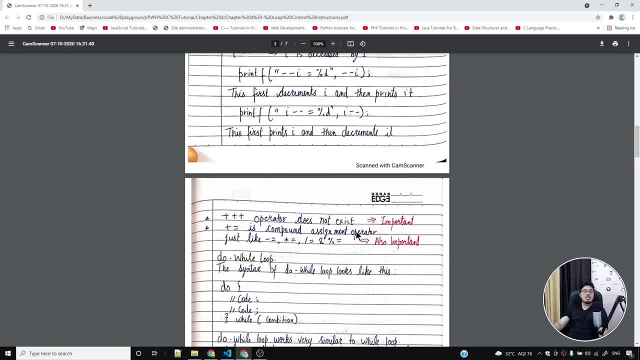 there is something called plus equals to, as well as it's called compound assignment operator. just like we have plus equals to, we also have minus equals to, times equals to, divide equals to and percent equal to. okay, and this is also important, you need to practice these operators as well. 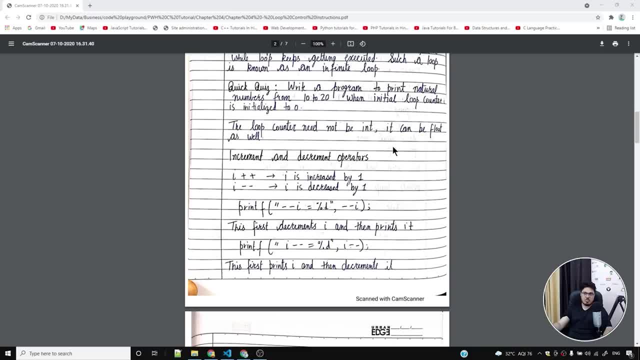 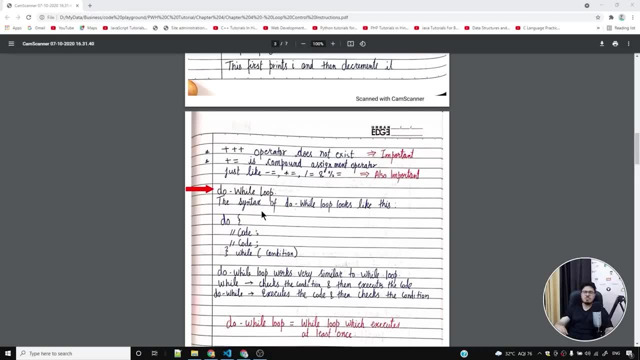 okay, so these were some of the increment and decrement operators you need to understand. now we'll talk about the do while loop and we'll write some program. do while loop is very, very similar to while loop, so you are going to understand it very, very easily. so let's now. 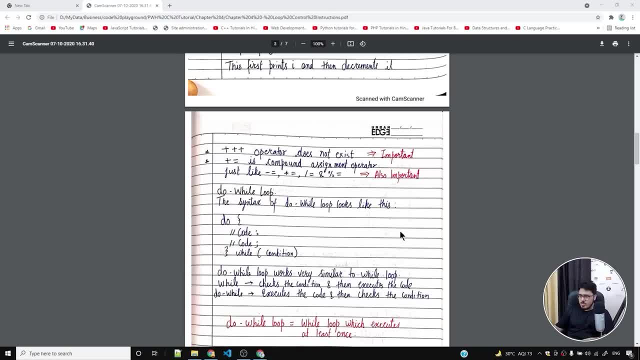 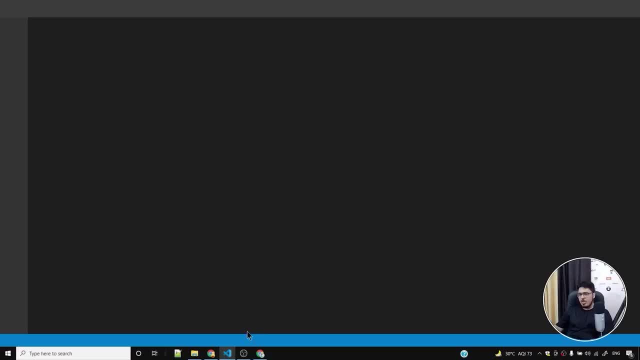 talk about do while loops. the syntax of do while loop looks like this: so we have a do, we have some code, then we have while, then we have some condition. but how does it all work? let me tell you. so what i'll do is i'll show you a code snippet of do while loop and. 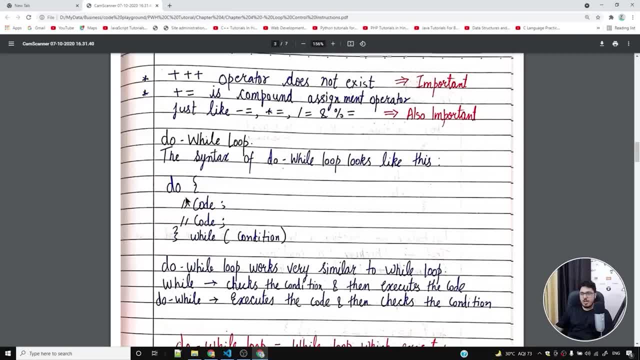 then i'll explain you how all these things are working together. so what we do is we write a do, we start a parenthesis and we start writing the code and at the end we write a while and then a condition inside that so do while loop works very similar to while loop. while checks the condition. 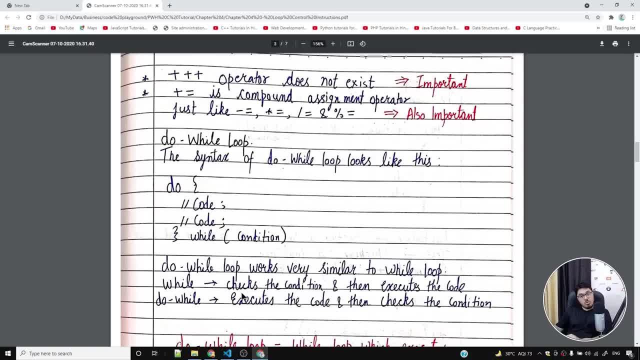 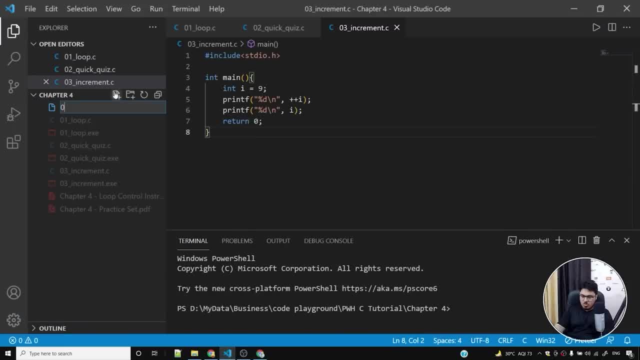 and then executes the code. do while loop first executes the code and then checks the condition. let's see how these two kinds of loops are different from each other. so what i'll do is i'll simply start, uh, writing a do while loop. so i'll simply say do while dot c, and the moment i do that and i add a boilerplate code. 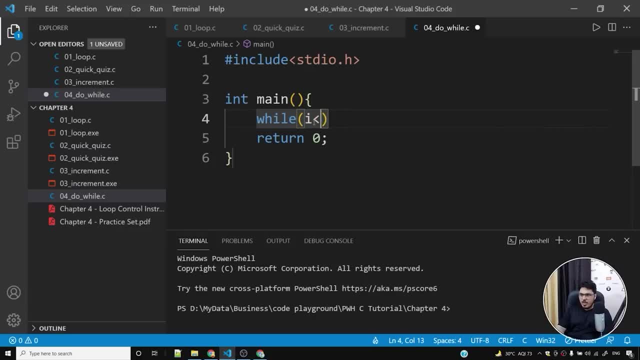 firstly, what i'll do is i'll show you a while loop and what i'll do is: and then i'll convert the same while to do while and show you how these loops are different from each other. so, if i have and if i have int, i is equal to 7 and if i do something like this, i'll say the value of i is. 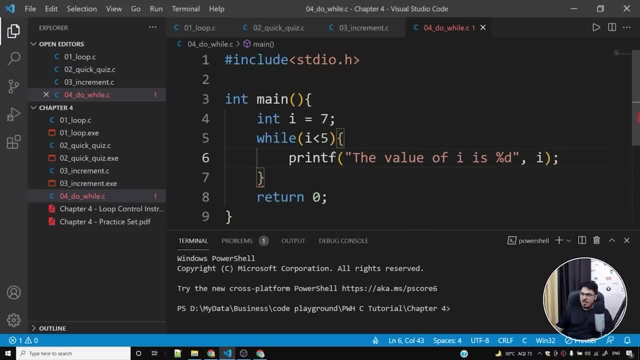 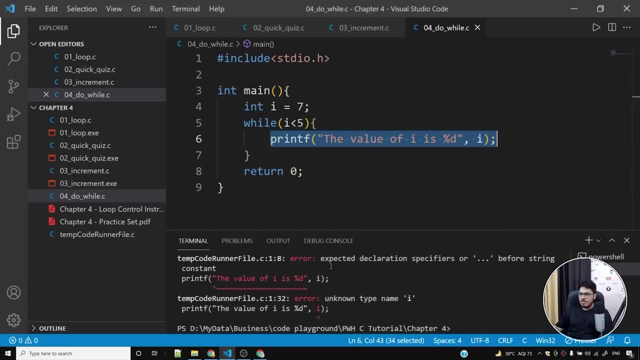 percentage d, and i now here, clearly i is not less than 5, so this loop is never going to execute. so, whatever i write here, this is never going to execute, because this condition is never going to be true. now, if i run this program and i think i'm making some mistake- actually i selected the code- 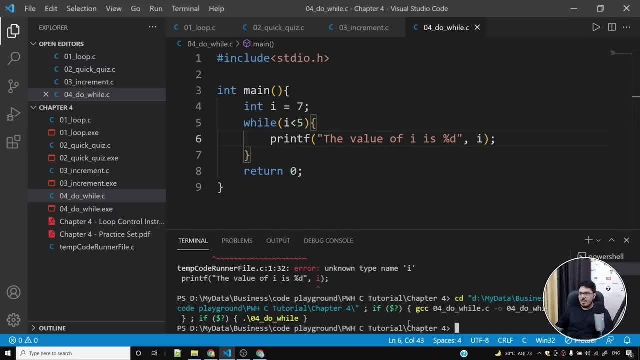 you don't have to select the code and run it. you simply run it and it is going to work. so this loop didn't get executed at all. why was that the case? that was the case because i is not less than 5. i is 7 and 7 is greater than 5. but what if we have a do-by-loop? let me convert this to a do-by-loop. 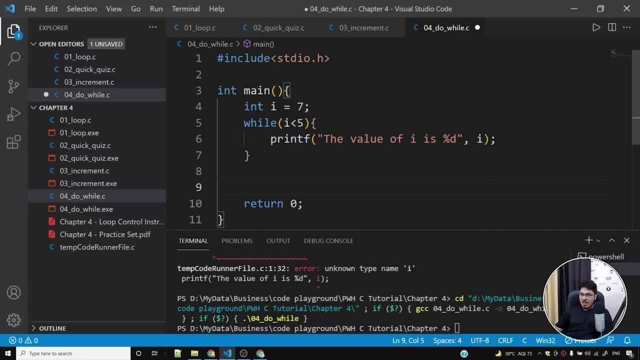 syntax. so what i will do is in do-by-loop we have a block first and while is at the end. so i'll have to bring this while at the end and i'll have to write do here. so this is the syntax of a do-by-loop. 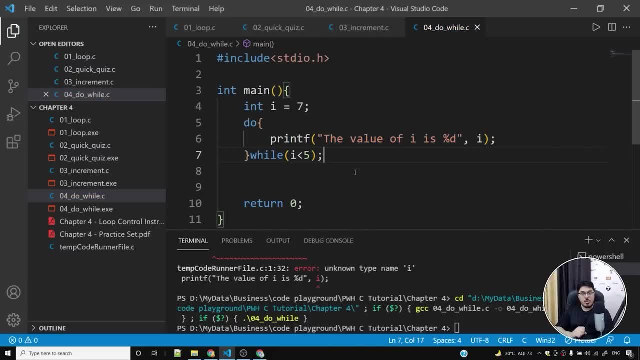 also, we need to keep a semicolon here. so this is very, very important in case of do-by-loops: whenever you are converting a while loop to a do-by-loop, make sure you add a semicolon here. okay, now what i'll do is save it and run it and, to your surprise, you will see the value of i is 7 being. 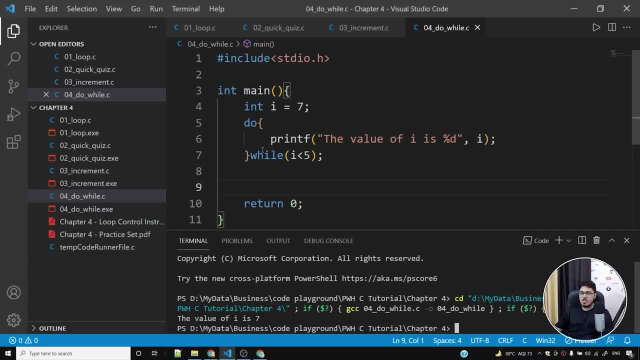 printed on the console. you might think that why is this the case when the condition is not at all true? so if you look at the structure of do-by-loop, you can you know, kind of. i'm giving you an analogy. the control will come here, it will start executing this. it will not see the condition yet. 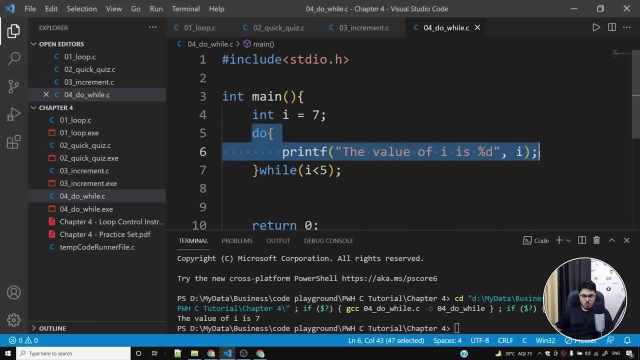 it will run this loop once for sure, no matter what the condition is. it might be true, it might be false- but the moment it checks for the condition, it will rerun the loop only if the condition is true, and if the condition is not true, it's not going to rerun anything. it's not going to do anything, okay. 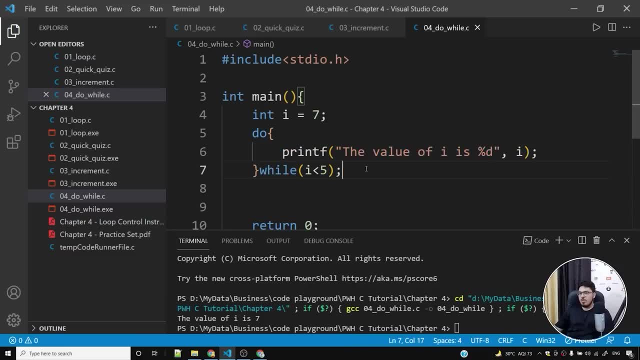 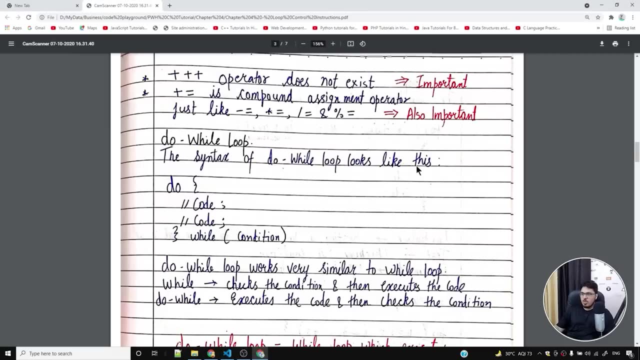 so this is how a do-by-loop works, and let me come back to the notes and show you how this thing works. do-by-loops look like this: do code, code while and then condition. do-by-loop works very similar to while loop. while loop checks the condition and then executes the code. do while executes the code and. 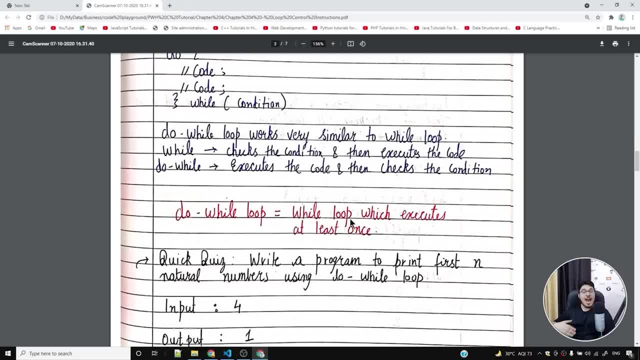 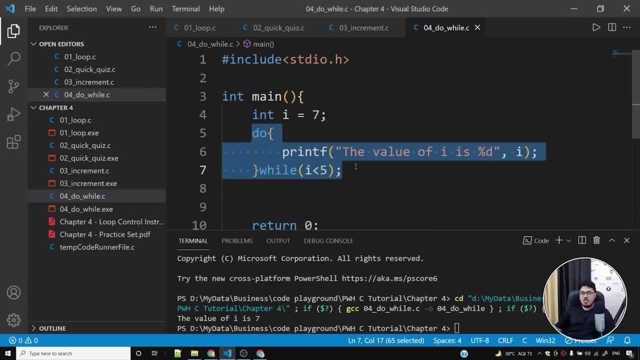 then checks the condition. so do-by-loop is a while loop which is executed at least once. okay, so this is something that you need to remember: whenever you have a do-by-loop, it has to be executed at least once by the compiler. okay, so this, no matter what, will be executed, at least. 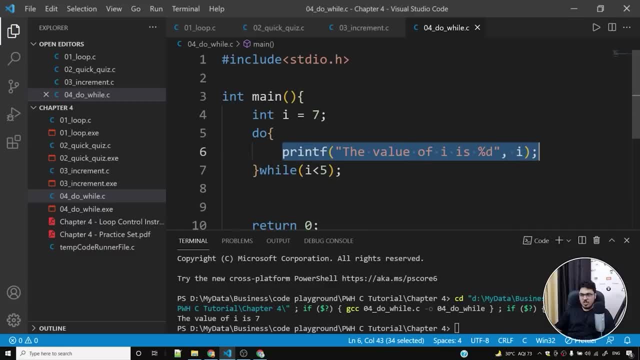 once. will it be executed again? depends upon the condition. as long as the condition is true, it will be executed. so you can look at do-by-loops as a while loop which is executed at least once for sure. will it be executed for the second time? maybe, maybe not. depends upon the condition. 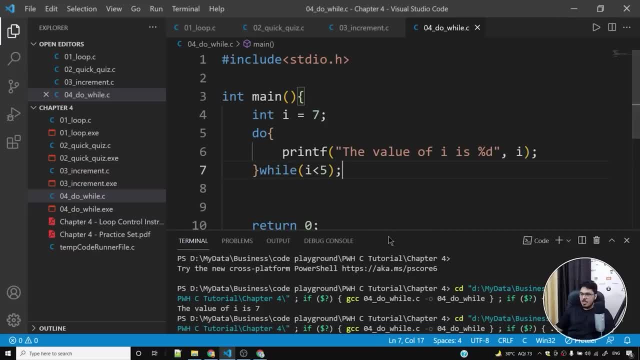 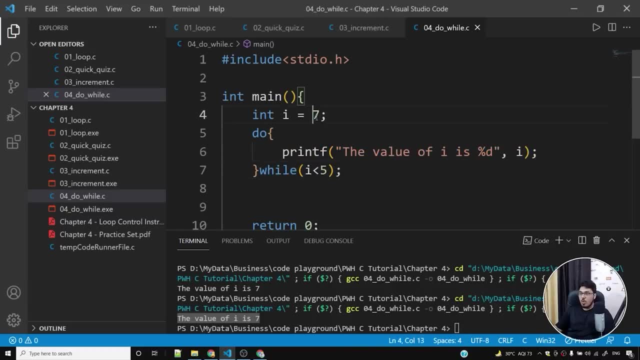 i'll show you something. so if i run this program, you'll see that the value of is7 is printed and this loop never repeats itself again. now what if i make it one so that the condition is true and also i'll keep on incrementing i inside the loop. what this will? 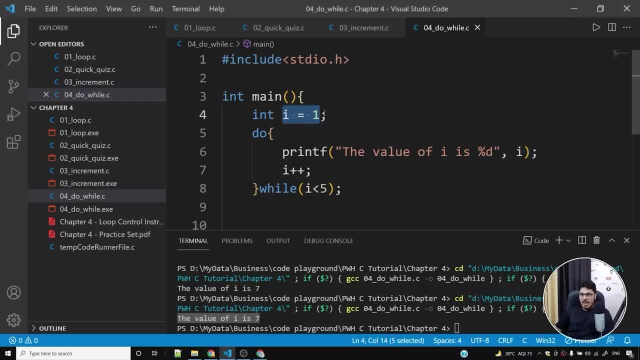 do is this will actually make the value of i as 2 in the second iteration, 3 in the third iteration, and so on. so for the first time, this while loop executes for sure and the value of i will become 2. so the value of i will be 2 and it will keep on incrementing and the do-by-loop will keep on. 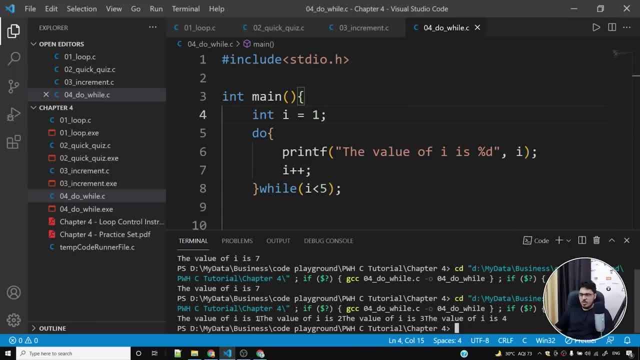 executing. let me show you: if i run this code, the value of i is 1, the value of i is 2, 3 and the moment the value becomes 5, you will have to halt the while loop because the condition is no longer true. so the do-by-loop will stop because the condition will be false and it will jump out. 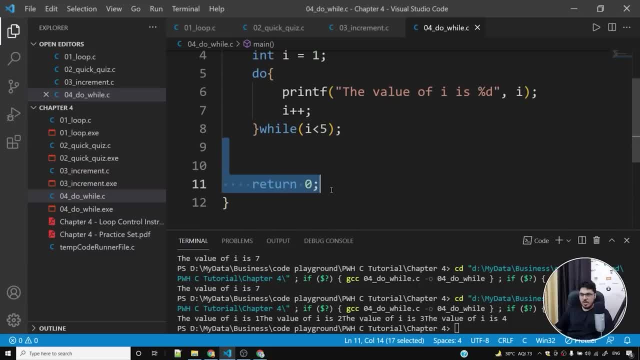 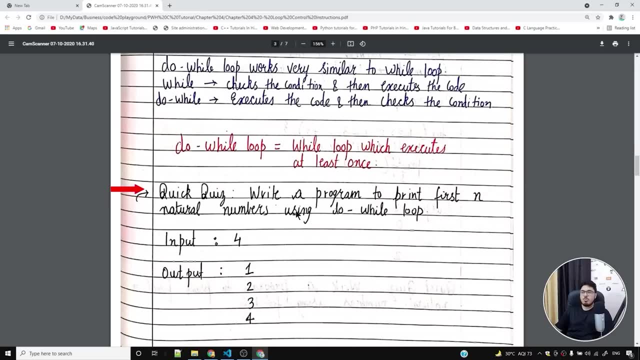 of this block and start executing the instructions here. okay, so this is how a do-by-loop works. i hope you got the hang of how this thing is working and here's a quick quiz for you. write a program to print first and natural numbers using do-by-loop. 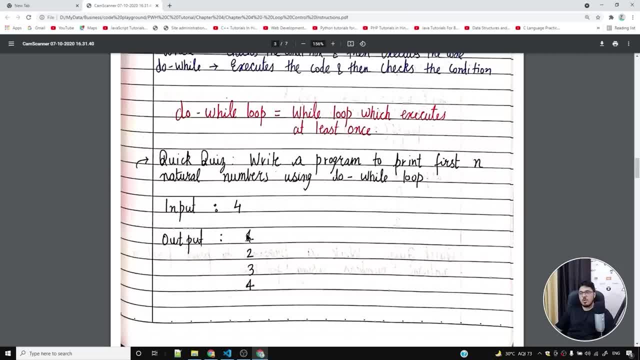 so if the input is 4, what you have to do is you have to write a program such that 1, 2, 3, 4 is printed like this. can you solve this? can you write a program for me? i want you to write this program. 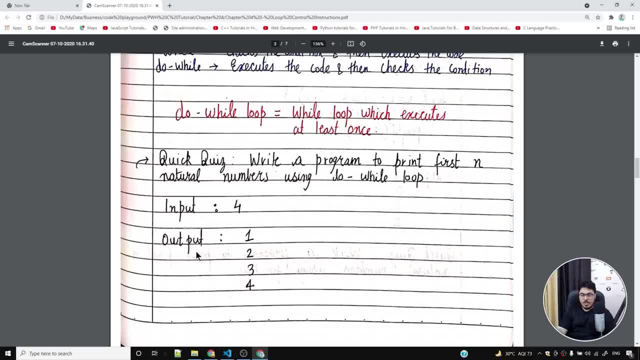 give me the time stamp of the video, wherever you are writing the program, and write a comment below. that way you will practice. i want you to comment and i want you to accept the challenge- right challenge, accepted in the comments at least- and just solve this problem. i mean, if you solve this, 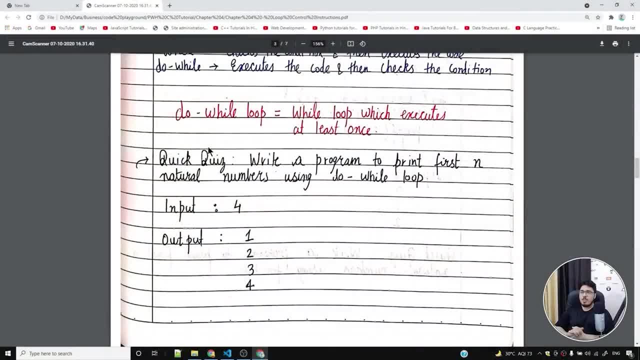 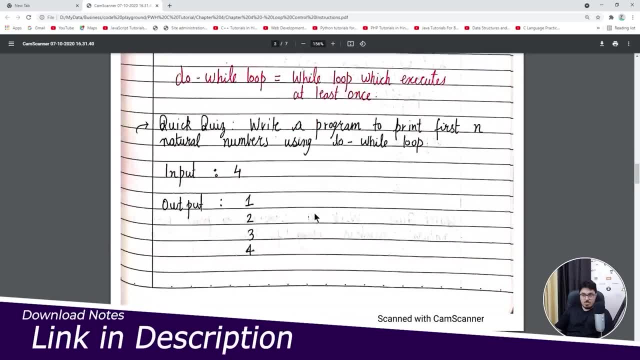 problem. you will understand the concepts, but if you keep on watching the video, i don't think that it is sufficient to understand and get hang of do-by-loop. just write one program at least and make sure you access these notes. i am saying it once, i'll say it again, i'll say it 10 times. let's. 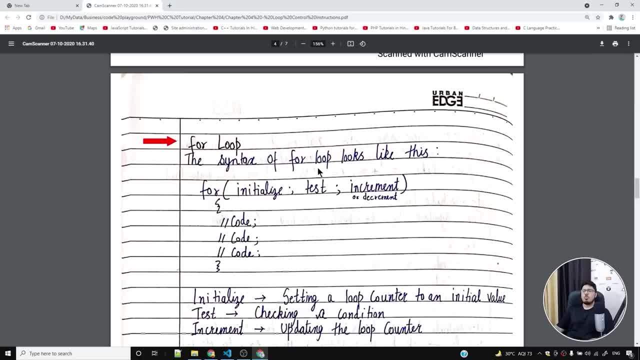 look into for loop. now. there is a syntax of for loop and whenever we talk about a loop, it's nothing but repetition of instructions. we have an instruction, we repeat it based on a condition and we repeat: if the condition is true, then once again we do the same thing and we keep on doing. 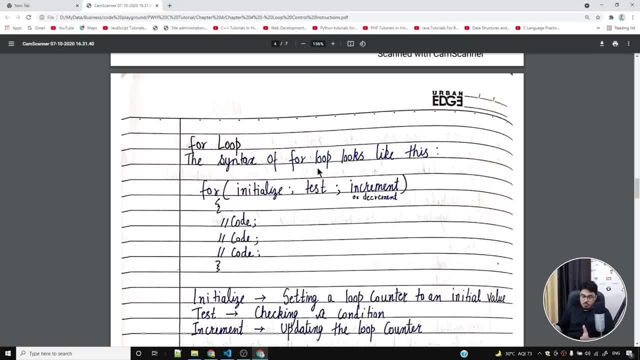 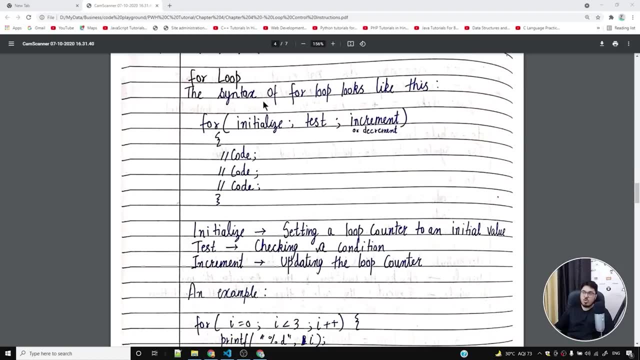 that until the condition is true. the moment it becomes false, that's it, the loop will terminate. okay, so the syntax of for loop looks like this: for initialize, test and increment or decrement, and then there is some code inside. let me explain this to you. this might sound very haunting to you. 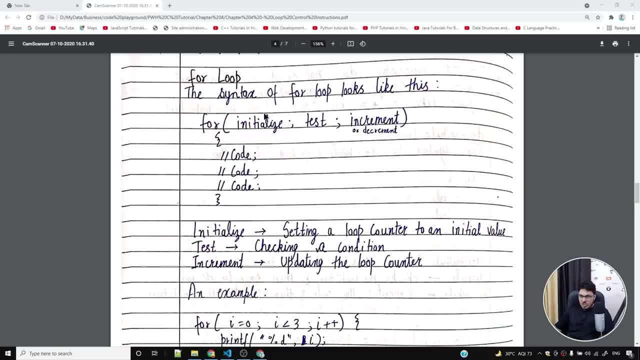 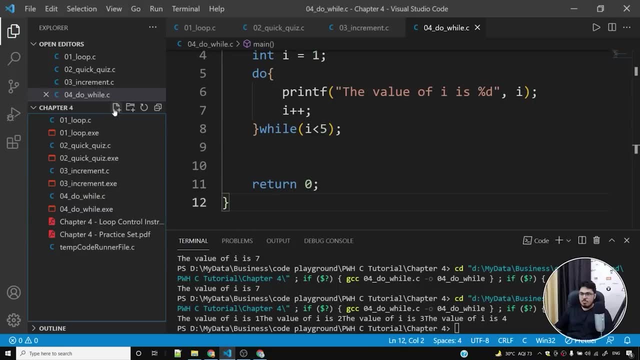 if you are a beginner, inside a for loop, we have an initialized block, a semicolon- then a test block, a semicolon, then some line of code which will increment or decrement or variable which we initialized here. so let me show you how this works. okay, and once i show you the example, it will be: 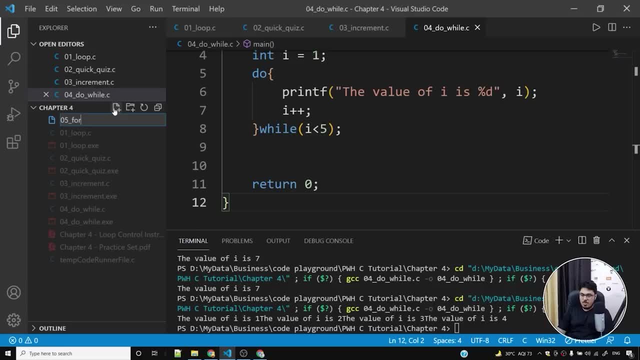 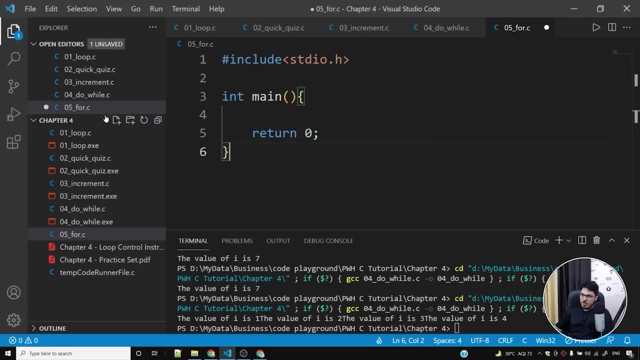 easy for you to understand how for loop works. so i'll simply say: for dot c i'll add a boilerplate code. let me start typing for, and the moment i start typing for, i should get some snippet. so if i say for, you can see that code snippet for for loop. 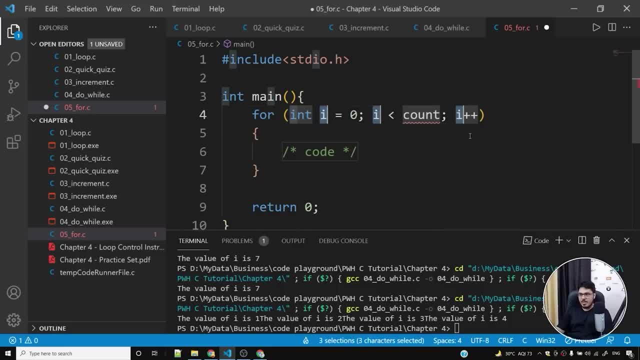 once i click this, i can change this. to end, i can press tab. i'll keep it as i. i'll make it seven once again, i'll press the tab key and i can write some code here. in case you are not able to get this snippet, you can type this out. you can type this line, this line and this line out sometimes. 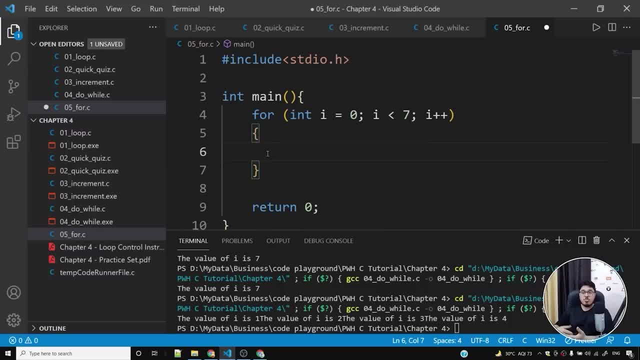 you might not get the snippet. sometimes the extension might not work. you might be on a slower computer. there are n number of things which can happen. do not stop. i have seen a lot of students stopping just because they are not getting the snippet suggestion. that's, that's not. 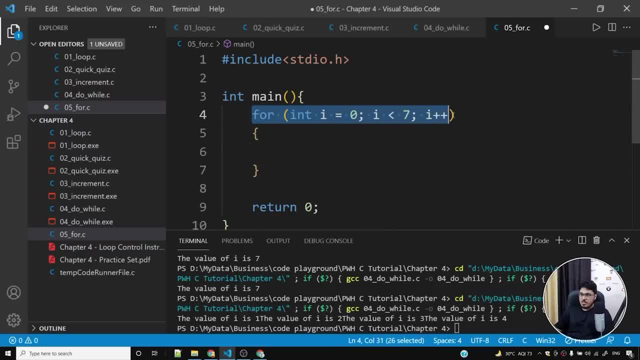 good. okay, now for int. i is equal to zero, i is less than seven, i plus plus. let's print the value of i. let's do the simplest task we can do with i and we can say the value of i is. i'll simply say percentage d and what i'll do is i'll print the value of i. also, i want to print a backslash n. 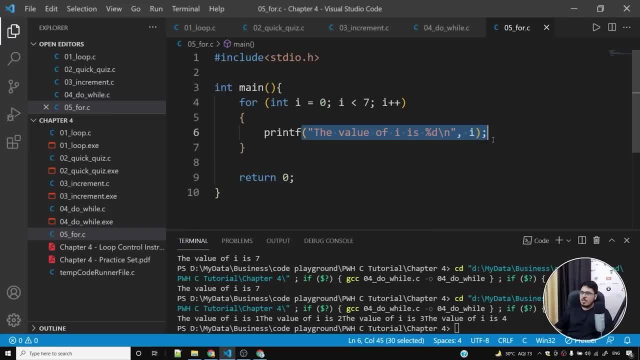 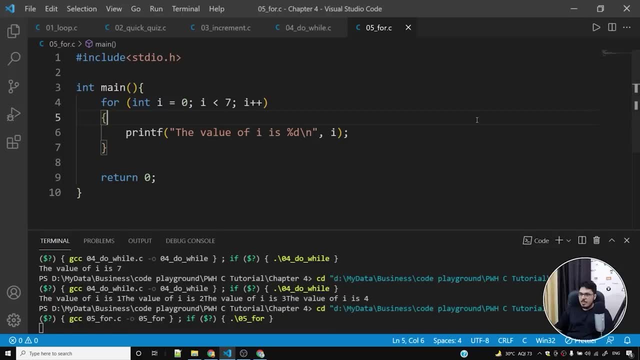 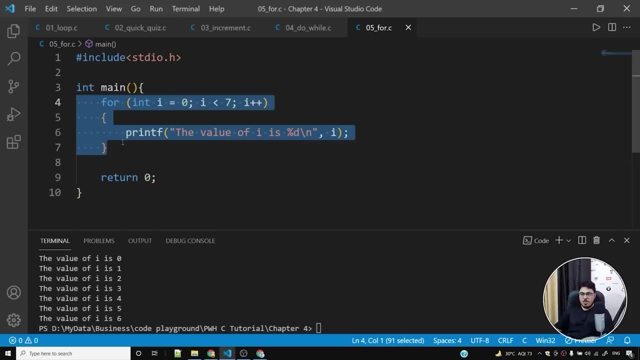 such that you'll be able to see a new line after the value of i is zero. one, two, three, four is being printed if i run this program. let me run this program and show you the output. i starts from zero and stops at six. how does this loop work? let me show you so whenever. 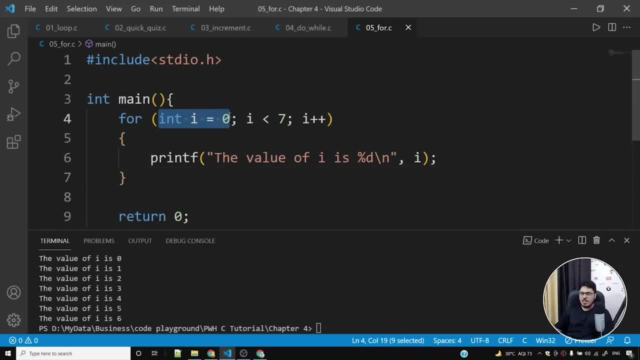 you have this for loop. this initialized part is executed just once, so int i is equal to zero will be executed once. then what happens is it will check for this condition. if this particular thing evaluates to true, then only it will move ahead. if it doesn't evaluate, 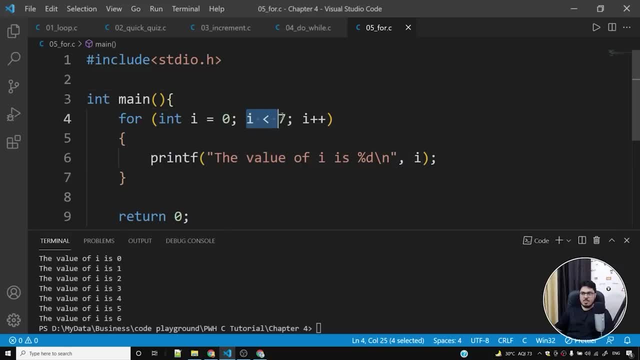 to true, it doesn't move ahead, okay. so is i less than seven? yes, it is. it will move ahead, okay, and it will execute this. so the value of i is zero will be printed, as we can see here. now what happens is: listen to me very, very carefully, because this is important, and once you understand, 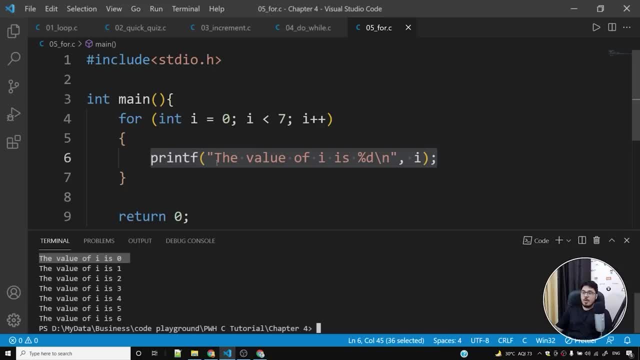 how for loops work. it'll be easy for you, believe me. so print f: the value of i is percentage d, and once this line is executed, what happens is this particular update piece of code runs, and what it does is it will simply increment the value of five by one. so if i was zero before, it will become one. 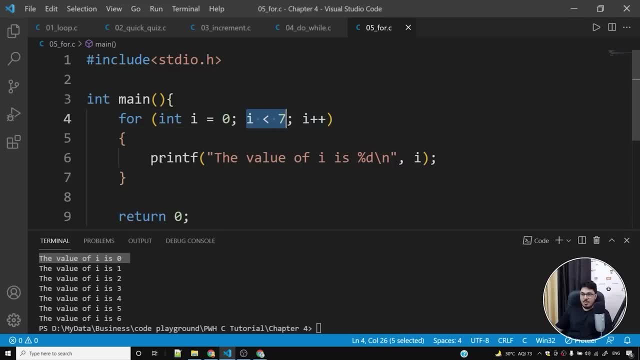 now what will happen is it will check this condition again and then it will print the value of i if the condition is true. if the condition is false, it will jump out of the for loop and it will stop the loop. okay, so i'm starting over. i'm telling you once again about the for loop, in case 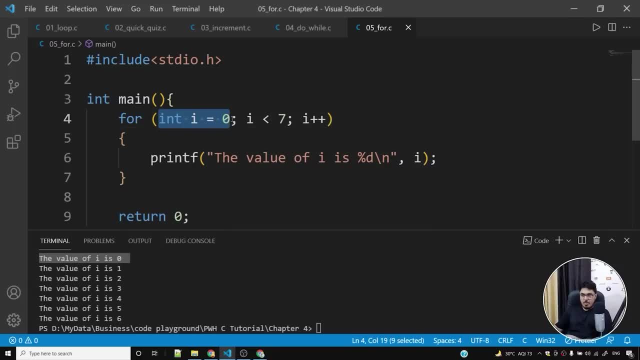 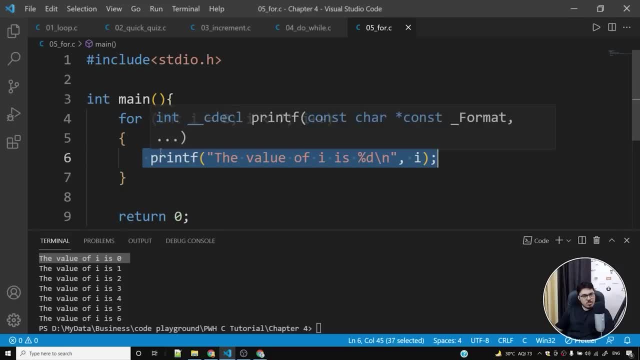 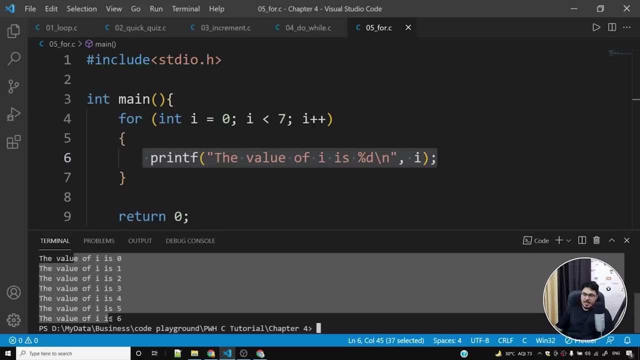 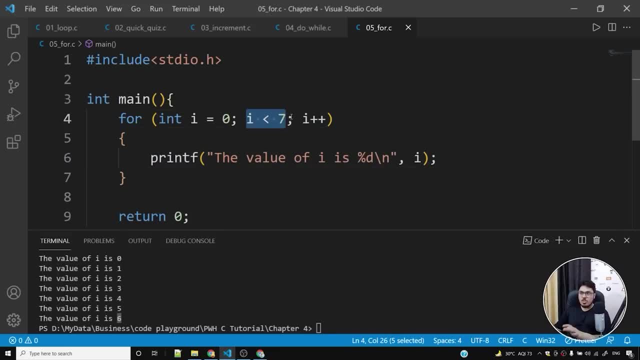 10. Is 7 less than 7?? No, This condition is false. 7 is not less than 7.. since this condition is false, what will happen is this: for loop will be stopped. we'll come out of this for loop and the moment we come out of this for loop, the instructions after the for loop. 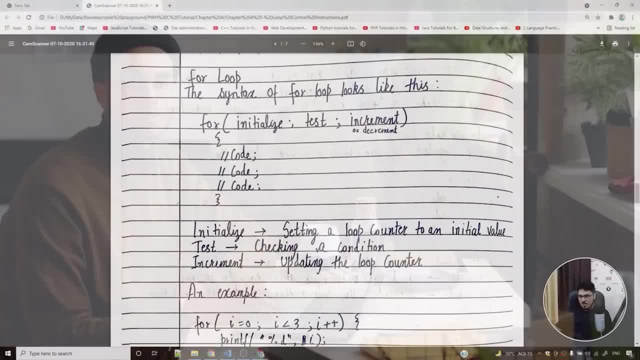 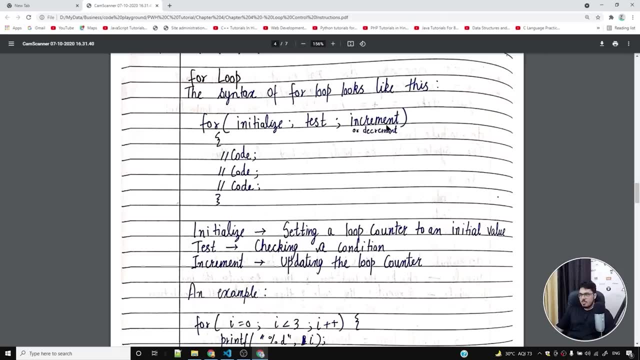 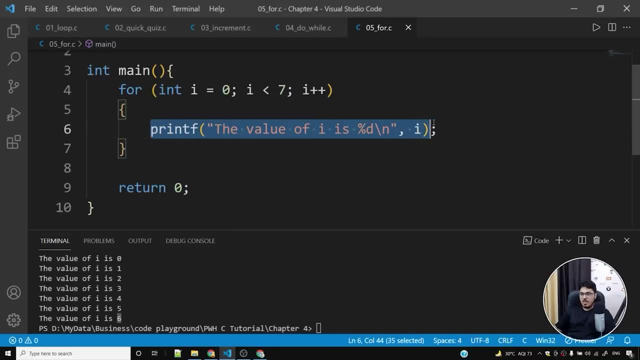 will be executed. i hope you understood how for loop works. we can come back to the nodes and we can see. the syntax of for loop looks like this for initialized test, increment or decrement, and then the code runs. it might be more than one line of code. in this example, i have just a single line. 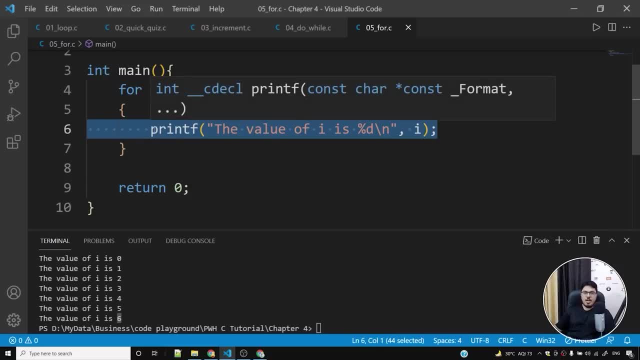 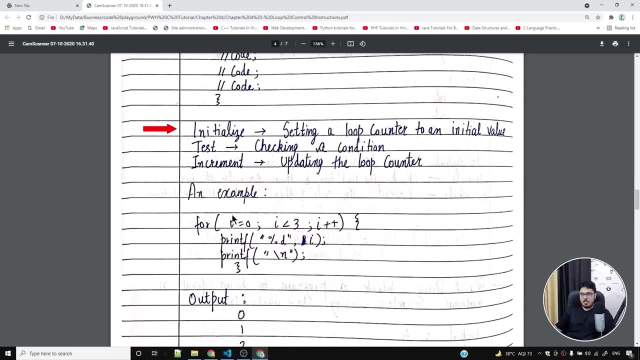 of code. it can be three lines, it can be four lines, it can be 10 lines, it depends. okay, you can add as many lines as you want. so, coming back to the nodes, initialize, test increment. i've explained a bit about what initializes, what test is and what increment is in most of the cases. initialize. 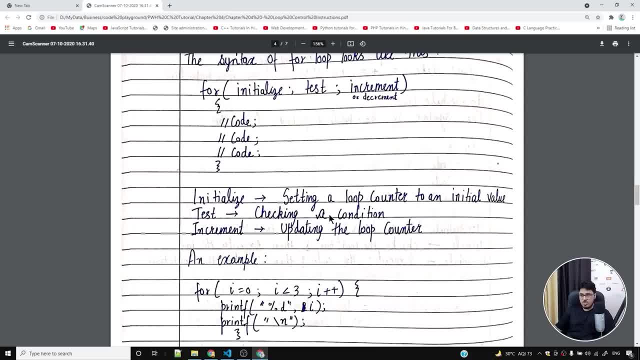 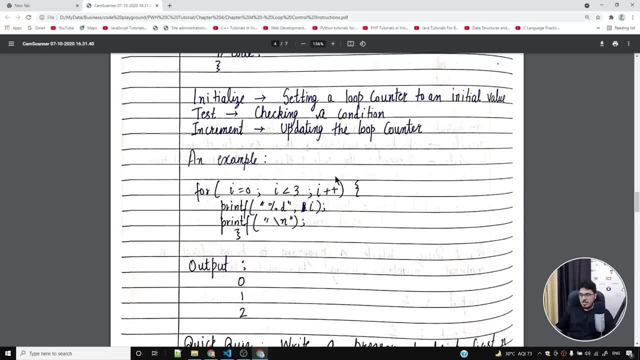 will be setting a loop counter to an initial value. test is checking for a condition. increment is updating the loop counter, and here is an example. so i've done the same thing. i've mistakenly written ampersand i, then i scribbled it off. so if i is equal to zero, is less than three i plus plus zero one, and 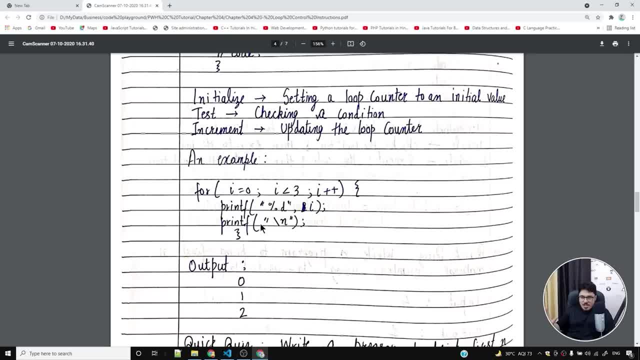 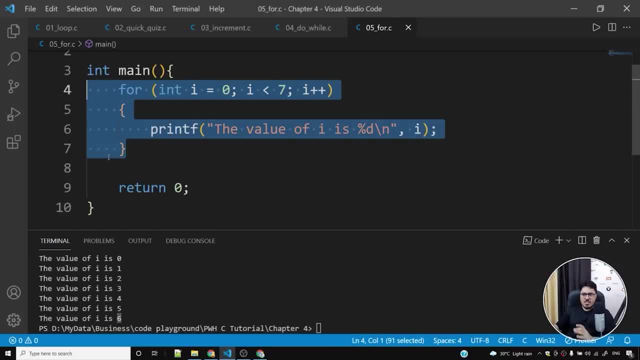 two will be printed, so you might want to remember this. i mean, when i say remember this, i don't want you to mug up the code and the output, but you should at least understand that this for loop will print value starting from zero to six, because here i is less than seven and i plus plus. but let 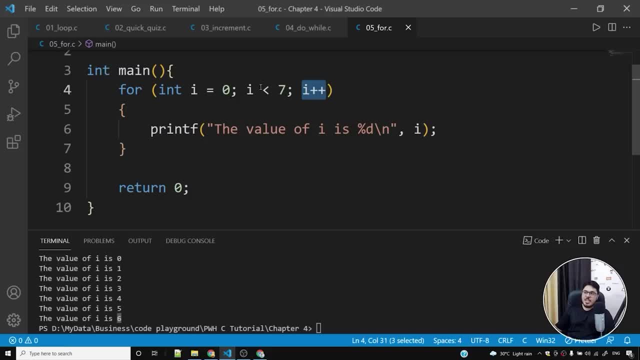 me tell you one thing: in some cases, your examiner might change these values to something that will produce an output different from the output you might expect. okay, so do not mug up the output. look at the for loop very, very carefully when you are solving a problem. but 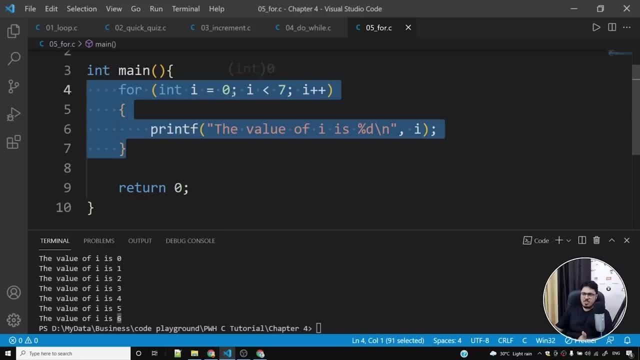 if you are looking at this loop, which is a very simple loop, yes, it will print from zero to six. but if i change the condition to something like this: say i, i make it, i minus, minus, then then the things are going to change. then you'll have to do the dryer and you'll have to see what the value. 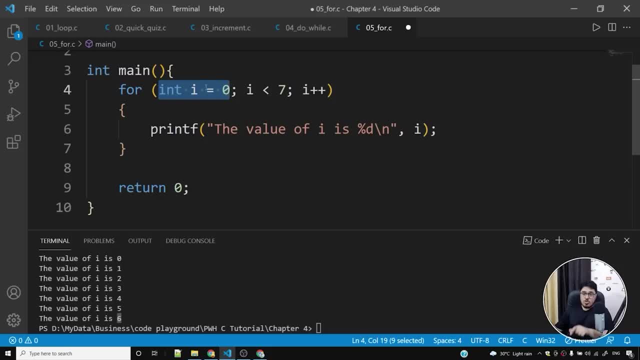 of i is you'll have to execute all these things one by one, so you will initialize: first check for the condition, execute this thing. if the condition is true, execute this thing. then check the condition, then execute this thing. if the condition is true, then you run this, then again check the condition. if the condition is true, you run this and you keep on. 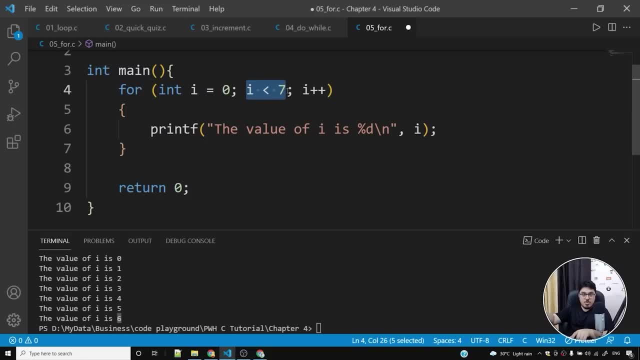 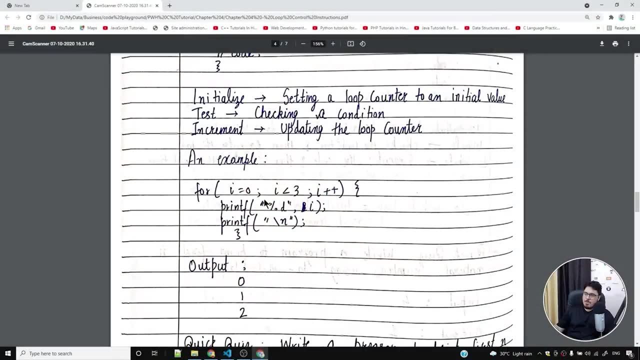 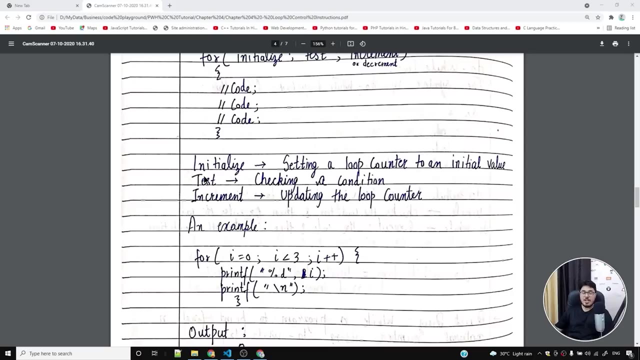 going until this condition becomes false. until this condition becomes false. okay, i hope you understood the for loop now. i hope that i was able to explain you how for loop works. okay, the output is going to be the same as the output. so i hope you understood the for loop and i hope that you. 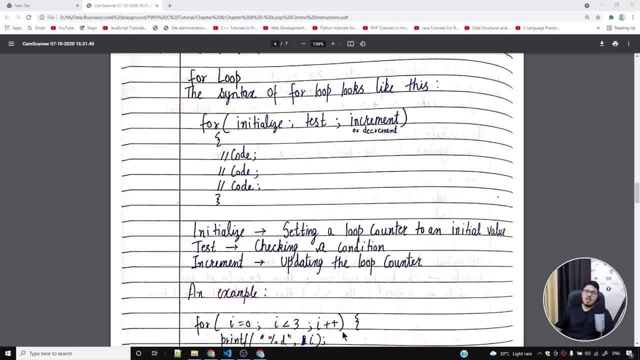 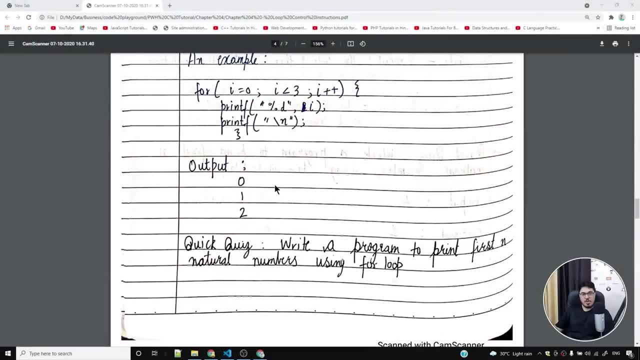 have written a code and also i have made things easier for you by writing all these things in the notes. i have written the meanings of initialize, test and increment, and i hope that you are going to love for loops. this is something that you're going to use a lot when it comes to programming. 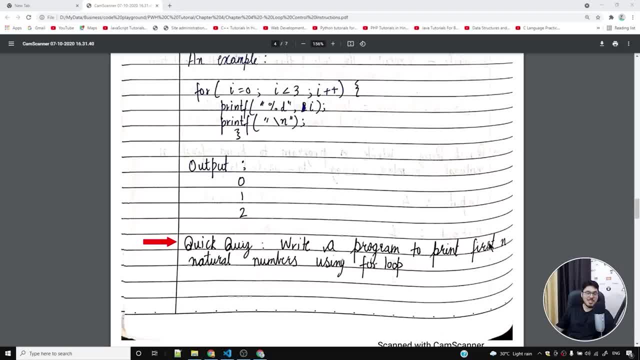 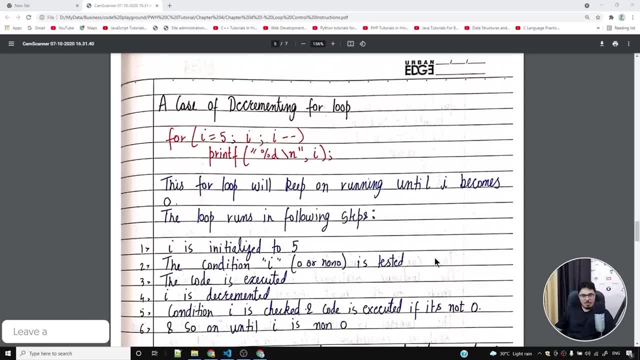 let's solve a quick quiz now. write a program to print first and natural numbers using for loop. we have already written that. but again i want you to use scanf function. take the value of n from the value of n. you drop me a comment below with the timestamp and tell me that you have solved this. 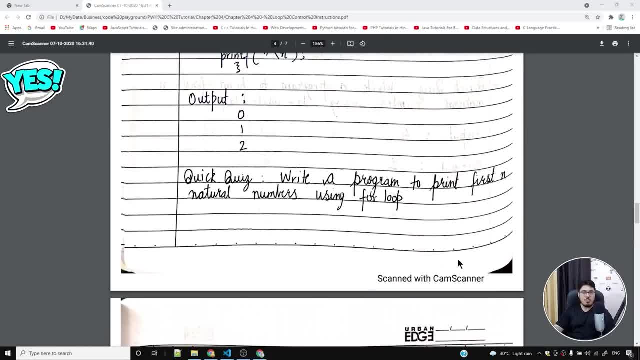 problem. were you able to solve this problem? i want a yes comment from all of you. that will really be very satisfying for me if i have a yes comment from all of you saying that, yes, we were able to solve this quick quiz. i can't tell you how good i feel when you guys comment and tell me that you 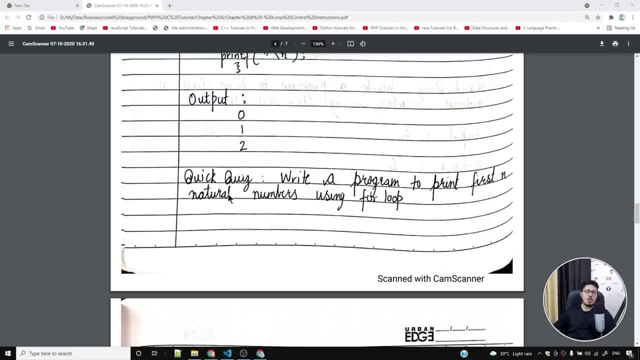 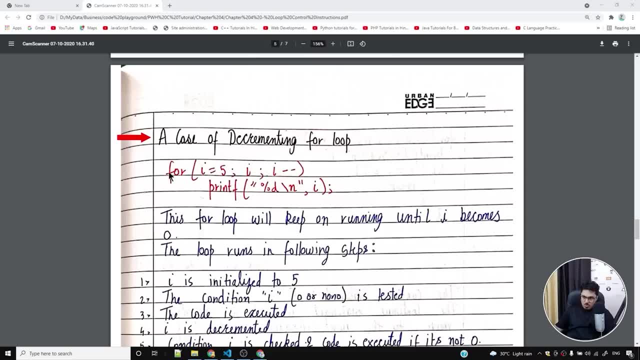 are able to do something. just make sure you write a comment below for me and tell me that you were able to solve this quick quiz. let's move ahead and let's look into the case of a decrementing loop. So we have a loop, we have a for loop, but these things are not looking as good, or rather as simple. 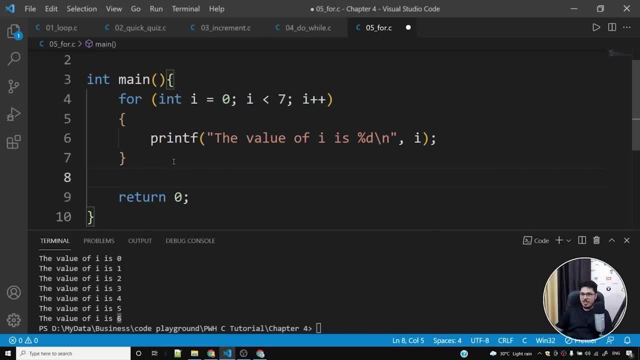 as they were looking here. This for loop looks pretty easy and we are able to make out that the value of i will be from 0 to 6 and this statement will be executed for the values of i from 0 to 6 seven times. From 0 to 6 is seven times. Okay, this was very simple for loop. Let's write a. 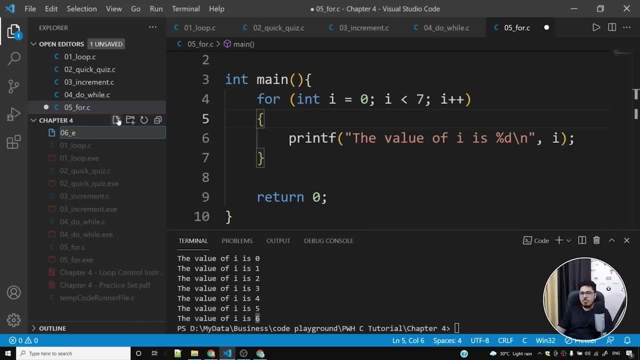 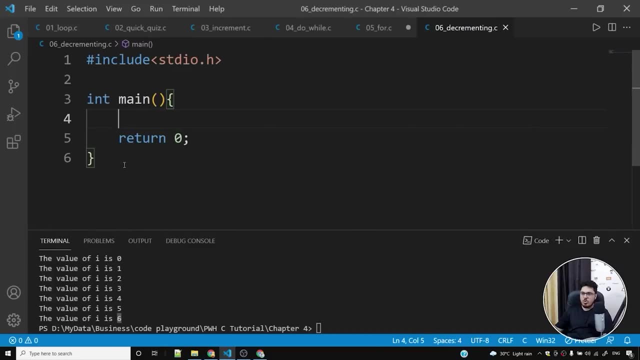 program and let's try to understand how this decrementing for loop works. So, decrementing dot c. So I've written a boilerplate code. Now what I'll do is I'll simply what I'll do is I'll save this program and I'll start writing this for loop. Okay, so I use the snippet, but I'll write this: 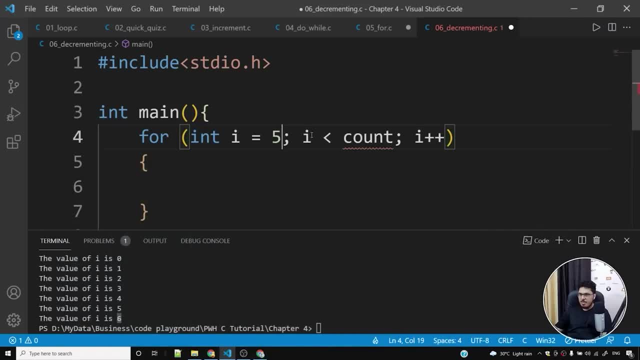 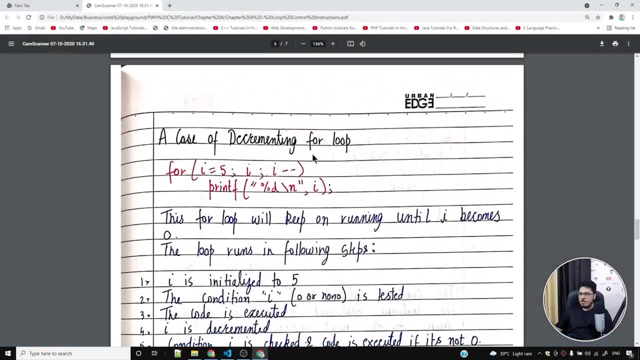 So I'll say: int i is equal to five, Then we have just i. here Is i a condition, We'll talk about it Just a moment. i minus minus. Let me write this down- and we are simply printing i. So what I'll do is I'll save. 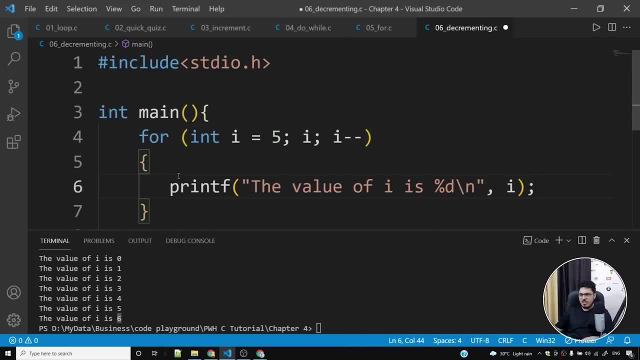 this. I'll copy this and that's it. I'll paste it here. So we are printing the value of i, So i, starting from five, then i, then i minus, minus. Let's try to use the skills that we learned. 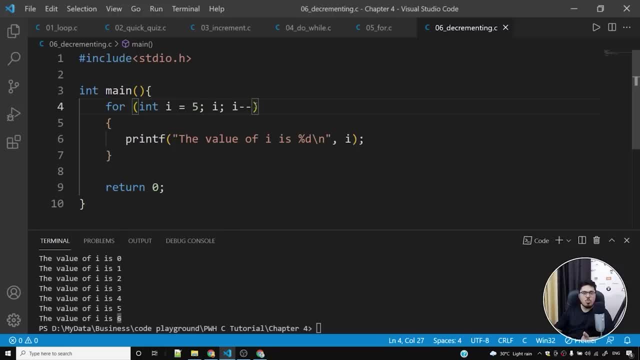 Let's try to use the concept of how for loop works to decode this and understand what will be printed on the console. Okay, let me close this terminal. So i is equal to five initially. Okay, This is a condition. So what happens is i will be initialized to five. This condition will be checked. Is five true? Yes, 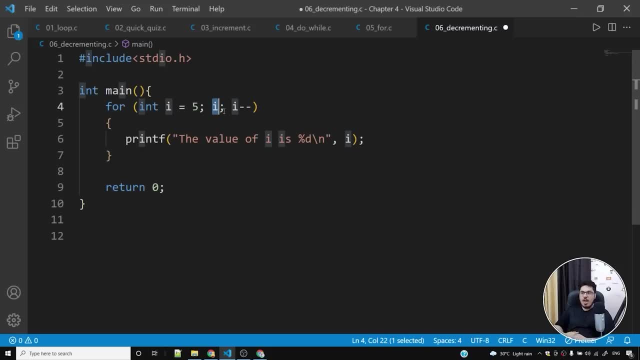 five is true. Any non zero value is true. I've told you before: Zero is false, but five is true. So since five is true, this will be executed for five. So what will be printed? The value of i is five will be printed and backslash n will be printed. 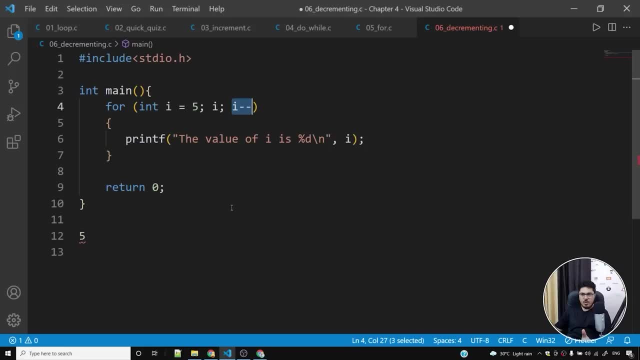 Now, what is the value of i? The value of i is four. Okay, So let me write the value of i. The value of i is four. This is the output and this is the value of i. Okay, Now is four true? Yes. 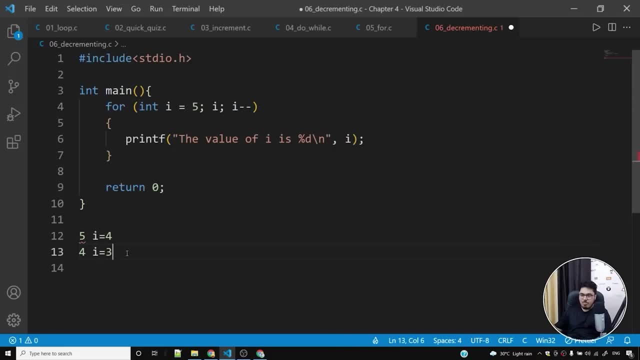 four. is true, Four will be printed, but the value of i will become three, because this will get executed. This is the updation condition. In a very, very similar way, three will be printed. Two will be printed. Sorry, the value of i will be two. Two will not be printed. Two will be. 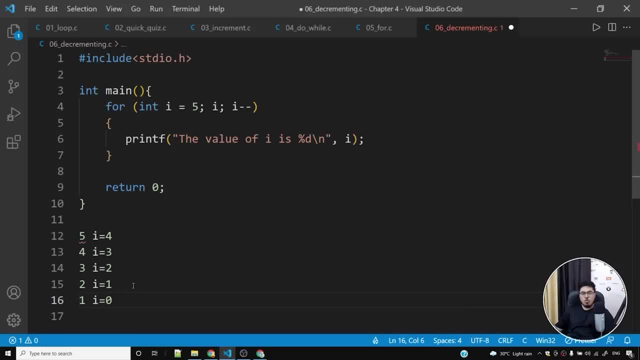 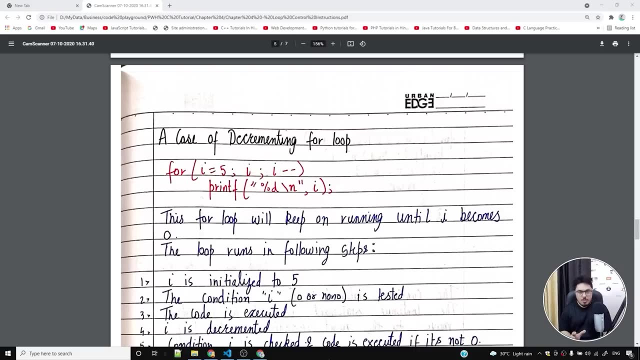 printed. Eventually, what will happen is the value of i will become zero, which will make this condition as false. I repeat, it will make this condition as false. So sometimes you'll have to run the loop one by one, one iteration at a time, and then only you will understand how this loop. 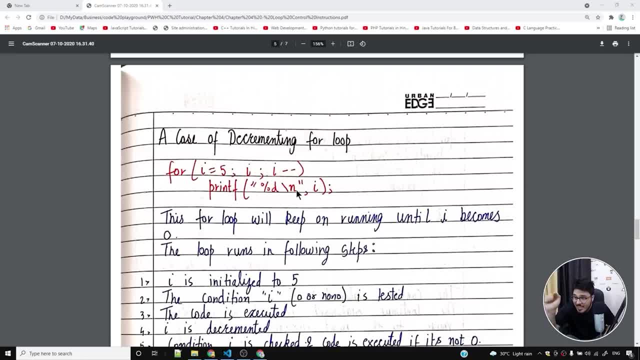 is working. But to make things easier for you, I have printed five, So two will be printed, but the download case will be etched every twoliq times. So this is the loop order, right? This will be have written how this decrementing for loop is working inside the nodes. so this for loop will 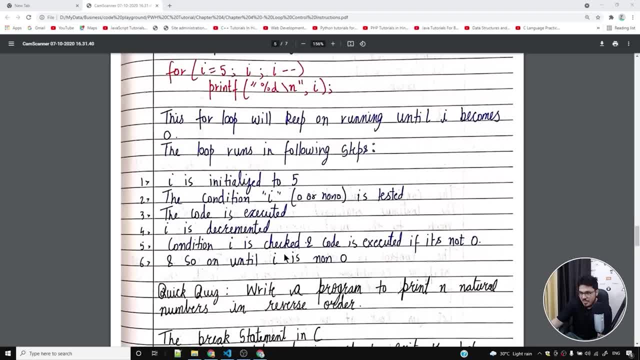 keep on running until i becomes zero. the loop runs in the following steps: i is initialized to five. condition i- zero or non-zero- is tested. the code is executed. i is decremented. condition i is checked and code is executed if it's not zero, because any non-zero value is true in c. we have seen that we. 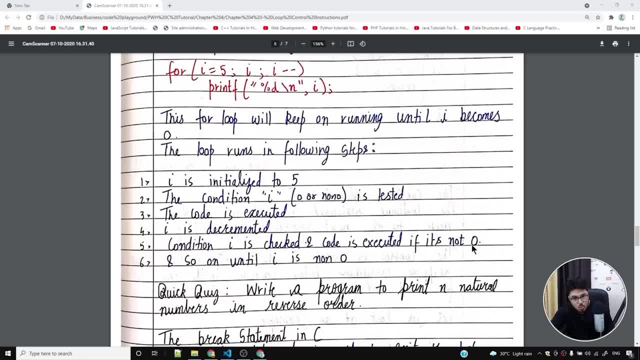 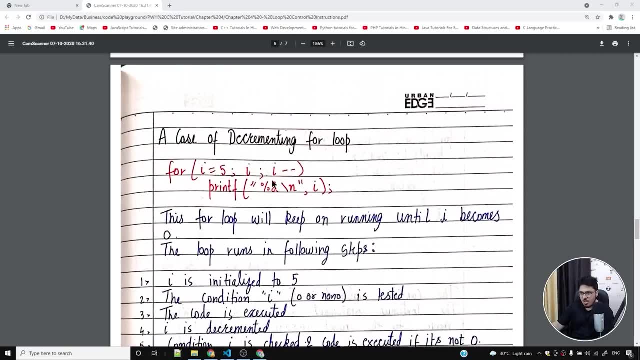 have learned about that. anything which is not zero is true. anything which is zero or evaluates to zero is false. in c and so on. until i becomes um, until i become zero, okay. so as long as i is non-zero, you will keep on seeing the iterations. as soon as i become zero, loop will halt, loop will finish, okay. 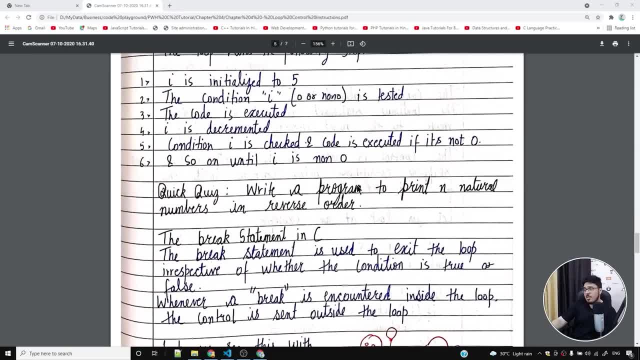 i hope i was able to explain you this: write a program to print n natural numbers and reverse order, and i want to you to do this. in fact, we have already done that, but i want you to like this program. just take input from the user using scan a function and start writing this code. i hope that you liked. 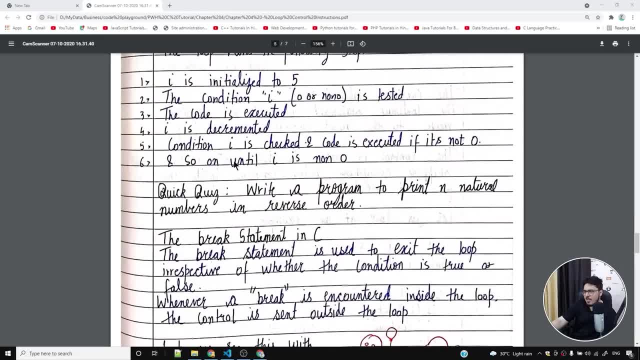 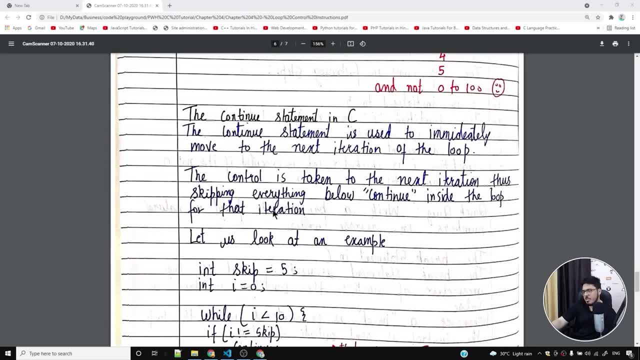 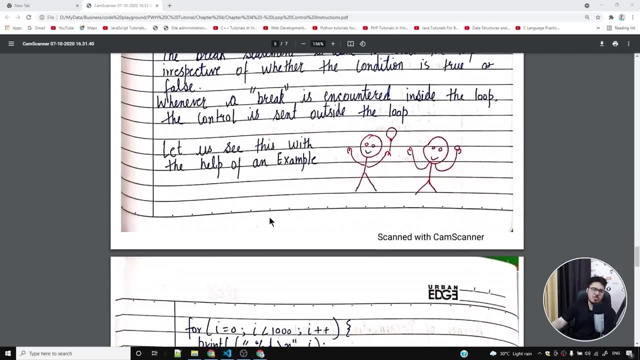 this concept of decrementing for loop. let's move forward and let's talk about the break statement in c and also let's talk about continue statement in c. both break and continue statements are really very important in c and we are going to look into these two statements. 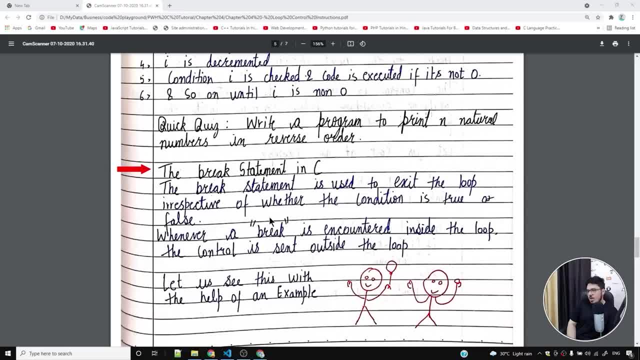 now. so what is a break statement? the break statement is used to exit the loop, irrespective of whether the condition is true or false. what does that mean? we have seen break in switch case statements, by the way, let me tell you. but now we are going to look at break statement. very, very. 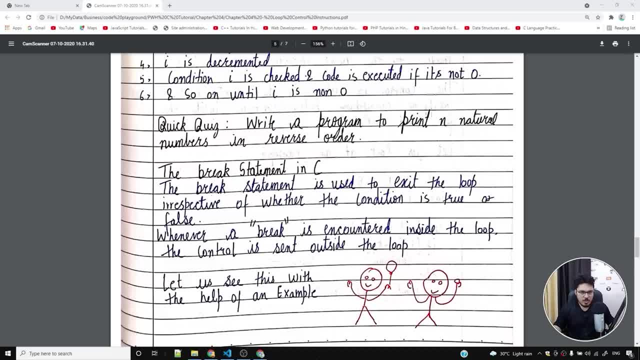 closely. so break means stop what you are doing, just execute the next instruction. so if you are executing a switch case statement, stop right here, go out of switch and execute something else. execute something else, and then you are going to look at the break statement very, very closely so. 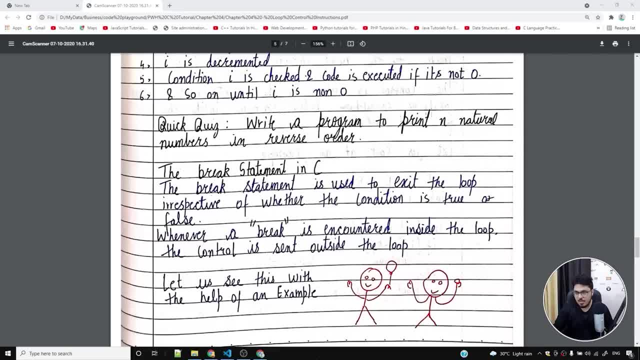 execute whatever is after the switch statement. similarly, if you are inside a while loop and i type break or i encounter a break statement, what that tells me is: stop this while loop right here and execute the next thing. what does it say? it says that stop this loop right here and execute. 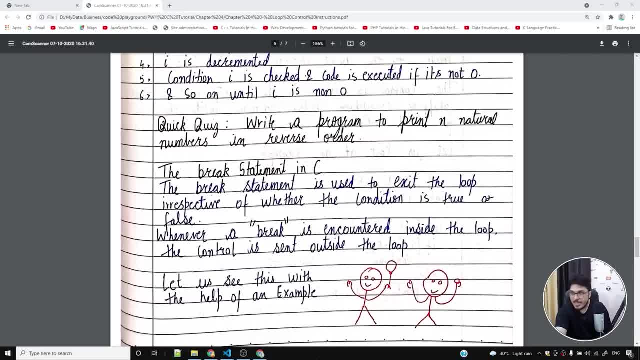 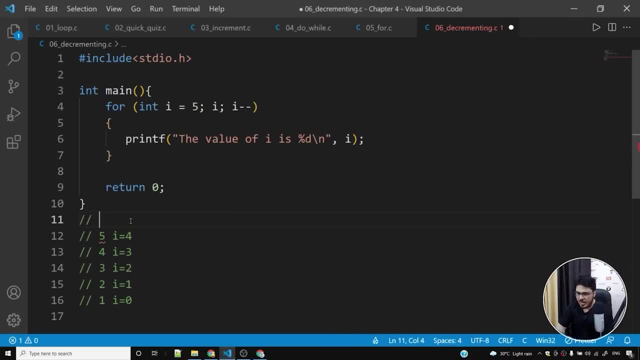 the next thing: it can be inside a while loop. it can be inside a do while loop, it can be inside a for loop, it can be inside any kind of loop. it can be inside a switch statement. let me show you how this works. so break statement is very, but let me comment this and let me also write down dry. 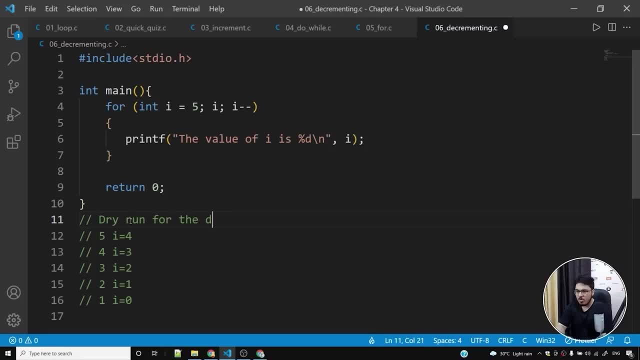 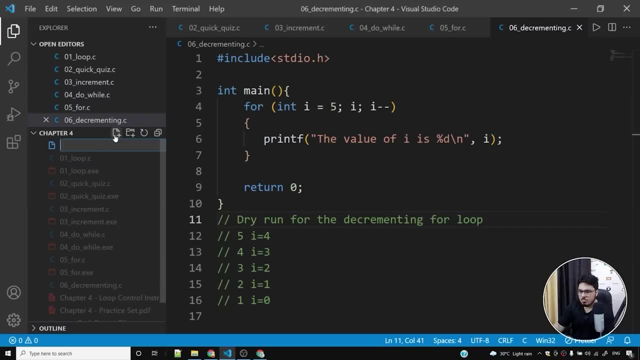 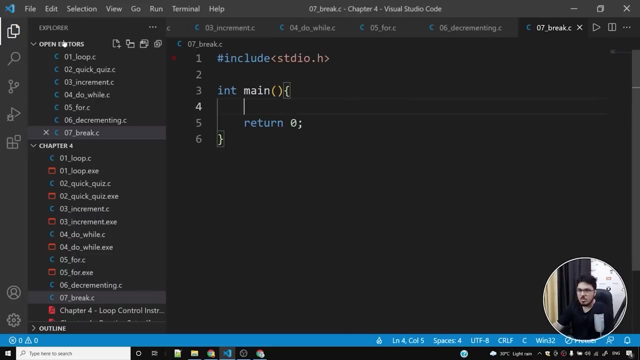 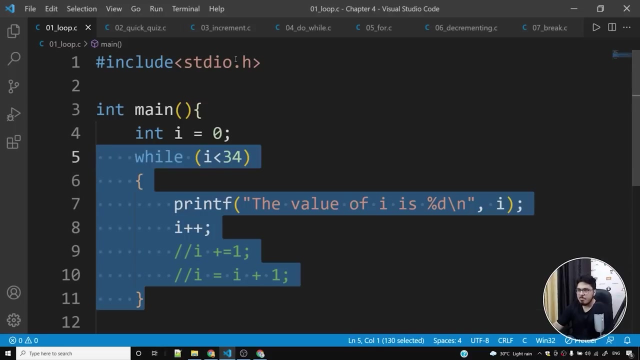 run for the decrementing for loop. okay, so let's now. let's now start writing this break: dot c. i'll add the boilerplate code and what i'll do is i'll write a very simple while loop. let me copy this while loop from here. this is a very simple while loop, and we have talked about this while loop a lot. 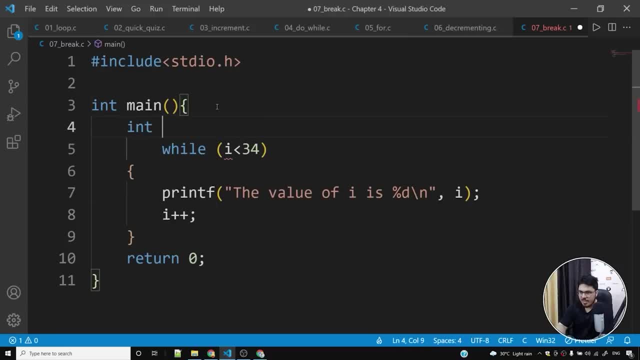 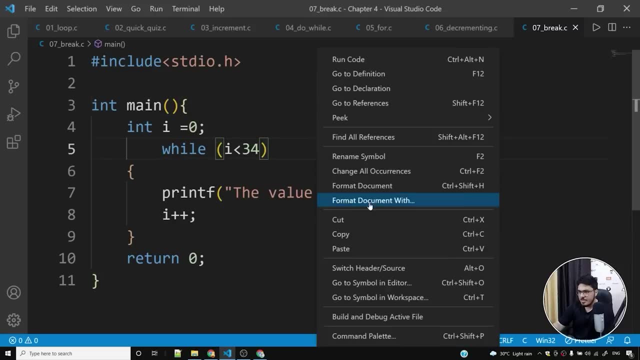 okay, we are simply incrementing the value of i, we are initializing the value of i to zero, and i think i copied the loop correctly. yes, i did. i'll simply say format document. it will document for me. by the way, you can do this if you, if you didn't know this, you can always do. 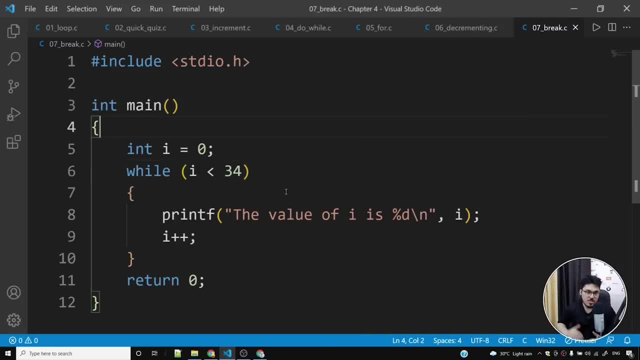 right click format document and that will format your c code in this beautiful fashion. okay, so int i is equal to zero, while i is less than, i'll make it eight. so this will print zero, one, two, three, four, all the way till seven. okay, if i make it less than. 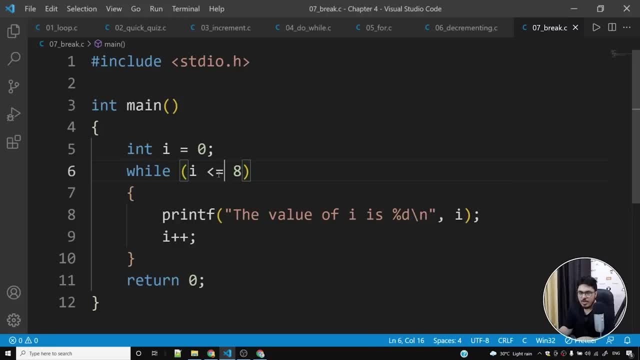 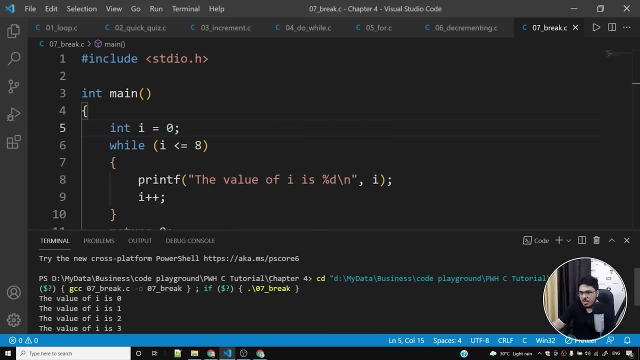 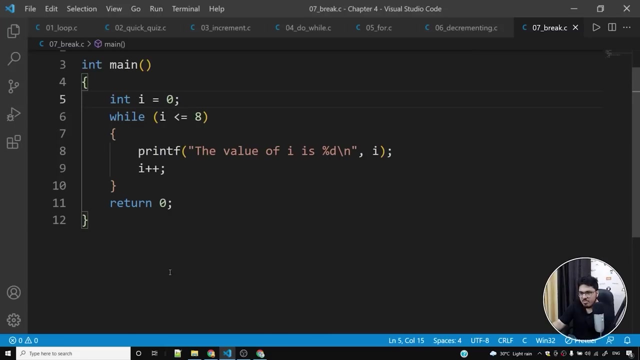 equal to it will print, starting from zero, all the way till eight: okay, zero one, two, three, four, five, six, seven, eight. and let me execute this and you can see the value of i: zero one, two, three, four, five, six, seven, eight. okay, so this is how it works. nothing new here, nothing fancy here, but let me tell you what is new now. 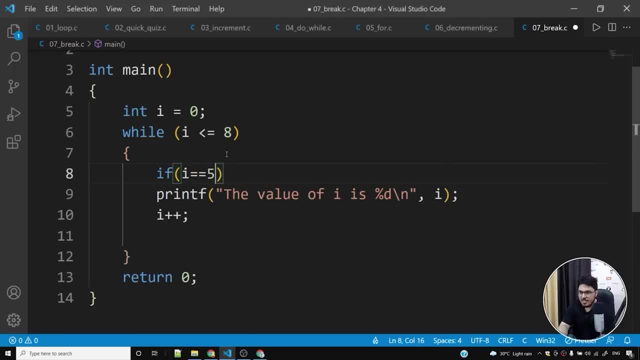 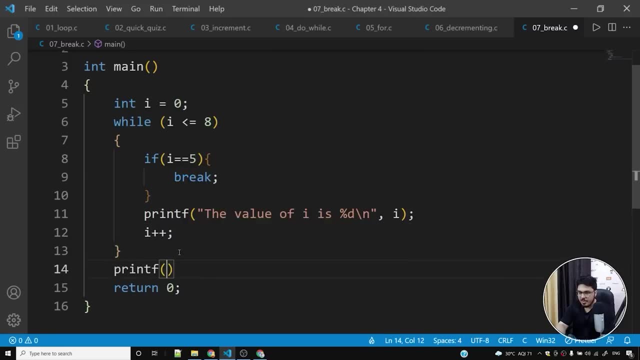 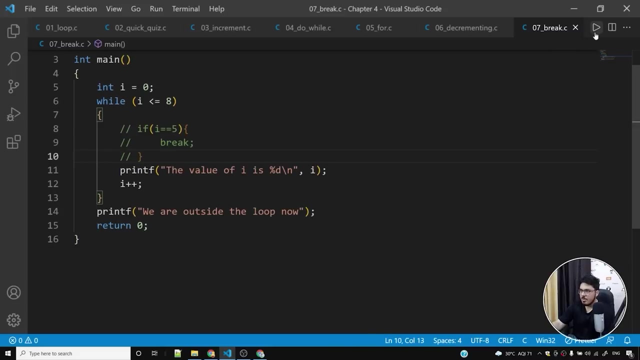 so i can write something like this: i can say: if the value of i is 5, i want to break out of this loop, and also i'll write a printf here and i'll say: we are outside the loop now, okay. so even if i even have this one and I run this code, you'll see that after the last statement we are. 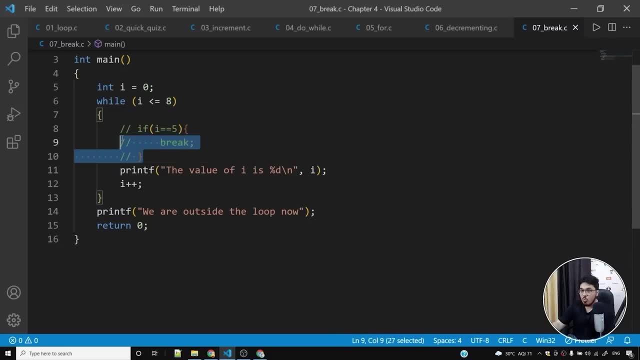 outside the loop. now is printed. okay, Now what will happen if this is present? What will this do? This is simply saying, if the value of i is 5, you break out of this loop. So 0 will be printed, 1 will be printed, 2 will be printed, 3 will be printed, 4 will. 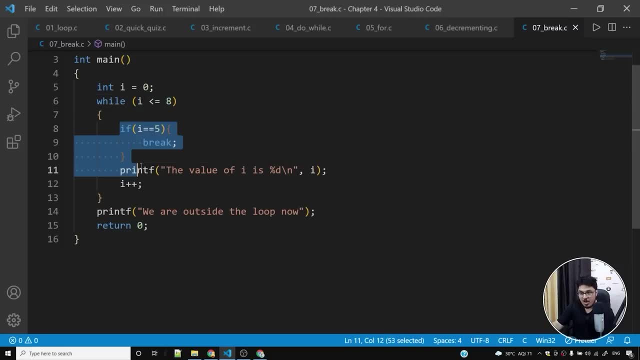 be printed, but the moment i becomes 5, this will be encountered. this condition will be true, break will be encountered. and the moment break is encountered, it instructs the C compiler to throw the control out of the while loop. So now, what will happen is it will come out. 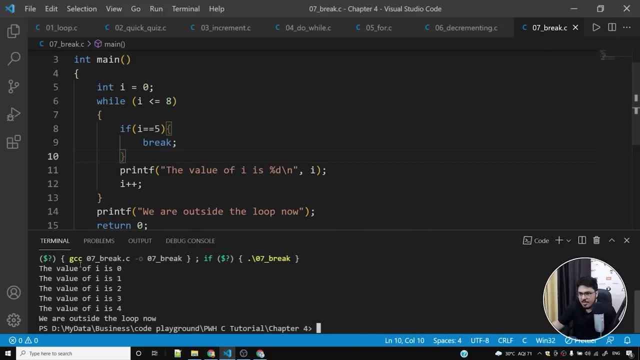 of the while loop. okay, So let me run this and 0,, 1,, 2,, 3,, 4, and the moment i becomes 5,. what will happen is this will get executed. And what does this mean? Break means break. 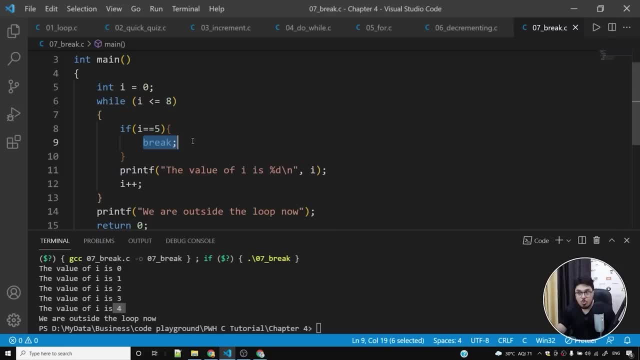 out of the loop. I don't want to execute this loop anymore. I want to stop right here and I want to jump out of this loop. So where was this loop? starting At line number 7,. this is the block of the. 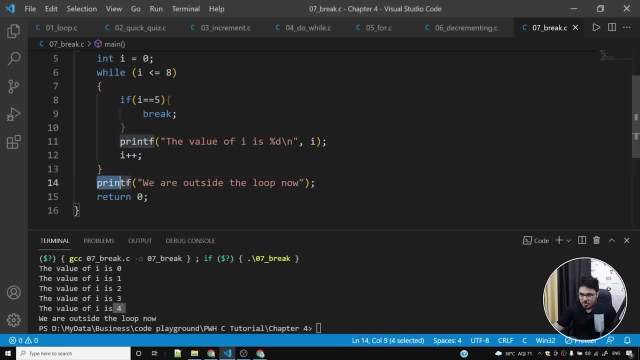 loop and it will jump out of this and will start executing statements from here. okay, I hope I was able to explain this. I hope I was able to explain it pretty well and I hope that you understood it okay. So let's come back to the notes and read about the. 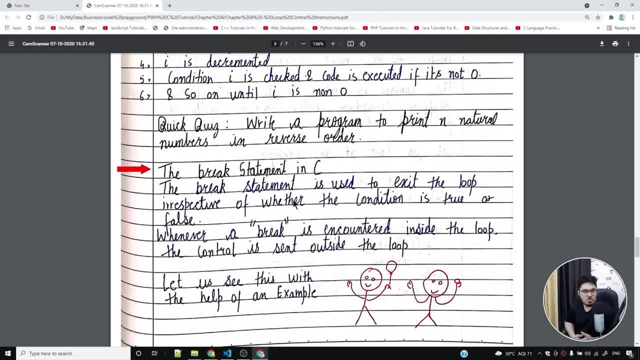 break statement. So what will happen is when i exit the loop, it is not going to execute the loop, whether the condition is true or false. So the while loop works on the basis of condition okay. It will check the condition again and again. if the condition is true, it will execute. 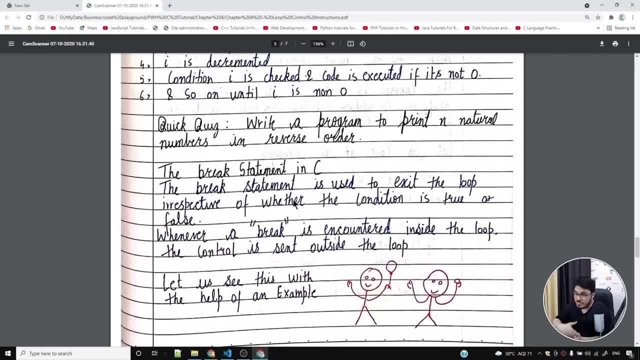 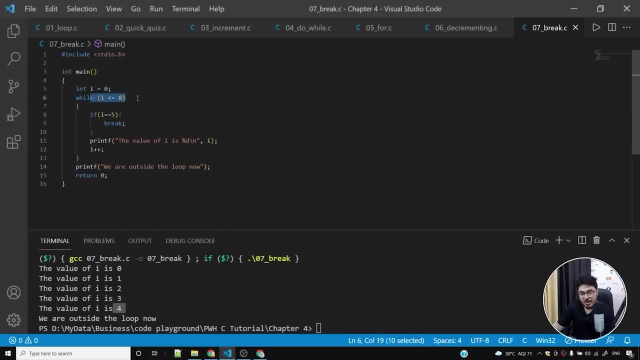 one iteration. If the condition is true, once again it will execute next iteration, and this keeps on happening. Now, what will happen is the moment the value of i becomes something which makes this condition of while loop false. the while loop will stop. This is one way. 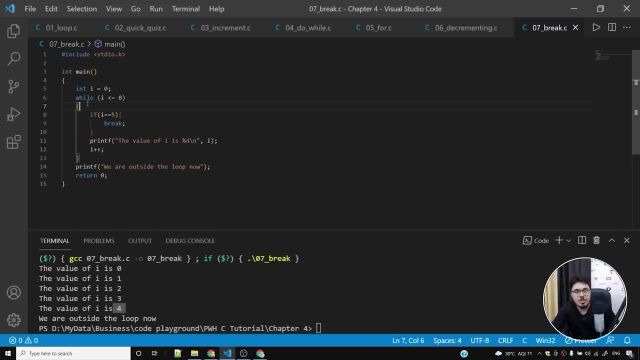 the while loop. This is how a while loop naturally terminates. But if I want to interfere into the natural termination of while loop and I want to terminate it based on some other condition, I can use break. So I can say: if the value of i is 5,, stop this while loop, I don't care about. 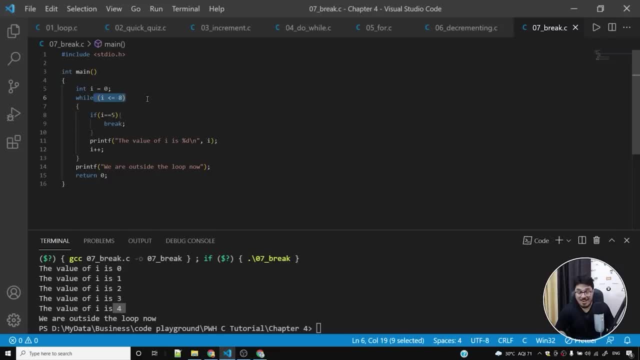 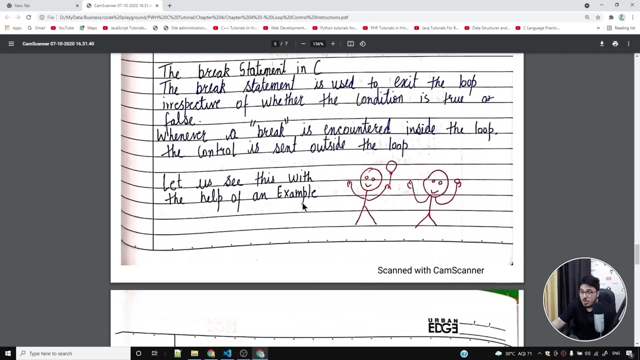 this condition: If the value of i is 5,, I want this while loop to be stopped. That's it, And this is what break statement is doing. So break statement is very easy. This way, you can understand it. Whenever a break is encountered inside the loop, the control is sent outside the 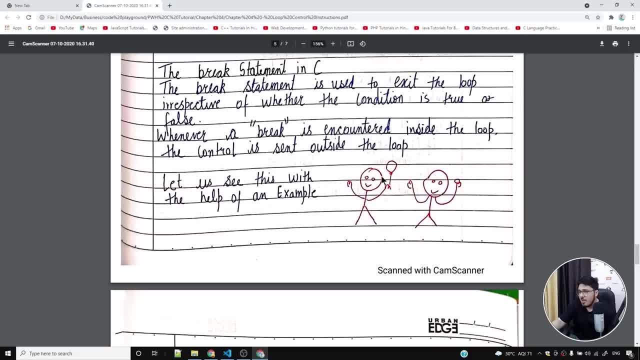 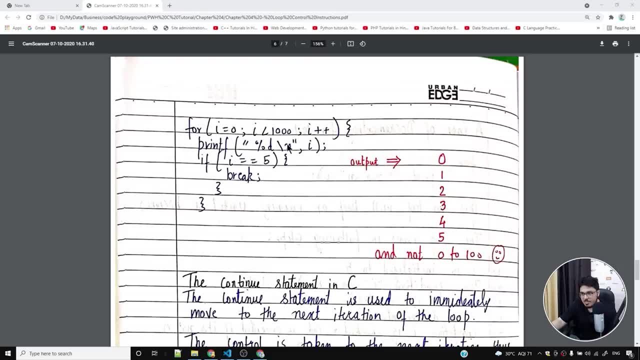 loop. Let's see this with the help of an example. How is my drawing? by the way, Just let me know in the comments if you like this drawing. Okay, for i is equal to 0,. i is less than 1000, i plus plus. 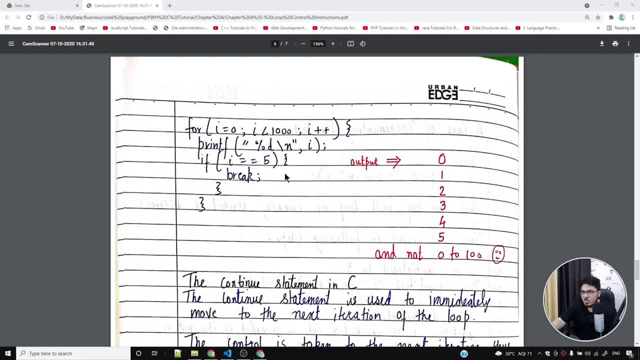 So here I'm saying: if the value of i is 5, you break. So what will happen is for the value of 0, this will be executed. this will be executed. So 0 is printed For the value of 1, this will. 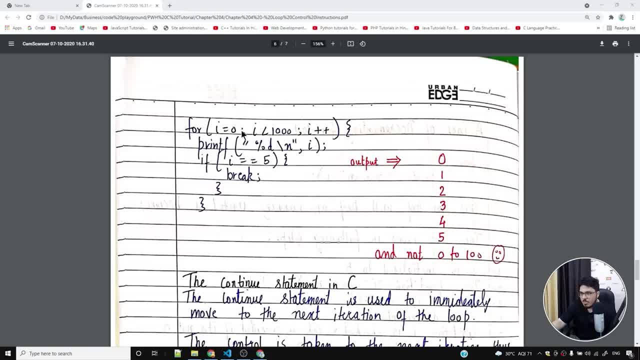 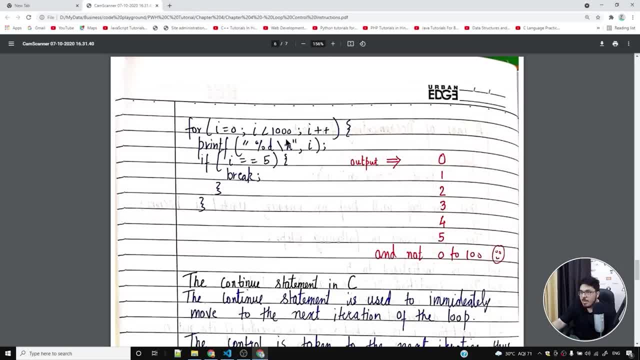 percentage deep acceleration. now, the moment five gets printed, what will happen is this: will evaluate to true. since this condition evaluates to true, we'll encounter a break statement. and since we are encountering a break statement, we will come out of the loop. okay, so this is how it. 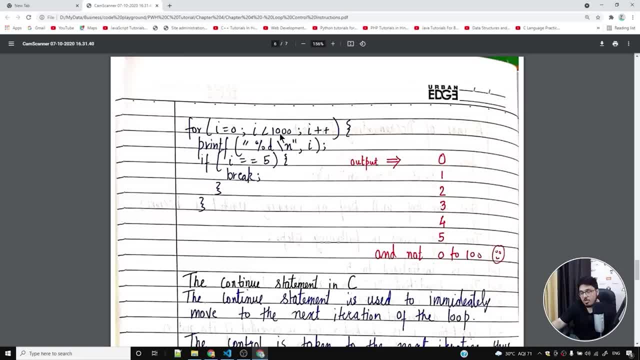 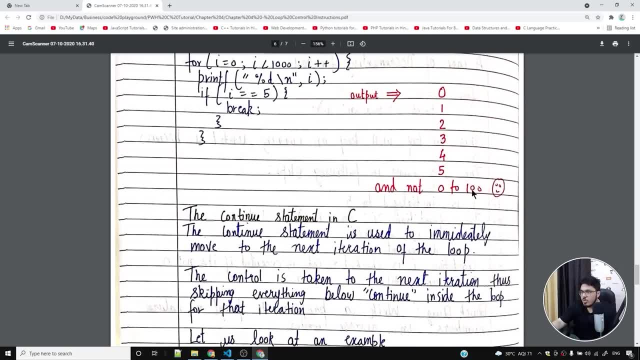 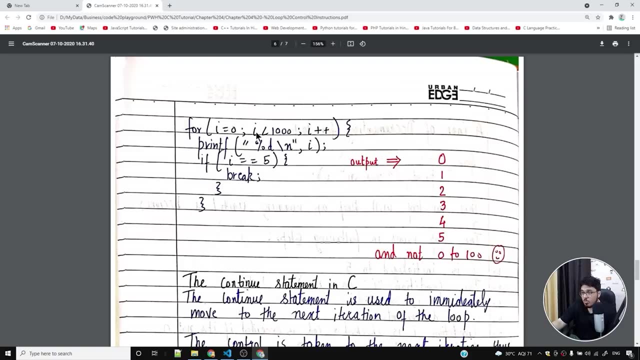 works and it will not go all the way till thousand or triple nine. it will not go till nine, nine, nine, it will go only till five. okay, so zero to triple nine will not be executed. so this is. this is something, uh, which is wrong. i should have written zero to nine, nine, nine, because naturally, this loop. 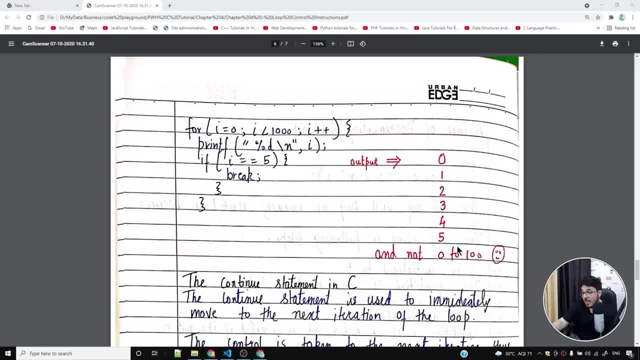 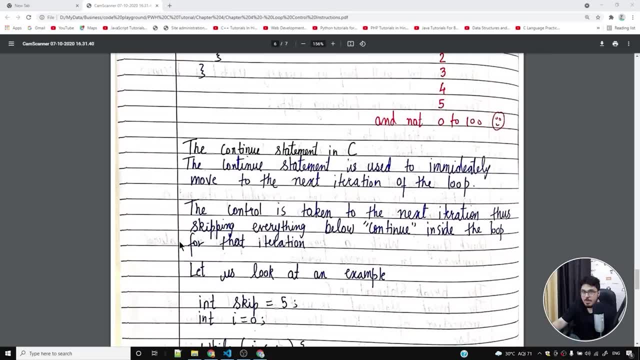 will go from zero to nine, nine, nine, so i should have written nine, nine, nine here, but i have mistakenly written hundred here, so my bad, um, anyways, you got the point. you got what break statement, and c is: let's talk about continue statement now. the continue statement is used to immediately move to the next iteration of 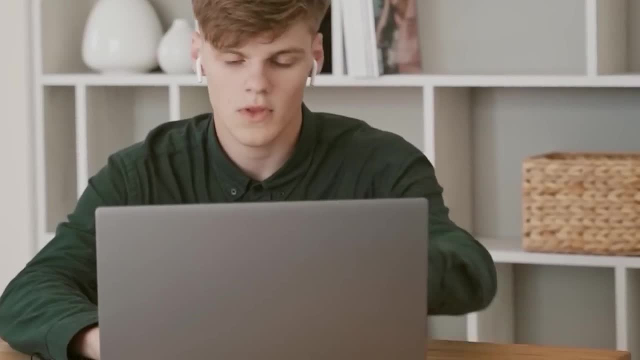 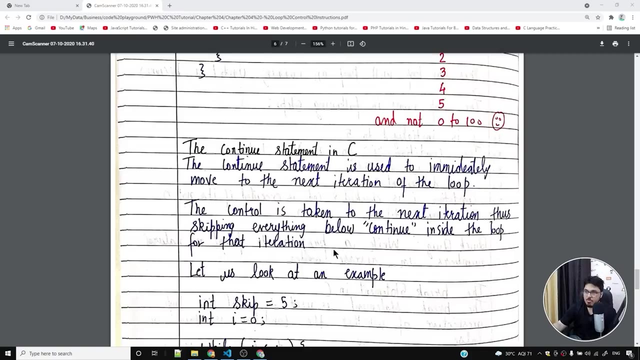 the loop and listen to me very, very carefully when i say this. a lot of people confuse between break and continue statements, but they are very different. okay, in the way that break statement will stop the loop forever, but continue statement will not stop the loop forever, rather what it will. 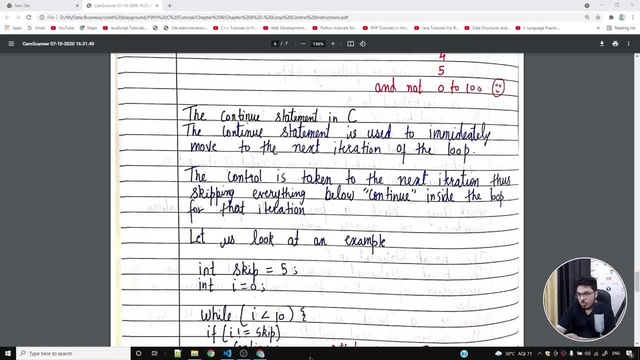 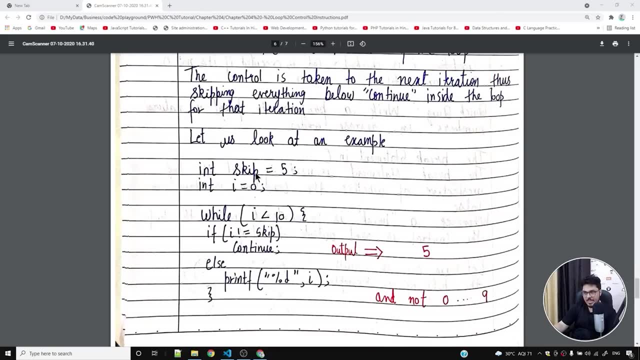 do is it will stop the loop just for this particular iteration. it will stop the current iteration of the loop and it will continue with the next iteration. let me tell you what continue statement means. so let us say we have a program: uh, int skip is equal to five, i is equal to zero, while i is less. 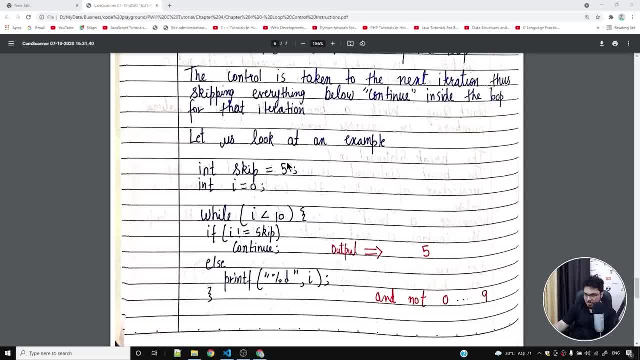 than 10 and i is not equal to skip. let us say we have this program. how will this program execute? i is less than 10. yes, it is zero is less than 10. if i is not equal to 5, continue, okay. so what will happen is this particular program will keep on executing the instructions inside the while loop. 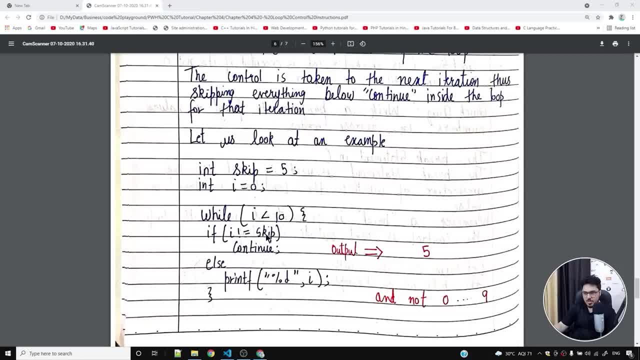 is i not equal to skip, for i is equal to zero. yes, this condition is true, so continue. continue means that do not execute anything after this, just continue with the next iteration. same goes for, same goes for three, four, but the moment i becomes 5, what will happen is: 5 is not equal to 5 is false. so this thing will be executed. let me 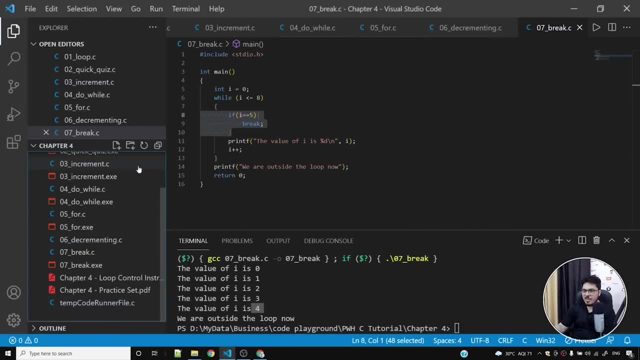 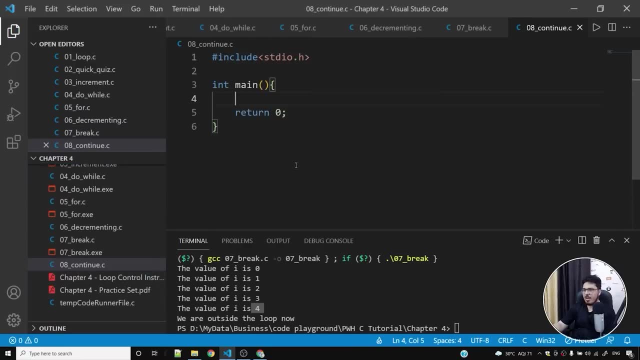 explain this to you by taking you to vs code, and let me write a program myself and explain this to you, and then you will understand this concept like anything. so i have put this boilerplate code for you. what i'll do is i'll simply put a very simple for loop here. let me save this program and now use. 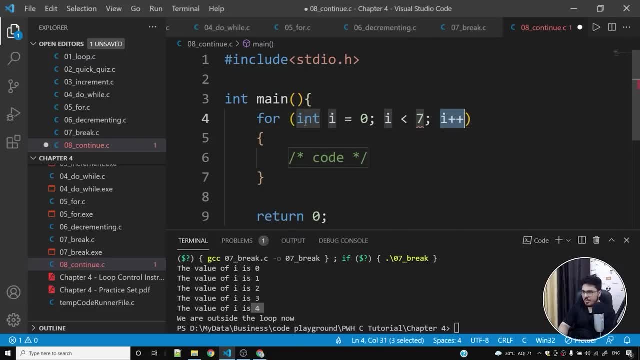 for: and yes, i got this snippet. now what i'll do is i'll simply say: for i is equal to 0, i is less than 7, i plus. plus means i'm going from 0 to 6. okay, now what i'll do is i'll simply say the value. 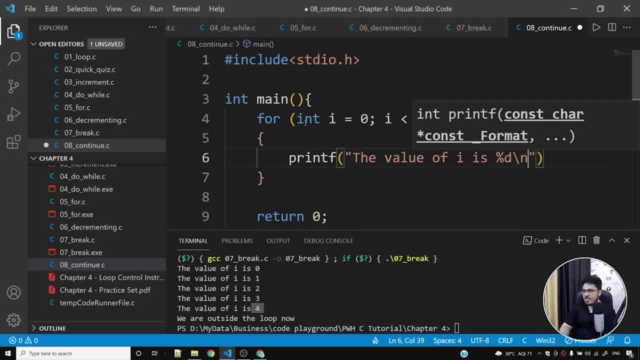 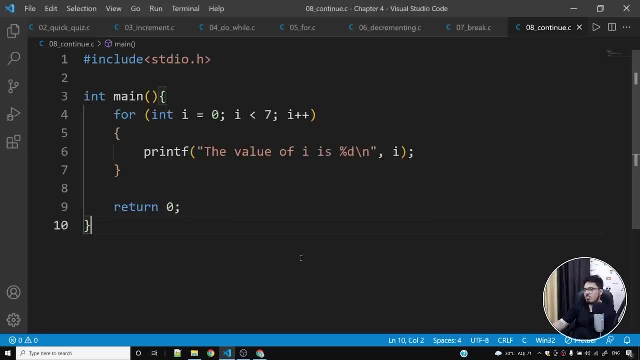 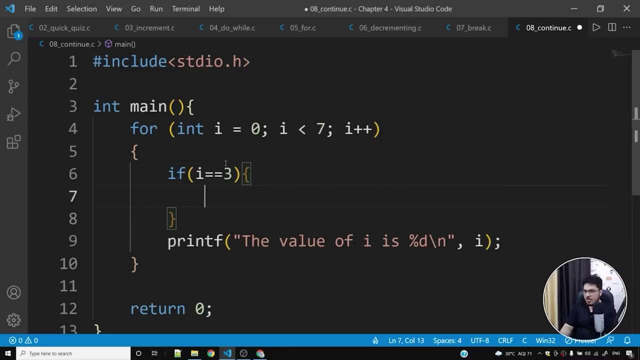 of i is, and i'll say percentage d backslash n, and then i okay. and once i do this, what will happen is i will be printed from 0 to 6- nothing fancy here: 0, 1, 0, 4, 5, 6. now what will happen is if i say: if, if i is equal to 3, continue. what does this mean? this means that 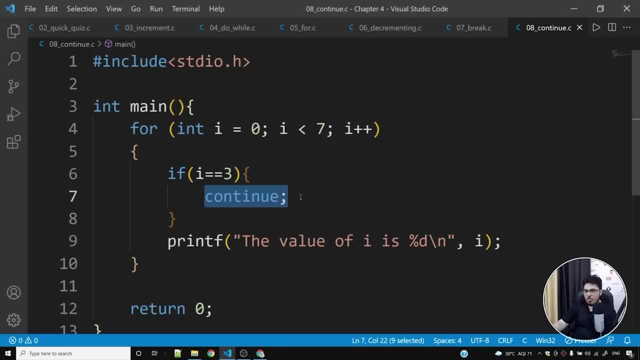 if i is equal to 3, we are going to continue. continue means that whatever is written below this inside the for loop we have to keep inside the for loop. we are inside the for loop, keeping the control inside the for loop. skip everything which is written inside the for loop and then. 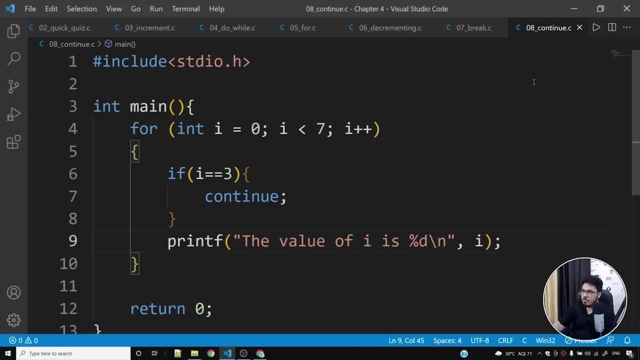 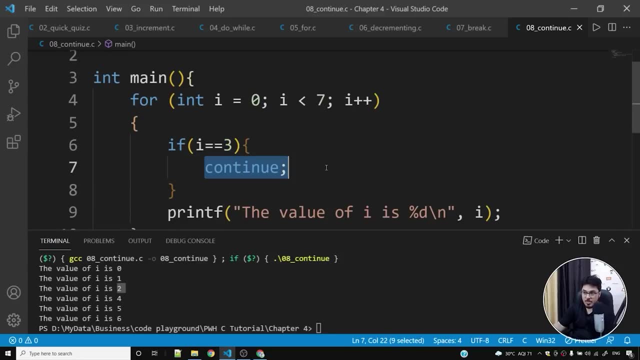 what i'll do is i'll just say from 0 to 6. if i want to continue, it will change right now. if i have a loop to be continued, i'll say from 0 to x is below continue. so this statement will not be executed. let me show you so if i run this program: 0 is printed. 1 is printed. 2 is printed. 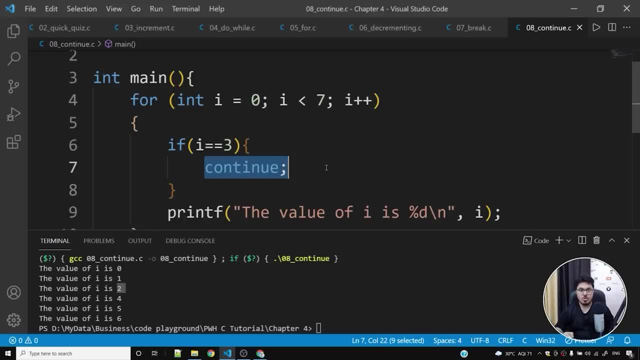 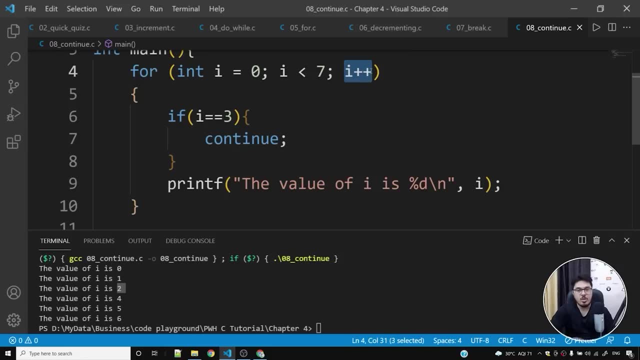 but the moment i becomes 3, continue means stop. no, don't stop the loop, just stop. stop this current iteration. do not continue from here on. rather, you go directly here and update the value of i and continue like you are continuing. okay. so what continue means is: do not execute anything, stay in the loop until i is equal to 0. 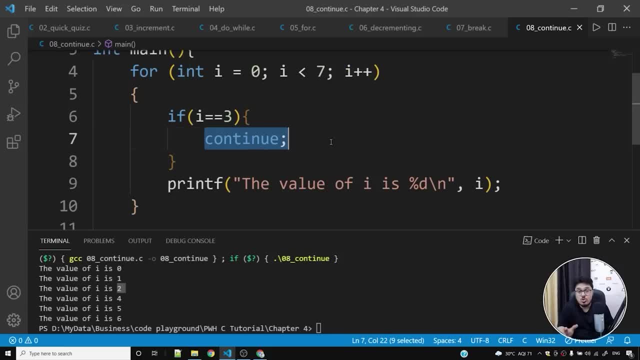 below me, but at the same time also do not stop the loop. i hope you got the point. so this is all about continue statement, and how is continue different from break statement? break statement simply says that just stop this loop. whatever be the case, stop this loop. we don't want to deal with. 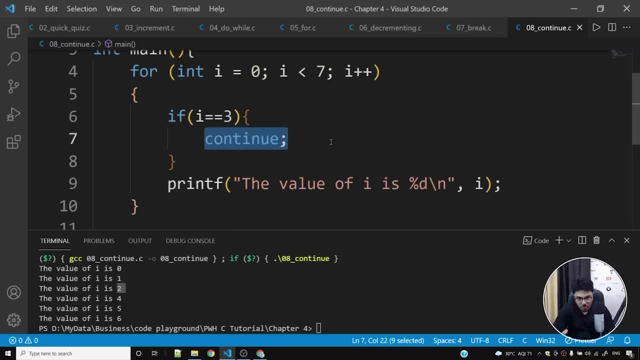 this loop anymore. continue means we want to deal with this loop, but we want to skip whatever we were doing in the current iteration. so we were about to print this, but no, we are not going to do that. the moment c compiler sees continue, what it will do is it will go directly here and update. 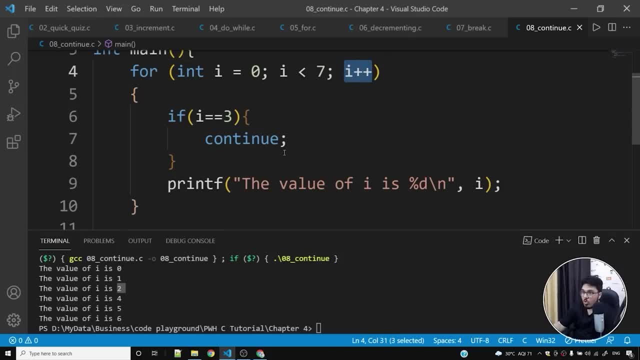 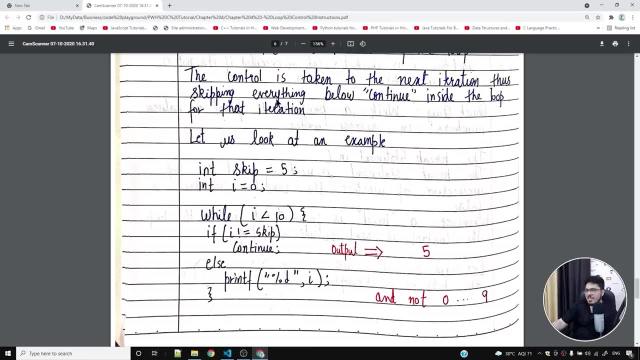 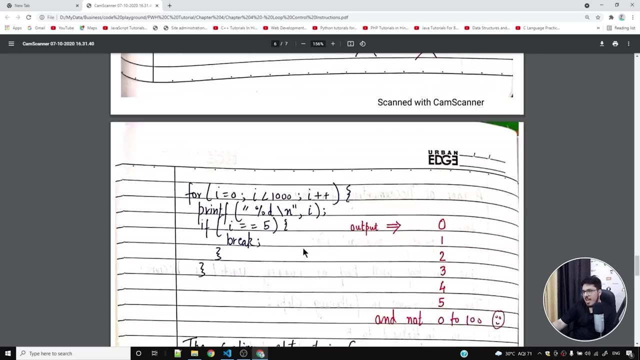 the condition and start executing the loop and if it encounters continue once again, it will again do this and it will keep on doing that. okay, so i hope you got this point and this is all you know i am trying to explain here. i have written all these things in the notes so you can have a read and 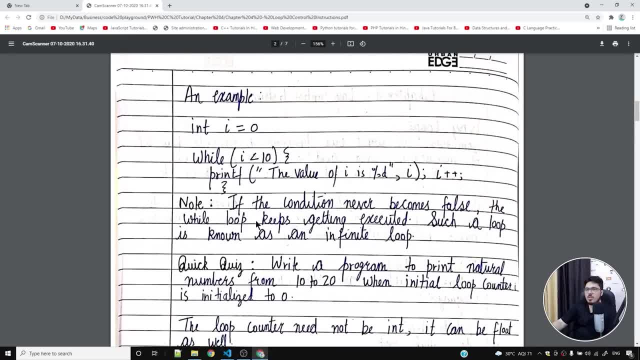 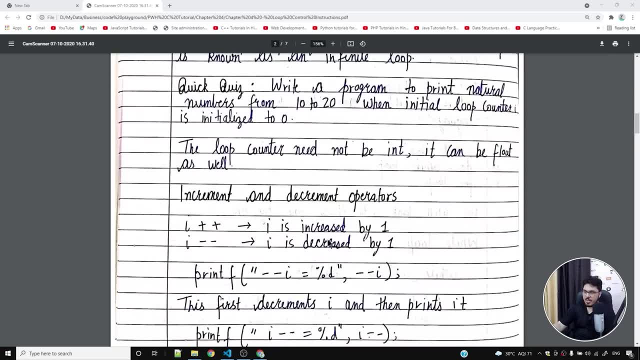 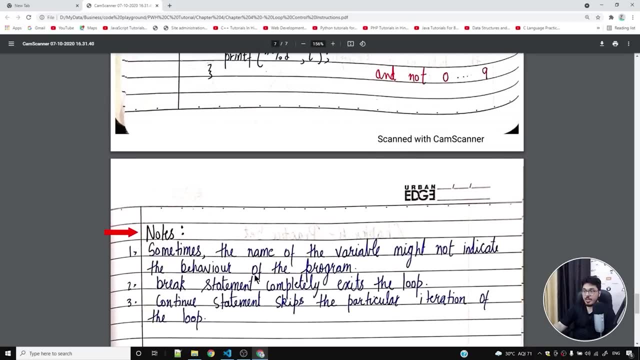 i hope that this chapter 4 notes will definitely help you and i hope this chapter 4 loop control instruction notes will definitely help you. let's let's see these notes which i have written for you. sometimes the name of the variable might not indicate the behavior of the program and you'll. 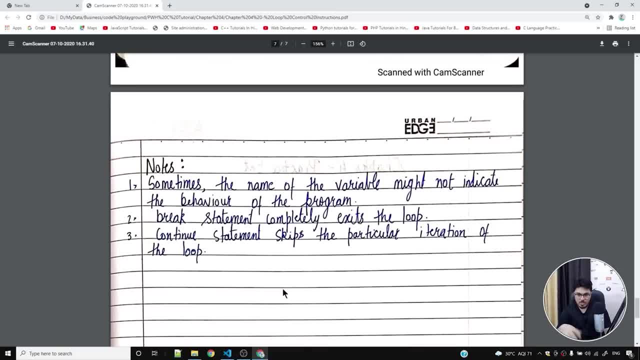 see this a lot. okay, sometimes they'll use index inside the loop, but that particular thing will not be the index. sometimes they will say integer variable, but actually it will be the float variable. so they'll do all these things to confuse you for the interviews. okay, you have to. 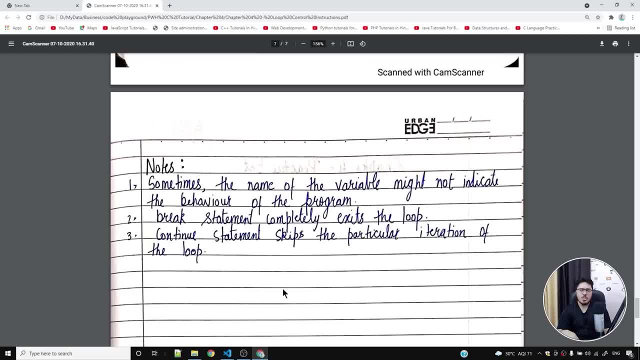 see what kind of variable it is. so if i say int integer variable is equal to 3, the value of integer variable is 3. but if i say float integer underscore value is equal to 3.1, it doesn't mean that it is going to be an integer variable. integer variable is the name of the variable, but actually it is. 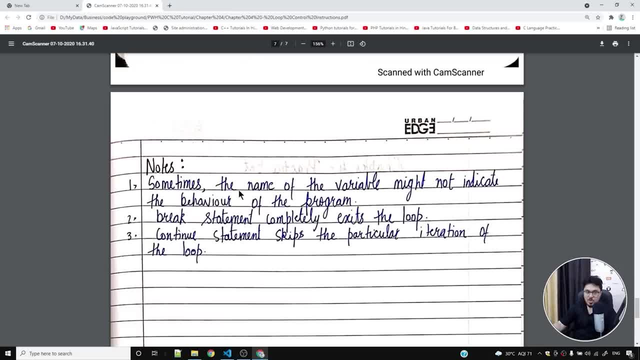 float, so sometimes people will try to confuse you. this way, you don't have to get confused. okay break. statement completely exits the loop. we have seen this. and continue. statement skips the particular iteration of the loop. the current iteration will be skipped. that's it. i hope you got the point. i hope these notes were useful. let's now. 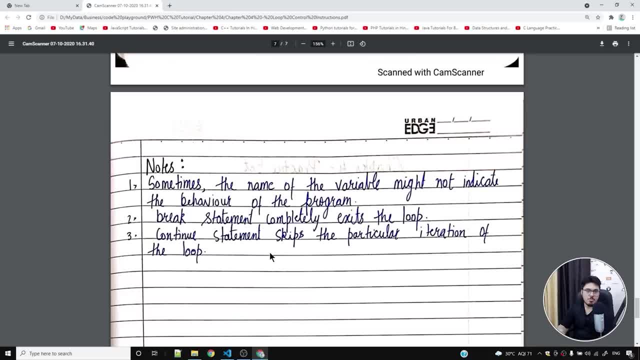 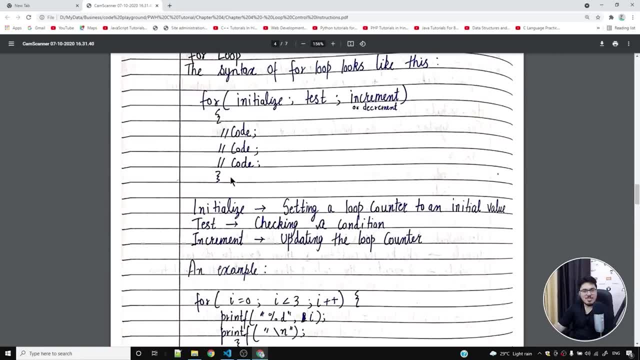 move on to chapter 4 practice set and solve some more problems and definitely we'll learn these concepts better there. let's move on to chapter 4 practice set now. so here is chapter number 4 practice set which i have prepared for you. let me open this practice set and after i 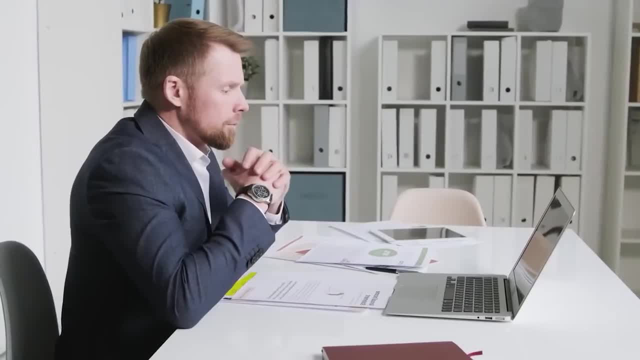 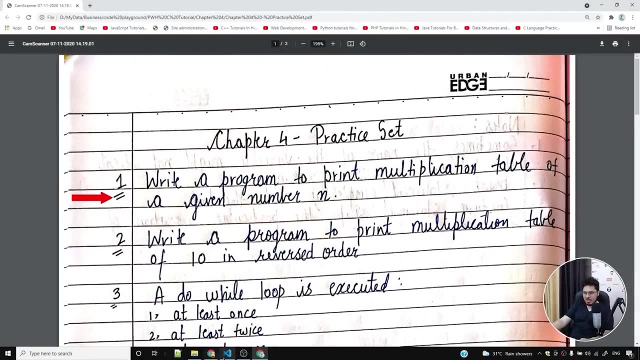 open this practice set. we'll solve some problems and definitely we'll learn some more problems. you will get a good hang of the concepts which we have learned in this chapter. so the first program says that write a program to print multiplication table of a given number, n. and yes, i have a choice. 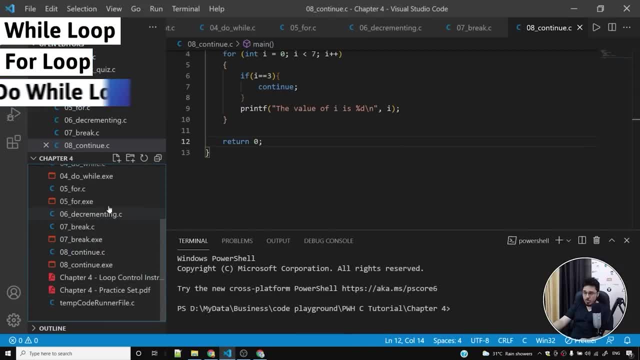 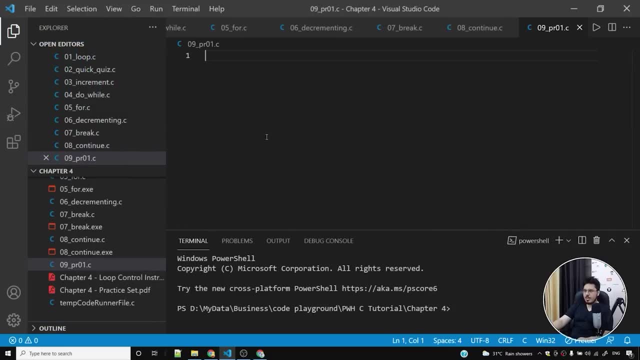 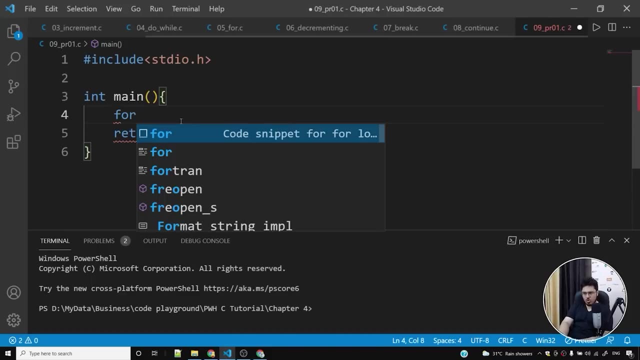 i can either use while loop, i can use for loop and i can also use do while loop, but i'll smartly use the loop that solves this problem in the easiest way for me. let me put the boilerplate codes index here, and i prefer to use for loops in most of the cases. but if you want to do it with while, 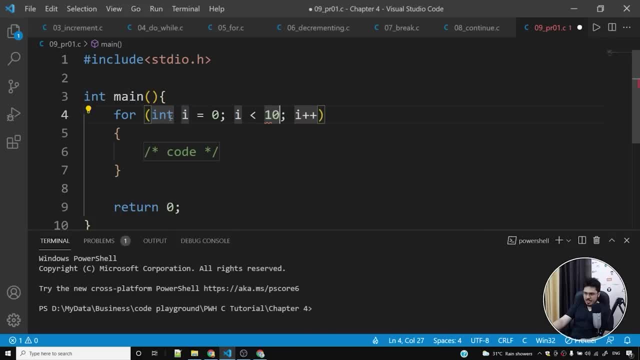 loop. you can definitely do it. so what i'll do is i'll simply say: int i is equal to 0, i less than 10, i plus plus. i'll press the tab key and what i'll do is i'll simply say: percentage d x percentage d. 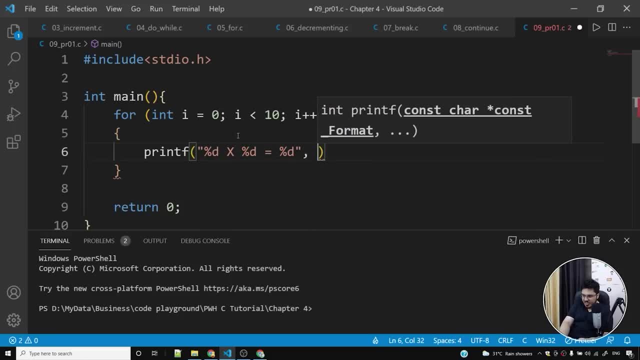 is equal to percentage d, and i'll put three integers here. first will be n, the number whose multiplication table i want to print. second is going to be the index i and third one is going to be the value n multiplied by n, and the second one is going to be the index i and the third one. 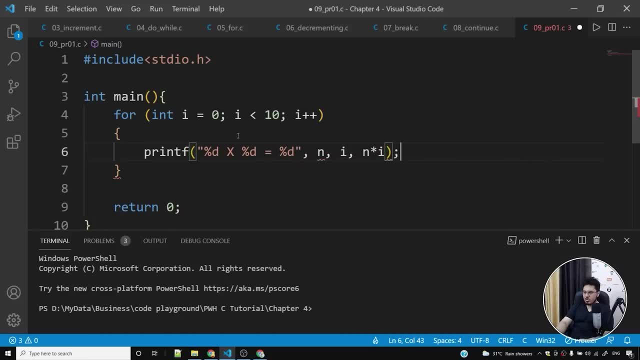 is going to be the value n multiplied by i, so n multiplied by i, and also the semicolon. and what i will do here is i'll say int. n is equal to say three, so i want to use the value three in place of n. so i'll also do one more thing. i'll simply say backslash n, so that you know whenever i'm 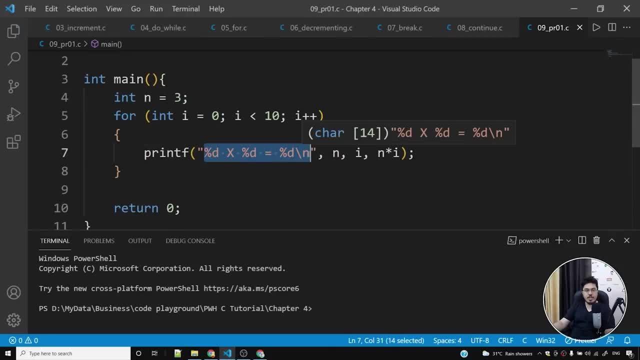 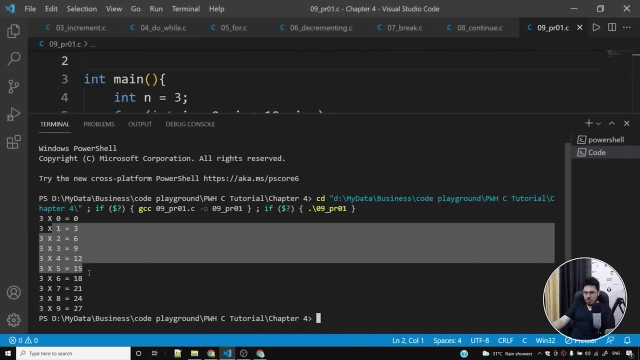 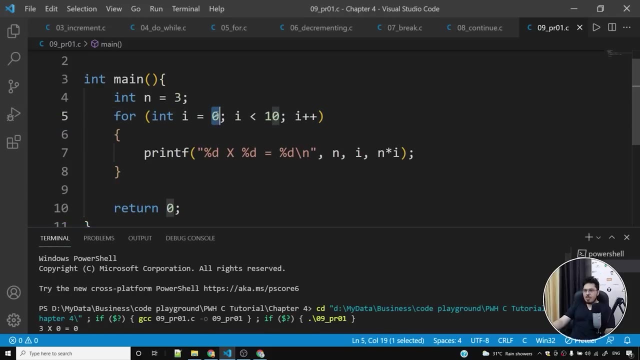 i'm printing one line. i want a new line right after that. so if i run this program you'll see something like this: three multiplied by zero all the way till three multiplied by nine. but i don't want my i to start from zero all the way till nine. i want to start my i from one and i want it to go from one all the way. 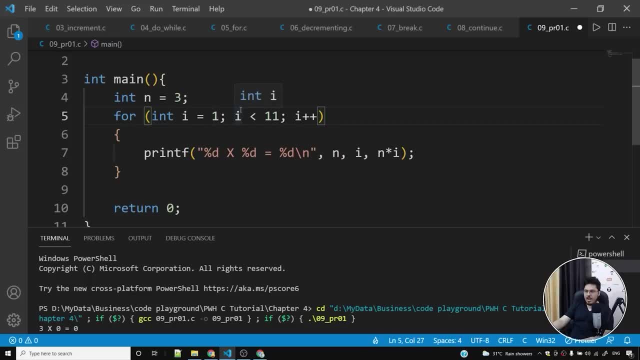 till n. so what i'll do is i'll start my i from one and i'll make it i less than 11.. what this is going to do is it will start i from 1 and it will take the value of i from 1 to 10 because i less than 11. 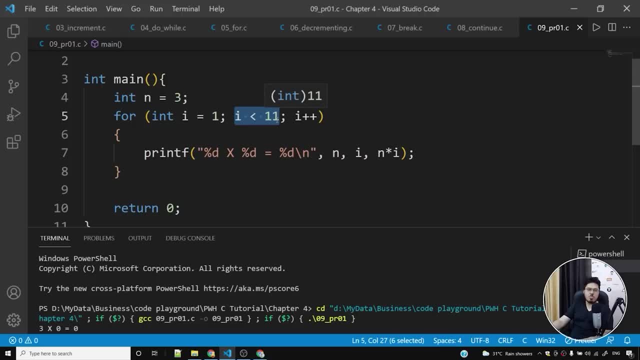 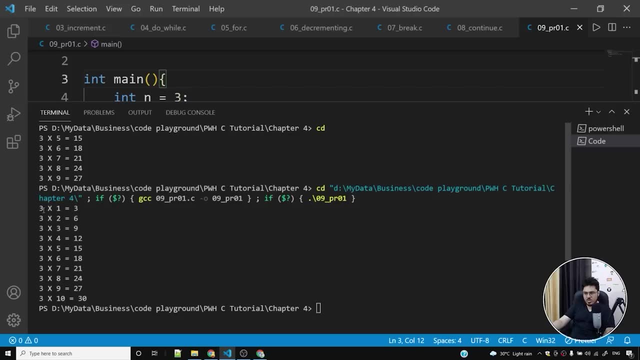 for the value of 11, this condition is going to be false. for the value of 10, it is going to be true. so let's run and let's see if we were able to achieve what we want to achieve here. three: multiply by one, multiply by two. three: 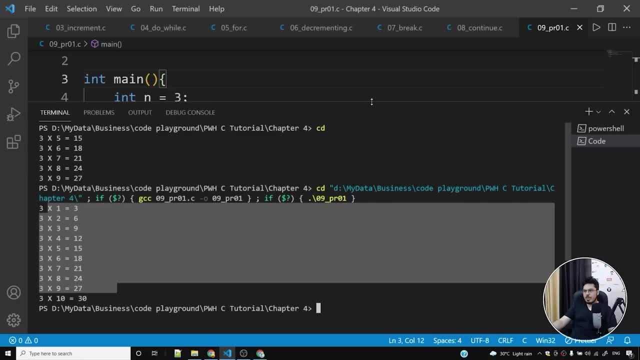 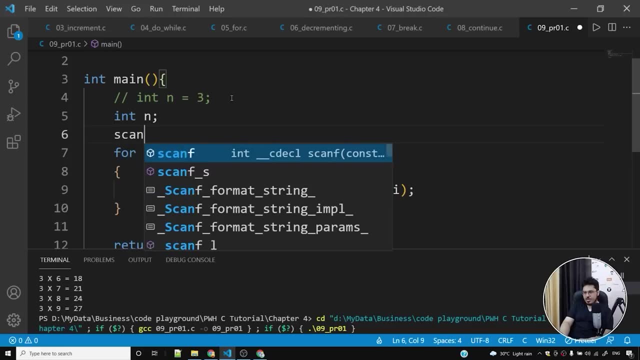 four, five, six, seven, eight, nine, and yes, we were able to print the multiplication table of a given number. in case you want to take the user input, what you do is you simply do something like this: int, n, and then you can use scanf, you can use percentage d and you can use ampersand n and 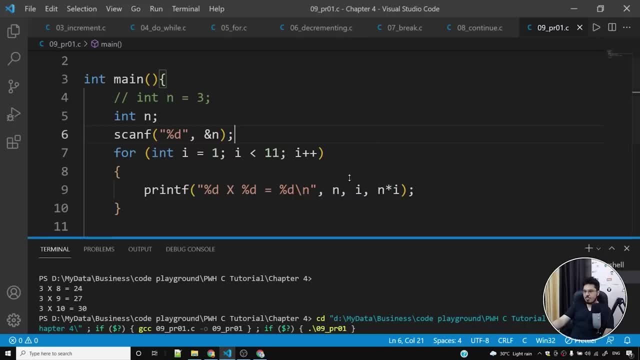 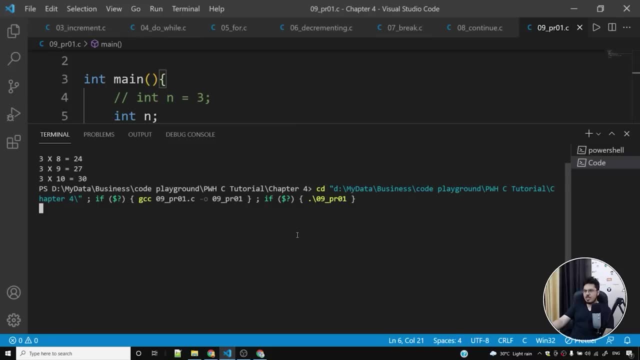 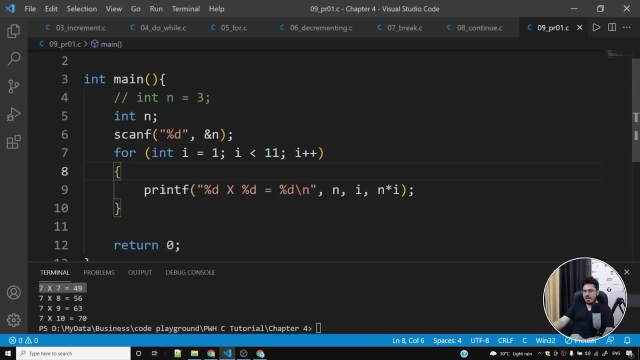 the moment you do this and run this program, let me show you something. i'll wait for this program to run, okay, so it's waiting for my input. the moment i press 7, i get the multiplication table of 7.. i can also say something like this, just so that user can know that: 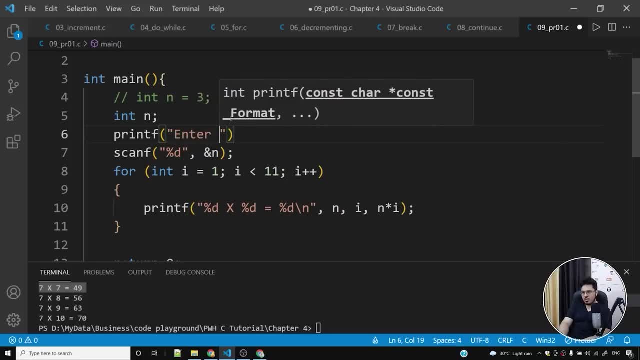 he needs to enter a value for this program to continue. enter the value of n, backslash n. if i run this program, i'm getting this prompt: enter the value of n. the moment i say 4, i'll press enter and you'll see something like this: 4 multiply by 1, 2, 3, 4, 5, 6, 7, 8, 9 and finally, 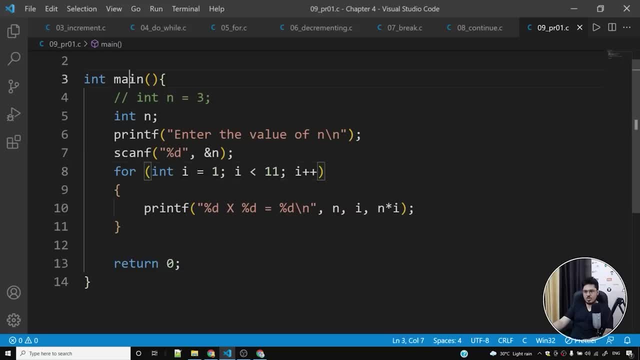 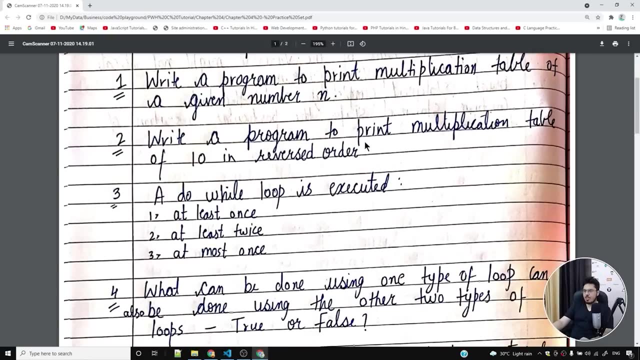 10.. i hope that you were able to understand how this works. i hope that you were able to get a hang of this thing. we'll now move on to the next question, and it is really very interesting because it says: write a program to print multiple. 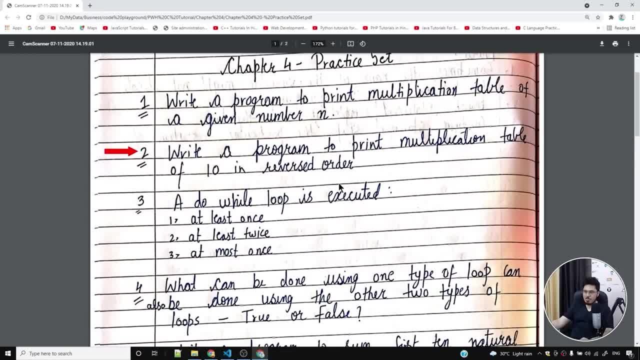 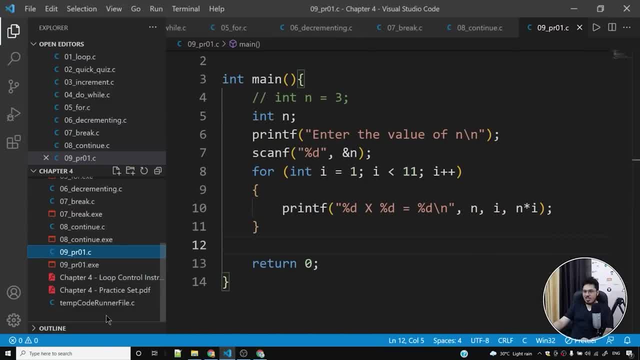 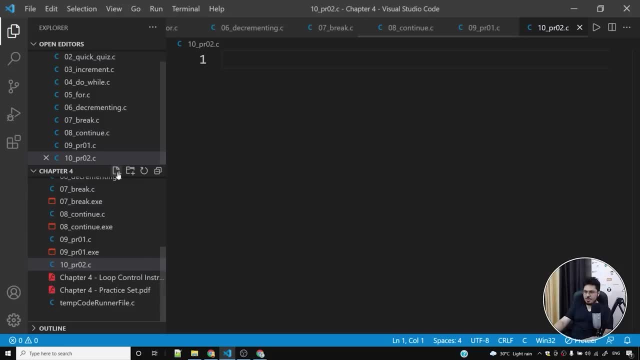 table of 10 in reverse order. so we have a multiplication table and we want to print it in reverse order. so we are going to use the same program but in a twisted fashion. what i'll do is i'll say 10 underscore and pr02.c. i'll press enter, i'll put. 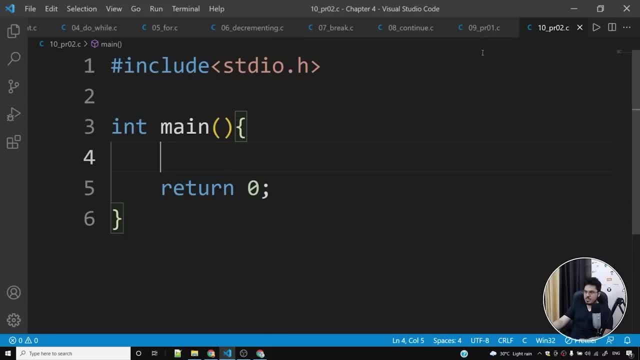 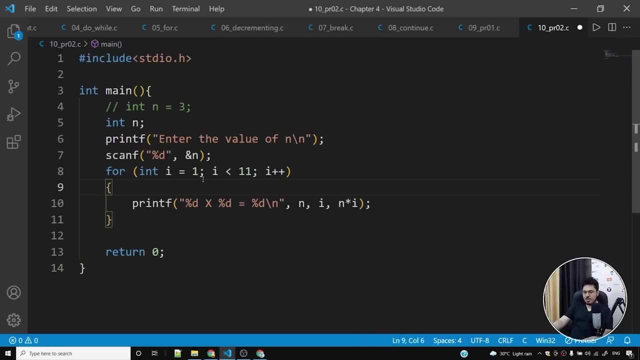 the boilerplate code, then what i'll do is i'll- or rather, what i'll do is i'll simply copy the previous program and i'll paste it here. so i'll copy the previous program and i'll paste it here. once i do this, i have a value, and the value is 10, if i'm not wrong. i'll get rid of this scan f and all. 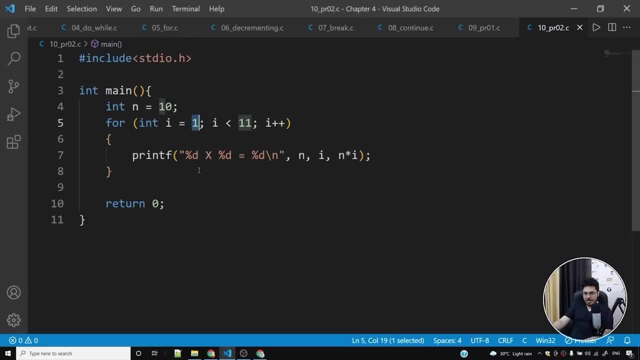 cancel, i'll save this program. i want to start my i from 11 and i want it to go all the way till one. okay, so i'll reverse this condition. why am i reversing this condition? i'll tell you and i'll make it i minus, minus. so i'm starting my i from 10, not 11, and also i'll say i greater than 0. 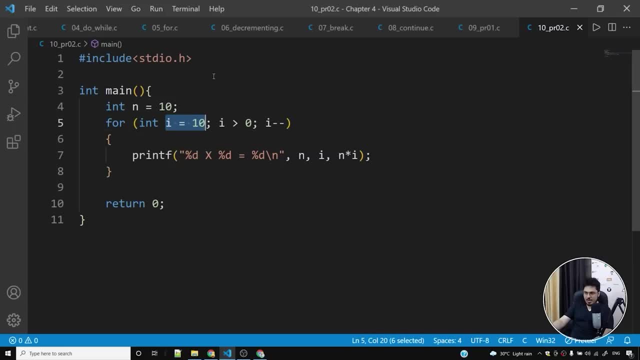 why did i do that? i want my i to start from 10 and after decrementing it will become 9 and then it will become 8, then 7, 6, 5, 4, 3, 2, 1. the moment it becomes 0, 0 is not greater than 0, so it will. 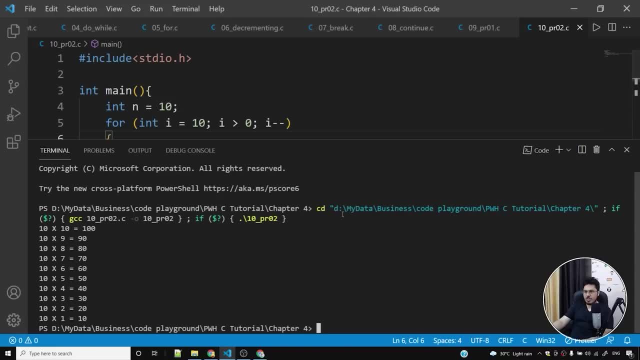 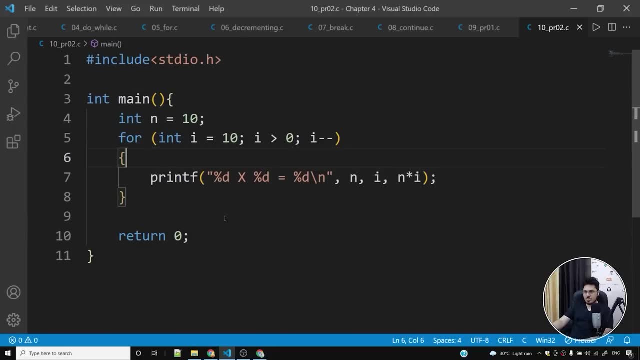 start from 10 and go all the way till 1. so if i run this program you can see the multiplication table has been printed in reverse order. let me explain you how this works, because this is something that you need to understand, although i have already explained you this thing in chapter. 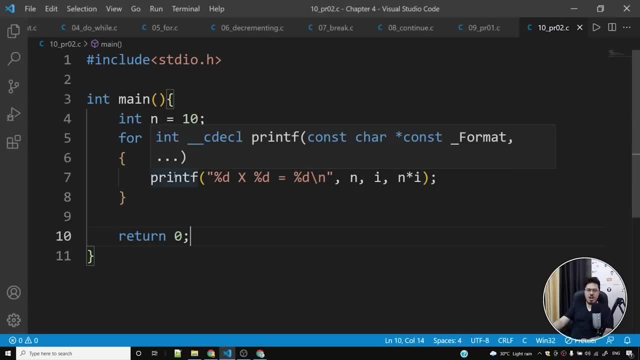 number 4, but i'm going to explain it once again just so that you have a good hang of it. so what we are doing here is we are starting a value of i from 10. then what we are doing is we are simply running this, for i is equal to 10, because this condition is true. so initially, what happens is: 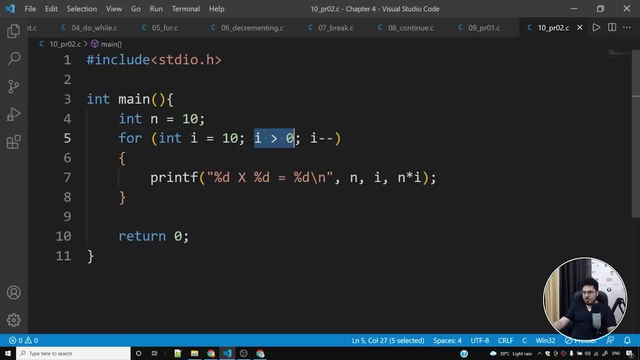 i is initialized to 10. then this condition is checked: is i greater than 0? yes, indeed, it's greater than 0. now what happens is this: gets printed. now what happens is this printed: particular update condition is ran. now the value of i becomes 9. after this, what happens is this: 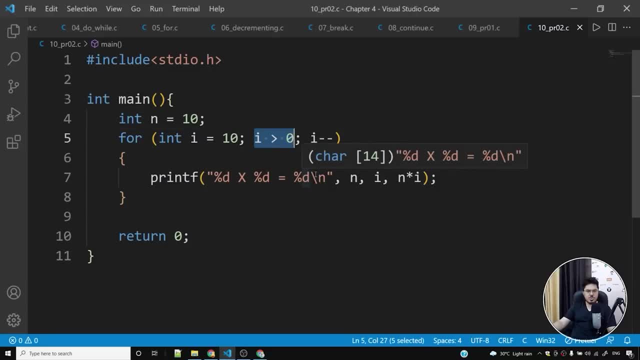 condition is checked for the value 9. is it true? yes, it is true. this will run. now i becomes 8, because i minus minus makes the value of i change from 9 to 8, because i minus minus will reduce the value of i by 1. okay, i hope you are understanding how these things work, and this keeps on going. 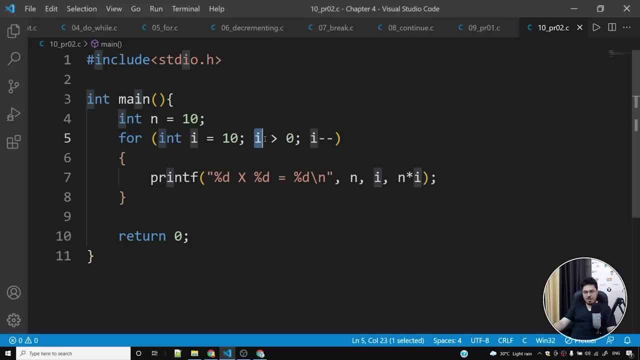 until the value of i becomes 0 and the moment value of i becomes 0. 0 greater than 0 is false and this will not run, for the value of i is equal to 0. so if i run this program, the value of i starts from 10 and it will go all. 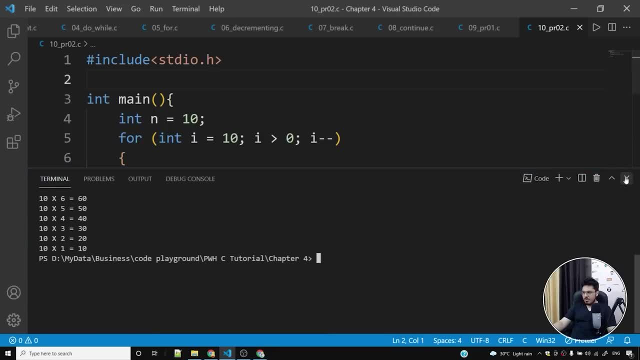 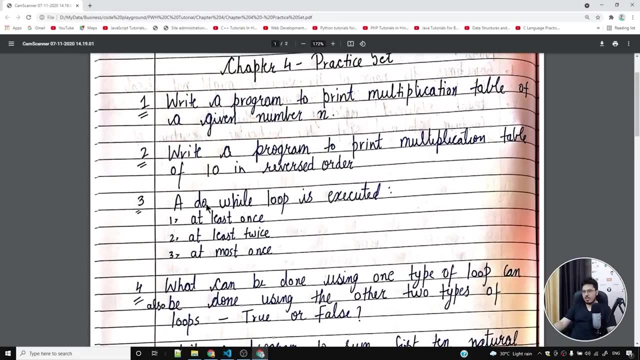 the way till 1. it will not become 0, okay, so i hope you understood this now. what we'll do is we'll move on to the next question, problem number 3 a: do by loop is executed. there are three options, and i need to choose one of these three options. 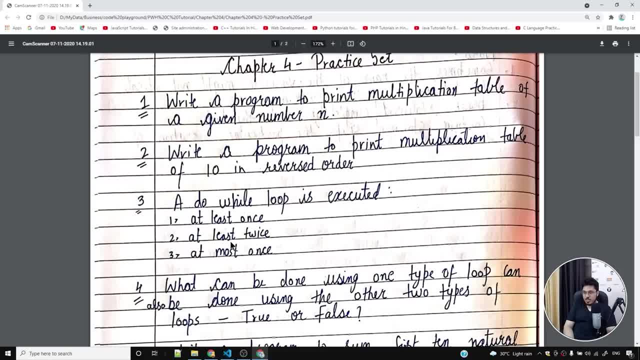 is it executed at least once? is it executed at least twice or at most once? and i want you guys to comment down below with the timestamp of the video, telling me what the correct answer is. i want answer from each and every one of you. i'll wait for you to comment. i hope everybody commented. 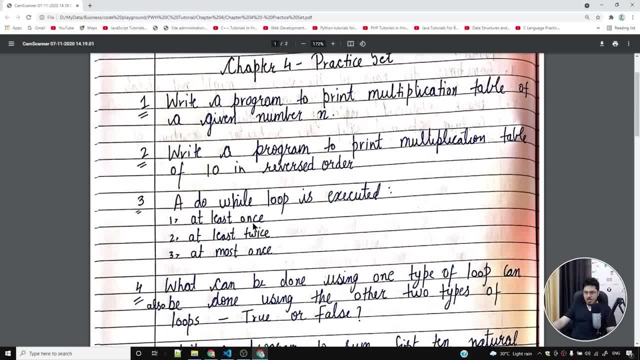 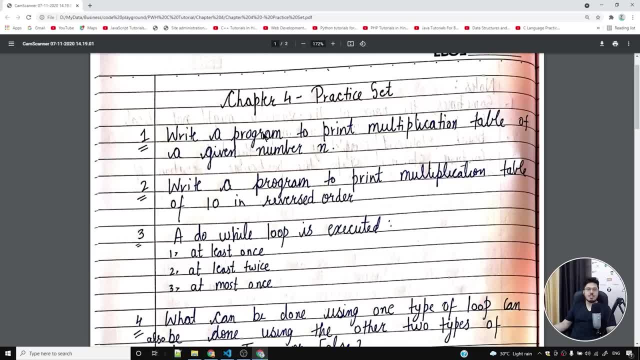 now let me tell you the answer. it's at least once. and why? why does it execute at least once? because in do by loop, we first run the loop body and then we arrive at the condition, and if the condition is true, we run that code inside the do block again and we keep on doing. 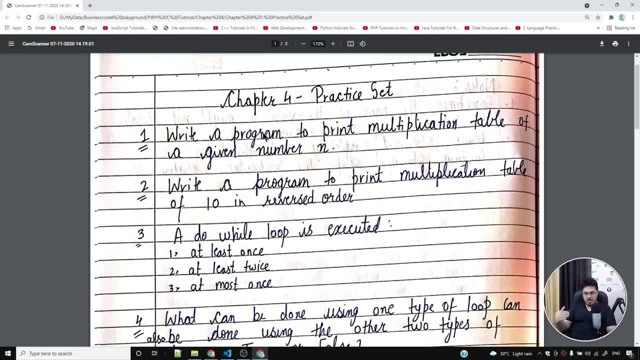 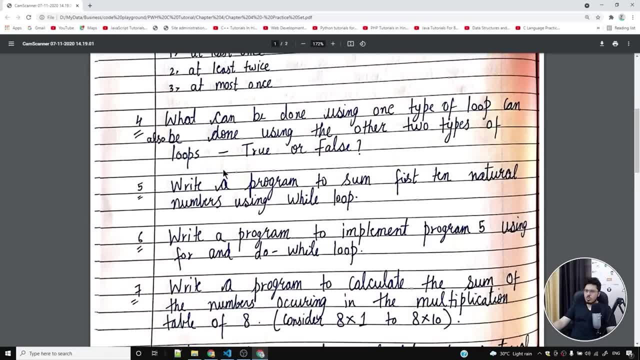 that until the condition is true. so initially it will execute, no matter what the condition is. so it is executed at least once. okay, moving on to the next question: what can be done using one type of loop can also be done using the other types of loops. is it true or is it false? it is indeed true. 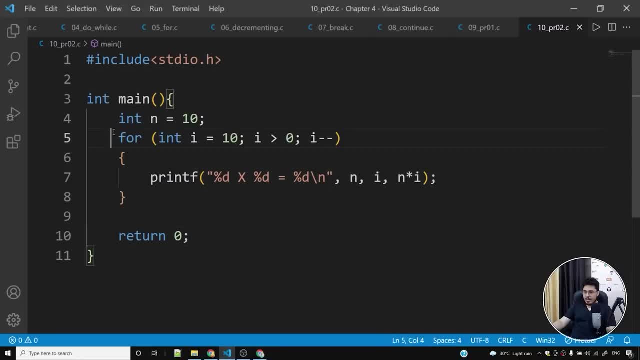 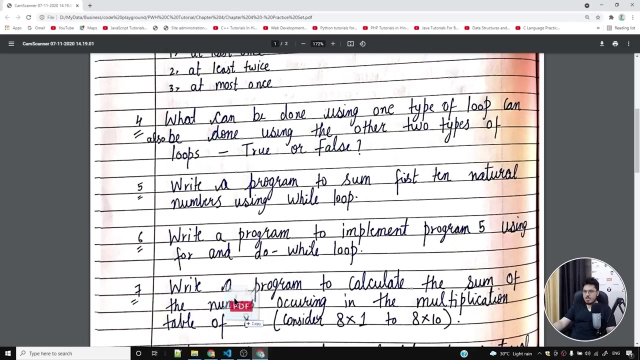 because we have already talked about it. this same thing can be done using a while loop, because i can always write this outside my while loop. i can put this condition inside the condition body of the while loop. let me show you where, let me open these nodes and explain you what i mean when i say that. 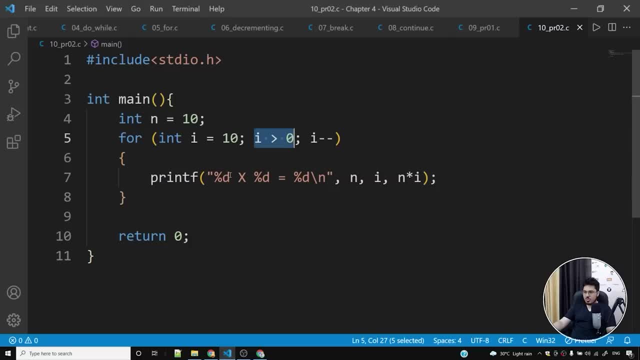 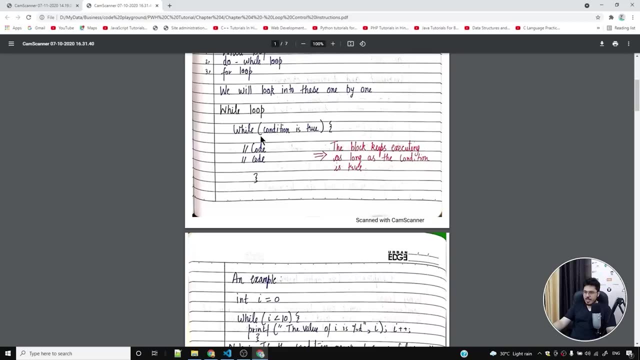 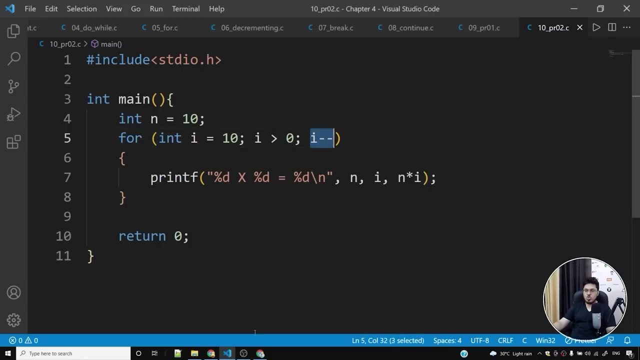 so, while i can put the condition, this for loop condition, inside the while loop, here inside the condition, and what i'll do is whatever is inside the for loop, i'll write inside the body of the while loop and even the update code. i can take this update code and i can actually write it after i have written the body. 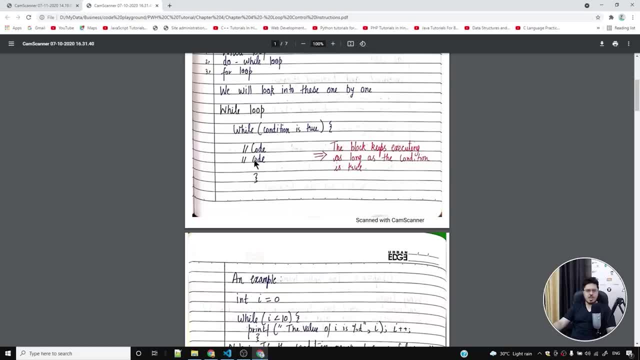 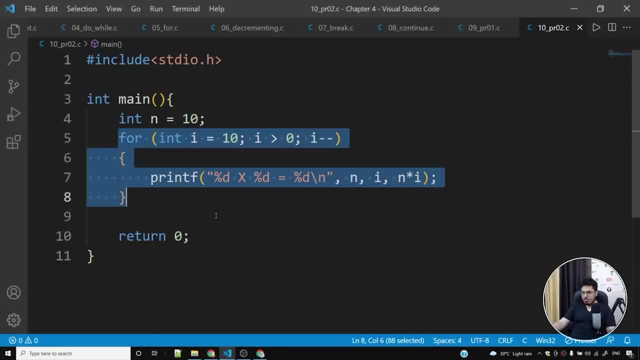 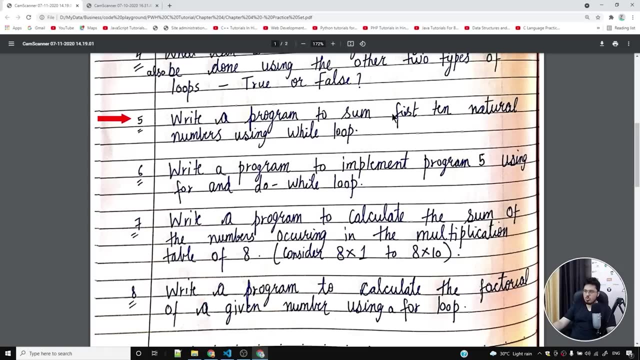 of my while loop. i hope that you were able to understand this. i hope i explained it pretty well to you and you can definitely do whatever you want to do with one type of loop, with other type of loop. okay, so this is true. okay, moving on to the next question: write a program to some first. 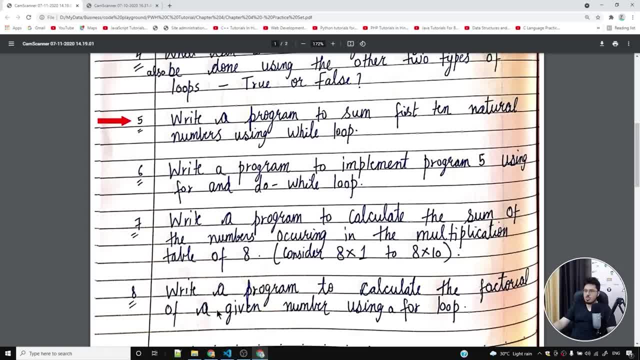 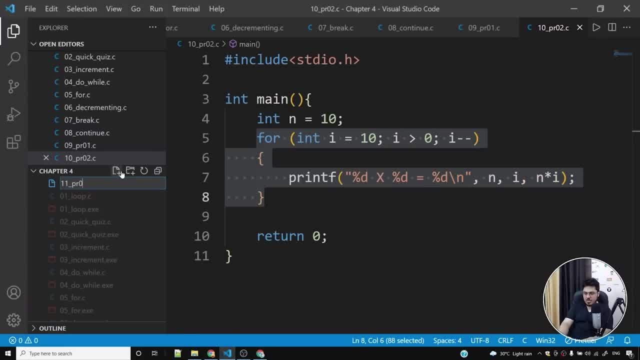 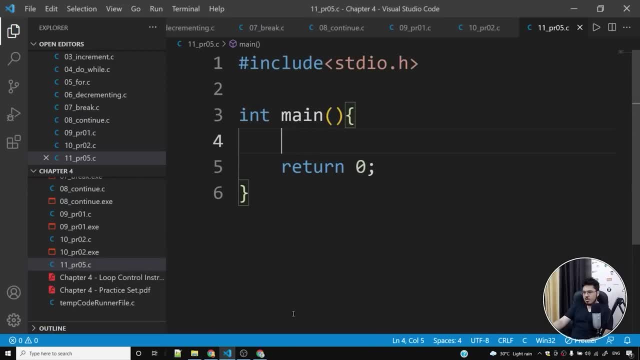 term natural numbers using while loop. let's solve this problem. so i'll say problem 5. so i'll simply say 11, underscore pr05, dot c. i'll put the boilerplate code and what i will do is i have to print sum of 10, first 10 natural numbers. so i'll start the value of i from 1. i'll say while i is less than. 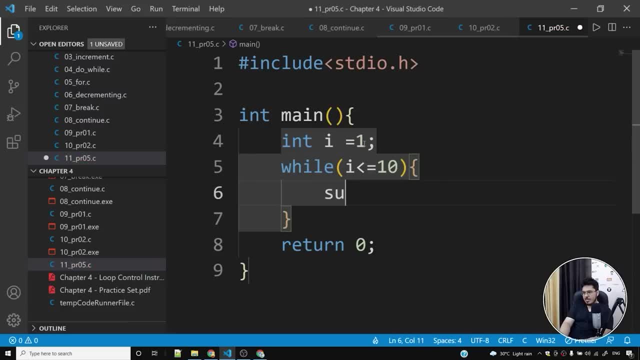 or equal to 10, and what i'll do is i'll put the boilerplate code and i'll put the boilerplate code and what i'll do is i'll simply say: sum plus equals to what? sum plus equals to i, i plus plus. and let me explain you what i've done. do i remember all these programs? no, i don't. i don't remember all. 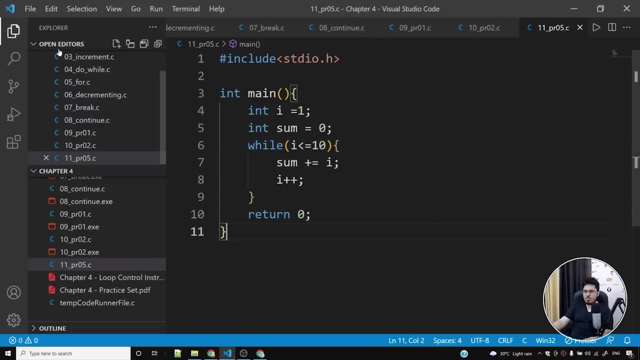 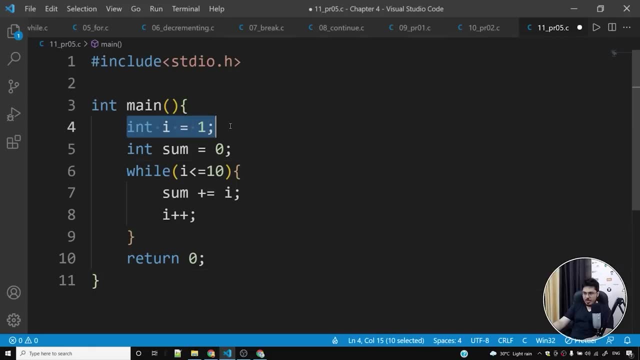 these programs. then what is happening? how am i able to write this program so fast? it's all about practice, but let me explain you how i wrote this program. i started i with 1, and what i'm doing is i'm taking this i from 1 all the way till 10, so this condition will be true for the value of i. 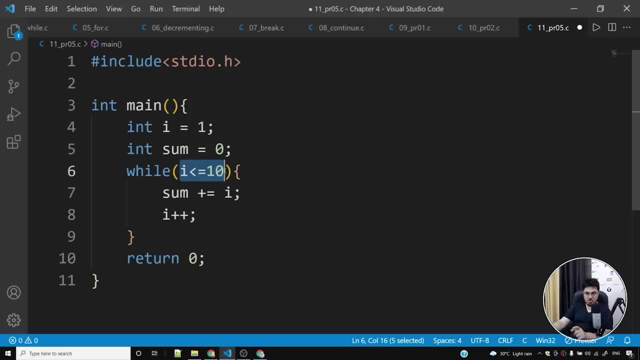 ranging from 1 to 10, and the moment i becomes 11, this condition will be false. okay, so i'm updating the value of sum, i'm keeping on updating this value until the value of i becomes 10 and finally, when it becomes 11, the loop body will not run. and finally, if i write a printf statement, i'll say: 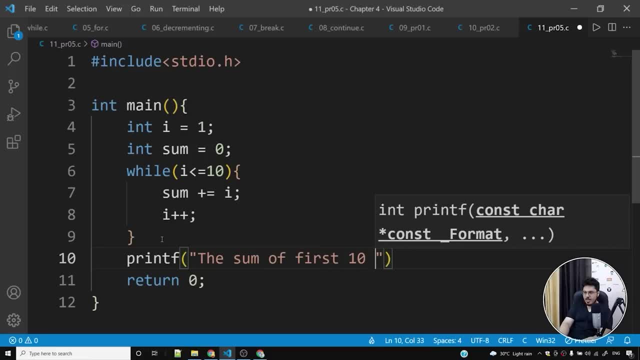 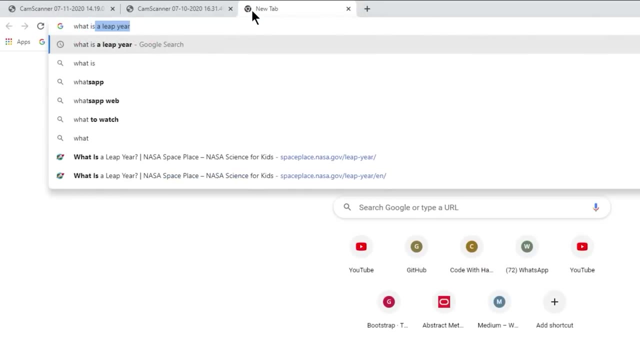 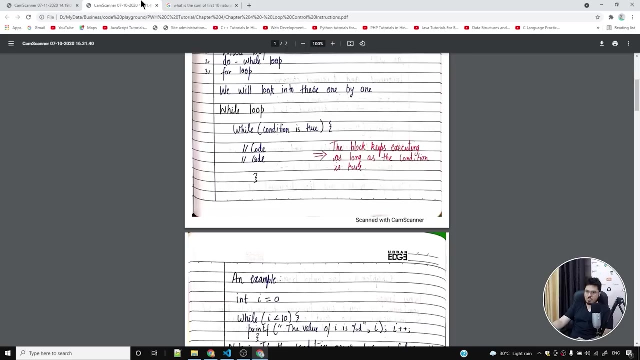 the sum of first 10 natural numbers is percentage t and i'll simply print sum and if i run this program, you'll see the value is 55. let me google this. what is the sum of first 10 natural numbers? it's 55. yes, it's 55. so i was able to find out the value of first. 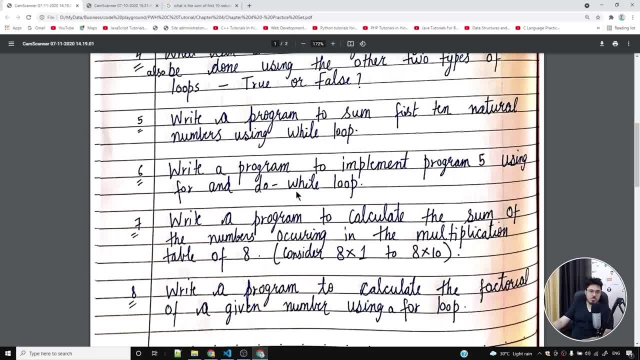 value of the sum of first 10 natural numbers, and it was 55. great. write a program to implement program 5 using for loop and a do by loop. can you do this? can you implement the same thing in question number 5, which i implemented using a y loop? can you do the same? 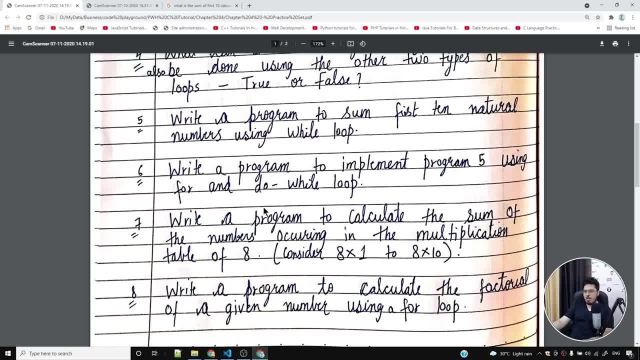 thing using for and do i loop. i want you to give it a go. i want you to give it a go because it will be very satisfying for you to solve the same problem using a for loop and using a do by loop. do give it a try and in case you are not able to solve it, definitely you'll be able to solve it. 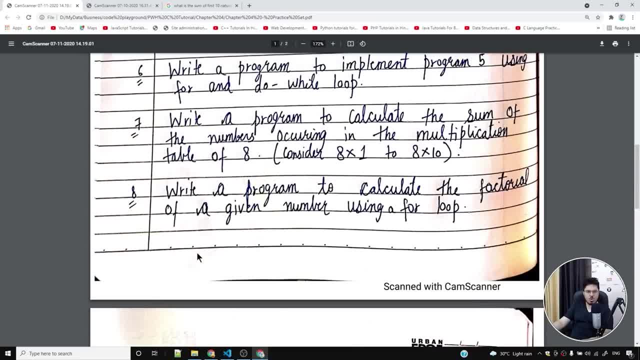 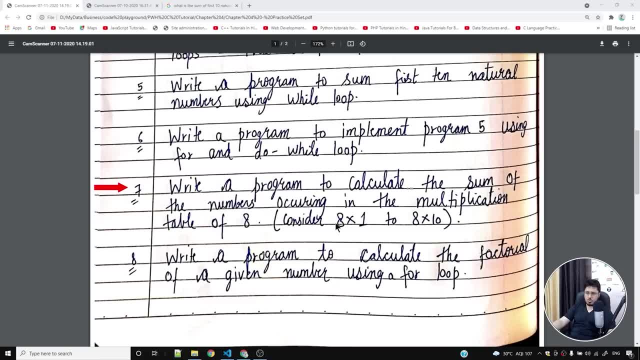 once i solve the other problems because we have done enough practice of for loops and do i loops. the next question says that write a program to calculate the sum of the numbers occurring in the table of 8. so we need to consider 8 multiply by 1, all the way till 8 multiply by 10. so we need 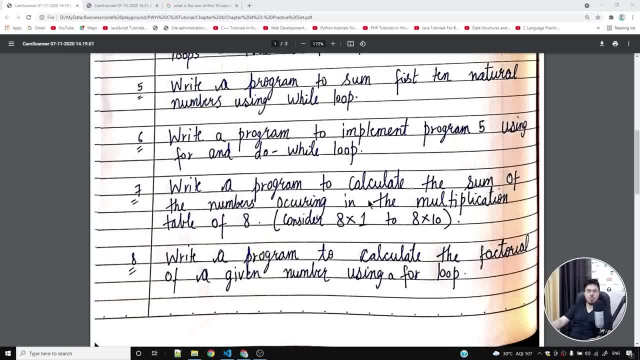 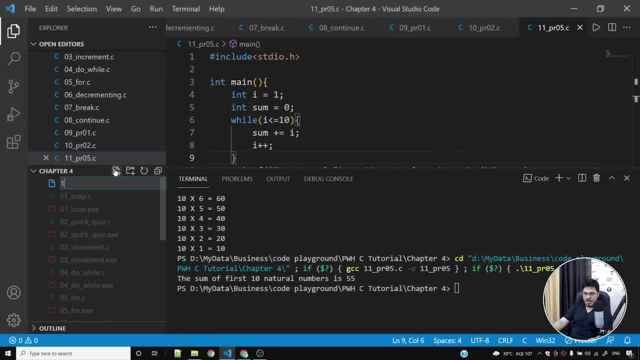 to add 8, 16, 24 and so on. let's see how we can do it. so what i'll do is: let me create a program for problem number 7, so i'll say 12, underscore pr07, dot c, i'll put in the boilerplate code and i'll 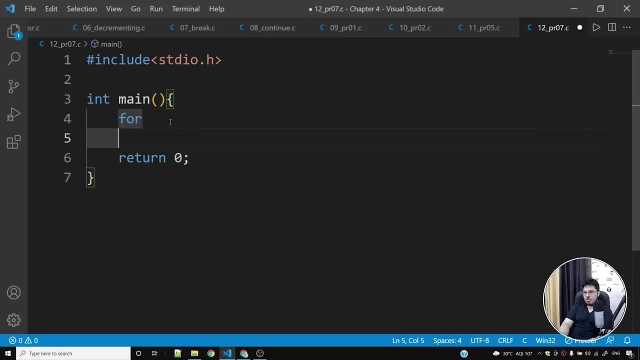 use a for loop. let me close the terminal, so i'll save this and after saving i'll write 4 and get the code snippet. i'll say: entire is equal to 0. i is less than 11 and i'll make it 1 because i want i to start from 1 and go all the way till 10. also, what i'll do is i'll say: 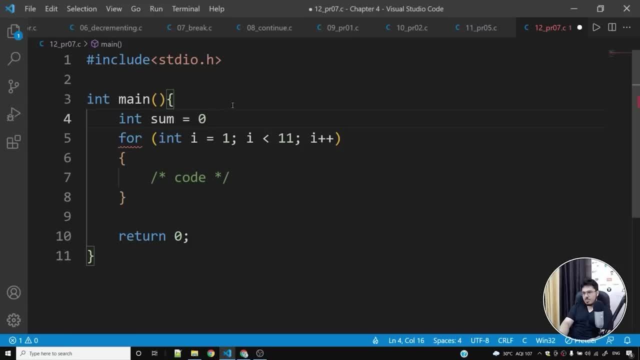 sum is equal to 0. what this will do is this will simply help me initialize sum and i'll keep on adding to this sum. now what i'll do is i'll simply say sum plus equals to, and i'll add: i multiply by this and let me see if i'm able to print the sum, the. i need to use double quotes, not single quotes. 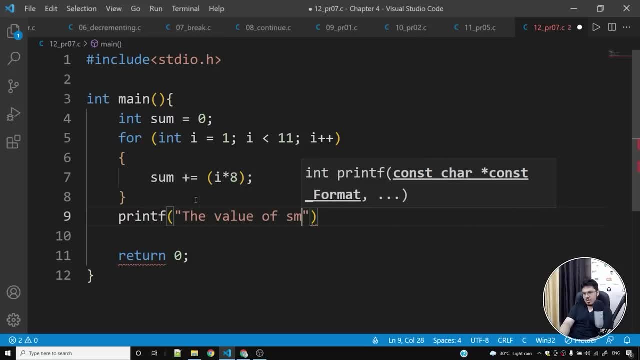 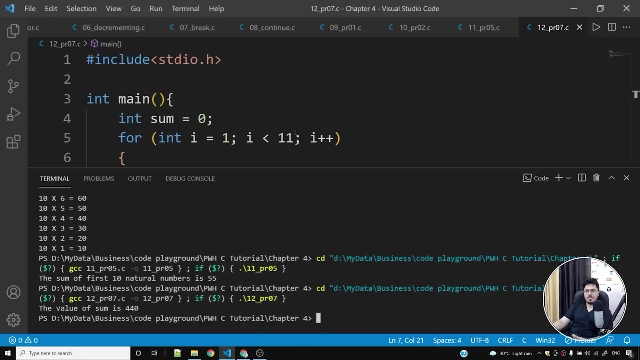 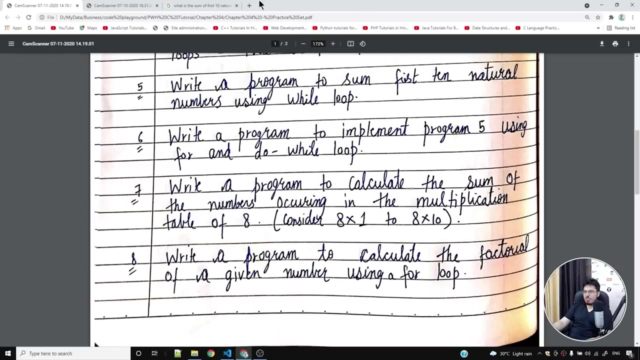 so i'll say the value of sum is percentage t and i'll print the sum. let me run it: the value of sum sum is 440. so if i add 8, 16, 24 and so on, it will add to 440. okay, so it'll be 55 multiplied by 8, and i'll tell you why. why did i say that? so the sum: 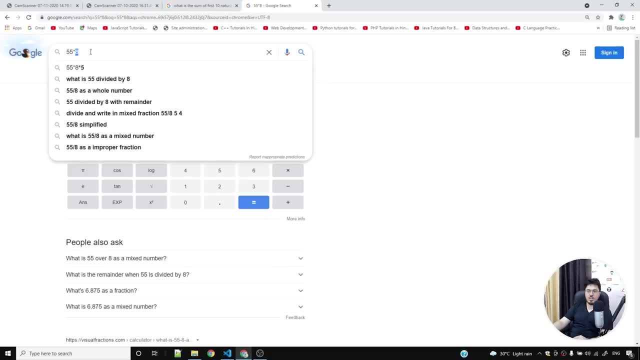 from 1 to 10 is 55 and we can take 8 common from the equation. so if i have 8 multiplied by 1 plus 8 multiplied by 2 and so on, i can take 8 common and what i'll get is 8 multiplied by 1 plus 2. 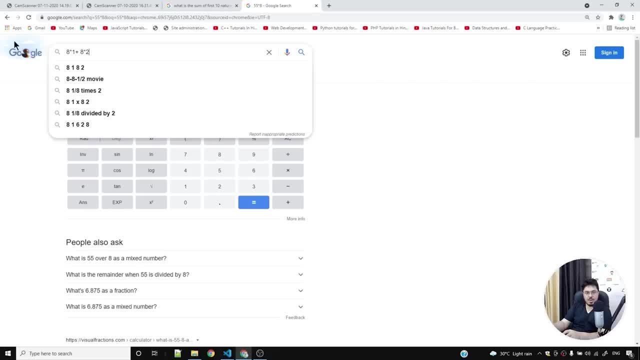 plus 3 plus 4, plus all the way till 10, which is 55. and if 55 is the sum of 1 till 10, the sum for 8 multiplied by 1 plus 8, multiplied by 2 and so on, will be 55 multiplied by 8, which is: 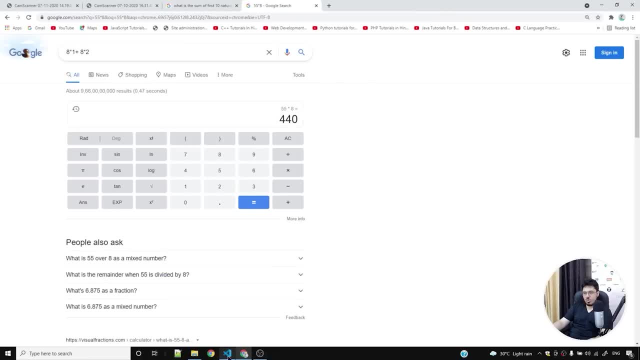 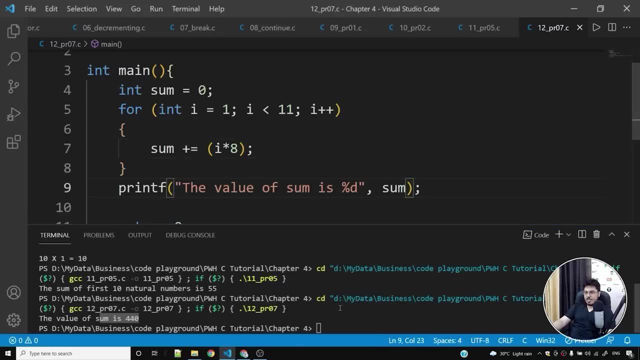 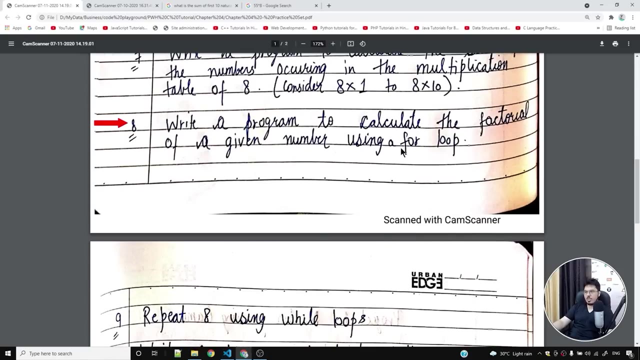 nothing but 440. okay, we just got that and we just cross-checked that. the problem that we solved is indeed correct. let's move on to the next question now. what is the next question? it says: write a program to calculate the factorial of a given number using a for loop. let's do this this. 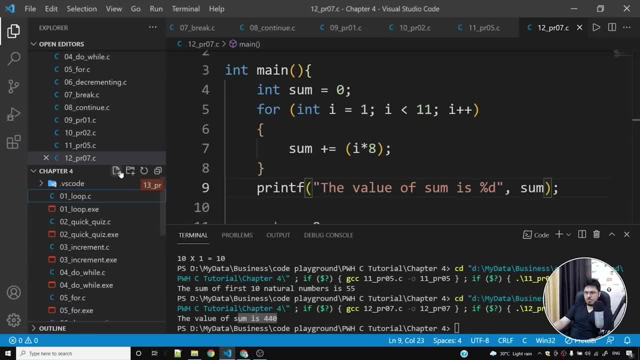 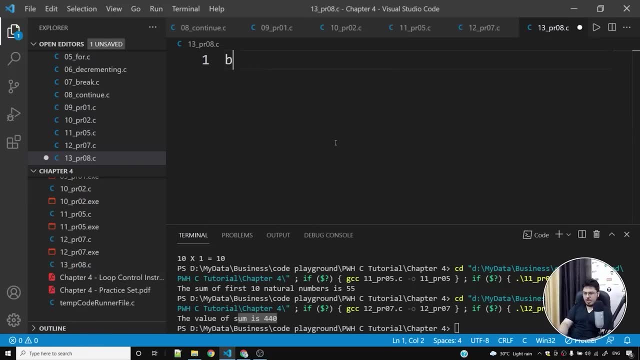 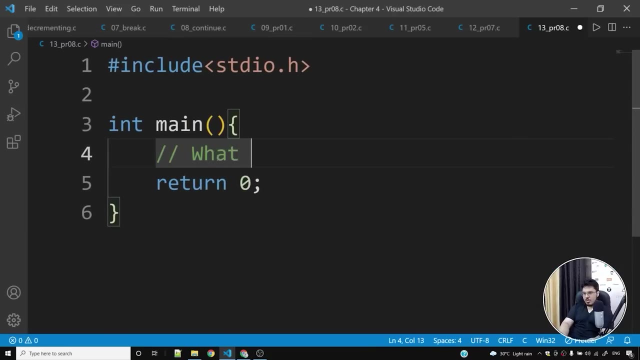 say 13 underscore pr. oops, i forgot to add this pr08 dot c. i'll put in the boilerplate code. by the way, what is a factorial? factorial of 1 is equal to. let me explain you what is a factorial, in case you don't know. uh, in case you know, you already know. just try out this program in the 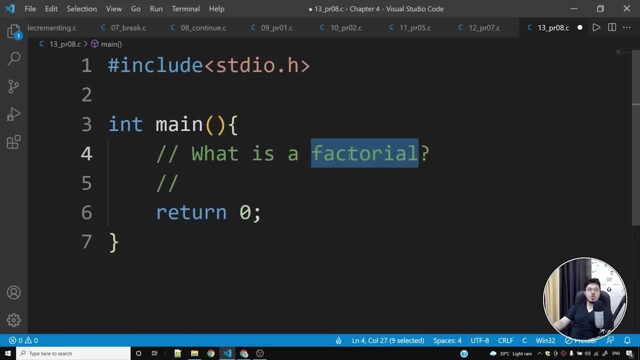 meantime- and i'm explaining people, uh, what factorial exactly is. so when i talk about n factorial, it's nothing but 1 multiplied by, 2, multiplied by, 3, multiplied by, and we'll go all the way till n. okay, now what will happen is, if i talk about this equation, 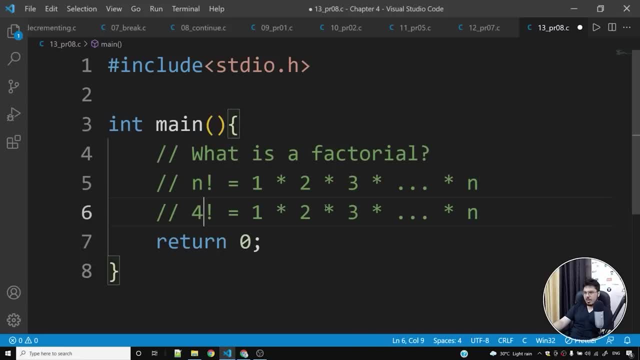 and let us say i want to calculate 4 factorial. what will be the 4 factorial? i'll go all the way till 4. so this is the value of 4 factorial, which is nothing but 4 multiplied by 3, which is 12, multiplied by 2 is 24. so 4 factorial is 24. 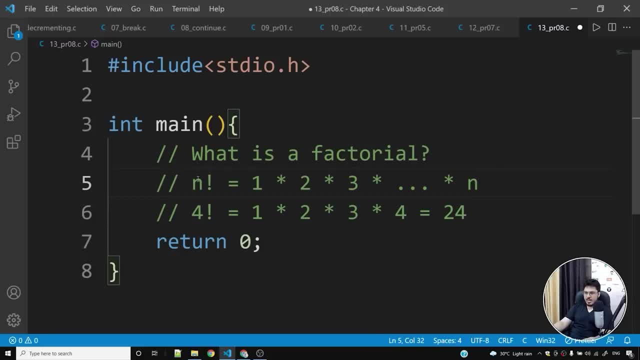 in a very similar way, i can always write: n factorial is equal to 1 multiplied by, 2, multiplied by, 3 multiplied by, and i can go all the way till the number whose factorial is being calculated. now what i'll do is i'll simply say 0 factorial. what is 0 factorial if i put it inside this? 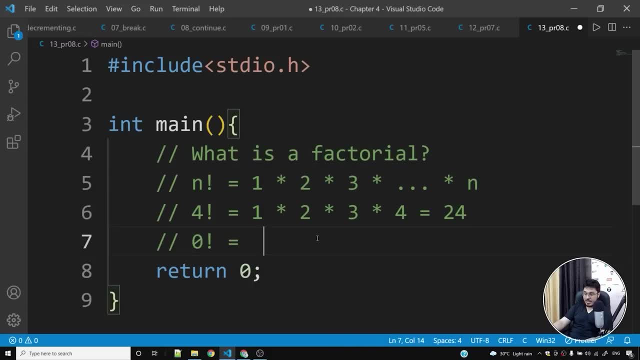 equation i'll not be able to calculate. so 0 factorial, let me tell you, is defined as 1. so by definition, 0 factorial is 1. so this is all about factorial. how will you calculate the factorial? using a for loop? pretty simple, just start with 1. 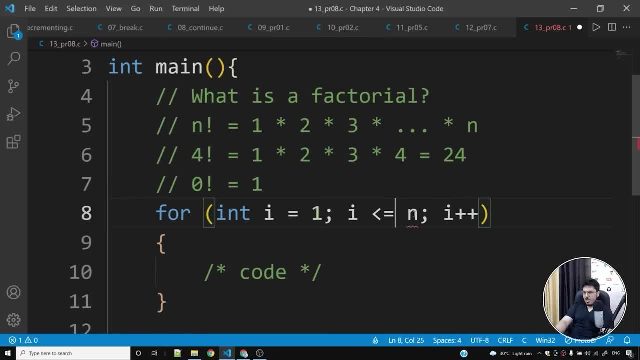 and go all the way till that number, and you need that number as well in the equation if you. if you look at this equation, 4 is there. so we need i less than equal to 4, because i want to start from 1 and i want to go all the way till 4, including 4. i want to include 4 as well. now what i'll do is: 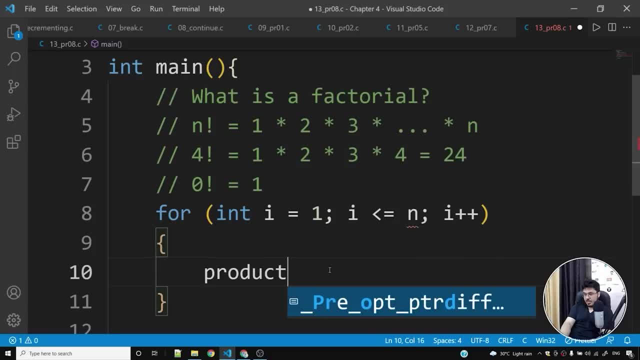 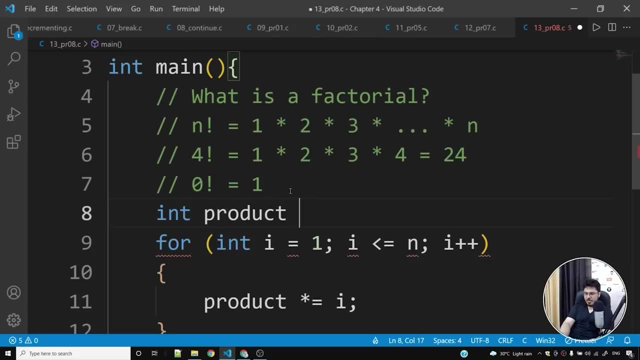 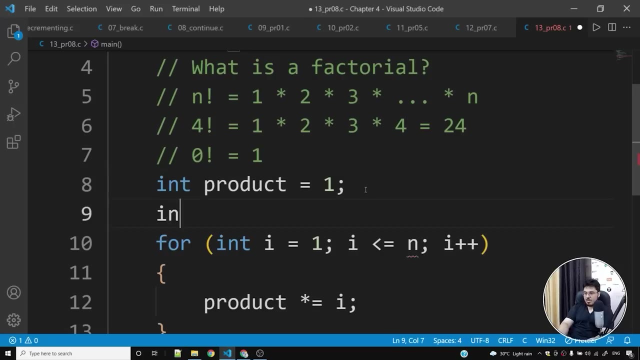 i'll simply say: product multiply is equal to what multiply is equal to i and what is product? product is nothing but 1. make sure you don't put product as 0, because if you make it as 0, then the answer will be 0, always okay, and 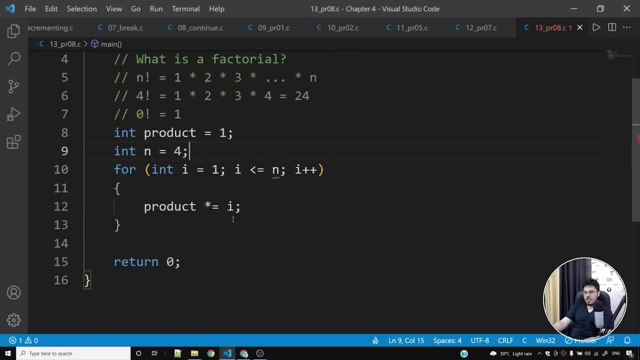 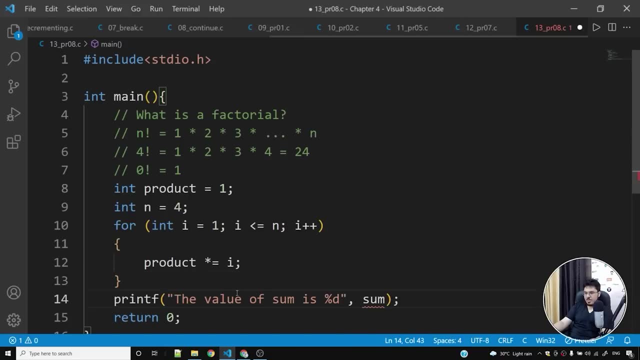 let's also define n. let me try it for 4, and what i'll do is i'll play some copy paste game here. i'll copy a line from here, just to save some time. i'll say: the value of factorial is, let me call it, factorial. 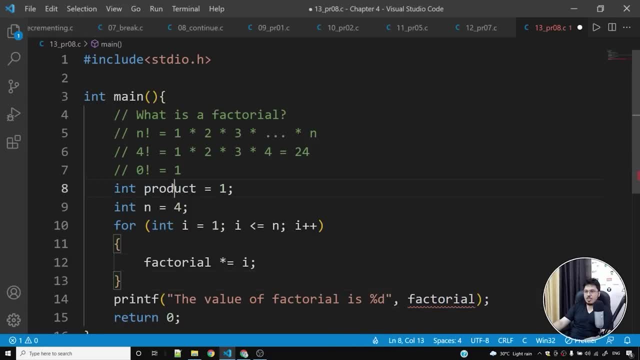 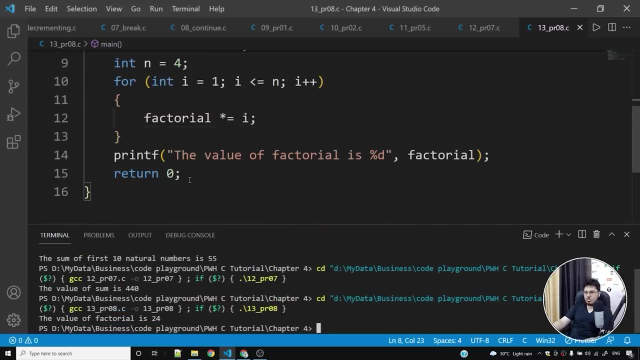 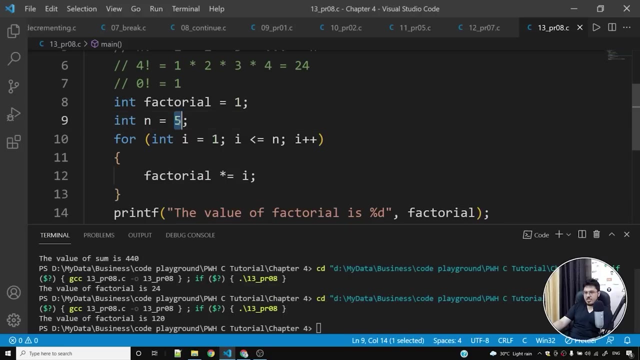 i just want to name my variables correctly. i want to name my variables such that it is easy for you to understand what that variable is doing. i'll save this. let me run this program. the value of factorial is 24. if i change this to 5, you'll see the value of factorial is 120.. if i change this to 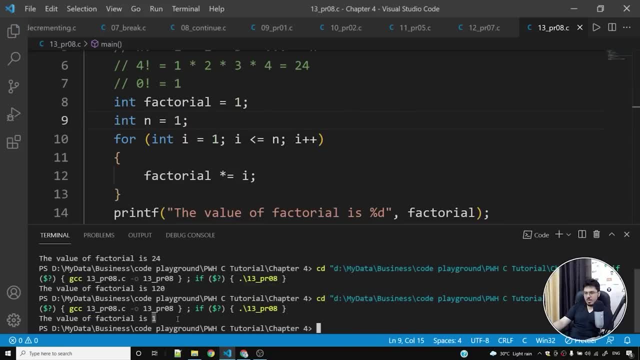 1. the value of factorial is 1.. what if i change this to 0? what is the value of factorial? it's 1, great. so why is it 1 for 0? because this loop will not run at all, for n equals to 0.. i is 1,, 1 is not less than equal. 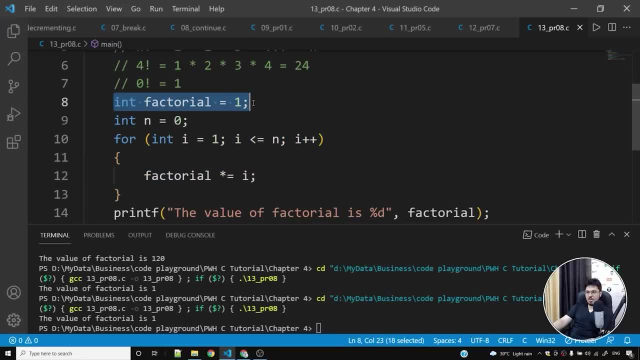 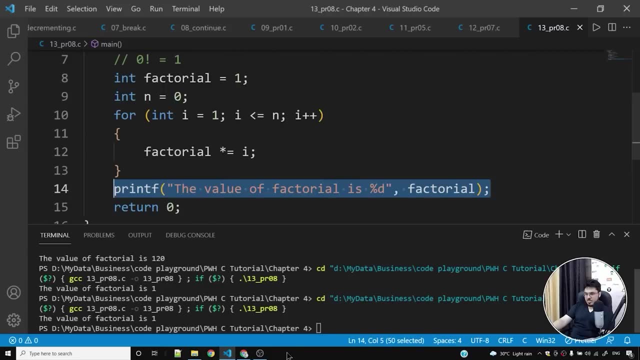 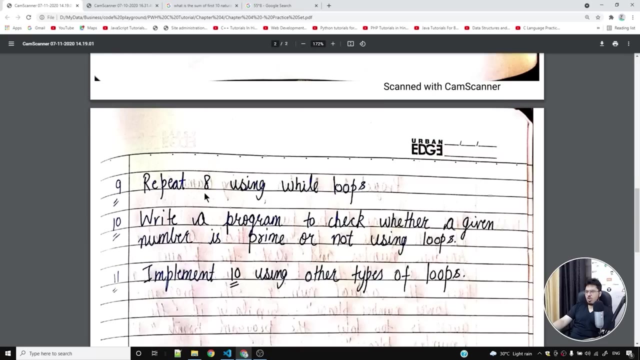 to 0, this loop will not run, keeping the factorial value as 1, and you'll see the value of factorial as 1 whenever you try to print this. okay, so, coming back to this question, write a program to calculate the factorial of a given number. we already solved this. repeat it using while loops. you need to. 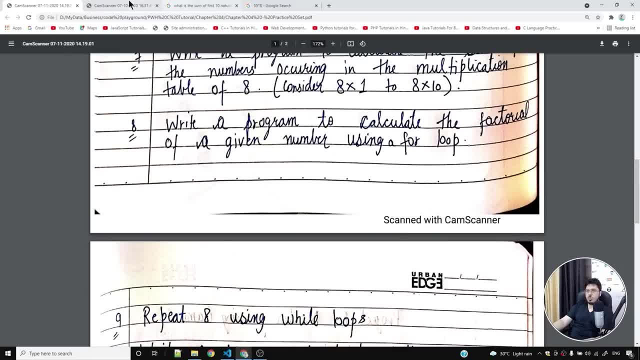 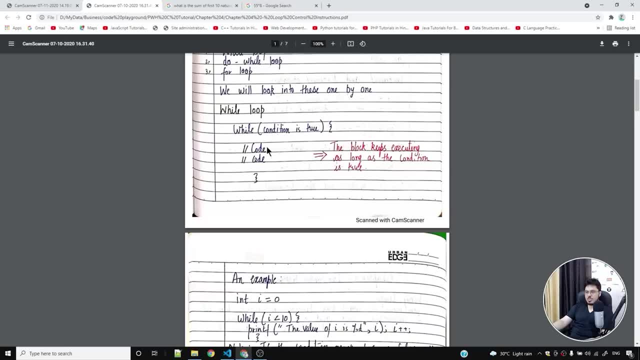 solve this problem using while loop, and it is pretty simple. all you will do is you'll simply write while. you will say while the value of i is less than equal to n, and you'll write the code inside. even the updation code you will write inside the while. 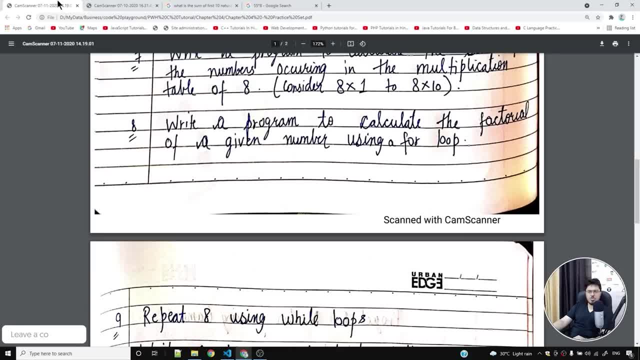 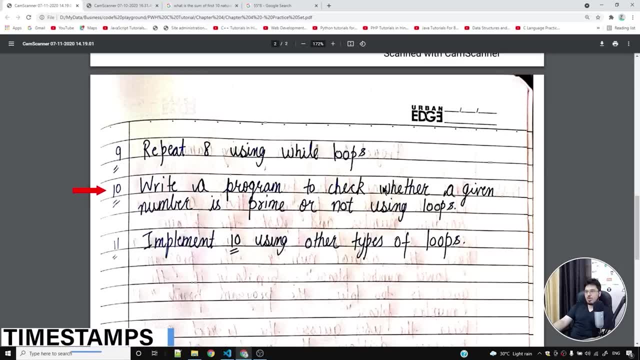 loop and, yes, it is very easy to solve. i want you guys to comment below if you can solve this problem using while loops or not. make sure to put the timestamp while you are commenting. write a program to check whether a given number is prime or not using loops. this is very simple. i'll solve it. 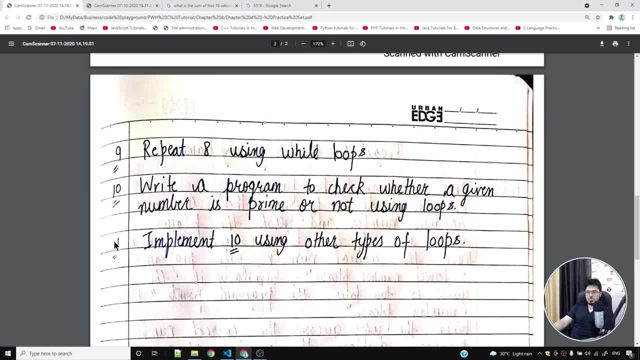 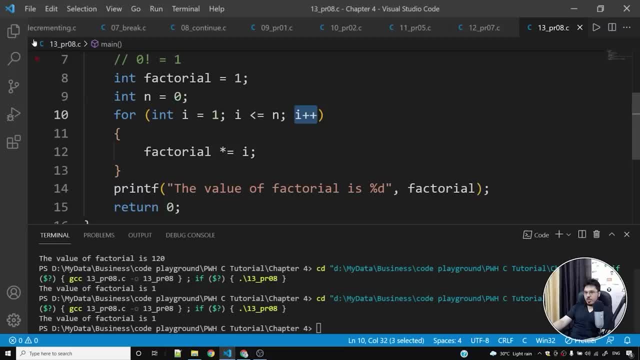 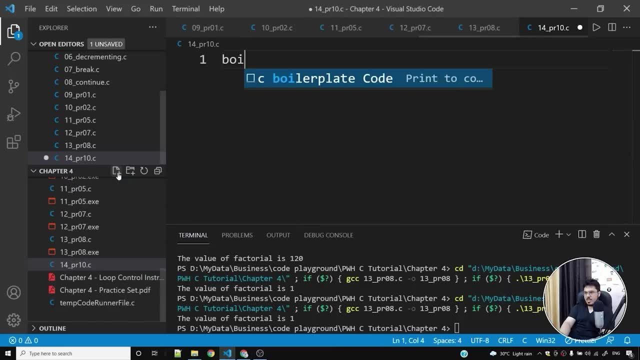 using while loop and then, as part of problem number 11, you can solve this problem using other kinds of loops. okay, let me solve this problem for you. so we need to find whether a given number is prime or not. this is problem number 14: pr10.c boilerplate code. so we need to find whether 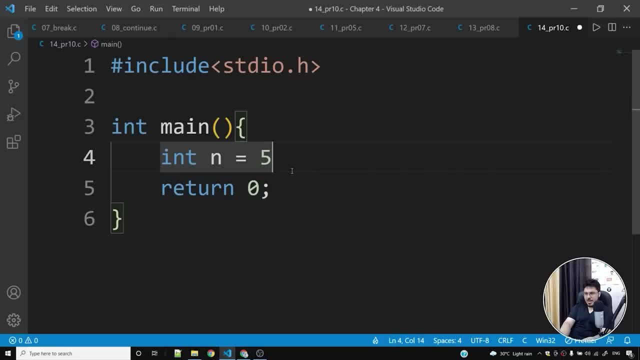 given number is prime or not. let's call this number as n. when is the number prime? a number is prime when it is divided by the number itself and one. there should not exist any other number which can divide n. okay, so how will i solve this problem? i'll write a for loop. i'll start i from one. i'll in fact start i from two, because 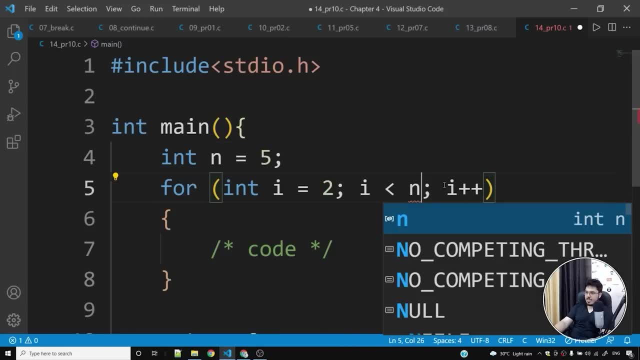 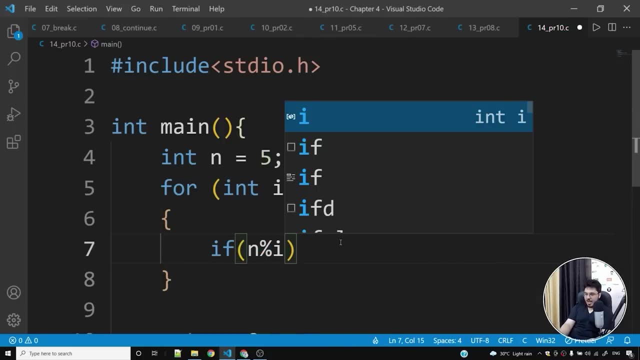 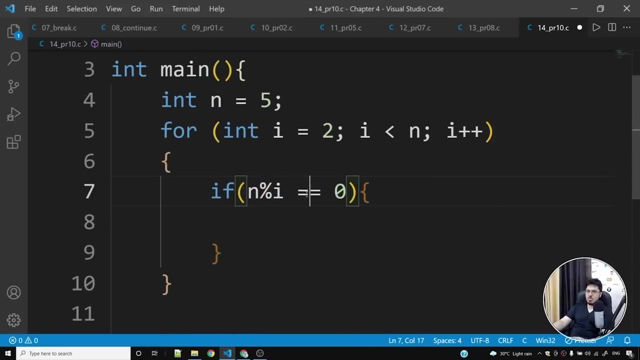 one will definitely divide that number and i'll go all the way till that number. and what i'll do is i'll simply say: if i percent, or rather n percent, i equals to, equals to zero, which is nothing. but if i divides this number n, so if the value of i is, say, five and n is 10, then yes, five divides 10. so we need to find out whether 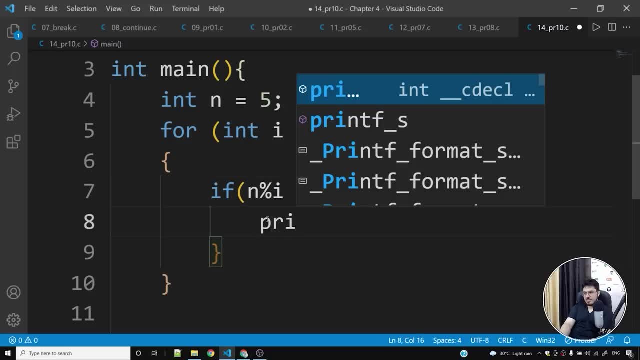 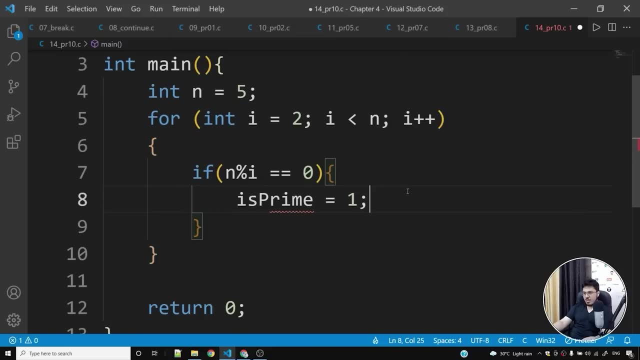 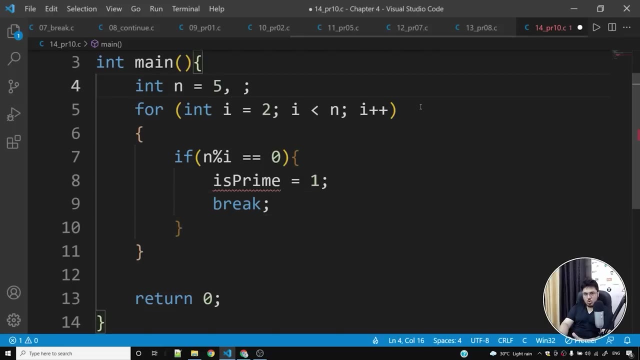 i divides n or not? if that is the case, we simply say prime is equal to one. okay, so let me call it is prime. so i'm saying: is prime is equal to one, and we'll break out of this loop. why am i breaking out of the loop? i'm breaking out of the loop because that's all i want to know. i want to know. 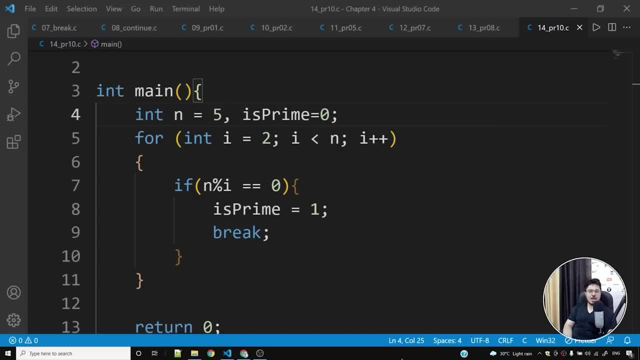 whether this number is prime or not. i'll by default make my is prime. variable is zero. why am i doing that? i'm doing that because i'm assuming that this number is not a prime number and i'll keep on assuming that i made a mistake here. i'll simply say is. 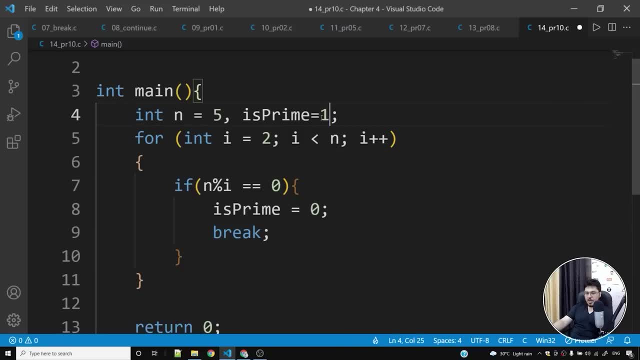 prime equals to zero. because it will not be a prime number and by default, what i'll assume is that it is a prime number until it is proved not to be a prime number. so i'll say: if n percent i is equal to zero, is prime is equal to zero. so if any number happens to divide this number, what i'll? 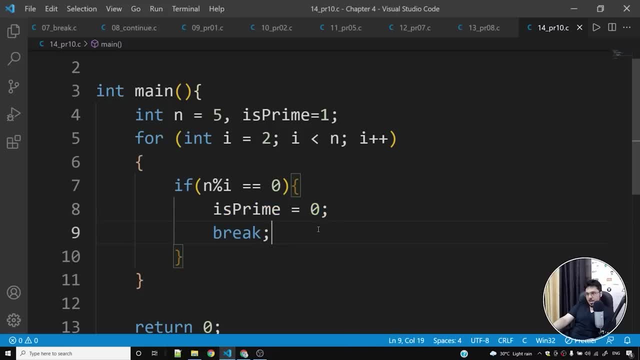 do is i'll simply say that this is not a prime number, and the moment that happens, i'll break out of this loop, because i now have this information that this is not a prime number and that's all i wanted to know. so i'll simply say: print f. the number is 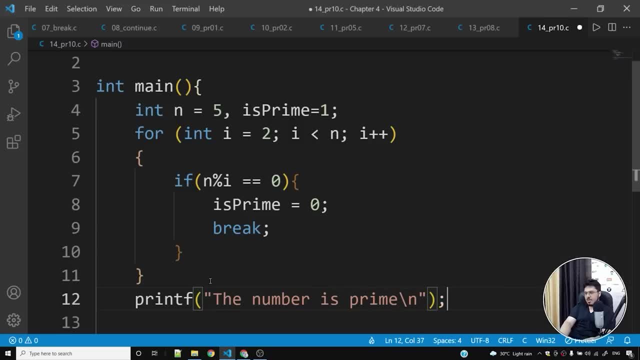 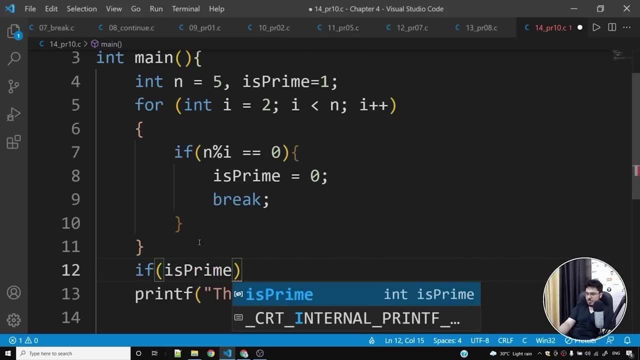 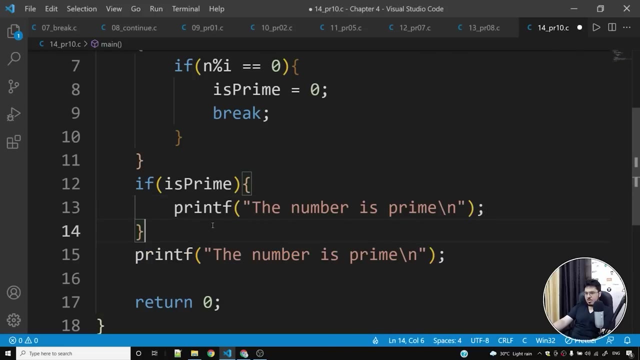 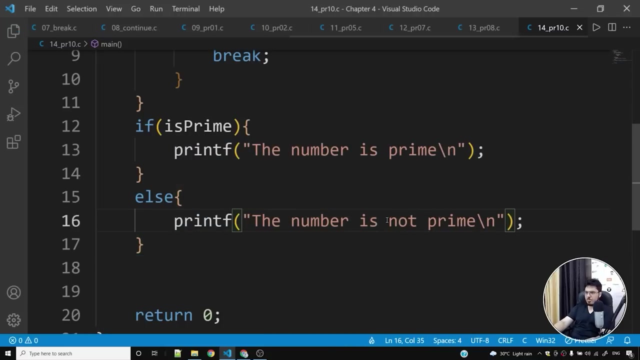 prime backslash n. when will i print this? i'll print this when the value of is prime is true. so if is prime, i'll print this. otherwise, what i'll do is i'll say this is not a prime number. number is not prime. okay, let's see if this program works, and i'm 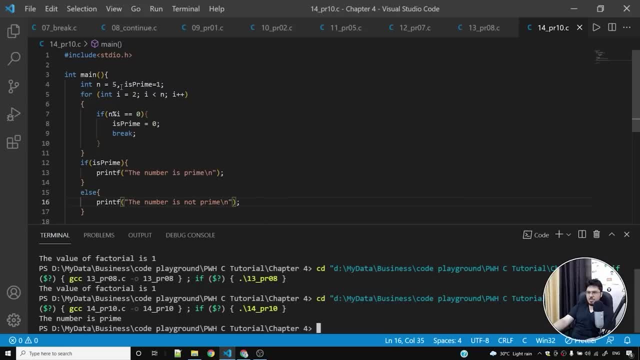 going to explain this program once again to you. so if n is five, yes, it is prime. let's check for six: no, it's not prime. so, yes, it's not prime. let's check for two. is it prime? two is prime. yes, two is prime. let's check for nine. nine is not prime, no, it's not prime. let's check for. two is not prime. 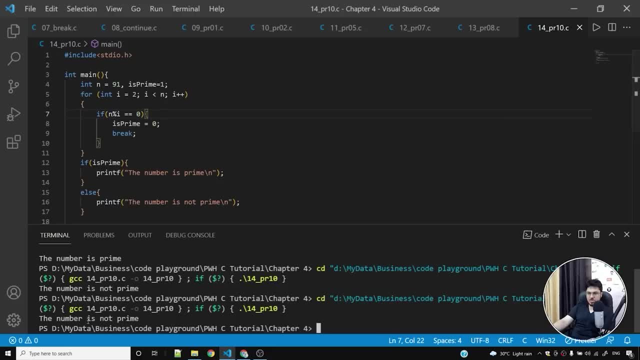 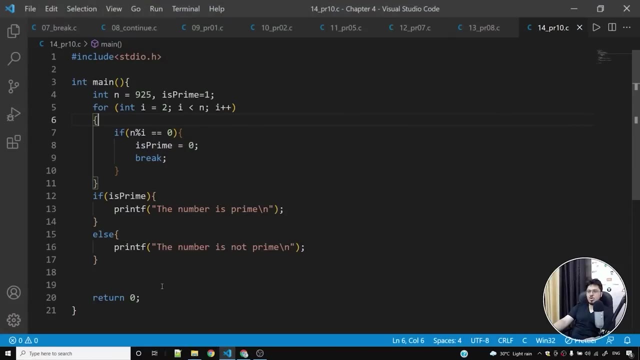 let's check for 91: it's not prime, 91 is not prime. let's check for nine to five: it's definitely divided by five. so it's not prime, it's not prime. okay, so i hope that you understood how this program to find out whether number is prime or not. um, i hope you understood the logic of this. 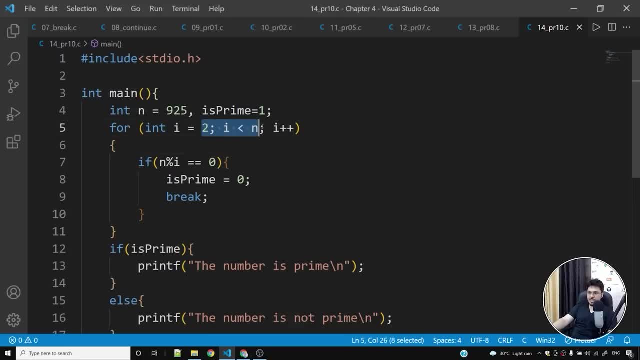 problem. basically, what we are doing is we are starting from two and going all the way till that number to find out whether there exists a number which can divide this number. and the moment we find that number, what we do is we break out of the loop and we declare the number is not prime and 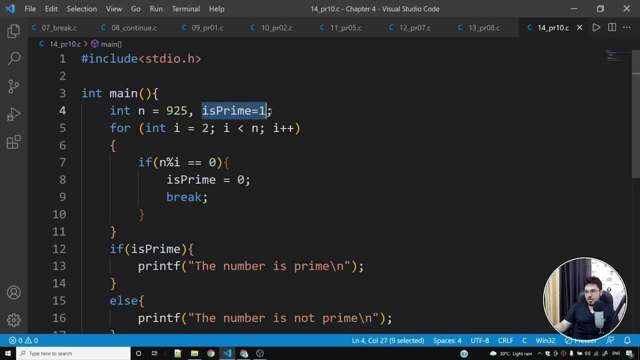 if we are not able to find such number, we assume- uh, or rather, we stick to the assumption which we initially made- that the number was prime, because we were not able to find any number which can divide this number, n, which clearly proves that n is a prime number. okay, so this is how the program. 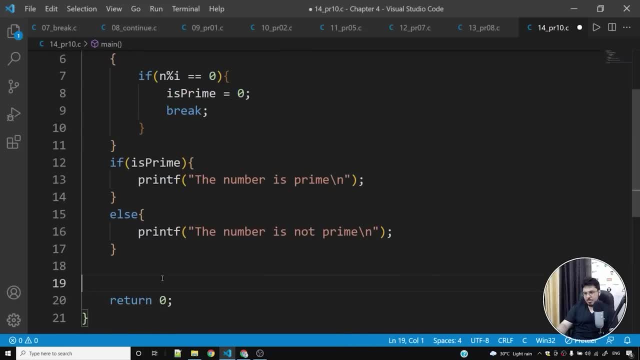 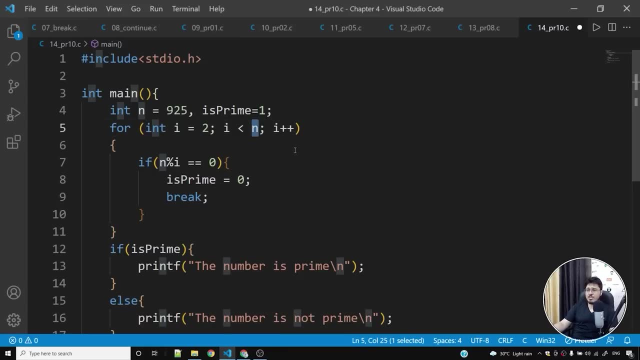 to write whether a number is prime works. now i'll tell you something: there is a way to make this program better by changing this into root n. but i'm not going into those details. i'm not going into data structures and algorithms and making programs efficient. i just want you to solve this problem so that you have 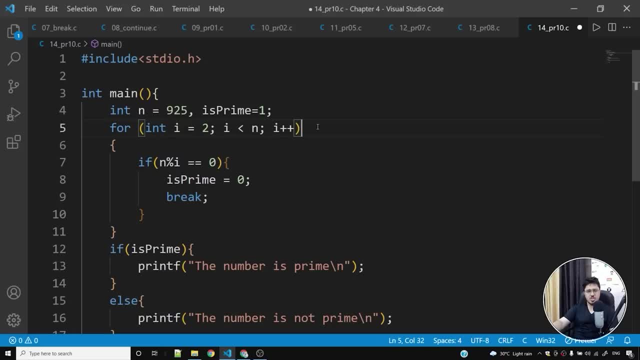 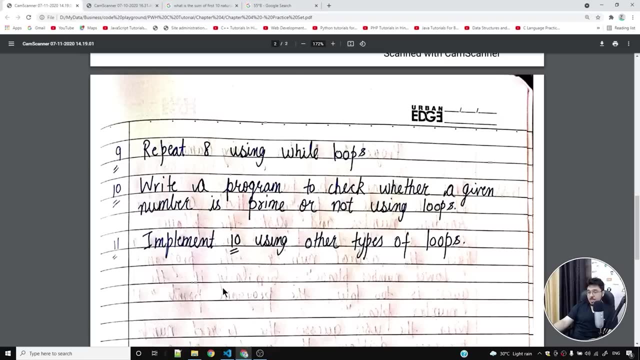 a good understanding of how c language ifl statements, conditionals, loops and all these things work. i hope you enjoyed this practice set. i'll save this program and i'll give you this program in the form of a zip. also, i'll give you the notes in the form of a zip so that you have 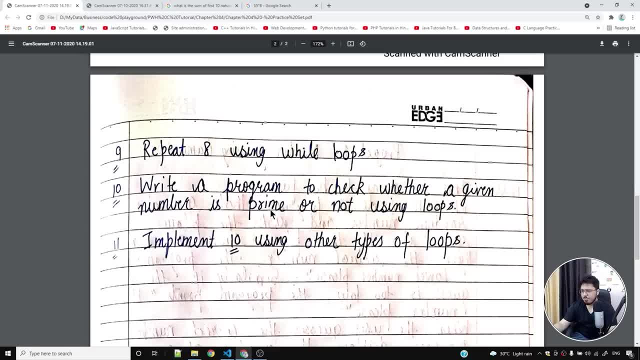 all the notes by end of this chapter. so implement 10 using other types of loops is something that you need to solve by yourself. i hope that you enjoyed this practice set. now we'll move on to chapter number five, where things will get even more exciting and we'll learn about more concepts. 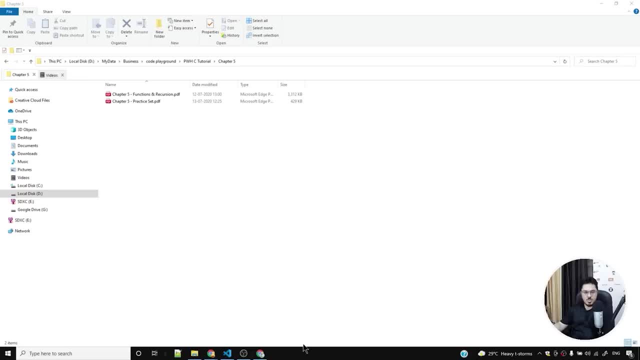 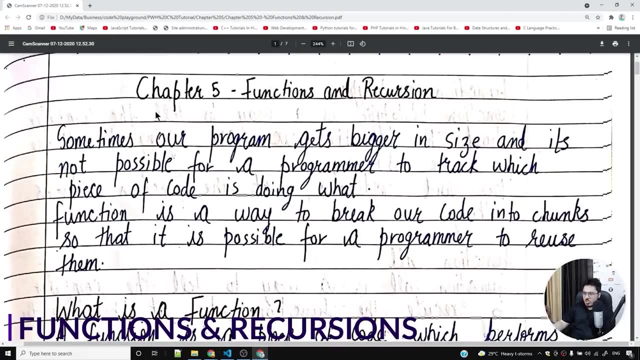 of c. so let's move on to chapter five now. from this video onwards, we are going to look into chapter number five, which is nothing but functions and recursions. what is function and what is recursion? we are going to study all these topics in this chapter. so i have written something in: 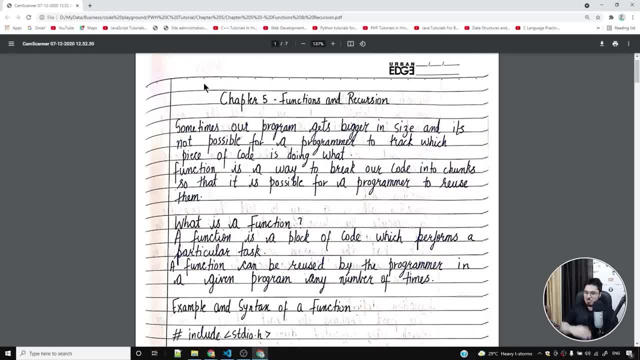 the notes. let's see what it is. sometimes our program gets bigger and bigger in size and it's not possible for a programmer to track which piece of code is doing what. so far, the programs written by us were very basic. they were not very complicated, they were. 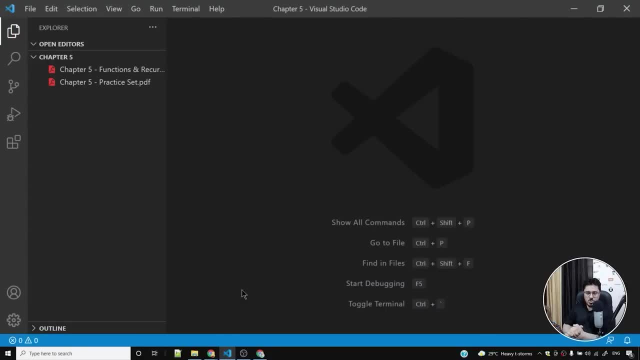 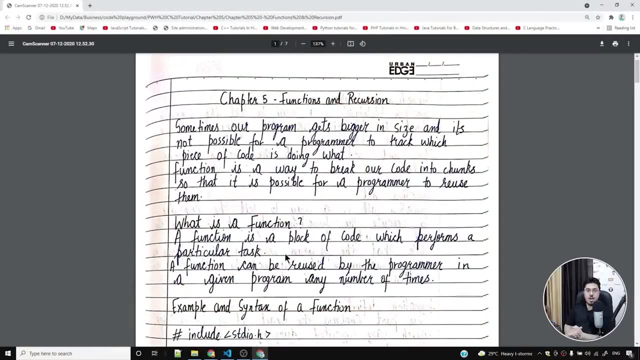 around 29, at max 30, 35 lines of codes. but what happens is when things get complicated, when you have something which is doing a lot of work, when you have a code base which contains, say, 452, 480 lines of code, then you unknowingly might be repeating a piece of logic. 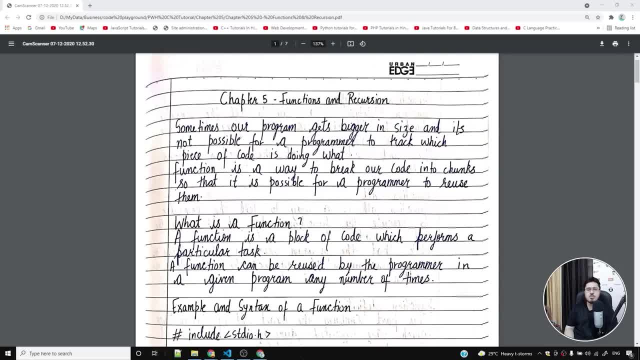 again and again. for example, let us say you are calculating average of seven numbers inside your program and you are doing that at 21 different places. so all those 21 different places which contain, say, four lines of code to calculate that average, can be replaced with a single function. 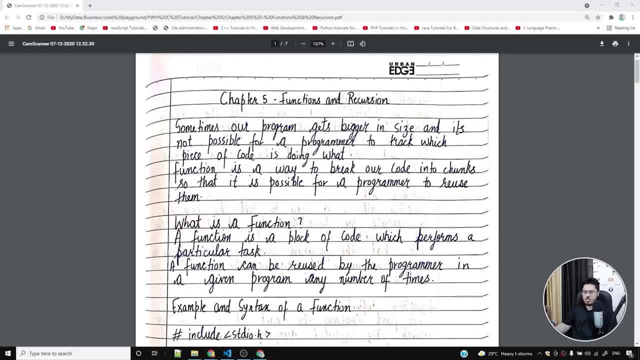 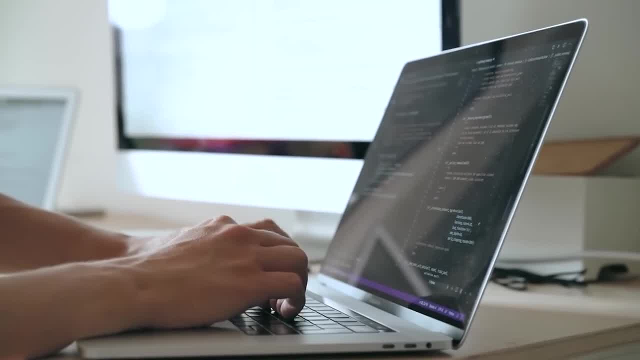 call. what is a function call? we'll see what a function call is in this chapter, but i'm just giving you an idea of how. functions promote code reusability. so we want to reuse the code again and again. the code which we have written has to be reusable. we do not want our code to be 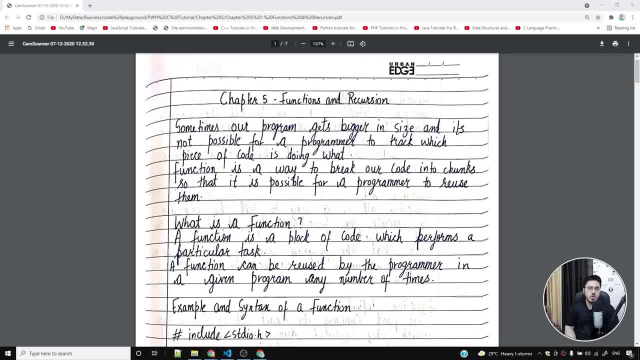 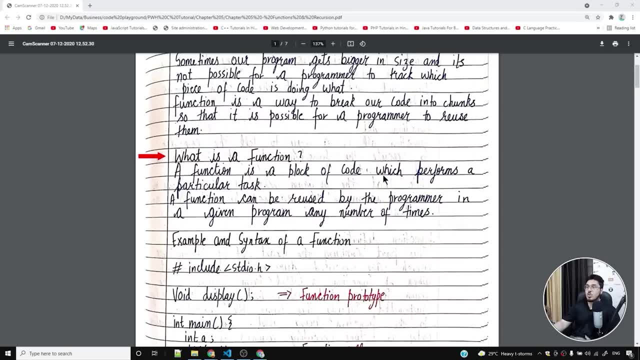 inconsistent or say we don't want to repeat our code in our program again and again. we'll look into all these things in this chapter. so what is a function? a function is a block of code which performs a particular task. so a block of code performing a particular task is function a. 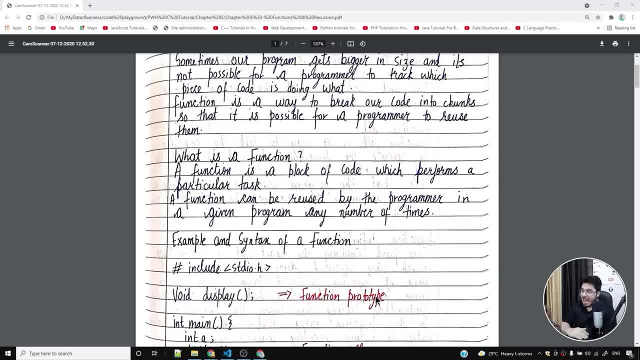 function can be reused by the programmer in a given program any number of times. for example, you have written a function which calculates average of three numbers. you can't reuse that particular function any number of times, and we'll talk about some of the syntax and some of the terminologies associated with the functions and then we'll use functions and see how they can. 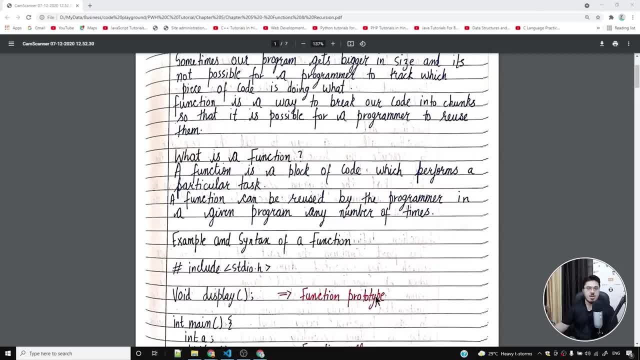 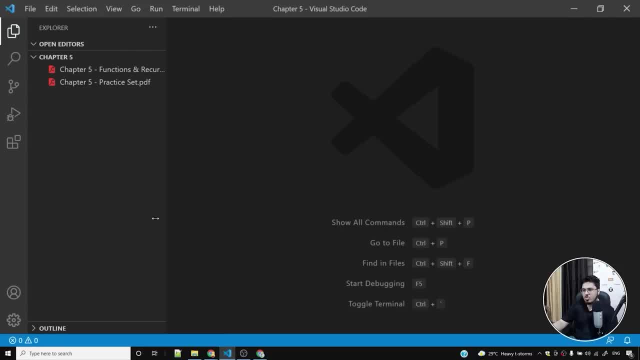 make our program more efficient and effective. so here is example syntax of a function. so here is a code which i've written for you. let me write this code once again in my vs code, and that way you'll be able to understand what a function is. so i'll simply say zero, one underscore function, dot c. 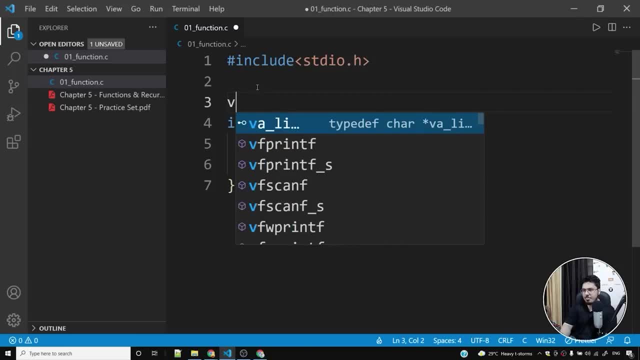 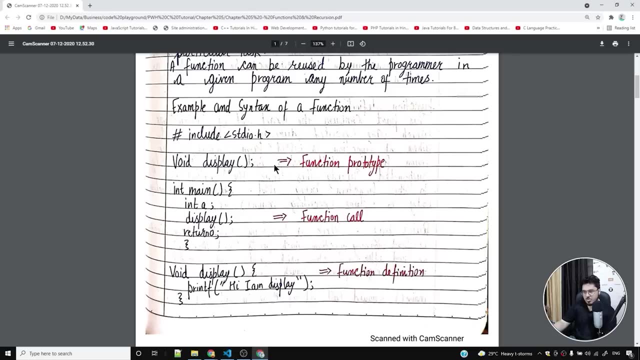 i'll add the boilerplate code and let me write something called void display. you might be thinking what this void display is and what this void display is doing. this is called function prototype. this is telling me that display is the name of the function it is going to return: void. 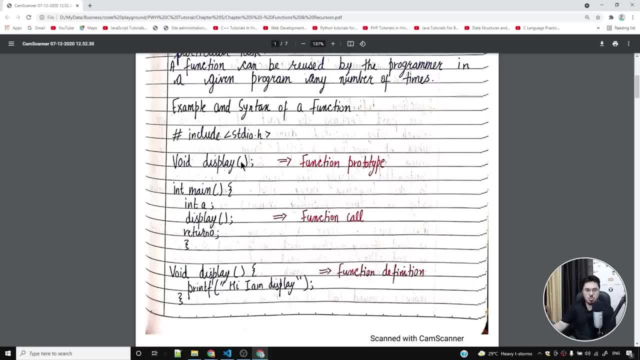 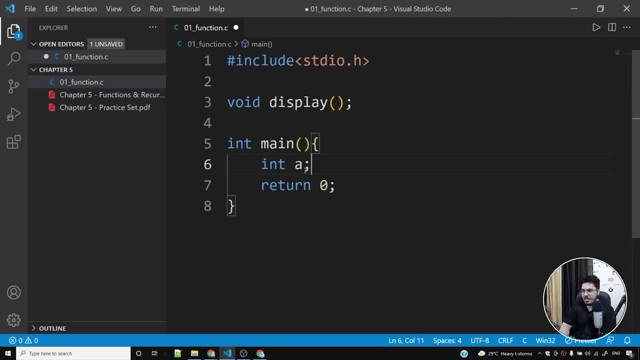 int a, display and return zero. so i'll simply say: int a, then display and then return zero is already here. okay, now what i'll do is i'll write what is called a body of the function. so this is the body of the function. i'll simply say: printf: hello, word, backslash n, backslash n, and i'll save this program. 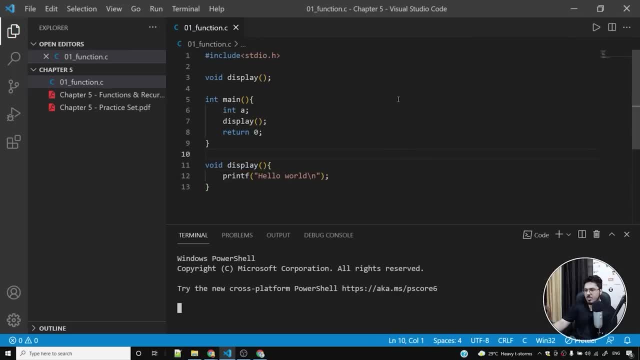 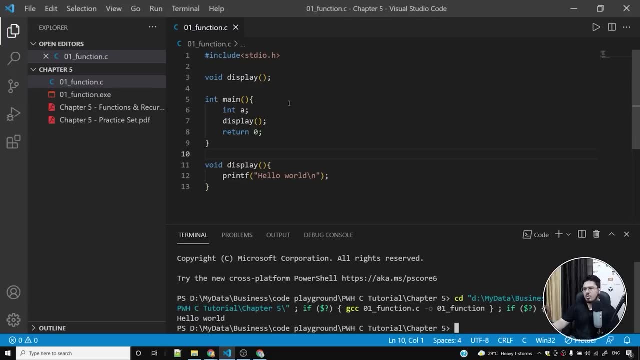 and let me run this and show you what happens. i'm waiting for this program to execute and hello word is printed on the screen. how does all these things work? let me tell you how all these things are going to work. this is something which is called function prototype. okay, this is something, this entire thing, from line number five to line. 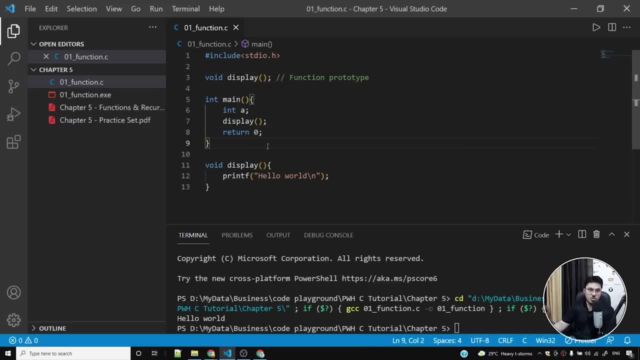 number nine. uh is the main function, so this is the main function. this is also a function. so this function basically contains the lines of codes which are executed from the beginning. so any program, or rather any c program, starts from the main function. now what happens is i'm writing the body of this. 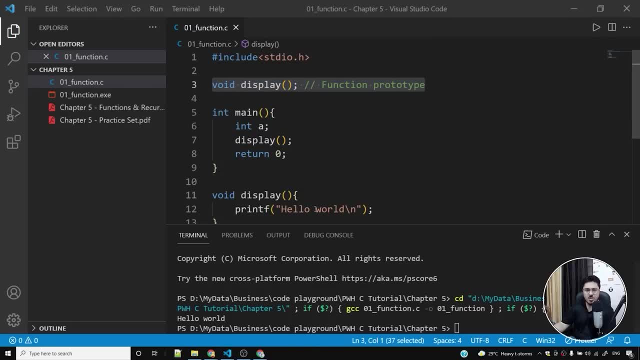 function. so whenever i write function prototype for any given function, i'll write the body of that function later, and inside this body what i'll do is i'll add some set of instructions and printf hello. word backslash n is one of those set of instructions. so now what i can do is i can use. 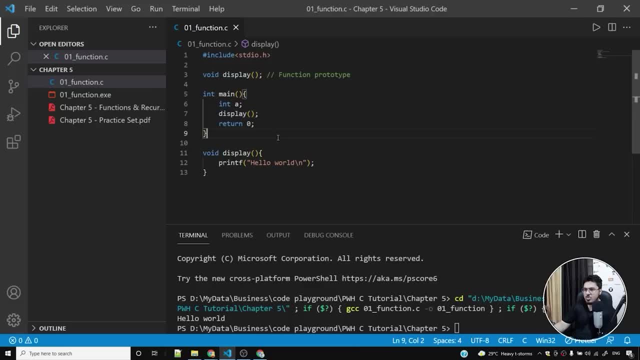 this display and these set of parentheses to simply run these set of instructions. isn't it cool i i can simply say display any number of times to print hello word. you must be thinking: why are we saying display to print hello word? why can't we simply printf hello word here itself? okay, you can do that. 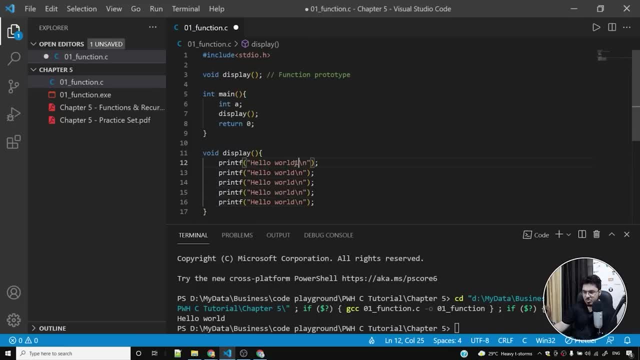 but what now? what if i want to print something like this? what if? what if i want to print hello word, hello two. hello word three, hello word, four, hello or five, something like this? what if i want to print this? i can simply say display and this will run these set of instructions. so if i run, 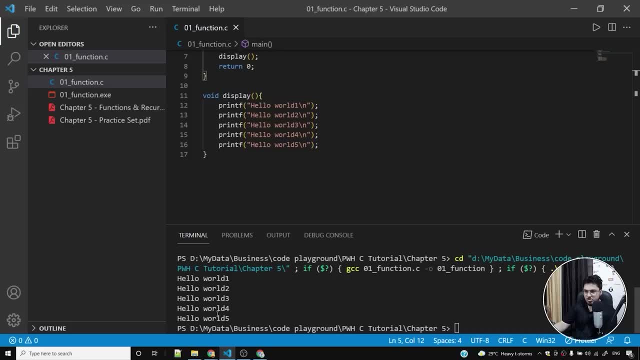 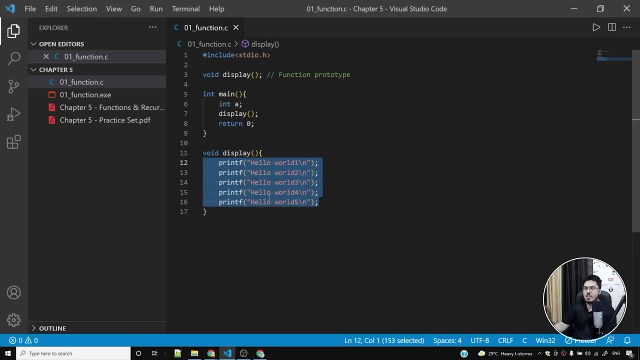 this program. now you'll see that hello, word one, two, three, four and five has been printed on the screen. so this is the magic of functions. you can have multiple lines of code inside the function body and you can say something like this display and this display. when you say display, this will execute all these lines. so there is. 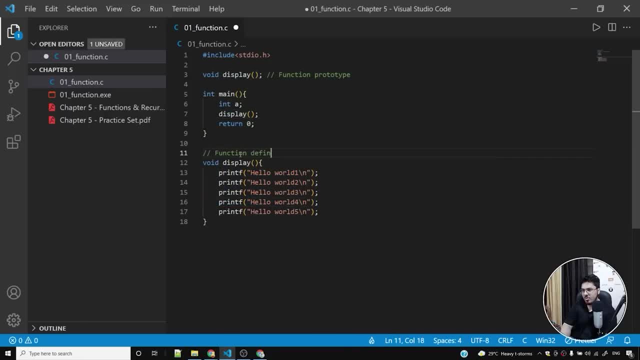 something called function prototype and there is something called function definition. there's also something called function call, which we are going to look into in a bit. so function call, so this is a function called display. so basically, what we are doing here is we are simply calling the function. 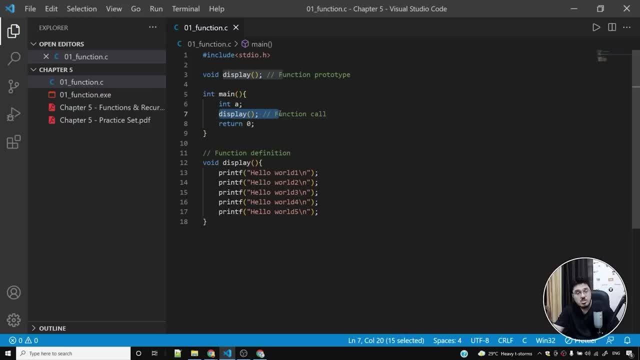 we are saying that run the body, or rather run the instructions inside the body of the function. so void, display whatever is written inside this set of parentheses. just start executing those lines. so hello word one, hello word two. hello word three, hello word four, hello word five. these lines will: 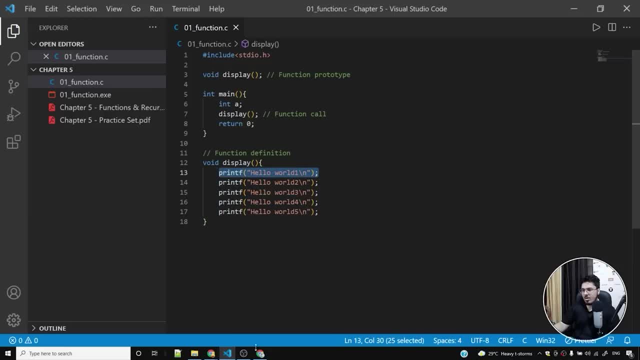 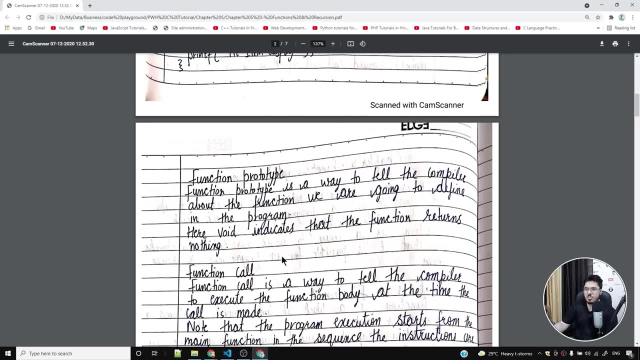 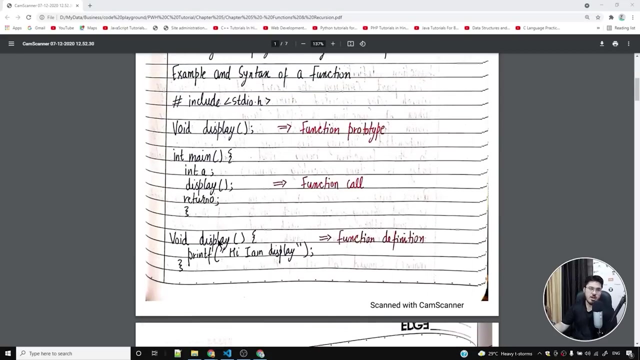 start getting printed because we have a printf statement. now, coming back to the notes, because we have a very good job in putting all these concepts together. I've talked about function prototype, call and definition inside these notes, but before we look into those definitions, I want to tell you how basically this works in a nutshell. so here is the function prototype, so void display. 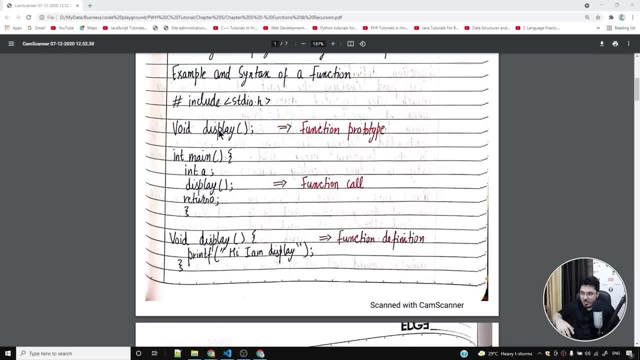 basically, I'm telling that display will be a function. it will take nothing as the input and it will output nothing. void means nothing. okay, now, whenever I'm writing the body of the function, it's called function definition. so I'm defining what this function will do. so in function prototype, I'm telling what this function will return and 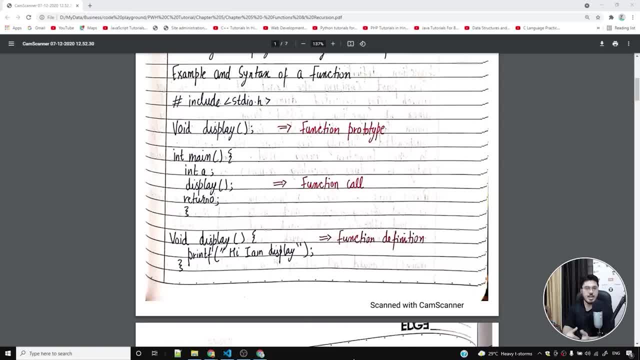 what this function's name is gonna be and what this function will take as input. function definition basically jots all those statements down which will be executed whenever I call the function. and what is the function call. and how do I call a function? I simply write the name of the function. 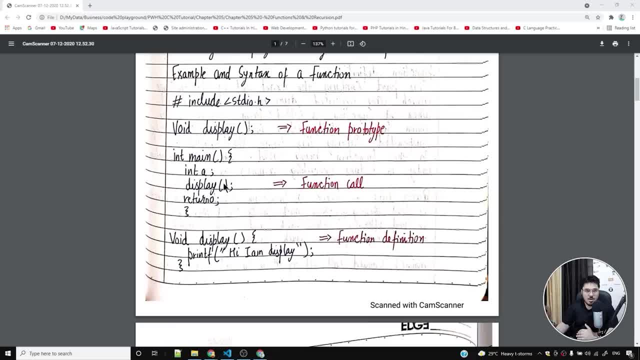 and give the arguments. I can pass a number. I can pass the things that this function needs. luckily, this function doesn't need anything, so I don't have to pass anything. this simply displays. I am printf whenever I say display and whenever I say display and the set of parentheses, semicolon. 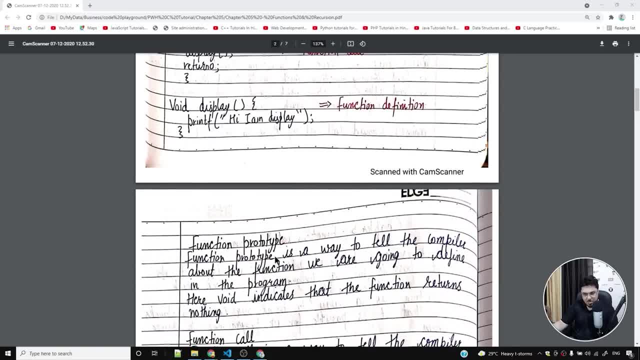 this is a function call and this will execute I am display and I am display will be printed. now let's look into the definition and see how I have explained prototype call and definition in the notes. so function prototype is a way to tell the compiler about the function. so I'm basically 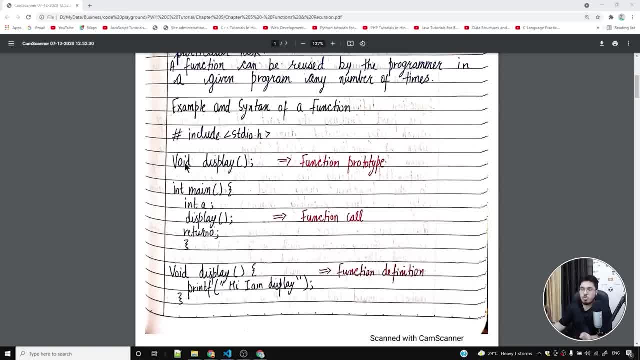 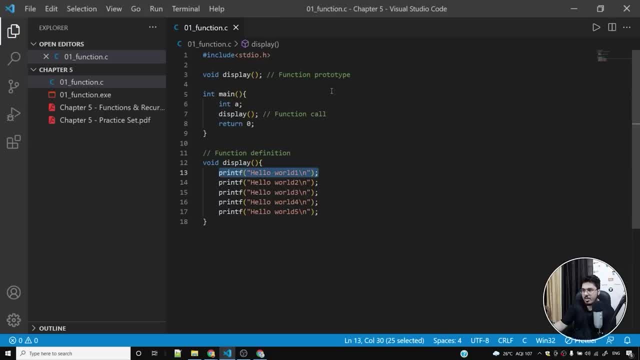 telling about this display function. the display is going to be a function. it is not going to return anything as an input. let us say you have an average function which is going to take three integers. so you can- you will have to write something like this. you might have another. 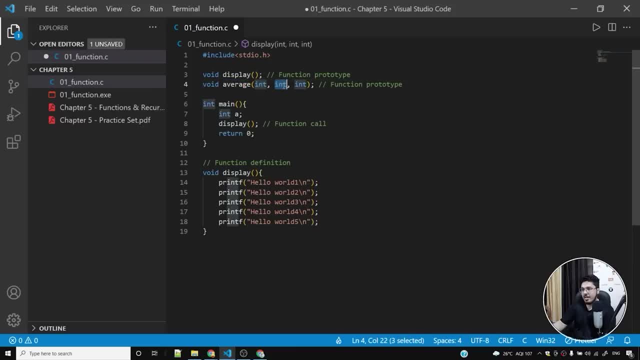 uh function called average, which might take in float in it. so you'll have to pass these three numbers whenever you're calling the, the average function. but we don't have any such function. let me keep this line. I'll simply comment this out. so this is the function prototype. I am not telling. 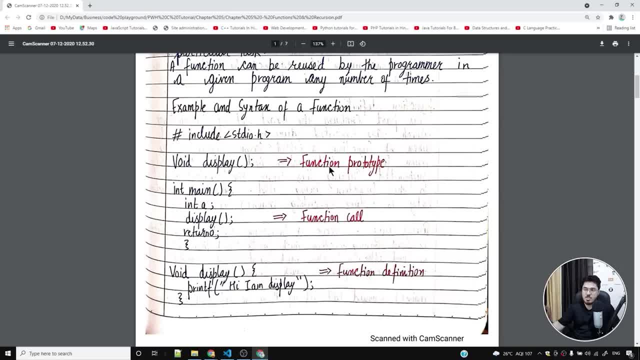 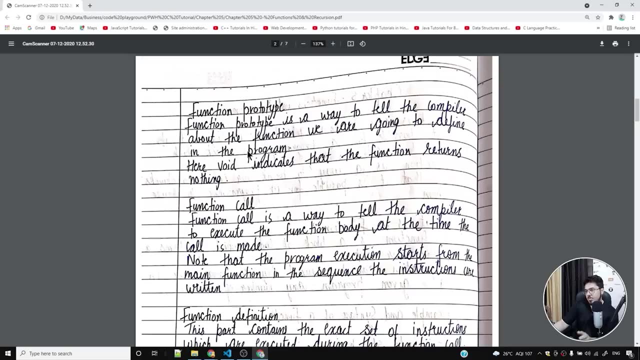 what this function will do inside the function prototype. but through function prototype, which is a single line, I am simply telling that I want a function which is whose name is display. it is going to return nothing and it doesn't take anything from the user, so there is no user input. so function prototype is a way to 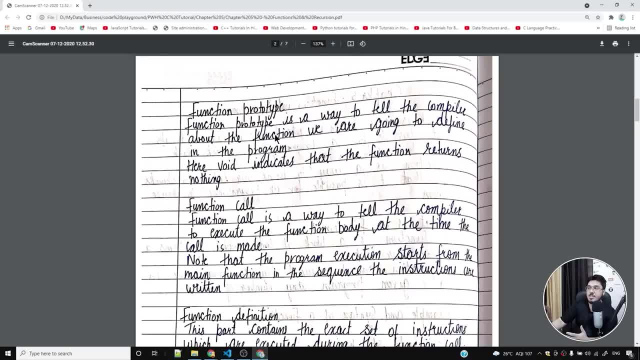 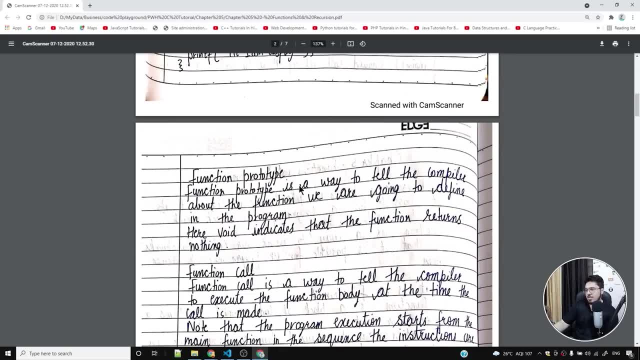 tell the compiler about the function we are going to define in the program. here, void indicates that the function returns nothing. so this void indicates that this function is not going to return anything. okay, so I hope that, uh, that that explains what a function prototype is in a good detail. uh, function call is a way to tell the. 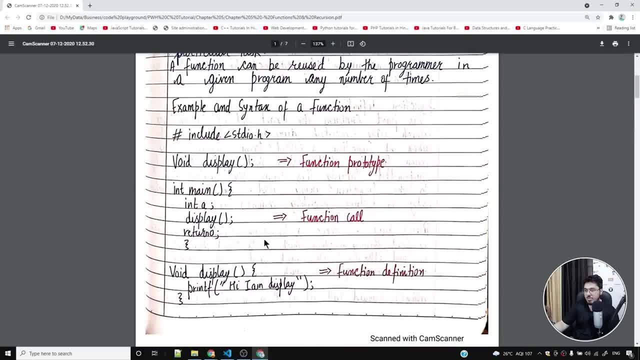 compiler to execute the function body at the time the call is made. so whenever compiler encounters this display and this parenthesis, what compiler will do is compiler will simply start executing these instructions. printf- hi, I am display. all these instructions will be displayed by the compiler whenever compiler sees such a thing. so I hope that you are able to understand how these 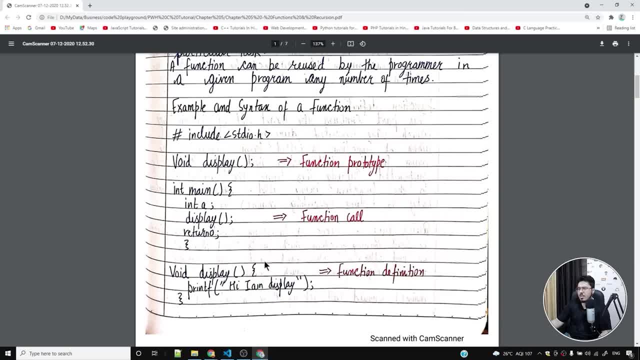 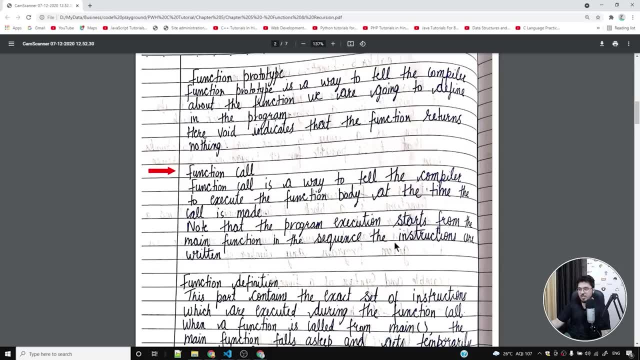 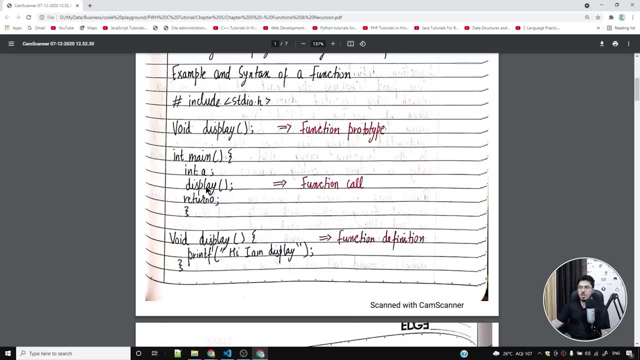 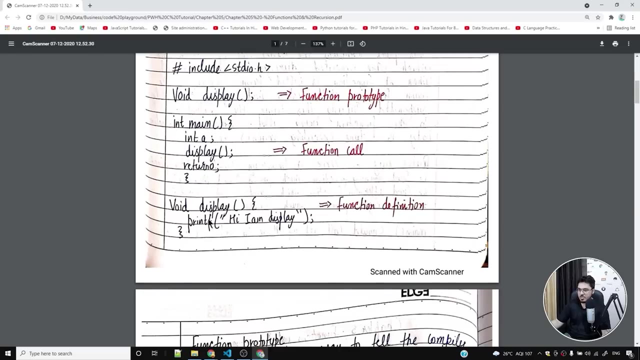 function works okay. coming back to the notes, uh, function call. we have just talked about function called. note that the program execution starts from the main function in the sequence instructions are written, so the program execution will start from here, and whenever this display call is encountered, what will happen is that this, this function will start executing all these instructions inside this. 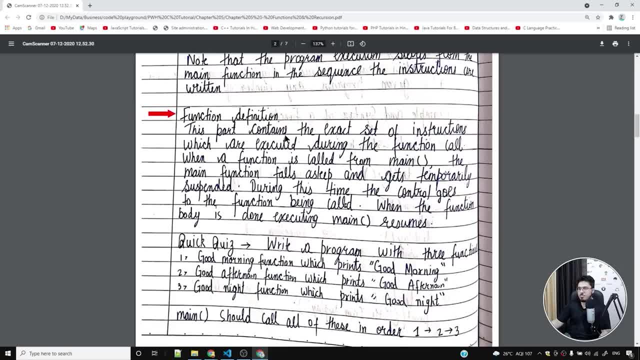 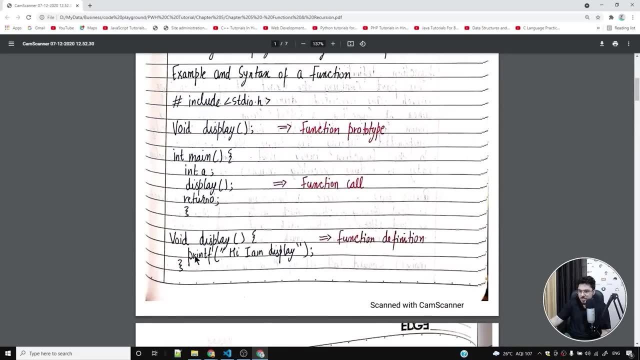 function will start executing now. function definition. this part contains the exact set of instructions which are executed during the function call. so whenever you call a function, you are definitely going to execute some set of instructions. what will be those set of instructions? those set of instructions are nothing but the lines which are written inside the function. 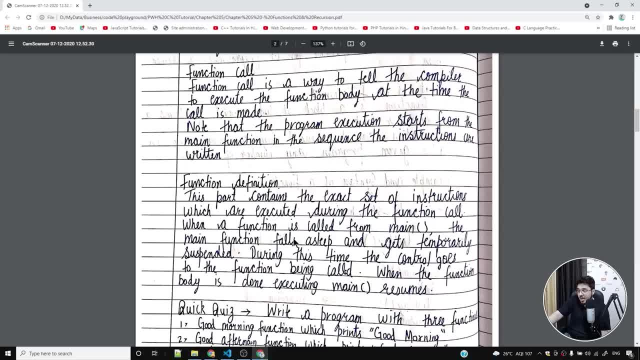 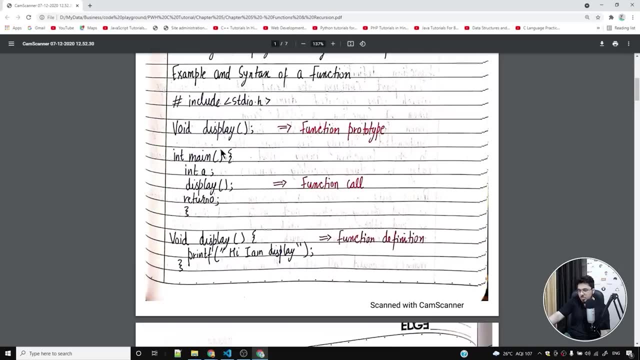 this is the function definition. it is also called function body, and this part contains the exact set of instructions which are executed during the function call. when a function is called from main, the main function falls asleep and gets temporarily suspended. so let me tell you what happens. so, whenever this program starts executing, what happens is- let me show you here, whenever- this: 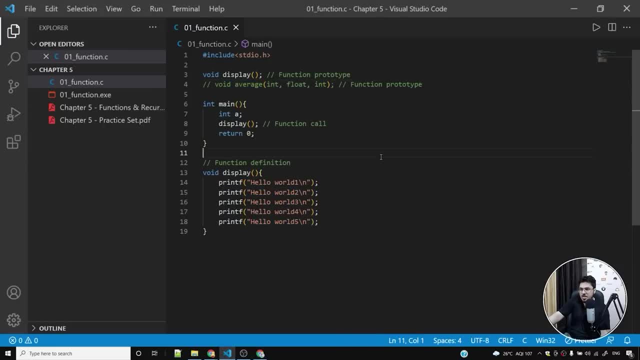 program starts executing. what happens is this line will be executed and whenever this line starts to execute, the main function will temporarily sleep. the main function will be given the instruction to sleep by the compiler. compiler will tell the main function that: hey, main function, please rest for some time. you need some rest. let display function do the job for some time and then we'll come back. 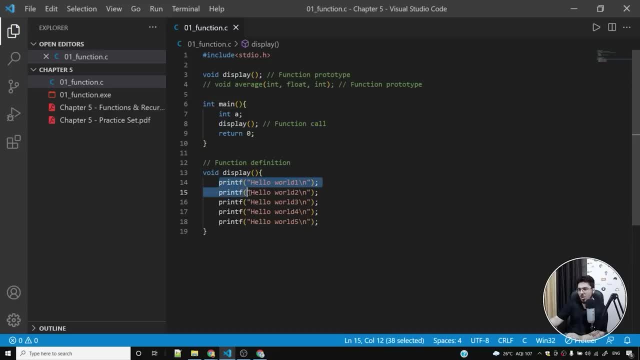 to you. so display function will be active and it will run all these instructions and the moment this display function stops executing, the control will come back to the main. so main function will be uh, awaked by the compiler. compiler will tell the main function: hey, main function, please wake up, you need to wake. 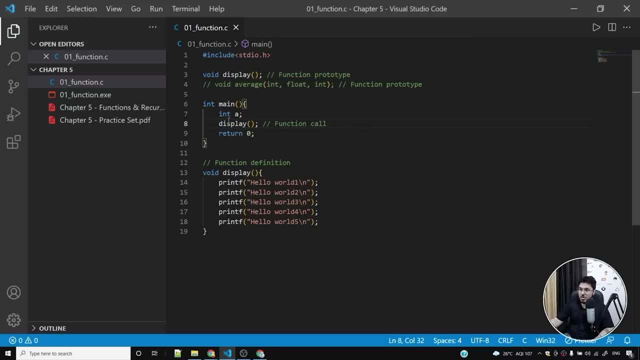 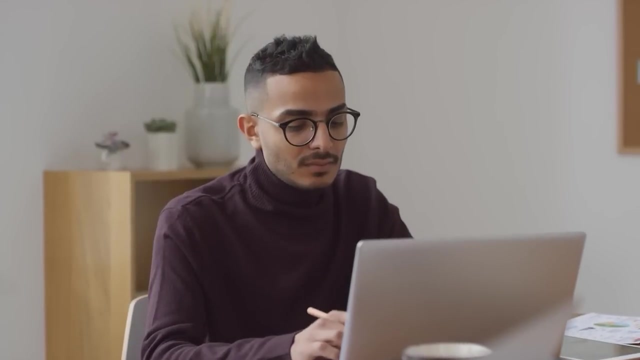 up and you need to start your execution and since the display call has already ended, this line will be executed and, finally, this body, or rather the main function, will stop its execution and hence the program will be terminated. I hope that you were able to understand how this function. 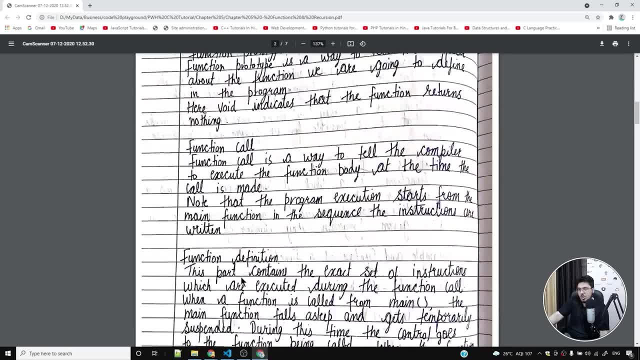 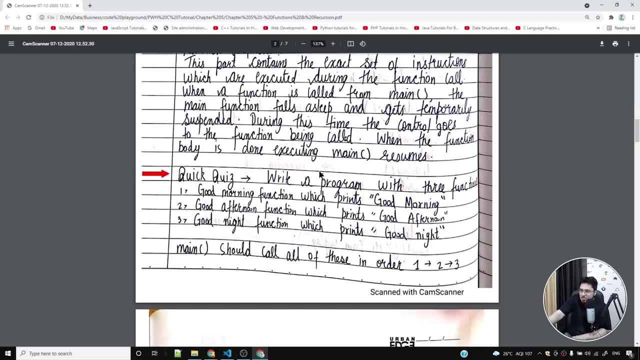 works. okay, coming back to the notes, we talked about function prototype. we talked about function call. we also talked about function definition. here is a quick quiz for you. you have to write a program with three functions. the first function is good morning function which prints good morning. second. 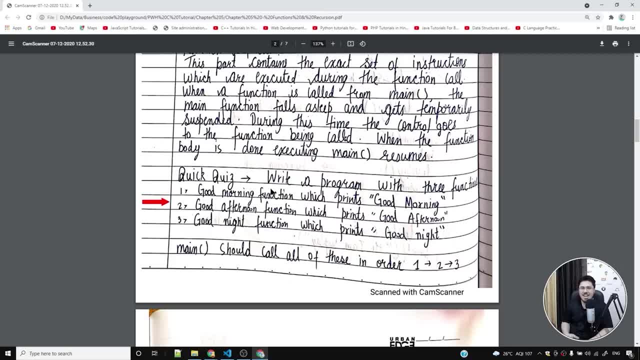 function is good afternoon, function which prints good afternoon, and the third one is good night. so let's see how we can solve these three problems. all you have to do is, uh, you have to write the body of these functions, and then there is something else which is given in the question, which is main. 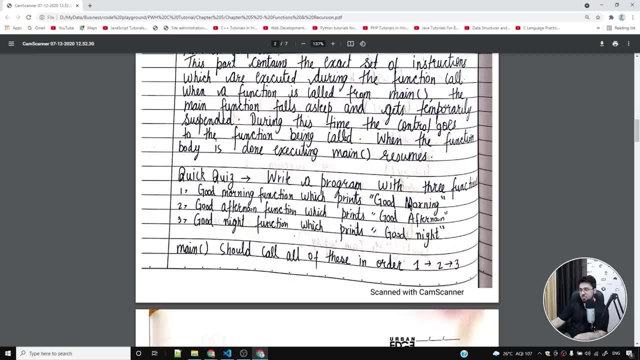 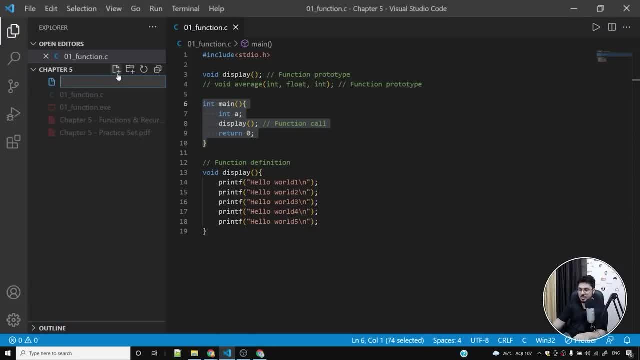 should call all of these functions in this order. so first one will be executed first, then second one will be executed, then the third one will be executed. so let's write this program. so what I'll do is I'll say: is we do two underscore, quick underscore, quiz dot C? and I'm going to write the. 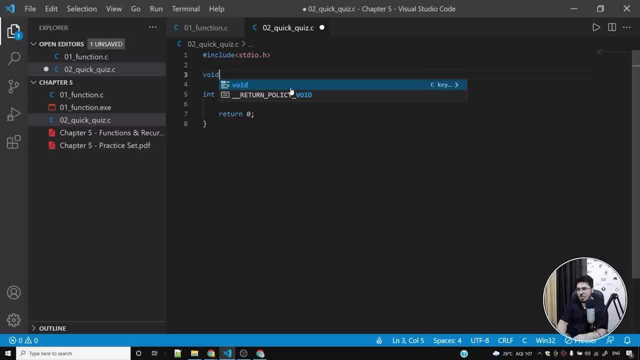 it. also, I'm going to write the function prototype, so I'll simply say void, uh, let me see the names of the function. so good morning, good afternoon. good morning is a function. good afternoon is going to be a function, good afternoon. and then good night is going to be a function. so good night is a 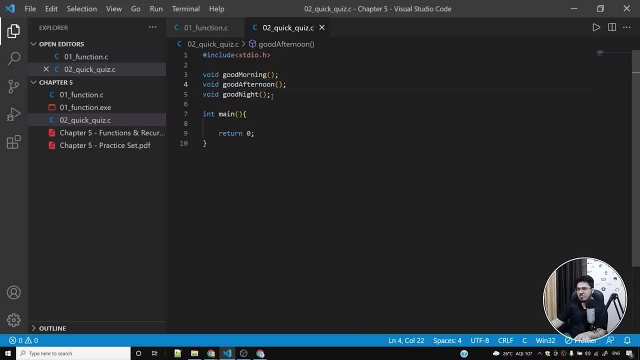 function. these three are functions. now I'm going to write the body of these functions, so what I'll do is I'll simply copy this, then I'll paste this and then I'll start writing printf, and what I'll say is: I'll say: good morning back. 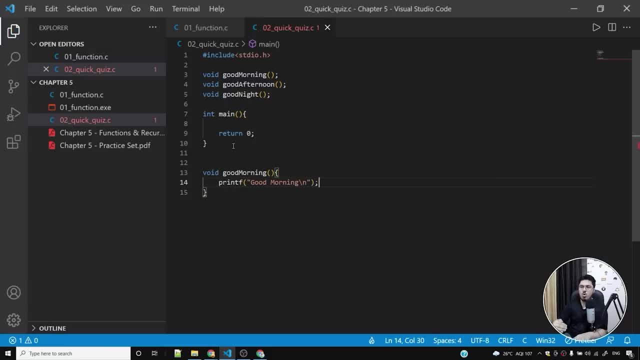 slash and backslash and simply means that I want to give a new line after this line is printed. so good morning will be printed, and then a new line will be printed, and what I'll do is I'll repeat the same thing for all these functions. so I'll write the same thing for good afternoon. I'll. 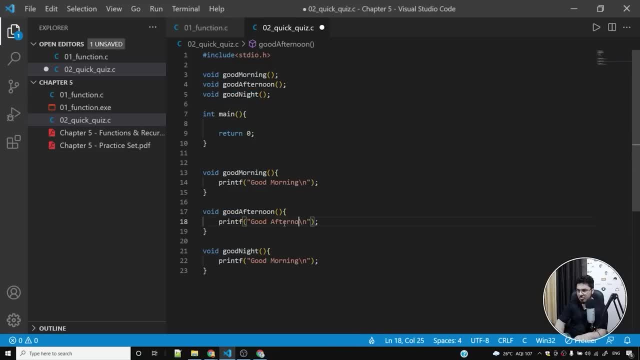 write the same thing for good night, so I'll say afternoon and I'll say night, okay. so good afternoon, good night, good morning, okay. so these three are the functions which we have written. let's execute them one by one. and in order to execute them one by one, 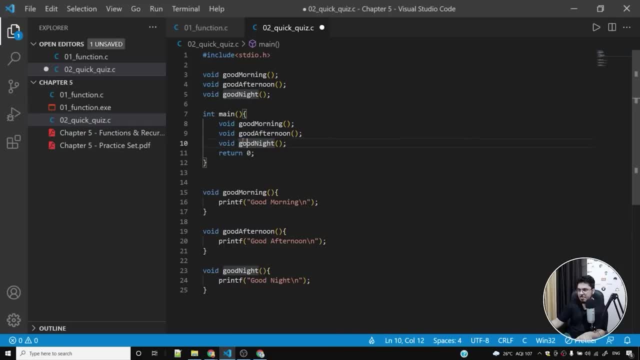 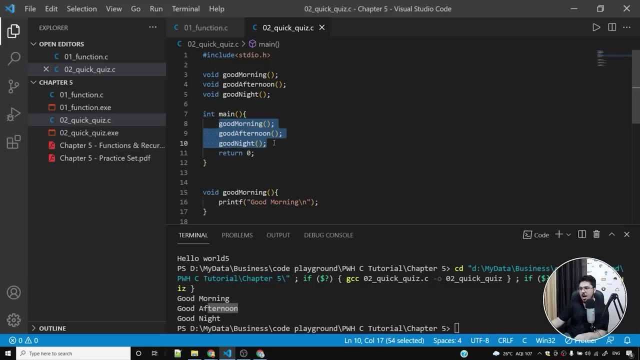 what I'll do is I'll copy this right here, I'll press the tab key now, I'll simply click here and I will remove this void. I'll save the program. let me run this. good morning, good afternoon, good night. so these three functions are hence executed in order. okay, I hope that this explains the concept of functions and you. 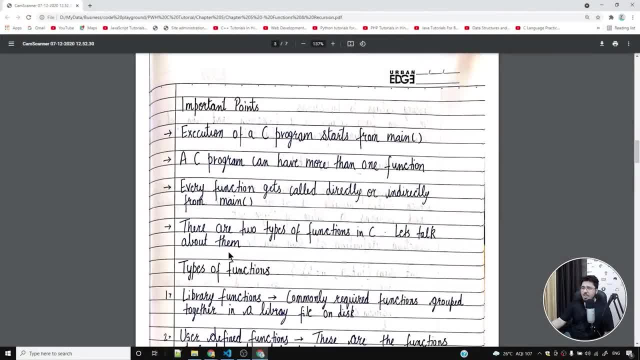 were able to understand what function definition, call and prototype is. now I have jotted down some important points for you, which are really very important because you would want to know about how to use, and when to use functions in C. so execution of a C program always starts from main. 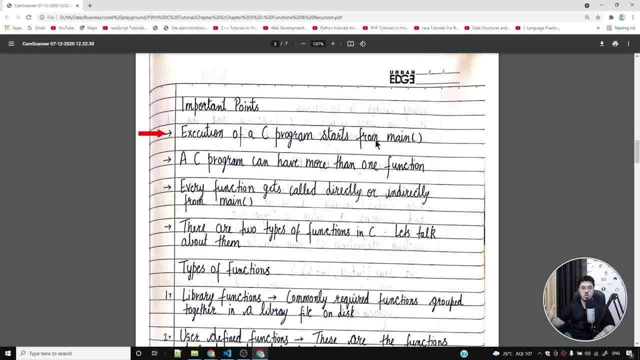 never think that any function which is at the top will be executed first. no, that's not going to happen. always and always, the C compiler will start looking for the main function first and it will execute it first. so execution of a C program starts from the main function. main function is the function which 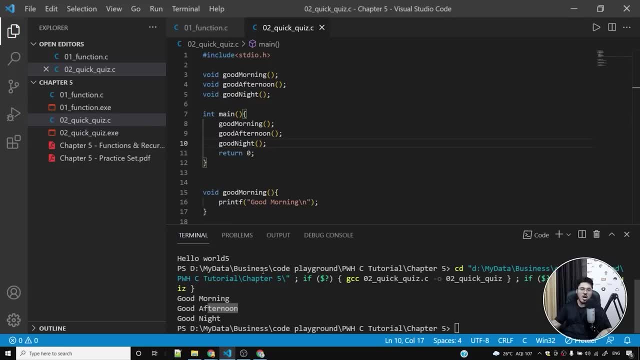 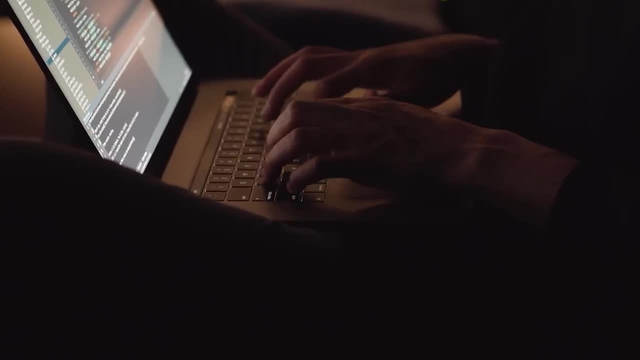 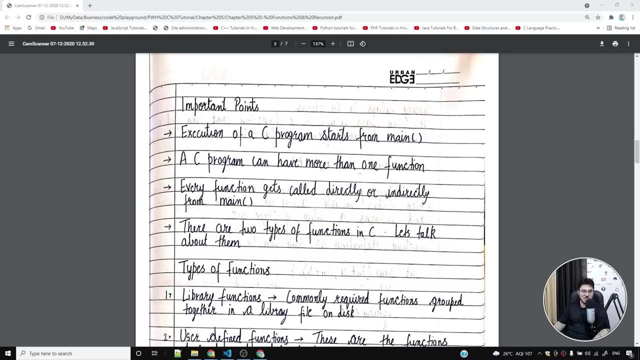 is actually executed as soon as the program starts executing. okay, we have some more important points. every function gets called directly or indirectly from main. so whenever you run a C program, main is a function which will start executing first. so naturally, any function which gets executed will directly or indirectly be called from main. so there are two types of functions in C. we'll talk. 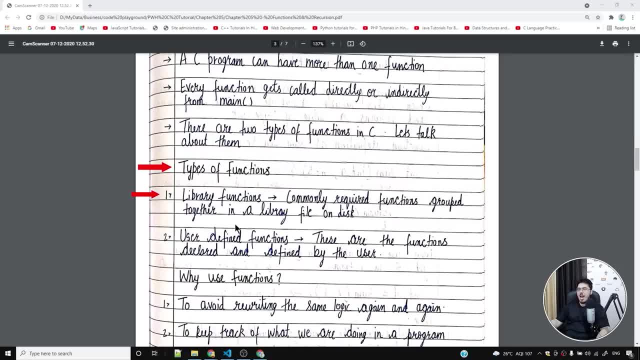 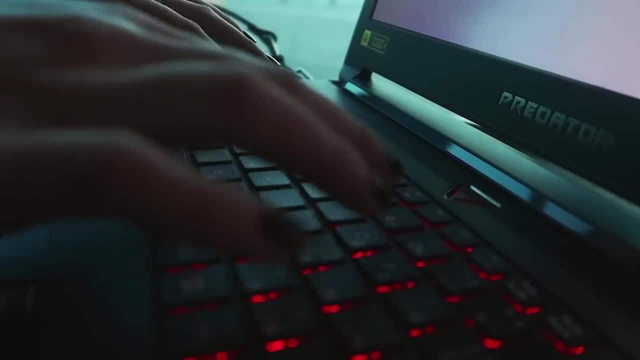 about them. there are two kinds of functions. the first one is library functions and the other one is user defined function. what is the library function? commonly required functions grouped together in a library file on disk. so library function is something that C programming library already has to offer you. you don't have to write the logic of those functions. what is user defined? 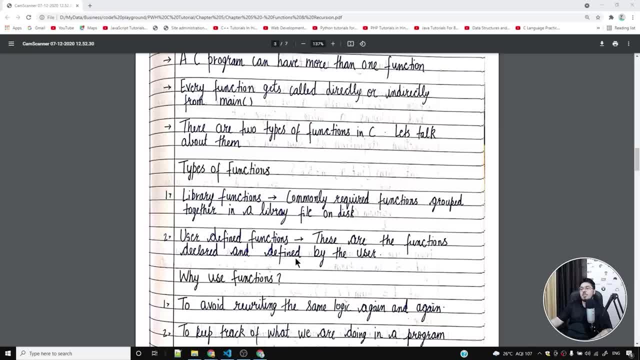 function. user defined function is a function which is declared and defined by the user. so if I want to write a custom function to calculate the number of shipments in my, uh say, courier company, I will have to write that function. nobody is going to provide me that. let us say I am going to, you know. 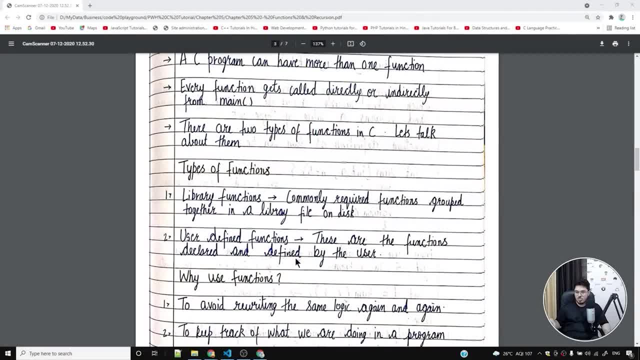 start making cell phones from tomorrow and I have to write a function which is going to tell me that how much money I am making per cell phone, per single sale of cell phone is making me, say, 10 rupees. I want to write a function which can look into the different parameters and 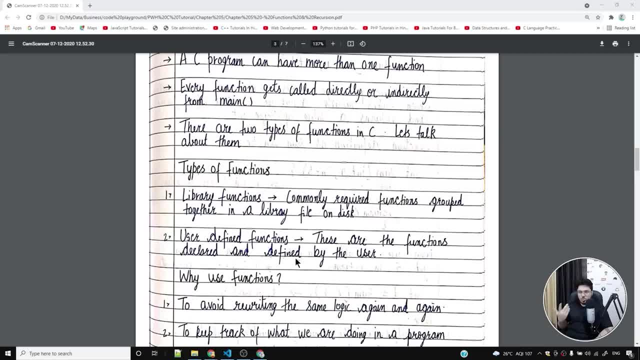 automatically calculate this number for me. I will have to write this function, so it has to be a user defined function. I cannot expect a C compiler to ship with this function. naturally I'll have to write it. so these are the functions which are custom, and they are custom tailored for your needs. so 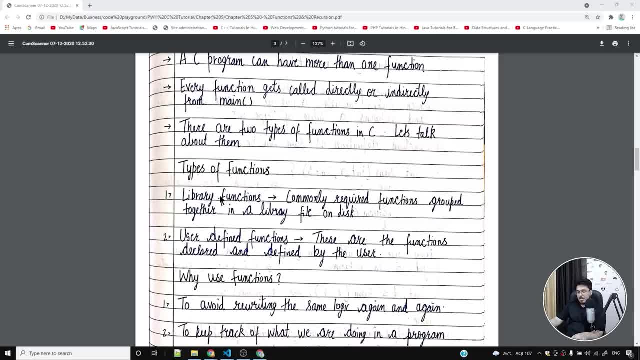 you'll have to write those. but there are some of the functions which you might need. for example, there is a function called pow- we have talked about power- which is used to raise a number to the power of another number. so these kinds of functions are library functions and these are readily available. 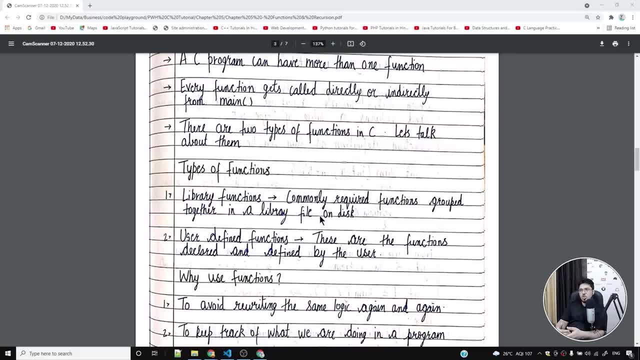 inside a library file. you might also want to talk about averaging three numbers inside your program, and if you want to average three numbers you might get a library function for that inside your program. let us say you want to sum 10 numbers. you want to find the sum of 10 numbers. 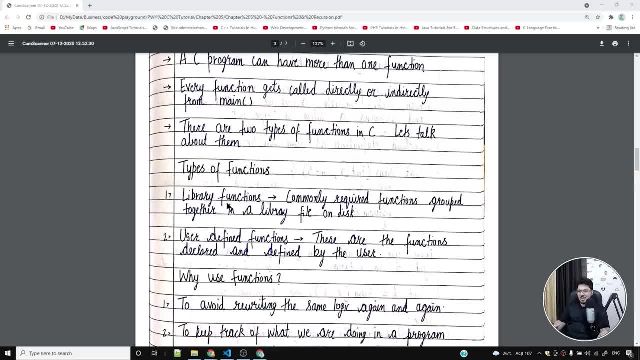 you might get library function for that. so anything that is not specific to your needs, anything that is very generic, you will get it in the library function. some or the other library will give you that function. we'll talk about some of the library functions later in this course, but uh, we. 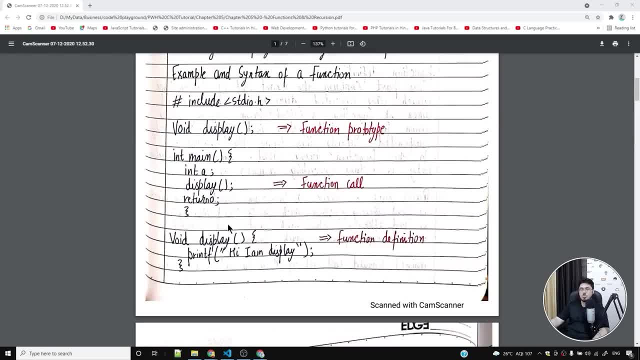 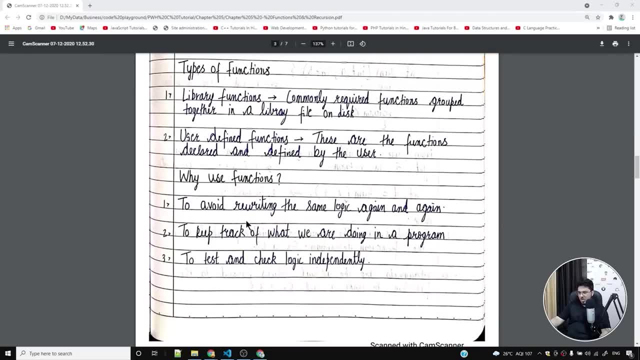 talked about user defined functions. in fact, our display function was a user defined function, so this is about user defined functions and library functions. I hope you were able to understand what these are. now we'll talk about why we need to use functions. why use functions to avoid rewriting the 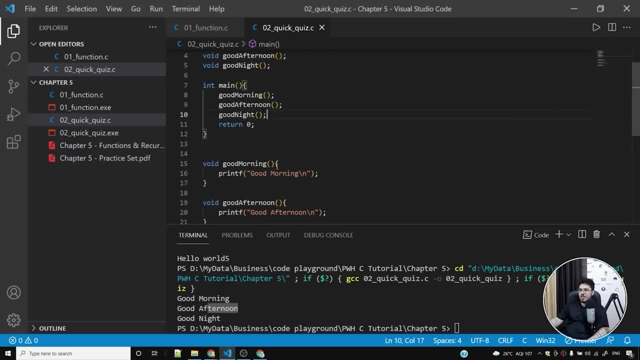 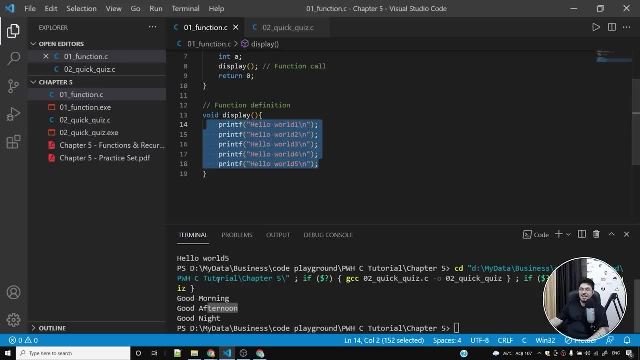 same logic again and again. so let us say I want to print good morning. or let me come back to this one. let us say I want to print this particular pattern: hello world one, hello world two, hello world three, four and five. let us say I want to. 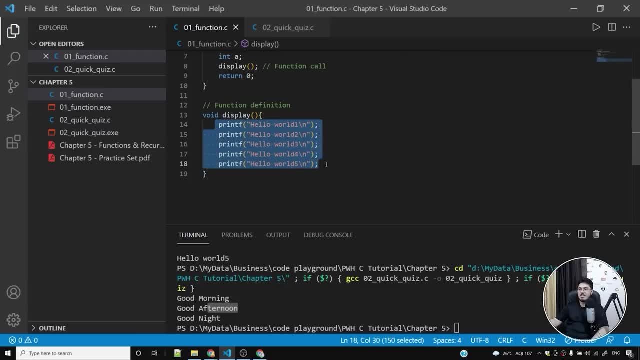 print this 10 times, so I don't have to copy these five lines and copy them again 10 times, making them 50 lines. I can actually do this by simply copying this any number of times I want it to execute. so if I wanted to execute 10 times, I can copy this particular line 10 times. 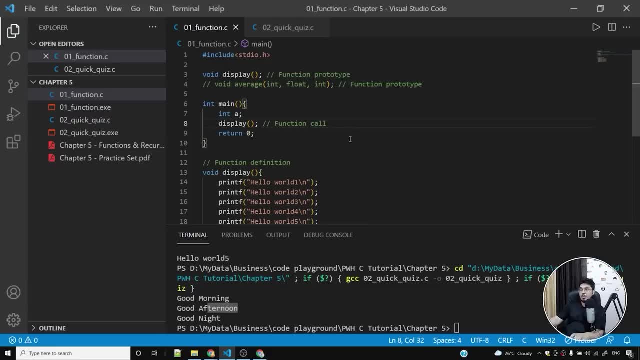 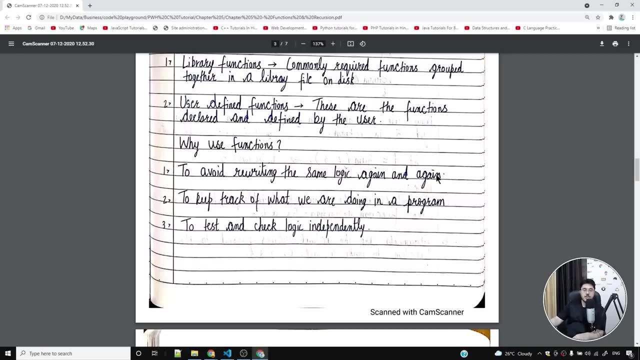 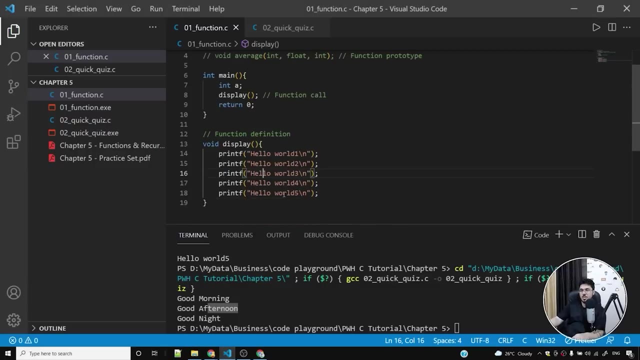 I hope that you are able to understand this, and I hope that you are able to see what I mean by uh, by saying that you will avoid rewriting the same logic again and again if you use functions. functions will also help you keep track of what you are doing in a program. so if we have our logic divided into, 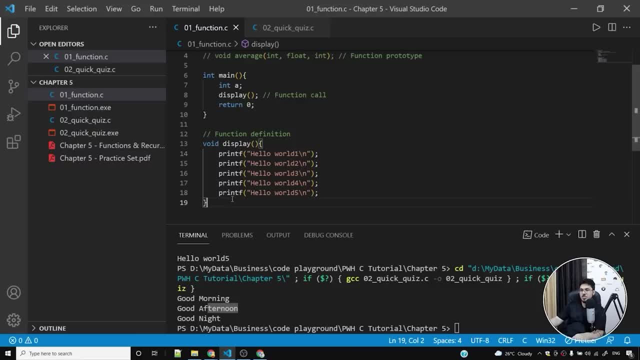 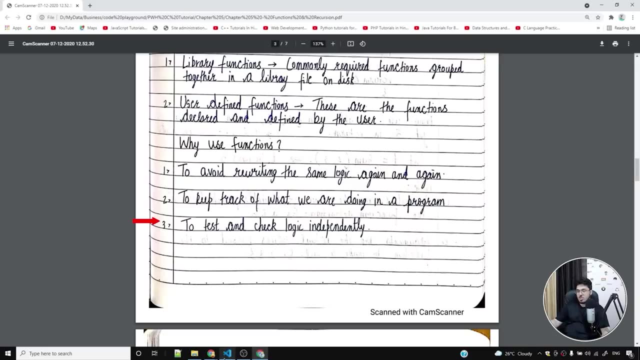 different functions. we can focus on one function and start debugging that function if that function is not performing as usual. the third thing is to test and check logic independently so I can actually have, say, a person called Rohan Das write this function and a person called Jacob write another. 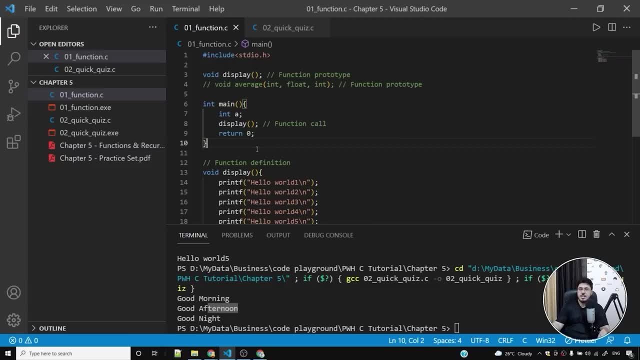 function and a and a person called, say, Sonali write another function, and these three people can work independently on three different functions and what I will give them is a function prototype. I'll tell them that I want this particular return value from my function and I want to give these. 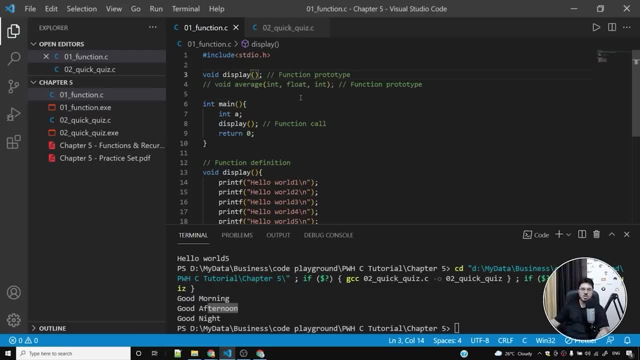 two or these three or these four values as an input to this function and those people will have that will be written inside the body of this function, if that makes sense. I hope that you were able to understand this. now we'll talk about passing values to the functions. passing values to: 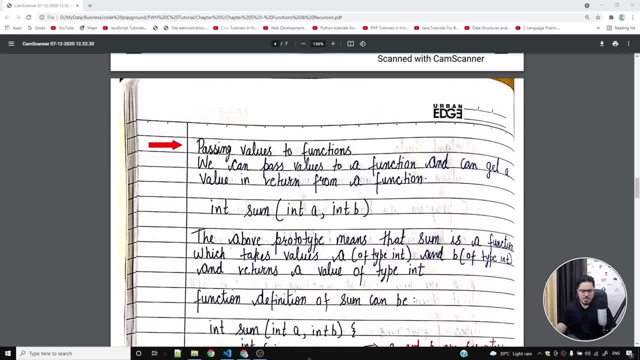 functions is something that you will definitely want to learn. what does it mean? it simply means that there is a function. it takes some values as an input and gives an output. you need to receive output by giving some inputs and you will definitely want to use a function like some where. 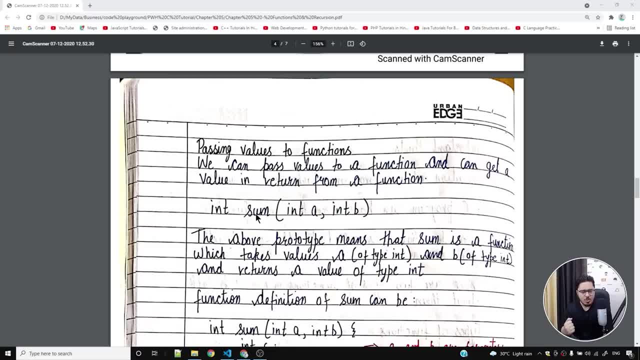 you are supplying two input values and you are expecting an output value from your function. let's see how these things work. we can pass values to a function and we can get a value in return from a function. for example, let us say sum is a function and we have two values which we are supplying to. 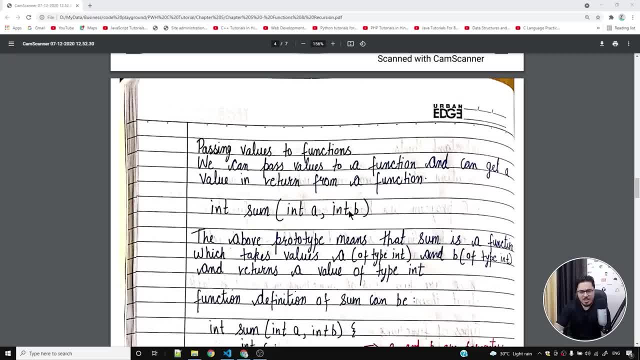 sum as an input. what are those two values? those two values are a and b. if these values are three and four, I will expect my sum to return an integer which is nothing but seven, because three plus four is seven. similarly, if a is five and b is three, I I would expect this sum to give me eight in return. 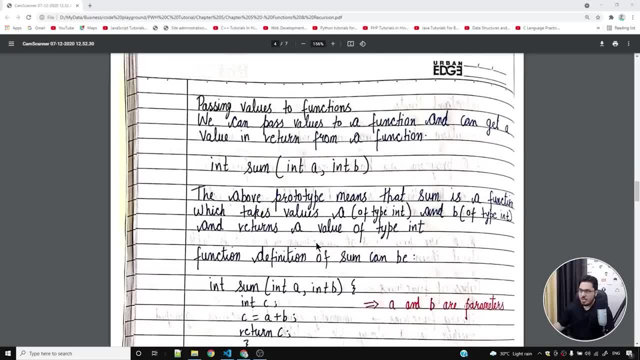 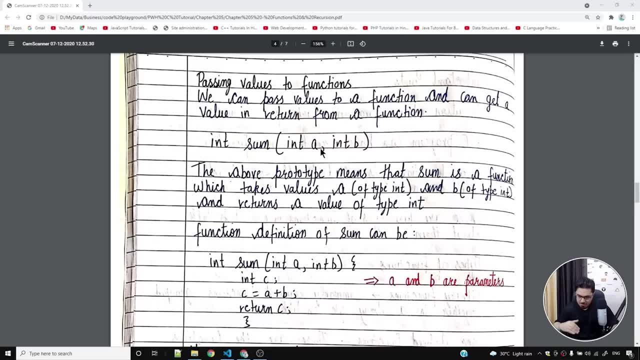 because some of these two numbers is eight. now the above prototype means that sum is a function which takes values a and b of type int. so a is an integer, b is an integer and whatever I'm getting in return is an integer. now it is not necessary that if you're supplying integers you will get an integer. you might get a float as well. 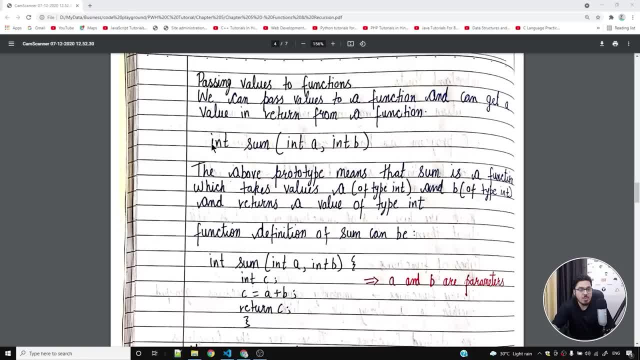 for example, in case of a function which calculates average of two numbers, you might expect a float or subtractingigen that. but no, it's ok, because may be eso. maybe in g and b it won't be. it can be l, because in g use U, it's ok, but in g it has three. salute its insunet in to its input. so 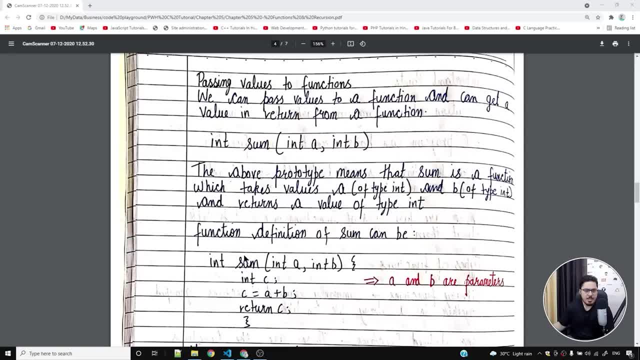 supposing that I'm giving a and B, which are integers, and I am expecting an output which is an integer. ok, so this will return a value which is of type int, so'samblerter the value of typing. now function definition of some can be something like this. so i'll say something like this, I'll say in: 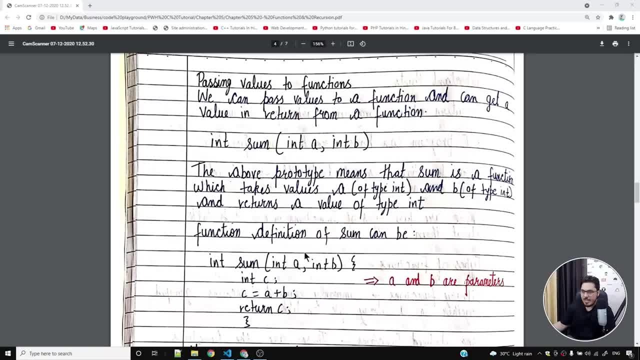 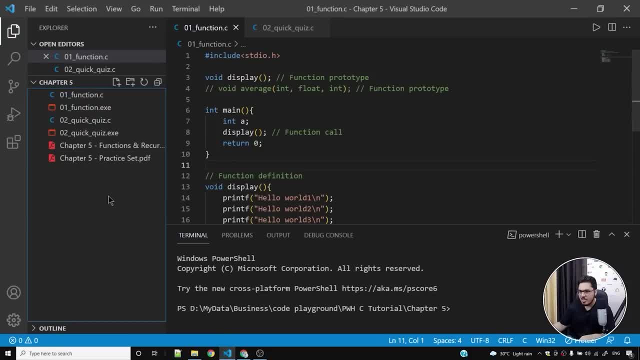 sum in of sum a minus i plus b and b are input tosum called parameters. i'm supplying a and b to sum and i'm expecting a value c which is calculated by this function sum. let's see how this thing works. what i'll do is i'll simply say passing. 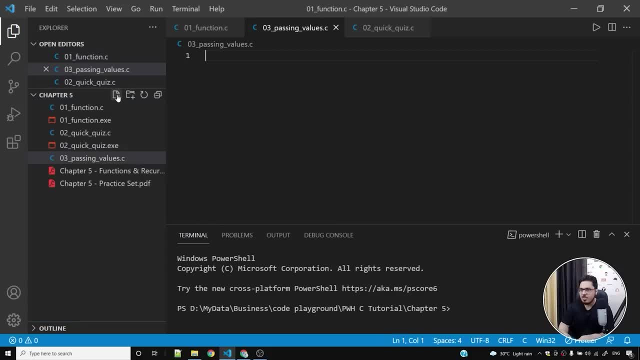 underscore values, dot c. i'll add a boilerplate template. and let me do one thing. i'll simply, you know, copy a function prototype from here, or let me write it. write it down once again. i'll simply say: sum, int, int. so what this means is that sum is a function. it returns an integer and takes 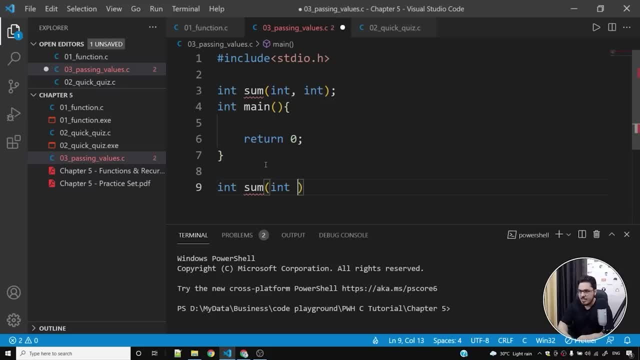 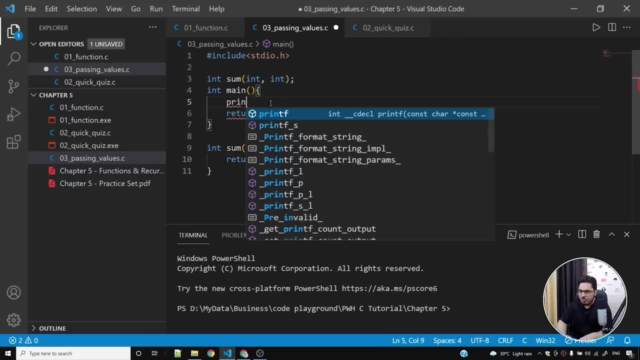 two integers. now i'll write the body of sum. i'll simply say int a, int b. sum is a function which takes a and b as an input. and what does it return? it returns a plus b. so we don't even need a variable c, we can simply say return a plus b and this will take care of everything. now, if i do, 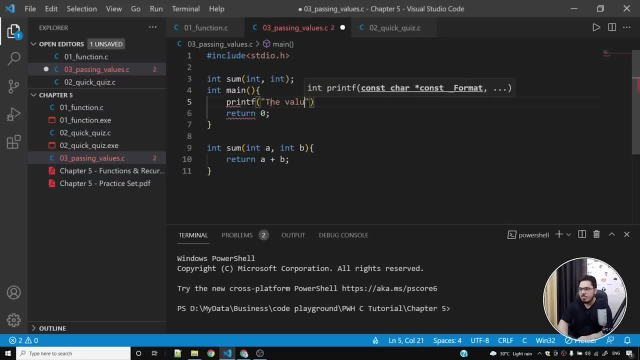 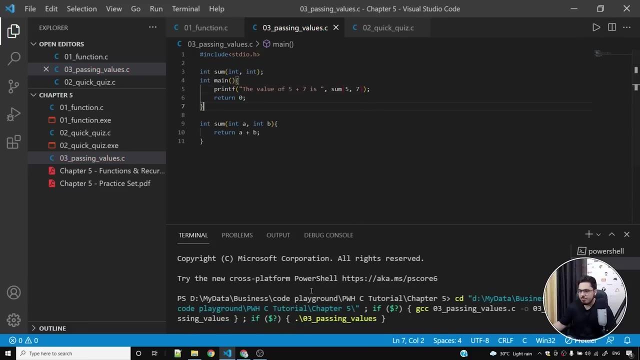 something like this and i say the value of four, five plus seven is. i can do something like this. i can say: sum five comma seven and this will actually calculate this five plus seven for me and it will print 12 for me. so five plus seven is i. 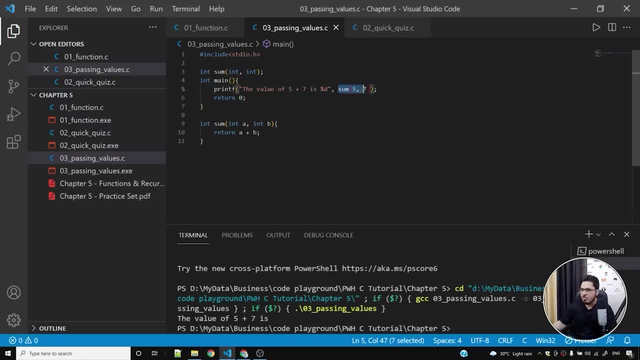 should have written percentage d, my bad. so this value will actually come here, so it will return b to l. let me show you: the value of five plus seven is 12. how does all these things work? so the execution of a program always starts from the main function. 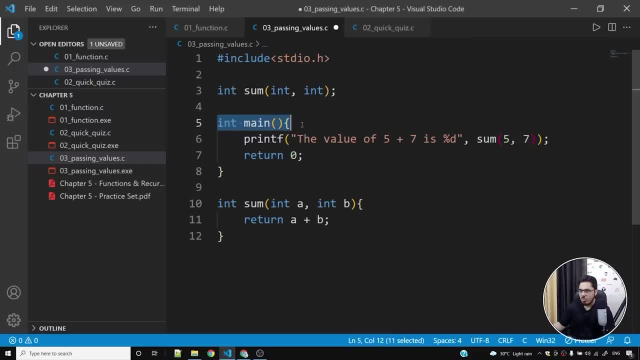 so when we are starting the program, we'll start it from here. this line will be the first line to get executed. but while this line is being executed, we'll encounter another function call. so what will happen is main call will be suspended. compiler will tell main: hey, main, you were executing, but 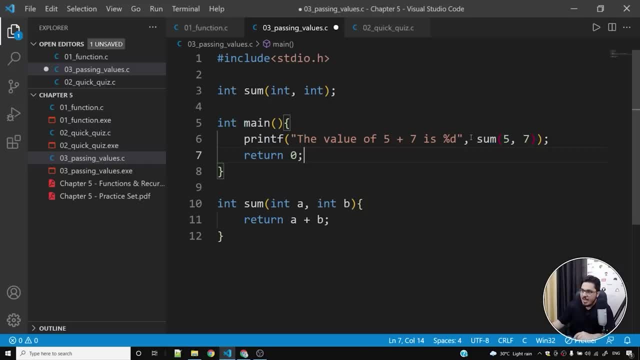 i want you to wait for some time, because now sum is executing and let sum bring its value. and once sum brings its value, we are going to put that value here and we are going to then continue your execution. then execution of the main function will continue. so what happens is this function, the main function, will get suspended for some time. 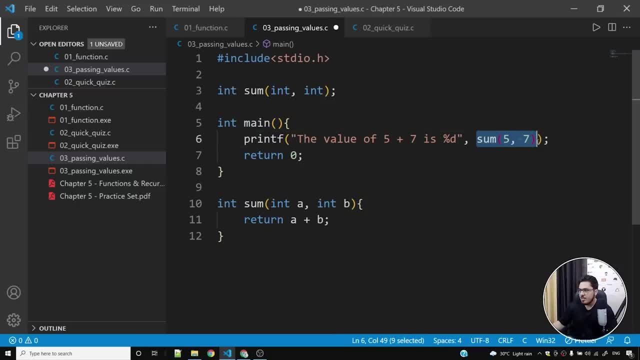 and some function will start to execute. i'm talking about this sum function. this function will start to execute and what happens is this calculates the value a plus b and it returns value twelve. so twelve is returned back to the main function. so So this can be replaced with 12.. 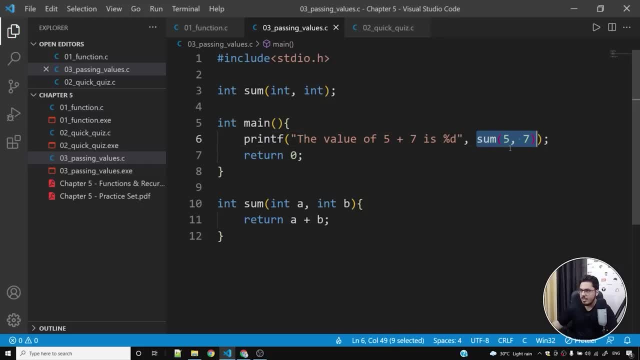 So I can do something like this. I mean in my mind, obviously in the program. we are not going to change the program, But during the execution what happens is this value is replaced by 12.. And what? what will this line print then? this will print: the value of five plus seven is. 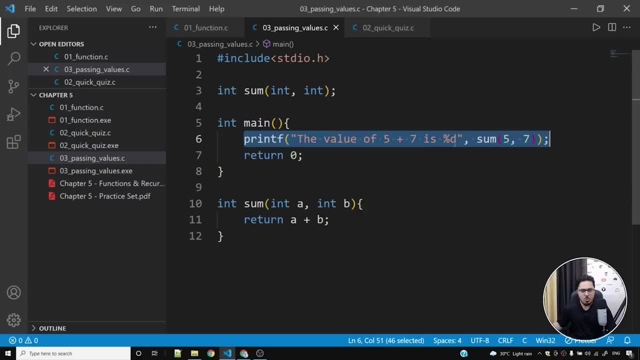 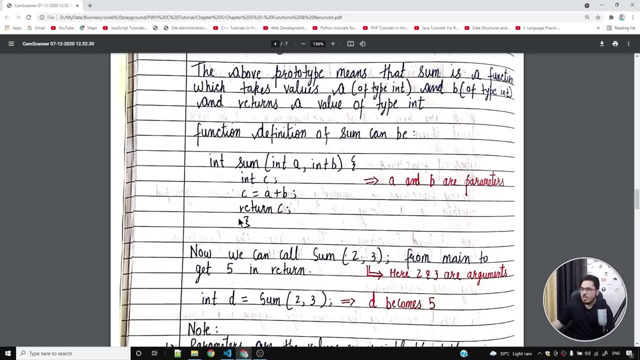 12.. So percentage t will be replaced by 12.. I hope you got the point. I hope you understood how we can pass values to a function and we can expect the value in return from the function. Now we can call sum two, three from mean to get five in return. 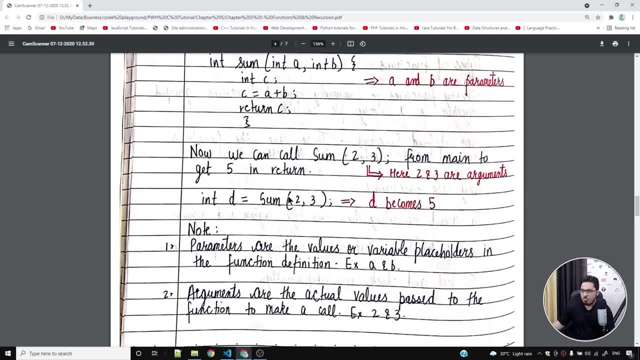 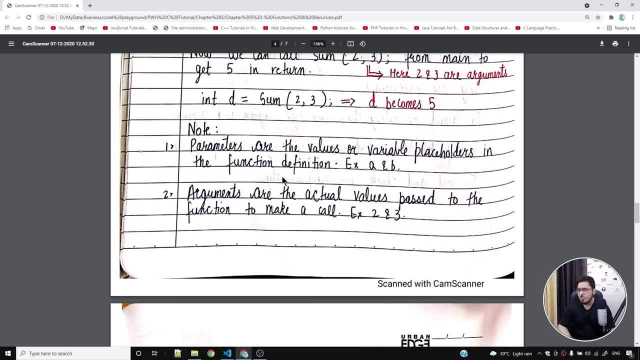 So if you say in D is equal to sum two comma three, sum two comma three will return five and D will become five, because this value will be replaced by five. I've written some notes here. So the note number one says parameters are the values or variable placeholders in the 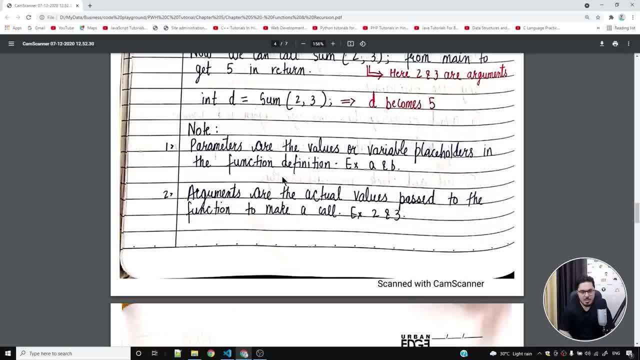 function definition, for example A and B. So parameters are nothing but values or variable placeholders. What are values and what are variable placeholders? Values can be two, three or something. It can also be a variable placeholder. For example, I can do something like this: 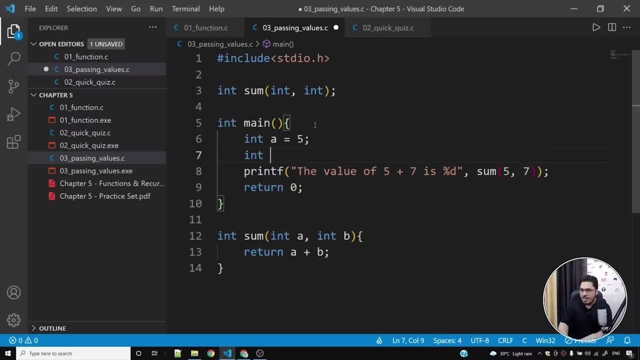 I can say int A is equal to five and int B is equal to seven, And I can actually say sum A comma B. that will also do. that is also valid. So A is five, B is seven. So this thing remains unchanged. the output will be the same. 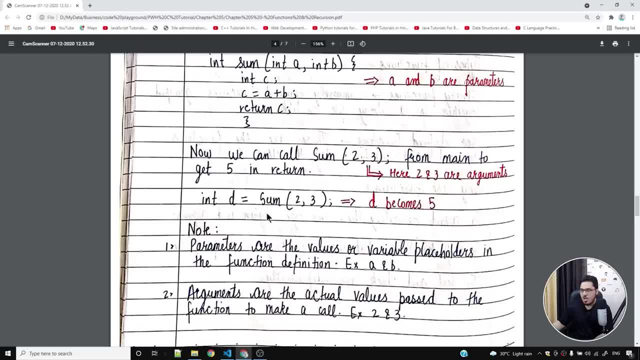 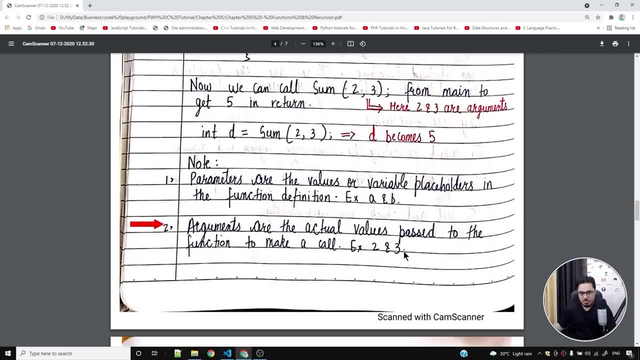 But just in case you want to use variables, you can always do that, Okay. The next thing is that arguments are the actual values passed to the function to make a call, for example, two and three. Okay, so I want you to understand the difference between parameters and arguments. 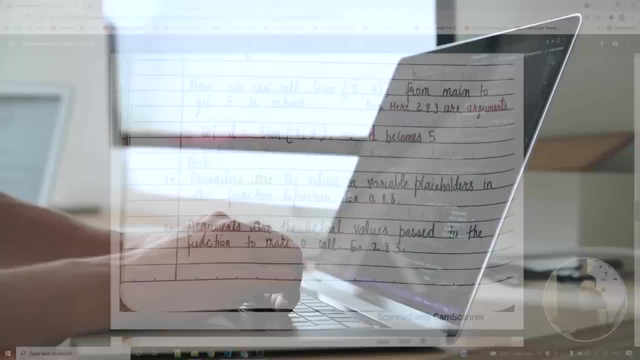 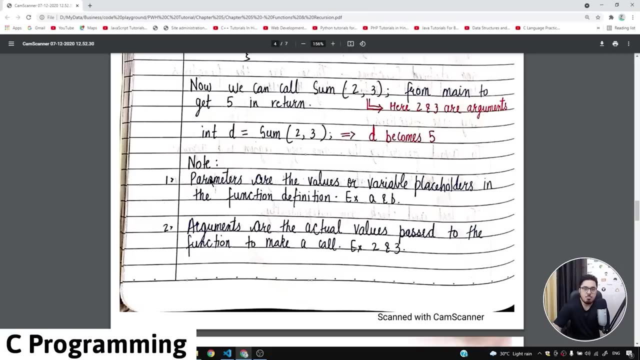 Now let me tell you one thing: If you are talking about code and programming or C programming with somebody, they might interchangeably use parameters and arguments, But again, you should know the core, key difference between parameters and arguments. What is the difference between parameters and arguments? 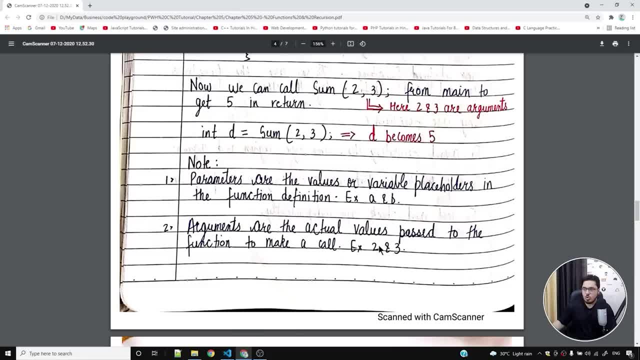 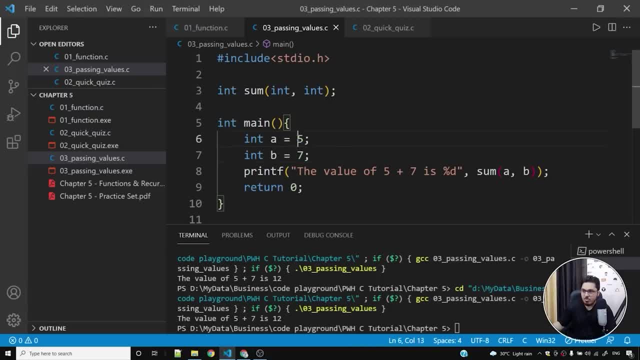 I'll tell you using An example. Okay, So two and three are the actual values which are being passed. So which values are passed? five and seven are passed, So five is an argument. seven is an argument in this case. okay, 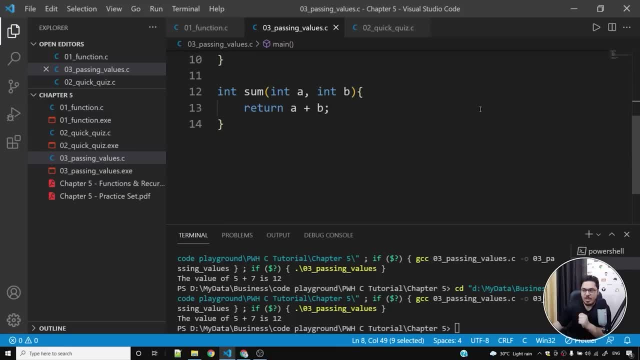 So actual values which are passed to the function are arguments. But what are parameters? A and B are parameters. So if I talk about this function, A and B are parameters for this function. But if I talk about this function, call A and B, or rather five and seven are the arguments. 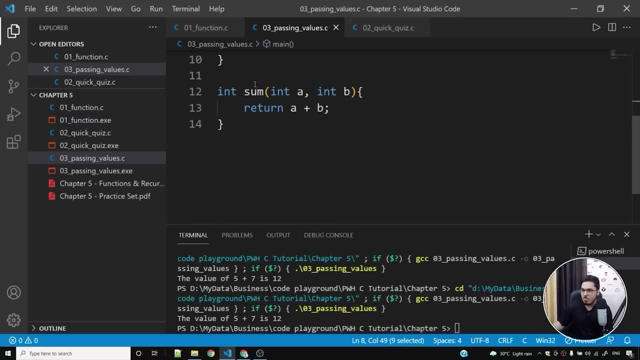 So when I'm looking here, I'll use the word argument- A and B are arguments- But when I'm looking here at the function body, I'll use the word parameter. Now again, nobody's going to ask you this question until and unless you are sitting. 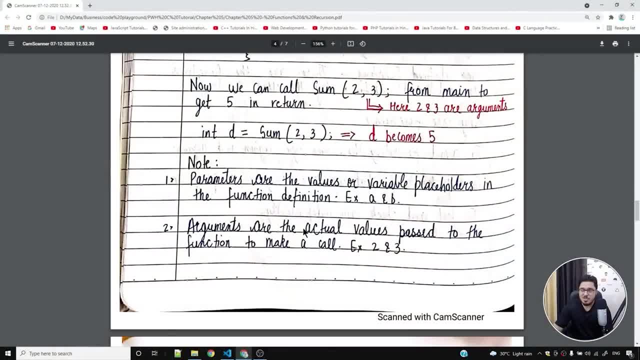 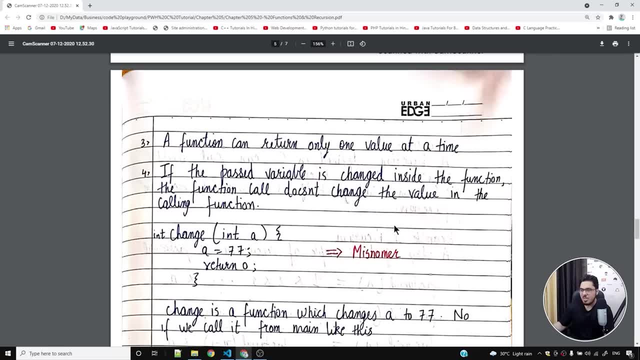 in some interview and your interviewer really take some interest in this question. But just in case you wanted to know the difference between parameters and arguments, this is the real difference and you should definitely know it. The third point says that function can return only one value at a time. 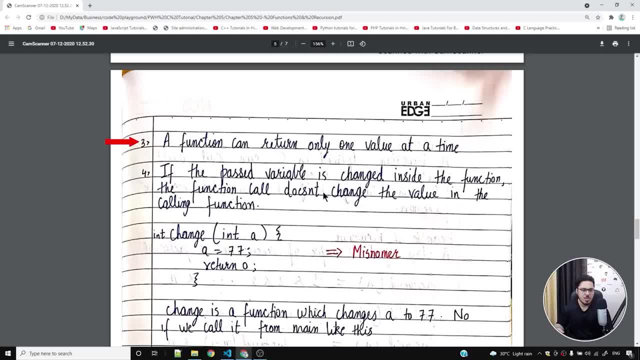 So one function can return only one value at a time. in C language, This is something that you should know. If the variable is changed inside the function, the function call doesn't change the value in the calling function. What does this mean? Let me give you an example. 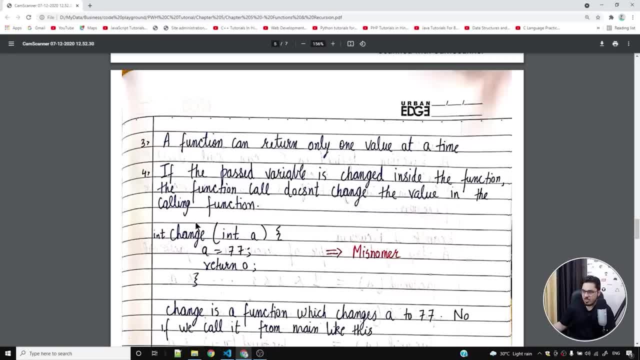 Okay, Now if the past variable is changed inside the function- for example, I have a function called change and I change- this value is equal to 77.. No, this will not change the value in the mean. Let me give you an example. 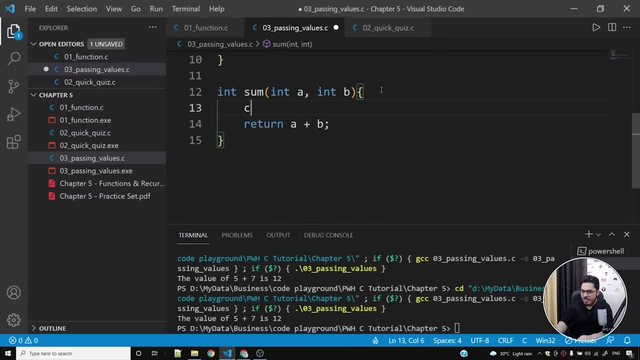 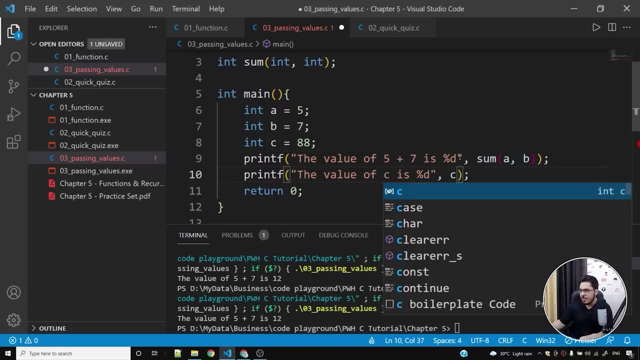 If I say something like this, oops, if I, if I say something like this, C is equal to nine And if I have int, C is equal to 88 here, and if I print, the value of C is: and let me print. 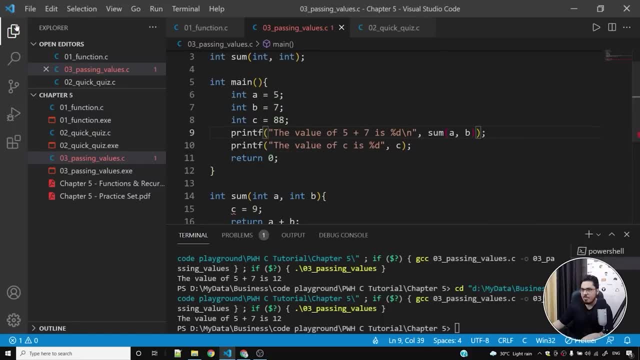 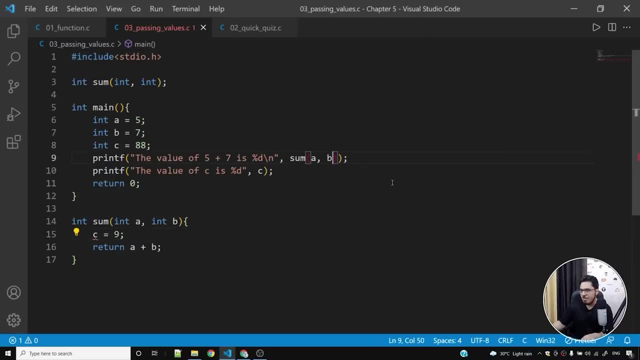 the value of C. also, I'll put a backslash and just so that my code looks good, If I run this, or let me even pass C, I know I don't have to pass C, but again I'm passing C. 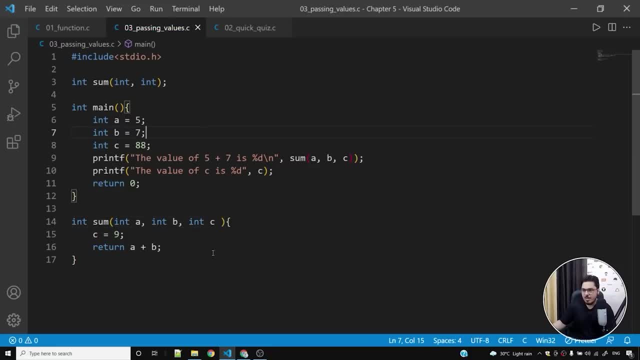 Let me pass C and C, but I'm only operating on A. Now let us say I am changing the value of C inside this function. I'm making it nine from 88.. What will be printed? Nine will be printed or 88 will be printed. 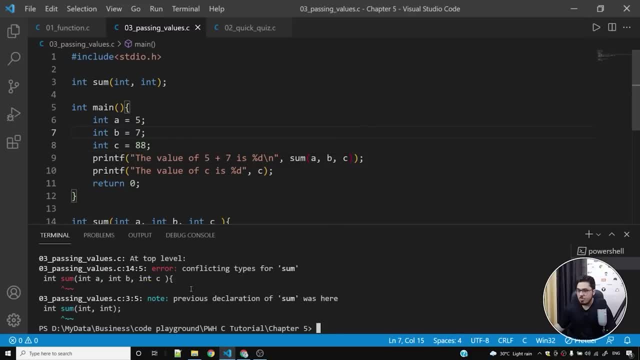 The answer is 88 will be printed. Let me run this program for you. Okay, So I need to change this function prototype as well, because I have two integers here. I need to make it three integers. Now. the value of C, uh, five plus seven is 12 and the value of C is 88.. 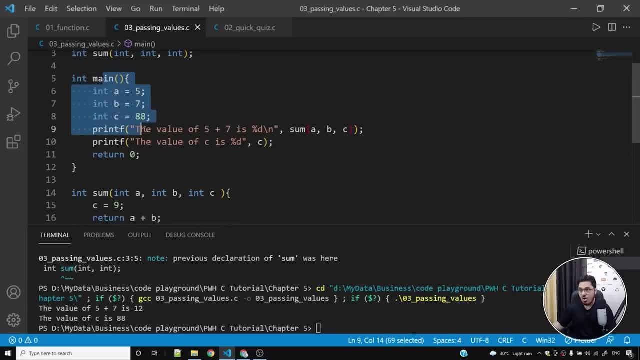 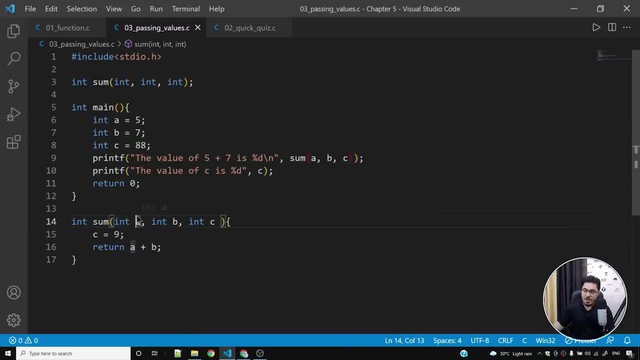 So we are not able to change the value- Okay- Of the main function inside the sum function. So this is something that you need to keep in your mind. This is really very important. And why does this happen? Whenever a function executes, it has its own set of variables. 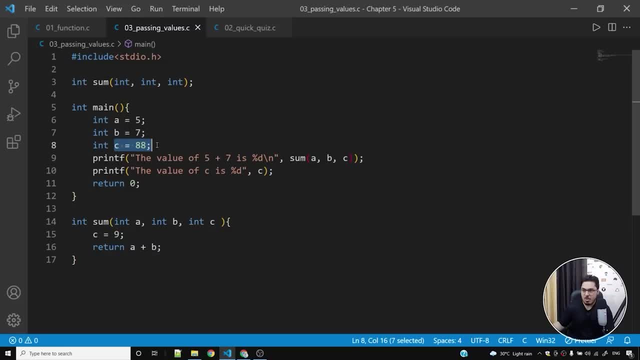 So A belongs to the main function. B belongs to the main function. C belongs to the main function. Now, once again, inside the sum function, this C belongs to the sum function. So this is maintained separately from this C. So this is a C of main function. 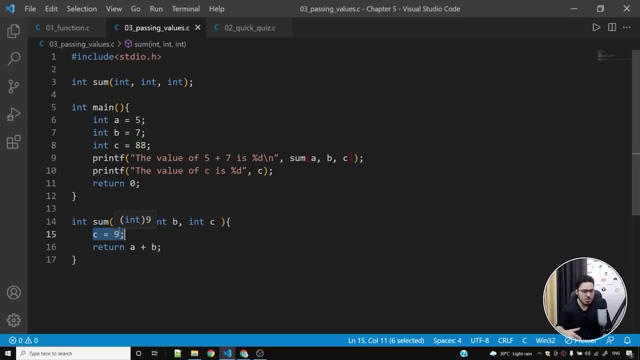 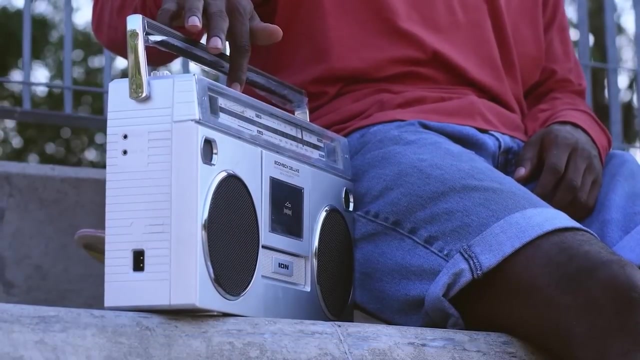 This is a C of sum function, So we also call these values as local variables. So these are local variables of sum and this is a property of mean. So we cannot change the property of mean from sum, Just like you cannot change- uh change- the volume of the radio of your neighbor sitting. 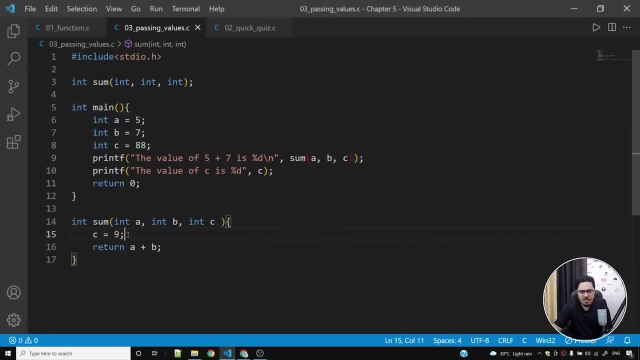 at your home, If that makes sense. You cannot do that Definitely. If he gives you the knob you can change. If, if he, you know uh, ties a thread to the knob and, you know, throws at your house. 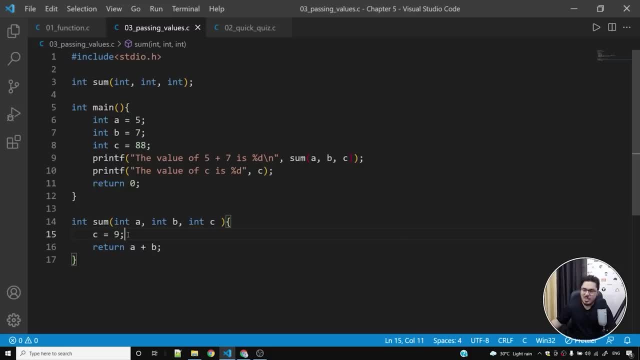 and you can pull the knob Somehow, Then definitely you can change. But again, directly you cannot change, merely sitting at your room You cannot change the TV channel of your neighbor. So this is maintained differently: Your TV is different, Your neighbor's TV is different. 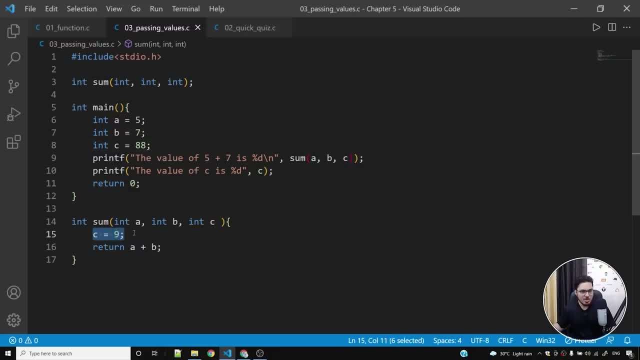 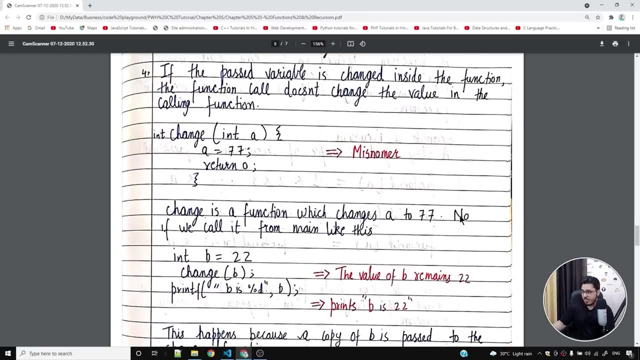 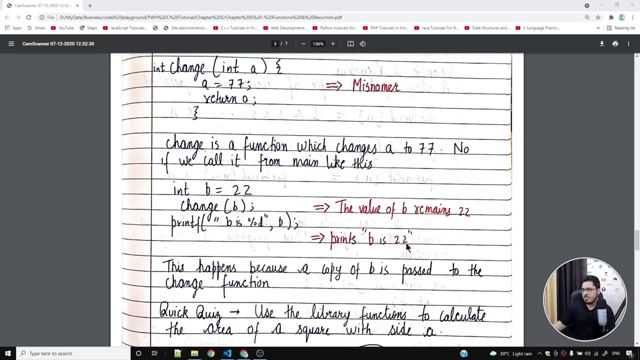 You cannot change your neighbor's channel by using your remote on your TV. Okay, I've given enough analogies and I've also written this in the notes. Changes: a function with changes A to 77.. Now, it should be now. now, if we call it from mean like this, then, uh, this will print. 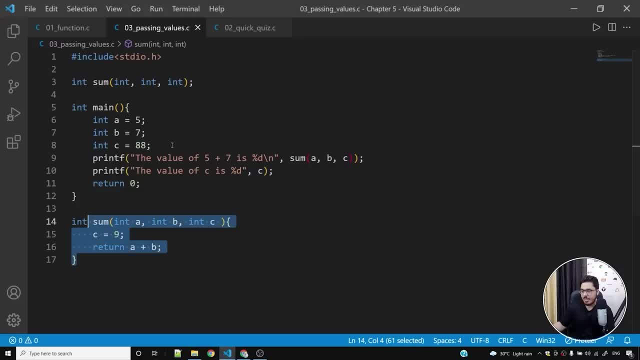 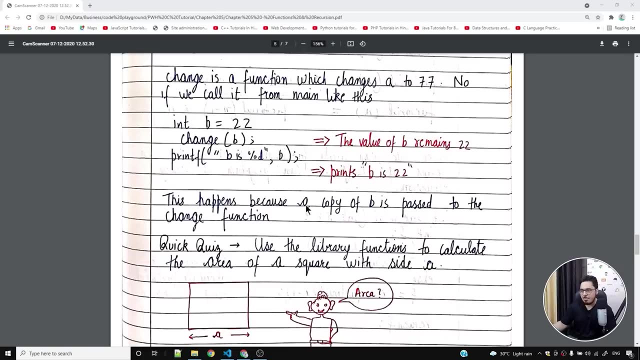 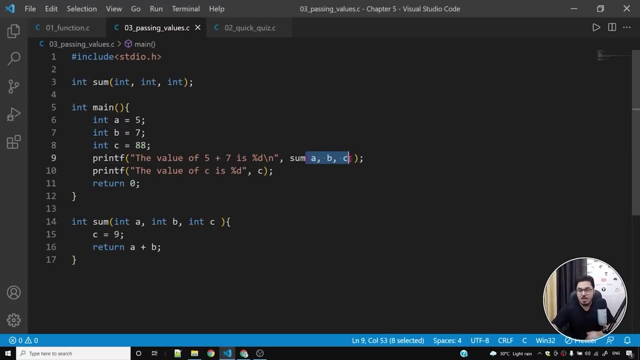 the value 22.. So we cannot change the value. Just like we saw an example here, we cannot change the value of main function variable from some other function. This happens because a copy of B is passed to the change function. So what happens is the these ABNC are not directly passed to some the copy of these. 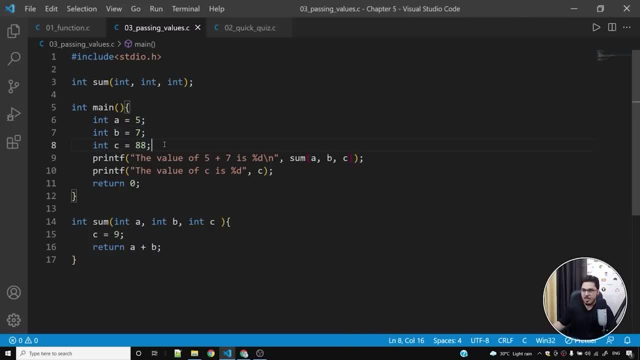 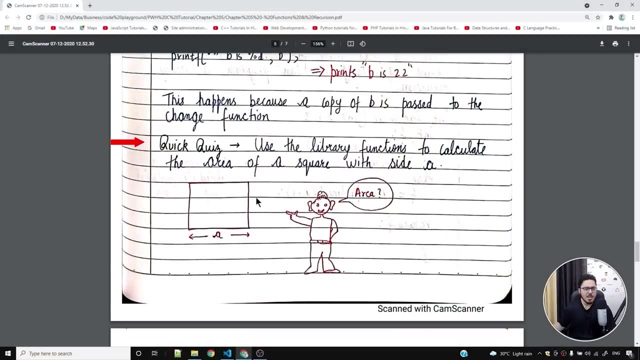 variables is passed to some. So this, this and this will remain unchanged if you're trying to change it from the sum function, Okay, So this is something that you need to keep in your mind. Now Let's do a quick quiz here. 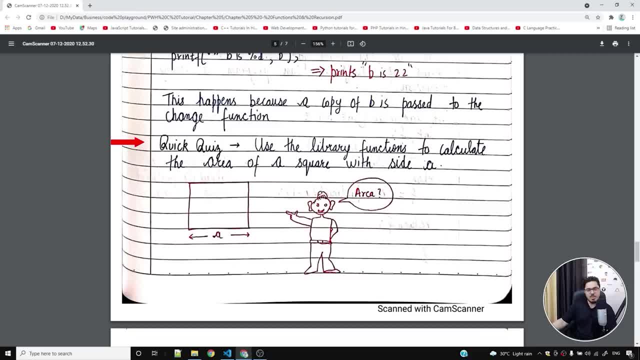 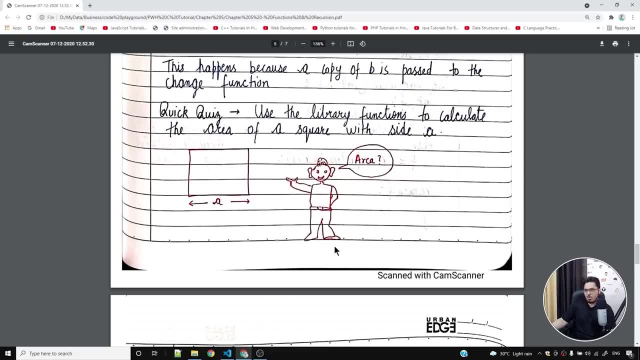 Use the library functions to calculate the area of a square with side a. So we need to use some library function to calculate the area of a square with side a. How do we do that? We can use a user defined function. In this case, we can simply say a square, because we know that a square is the area. 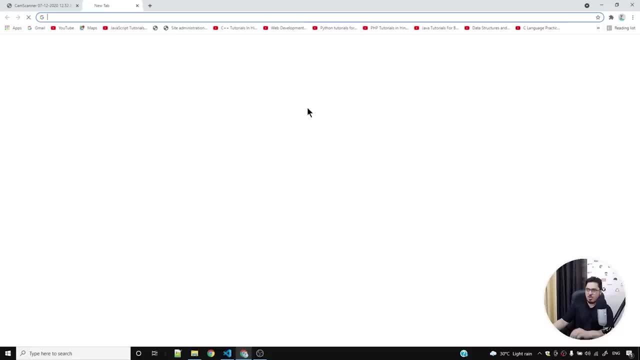 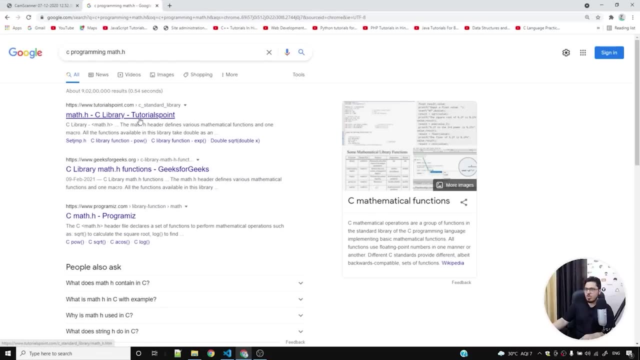 But since we have to use library function, we can use a library called mat dot edge. So I'll say C programming mat dot edge. So all you need to do is Include this mat dot edge. So I'll use the first result that comes up on Google. 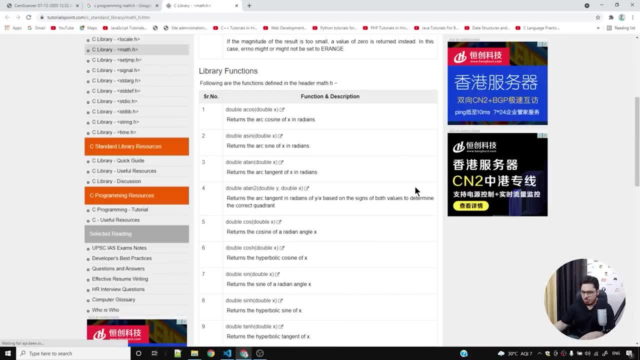 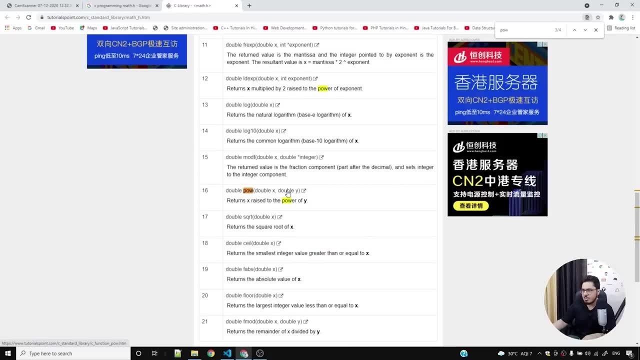 Let me show you how POW function from mat dot edge works. So POW is a function, double power, double X, double Y- So I'll show you how this works. So, firstly, what you need to do is you need to include this library: mat dot edge. 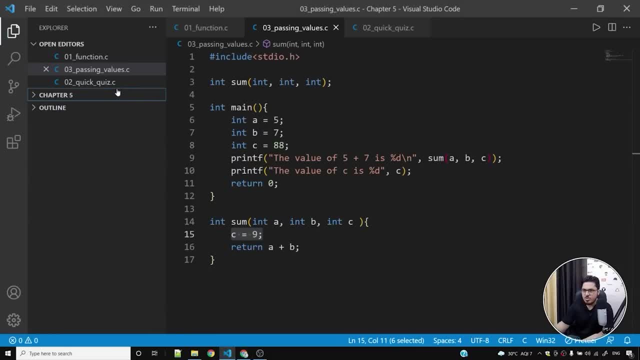 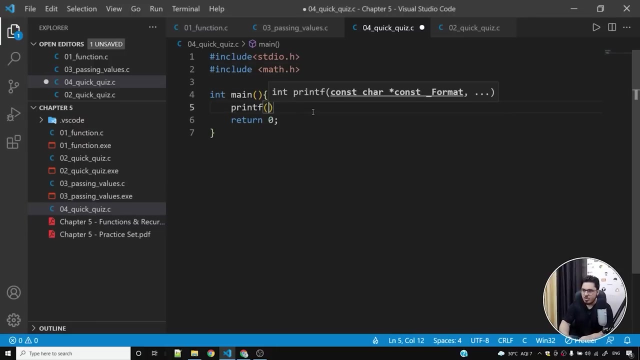 So let me make a program: Zero four underscore quick quiz. Zero four underscore quick quiz. Okay, Okay. Zero four underscore quick underscore quiz: dot C: Let's enter boiler plate code, Let's include mat dot edge And I'll simply use printf. the area of the square is: 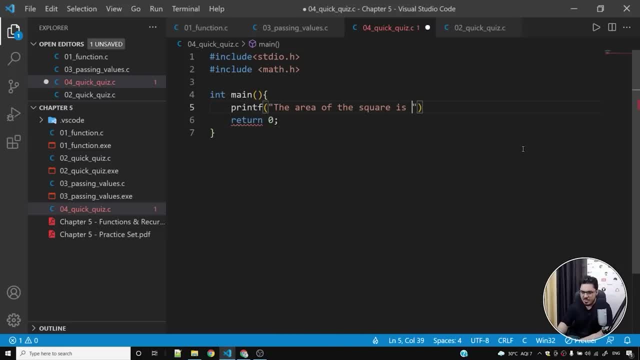 All I'll do here is I'll say the area of the square is, I'll say percentage D, And what I'll do is I'll use the POW function And all I'll do is I'll simply say a to the power two. 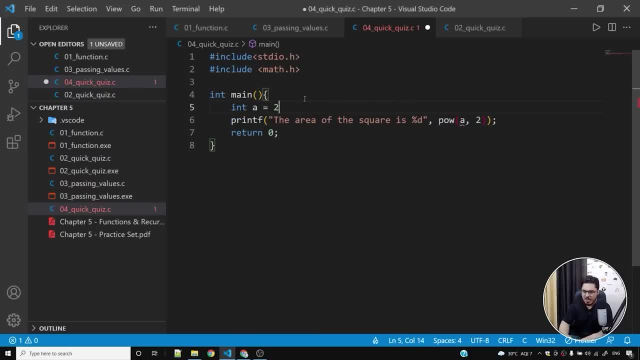 And what is a A is the side of the square, So if I have two, I should be getting four as the area. Okay, Let me use a double variable. Okay, Let me use a double variable so that we can use values with decimal precision. 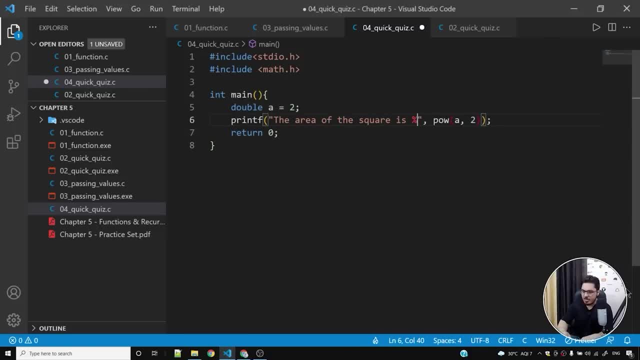 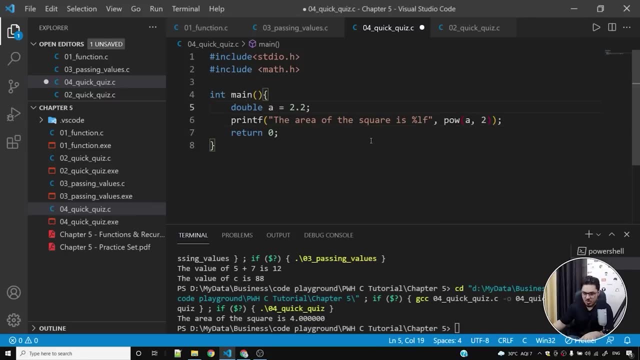 So double A is equal to two And we don't use percentage D for double, we use percentage LF for double And if I run this program you'll see the area of square is four. So even if I have 2.2, you'll see something like this: 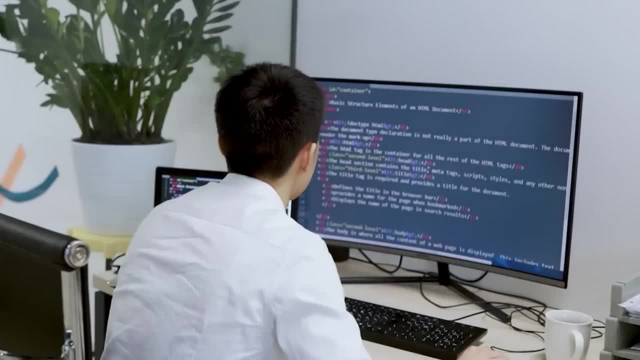 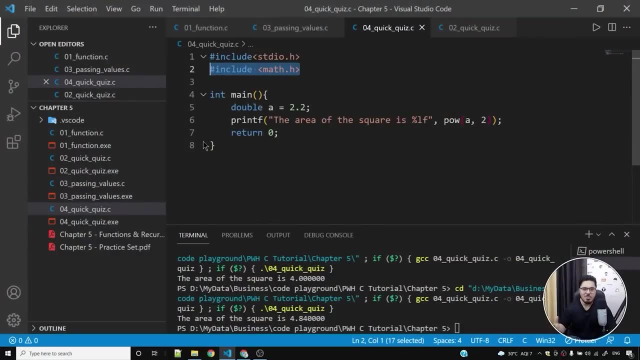 So the area of the square is 4.84.. I hope that makes sense And you are able to understand how we solve this quick quiz using library functions. Now, if you are getting confused with what these library functions are and how we are going to use it in the later chapters, do not get worried about all these things. let 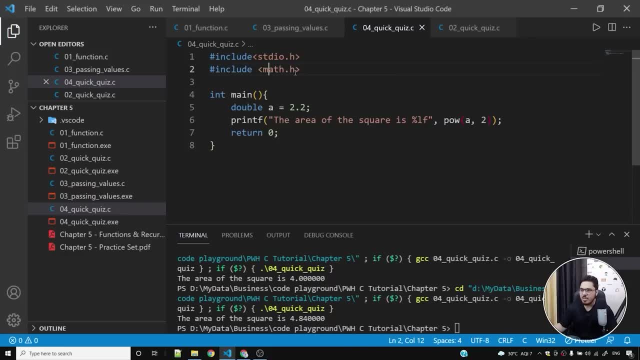 me tell you. All you need to know at this point is that we have used math and a function for math which simply raises a number with the power of two. in this case, We can even raise it to the power of three, four or any other number. 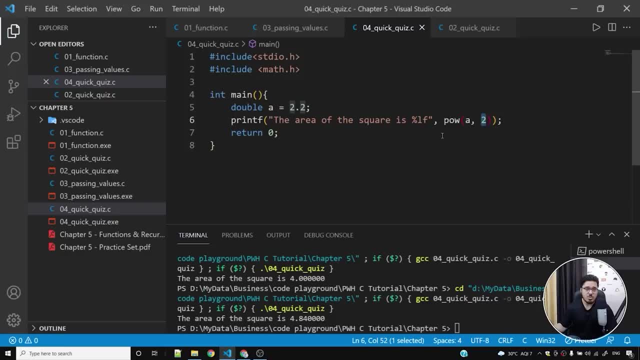 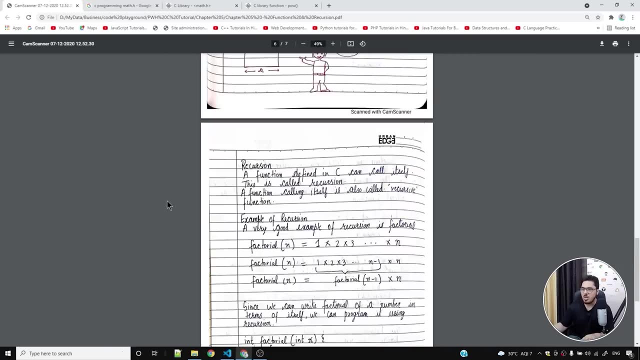 But in this case we are simply raising it to the power two. So power is a function from math. This is all you need to know at this point. Coming back to the nodes, We'll talk about recursion now. Recursion is really a very important topic when it comes to C programming. 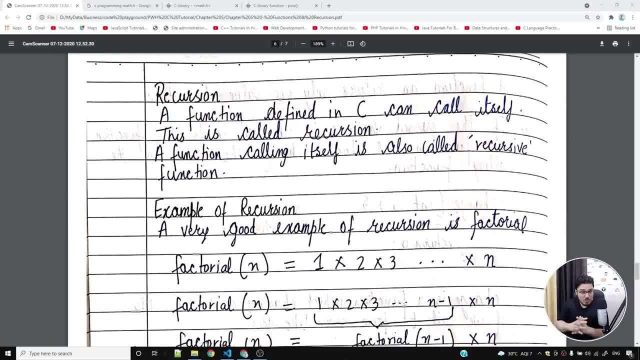 And we are going to discuss it in great detail. Let's talk about what we have in recursion. A function defined in C can call itself. This is called recursion. A function calling itself is also called a recursive function. Okay, so this is something that you need to know. 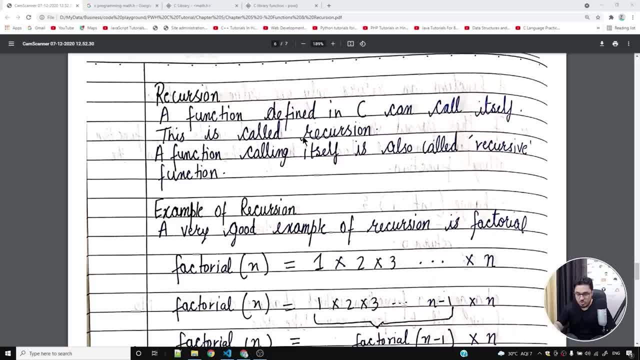 A function defined in C can call itself. So if I have a function called recursion, It can call some once again, and this is called recursion in C language. So a function calling itself can also call, is also called recursive function. So we can call a function which calls itself as a recursive function. 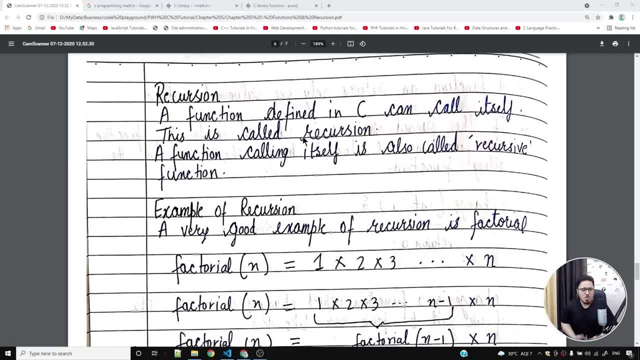 Now you must be thinking what this recursion is. And why should I even bother about recursion when I can write programs in other ways? Recursion is sometimes the easiest way to solve a problem because the formula contains recursion for solving the problem. I'll tell you what this means. 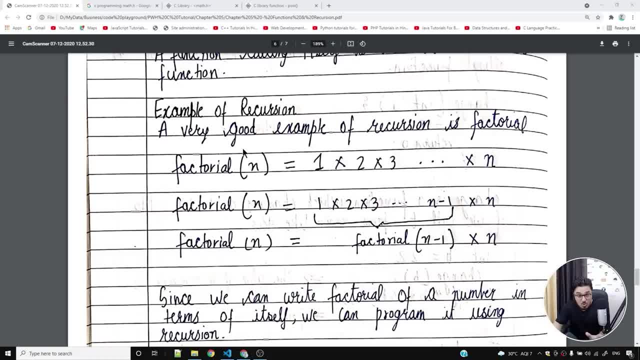 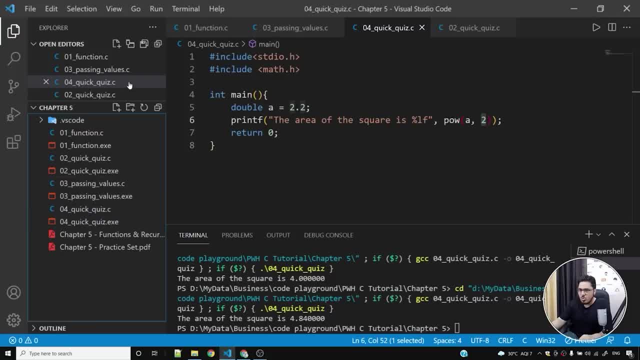 And we'll take an example of factorial in this case, and this is going to explain you everything, because factorial is an example which explains recursion very well. So let's come to the notes- sorry, the code- And what we'll do is we'll create a program called factorialc. 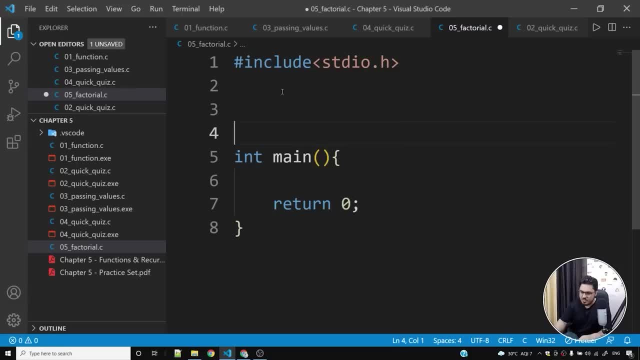 Let me write a boilerplate code. And I told you what factorial is already, But let me tell you once again: Factorial- what is factorial? Factorial 5 is nothing but 5 multiplied by 4, multiplied by 3, multiplied by 2, multiplied. 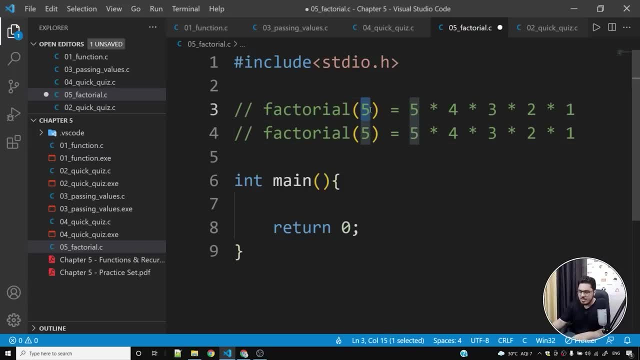 by 1.. Okay, And factorial n is nothing, but you start from n, you keep on reducing number to n minus 1,, then you keep doing this for n minus 2,, then you do this for n minus 3, and you go. 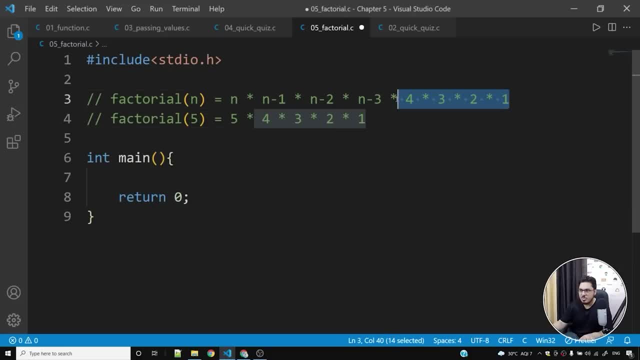 all the way till 1.. So n n minus 1, n minus 2, n minus 3.. And you go all the way till 1, okay, So this is how factorial works, And if it is 5 here, you'll go from 5 and you'll keep on reducing integer until it becomes. 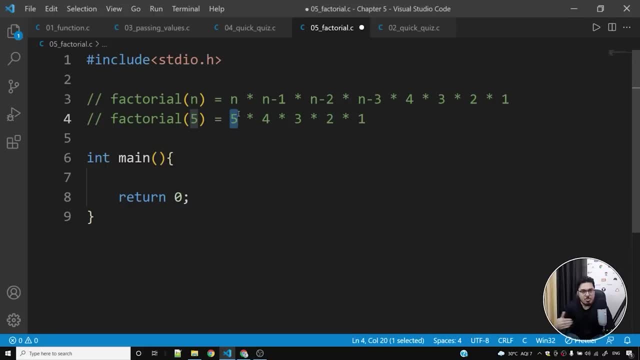 1.. If it is 9, you'll keep on reducing the number and keep on multiplying those numbers till it becomes 1.. So 5,, 4,, 3,, 2,, 1.. And once again, if the value is 13,, 13,, 12,, 11,, 10,, 9,, 8,, 7,, 6,, 5,, 4,, 3,, 2,, 1, and so. 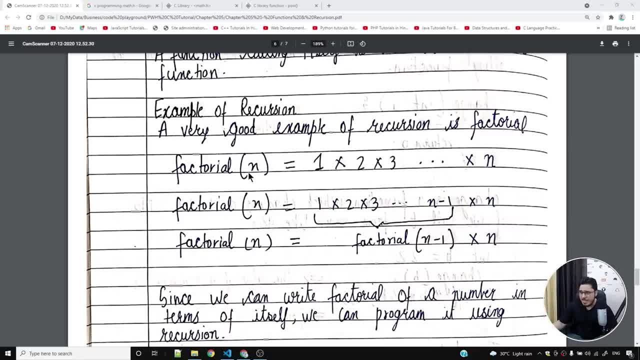 on. So you understood how factorial works now. Now The same thing has been written in the notes as well. I've written: factorial n is 1 multiplied by 2, multiplied by all the way till n. So you can either write it like this or you can write it in a reverse manner: 1,, 2,, 3,. 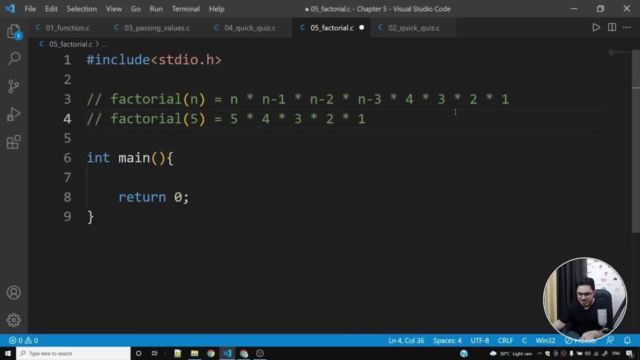 4, all the way till n. It's the same thing, okay, But we have a special case of factorial 1, which is very clear that the value of factorial 1 is 1.. This one is clear, but we have a special case of factorial 0.. 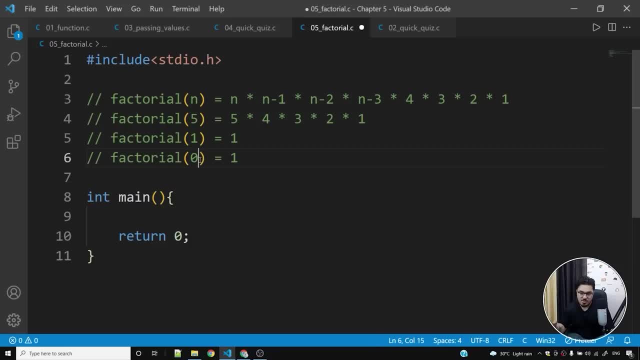 What if the value is 0?? So factorial 0 is defined as 1.. This is something that you need to keep in mind. So this is a mathematical formula, and we now understand how factorial works. Now listen to me very, very carefully. 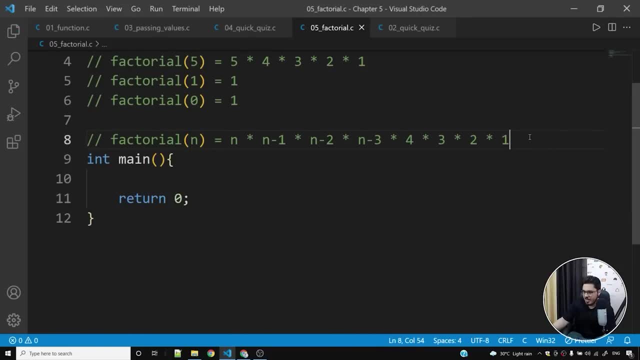 Let us say we have this formula: Factorial n is equal to this thing, and I want to change it. I mean, I want to write it in a different way. How can I do that? Can I not write: factorial n is equal to n multiplied by this thing? 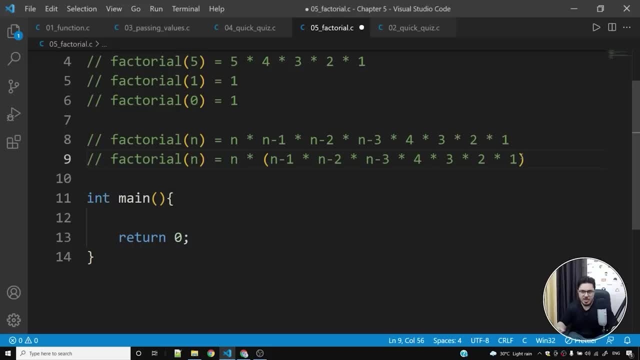 Yes, we can. We can write it. It's what it is written. okay, This is what is written here. Now, what is this value? What is the value n minus 1 multiplied by n minus 2, all the way till 1?? 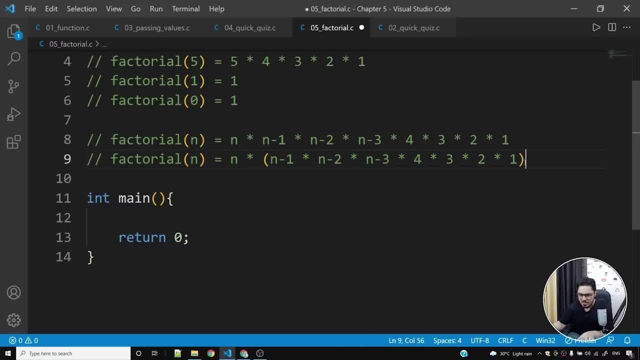 Isn't it not factorial n minus 1?? I hope you understood that this is factorial n minus 1.. So I can replace this with factorial n minus 1.. I can do that, right, I can, Yes, I can do that. 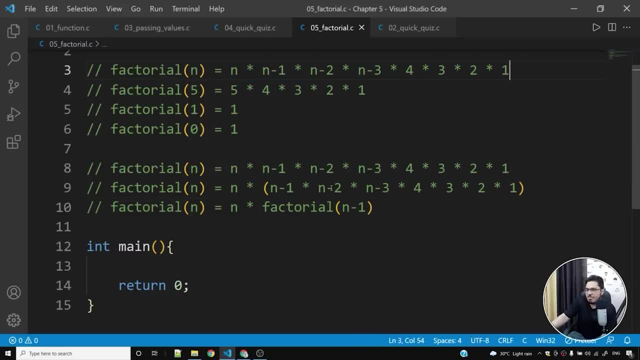 Because, by definition of factorial n, this is the formula and factorial n minus 1 will be this value. So factorial n is equal to n into factorial n minus 1.. And we are going to use this to our advantage. We are going to use this formula to calculate the values of factorial 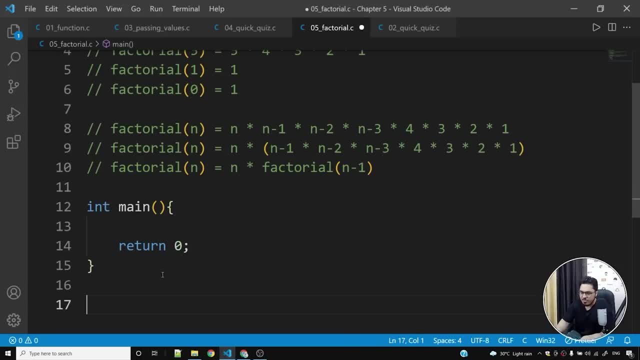 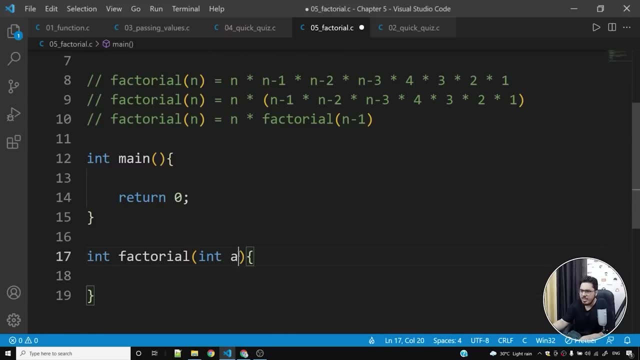 Let's see how we can do that, okay. So what I'll do is I'll write a function called factorial, and this simply takes a number, a, or rather n. let me call it n, because I'm calling it n here as well. 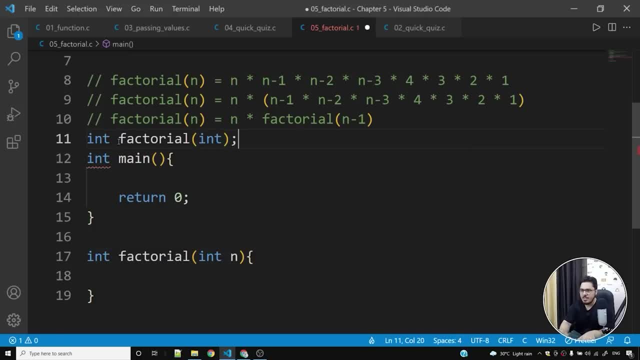 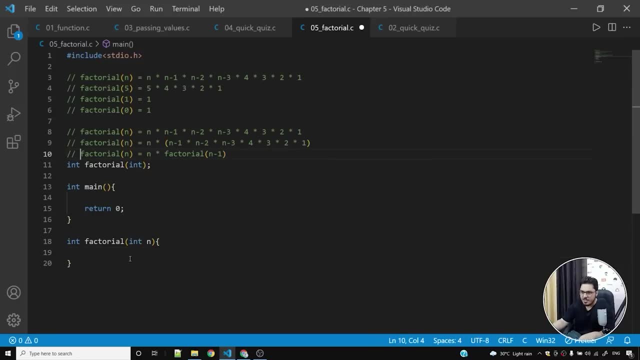 Also I'll write a prototype factorial n, that's it okay. Now what I'll do is I'll simply write this formula. I'll say: return: Okay, What is factorial n? Factorial n is n multiplied by factorial n minus 1.. 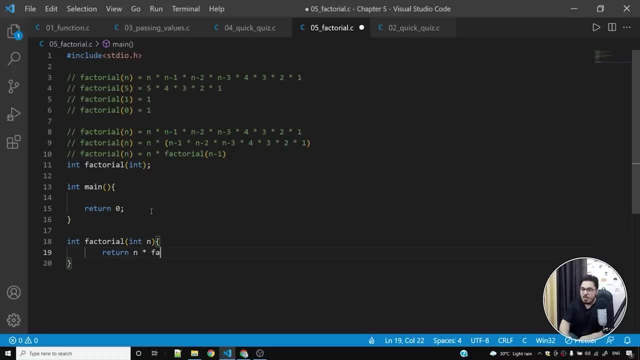 I'll say: return the value n multiplied by same function for n minus 1,. okay, And that's it. That's it. So what will happen is it'll keep on reducing the value of n and it'll keep on calculating the factorial. 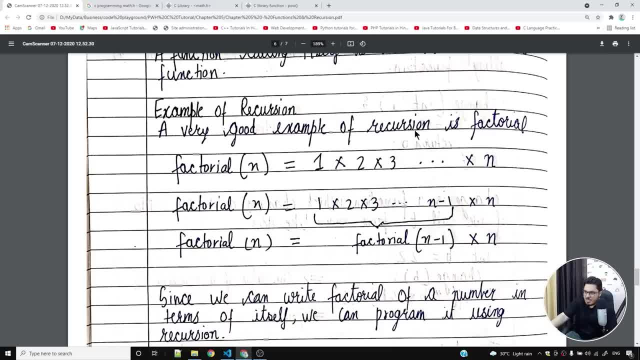 I'll show you the tree how this will work. So a very good example of recursion is factorial. I've written factorial n's value. Then I've showed you that factorial n is equal to n multiplied by factorial n minus 1.. Okay, 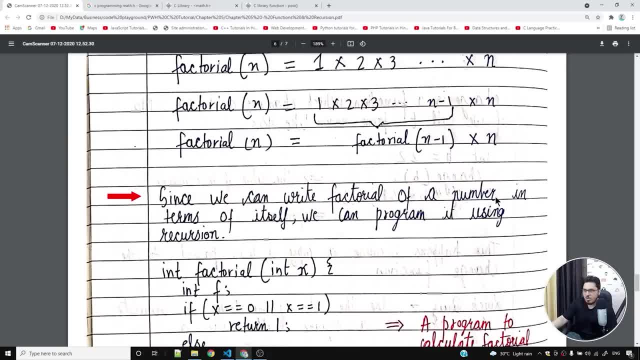 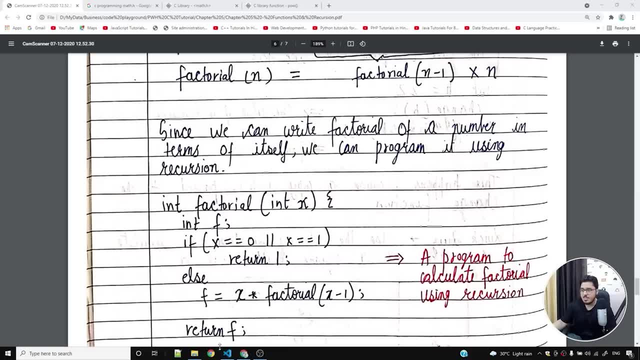 Now, since we can write factorial of a number in terms of itself, we can program it using recursion. How will we program it using recursion? Let's see. Let us say I've supplied 4 to this, So it will calculate 4 multiplied by then it will wait for factorial of 3.. 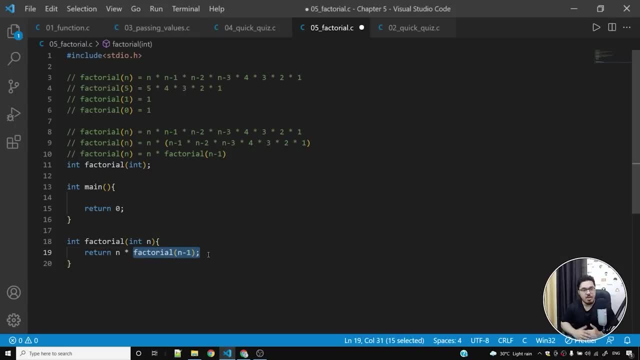 It will say 4 multiplied by, then it will start calculating the value of factorial 3.. Then it will be 3 multiplied by, it will start calculating the factorial of 2, and so on. So there'll be a time that this value will start going into negative. 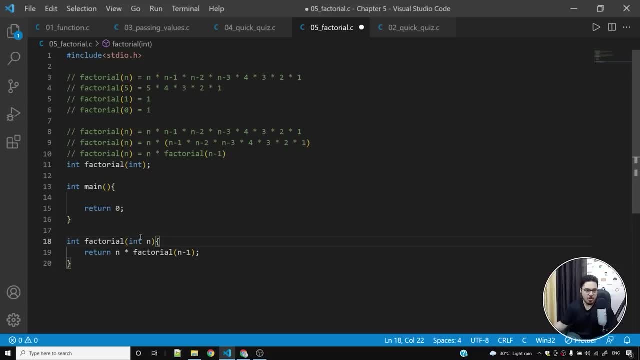 Factorial n minus 1.. Factorial minus 1.. Factorial minus 2.. We don't want that. So what we do is we write a base condition. We say, if the value of n is 1, or the value of n is what, 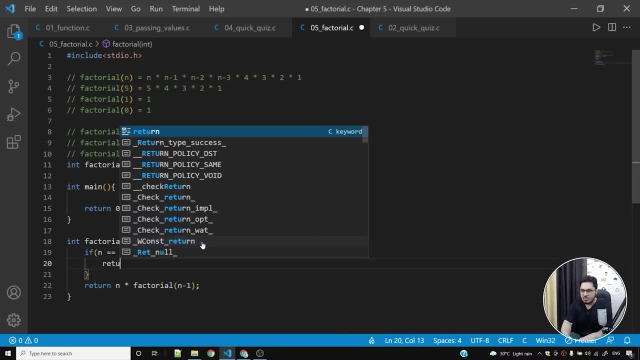 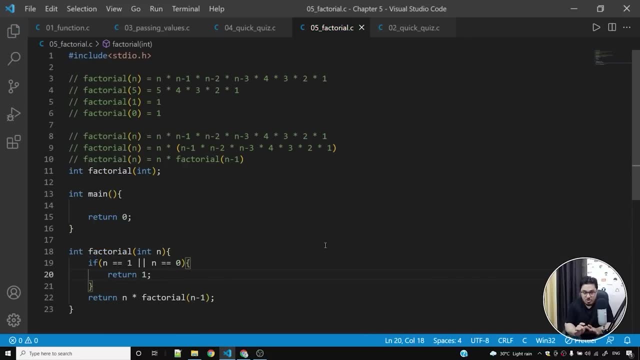 Or the value of n is 0, simply return 1.. So we say return 1. if this is the case, Okay, And that's all. That's the program to write factorial. I'm not saying that you understood how factorial program works. I'm going to explain it even. 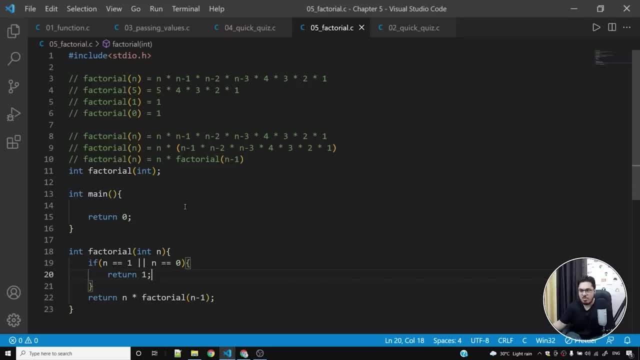 more, But I'm telling you that this is all I need to write to calculate factorial. Okay, Let's see if this program works. The value of factorial 4 is %t, So I'll simply say factorial 4.. Now, what I'll do is I'll run this program. The value of factorial 4 is 24.. Let's check: 4 multiplied by 3 is 12,. multiplied by 2 is 24.. Yes, It is correct. Let's change this to 5. And let's see if it turns out to be 1,, 2,, 3.. 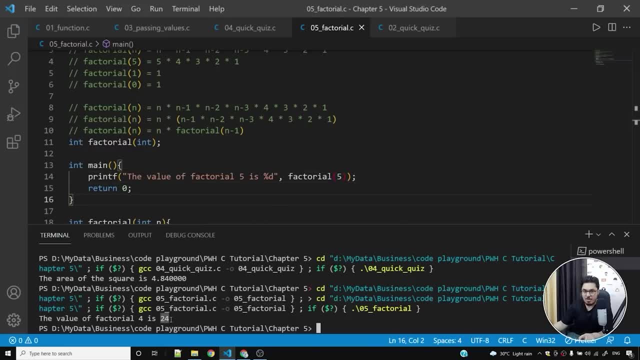 Okay, It turns out to be 120, because 24 multiplied by 5 is 120.. Let's see if this works. And yes, it works: 24 multiplied by 5 is 120. Great. Now, if I make it 6, I'll have to multiply this by 6.. 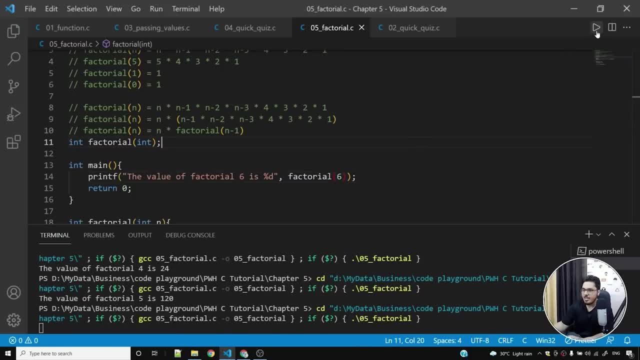 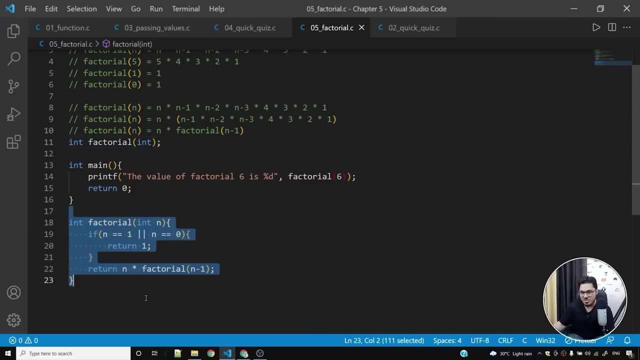 And it should turn out to be 720.. Let's save this program and run it 720.. Yes, this works, But how does it work? Let's try to understand it even more how this function is working. So, whenever a value n is received, 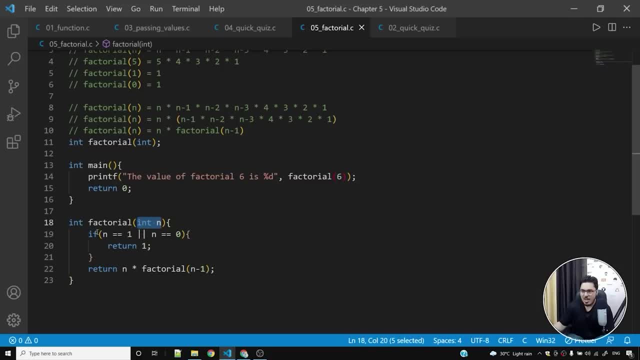 Let's see, Let's say, 4 is received. What happens is: this condition is not true, because n is not 1, n is not 0, n is 4.. So what happens is: let me show you here, I'm saying factorial 4.. 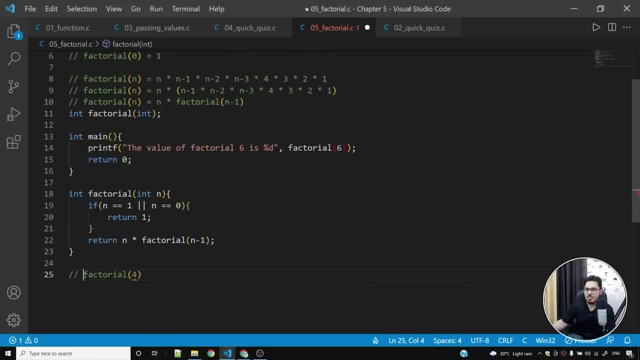 What happens is that the C compiler will start running factorial function for the value 4.. But what I'm returning here is I'm breaking it down to 3 multiplied by factorial of 3.. So I'm simply saying sorry, 4 multiplied by factorial 3, n multiplied by factorial. 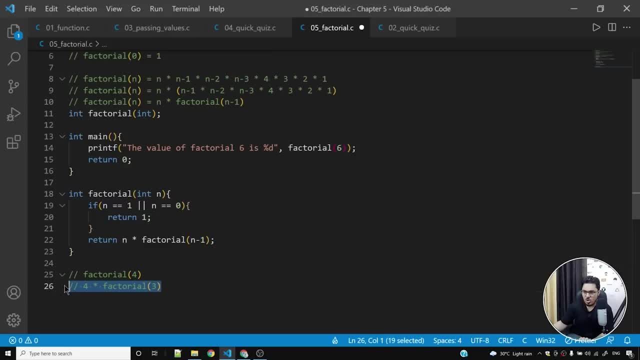 n minus 1.. So I'm doing something like this, But this is not yet resolved. I need to further calculate the value of factorial 3.. So now it becomes 3 multiplied by factorial 2.. Now factorial 2 is still not resolved. 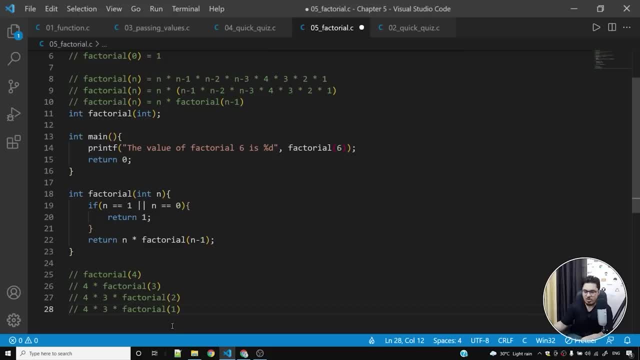 I'll try to resolve it once again, and it'll be 2 multiplied by factorial 1.. But as soon as I reach 1, what will happen is this condition will become true And instead of returning this, what will I return? I'll return this. 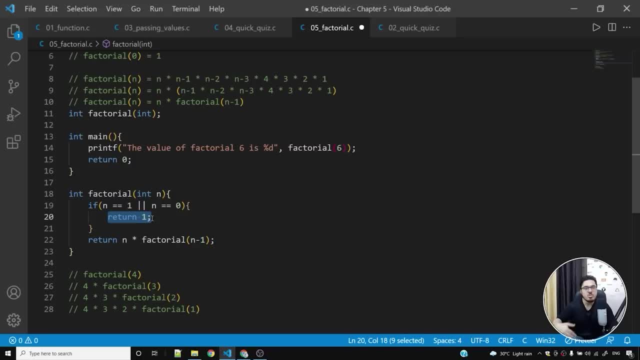 Okay, Let me tell you something. As soon as a function encounters a return statement, it will not execute anything below that. So as soon as I see return, it means stop the function. We are done, We got the value and we don't need to run this function any further. 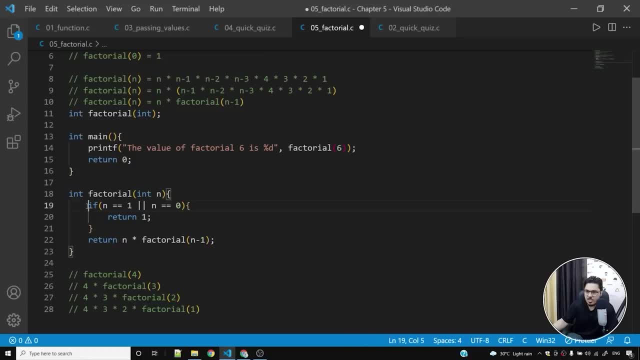 So as soon as factorial 1 starts running, this condition will be true, because the value of n is 1.. It's n equals to 1 or n equals to 0 is true because n is 1.. So what happens is 1 is returned. 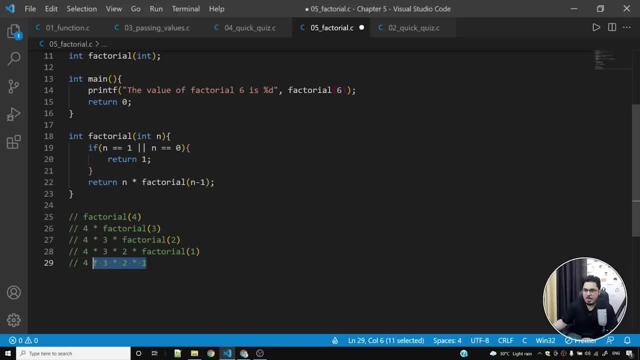 And now all the values are resolved, So compiler can now start to calculate this value, which is nothing but 24.. Okay, 3 multiplied by 2 is 6.. 6 multiplied by 4 is 24.. So this is how this program is working. 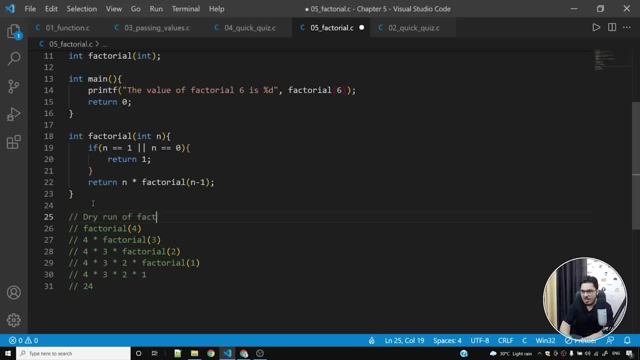 So this is the dry run. This is called dry run of factorial 4.. And I'm going to give you all these programs in the form of a zip file. Make sure you download all the programs that I'm giving you. It is really very important for you to download nodes as well as all these programs which I'm 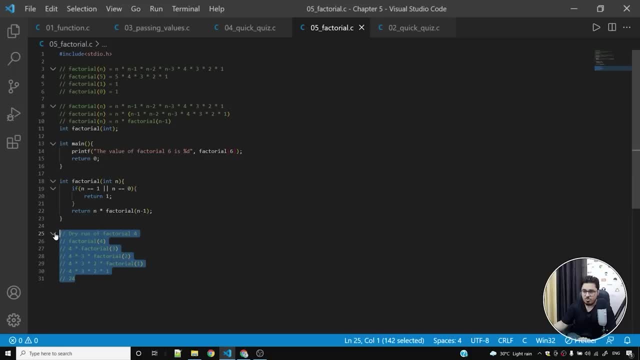 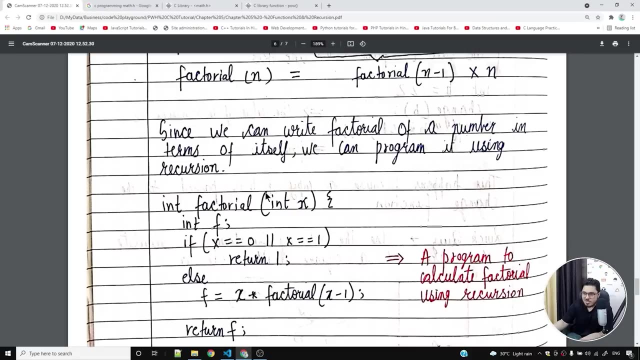 giving you All. these programs also contain a lot of good concepts, like dry run, And I've written a lot of comments in the programs just for you. Okay, So this is how this works. Now let's come back to the nodes and see how this works. 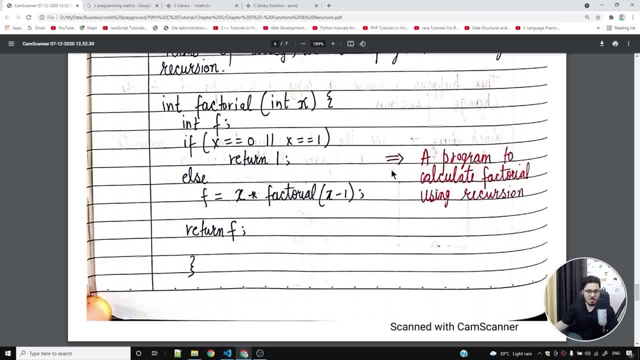 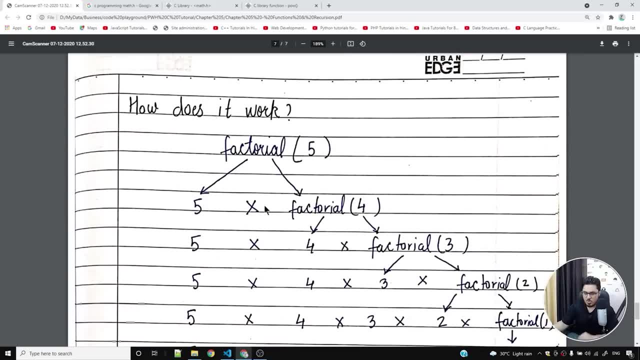 So I've written the same thing in the nodes as well: A program to calculate factorial using recursion. So this is the program, in case you want to see the nodes and type it out. Now, how does this work? I've explained the same thing. 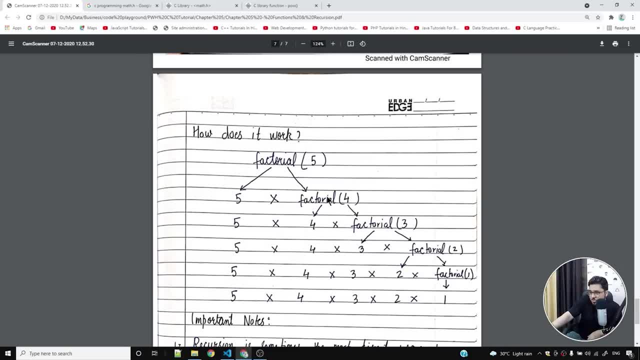 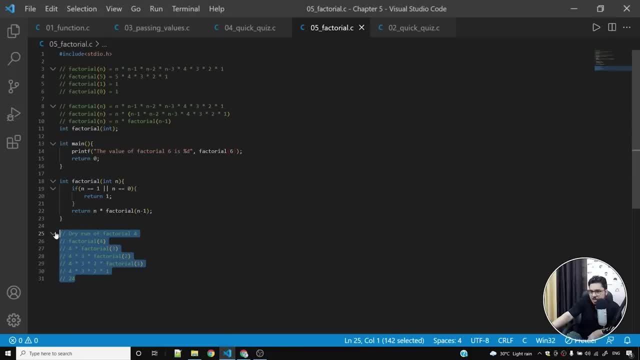 Factorial 5 will be broken down into 5, into factorial 4.. Now, further, 4 will be broken down into 4, into factorial 3.. And so on, until we encounter this. I've explained it here. I've explained it for the value of factorial 4.. 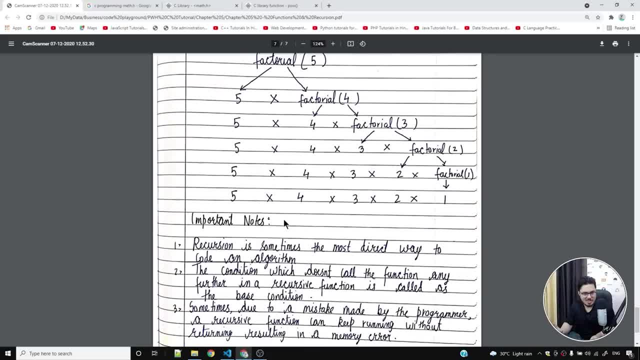 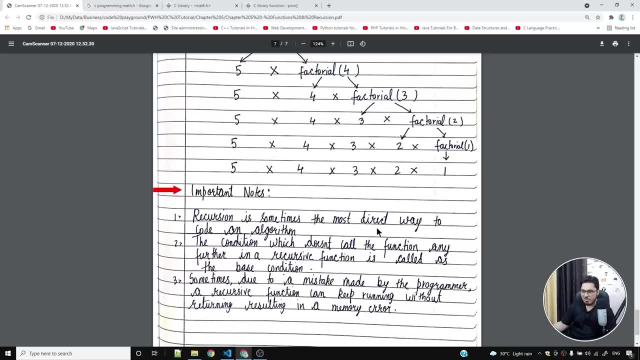 In the nodes I've explained it for the value of factorial 5.. I hope all this makes sense. Okay, Now I have written some important nodes for you, And the nodes are: recursion is sometimes the most direct way to code an algorithm, Just like we saw in the example of factorial. 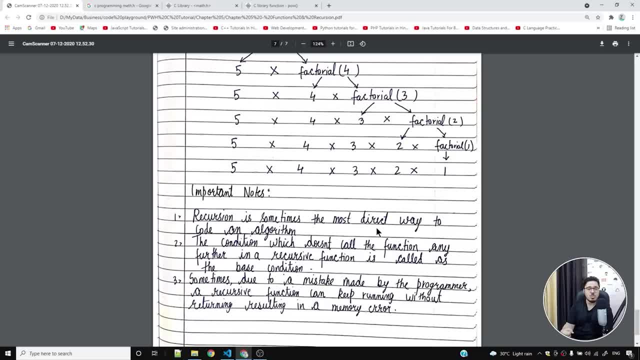 There is another example, a very classic example of recursion. It is called Fibonacci series. We are going to see that in the practice. But again, I'm just telling you, sometimes a mathematical formula can directly be written inside the function and we are all done. 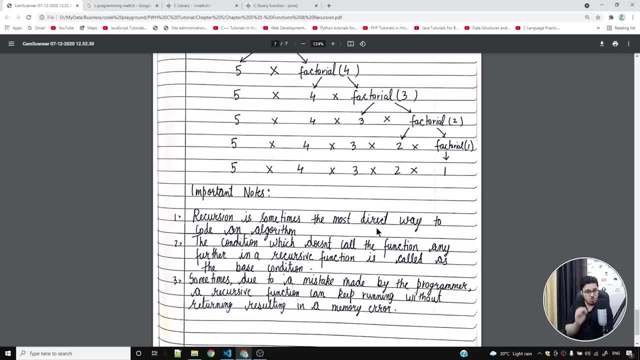 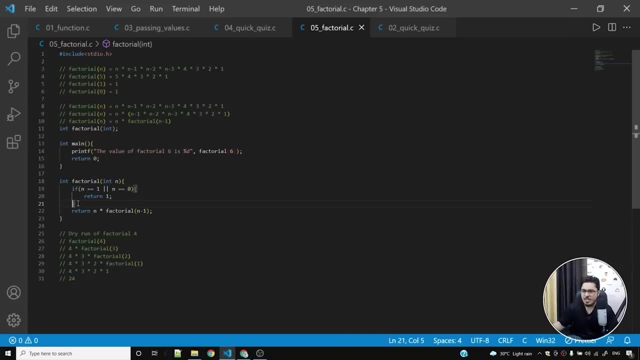 So recursion is sometimes the most direct and easiest way to solve a problem. Now, the condition which doesn't call the function any further in a recursive function is called as the base condition. What is the base condition here? This is the base condition. Base condition ensures that we are not calling the function infinitely. 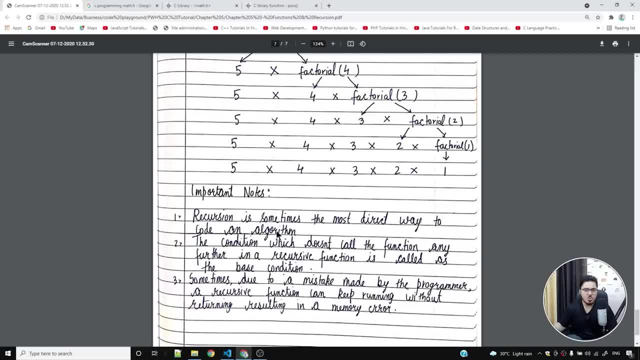 We don't want that. We don't want to do that. We always want to stop somewhere, and base condition takes care of that. Okay, Sometimes, due to a mistake made by the programmer, a recursive function can keep running without returning result, resulting in a memory error. 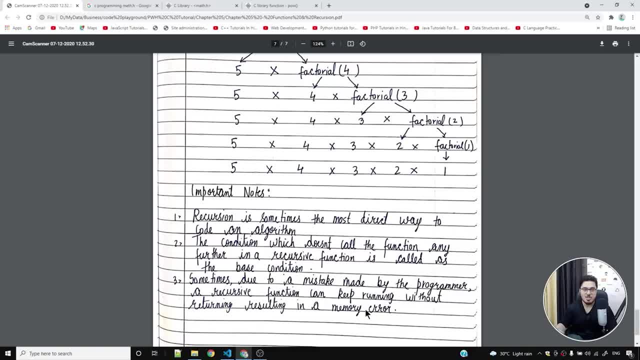 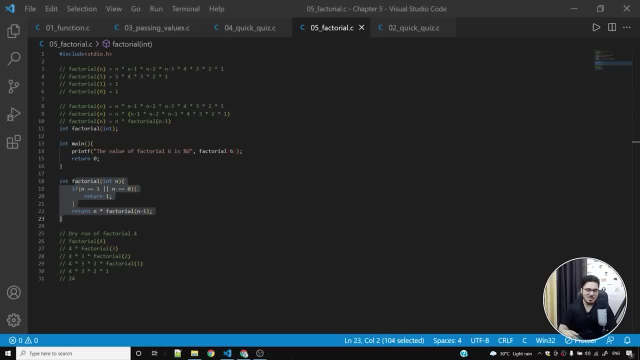 So sometimes you might make your program throw a memory error just because you have made a mistake. For example, let us say, if I forget to write this base condition, what will happen is this particular function will keep on running and running and running. Okay, 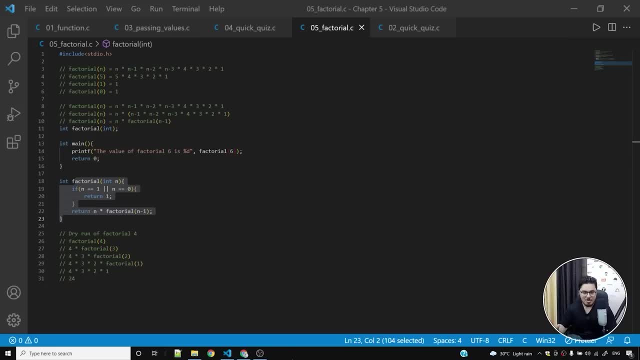 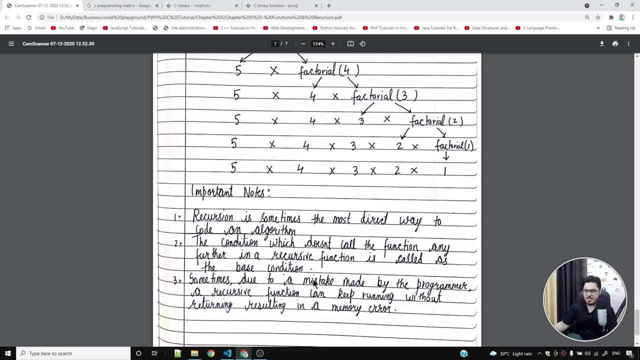 So we will keep on running until the memory is full and we don't want that. We don't want memory or errors from our program. So we need to be very, very careful when we are writing programs using recursions. I hope that makes sense and you were able to understand functions and recursions. 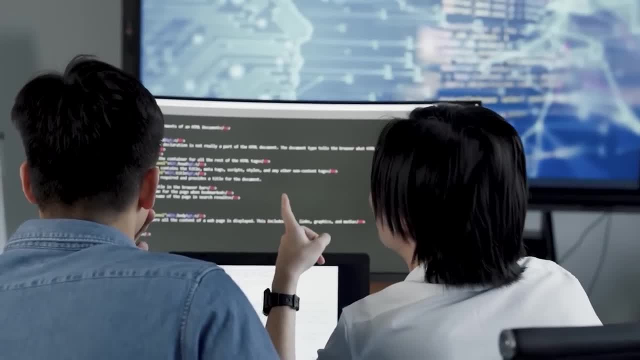 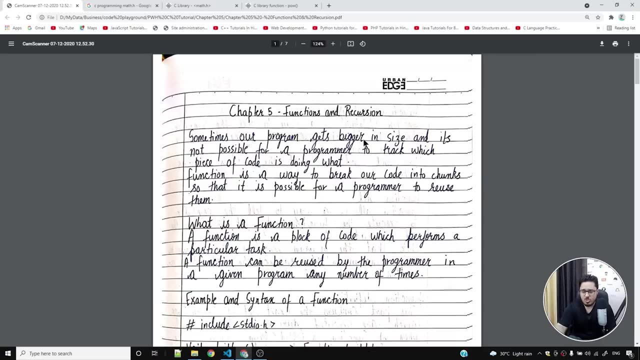 This chapter was about function and recursions. I hope I was able to explain all the things in a very good way. Make sure you download the notes, Make sure you download the code. It is going to really help you with the revision, and I also advise you to download these notes. 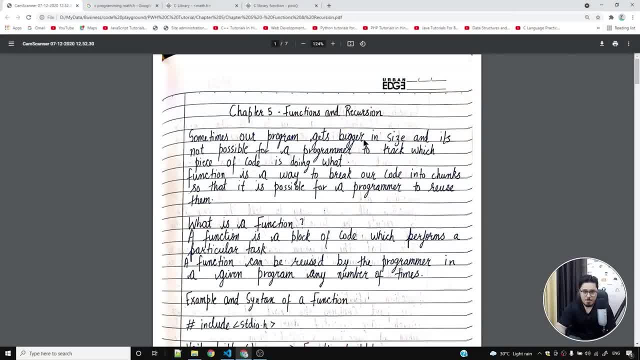 and take a printout from your nearest Xerox center- Go ahead center. that would be better than the pdf, but if you are a pdf person you can download the pdf as well. i have everything in the description. let's now move on to chapter 5: practice set and see. 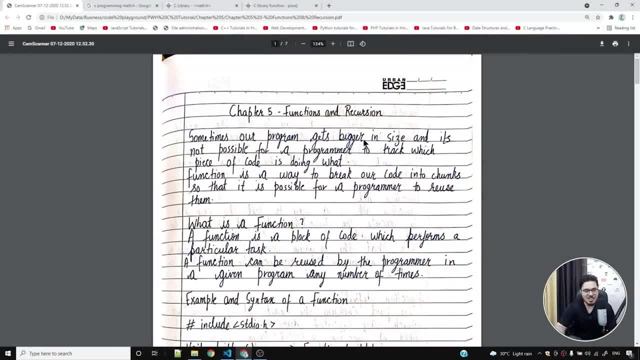 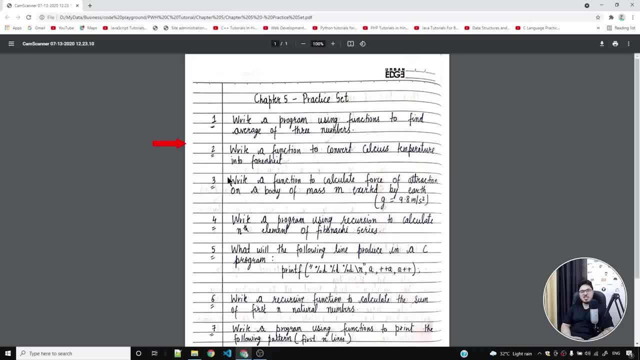 what are the problems that we can solve for functions and recursions? let's move on to chapter 5 practice set now. so here is the chapter 5 practice set which i have created for you. this practice set contains a lot of problems which can help you understand functions and recursions. so 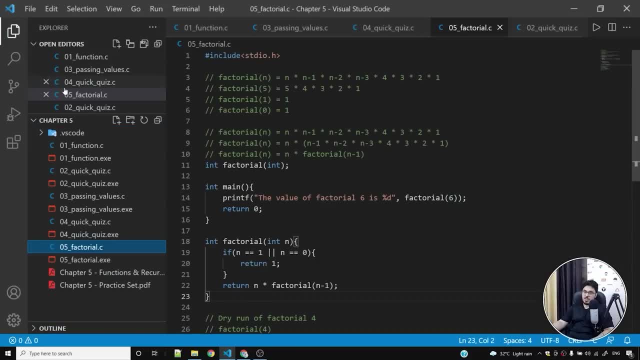 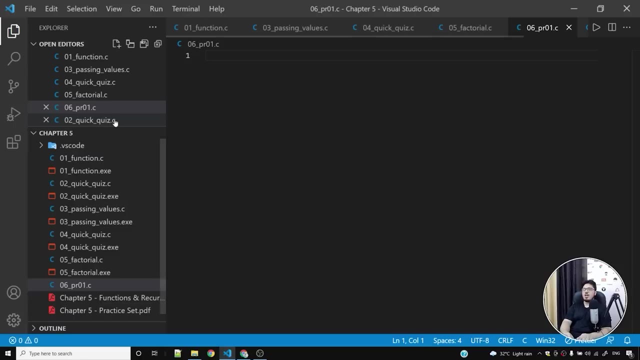 let's move ahead towards visual studio code and start solving some of these problems. so question number one says that write a program using functions to find average of three numbers. so let's start writing this code. so what i'll do is i'll simply say 06, underscore pr01.c. i'll add: 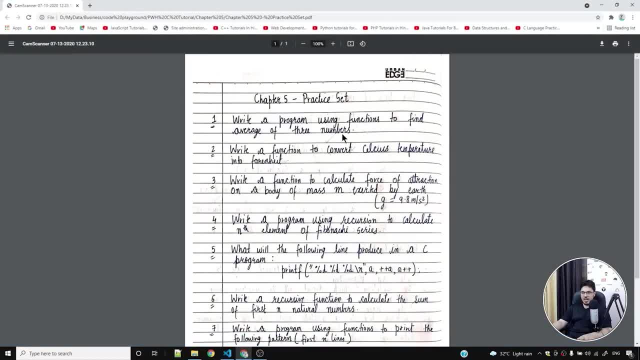 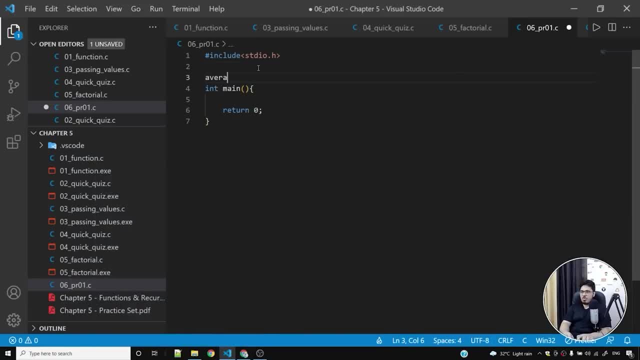 the boilerplate code and all i have to do at this point is i have to write a program using functions to find average of three numbers. so what will be the return type of my function? so if the name of my function is 06 and i have to write a program using functions to find average of three numbers, 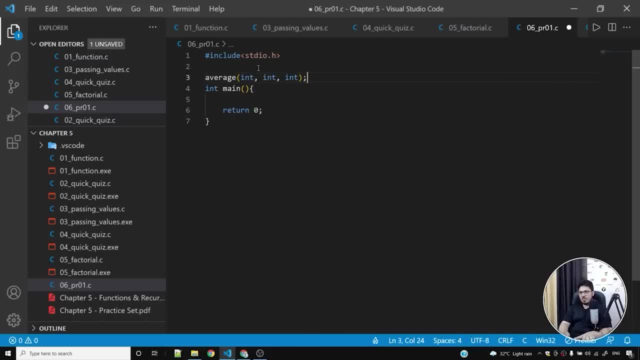 average, and let us say it takes three integers. what will be the return type of this function? i want you guys to comment down below and tell me what will be the recurrent return type. what is the ideal return type that i should write here? i'm waiting for your comment. all right, in case you. 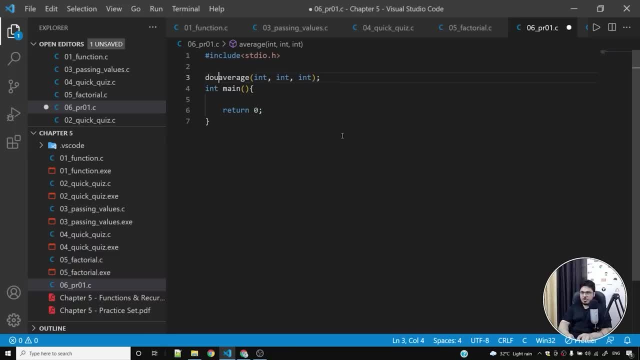 commented i. i will tell you what should be the return type. it should be double or float. float is also the correct answer. double is a bit more precise because if you have a very large number, double will take care of that. but why did we use double here? we use double here because we might get the average as a decimal number. 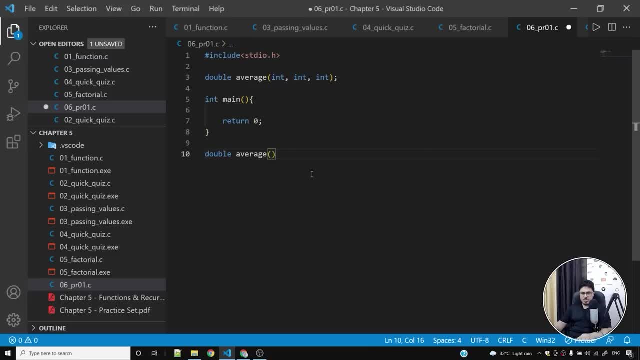 so let us say the average of one, two and three, three plus three is six, divided by three is two, it's an integer, so no problems. but let us say i want to find average of one, one and one- it's one by three, or 0.33, and 0.33 cannot be stored in an integer, it can be stored in a double or in a. 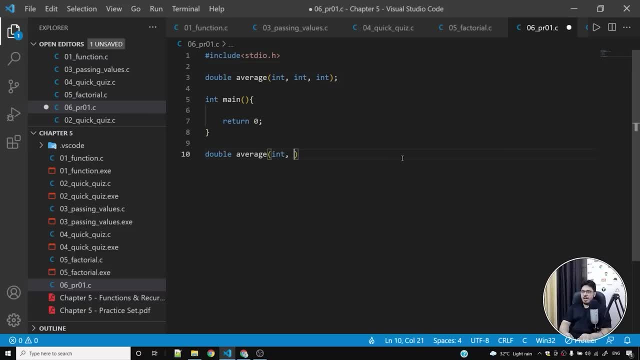 floating point number. okay, so i can either use a floating point variable or i can also use a double type variable, but i cannot use integer. i might lose precision in case i use integer. so i'll simply say in a, in b and in c. so i have three numbers and it's returning a double. so what i'll do is i'll simply return a. 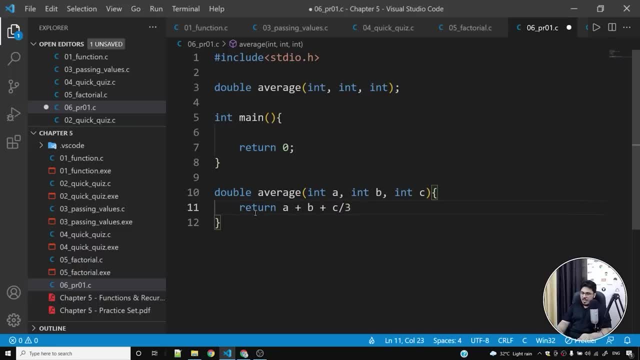 plus b plus c divided by 3. and also just to be sure that a plus b plus c is calculated before this, this number is divided by three. i'll put on the parenthesis. so this is the average of three numbers, and we all know about averages. average is something which is a very, very easy thing and we all know about it, but again we have 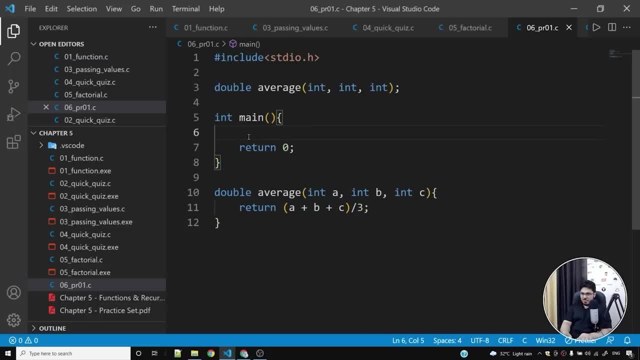 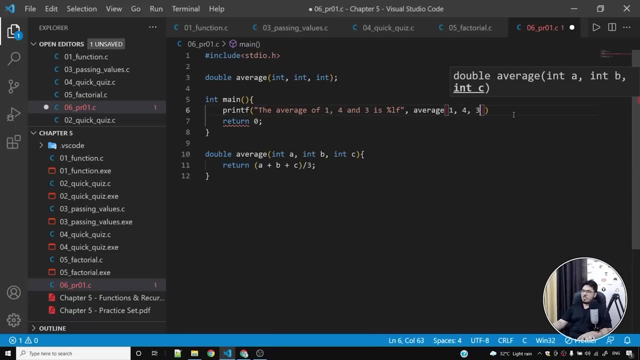 to write a program to calculate average of three numbers using functions. okay, so i'll simply say printf: the average of one, four and three is percentage. i'll say percentage lf. and also what i'll do is i'll simply write one, four and three, because i want to calculate the average of these. 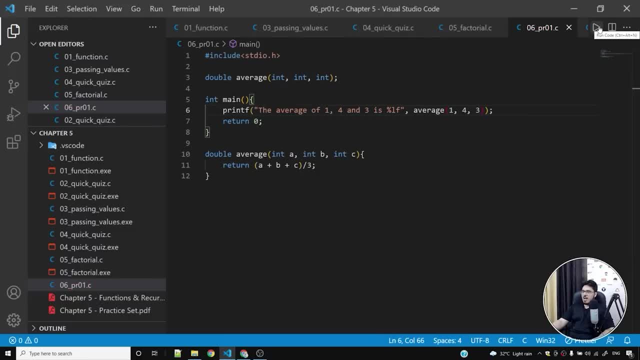 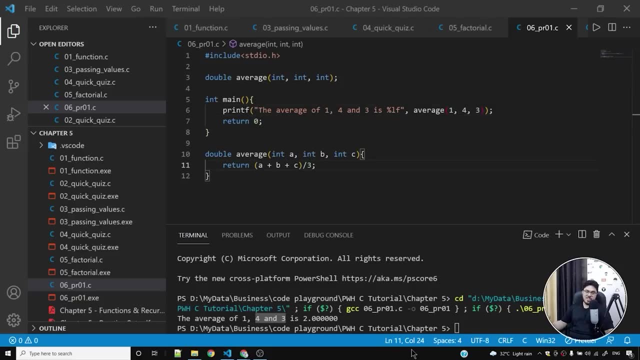 three numbers. let me go to semicolon here, return zero and let's see what answer we get. so it's two. so four plus one is five. five plus three is eight. you must be thinking: why is this the case? why are we not getting the correct answer? the average of one, four and three is definitely not two, but why? 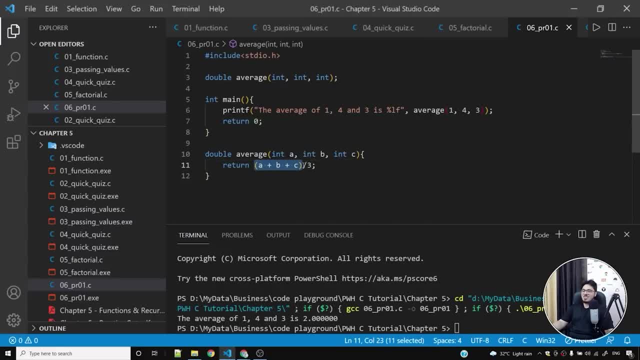 are we getting two? it's because this entire entity is going to be an integer. a plus b plus c is going to be an integer because it's a sum of three integers and three is an integer. an integer divided by integer is going to return an integer and you're going to lose precision. so, in order to 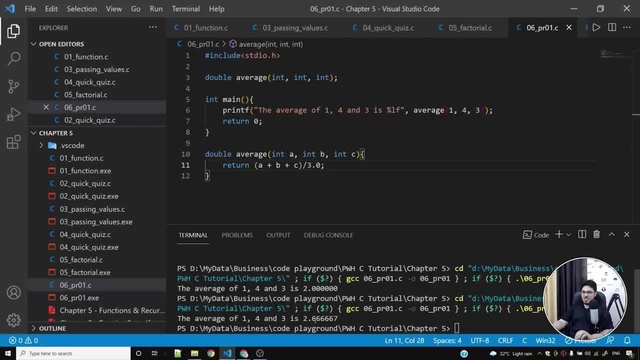 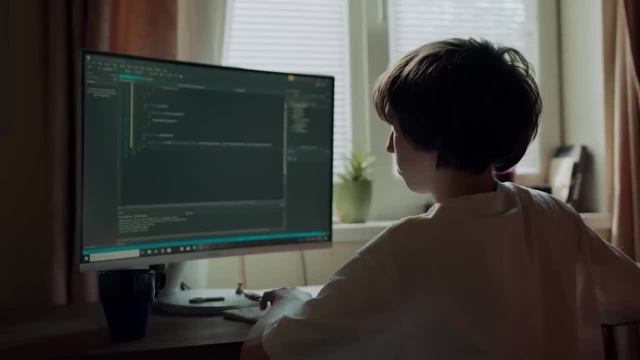 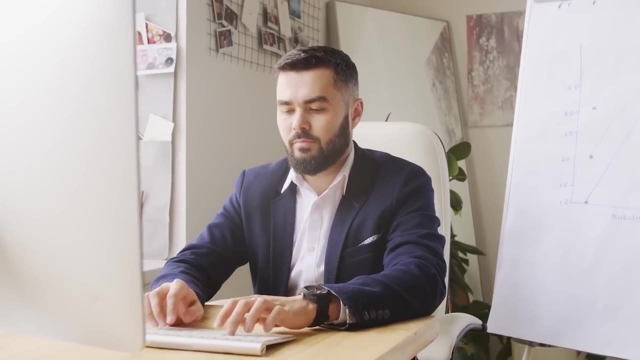 fix this. i'll simply say 3.0 and i'm going to get the correct answer. i hope you understood how you know. very basic things in c can get you some error. c is a very basic programming language and you need to take care of each and every bit if you want your program to do the intended task. 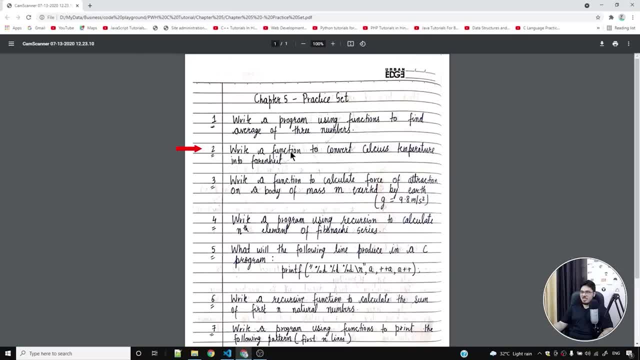 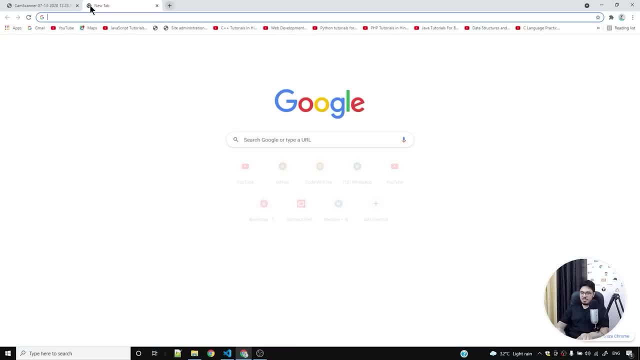 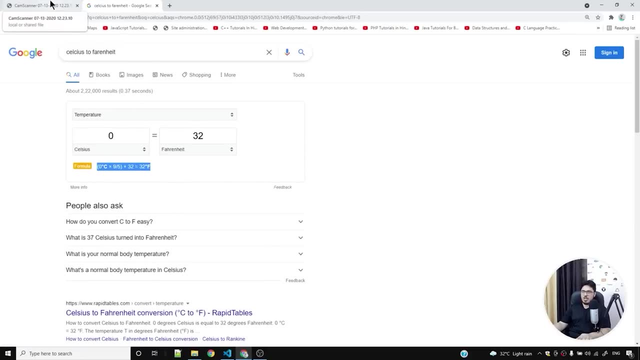 i hope you enjoyed this problem. the next question says that write a program using function to convert celsius temperature into foreignite. so if i say celsius to foreignite, there is a formula that i'm going to use. i'm going to directly use this formula and once i use this formula i will be able to write a function which. 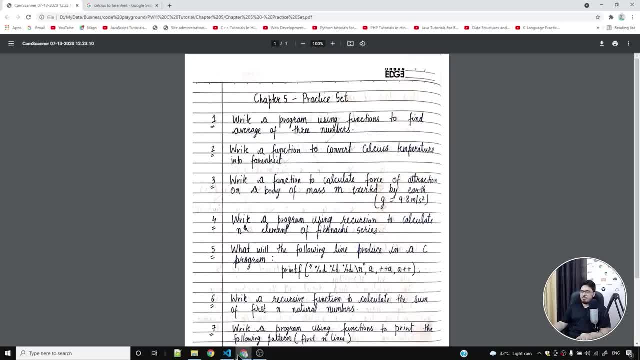 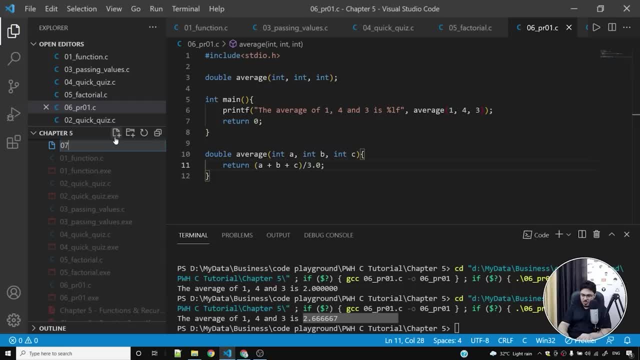 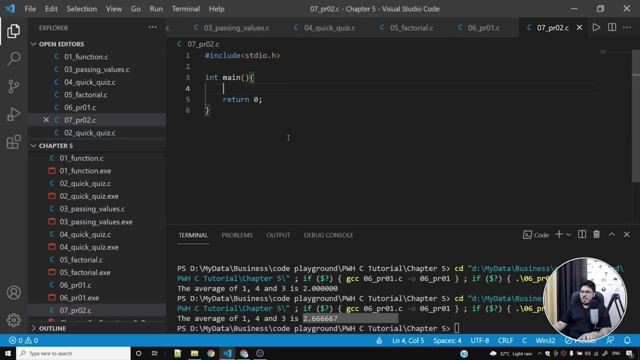 will convert celsius to foreignite. okay, so let's do one thing. let's let's try to, you know, create another program and keep the things in a very nice order so that you know when you come back to these programs. you can simply see where i have written which program and you will be able to understand the entire course. 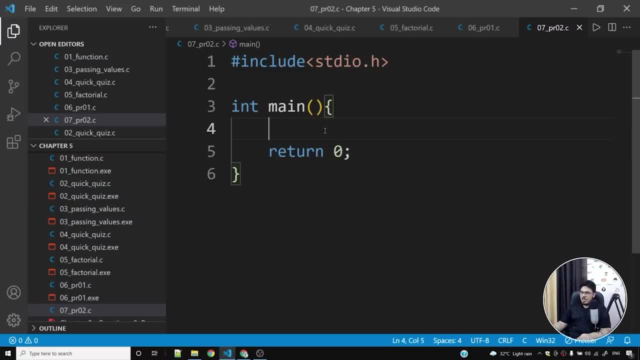 very well if i have all these programs in a good structure. so let's do one thing: uh, let's start solving this problem, and what i'll do is i'll simply say int. celsius, or let me call it in c, and i'll say in f, and what i'll do is i'll simply write down this: 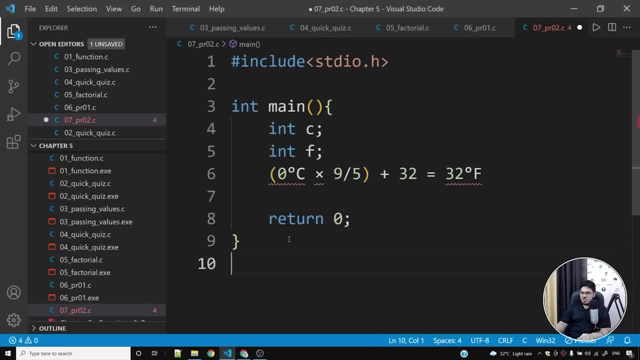 formula, but i have to use functions. okay, so i'll simply say: uh, float, let me use loads, this time celsius to foreignite, and uh, celsius to foreignite or foreignite to celsius. convert celsius temperature into foreignite. okay, cool, so i need to convert celsius to foreignite, and what? what will be the? 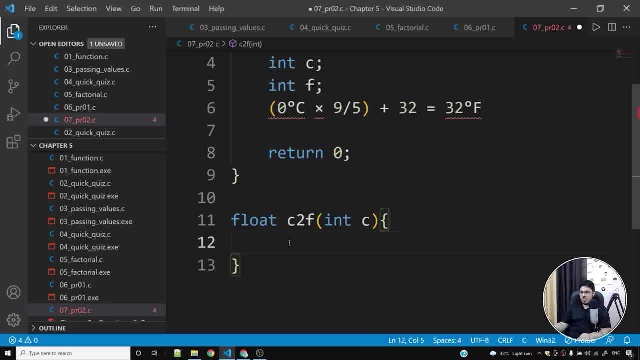 input of this function. celsius and c will be the input. now, what i'll do is i'll copy this code here. uh, definitely, it's not a code. i'll simply say: int f is equal to: and let me make this as float as well. let's keep everything in float. 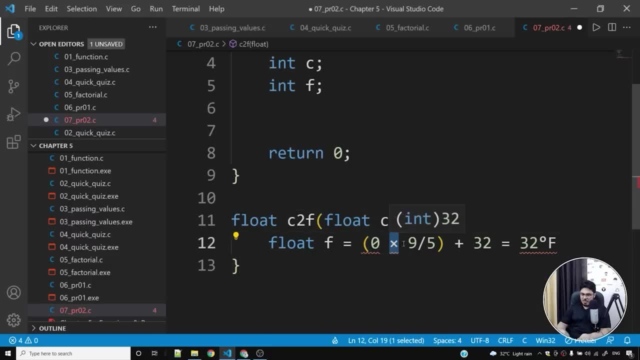 degree celsius multiply will be replaced with star and c 9 by 5.0, just in case, and here will be c and what else? what else? what else? i need to remove this, okay, so what i'll do is i'll simply put a semicolon here, and this is fahrenheit temperature using celsius. 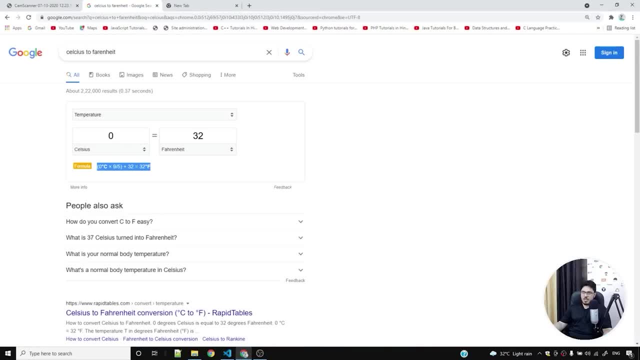 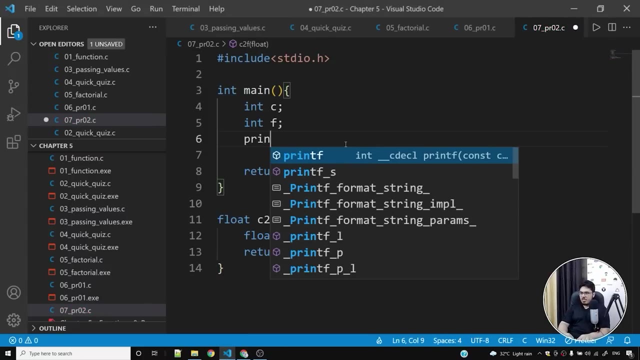 temperature. so let me check the formula once again. so if i want to convert a celsius to fahrenheit, i simply put c here and that will give me the fahrenheit temperature. cool, i think i'm doing it right. i i need to return f now and also i need to write a printf and and i'll say: 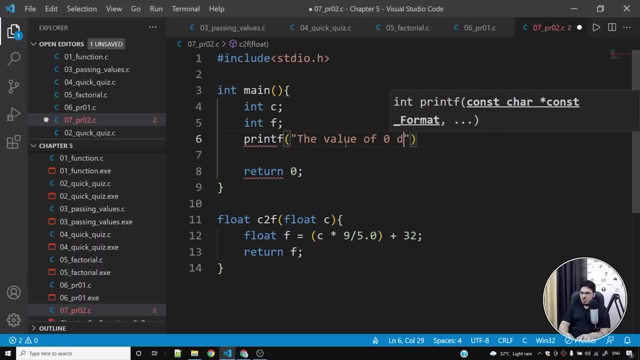 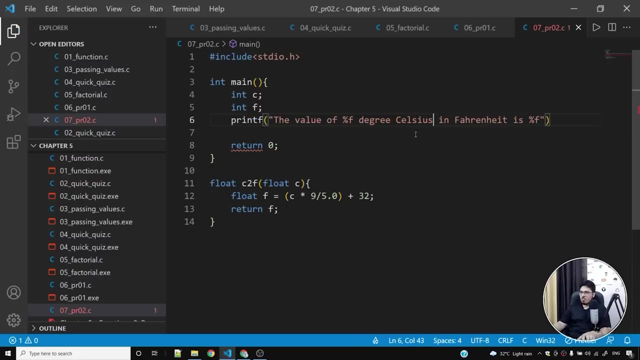 the value of zero, zero, zero degree in fahrenheit is percentage lf or percentage f. because we are using float here, let me call it percentage f as well. so of the first value is celsius c and the second value is f, and yes, i'm going to use this formula. 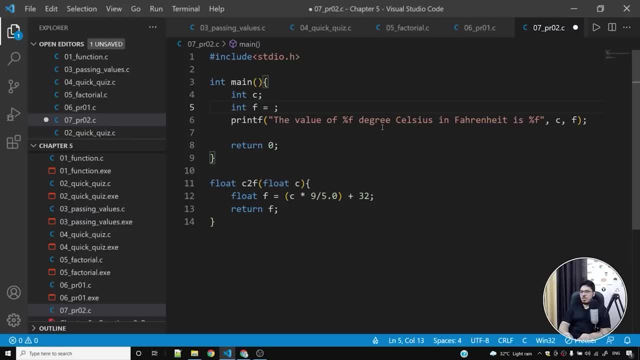 i'm going to use this function. i'll say int f is equal to c to f and i'll pass in the c. that's it. and also i'll convert this to float and let me say: float c is equal to zero, so c is zero. let's see what we get. okay, so i i need to put. 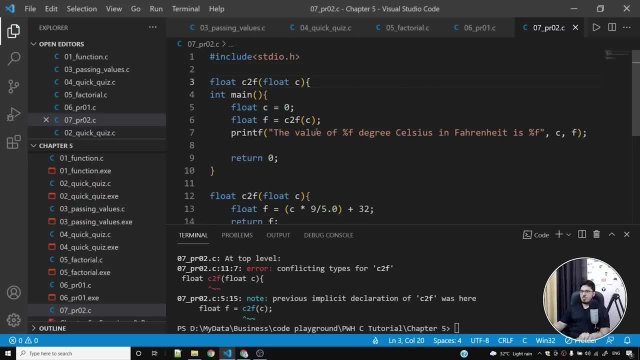 this: uh, let me do something like this. i'll say 0.0, i'll simply use float here, and this is the function prototype. it will apply to these values, to this value. let me run this program now. and the value of this much in fahrenheit is this much? how much is uh, 37 degrees celsius in fahrenheit? let's check that. so it should. 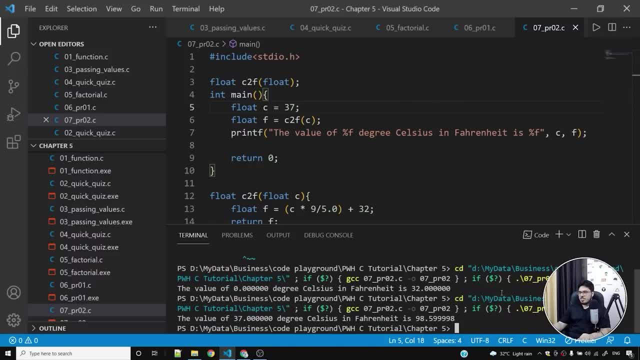 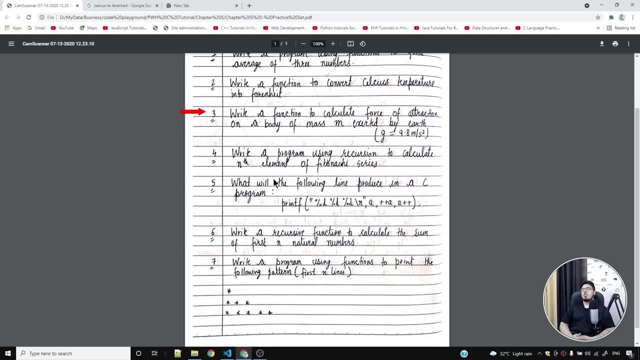 be around 98, and yes, it's around 98 and yes, the program works and, uh, works pretty great. now let's um start with the third problem, which says: write a function to calculate force of attraction on a body of mass m exerted by the earth. so how much is the force exerted on the earth? so this is the. 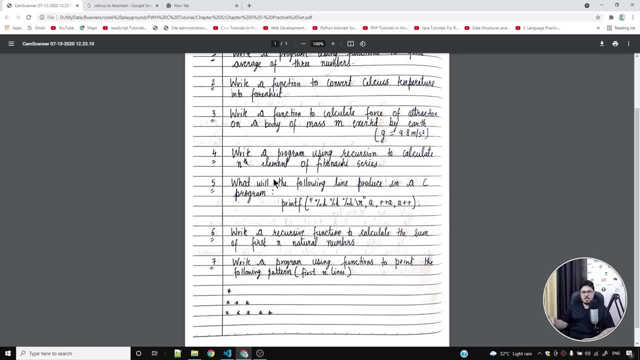 by earth on a body of mass m, the force is equal to mass into acceleration, and here the force is going to be mg. so what we'll do is we'll simply multiply m with g, and i want you to solve this problem, so simply use your visual studio code and write this program. the function should return the. 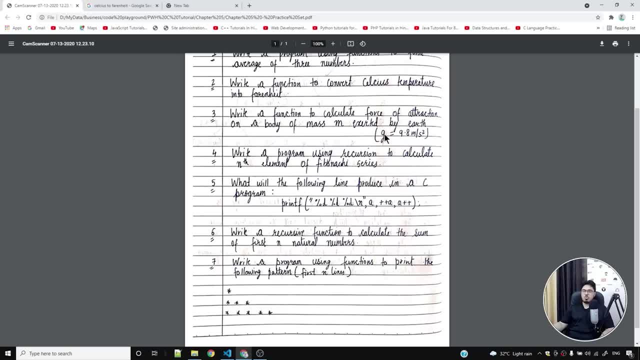 mass multiplied by g, whose value is 9.8. i hope that you will be able to solve this, and this is really very simple and straightforward problem as well. so i want you to solve this on your own and i'll move on to the next problem, and this is the problem i was waiting for. the problem is super. 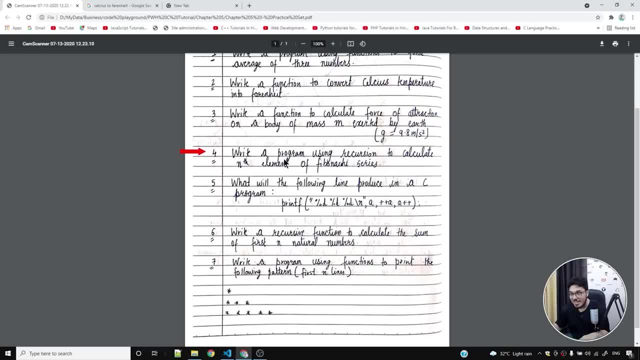 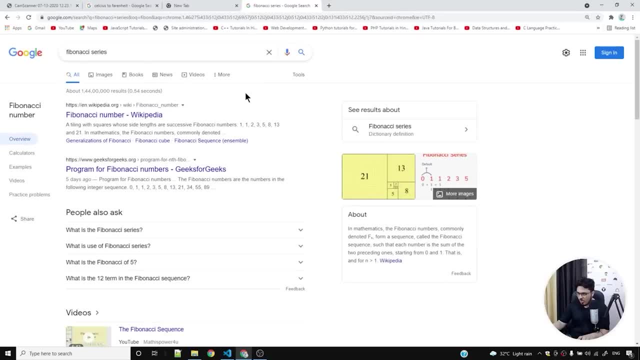 simple. it simply says that write a program using recursion to calculate nth element of fibonacci series. now, in case you don't know what is fibonacci series, let me tell you. so fibonacci series starts from 1, 1, 2, 3, and any next number is going to be the sum of previous two numbers. so if i were to, 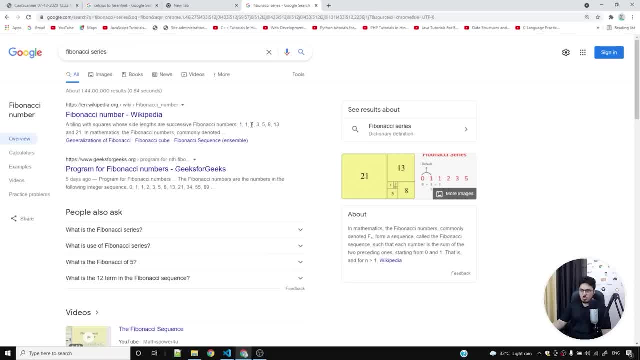 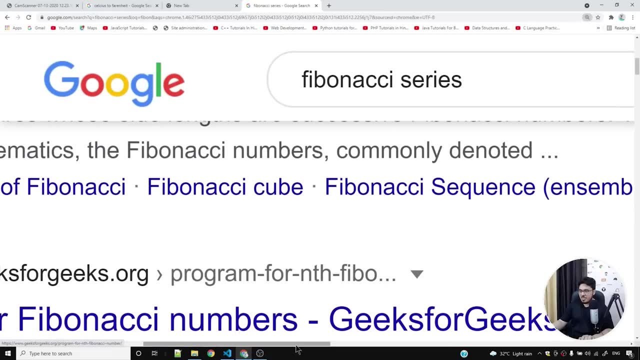 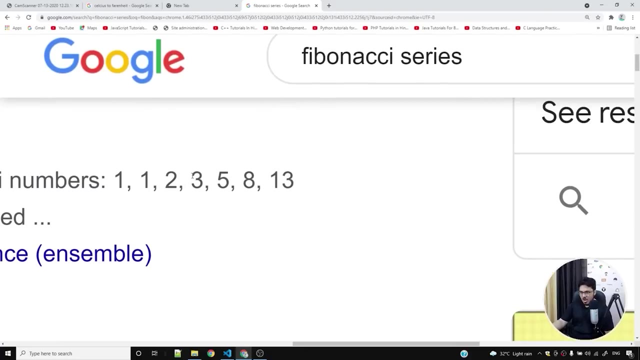 find out. third element of a fibonacci series. it will be 2. how did i get this 2? let me zoom in a bit. how did i get the get to this 2? i simply added the first two numbers. i simply added first two numbers, 1 and 1, and here is the next number of fibonacci series. how to get the next number? i? 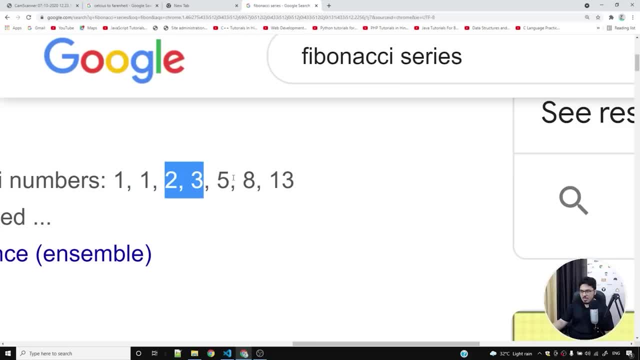 simply add the previous two numbers. how to get the next number? i simply add the previous two numbers. how to get this: 8, 5 plus 3. how to get this: 13: 8 plus 5. how to get the next number. it's going to. 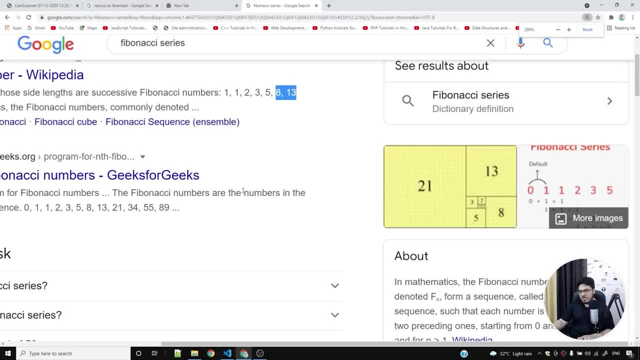 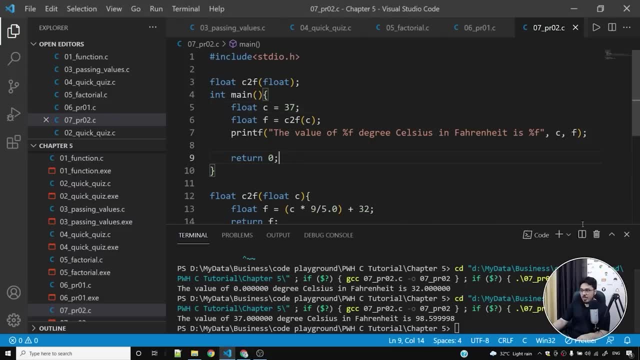 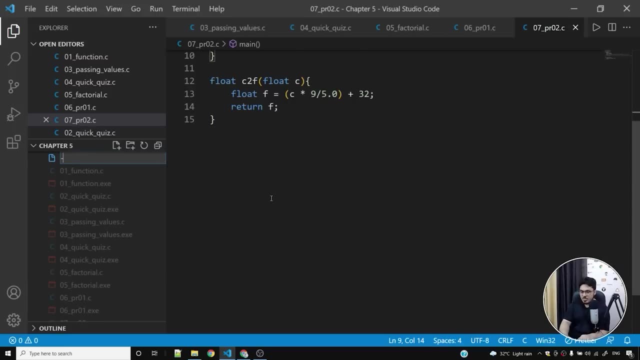 be 13 plus 8, which is 21. we have to automate this, and we are. we are going to use recursion to do this. how do we use recursion? we'll simply write a function that calls itself, and we are going to create a formula for calculating nth term of a fibonacci series. so let's write a program which is program number. 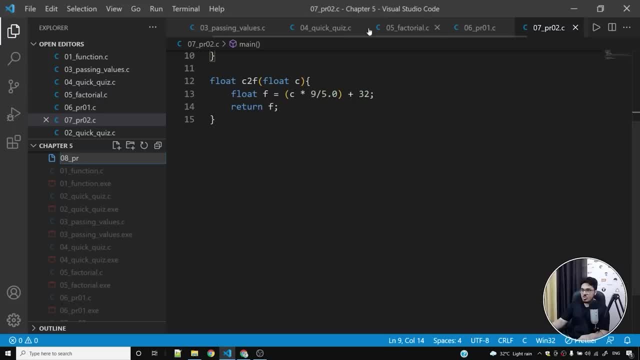 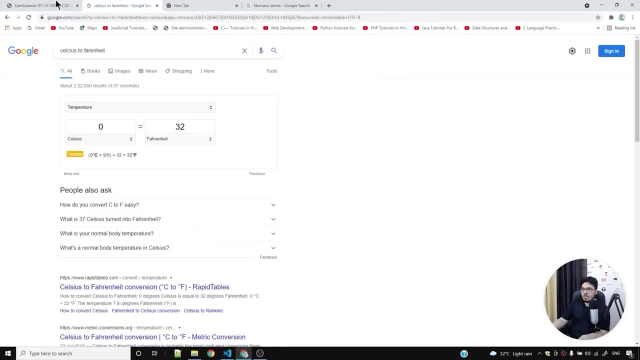 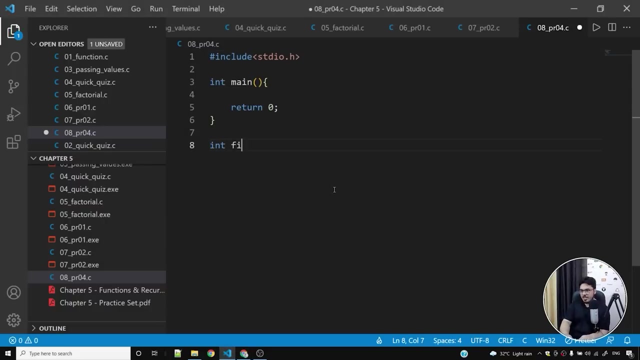 8 of this, of this chapter, and this is problem number 4, if i'm not wrong, and i'm going to write dot c and yes, it's problem number 4. so what i'll do is simply put the boilerplate code first. i'll write a function. i'll say in fibonacci series, element. 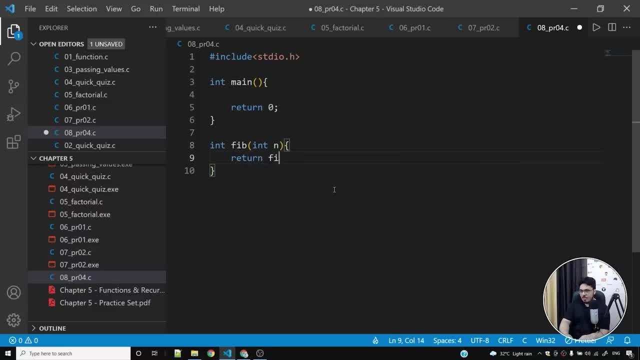 number n is going to be fibonacci n minus 1 plus fibonacci n minus 2. so this is the previous number and this is previous to previous number. so if i add previous two numbers i should get this the nth fibonacci number. and let's start this n with the 1, because i want to count it from. 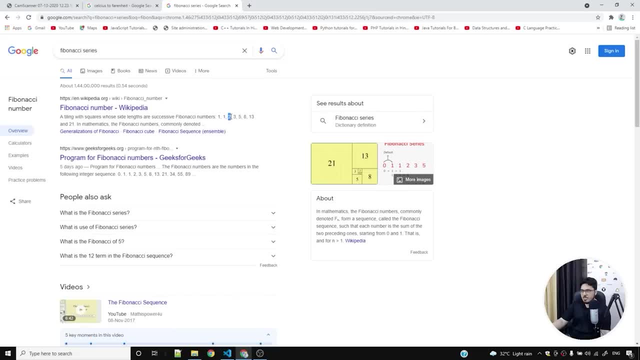 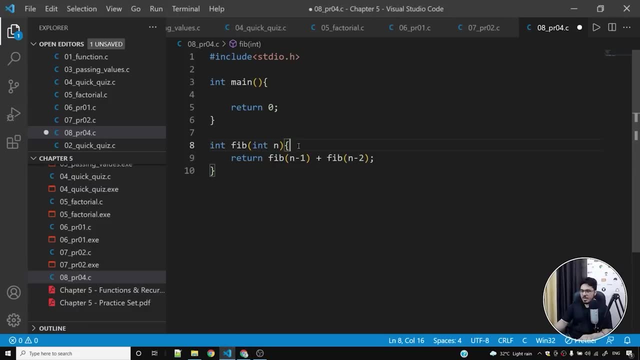 1. the first number is this. second number is this. third number is this. so what is fib 1? it's 1. what is fib 2? it's 1. so what i'll do is i'll simply write a base condition where i'll say: if n equals, 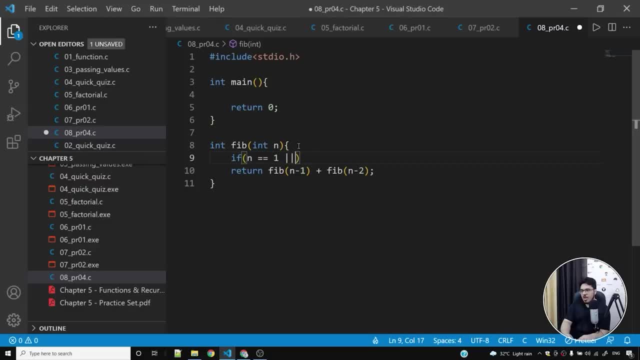 to 1 or or n is equal to 2. what should i do? i should simply return 1, because fibonacci 1 is going to be 1, fibonacci 2 is going to be 1, so i'm returning 1, otherwise i'm adding the previous two numbers. now i can simply say print f. i'll say the. 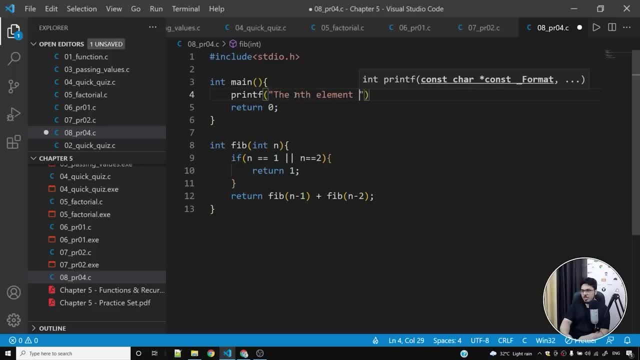 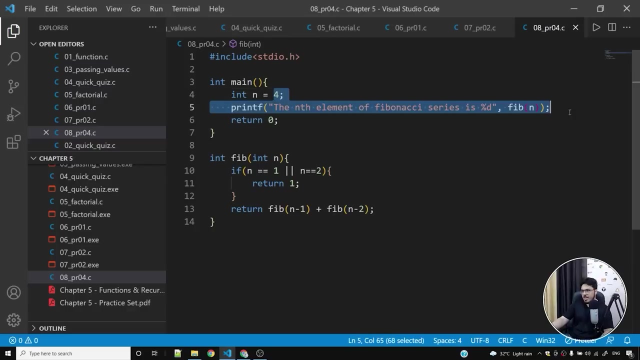 nth element of fibonacci series is percentage d. now what i'll do is simply simply put fib n and i'll create a variable n. i'll simply say n is equal to 4. and now what is? since I have written fib4, how will it calculate? it will simply break fib4 down to fib3 plus. 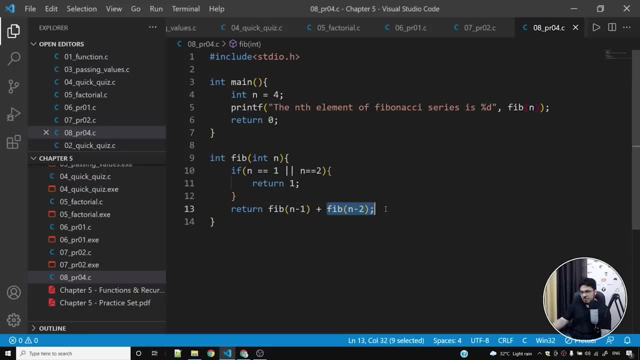 fib2. okay, now it will start to calculate fib2 as fib1 plus. okay, so fib2 is already 1, it will return 1, and so let's see if I am able to get the fourth element of Fibonacci series. I have made some mistake, it seems. what is the mistake? no, I actually selected. okay, so. 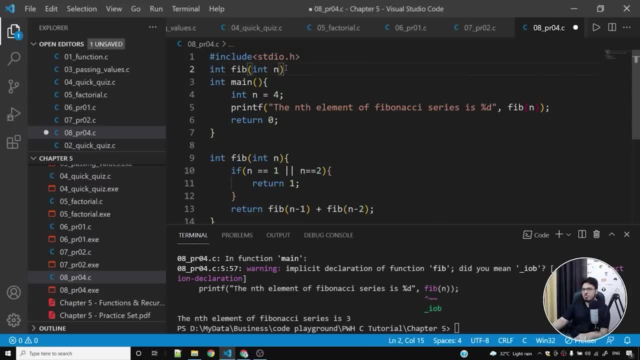 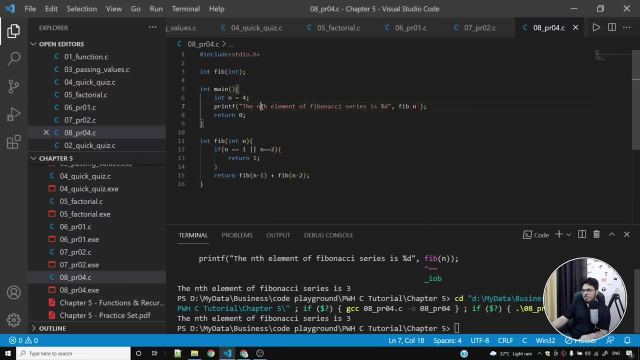 I haven't written function prototype, so let me write function prototype. and let me tell you something: if you write the function before main function, you don't even have to write function prototype, but it's always a good practice to write function prototype. let me save this and let me run it again at the nth element of Fibonacci series, and let me do: 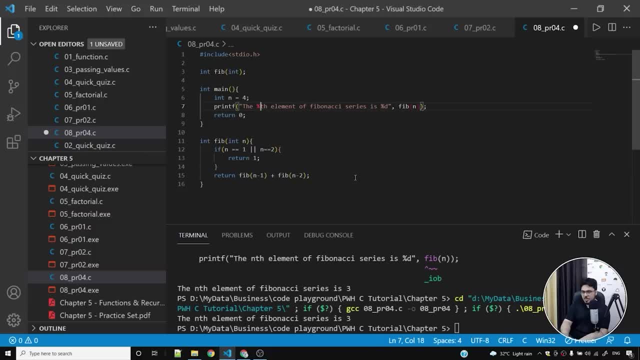 one more thing: instead of doing nth, I will simply say %t and I will simply say n, so that I can say that the element 4 of Fibonacci series. let me get rid of this %t from here and let me format it like this: so: element 4 of Fibonacci. 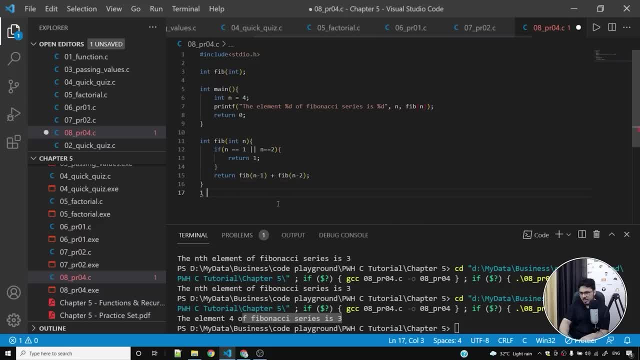 series is 3, is it true? let me check. so 1 and 1, then 1 plus 1 is 2, then 2 plus 1 is 3, so fourth element is 3. indeed, how about let me generate Fibonacci series? then 3 plus 2 is. 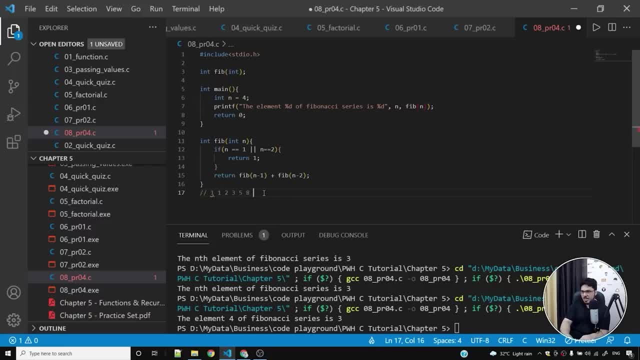 5, then 5 plus 3 is 8, 8, then 8 plus 5 is 13, then 13 plus 8 is 21, and so on. this is a Fibonacci series. let me now run this program, for n is equal to 8. ok, run this. n is equal to 8. 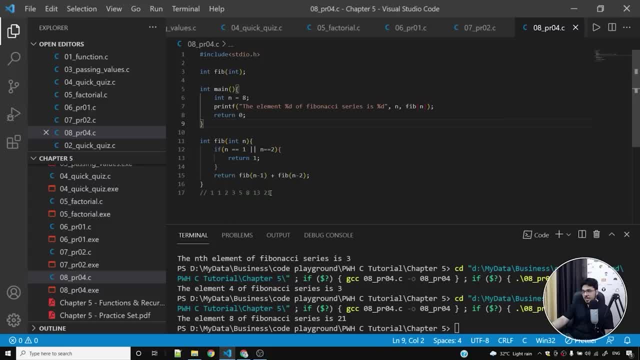 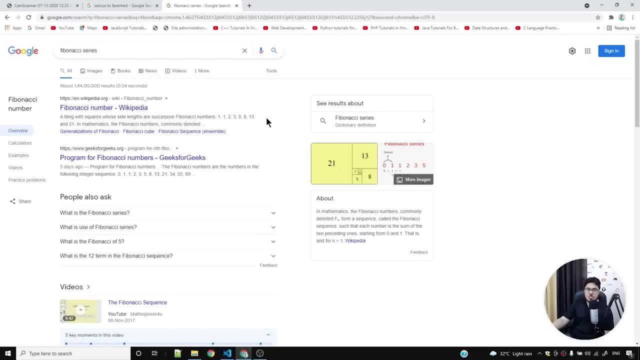 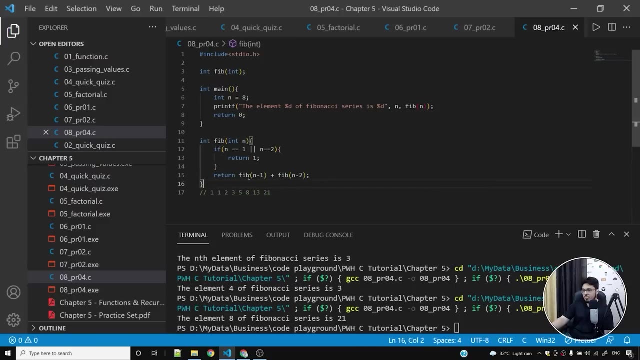 and 8. th element is 21: 1, 2, 3, 4, 5, 6, 7, 8. yes, it's right. so this way we are able to find the next elements of Fibonacci series using recursion. so recursion is a function that calls itself. in case you are still wondering how I got to this equation, Fib n minus 1 is 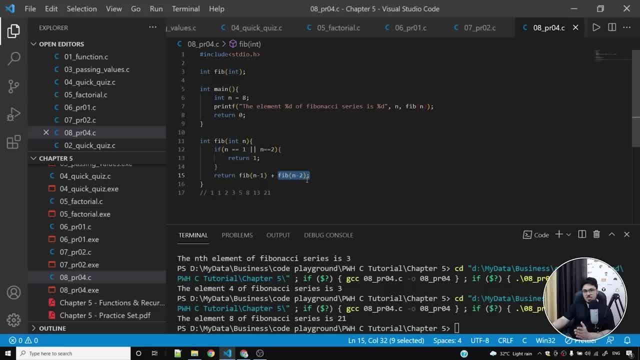 a previous number and Fib n minus 2 is a previous number and Fib n minus 3 is a previous number and fib n minus two is the previous to previous number. okay, so if we add these two numbers, we are going to get the next number, and this is the base condition, which simply says that the first and the 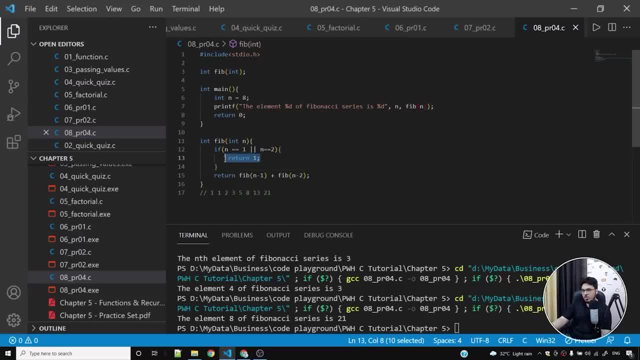 second element is going to be one, and since i have already told you that return one will simply stop the function execution. so as soon as a function sees return, it will halt there itself. it will not execute any further instruction. so in case you are wondering if this is executed, i mean if return- 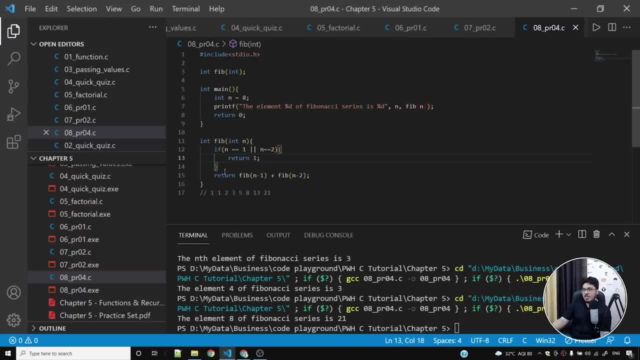 one is met by the c compiler, will this line also get executed, or something else which is below return will get executed or not? no, it will not get executed. so if i'm writing anything below return, it's not going to get executed, just because return means finish the function call. that's it. 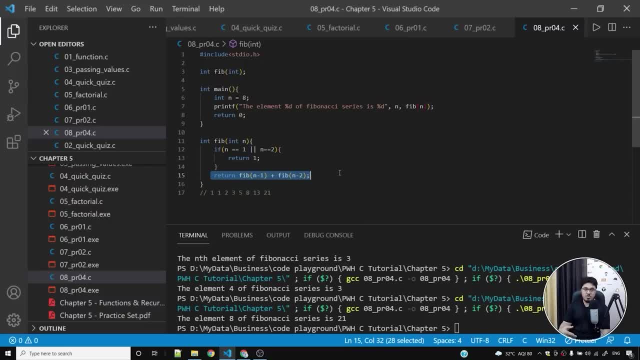 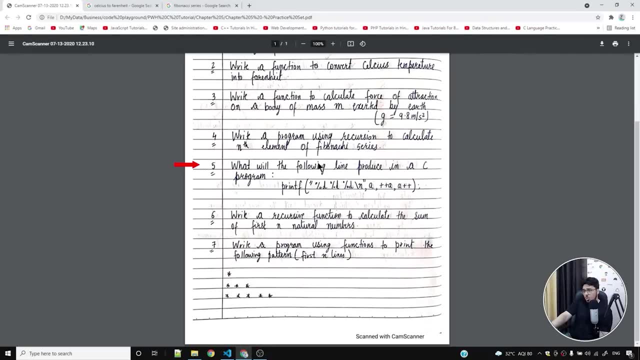 we got the value we needed and we are not going to run this function anymore. okay, so i hope you were able to understand this. let's now move on to the next question, which says what will be the following: uh, what will the following line produce in a c program? so, 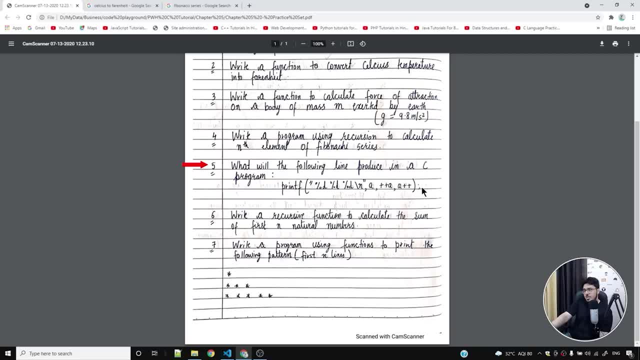 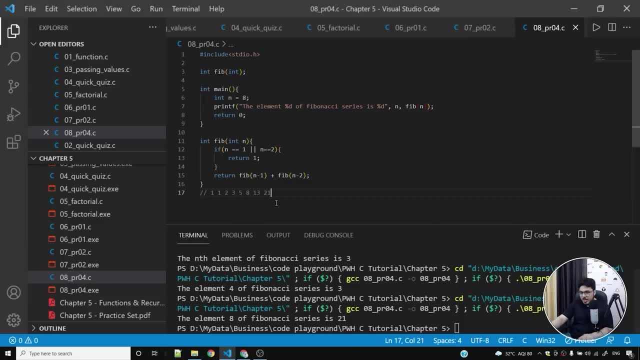 we have to find. what will the following line produce in a c program? let us assume the value of a as three and let's let's try this out. so what i'll do is i'll simply copy this program and i'm going to write program number nine, which is problem number five, and 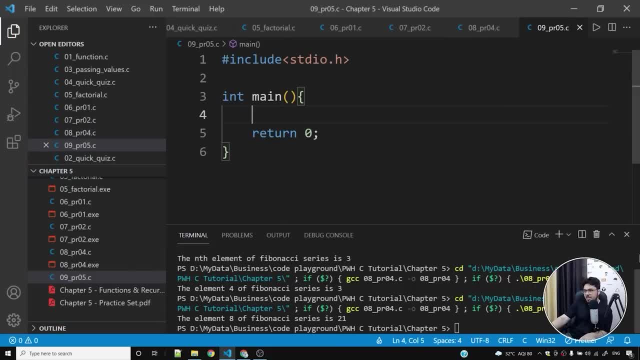 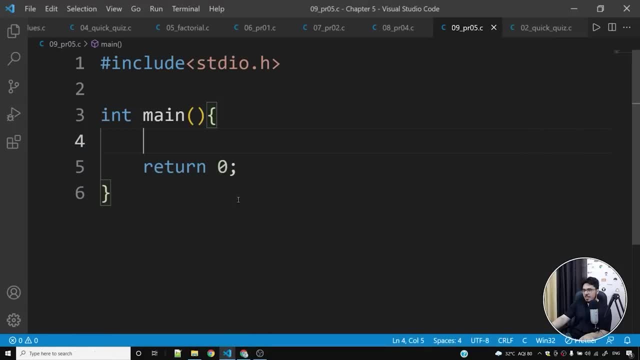 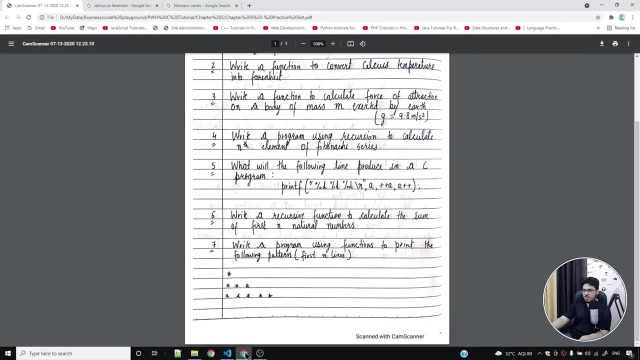 okay, i'll simply add boilerplate code here and also what i'll do is i will. i will simply type this printf: three percentage d. i'll say percentage d, percentage d, percentage d, and what i'll do is three percentage d, then backslash n, backslash n, backslash n. now what i'll do is i'll type this: 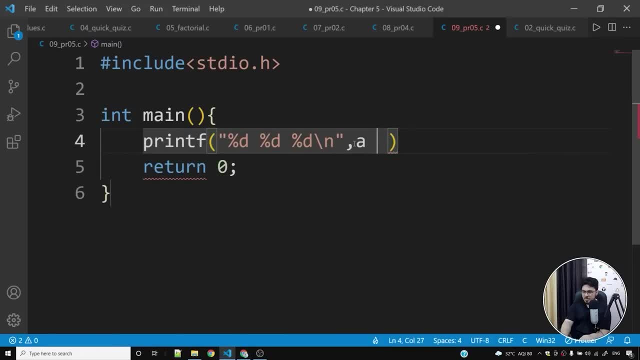 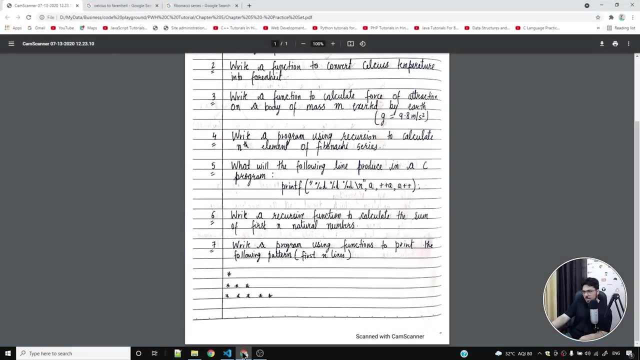 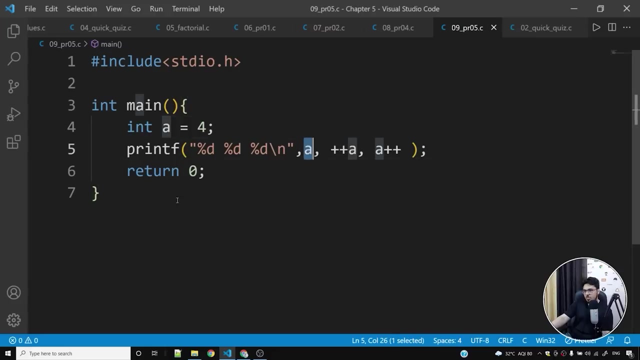 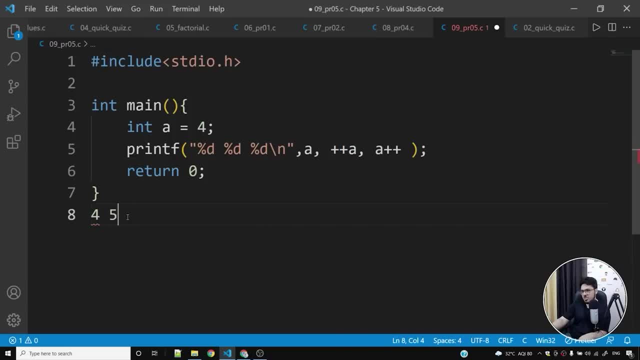 increment the value of four to five and then print the value of a, which is five. but since the value of a is now five, a plus plus will first print the value of five, then increment it to six. so now the value of a is six, but we are not printing the value of a anymore. so if i comment this out now, you must be thinking that this is the final answer. i'll show you something. if i run this program, you'll see that six, six, four is being printed on the screen and you must 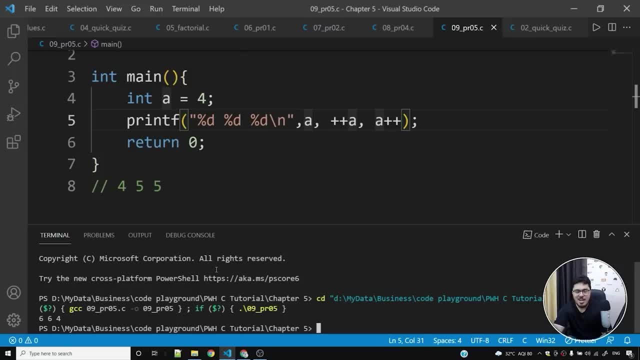 be thinking: what is happening? what is this? and let me tell you something: why this happens. and also, i want to tell you something which is also very important. if you are tackling such questions in an interview, okay, first of all, writing such a statement in your c program is not at all recommended. 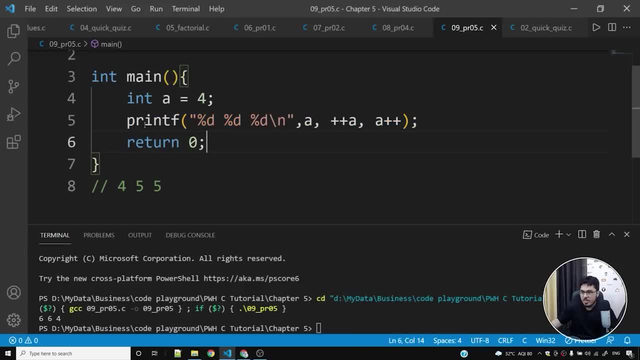 because different compilers are going to deal with this particular line in different ways. one way to evaluate this was this, where we got four, five and five as the answer, but it turns out that the compiler which is installed on this machine is decoding this as this, so we'll we'll try to. 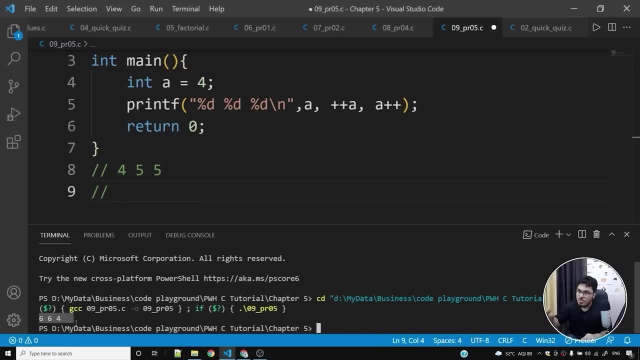 understand why six, six and four is the output of this program for this compiler. what has this compiler done to get to this output? and then we'll talk about whether you should answer these questions in an interview in this way or not. okay, okay, let's get started. so. 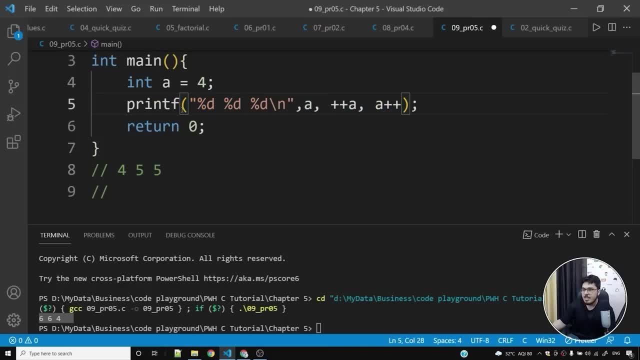 what this compiler is doing is. this compiler is basically receiving a plus plus a and a plus plus as an argument of printf. what happens is this compiler is designed in a way that it evaluates all these three lines from right towards the left. okay, so a plus plus will be evaluated first. 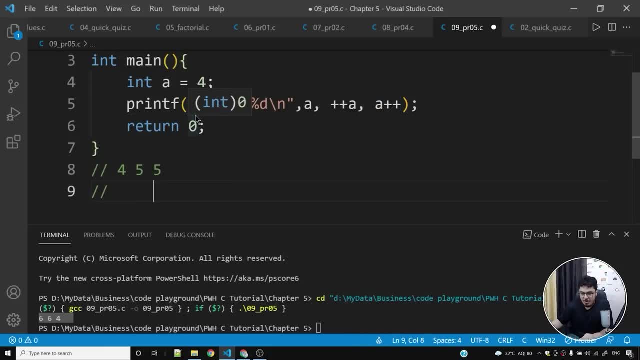 so a plus plus will be evaluated first and a will be printed. four will be printed then, since the value of a is now five. a plus plus means that print value as four and make the value of a as five. now when i say plus plus a, the value of a becomes six and six is printed because we are incrementing first and 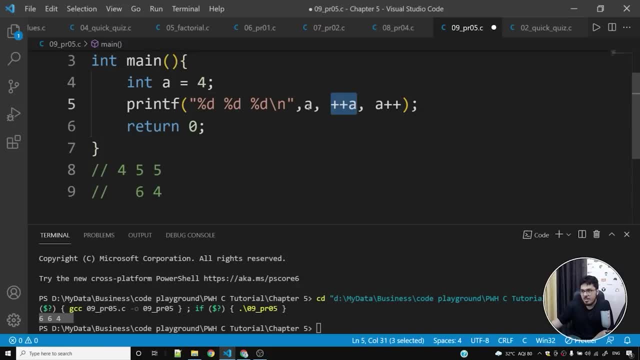 then printing, so five becomes six and six is printed. and when i print a, the final value of a is printed, which is nothing but six. so hence the output. but what if you get this question on a whiteboard? you should reply that compiler might either choose a or b or b plus, or b plus or b plus. 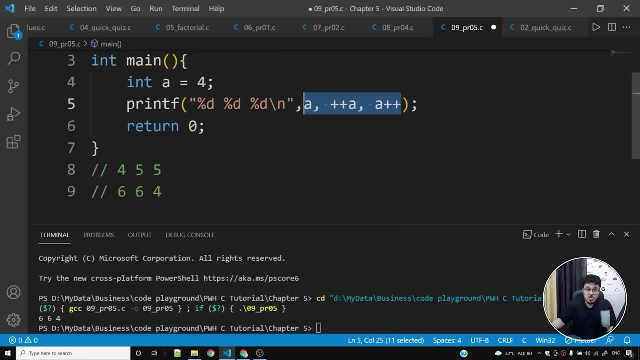 to. you know, either choose to resolve these three lines from right to left or left to right. one of the smartest way to solve this problem is you can tell your interviewer that i can solve it from left to right, and most other people are going to solve it left to right, so i'm going to solve. 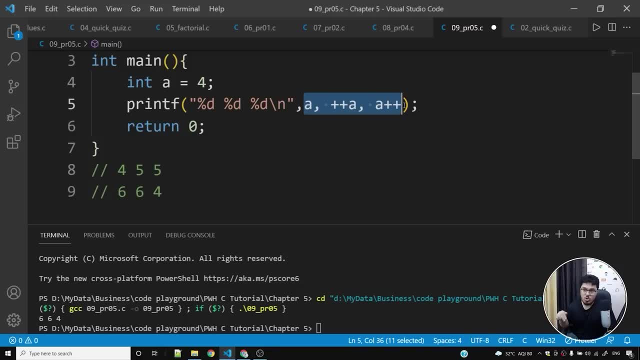 this right to left inch way to you. this way your interviewer will know that you know all these concepts. you understand that a compiler might deal with this particular line in a different way. writing a c program: never, ever, use such kind of thing inside a printf statement because different. 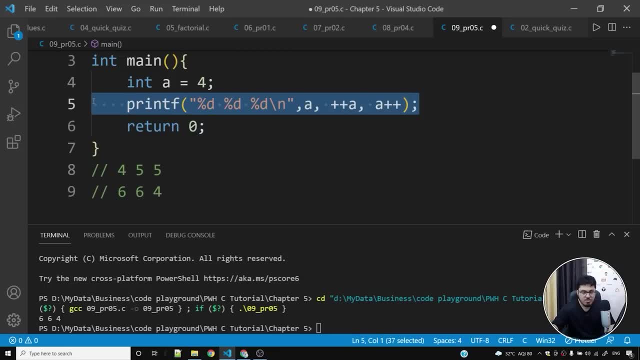 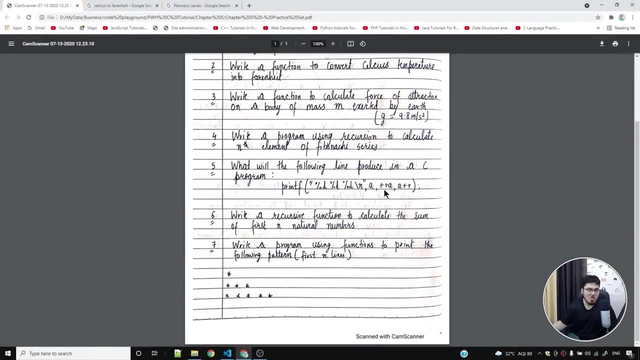 kind of compilers might look at this code in a very different way. so i hope that this question helped you a lot and you were able to understand intricacies of printf and increment operators. the next question says that find a write a recursive function to calculate sum of first. 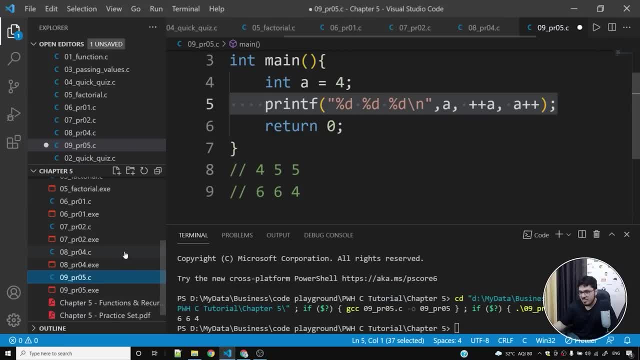 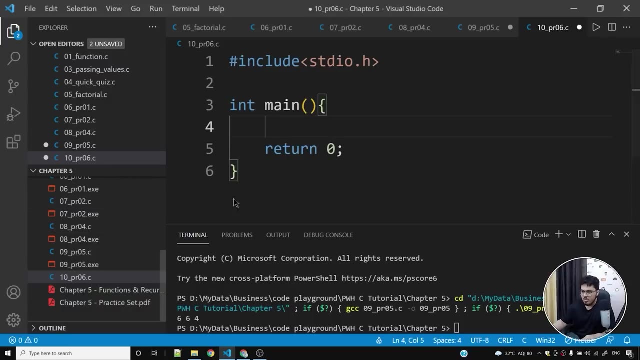 and natural numbers- recursive function. right, okay, let's write it. let's solve this problem. this is problem number six. program number ten: 10, underscore: pr06 06 dot c. let me write the boilerplate code and let me try to see what sum of first and natural number is. it's nothing but one plus two plus all the way till n, so we'll have. 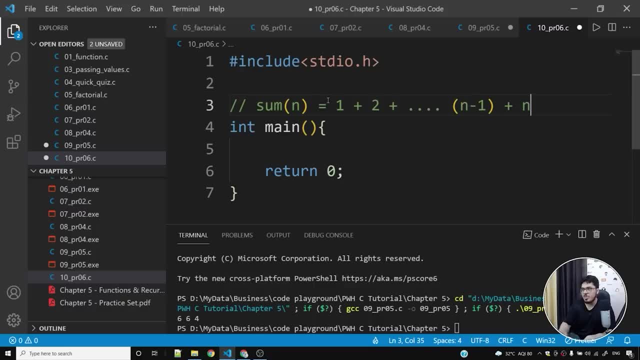 n minus one somewhere here, and then we'll have n. okay, this is how sum is calculated. okay, can i not write: sum of n is equal to sum of n minus one plus n. can i do this? yes, definitely, i can do this, and our recursive function is ready. so what i'll do is i'll simply say: in sum n. i'll say: 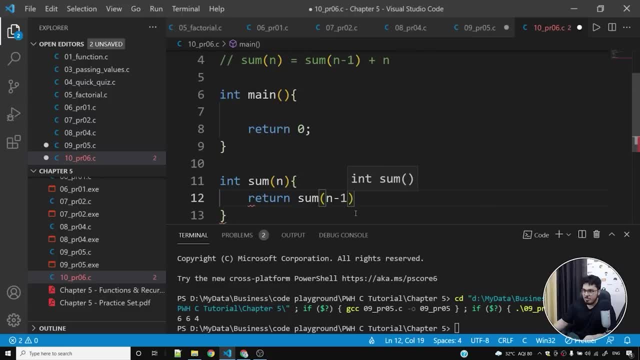 return sum of n minus 1 plus n. so that's all. but i'll have to define a base condition. i'll say: if n equals to 1, what you do is you return 1. so the moment we start receiving 1 as the input, what will happen is the moment it becomes sum 1. 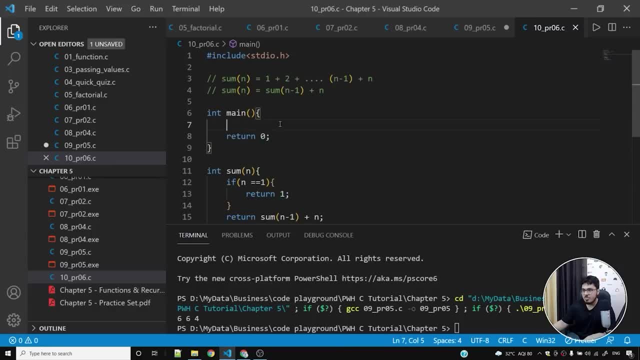 we are going to get 1 as the output. let's see if this works. i'll say printf and then i'll say: sum of first five natural numbers is percentage d and i'll simply say sum 5 and i'll put a semicolon. let's see if this works. i'll save that and then i'll save the output. so let's do that and i'll say: 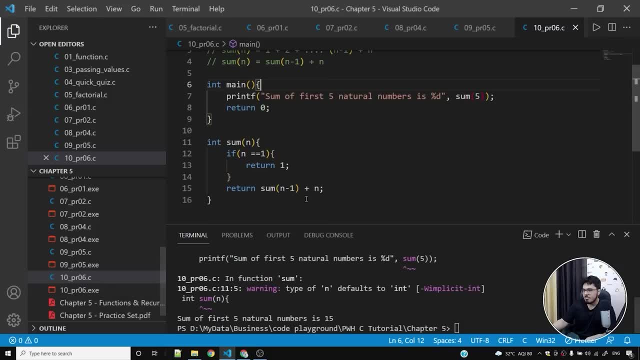 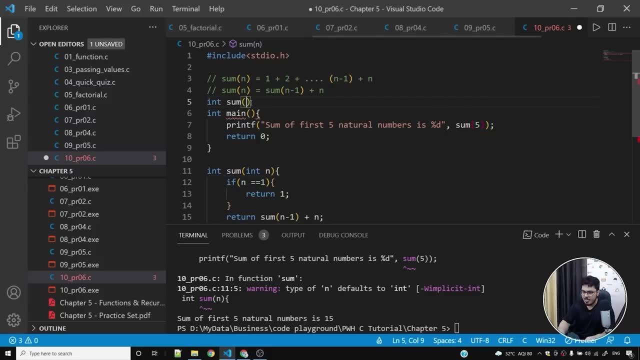 some of first five natural numbers is percentage d and i'll simply say some five and i'll put a semicolon: this program as well. uh, the moment i run this. okay, so i need to write function prototype and also i should write int here. my bad, i should write int here like this: and yes, this should work. now let's. 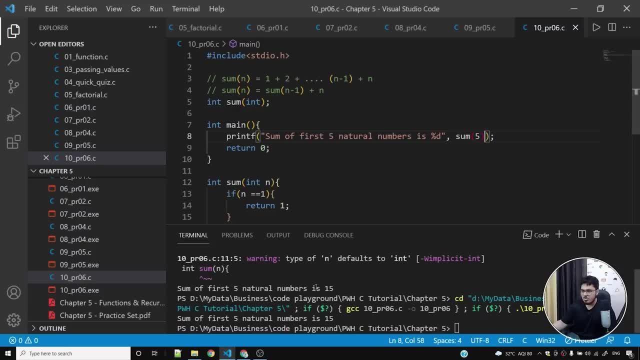 see what it gives me. so is 1 plus 2 plus 3 plus 4 plus 5, 15. let's check. so 1 plus 2 is 3, 3 plus 3 is 6, and then 6 plus 4 is 10, and 10 plus 5 is 15. and yes, we are right. okay, let's try to find sum of. 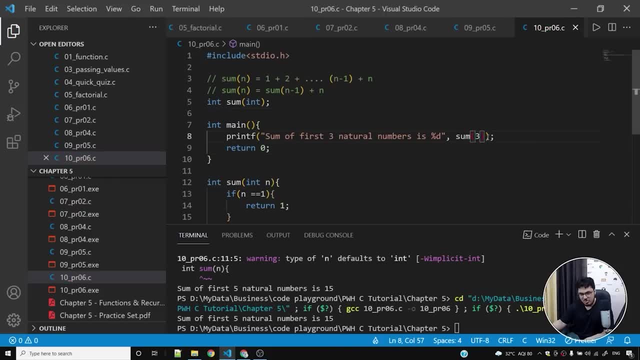 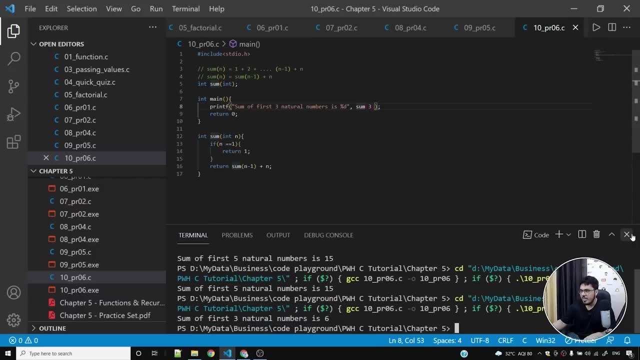 first three natural numbers and i know for sure that sum of first three natural number is six. so if i run this program you'll see sum of first three natural numbers is six. so all it takes to solve a problem using recursion is to come up with a recursive relationship and plug it into. 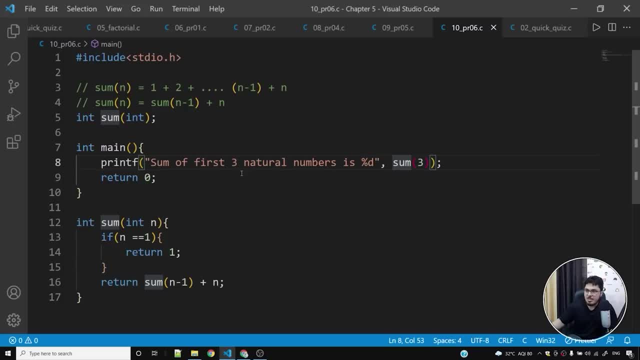 the function and that's it. you just type the mathematical formula in a very smart way inside a function with a base condition. this is important: always use a base condition, because if you don't use base condition, you you are, you are going to deal with a lot of problems. your function. 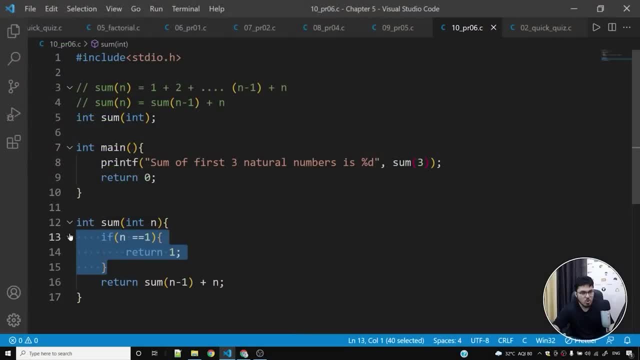 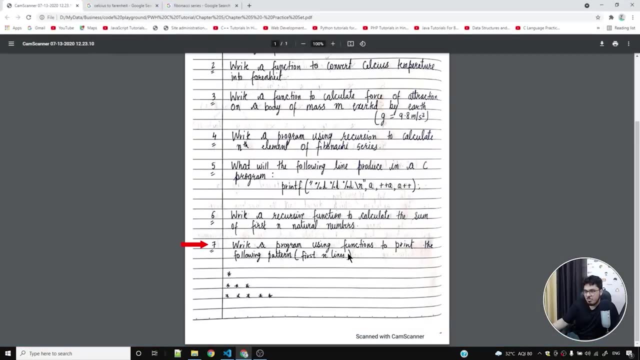 might keep on running indefinitely, and you would definitely not want that. okay, now the last problem, which is write a program using functions to print the following pattern. so you have to print first n lines of this pattern. what is this pattern, by the way? so the first line contains, or rather first: 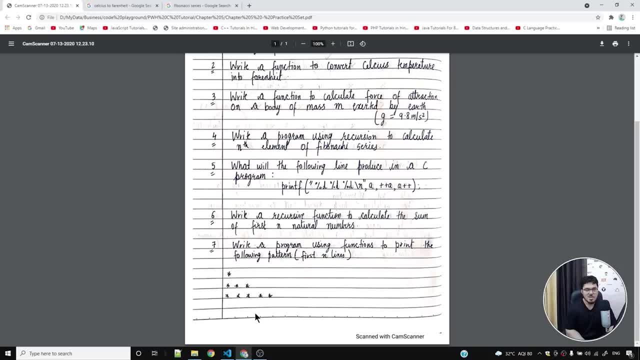 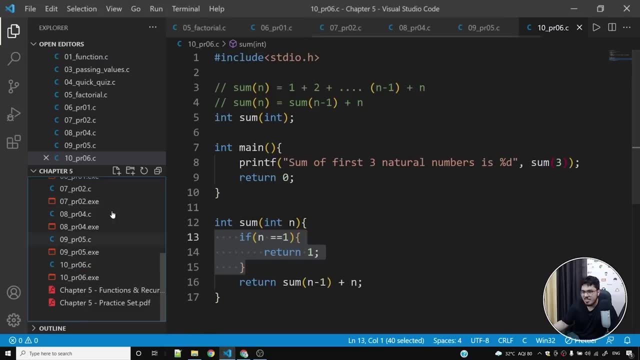 line contains only one star. the second row contains three stars. the third row contains five stars. so i i will have to generate the odd number one, three, five, seven, nine and so on, and i'll have to print those many stars. let's see if i can do it. i'll give it a try. 11 underscore, pr07, dot c. 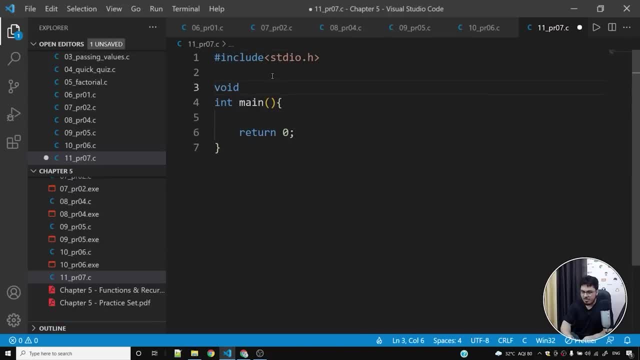 boilerplate code i. i'm going to give it void, star and int and i'll say void star, int n. all the logic will come here and i'll simply call star four. let us say okay. so i have to write first n line. so definitely, i'm going to use a for loop. 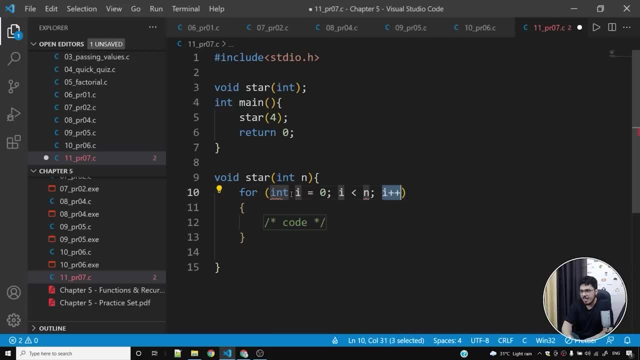 i'll say: int. i is equal to zero, i is less than n. i plus plus. and after that, what i'll do is i'll simply print a backslash n. and you must be thinking what i'm doing, how i know that i have to print a backslash n. so the thing is, all i need to do is 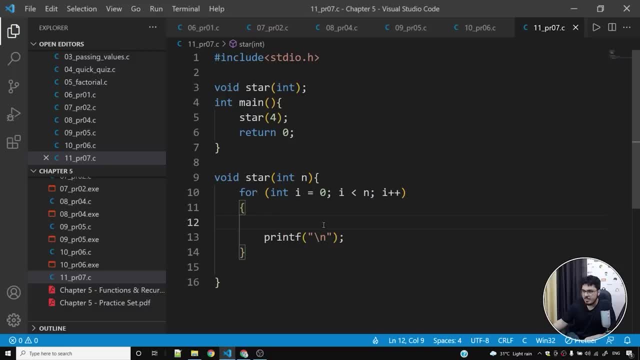 i just have to- you know, print. i'll simply write down in very plain and simple english. i'll say print two n minus one stars, or rather two n plus one. sorry, because i'm starting my eye from zero. what does it mean? here i'm saying print two n plus one stars. 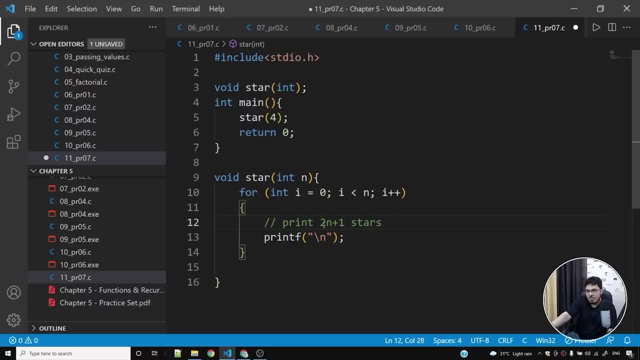 so whenever you have to write a odd number in the form of n, what you do is- or let me change it to 2i plus one, because we are starting i from zero. two i plus one stars means when i, when the value of i is zero, this will be one. when the value of i is one, this will be three. then, when the value of i is two, 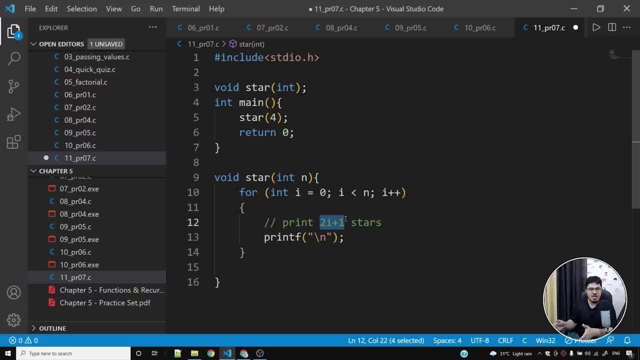 this will be five, so we are able to generate one, three, five, seven, nine using two i plus one. i hope you understood that. now. i'll simply replace this with a loop and i'll simply say: for j is equal to zero, j is less than two multiplied by i plus one. what is this two? 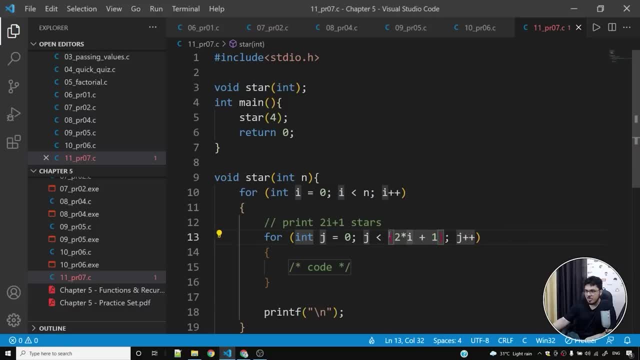 multiplied by i plus one, this will result into uh 2i plus one star. so if i have to print one star, this, this will be one, and then for the next iteration it will be three, then five, then seven, then nine. and here what i'll do is i'll simply say: 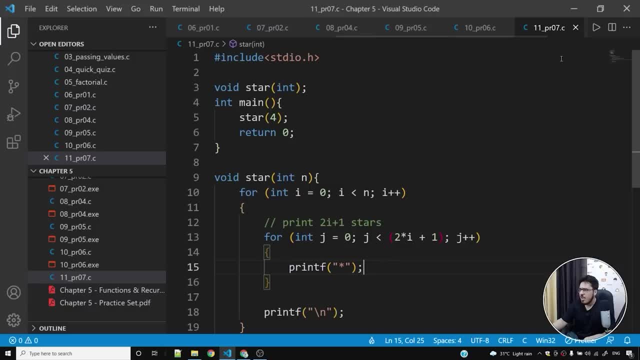 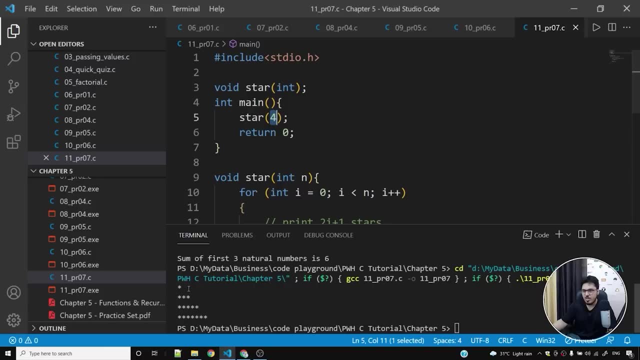 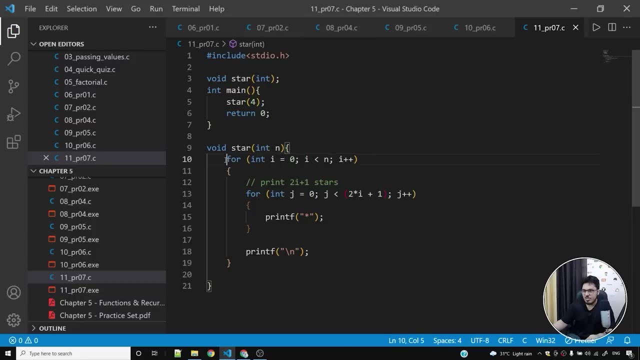 print f star semicolon. and the moment i run this, you'll see that i am able to get the pattern that i wanted. so, for the value of n is equal to four. i'm getting four lines once again. if i were to tell you how this works, i am calling this function here and inside the function. what i'm uh doing is: 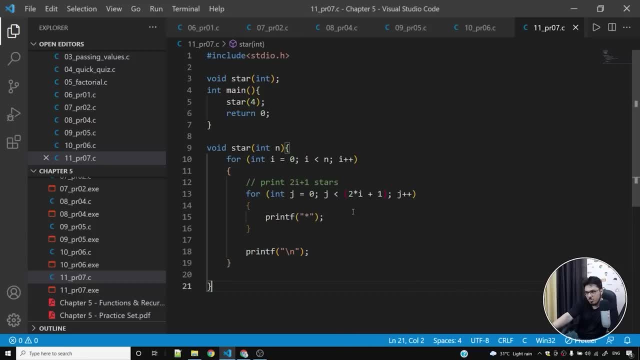 i'm having a nested for loop, so our for loop inside a for loop. what this for loop is doing is it is generating the value of i all the way from zero to n minus one. okay, so if the value of n is four, it is generating zero, one, two and three. now 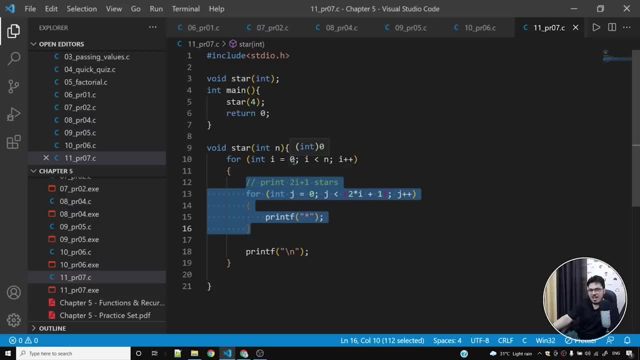 what this for loop is doing is. it is using those values of i, which is zero, one, two and three, and generating one star, three star, five star, seven star, nine star, odd number of stars for me. okay. so how this works is i'll use in: j is equal to zero, j is less than two plus one. 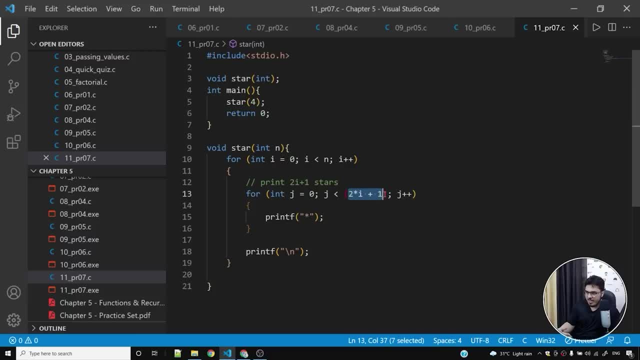 2i plus 1 means odd number. so when the value of i is 0, i get 1. for 1, i get 3. for 2, i get 5, and so on. for 3, i'll get 7. if you plug 3 here, you will get 7. so this is the odd number. so we are. 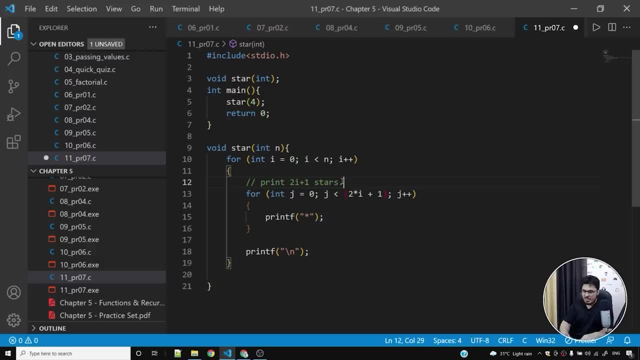 printing stars: odd number of time. 2i plus 1 will yield. let me write it here: 2i plus 1 will yield 1, 3, 5, 7, 9 and so on, for i is equal to 0, 1, 2 and so on. okay, so this is how it works. i hope i was. 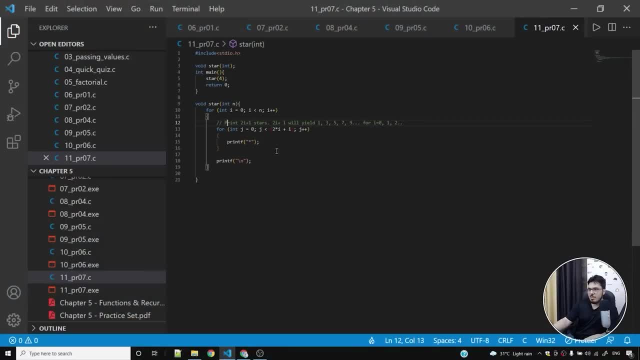 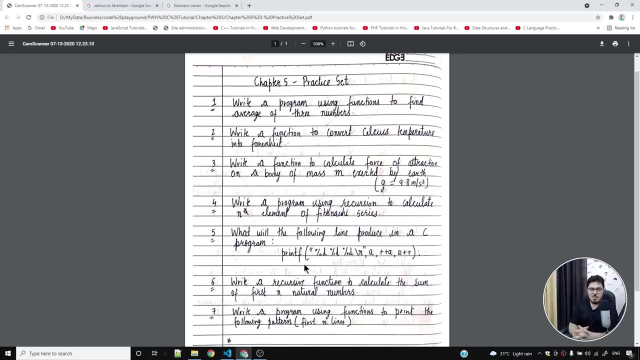 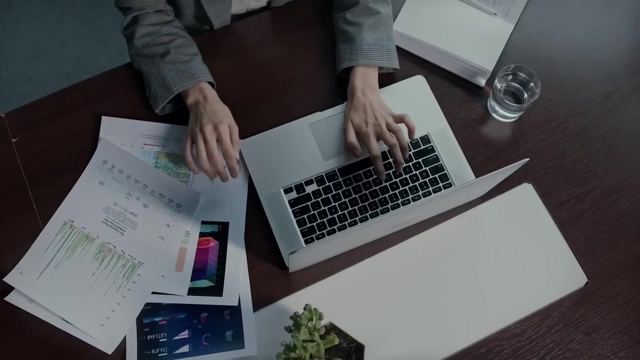 able to explain this to you and you were able to print the star pattern yourself. so if you get some other star pattern in the future, i hope you will be able to print that. so this was all about the star patterns, the functions, recursion. we learned a lot of stuff in this chapter. i hope you enjoyed this chapter. let's now move on to the 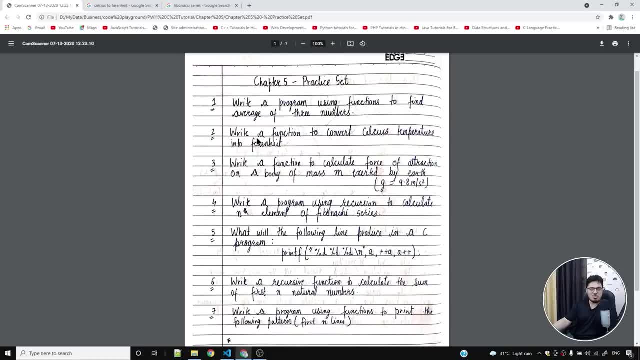 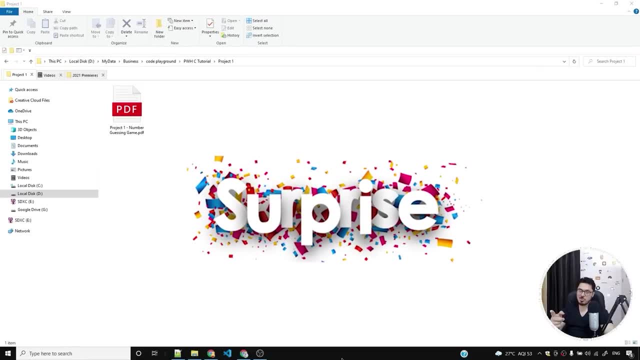 next chapter and we'll understand more concepts of c. let's move on to chapter 6 now. now, before we move on to the next chapter, i have a surprise for you. we are going to solve this project and this is going to be our first game. if you are new to programming, this is going to be the first ever. 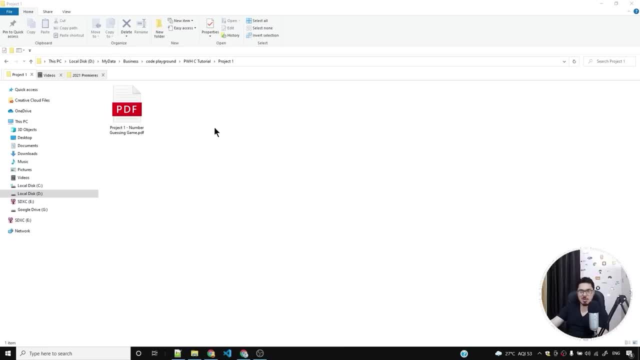 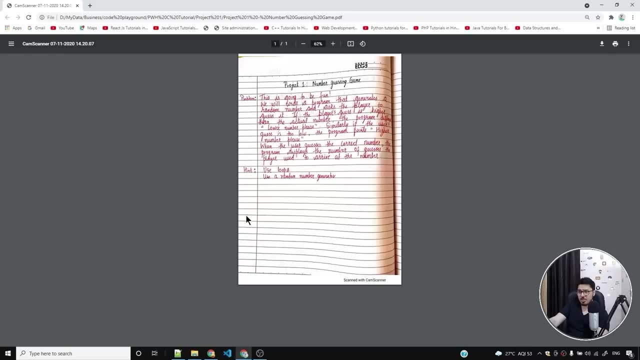 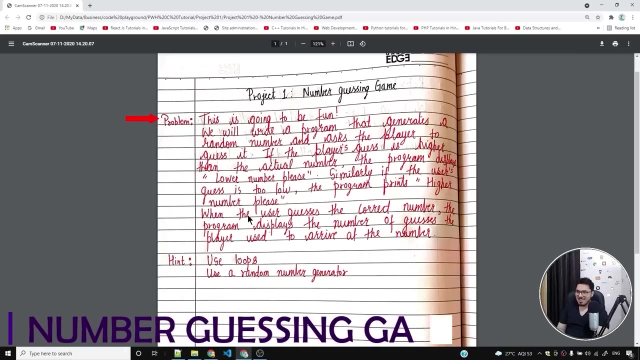 game of your life. so congratulations. once you complete this game, you'll be able to showcase it to your friends, or maybe you can put it inside your resume. let's see what this question has to say. so this project number one number guessing game says that this is going to be fun indeed. we will write a program that generates a. 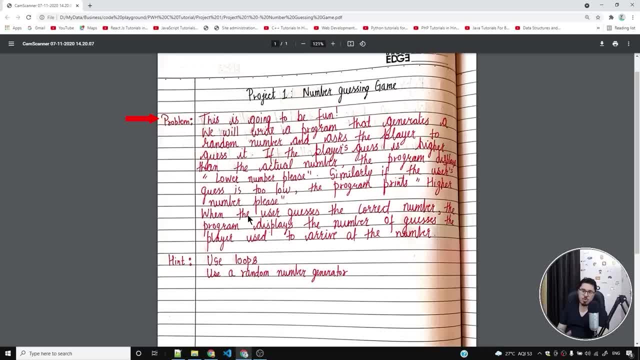 random number and ask the player to guess it. so what we are going to do is we are going to generate a random number and then we'll ask the user to guess it. so let us say i'm generating a random number between 1- 200 and i ask you to guess it. let us say the number is 50. uh, you, you might guess 60. 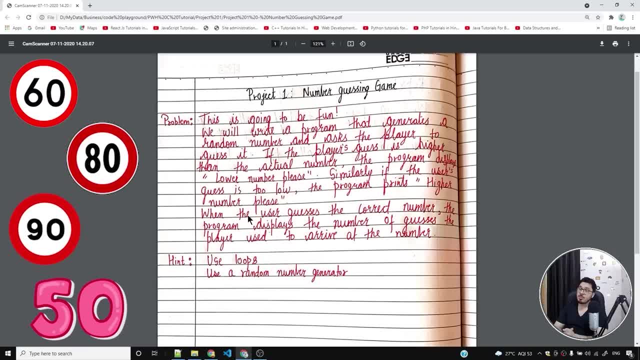 or 80 or 90. the actual number is 50. and then we're going to generate a random number and then we're going to say: the number is 50. now what will happen is if the player's guess is higher than the actual number. so let us say you guessed 66, the number was 50. what i'll do is i'll tell you whether your 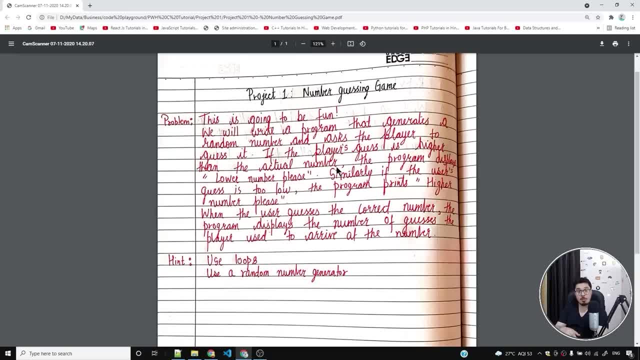 guess was greater than my number or lesser than my number. this will help you guess it correctly the next time. so if the number is 50 and you said 66, so next time you will not say 67 or 70 for that matter, because you know the number is lesser than 66. so you might give it a try and say: 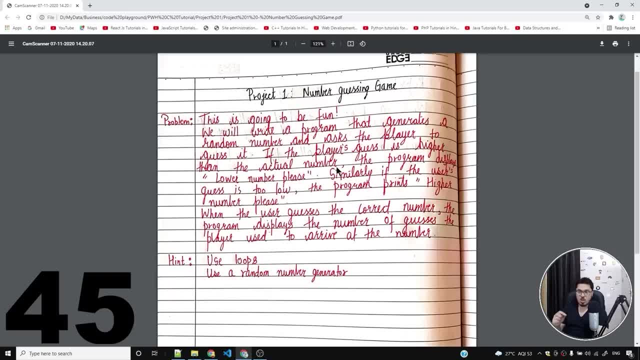 45. now i'll tell you that no, the number is not lesser than 45, it's actually greater than 45. so you'll say: okay, so it's between 45 and 66 now. so you might guess 49. i'll again tell you that. 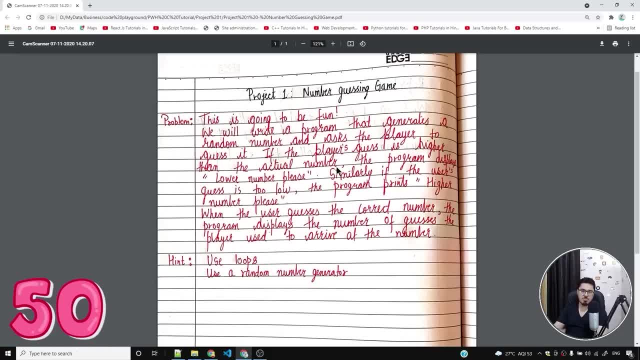 you need to increase it and eventually you'll reach that number. you will tell me 50 and, yes, 50 will be the number. so the number of guesses that you took will tell me your ability to guess a number correctly, and the number of guesses you took will be your guess and the number of guesses. 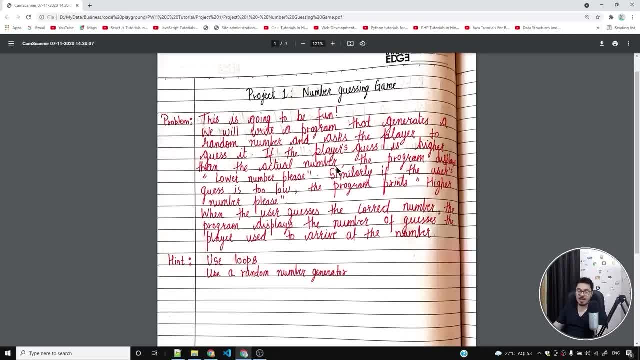 will be your score. now, if somebody else has guessed it in lesser number of guesses, he'll be the winner. okay, i hope that you understood what this problem is about. the fun is not in the game itself, to be honest, it is in the code. it is the fact that you have created the game and you are 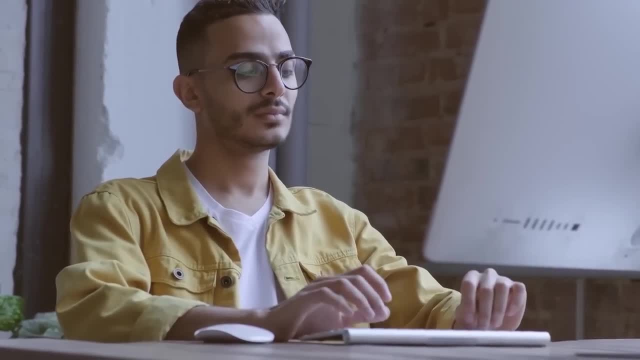 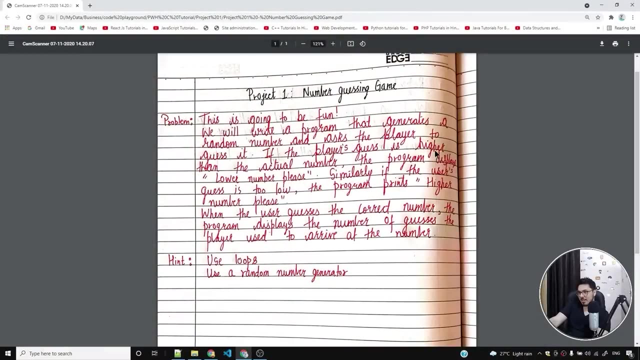 the creator of the game that you are playing. that feeling, that feeling of you know the creator of the game that you are playing, is going to be absolutely brilliant, believe me. so if the player guesses the number is higher than the actual number, the program will display no number, please. 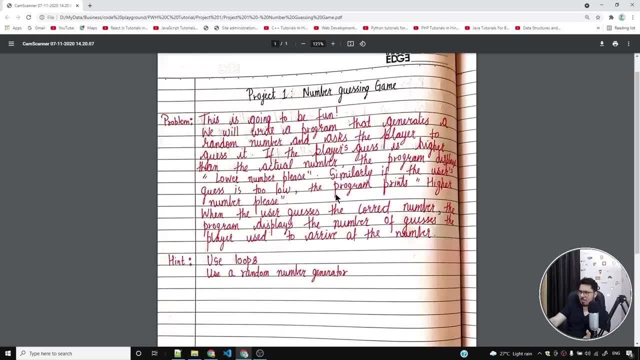 similarly, if the user's guess is low, the program is going to print higher number, please. when the user guesses the number correctly, the program displays the number of guesses the player used to arrive at the guess okay. so the hint says: use loops, use a random number generator. now you might. 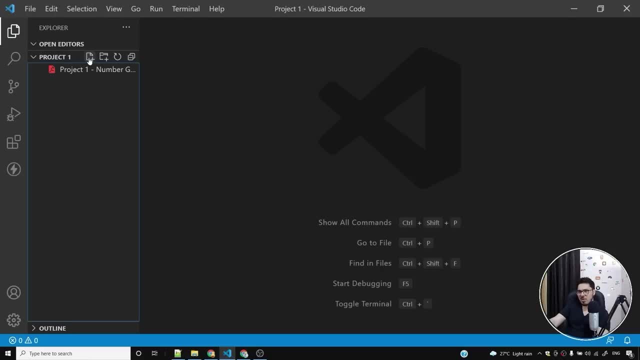 say, harry, you didn't tell me about random number generator. so what we are going to do is we are going to talk about random number generator, dot c: how do you generate a random number in c? so let me put in a boilerplate code for you, and now i'll discuss about how to generate. 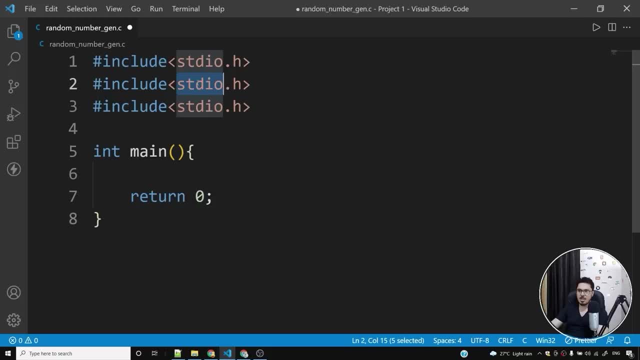 a random number in c. so in order to generate random number in c, you need to include couple of libraries. so the first one that we are going to include is std lib and the other one is timeh. now what i'm going to do is i'm going to say a number. this is the number that i'm going to. 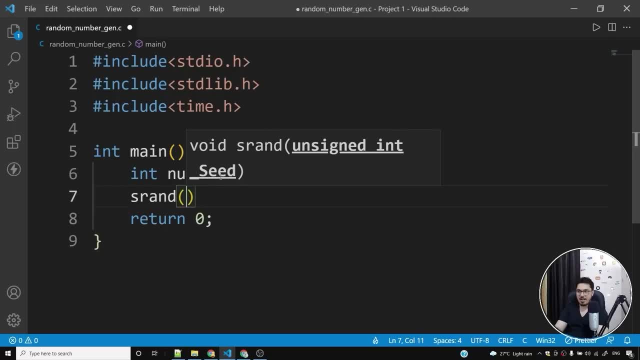 generate randomly and i'm going to use a function called srand and srand is going to take an unsigned number. so let's say i want a random integer, i'll take the system time. so time 0 is a function from timeh which is going to give me a random number. time- the current time is going to be very random. 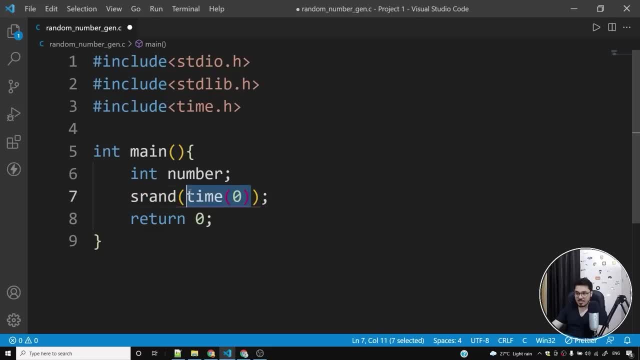 okay. so why do we do this? why do we say srand time 0? because this is the seed. this is the seed of my random number generator. so if the seed is same, i'm going to generate exactly the same random number. so let me show you how to generate a random number first, and then i'll come back to this srand call. so 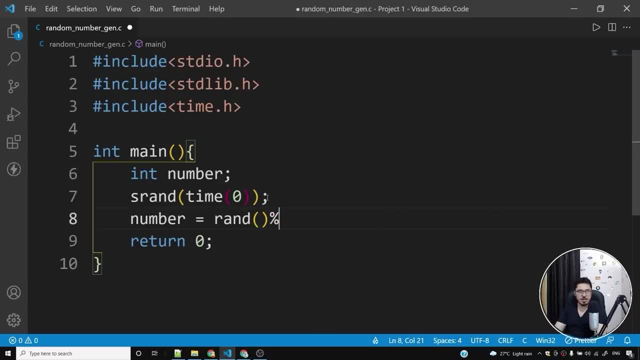 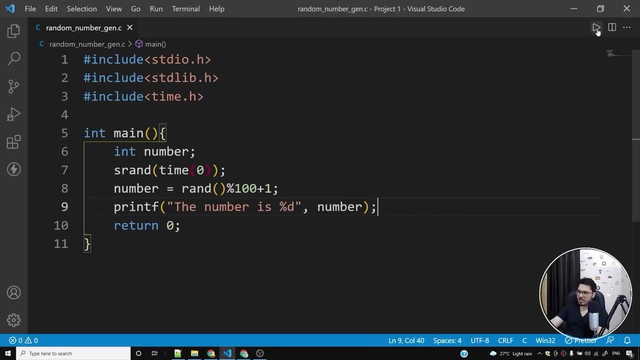 all you need to do is you need to say ram person 100 plus one, and i'll tell you the logic for this as well. let me print the number for you first. you'll say the number is percentage t and i'll say number. okay, let me run this program and show you that this actually generates a random number. 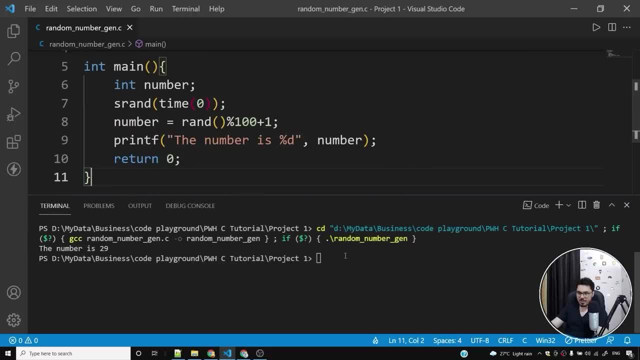 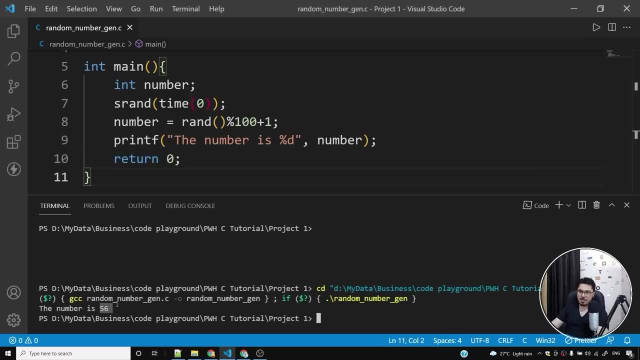 okay, and this is going to generate a random number from 1 to 100. let me tell you so. the number is 29- 49. so every time you run this program, you're going to get a different number between 1 and 100. so between this number and this number, you are going to get a number. okay, if you, if you talk. 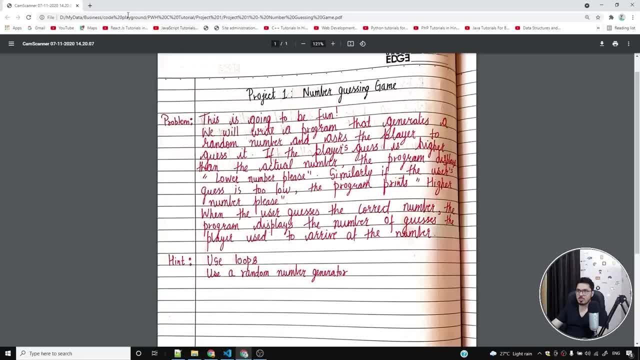 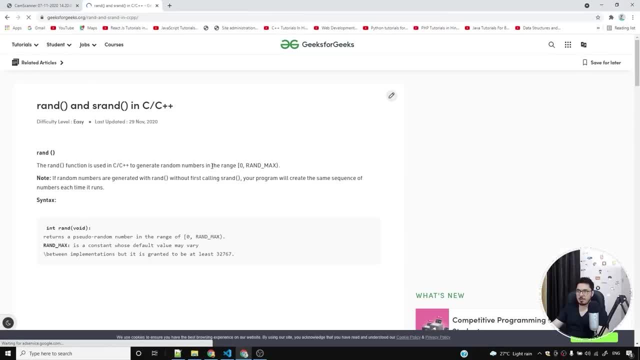 about rand function. what does rand function do? you can always google search. you can say rand in c and rand is actually a function. it is used to generate random number in the range 0 to rand max. 0 is included, rand max is not included. okay, so this is how rand function works. 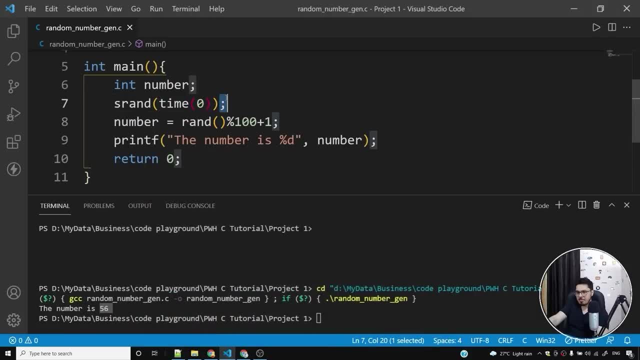 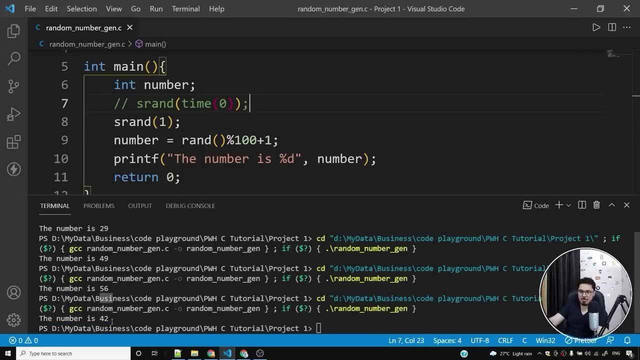 okay, so why did we use this s rand time 0? let me show you what happens if i put a constant value inside s rand. so if i put a constant value inside s rand, what happens is 42 is generated. if i program, if i run this program once again, once again, 42 is generated. if i run this program once again, 42 is. 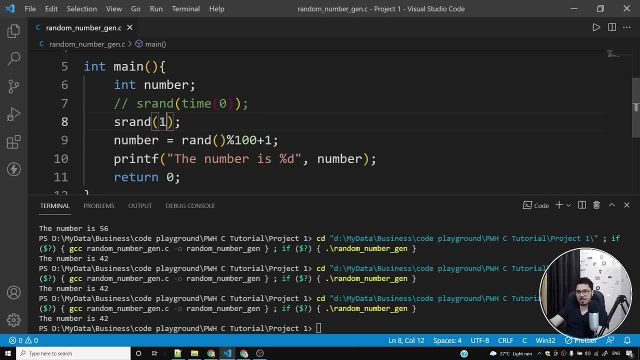 generated. so if you put a constant inside s rand, this is going to be the seed of the random number generator and for the same seed the number generated will always be the same. i don't want that. i want something random so that i can make this game fun. so something random is a system time. i can use the system time. 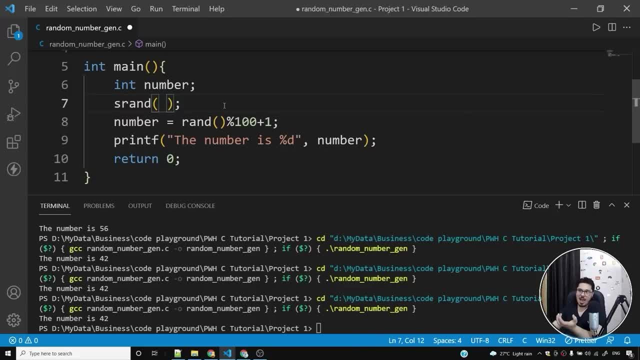 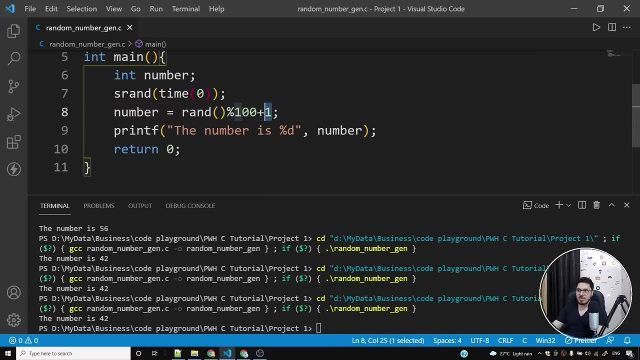 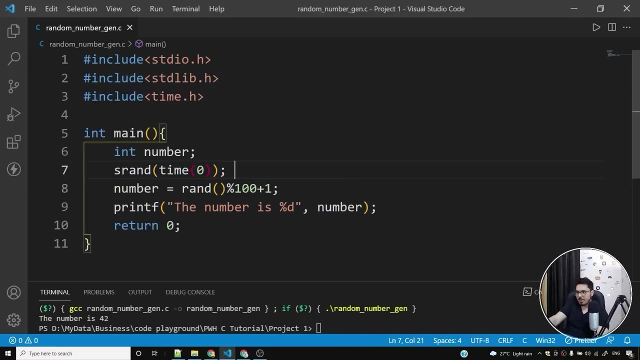 i can use time 0. this will give me the system time as an integer and i can use this as my random number seed. i hope the logic is clear to all of you, so i can generate a random number starting from 1 to 100. okay, so let us see how we can use this particular logic to program our game. so let's. 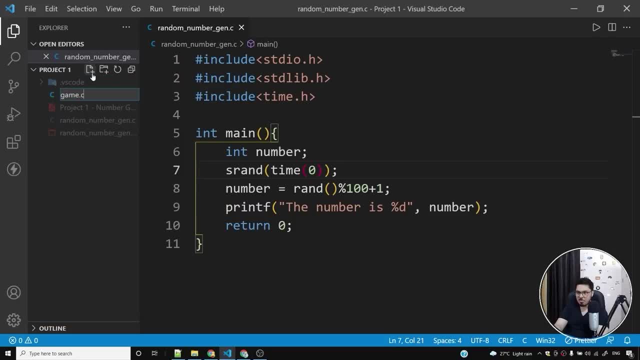 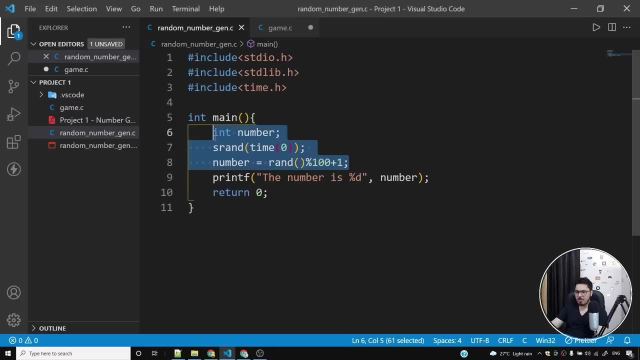 start our game. so i'll simply say gamecom, and i'm going to say gamecom, and i'm going to say gamecom c, i'll put the boilerplate code and the very first thing that i'm going to do is i'm going to generate a random number. let's do one thing: let's create a function. i can create a function to: 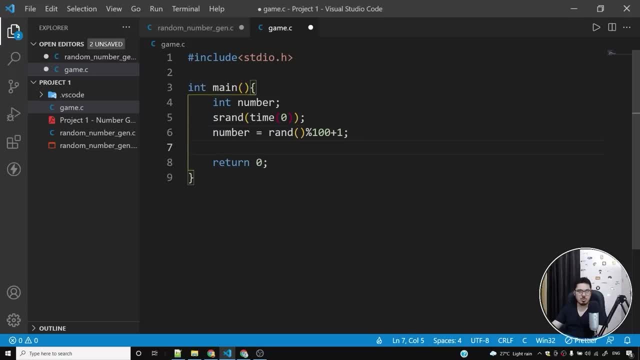 generate a random number. but let's not do that. let's keep the program simple. so i'll simply say int number, then i'll simply say time: 0 s rand. this is something that i'll have to do now. this is the number that i have generated. okay, i'll create another variable. i'll say guess, i'll create. 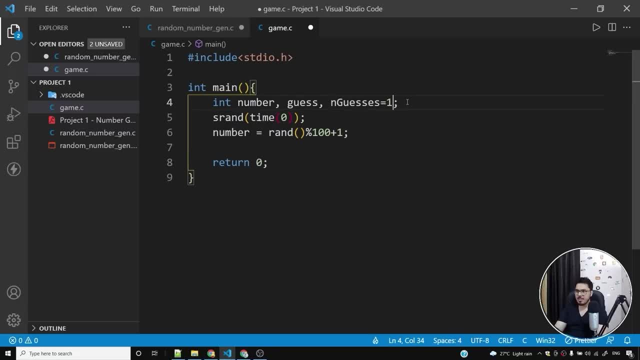 a variable, which will be number of guesses, n guesses, and i'll initialize n guesses with one. okay, so initially, the number of guests that you're going to take, no matter what, will be one, so you need at least one guess to guess the number correctly. okay, you cannot guess it in zero guesses. 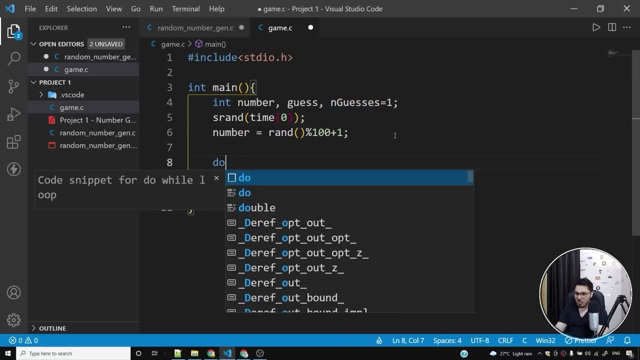 obviously, what i'll do is i'll use a do y loop. and why am i using do y loop? because i'm going to give you one chance for sure. okay, so this is a very good use case of do y loop. i'll simply say: guess the number. i'll say: guess. 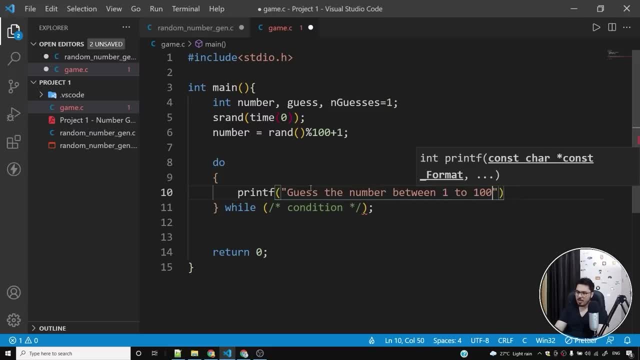 the number between 1 to 100. and yes, backslash n is important to format and i'll use scanf percentage d and i'll say amp, percent guess, because this is going to be your guess. okay, now what will happen is: i'll simply see if your guess is greater than the number. so there are only 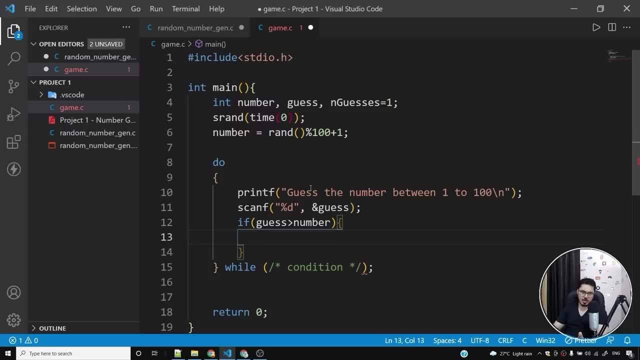 three cases possible. your guess will be either greater than the number, it might be lesser than the number, or the number which you can guess is lower than the number. so, in case your guess is greater than the number, i'll say: lower number, please. and what this will do is this will tell you. 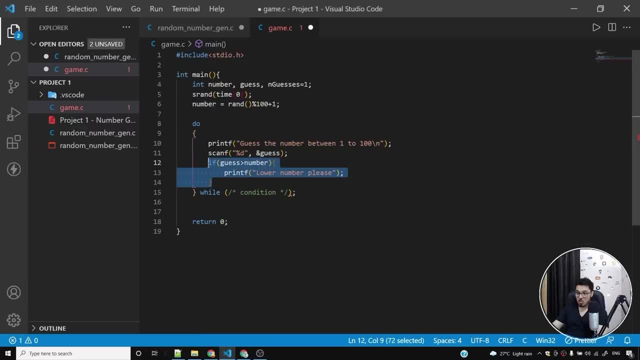 that you need to. you need to punch in a lower number. i'll use else if i'll say else. if the number is lesser, i'll say greater number, please. i'll say greater number, please. okay, now, if both of these scenarios are not true, what will happen is this: particular else is ulcf. 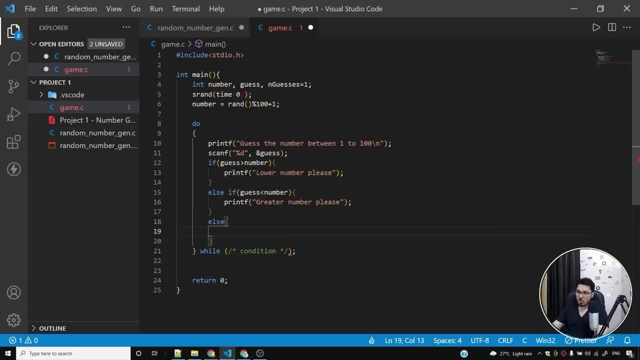 is likely square lighter than or equal to greater than. so you just by one checking and confused what will happen. if my guess is zero and right reference, i'll say seen between three. we get neither right reference. so here's my check. code is going to run and what it will do is printf. the spelling is wrong: printf. 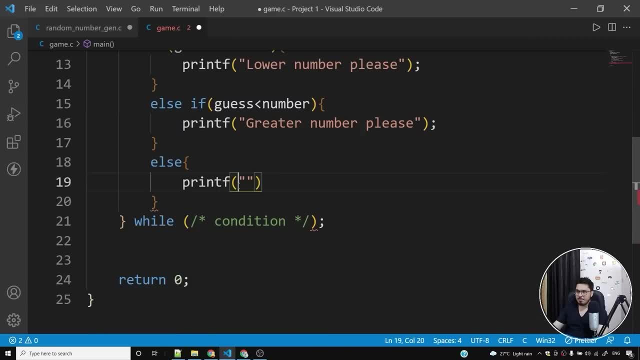 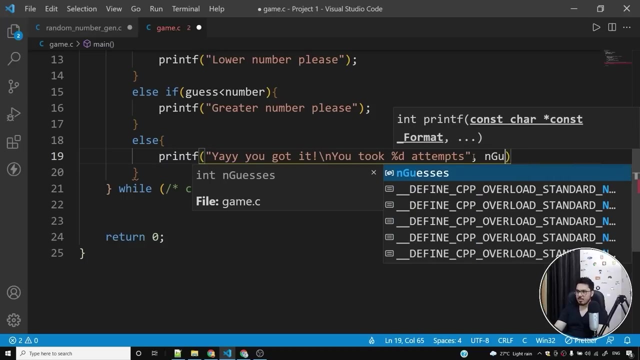 and let me zoom in a bit for you. i'll say, yay, you guessed, you got it. okay. i'll say, yeah, you got it in percentage d attempts. or let me let me do something like this: i'll say: you took percentage d attempts, how many attempts n guesses? and every time you are guessing, what i'll do is i'll. 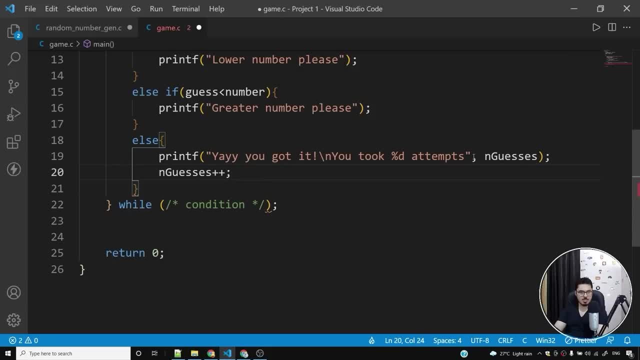 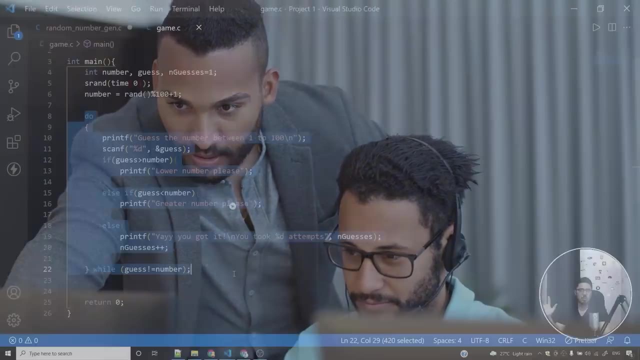 increment n guesses. so i'll say n guesses plus plus. okay, so this is how i'll increment n guesses and this while loop will keep on running until the guess is not equal to number. the moment guess becomes equal to the number. i want to get out of this loop. i hope the logic is very clear for you. 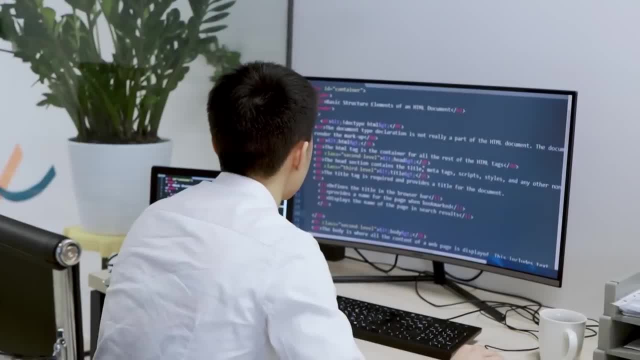 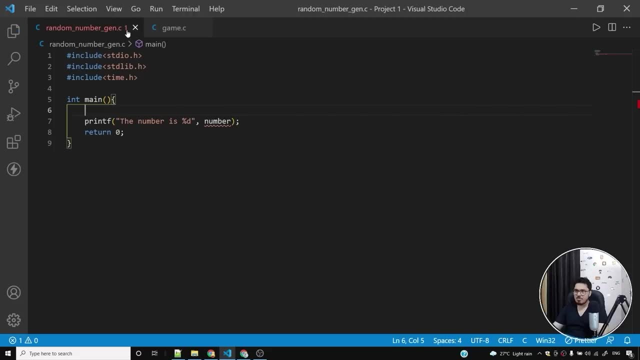 if it is not, just pause the video and look at the logic. you will definitely get it. this is super simple logic. let's try to play this game and see if this works. let me save this program and close it. oops, let me save this program and close it, and let me. 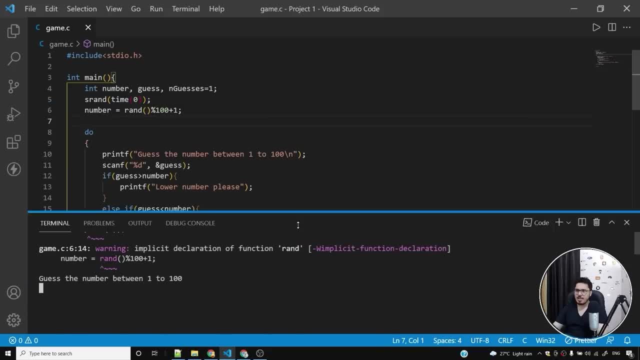 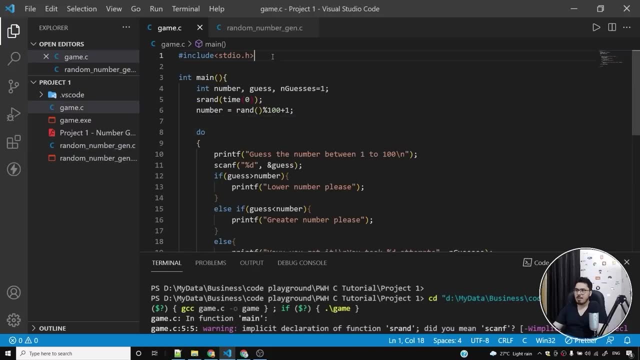 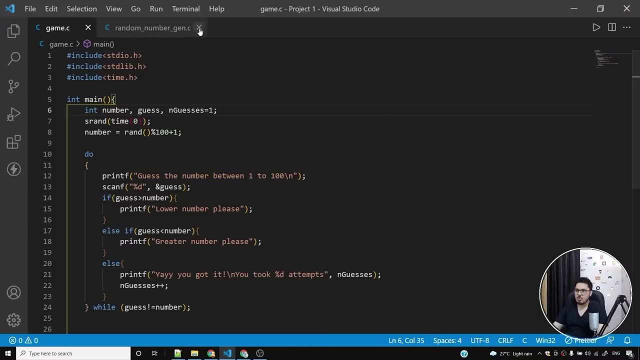 run this code and it gives me some errors. i think i forgot to include these header files, the ones that i included in this one. i'll replace all these header files and i'll once again run this program from scratch. let me close this random number generator dot c, and this time it compiles without any warnings. so guess the? 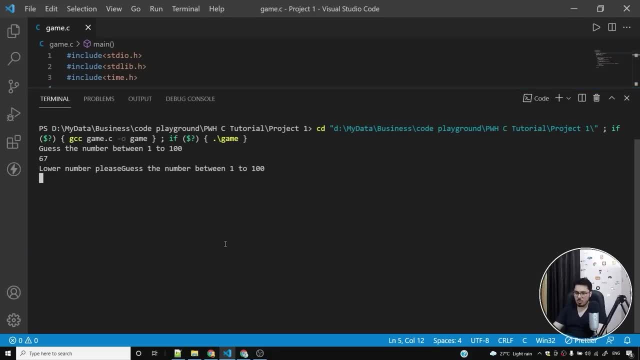 number. so i'll say 67. is it 67? no, it says lower number: please 40. okay, lower number: 23. lower number: let me say 12. greater number: 19. oh wow, you took it in one attempt, which is wrong. obviously i didn't. i. i didn't guess it in one attempt. so what i need to do is i need to 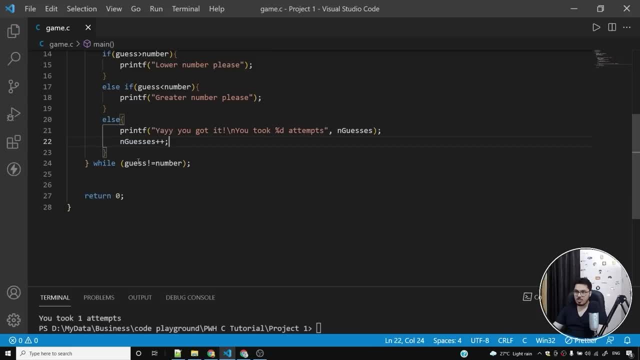 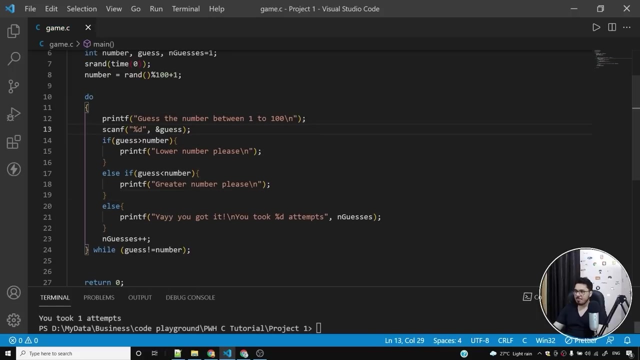 put this out outside this else. so initially it was inside the. else i need to put n guesses plus plus outside else. another thing i need to do is i need to format my program such that it actually prints a new line after these lines, because the program looks a bit ugly. let's run this code once again. 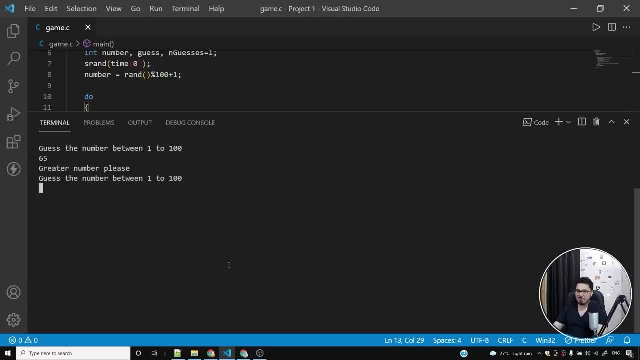 and this time, hopefully, everything will be right. 65 greater number, please, okay. 77 lower number, please. okay, that's interesting. 70 greater number, please. 73 lower number, please. is it 72? yeah, i got it in five attempts: one, two, three, four and five. so i got it. 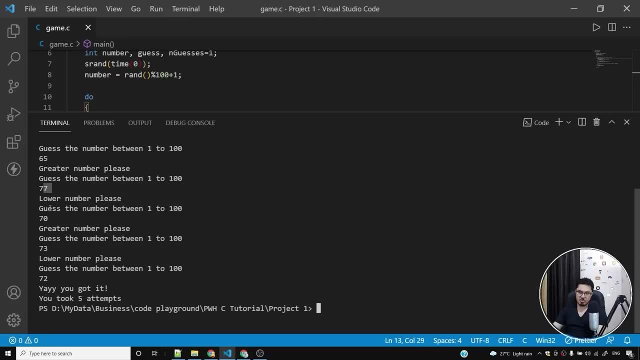 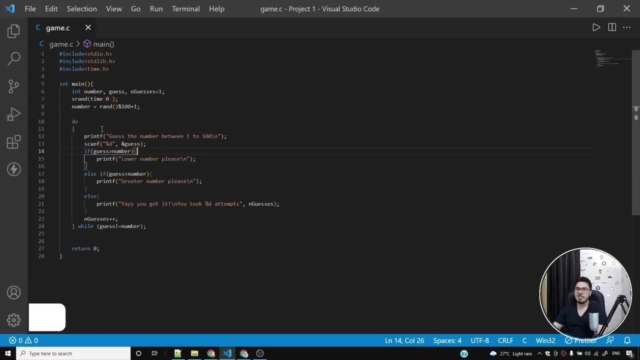 in five attempts. yes, correct. so my first attempt was this, then second was this, third, fourth, fifth. i got it in five attempts. this game was fun. let me know how is this game in the comments? everybody should write a comment below and tell me how was your first ever game if this was your. 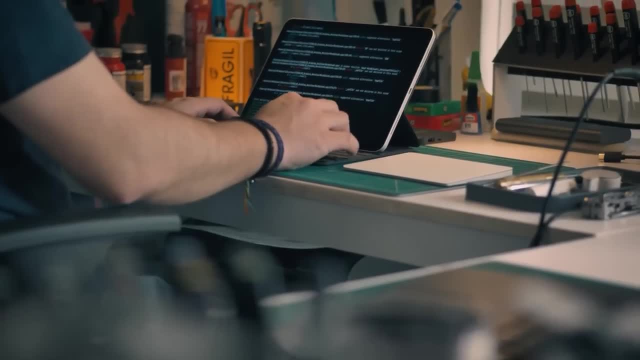 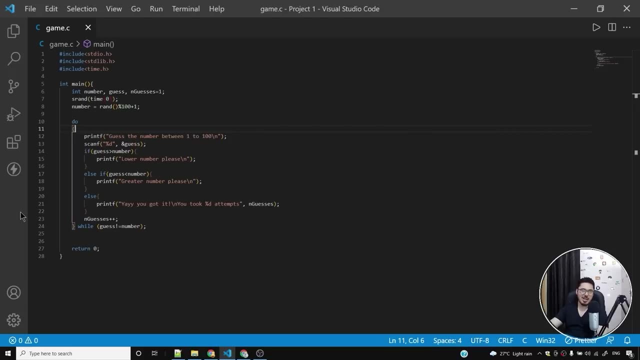 first ever game, even if it was your first ever c programming game. right, congratulations for all of us in the comments. it's going to bring up the energy. please do that. please go ahead and drop in your comment. do your bid. let's now continue this course and move on to the next chapter. so now, 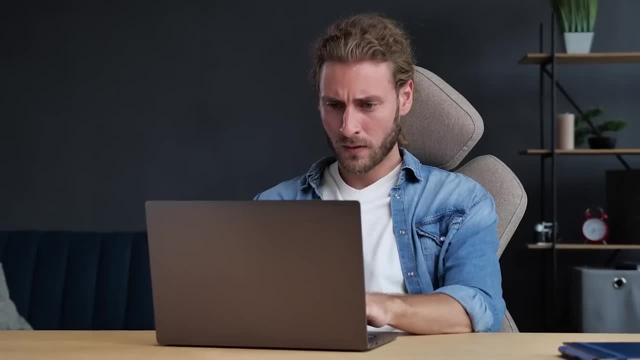 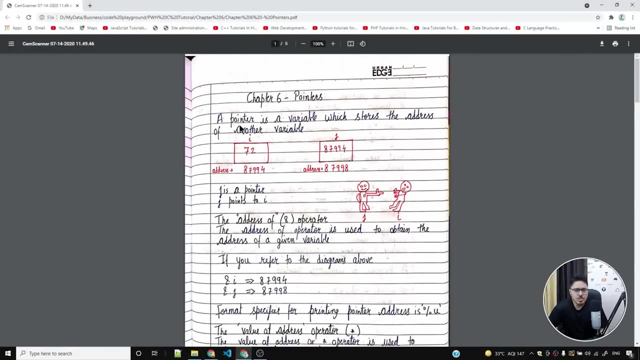 is the time that we discussed one of the most confused topics in the c programming language, and the name of the topic is pointers, and i have a dedicated chapter to this topic. why? because this is one of the most confused topic and we are going to see how easy the concept of pointers is. 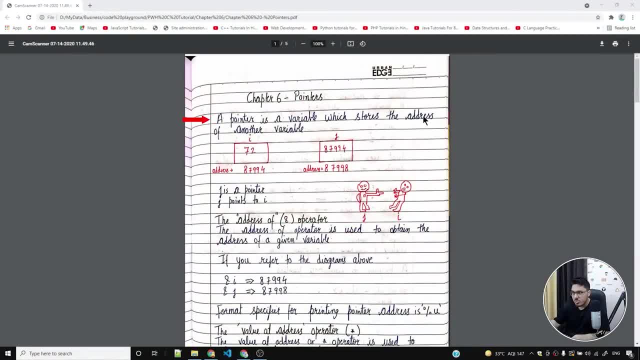 and you're going to appreciate it a lot. so a pointer is a variable which stores the address of another variable. so far, we have looked into int, we have looked into float, we also looked into double, we also looked into char, which was able to store character variables. now there is another type of 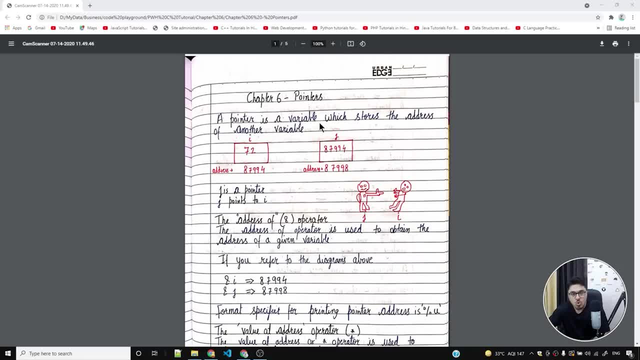 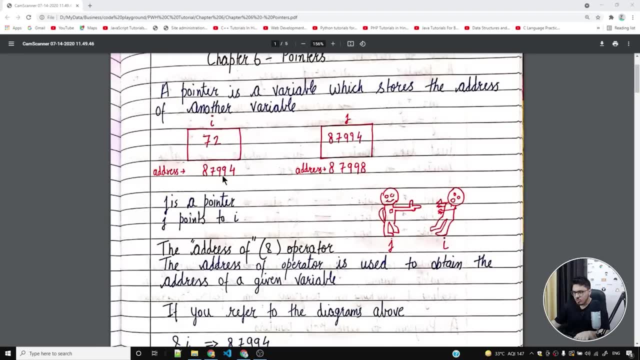 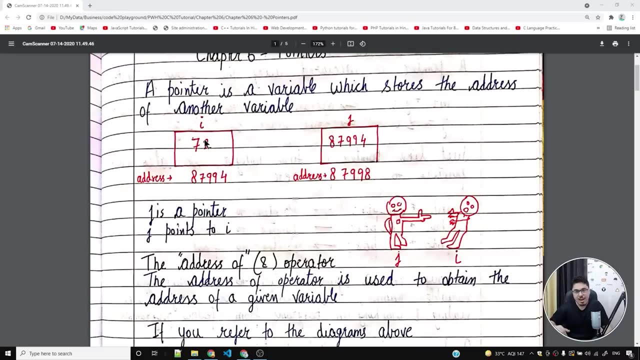 variable which does nothing but it simply stores the address of another variable. let's try to understand this, okay, so let us say this is a variable called i. what is the value inside this i? it's 72, so 72 is the value stored in i. i hope so far it is clear what i is. i is a variable. let me 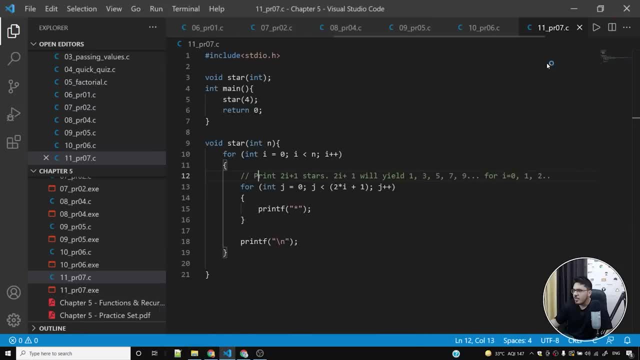 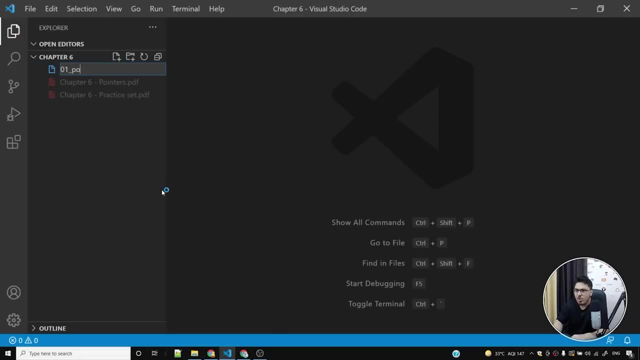 also open vs code and i want to open this particular folder in vs code. so i'll simply right click and click on open with code and i'm going to create a program called pointersc. okay, i'll put in the boilerplate code here and i'll simply write int i. so the moment i say int i and the value is: 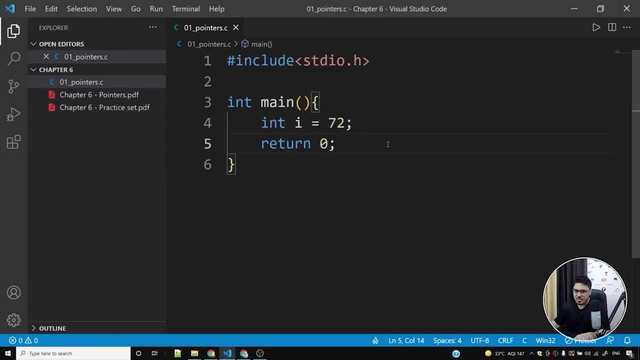 int i is equal to 72. what happens is in my main memory, in my ram, in my random access memory. what happens is this particular variable is stored inside some address in the memory, so memory has some address, just like you have a locality. that locality has different houses. each house has some. 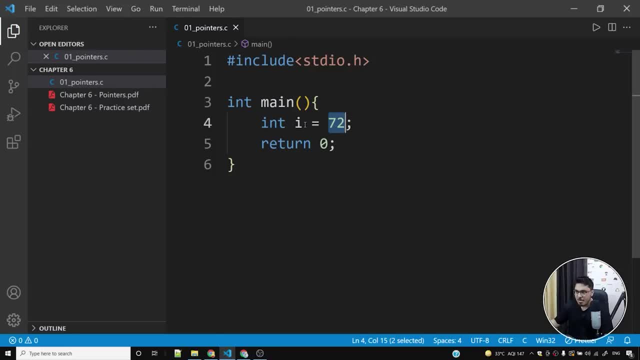 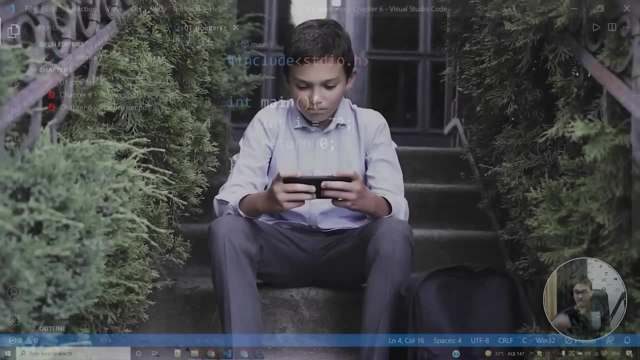 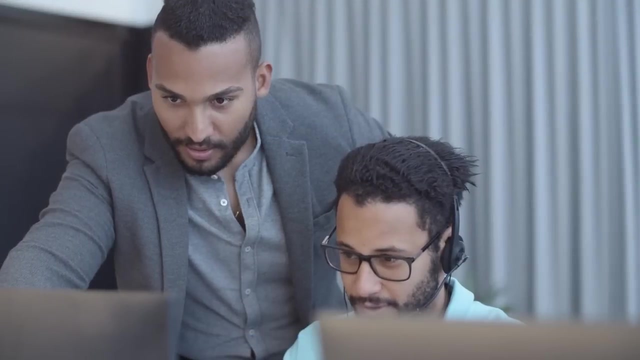 address in a very similar way. we have main memory and inside the main memory we have a lot of blocks in an address. try to understand this very, very carefully. try to listen to me very, very carefully, because this concept is really very important and if you listen to me, i can guarantee that you're. 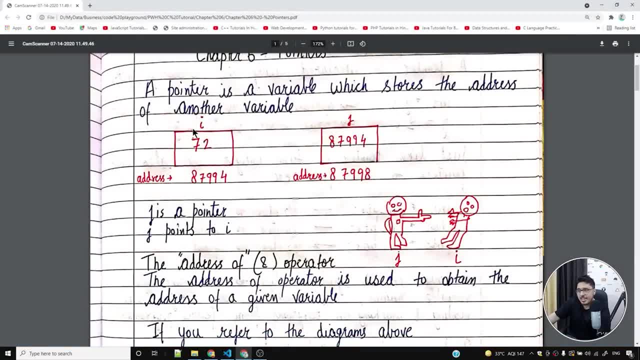 going to understand. so the moment i say in time is equal to 72, 4 bytes in ram are reserved, 4 bytes in memory are reserved, and i will start from some address and i'll keep on going till 4 bytes are in memory and those 4 bytes are not in the memory, and i'll keep on going until 4 bytes are covered, or 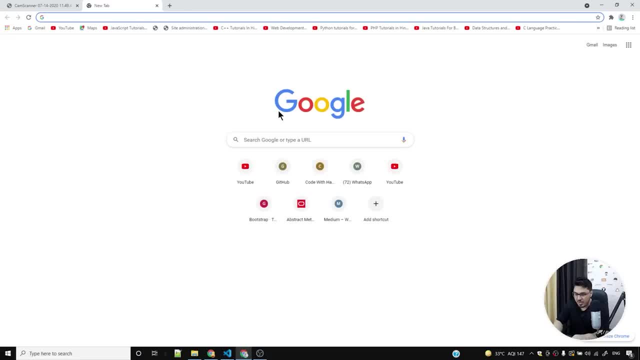 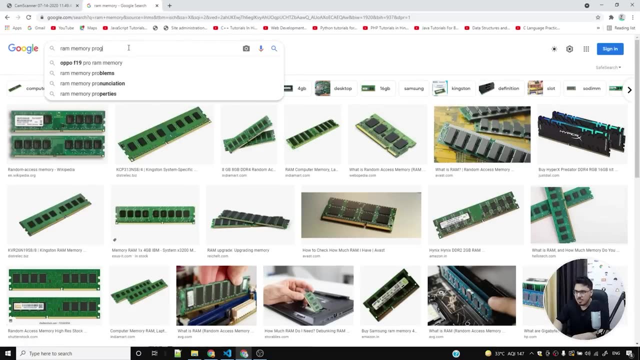 me and those 4 bytes are still in the memory, and i will keep on going till 4 bytes are still in. the bytes will be used to store this integer. let me try to explain. i'll simply say ram memory, and i simply need some images. so that, uh, so this is how it physically looks like, but i want to show. 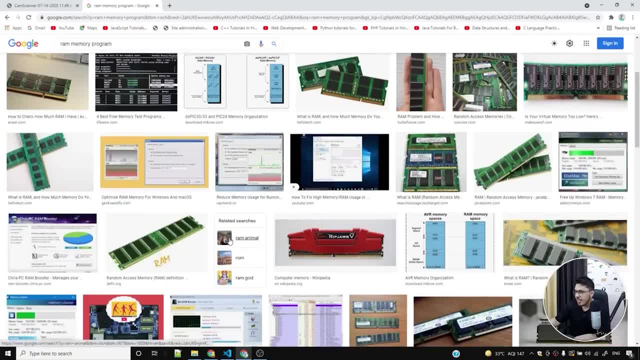 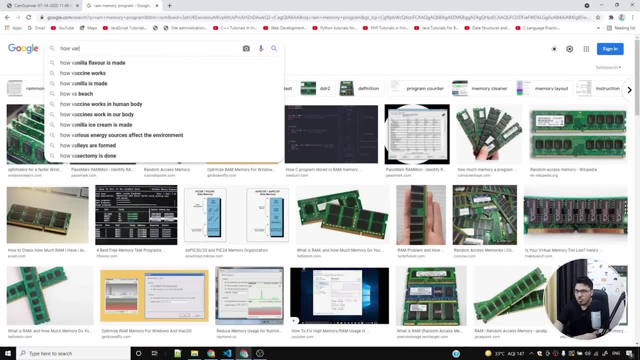 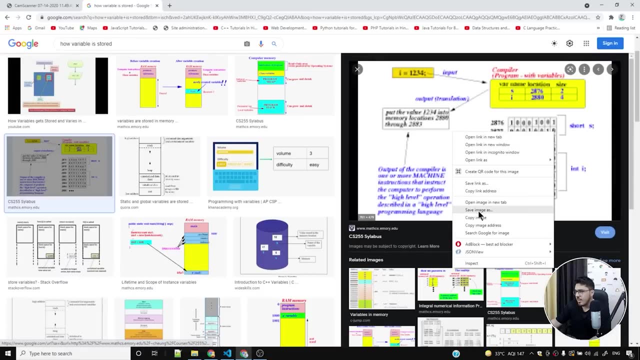 you some schematic representation of memory so that i can explain you how a variable is stored inside a memory. so let me, let me google how variable is stored, okay, and we should get something. yes, uh, okay, so here here. here is an image that i'm going to use to explain this to you. 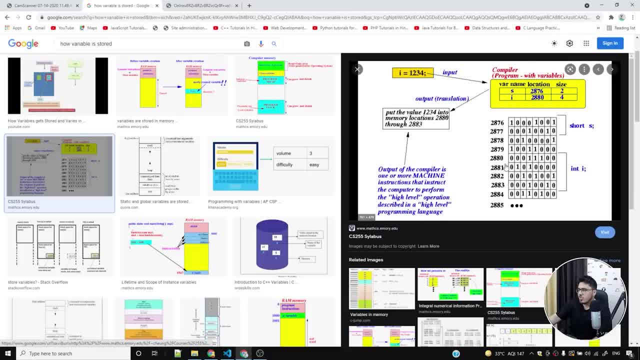 so this image is a bit blurred, so we can see this image, by the way. so these are nothing but blocks in the memories. each block can store either zero or one, and we have a lot of blocks in our memory. now what happens is one block is one bit, so one bit can store either zero or one. now one, two, three. 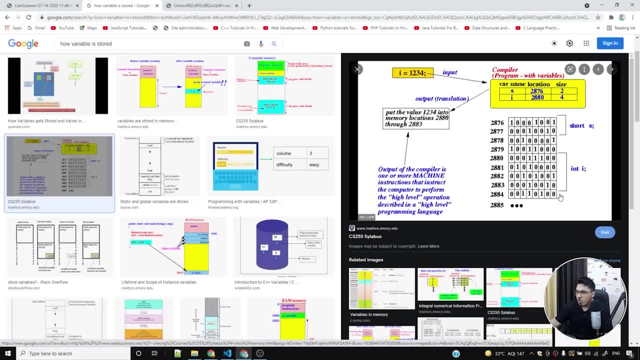 four, five, six, seven, eight, eight bits will form a byte. eight bits will form a byte and 1024 bytes will actually form a megabyte, which is called an mb. you must have heard about mb, 12 mb, 30 mb, 512 mb and 1024. mb is going to. 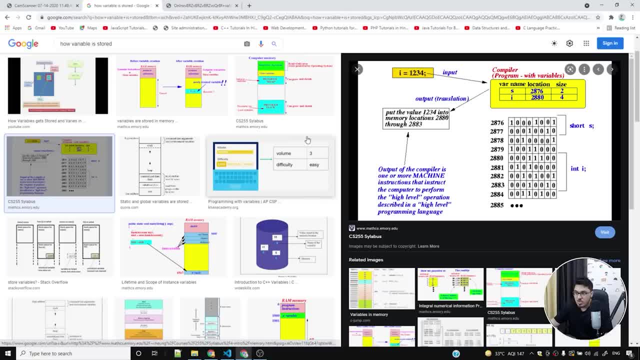 be 1 gb. we, we all use memory, we all use hard disk. but what happens is, when we have so much of memory, we can store a lot of things inside the memory, but at the very basic level, what a memory can store is simply a 0 or a 1.. so let us say, i say int, i 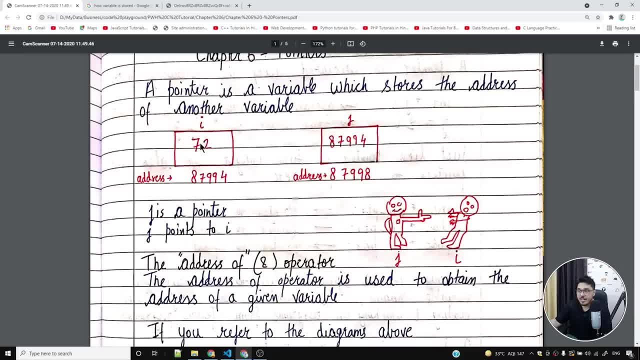 is equal to say: uh. in this case i said i is equal to 72.. i am storing an integer and in order to store an integer, i need 4 bytes. integer is 4 bytes. in some of the compilers it is even 2 bytes, but let's look at an integer as 4 bytes for now. okay. so if integer is 4 bytes, how much memory do i? 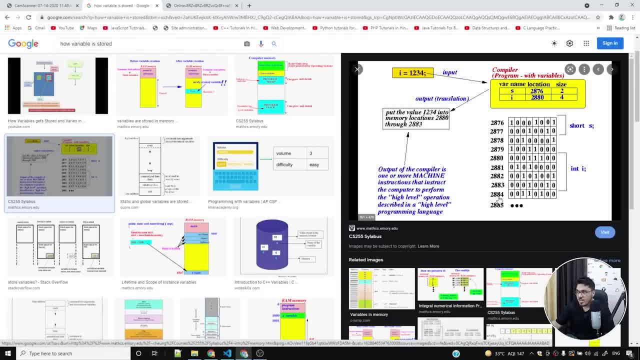 need to actually store this integer. i need one, two, three, four. i need these four rows to store an integer because one row is nothing but one byte and i need four bytes to store an integer, so i need this much of space. one, two, three, four. i need two, eight, eight. one all the way till two, eight. 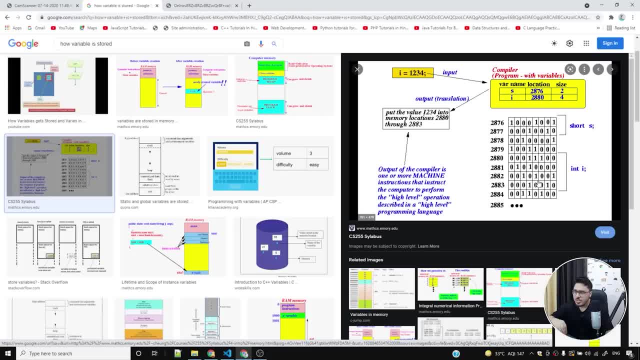 eight four to store this integer. okay, now, how will this integer be stored in the form of zeros and one is is another question, and i'm not not going to discuss that question just yet. what we're trying to understand here is how this variable is going to store in memory. now, 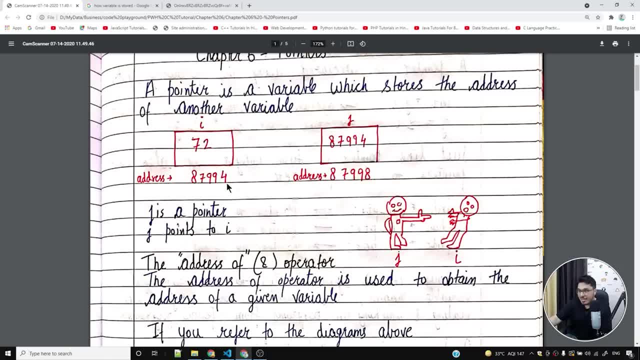 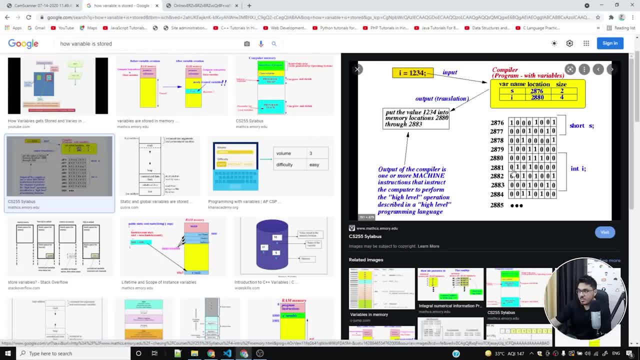 whenever we store a variable in a memory, there will be some address of the memory where that variable has been stored. so let us say in this case, 2881 is the starting address where this integer is going to be stored. i can say that this integer is stored at 2880. you can. 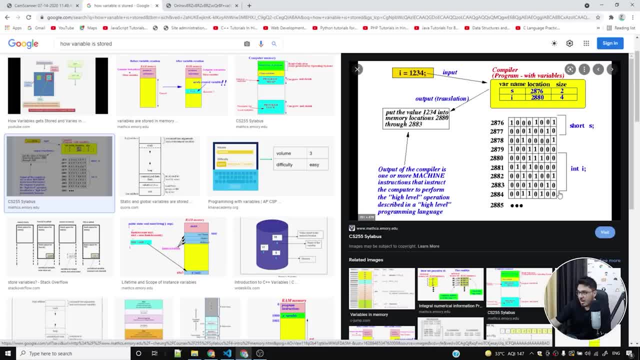 see that int i is marked. one, two, three, four bytes are marked and this int i- will start from 280, if you look at this image very carefully- is a variable which starts at 2880 and takes four bytes from there. so 2881 is occupied, 2882. 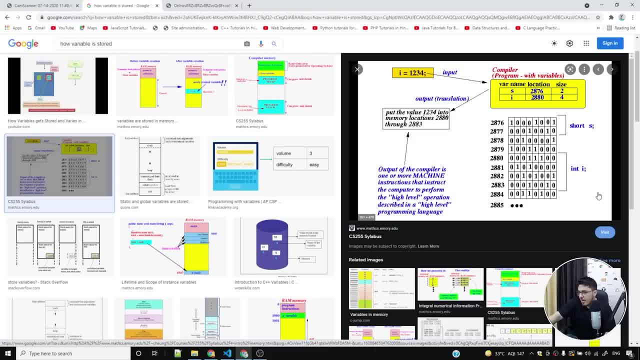 is occupied. 2883 is also occupied. you can see that int i has been marked and these four rows have been marked, which simply denotes that these four rows are holding this integer. how are these holding this integer? that is a question for another day. just understand that this is a lot of work. 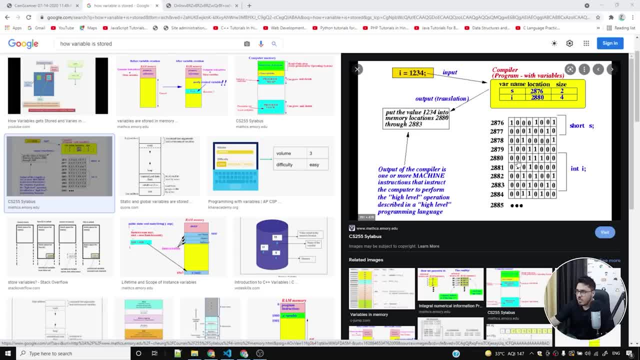 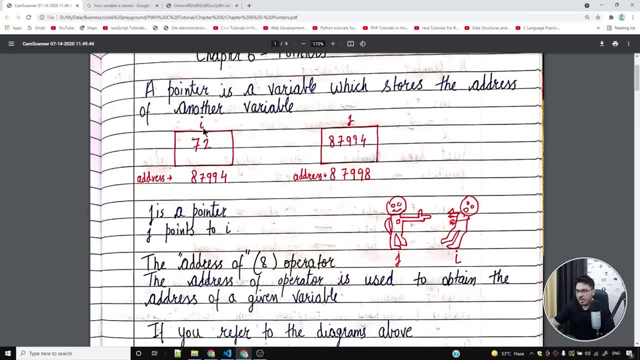 that zeros and ones can be used to store an integer. So 72 is stored in this space. okay, Now if I say what is the address of this integer, What is the address of i? It's 87994.. In this case it is 2880.. 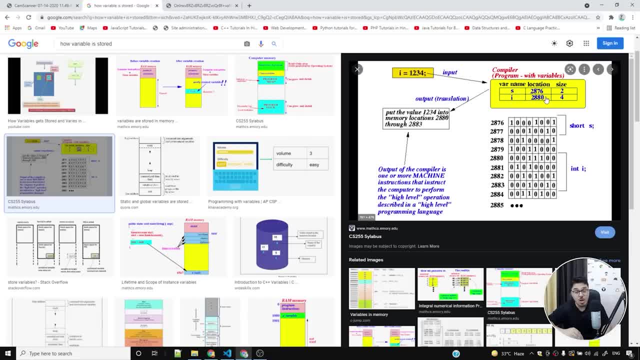 You can see that address of i is 2880.. That depends upon how compiler is storing this variable. It might start the address from 2888.. It might start the address from 178822994.. It can be anything. We don't have to worry about it. 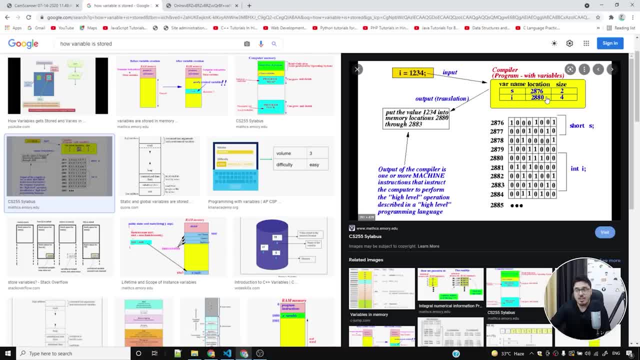 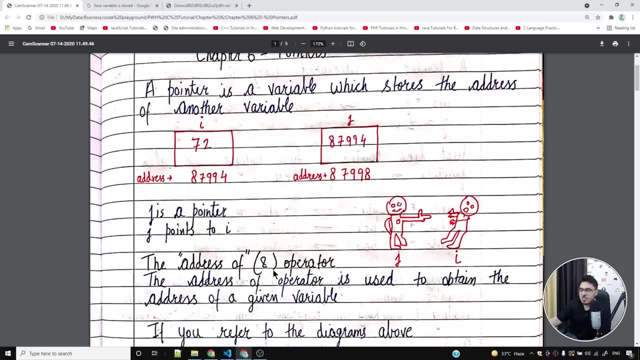 You will get different types of addresses, In fact different address locations on different computers, as and when you run the program. So in order to see the address, we use ampersand operator. okay, Now, I know that this might sound really very complicated. 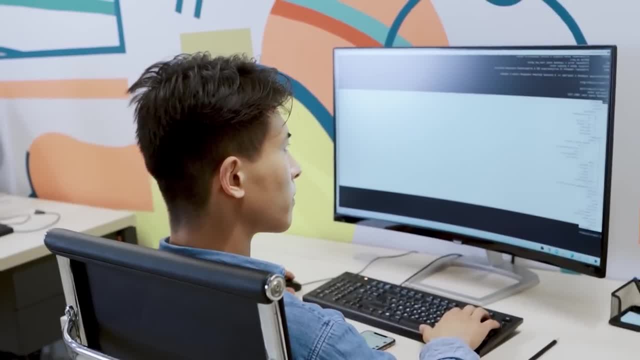 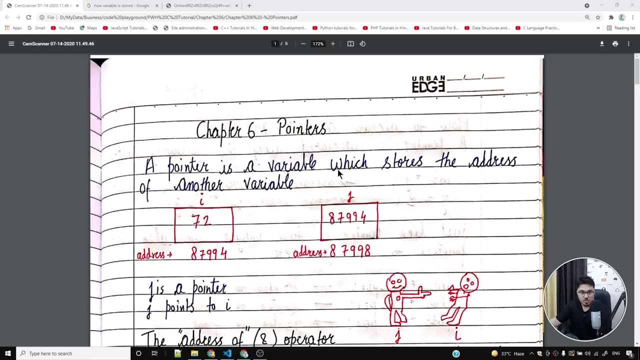 to some of the people who are just starting their programming journey. But, believe me, you are going to understand each and everything as we move ahead towards this pointers journey. okay, So for now, what we are doing is we are saying that i is a variable. 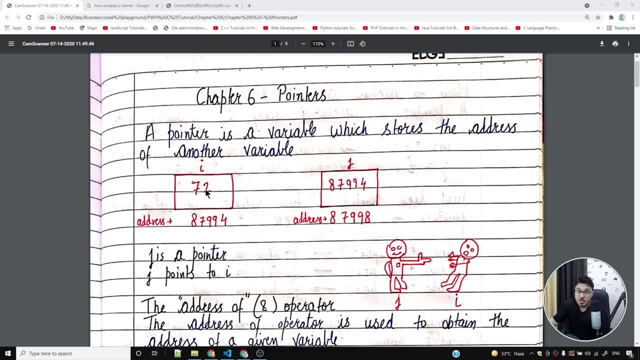 i is simply a variable. It stores 72.. It's an integer variable. Now what I'm saying is: the address of i is 87994.. This is for the fact. Okay, 87994 is the address. Now I'm creating another variable to store this value: 87994.. 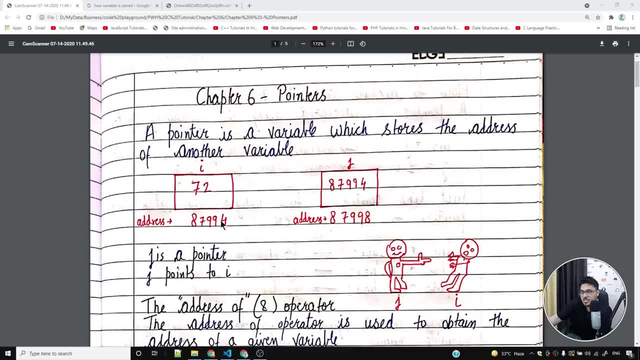 I can create a variable to store this value: 87994.. It's a value which can be stored in another variable. Will it be doing it be an integer? no, it will not be an integer. you might argue that why? why can it not be an integer? 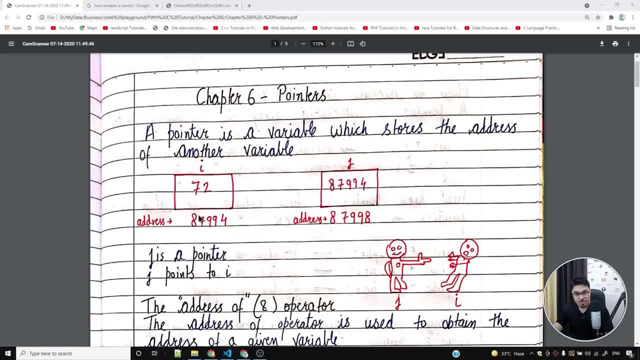 but when we are storing addresses in c, we simply use pointers. pointer is a special kind of variable which stores address of some other variable. so i holds 72 and j holds 87994. i is an integer, j is an integer pointer, j is an integer pointer. this is something that you need to understand. 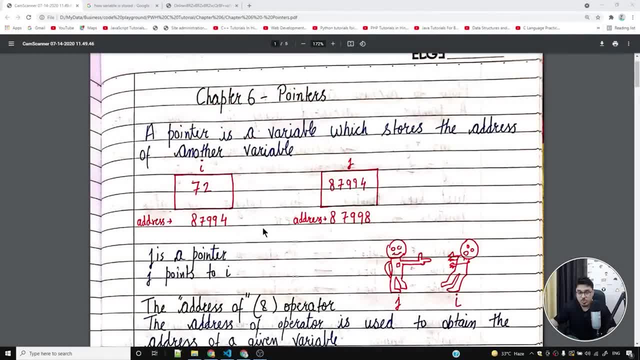 listen to me very, very carefully. this is an area where you cannot sleep. you will have to listen to me. please rewind- if you were sleeping while i was talking about pointers- and listen to me very, very carefully. what pointer is? so i is an integer variable. j is an integer pointer, integer pointer. 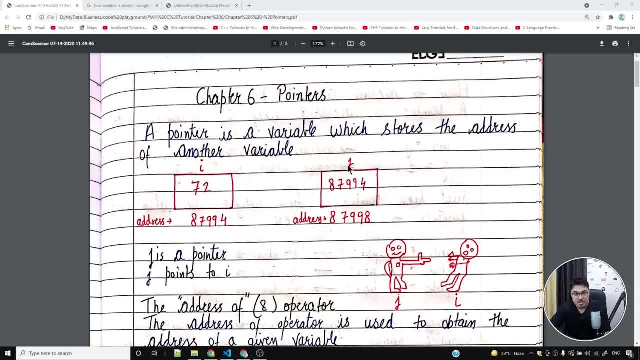 means a pointer which stores the address of an integer. so j is an integer pointer, so j will hold address of integers, only integers. okay, so i can simply assign 87994 to j, you and I can even assign address of some other integer to j, and so on, okay, 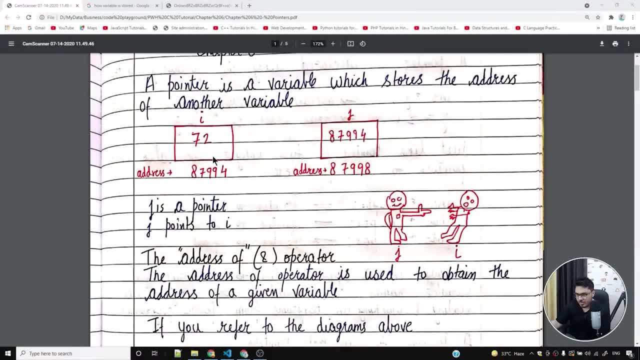 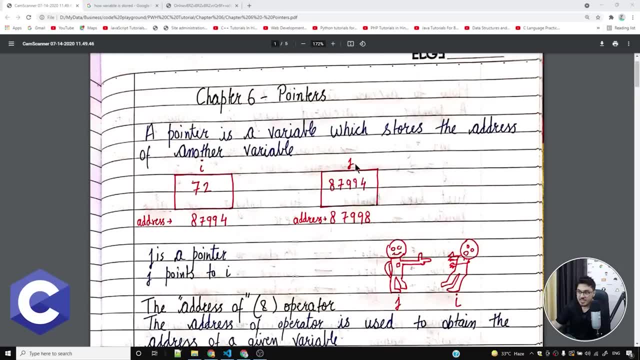 I hope you understood this much. Now. j is a pointer and j points to i, So we simply say in C language terminology that j points to i. When I say j points to i, it simply means that j is holding the address of i. 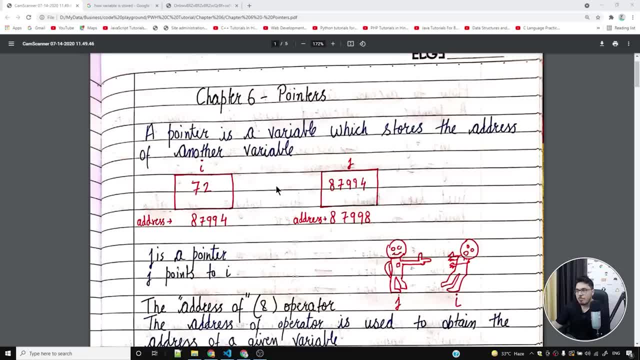 So i is holding 72, j is pointing to i. Pointing to i means it's holding the address of i. okay, I hope that this is clear so far and I was able to understand. I also created this visual to better explain you. 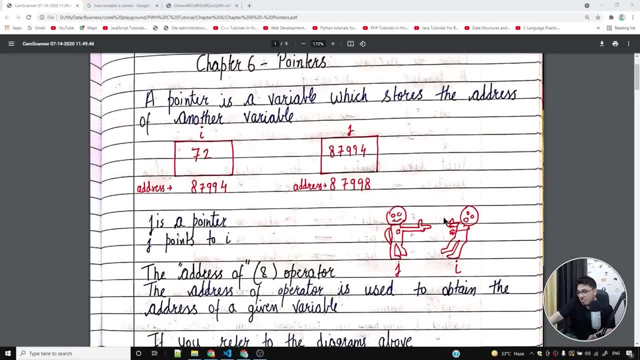 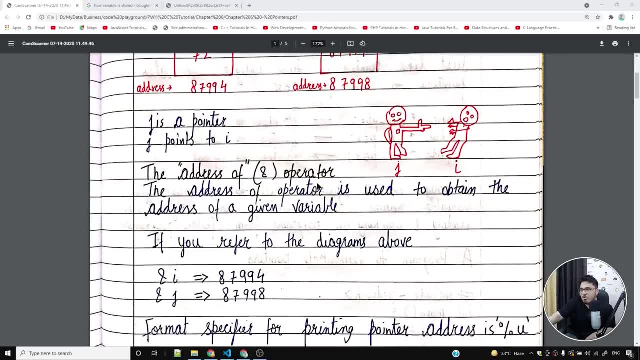 what j points to. i means You'll be able to remember all these things if I create these funny visuals for you. okay, Now let's talk about what is address of operator- ampersand operator. Okay, is this the first time we are using ampersand operator? 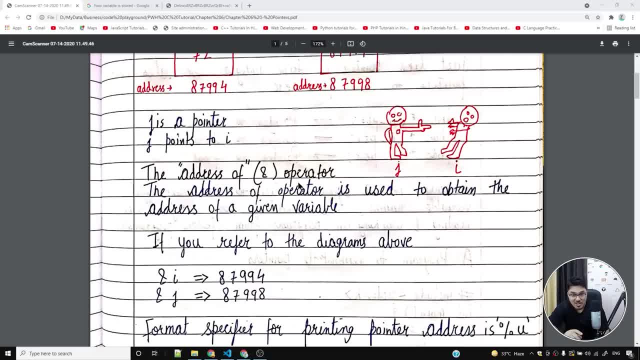 No, we have already seen ampersand operator where we looked into this ampersand operator. while we were talking about scanner function, We discussed that in order for scanf to work properly, we need to supply the address of the variable we want to take as input from the user. 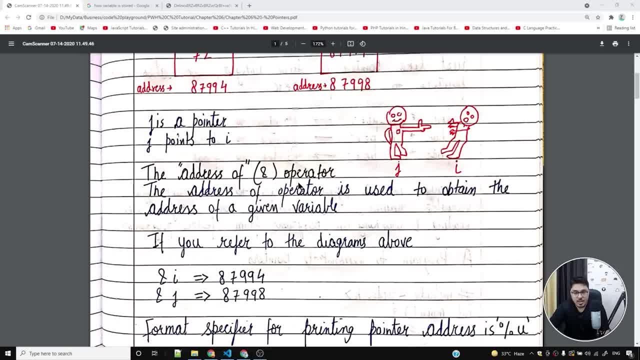 So we use ampersand in order to take the address of a variable and supply it to scanf. But let's see what this ampersand means. Ampersand will simply return the address of the variable. So when you say int i is equal to 72,. 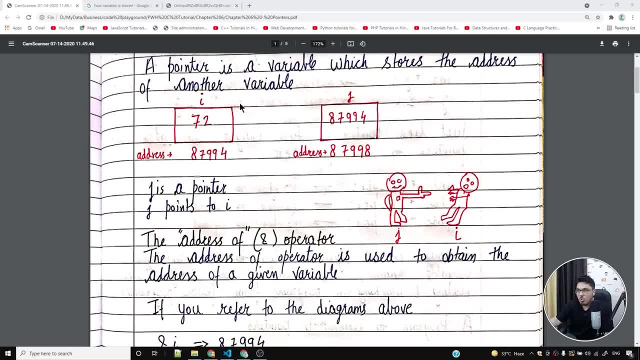 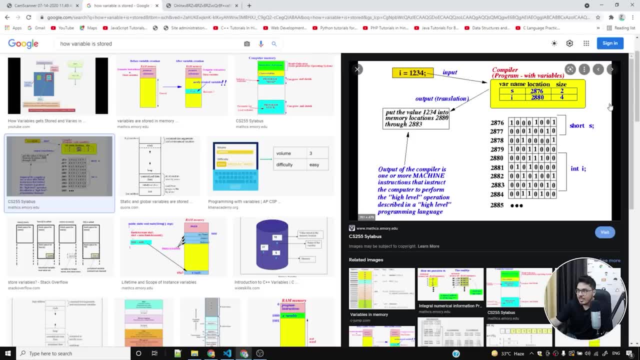 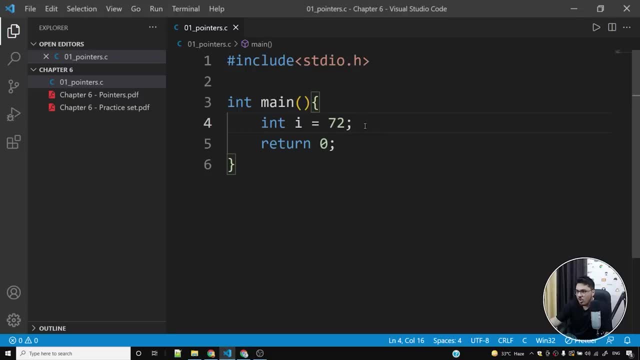 i will be located somewhere in the memory, the value 72, and wherever this i is in the memory ampersand, i will tell me this value. in this case, ampersand, i will simply return 2880. i hope that this is very clear. so, in order to, in order to, 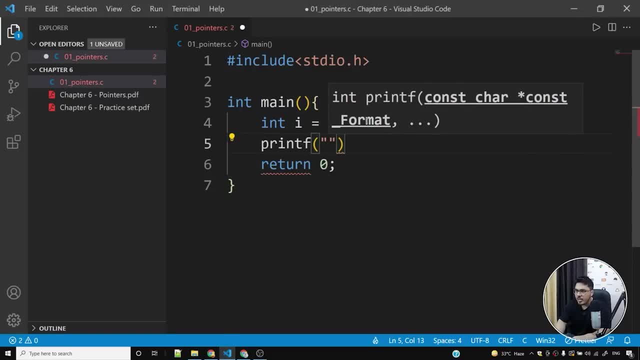 understand, or rather in order to look into the address of i. the address of i is percentage u. and what is this percentage u? yes, you guessed it right. it's a special format specifier for pointers. okay, so i'll simply say ampersand i and i'll get the address of i, okay. 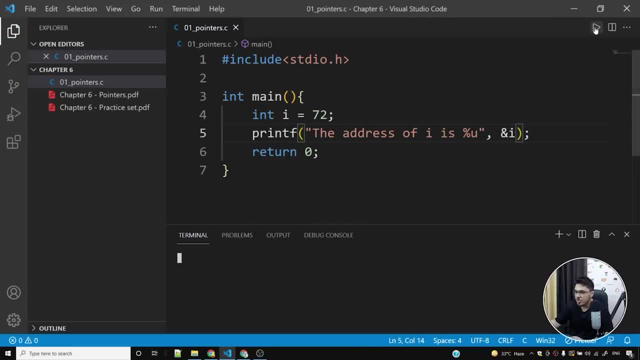 let me also make this ts capital and run this program for you. the moment i run this program, you will see the address of i is this: so this is the address in memory which was provided to this particular variable i. okay, so i was stored here starting from here, and it will occupy four bytes, or two bytes depending. 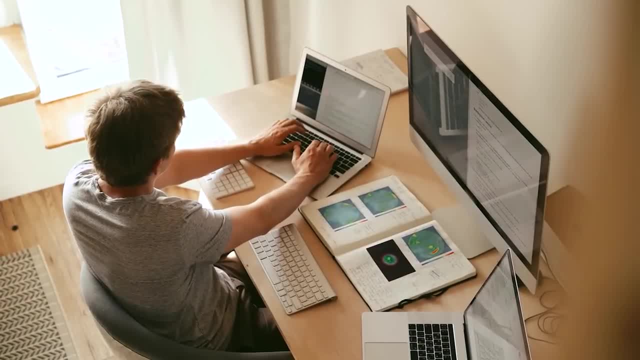 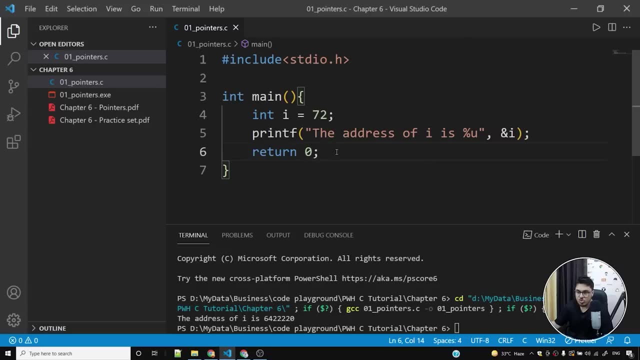 upon the architecture. if you are in some other computer which uses some different architecture, integer might be two bytes there, okay, so this is something that you need to remember. you, you don't have to memorize that integer is four bytes and it cannot be two bytes. it can be two bytes, it can. 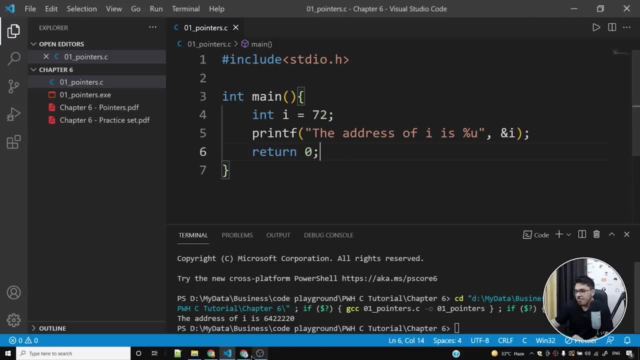 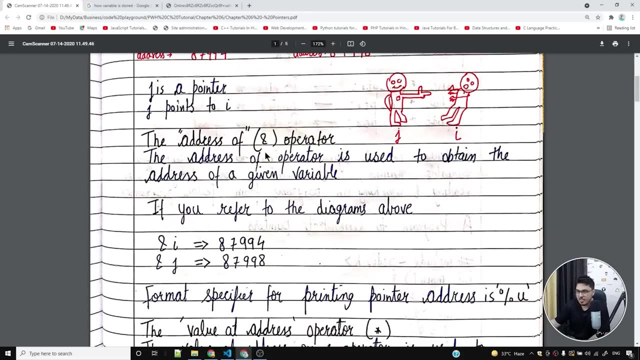 be four bytes. that depends upon the architecture. okay, now coming back to the notes. the address of operators is used to obtain the address of i of a given variable. so address of operator. address of is an operator which is nothing but ampersand. this ampersand is used to obtain the address of a given variable. so if i was to obtain the address, 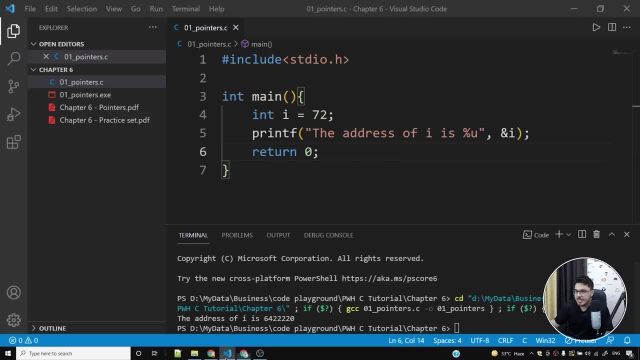 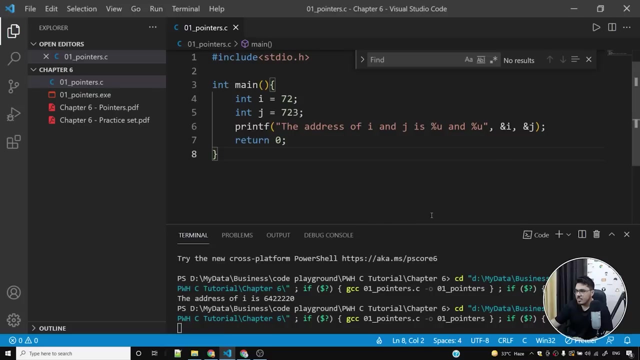 of a given variable. i'll use ampersand, just like this. okay, now for different variables. this will give different addresses. so if i have int j is equal to something, let me say int j is equal to 723 and percent u, and i'll say ampersand j. the address of i and j is this and this. so the address of i is this and. 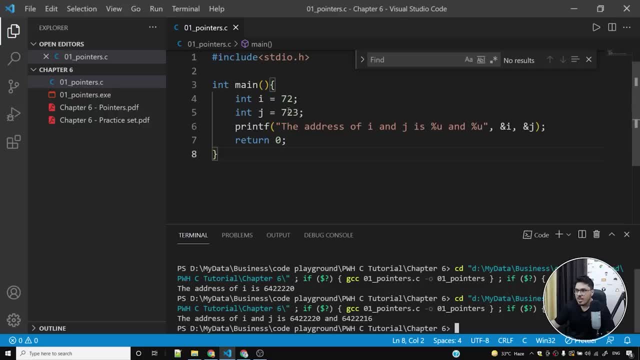 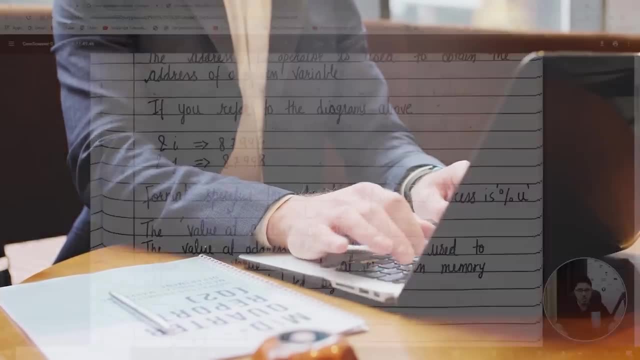 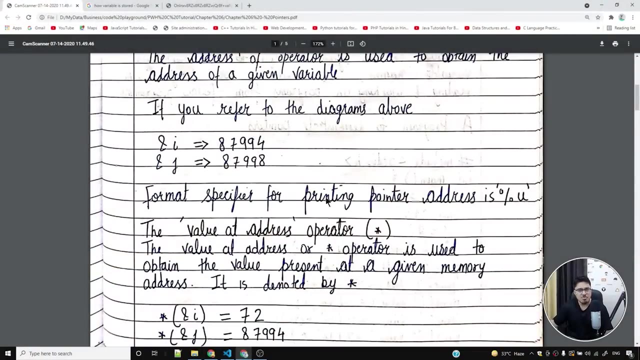 address of j is this. so this is how address of i and j can be written using a c program. okay, so far, so good. i hope you understood how we can take the address of a given variable and print it on the console. format specifier for print: we have seen format specifier for integers, which was percentage d. we saw format specifiers. 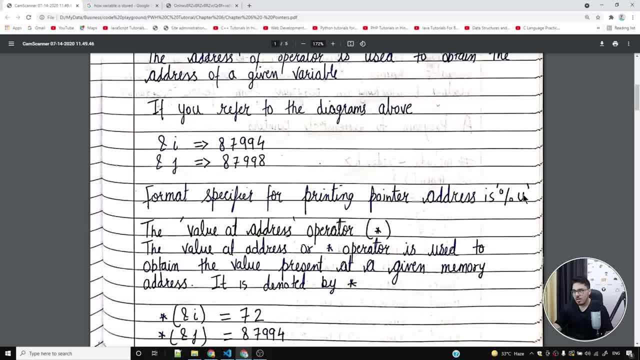 for floating point numbers, percentage f, for we saw it for double, we saw it for a lot of other variables. you can even google for format specifiers, but percentage u is something that you need to remember. just like you remember percentage d for integers, you need to remember percentage u for the. 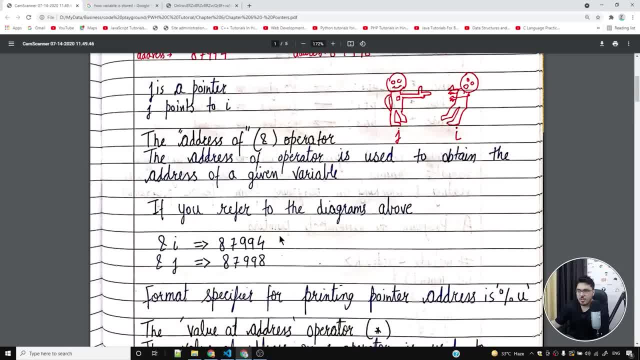 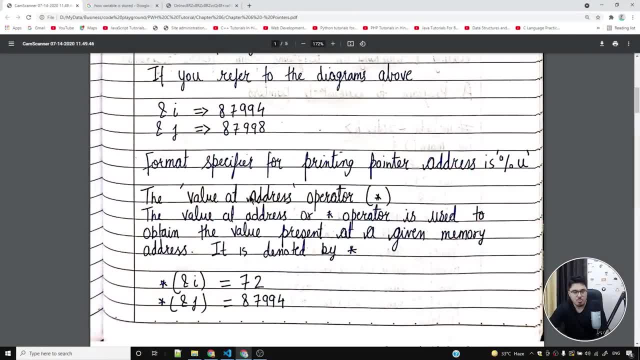 pointers. now, just like we saw ampersand operator, we look into a star operator, and this is something that might confuse you, but i'm going to make it as simple as possible for you and if you listen to me very, very carefully, i can give you a guarantee, 100 guarantee- that you will. 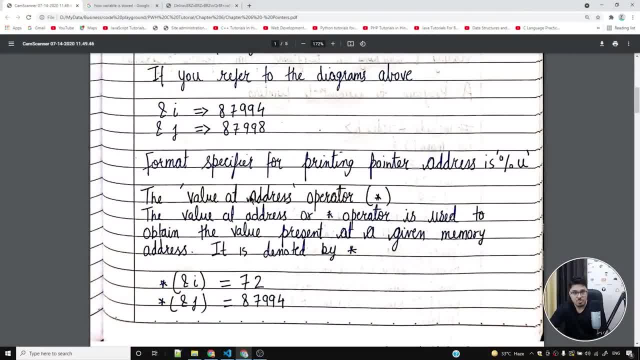 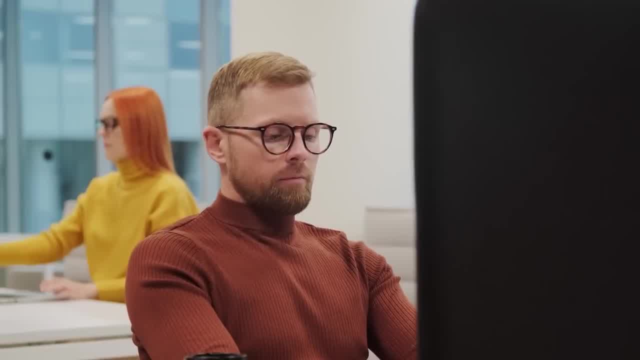 understand this because when i started learning this i was very confused. so i can tell you that how your confusion can be removed and what are the things that will confuse you. listen to me very carefully. the value at address or star operator is used to obtain the value present. 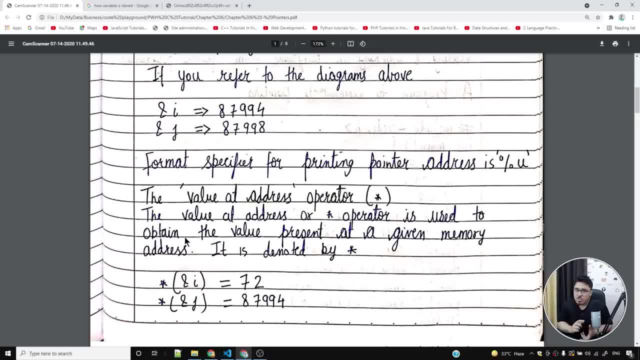 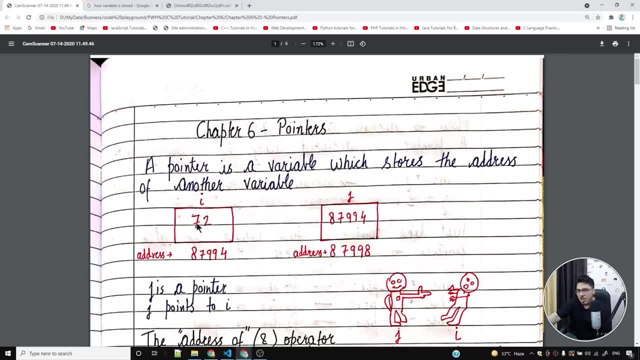 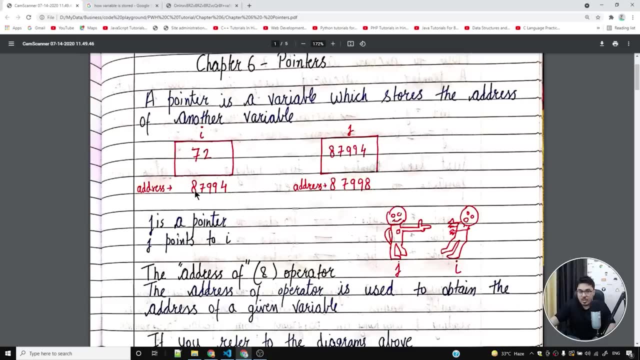 at a given memory address. so it's kind of an inverse of ampersand operator. let me tell you how. so if you have a variable i and you have the value stored inside the variable 72, you use ampersand operator. you will get to address. what if i give you the address and i want you to? 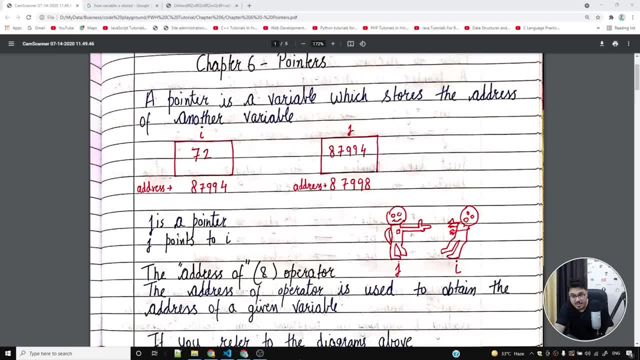 tell me what is the value stored at this address? so if i hand you 87994 and then i ask you, tell me the value stored inside this address, how will you tell me which value is stored inside this address? you might say i don't know. i don't know, i cannot look into the memory, i cannot open the screws of my. 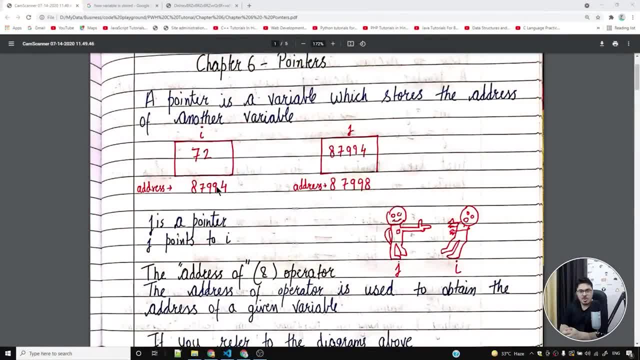 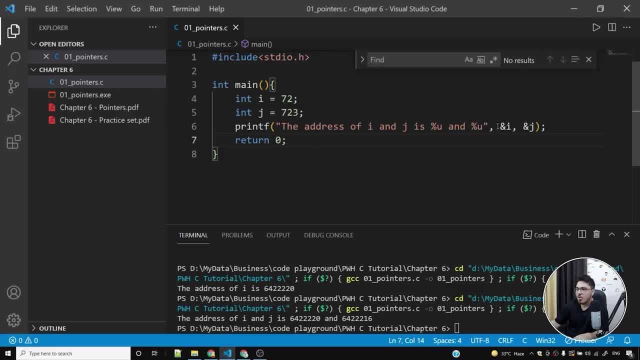 laptop and look into the memory and read which value is there. you cannot read, but you can always write a program and i'll show you how that is done. so just like we have ampersand operator to get the address, we have star operator to decode that address and get the value at that address. so if i 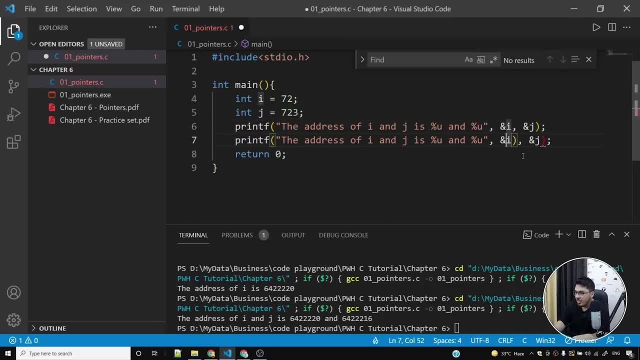 enclose this with with a star. let me show you. so, if i say star of ampersand of i and star of ampersand of j, let me show you something: star means value at address of i, value at address of i. let us say you are living alone at. 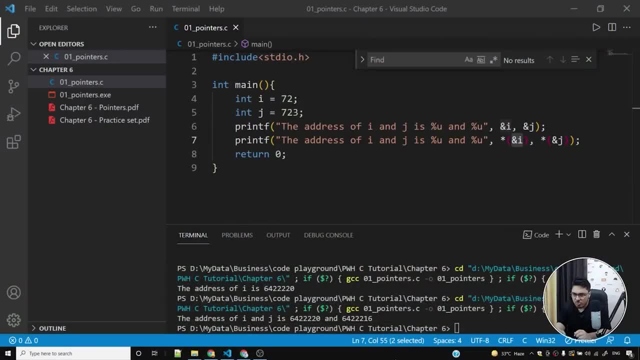 your house, inside your room, and let us say your house number is 24, what if i say house number of harry and the person inside it? so if i ask you is a person inside house number 24 of harry, what will happen? who will be that person? it will be. 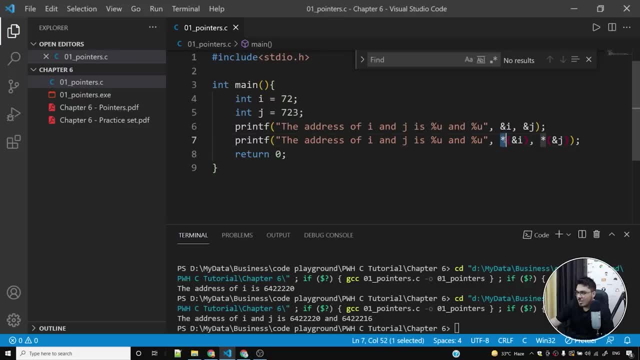 harry. okay. so in a very similar way, if i say value at address of i, it will be i. what is the value 72 in? in a very similar way, value at address of j will be j. so let me change this value of i and j's. 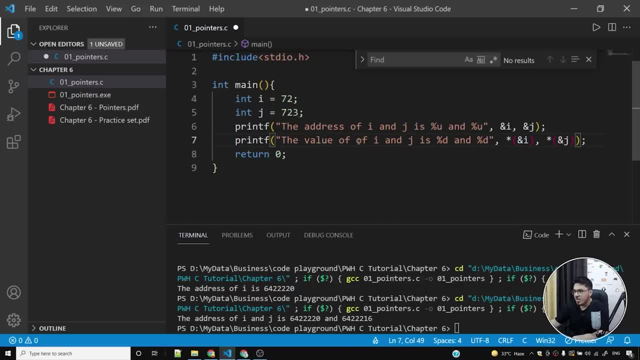 i'll say percentage d, percentage d. okay, so value of i and j's will be printed using this. definitely you will never use this kind of concept. to you know, print the value of i. you will simply use percentage d and i to print i. but just in case you are given, 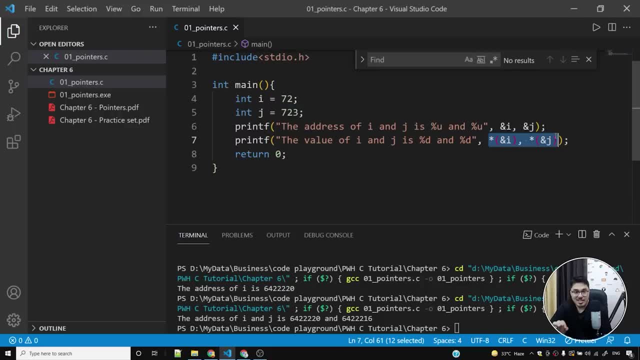 a question and you are asked: what will this line print in a c program? you should be able to answer: okay. so if i run this program and if i show you the value of i and j is 72 and 723, let me write a backslash and beautify this. so if i save this program and if i run this, you will see the value. 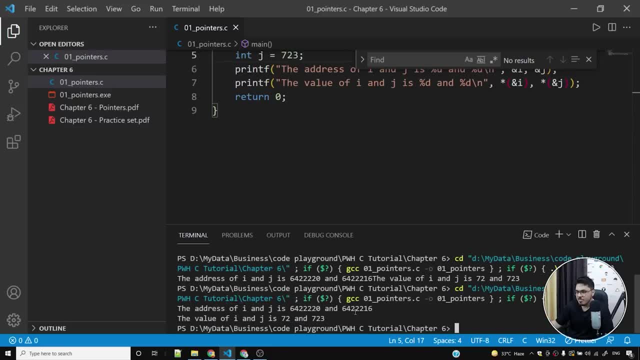 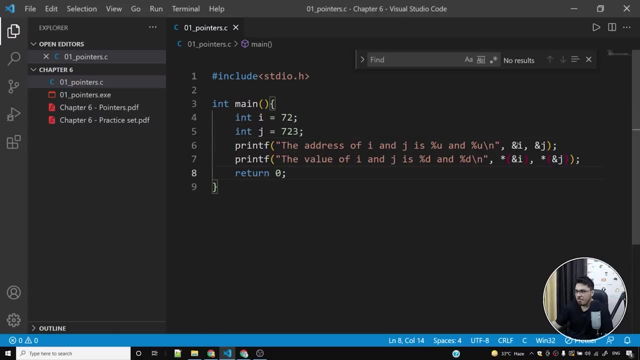 of i and j, 72 and 723 and the address 220 and 216. okay, so these are the addresses which were allocated to i and j, and 72 and 723 were the values. so i hope you understood ampersand and star operators. ampersand is address of and star means value at. okay, so this, this was pretty simple. 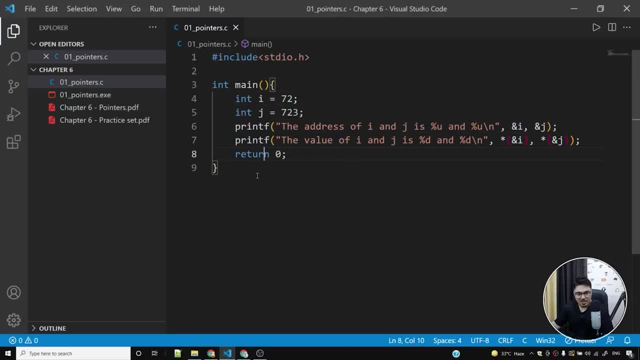 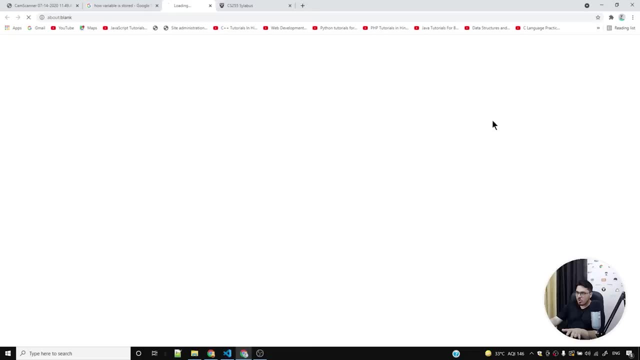 so far and if you listen to me carefully, definitely you should have understood how these things work. okay, so the image that we were talking about, uh, i, i clicked on this image and i opened this. i don't know which link is this, where is this coming from, but i gave it a read and it. 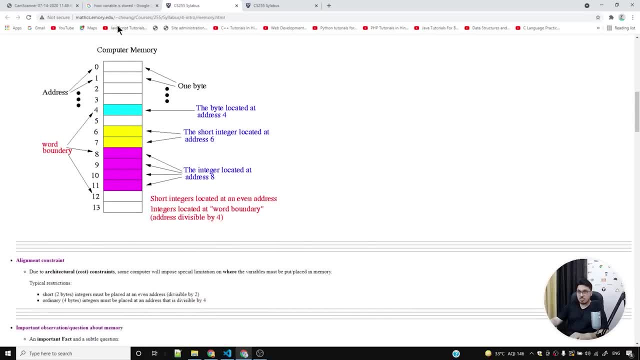 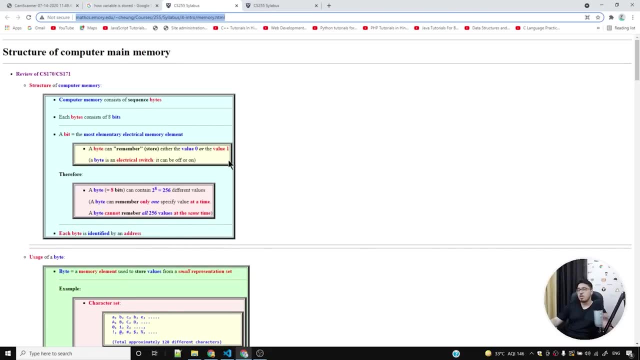 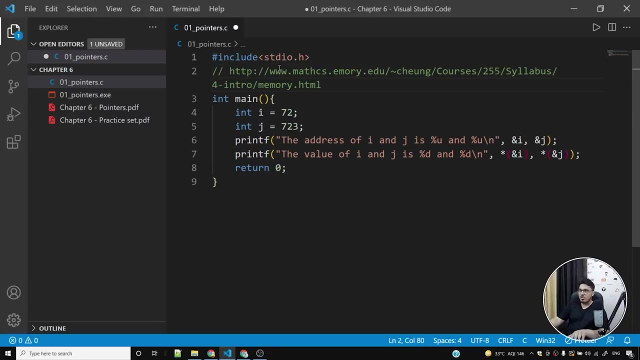 was actually good and it will make you understand how computer memory works. so just in case you want to deep dive into computer memory and look into how memory works, i think you can use this resource because i i gave it a read and it really explains it well, so let me paste this link for you here. i'll write a comment here you. 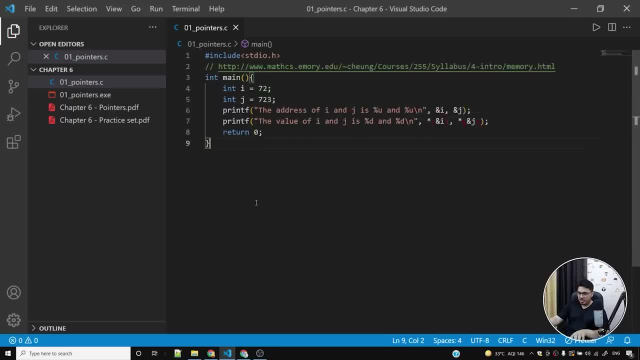 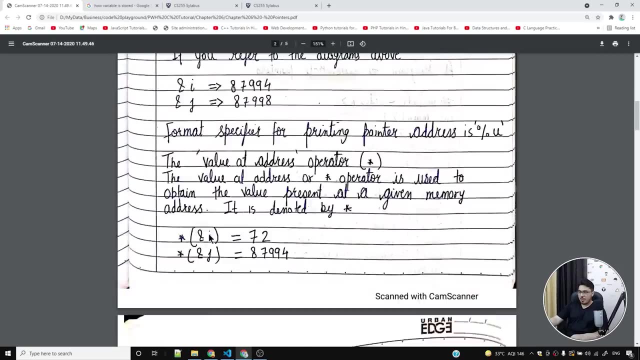 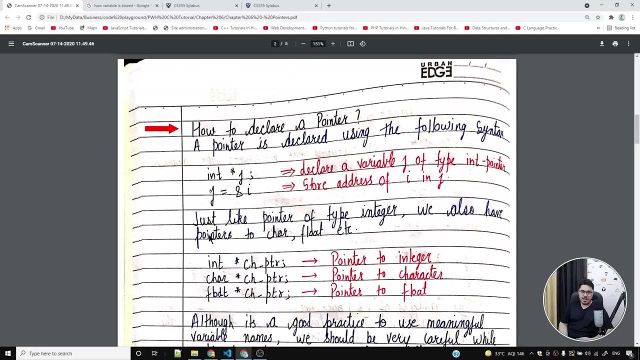 can click here and you can go to this particular page and, yes, it is good. now we'll move on further and talk about the further concepts. okay, so now that you know what ampersand operator is, what star operator is, we look into how to declare a pointer. how is the pointer declared? 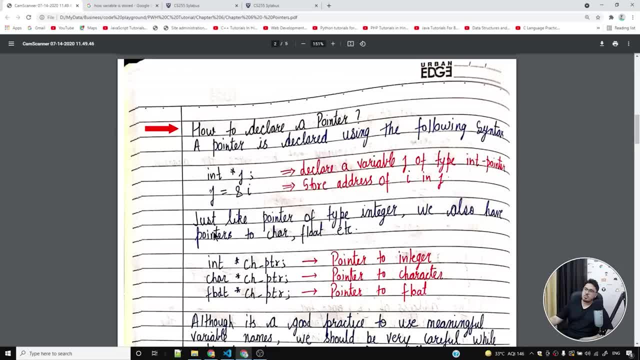 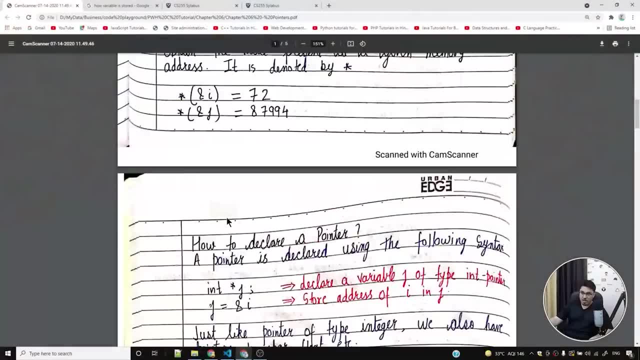 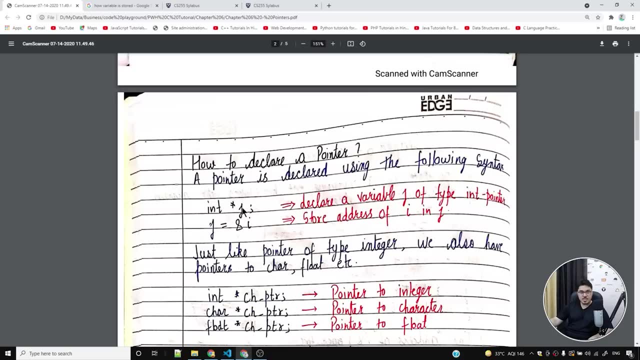 so a pointer is declared using the following syntax: so this is a syntax which we can use to declare a pointer int star j. so do not confuse the star with this value at address operator. when i say in star j, i'm simply saying that j is a pointer. that's it now. this might be very confusing. 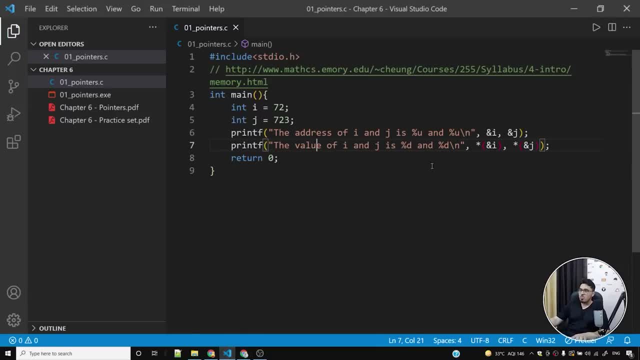 for you, because you you'll tell me that, hey, harry, you just told me that star means that decode this address and give me the value of this. and you are saying that in star j can be used to create pointers. so, yes, let me show you something. so, let me show you something. so let me show you something. 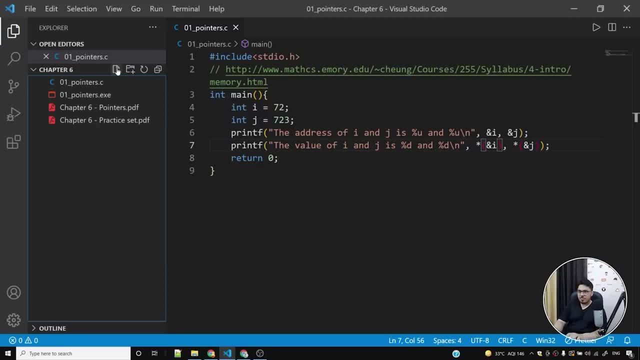 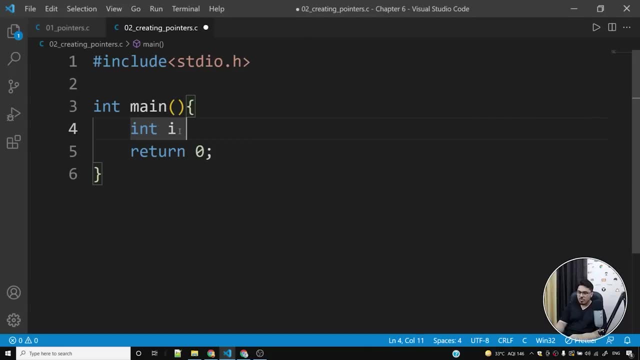 creating pointers. let me add boilerplate code. let us say i want to create a variable which is going to store address of an integer. so if i say int, i is equal to 72. now let us say i want to create a variable which will store the address of i. so if i do something like this, in j is equal to. 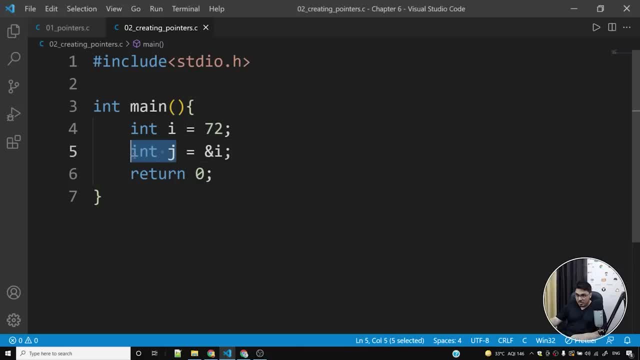 ampersand i, j is an integer. i cannot store address as an integer in c. in order to store the address, i'll have to create a special kind of variable, which is a pointer variable, and in order to mark this j as a pointer- when i mark j as pointer, i'm simply saying that j. 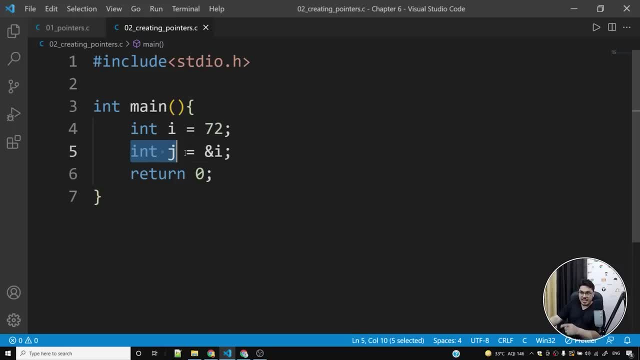 will now store address of some integer. when i say int j, i'm saying that j will store an integer. when i say in star j, i'm saying that j will store address of an integer. so if i say in star j is equal to ampersand i, it simply means that j is a variable which is going to store address of an. 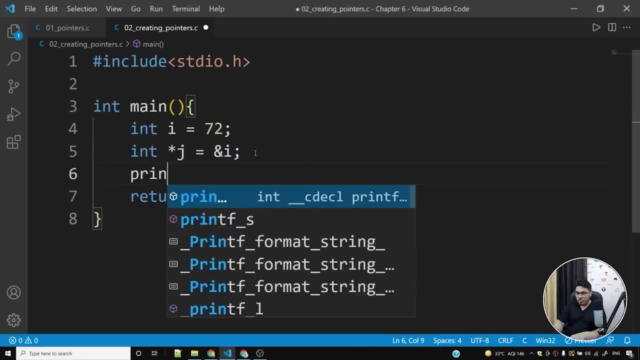 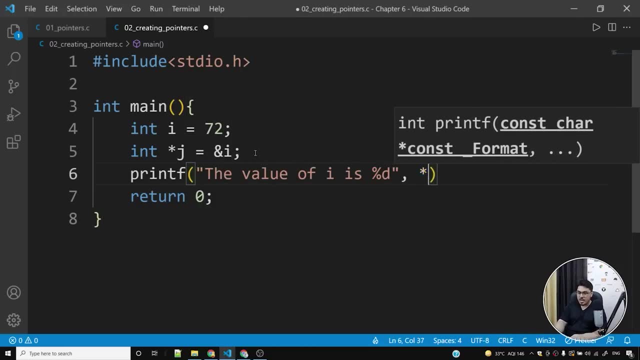 integer which holds the address of i. now i can do something like this. now i can say that the value of i is percentage d and what i can do is i can say star j. okay. so the moment i say star j, what it means is it means that decode the value at address j. okay. so if i run this program, i'll get. 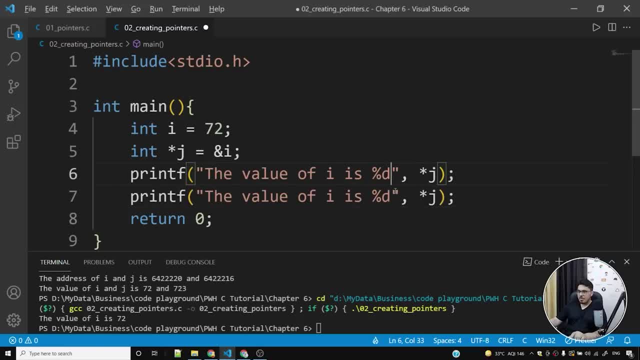 the value of i is 72. let me show you another example and also i'll add a backslash and so that things look good. if i say value or other address of i is percentage u and i simply say j, so j is nothing but address of i. so when i say int star j is equal to ampersand i, it simply means that j will now hold. 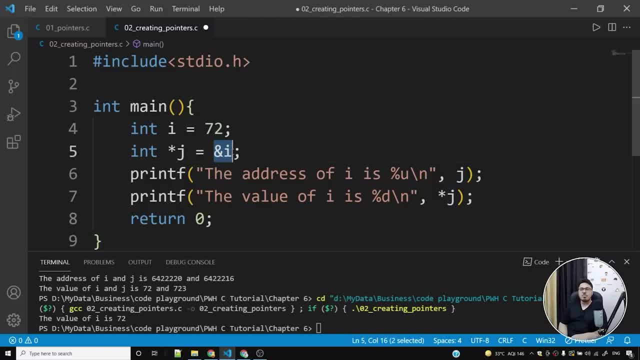 address of i. now this might seem really very complicated to some of the people who try to map. you know the the use of the star operator with declaration of a pointer. this is a pointer declaration and star, when used with a variable, simply means what is the value at this. 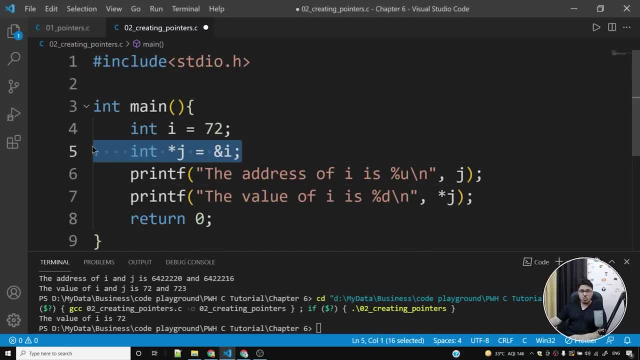 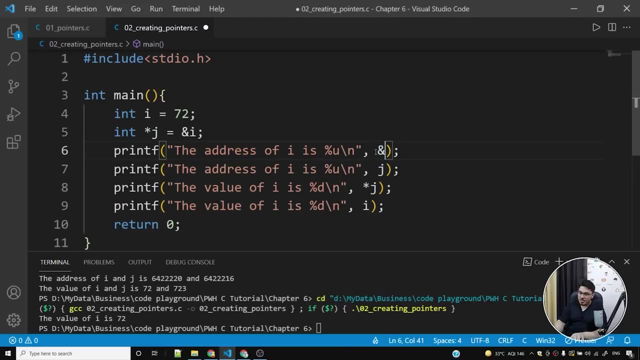 address. okay, so this is something that you nearly need to wrap around your head now. the address of i is this. the value of i is this: what else is the value of i? i can simply write i. this will also give me the value of i. j will give me the address of i ampersand. i will give me the address of i. 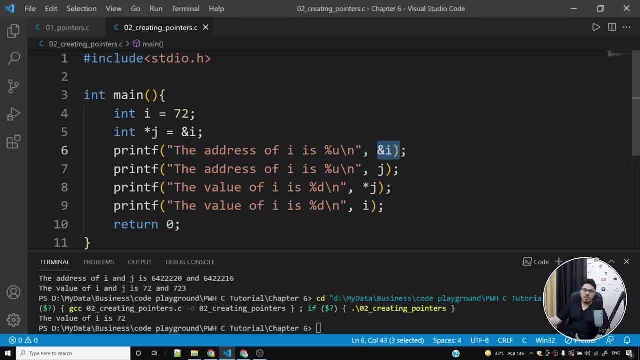 so i can say percentage u ampersand i. this will give me the address of i. i can say percentage u directly j, since i have used a pointer variable and i've said in start j is equal to ampersand i. this will give me the address of i. this will give me the value of i, because what i'm doing is i'm. 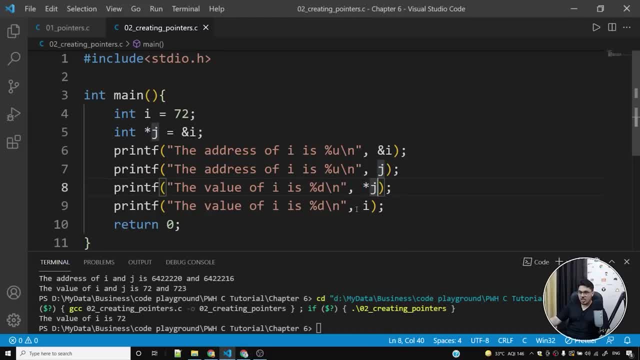 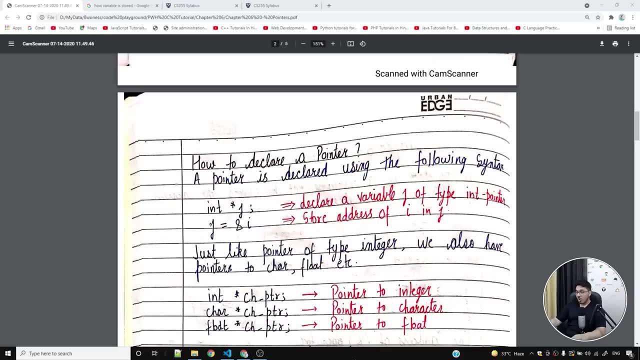 using value at operator and i'm simply using j and i can also say: the value of i is percentage di. this will also give me the value of i. now, if you come back to the notes, you'll find out that i have told you how to declare a pointer here. so a pointer is: 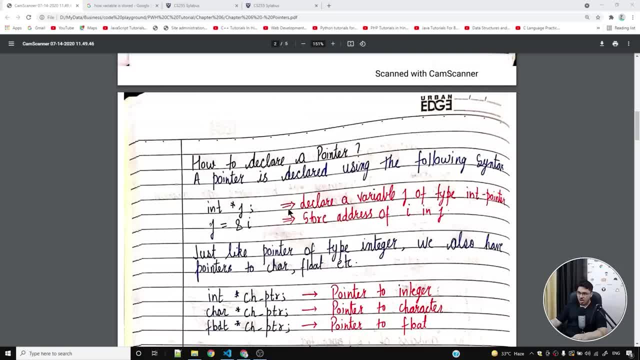 declared using the following syntax is what i've written here: int star j declare a variable j of type int pointer. you can simply declare an integer pointer by typing int star j. so when you say int star j j will be an integer pointer. now you can use j is equal to ampersand i to assign the address. 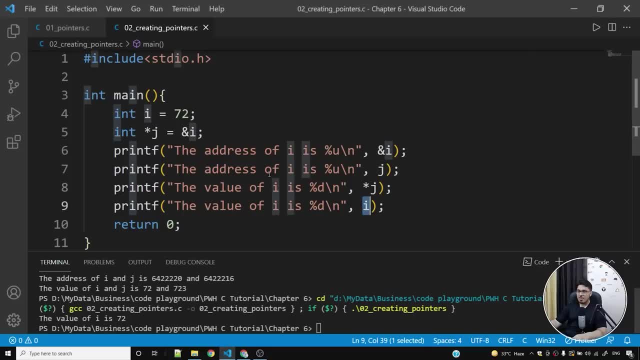 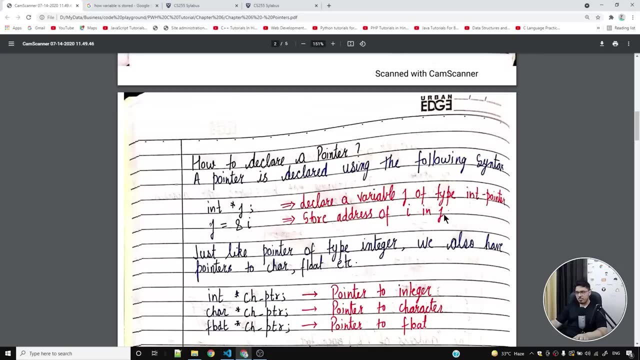 of i inside this j we have. we have already seen this in the program and once you run this program you will understand a lot of things. i've written those things in the notes as well, so store address j using this just like pointer of type integer. we also have pointers of type character load double. 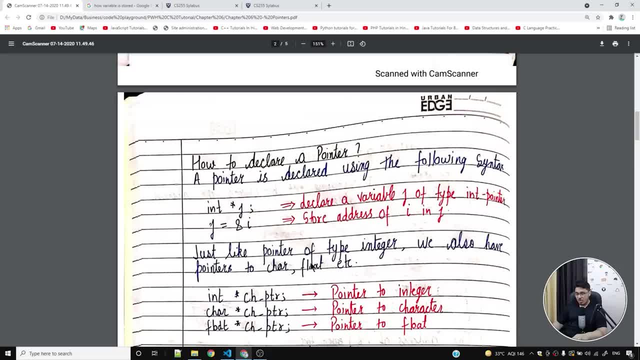 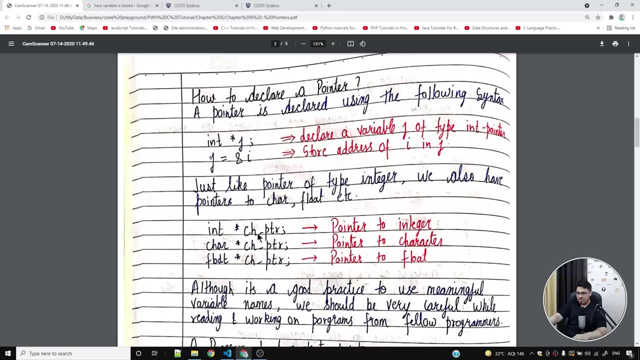 you can have pointers to any data type now. we'll also learn about custom data types in later chapters and you can even have pointers to those custom data types. but let's start easy and let's look into integer pointer, character pointers and float pointer. so when i say int, star, chptr, this: 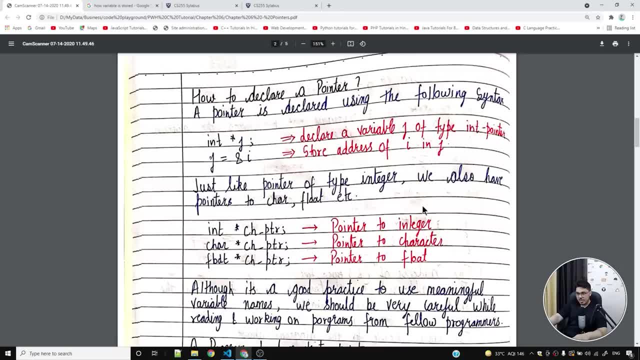 can be any name. i'm using chptr, this is pointer to an integer. if i say char star chtr, this is a pointer to a character, because i've written char here. now, if i say float star chptr, it's pointer to a float, because i've written a float here. okay, int star chptr, char star chptr, float star chptr. 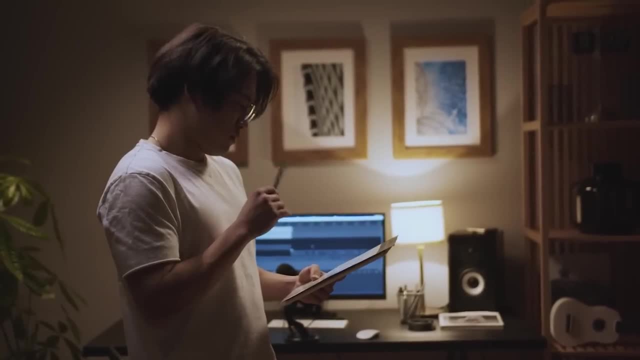 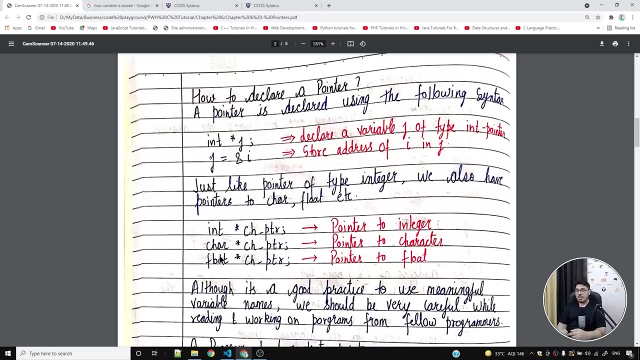 now what happens is a lot of students. they get confused with the name of the variable. you should never look and rely on the name of the variable. so if the variable name says amount of sugar in coffee, that doesn't mean that the amount of sugar that that person has drank in his coffee in the morning will be same as the value of that. 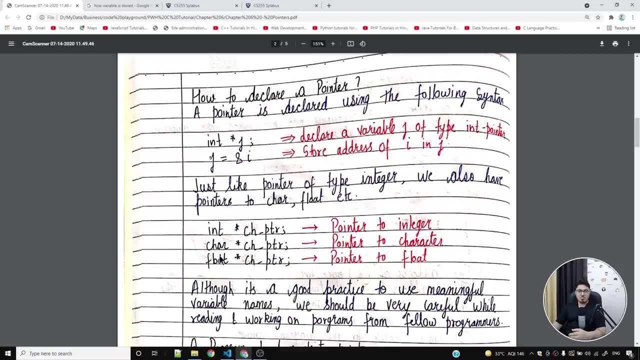 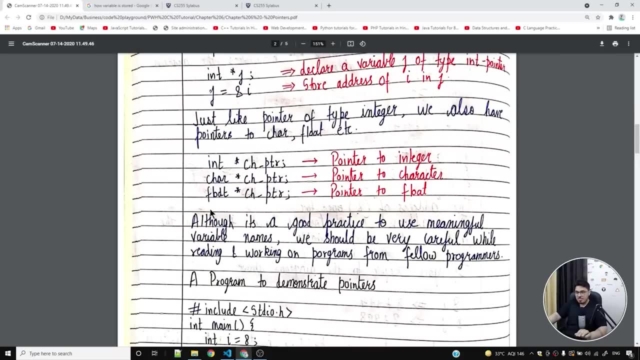 variable. people will write anything in their programs and it's your duty to verify whether a given pointer is a character pointer, integer pointer or a float pointer. merely naming a variable as chptr doesn't make it a character pointer. what exactly that variable is matters, okay. so i've written the same thing here. i'm saying here that, although it's a good practice, 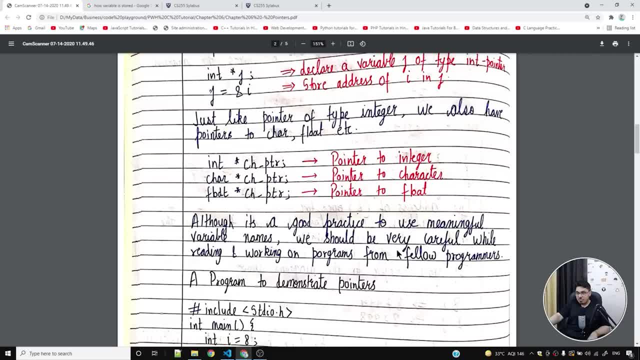 to use meaningful variable names. we should be very careful while reading and working on programs from fellow programmers. so if you are working on programs from your fellow programmers who have written some code and you want to make sure that whatever they have written is right or not, you need to verify from the ground truth and not from. 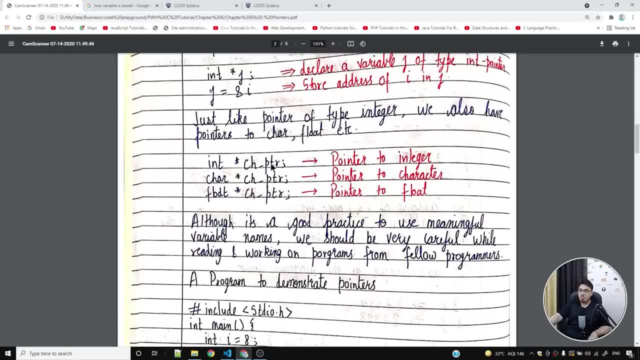 the name of the variable. in this case, if you say that this is a character pointer, it will be wrong because it's an integer pointer. i've used int star. simply naming a variable as chptr doesn't make it a character. simply naming a variable as chptr doesn't make it a character. simply naming a. 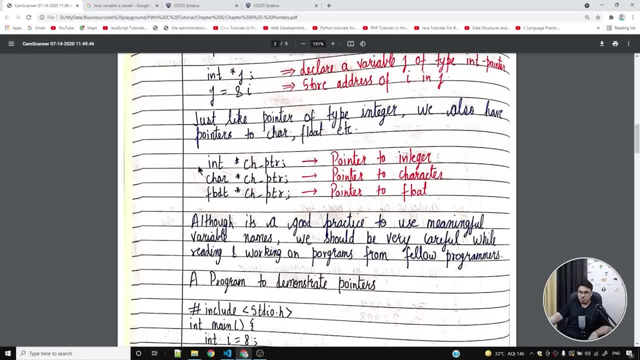 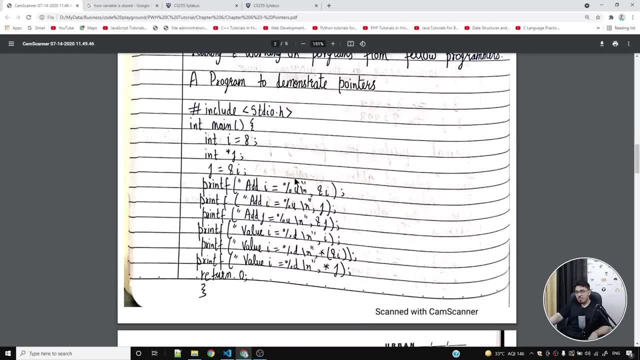 variable, as chptr doesn't make it a character. you should verify whether it's an integer, whether it's an integer pointer or some other type of variable. so i hope you got this point. now i have a program to demonstrate pointers here. i have already demonstrated you pointers. 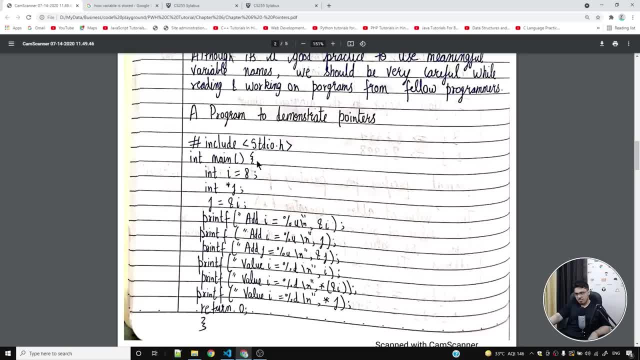 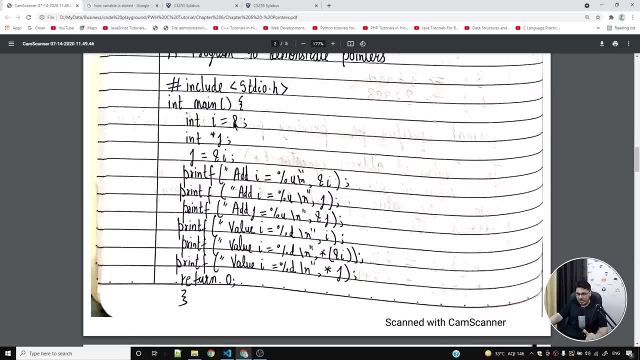 using this program, but i have written this program in the notes as well. let's try to see what this program is doing. so int i is equal to 8- simply assigns the value 8 to this variable i. and when i say int star j, i'm simply creating a pointer. 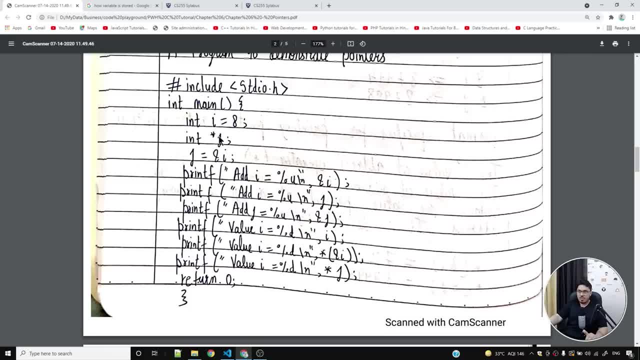 which is an integer pointer, and the name of that variable is j. now i can assign address of an integer inside this j by doing j is equal to ampersand i, so this j will now hold the address of this variable, which is i. okay, so what will happen if i say printf address i is equal to. 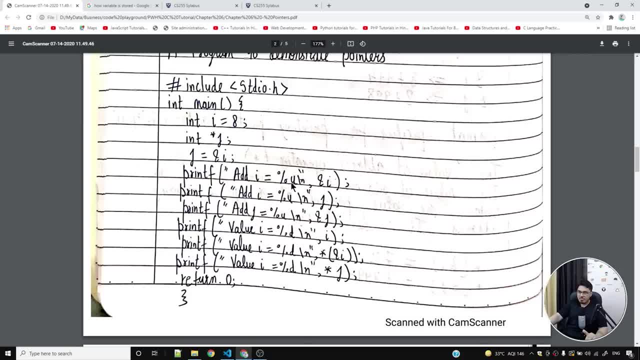 percentage u- ampersand i. percentage u- ampersand. i will print the address of i in a similar way. since j stores the address of i, what we can do is we can simply print the address of i. say: address of i is equal to percentage u, backslash n and j. what this will do is this will also print. 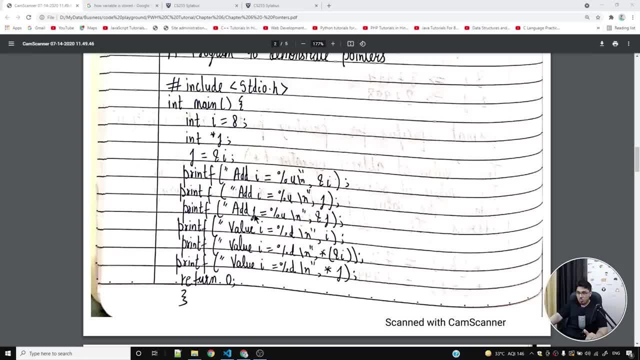 the same thing as this. this will print the address of i, but what if i print the address of j? now, j is also a variable. it's, it's a pointer variable. what is j? j is something which stores the address of i does. it has its own address. yes, it does. it does has its own address. now, this is something that. 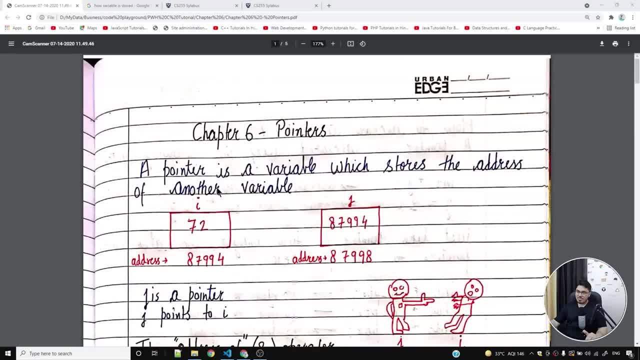 comes into some of the people. so let us say i have this variable 72, it is stored at address 87994. if i say address of i, this is the address of i, but if i create another variable, j, and i store the address of i inside this variable, this in itself is a variable which will have some other. 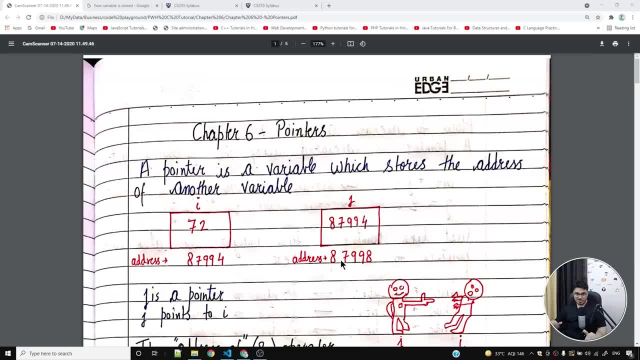 address. so address of address also exists. so this is a variable i. it has this address. this is a variable j, which is a pointer, which means that j is the address of i. so i will create another variable made to store the address of integers. this will also has its own address, which is 87998. 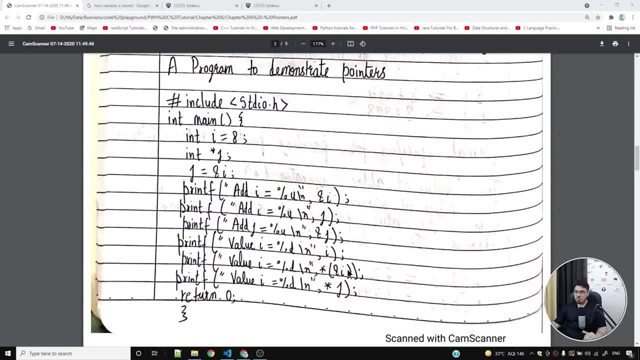 okay. so in a very similar way, when i say ampersand j, this will be some other address and it will be address of j's. j is a variable. at the end of the day, j is a variable. it is a pointer variable which stores the address of an integer variable, but at the end of the day, it in itself is a variable. 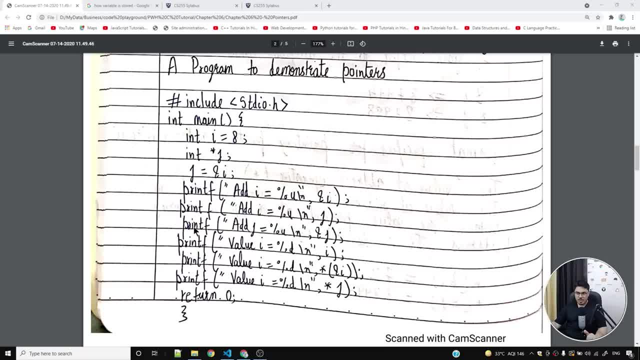 so when i say something like this, ampersand j, this will print address of j in a very similar way. i can print value of i just like the traditional way. i can also say ampersand i and wrap it and put a star operator which will decode the value by using the address, and this will also. 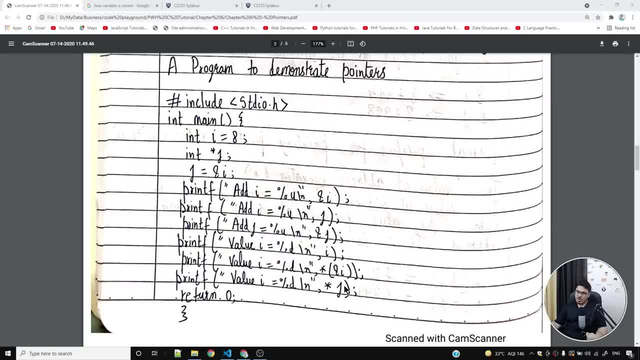 print the value of i in a very similar way. this will also print the value of i, because j is nothing but ampersand i, j is nothing but address of i and if i decode this address, if i find the value at this address, this will give me the value of i, so this program will return this. this is the address of i. this is: 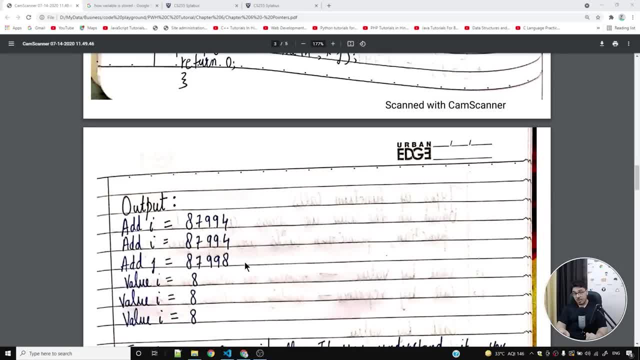 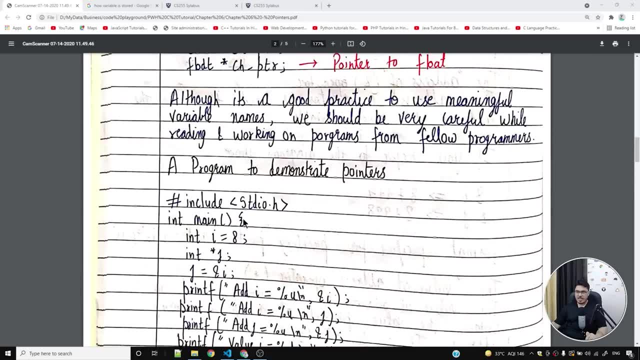 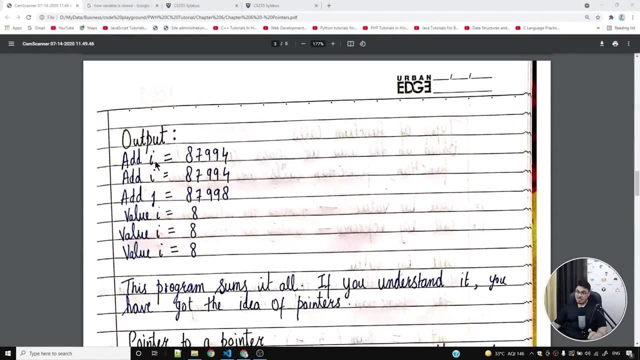 the address of i. this is the address of j, which is storing the address of i, but at the end of the day, j is a variable. it will have some address. so this is the address of j and the value of i is 8, as we have already seen. so type this program inside your visual studio code and see. see this. 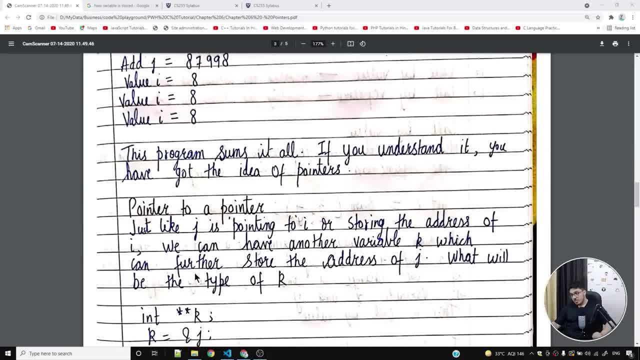 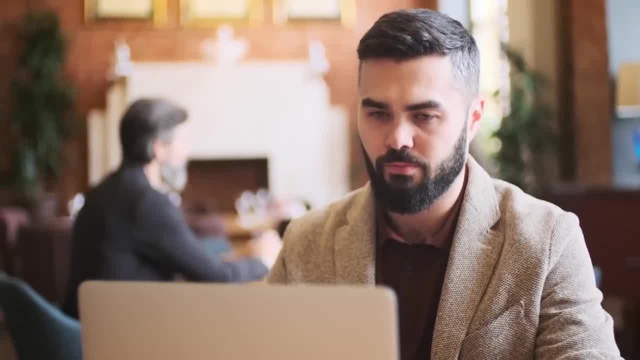 output. okay, now what we'll do is we'll talk about pointer to a pointer. so this program sums it all. you, if you understand it, you have got the idea of pointers. so make sure that you understand this program, because i don't think you need anything else to understand pointers. 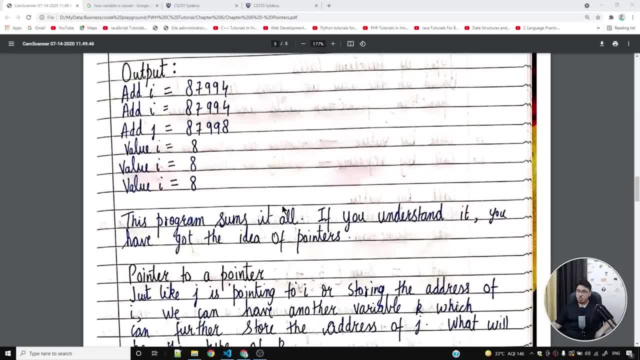 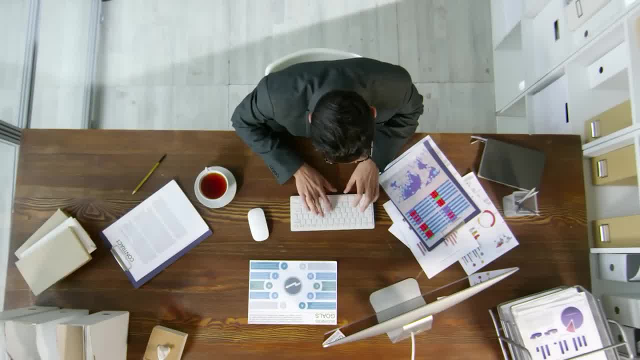 in case you haven't understood what pointers are, you need to watch this chapter once again. it means you are not paying attention. if you have paid attention and you have listened to me carefully, and if you have coded along with me, i can give you a hundred twenty percent guarantee that you 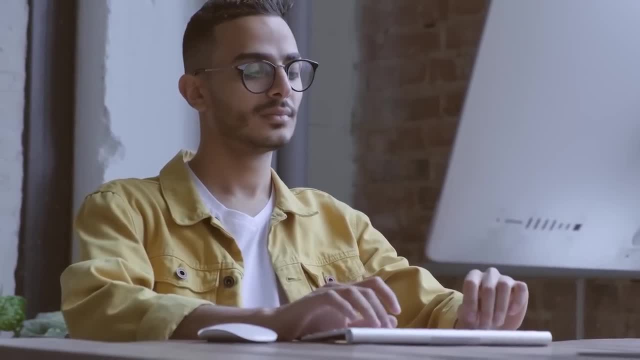 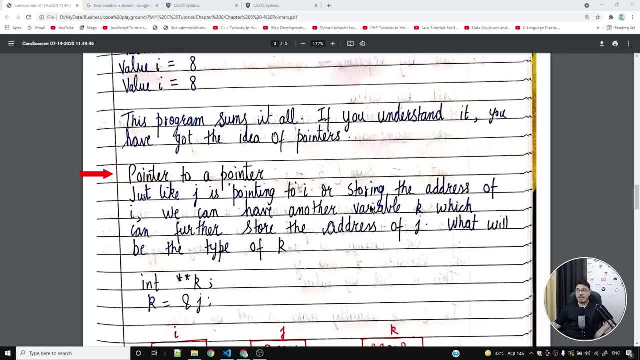 understand what pointers is. this is the amount of confidence that i have in myself. now, pointer to a pointer, just like j is pointing to i or storing the address of i, we can have another variable k which can further store the address of j. what will be the type of k? tell me. 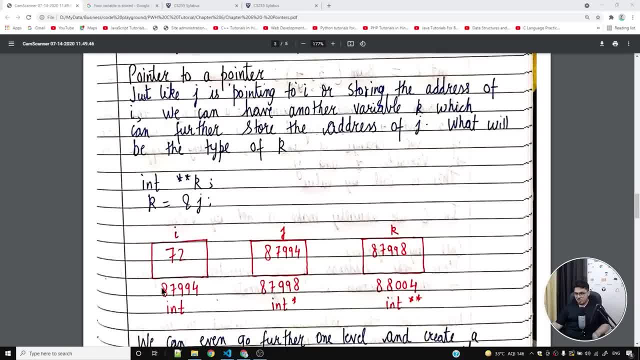 it will be pointer to an integer pointer. okay, so let's, let's try to understand this, and in order to create this pointer to an integer pointer, i'll have to put double star. so int star j simply means that j is a pointer to integer int star, star j, or rather int star. 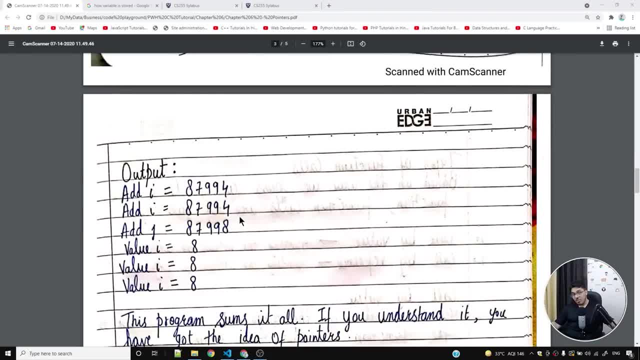 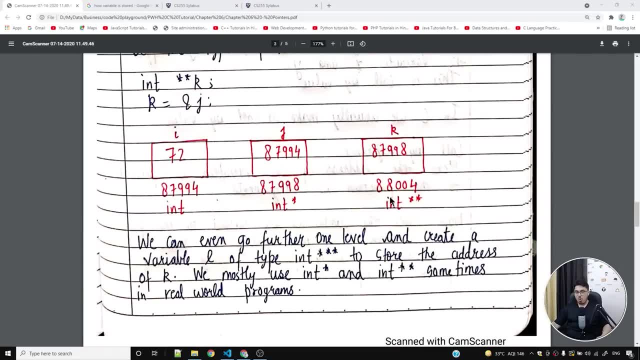 star k will mean that k will store address of an integer pointer okay, and we can take this chain as long as possible, but in most of the cases you will not see pointer to a pointer. you'll definitely see pointers, but even pointer to a pointers are very rare. but we need to understand. 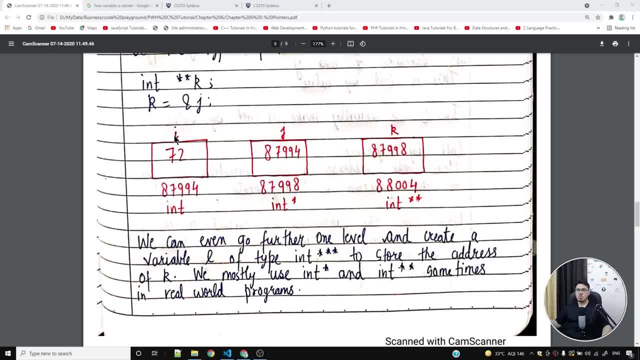 this. let us say i created a variable i. i stored 72. i has the value 72. this i will hold some address in memory. what is the type of i? it's an integer. i've done nothing so far. i've simply created an integer i and assigned a value 72 to it. now, if i say int star j and if i store the address of 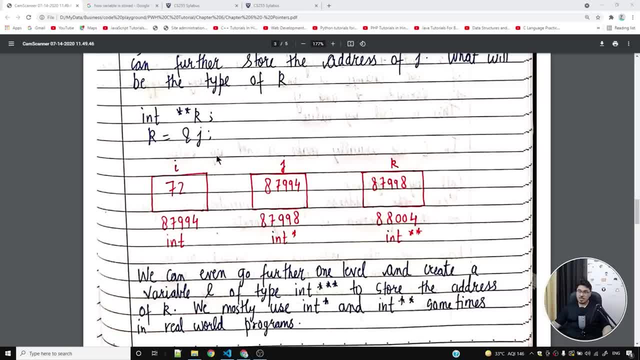 i inside j. what is the type of j? it's int star, which means pointer to an integer. this variable, this j variable, stores address of an integer and it will definitely have its own address in memory. since it's storing in memory, it will have some address in memory. what is that address? let us 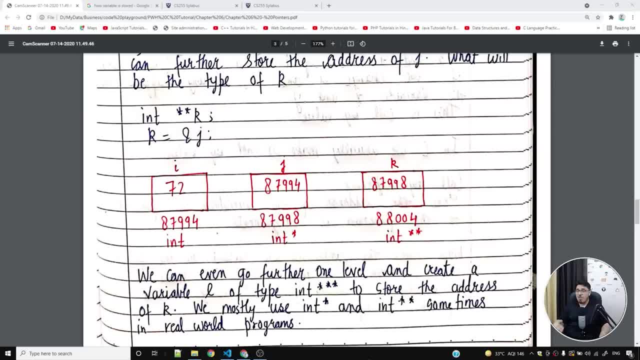 assume this is the address of j and it will definitely have its own address in memory, so that address is 87998. now what i want to do is i want to go a step further and i want to create a variable k which will further store the address of j. what will be the type of this variable? it? 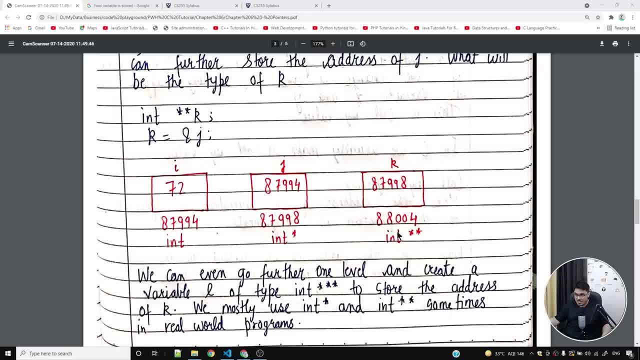 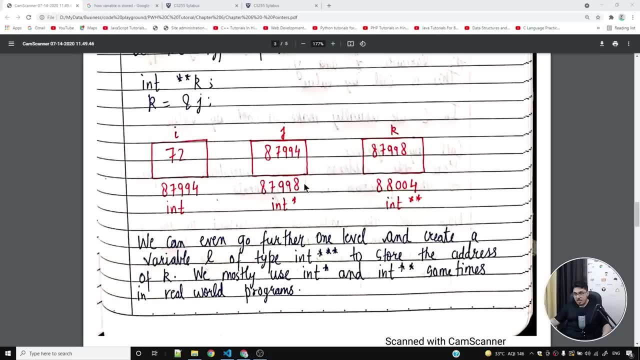 will be int star star. int star star means pointer to a pointer of an integer. so pointer to an integer pointer, so this is pointer to a pointer. okay, so k will store the address of j and it will store the address of something which was storing address of an integer. okay, so we simply denote it. 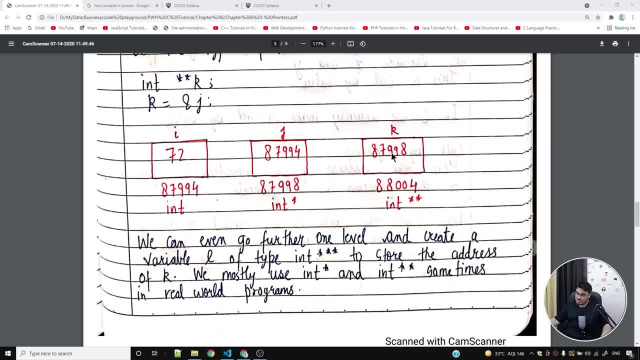 as a in triple, sorry, in double star, and this in itself will also have some address. and we can have another variable, k, sorry, l, which will store this address, and we'll have to write in triple star. but again, that is very rare and you don't have to, you know, think that much. we can go even further. 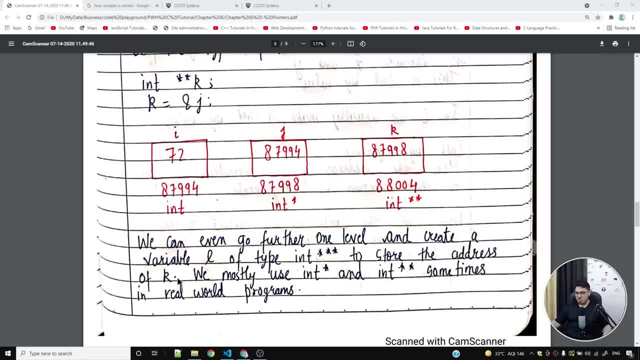 one level and create a variable l of type in triple star to store the address of j and we can have the address of k. we mostly use int star in. in most of the cases you will encounter pointers. even pointer to a pointer is sometimes um you can see in real world programs but it's very rare. 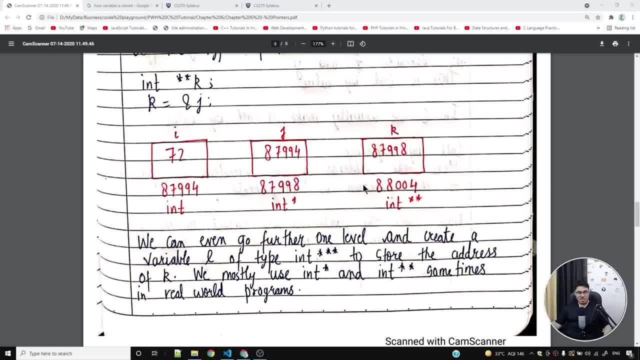 in triple star is really very rare, okay, but again, you need to understand that pointer is nothing but a variable. it's simply a variable which stores address of another variable. i hope you understood what pointer says. now we are going to look into the two types of function calls, which is called: 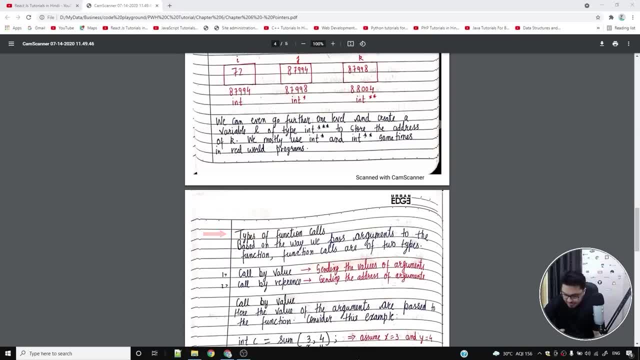 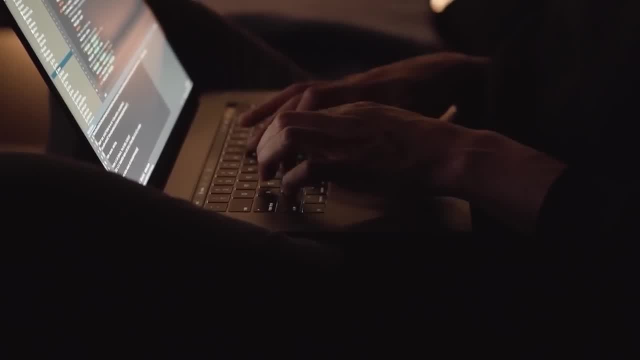 by value and called by reference. this is something that you will definitely need when you are programming in c, and this is something that you are going to encounter a lot of times. even if you are writing a c program with even a little bit of complexity, you are going 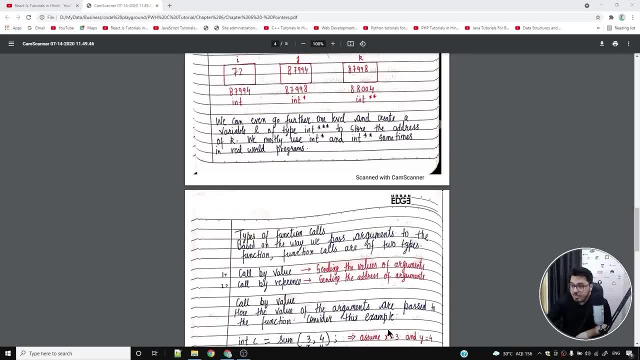 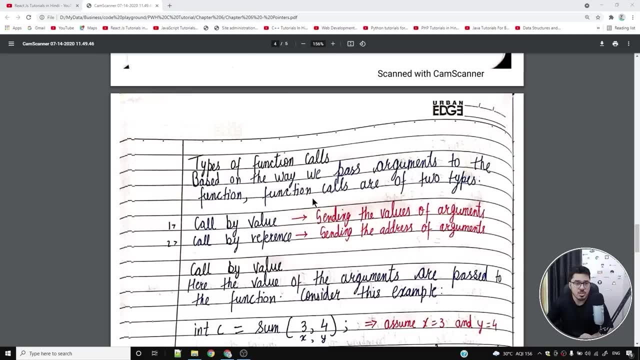 to look into these types of function calls. so it gets really very important for us to understand what these types of function calls are. so, based on the way we pass arguments to the function, function calls are of two types: called by value and called by reference. you must be thinking we. 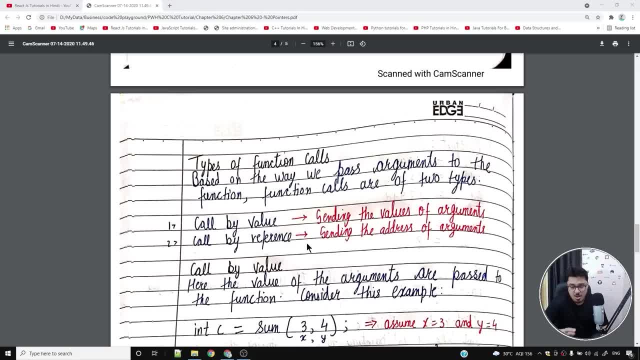 have already looked into functions and function calls, but let me tell you a little bit about the function calls that we have in triple star. let me tell you something: you can either pass the value of arguments or you can pass the address of the arguments. let me tell you what it means. let's talk about call by value. so 03 underscore. 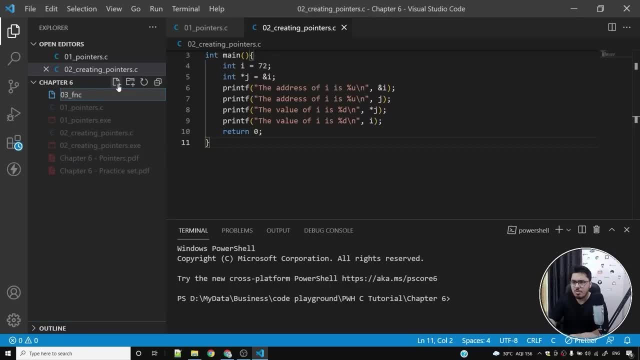 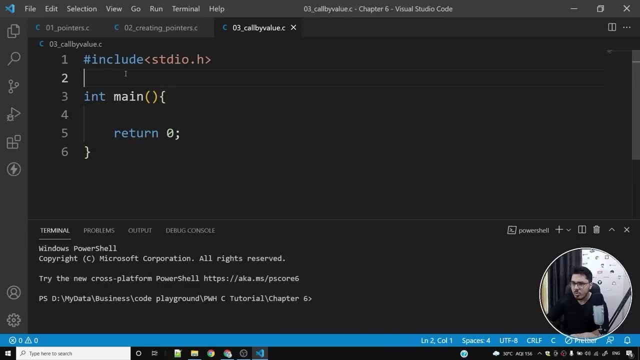 it's called call by value dot c- call by value dot c. let me put the boilerplate code, and what i'm going to do right now is i'm going to say int, sum, int, int, and this is a function that's going to return. it's going to take two integers, so all i need to do here is i'll say int a and then in b, and then i'll 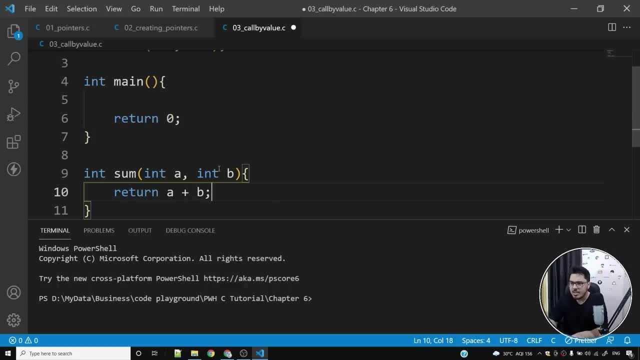 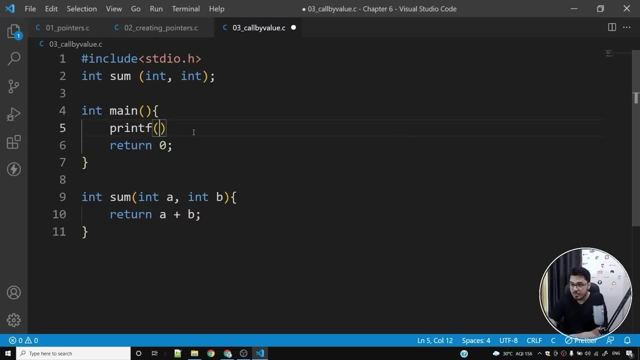 say return a plus b, and this is my function. pretty straightforward, okay. what i'll do is i'll say printf, i'll simply say the value of a plus b is, and i'll say percentage d. and what is my percentage d? it's sum, say 3 comma 6, and if i run this program, you can see the value of a plus b is 9, nothing surprising. 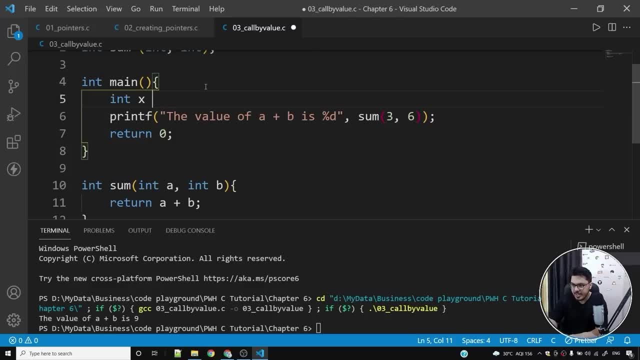 so far. what if i have two variables here? i'll say int x is equal to 5 and y is equal to 4, and i'll simply say x comma y. now if i do something like this and if i run this, you can see that the value 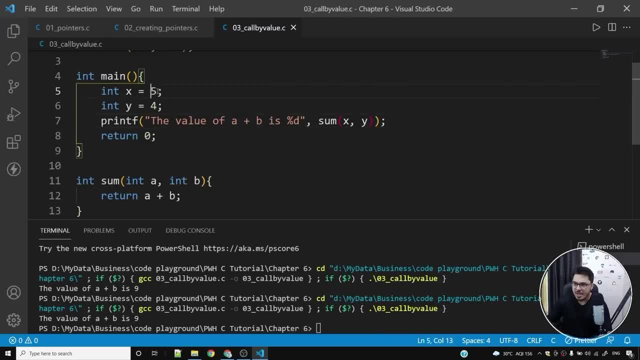 of a plus b is 9, so it's simply adding 5 and 4. so how? how does this work? let's try to understand how this works. so whenever we are giving a function call like this: sum x, comma, y, what happens is that x and y, both of these values- they are passed. 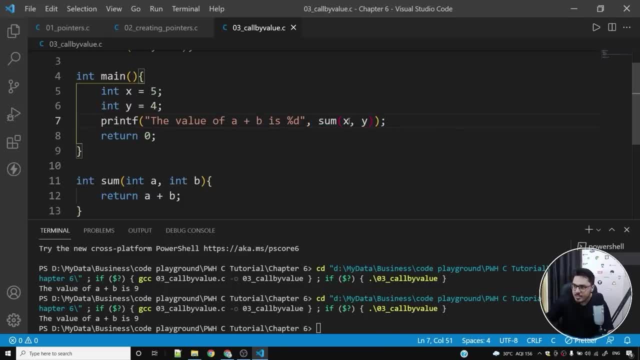 to this particular function sum. so x is 5 and y is 4, so 5 and 4 are copied into a and b. i'll repeat this for you: the values x, y, which are nothing but 5 and 4, are copied into a and b, and 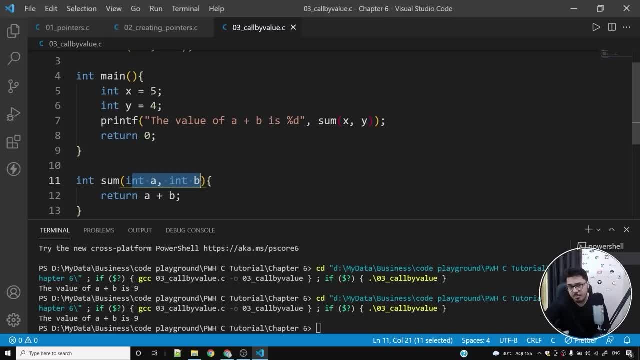 so a becomes 5 and b becomes 4. okay, so now this function will return 5 plus 4, which is 9. so basically, what happens is when, when i say in sum, int a, int b, a will be equal to this value and b will be equal to this value and a will simply be assigned. whatever the value of x is, b will. 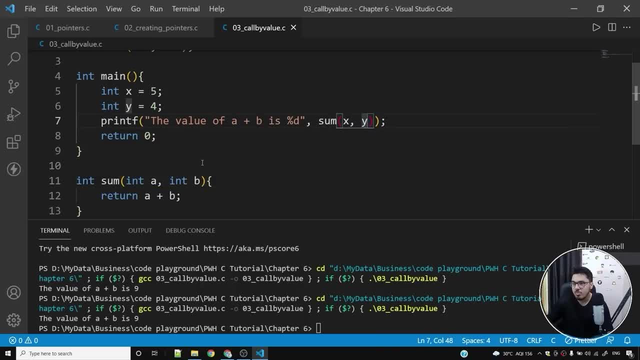 simply be assigned whatever the value of y is. so we are creating a copy of x and y, so will x and y be changed? what if i say the value of x and y is: uh, x and y is. let me make it x and y. i i wrote it as: 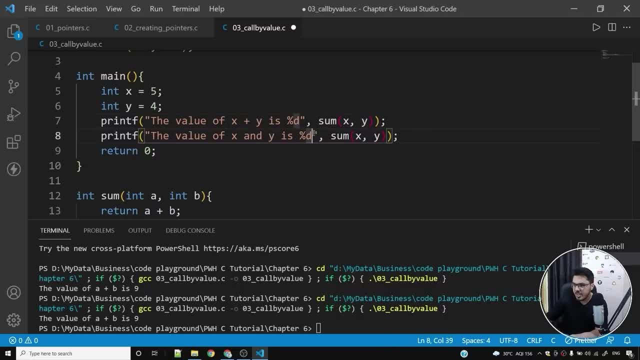 a and b. but let me write it: x and y is percentage d and once again i'll say percentage t and i'll simply say x comma y, because i want to. i want to print the values of x and y. so i'll save this program and i'll also use backslash n so that i can see a new line after this. so the moment i run, 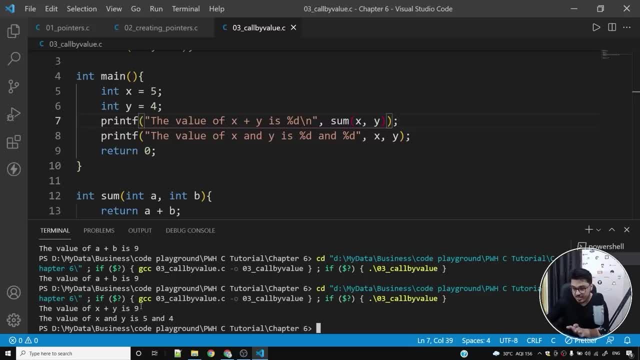 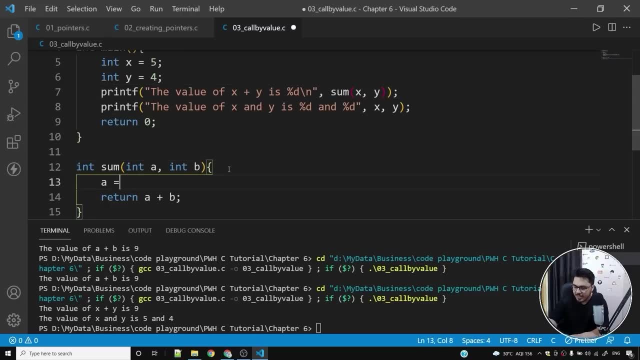 this you can see the value of x plus b is 0, so i'm going to print this and then i'm going to: 5 is 9, x plus y is 9 and the value of x and y is 5 and 4. okay, now what if i do something like this: 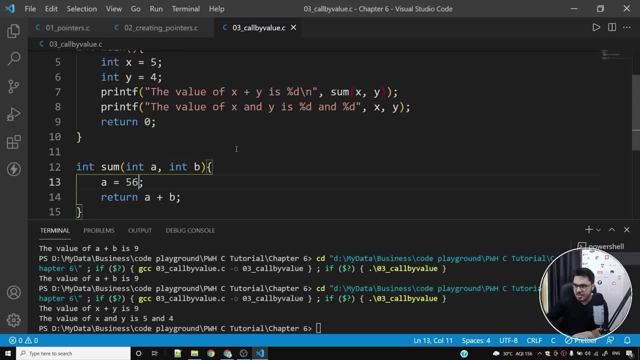 i'll say a is equal to say 56. can i do something like this? let's try to run this program. when i try to run this program, you can see the value of x plus y is 60, but the value of x and y is 5 and. 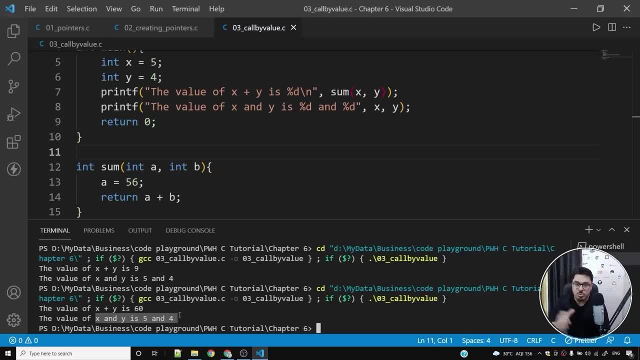 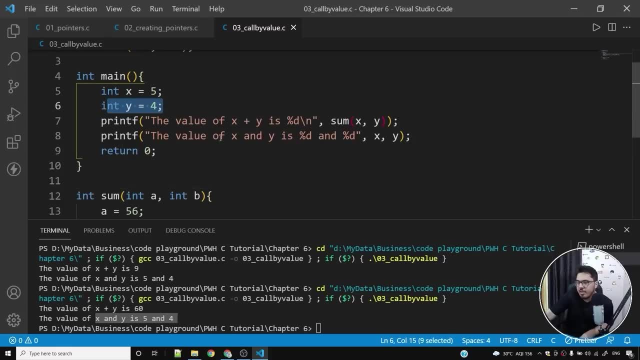 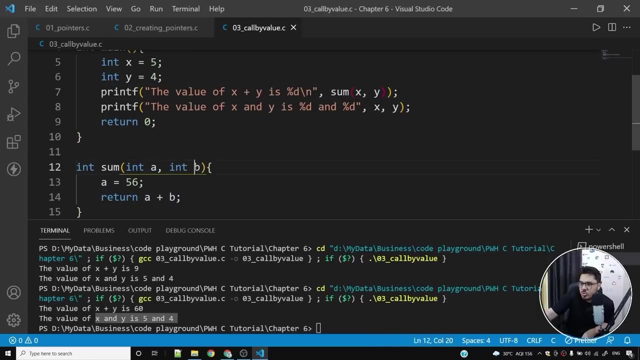 4. what is happening in this program? let's try to understand, let's try to dissect this program. you'll see that the value of x is 5 here and value of y is 4 here. and when i say the value of x plus y is percentage d. basically 5 and 4 are copied into a and b. so a is 5 and b is 4. but here i've changed. 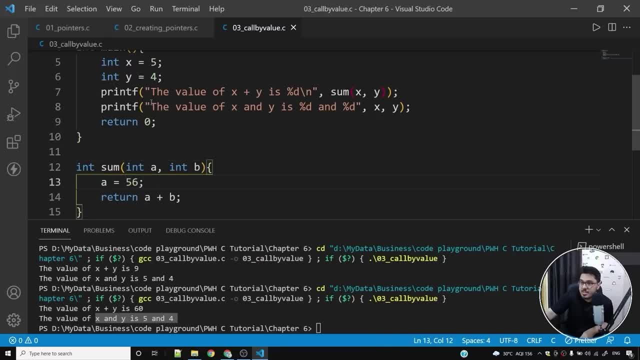 the value of a. so now a is 56 and b is 4. initially a was 5, b was 4, but now a is changed to 56, b is unchanged, which is 4. so 56 plus 4 is 4 and b is 4. so now a is 56 and b is 4. so now a is 56 and b is. 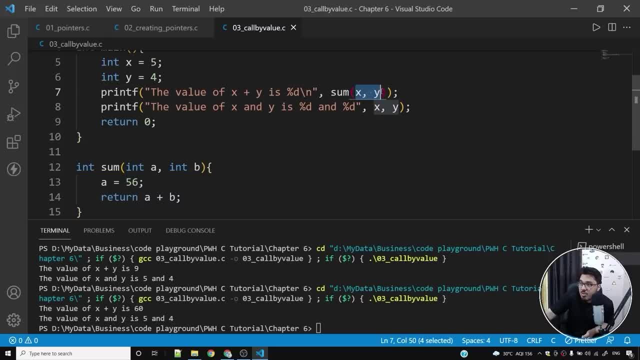 4 will be 60. but since the values x and y were copied, the copy of x and y were changed. so x and y will remain unchanged. so x and y will be nothing but 5 and 4. because i cannot change one function's value from other function directly. i can't do this directly. i can't say a is equal to 56 and 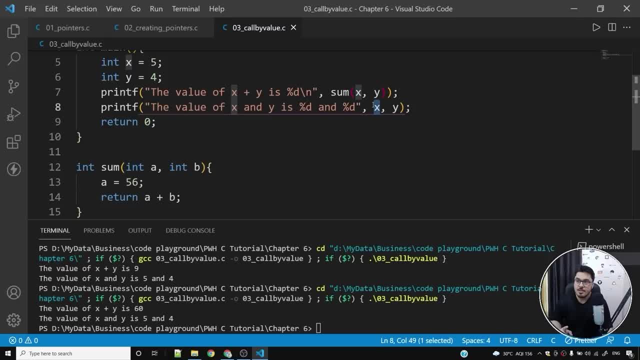 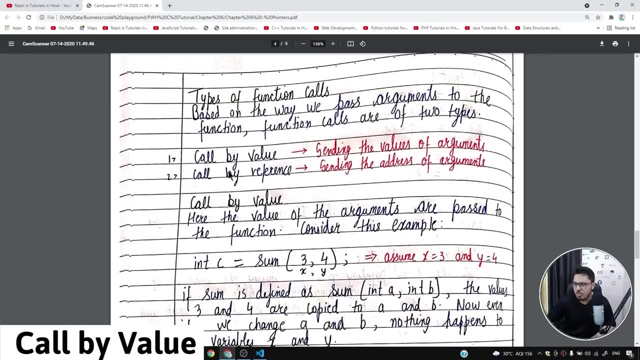 get this reflected here. that doesn't happen, but this is the normal scenario. this is called call by value. we have already seen this scenario. we were just understanding how the scenario works. so if you come back to the nodes, you'll see, based on the way we pass. 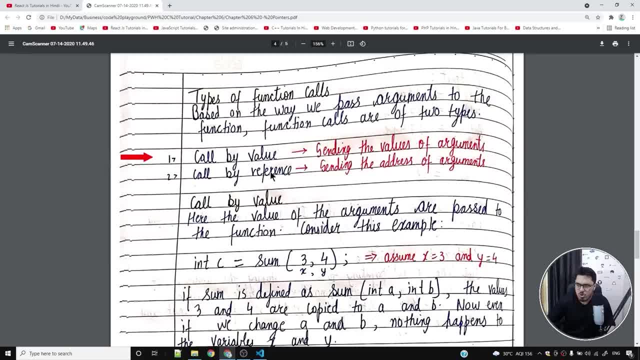 arguments to the function. function calls are of two types: call by value and call by reference. call by value means sending the values of argument. call by reference mean you are sending the address itself. now let's talk about this one. what happens when i'm sending the address itself? now let's talk. 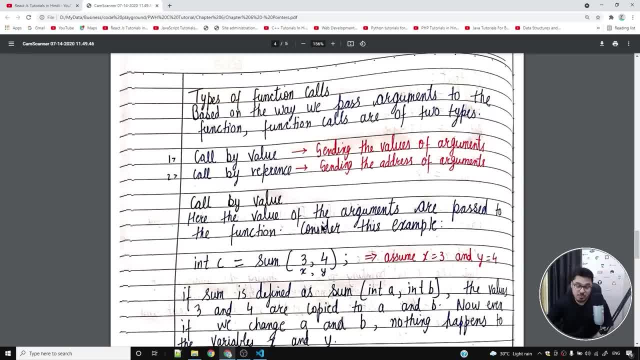 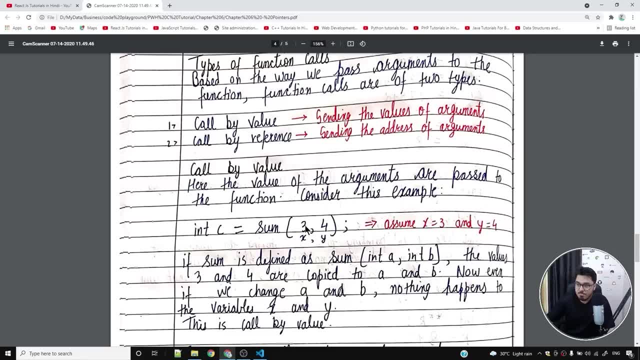 about call by value. here the value of the arguments are passed to the function. we have seen this. this is a normal scenario. you can consider this example when i say in: c is equal to sum 3, comma 4, 3 is copied as x and y is copied to sorry. 4 is copied to y and simply what happens is the sum is. 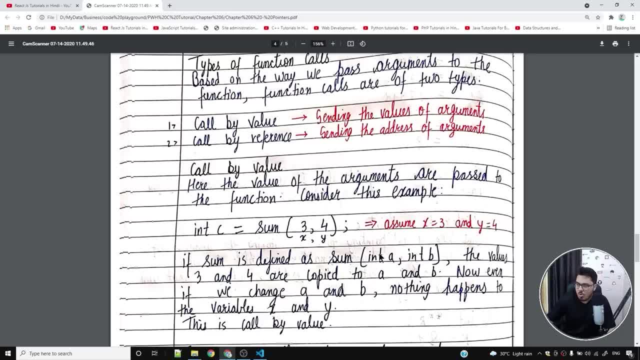 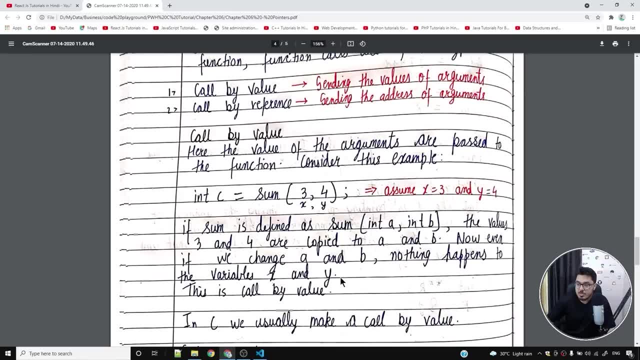 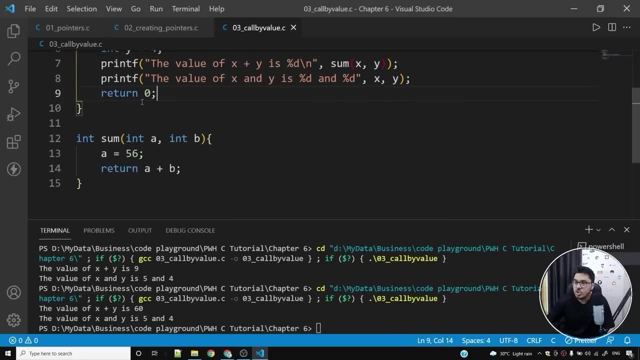 defined as sum: int a, int b. these two values are copied into a and b, and the values 3 and 4 are copied to a and b. now, even if we change a and b, nothing happens to the variables x and y. we have seen this. we have seen this here: nothing happens to x and y. okay, why? why? because i cannot change. 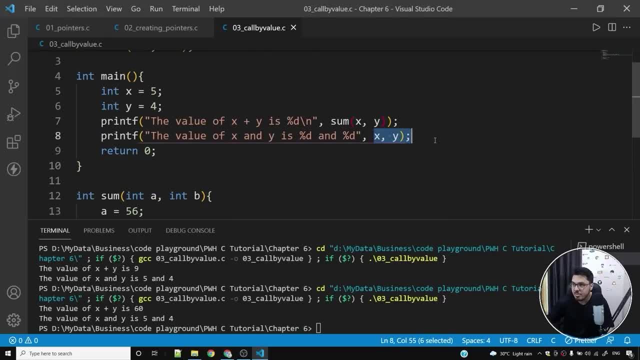 the copy this: a and b are different variables, x and y are different variables. when i say sum x, comma, y, the value of x will be copied to a and value of y will be copied to b. and now if i change a and b, it has nothing to do with x and y. i hope. 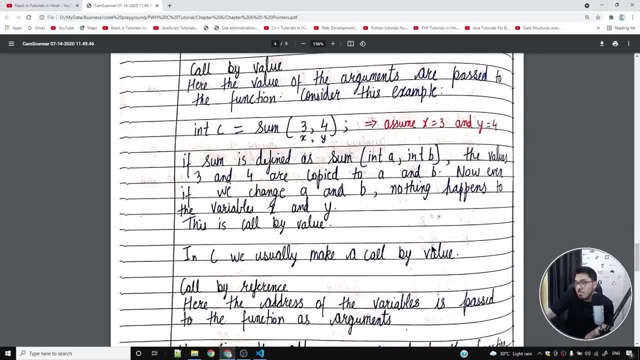 you got this one now. in c, we usually make a call by value. so far, we have made call by value. now listen to me very carefully: call by reference. this is something new. this is something that we have not seen. so i'm going to write a program to describe call by reference. so let me say something. 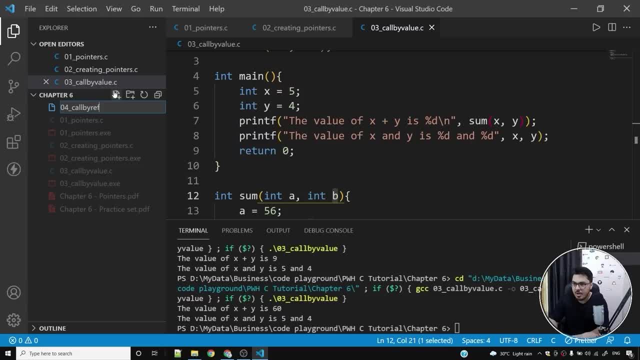 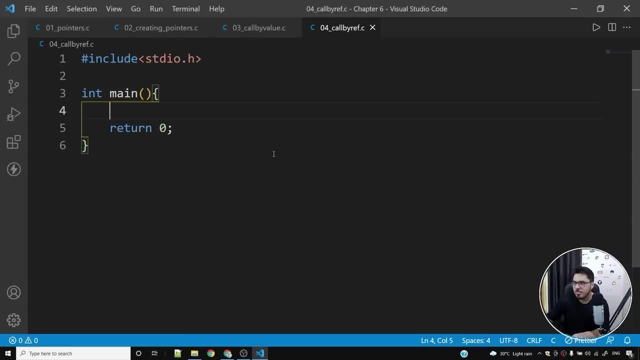 like this. i'll say call by reference, dot c, i'll put the boilerplate code and what i'll do is i'll simply copy this program and i'll paste it now in call by reference. listen to me very carefully. and then we'll go back to the notes and see what is there in the notes. instead of sending the values, we send the address. 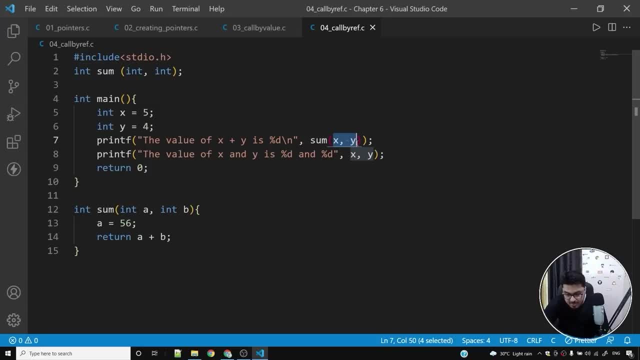 of the values. listen to me very carefully. instead of sending the values, we send the address of the values. we are going to Close this and this one. and now, if i see how complex is it here, simply now i have generated letters, so here is the word address and i am going to do, if i give it expr and 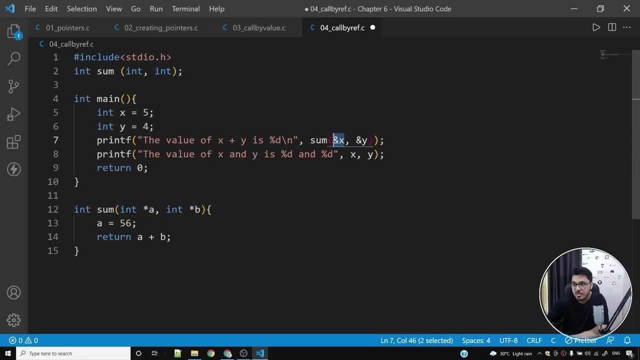 i am going to write an entire surfaces in here: inequality, which is necessary to express v in takingables, that point with v up, which is going to be v when acting on two separate borders. and if you can do this, id will make it, so i can give that to me and if i accept, 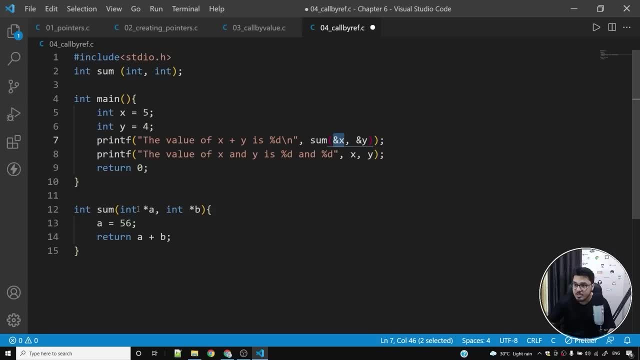 these address, then i give it what is empty. ahh, so there is a different persona, so i'm going the bit corporate address. so if i this is a b, then that will make this a. that one is that area and address will be passed into this variable, which is an integer pointer. is this valid? definitely, 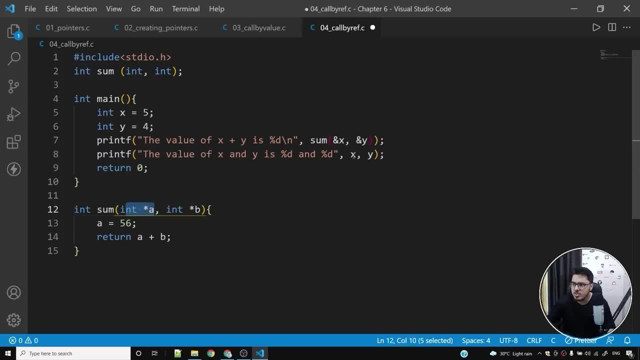 this is valid. you can definitely use this kind of syntax to pass the address of x and y variables. okay, so far, so good. so far, so good. now, in order to change the value of a, what will i do? a is an address, a is an address, so i'll decode this value. i'll say star a is equal to 56. i'll. 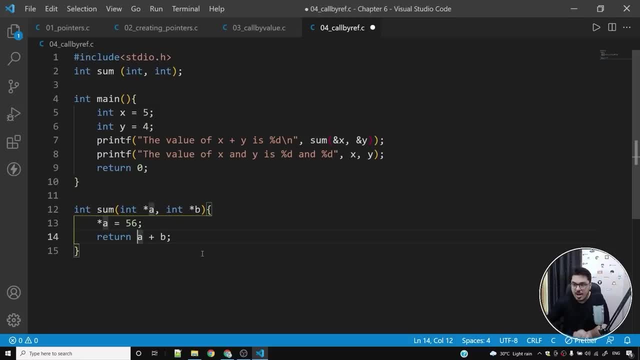 say, value at address of a is 56, and i'll simply say a value of a plus value of b. okay, now the sum function will definitely work, but my question to you is: will the value of x and y change? a very simple question in front of you, and then we'll try to see what happens and why this thing. 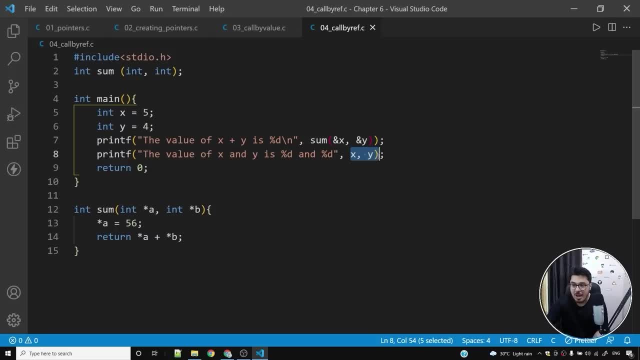 happens. okay, i want you to write down comments and tell me what will happen. will the value of x and y be changed? if you have commented, uh, well and good. if you said that it will not be changed, listen to me very carefully. you are wrong. it will be changed. the value of x and y will now be 56 and 4.. how come this function? 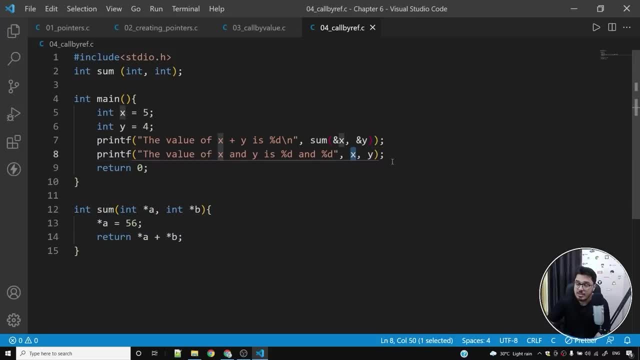 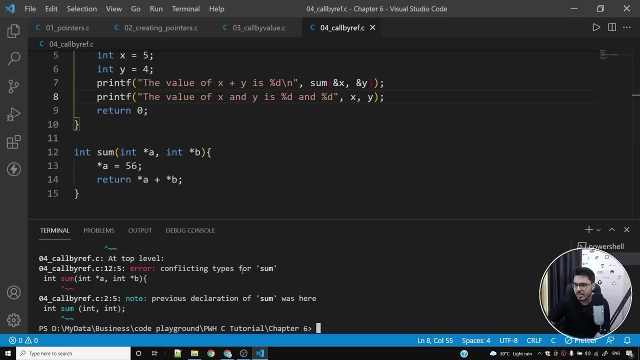 was able to change the value of x. we'll see. let me run this program for you and show you that actually the value will be changed. so it is saying conflicting types for some. okay, i'll have to say in star and start here. my bad, i'll have to pass um the. 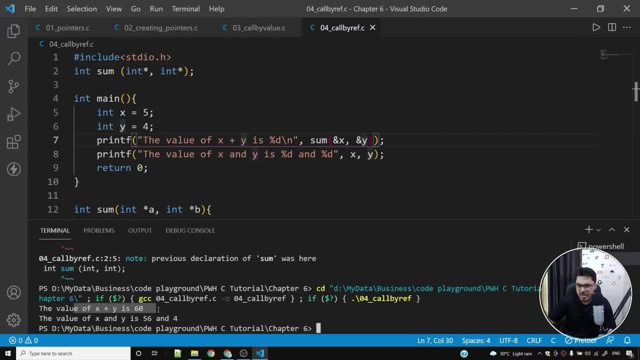 uh, pointers in the prototype and you can see: the value of x plus y is 60, and now the value of x and y is 56 and 4.. so the value of x actually changes. why does this happen? so let me try to explain this. 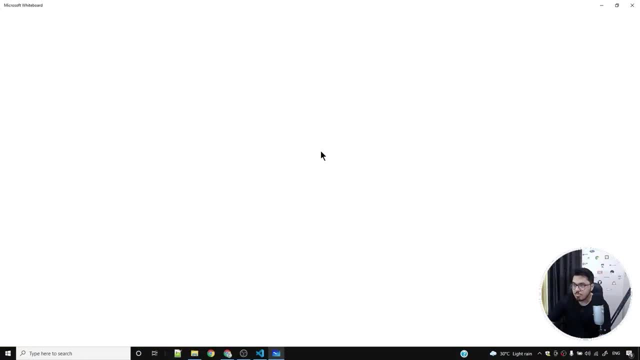 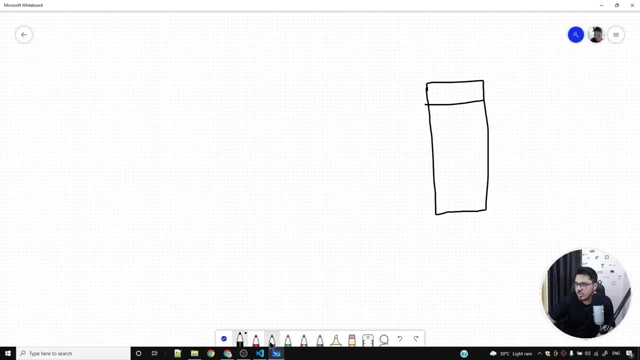 to you using a whiteboard. okay, so let me show you something. so let us say: this is the main memory of my computer, this is the main memory of my computer. and let us say: this red region, this red region is variable x, so this region contains variable x. okay, and let us say this: 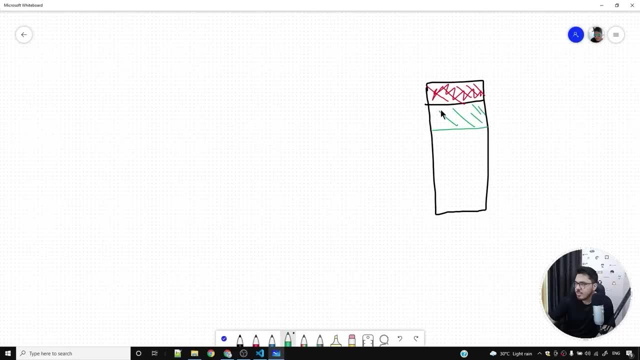 green region. this contains variable y. okay, now let us say the address of this is one. i'm just assuming address to be one. for simplicity it's not going to look like this, but let's assume the address is one here and address is two for this one. so the address of 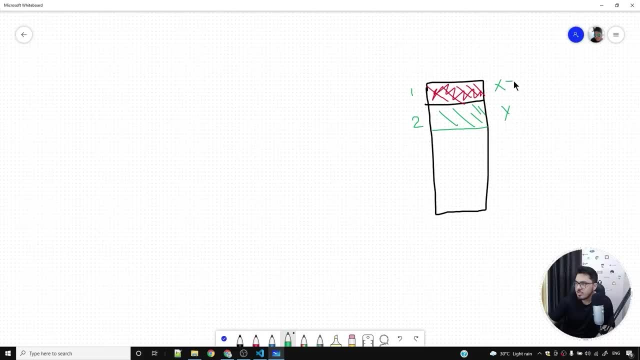 x is one address of y is one and the value of x is what it was. uh, let me check: five and y was four, so this was five and this was four. now what happens is if i pass these addresses, if i say one and two, let's say take one and two- and somebody says that change the value at one, change the value at two. 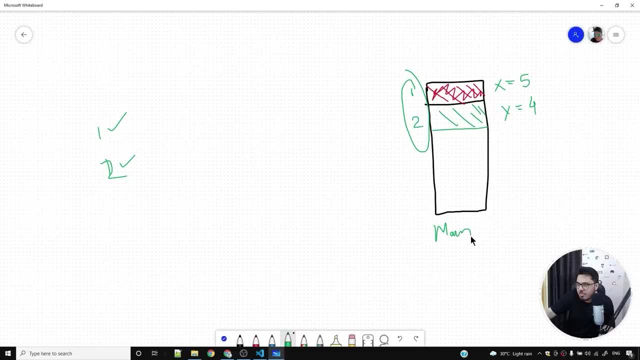 this is my main memory. i have one main memory. i have the main memory of my computer. if somebody goes to that main memory and changes the variables, it will be reflected everywhere, and this is what happens in call by reference, instead of copying the value. when i'm using call by value, i'm simply 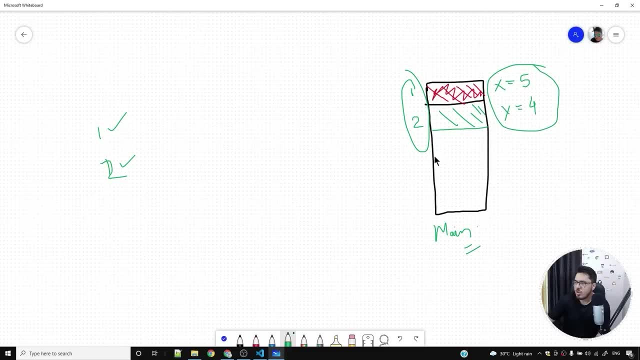 copying these values. i'm saying: whatever is there in five and four, copy it in a and b. so i'm simply saying i have change the value of value in matches에요 these values. i'm just hopefully we can use this, this again, because we're only going to change the values in four and say actually: 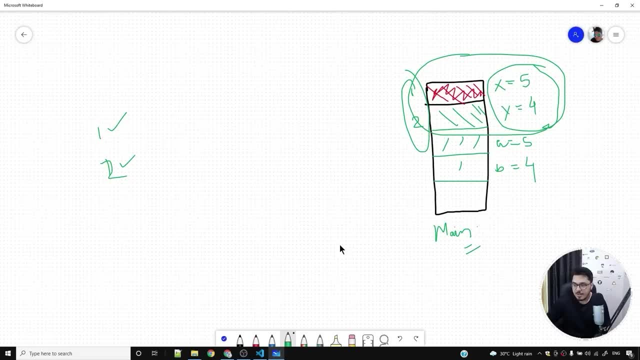 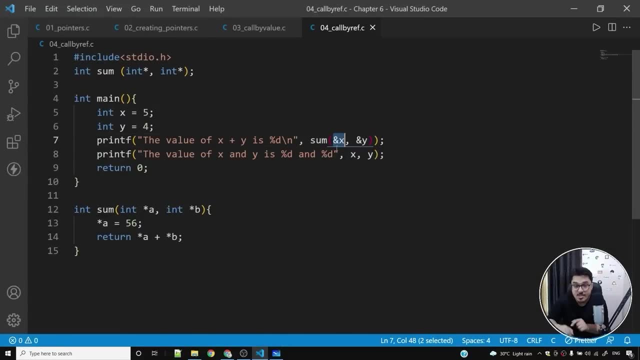 we will also be five, b will also be four. and now, if you change these values, these values, these x and y, will will be unchanged. but in call by reference, what we are doing is we are actually taking the address of this variable itself and we are decoding this address and saying that the value 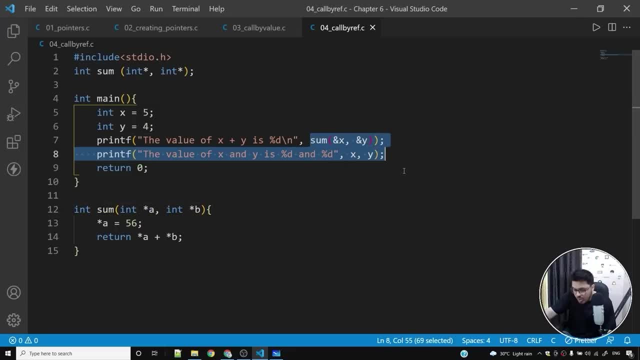 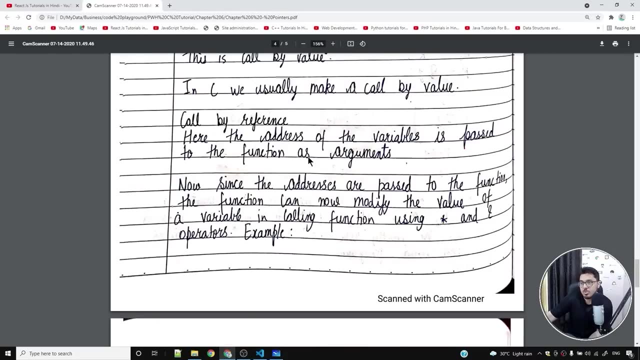 at this address must be changed, and when we are doing something like that, the value of x and y. now let's come back to notes and try to understand this even further. so call by reference: here the address of the variables is passed to the function as argument. so arguments. 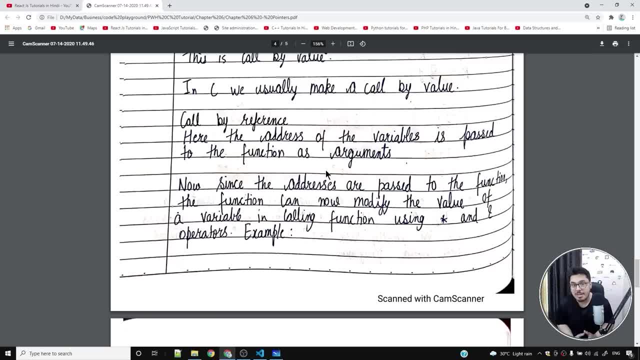 are passed. before we were passing the values, but now we are passing the address, and now that we have the address we can alter the value at that address. and value at a given address will be reflected everywhere because that is the physical value of that variable. okay, so when you say value, 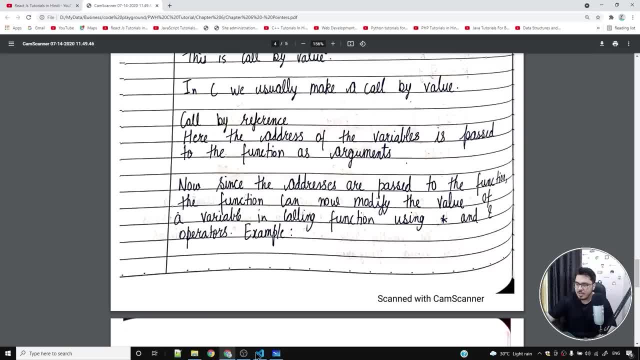 at this address. it has to be changed because we are taking the address of variable x in main memory and we are changing the value at that address now, since the addresses are passed to the function, the function can now modify the value of a variable in calling function using: 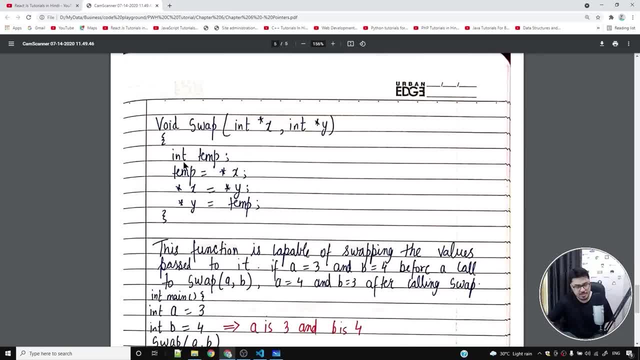 asterisks and ampersand operators. i've given an example here. i've shown you how this works and this function is capable of swapping values passed to it, and this is a typical function using pointers, which is used to swap two variables. so let me show you this. 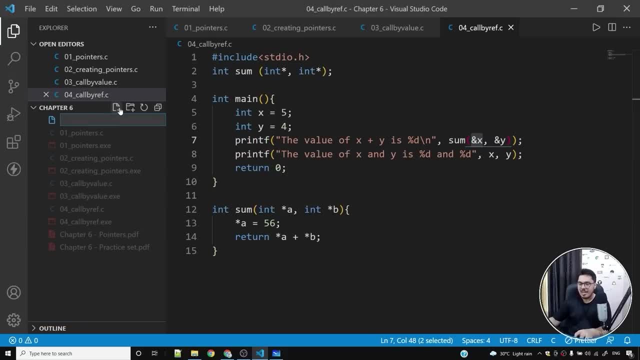 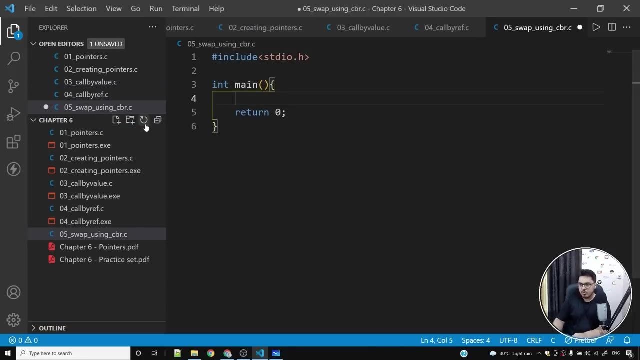 logic and this will definitely help you understand call by reference more clearly. so i'll say: swap using call by reference. so i'm saying swap using cbr. cbr means call by reference, remember this, okay. so i'll put a boilerplate code here and i'll simply say: void swap. and swap will simply put the value of x into y and y into x. let's 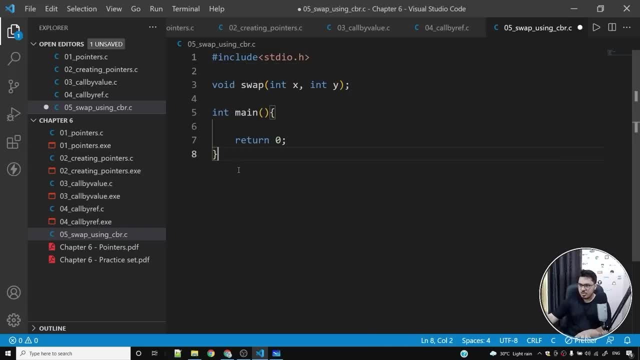 see how and i'll define my function somewhere here. and also, i don't need x and y here. this is a prototype. i don't need x and y, so i'll simply do this now. i'll simply say: int a is equal to 5 and b. 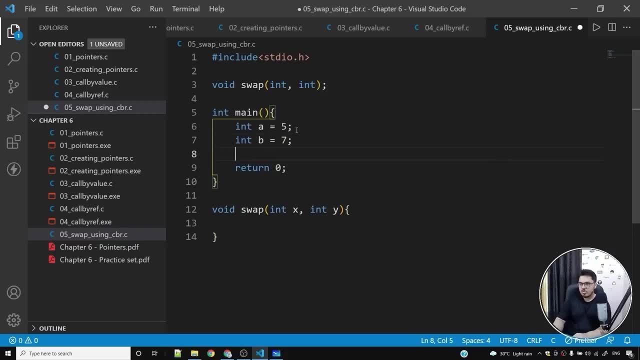 is equal to 7 values. sorry printf. i'll say value of a and b. before swap they were percentage d and percentage d and i'll simply say a comma b, and then i'll do the same thing after the swap. what happens after the swap? so let me put backslash n here and i'll simply run swap. i'll say swap a comma b. so let's. 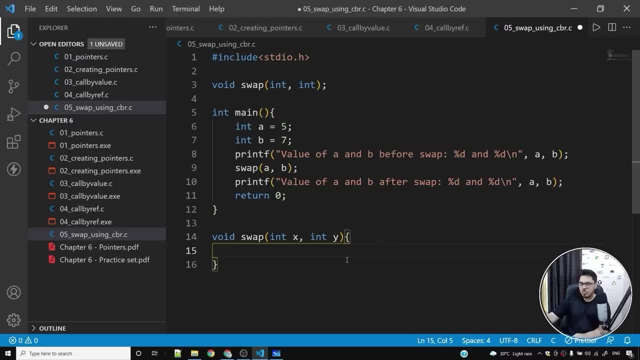 run the] here and then i'll say: only at that time i'll say whatever is required, and then i'll just use the same things. i'll just give a white shirt and change this result to that regard instead of just leaving it as it is. um, it just changes my story straight away. so can we смож? 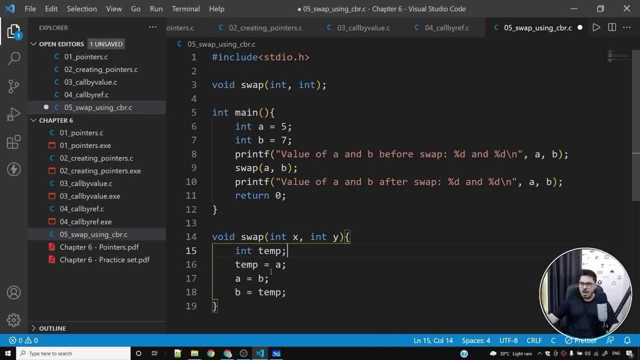 This is just going to be a simple scenario. when i say swap a and b, what i can do is there is a very bel simple sentence logic. let me tell you. i'll simply create a temporary variable. i'll say the value at and store the value of a. so at this line the value of a is equal to five, the value of temp. 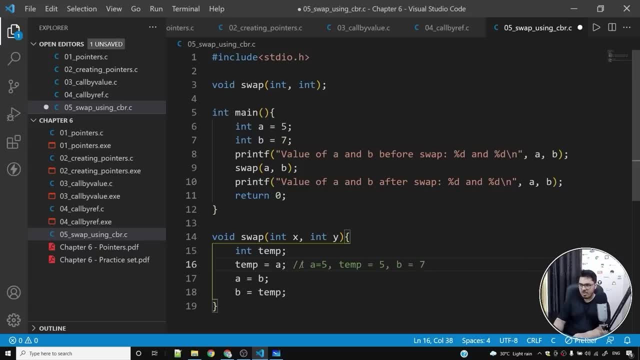 is equal to five and the value of b is equal to seven. okay, so i'm going to do the dry run of this program for you now. when i say a is equal to b, basically i'm assigning the value of b into a, so the value of a is seven, temp is five and b is seven. at this line, now, the moment, the control 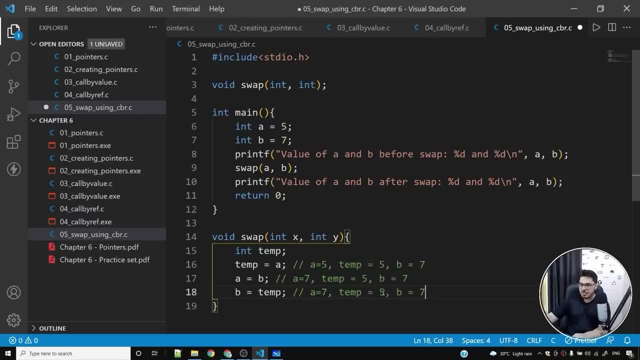 comes to this line, the line number 18, i'm saying b is equal to temp. so what is there in the temp will come into b and you can see the value of b is five. now. so, using this, what i've done is the a was five, b was seven. i made a as seven, b as five. so this is a typical logic to swap two integers. 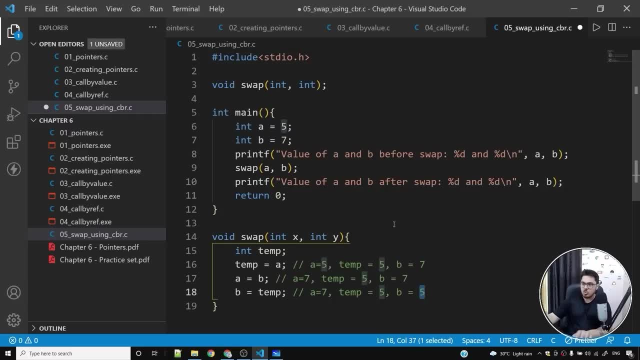 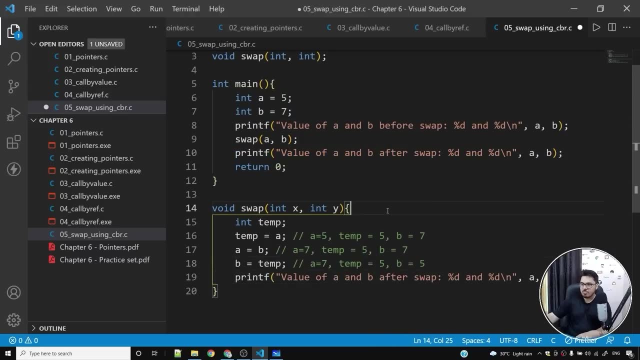 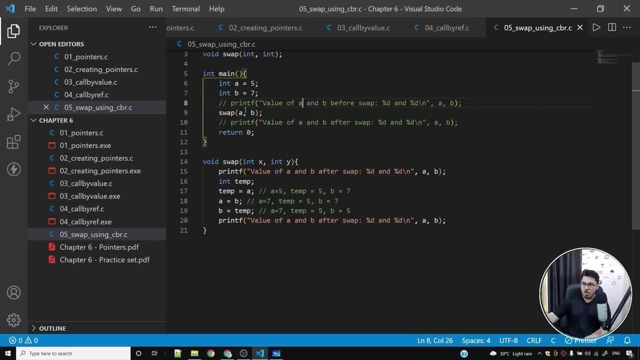 but there is a catch here. there is a catch here. let me show you what that catch is. let me print these values right after this function runs and right before this function runs. so when i talk about this function inside this function, i'll be able to swap. so let me show you. i'll comment these two lines. i'm simply running swap. 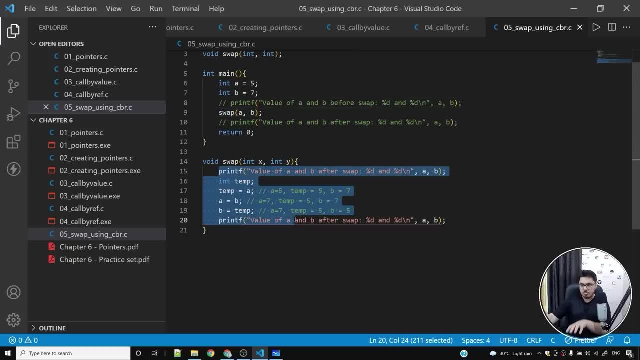 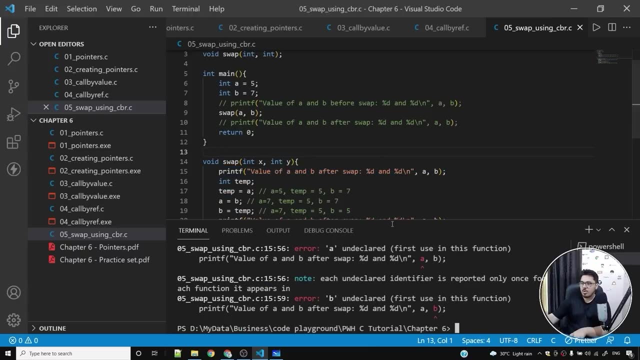 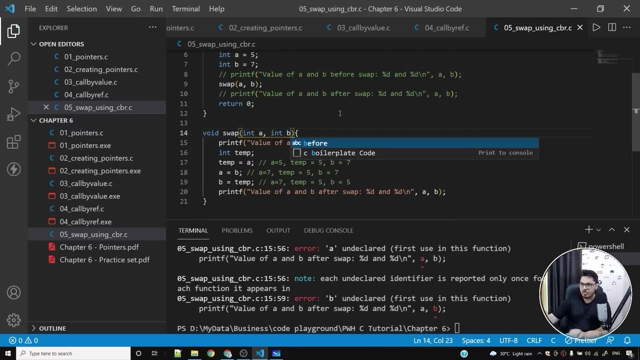 a, comma b, and i'm trying to swap it inside the function. so when i look at these two variables from inside this function, the variables will be swapped. let me show you. um, it says b is undeclared. let me see: okay, so i need to use a and b here. i wrote x and y. 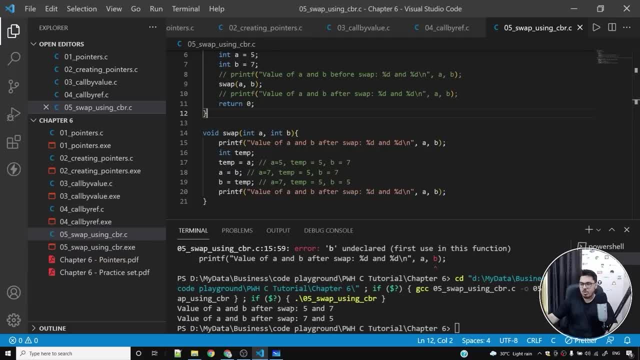 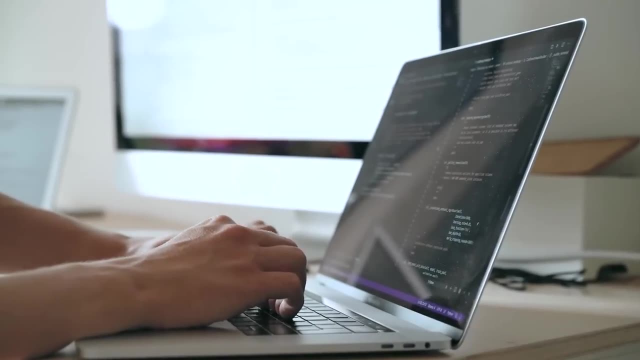 um, okay, now it should work. so the value of a and b before the swap, uh, okay, before the swap. before the swap will be uh, five and seven, and after the swap it will be seven and five. okay, so when i look at these two variables from inside the function, i was able to swap the values. 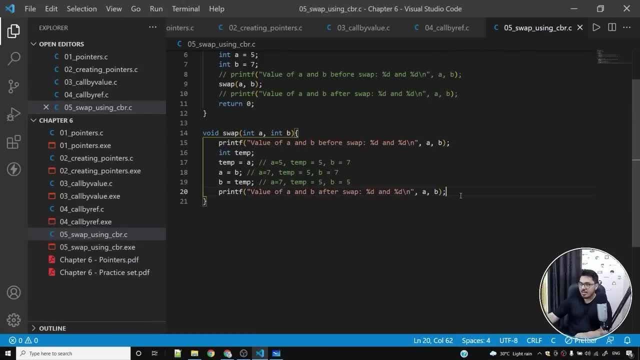 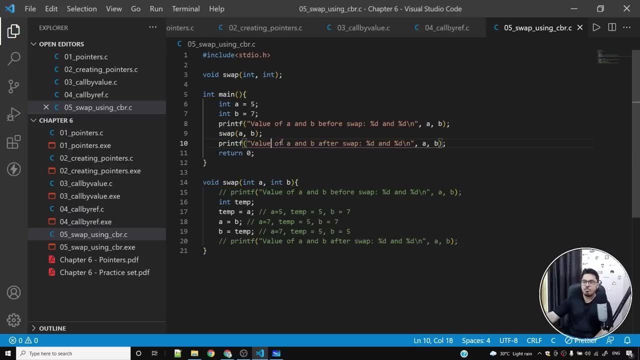 but what will happen if i look at these two values from from the main function? in the main function, the value of a and b will remain unchanged because we are passing the values of a and b by value. when we pass by value a copy of these two, 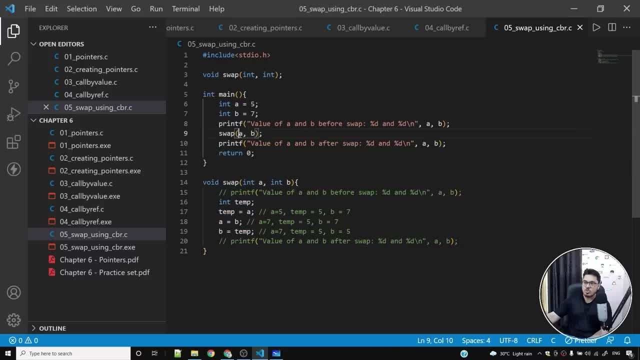 variables will be made inside this function and the values of a and b inside the main function will remain unchanged. also note that i have used a and b in the main function as well, and i have used the same nomenclature of these variables in the swap function as well, and it's totally okay. 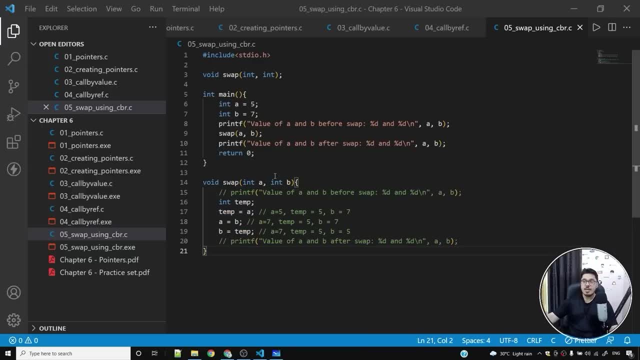 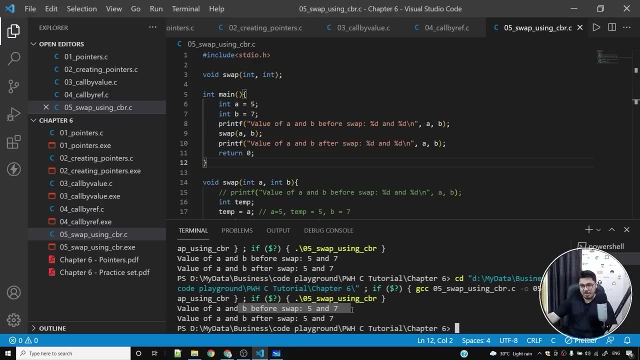 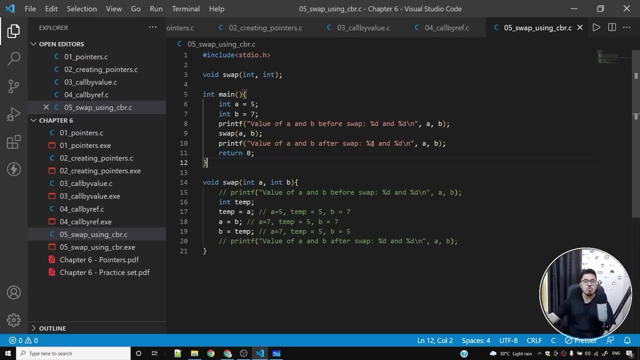 to do that. swap will maintain a separate copy of a and b and main will maintain a separate copy of a and b. so if i run this program you can see the value of a and b before swap five and seven. after swap five and seven it doesn't swap the values a and b. so what to do if i want to swap? 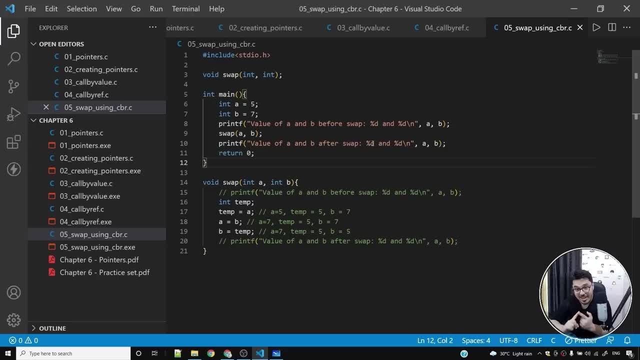 the values a and b in the main function, i will have to pass the addresses of a and b, addresses of these two variables. literally i'll have to pass address of this particular variable and then i'll have to pass address of this particular variable. and then what will happen? 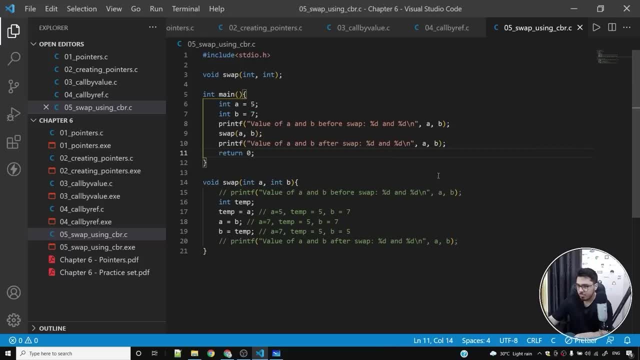 is i'll be able to change these two variables. let me show you, you let me show you how this can be done. okay, so what i'll do is i'll accept pointers inside my swap function and i'll simply say: in star a, in star b. so a and b are now addresses, now that a 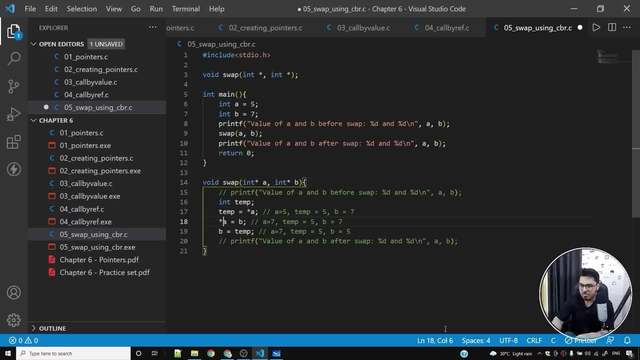 and b are addresses, i'll have to use the values by using the s tricks operator, which is nothing but value at address operator. so value at this particular address will be star a. value of b will be star b. value of uh, this particular will be uh. let let me call it a ptr so that you are easily able to understand. 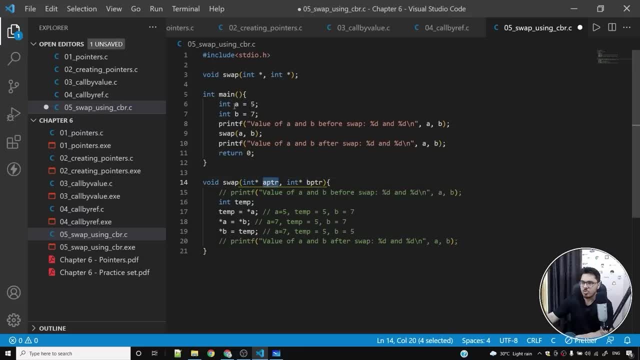 that this particular a, ptr, is the pointer to this a. okay, it'll be easy for you. you can name the variables whatever you want, but i'm just trying to make things easy for you to understand, so i'll also make it b, ptr, b, ptr. and let me show you that this changes the values um a and b to b and a. 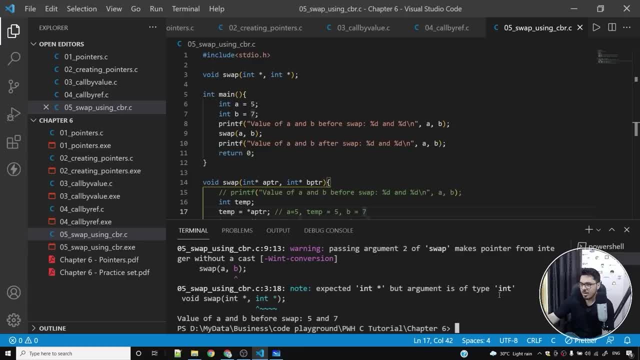 so i've said in star, it said in star, but argument is of type int, uh, in star, bbtr. okay, so i'll have to say ampersand a, ampersand b. i'll have to pass the addresses of a and b, and now this will swap. 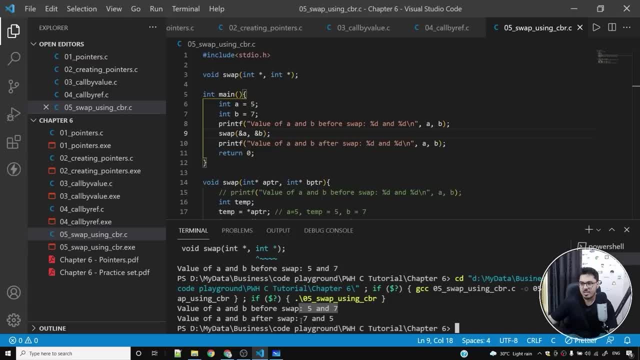 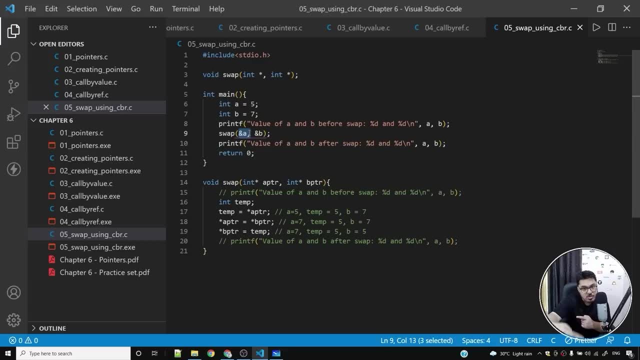 the values. no surprises whatsoever. so five and seven, seven and five. okay why? why did this happen? because we passed the address of the variable. so when we pass the address of the variable, what happens is we can find the value of that variable using star operator, so this particular a can be. 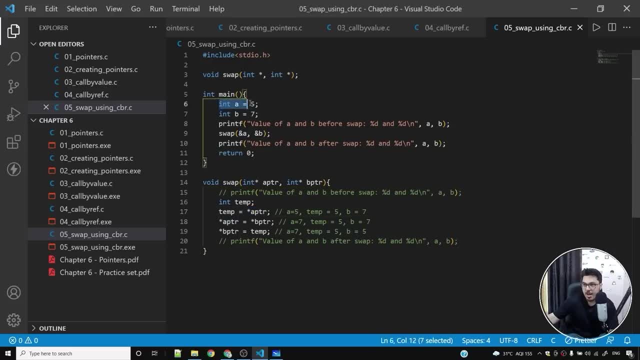 called by using star aptr. this address is passed to swap and not the exact value is copied to swap. previously we were copying the value of a to swap. now we are copying the address. but when we use asterix operator, asterix at that address will literally be this variable and it will be changed. 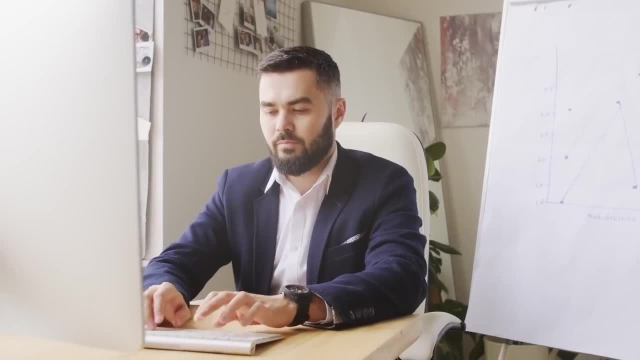 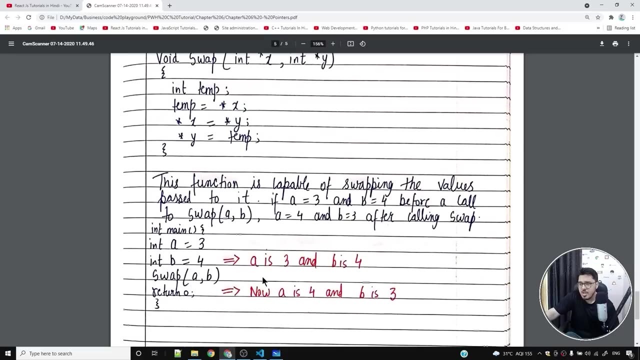 okay, so this is how call by reference works. i hope that you are able to understand how call by reference works and how these things are used in c programming language. so, if i come back to the notes, i have written the same thing. function is capable of swapping the values passed to it. because we are now using 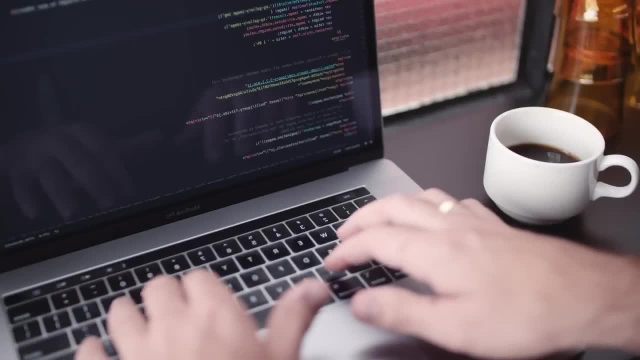 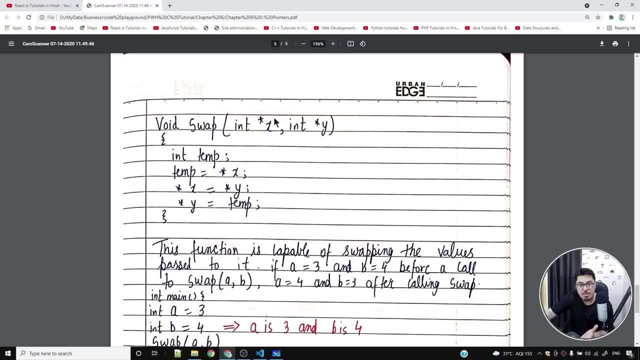 pointers. we are now using the addresses and we are decoding those addresses to find the value at those addresses and we are altering those values at that address, so we are literally able to change the variables of the main function. so i hope that you were able to understand all this. 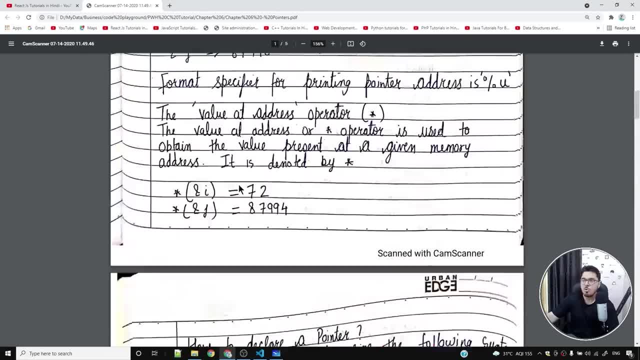 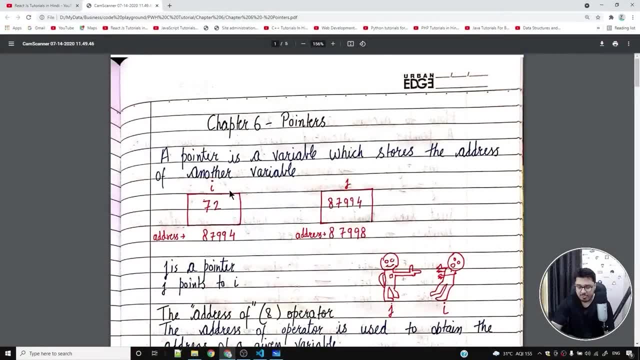 this finishes the chapter number six. i hope you had fun. this was one of the most important chapters of the c programming language. i hope that you were able to understand and even if you have to- you know- watch this chapter more than once. feel free to do that. it's worth it. watch it once more and make sure you. 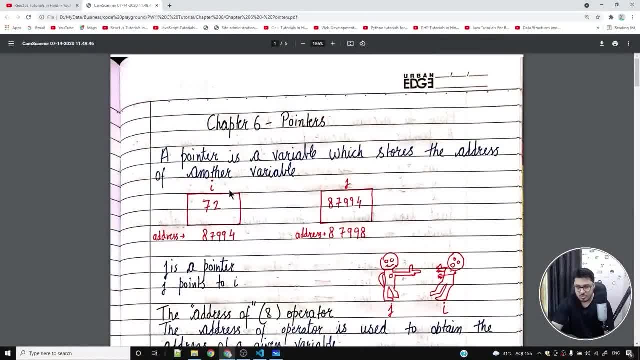 read the notes more than once, because these are the concepts that will definitely see. these concepts are famous for being difficult, but actually they are not difficult because if you understood all the things that i taught you, all the things that i told you, all the concepts of amp as an operator star, 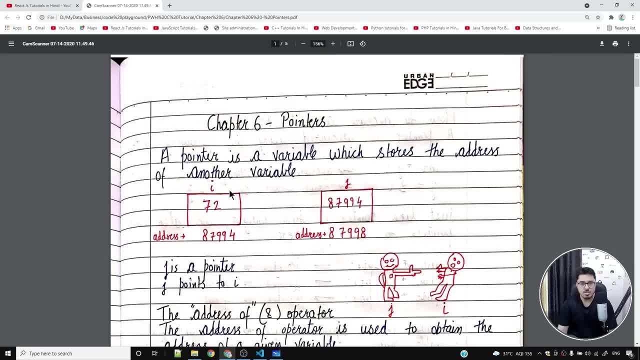 operator you'll be able to understand. it's not like this is something that that is difficult for people to understand. it's just that it takes time if you don't have the right resource. but i hope that i was able to explain this to you pretty well, so we'll now move on to chapter six, practice set. 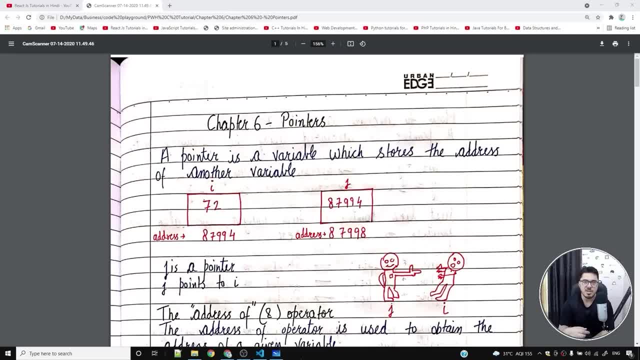 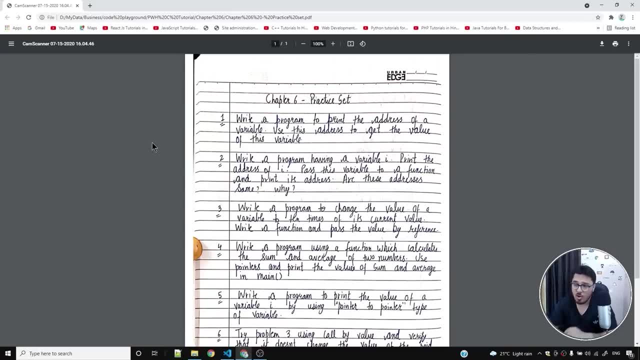 and solve some questions. let's move on to chapter six, practice set now. all right, so now that we have some concept of pointers and we have some concepts of pointers and we have some concepts of pointers in our head, let's try to solve some of the questions on pointers. so the very first problem. 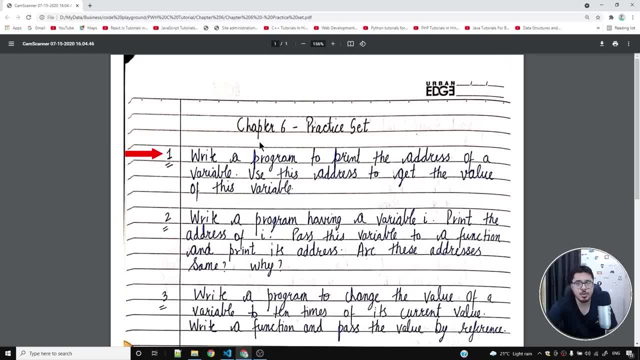 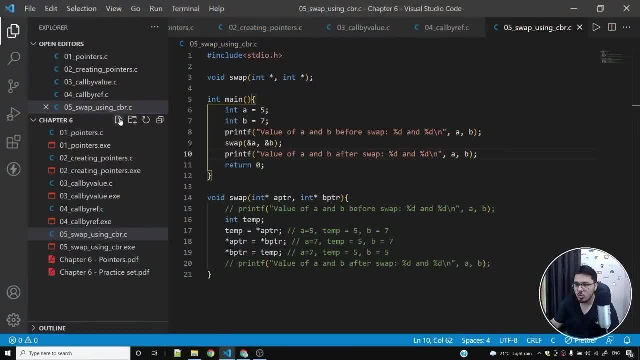 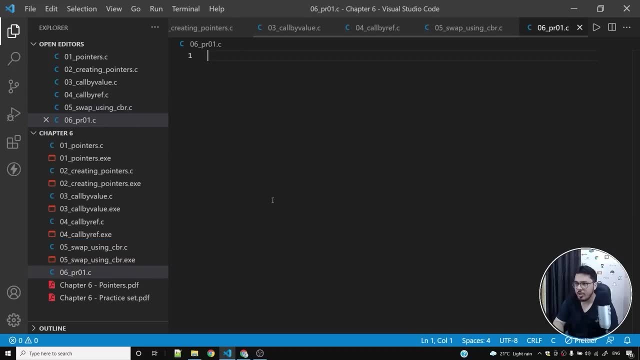 of this. chapter 6 practice set says that write a program to print the address of a variable. use this address to get the value of that variable. so this is a pretty simple program. let me show you and let me code this for you. so i'll simply say pr01.c. i'll put in the boilerplate code. 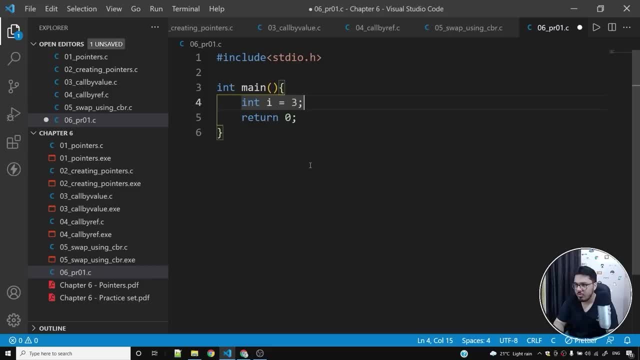 and what i'll do is i'll simply say int i is equal to 3, and what i'll do is i'll simply use printf, and then i'll simply use the address of i is, and i'll use percentage u and i'll say ampersand i, because we know that the ampersand operator is going to give us the. 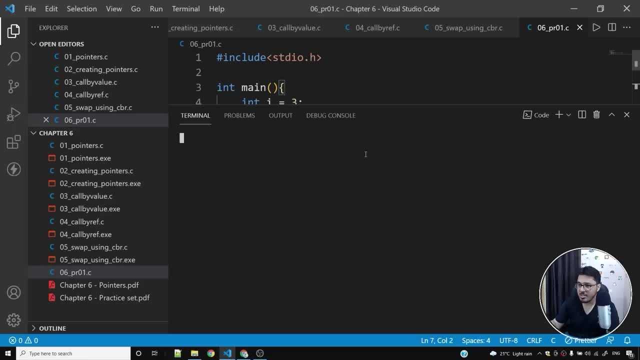 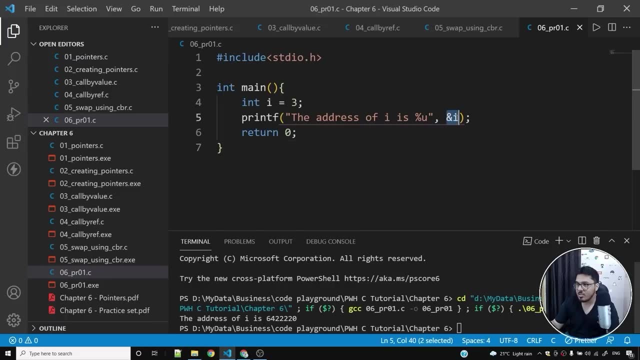 address of i. okay, so let's try to run this so this prints the address of i as this. so now that we have the address of i, we can actually find the value of i. so i can say: value of i is d, and what i can do is i can simply say star ampersand i, and what this will do is: 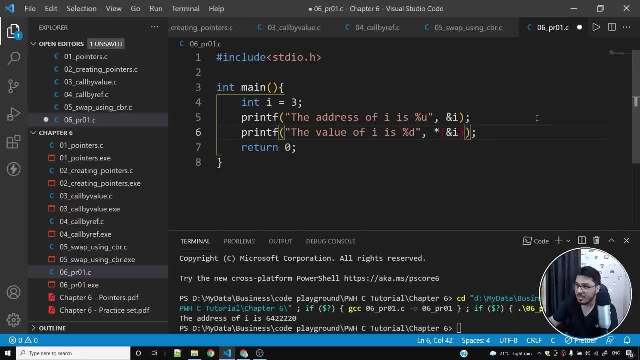 it will find out the value at address, ampersand i, which is value at the address of i, which is nothing but the value of i. so it's going to print 3, which is why i have used a percentage d here. so i'll save this program, i'll run this program and you can see the value of 5. 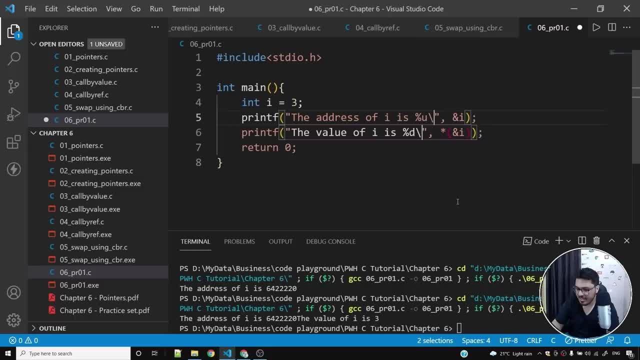 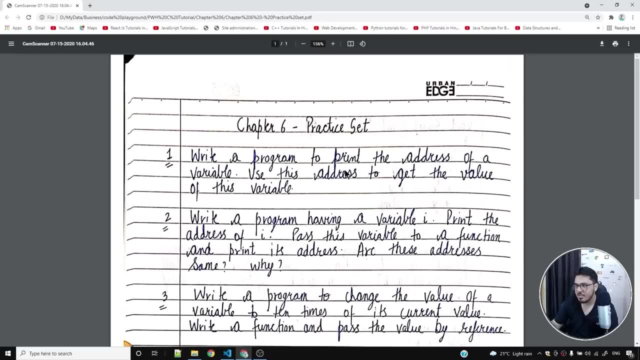 is three, and also just to format our programs nicely. what we'll do is we'll use these backslash n's and let me come back to the practice set. so this problem is done. pretty straightforward, simple problem: write a program to print the address of a variable. we printed the address. 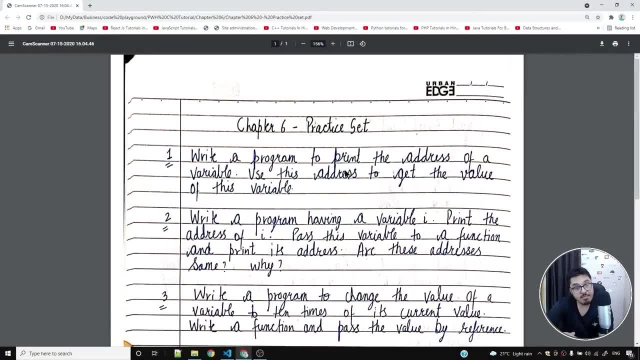 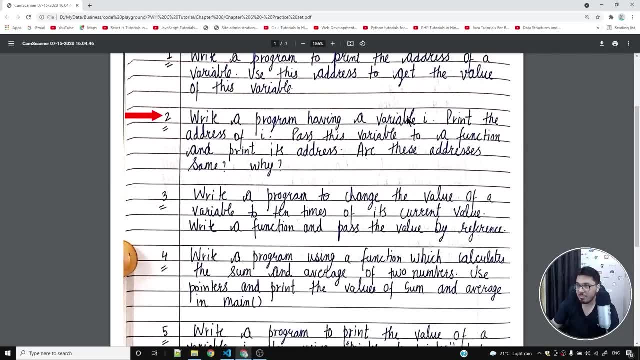 of the variable. we also used this address to get the value of this variable using the asterisk operator. let's look into the question number two. write a program having a variable i. so this program is going to have a variable i and we'll print the address of i. now we're going to pass. 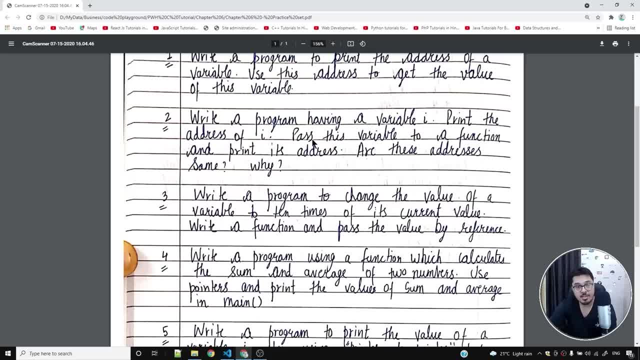 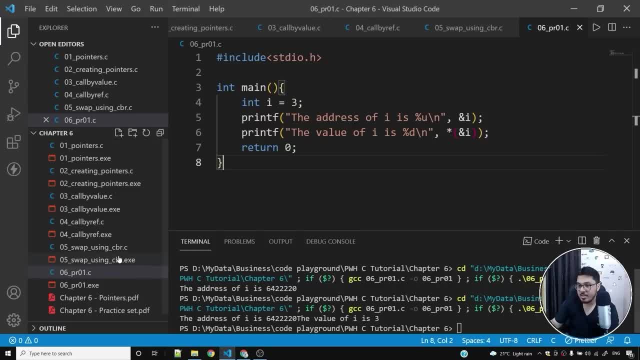 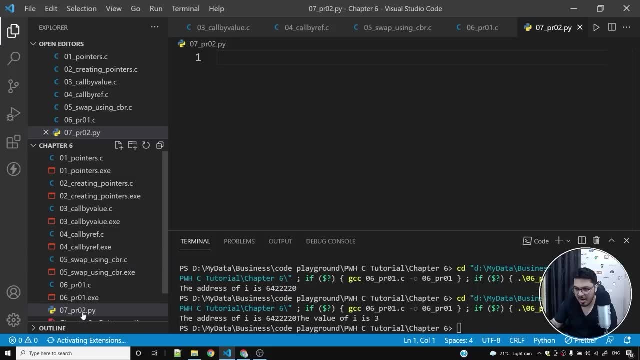 this variable to a function and print its address. are these addresses same? why so? let's see, uh, what this problem is asking us to do. so i'll say 0, 7, underscore pr 0, 2, dot py. uh, oops, i, i meant c, not. 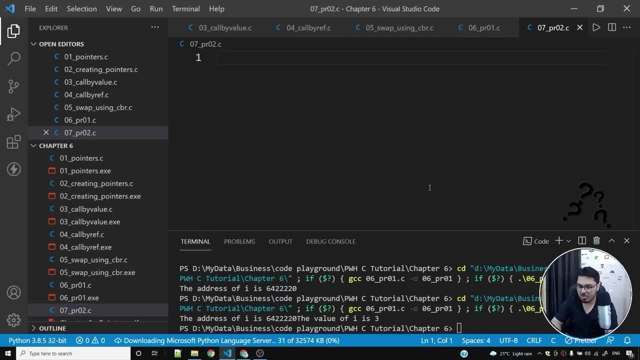 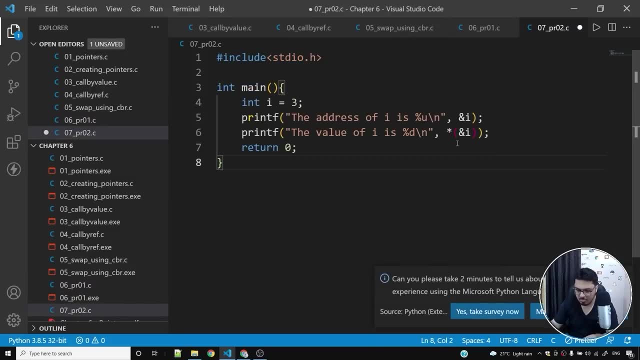 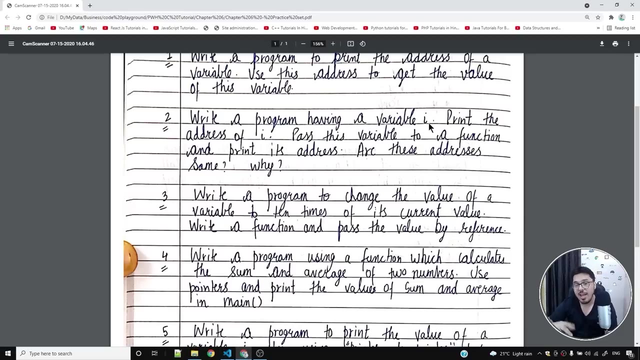 py. so this is c programming course, not python programming course. my bad c boilerplate code. uh and um, what i'll do is i'll start this template, i'll use this template to start with, and what i'll do is this: question said: write a program having variable i. we already had variable, which is why. 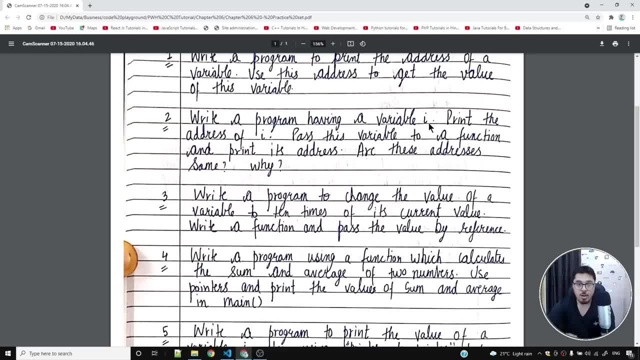 i used that program for this question as well. now, print the address of i. so we are printing the address of i. yes, we are doing that, indeed, so this part is done. now we have to pass this variable to a function and print its address. so, in order to pass this to a function, 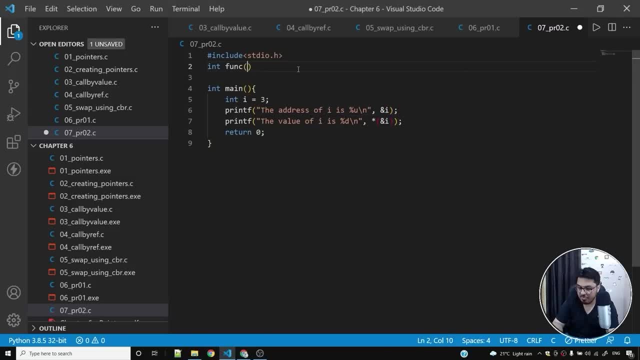 what we'll do is we'll create that function, we'll say func and then we'll say int star. so func is a function which returns an integer and it takes a pointer. so i'll say int star, ptr. and i'm not sure about the return value of this func. but for now i've written func. sorry, int, but 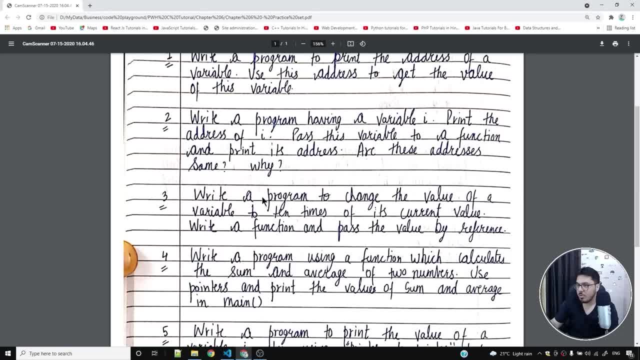 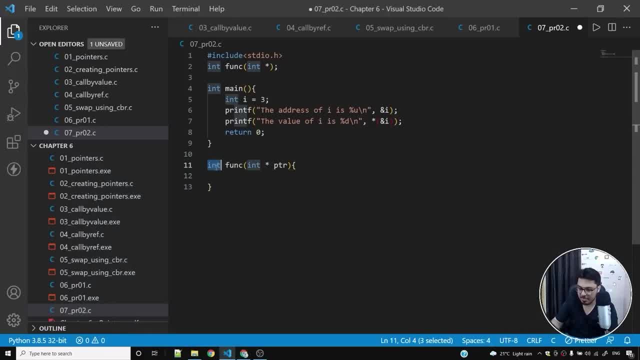 i'll change it if need be. so what i'll do is: i'll see what this function says. so we have to print its address in the functions. so let me do one thing. let me change this to void, because i don't want to return anything back from. 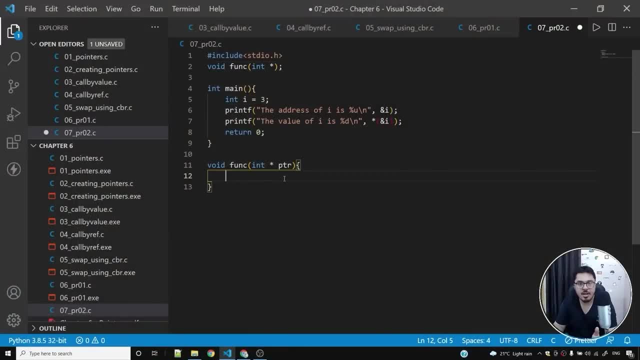 this function. so what this function says is simply print the address ptr. so i'll simply say the value of address ptr from function func is, i'll say percentage u and i'll simply print ptr. and, as part of the best practice, what i'll do is, uh, i'll use back. 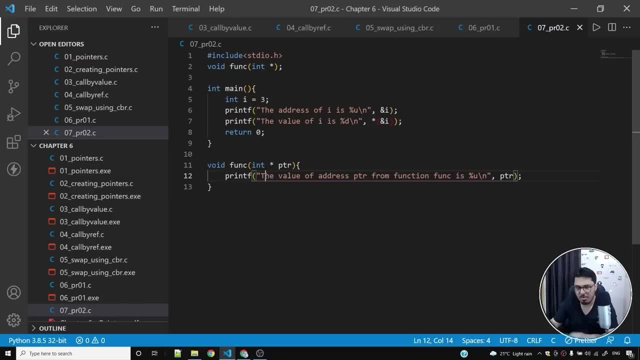 ptr n at the end of the line, so that all the things are formatted very nicely with the new lines printed. so we are passing the address to a function. so let me call this function and let me give ampersand i to this function. so this function takes the address of i and it simply prints that. 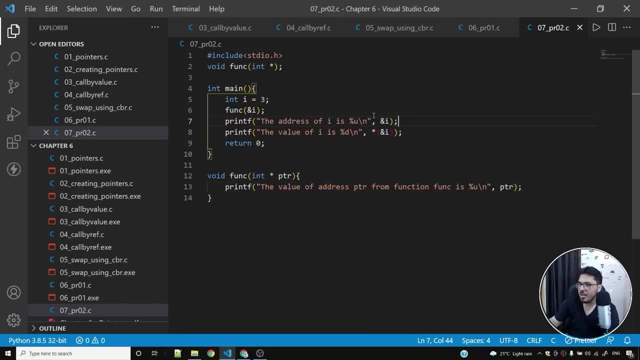 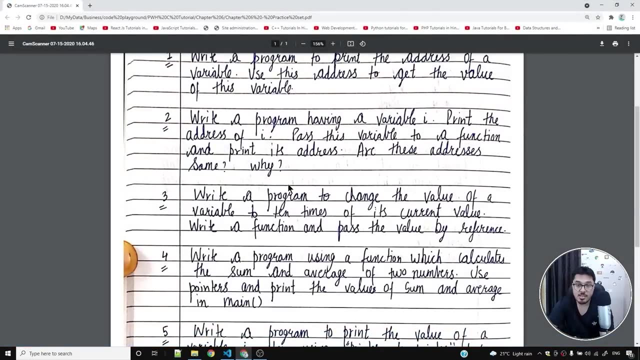 address of. i just like this. okay, let's see what it prints. so the question says that: will the address printed by the function and the address which is printed by the main be the same? will it be the same? so are these addresses same? which addresses we have to pass? we have to print the address of. 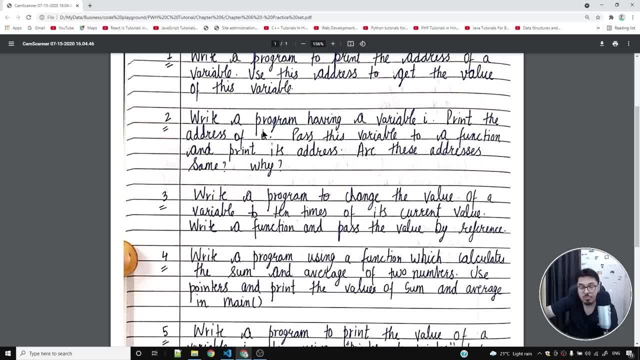 i in the main function and then we have to pass the address of i to the func and we'll have to print that address inside the func to see whether the addresses will be same or not. do you want to guess whether the addresses will be same or not? i want you guys to guess in the comments. uh, leave. 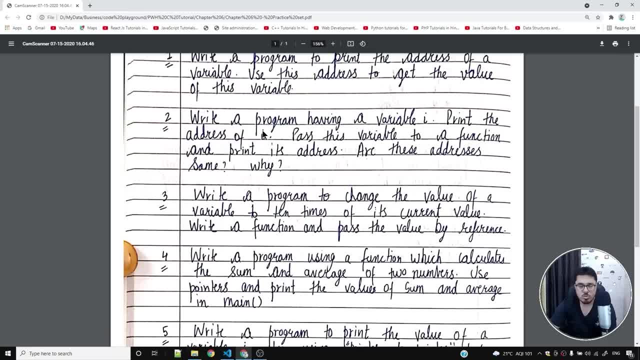 a comment and let me know which question you are answering in which comment and post your answer. i want all of you to post your answers and i'll wait for um for you all to you know, post your comment. i hope everybody posted the comment. so the answer is yes, these addresses are going to be the same. 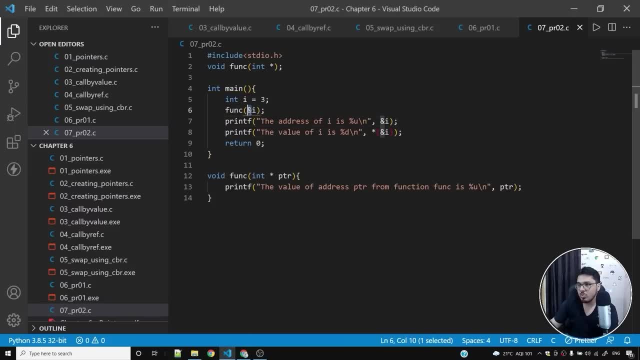 because this value, and the value we are passing to this function, is the address of i, is the address of this particular variable in the main memory, which is going to be the same. so let me run this program for you and show you that these addresses are going to be the same. 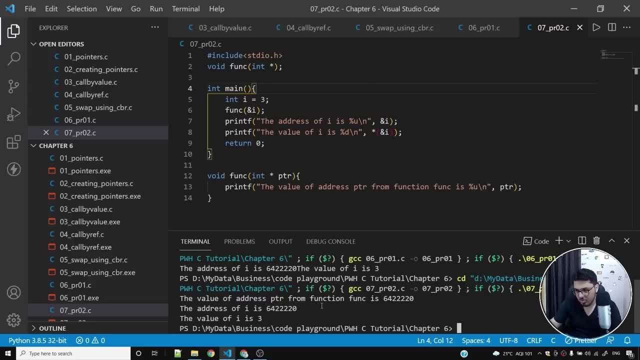 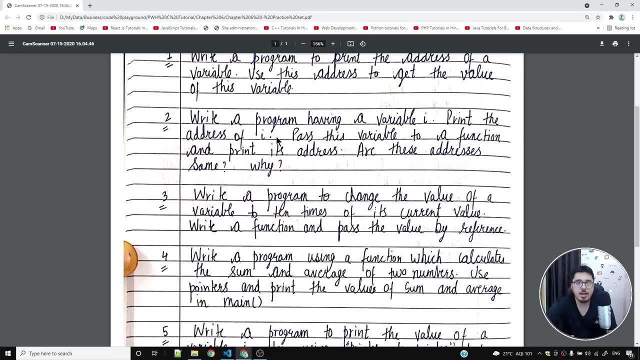 so this value and this value is going to be the same. so this is the value which we printed from the function and this is the value which we printed from our main. so this is how this question was structured. this is what it wanted: to tell you that the address of i is going to be the same. 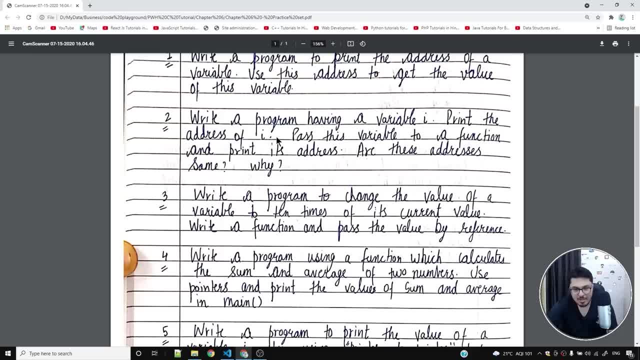 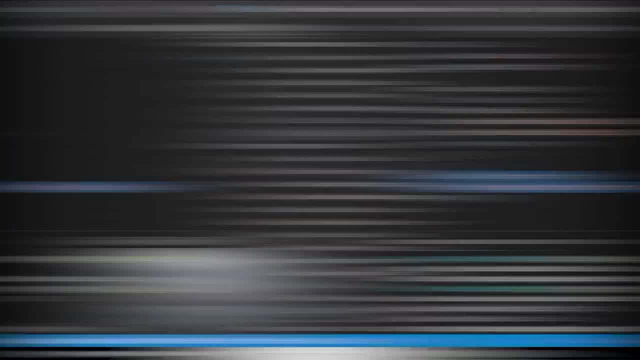 in the function as well as in the main. in fact, main is also the function. when i say function, i mean this func function, the function that we created, that user defined function that we created. coming back to the practice set, the third question says that write a program to change the value of. 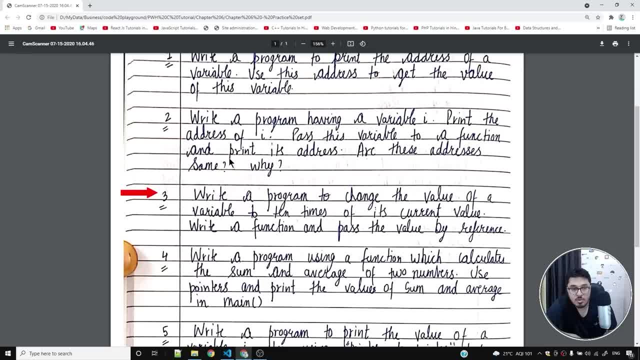 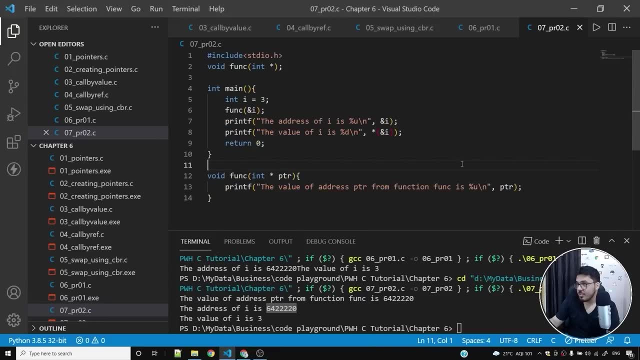 a variable to 10 times of its current value. you write a function and pass the value by reference. so this problem says that: create a function, pass the address of a variable to that function and change its value. so let's start from this function itself. let me create the eighth program. i'll say: 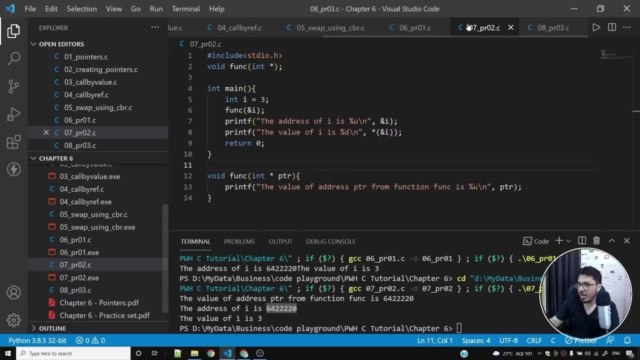 0, 8 underscore: pr 0, 3, dot c. and what i'm going to do is i'm going to create a function which is going to change the value of a variable to 10 times of its current value. so what i'll do is i'll. 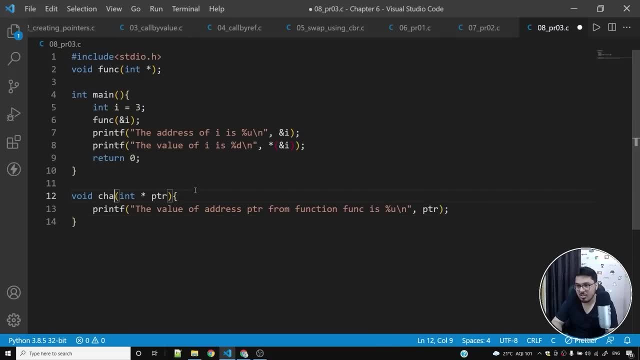 copy this particular program and i'll start from here now. i'll rename my func as change because it better reflects what this function is doing. so i'm simply saying void change in star and inside this function what i'm doing is i'll simply say: value at this address is equal to. 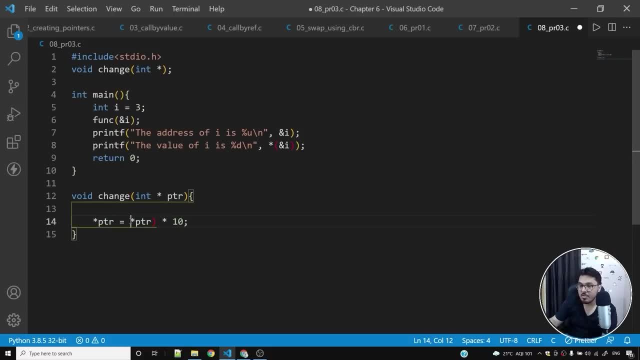 value at this address multiply by 10, because we have to change the value of this function to 10 times the value of uh of the variable. okay, so let me run this function so i'll say the value of i. let me remove this. i'll say value of i before uh change ran is and i'll say after change then is. 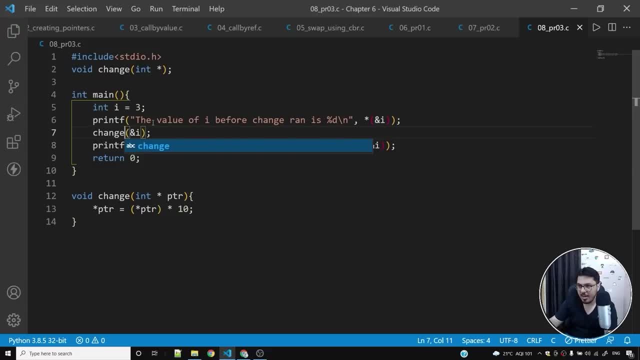 and let me also call change with the address of i, and let me not use this fancy syntax, let me straight forward say i. so i'll simply say i. i don't want to use this fancy syntax star of asterix of i, which is going to be the same as i, but i just want to use this clean syntax i. so let's see if the 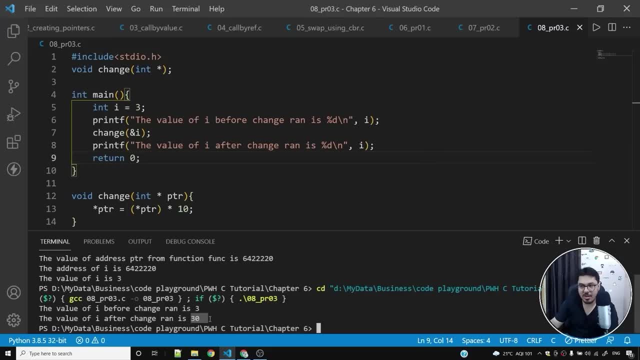 value changes. so the value was 3 and it is now 10 times of 3, which is 30.. what if the value is 6? it should be 60 after the function change runs. yes, it is 60.. let's see if this works for some. 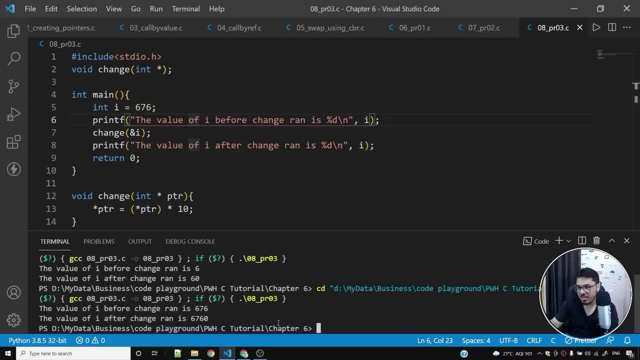 larger value like 676? yes, it does. let's see if it works for zero. yes, it should, and it will, because 10 times of 0 is 0.. what is 10 times of 30? it's 300. so we should get 300 and we are getting 300. 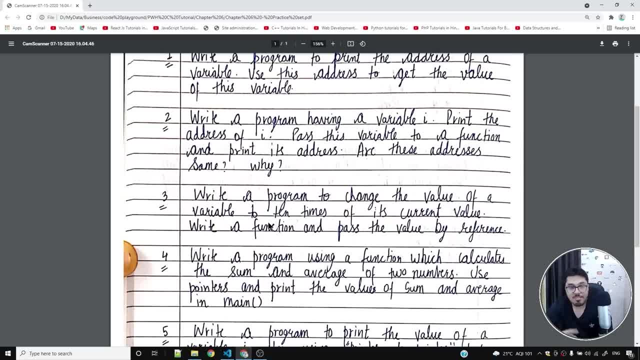 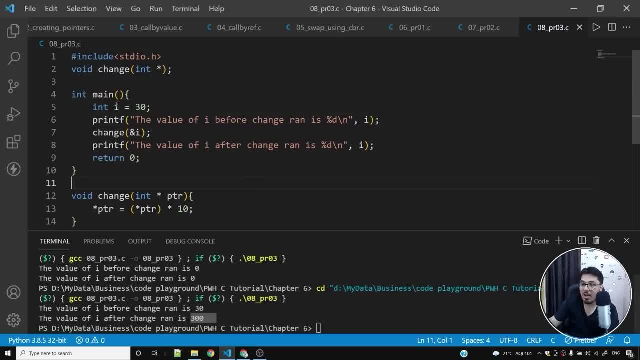 so this is how we can pass by reference to a function and change the value uh of a variable inside that function without actually having to have that variable inside this function. so did you notice one thing? this is the value of the variable inside this function. so let's see. 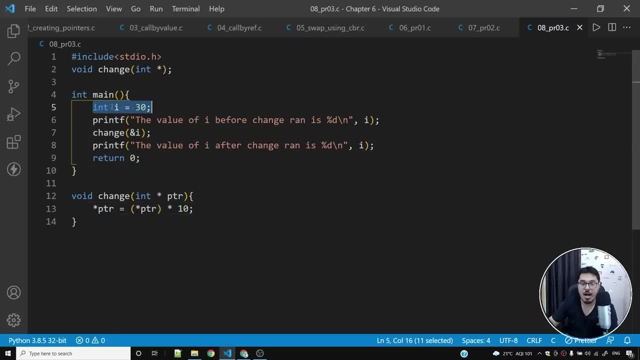 this. i was inside the main function, this variable. i was inside the main function, but it was changed by a function which is totally different from main how using the addresses. so if you get the address of a variable, you can even change it from some other function. so this is what this problem teaches. 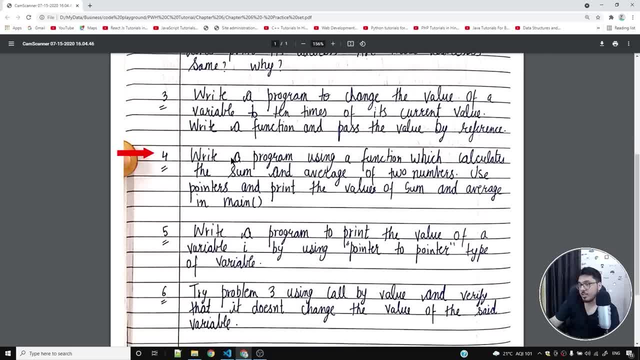 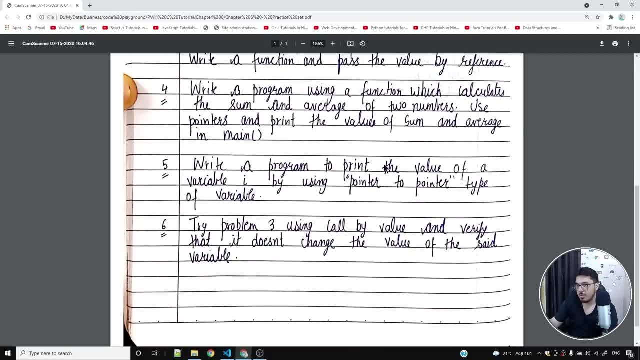 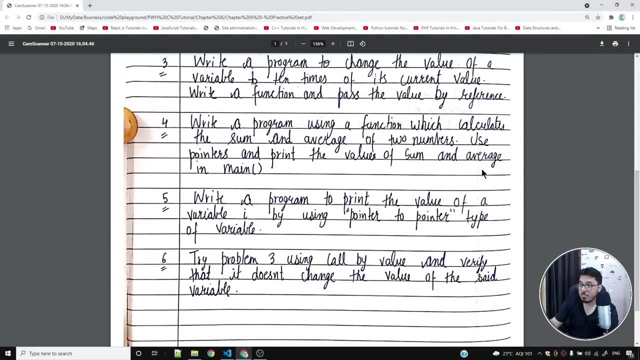 you coming back to the practice set and question number four says: write a program using function which calculates the sum and average of two numbers. so you have to create a function which calculates sum and average of two numbers, use pointers and print the values of sum and average. 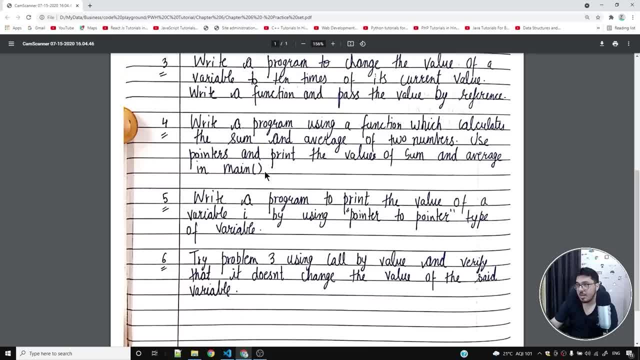 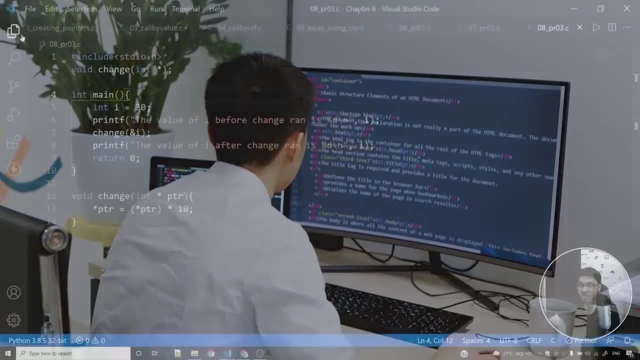 in main. so this program says that you have to use pointers and you have to print the values of sum and address of two numbers. so we have to use pointers and then we'll have to print the value of sum and average in main. so this is a very interesting problem and i want you to pay attention. 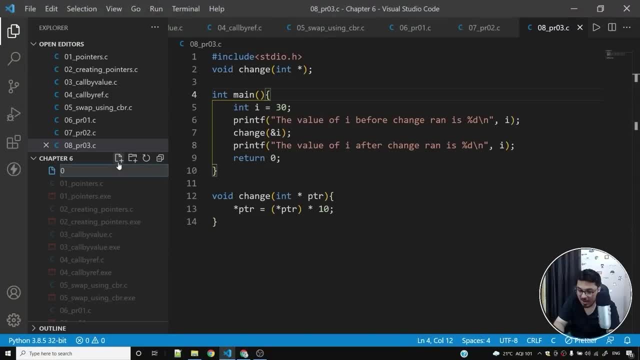 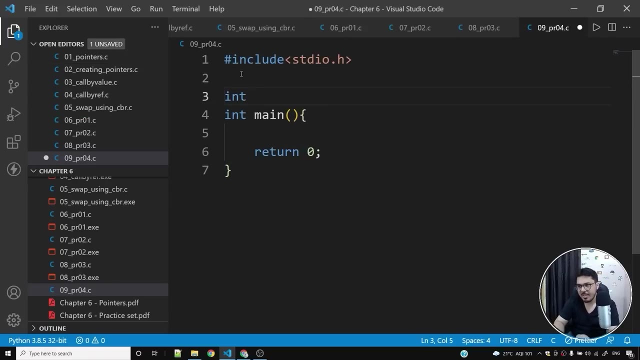 so we are going to create a program called 09, underscore pr03, uh, pr04, i guess. yes, dot c, and what i'm going to do is i'm going to use this as boilerplate code or let me write it from scratch. i want to write it from scratch. so what i'll do is i'll say int, average and sum this: 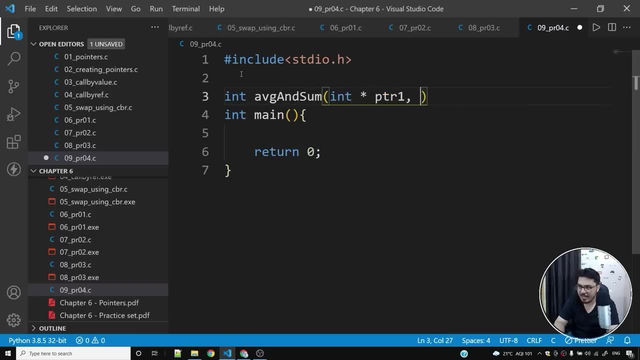 is the name of a function, and what i'll do is i'll take two pointers inside this function and you'll ask me: why am i doing this? i'll answer you. i'll answer you shortly, but for now, just assume that it is required for us to take two points. 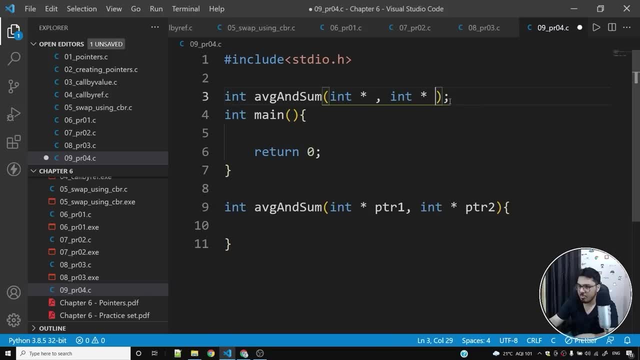 this inside this function also. i'll remove these from here, because this function prototype, this is the function body. so let us say the numbers are a and b. so i'll simply say: uh, int a is equal to six. let me call it float, because we are um, we are actually calculating the average. 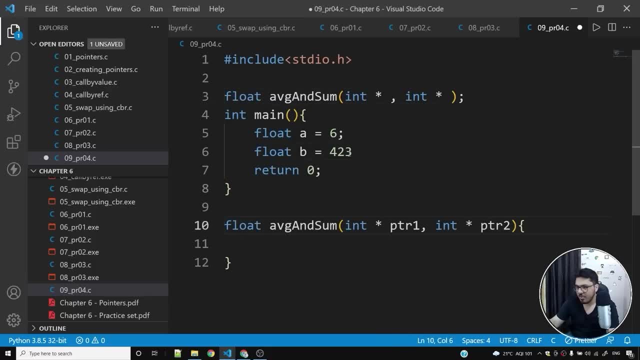 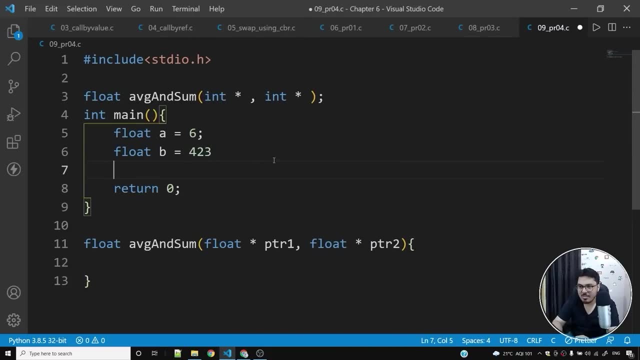 and i want some sort of precision. so i'll make it float and this as float 2, and what i'll do is i'll simply pass the address of a and address of b to average and sum. now what happens is this average and sum function will take the values a, b as well as the address of two more variables, which are c. 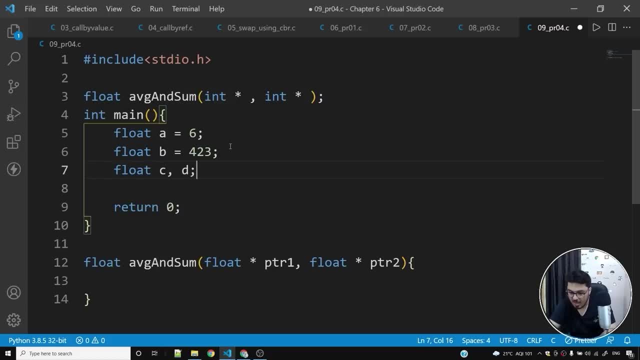 and d. so i have created two additional variables, c and d. now let me explain you what i'm going to do. so i'm going to add int- int as well, and i'm going to take the value of- uh, sorry, i meant float B. let me make it float, because we are dealing with the floating point numbers. okay, and float. 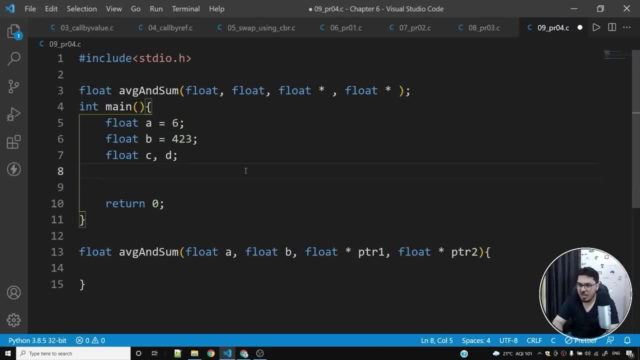 here as well. so we are going to deal with float pointers. now what I'll do is I'll say: call this function with the values A and B and also with two pointers, which are nothing but the address of C and address of D. so listen to me carefully now. what I've done is I've passed the value 6 and 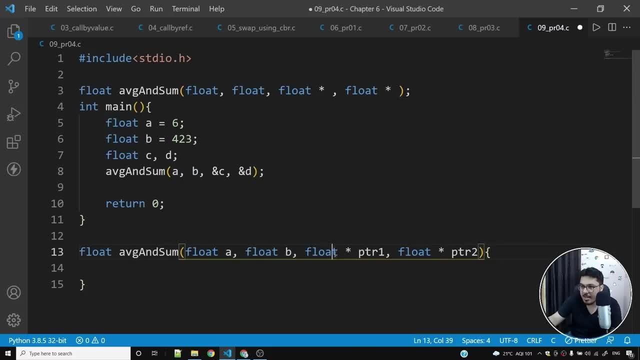 423, which is going to get copied inside this A and this B, and also, what I'm doing is I'm passing the address of C and I'm passing the address of D to this function. why am I passing the address? I'm passing the address so that I can update these two variables, which are C and D, from this function. 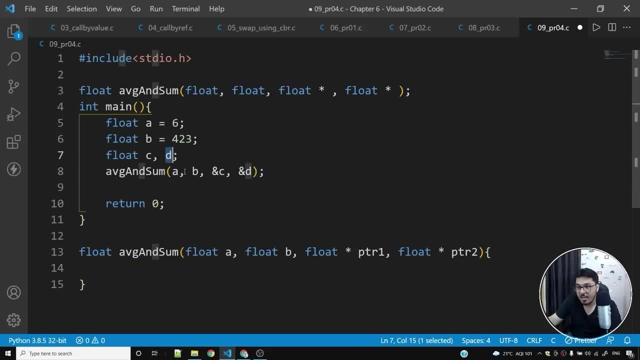 so I'll set C to the average and I'll set D to the sum. to make things more clear, let me call this float sum and float AVG. so I'll pass the 423 and 423, which is going to get copied inside this A and this B, and also, what I'm doing is I'm 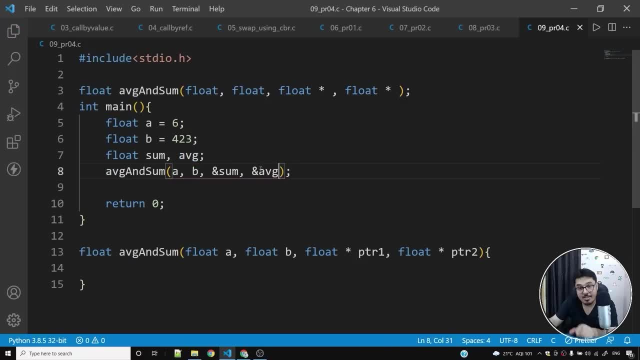 of sum and address of avg, so that i can update sum and avg variables from this function. now listen to me. what i'll do is i'll simply say the value at ptr1, which is nothing, but the value of sum should be equal to a plus b, and the value at ptr2 should be equal to a plus b divided by 2, which is nothing. 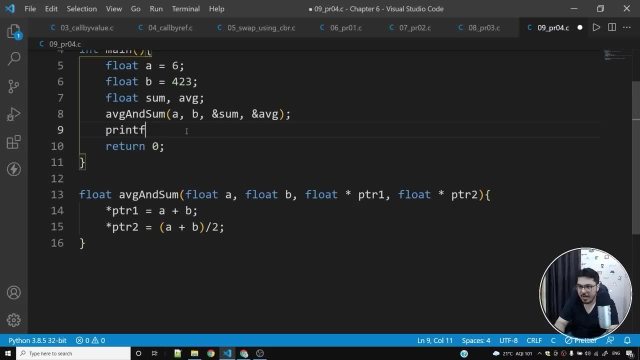 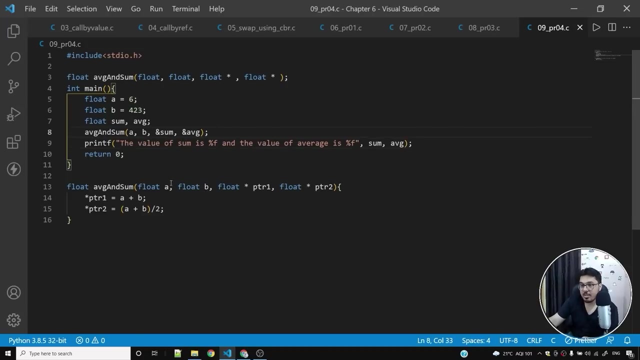 but the average. and now here i can print: the value of sum is percentage f and the value of average is percentage f. so i'll simply say sum and i'll simply say avg, and i can print the values of sum and address which are set using this function. so did you get it? we are not returning anything. 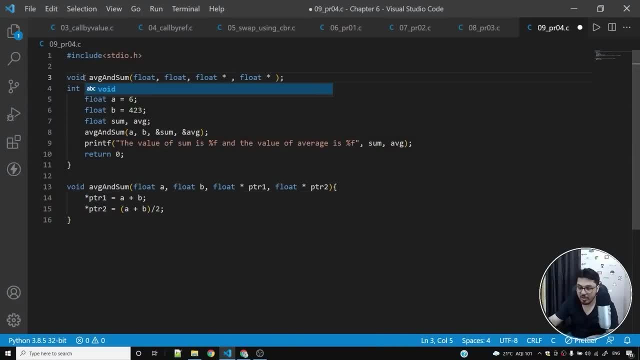 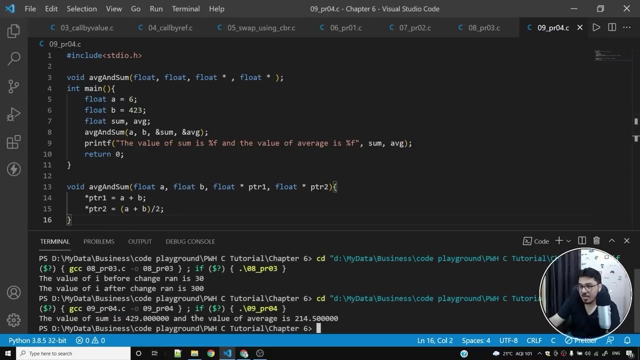 from this function. let me return void from this function. you we're not returning back anything from this function, but what we are doing is we are essentially setting the values of sum and average from this function. i hope that you understood this. let's see if the program works. so it says the value of sum is 429, which is correct because 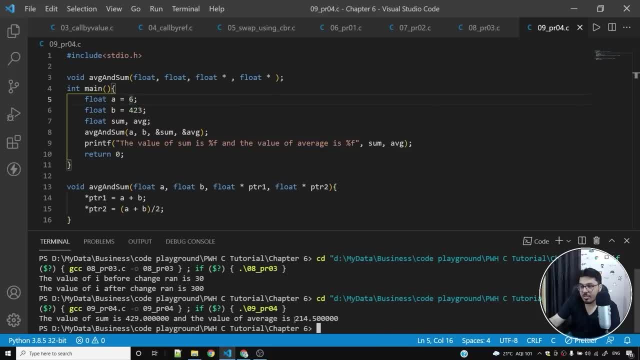 423 plus 6 is 429 and the value of average is 214.5. so if you add these numbers, it will turn out to be 429, and if you divide 429 by 2, it will turn out to be 214.5. 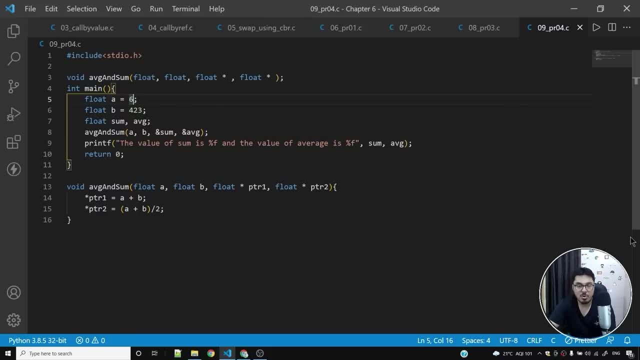 how was this program? let me know in the comments: was this something that you saw for the first time in your programming career or was it something that you have seen before? if you are a c beginner, or programming beginner for that matter, this is something that you might have seen for the first. 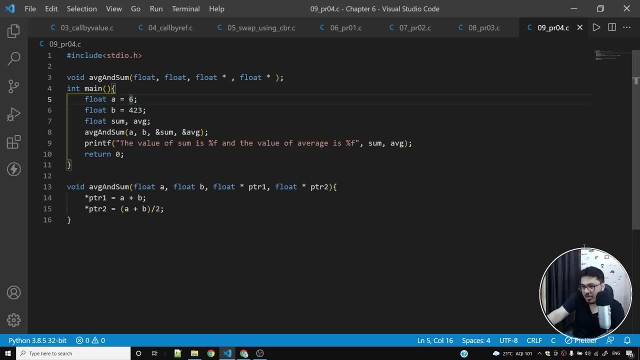 time and you should definitely appreciate the power of pointers. see, we didn't even pass sum and avg. we simply passed the addresses of sum and avg to this function and we got the value of sum and these addresses were captured inside ptr1 and ptr2 and the values at ptr1 and ptr2 were updated. 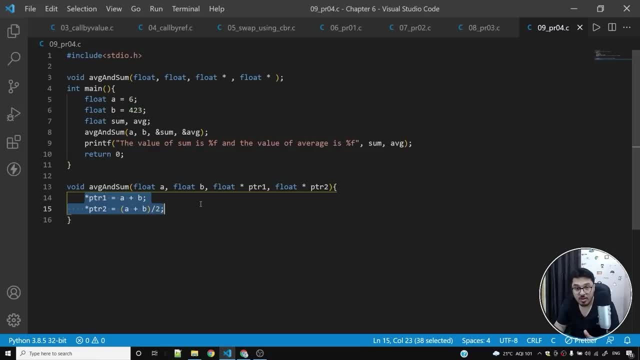 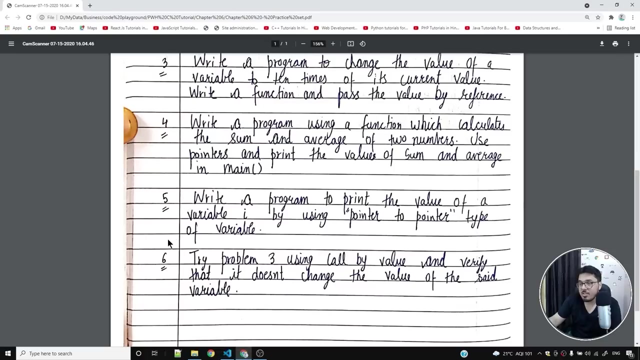 inside this function. i'm not returning anything from this function directly. i'm not returning anything from this function, but indirectly i am kind of returning something from this function. what is that? i'm setting the values of variables in the main function from this function. so this program is actually very important. mark this program as important and if you haven't understood, 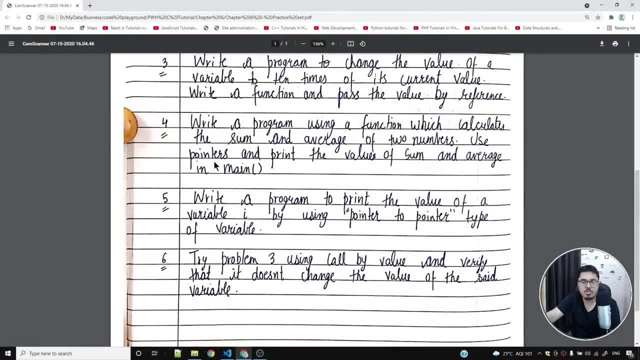 what we did in the previous video, then you can do that by clicking on the link in the description in this program. i want you to watch this question once again. coming back to the practice set and to the question number five, write a program to print the value of a variable i by using pointer to. 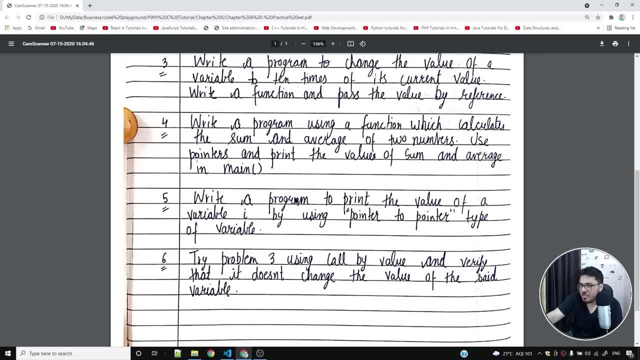 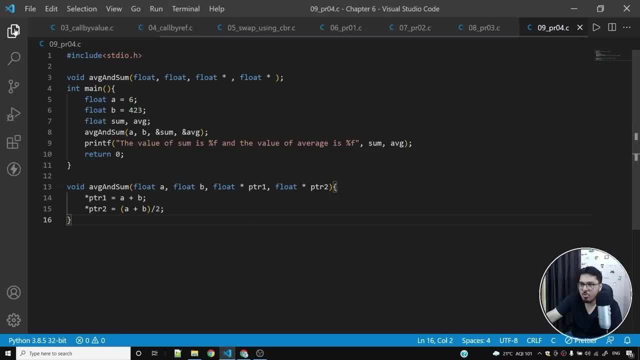 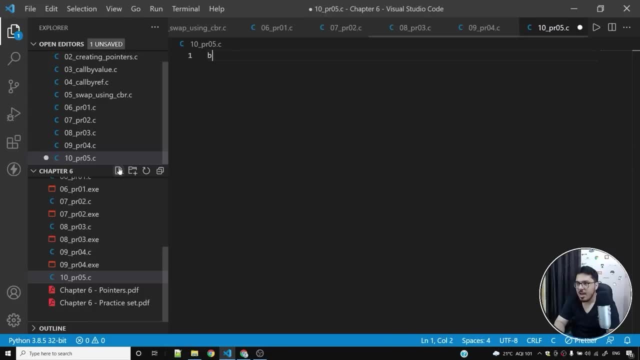 pointer type of variable. so what we'll do is we'll simply write a program which uses pointers to pointers. so let's write a program which uses this: pointers to pointers. so this is 10th program. problem number five: ten: underscore pr, zero, five dot c, and i'll put in this program and i'll put in. 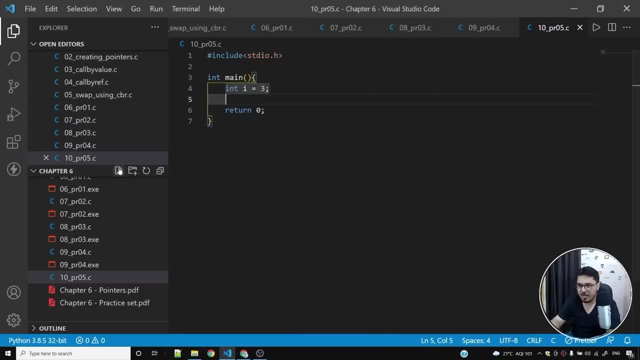 the boilerplate code. so i is a variable. it has three inside of it. let me create a pointer, one i'll say it's an integer pointer- which contains the address of i. so far, so good. i'll say, i want a pointer to pointer which is ptr2, which contains the address of ptr1. so ptr1 is a pointer variable. 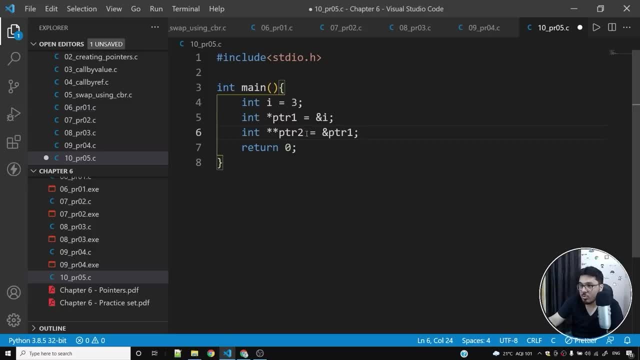 and its address is stored inside ptr2, which is a pointer to pointer. so ptr1 is a pointer variable, ptr2 is a pointer to a pointer. okay, now let me show you something. what is the value of i? yes, it's, it can be printed this way. but uh, no surprises, this will print the. 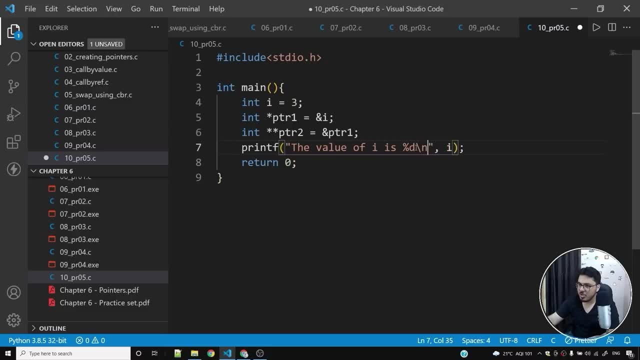 value of i. what's new? i'll show you what's new- in fact, not even new, because we have already talked about all these concepts in the chapter. so i can say: the value of i is star ptr1. can i say this or not? why can i say this? why is the value of i star ptr1? ptr1 is simply storing. 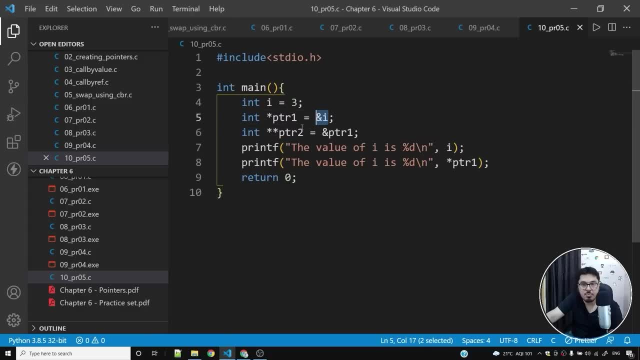 the address of i. ptr1 holds the address of i and since ptr1 holds the address of i, i can always dereference ptr1 and i can say star, ptr1 and star ptr1 will give me the value at this address, which is the address of i. so what is the value at the address of i? it's the value of i, which is three. 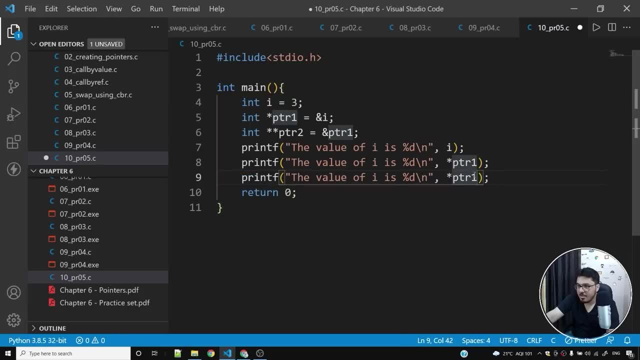 now i can also say: the value of i is star of star of ptr2. okay, so i can actually write ptr1 as star of ptr 2. can i do this? yes, i can do this. i can always do this, because ptr1 can be written as star ptr2. now, if you, if you haven't understood why this is the case, try to map this with y: the value of i: 1.. ﷺ. 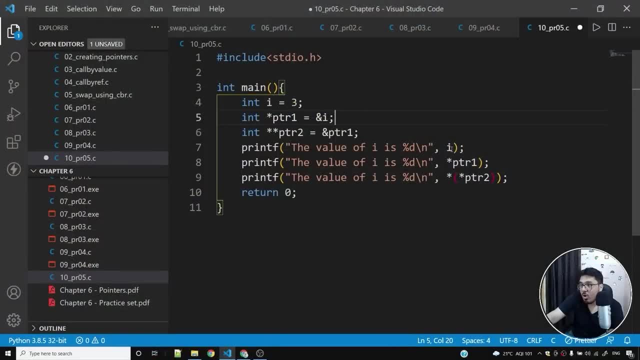 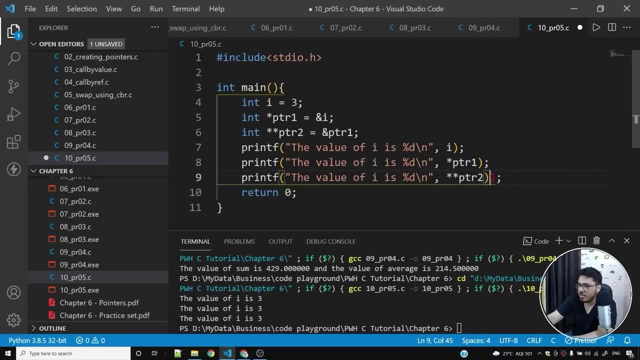 END was star ptr1, then you will be able to understand why the value of ptr1 is star ptr2. and if i run this program, let me show you all these lines will print: the value of i is 3. i can also get rid of this: the these parentheses and this will actually print the same thing. so this is how we can print. 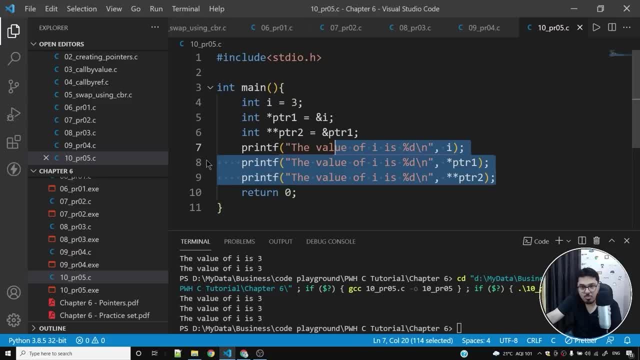 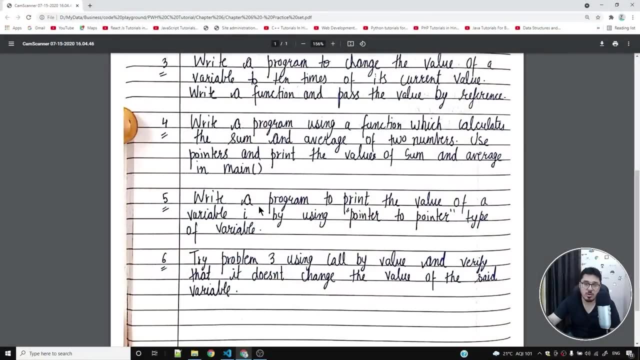 the value of i using pointer direct value, pointer to a pointer. okay, i hope you understood this. so this was simply the question which was created by me to explain you: pointer to pointer variable. so problem number six now says that. try to attempt problem number three using call by value and. 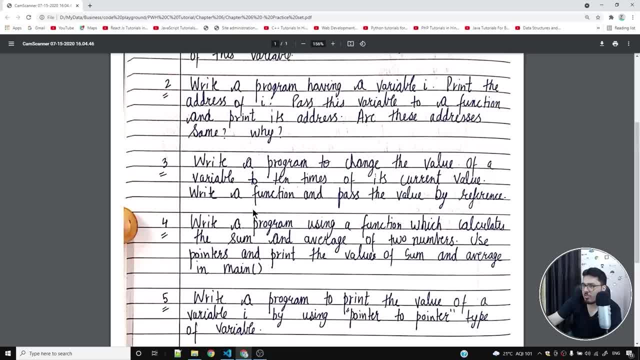 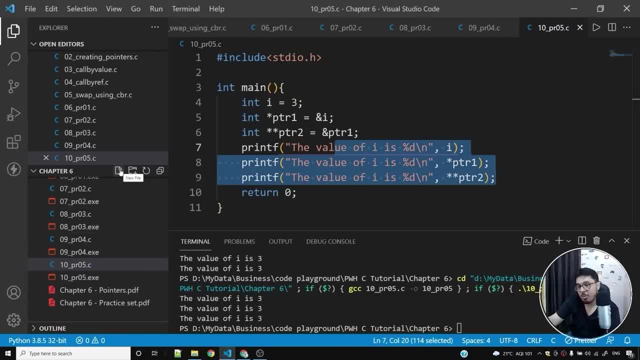 verify that it doesn't change the value of the set variable. so what was problem number three? problem number three was um. let's, let's see we solve problem number three. so let's create a program and we'll copy the code of problem number three. so i'll say 11 underscore, 11 underscore, pr. 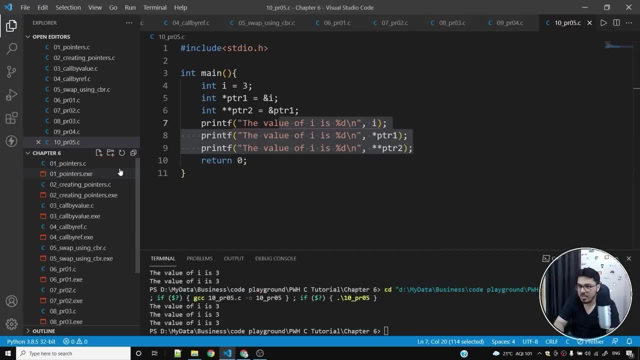 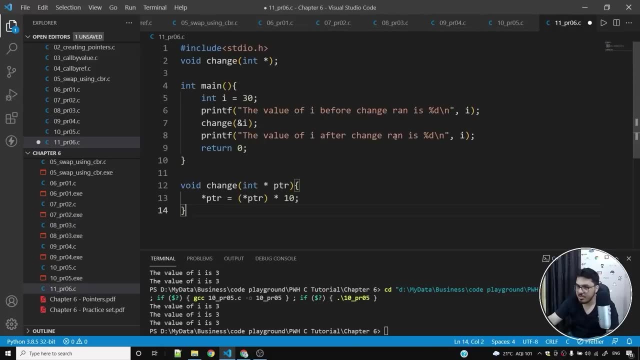 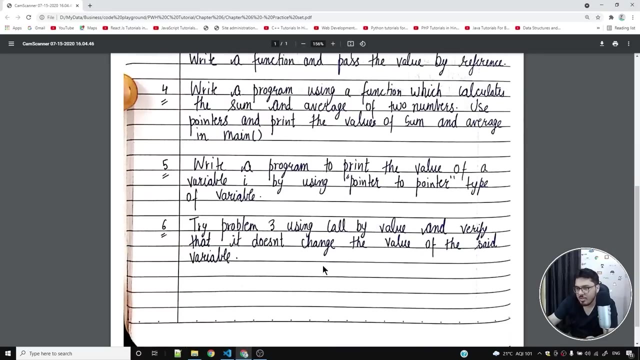 pr06 dot c. i'll put the boilerplate code in. in fact, i'll not put the boilerplate code. i'll copy the problem number three and i'll paste it inside problem number six. so problem number six is talking about problem number three. it says that what if we use call by value instead of reference? 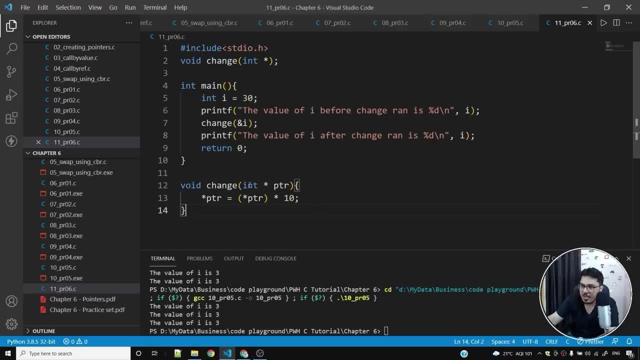 it simply says that you are actually passing the address of i. what if you actually pass i and not the address of i? so what if i do something like this- and let me not even call it pointer in that case, because it's not a pointer- and what if i do something like this? i'll say i is equal to i. 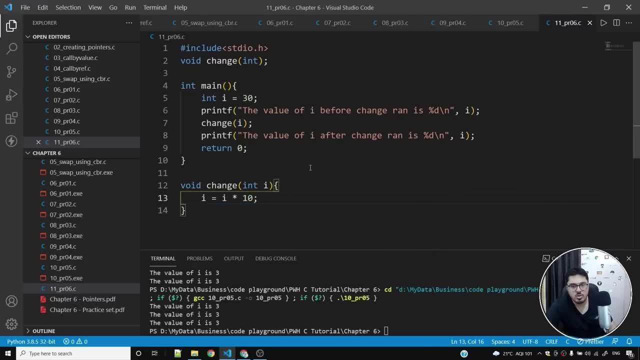 multiply by 10. can i do this? yes, obviously i can do this, but it's not going to change the value of i inside main function. let me show you so. if i run this program, you'll see the value of i before change ran is 30 and even after change ran, it is 30. we were expecting it to be 300, because we are. 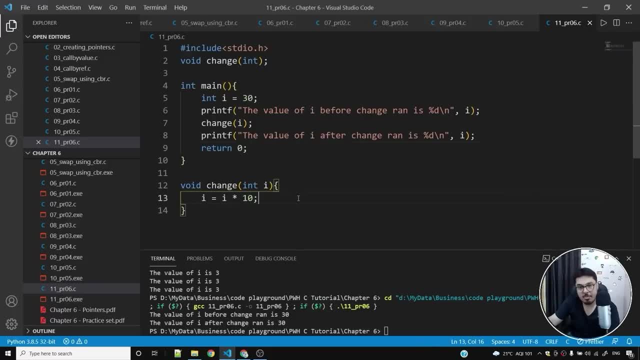 actually changing the value of i to be i multiply by 10. why does this program not work? why did this uh fail to update the value of i? this happened because what we are doing here is we are simply saying int i is equal to 30. now we are printing the value of 30, now we are passing a. 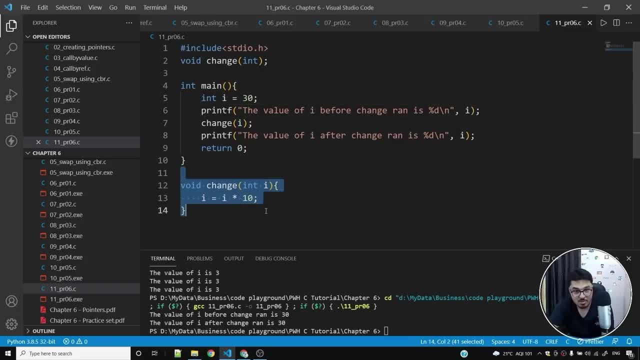 copy of i to change function, a copy will be passed. so if i have this keyboard and i create copy of this keyboard and i distribute it to my friend and he breaks the keyboard, will this keyboard also work? no, it will not get broken, because why, why, why will this keyboard get broken? so if you are buying 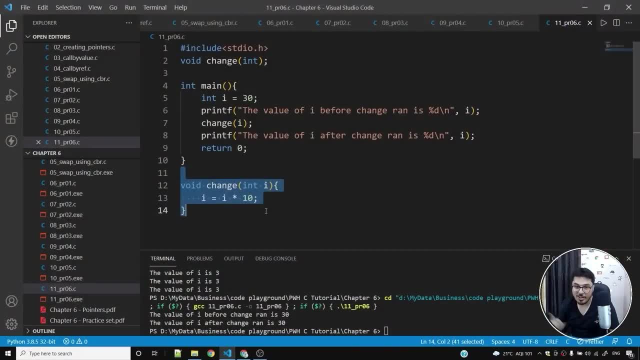 two iphones- one for your friend, one for yourself- and your friend actually throws the iphone um inside- um inside, say, inside the fire- and he burns his iphone. will your iphone also get burned? obviously not so. this is why the value of i is not changed inside the main function. but if i'm 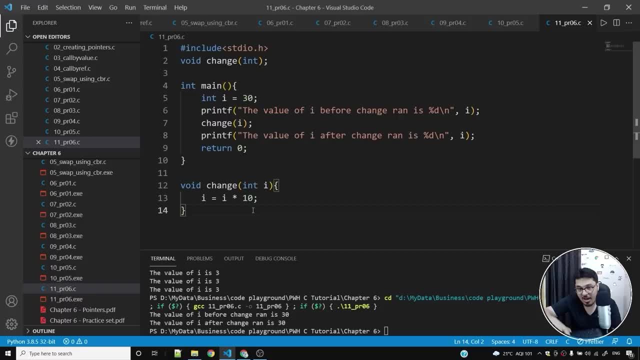 passing the address, or if i'm giving the reference of my iphone and i'm saying: this is my iphone and your friend actually throws your iphone inside the fire, so your iphone will get burned. i hope that this analogy makes sense. i know this is funny but again, i hope that it it will help you in some way to understand all these concepts. so, with that said, 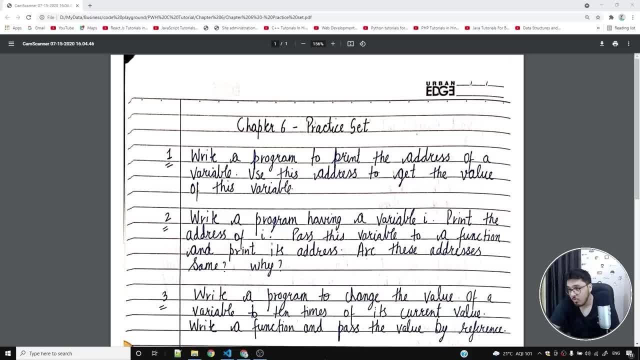 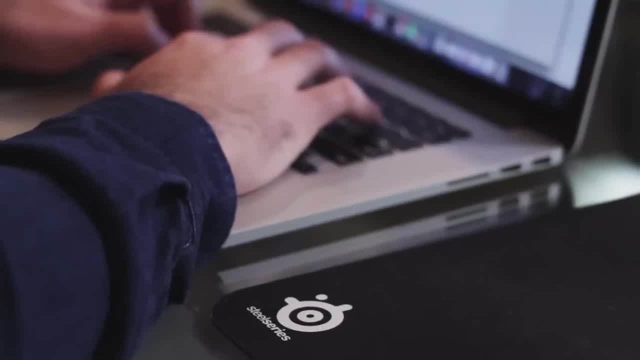 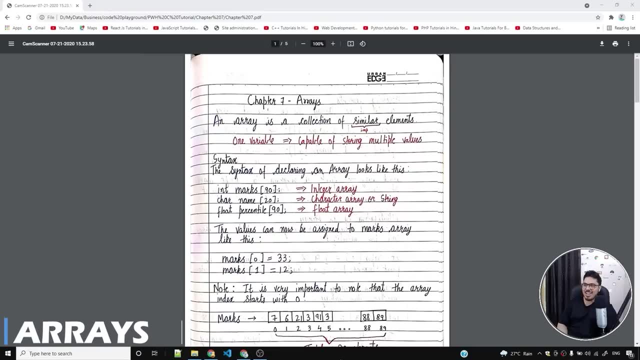 the chapter number six is finished, so we'll move now to the next concepts and we'll explore c programming language even further. so, now that we have completed so many concepts of c programming language, we are going to look into arrays. what exactly it is an array? an array is a. 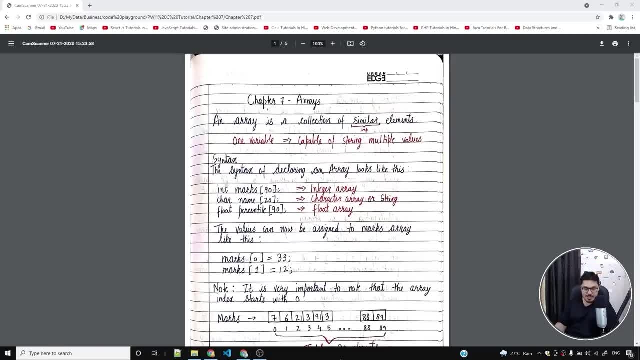 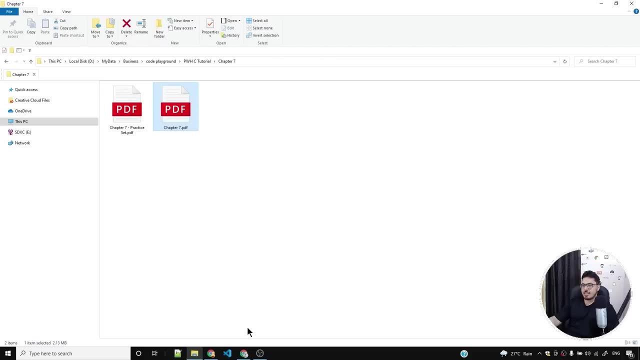 collection of similar elements, and this is really very important. these elements have to be similar because you cannot add an integer and a character inside an array. but since we just started out, i don't want to confuse you. i'll show you some of the very basic syntax of arrays and then we'll 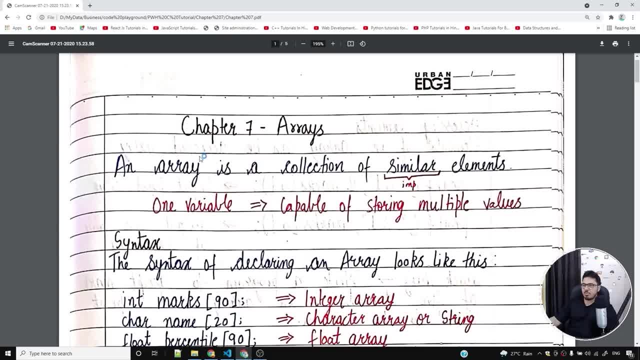 raise the bar from there. so let's get started with what an array is. so sometimes you might want to store marks of, say, 100 students. how will you do that? you might be tempted to create 100 variables saying marks 1, marks 2, marks 3, marks 4, but c. 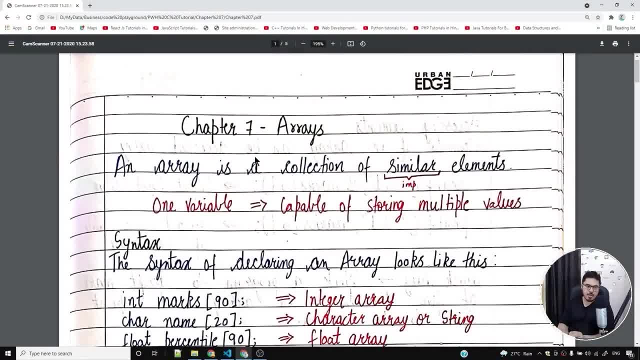 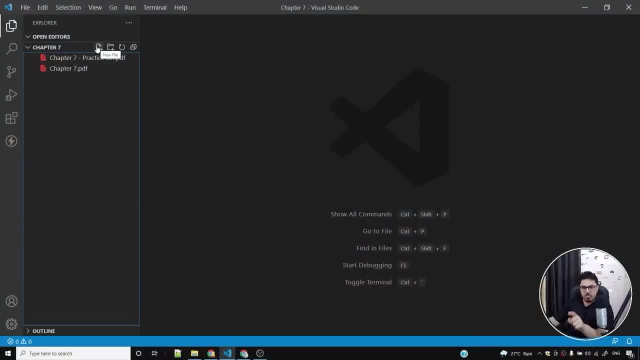 programming language provides you a very elegant way of doing the same thing. what is that elegant way? you can add all the marks of 100 students inside one variable which is nothing but an array, collection of similar items, in this case the marks of students. let me give you a very brief idea of what array is. i'll say 0, 1 underscore. array basics, dot c. 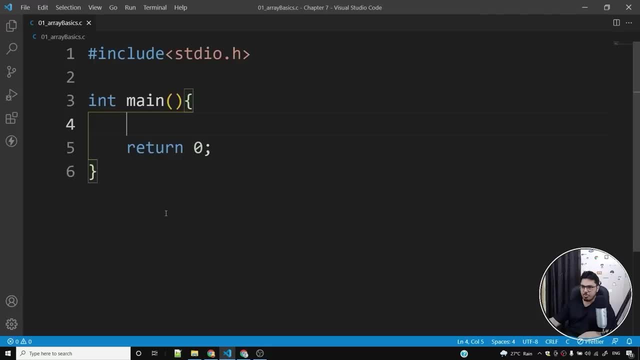 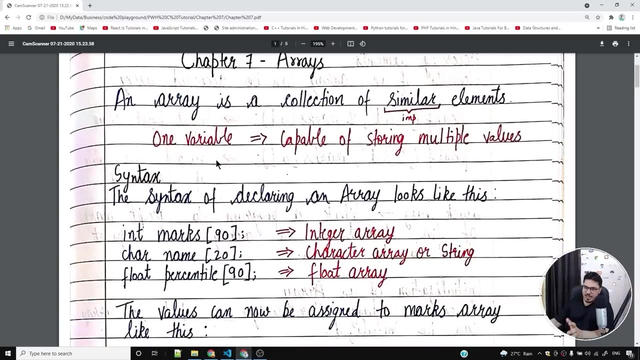 i'll put in the boilerplate code, i'll zoom in a bit, i'll close the explorer and let me show you what an array is. so if i do something like this, this is the syntax of writing an array. so basically, it's a single variable and it's capable of storing multiple values. so i just gave you an. 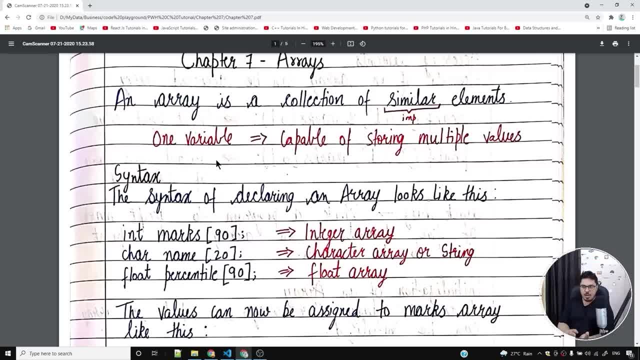 example of marks. let us say you want to store 100 marks. so let's say you want to store 100 marks of 100 students, with raw number ranging from, say, 1 to 100. you might want to store all these values inside one single variable instead of storing it in 100. 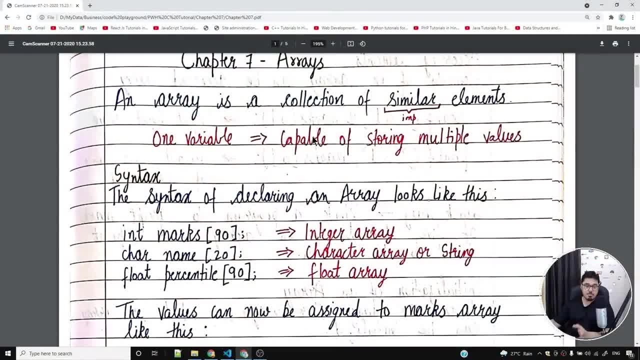 variables, because creating 100 variables might be very cumbersome task. you cannot do that and even if you are able to create 100 elements, it will be really very difficult for you to create thousand variables for thousand elements, or say, ten thousand or one one million variables for one million values. you got the point. so what is the syntax of creating? 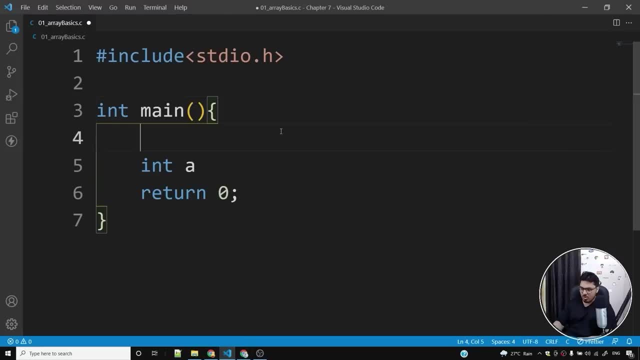 an array. so let us say i want to store marks, of marks of 30 students, or let me make it, uh, eight students, because 30 is just too much. okay, so i can do something like this. i can say in a1 and a2, then a3, then a4, then a5, then a6, then a7. you must be thinking what i'm doing here, but i'm trying to. 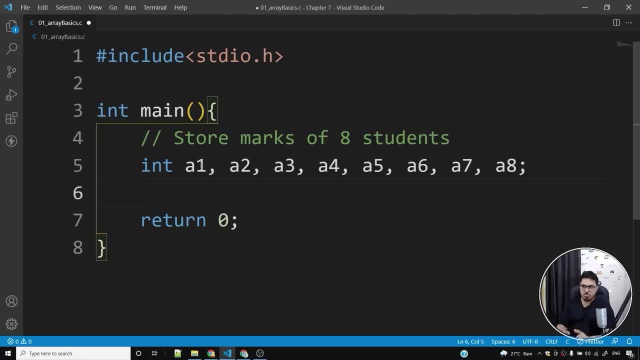 create eight variables for storing marks of eight students. so these are eight variables, and all of these eight variables will store marks of eight students. i can do something like this: i can say a1 is equal to this, and then i can say a6 is equal to say a87, and so on. i can assign marks. 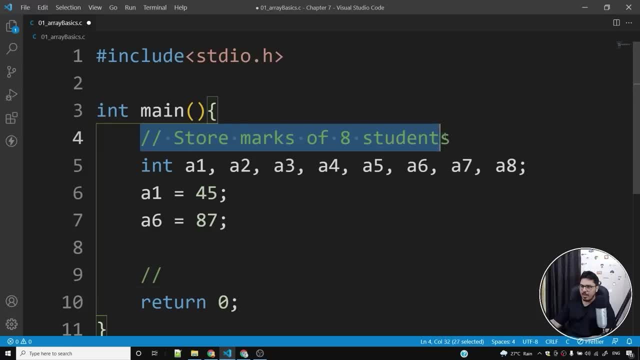 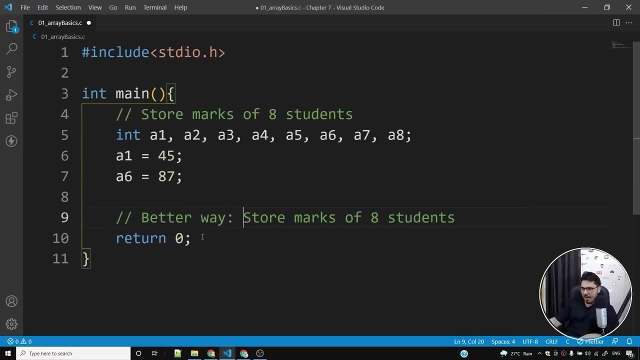 to these variables. but there's a better way, and let me tell you what that better way is. so i'll say better way, and. and a better way to store marks of eight students is something like this: you create an array, you say a and you simply say the number of values. 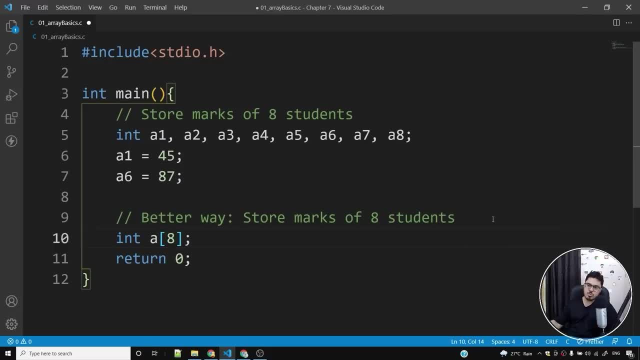 you want to store and that's it. that's it and how you store. uh, or rather assign marks. let me assign marks for all the variables. let me make it 49. i'm just taking random values for a1, a2, a3, a4, a5, a6 and so on. um i i could have actually added 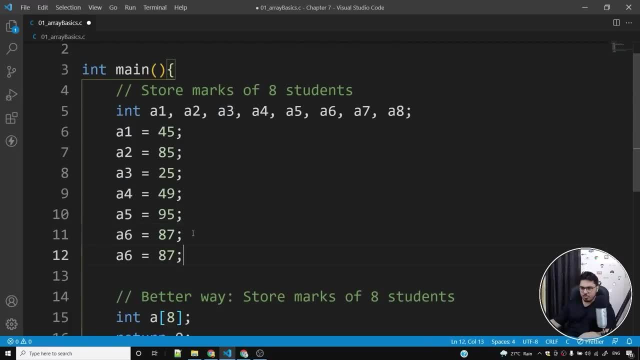 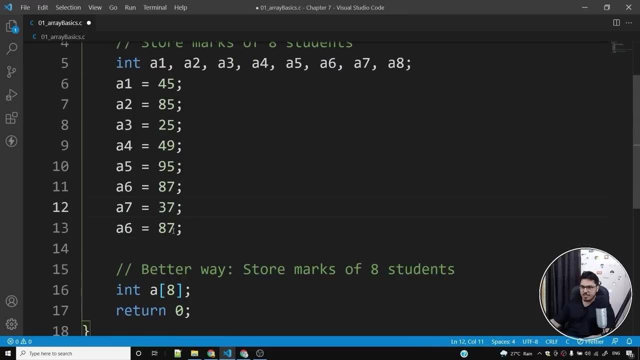 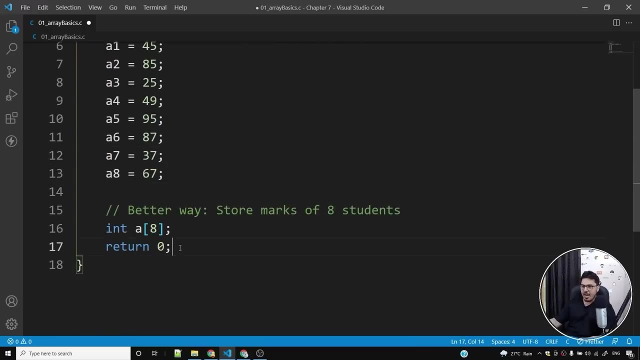 values here itself. but again, i just want to show you how this maps to the better way of storing marks. so let me say 37, and let me say 67 for a8. okay, here what i'll do is i can actually start accessing all these variables starting from index zero. now this is important. 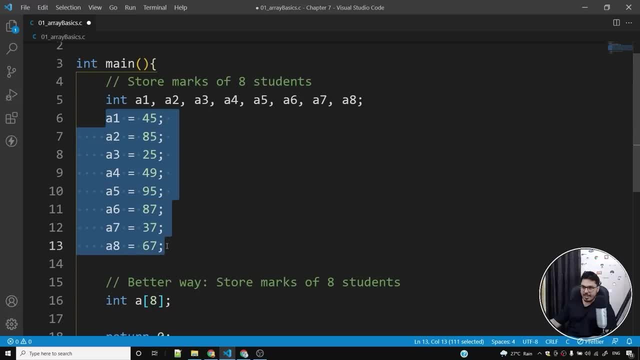 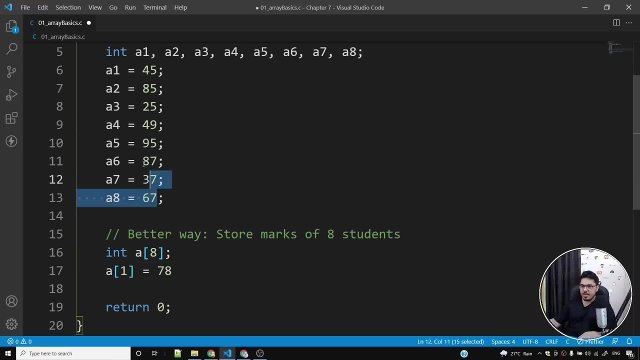 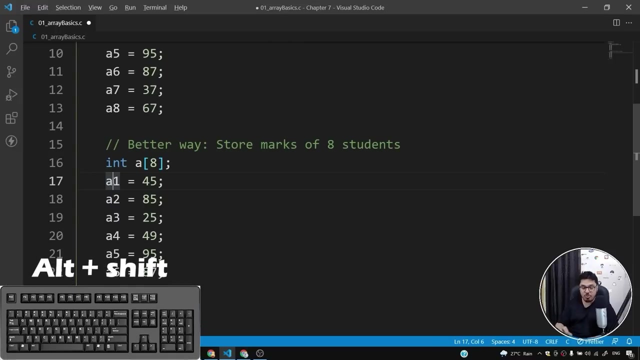 here i started writing a1, a2, a3, all the way till a8, but here, instead of doing this, a1 is equal to 78 and let me copy. copy this so that i can actually show you how this really maps, and i'll press alt shift on my keyboard. alt and shift i'm pressing together. 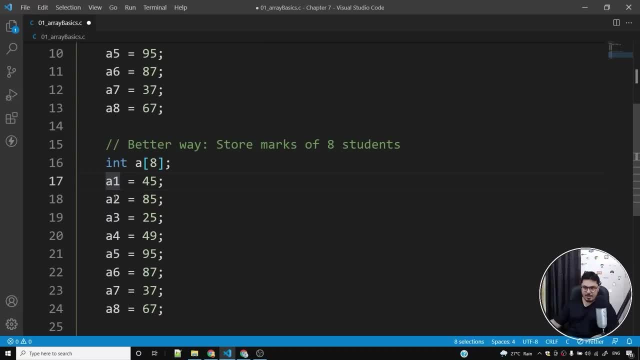 on my keyboard and i just clicked here and i'm getting all the cursors this way. so what i'll do is i'll put in the square bracket and i'll use arrow keys and once again, i'll put another square bracket. now this is a syntax. this is part of the syntax. if you don't know how the syntax works, 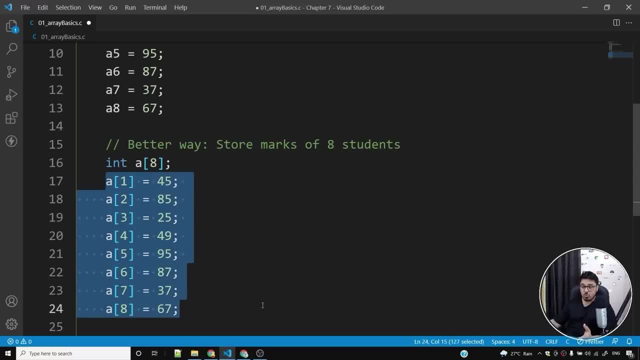 you might want to manually do this if this is not supported by your code editor. if you're using some other code editor or the other way around, you can use this as well. so i'm going to show you rather than visual studio code. your editor might not support this type of syntax and in that case, 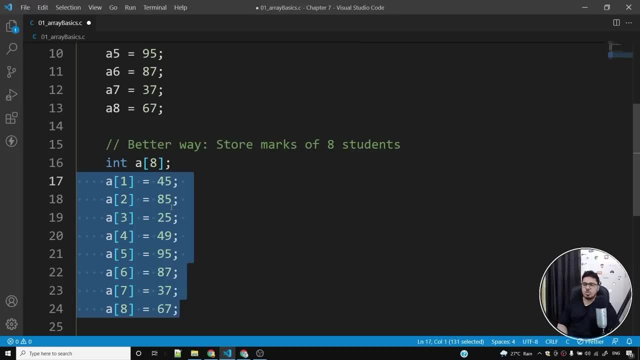 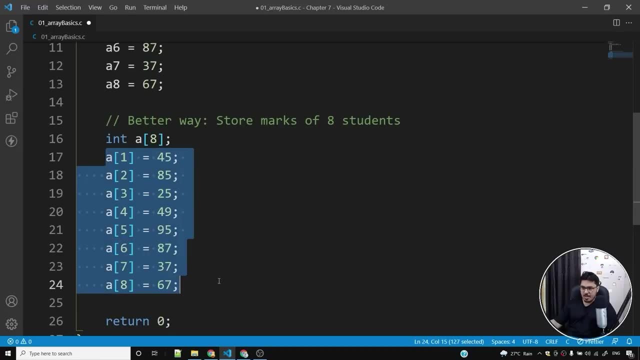 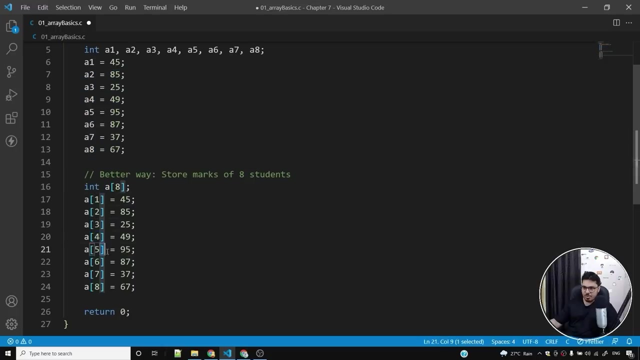 what you will do is you can simply uh use, you know, manually put all these uh square brackets. now i can do something like this, but this doesn't directly map to this. now you must be thinking that we can uh say a1, a2, a3, a4, a5a6. 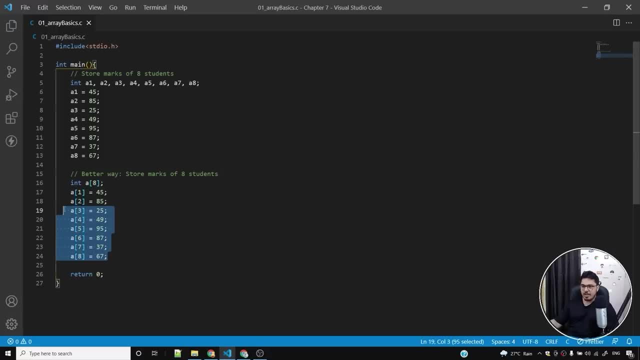 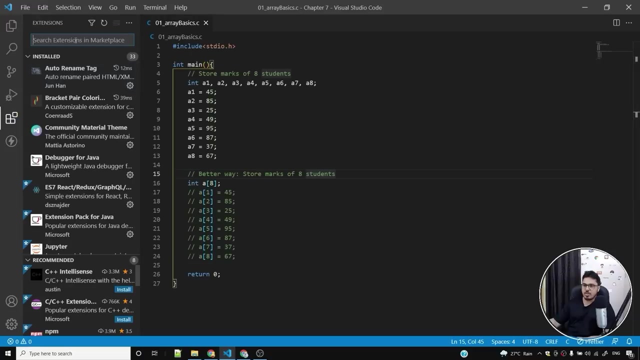 let me, let me show you, let me run this program for you. uh, i'll get rid of this part. i'm getting rid of this part because this part is going to throw an error. i'll tell you why. but again, i can assure you that this particular syntax is correct and we can actually run this. so let me enable code runner i. 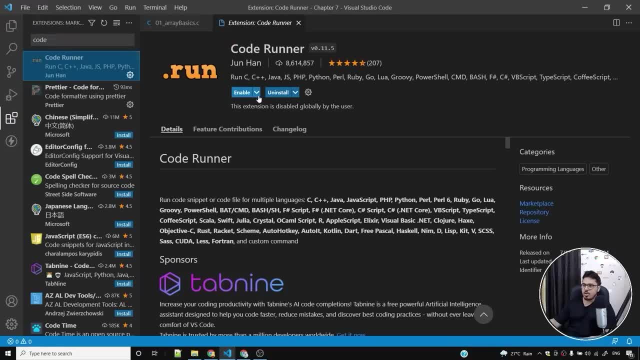 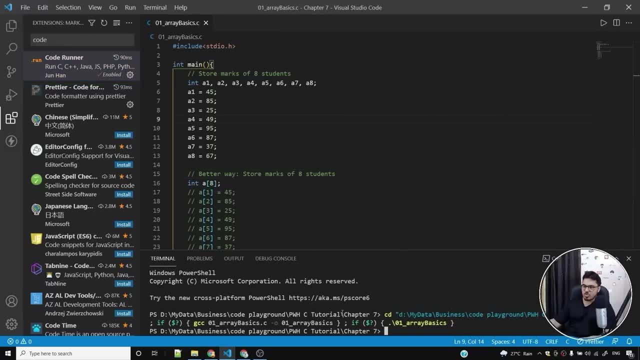 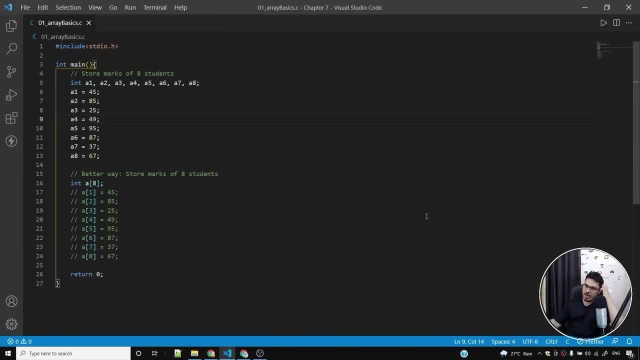 think i disabled code runner, so code runner is by default disabled. i want to enable it in this workspace and i'll run this code. and this code is not throwing any error, which means we are good and this code works. so what i'll do now is i'll simply say: is 1 is equal to 45, and i'll i'll show. 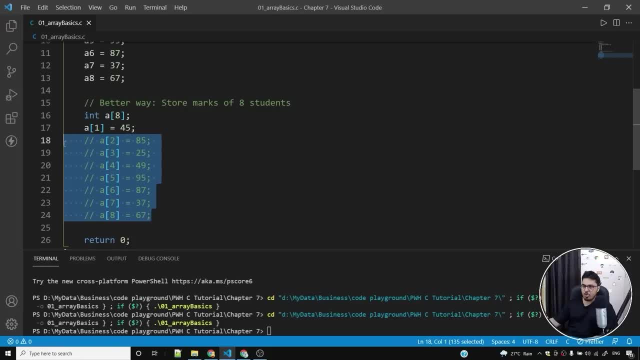 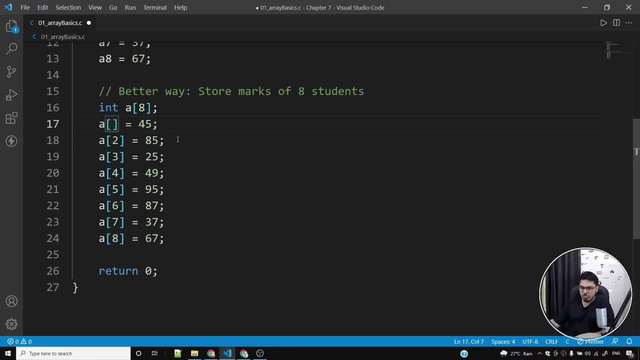 you and run this and show you, and i can keep on doing this. so the problem with this syntax is: instead of starting from 1, we actually start from 0. so we start from 0 and then we go from 1, 2, 3, 4, 5, 6, 7, so for 8 words. 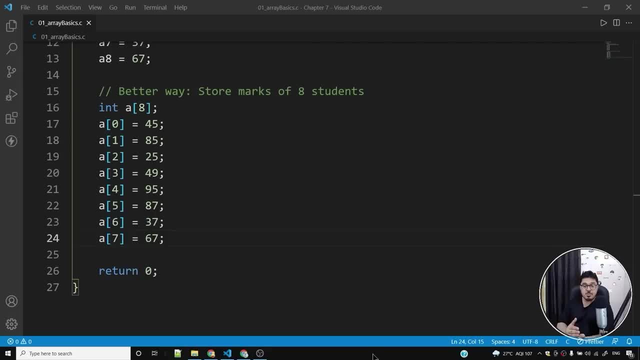 we start from zero and we'll go all the way till seven. the numbers from zero to seven are actually eight numbers, if you, if you count it. zero to two are three numbers. zero one and two. zero to four are five numbers: zero, one, two, three and four. so these are five numbers. so this is something that 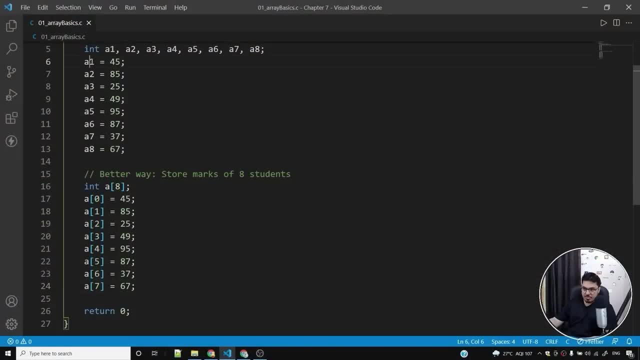 you need to understand. and we don't start the index from one. we start the index from zero. so you might have heard this in the memes and the jokes: that index starts from zero. counting starts from zero in most of the programming languages, and that's the case with c as well. so we do. 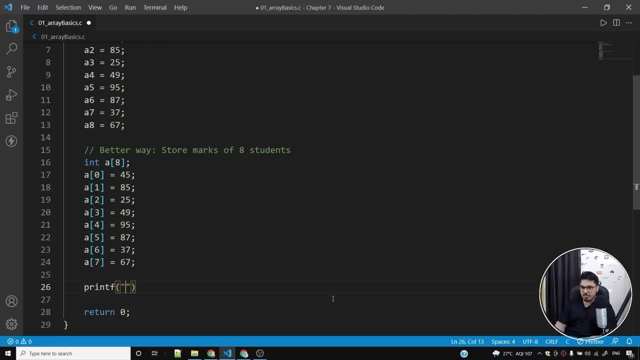 something like this, and i can actually use this variable by doing something like this. i can say the value of student number zero is. so we start the counting from zero and the value is going to be a zero. so this is going to print: uh, let me also put backslash n for better readability. 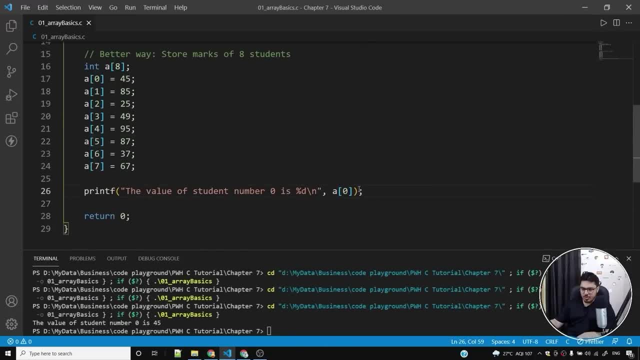 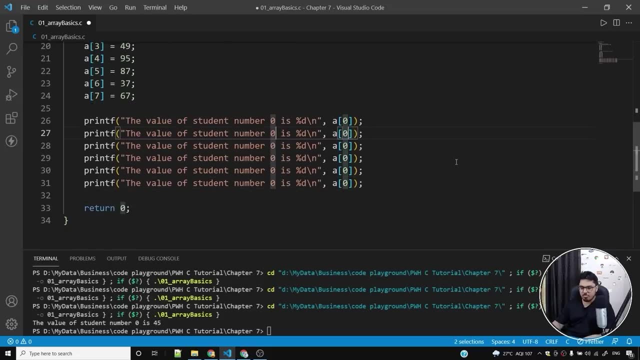 this will print 45 for me and i can do the same thing for a student. you can do the same thing for a student and i can do the same thing for a student. one student, two, three, four, five, six. i can do this for all the students, so i'll put in one here. 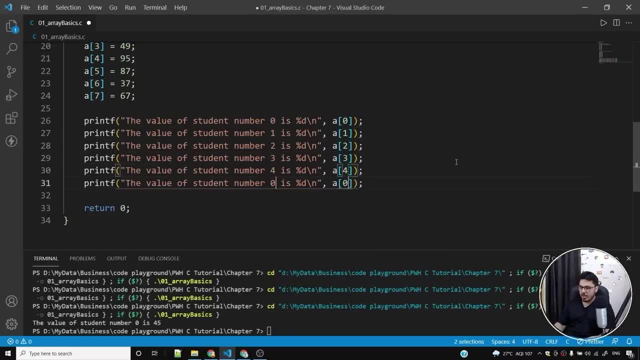 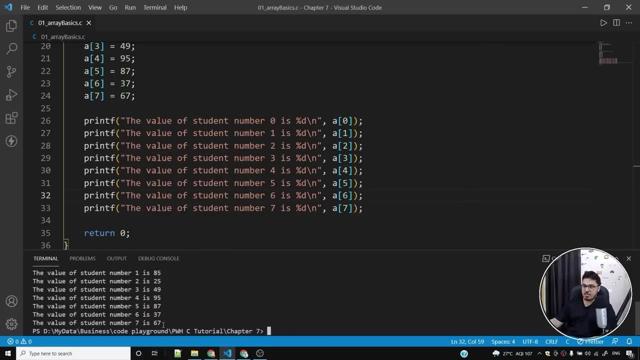 then i'll put in two here, then i'll put in three here, four here, five here, and you can print all, all of these variables. but uh, okay, let me, let me do it for all the variables. so i'm simply using multi-cursor functionality of vs code. um, i'll run this and you'll see all the marks that i have. 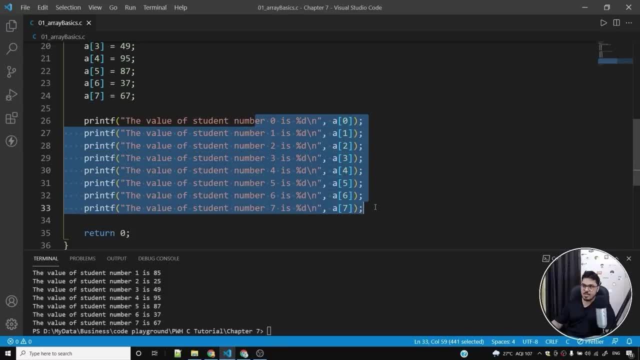 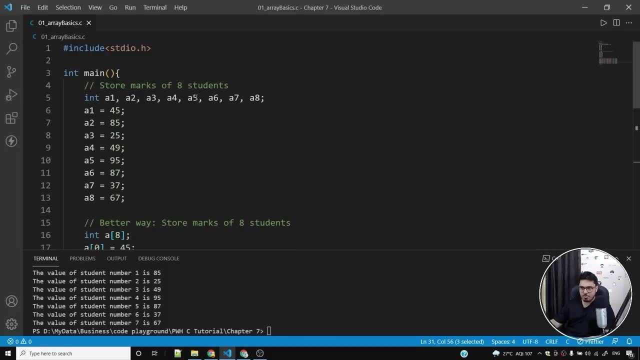 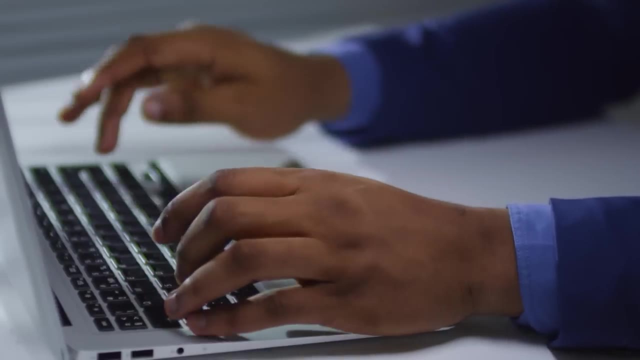 assigned here are printed, so i can actually use this as a single variable. i can use the a7 as a variable. i can use a5 as a variable. now we have marks of eight students at this point. so this approach will actually take a lot of lines of code. it will take a lot of typing, if you 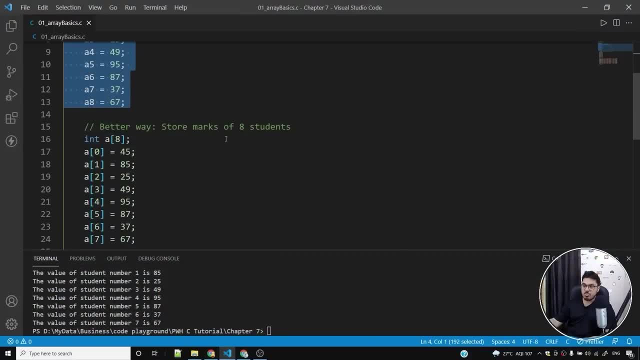 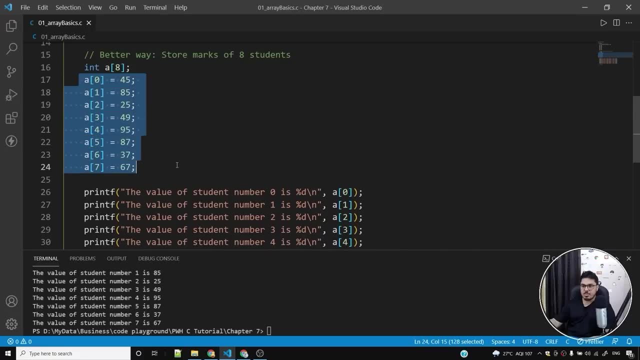 try to create, say, thousand variables. but if you try to create thousand variables using this approach, all you need to do is you have, you need to replace this eight with thousand and you can keep on using your variables as and when required. also, you can use a for loop and you can assign all. 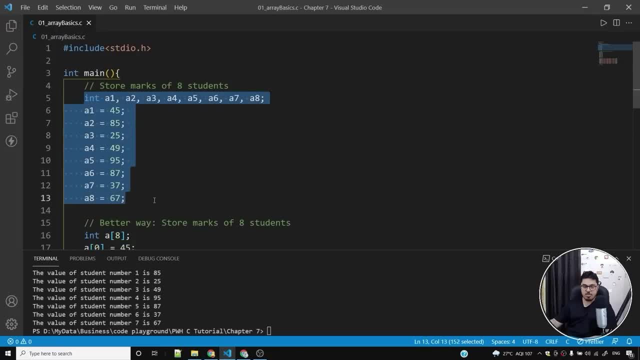 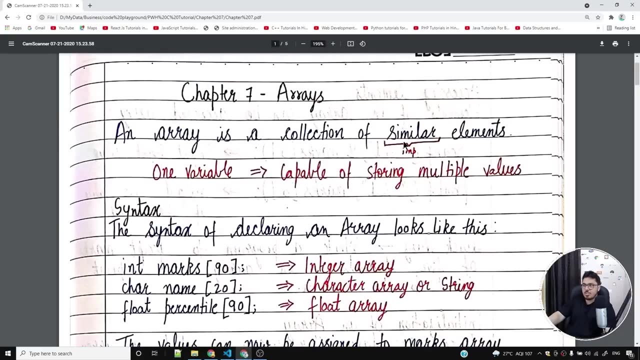 these values, but in this case there is a lot of variables that you can use to create a thousand. there's no way to assign values using a for loop. we'll see that. we'll see that in, uh, in this chapter itself. so, coming back to the arrays, it's a collection of similar elements. in this case it 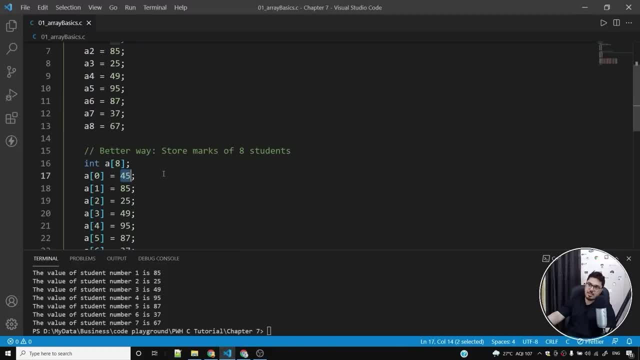 was collection of integers. it can be a collection of characters, it can be a collection of floating point numbers and so on. so we can create a float array, we can create a car array, and so on. okay, so an array is a collection of similar elements. it's a single variable capable of storing multiple. 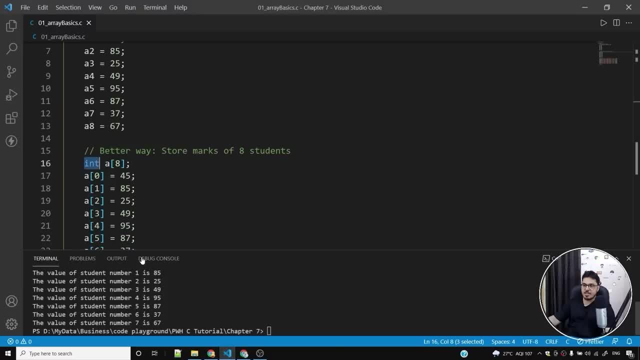 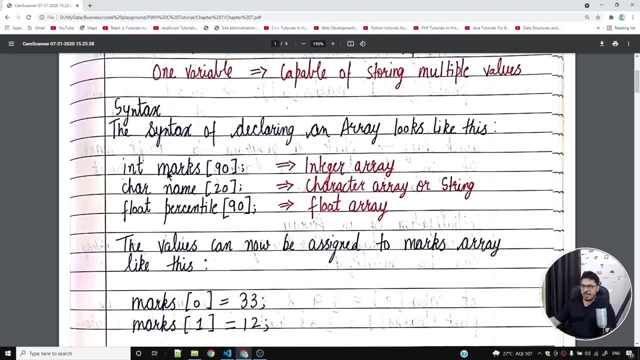 values. so this is a single variable. in this case, the variable was a, but it was actually capable of storing eight values. so the syntax looks something like this. you can do something like int: marks 90. this is an integer array. you can store values inside marks 0, marks 1, marks 2, marks 3, marks 4, 5, 6, all the way till. 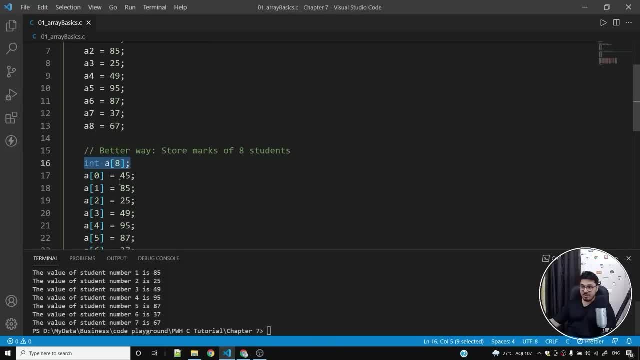 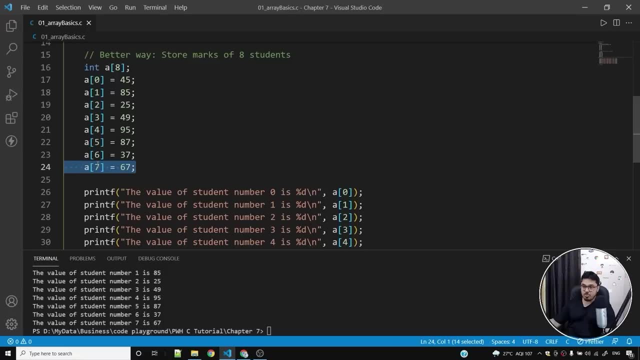 89, not 90. make sure, because when we had array of size 8, the maximum index we can go up to is 7 and not 8. if you try to use a 8, you will get into troubles, you will get into memory leaks and 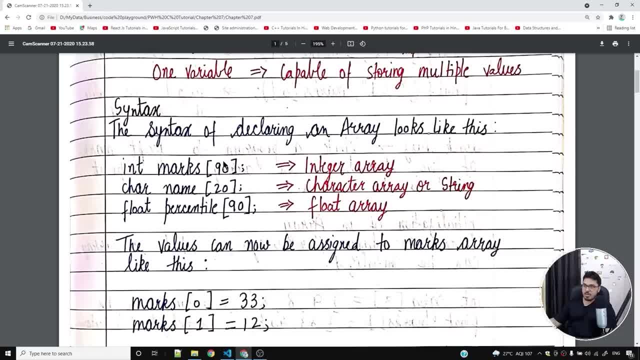 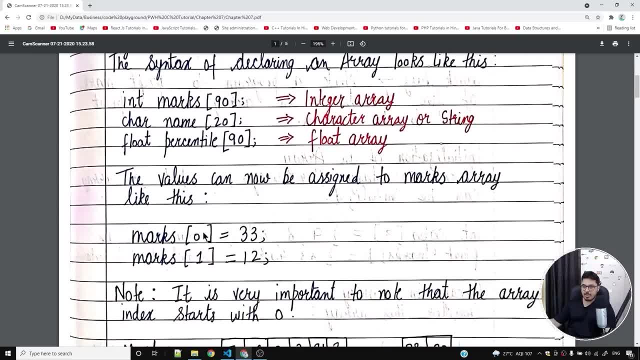 all. we don't want that syntax of declaring an array looks like this: this is for integer array, this is for character array, this is for floating point array, and so on. the values can now be assigned to marks array like this: i've written this in the notes so that you can easily revise. 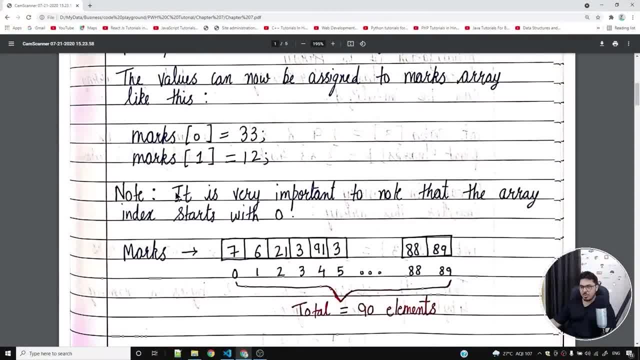 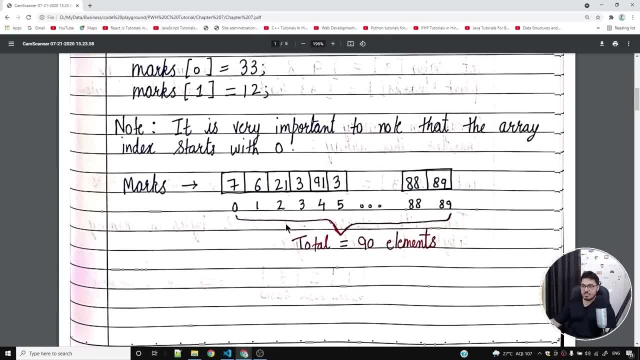 this in the future. now there is a note here, there's a side note i've written here. it is very important to note that the array index starts with zero. this is really very important for you to understand that if we have total of 90 elements, the counting starts from zero and not from the 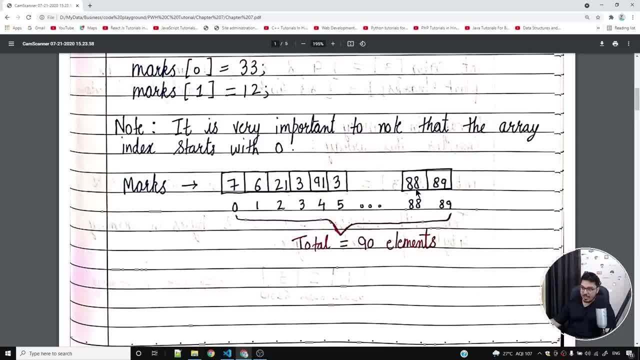 one. if you start it from one, we can go all the way till 90. but if you start the counting from zero, you can go all the way till 89 for 90 elements. you can do this. you can try this for eight elements and you can start writing 0, 1, 2, 3, 4, 5, 6, 7, 8 for eight elements. let me show this for you for six: 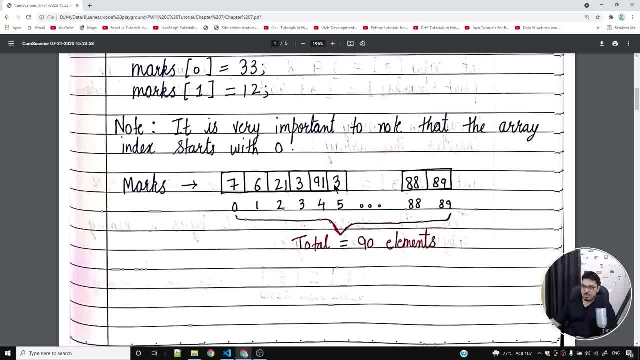 elements. so these are six elements: 1, 2, 3, 4, 5, 6. but if you start the counting from zero, you can only go till 5 and not 6. you can see that 0, 1, 2, 3, 4, 5, because one additional space will be taken by. 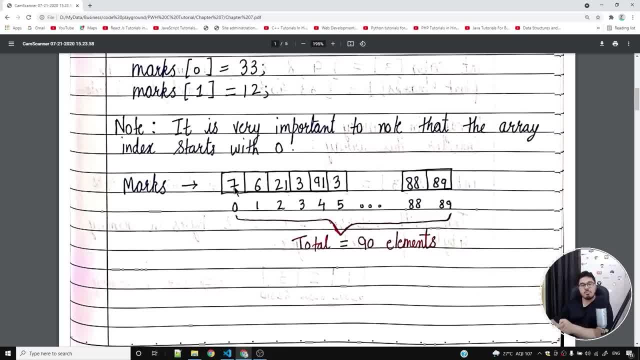 0. if you start the counting from 1, you can go all the way till 6, but in this case, you can go all the way till 5, starting from 0. so this is something that is very important and straightforward as well: start the counting from 0 and go up to n minus 1 if there are n elements. so in this case, 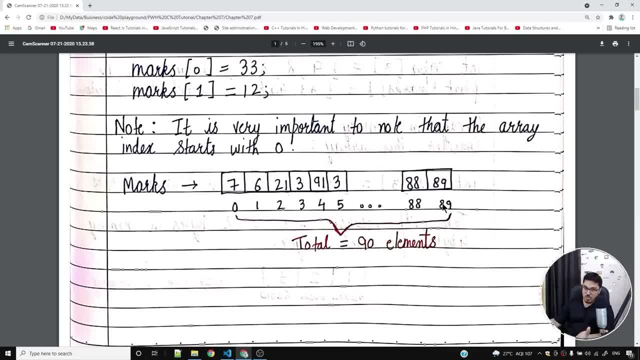 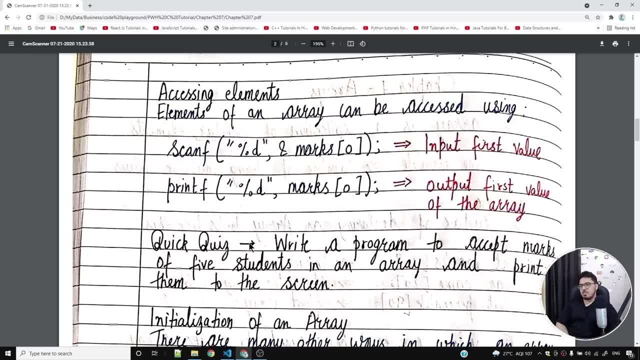 if there are 90 elements, you go till 89, which is n minus 1. 90 minus 1 is 89. okay, so we understood what array is, how this works. let's try to understand how this works. so let's try to understand how this. 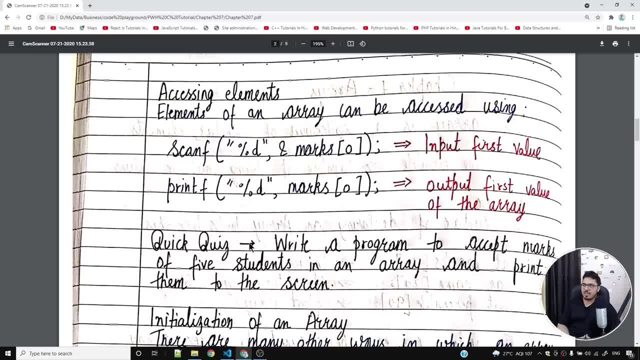 works. so let's try to understand how this works. so let's try to understand how we can assign elements. we can assign elements to an array, so elements of an array can be assigned or accessed using this, to an array, so elements of an array can be assigned or accessed using this and assigned using this. so. 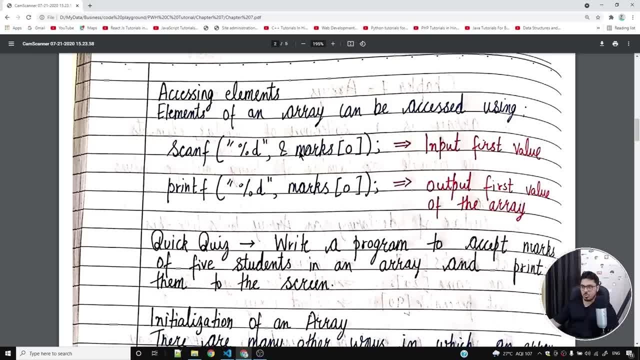 and assigned using this. so you can use scanf %t and you can say marks 0, and what this will do is: you can use scanf %t and you can say marks 0, and what this will do is this will actually uh put the. this will actually uh put the value entered by the user inside mark 0. note this ampersand sign: we. 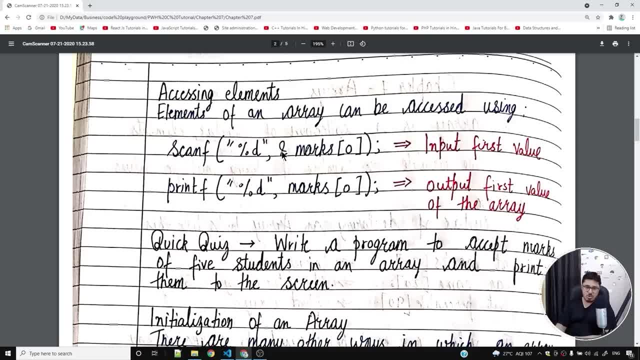 value entered by the user inside mark 0. note this ampersand sign. we are using this. you know exactly, are using this. you know, exactly like an integer variable. not even similar to an integer variable. like an integer variable. not even similar to an integer variable. exactly like an integer variable. 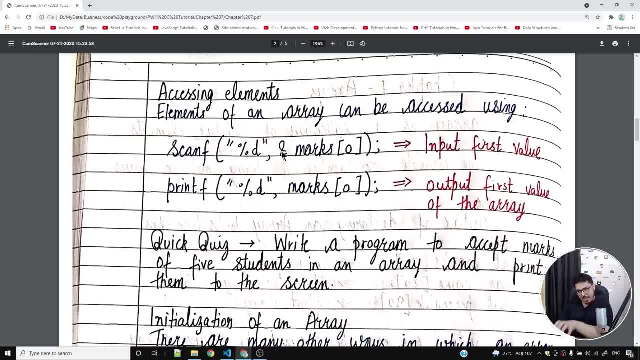 so mark 0 is like an integer variable. marks 1 is like another integer variable and we'll use amp. so mark 0 is like an integer variable. marks 1 is like another integer variable and we'll use amp percent to give the address. uh, so this is something which is important. so this is to input first value. 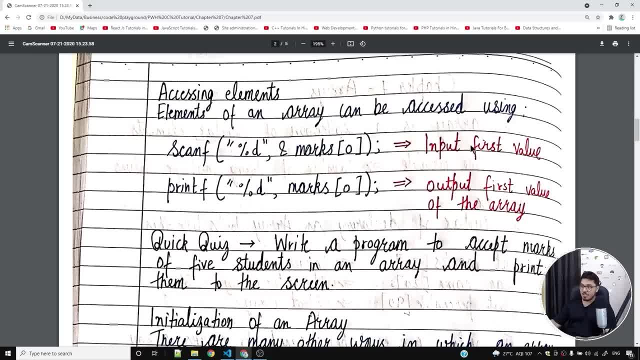 percent to give the address. uh, so this is to input first value and this is to output first value of. and this is to output first value of the array by first value because the index is starting from the array. by first value, because the index is starting from zero, so zero is the first value one. 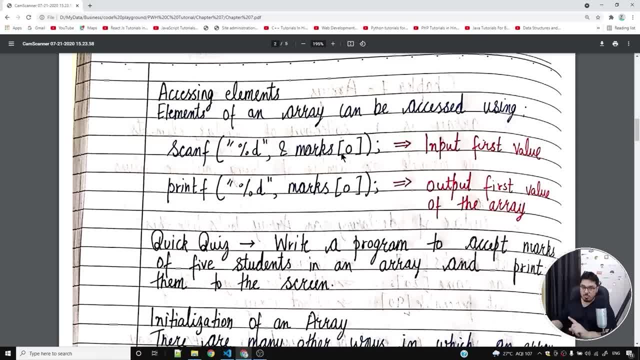 zero. so zero is the first value, one is the second value. marks two is the third value if you count is the second value. marks two is the third value if you count from zero, zero, one, two third value. so from zero, zero, one, two third value. so this is something that you need to you know, understand. 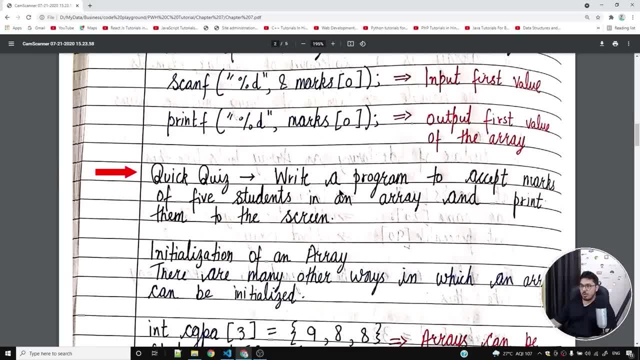 this is something that you need to you know, understand and put in your head. so, and put in your head. so now, quick quiz, quick quiz for you. write a now quick quiz. quick quiz for you. write a now quick quiz, quick quiz for you. write a program to accept marks of five students. 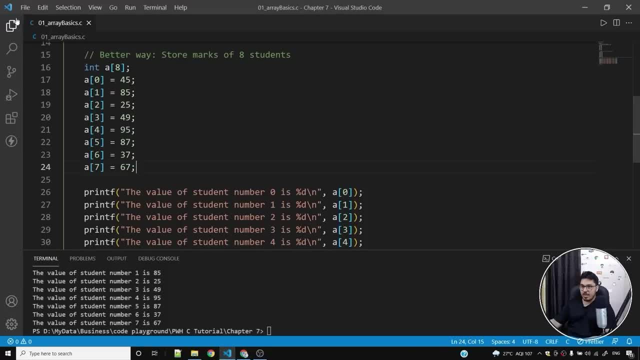 program to accept marks of five students. program to accept marks of five students in an array and print them to the screen in an array and print them to the screen in an array and print them to the screen. so let's, let's solve this quick quiz this. 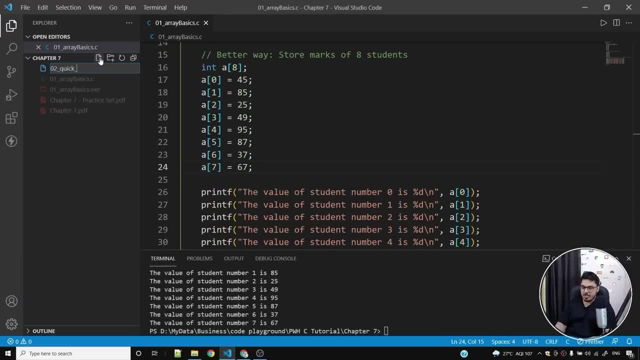 so let's, let's solve this quick quiz, this. so let's, let's solve this quick quiz. this is very interesting. so uh is very interesting. so uh is very interesting. so uh, quick quiz, quick quiz, quick quiz. oops, i forgot to write dot c. i need to. 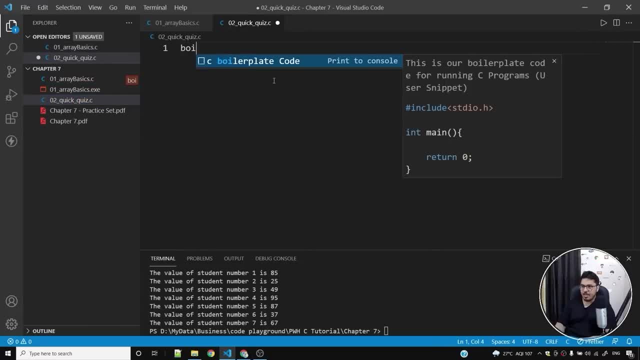 oops, i forgot to write dot c. i need to. oops, i forgot to write dot c. i need to mention the extension, then mention the extension, then mention the extension, then then i'll come here and put the boilerplate. i'll come here and put the boilerplate. 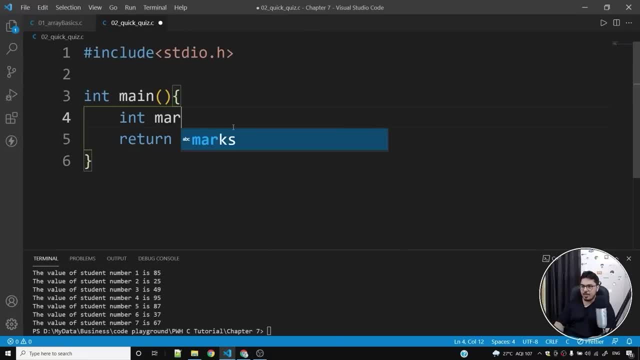 i'll come here and put the boilerplate code, and what i'll do is: i'll simply do code, and what i'll do is: i'll simply do code, and what i'll do is: i'll simply do it the old school way. it, the old school way. 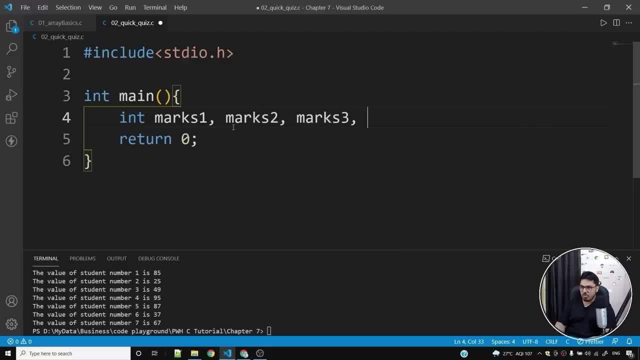 it the old school way: marks one marks two marks three marks one marks two marks three marks one marks two marks three marks four, marks four, marks four, marks five. okay, i'm doing it, the old marks five. okay, i'm doing it, the old marks five. okay, i'm doing it the old school way, just to show you. 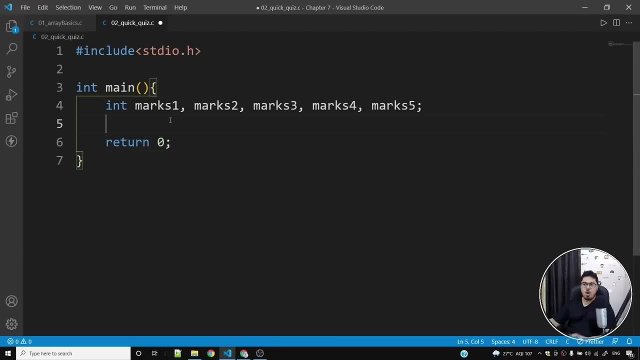 school way just to show you school way, just to show you how easy using arrays is and uh, how, how, how easy using arrays is and uh, how, how, how easy using arrays is and uh, how, how much time it saves you you'll. much time it saves you, you'll. 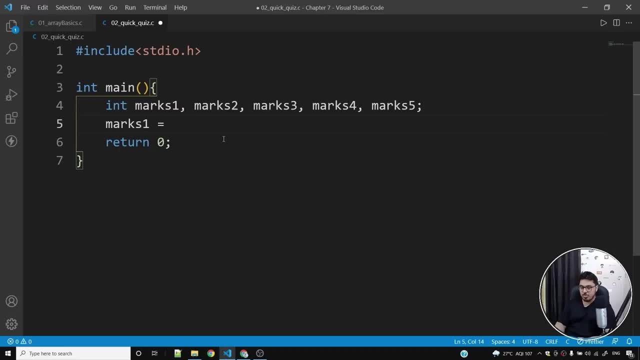 much time. it saves you. you'll get a good idea of this. so i'll say marks. get a good idea of this. so i'll say marks. get a good idea of this. so i'll say marks. one is equal to, one is equal to, one is equal to. or rather, let me use scanf function, i'll 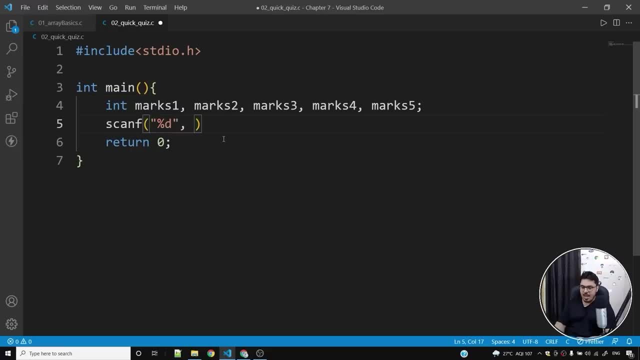 or rather, let me use scanf function. i'll, or rather let me use scanf function. i'll say scanf, say scanf, say scanf, percentage d, and i'll say amp percent percentage d, and i'll say amp percent percentage d and i'll say amp percent marks one. and also, what i'll do is: 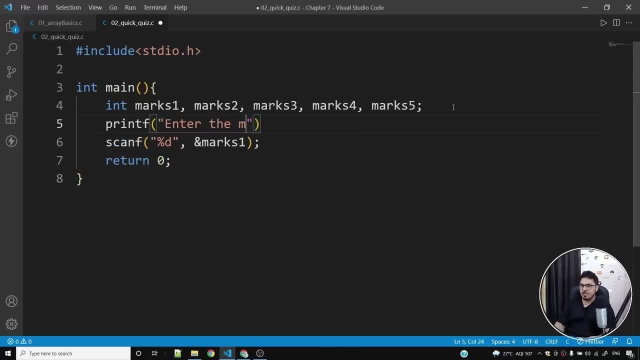 marks one, and also what i'll do is marks one. and also what i'll do is i'll say printf, i'll say printf, i'll say printf. enter the marks of. enter the marks of. enter the marks of student one. student one, student one. so, in order to enter the marks of: 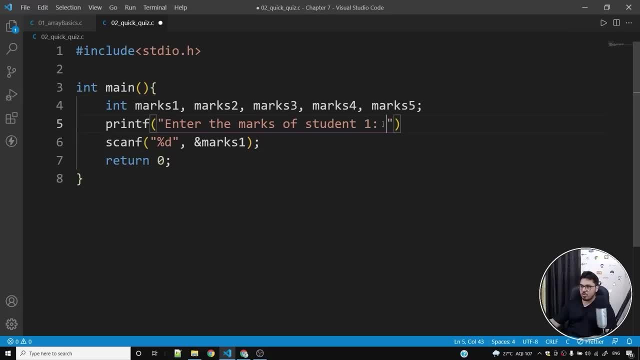 so, in order to enter the marks of, so, in order to enter the marks of student one, student one, student one, you'll enter it and also i'll put a, you'll enter it and also i'll put a, you'll enter it and also i'll put a backslash. 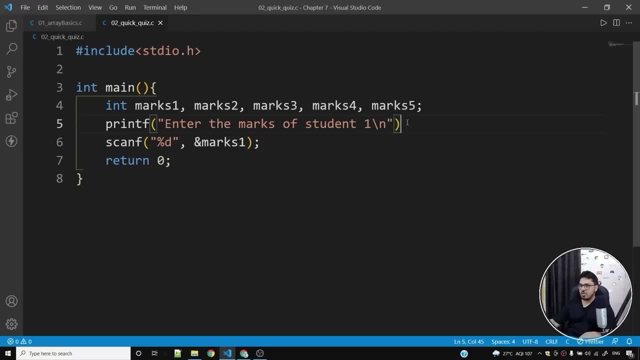 backslash, backslash n here. let me put a backslash n here, so n here. let me put a backslash n here, so n here. let me put a backslash n here, so that it looks good, that it looks good, that it looks good. do not forget the semicolon. and now what? 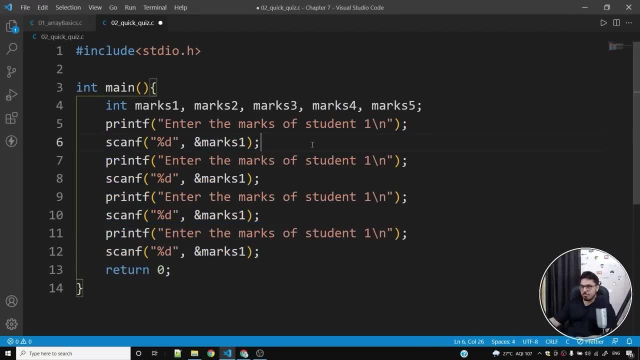 do not forget the semicolon. and now what? do not forget the semicolon. and now what i'll do, is i'll do, is i'll do, is i'll replicate this for, i'll replicate this, for, i'll replicate this for, for students one, two, three, four and 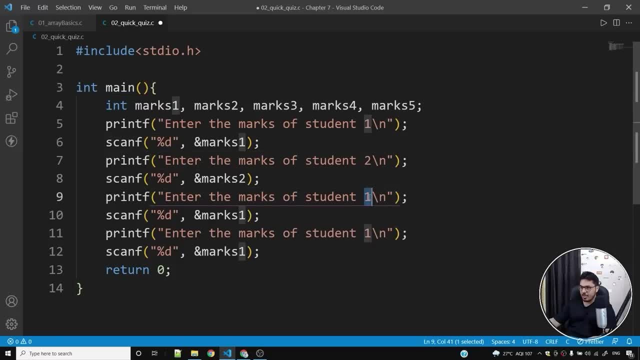 for students one, two, three, four, and for students one, two, three, four and five. so let me put two in here, five, so let me put two in here, five, so let me put two in here, three here, four here, three here, four here, three here, four here, and we need one more, which is five, and 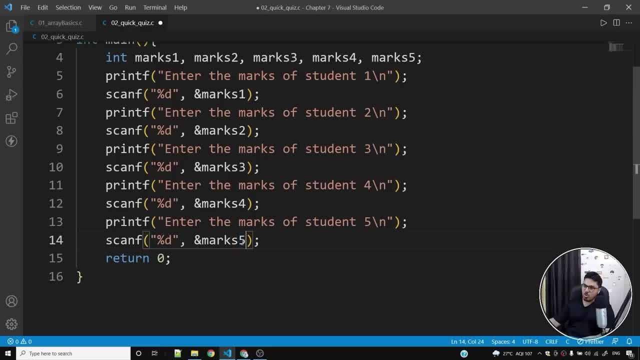 and we need one more which is five, and and we need one more which is five, and this is getting cumbersome. this is getting cumbersome. this is getting cumbersome till five. i don't know how cumbersome it till five. i don't know how cumbersome it till five. i don't know how cumbersome it will get if we have 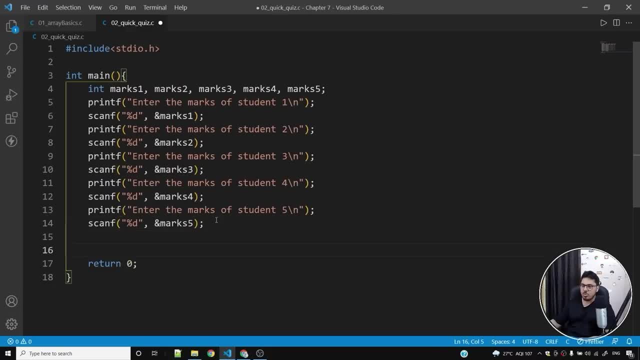 will get if we have. will get if we have 100 or 200 students, but again i'm trying 100 or 200 students, but again i'm trying 100 or 200 students, but again i'm trying to do this the old school way to show. 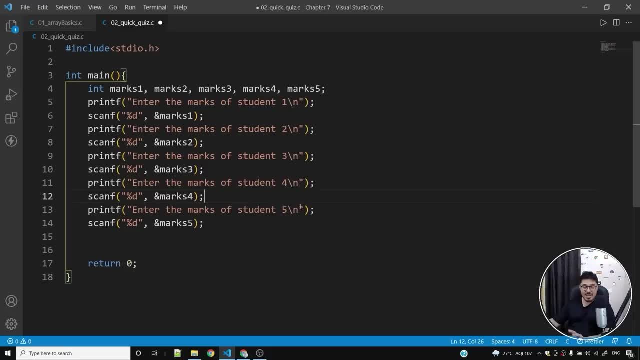 to do this the old school way to show. to do this the old school way to show you how you, how you, how, how much time the arrays are using the. how much time the arrays are using the. how much time the arrays are using the array save. array save. 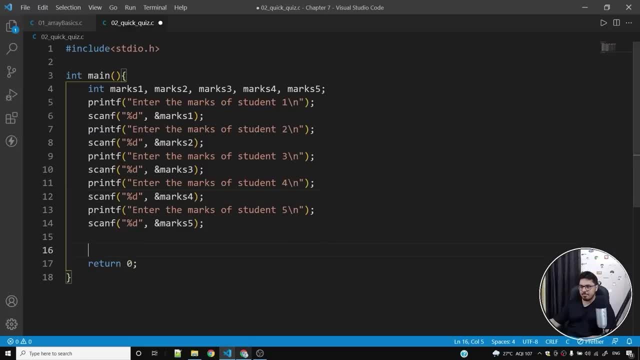 array save, so i can do the same thing i can. so i can do the same thing i can. so i can do the same thing. i can take the values and then print them on. take the values and then print them on. take the values and then print them on the screen. so i can do something like: 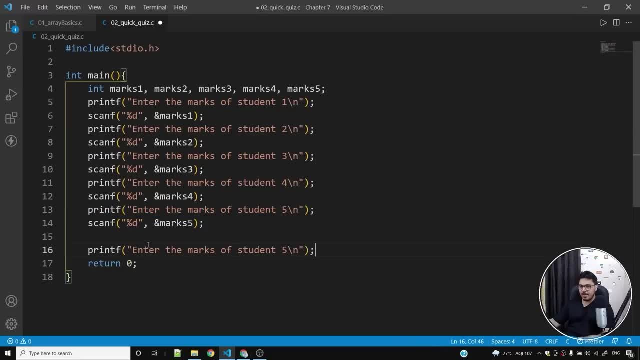 the screen so i can do something like the screen, so i can do something like this, this, this, uh, i'll say printf- the marks of, uh, i'll say printf the marks of, uh, i'll say printf the marks of the marks scored by, the marks scored by. 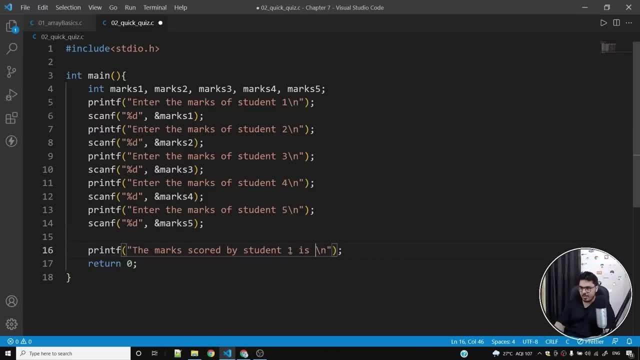 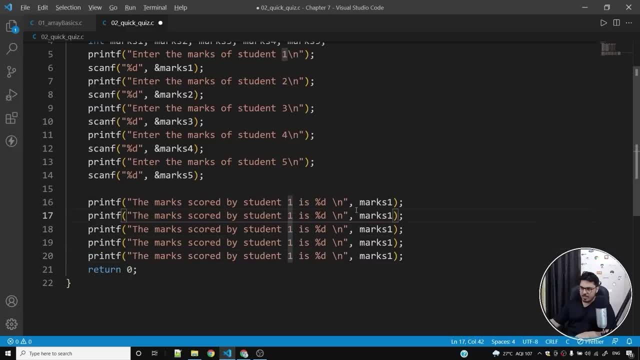 marks one, and let's do the same thing. marks one, and let's do the same thing for uh, for the five students. so what i'll for uh for the five students, so what i'll for uh for the five students. so what i'll do is i'll simply: 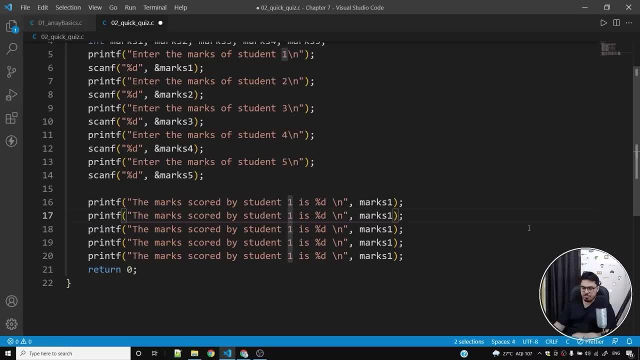 do is i'll simply do is: i'll simply use my alt key and i'll keep clicking. use my alt key and i'll keep clicking. use my alt key and i'll keep clicking wherever i want multi cursors, wherever i want multi cursors, wherever i want multi cursors, and then i'll say three, four and five. 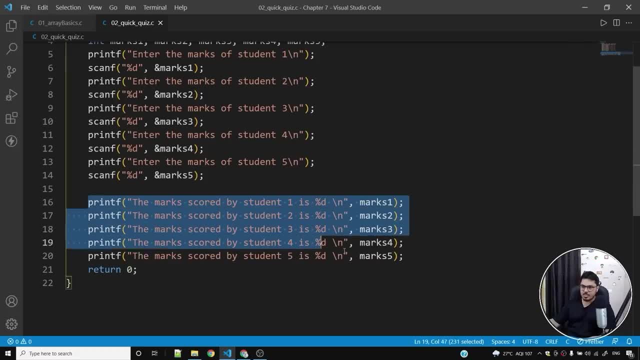 and then i'll say three, four and five, and then i'll say three, four and five. this is this is why i recommend visual. this is this is why i recommend visual. this is this is why i recommend visual studio code. because of all these studio code, because of all these. 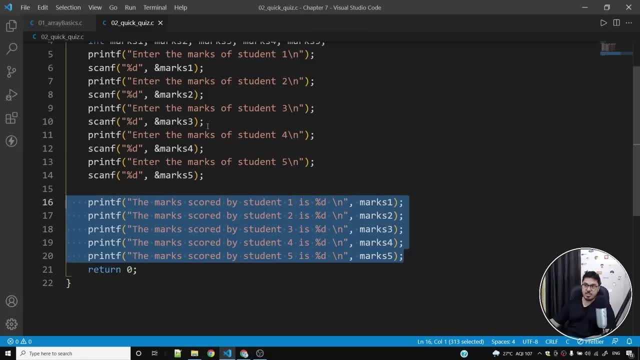 studio code, because of all these functionalities and the light code functionalities and the light code functionalities and the light code, nature, nature, nature, lightweight nature it has. because, even if lightweight nature it has, because even if lightweight nature it has, because even if you are on a computer with very low, 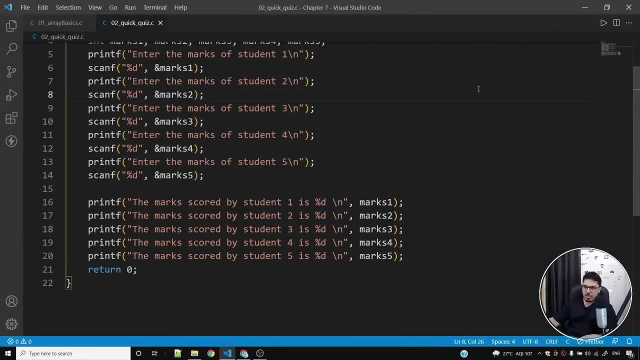 you are on a computer with very low. you are on a computer with very low memory, memory, memory. this works like a charm. so let's try to. this works like a charm. so let's try to. this works like a charm, so let's try to run this program. 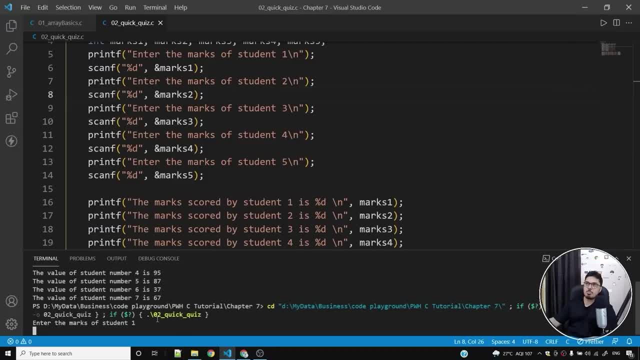 run this program. run this program. i'll run this program. so they are flying. i'll run this program. so they are flying. i'll run this program. so they are flying- a plane above my house. i don't know why- a plane above my house, i don't know why. 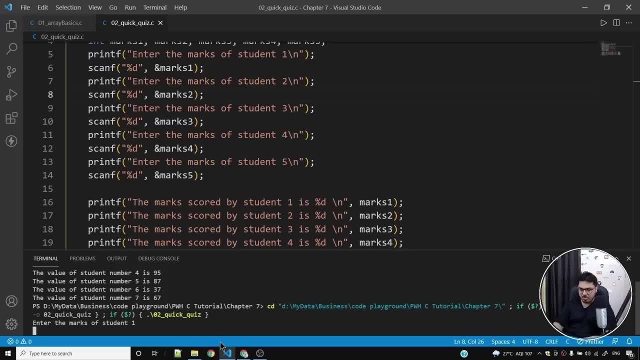 a plane above my house. i don't know why they have to fly a plane. they have to fly a plane. they have to fly a plane above my house every time. i don't know above my house every time. i don't know above my house every time. i don't know that. so let us say the marks of student. 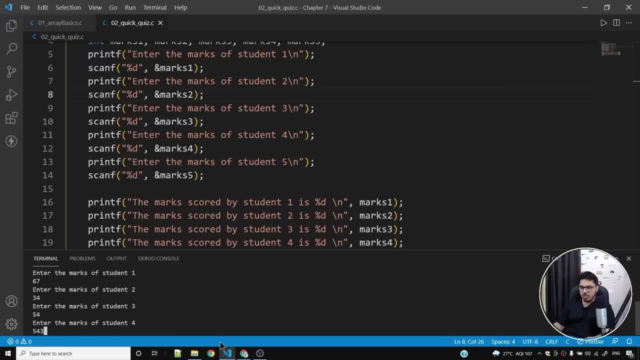 that. so let us say the marks of student, that. so let us say the marks of student. one is 67, one is 67. one is 67, 34, 54. let's make it 87, let's make the last. let's make it 87, let's make the last. 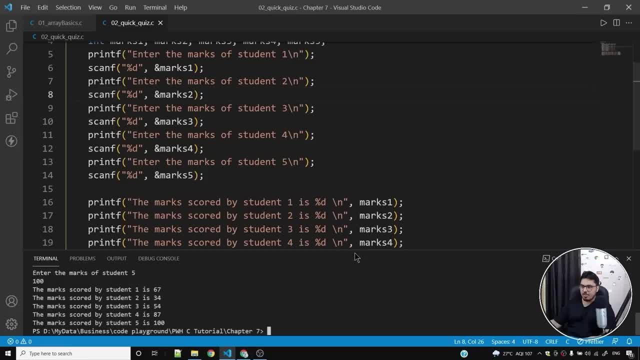 let's make it 87. let's make the last student's marks to be 100, student's marks to be 100, student's marks to be 100, and you can see all the values are and you can see all the values are and you can see all the values are printed on the screen. so this program. 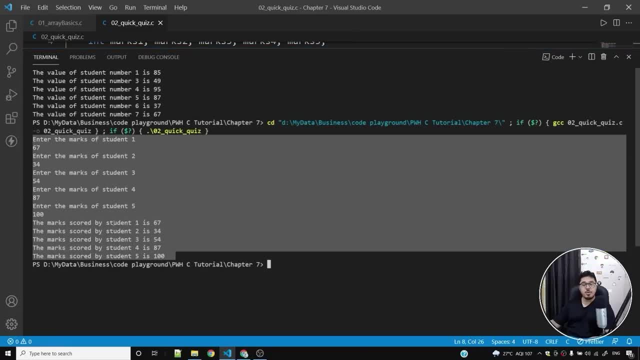 printed on the screen. so this program printed on the screen. so this program works, no surprises works, no surprises works, no surprises. but is this the best way to do? this is, but is this the best way to do? this is: but is this the best way to do this? is this the best way to achieve this? 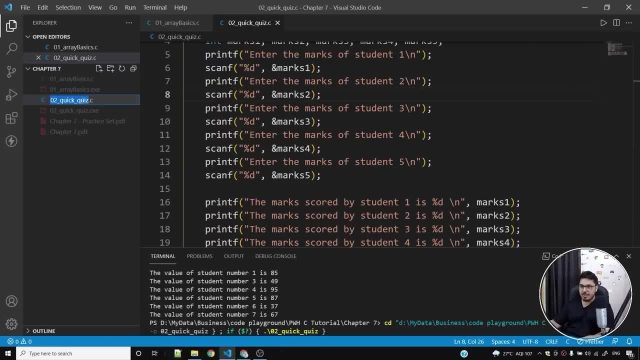 this the best way to achieve this? this the best way to achieve this, and the answer is no. so what i'll do is, and the answer is no, so what i'll do is, and the answer is no, so what i'll do is i'll. i'll rename this program to: 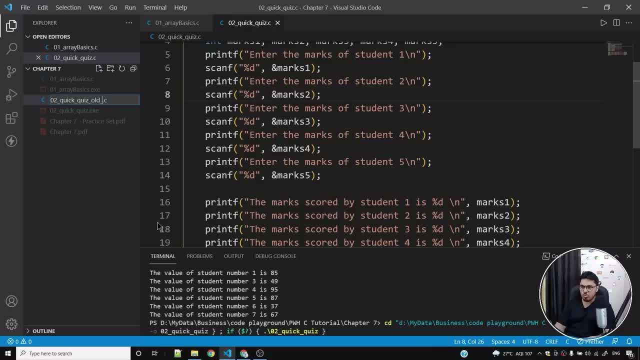 i'll. i'll rename this program to: i'll. i'll rename this program to: quick quiz underscore old school. so quick quiz underscore old school. so quick quiz underscore old school. so this is the old school way. this is the old school way. this is the old school way, and now we'll use the modern approach. 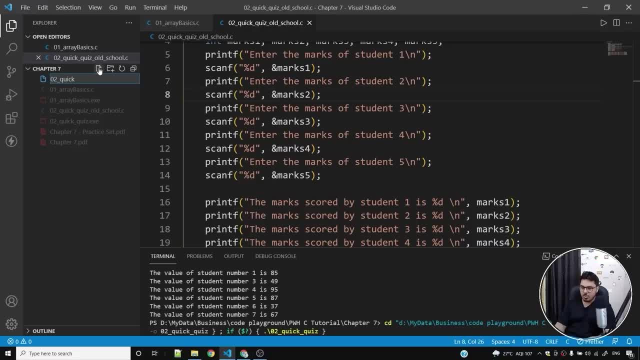 and now we'll use the modern approach. and now we'll use the modern approach to code this. so what i'll do is to code this. so what i'll do is to code this. so what i'll do is: quick quiz, better solution. so i'll say: 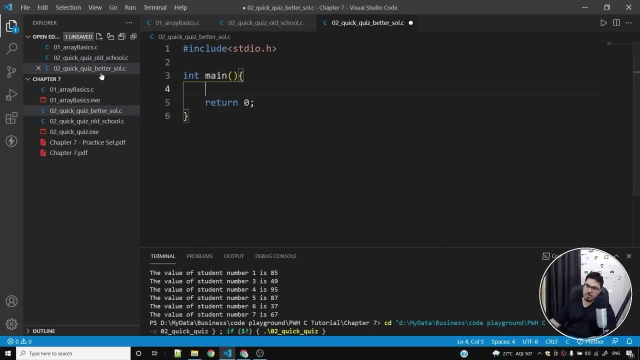 quick quiz, better solution. so i'll say quick quiz, better solution. so i'll say better solution: dot c. let me put in the better solution: dot c. let me put in the better solution: dot c. let me put in the boilerplate code: boilerplate code, boilerplate code. let me close this. and once i close this, 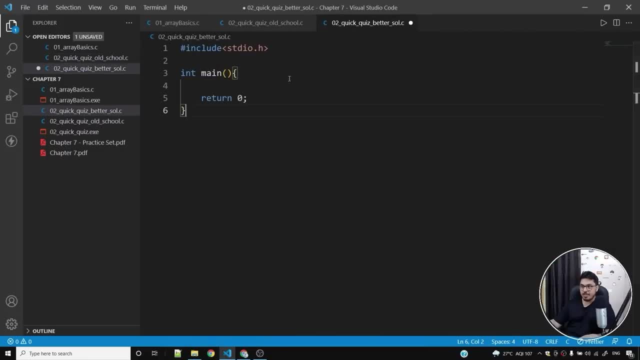 let me close this, and once i close this, let me close this and once i close this, i can actually do something like this. i can actually do something like this. i can actually do something like this. i can create an array, so firstly what. i can create an array, so firstly what. 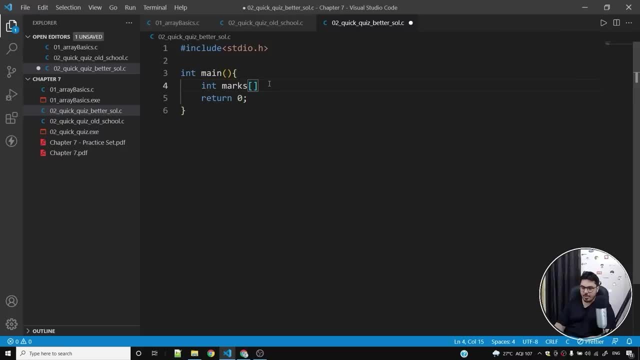 i can create an array. so, firstly, what i'll do is i'll do, is i'll do, is i'll create the marks array and how many. i'll create the marks array and how many i'll create the marks array and how many. so i'll save this program. i'll use a for. 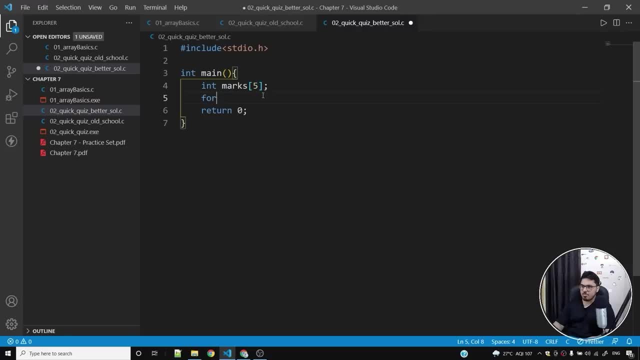 so i'll save this program. i'll use a for, so i'll save this program. i'll use a for loop. loop, loop. come on, come on c language. suggest me the. come on, come on c language. suggest me the. come on, come on c language. suggest me the for loop. 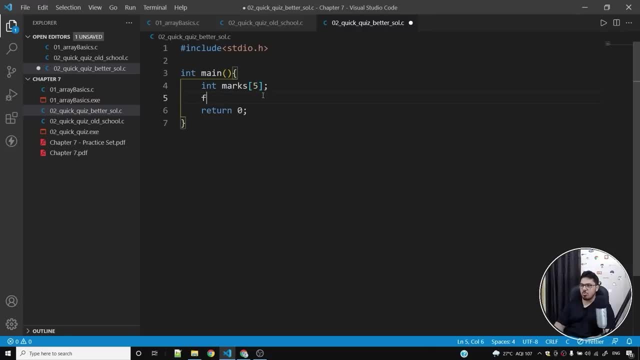 for loop, for loop. come on, you can do that. i don't know why, come on, you can do that. i don't know why, come on, you can do that. i don't know why it's not suggesting me the for loop. it's not suggesting me the for loop. 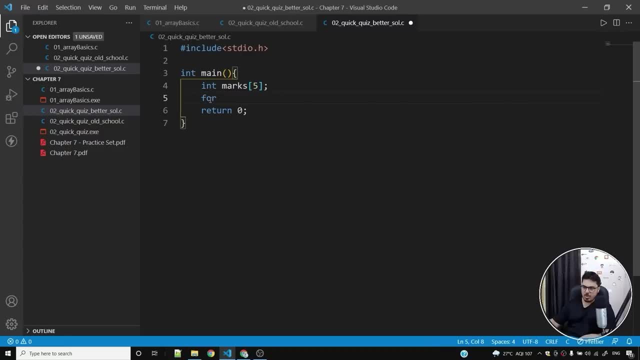 it's not suggesting me the for loop. i'm not sure i need the snippet for for. i'm not sure i need the snippet for for. i'm not sure i need the snippet for for loop. i think i forgot to. i think i forgot to. i think i forgot to turn on the c++ extension so recently. i 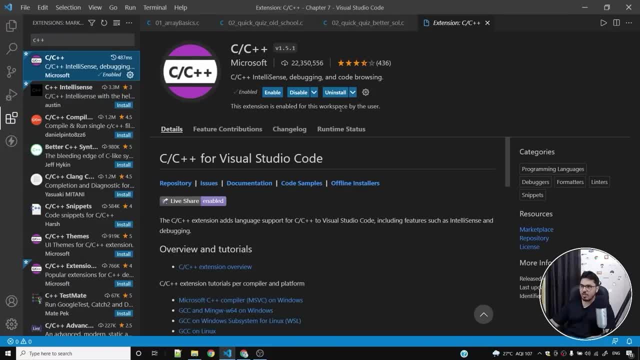 turn on the c++ extension. so recently i turn on the c++ extension. so recently i had a lot of extensions enabled, so i had a lot of extensions enabled. so i had a lot of extensions enabled. so i disabled all the extensions by default. disabled all the extensions by default. 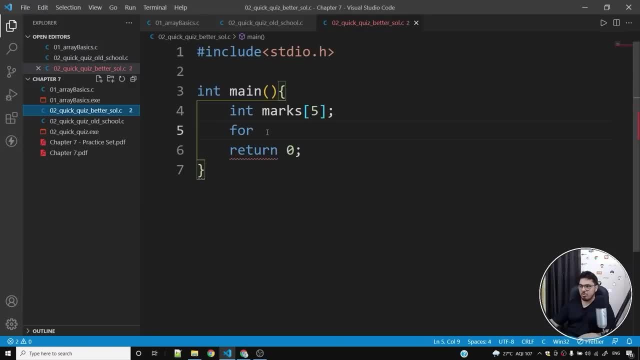 disabled all the extensions by default because, because, because it sometimes takes a lot of your, it sometimes takes a lot of your, it sometimes takes a lot of your memory. so, which is why i'm not getting the for memory, so which is why i'm not getting the for. 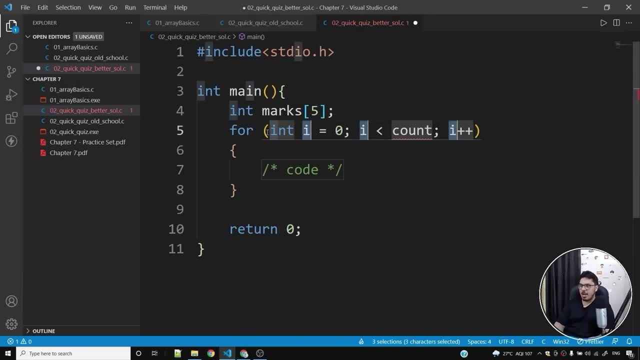 memory. so, which is why i'm not getting the for loop now i should get it. so i'm loop, now i should get it. so i'm loop, now i should get it. so i'm getting the suggestion of for loop. i'm getting the suggestion of for loop. i'm. 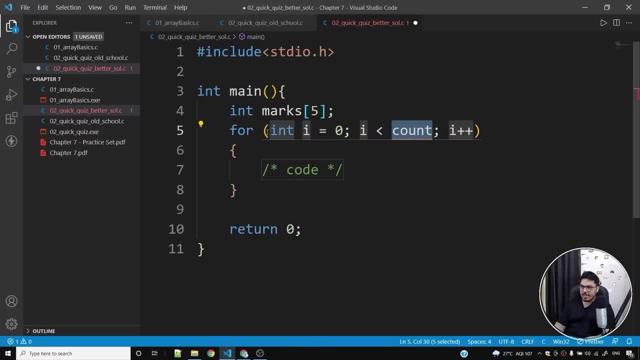 getting the suggestion of for loop. i'm saying int i is equal to zero. saying int i is equal to zero. saying int i is equal to zero. int i is equal to zero. i is less than int i is equal to zero. i is less than int. i is equal to zero. i is less than five and i plus plus. and in the code: 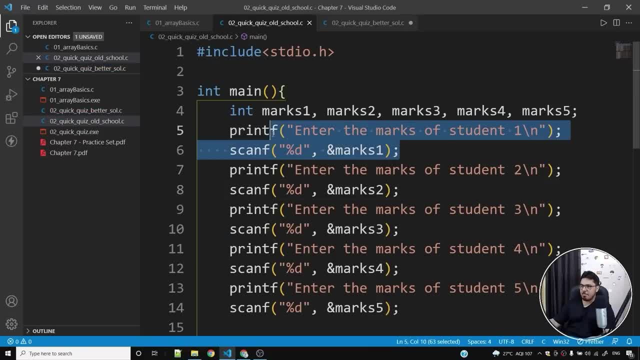 five and i plus plus and in the code: five and i plus plus. and in the code. what i'll do is i'll write the same. what i'll do is i'll write the same. what i'll do is i'll write the same thing, but i'll play a bit cleverly here. 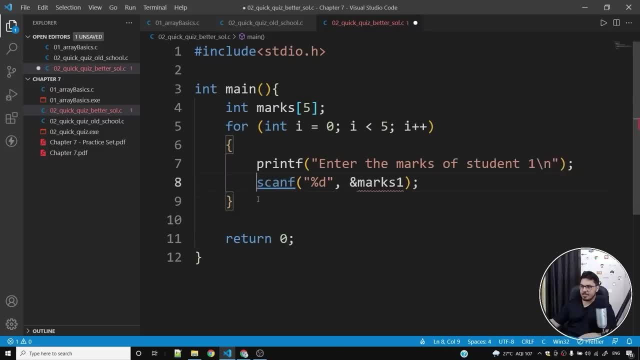 thing, but i'll play a bit cleverly here thing. but i'll play a bit cleverly here. what i'll do is what i'll do is. what i'll do is: i'll write this. i'll say: enter the marks. i'll write this. i'll say: enter the marks. 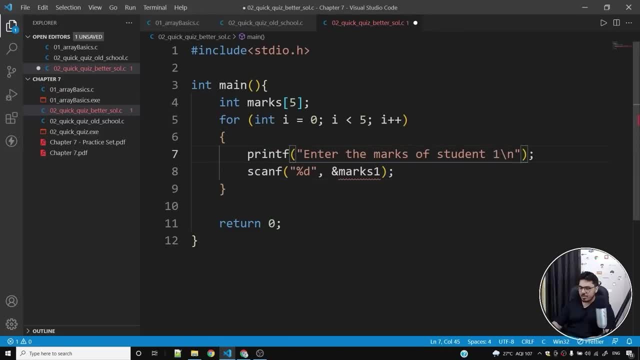 i'll write this. i'll say: enter the marks of. i'll write this. i'll say: enter the marks of: this is something that i can do. this is, this is something that i can do. this is this is something that i can do. this is totally fine valid. 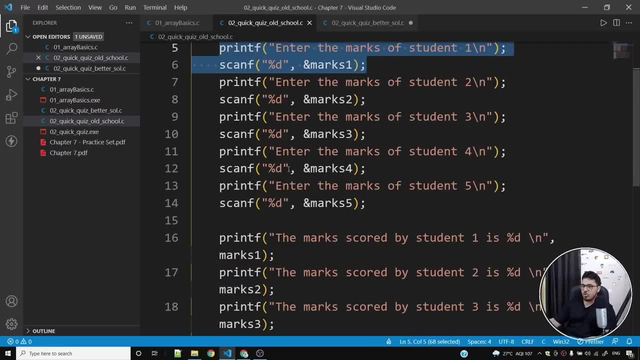 totally fine, valid. totally fine, valid. no surprises there. and i can use another- no surprises there. and i can use another- no surprises there. and i can use another for loop to print the marks. so i can do for loop to print the marks, so i can do for loop to print the marks. so i can do something like this, so i can say: 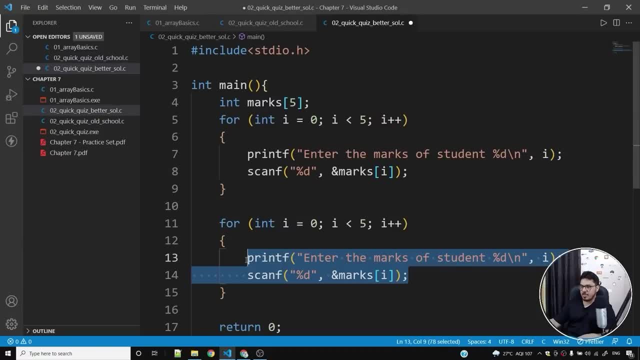 something like this, so i can say something like this, so i can say: the marks scored by this student is the marks scored by this student, is the marks scored by this student, is this, is, this, is this is, and also. instead of saying marks one and also. instead of saying marks one. 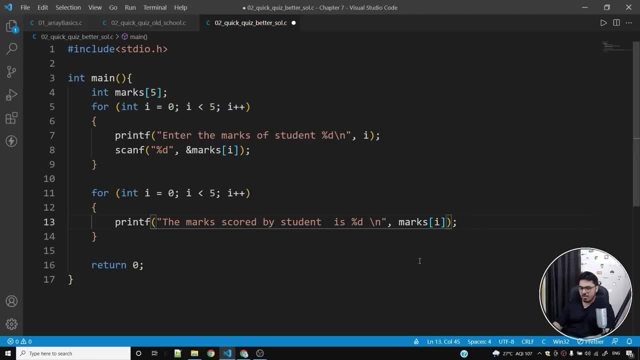 and also, instead of saying marks one, i can say marks i here, and instead of i can say marks i here, and instead of i can say marks i here. and instead of saying, saying, saying student one, i can say percentage d, student one, i can say percentage d. 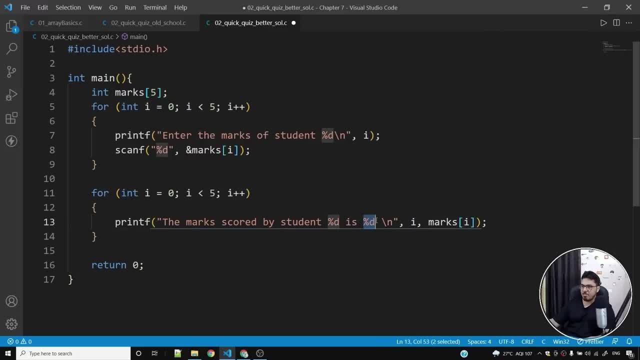 student one, i can say percentage d, and this percentage d maps to this i, and. and this percentage d maps to this i, and. and this percentage d maps to this i. and this percentage d maps to this max i. this percentage d maps to this max i. this percentage d maps to this max i. in a very similar way, this percentage d. 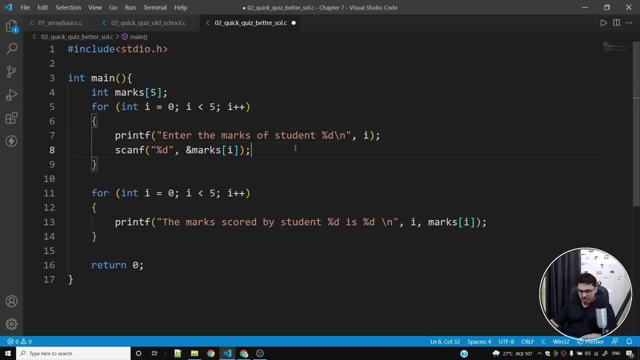 in a very similar way, this percentage d in a very similar way, this percentage d marks to this, i marks to this, i marks to this. i and scan f everything works. this program and scan f everything works. this program and scan f everything works. this program should work. 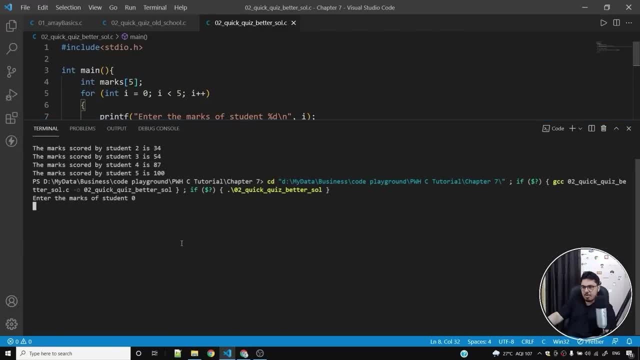 should work, should work, let's try to run this program. and yes, let's try to run this program. and yes, let's try to run this program. and yes, it's asking me for the marks of student. it's asking me for the marks of student. it's asking me for the marks of student zero. what i'll try to do is: i'll try to. 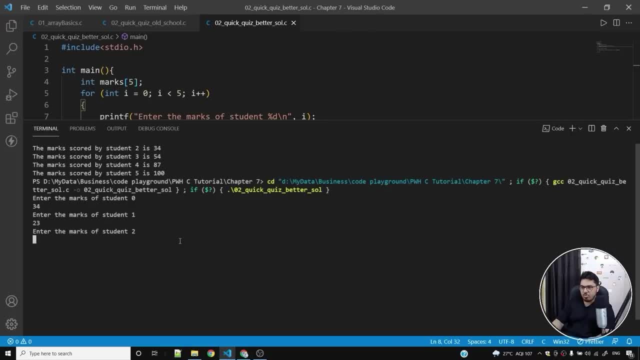 zero. what i'll try to do is: i'll try to zero. what i'll try to do is i'll try to put the same marks. put the same marks. put the same marks. or let me use 34 23 then, or let me use 34 23 then. 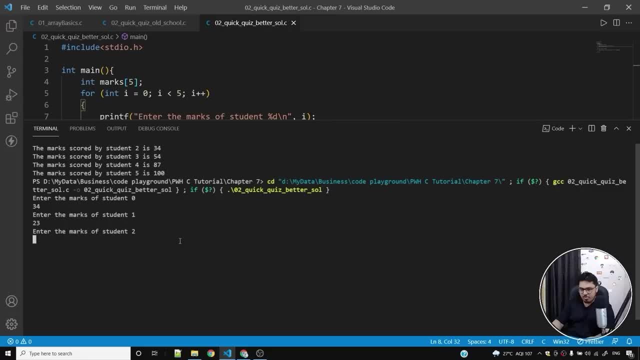 or let me use 34, 23, then we have 30, 54, 54, we have 30, 54, 54, we have 30, 54, 54, and then 87, and then 87, and then 87 and 100. okay, so you can see that this. 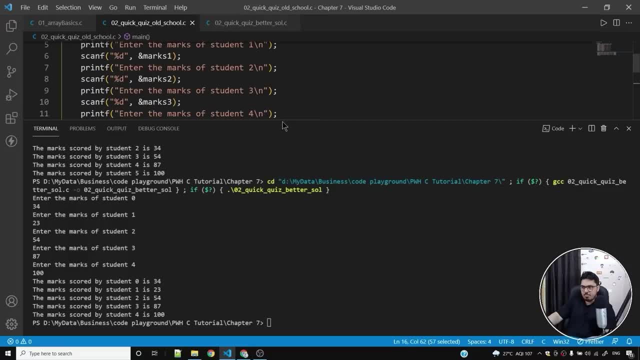 and 100. okay, so you can see that this and 100. okay, so you can see that this program behaves in a very similar way. program behaves in a very similar way. program behaves in a very similar way to this program and writing this program to this program and writing this program was 22 lines of code writing this: 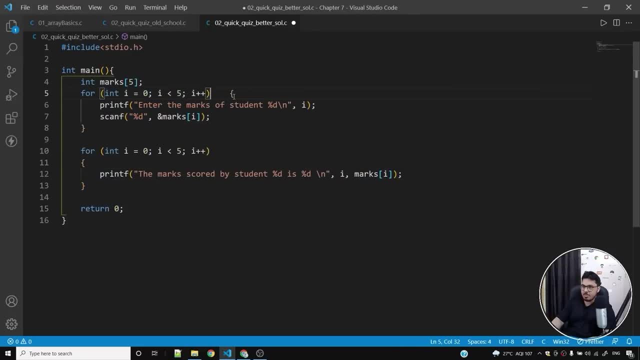 was 22 lines of code. writing. this was 22 lines of code. writing. this program was actually 17 lines of code. program was actually 17 lines of code. program was actually 17 lines of code, but even less than that because you know. but even less than that because you know. 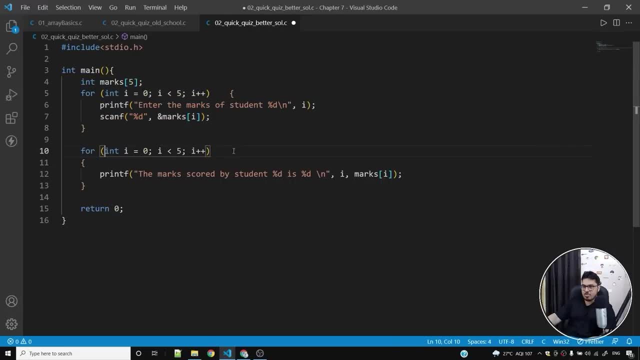 but even less than that, because you know we are using a for loop and we are using a for loop and we are using a for loop and we used some new lines here. so if i we used some new lines here, so if i we used some new lines here, so if i try to get rid of all these new lines and 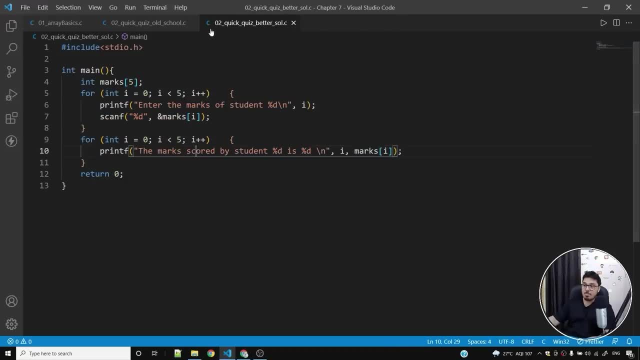 try to get rid of all these new lines. and try to get rid of all these new lines and show you, you'll see that you show you, you'll see that you show you, you'll see that you maintaining this program is very easy. so, maintaining this program is very easy, so. 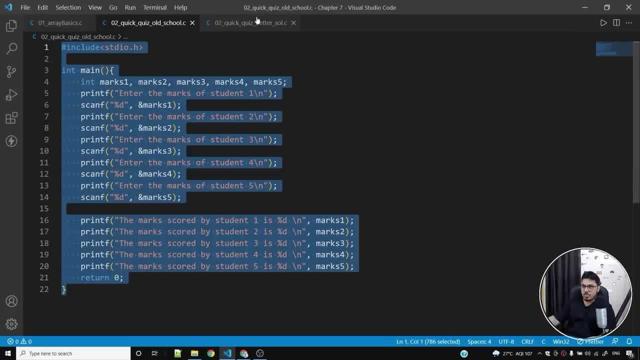 maintaining this program is very easy. so if this was 21 lines of code, if this was 21 lines of code, if this was 21 lines of code, 22 lines of code. this is just 13 lines. 22 lines of code. this is just 13 lines. 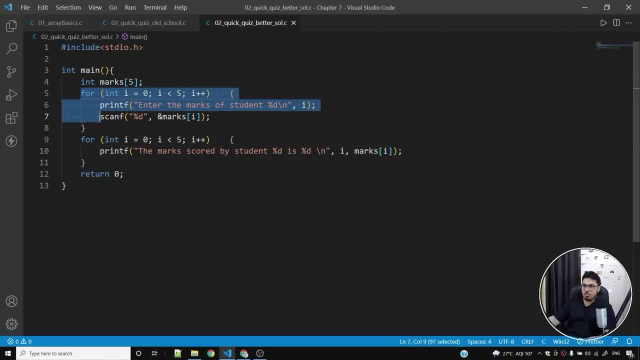 22 lines of code. this is just 13 lines of code and maintaining it is super of code and maintaining it is super of code and maintaining it is super simple because we just have two for simple, because we just have two for simple, because we just have two for loops here. look at this and look at this. 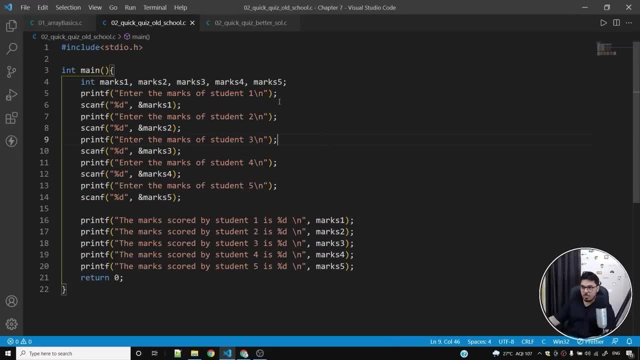 loops here, look at this and look at this. loops here, look at this and look at this. and this program is small. i mean just 22, and this program is small. i mean just 22. and this program is small. i mean just 22 lines of code, because we have only five. 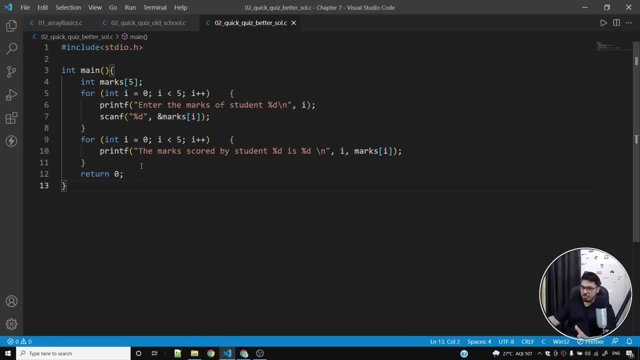 lines of code, because we have only five lines of code, because we have only five variables- variables, variables- this program is capable of handling. this program is capable of handling. this program is capable of handling thousand variables, maintaining the same thousand variables, maintaining the same thousand variables, maintaining the same lines of code. so this program is much. 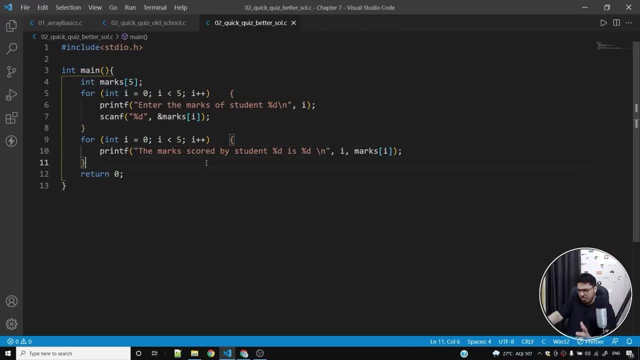 lines of code. so this program is much lines of code. so this program is much better using for loops and using arrays, better using for loops and using arrays, better using for loops and using arrays. so so, so many of you might think that why are we? many of you might think that why are we? 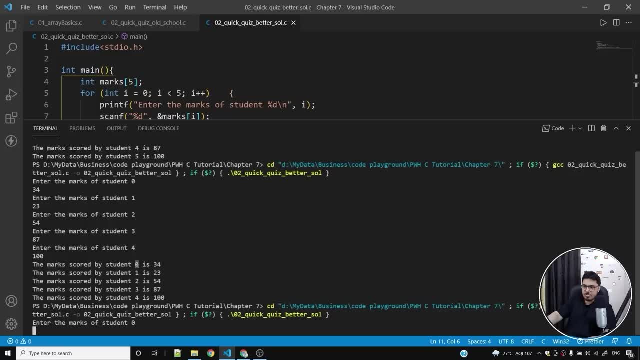 many of you might think that why are we using student zero? why are we not saying using student zero? why are we not saying using student zero? why are we not saying student one here? why did we say student student one here? why did we say student student one here? why did we say student zero? if you want student one here, you can. 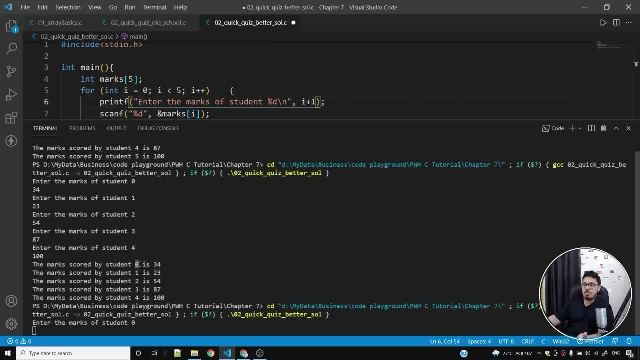 zero. if you want student one, here you can zero. if you want student one, here you can print i plus one, print i plus one and actually store the value of and actually store the value of and actually store the value of student one in mark zero. student two in: 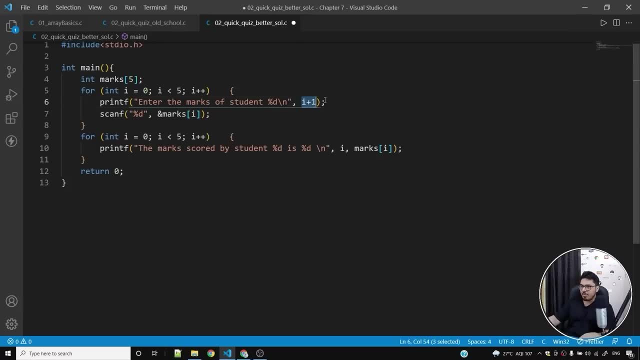 student one in mark zero, student two in student one in mark zero, student two in marks one, and so on, marks one and so on, marks one and so on. so let me cancel this, let me save this, so let me cancel this. let me save this, so let me cancel this. let me save this program and show you this works. 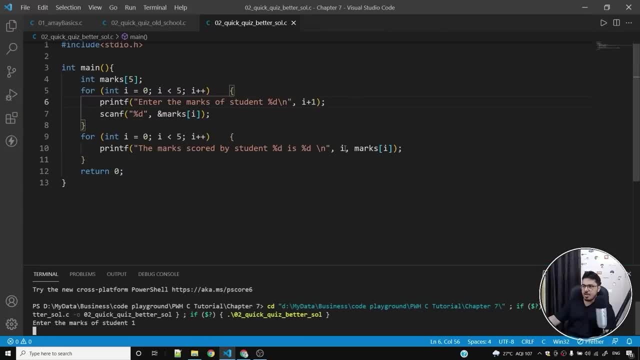 program and show you this works program and show you this works and this will say marks of student one is, and this will say marks of student one is, and this will say marks of student one is this, student two is this, but i'll also this. student two is this, but i'll also. 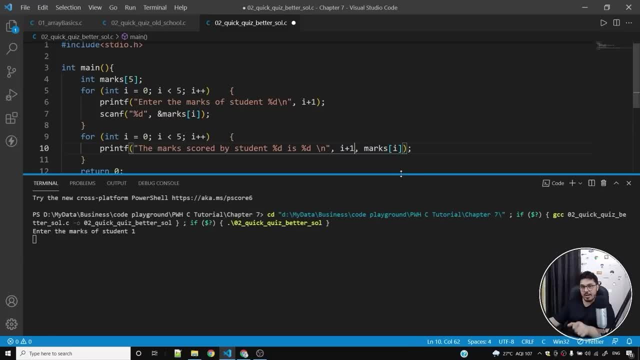 this student. two is this, but i'll also print. i plus one here because i want it print. i plus one here because i want it print. i plus one here because i want it to go from one to five and not from zero, to go from one to five and not from zero. 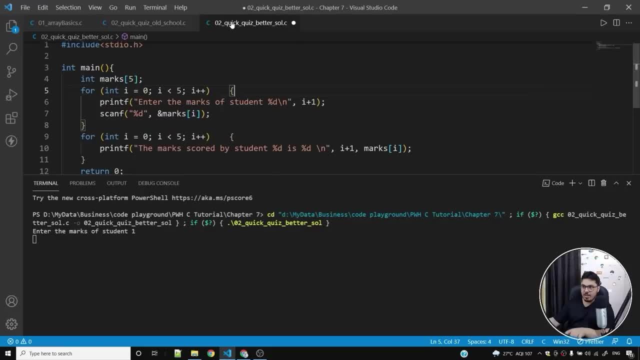 to go from one to five and not from zero to four. so i'll use i plus one here to four. so i'll use i plus one here to four. so i'll use i plus one here. so this program and this program will. so this program and this program will. 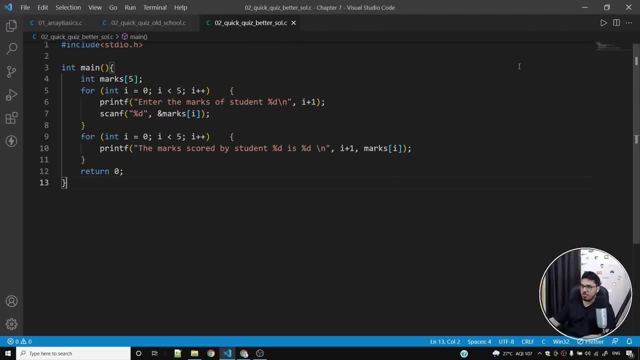 so this program and this program will exactly run, exactly, run, exactly, run, uh, with the same output. okay, so let me uh with the same output. okay, so let me uh with the same output. okay, so let me run this for you and let me show you i'll. 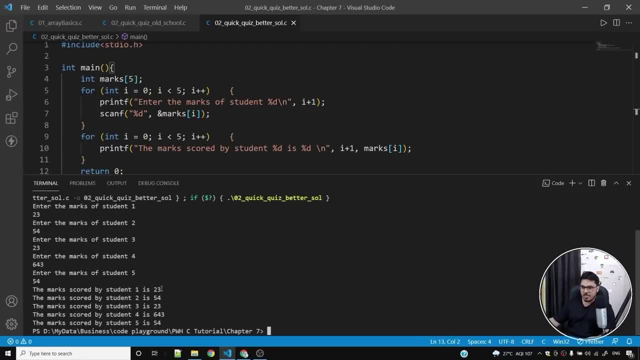 run this for you and let me show you. i'll run this for you and let me show you. i'll simply punch in some random values, simply punch in some random values. simply punch in some random values. so you can see that the. so you can see that the. 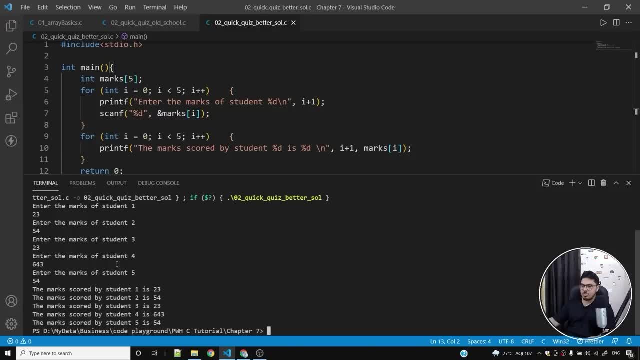 so you can see that the marks scored by strength. what is this marks scored by strength. what is this? marks scored by strength. what is this two? is this three, four, five, two? is this three, four, five, two? is this three, four, five? so this program works in an exactly the 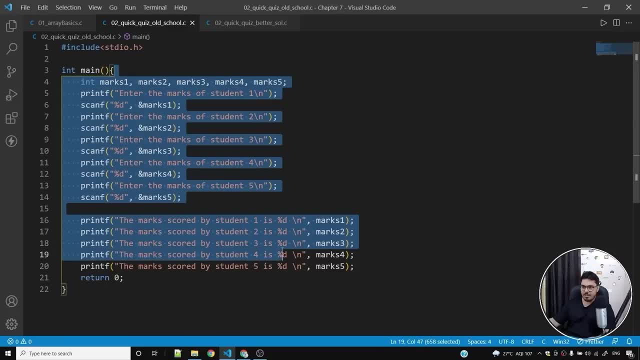 so this program works in an exactly the. so this program works in an exactly the same way as this program, same way as this program, same way as this program, the difference being that here, the, the difference being that here, the, the difference being that here the program is not maintainable. i'll show. 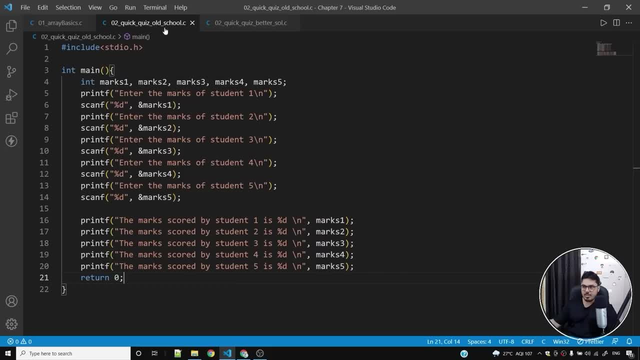 program is not maintainable. i'll show program is not maintainable. i'll show you an example of how you, an example of how you, an example of how this program is not maintainable, why this program is not maintainable, why this program is not maintainable, why this old school program is. 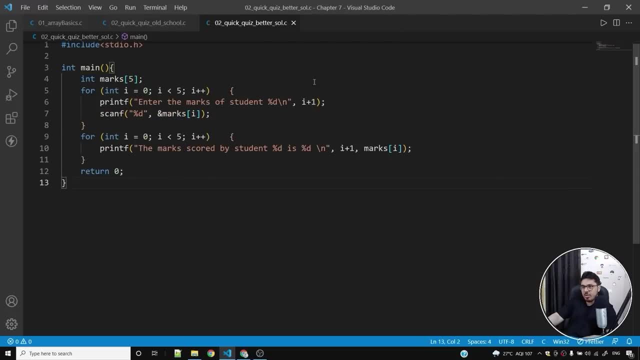 this old school program is. this old school program is even more worse than it looks like. so, even more worse than it looks like. so, even more worse than it looks like. so let us say i want to change. let us say i want to change. let us say i want to change the marks to enter the score of student. 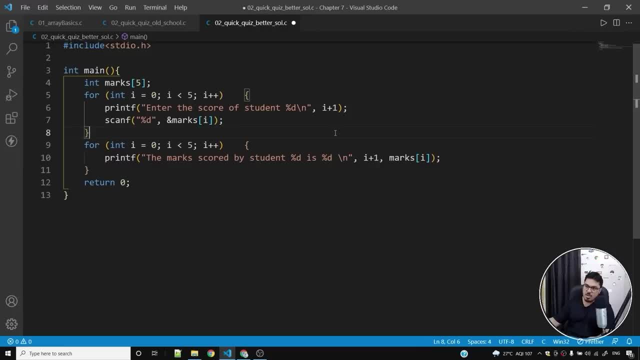 the marks to enter the score of student. the marks to enter the score of student. let us say somebody instructed me to use. let us say somebody instructed me to use. let us say somebody instructed me to use the word score and not marks, the word score and not marks. 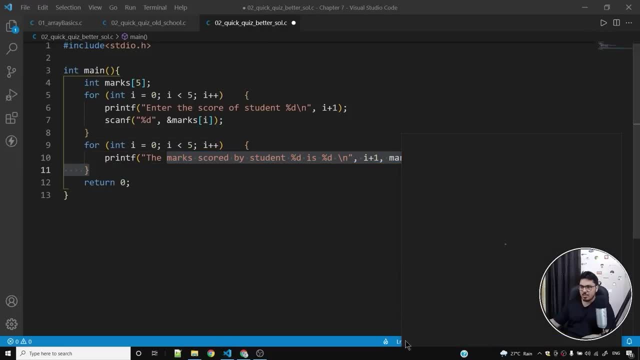 the word score and not marks, so i'll use oops. i'll use score. i'll use oops. i'll use score. i'll use oops. i'll use score. i'll use score scored by student percentage d. i'll use score scored by student percentage d. 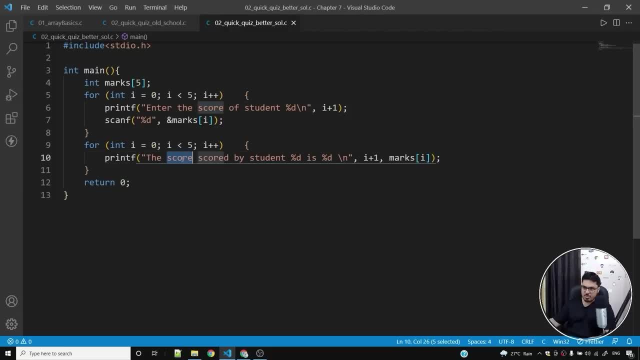 i'll use score scored by student. percentage d is percentage d, so here i just need to is percentage d. so here i just need to is percentage d. so here i just need to change these two lines and, if i run, change these two lines and if i run. 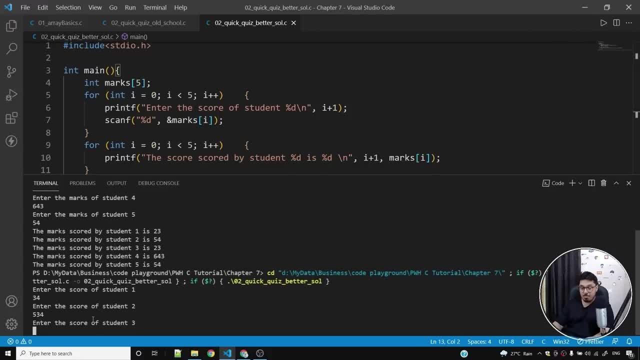 change these two lines and if i run all the lines will say score instead of all the lines, will say score instead of all the lines. will say score instead of mask. mask mask marks- okay. so if i do something like this, marks okay. so if i do something like this: 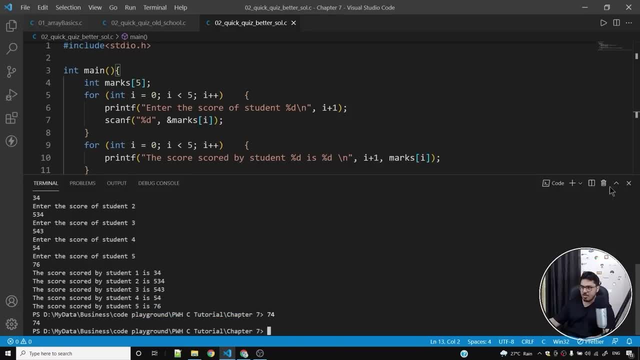 marks. okay. so if i do something like this, you'll see that all the values are now. you'll see that all the values are now. you'll see that all the values are now saying score and not marks. saying score and not marks. saying score and not marks. but if i was to change the same thing, 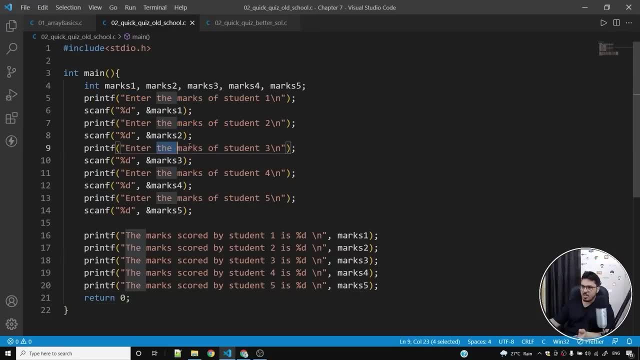 but if i was to change the same thing, but if i was to change the same thing here, i'll have to actually go to each here. i'll have to actually go to each here. i'll have to actually go to each and every line and change, and every line and change. 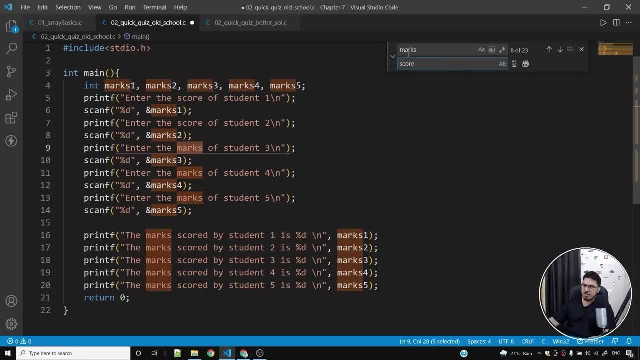 and every line and change this to score. but here is another, this to score, but here is another, this to score. but here is another problem. if i try to change these marks- problem. if i try to change these marks problem. if i try to change these marks to score, these variables will also get. 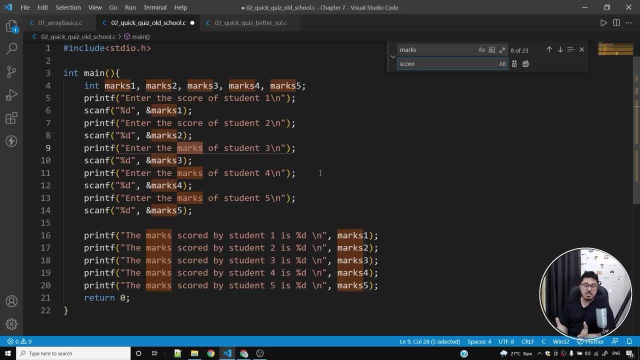 to score. these variables will also get to score. these variables will also get changed and there might be something in changed and there might be something in changed and there might be something in the program which might get changed, the program which might get changed, the program which might get changed accidentally, and i might get into. 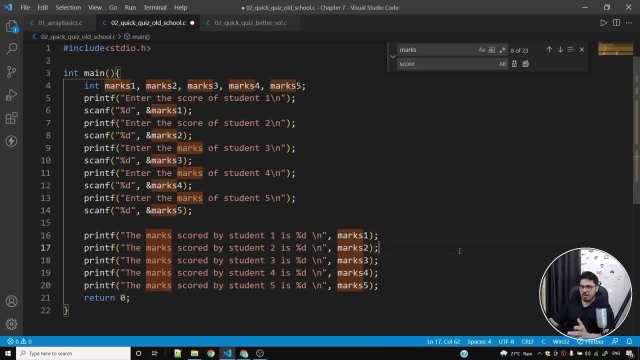 accidentally and i might get into accidentally and i might get into trouble. so i don't want to write program trouble. so i don't want to write program trouble. so i don't want to write program this way. okay, this is the gist of it, this way. okay, this is the gist of it. 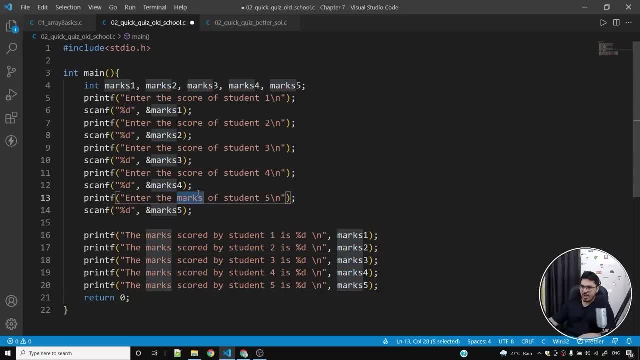 this way. okay, this is the gist of it. yes, i can always use some automated. yes, i can always use some automated. yes, i can always use some automated means to means to means to do, find and replace, but here the number. do find and replace, but here the number. 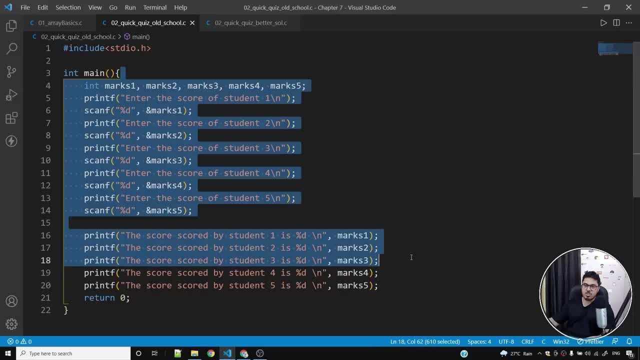 do find and replace, but here the number of variables is really very of variables is really very of variables is really very uh small, which is five, but if you have uh small, which is five, but if you have uh small, which is five, but if you have, say, 20 variables or 30 variables, or 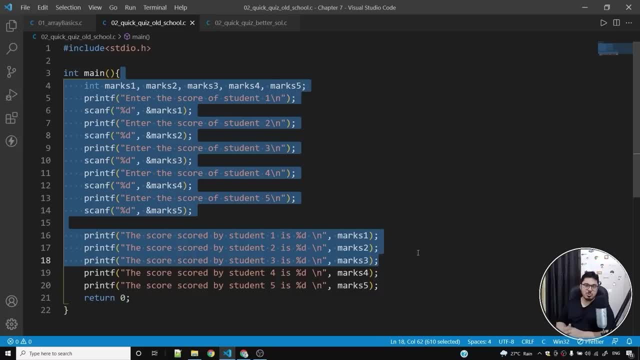 say 20 variables or 30 variables, or say 20 variables or 30 variables, or even 1800, for that matter. how will you even 1800, for that matter? how will you even 1800, for that matter? how will you maintain the code? 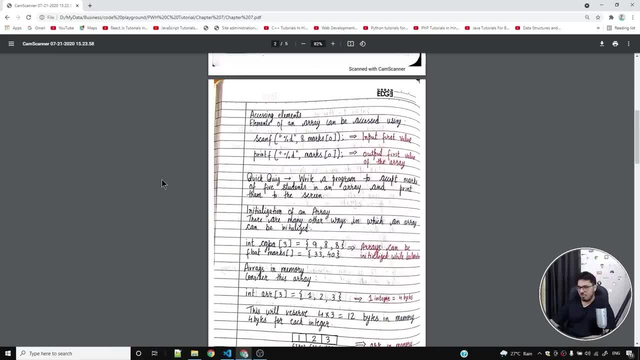 maintain the code. maintain the code. so this is why arrays are actually very so. this is why arrays are actually very so. this is why arrays are actually very useful, so useful. so this is why arrays are actually very useful. so we spent quite a good amount of time. 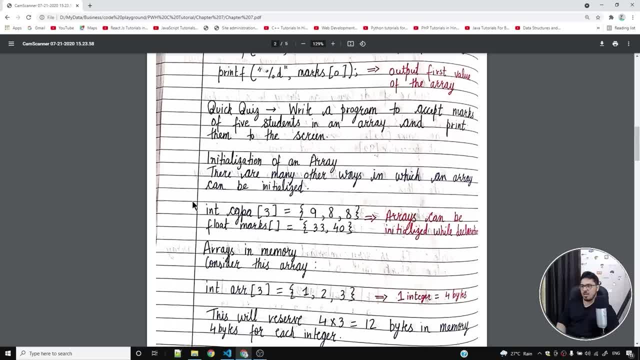 we spent quite a good amount of time. we spent quite a good amount of time in this quick quiz, but i hope that you in this quick quiz, but i hope that you in this quick quiz, but i hope that you understood how this understood, how this understood, how this uh syntax works and why arrays are. 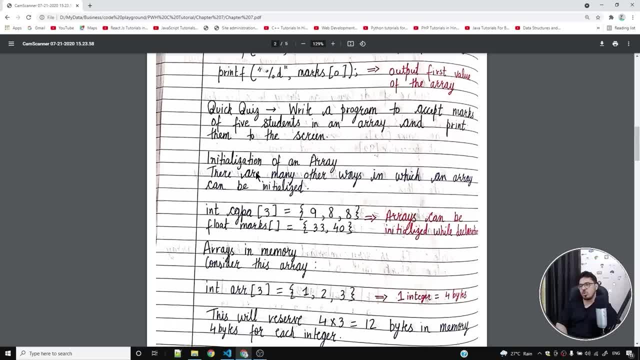 uh syntax works and why arrays are- uh syntax works and why arrays are helpful, okay, helpful, okay, helpful, okay, let's talk about initialization of an. let's talk about initialization of an. let's talk about initialization of an array. what are the ways to initialize an array? what are the ways to initialize an? 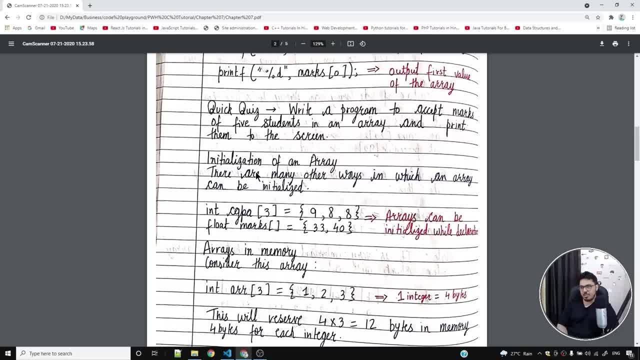 array. what are the ways to initialize an array? so there are many other ways in array. so there are many other ways in array. so there are many other ways in which an array can be initialized. a lot which an array can be initialized. a lot which an array can be initialized. a lot of ways can be used to initialize an. 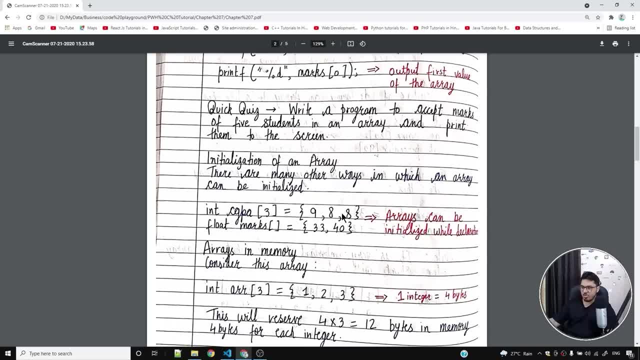 of ways can be used to initialize an of ways can be used to initialize an array. so if you look at this in cgpa3 is array. so if you look at this in cgpa3 is array. so if you look at this in cgpa3 is equal to nine, eight and eight. this is. 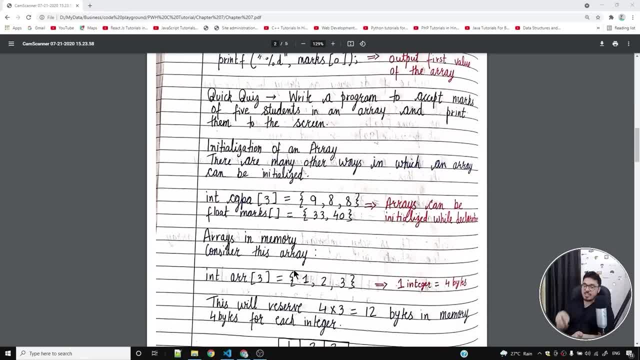 equal to nine, eight and eight. this is equal to nine, eight and eight. this is nothing but a very quick way to nothing, but a very quick way to nothing, but a very quick way to initialize arrays. so if you say in initialize arrays, so if you say in: 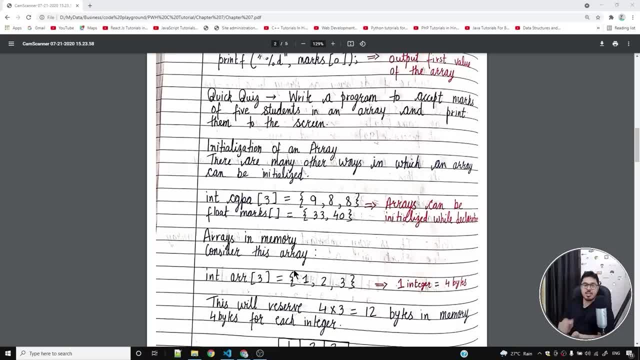 initialize arrays. so if you say in cgpa3 is equal to 988, it's going to say cgpa3 is equal to 988. it's going to say cgpa3 is equal to 988. it's going to say cgpa0 is 9, cgpa1 is 8. 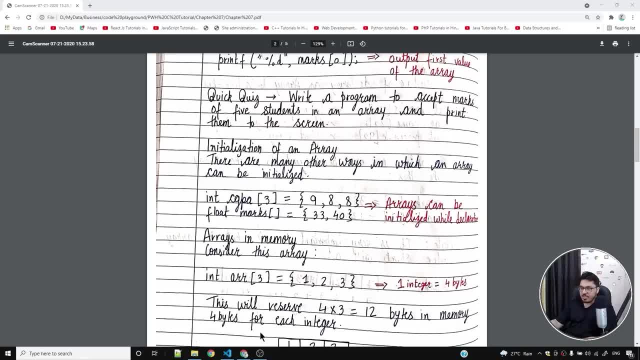 cgpa0 is 9, cgpa1 is 8, cgpa0 is 9, cgpa1 is 8, and it will set cgpa2 to 8 once again, and it will set cgpa2 to 8 once again, and it will set cgpa2 to 8 once again. so let's try the syntax, let's create a. 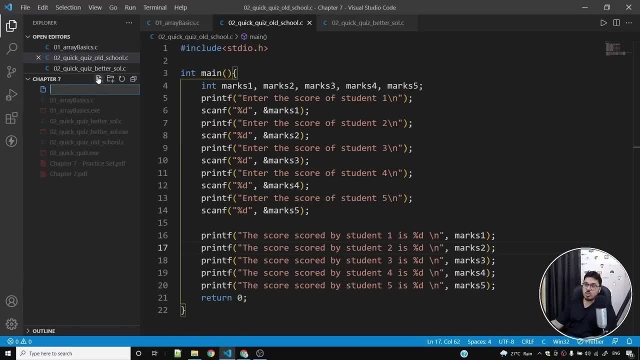 so let's try the syntax. let's create a. so let's try the syntax. let's create a program, program, program. and i'm going to call this program as. and i'm going to call this program as: and i'm going to call this program as initialization of. 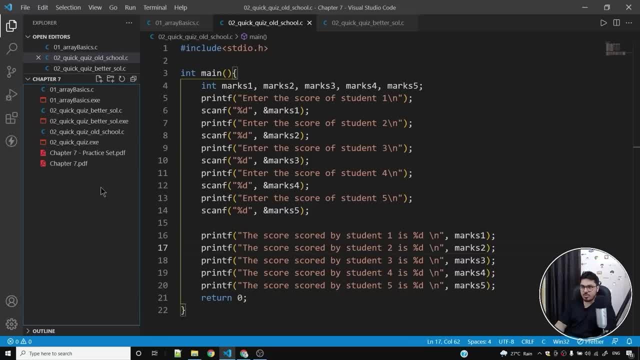 initialization of initialization of array. so i'll say initialize arrayc array. so i'll say initialize arrayc array. so i'll say initialize arrayc. i'll put in the boilerplate code. i'll put in the boilerplate code. i'll put in the boilerplate code. note that i have named this program as: note that i have named this program as. note that i have named this program as two and this s2 as well, because these two and this s2 as well, because these two and this s2 as well, because these are the same problems- are the same problems. 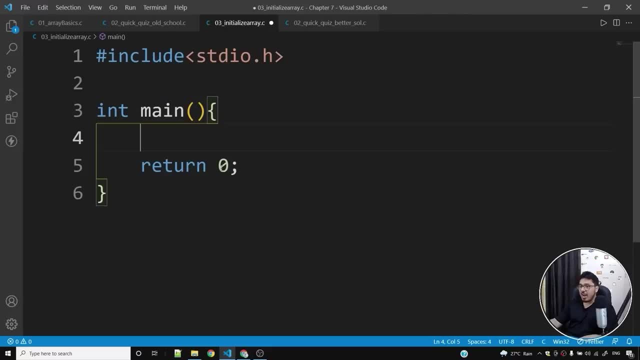 are the same problems, uh solved using different approaches. so uh solved using different approaches. so uh solved using different approaches. so let's try to create an array called, let's try to create an array called, let's try to create an array called marks, and let's try to use this syntax. 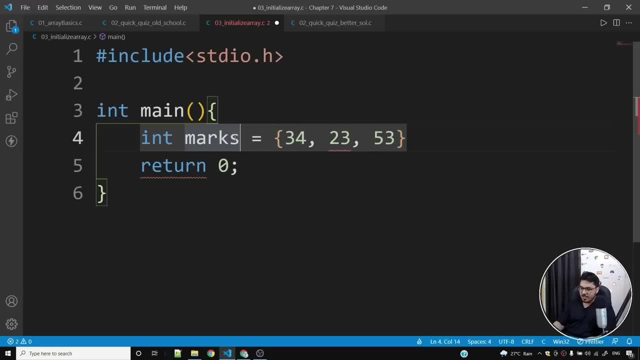 marks, and let's try to use this syntax marks, and let's try to use this syntax uh. and let's say the marks is uh, and let's say the marks is uh, and let's say the marks is an array of three marks, and let's see if 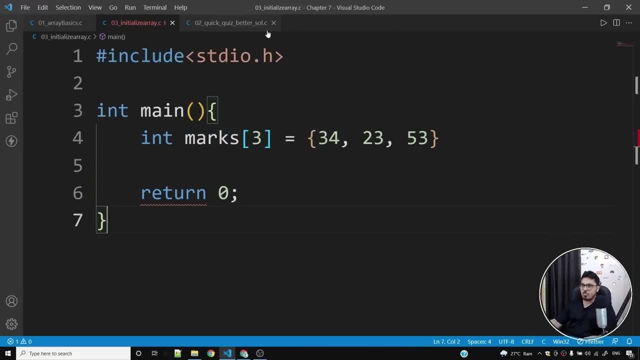 an array of three marks and let's see if an array of three marks and let's see if the syntax works. so what i'll do is the syntax works. so what i'll do is the syntax works. so what i'll do is i'll come back to my this index. i'll 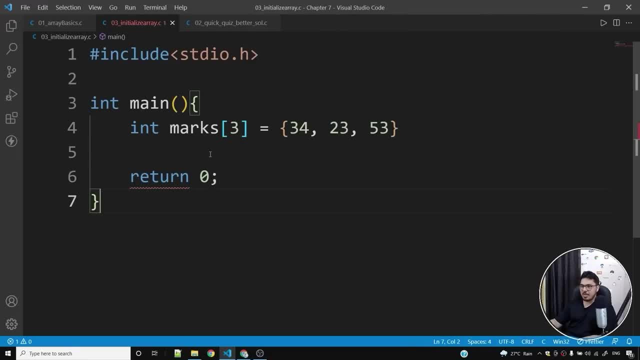 i'll come back to my this index. i'll i'll come back to my this index. i'll copy this for loop, and what i'll do is copy this for loop, and what i'll do is copy this for loop, and what i'll do is i'll simply paste this code in here and 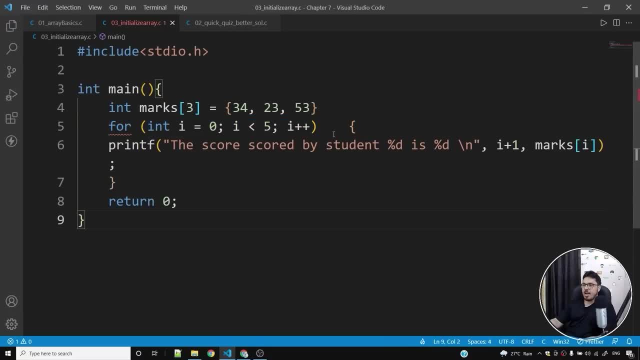 i'll simply paste this code in here, and i'll simply paste this code in here and i'll simply format this. i'll simply format this. i'll simply format this like this, and what i'll do now is like this, and what i'll do now is: 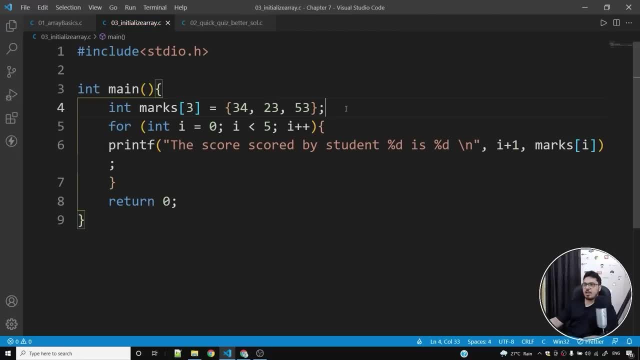 like this, and what i'll do now is simply, i'll use a semicolon here i have. simply, i'll use a semicolon here i have. simply, i'll use a semicolon here. i have made a mistake, i am not using semicolon. made a mistake, i am not using semicolon. 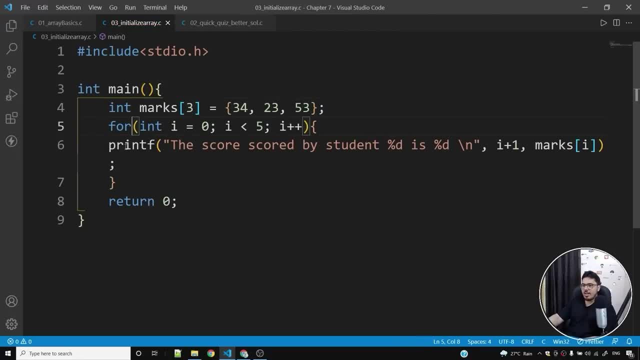 made a mistake. i am not using semicolon here, here, here, which is why it was throwing some error, which is why it was throwing some error, which is why it was throwing some error. so now, what i'll do is so, now, what i'll do is. so, now, what i'll do is i'll simply fix my indents. and now what? 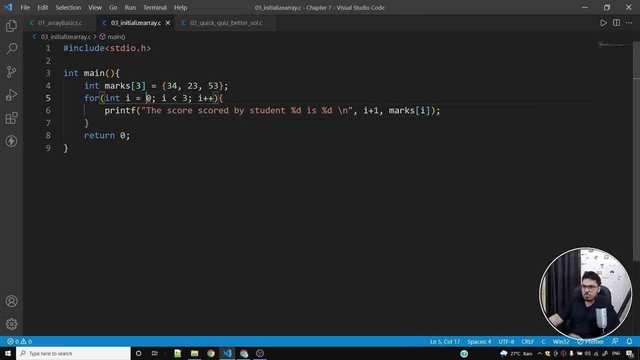 i'll simply fix my indents. and now what? i'll simply fix my indents. and now what i'll do is i'll simply put in three. i'll do is i'll simply put in three. i'll do is i'll simply put in three years, so that the value of i goes from. 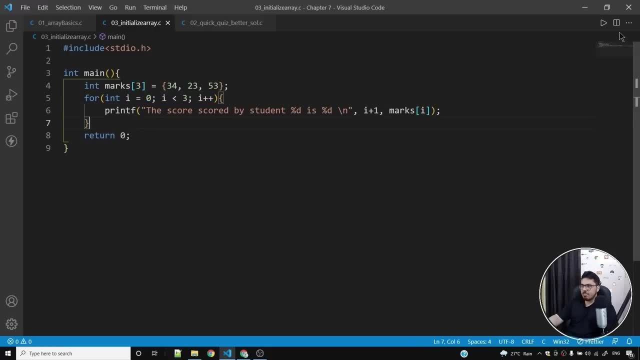 years, so that the value of i goes from years, so that the value of i goes from zero one and two. and let's see if it is zero one and two, and let's see if it is zero one and two, and let's see if it is printing the correct values of marks. 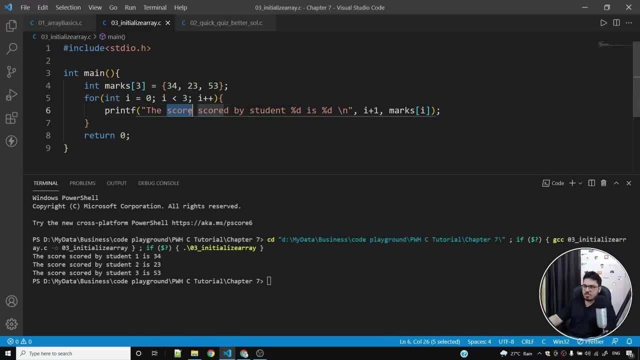 printing the correct values of marks, printing the correct values of marks. so it is indeed printing the correct. so it is indeed printing the correct, so it is indeed printing the correct value of marks. value of marks, value of marks. so i'll call it marks and not score. so 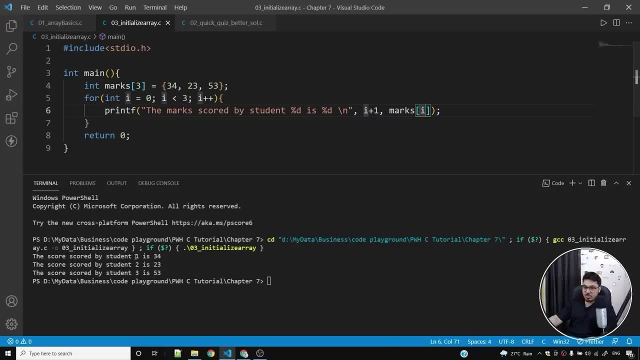 so i'll call it marks and not score. so so i'll call it marks and not score. so i'll say the mark scored by student. i'll say the mark scored by student. i'll say the mark scored by student. this is this which is certain. one is 34. 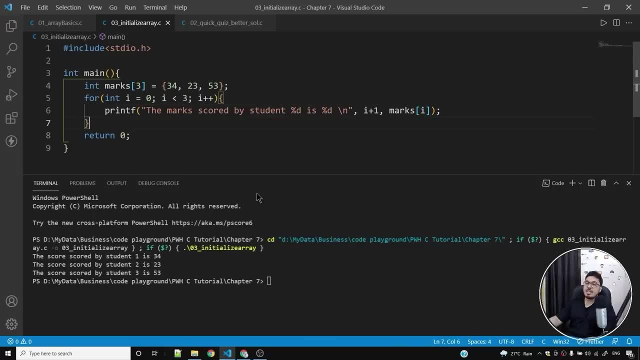 this is this which is certain. one is 34. this is this which is certain. one is 34. 2 is 23, 3 is 53. so this is indeed printing the correct 53. so this is indeed printing the correct 53. so this is indeed printing the correct values of marks. 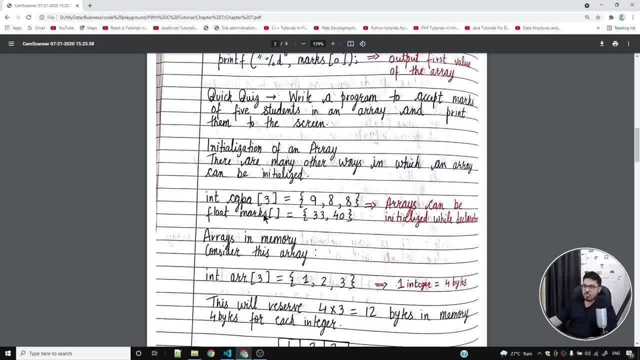 values of marks. values of marks: now. let us try this syntax. let us try now. let us try this syntax. let us try now. let us try this syntax. let us try uh float instead of int, and definitely uh float instead of int, and definitely uh float instead of int, and definitely i'll have to use percentage. 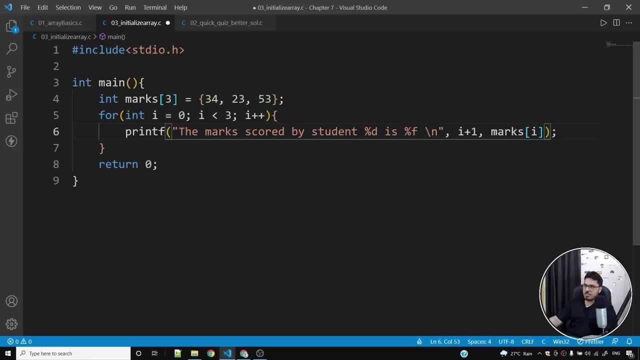 i'll have to use percentage. i'll have to use percentage f instead of this percentage d, because f instead of this percentage d, because f instead of this percentage d, because this value will be a floating point. this value will be a floating point. this value will be a floating point number. 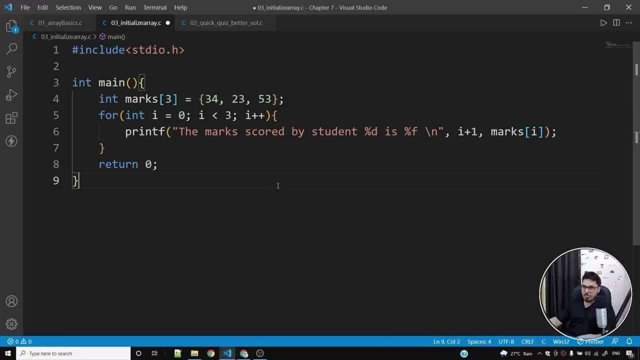 number, number. make sure that this is percentage d. make sure that this is percentage d. make sure that this is percentage d, because index is always going to be an, because index is always going to be an, because index is always going to be an integer. okay, so i'll simply make this: 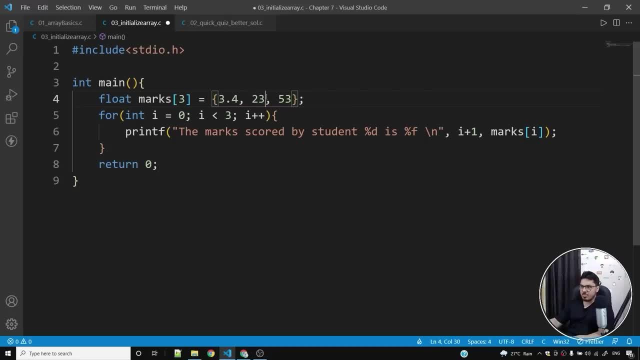 integer okay, so i'll simply make this integer okay. so i'll simply make this float and let me see if these values float, and let me see if these values float, and let me see if these values are working, and i'll say 5.3 here. 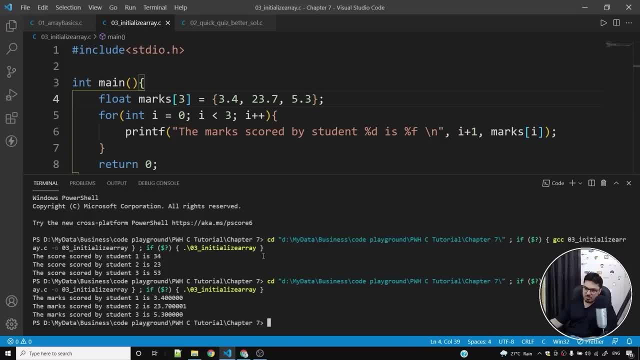 are working and i'll say 5.3 here are working and i'll say: 5.3 here, let me run this program. and yes, these, let me run this program. and yes, these, let me run this program. and yes, these values work okay. so these values are. 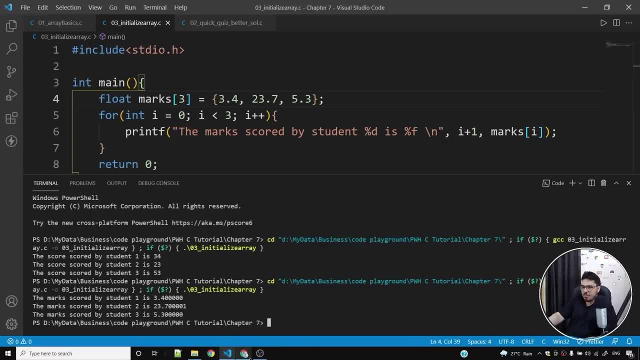 values work okay, so these values are values work okay, so these values are working in a very perfect way, working in a very perfect way, working in a very perfect way. now, what i'll do is i'll simply come. now, what i'll do is i'll simply come. 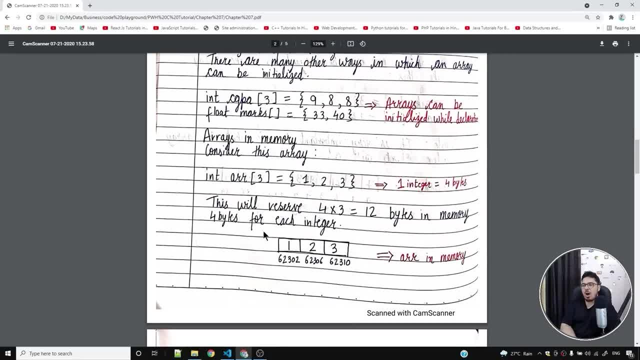 now what i'll do is i'll simply come back to my notes and try to explain back to my notes and try to explain back to my notes and try to explain you how arrays look in memory. so you how arrays look in memory, so you how arrays look in memory. so consider this array. it is an array of. 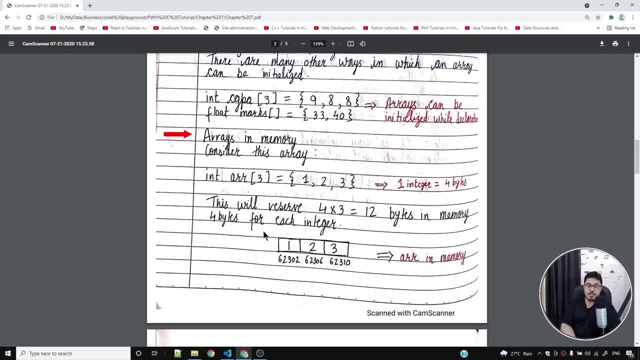 consider this array. it is an array of. consider this array. it is an array of three integers, and it contains one, two, three integers. and it contains one, two, three integers. and it contains one, two and three as the values. uh, so you need. and three as the values. uh, so you need. 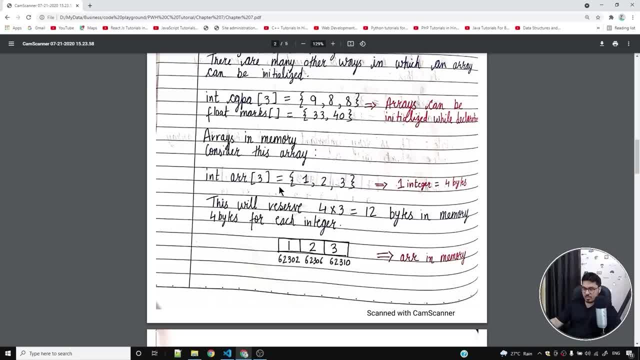 and three as the values. uh, so you need to make sure that one integer is four, to make sure that one integer is four, to make sure that one integer is four. bytes in this architecture: now it might bytes in this architecture now it might bytes in this architecture: now it might be two bytes or it might be some other. 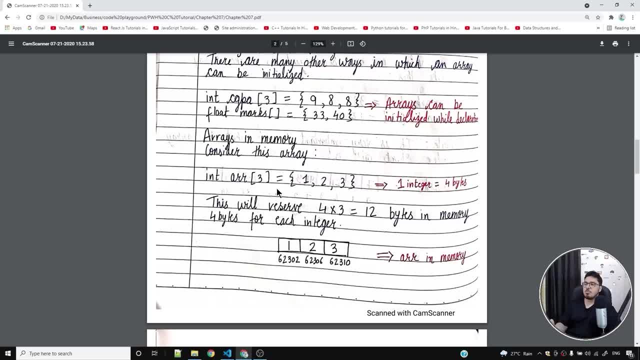 be two bytes or it might be some other. be two bytes or it might be some other. value in some other architecture. it value in some other architecture. it value in some other architecture. it depends on the machine, but let us assume. depends on the machine, but let us assume. 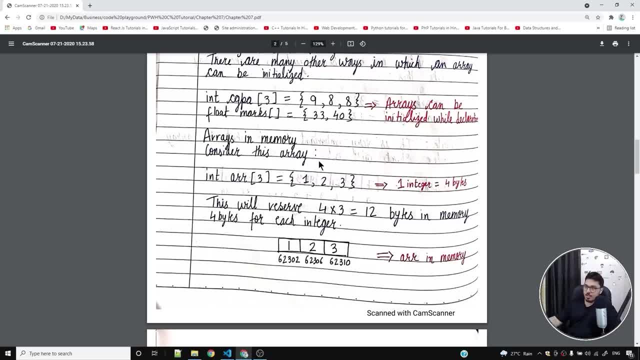 depends on the machine. but let us assume that we are on a machine where one, that we are on a machine where one, that we are on a machine where one integer is four bytes- okay. integer is four bytes. okay. integer is four bytes- okay. this will reserve four multiplied by. 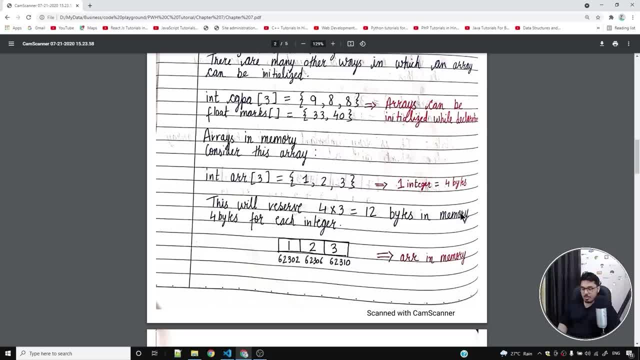 this will reserve four. multiplied by this will reserve four. multiplied by three is equal to 12 bytes in memory. three is equal to 12 bytes in memory. three is equal to 12 bytes in memory. now i want to tell you something about. now. i want to tell you something about. 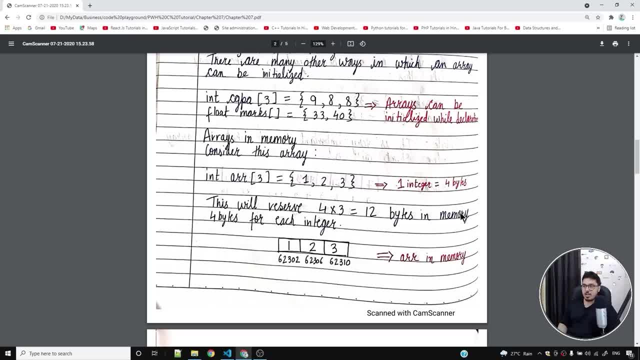 now i want to tell you something about the memory memory is contiguous, which the memory memory is contiguous, which the memory memory is contiguous, which means that you can simply store zero one, means that you can simply store zero one, means that you can simply store zero one, zero one, zero one. in this manner. now, if 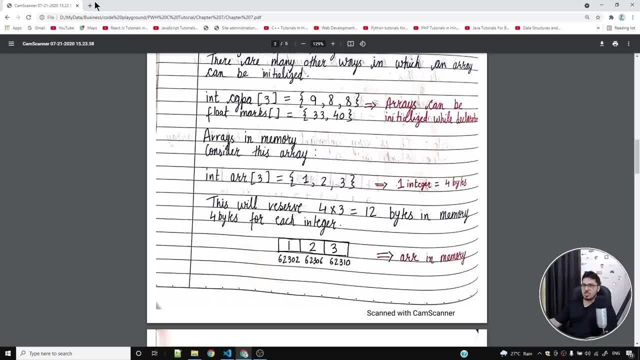 zero one, zero one, zero one in this manner now, if zero one, zero one, zero one in this manner now, if you want to store an integer, you, you want to store an integer, you, you want to store an integer, you need four bytes, which is nothing but four. 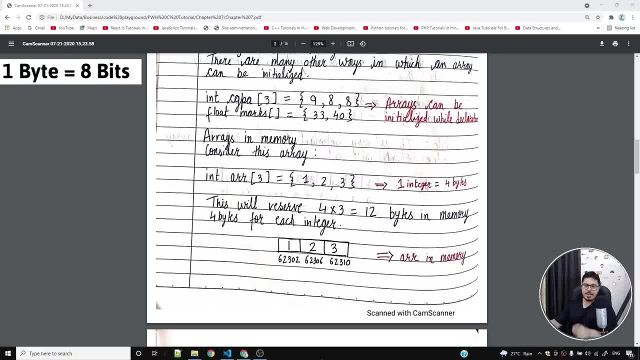 need four bytes, which is nothing but four. need four bytes, which is nothing but four, multiplied by eight bits. one byte is multiplied by eight bits. one byte is multiplied by eight bits. one byte is eight bits. so this is how memory works: eight bits. so this is how memory works. 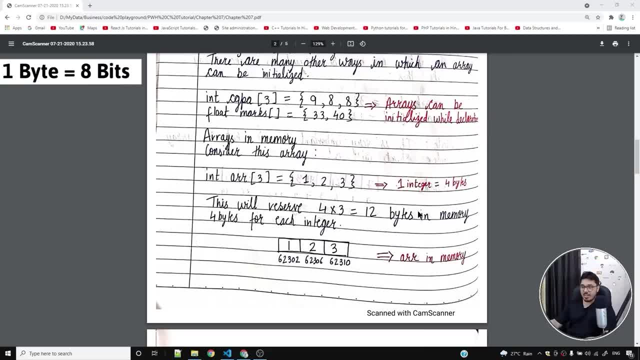 eight bits. so this is how memory works. so what this will do is this will. so what this will do is this will. so what this will do is this: will uh save, or rather reserve 12 bytes in uh save, or rather reserve 12 bytes in uh save, or rather reserve 12 bytes in memory. 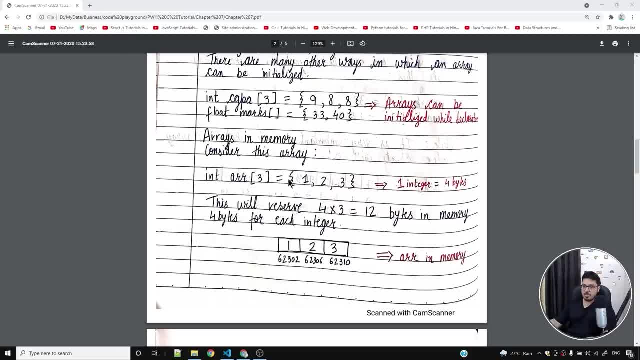 memory, memory of four bytes for each integer. so if of four bytes for each integer, so if of four bytes for each integer. so if six, two, three zero two will hold this, six two, three zero two will hold this. six two, three zero two will hold this integer, four bytes will. 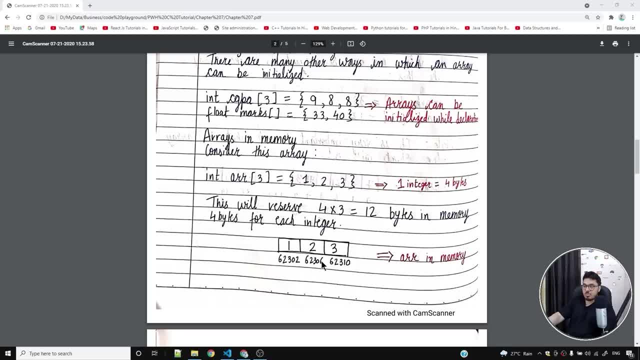 integer four bytes will integer four bytes will be used by this particular integer, then be used by this particular integer, then be used by this particular integer, then again, again, again. six, two, three, zero, six onwards, uh, this six. two, three zero, six onwards. uh, this six, two, three zero, six onwards, uh, this integer will store this two. 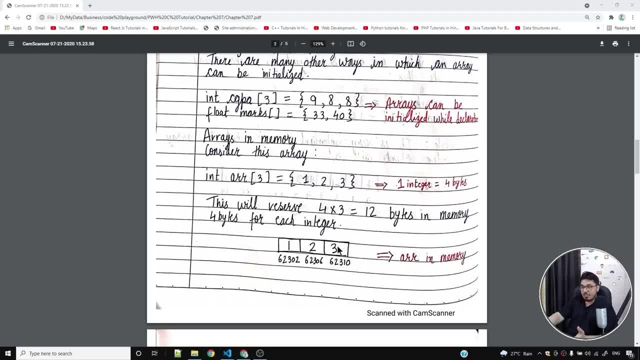 integer will store this two. integer will store this two. this place will get four bytes. this place, this place will get four bytes. this place, this place will get four bytes. this place will once again get four bytes, will once again get four bytes, will once again get four bytes. and this is how? uh, this is how. 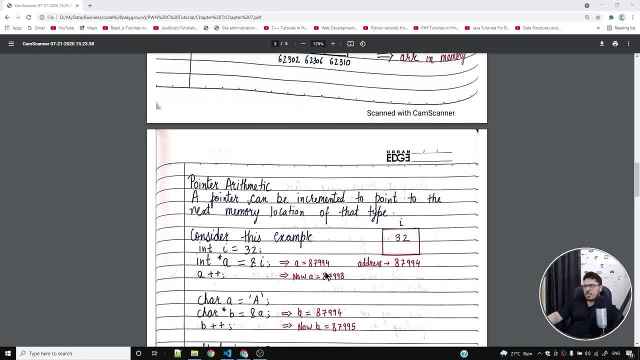 and this is how. uh, this is how and this is how. uh, this is how memory management of array works. okay, memory management of array works. okay. memory management of array works okay. now let's talk about pointer arithmetic. now, let's talk about pointer arithmetic. now let's talk about pointer arithmetic, which is: 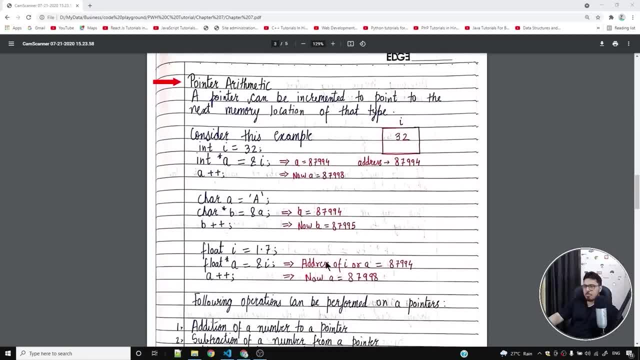 which is, which is something you might not know, or you might something you might not know, or you might something you might not know, or you might know, know, know. but let me tell you something about array. but let me tell you something about array, but let me tell you something about array and pointers. okay, so, 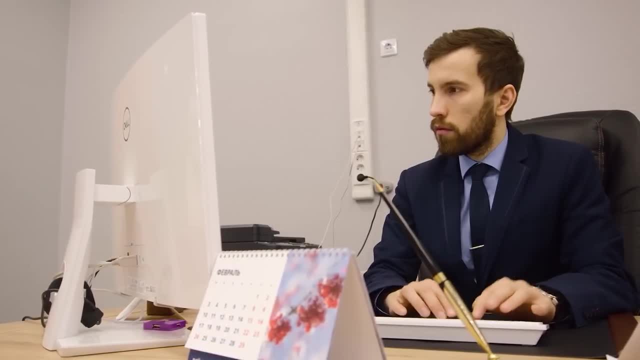 and pointers. okay, so, and pointers, okay. so let's create a program called array and let's create a program called array and let's create a program called array and pointers. and i want you to be very pointers, and i want you to be very pointers and i want you to be very attentive. 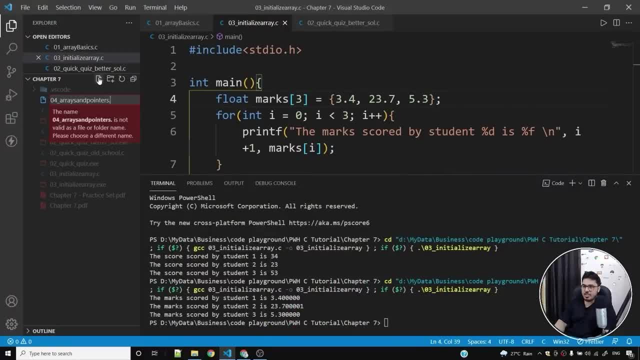 attentive, attentive, when i teach you this arrays and when i teach you this arrays and when i teach you this arrays and pointers dot c, pointers dot c, pointers dot c. so let's put in a boilerplate code. so let's put in a boilerplate code. so let's put in a boilerplate code. and let me tell you something. if i say: 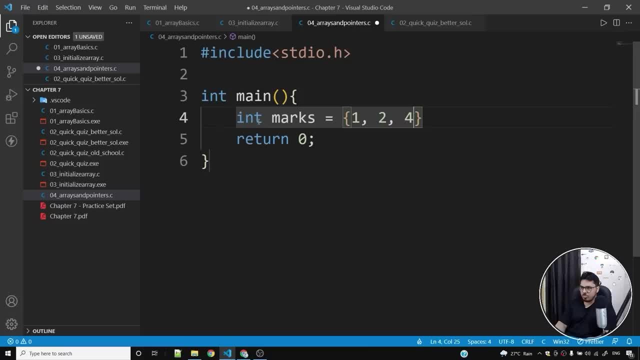 and let me tell you something: if i say: and let me tell you something: if i say int marks is equal to int marks is equal to int marks, is equal to one, two, three, and then i have to make it one, two, three, and then i have to make it. 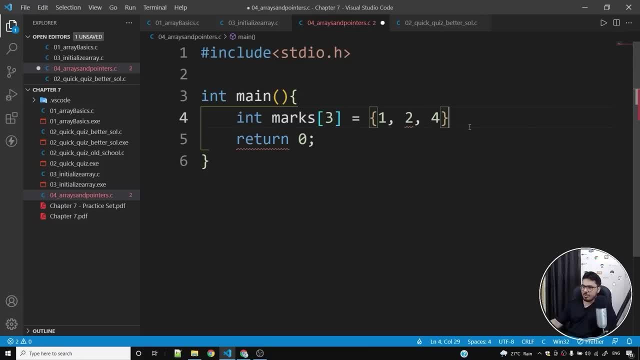 one, two, three, and then i have to make it marks three, marks three, marks three, and i'll put a semicolon here when i do, and i'll put a semicolon here when i do, and i'll put a semicolon here when i do something like this. 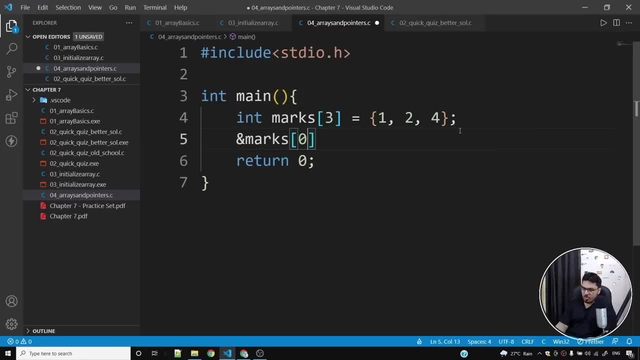 something like this, something like this, this ampersand mark zero, this ampersand mark zero, this ampersand mark zero, which is the address of first element, which is the address of first element, which is the address of first element, can be written as marks, can be written as marks. 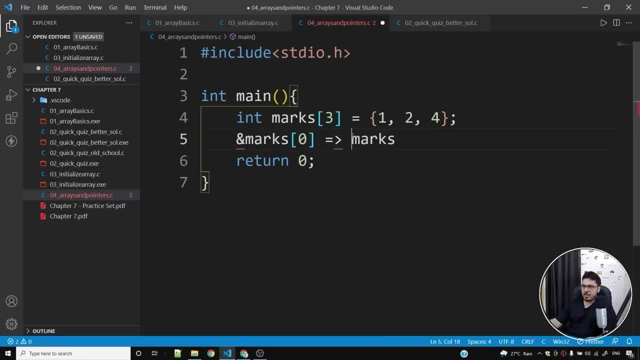 can be written as marks. so this particular thing and this, so this particular thing and this, so this particular thing and this particular thing, particular thing, particular thing is exactly the same thing, which means is exactly the same thing, which means is exactly the same thing, which means that if i want to change this value, 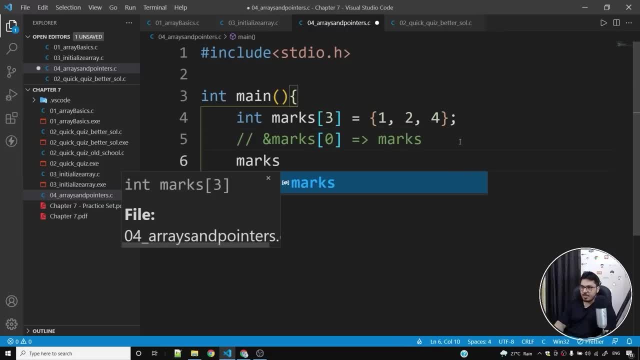 that if i want to change this value, that if i want to change this value, i can do something like this. i can do something like this. i can do something like this. i can say, i can say, i can say: marks, star marks, is equal to 89. 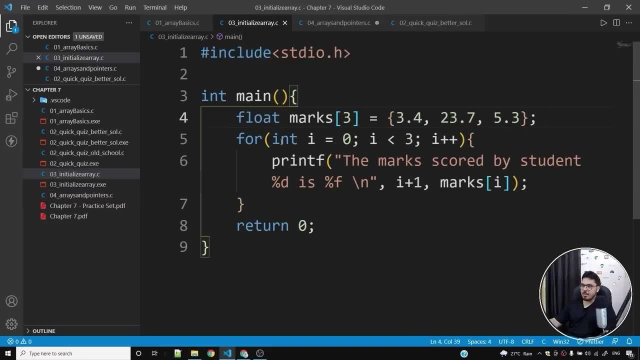 marks star marks- is equal to 89. marks star marks is equal to 89. if i do something like this, if i do something like this, if i do something like this and- and i try to print say mark zero, i try to print say mark zero. i try to print say mark zero. let me try to print mark zero. 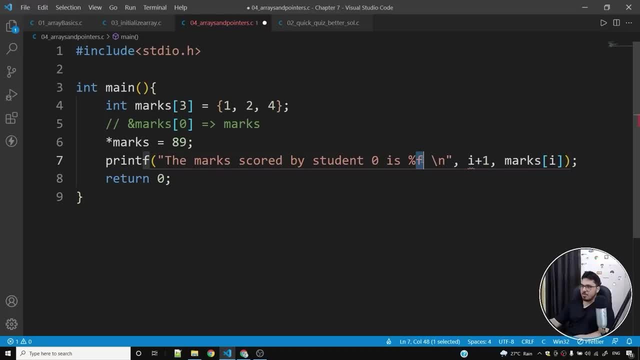 let me try to print mark zero. let me try to print mark zero. i'll say: mark stored by student zero is. i'll say mark stored by student zero is. i'll say mark stored by student zero is a percentage percentage d, a percentage percentage d, a percentage percentage d, and i'll simply say mark zero. 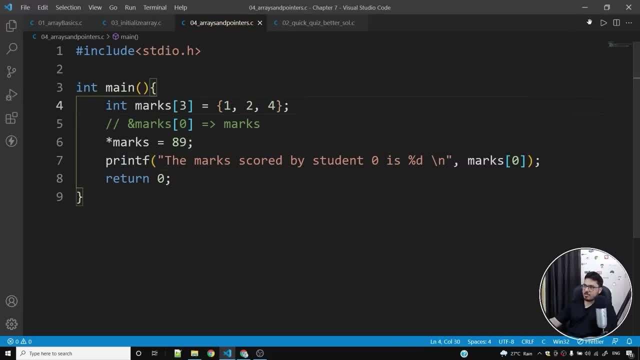 and i'll simply say mark zero. and i'll simply say mark zero if i run this program, if i run this program, if i run this program, i'll not get one as mark zero, rather i'll. i'll not get one as mark zero, rather i'll. 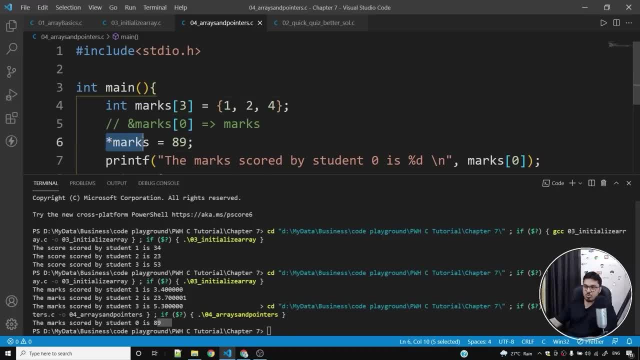 i'll not get one as mark zero. rather, i'll get 89 as mark zero. get 89 as mark zero, get 89 as mark zero. why? because i have used this pointer. why because i have used this pointer. why because i have used this pointer, syntax, to change the value of mark 0. 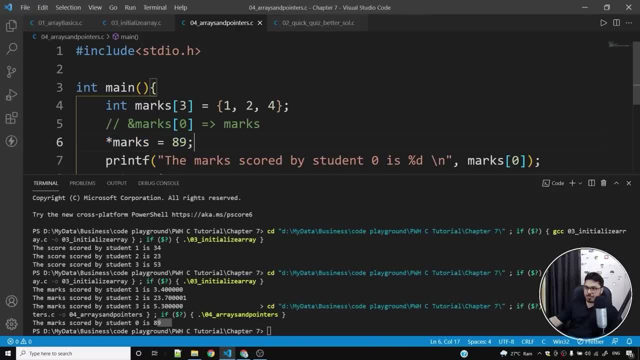 syntax to change the value of mark 0. syntax to change the value of mark 0 to 89. so what i'm saying is i'm saying to 89. so what i'm saying is i'm saying to 89. so what i'm saying is i'm saying the address of mark 0 is nothing but. 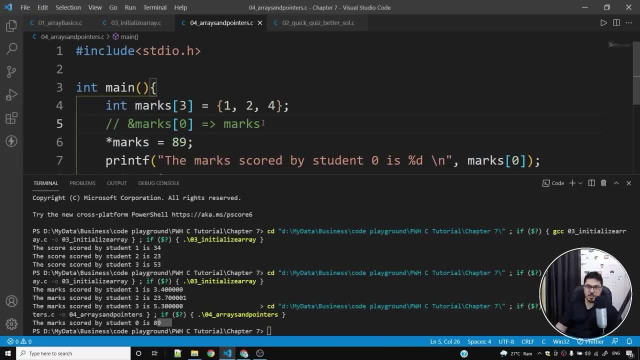 the address of mark 0 is nothing but the address of mark 0 is nothing but marks. i can actually use value at marks. i can actually use value at marks. i can actually use value at operator which is star operator. i can. operator which is star operator: i can. 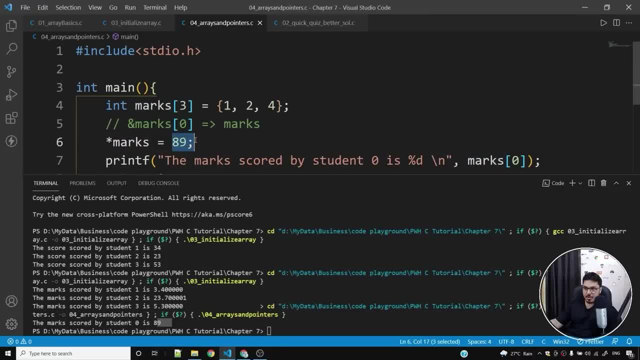 operator, which is star operator, i can say value at marks. say value at marks. say value at marks is equal to 89. when i do something like is equal to 89. when i do something like is equal to 89. when i do something like this, what happens is value at this. 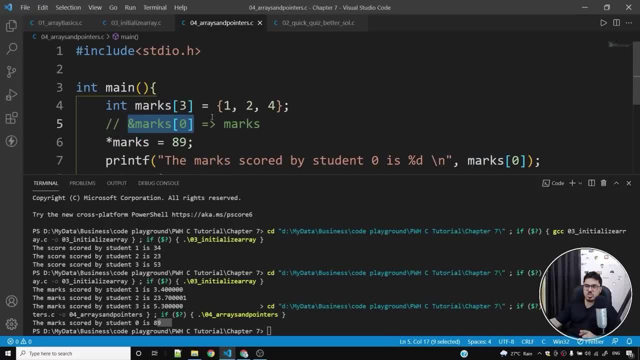 this. what happens is value at this, this, what happens is value at this particular address, which is ampersand particular address, which is ampersand particular address, which is ampersand mark 0, which is address of this mark 0, which is address of this. 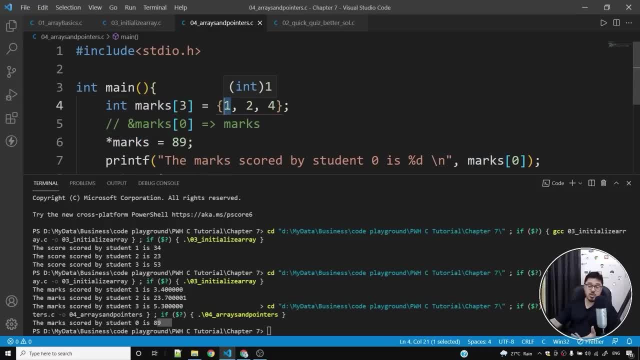 mark 0, which is address of this particular, uh, particular, uh, particular uh place where this number is stored, uh place where this number is stored, uh place where this number is stored, uh. this changes the value of this. changes the value of this. changes the value of mark 0, which was 1 before, to 89 now. 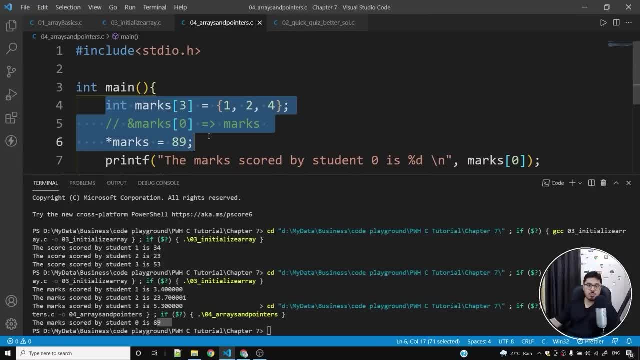 mark 0, which was 1 before to 89, now. mark 0, which was 1 before to 89 now. so this is how so, this is how so, this is how all the syntax works and you can all the syntax works and you can all the syntax works and you can actually change the value of. 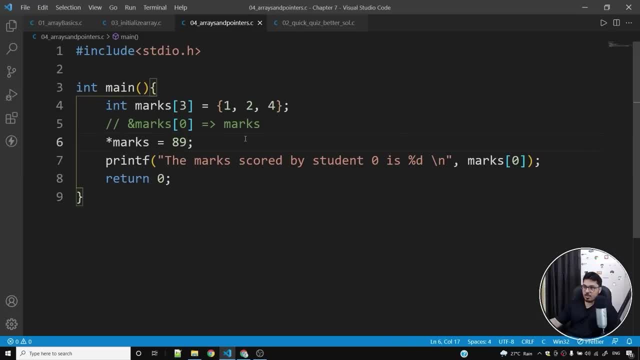 actually change the value of, actually change the value of this two as well, and how do i change the this two as well? and how do i change the this two as well, and how do i change the value of two, value of two, value of two. i can increment this pointer and if i say: 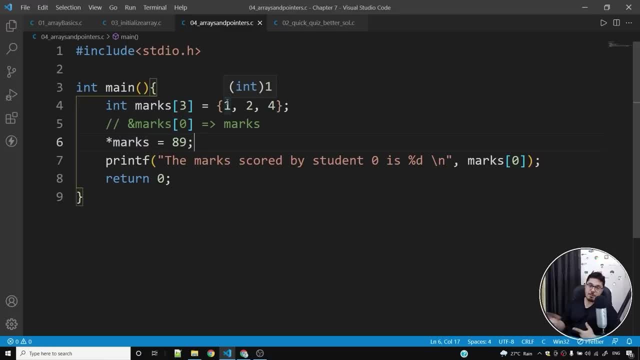 i can increment this pointer. and if i say i can increment this pointer and if i say marks plus plus, it will not be marks plus plus, it will not be marks plus plus, it will not be. one plus the original address it will. one plus the original address, it will. 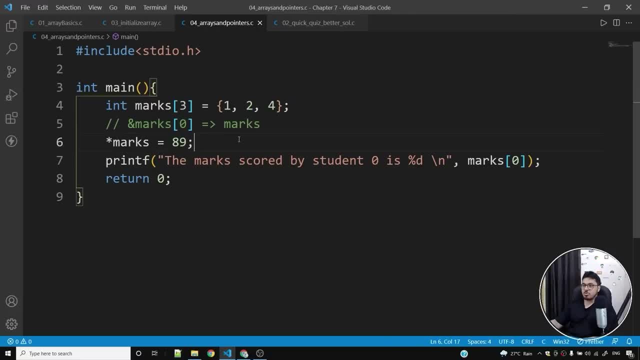 one plus the original address, it will actually go to the next address- actually go to the next address, actually go to the next address. this might sound strange, so let us look. this might sound strange. so let us look, this might sound strange. so let us look into this. 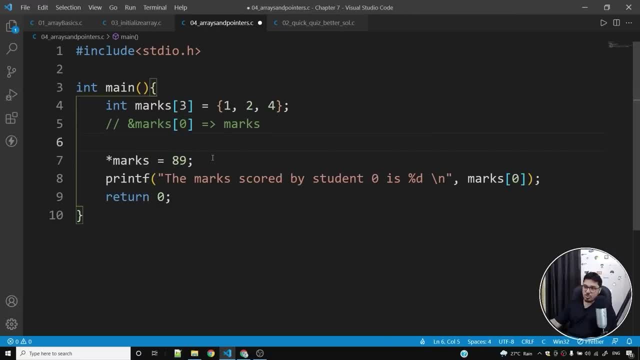 into this, into this more uh in a more systematic way. i more uh in a more systematic way, i more uh in a more systematic way. i should say: should say, should say. so what i'll do is i'll say in star ptr. so what i'll do is i'll say in star ptr. 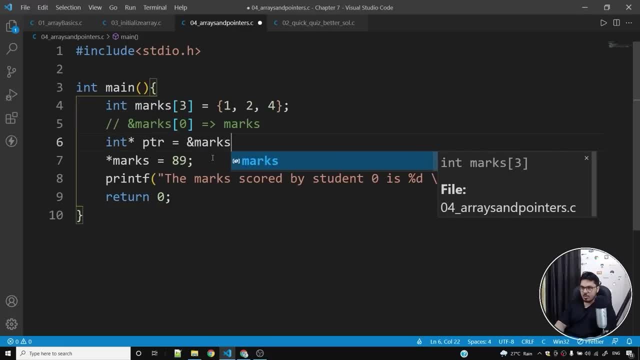 so what i'll do is i'll say in star: ptr is equal to amp percent is equal to amp percent is equal to amp percent mark zero. but i'll not do something like mark zero. but i'll not do something like mark zero, but i'll not do something like this. 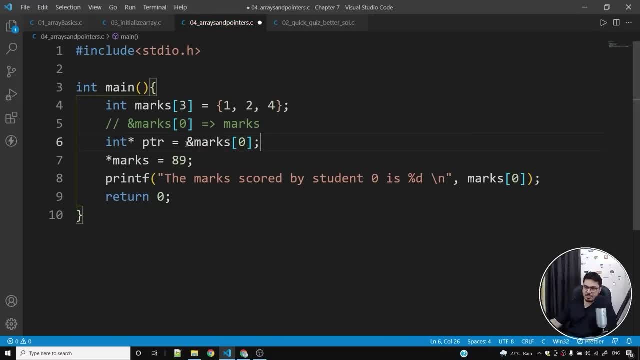 this, this: i can actually do amp percent ptr. uh, i can actually do amp percent ptr. uh, i can actually do amp percent ptr. uh, sorry star pdr is equal to ampersand. sorry star pdr is equal to ampersand. sorry star pdr is equal to ampersand mark zero. 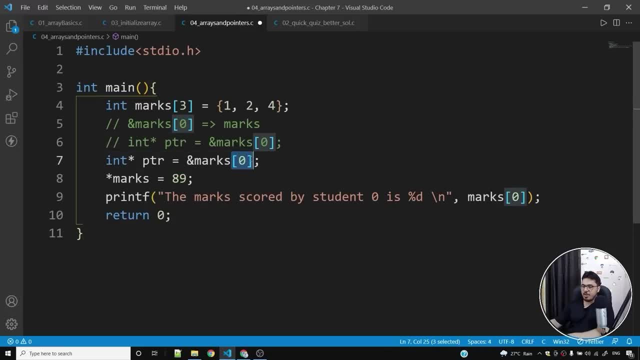 mark zero, mark zero. but in order to explain you, i'll do. but in order to explain you, i'll do. but in order to explain you, i'll do something like this. i'll get rid of this, something like this: i'll get rid of this because i have told you. 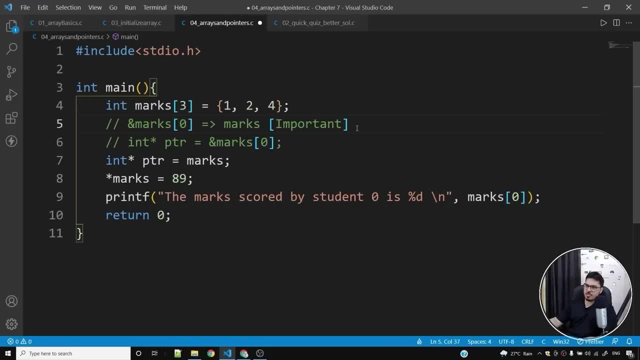 because i have told you, because i have told you, and let me write important here, and let me write important here, and let me write important here: this is, this is the core concept here. this is, this is the core concept here. this is this is the core concept here- that ampersand mark zero can be written. 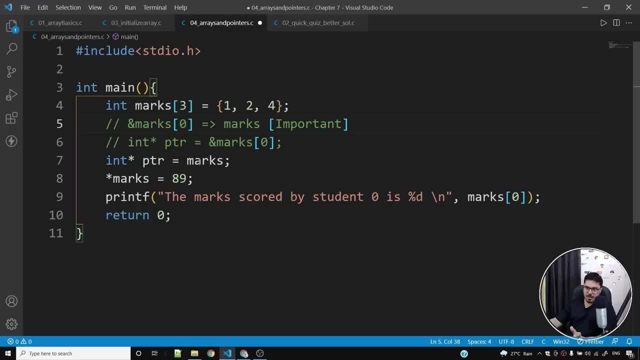 that ampersand mark zero can be written, that ampersand mark zero can be written as marks, as marks, as marks. so i simply said in star ptr is equal to. so i simply said in star ptr is equal to. so i simply said in star ptr is equal to marks. i could have said this: 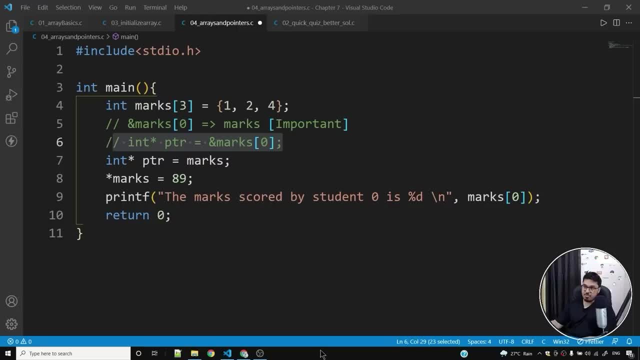 marks. i could have said this, marks. i could have said this, and the program would have worked in, and the program would have worked in, and the program would have worked in exactly the same way, exactly the same way, exactly the same way. but i want to teach you this index. i want. 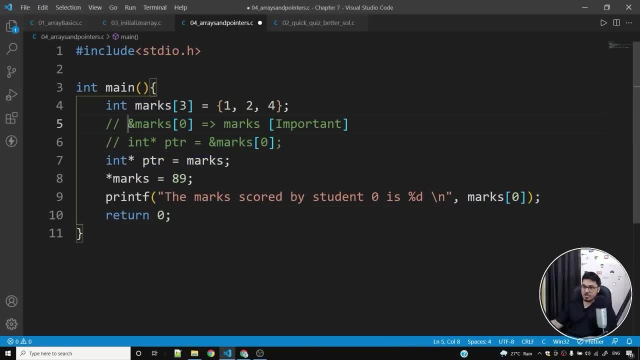 but i want to teach you this index. i want, but i want to teach you this index. i want to teach you that, to teach you that, to teach you that marks is nothing but ampersand mark zero. marks is nothing but ampersand mark zero. marks is nothing but ampersand mark zero. this is important. 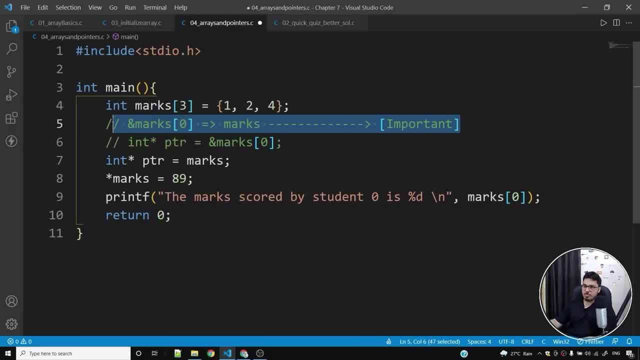 this is important. this is important. this is very important, which is why a this is very important, which is why a this is very important, which is why a mark. this is important. this concept is mark. this is important. this concept is mark. this is important. this concept is important now, instead of using star marks. 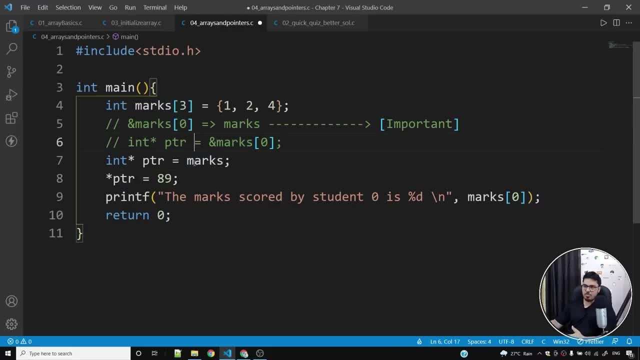 important now instead of using star marks. important now instead of using star marks. i can use star ptr because pdr is a. i can use star ptr because pdr is a. i can use star ptr because pdr is a pointer, pointer, pointer which is pointing to this. so i'm saying: 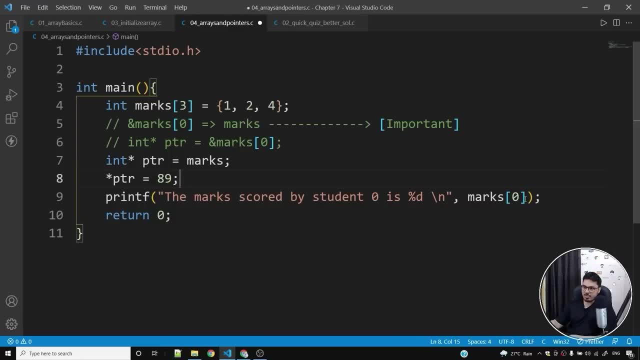 which is pointing to this. so i'm saying which is pointing to this. so i'm saying star ptr is equal to 89, star ptr is equal to 89, star ptr is equal to 89, and this changes the value of mark 0 as. and this changes the value of mark 0 as. 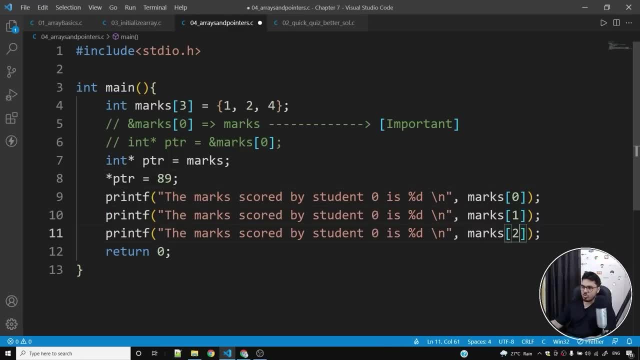 and this changes the value of mark 0 as 89, 89, 89. what will the values of marks 1 and what will the values of marks 1 and what will the values of marks 1 and marks 2, marks 2, marks 2- and i know that you must be thinking why. and i know that you must be thinking why, and i know that you must be thinking why would these values change? and you are. would these values change? and you are, would these values change? and you are right, these values will not change, right, these values will not change. 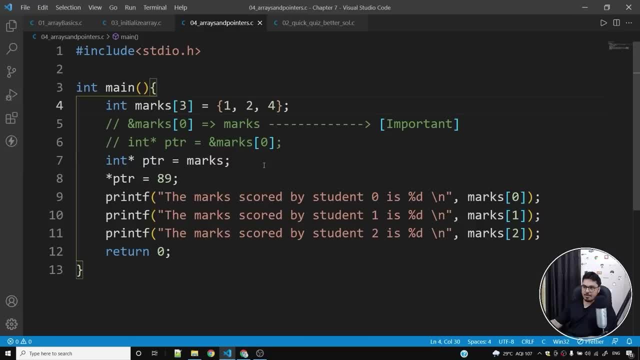 right. these values will not change. these values will be two and four. these values will be two and four. these values will be two and four. but listen to me carefully now if i do. but listen to me carefully now if i do. but listen to me carefully now if i do something like this: ptr plus plus. 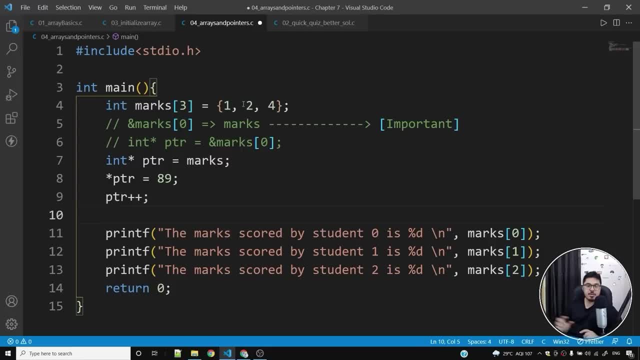 something like this: ptr plus plus. something like this: ptr plus plus. ptr plus plus means point to the next, ptr plus plus means point to the next. ptr plus plus means point to the next element, element, element. now, this is something that you need to now. this is something that you need to. 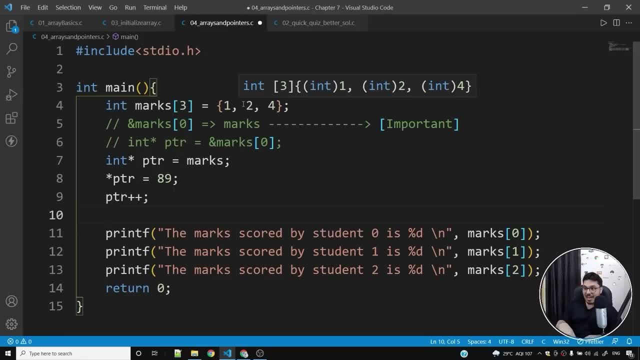 now, this is something that you need to understand, understand, understand. pointer arithmetic will not add one pointer. arithmetic will not add one pointer arithmetic will not add one integer to the address, integer to the address, integer to the address. but rather what it will do is if we have 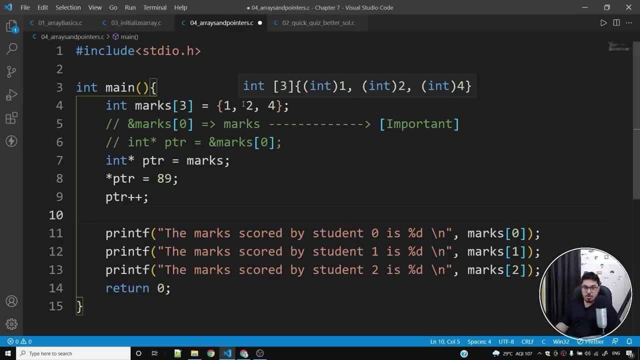 but rather what it will do is if we have, but rather what it will do is if we have an integer pointer, it will point to the an integer pointer. it will point to the an integer pointer. it will point to the next integer because the first four. next integer because the first four. 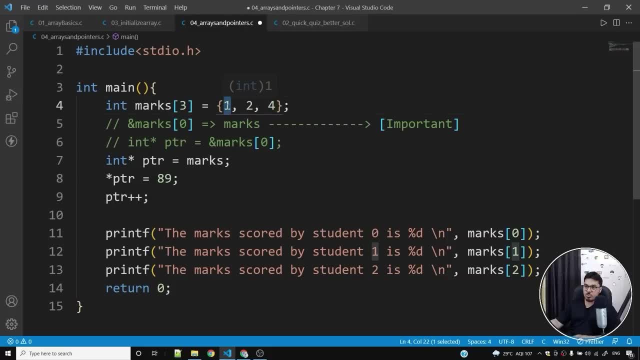 next integer, because the first four bytes are reserved for this particular bytes are reserved for this particular bytes are reserved for this particular integer. so it will not touch those four integer. so it will not touch those four integer. so it will not touch those four bytes if i say ptr plus, plus, it will. 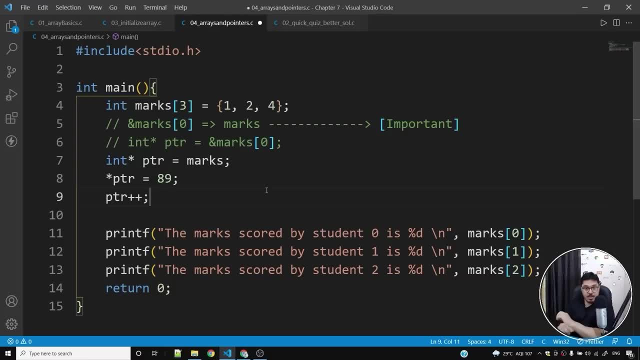 bytes. if i say ptr plus plus, it will bytes. if i say ptr plus plus, it will point at the starting of next integer point, at the starting of next integer point, at the starting of next integer in the case of arrays. and even if we are in the case of arrays, and even if we are, 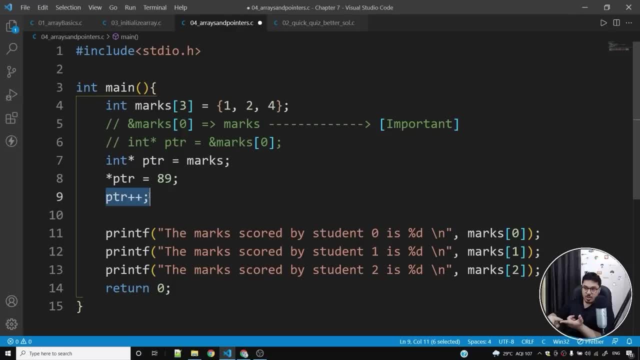 in the case of arrays, and even if we are not not not dealing with arrays, ptr plus plus will dealing with arrays. ptr plus plus will dealing with arrays. ptr plus plus will point to the next value. so if the first point to the next value, so if the first, 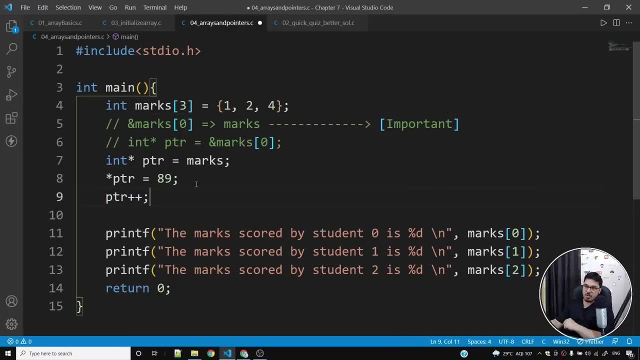 point to the next value. so if the first value is one, value is one, value is one. next value is two. this ptr plus plus will. next value is two. this ptr plus plus will. next value is two. this ptr plus plus will actually point to ampersand. 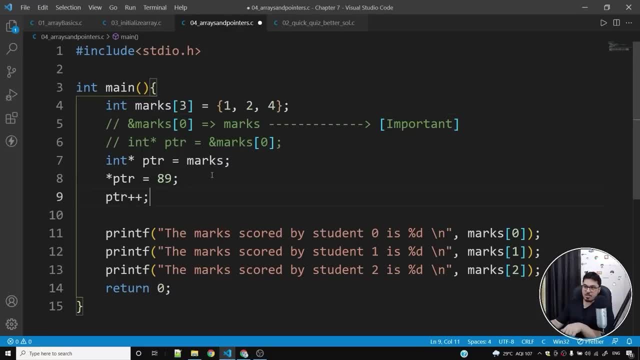 actually point to ampersand, actually point to ampersand marks one. so ptr is now ampersand marks marks one. so ptr is now ampersand marks marks one. so ptr is now ampersand marks one. which is why one, which is why one, which is why i can do something like this. i can say: 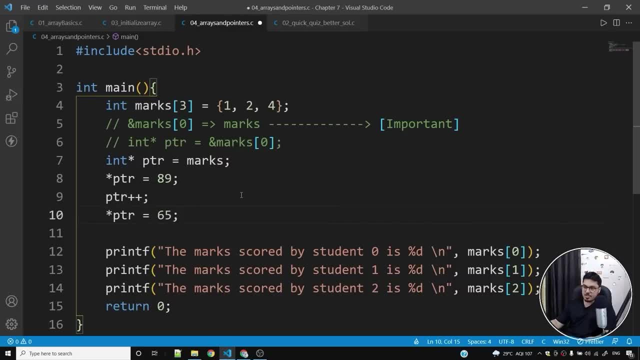 i can do something like this. i can say: i can do something like this. i can say: ptr is equal to ptr is equal to, ptr is equal to 65, and this will change the value of 65 and this will change the value of 65 and this will change the value of marks 1. 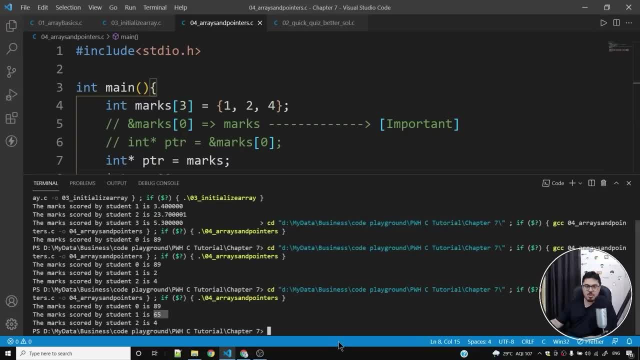 marks 1. marks 1 to 65. let me show you so the value of to 65. let me show you so the value of to 65. let me show you so the value of marks 1 is now 65. marks 1 is now 65. 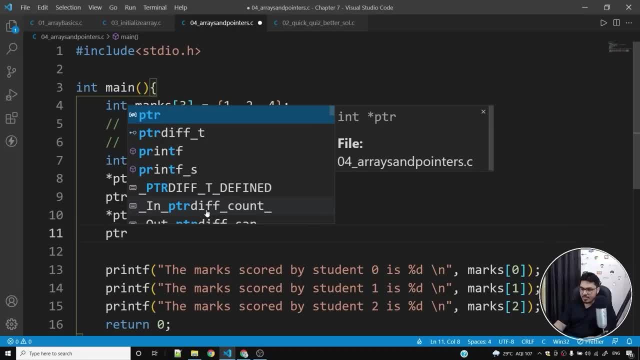 marks 1 is now 65. can i do the same thing again? can i do? can i do the same thing again, can i do? can i do the same thing again? can i do ptr plus plus once again, ptr plus plus once again, ptr plus plus once again. and will this ptr point to 4 this time? 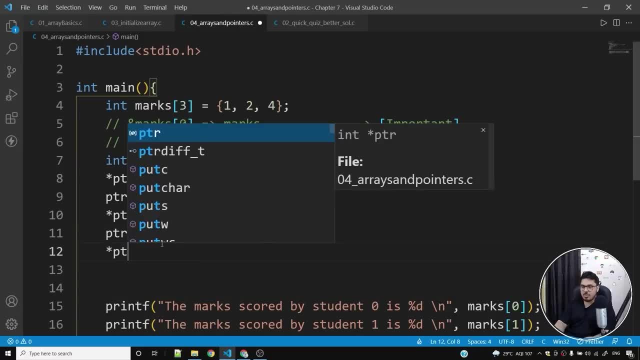 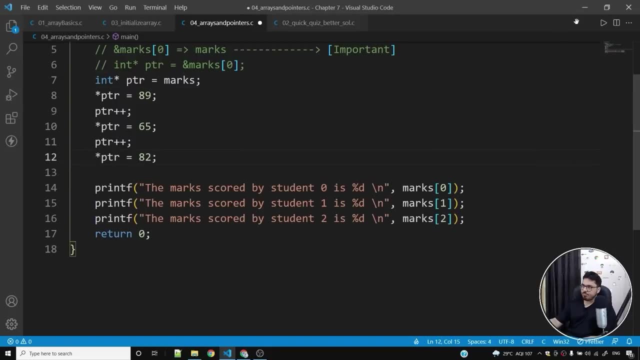 and will this ptr point to 4 this time? and will this ptr point to 4 this time? yes, you are right, this ptr will now. yes, you are right, this ptr will now. yes, you are right, this ptr will now point to 4. point to 4, this ptr point to 4. this is now 82, so this is how pointer. 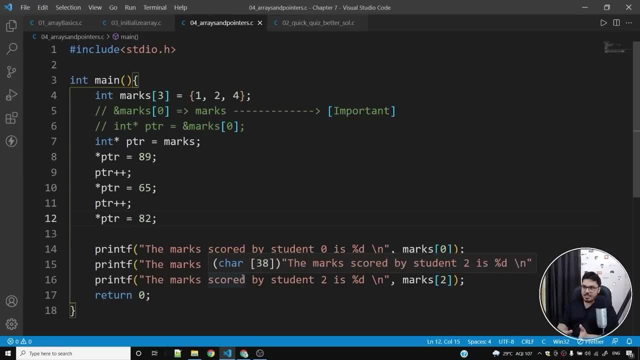 is now 82. so this is how pointer is now 82. so this is how pointer arithmetic works. instead of changing an arithmetic works, instead of changing an arithmetic works, instead of changing an address by adding a number to it address, by adding a number to it address, by adding a number to it, it will change the address by adding 4. 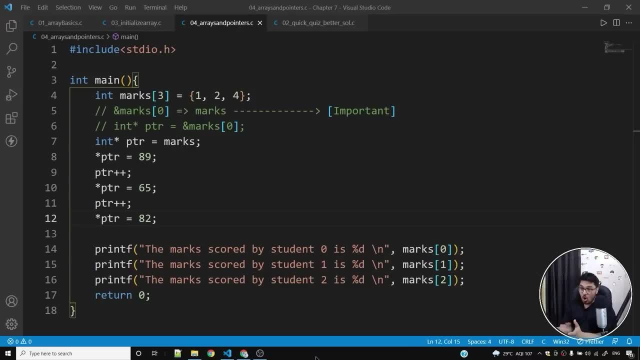 it will change the address by adding 4. it will change the address by adding 4 to it. it will make that address point to it. it will make that address point to it. it will make that address point to the next integer or point to the next. 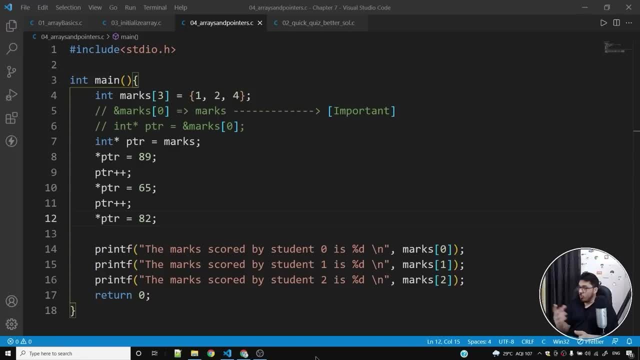 to the next integer or point to the next to the next integer, or point to the next character, or point to the next floating character, or point to the next floating character or point to the next floating point, point, point, next double, next long double, and so on. next double, next long double, and so on. 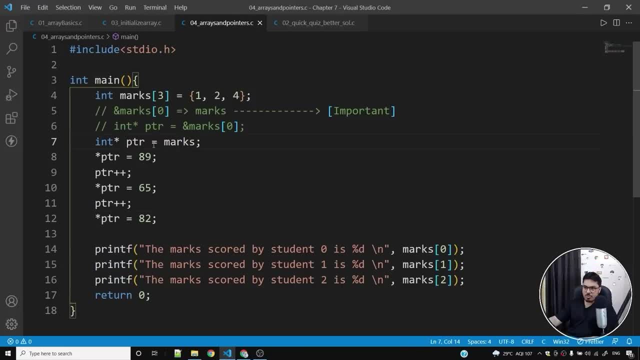 next double, next long double, and so on. so in this case the pointer is of type. so in this case the pointer is of type. so in this case the pointer is of type integer, so it will actually increment it integer. so it will actually increment it integer. so it will actually increment it by four instead of incrementing it by one. 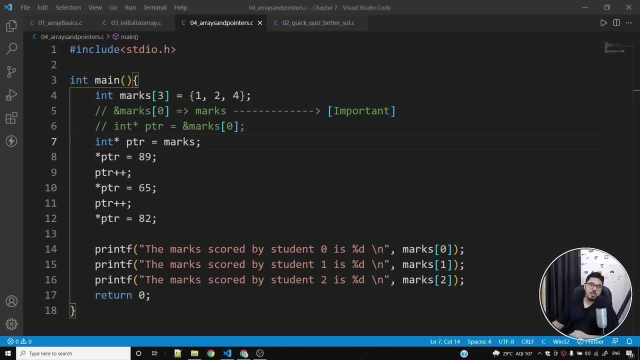 by four instead of incrementing it by one, by four instead of incrementing it by one. because integer in this architecture is because integer in this architecture is because integer in this architecture is taking four bytes. okay, let's now come taking four bytes. okay, let's now come. 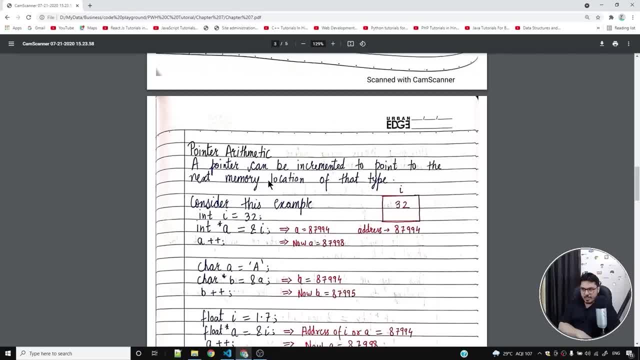 taking four bytes. okay, let's now come to the nodes and try to understand this to the nodes. and try to understand this to the nodes. and try to understand this thing. so a pointer can be incremented to thing. so a pointer can be incremented to thing. so a pointer can be incremented to point to the next memory location of that. 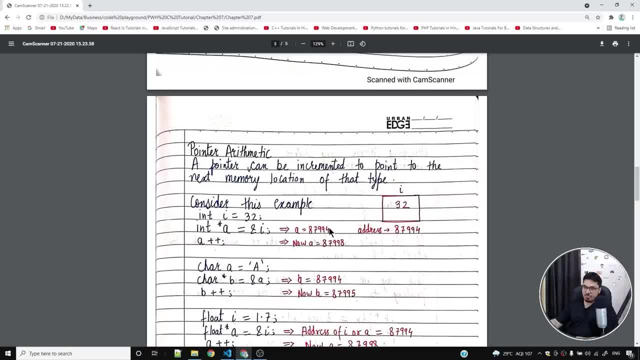 point to the next memory location of that point, to the next memory location of that type. type, type: note that if the address is 87994 ptr, note that if the address is 87994 ptr, note that if the address is 87994 ptr, plus plus will not make it 87995. 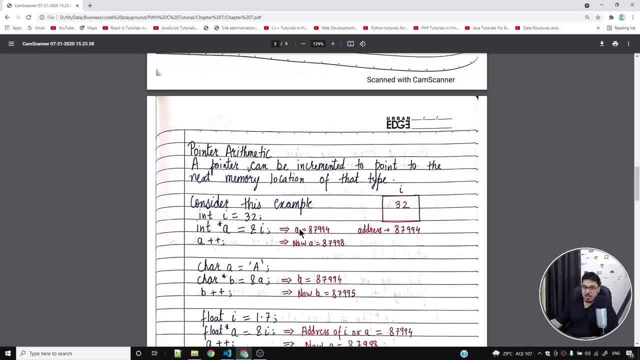 plus plus will not make it 87995. plus plus will not make it 87995, but it will check what is the type of a. but it will check what is the type of a. but it will check what is the type of a if it is integer. 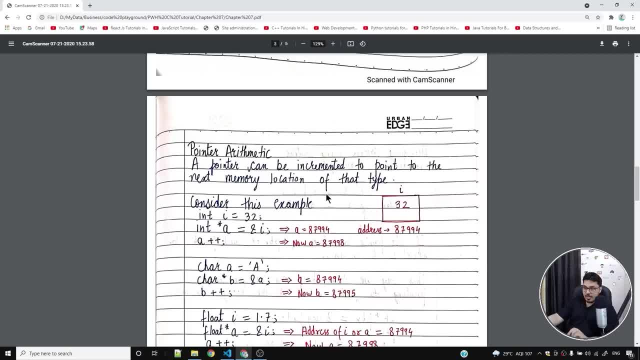 if it is integer. if it is integer, it takes four bytes. it will add four to it. takes four bytes, it will add four to it. takes four bytes. it will add four to it and not one. okay, let's it and not one. okay, let's it and not one. okay, let's understand this example thoroughly now. 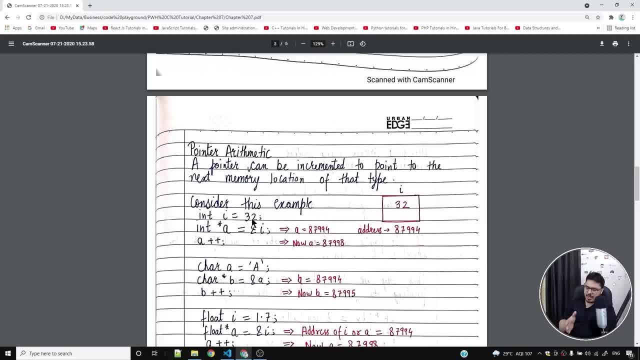 understand this example thoroughly now. understand this example thoroughly now. so ind i is equal to 32. so ind i is equal to 32. so ind i is equal to 32. simply, we are assigning the value 32. simply. we are assigning the value 32 simply. we are assigning the value 32 inside i. 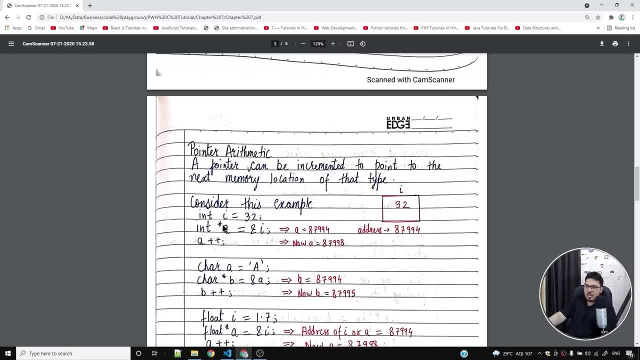 inside i, inside i. in star a is equal to ampersand i, so in star a is equal to ampersand i, so in star a is equal to ampersand i. so the value uh of this pointer, which is a, the value uh of this pointer, which is a: 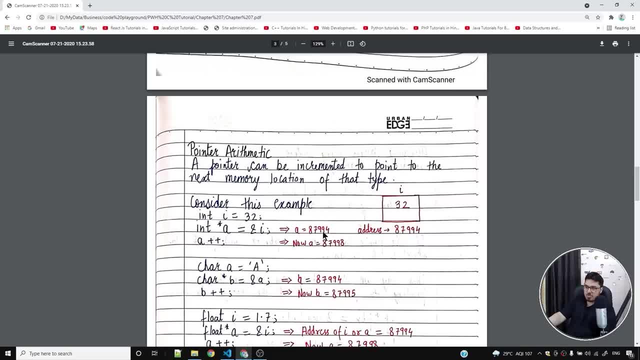 the value, uh, of this pointer which is a. a is an integer pointer- is nothing but a is an integer pointer is nothing but a is an integer pointer is nothing but the address of i, the address of i, the address of i. so let us assume this address of i is. 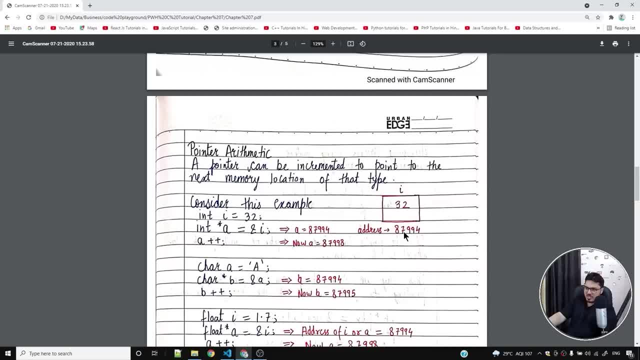 so let us assume this address of i is. so let us assume this address of i is eight, seven, nine, nine, four. so address eight, seven, nine, nine, four. so address eight, seven, nine, nine, four. so address of this integer is eight, seven, nine. of this integer is eight, seven, nine. 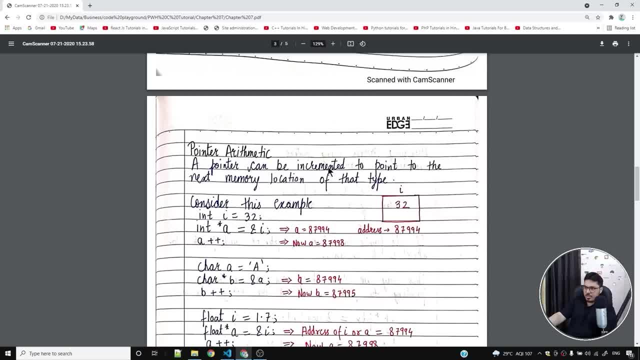 of this integer is eight, seven, nine, nine, four, and this integer contains 32, four, and this integer contains 32, four, and this integer contains 32. the name of the variable is i. i hope you. the name of the variable is i. i hope you. the name of the variable is i. i hope you don't have any doubt so far. 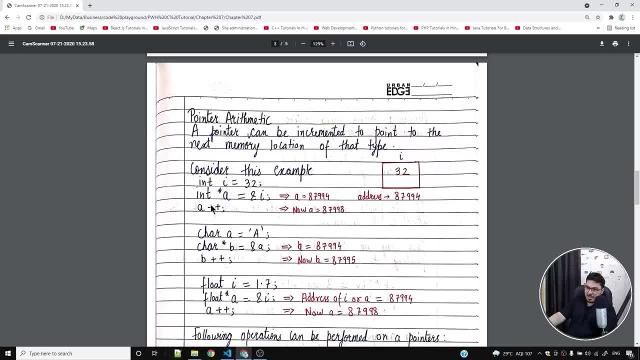 don't have any doubt so far. don't have any doubt so far. let's try to deep dive now. if i do, let's try to deep dive now if i do. let's try to deep dive now if i do. something like a plus plus. something like a plus plus. 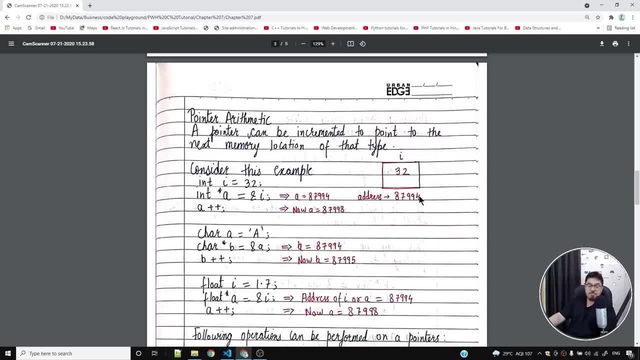 something like a plus plus. you might think that this address will. you might think that this address will. you might think that this address will change to 87995, but no, it will not change to 87995. but no, it will not change to 87995. but no, it will not change to 87995, it will change to. 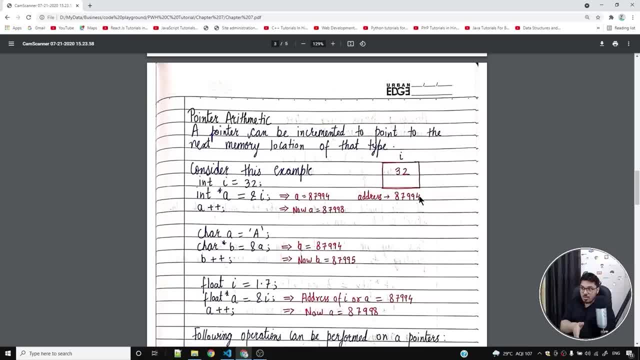 change to 87995. it will change to change to 87995. it will change to 87998. why, why were these four 87998? why, why were these four 87998? why, why were these four points added to this particular address? points added to this particular address. 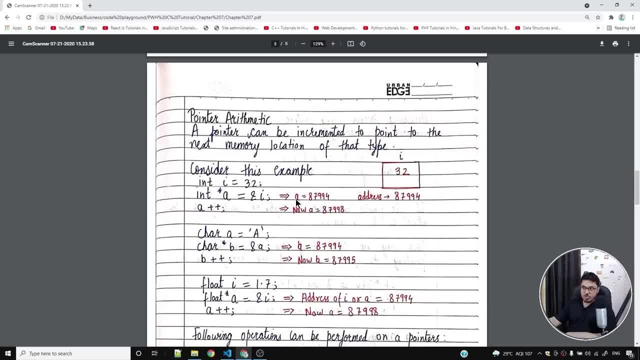 points added to this particular address because this is of type integer, integer. because this is of type integer, integer. because this is of type integer: integer takes four bytes, so it will point to: takes four bytes, so it will point to: takes four bytes, so it will point to the next integer, so it will add four to. 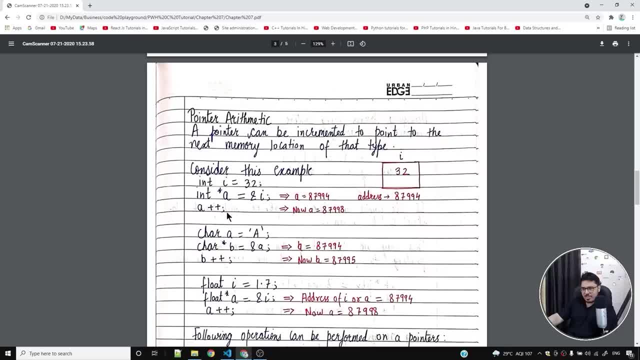 the next integer, so it will add four to the next integer. so it will add four to it and not one. okay, i hope this is clear it and not one. okay, i hope this is clear it and not one. okay, i hope this is clear. now let's try to understand the same. 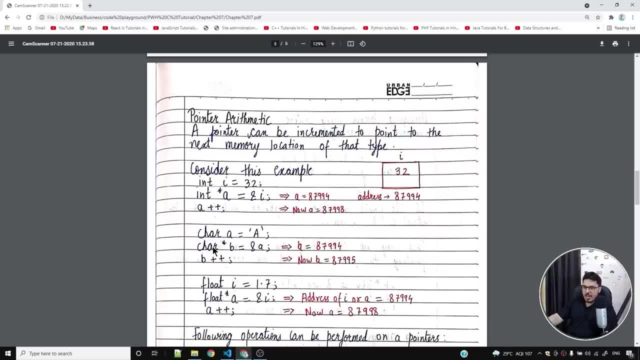 now let's try to understand the same. now let's try to understand the same thing using character. so if i say care a thing using character, so if i say care a thing using character, so if i say care a is equal to a and i say care star, b is, 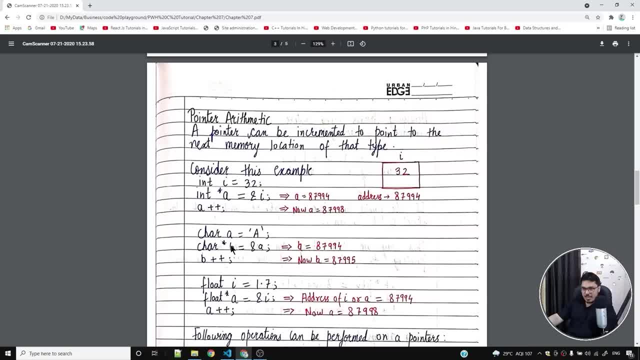 is equal to a and i say, care, star b is is equal to a and i say: care, star b is equal to ampersand a. so i'm creating a equal to ampersand a. so i'm creating a equal to ampersand a. so i'm creating a pointer b, which is actually the address. 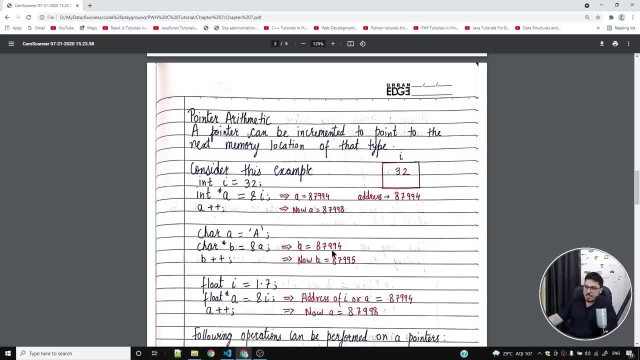 pointer b, which is actually the address, pointer b, which is actually the address of this character a. and let us assume of this character a, and let us assume of this character a, and let us assume that b is 87994. b is the address of a, that b is 87994 b is the address of a. 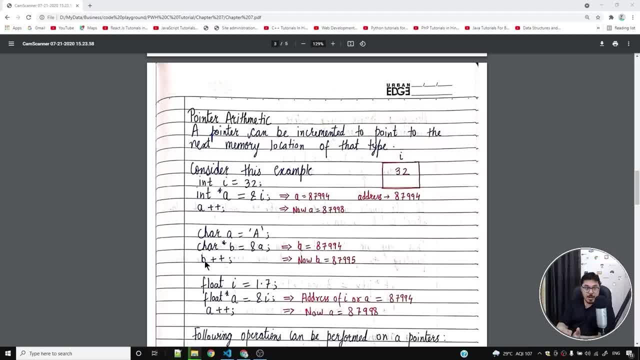 that b is 87994, b is the address of a, one to b, but because character takes one to b, but because character takes one to b, but because character takes one byte, so since character takes one, one byte, so since character takes one, one byte, so since character takes one byte, one is added to this address. 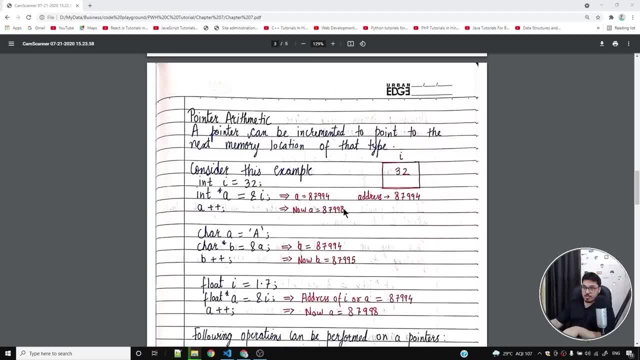 byte one is added to this address. byte one is added to this address since integer takes four bytes. four is since integer takes four bytes. four is since integer takes four bytes. four is added to this address. if we have added to this address, if we have added to this address, if we have another data type that takes, say, nine. 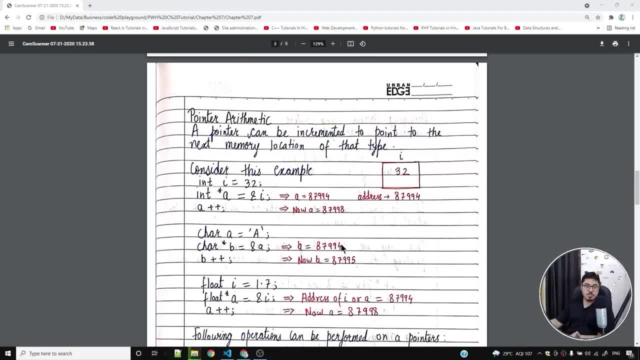 another data type that takes, say, nine. another data type that takes, say, nine, bytes for some reason, bytes for some reason, bytes for some reason. we'll add nine to this address. i hope we'll add nine to this address. i hope we'll add nine to this address. i hope you now understood how pointer. 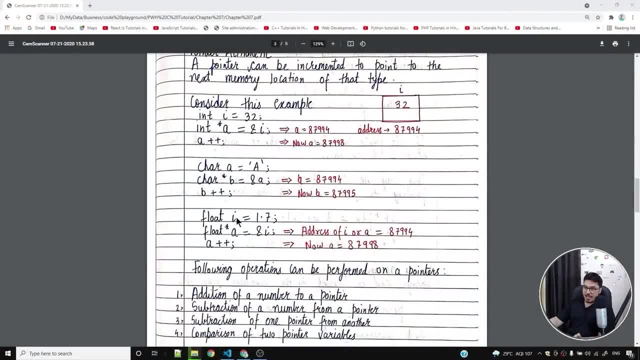 you now understood how pointer you now understood how pointer arithmetic works, arithmetic works, arithmetic works. so if we have something like this float, so if we have something like this float, so if we have something like this float, i is equal to 1.7 and float star a is: 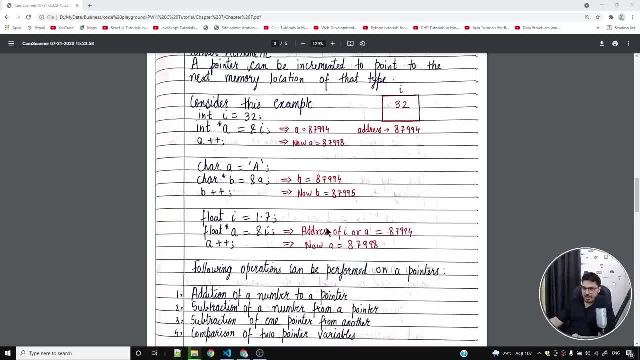 i is equal to 1.7 and float star a is. i is equal to 1.7 and float star a is equal to m percent. i a is actually equal to m percent. i a is actually equal to m percent. i a is actually holding the address of i and since 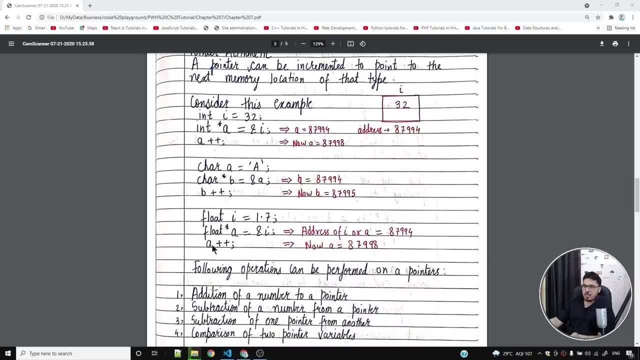 holding the address of i and since holding the address of i, and since float takes four bytes in this float takes four bytes in this float takes four bytes in this architecture, architecture, architecture. a plus plus will change a from 87994. a plus plus will change a from 87994. 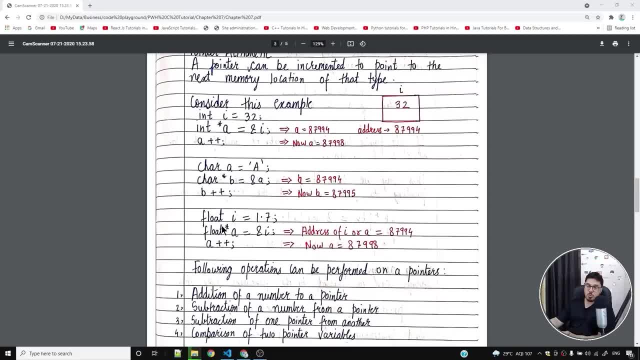 a plus plus will change a from 87994 to 87998, so it will add four to it. why to 87998, so it will add four to it. why to 87998, so it will add four to it. why? because float takes four bytes in memory. 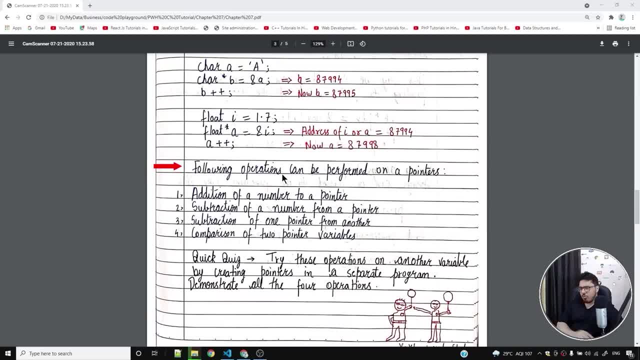 because float takes four bytes in memory. because float takes four bytes in memory. i hope you are clear with all these. i hope you are clear with all these. i hope you are clear with all these. things now. so things now. so things now. so following operators can be performed. 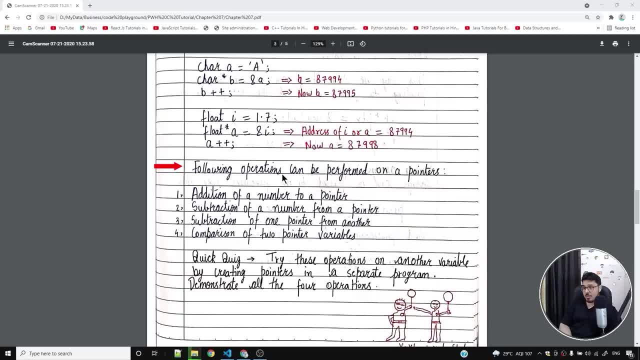 following operators can be performed: following operators can be performed: sorry following operations can be sorry: following operations can be sorry: following operations can be performed on the pointers: performed on the pointers: performed on the pointers: you can add addition of a number to a. you can add addition of a number to a. 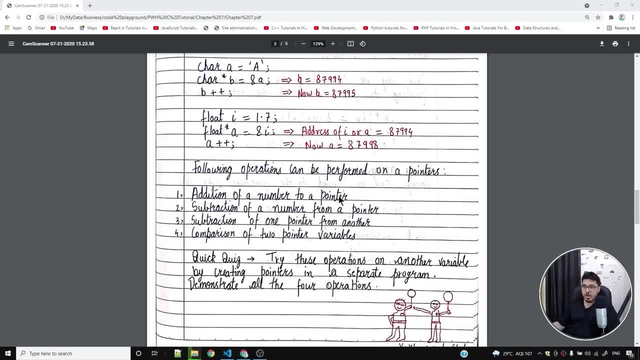 you can add addition of a number to a pointer. you can add a number to a pointer. you can add a number to a pointer. you can add a number to a pointer. if you add two to a pointer, it pointer. if you add two to a pointer, it. 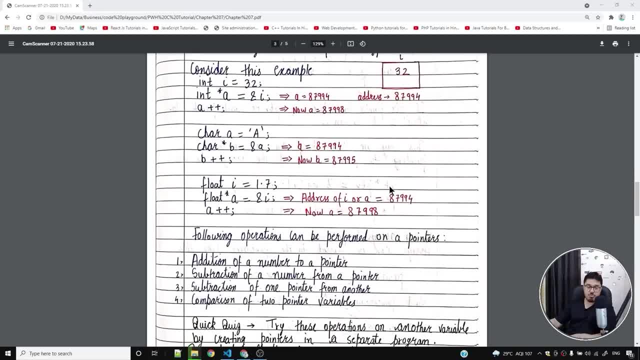 pointer. if you add two to a pointer, it will point to the next to next integer will point to the next to next integer will point to the next to next integer, if it is of integer type. subtraction of: if it is of integer type, subtraction of: if it is of integer type. subtraction of a number from a pointer is also possible. 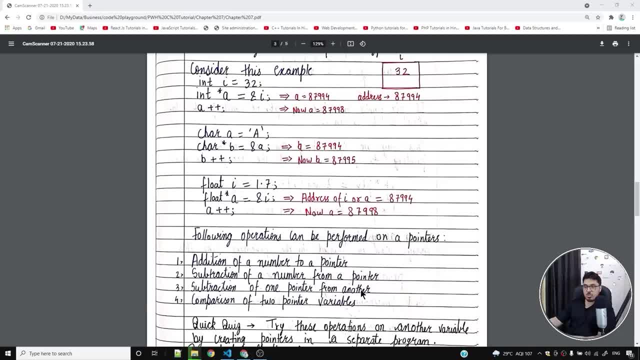 a number from a pointer is also possible. a number from a pointer is also possible. subtraction of one, subtraction of one. subtraction of one pointer from another is also possible. pointer from another is also possible. pointer from another is also possible. comparison of two pointer variables is. comparison of two pointer variables is. 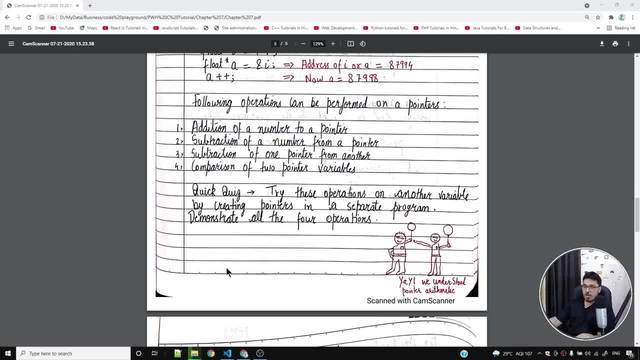 comparison of two pointer variables is also possible. so you can do all these also possible. so you can do all these also possible. so you can do all these operations, operations, operations. you can compare two pointers, you can add. you can compare two pointers, you can add. you can compare two pointers. you can add and subtract two pointers, and so on. so i 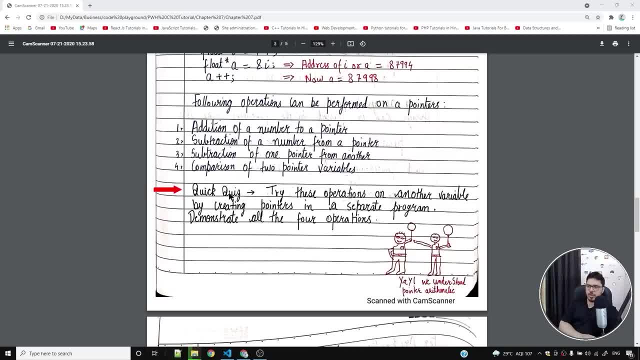 and subtract two pointers and so on. so i and subtract two pointers, and so on. so i hope you understood pointer arithmetic. hope you understood pointer arithmetic. hope you understood pointer arithmetic now. now, there is a quick quiz for you now. now, there is a quick quiz for you. 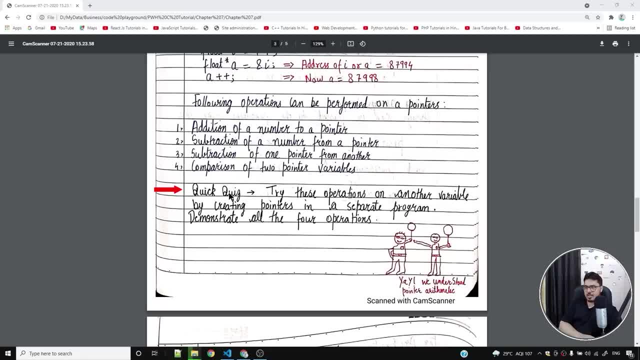 now. now there is a quick quiz for you. try these operations on another. try these operations on another. try these operations on another. variables- by creating pointers in a variables. by creating pointers in a variables. by creating pointers in a separate program. demonstrate all the separate program. demonstrate all the. 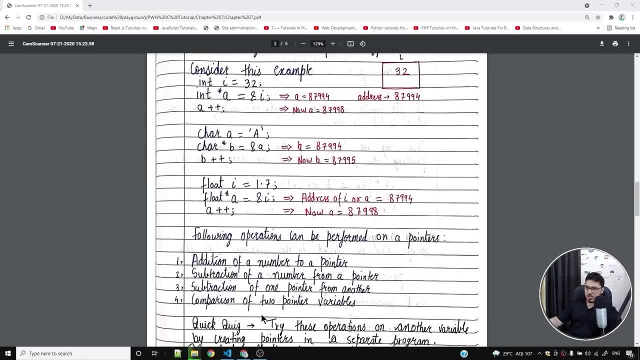 separate program. demonstrate all the four operations. so you need to four operations, so you need to four operations, so you need to demonstrate all these four operations. so demonstrate all these four operations, so demonstrate all these four operations. so let's try to, you know, demonstrate this. let's try to, you know, demonstrate this. 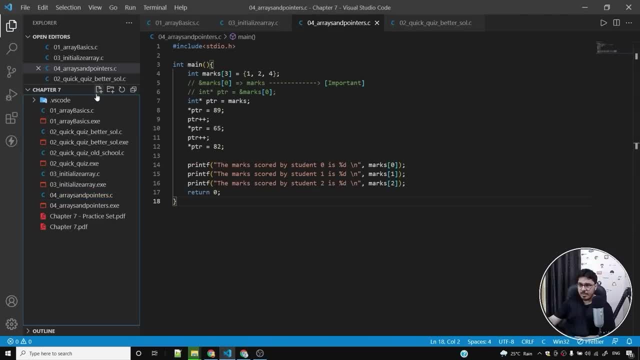 let's try, to you know, demonstrate this using code. so what i'll do is i'll create using code. so what i'll do is i'll create using code. so what i'll do is i'll create a new file, a new file, a new file. i'll say five underscore and i'll say: 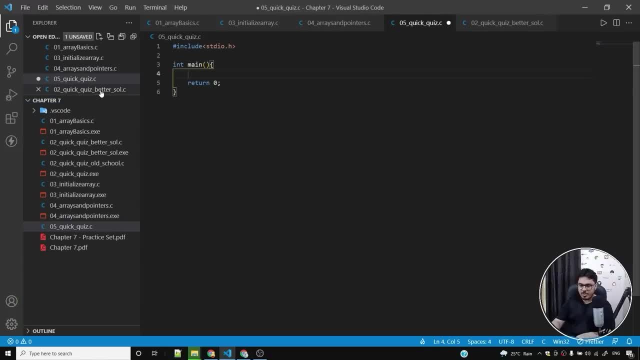 i'll say five underscore and i'll say i'll say five underscore and i'll say quick quiz, quick quiz, quick quiz. dot c. i'll put in the boilerplate code: dot c. i'll put in the boilerplate code: dot c. i'll put in the boilerplate code, i'll zoom in and what i'll do is: 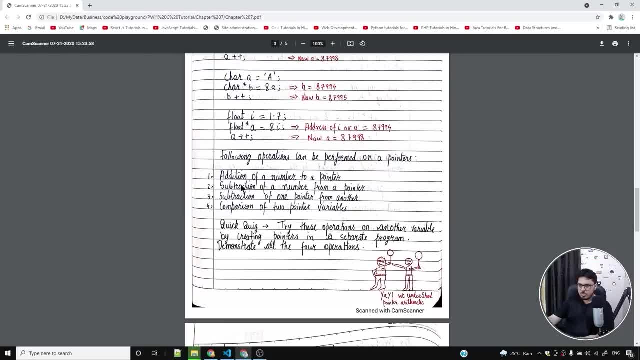 i'll zoom in, and what i'll do is: i'll zoom in and what i'll do is simply, uh, try to demonstrate all these. simply, uh, try to demonstrate all these. simply, uh, try to demonstrate all these things to you, so things to you, so things to you. so the very first operation says: addition of 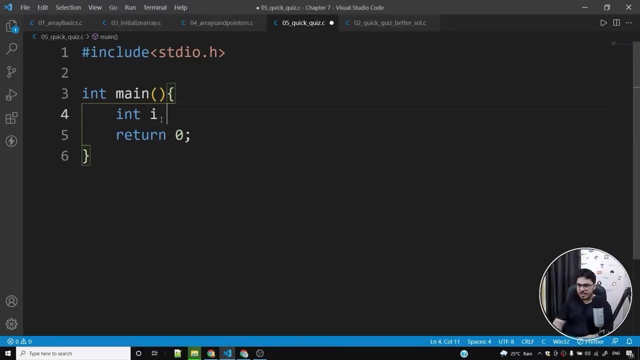 the very first operation says addition of the very first operation says addition of a number to a pointer. but before we do a number to a pointer, but before we do a number to a pointer, but before we do all this, let's say in: i is equal to. 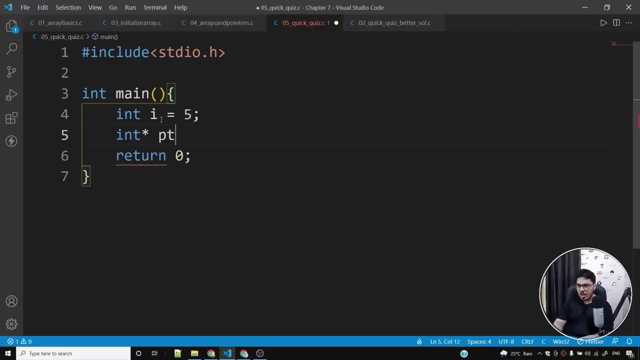 all this, let's say in i is equal to all this. let's say in i is equal to five. and uh, let's say in star, ptr is five. and uh, let's say in star ptr is five. and uh, let's say in star ptr is equal to ampersand i. so now ptr stores. 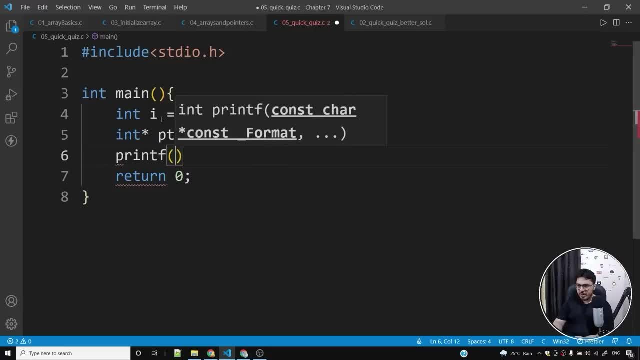 equal to ampersand i. so now ptr stores equal to ampersand i. so now ptr stores the address of i and i will write a the address of i and i will write a the address of i and i will write a bunch of printf statements. what i'll say: 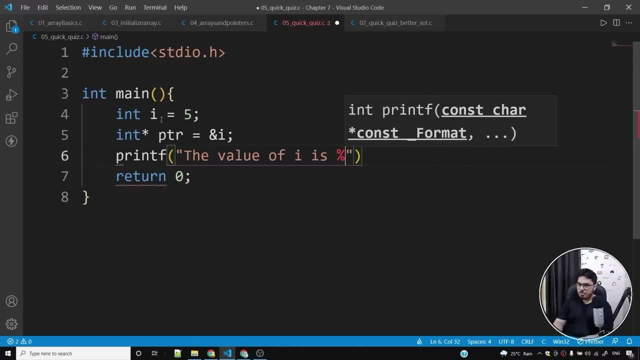 bunch of printf statements. what i'll say? bunch of printf statements. what i'll say is: the value of i is a percentage t is the value of i is a percentage t is the value of i is a percentage t. backslash n, backslash n, and i'll simply. 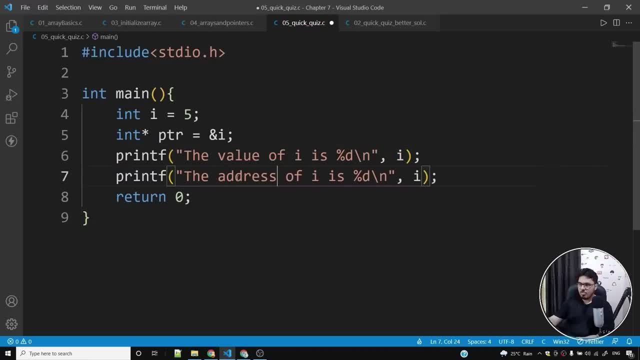 backslash n, backslash n, and i'll simply backslash n, backslash n, and i'll simply say i, and i'll say: the address of i is say i, and i'll say the address of i is say i, and i'll say the address of i is, i'll say ampersand i, or what i'll do is. 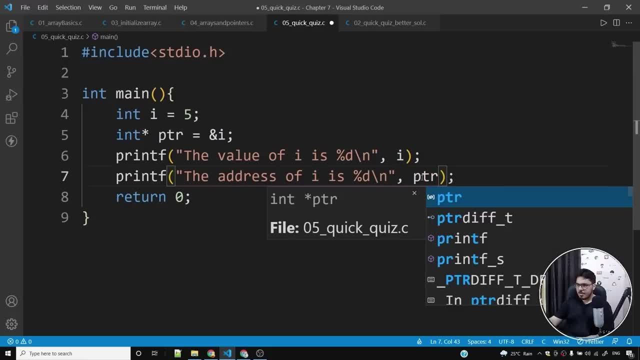 i'll say ampersand i. or what i'll do is: i'll say ampersand i. or what i'll do is i'll say ptr, i'll say ptr, i'll say ptr or other, let me say ampersand i. but uh, what i'll do is i'll say: but uh, what i'll do is i'll say: but uh, what i'll do is i'll say the value of ptr is. i'll also print the the value of ptr is. i'll also print the the value of ptr is. i'll also print the value of ptr. 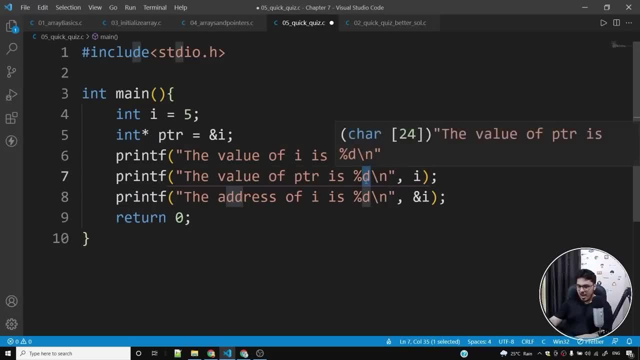 value of ptr. value of ptr: okay. so the value of ptr is percentage u. okay, so the value of ptr is percentage u- okay. so the value of ptr is percentage u and percentage u here as well. because. and percentage u here as well because. and percentage u here as well, because this is an address and i'll say pdr okay. 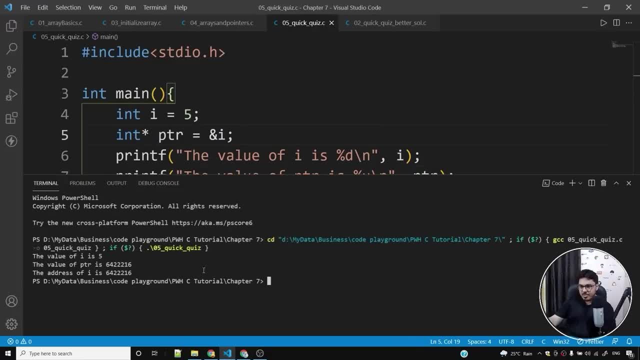 this is an address. and i'll say: pdr, okay, this is an address. and i'll say: pdr, okay, let me run this program for you and see, let me run this program for you, and see, let me run this program for you and see, uh, how this prints, uh, the address of. 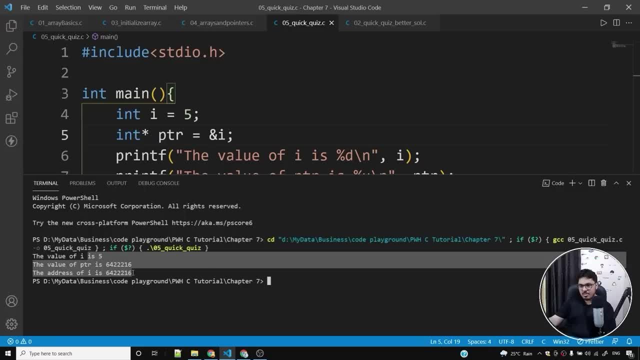 uh, how this prints, uh the address of: uh, how this prints: uh, the address of and the values of i, so value of i is and the values of i, so value of i is and the values of i so value of i is five. address is this. address is this: 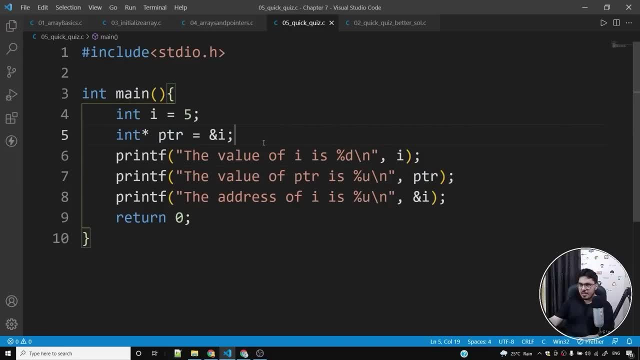 five address. is this address? is this five address? is this address? is this sounds great. now what i'll do is: i'll sounds great. now what i'll do is: i'll sounds great. now what i'll do is: i'll simply say ptr plus plus. simply say ptr plus plus. 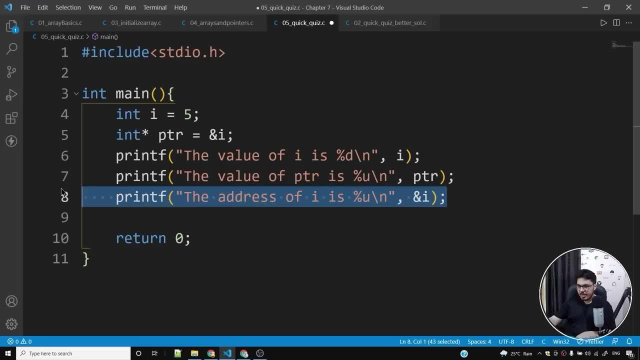 simply say ptr plus, plus. uh, let me, let me do something like this. uh, let me, let me do something like this. uh, let me, let me do something like this. let me copy these two lines. and let me let me copy these two lines. and let me let me copy these two lines and let me replicate. 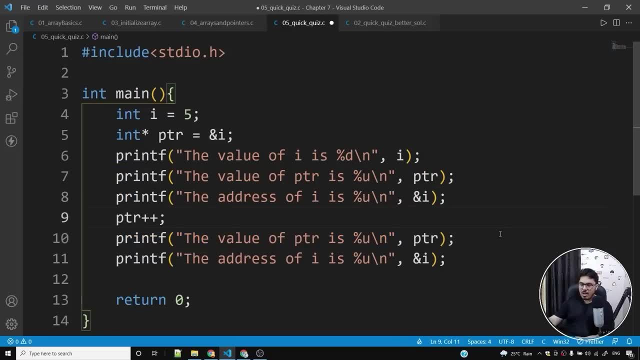 replicate, replicate, and i'll say ptr plus plus. okay, so i and i'll say ptr plus plus. okay, so i and i'll say ptr plus plus. okay, so i have in fact added one to have in fact added one, to have in fact added one to ptr. okay. so let's see the value of ptr. 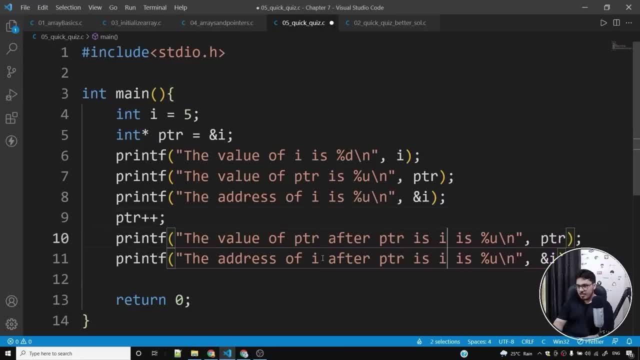 ptr- okay, so let's see the value of ptr. ptr- okay, so let's see the value of ptr after increment, after increment, after increment, after ptr is, after ptr is, after ptr is incremented, is incremented, is, incremented is. so let's see what the value of i is. 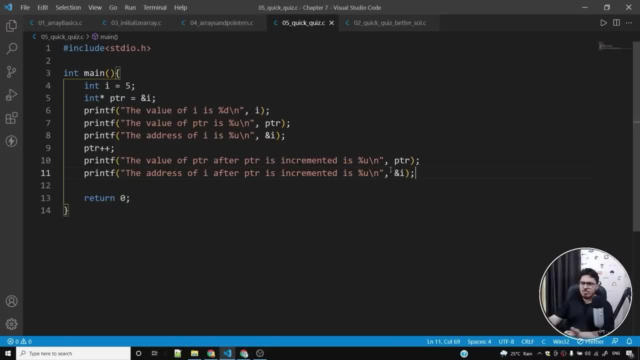 so let's see what the value of i is. so let's see what the value of i is after ptr is incremented, what the value after ptr is incremented, what the value after ptr is incremented, what the value of ptr is of ptr is of ptr is. so the value of i is not going to change. 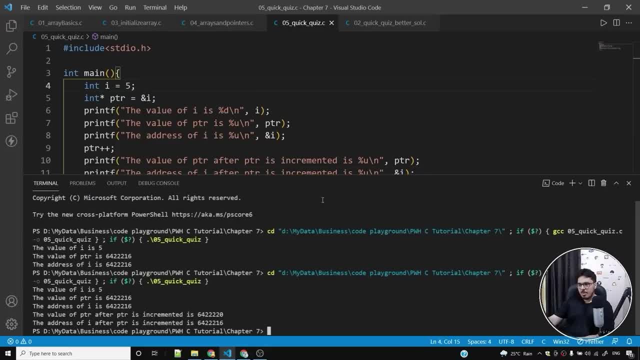 so the value of i is not going to change. so the value of i is not going to change, it will be five, it will be five. it will be five, just like it was before um, the just like it was before um, the. just like it was before um. the address of i will not change because 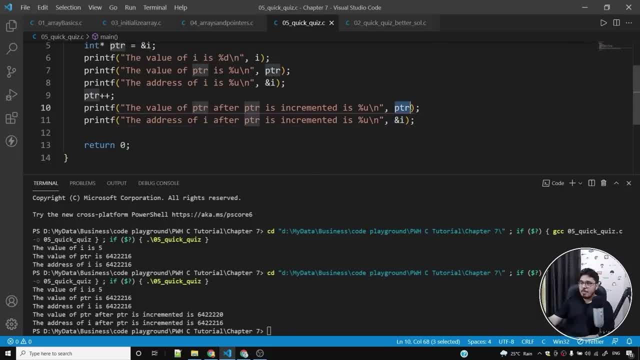 address of i will not change because address of i will not change because it's directly taking address of i. it's directly taking address of i. it's directly taking address of i and the ptr will change and four will. and the ptr will change and four will. 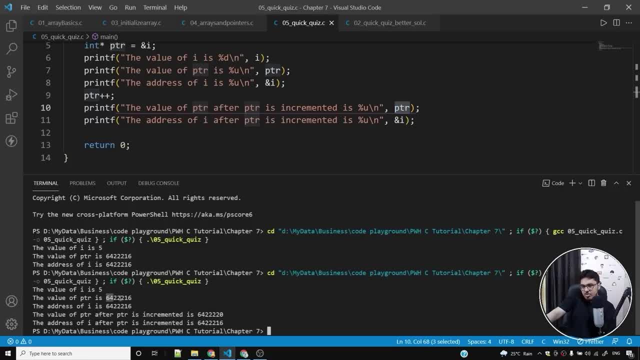 and the ptr will change and four will be added to it. can you see that be added to it? can you see that be added to it? can you see that? so the previous value of ptr was this. so the previous value of ptr was this. so the previous value of ptr was this. now four is added. it's uh 20 previously. now four is added. it's uh 20 previously. now four is added. it's uh 20. previously it was 216, it was 216, it was 216. at the end. now it's two to zero. because at the end now it's two to zero, because 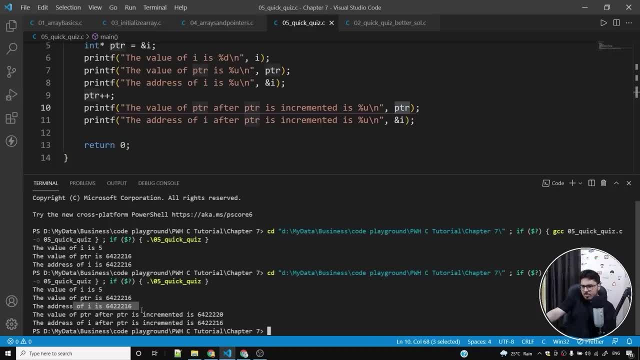 at the end. now it's two to zero because four is added. four is added, four is added. and what about the address of i address of? and what about the address of i address of? and what about the address of i address of? i is not going to change. address of i. i is not going to change address of i. i is not going to change address of i. is the address of i it's not going to. is the address of i? it's not going to. is the address of i. it's not going to change, just like your address is not. 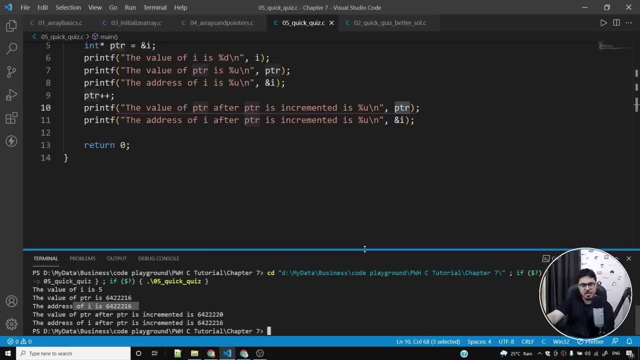 change, just like your address is not change. just like your address is not going to change if you live in going to change. if you live in going to change, if you live in, say mumbai, your address is not going to say mumbai, your address is not going to. 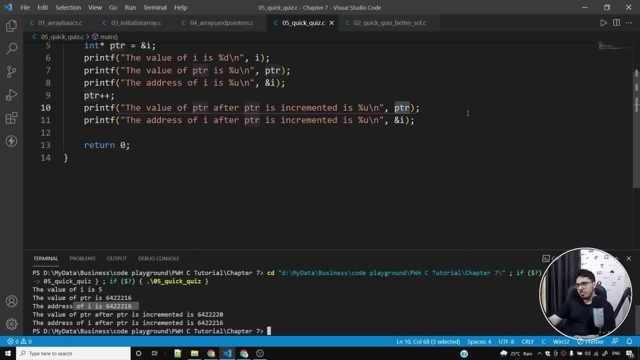 say mumbai, your address is not going to change if you live in change. if you live in change, if you live in hyderabad, your address is not going to hyderabad. your address is not going to hyderabad. your address is not going to change until, unless you are vacating the 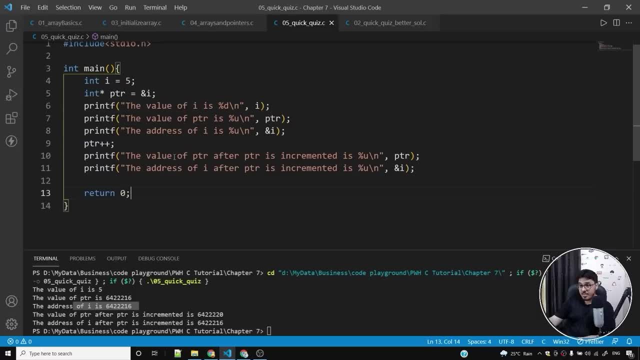 change until unless you are vacating the change, until unless you are vacating the house and moving to some new place house and moving to some new place house and moving to some new place. so i'll say: save this program and what. so i'll say: save this program and what. 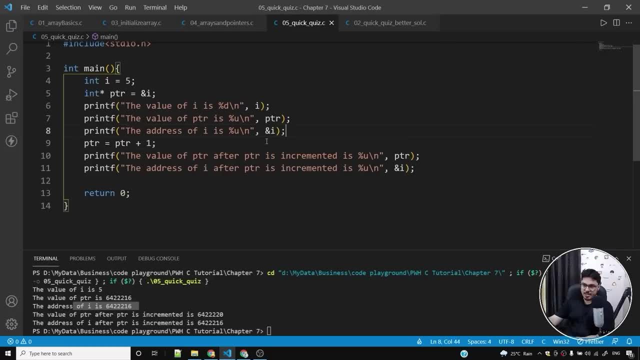 so i'll say: save this program. and what i'll do is i'll say ptr is equal to ptr. i'll do is i'll say ptr is equal to ptr. i'll do is i'll say ptr is equal to ptr plus one. so i can either say ptr plus. 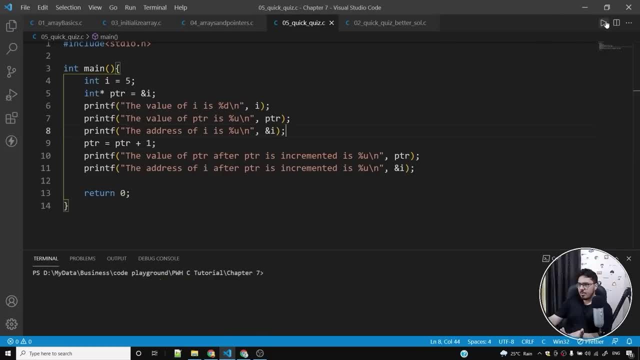 plus one. so i can either say ptr plus plus one. so i can either say ptr plus plus, or i can say ptr is equal to ptr plus, or i can say ptr is equal to ptr plus, or i can say ptr is equal to ptr plus one plus one. 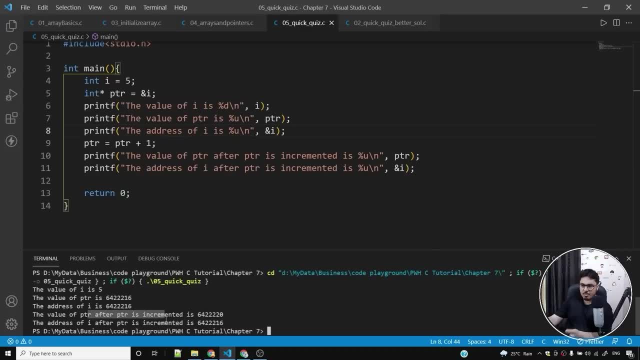 plus one, so we'll get the same results. the value, so we'll get the same results. the value, so we'll get the same results. the value of ptr: after ptr is incremented: is this of ptr? after ptr is incremented: is this of ptr? after ptr is incremented: is this? let me get rid of this line because the 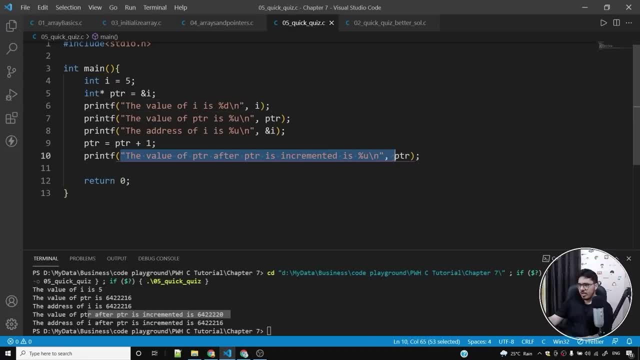 let me get rid of this line because the let me get rid of this line because the address of i is not going to change, address of i is not going to change. address of i is not going to change. uh, let me keep one line, uh, to demonstrate. 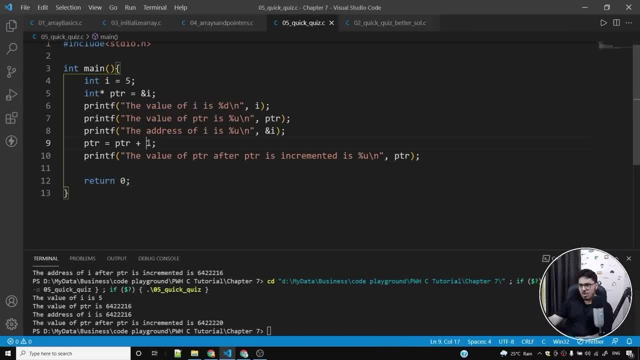 uh, let me keep one line, uh to demonstrate. uh, let me keep one line, uh to demonstrate that ptr is changing now. the ptr is that ptr is changing. now the ptr is that ptr is changing. now the ptr is two to zero. what if i say ptr is equal? 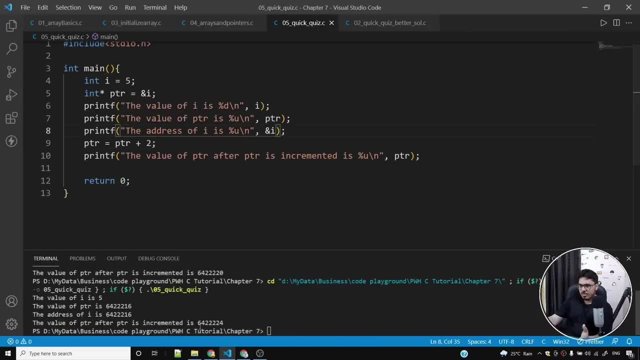 two to zero. what if i say ptr is equal two to zero? what if i say ptr is equal to ptr plus two to ptr plus two to ptr plus two? if i add two to a pointer, eight is going. if i add two to a pointer, eight is going. 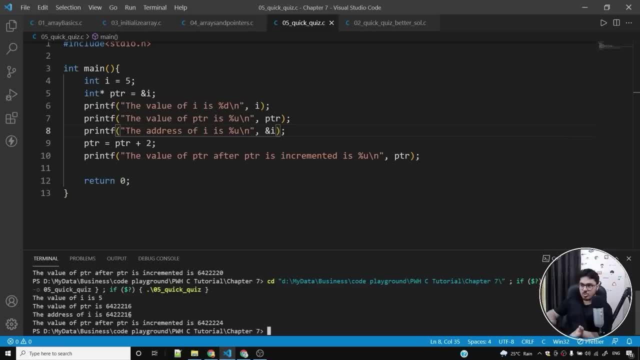 if i add two to a pointer, eight is going to be added to the address of the. to be added to the address of the. to be added to the address of the pointer because it's going to shift the pointer. because it's going to shift the pointer, because it's going to shift the pointer by two places. 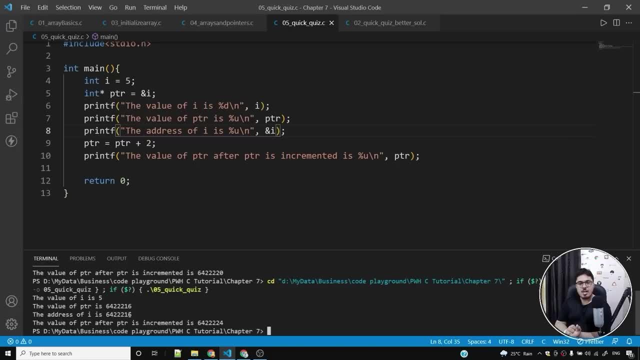 pointer by two places, pointer by two places. and when i say shift the pointer by two, and when i say shift the pointer by two, and when i say shift the pointer by two places, it simply means that places, it simply means that places, it simply means that it's going to shift it by 2. 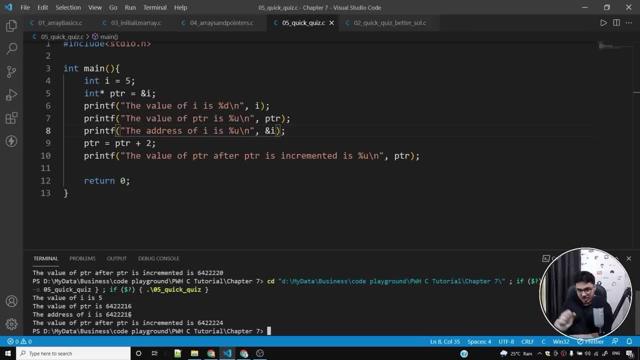 it's going to shift it by 2. it's going to shift it by 2 multiply by the number of bytes taken. multiply by the number of bytes taken. multiply by the number of bytes taken by integer, which is 2 multiplied by 4. by integer, which is 2 multiplied by 4. 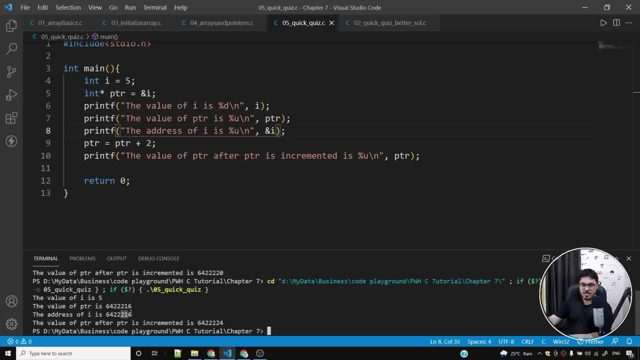 by integer, which is 2 multiplied by 4, which is 8, and hence 8 is added to this, which is 8, and hence 8 is added to this, which is 8, and hence 8 is added to this previous address. i hope that makes sense. 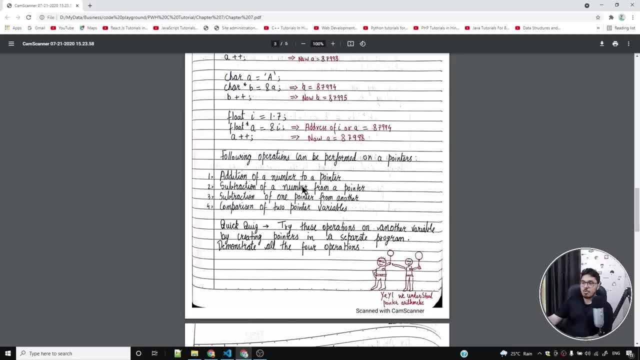 previous address. i hope that makes sense. previous address. i hope that makes sense. so we have added a number to a pointer. so we have added a number to a pointer. so we have added a number to a pointer. now let's subtract a number from a. now let's subtract a number from a. 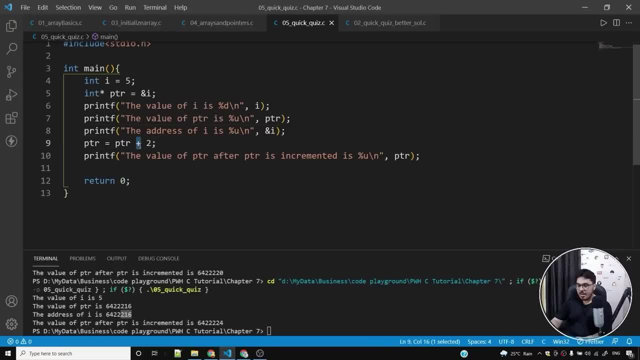 now let's subtract a number from a pointer. i can subtract a number from a pointer. i can subtract a number from a pointer. i can subtract a number from a pointer. so what if i say pointer? so what if i say pointer? so what if i say ptr minus 2? it will be decremented from. ptr minus 2. it will be decremented from ptr minus 2. it will be decremented from the pointer. let me show this to you. so the pointer. let me show this to you. so the pointer. let me show this to you. so it was, it was. 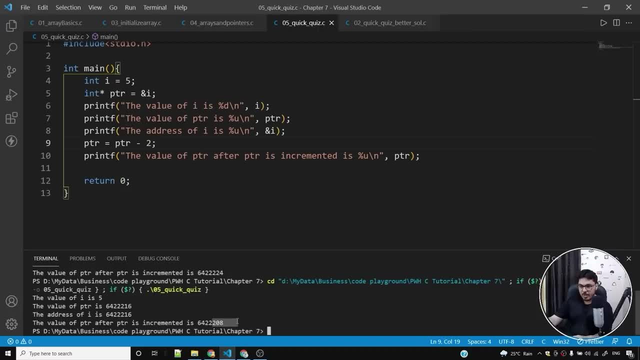 it was 216 before. 216 minus 8 is 208, so it's 208. 216 before 216 minus 8 is 208, so it's 208. 216 before 216 minus 8 is 208, so it's 208 now. 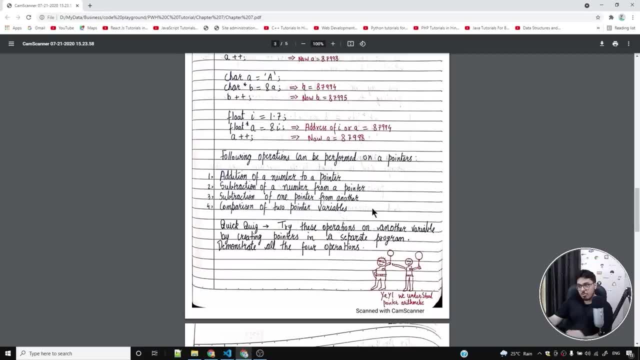 now. now, i hope that makes sense as well. i hope that makes sense as well. i hope that makes sense as well. subtraction of a pointer from another now. subtraction of a pointer from another now. subtraction of a pointer from another now. this is very interesting. this is very interesting. 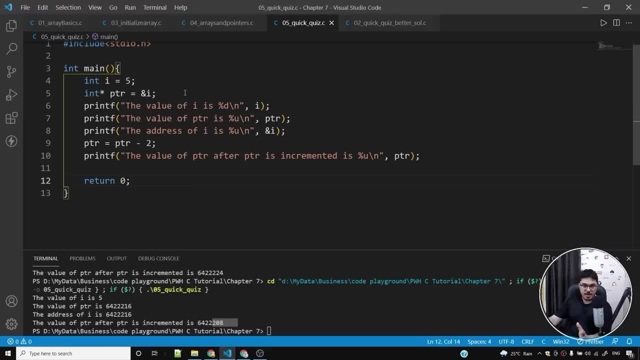 this is very interesting. so let us say i give you. so let us say i give you. so let us say i give you an array okay marks and i tell you that an array okay marks and i tell you that an array okay marks and i tell you that there are 100. 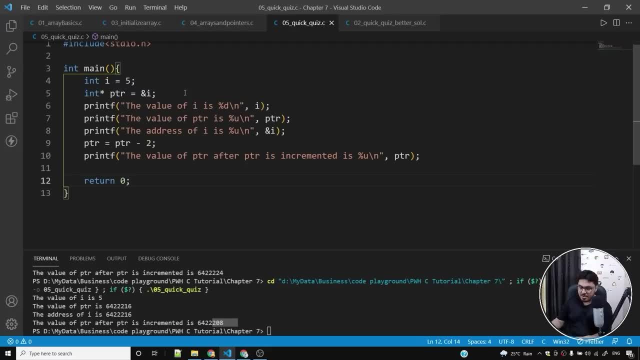 there are 100. there are 100 items in this array. so marks is an array items in this array, so marks is an array items in this array, so marks is an array. there are 100 items in this array i want. there are 100 items in this array i want. 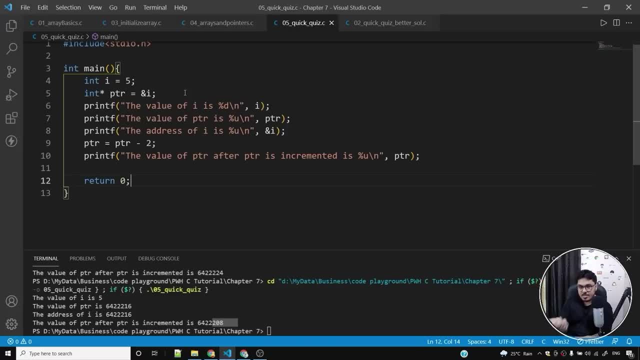 there are 100 items in this array. i want to ask you, to ask you, to ask you: how many bytes does this, how many bytes does this, how many bytes does this array element takes, so you can say array element takes. so you can say array element takes, so you can say marks one minus marks zero. that will be. 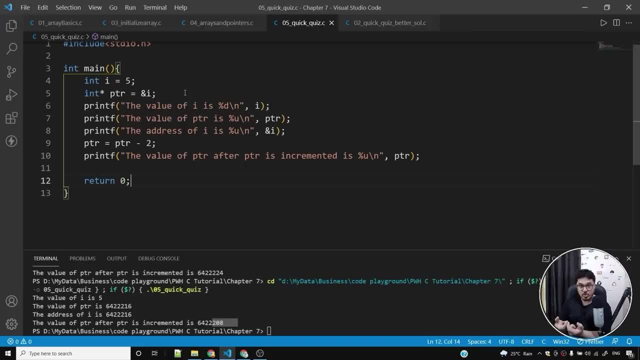 marks one minus marks zero, that will be marks one minus marks zero. that will be the address of marks one minus address. the address of marks one minus address. the address of marks one minus. address of marks zero. and if you of marks zero, and if you of marks zero, and if you, you know, decrement, uh, the value of. 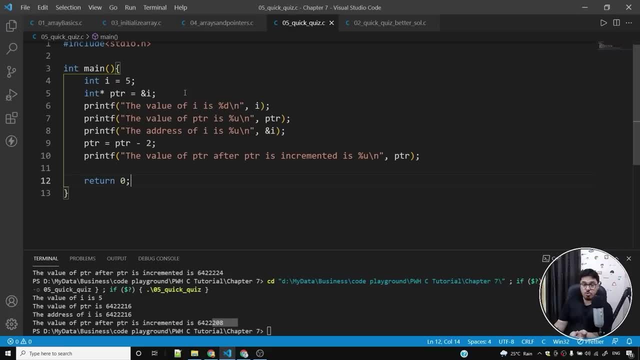 you know decrement, uh, the value of. you know decrement, uh, the value of marks zero from marks one, you'll get marks zero. from marks one, you'll get marks zero. from marks one, you'll get four. if it is an integer, so the four. if it is an integer, so the. 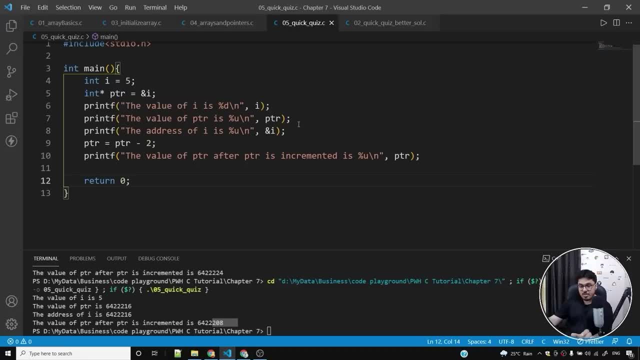 four if it is an integer. so the difference between two addresses will difference between two addresses, will difference between two addresses will actually tell you how many bytes actually tell you how many bytes actually tell you how many bytes each entity is consuming. let me show each entity is consuming. let me show 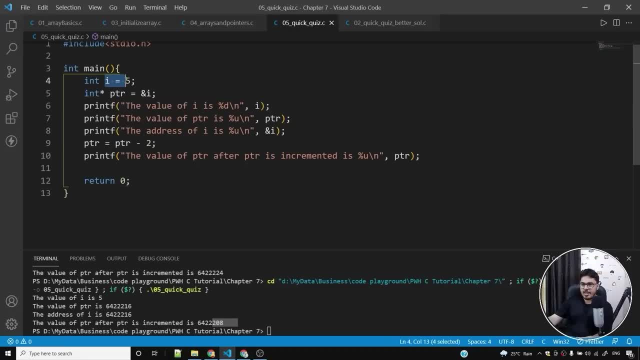 each entity is consuming. let me show this to you. so if i say this to you, so if i say this to you, so if i say int, i is equal to 5 and if i say ptr is, int i is equal to 5 and if i say ptr is, 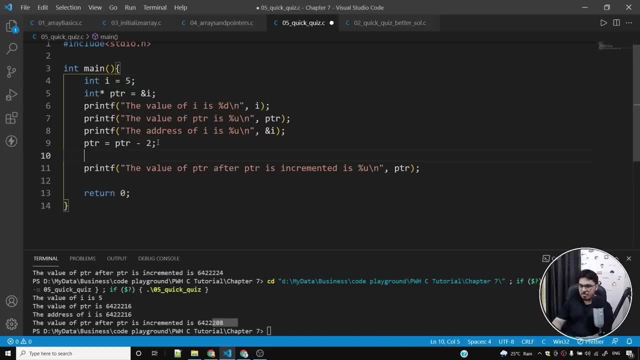 int i is equal to 5, and if i say ptr is equal to ptr minus 2, equal to ptr minus 2, equal to ptr minus 2. what if i say ptr minus instead? of? what if i say ptr minus instead? of? what if i say ptr minus instead of printing the ptr? what if i print ptr? 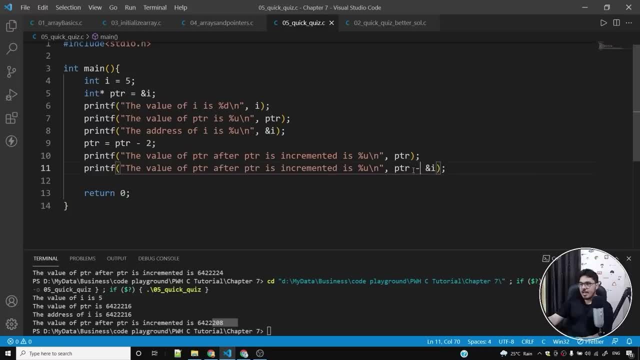 printing the ptr. what if i print ptr? printing the ptr. what if i print ptr minus ampersand i? it will actually tell minus ampersand i. it will actually tell minus ampersand i. it will actually tell me that you have incremented the value, me that you have incremented the value. 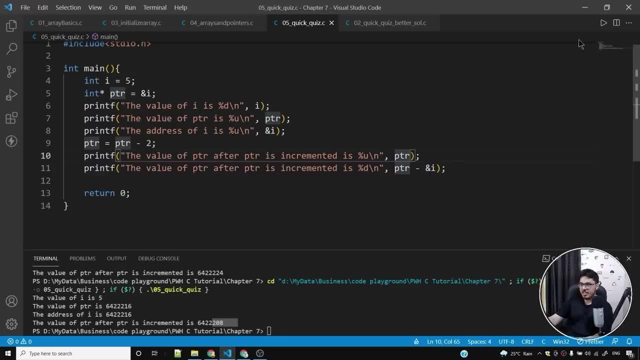 me that you have incremented the value of pointer by these many units. so let me of pointer by these many units. so let me of pointer by these many units. so let me put a percentage d here and let me show. put a percentage d here and let me show. 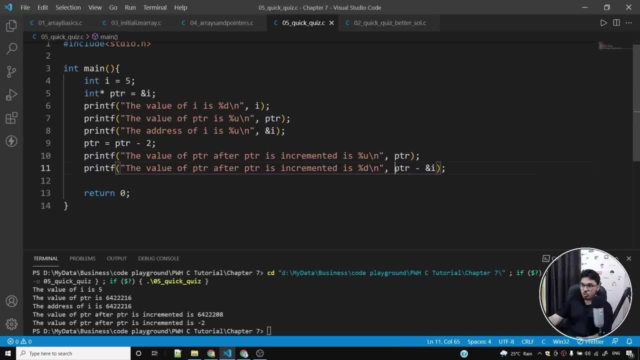 put a percentage d here and let me show you how this works. so when i say you how this works, so when i say you how this works, so when i say percentage d, it will show me two percentage d, it will show me two percentage d, it will show me two and it will not show me the absolute. 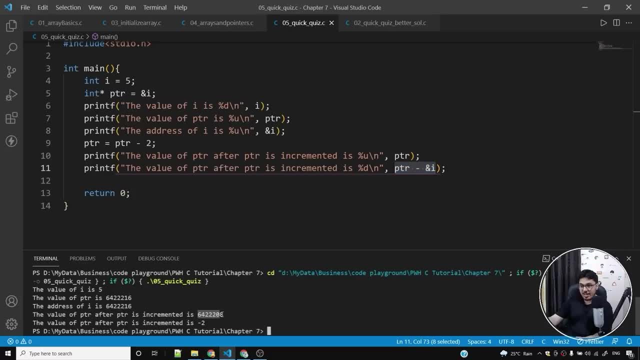 and it will not show me the absolute and it will not show me the absolute difference between these two numbers. no difference between these two numbers, no difference between these two numbers. no, it will not show me that it will. it will not show me that it will. it will not show me that it will actually show me the absolute. 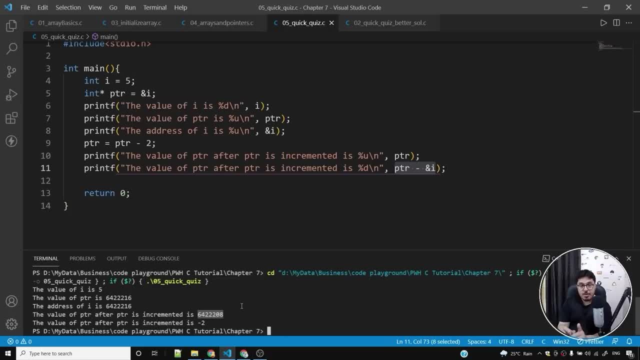 actually show me the absolute. actually show me the absolute difference divided by the number of difference, divided by the number of difference, divided by the number of bytes taken by one unit, which is four bytes, taken by one unit, which is four bytes taken by one unit, which is four. so it will tell me minus four divided. 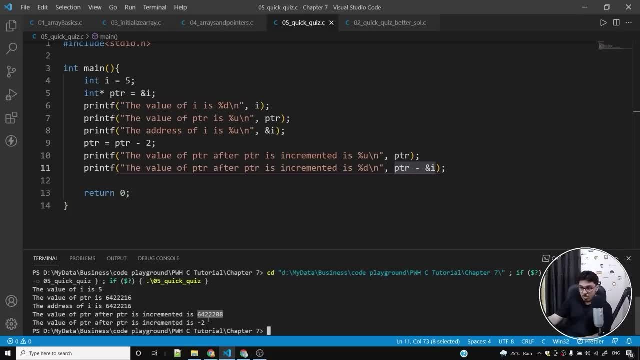 so it will tell me minus four divided. so it will tell me: minus four divided minus eight, divided by minus eight. divided by minus eight, divided by four, which is nothing but minus two, so i four, which is nothing but minus two. so i four, which is nothing but minus two. so i hope this helps you. so this is basically. 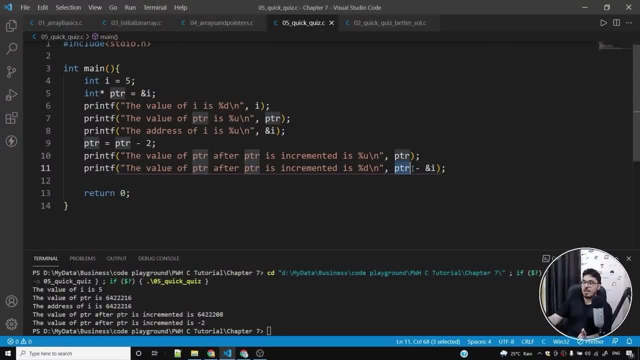 hope this helps you. so this is basically hope this helps you. so this is basically telling me, telling me, telling me. uh, how behind is ptr from the address of? uh, how behind is ptr from the address of? uh, how behind is ptr from the address of? i because we have already decremented. 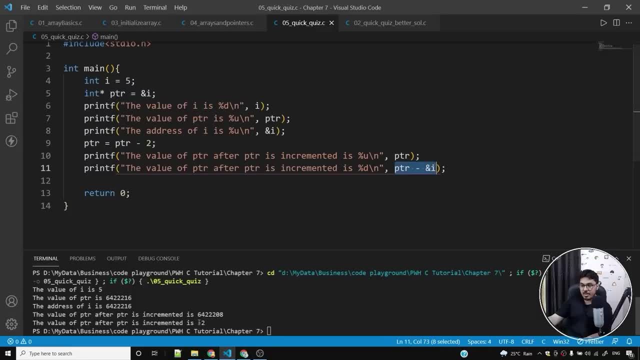 i, because we have already decremented. i because we have already decremented minus two. so it's simply telling me that minus two. so it's simply telling me that minus two. so it's simply telling me that you are, you have decremented, you are, you have decremented. 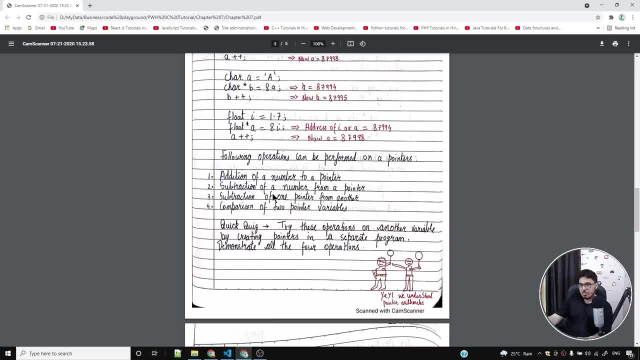 you are. you have decremented the pointer by two. so this is uh how the pointer by two. so this is uh how the pointer by two. so this is uh how subtraction of one pointer from another, subtraction of one pointer from another, subtraction of one pointer from another works. 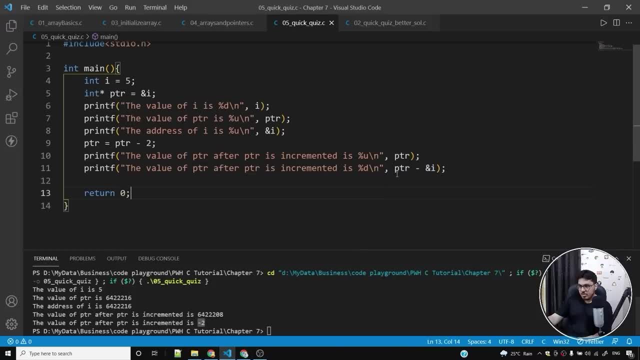 works, works. comparison of two pointers. you can actually comparison of two pointers. you can actually comparison of two pointers. you can actually compare two pointers. so let me show you compare two pointers. so let me show you compare two pointers. so let me show you how comparison of two pointer works. so 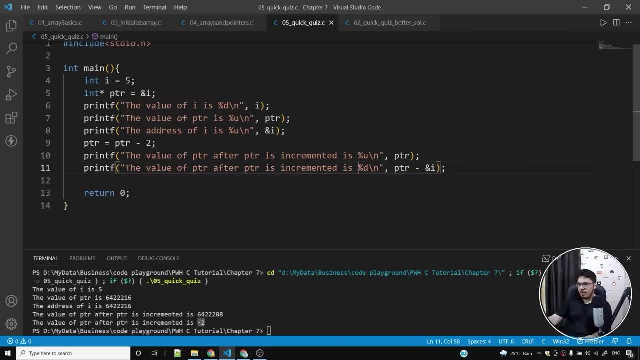 how comparison of two pointer works, so how comparison of two pointer works, so, um, let me get rid of this, um, let me get rid of this, um, let me get rid of this and let me say, uh, the value of comparing, and let me say, uh, the value of comparing. 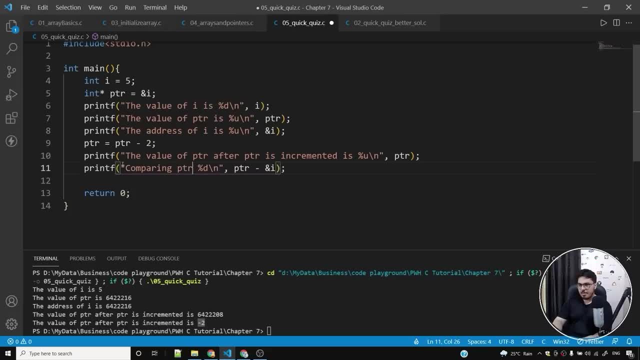 and let me say, uh, the value of comparing two pointers, two pointers, two pointers. let me say comparing ptr with ampersand. let me say comparing ptr with ampersand. let me say comparing ptr with ampersand i or. let me get rid of this and let me. 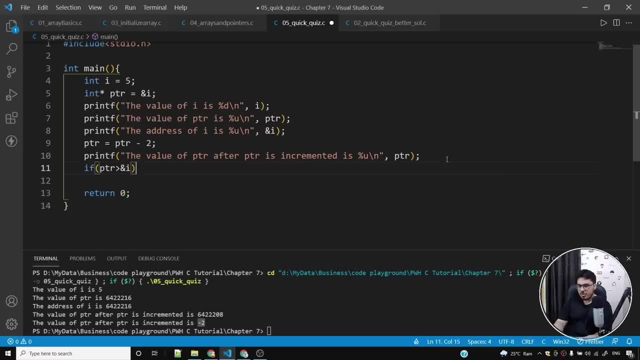 i or let me get rid of this and let me. i or let me get rid of this and let me simply say. simply say: if ptr is greater than ampersand i, i. if ptr is greater than ampersand i, i. if ptr is greater than ampersand i, i can do something like this: 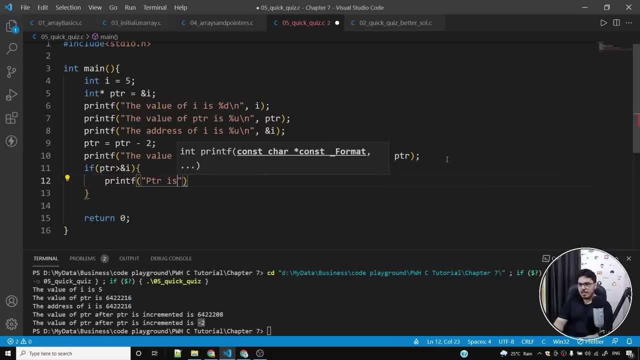 can do something like this, can do something like this, and what else do is? i'll say ptr. and what else do is? i'll say ptr. and what else do is? i'll say ptr is greater and i'll copy: this is greater and i'll copy this. 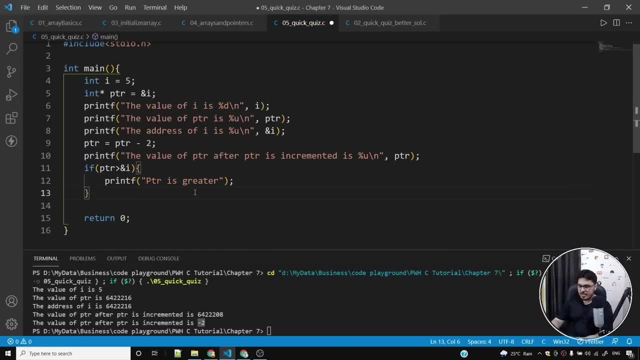 is greater, and i'll copy this particular line and i'll simply say particular line and i'll simply say particular line and i'll simply say else and i'll say: ptr is not greater so this, and i'll say: ptr is not greater so this, and i'll say: ptr is not greater so this will actually tell me whether ptr is. 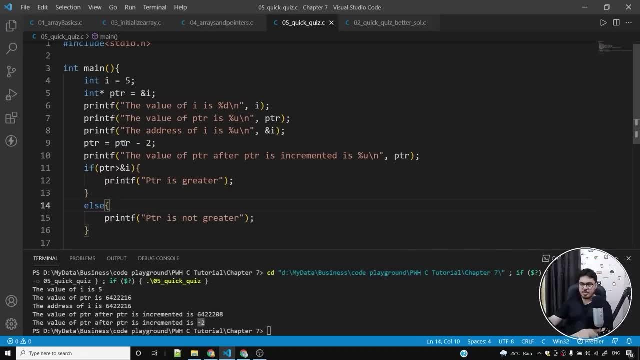 will actually tell me whether ptr is. will actually tell me whether ptr is greater or not, greater or not greater or not. in this case, is ptr greater? no, it's. in this case, is ptr greater? no, it's. in this case, is ptr greater? no, it's not greater, because we have already 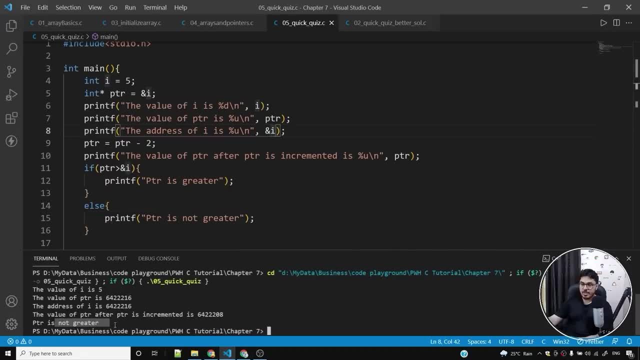 not greater, because we have already not greater, because we have already decremented it by two, so decremented it by two, so decremented it by two. so it should give me ptr is not greater, but it should give me ptr is not greater, but it should give me ptr is not greater. but what if i make it ptr plus two? 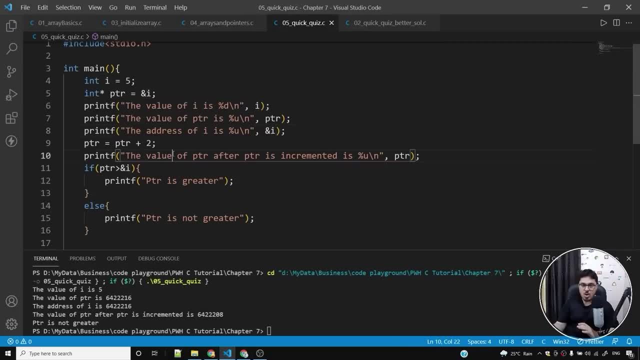 what if i make it ptr plus two? what if i make it ptr plus two? so i can actually find out whether my? so i can actually find out whether my. so i can actually find out whether my address is behind ampersand i. address is behind ampersand i. 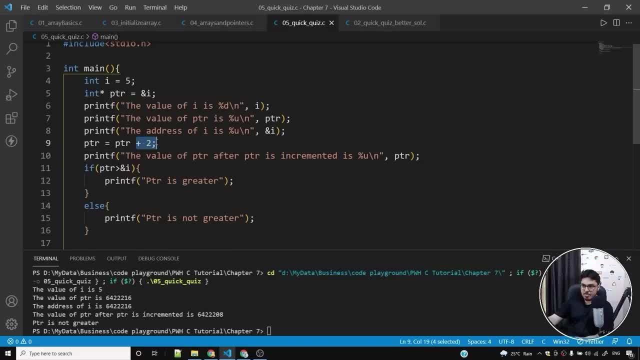 address is behind ampersand i, or is it not behind ampersand i? so, or is it not behind ampersand i? so, since i have incremented two, which is since i have incremented two, which is since i have incremented two, which is i have shifted it by two, values by two. 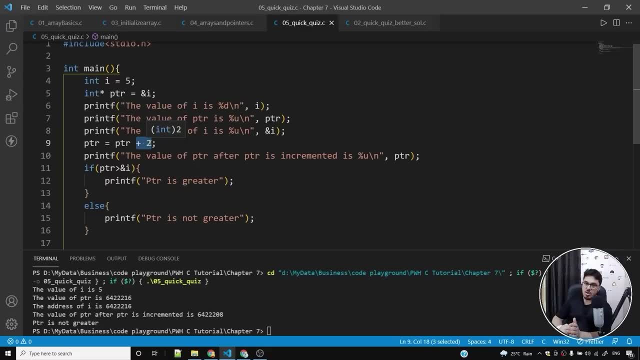 i have shifted it by two values by two. i have shifted it by two values by two: integers, integers, integers, which means that eight units, eight bytes, which means that eight units, eight bytes, which means that eight units, eight bytes, rather have been added to the initial, rather have been added to the initial. 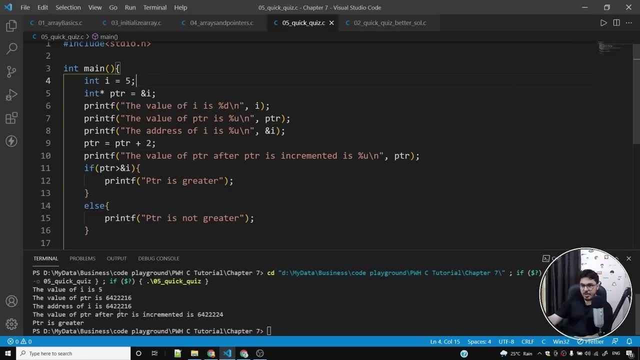 rather have been added to the initial address address: address. so ptr has to be greater now, so ptr is. so ptr has to be greater now, so ptr is. so ptr has to be greater now, so ptr is greater, greater, greater. so we can do pointer comparison, just like. 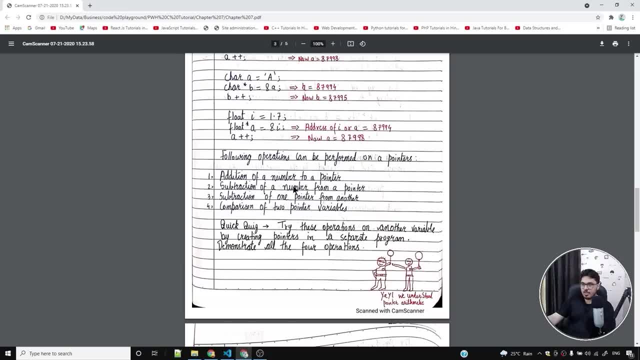 so we can do pointer comparison just like. so we can do pointer comparison just like. we did a pointer subtraction addition. we did a pointer subtraction addition addition. we did a pointer subtraction addition and suppression of a number from a. and suppression of a number from a and suppression of a number from a pointer. i hope that this quick quiz. 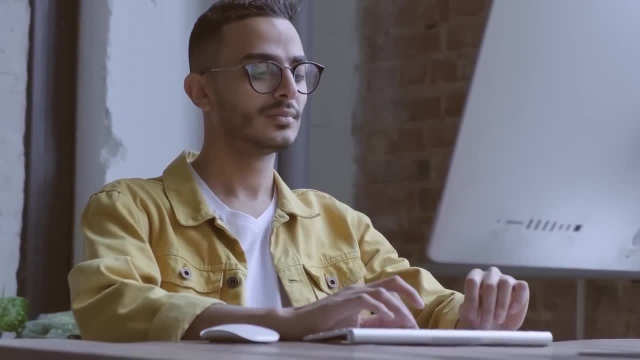 pointer. i hope that this quick quiz pointer. i hope that this quick quiz helps you a lot and will help you, helps you a lot and will help you, helps you a lot and will help you understand all these concepts more, understand all these concepts more, understand all these concepts more clearly. 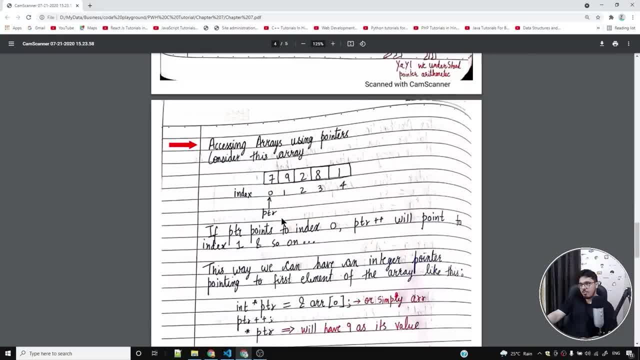 clearly, clearly now accessing arrays using pointers. so now accessing arrays using pointers. so now accessing arrays using pointers. so this is something that i have already. this is something that i have already. this is something that i have already told you that you can actually access, told you that you can actually access. 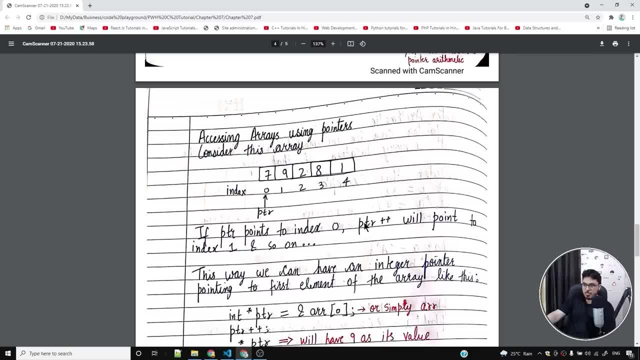 told you that you can actually access an array using pointers. so if ptr points an array using pointers, so if ptr points an array using pointers, so if ptr points to index 0 ptr plus plus will point to. to index 0 ptr plus plus will point to. 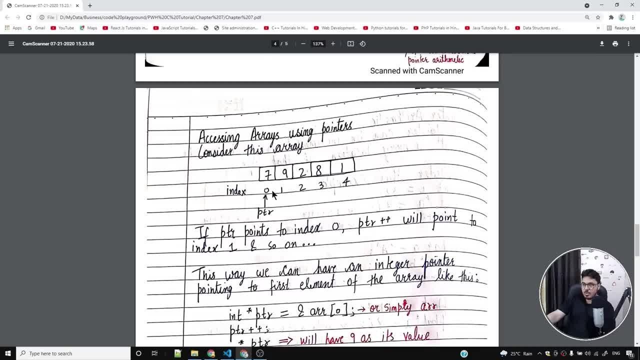 to index 0. ptr plus plus will point to index 1 and so on. so if i say ptr is index 1 and so on, so if i say ptr is index 1 and so on, so if i say ptr is equal to, equal to, equal to amp percent of, let us say, mark 0, which, 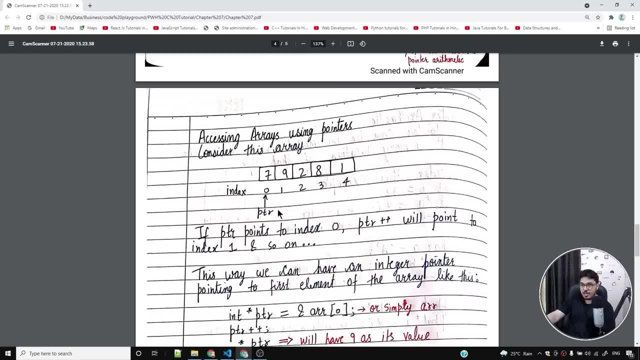 amp percent of, let us say mark 0. which amp percent of let us say mark 0, which is ptr, is pointing to the first element? is ptr is pointing to the first element? is ptr is pointing to the first element of this array? i can do ptr plus plus to. 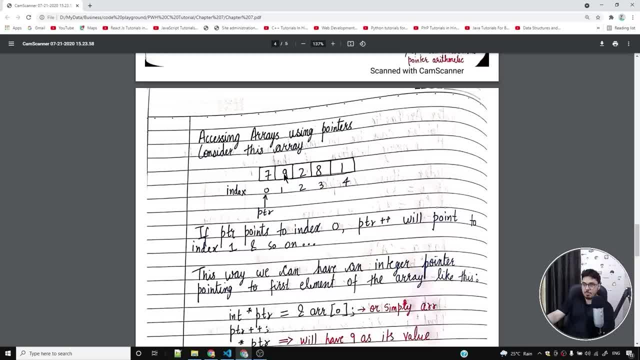 of this array. i can do ptr plus plus to of this array. i can do ptr plus plus to make it point to this number. i can do make it point to this number. i can do make it point to this number. i can do ptr is equal to ptr plus 2 to make it. 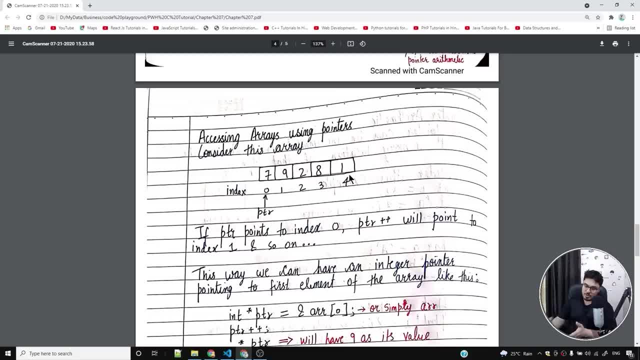 ptr is equal to ptr plus 2. to make it: ptr is equal to ptr plus 2, to make it point to this number, and so on, i can point to this number, and so on, i can point to this number, and so on. i can keep on incrementing this pointer and it. 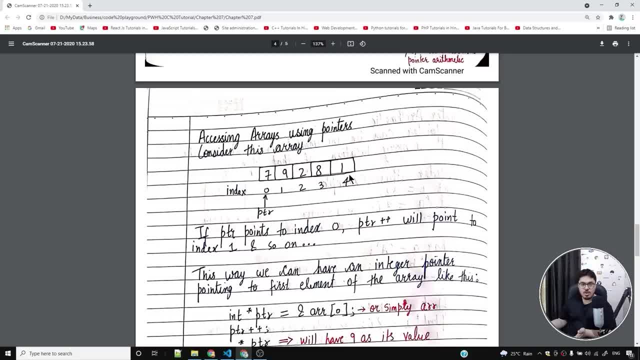 keep on incrementing this pointer, and it keep on incrementing this pointer and it will shift itself to the next value. uh will shift itself to the next value. uh will shift itself to the next value. uh, as in when i keep on incrementing a, as in when i keep on incrementing a. 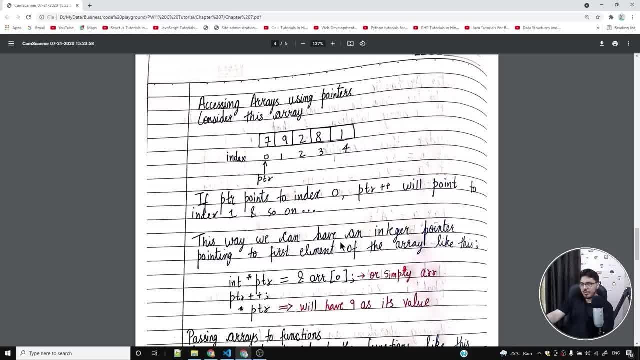 as in when i keep on incrementing a number to it, number to it, number to it. so this way we can have an integer. so this way we can have an integer. so this way we can have an integer. pointer pointing to first element of the pointer, pointing to first element of the. 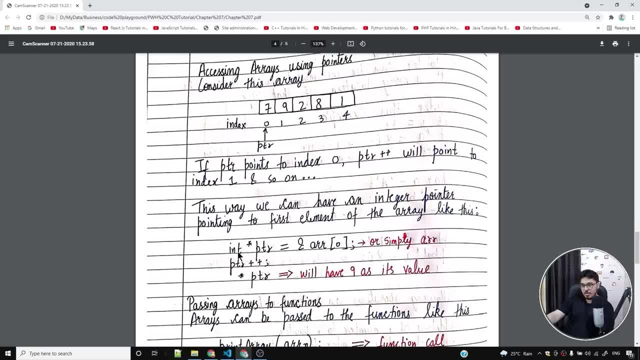 pointer pointing to first element of the array, like this. so i can have integer array. like this. so i can have integer array. like this, so i can have integer pointer pointer, pointer which is in star ptr pointing to the which is in star ptr pointing to the which is in star ptr pointing to the first element of the array. so i can. 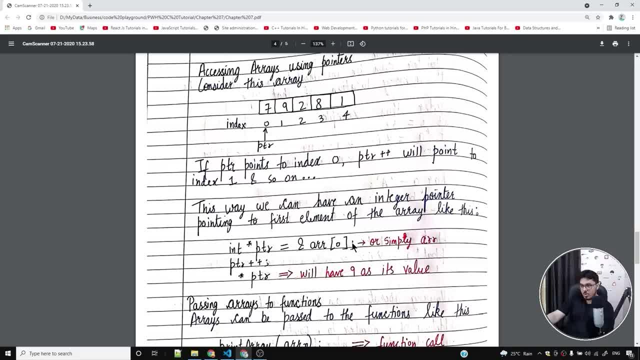 first element of the array, so i can. first element of the array, so i can either say int star ptr is equal to amp, either say int star ptr is equal to amp, either say int star ptr is equal to amp percent and a zero percent and a zero. 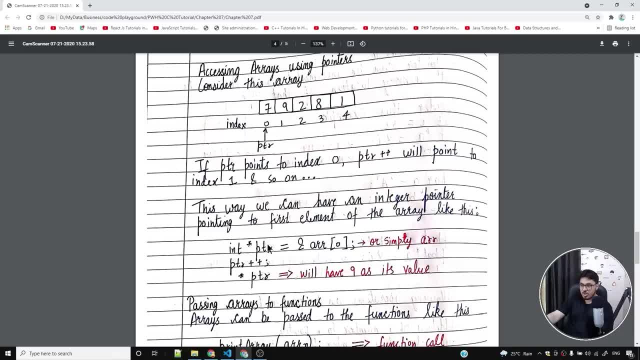 percent and a zero, or i can simply say arr. i can also say: or i can simply say arr. i can also say: or i can simply say arr. i can also say: int star ptr is equal to arr. int star ptr is equal to arr. int star ptr is equal to arr. something i told you here, i've already. something i told you here, i've already. something i told you here i've already told you in arrays and pointers. so either told you in arrays and pointers, so, either told you in arrays and pointers, so either you can do something like this. you can do something like this: 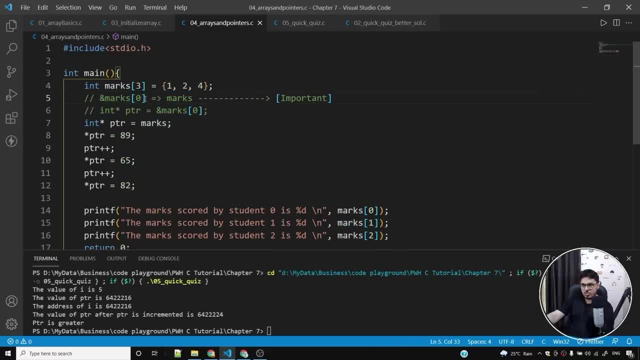 you can do something like this: or you can simply say: marks this also, or you can simply say: marks this also, or you can simply say: marks- this also is equivalent to saying: ampersand mark is equivalent to saying: ampersand mark is equivalent to saying: ampersand mark zero. this will point to the first. 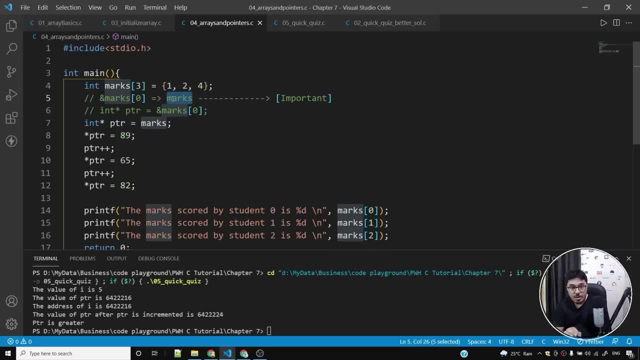 zero. this will point to the first zero. this will point to the first element of the array, the name of the element of the array. the name of the element of the array, the name of the array, will point to the first element of array. will point to the first element of. 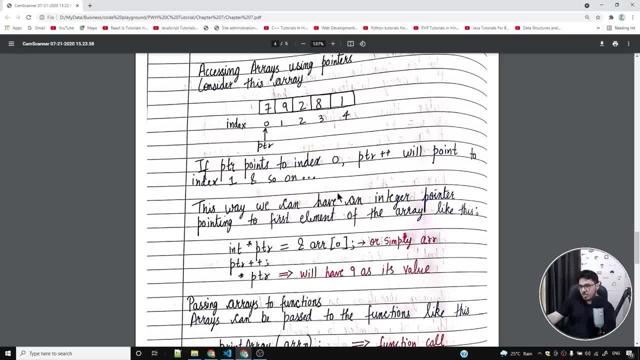 array will point to the first element of the array. this is how you can remember the array. this is how you can remember the array. this is how you can remember it. okay, it okay, it okay. so ptr plus plus will make it point to. so ptr plus plus will make it point to. 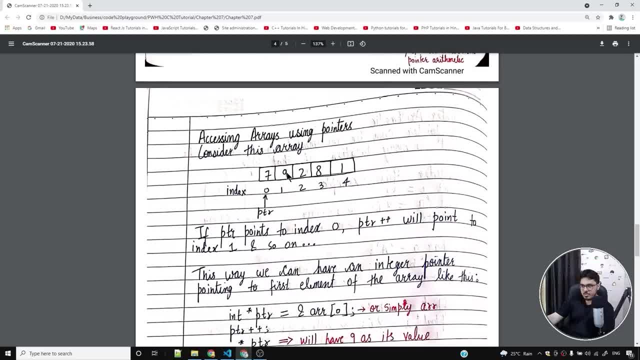 so ptr plus plus will make it point to the next integer. so if you do star ptr, the next integer. so if you do star ptr, the next integer. so if you do star ptr, you will get nine, because this is the. you will get nine because this is the. 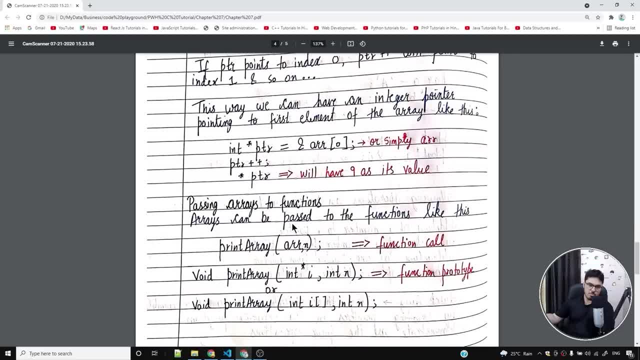 you will get nine, because this is the next integer, next integer, next integer, and so on. you can keep on incrementing and so on, you can keep on incrementing and so on. you can keep on incrementing the pointer and you will keep on the pointer, and you will keep on. 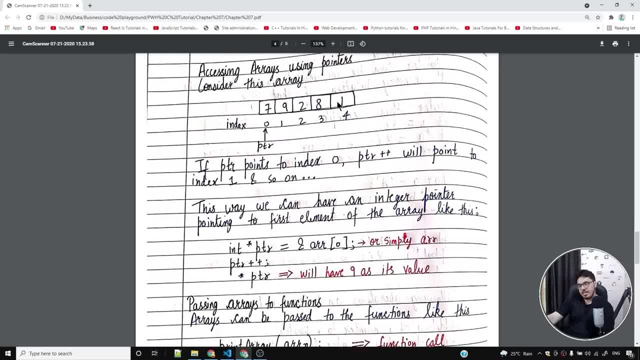 the pointer and you will keep on. you know moving the pointer to the next. you know moving the pointer to the next. you know moving the pointer to the next, next, next, next and the next element and next, next, next, next and the next element and next, next, next, next and the next element, and so on. 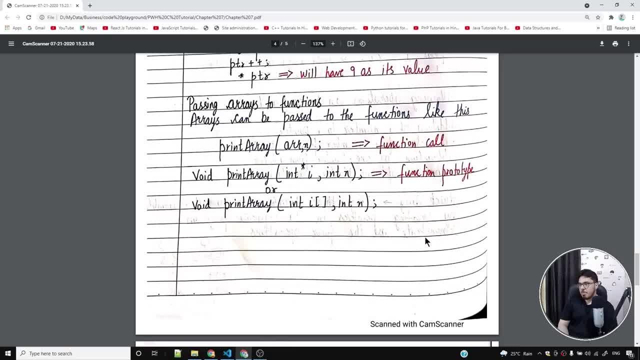 so on, so on. okay, now here comes the interesting part. okay, now here comes the interesting part. okay, now here comes the interesting part wherein we can pass arrays to functions, wherein we can pass arrays to functions, wherein we can pass arrays to functions. we can actually pass arrays to functions. 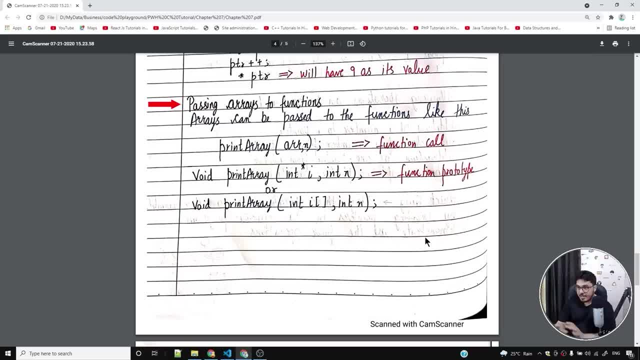 we can actually pass arrays to functions. we can actually pass arrays to functions, and when we are passing arrays to the, and when we are passing arrays to the, and when we are passing arrays to the functions, functions, functions. an entire copy of the array will not be. an entire copy of the array will not be. 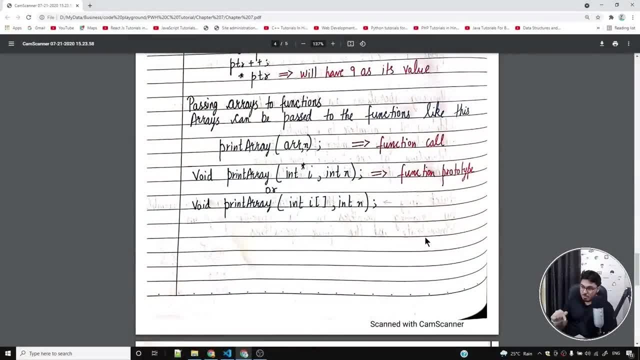 an entire copy of the array will not be created. this is something that you need created. this is something that you need created. this is something that you need to keep in your mind. so many people to keep in your mind, so many people to keep in your mind. so many people think that if they pass an array to 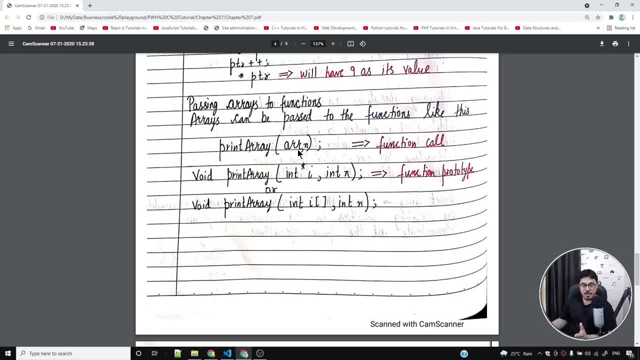 think that if they pass an array, to think that if they pass an array to a function, a copy of the entire array, a function, a copy of the entire array, a function, a copy of the entire array, will be created. no, that is not the case- will be created. no, that is not the case. 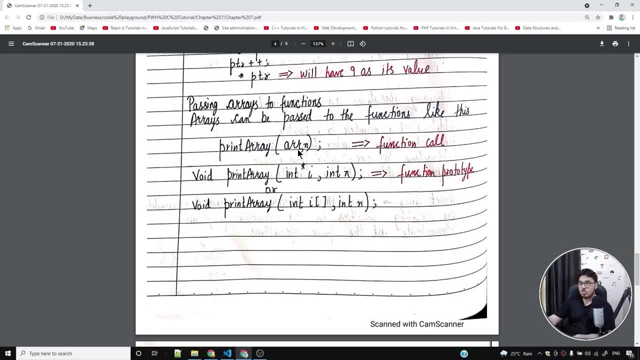 will be created. no, that is not the case. just the address of first element is just the address of first element is just the address of first element is passed and i'm going to demonstrate this. passed and i'm going to demonstrate this. passed and i'm going to demonstrate this to you. so arrays can be passed to the. 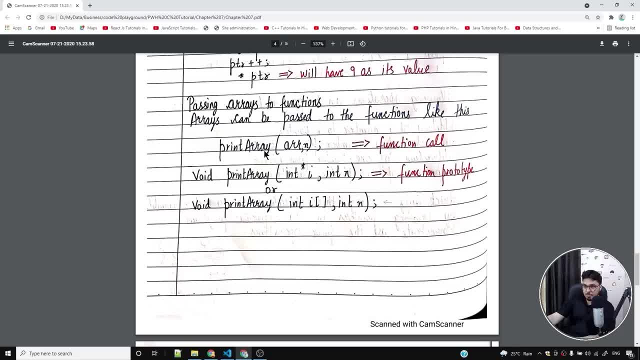 to you so arrays can be passed to the. to you, so arrays can be passed to the function like this: so you can make a function like this: so you can make a function like this. so you can make a function call like this: you can say print. function call like this: you can say print: 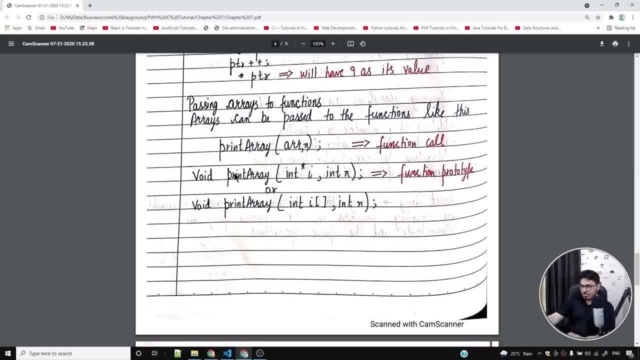 function call like this: you can say print array- arr n and is the size of the array. array arr n and is the size of the array array arr n and is the size of the array. and you can say void print array array and you can say void print array. 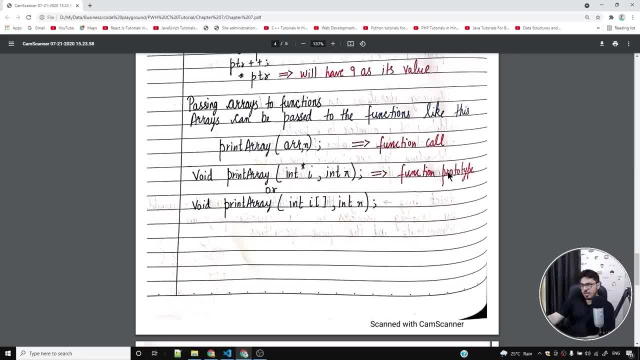 array and you can say: void print array in star i, int n, in star i, int n, in star i, int n. and this is the function prototype. okay, and this is the function prototype. okay, and this is the function prototype. okay, this is the function prototype void. this is the function prototype void. 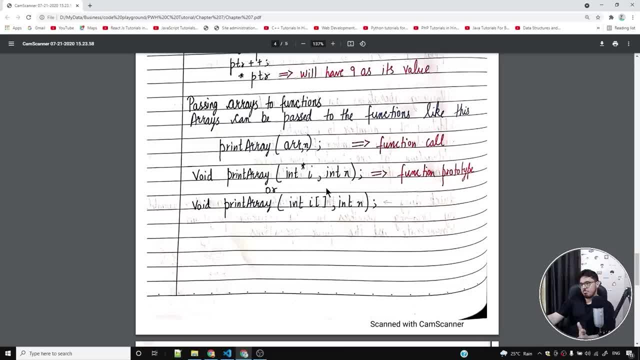 this is the function prototype. void print array: int i- int n. print array int i- int n. print array int i- int n. this is the function prototype, or this: this is the function prototype, or this: this is the function prototype, or this can be the function prototype you can. 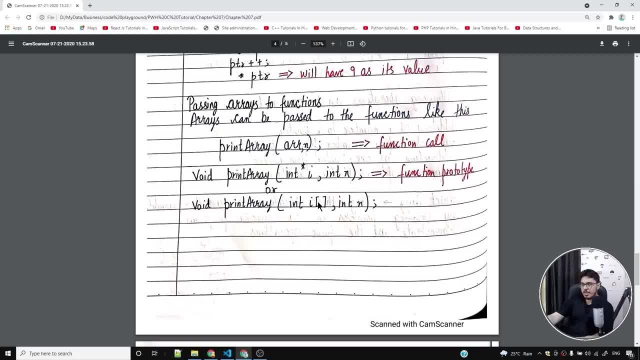 can be the function prototype. you can can be the function prototype. you can either accept this as an address, or you either accept this as an address, or you either accept this as an address, or you can simply, can, simply, can simply accept the array. okay, so this will also. 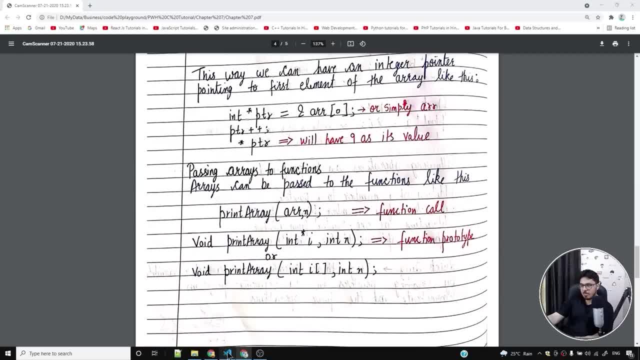 accept the array. okay, so this will also accept the array. okay, so this will also work. the same way, i'll show you how this work. the same way i'll show you how this work. the same way i'll show you how this works, works, works. so let's come to the vs code and let's 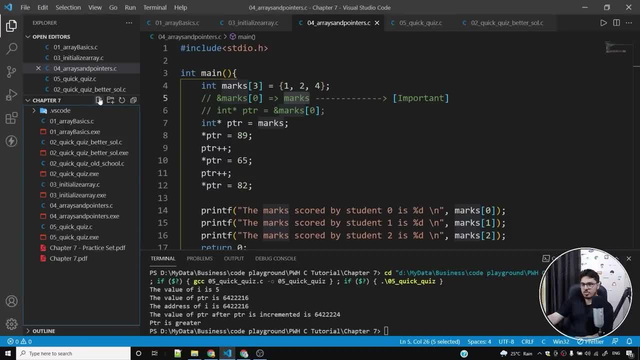 so let's come to the vs code and let's so let's come to the vs code and let's see how we can pass array to functions, see how we can pass array to functions, see how we can pass array to functions. so let me create a file and say 06. 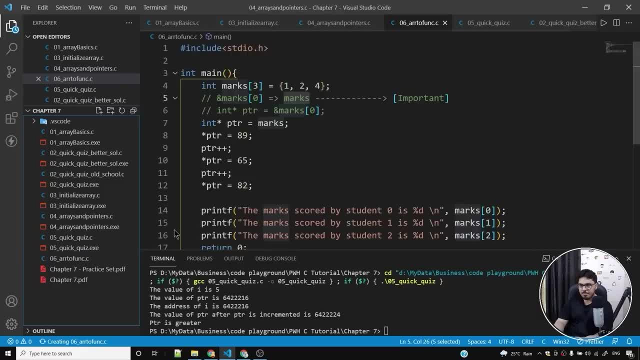 so let me create a file and say 06. so let me create a file and say 06. underscore array to functions dot c. underscore array to functions dot c. underscore array to functions dot c. let me put in the boilerplate code. let me put in the boilerplate code. 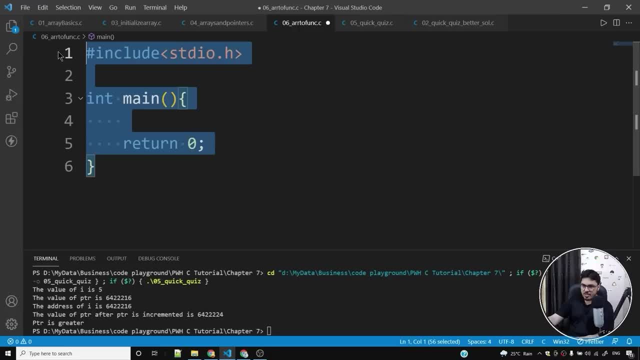 let me put in the boilerplate code and also what i'll do is okay, so i'll. and also what i'll do is okay, so i'll. and also what i'll do is okay, so i'll fix one thing with my snippet, i'll show. fix one thing with my snippet, i'll show. 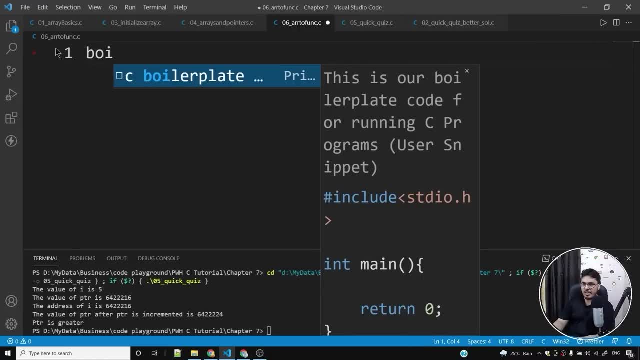 fix one thing with my snippet. i'll show you what is the problem with my snippet you, what is the problem with my snippet you, what is the problem with my snippet. so when i say so, when i say so, when i say c boilerplate and i press enter, and when 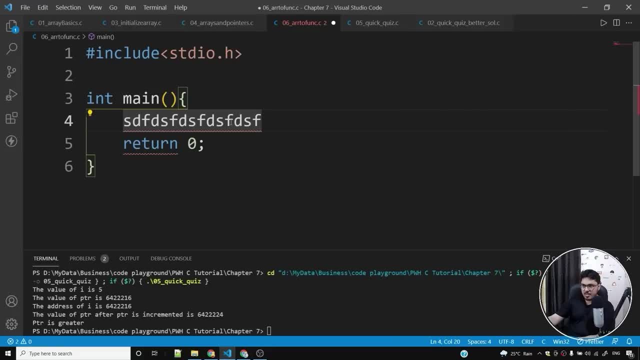 c boilerplate and i press enter, and when c boilerplate and i press enter, and when i'm typing something, can you see this? i'm typing something. can you see this? i'm typing something. can you see this? highlighted stuff here. highlighted stuff here. highlighted stuff here. this is basically telling me that when 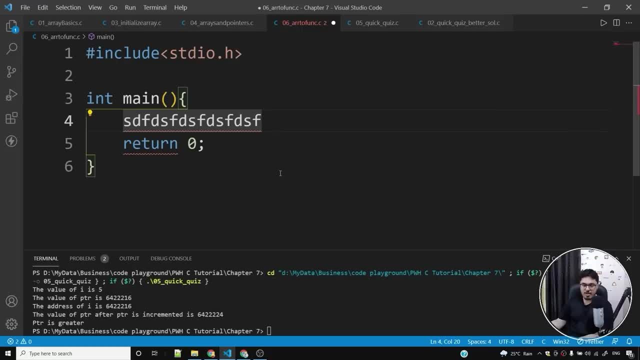 this is basically telling me that when this is basically telling me that when you press tab, you are going to you press tab, you are going to you press tab, you are going to move to some other place. so when i press, move to some other place. so when i press. 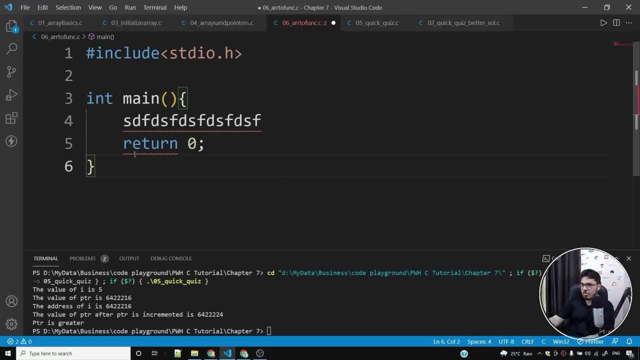 move to some other place. so when i press tab, i'm actually moved to this last line tab. i'm actually moved to this last line tab. i'm actually moved to this last line, but i did not come to this last line. so but i did not come to this last line, so 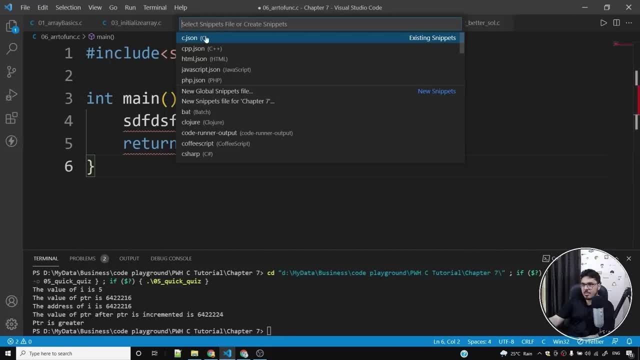 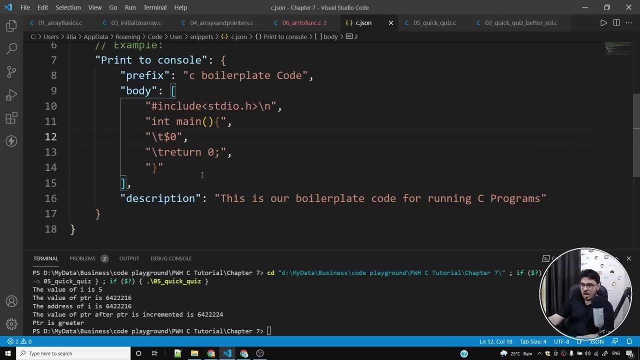 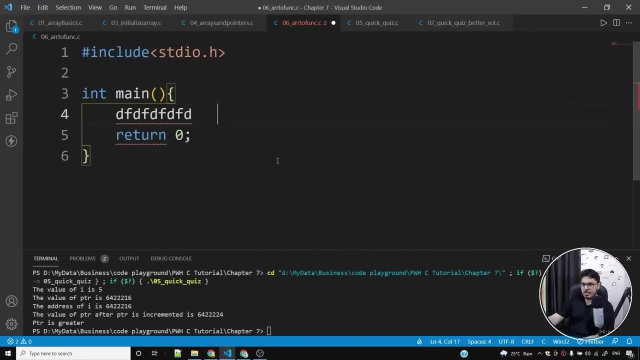 but i did not come to this last line. so in order to fix this, i'll go to my user. in order to fix this, i'll go to my user. in order to fix this. i'll go to my user thing here. pressing tab will not lead me. 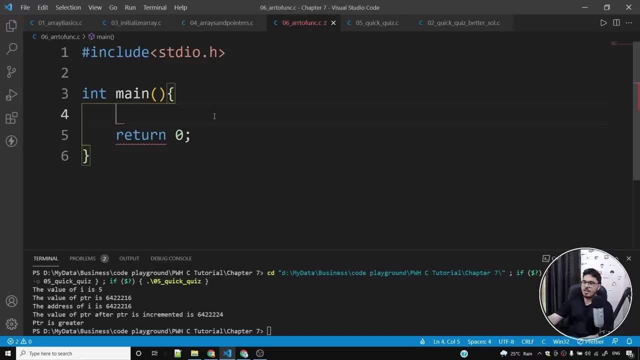 thing here: pressing tab will not lead me. thing here, pressing tab will not lead me here anymore. okay, so this was a basic here anymore. okay, so this was a basic here anymore. okay, so this was a basic problem with my snippet problem with my snippet problem with my snippet and i was just silent about it. i'm glad. 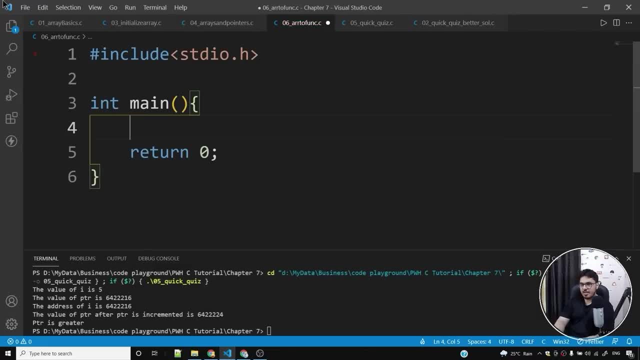 and i was just silent about it. i'm glad and i was just silent about it. i'm glad that i've fixed it, so that i've fixed it, so that i've fixed it, so i can do something like this and i can. i can do something like this and i can. 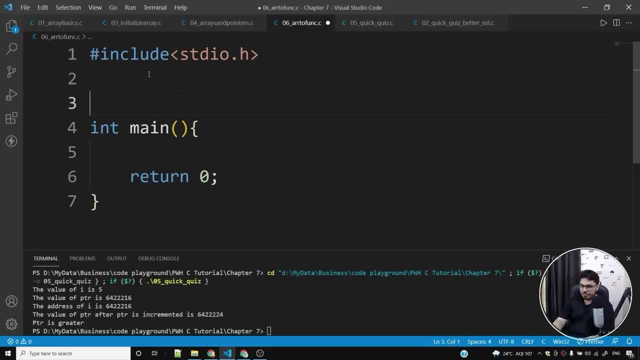 i can do something like this and i can start typing. start typing, start typing anyways. let's try to create a function anyways. let's try to create a function anyways, let's try to create a function. let me call it void funk and it simply. let me call it void funk and it simply. 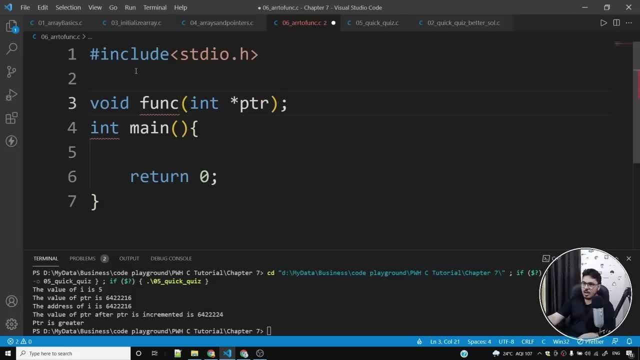 let me call it void funk- and it simply takes up an integer pointer, takes up an integer pointer, takes up an integer pointer. and let me also do something like this. and i don't need do something like this. and i don't need do something like this and i don't need this ptr here. this is a function. 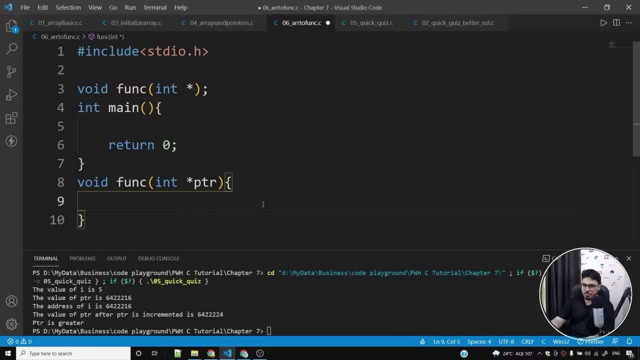 this ptr here. this is a function, this ptr here. this is a function prototype with the semicolon, and this is prototype with the semicolon, and this is prototype with the semicolon, and this is a function body, a function body, a function body. so let us say, i have an array called 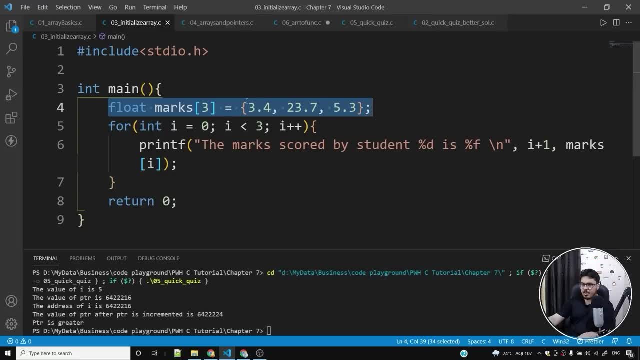 so let us say i have an array called. so let us say i have an array called marks. let me copy it from here. marks. let me copy it from here. marks. let me copy it from here. and i need i need integer array, so let. and i need, i need integer array, so let. 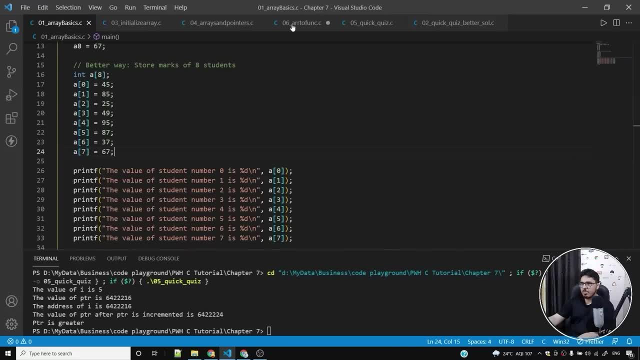 and i need, i need integer array. so let me try to me, try to me. try to get some integer array from somewhere. i'm get some integer array from somewhere. i'm get some integer array from somewhere. i'm too lazy to type. i don't know why. too lazy to type. i don't know why. too lazy to type, i don't know why. let me know in the comments. if you are, let me know in the comments. if you are, let me know in the comments if you are lazy as well. i'm really very lazy, i'm 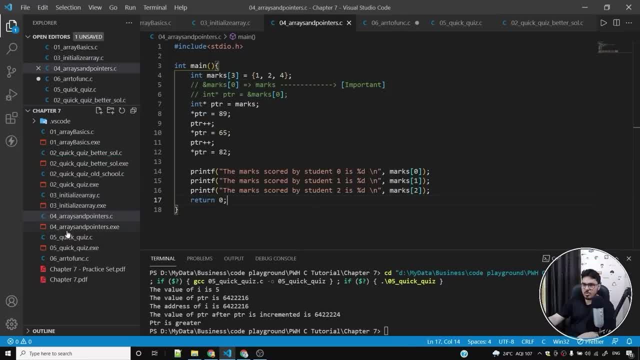 lazy as well. i'm really very lazy. i'm lazy as well. i'm really very lazy. i'm just searching for some array to copy, just searching for some array to copy, just searching for some array to copy from from from. so i unfortunately can't find an array. 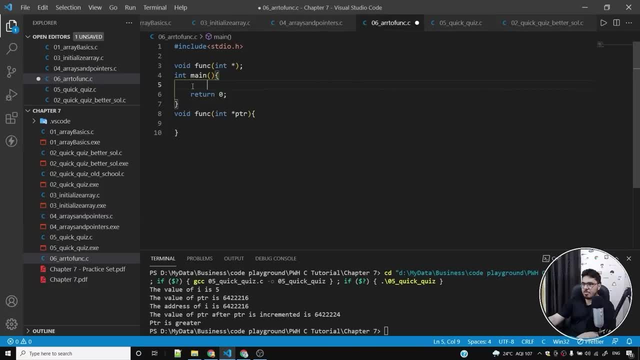 so i unfortunately can't find an array. so i unfortunately can't find an array. okay, i just found an array i can copy. okay, i, i just found an array i can copy. okay, i, i just found an array, i can copy this and i can paste it here. 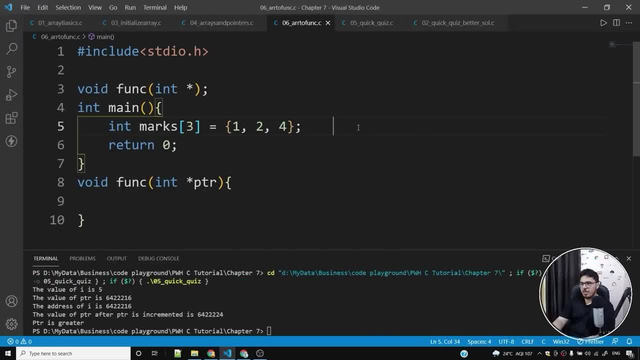 this and i can paste it here. this and i can paste it here, and what i'll do is: i can now simply, and what i'll do is: i can now simply, and what i'll do is: i can now simply use marks 0, marks 1, marks 2 to access. 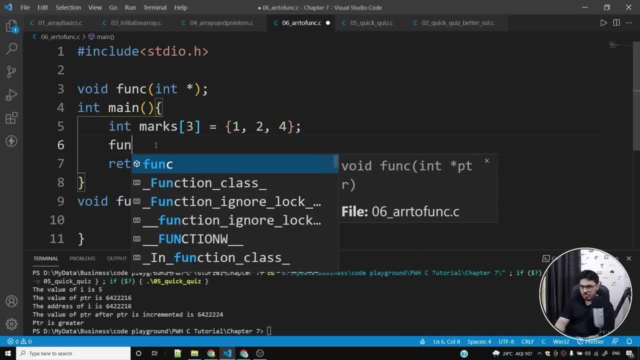 use marks 0, marks 1, marks 2 to access. use marks 0, marks 1, marks 2 to access the elements of this. marks but the elements of this marks, but the elements of this marks. but what if i say func and marks? what if i say func and marks? 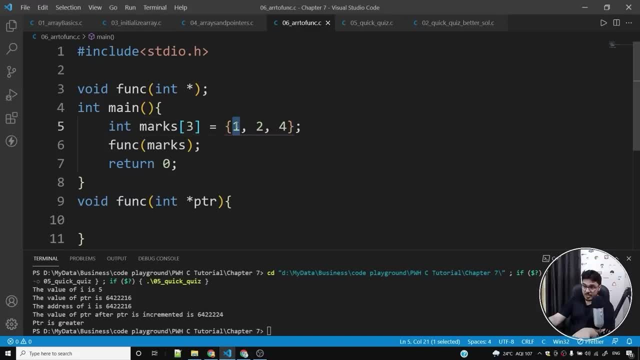 what if i say func and marks? what will happen is the address of the. what will happen is the address of the. what will happen is the address of the first element of the array will be copied. first element of the array will be copied. first element of the array will be copied to ptr. 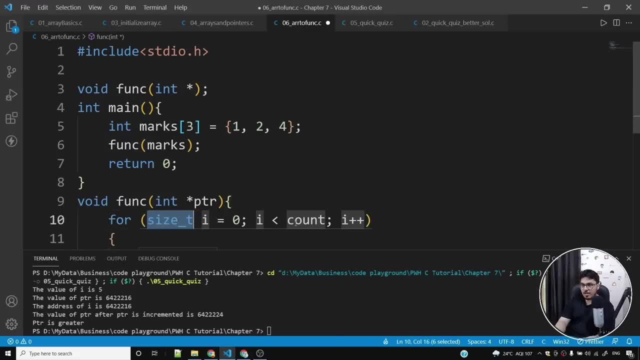 to ptr, to ptr. and now what i can do is i can write a. and now what i can do is i can write a. and now what i can do is i can write a for loop and for loop and for loop, and i can do something like this. i can say: 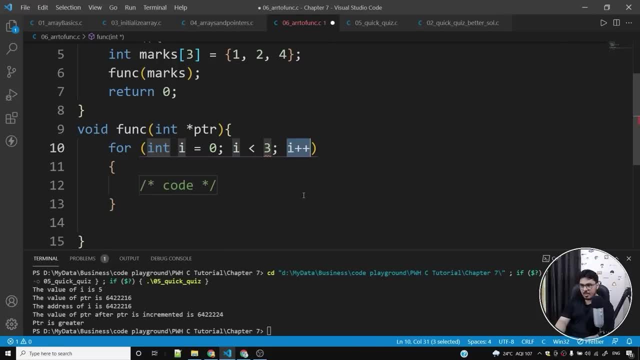 i can do something like this. i can say: i can do something like this. i can say: int. i is equal to zero, i is less than int. i is equal to zero, i is less than int. i is equal to zero, i is less than three. uh, and i plus plus. i can do print. 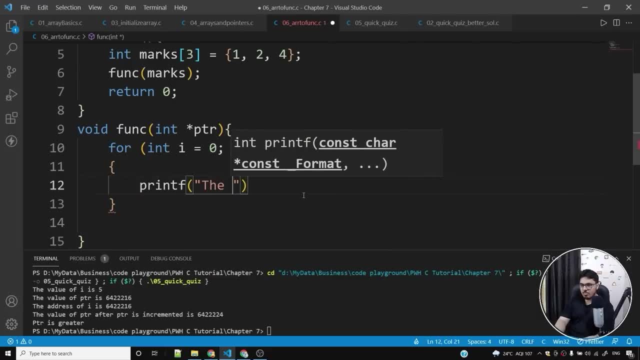 three, uh, and i plus plus i can do print three, uh, and i plus plus i can do print f and i can say f and i can say f and i can say uh, the value of marks, percentage d marks, percentage d marks, percentage d is percentage d. 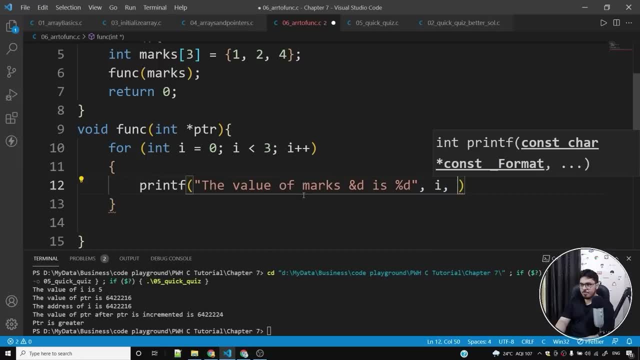 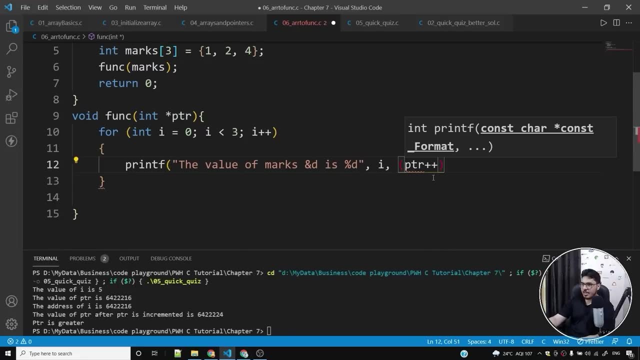 is percentage d is percentage d, and i can do something like this: i and, and i can do something like this, i and, and i can do something like this: i and ptr, ptr, ptr plus plus. okay, so this will actually plus plus. okay, so this will actually plus plus. okay, so this will actually increment the value of pointer and at 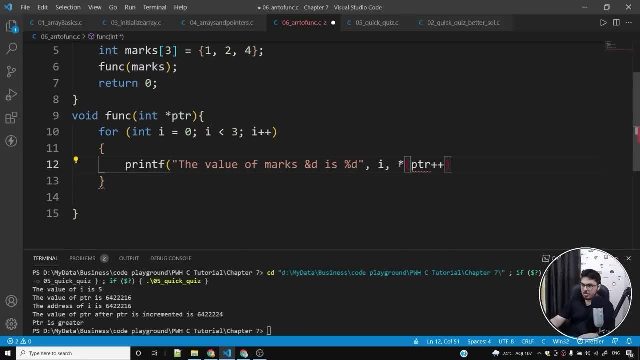 increment the value of pointer and at increment the value of pointer and at the same time it will dereference it. so the same time it will dereference it. so the same time it will dereference it. so i'll say star ptr plus plus. i'll say star ptr plus plus. 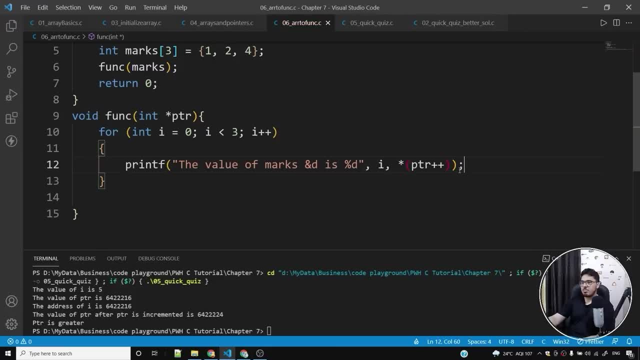 i'll say star, ptr, plus, plus, and this will make sense to you. let me- and this will make sense to you- let me- and this will make sense to you, let me finish, and this will definitely make finish, and this will definitely make finish, and this will definitely make sense to you. 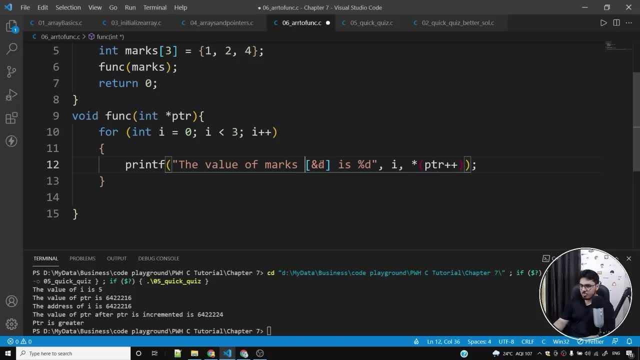 sense to you, sense to you, and also let me add these square and also let me add these square and also let me add these square brackets here. so i'll add these square brackets here. so i'll add these square brackets here. so i'll add these square brackets. 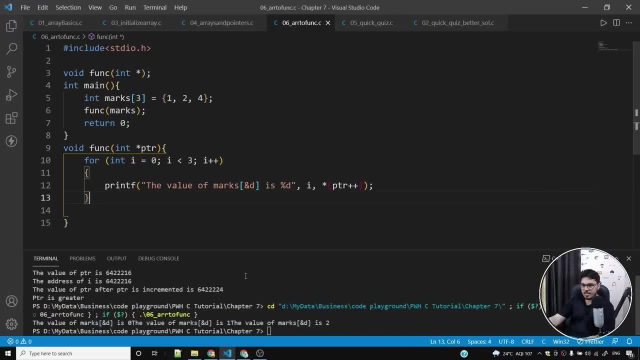 brackets like this, and let me run this for you. like this, and let me run this for you. like this, and let me run this for you: once i run this: uh, okay. so, once i run this, uh, okay. so, once i run this, uh, okay. so i need to save percentage d and not amp. 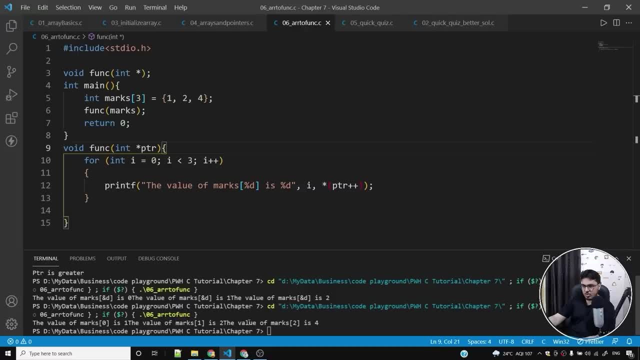 i need to save percentage d and not amp. i need to save percentage d and not amp, percent d, percent d, percent d. so the value of mark zero is one- two, and so the value of mark zero is one- two, and so the value of mark zero is one- two, and which is correct. how is this working? 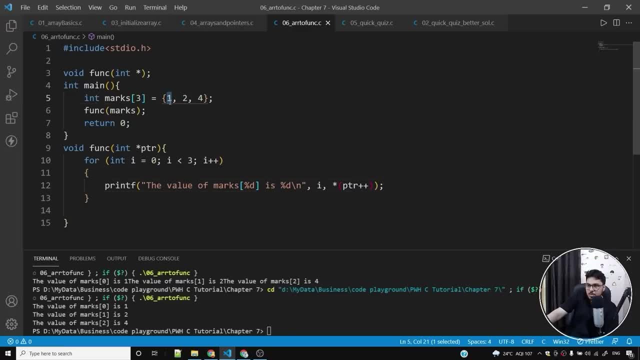 which is correct. how is this working, which is correct. how is this working? so, basically, what i'm doing is i'm so. basically, what i'm doing is i'm so. basically, what i'm doing is i'm copying the address of this particular. copying the address of this particular. 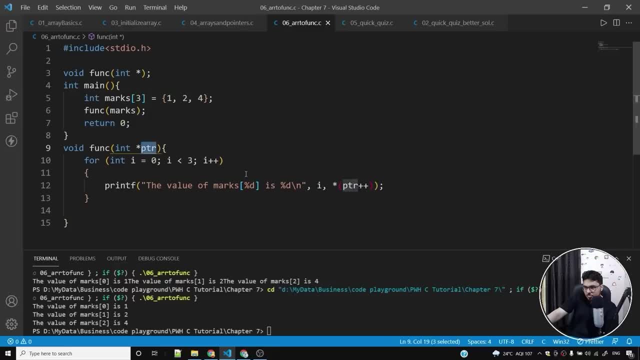 copying the address of this particular thing inside thing inside thing inside, uh, inside of here. okay, now, what i'm uh inside of here. okay, now, what i'm uh inside of here. okay, now, what i'm doing is i'm dereferencing this pointer. doing is i'm dereferencing this pointer. 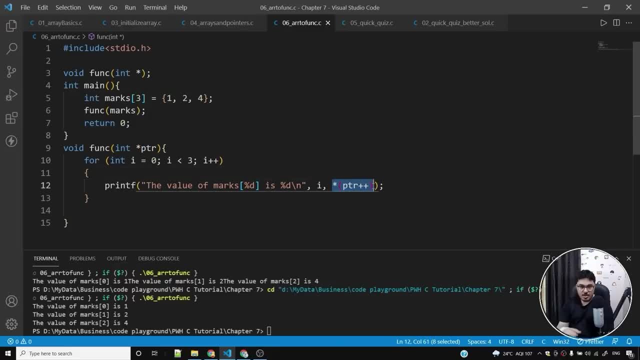 doing is i'm dereferencing this pointer and at the same time i'm incrementing it, and at the same time i'm incrementing it and at the same time i'm incrementing it so that the next time, so that the next time, so that the next time the next iteration of the for loop runs i. 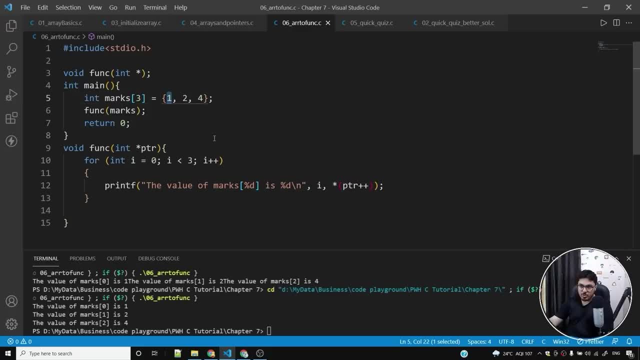 the next iteration of the for loop runs i the next iteration of the for loop runs. i will get the incremented pointer. so will get the incremented pointer. so will get the incremented pointer. so initially the pointer was pointing to one. initially the pointer was pointing to one. initially the pointer was pointing to one. i printed one in the next iteration of. 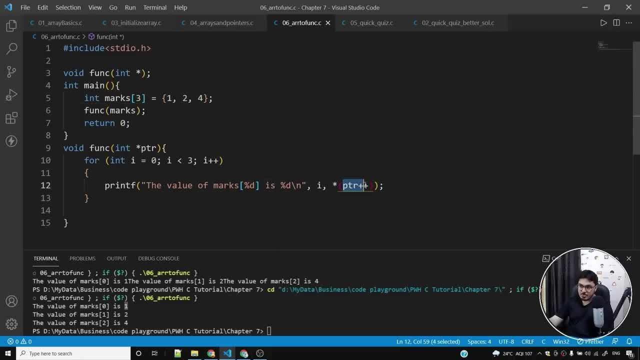 i printed one in the next iteration of. i printed one in the next iteration of. the for loop pointer will point to two. the for loop pointer will point to two. the for loop pointer will point to two because i am saying ptr plus plus every. because i am saying ptr plus plus every. 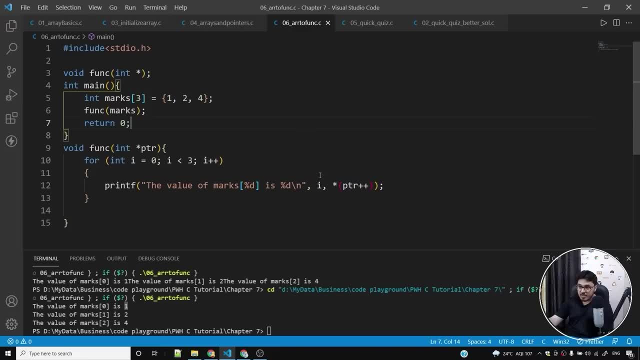 because i am saying ptr plus plus every time. i'm running this iteration of the time, i'm running this iteration of the time, i'm running this iteration of the for loop. so if i say ptr plus plus once for loop, so if i say ptr plus once again, the pointer will point to this. 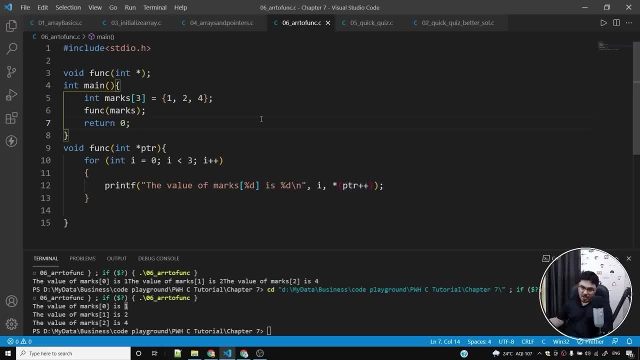 again, the pointer will point to this. again, the pointer will point to this, and so on. it will keep on incrementing, and so on. it will keep on incrementing, and so on. it will keep on incrementing itself until it reaches the last item of itself, until it reaches the last item of 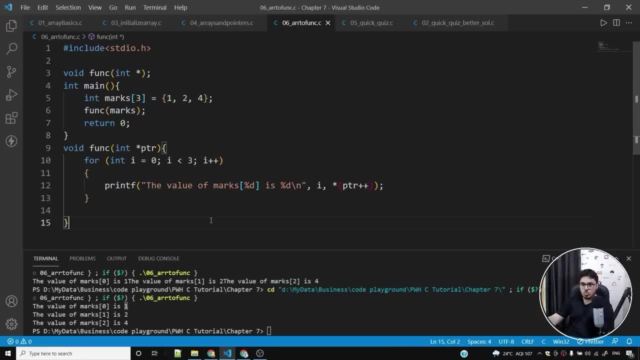 itself until it reaches the last item of the array, the array, the array. and this is how we can pass arrays to, and this is how we can pass arrays to, and this is how we can pass arrays to the functions. what if i do something like the functions? what if i do something like? 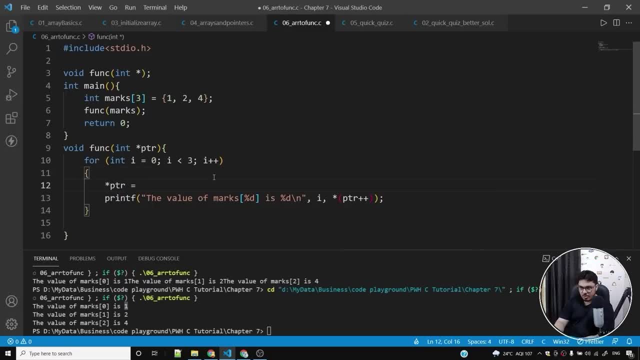 the functions. what if i do something like this? what if i say this? what if i say this? what if i say: star ptr is equal to um. say 56. for some, star ptr is equal to um. say 56. for some, star ptr is equal to um. say 56. for some reason. what if i? what if i change the? 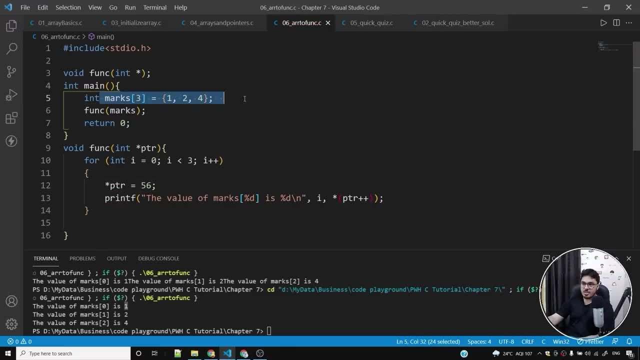 reason. what if i? what if i change the reason? what if i? what if i change the items to 56? uh. but if i change marks 0 items to 56? uh. but if i change marks 0 items to 56, uh. but if i change marks 0, 1 and 2 to 56? for some reason will they? 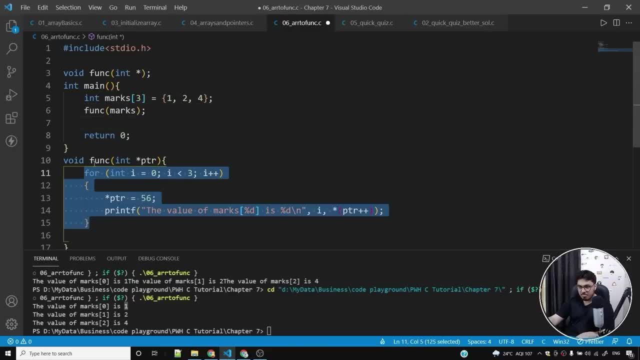 1 and 2 to 56. for some reason will they 1 and 2 to 56? for some reason will they be reflected here? be reflected here. be reflected here. what if i try to access the value of? what if i try to access the value of? 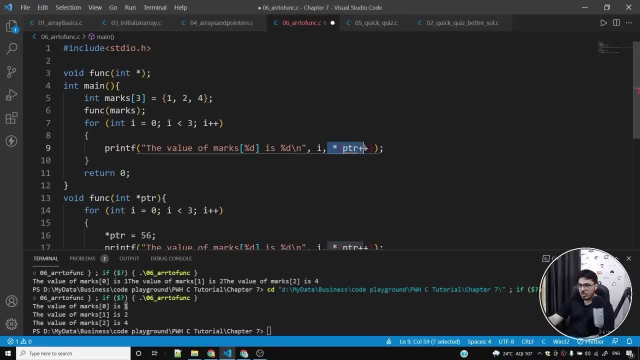 what if i try to access the value of marks, marks, marks zero, marks one and marks two. will they be zero, marks one and marks two. will they be zero, marks one and marks two. will they be changed? here is the question changed. here is the question changed. here is the question and you need to answer this in the. 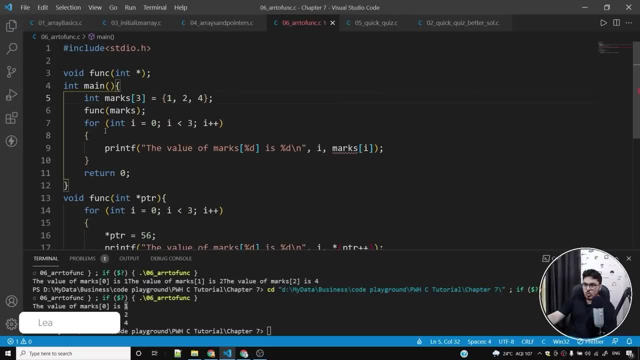 and you need to answer this in the and you need to answer this in the comments. so i'll say: mark psi comments. so i'll say: mark psi comments. so i'll say: mark psi, tell me whether this value will be. tell me whether this value will be. 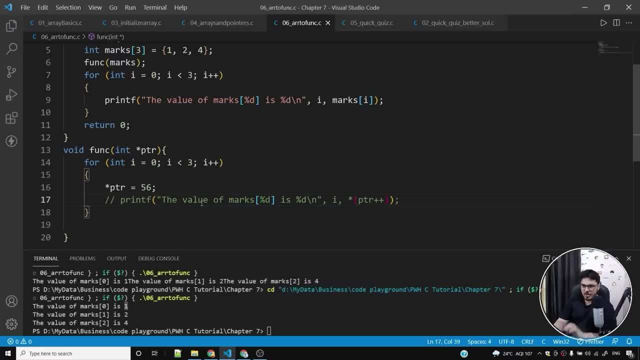 tell me whether this value will be changed to 56 or not. changed to 56 or not? changed to 56 or not? let me get rid of this printf statement. let me get rid of this printf statement. let me get rid of this printf statement. so whatever is printed now will be. 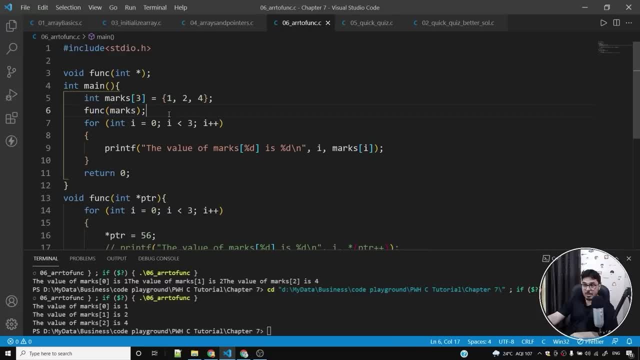 so whatever is printed now will be so whatever is printed now will be printed from here. so we are running this printed from here. so we are running this printed from here. so we are running this function. will this function be able to function? will this function be able to? 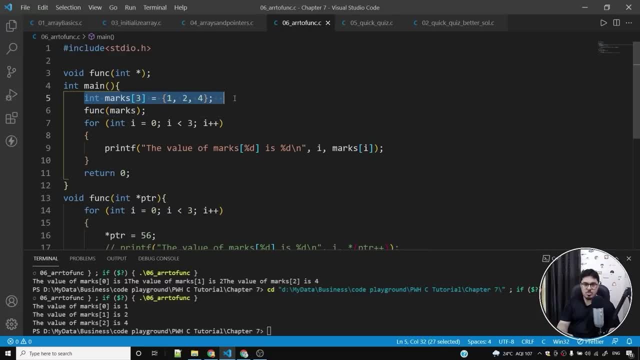 function. will this function be able to make changes to this array? this is the make changes to this array. this is the make changes to this array. this is the question answer. mean yes or no? and you question answer mean yes or no? and you question answer mean yes or no. and you can use time stamps of the video to can use time stamps of the video to can use time stamps of the video to tell me which question you are answering. tell me which question you are answering. tell me which question you are answering. i'm waiting for your comment. make sure. i'm waiting for your comment. make sure. 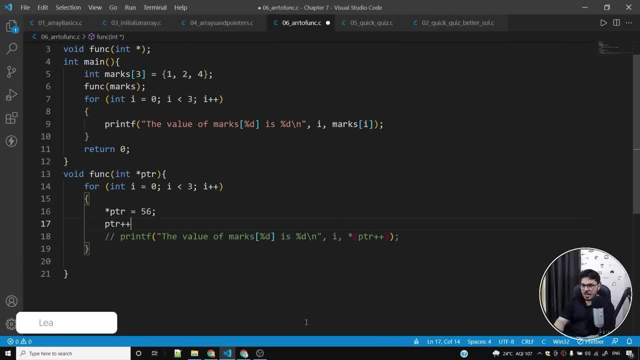 i'm waiting for your comment. make sure you post the comment. and one more thing: you post the comment. and one more thing: you post the comment. and one more thing i'll need to do here is ptr plus plus. i'll need to do here is ptr plus plus. 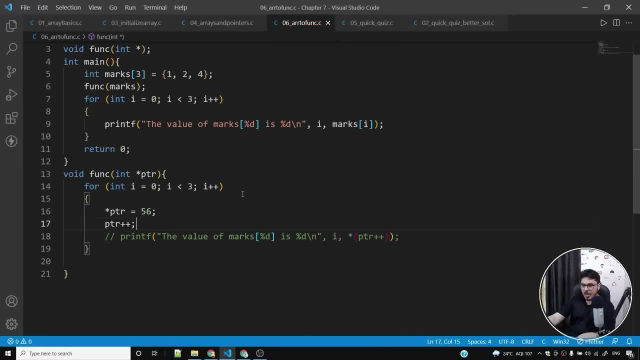 i'll need to do here is ptr plus plus, because i'm getting rid of this line. so because i'm getting rid of this line, so because i'm getting rid of this line, so i'll do ptr plus plus. now tell me, i'll do ptr plus plus. now tell me. 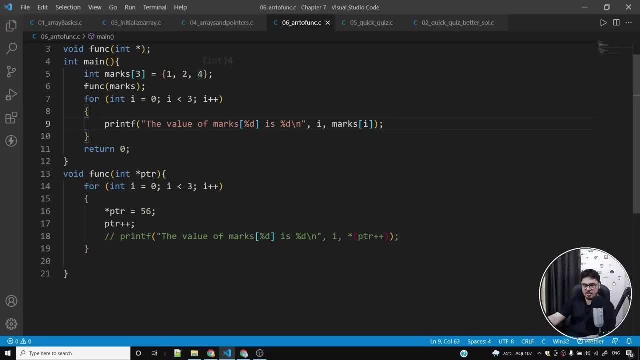 i'll do ptr plus plus. now tell me whether whether whether this will change the area to 56 56 56 or this will change the area to 56 56 56 or this will change the area to 56 56 56 or not. 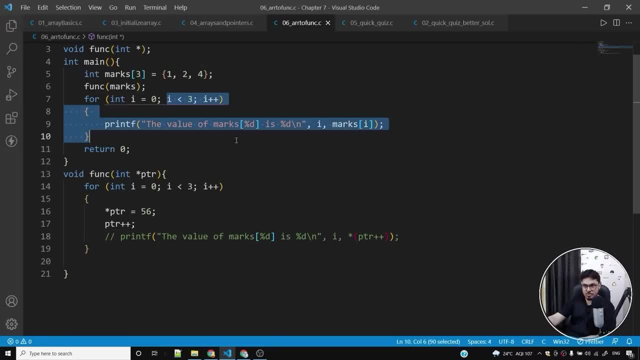 not not. so i'll now run this program to show you. so i'll now run this program to show you. so i'll now run this program to show you that all these values will be changed to that. all these values will be changed to that. all these values will be changed to 56, 56 and 56, as you can see. 56, 56 and 56. as you can see, 56, 56 and 56. as you can see, the value of 0, 1 and 2 is changed to 56. the value of 0, 1 and 2 is changed to 56. 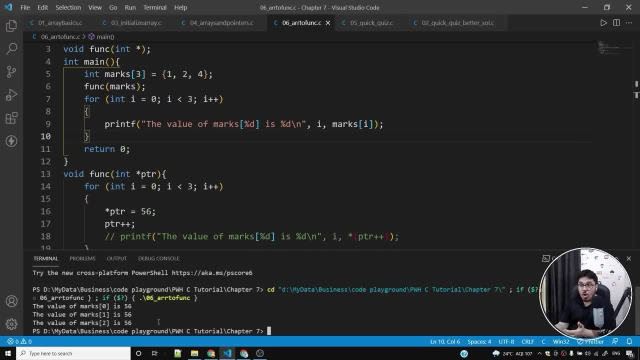 the value of 0, 1 and 2 is changed to 56 because we are dealing in addresses. because we are dealing in addresses, because we are dealing in addresses, this time we are passing the address of this time. we are passing the address of this time, we are passing the address of the first element of the array to this: 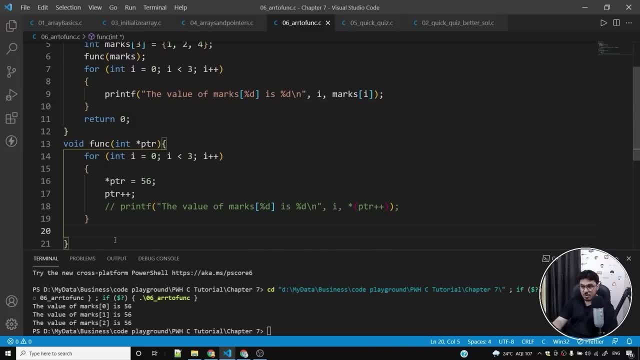 the first element of the array to this, the first element of the array to this function. and since we are passing the function, and since we are passing the function, and since we are passing the address to this function, what happens is address to this function. what happens is: 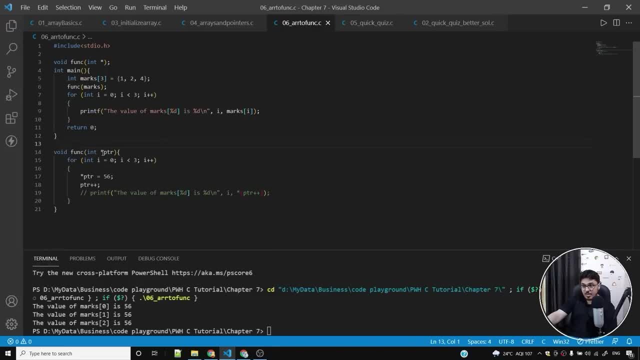 address to this function. what happens is that this um, that this address, that this um, that this address, that this um, that this address is actually dereferenced and is actually dereferenced and is actually dereferenced, and the actual value of marks 0, 1 and 2. 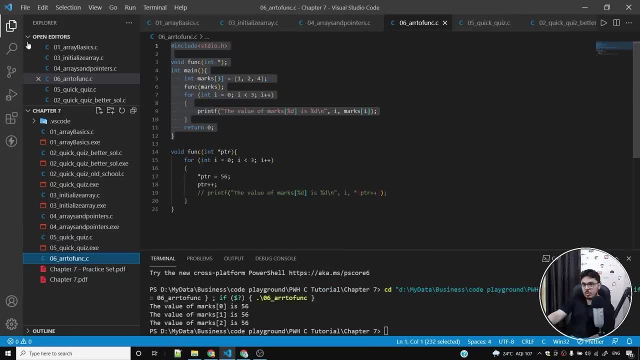 the actual value of marks 0, 1 and 2. the actual value of marks 0, 1 and 2 is changed. so i hope this makes sense is changed. so i hope this makes sense is changed. so i hope this makes sense. and these are the programs that i'll. 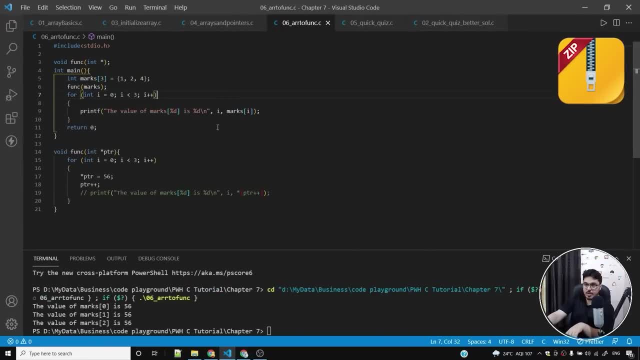 and these are the programs that i'll and these are the programs that i'll zip, and you know, put it in the zip. and you know, put it in the zip and you know, put it in the description somewhere so that you can description somewhere so that you can. 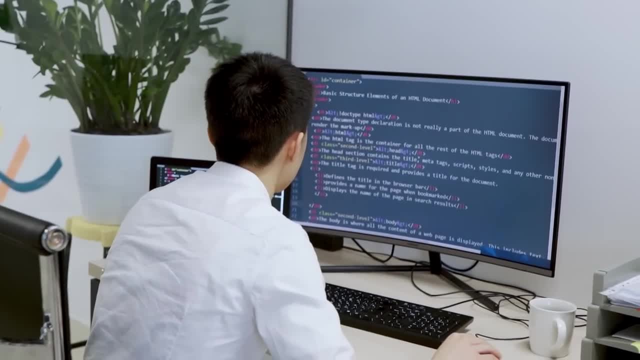 description somewhere so that you can access and all these codes are going to access and all these codes are going to access and all these codes are going to help you a lot. believe me, so you can help you a lot. believe me, so you can help you a lot. believe me, so you can access these codes. try to run them on. 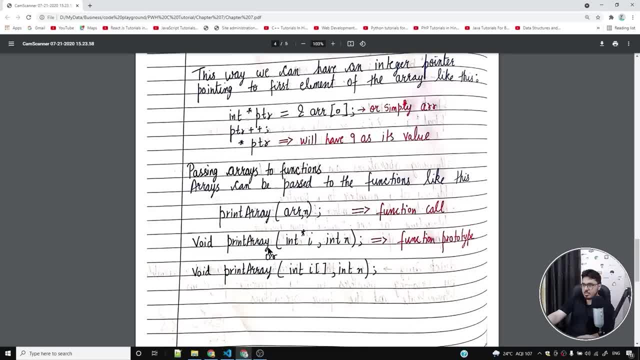 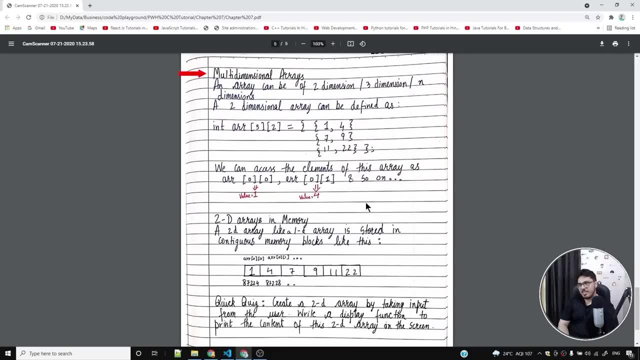 access these codes. try to run them on. access these codes, try to run them on your own and you'll definitely get a your own. and you'll definitely get a your own. and you'll definitely get a lot of times if you're writing simple, lot of times if you're writing simple. 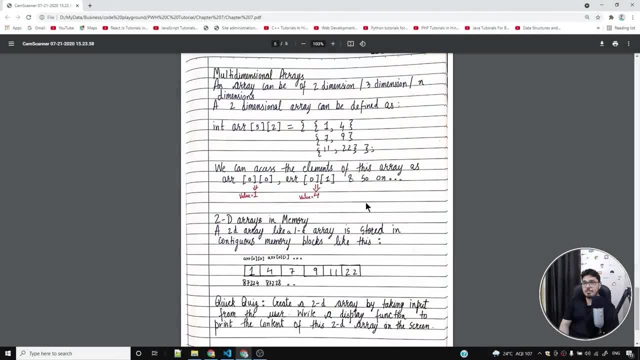 lot of times if you're writing simple programs, but if you want to say write programs. but if you want to say write programs, but if you want to say write programs on matrices, or you want to programs on matrices, or you want to programs on matrices, or you want to visualize a 2d grid or a 2d table, 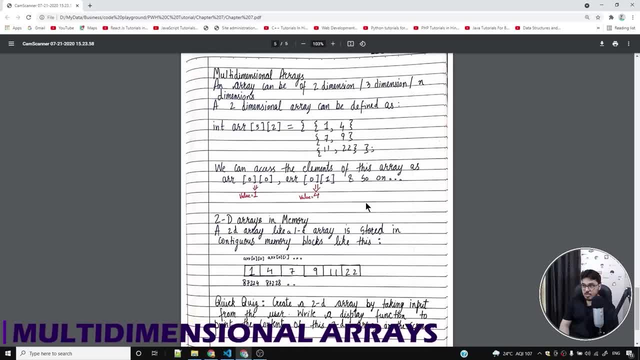 visualize a 2d grid or a 2d table. visualize a 2d grid or a 2d table containing numbers. you might want to use containing numbers. you might want to use containing numbers. you might want to use multi-dimensional arrays. look at multi-dimensional arrays. look at. 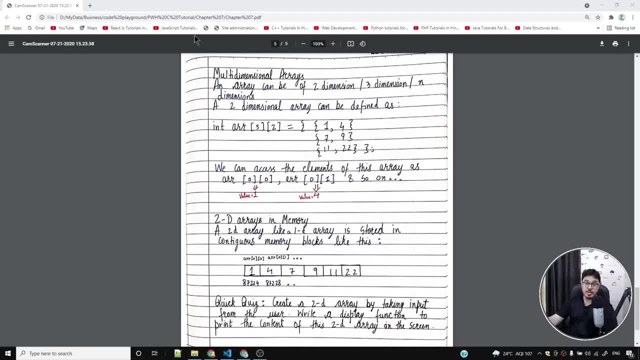 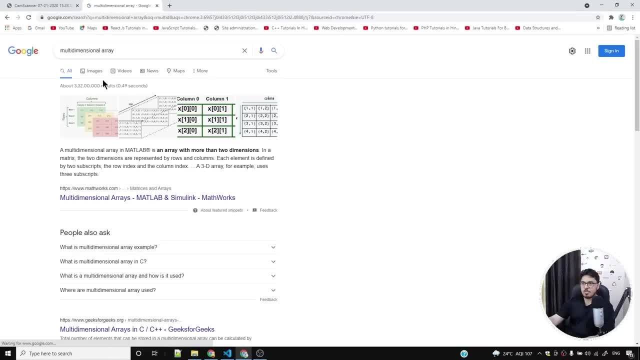 multi-dimensional arrays. look at multi-dimensional arrays as a multi-dimensional arrays, as a multi-dimensional arrays, as a two-dimensional grid. let me search two-dimensional grid. let me search two-dimensional grid. let me search multi-dimensional array. and let me multi-dimensional array and let me multi-dimensional array. and let me go to images and let me see if i can. 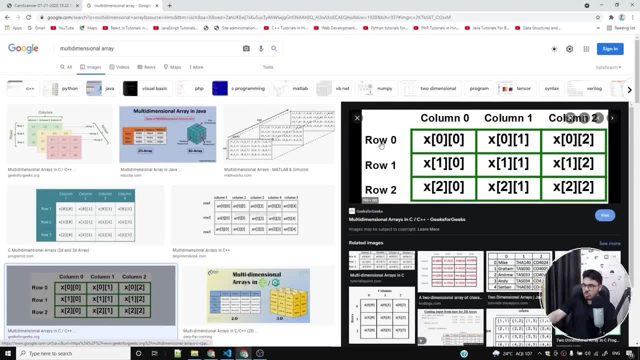 go to images and let me see if i can go to images and let me see if i can actually show you something. so this is a actually show you something. so this is a actually show you something. so this is a very good image to start with. so row 0: very good image to start with, so row 0. very good image to start with, so row 0. row 1. row 2, column 0, column 1, column 2. so row 1, row 2, column 0, column 1, column 2: so. 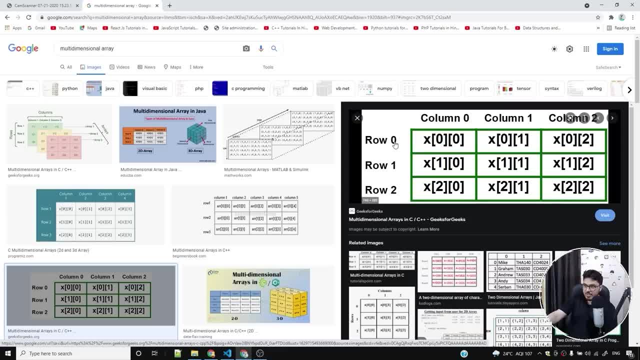 row 1. row 2, column 0. column 1- column 2. so the rows starts from 0. column starts the rows starts from 0. column starts the rows starts from 0. column starts from 0. so if i say arr 0- 0, this will or. 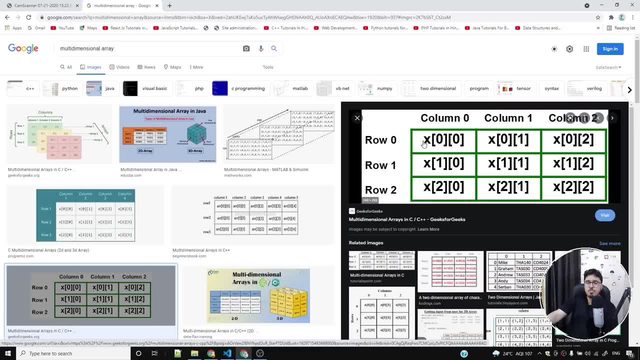 from 0, so if i say arr 0, 0, this will. or from 0, so if i say arr 0, 0, this will. or rather, let us say the name of the rather, let us say the name of the, rather, let us say the name of the variable. the name of the array is x, so i. 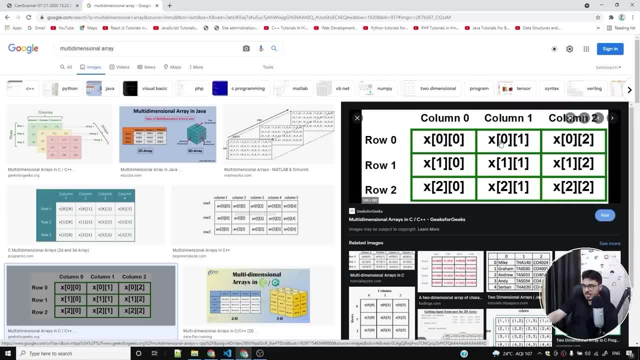 variable: the name of the array is x, so i variable: the name of the array is x, so i can actually reference this value as x can actually reference this value, as x can actually reference this value as x 0, 0. this is x 0, 1, this is x 0, 2 and so. 0, 0, this is x 0, 1, this is x 0, 2, and so 0, 0, this is x 0, 1, this is x 0, 2, and so on. so i can visualize this particular on. so i can visualize this particular. 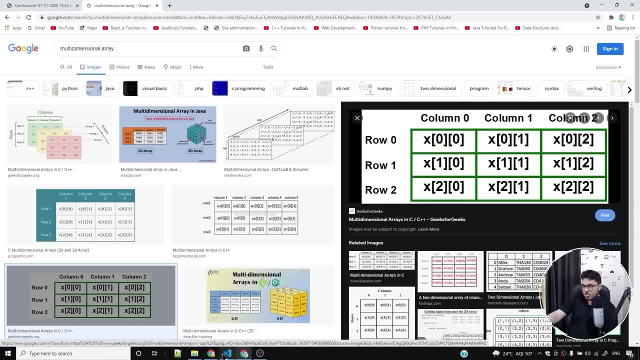 on, so i can visualize this particular two-dimensional grid and i can set all two-dimensional grid and i can set all two-dimensional grid and i can set all these values. so let me show this to you, these values. so let me show this to you, these values. so let me show this to you by writing a program. 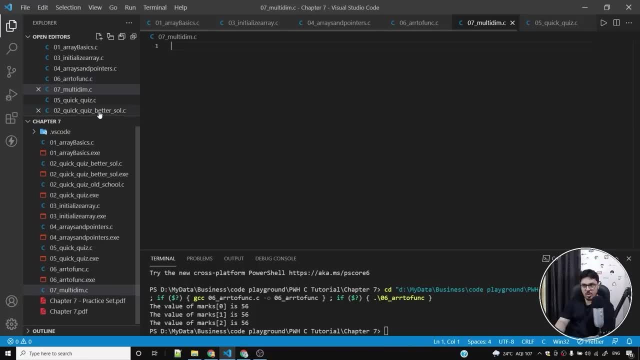 by writing a program, by writing a program: 07 underscore, 07. underscore, 07 underscore. multi-dimensional array dot c. multi-dimensional array dot c. multi-dimensional array dot c, boilerplate code, boilerplate code, boilerplate code, and let me say int and let me say int. 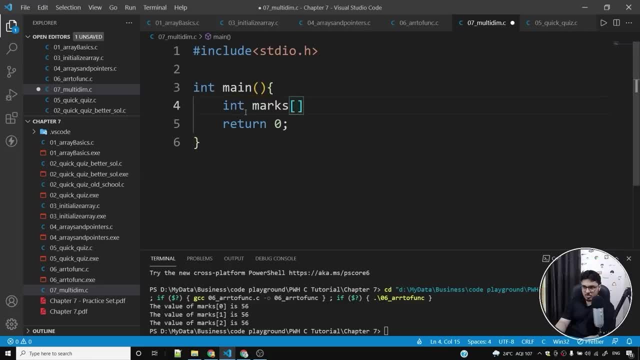 and let me say int marks, marks, marks. let us say i want to express marks of. let us say i want to express marks of. let us say i want to express marks of four students, four students, four students from two classes, from two classes, from two classes. so 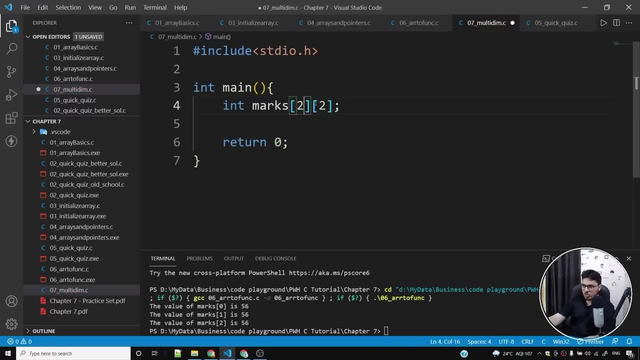 so, so marks, marks, marks. or let me make it two, four so two, or let me make it two, four so two, or let me make it two, four so two. classes, four students, so students are in classes four. students, so students are in classes four. students, so students are in the columns. 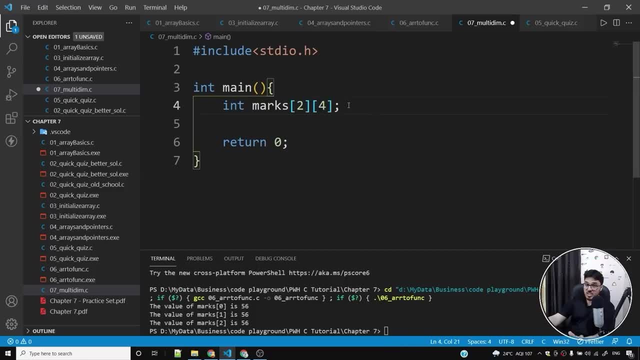 the columns. the columns and the classes are in rows. so let us say: and the classes are in rows. so let us say: and the classes are in rows. so let us say: we have two sections, section a, and we have two sections, section a. and we have two sections, section a and section b. section a has four students. 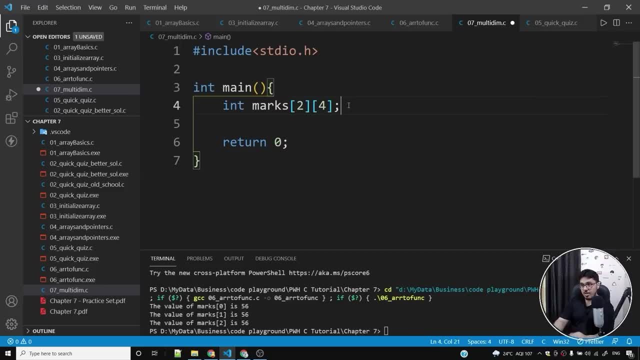 section b, section b. section a has four students. section b, section a, has four students. section b has four students. i'm keeping section b has four students. i'm keeping section b has four students. i'm keeping these numbers as low so that you can, these numbers as low so that you can. 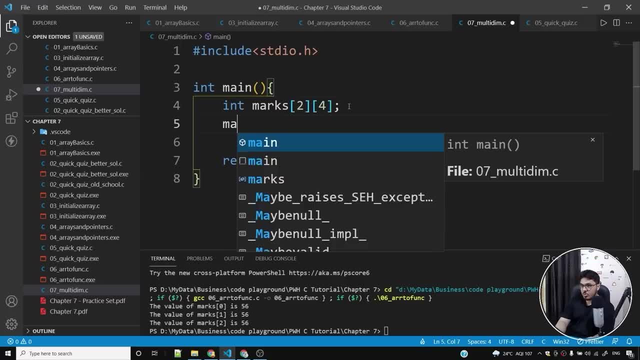 these numbers as low so that you can- uh, you know, easily visualize what is- uh, you know, easily visualize what is, uh, you know, easily visualize what is happening, happening, happening now. what i'll do is i'll simply say: now, what i'll do is i'll simply say: 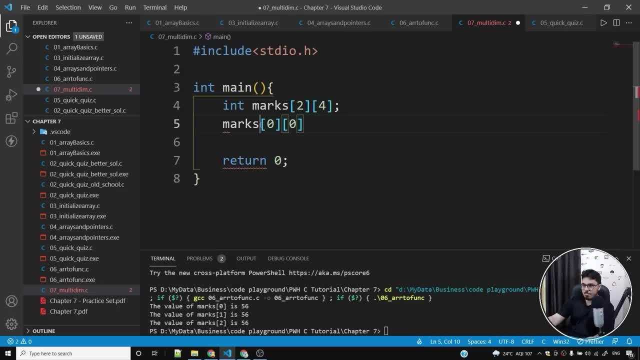 now what i'll do is i'll simply say: mark zero zero, mark zero zero, mark zero zero. so uh, mark zero is section a. so uh, mark zero is section a. so, uh, mark zero is section a. so first student of section a has got, so first student of section a has got. 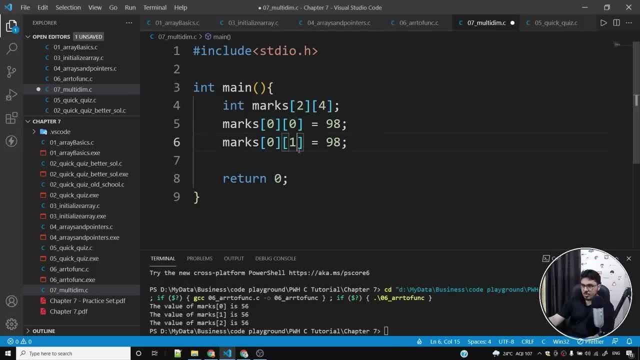 so first student of section a has got 98 marks, 98 marks, 98 marks now. second student of section a got now. second student of section a got now. second student of section a got say 93 marks, say 93 marks, say 93 marks. let us assume that the section a 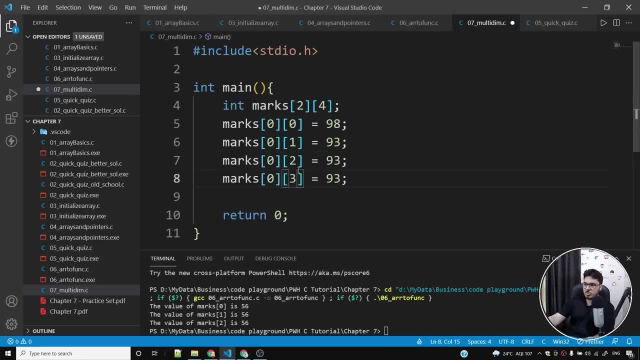 let us assume that the section a, let us assume that the section a contains, contains, contains: you know list of brilliant students, so you know list of brilliant students. so you know list of brilliant students. so, second student, sorry. third student of second student, sorry. third student of second student, sorry. third student of section a. let us say: he got, he was. 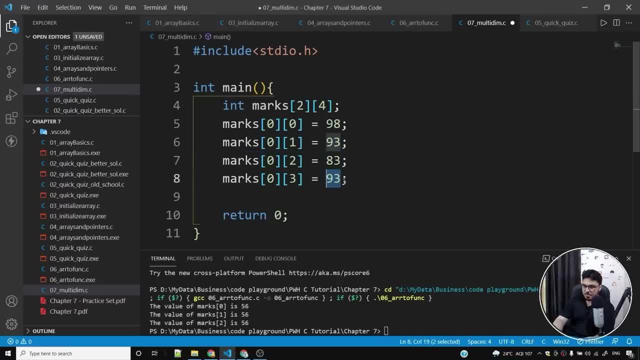 section a. let us say he got, he was section a. let us say he got. he was unlucky and he got 83 marks. unlucky and he got 83 marks. unlucky and he got 83 marks. and this is the lowest score. and let us, and this is the lowest score, and let us. 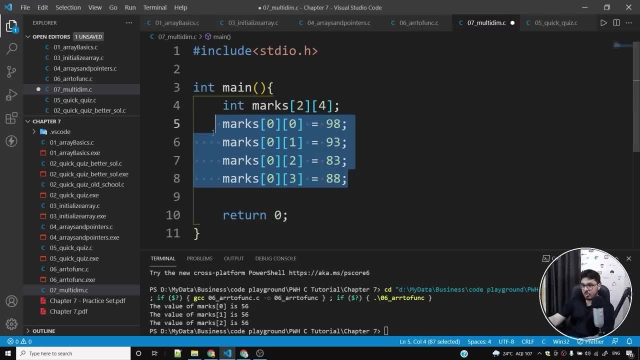 and this is the lowest score. and let us say the say, the say. the last student of section: he got 90. sorry. last student of section: he got 90. sorry last student of section, he got 90. sorry, 88 marks, 88 marks, 88 marks. now i'll do the same for section. 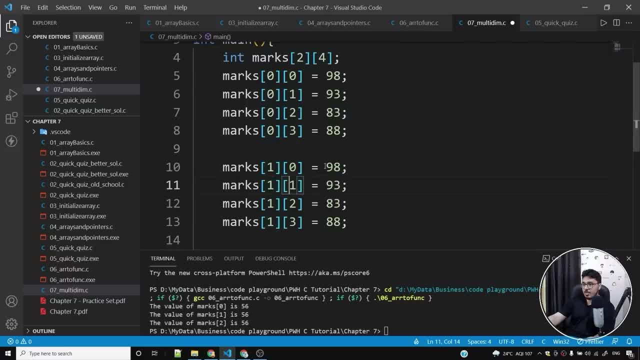 now i'll do the same for section. now i'll do the same for section: uh, section b. and let us say all these uh section b, and let us say all these uh section b. and let us say all these people, people, people have no interest in studies, they are. 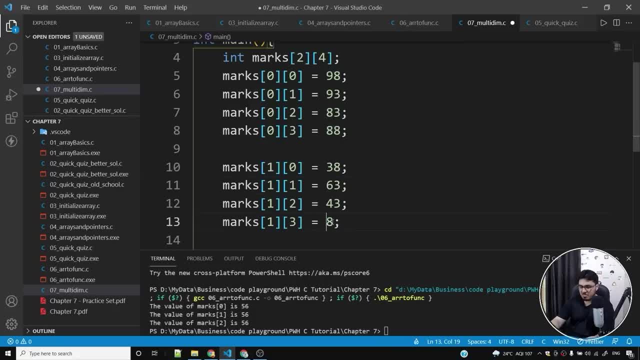 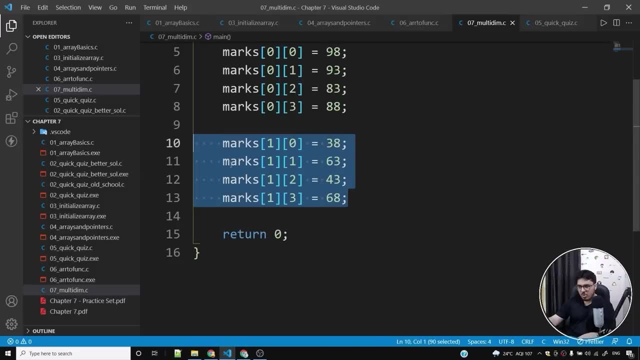 have no interest in studies. they are have no interest in studies. they are. so these are lazy people who are not so. these are lazy people who are not so. these are lazy people who are not able to score marks- okay, able to score marks, okay. able to score marks, okay. now. int marks 2, 4, 98, 93, 83, 88. 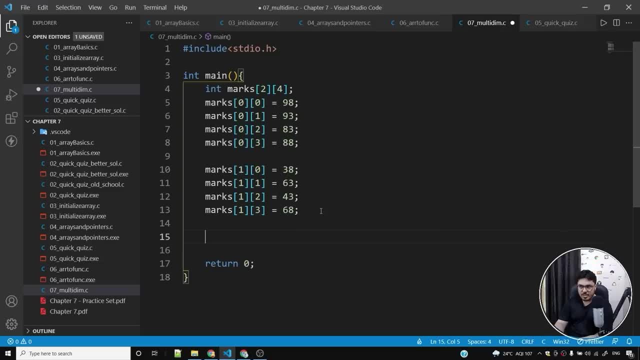 now int marks 2, 4, 98, 93 83 88, now int marks 2, 4, 98, 93 83, 88, and so on. okay, now what i've done here and so on. okay, now what i've done here and so on. okay, now, what i've done here is i have actually 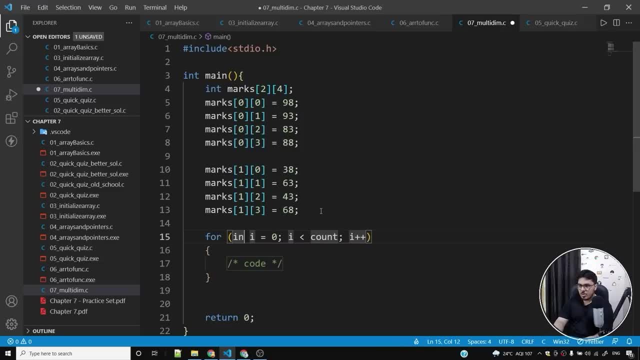 is. i have actually, is i have actually set all these values. now i can use a set all these values. now i can use a set all these values. now i can use a double for loop to double for loop, to double for loop to, you know, iterate all these values. so let 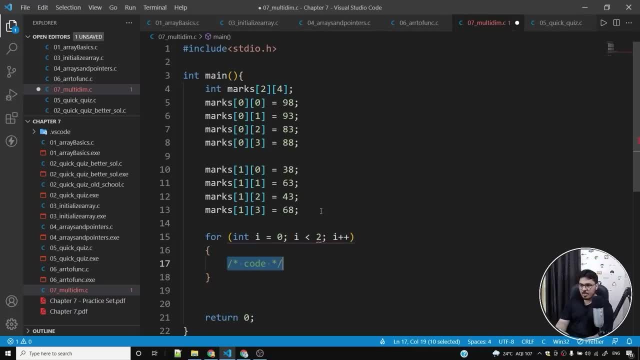 you know, iterate all these values. so let you know, iterate all these values. so let me show you how this works, me show you how this works, me show you how this works. so i'll put two here, another tap. so i'll put two here, another tap. so i'll put two here, another tap, another for loop. so 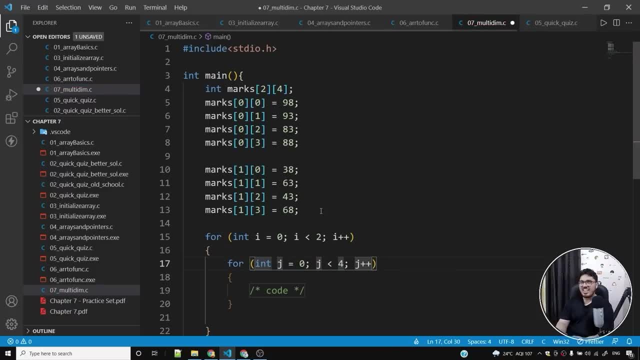 another for loop, so another for loop. so this might really, uh, you know sound, this might really, uh, you know sound, this might really, uh, you know, sound very confusing to you and you might very confusing to you and you might very confusing to you and you might think that is this something that i 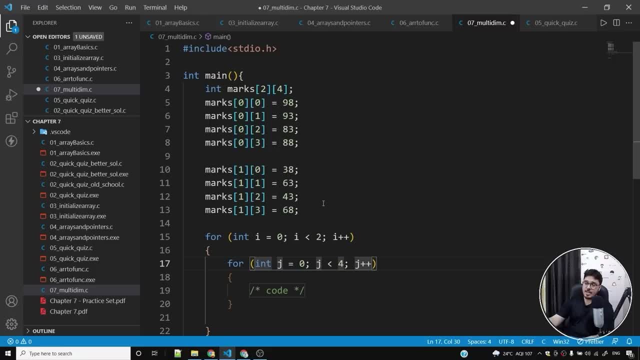 think that is this something that i think that is this something that i even need. is this something that i even even need? is this something that i even even need? is this something that i even need to study? need to study, need to study. but let me tell you something. two: 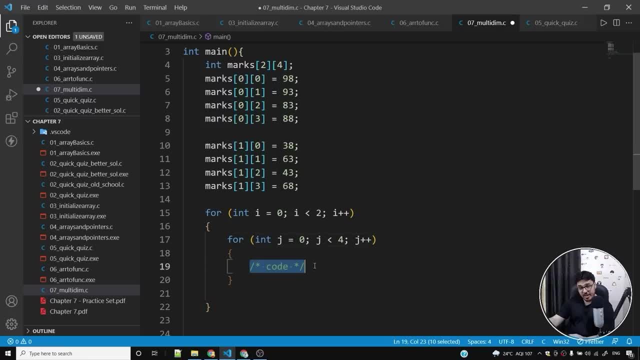 but let me tell you something. two, but let me tell you something. two: dimensional array is something that you dimensional array is something that you dimensional array is something that you will ever need. if you're writing, some will ever need. if you're writing, some will ever need if you're writing some complex programs. i'm not saying that. 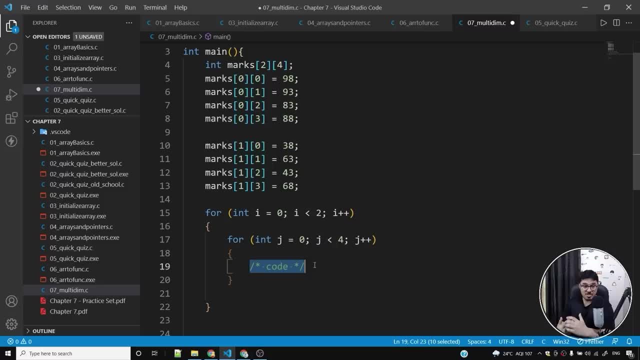 complex programs. i'm not saying that complex programs. i'm not saying that you'll not need three dimensional five. you'll not need three dimensional five. you'll not need three dimensional five dimensional ten dimensional areas. i've dimensional ten dimensional areas. i've dimensional ten dimensional areas. i've seen people working with 50 dimensional. 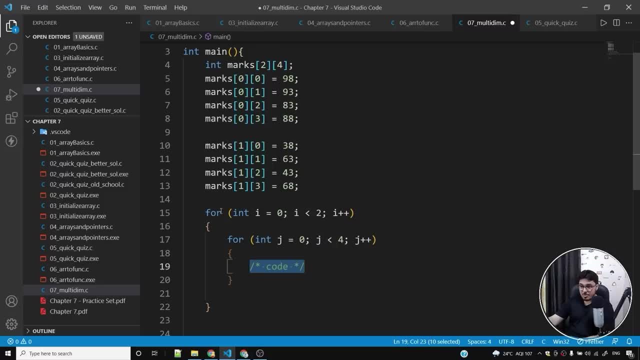 seen people working with 50 dimensional, seen people working with 50 dimensional arrays, but again that is very, very rare arrays. but again, that is very, very rare arrays, but again that is very, very rare. so two dimensional array is something, so two dimensional array is something. so two dimensional array is something that you need to target. 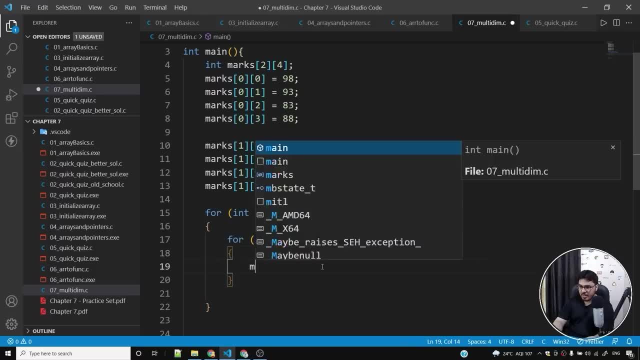 that you need to target, that you need to target initially and later. everything will initially and later, everything will initially and later. everything will seem very easy to you. so here what i'll seem very easy to you. so here what i'll seem very easy to you. so here what i'll do is i'll say marks ij. 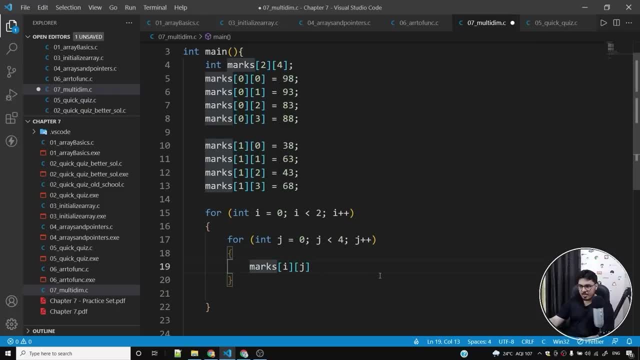 do is, i'll say marks ij. do is, i'll say marks ij. marks ij is nothing but the marks ij is nothing but the marks ij is nothing but the some value which is which this, some value which is which this, some value which is which this particular thing is currently at. let me, 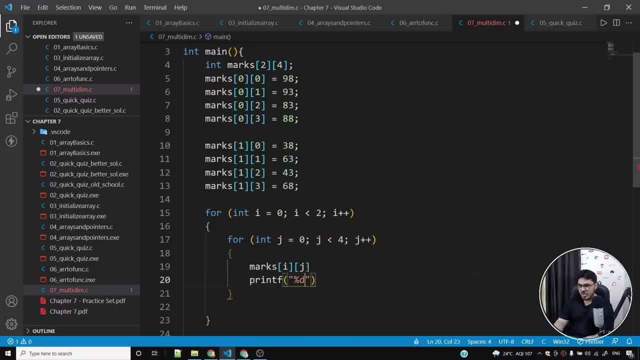 particular thing is currently at. let me particular thing is currently at. let me show you something. i'll say print f. show you something. i'll say print f. show you something. i'll say print f and i'll say percentage d and i'll. and i'll say percentage d and i'll. 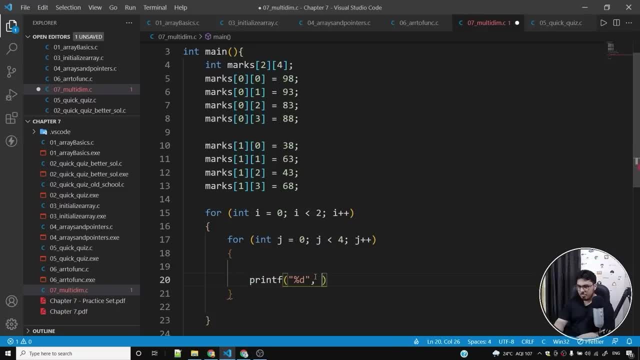 and i'll say percentage d and i'll simply put this marks ij here. okay, so simply put this marks ij here. okay, so simply put this: marks ij here. okay, so let me put marks ij here. let me put marks ij here. let me put marks ij here. if i run this program, what will happen is: 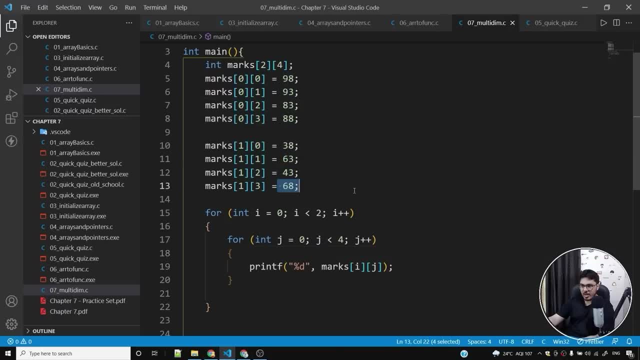 if i run this program. what will happen is: if i run this program, what will happen is all these values will get printed, all these values will get printed. all these values will get printed without any space, without any new line, without any space, without any new line, without any space, without any new line, which will really get very confusing. so 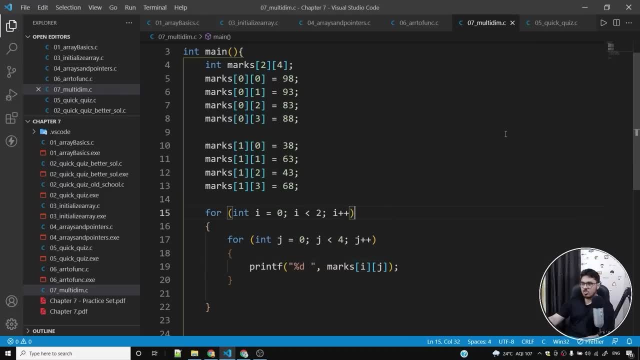 which will really get very confusing. so which will really get very confusing. so what i'll do is i'll add a space here. what i'll do is i'll add a space here. what i'll do is i'll add a space here after percentage d. so if i run this, 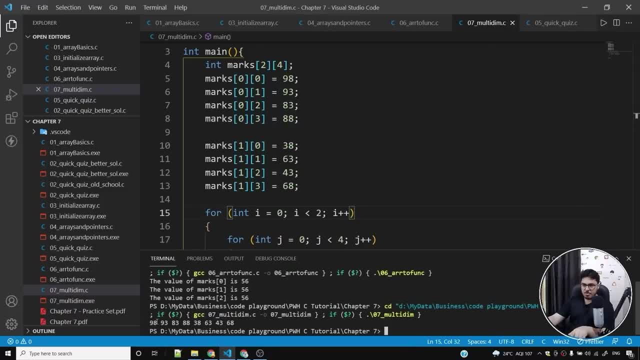 after percentage d. so if i run this after percentage d, so if i run this program, all these numbers will be program. all these numbers will be program. all these numbers will be printed with a space between them, but i printed with a space between them, but i printed with a space between them. but i don't want them to print this way. i want. 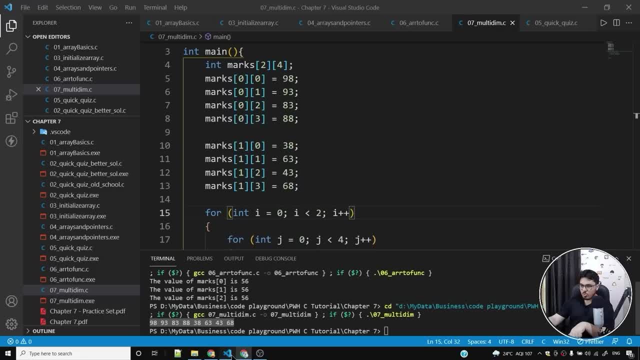 don't want them to print this way. i want, don't want them to print this way. i want to, to to print them in this way, in this fashion. so print them in this way, in this fashion. so print them in this way, in this fashion. so how do i do that? 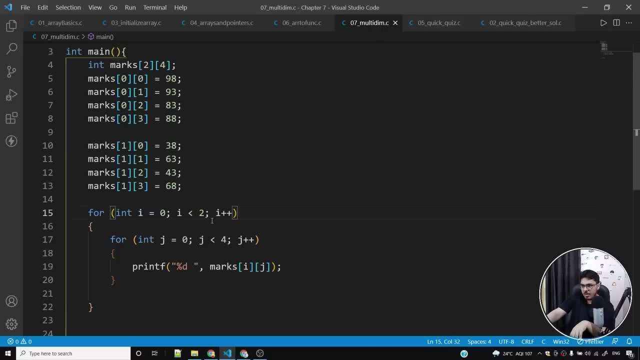 how do i do that? how do i do that? so let's try to understand how this. so let's try to understand how this. so let's try to understand how this double for loop is working. double for loop is working. double for loop is working. so this for loop is for rows. let me write. 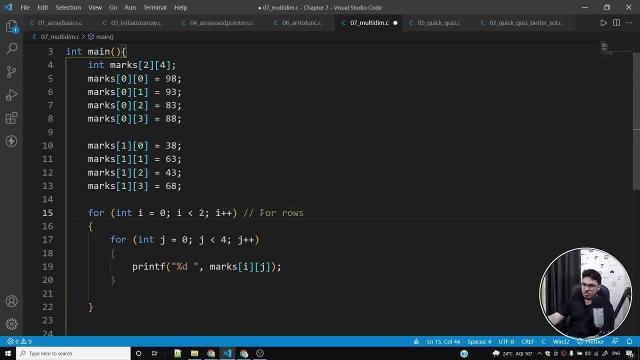 so this for loop is for rows. let me write: so this for loop is for rows. let me write a comment here, a comment here, a comment here for rows. so we are saying for the first for rows, so we are saying for the first for rows, so we are saying for the first row, you do this and you once again do. 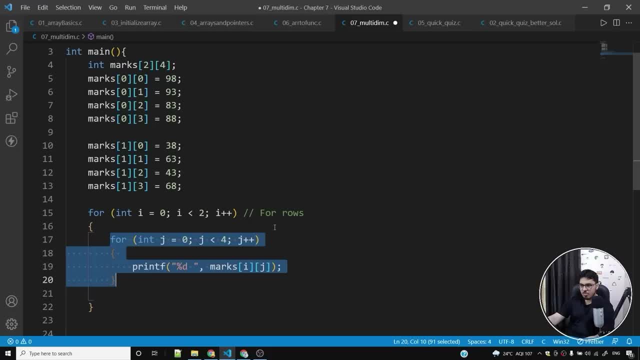 row, you do this and you once again do row, you do this and you once again do this, this, this for the second row, and this is for for the second row, and this is for for the second row and this is for columns. this is painting the columns. 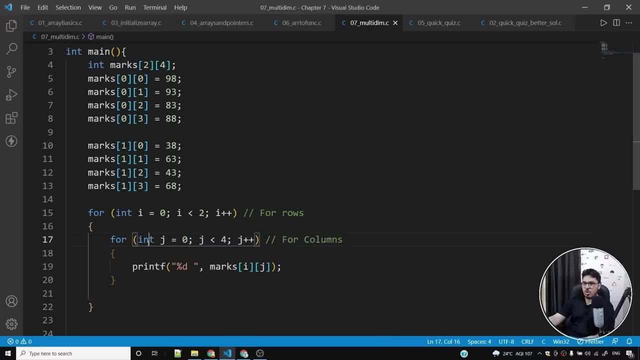 columns: this is painting the columns. columns: this is painting the columns. so this will paint column one for the. so this will paint column one for the. so this will paint column one for the first row. column two for the first row. first row. column two for the first row. 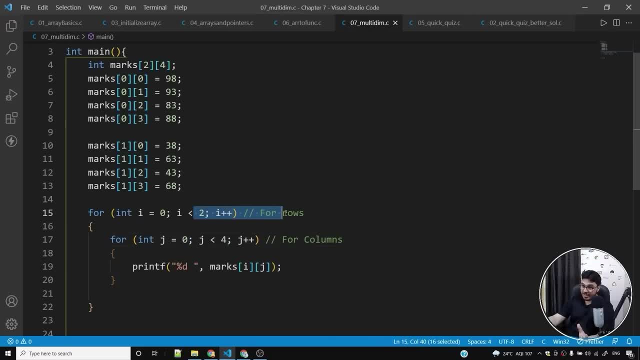 first row, column two, for the first row, then once again when the row, then once again when the row, then once again when the row is the second row. the row being painted is the second row. the row being painted is the second row. the row being painted is second row. this will print the first. is second row, this will print the first is second row. this will print the first element, then second element of the row element, then second element of the row element, then second element of the row, then third element of the row, and so on, then third element of the row, and so on. 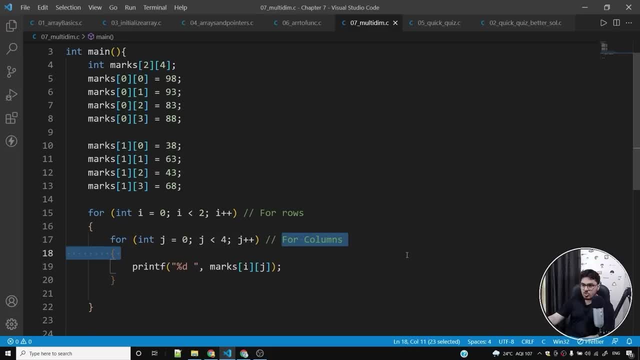 then third element of the row, and so on. so this is for columns. it's basically so. this is for columns. it's basically so. this is for columns. it's basically painting the columns. okay, so what i can painting the columns? okay, so what i can painting the columns- okay. so what i can do is every time- uh, it is done, painting. 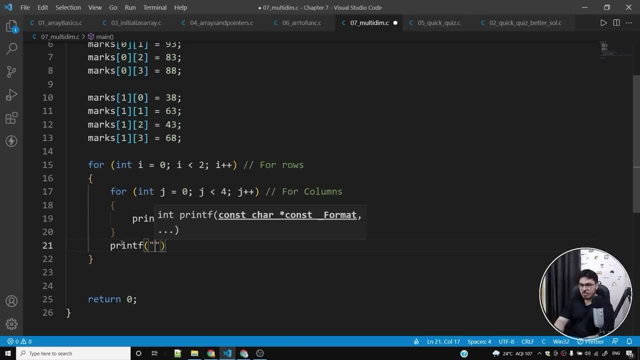 do is every time, uh, it is done. painting: do is every time, uh, it is done. painting all the columns. i can say all the columns, i can say all the columns. i can say print backslash n, so i can say print f, print backslash n, so i can say print f. 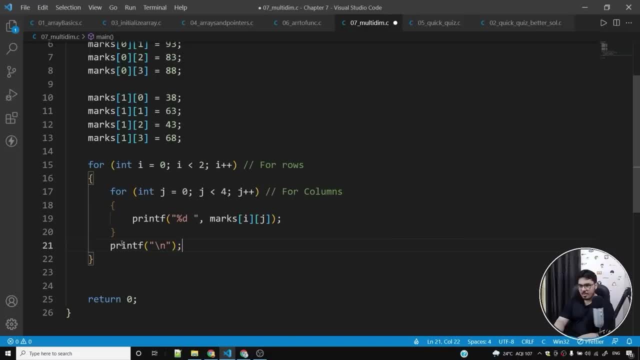 print backslash n, so i can say print f, and i can do something like this. i can, and i can do something like this. i can and i can do something like this. i can say backslash n, say backslash, n, say backslash n. so i'm printing a new line every time. 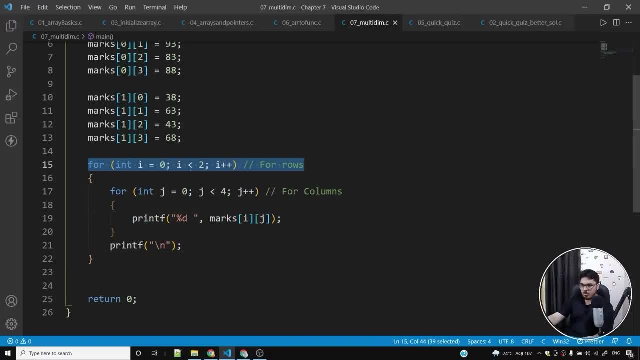 so i'm printing a new line every time. so i'm printing a new line every time. entire row gets painted, so this will run. entire row gets painted, so this will run. entire row gets painted, so this will run for the first row and once. for the first row and once. 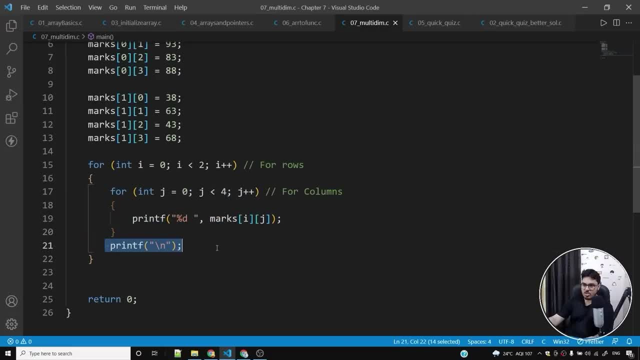 for the first row. and once all the elements are painted for the, all the elements are painted for the, all the elements are painted for the first row, i'll print a backslash n first row. i'll print a backslash n first row. i'll print a backslash n. try to visualize this. try to do the dry. 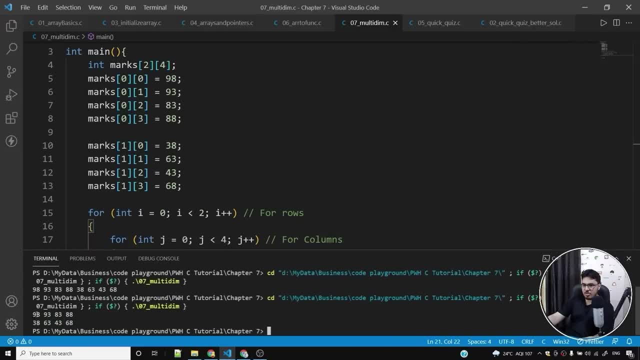 try to visualize this, try to do the dry. try to visualize this, try to do the dry. run of this program, run of this program, run of this program. and if i run this program now you'll see. and if i run this program now you'll see. and if i run this program now you'll see. for the first row, these values are: 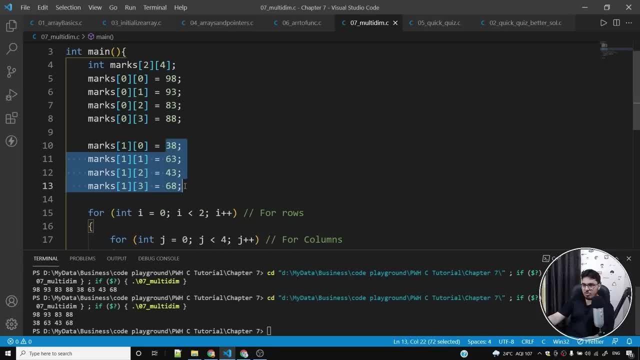 for the first row. these values are for the first row. these values are printed for the second row. all these printed for the second row. all these printed for the second row. all these values are printed. values are printed. values are printed. so these people have no interest in. 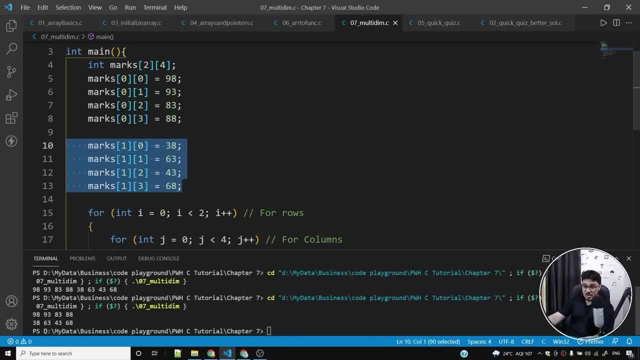 so these people have no interest in. so these people have no interest in studies. they studies, they studies, they score. i know relatively low marks and score. i know relatively low marks and score. i know relatively low marks. and the first row is the list of students. the first row is the list of students. 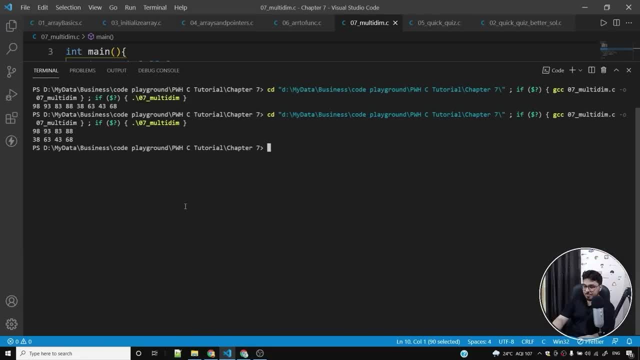 the first row is the list of students who, who, who, actually achieve good marks. so actually achieve good marks, so actually achieve good marks. so if i do something like this, you'll see. if i do something like this, you'll see. if i do something like this, you'll see. first row has: 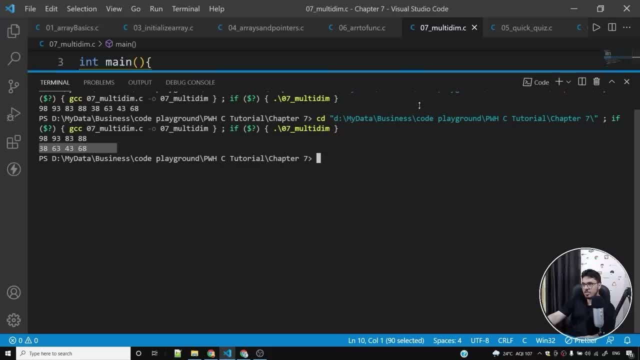 first row has: first row has four columns. second row has four columns, four columns. second row has four columns, four columns. second row has four columns. so two rows, four columns. so two rows, four columns. so two rows, four columns. this is what we you know initially. this is what we you know initially. 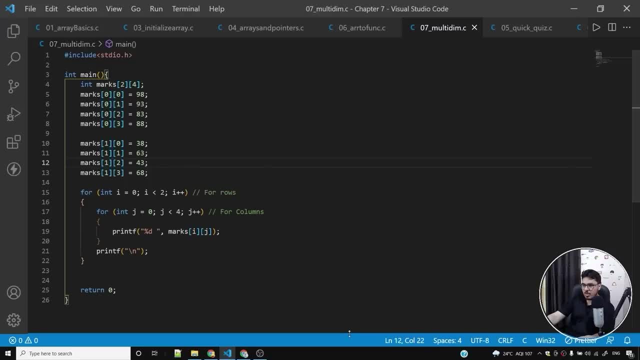 this is what we, you know, initially declared and this is how this works. so declared and this is how this works. so declared and this is how this works. so, if you want to, if you want to, if you want to, you know, visualize this directly, you can. you know, visualize this directly, you can. 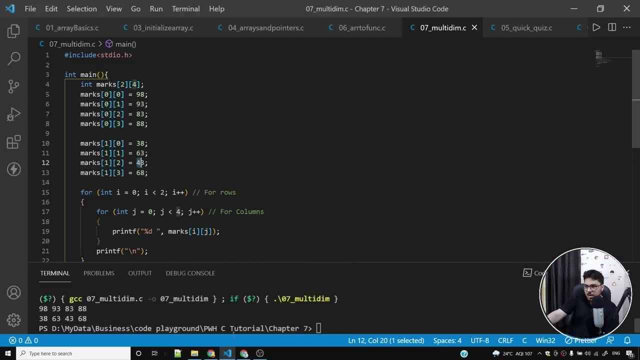 you know, visualize this directly. you can clearly see that, clearly, see that, clearly see that marks one: two is 43 and where is one two marks one, two is 43 and where is one two. marks one, two is 43 and where is one: two coming coming. 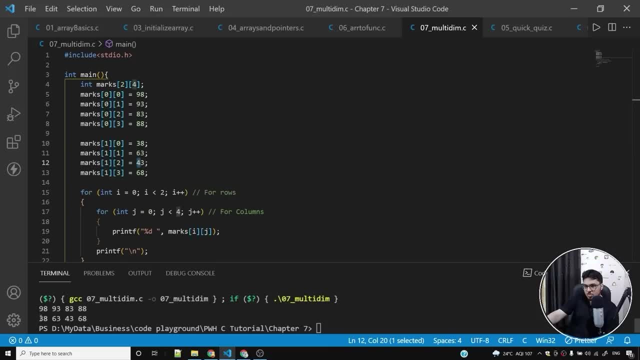 coming one, two will come somewhere here. let me one. two will come somewhere here. let me one. two will come somewhere here. let me show you here itself, show you here itself, show you here itself. so first row, sorry. second row marks one. so, first row, sorry. second row marks one. 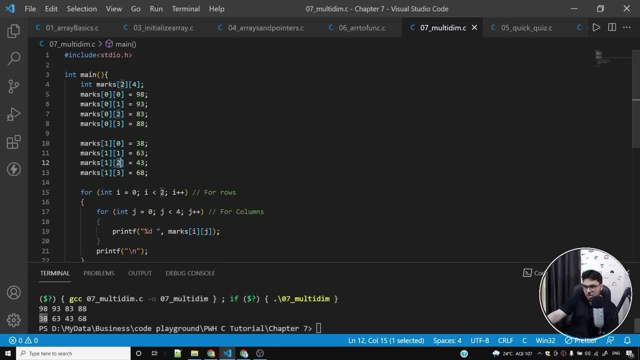 so first row. sorry, second row marks one is second row is second row is second row. and zero one. two third column, so zero one and zero one. two third column, so zero one and zero one. two third column, so zero one. two. this should be 43. two. this should be 43. 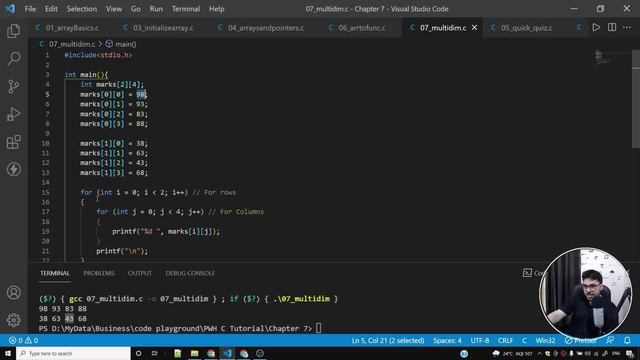 and yes, it's indeed 43 mark zero. zero is, and yes, it's indeed 43 mark zero. zero is, and yes, it's indeed 43 mark zero. zero is ninety eight mark zero, zero through ninety eight mark zero. zero through ninety eight mark zero. zero through zeroth column. this is zero through first. 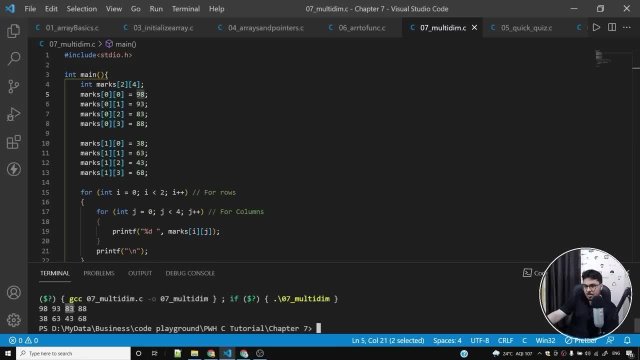 zeroth column. this is zero through first zeroth column. this is zero through first column, which is 93. this is zero through column, which is 93. this is zero through column, which is 93. this is zero through third column, third column, third column. um sorry, zero through zero one, two. 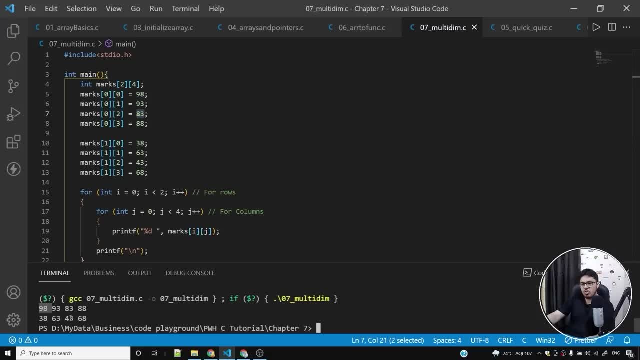 um sorry, zero through zero one two. um sorry, zero through zero one two. second column, which is 83, and so on. so second column, which is 83, and so on. so second column which is 83, and so on. so this is how you can visualize a two. 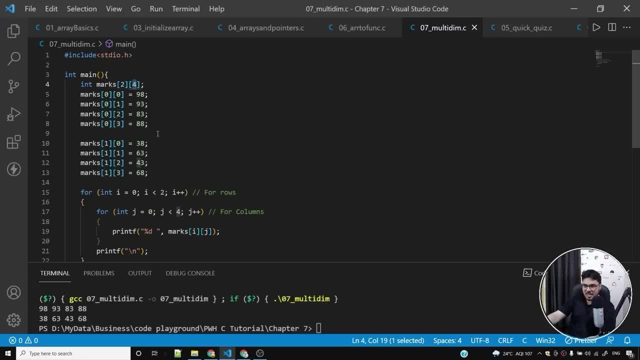 this is how you can visualize a two. this is how you can visualize a two dimensional array. now you can make it 20 dimensional array. now you can make it 20 dimensional array. now you can make it 20 and 40. you can make it as big of a. 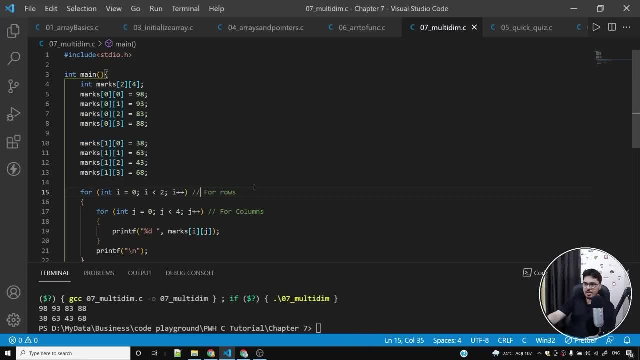 and 40. you can make it as big of a and 40. you can make it as big of a number as you want, but this is the idea number as you want, but this is the idea number as you want, but this is the idea. so i hope, i, uh, i hope that i was able to. 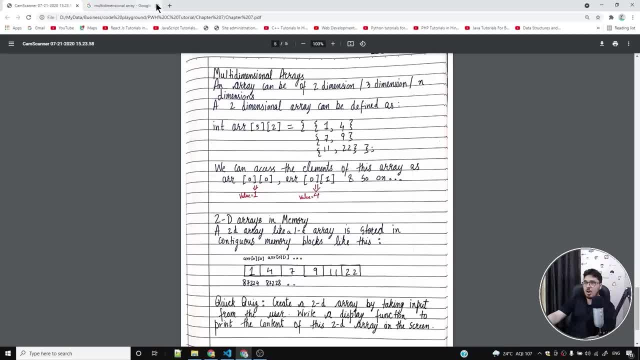 so i hope, i, uh, i hope that i was able to. so i hope i, uh, i hope that i was able to explain you all these things and you explain you all these things and you explain you all these things, and you understood, understood, understood how these multi-dimensional arrays work. 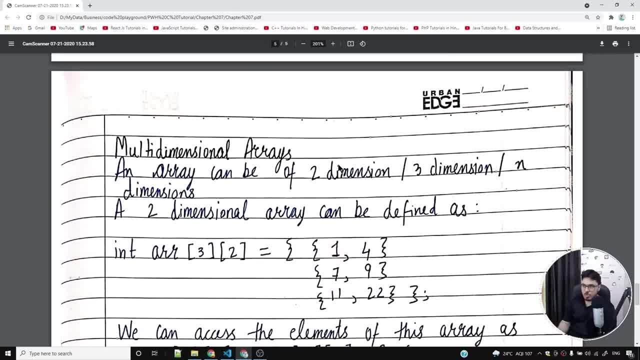 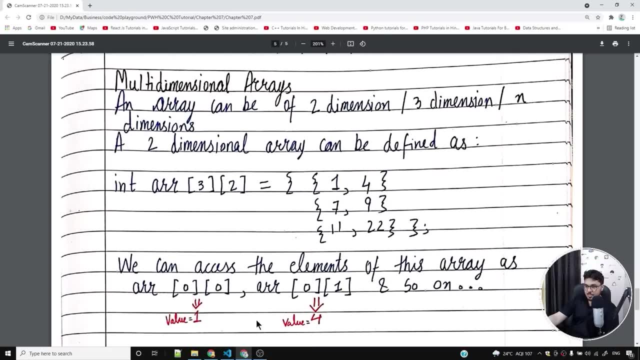 how these multi-dimensional arrays work, how these multi-dimensional arrays work. so i've written the same thing in the. so i've written the same thing in the. so i've written the same thing in the notes as well. an array can be of two notes as well. an array can be of two. 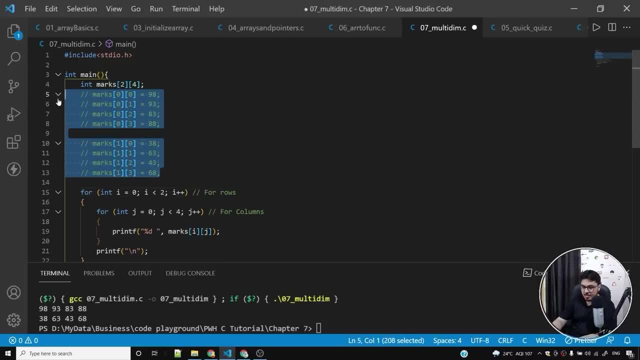 notes as well. an array can be of two. instead of doing this, instead of doing this, instead of doing this, i could have done, i could have done. i could have done. let me show you what i could have done. let me show you what i could have done. 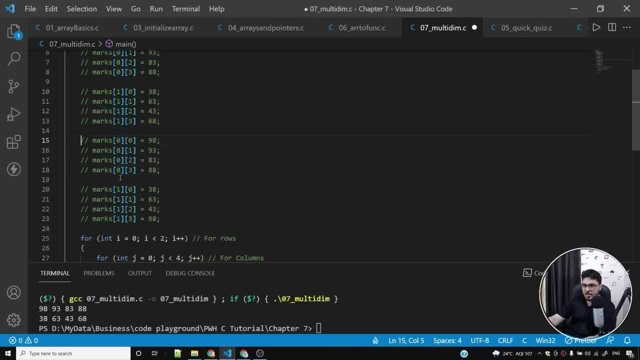 let me show you what i could have done- uh this, uh this, uh this. and let me try to use my visual studio. and let me try to use my visual studio and let me try to use my visual studio code skills here, code skills here, code skills here. so what i'll do is i'll simply take all 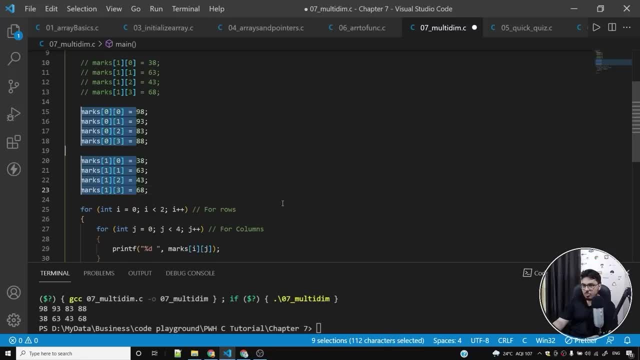 so what i'll do is i'll simply take all. so what i'll do is i'll simply take all the cursors here, the cursors here, the cursors here. i'll say shift home, so shift home will. i'll say shift home, so shift home will. 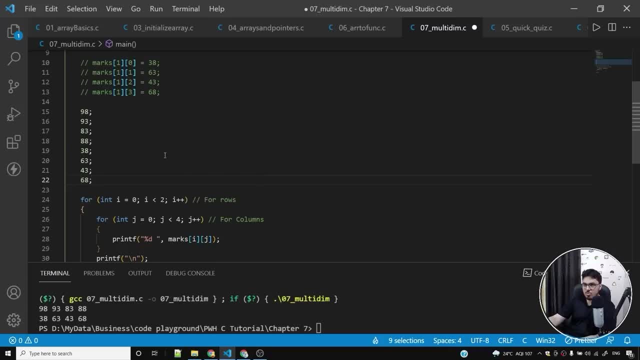 i'll say shift home will actually actually actually get me here. i'll press a backspace. get me here, i'll press a backspace, get me here, i'll press a backspace which will make me get rid of all these, which will make me get rid of all these. 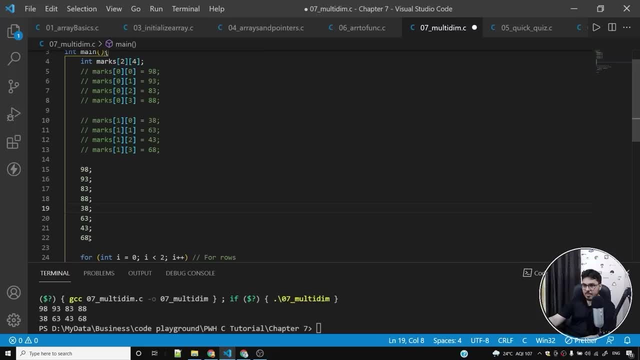 which will make me get rid of all these numbers, numbers, numbers. so one, two, three, four, five, six, seven. so one, two, three, four, five, six, seven. so one, two, three, four, five, six, seven, eight and four multiplied by two is eight, eight and four multiplied by two is eight. 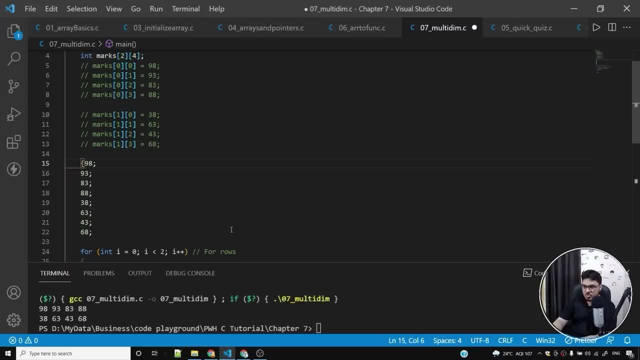 eight and four multiplied by two is eight. so we have all the numbers, so we have all the numbers. so we have all the numbers. now, what i want is i want to start this now. what i want is i want to start this now. what i want is i want to start this, uh. so i want to actually change all. 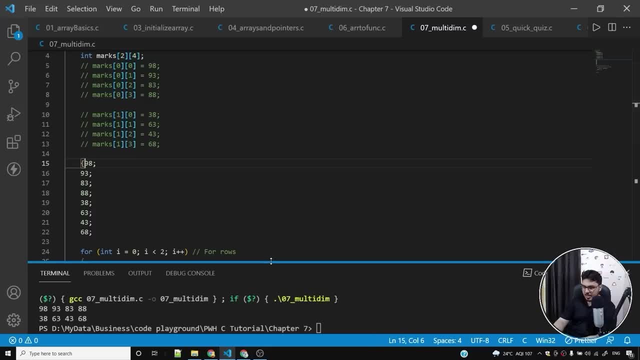 uh. so i want to actually change all uh, so i want to actually change all these two comma, these two comma, these two comma, uh, so what i'll do is i'll do something. uh, so what i'll do is i'll do something. uh, so what i'll do is i'll do something like this: 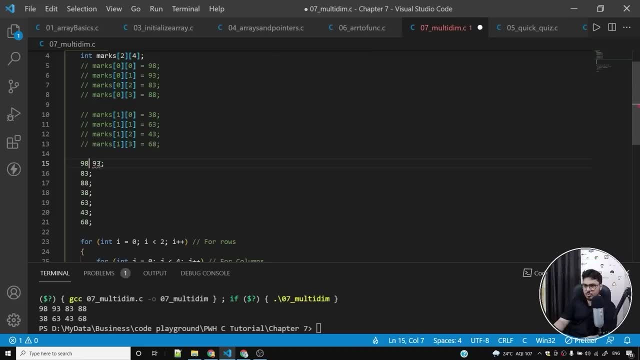 like this, like this: i'll, i'll take, uh, i'll, i'll take, uh, i'll, i'll take, uh, i'll do something like this. so there are, i'll do something like this. so there are, i'll do something like this. so there are four elements in one row. 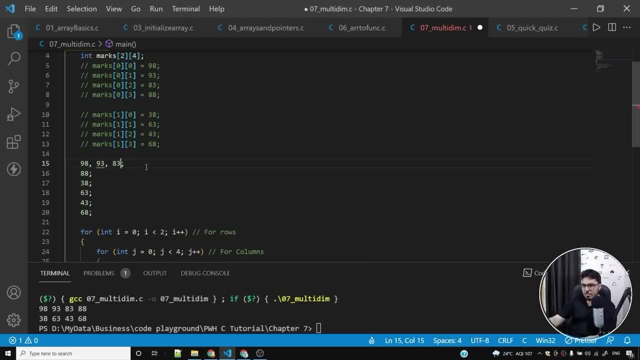 four elements in one row. four elements in one row. so i'll have to do something like this. so i'll have to do something like this. so i'll have to do something like this. i could have replaced this uh semicolon. i could have replaced this uh semicolon. 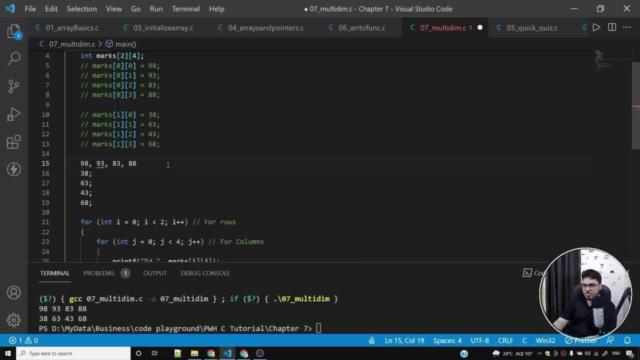 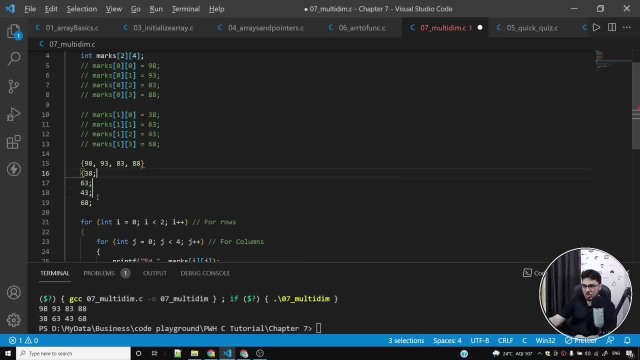 already here. let me show you how. so what i'll do is: let me show you how. so what i'll do is: let me show you how. so what i'll do is: i'll simply replace all these. i'll simply replace all these. i'll simply replace all these semicolons with a comma. 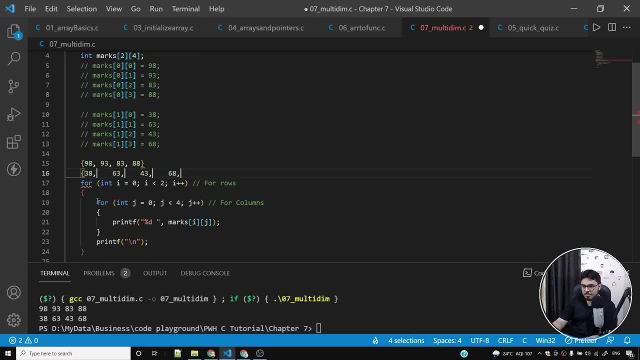 semicolons with a comma, semicolons with a comma, and i'll do something like this, and i'll do something like this, and i'll do something like this, and uh and uh and uh, and i think i'll simply use uh, and i think i'll simply use uh. 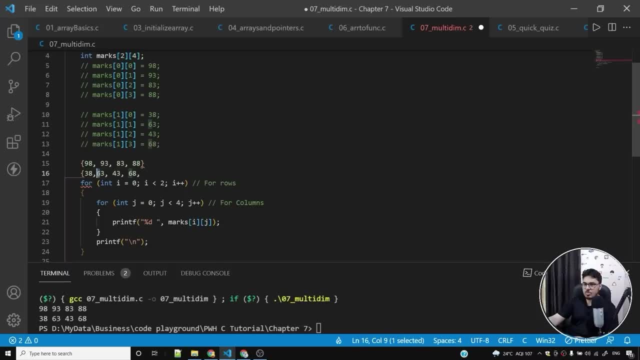 and i think i'll simply use, uh, keyboard, keyboard, keyboard. okay, so this was a bit time consuming. okay, so this was a bit time consuming. okay, so this was a bit time consuming for me, for me, for me, but again it's going to be worth it. but again it's going to be worth it. 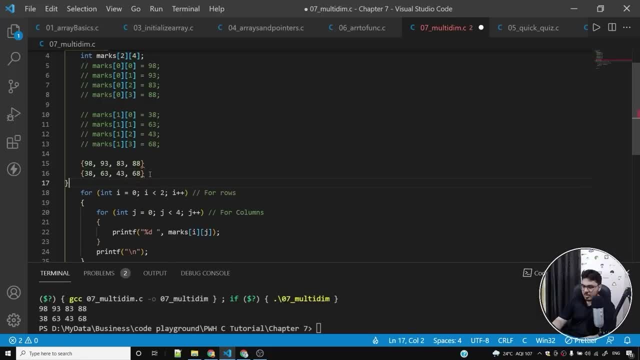 but again, it's going to be worth it for you because i'm going to explain you for you, because i'm going to explain you for you, because i'm going to explain you how two division arrays work, how two division arrays work, how two division arrays work. so let me put this curly brace here and 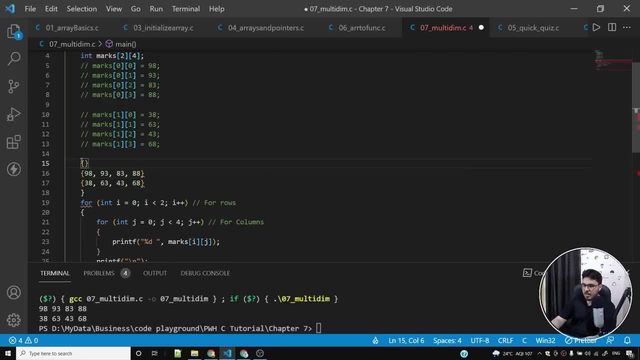 so let me put this curly brace here, and so let me put this curly brace here, and also, let me also, let me also, let me put another curly brace here. so put another curly brace here, so put another curly brace here. so basically, what? what is happening here? 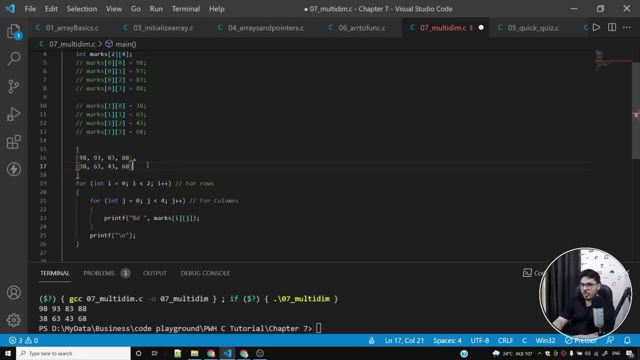 basically what? what is happening here? basically what. what is happening here is: let me put a comma here. let me put is: let me put a comma here. let me put is: let me put a comma here. let me put another comma here. okay, i don't need a. 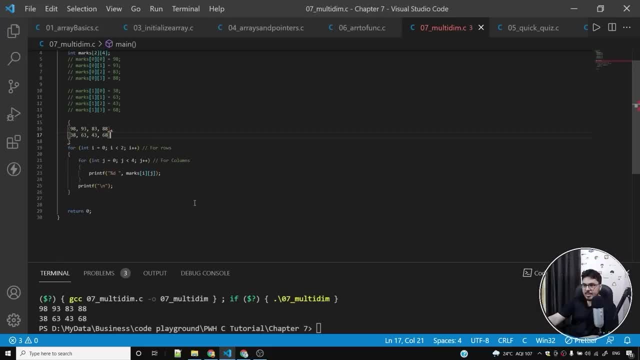 another comma here. okay, i don't need a another comma here. okay, i don't need a comma here, comma here, comma here. so i'll simply save it. and what is this error for expected a? what is this error for expected a. what is this error for expected a semicolon. 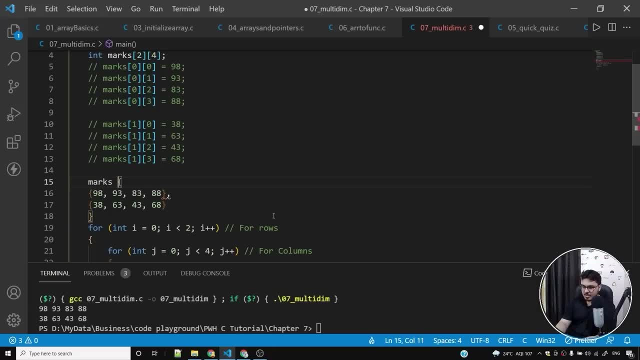 semicolon, semicolon. okay, so i'll do something like this. i'll okay, so i'll do something like this. i'll okay, so i'll do something like this. i'll say: say, say, marks, marks two, four is equal to, or rather i. marks two, four is equal to, or rather i. 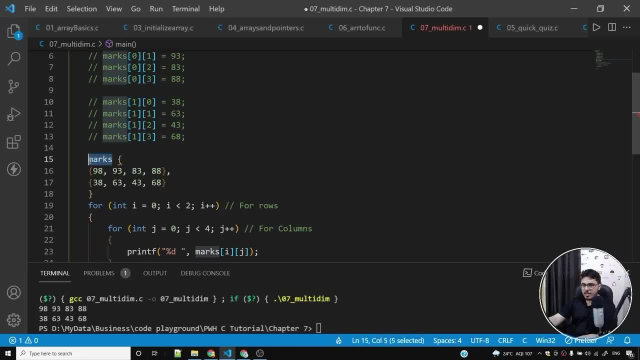 marks two, four is equal to. or rather, i can do, can do. can do this directly. instead of writing the this directly, instead of writing the this directly, instead of writing the declaration separately, i'll do this declaration separately. i'll do this declaration separately. i'll do this directly. 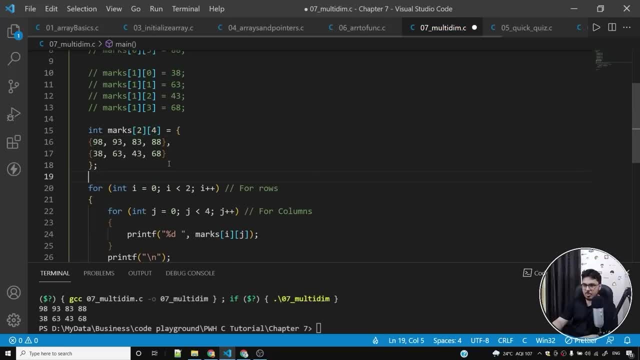 directly, directly, i'll do something like this and this will. i'll do something like this and this will work, and also i'll put a semicolon work, and also i'll put a semicolon work and also i'll put a semicolon here. so what is happening here is try to. 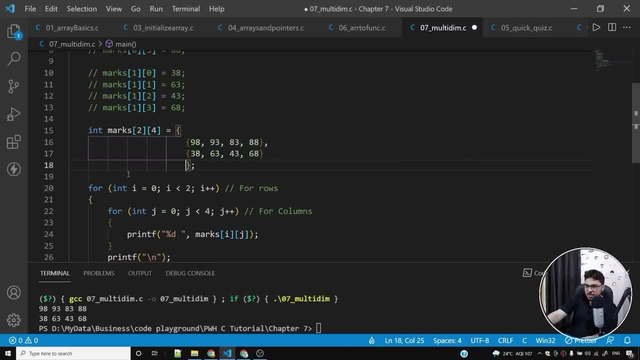 here. so what is happening here is try to here. so what is happening here is, try to understand this. what is happening here, understand this. what is happening here, understand this. what is happening here is, i am saying, is, i am saying, is i am saying: give me an array of arrays two. 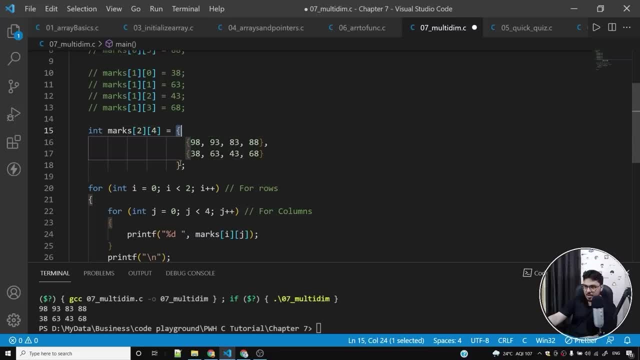 give me an array of arrays two. give me an array of arrays. two dimensional array is nothing but array. dimensional array is nothing but array. dimensional array is nothing but array of arrays. so this is an array. and inside of arrays, so this is an array. and inside of arrays. so this is an array, and inside this are a lot of arrays. so there are two. 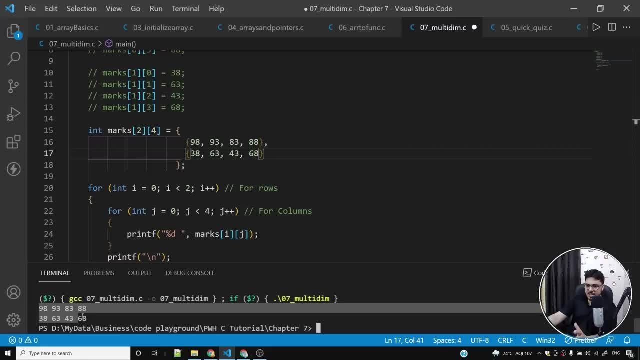 this are a lot of arrays, so there are two. this are a lot of arrays, so there are two arrays inside of this. so basically i'm arrays inside of this, so basically i'm arrays inside of this. so basically i'm writing this grid as is, so if i run this, 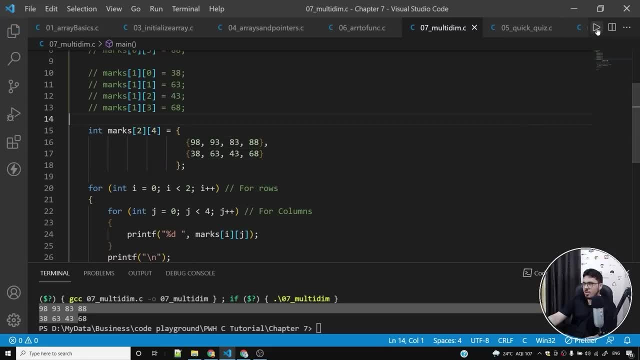 writing this grid, as is so. if i run this, writing this grid, as is so, if i run this program, i'll save it and run this program. i'll save it and run this program. i'll save it and run this program. you'll get the same output. you'll. 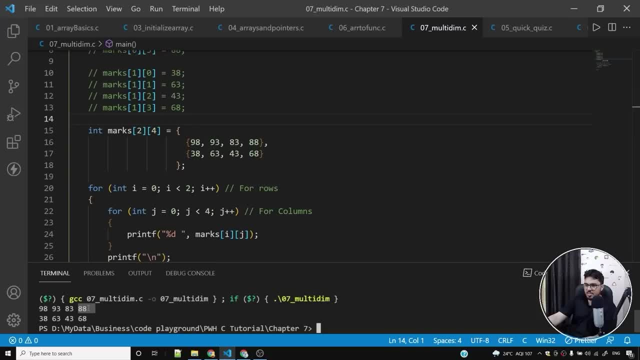 program, you'll get the same output. you'll program, you'll get the same output. you'll get the same grid as the output. no, get the same grid as the output. no, get the same grid as the output. no surprises whatsoever. so 83, 88, 38, 63, 43. 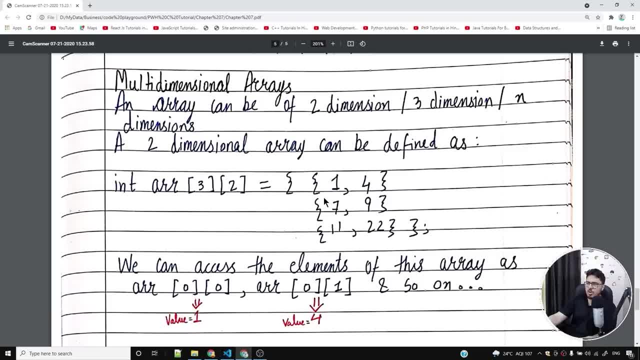 surprises whatsoever. so 83, 88, 38, 63, 43, surprises whatsoever. so 83, 88, 38, 38, 63, 43, 68 and so on. okay, so this is another 68 and so on. okay, so, this is another 68, and so on. okay, so this is another way of writing. um, all the values of a. 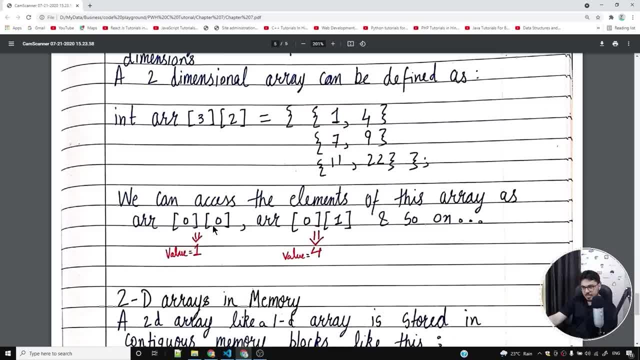 way of writing um all the values of a way of writing um all the values of a two-dimensional array. we can access the two-dimensional array. we can access the two-dimensional array. we can access the elements of this array as ar 00- ar 01. elements of this array as ar 00- ar 01. 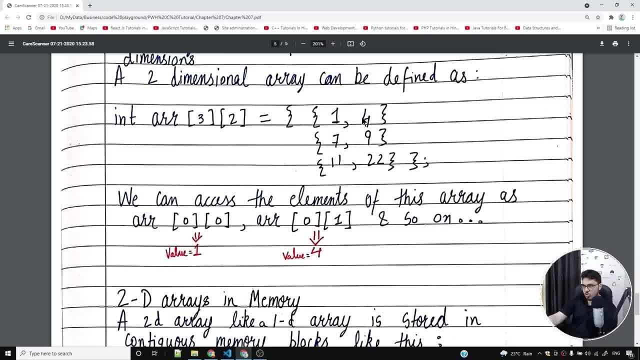 elements of this array as ar 00, ar 01, and so on. so ar 01 is four because, and so on. so ar 01 is four because, and so on. so ar 01 is four because. zero through and the this particular. zero through and the this particular. 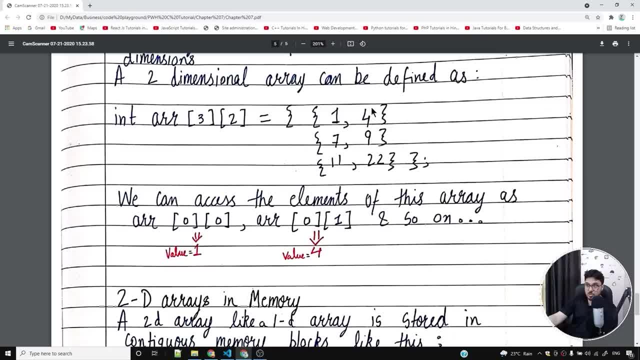 zero through and the this particular element zero, one element zero, one element zero, one first column starting from zero. so this first column starting from zero, so this first column starting from zero. so this is: how is? how is how two-dimensional arrays work and you can two-dimensional arrays work and you can. 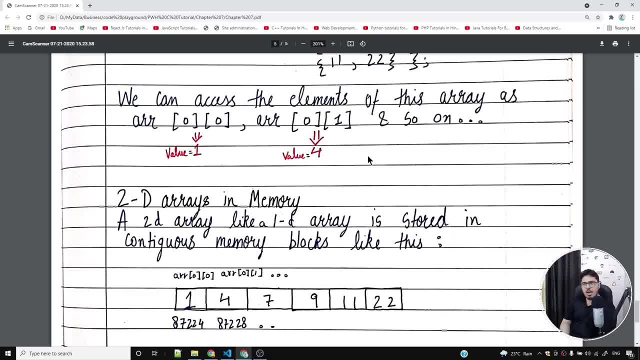 two-dimensional arrays work and you can have three dimensional arrays. you can have three dimensional arrays. you can have three dimensional arrays. you can have ten dimensional arrays. you can have have ten dimensional arrays. you can have have ten dimensional arrays. you can have nine, nine, nine dimensional arrays, and so. 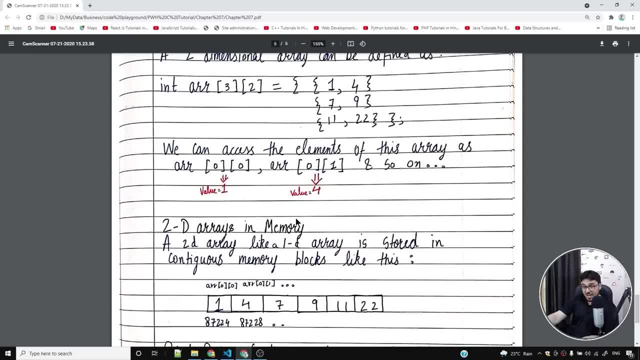 nine, nine, nine dimensional arrays, and so nine, nine, nine dimensional arrays, and so on, although it's very rare to see on, although it's very rare to see on, although it's very rare to see, uh, an array which is greater than three, uh, an array which is greater than three. 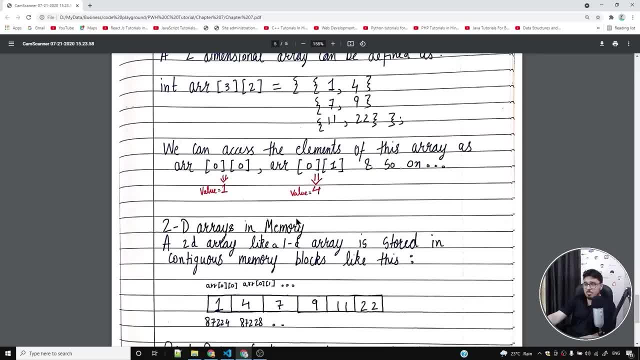 uh, an array which is greater than three. dimension three is the dimension three is the dimension three is the max and, in fact, two is something that is max and, in fact, two is something that is max and, in fact, two is something that is very rarely used. one dimensional arrays. 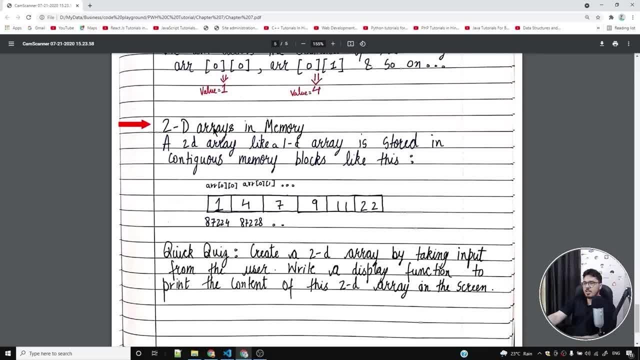 very rarely used one dimensional arrays. very rarely used. one dimensional arrays are very, very common. so are very, very common. so are very, very common. so let's try to see two dimensional arrays. let's try to see two dimensional arrays, let's try to see two dimensional arrays in memory. so a 2d array like a 1d array. 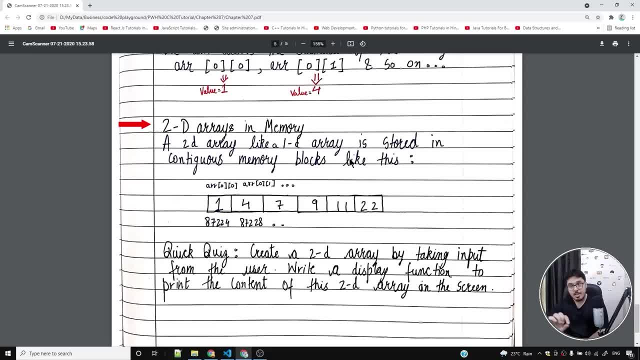 in memory. so a 2d array like a 1d array in memory. so a 2d array like a 1d array stored in contiguous memory blocks. always stored in contiguous memory blocks, always stored in contiguous memory blocks. always remember that the memory in our 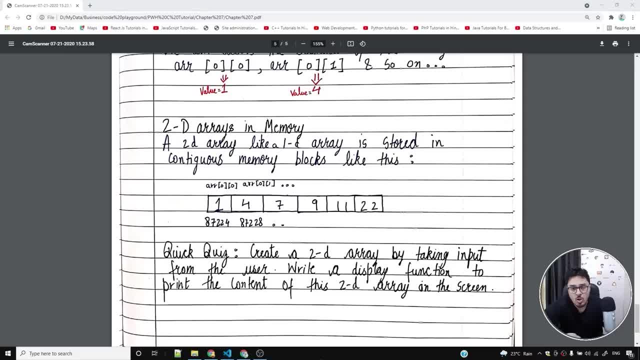 remember that the memory in our, remember that the memory in our computer consists of contiguous memory. computer consists of contiguous memory, computer consists of contiguous memory blocks, so the contiguous memory locations blocks, so the contiguous memory locations blocks, so the contiguous memory locations simply work this way that if we have two, 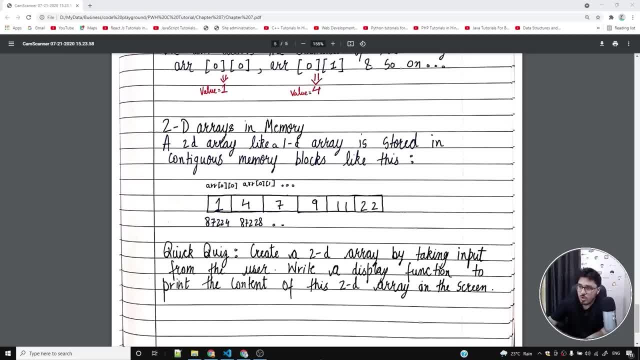 simply work this way, that if we have two, simply work this way, that if we have two to two, then the next memory location to two to two, then the next memory location to two to two, then the next memory location will be two to three, and so on. so if we 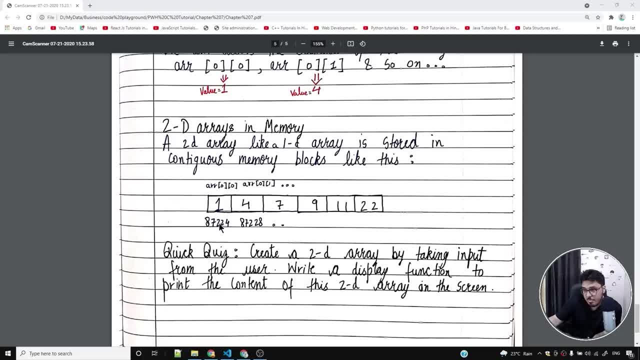 will be two to three and so on. so if we will be two to three and so on, so if we have have have an array which contains integers, the, an array which contains integers, the an array which contains integers, the memory locations will look like this. so, memory locations will look like this. so 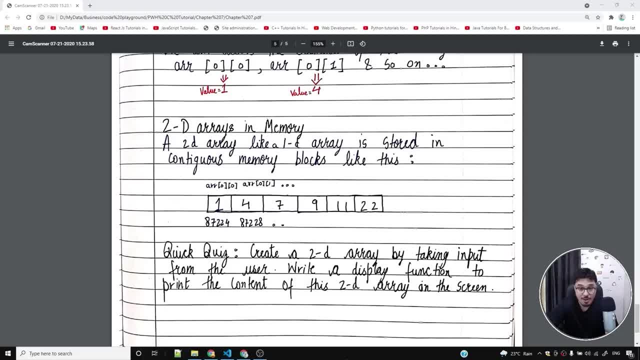 memory locations will look like this. so if we have an array of integers, uh, the. if we have an array of integers, uh, the. if we have an array of integers, uh, the memory locations will have a gap. of memory. locations will have a gap of memory. locations will have a gap of four between them. so if we have one, four, 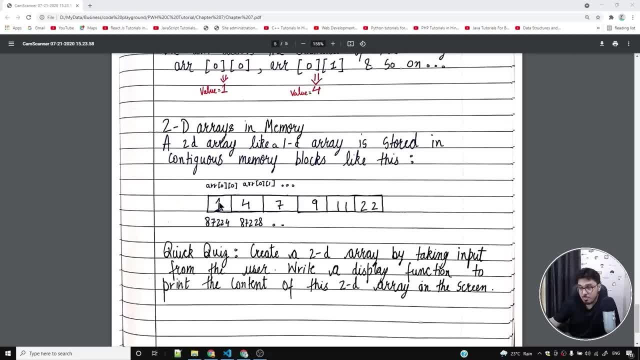 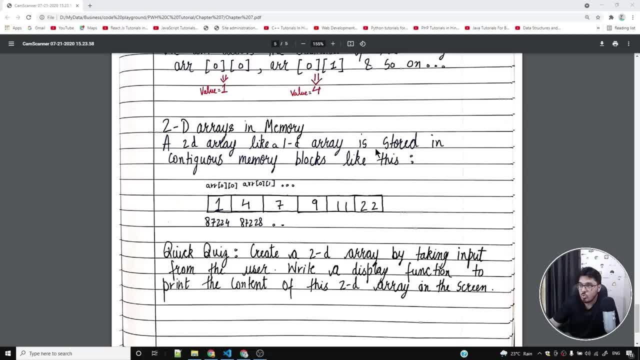 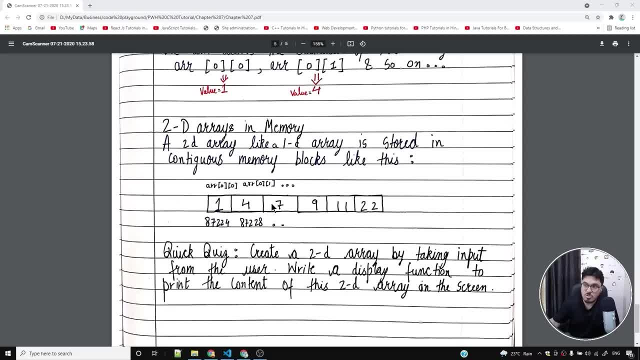 contiguous blocks like this: error 0 0. contiguous blocks like this: error 0: 0 will be stored here. error 0: 1 will be: will be stored here. error 0: 1 will be: will be stored here. error 0: 1 will be this. so they are actually one. 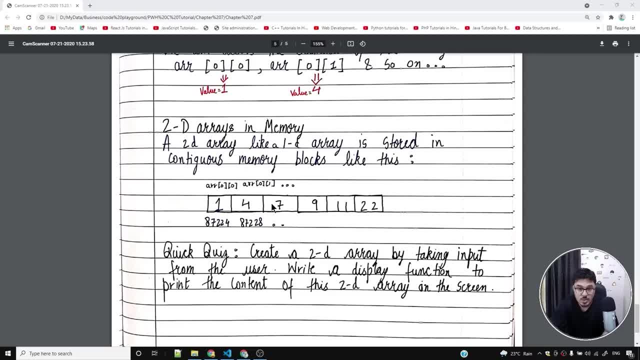 this, so they are actually one. this, so they are actually one dimensional, but they appears to be dimensional. but they appears to be dimensional, but they appears to be two-dimensional to us, two-dimensional to us, two-dimensional to us. try to think about it, so they are. try to think about it, so they are. 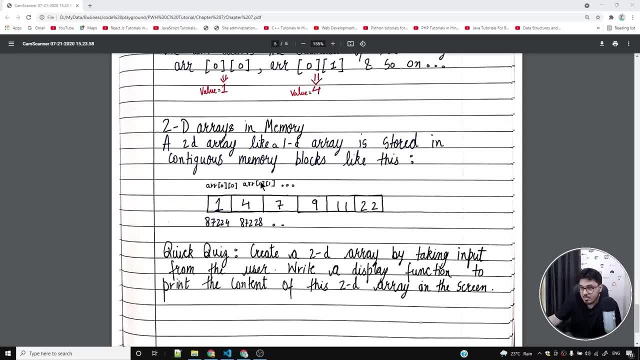 try to think about it. so they are contiguous memory blocks. the first block, contiguous memory blocks. the first block contiguous memory blocks. the first block is error 0- 0, next is error 0. 1 is error 0: 0, next is error 0- 1. 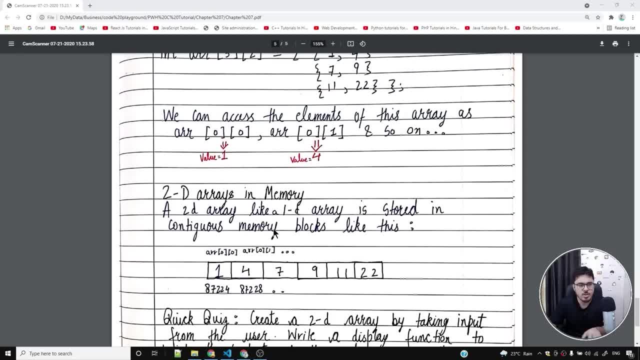 is error 0: 0. next is error 0: 1. and they are simply accessible using, and they are simply accessible using, and they are simply accessible using, these two indices zero one, zero two. these two indices zero one, zero two. these two indices zero one, zero two, two, two, three, two, so you can actually 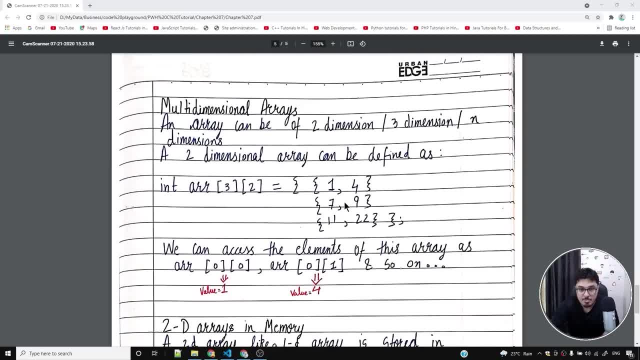 two, two, three, two. so you can actually two, two, three, two. so you can actually visualize a two-dimensional array like: visualize a two-dimensional array like: visualize a two-dimensional array like this, but actually deep within the memory. this, but actually deep within the memory. this, but actually deep within the memory. they are in a contiguous block. do not get. 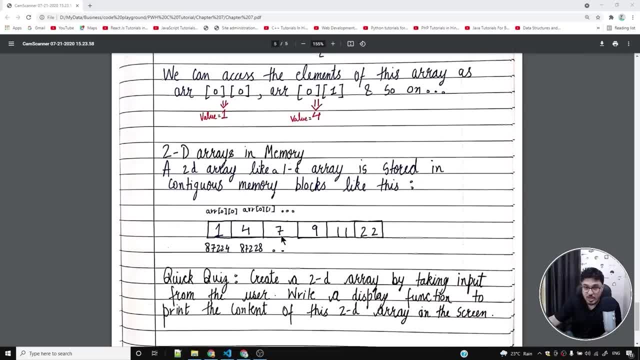 they are in a contiguous block. do not get. they are in a contiguous block, do not get. confused with this topic today, 2d. confused with this topic today. 2d. confused with this topic today 2d: arrays in memory. i just wanted to tell arrays in memory. i just wanted to tell. 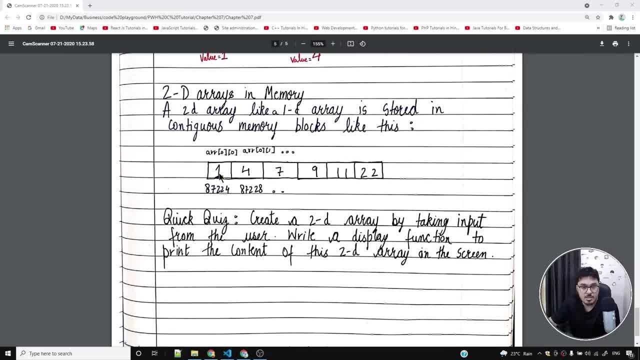 arrays in memory. i just wanted to tell you that all the data you, that all the data you, that all the data on your memory is stored in the form of on your memory is stored in the form of on your memory is stored in the form of contiguous blocks. so a 2d array, like a: 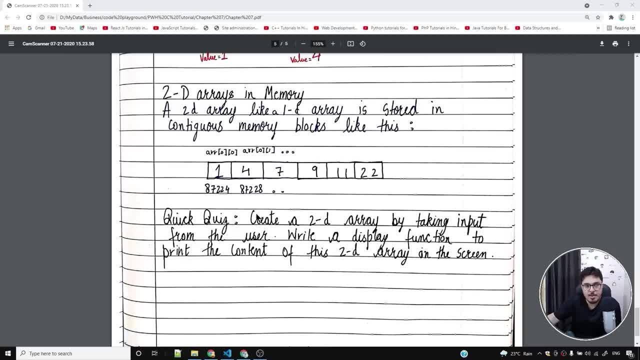 contiguous blocks. so a 2d array like a? contiguous blocks. so a 2d array like a 1d array stored in continuous blocks. 1d array stored in continuous blocks. 1d array stored in continuous blocks. and uh, there's a quick quiz for you. i. 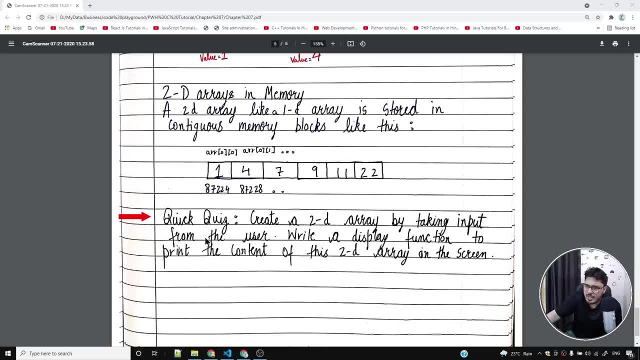 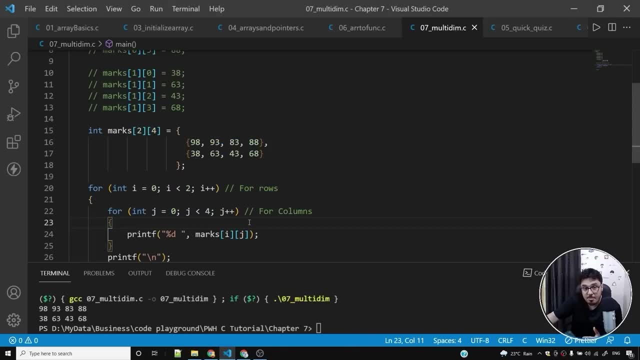 and uh, there's a quick quiz for you. i and uh, there's a quick quiz for you. i hope you understood this concept. you hope you understood this concept. you hope you understood this concept. you meant a 2d array, but you need to wrap. meant a 2d array, but you need to wrap. 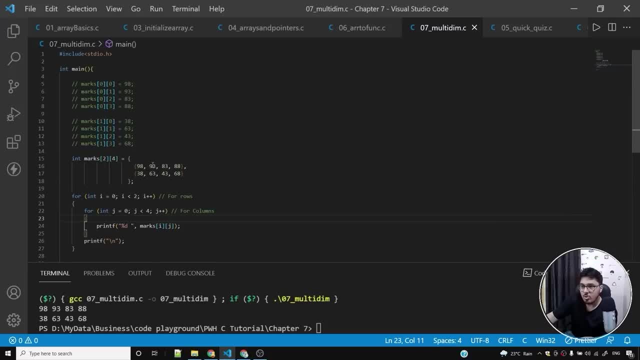 meant a 2d array, but you need to wrap it inside a display function and i hope it inside a display function and i hope it inside a display function and i hope that you understood this, that you understood this, that you understood this. i hope that this made complete sense to. 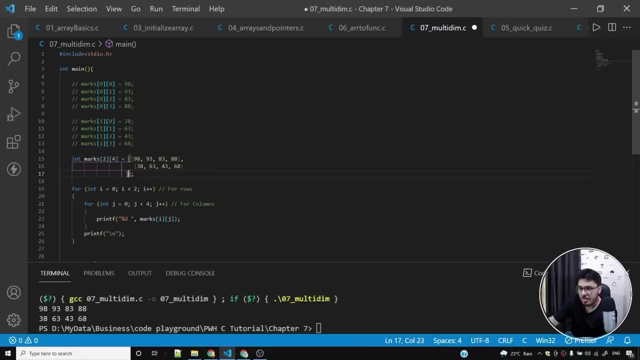 i hope that this made complete sense to. i hope that this made complete sense to you. you can actually get rid of the you. you can actually get rid of the you. you can actually get rid of the number of spaces here. number of spaces here, number of spaces here. if you think that the number of spaces 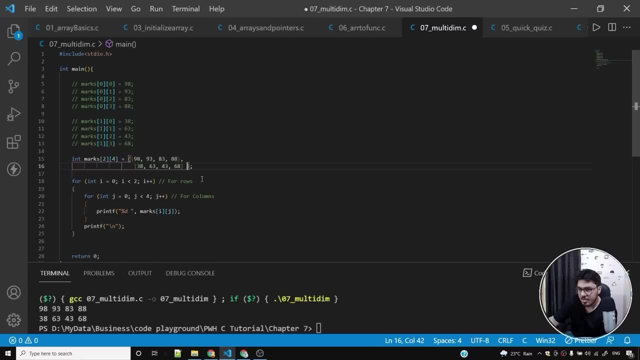 if you think that the number of spaces, if you think that the number of spaces being used are too much being used, are too much being used, are too much, so you can do something like this. you, so you can do something like this. you, so you can do something like this. you can get rid of these spaces. 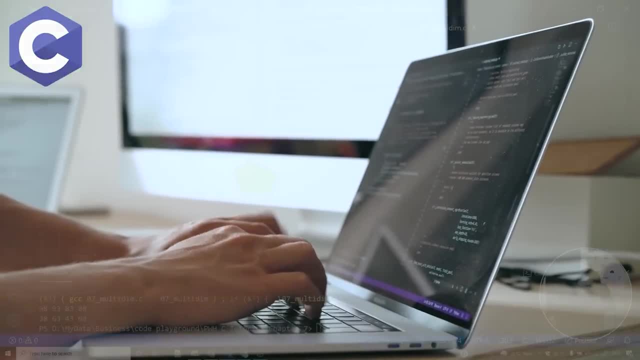 can get rid of these spaces. can get rid of these spaces if you add spaces inside c programming. if you add spaces inside c programming, if you add spaces inside c programming. language: it doesn't mind, so you can do. language: it doesn't mind, so you can do. 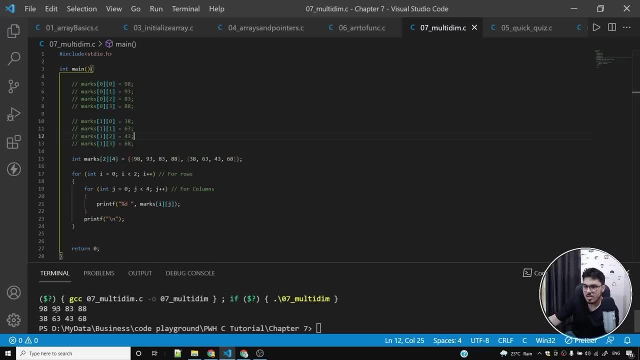 language, it doesn't mind. so you can do something like this as well, and the something like this as well, and the something like this as well, and the program will program, will program will very well work. so i hope that this very well work. so i hope that this 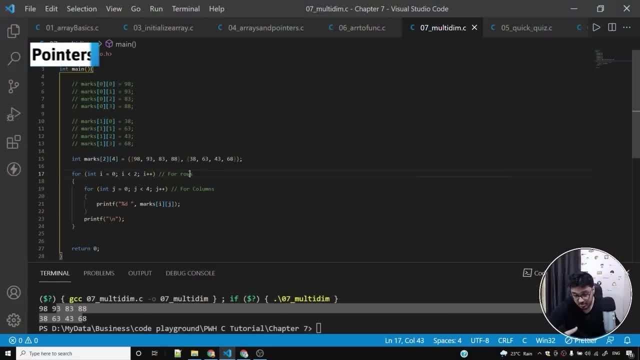 very well work. so i hope that this chapter made sense to you. we learned a chapter made sense to you. we learned a chapter made sense to you. we learned a lot of concepts. we learned about lot of concepts. we learned about lot of concepts. we learned about pointers- how arrays and pointers work. 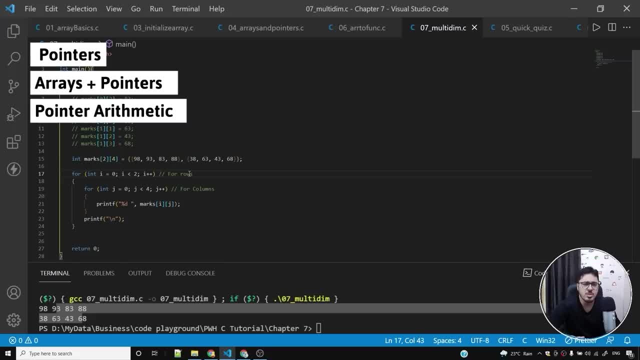 pointers, how arrays and pointers work. pointers, how arrays and pointers work together, how pointer arithmetic works so together, how pointer arithmetic works, so together, how pointer arithmetic works. so a lot of concepts in this chapter, a lot of concepts in this chapter. a lot of concepts in this chapter. in case we have not understood any: 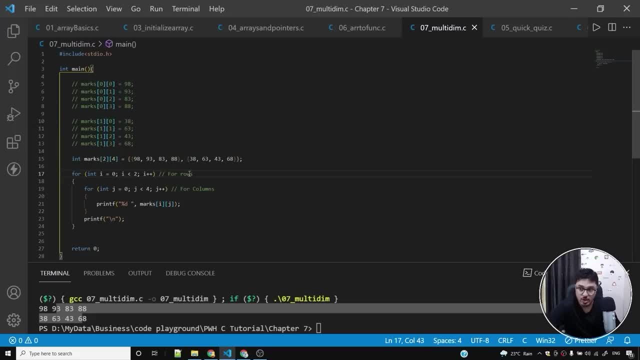 in case we have not understood any, in case we have not understood any concept: i concept, i concept. i urge you to remind this video and look at. urge you to remind this video and look at. urge you to remind this video and look at those concepts before proceeding. 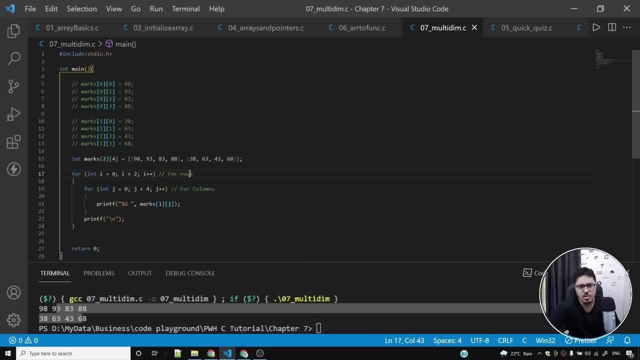 those concepts before proceeding, those concepts before proceeding. so we'll now move on to the next chapter. so we'll now move on to the next chapter. so we'll now move on to the next chapter, and we are going to look into more, and we are going to look into more. 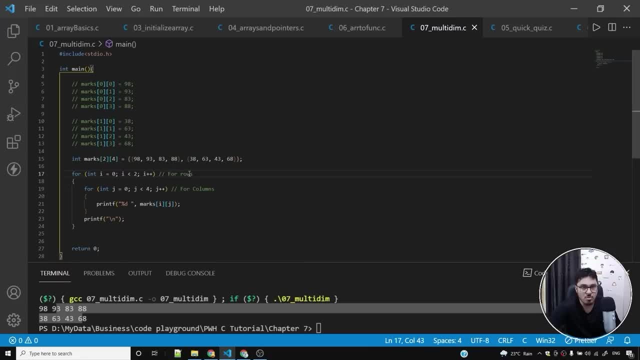 and we are going to look into more concepts. but before that we are going to concepts, but before that we are going to look into more concepts, but before that we are going to look into more. solve chapter seven practice set. so solve chapter seven practice set. so solve chapter seven practice set. so let's move on to chapter seven practice. 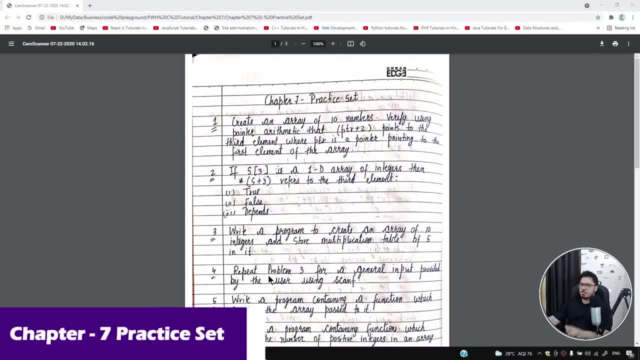 let's move on to chapter seven: practice. let's move on to chapter seven: practice set now, set now set now. all right. so time to solve the practice. all right, so time to solve the practice. all right, so time to solve the practice. set this practice set. set this practice set. 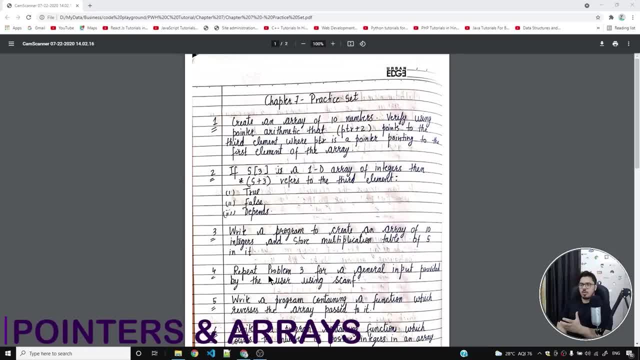 set. this practice set is related to pointers and arrays, so is related to pointers and arrays. so is related to pointers and arrays. so let's talk about this practice set. we'll. let's talk about this practice set. we'll. let's talk about this practice set. we'll talk about arrays in this practice. we'll. 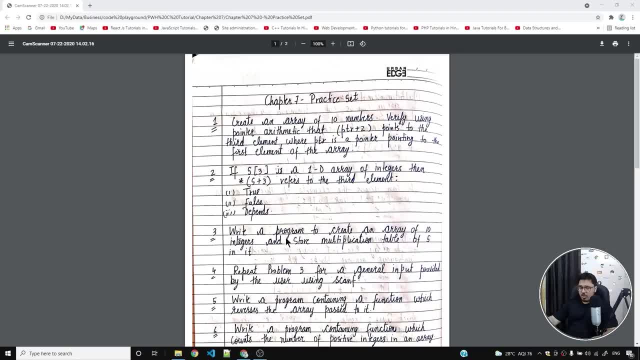 talk about arrays in this practice. we'll talk about arrays. in this practice. we'll practice problems on multi-dimensional practice set. we'll practice problems on multi-dimensional practice set. we'll practice problems on multi-dimensional arrays. let's see what all this arrays. let's see what all this. 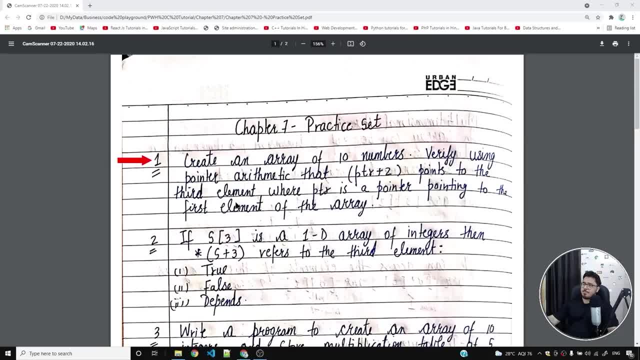 arrays. let's see what all this practice that has to offer. let's move to practice that has to offer. let's move to practice that has to offer. let's move to question number one: create an array of 10. question number one: create an array of 10. 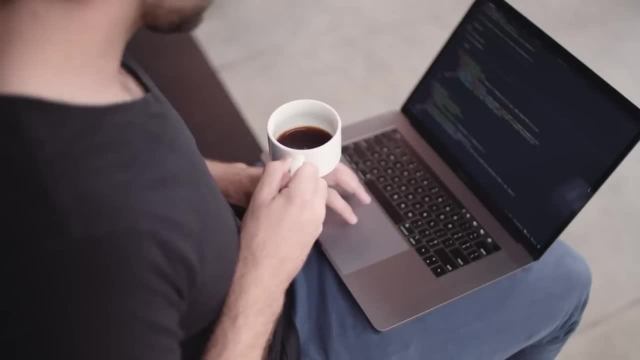 question number one: create an array of 10 numbers. you have to create an array of numbers. you have to create an array of numbers. you have to create an array of 10 numbers, which is pretty straightforward. 10 numbers, which is pretty straightforward. 10 numbers, which is pretty straightforward. at this point, if you are watching this, 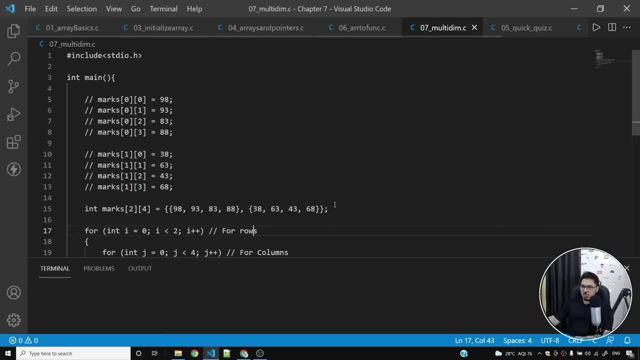 at this point, if you are watching this at this point, if you are watching this course, so let me open this particular course. so let me open this particular course. so let me open this particular folder on vs code and let me also create folder on vs code and let me also create. 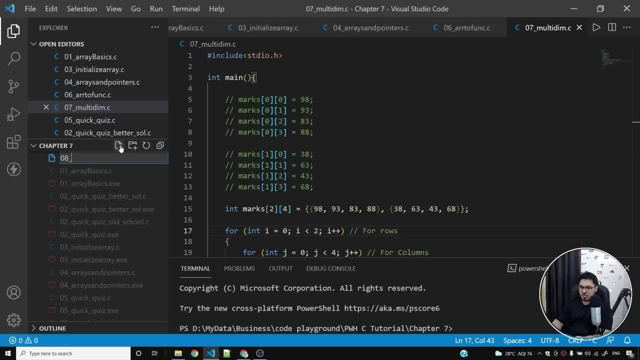 folder on vs code and let me also create a program for this first question. we a program for this first question, we a program for this first question. we want to start this question with problem, want to start this question with problem. want to start this question with problem number one. so let me say: 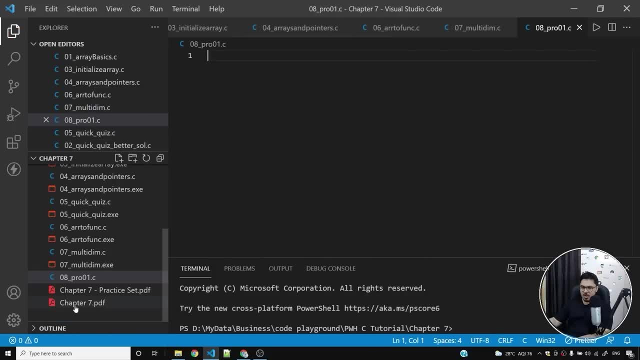 number one. so let me say number one. so let me say 08 underscore pr, not pro. 08 underscore pr, not pro. 08 underscore pr, not pro. i wanted to say pr pr01.c. i wanted to say pr pr01.c, i wanted to say pr pr01.c. and let me put the boilerplate code here. 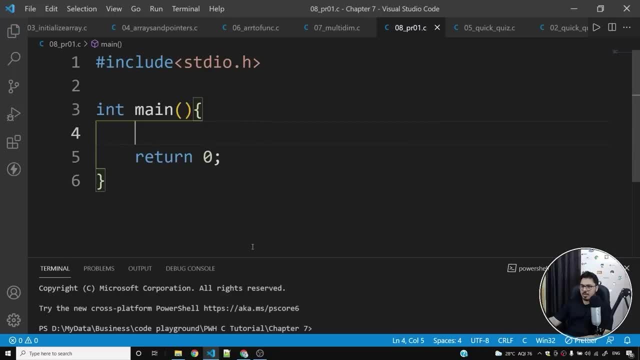 and let me put the boilerplate code here, and let me put the boilerplate code here, and and and. after putting the boilerplate code. what? after putting the boilerplate code? what after putting the boilerplate code? what i'll do, is i'll do, is i'll do is: i will simply create an array of 10. 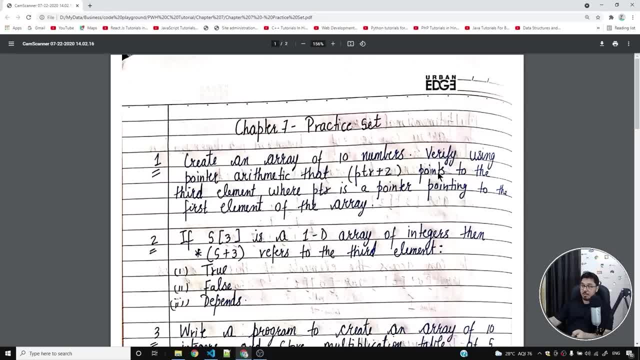 i will simply create an array of 10. i will simply create an array of 10 numbers, numbers, numbers. verify using pointer arithmetic that ptr. verify using pointer arithmetic that ptr. verify using pointer arithmetic that ptr plus two points to the third element plus two points to the third element. 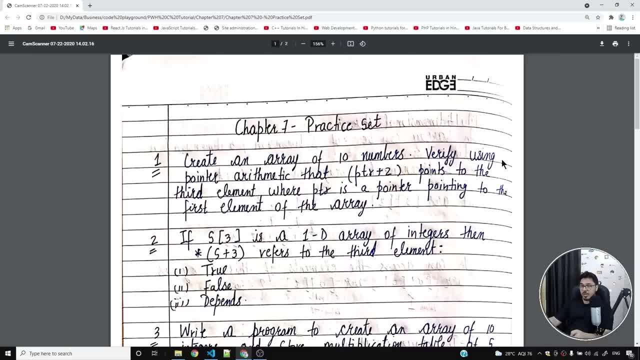 plus two points to the third element, where ptr is a pointer pointing to the, where ptr is a pointer pointing to the where ptr is a pointer pointing to the first element. first element, first element of the array. okay, so, let's, let's of the array. okay, so, let's, let's. 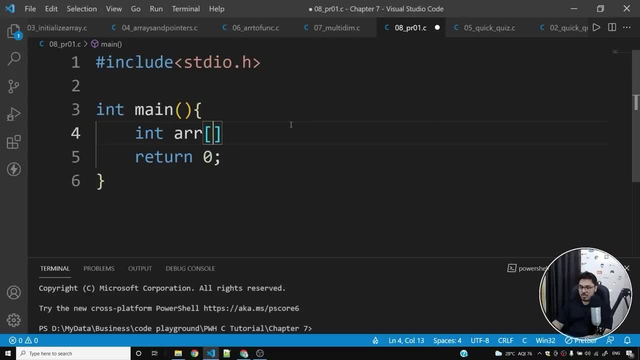 of the array. okay, so let's let's start discussing that, start discussing that, start discussing that. so what i'll do is i'll create an array. so what i'll do is i'll create an array. so what i'll do is i'll create an array of 10 numbers. 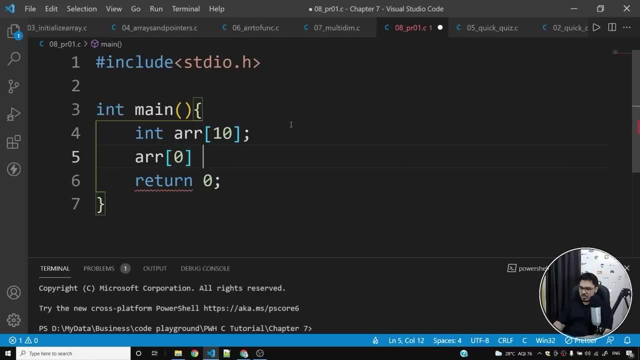 of 10 numbers, of 10 numbers. i've done that. i'll simply say arr 0. i've done that. i'll simply say arr 0. i've done that. i'll simply say arr 0 is equal to, is equal to, is equal to 7, and let me also fill in the values of: 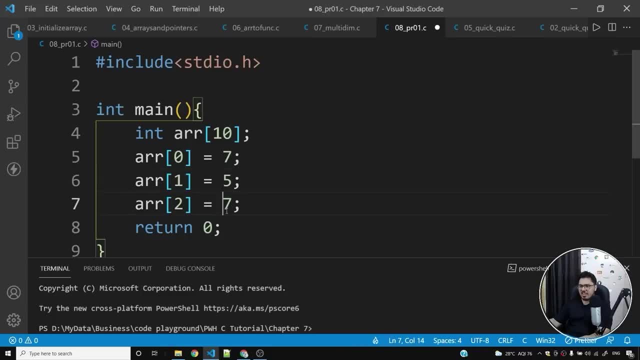 7, and let me also fill in the values of 7. and let me also fill in the values of error 1 and 2: error 1 and 2, error 1 and 2. i need not fill the values of arr 3. i need not fill the values of arr 3. 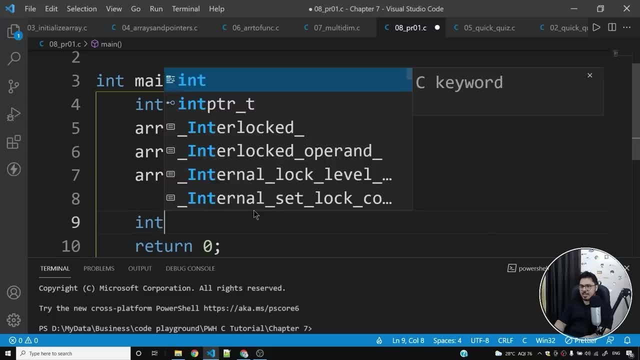 i need not fill the values of arr 3 onwards. let's skip that onwards. let's skip that onwards. let's skip that now. what i'll do is i'll say instar ptr. now, what i'll do is i'll say instar ptr. now, what i'll do is i'll say: instar ptr is equal to, so ptr is a pointer, and 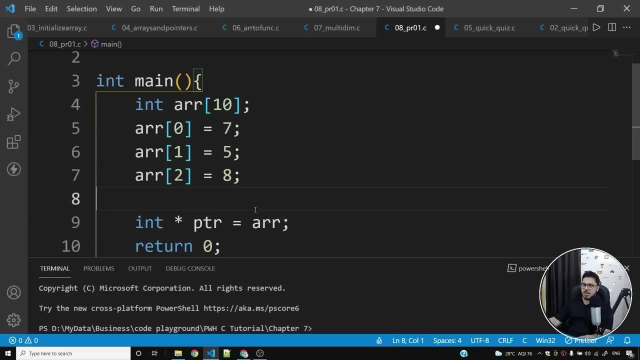 is equal to so. ptr is a pointer and is equal to so. ptr is a pointer and this pointer is pointing to the first. this pointer is pointing to the first. this pointer is pointing to the first element of the array. okay, element of the array. okay, element of the array. okay. so i can either say this, i can also say: 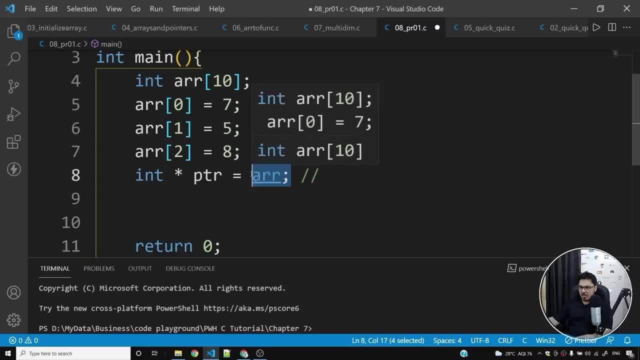 so i can either say this. i can also say so, i can either say this, i can also say this. this is also valid. this, this is also valid. this, this is also valid. uh instar ptr is equal to uh instar ptr is equal to uh instar ptr is equal to arr. 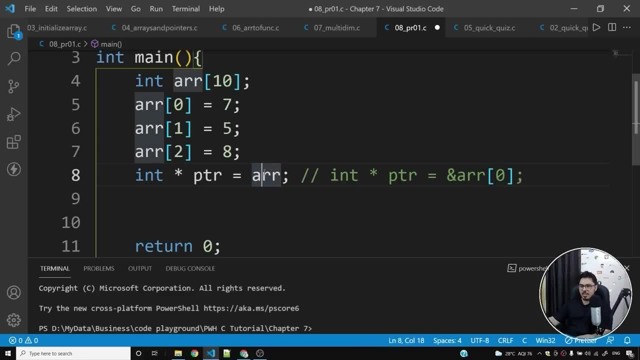 arr. arr. ampersand of error 0. this is also valid. ampersand of error 0. this is also valid. ampersand of error 0. this is also valid. this is the same thing. arr points to the. this is the same thing. arr points to the. 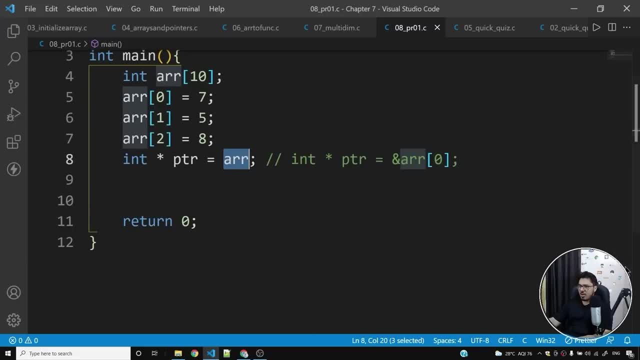 this is the same thing. arr points to the address of first element. we have address of first element. we have address of first element. we have already seen this. if, if you are, if you already seen this, if, if you are, if you already seen this, if, if you are, if you are still stuck, why this is the case? are still stuck. why this is the case, are still stuck, why this is the case? i think you have not watched the chapter. i think you have not watched the chapter. i think you have not watched the chapter carefully. i want you to watch the carefully. i want you to watch the. 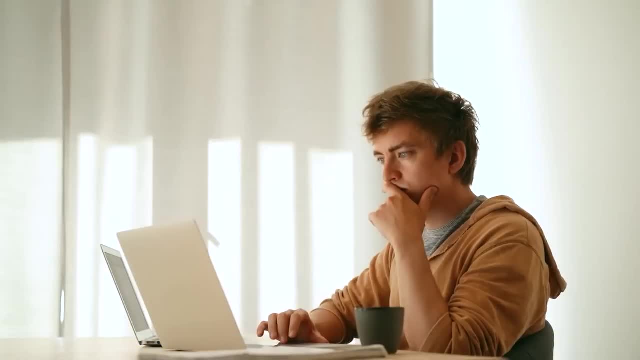 carefully. i want you to watch the chapter 7 carefully, and if you haven't chapter 7 carefully, and if you haven't chapter 7 carefully, and if you haven't done that, please go back to chapter 7. done that, please go back to chapter 7. 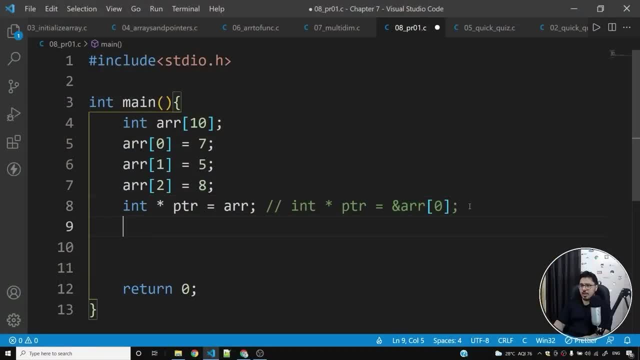 done that, please go back to chapter 7 and watch it carefully now. and watch it carefully now and watch it carefully now. instar ptr is equal to arr. now, what i'll- instar ptr is equal to arr now. what i'll do is i'll simply say: ptr is equal to. 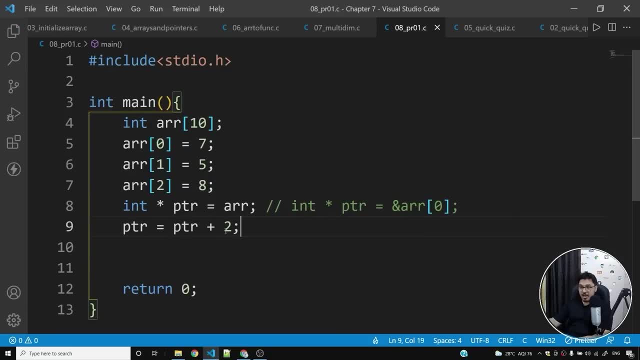 do is: i'll simply say ptr is equal to do is: i'll simply say ptr is equal to ptr plus 2, which means i'm updating ptr, ptr plus 2, which means i'm updating ptr, ptr plus 2, which means i'm updating ptr to 2. so let's now print the value. 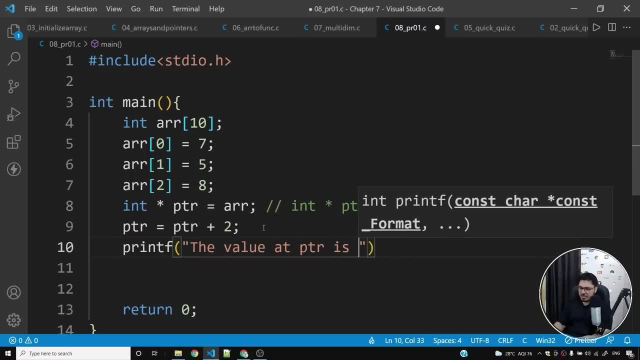 to 2. so let's now print the value to 2. so let's now print the value at ptr is and i'll simply say percentage at ptr is and i'll simply say percentage at ptr is, and i'll simply say percentage d, d, d, percentage d, and i'll simply. 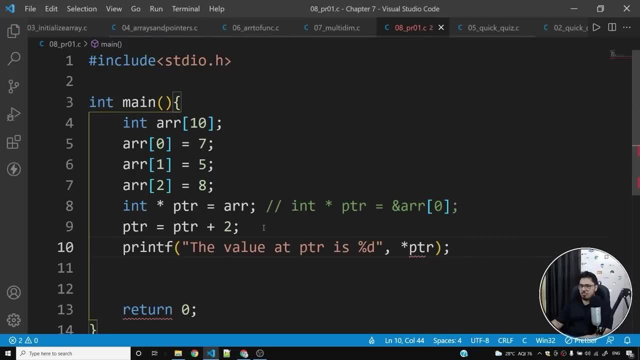 percentage d, and i'll simply percentage d, and i'll simply use the value at operator. use the value at operator, use the value at operator. which is star ptr, and let me also which is star ptr, and let me also which is star ptr, and let me also say the same thing here. so initially, 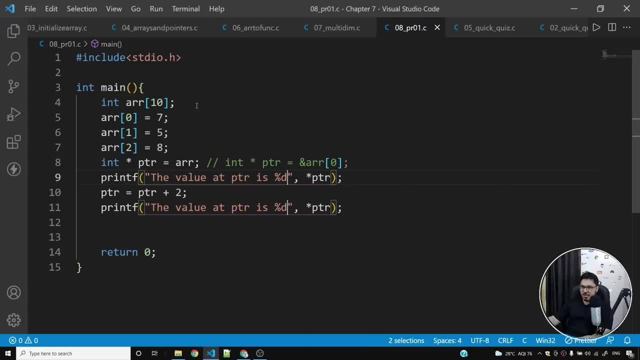 say the same thing here. so initially, say the same thing here. so initially, what will happen is the value at ptr. what will happen is the value at ptr. what will happen is the value at ptr will be 7 and later it's going to be will be 7 and later it's going to be. 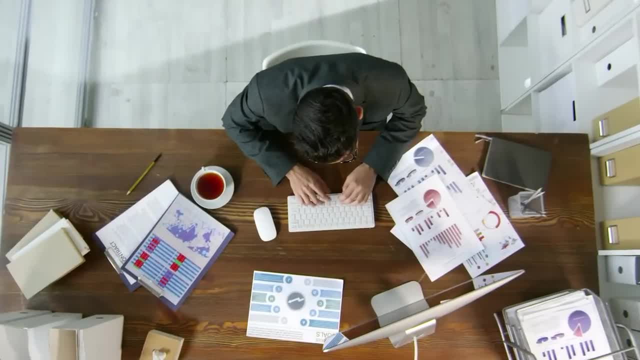 will be 7 and later it's going to be 8. okay, let's verify this. 8. okay, let's verify this 8. okay, let's verify this. and this is very straightforward. let me- and this is very straightforward- let me- and this is very straightforward- let me tell you: 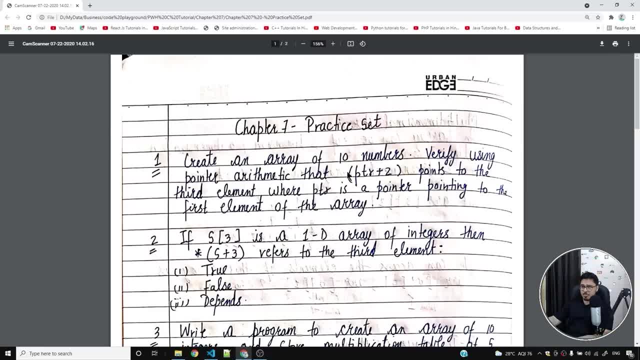 tell you. tell you so: initially it is 7, after that it is 8. so initially it is 7, after that it is 8. so initially it is 7, after that it is 8. because this is pointing to the third, because this is pointing to the third. 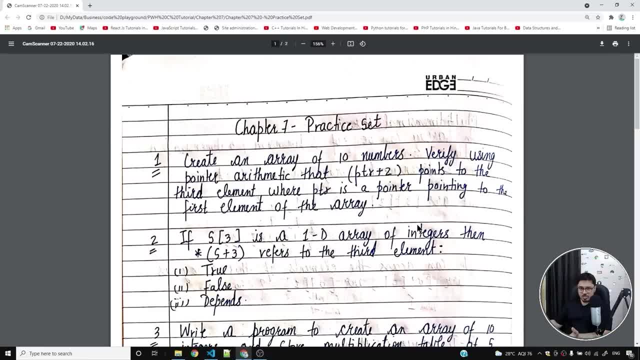 because this is pointing to the third element. now we have incremented element. now we have incremented element. now we have incremented the pointer by 2, which means initially it the pointer by 2, which means initially it the pointer by 2, which means initially it was pointing to the first element. 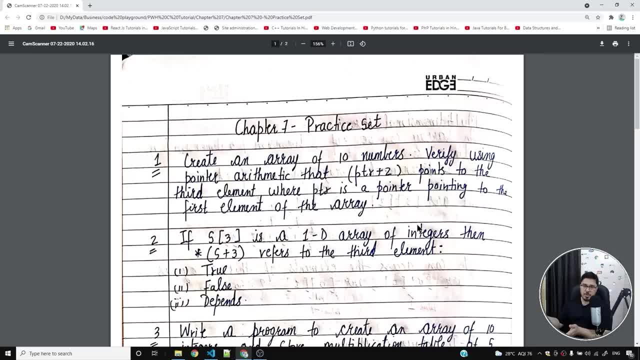 was pointing to the first element was pointing to the first element, then i shifted it by 2, which means it. then i shifted it by 2, which means it. then i shifted it by 2, which means it will now point to the third element. okay, will now point to the third element, okay. 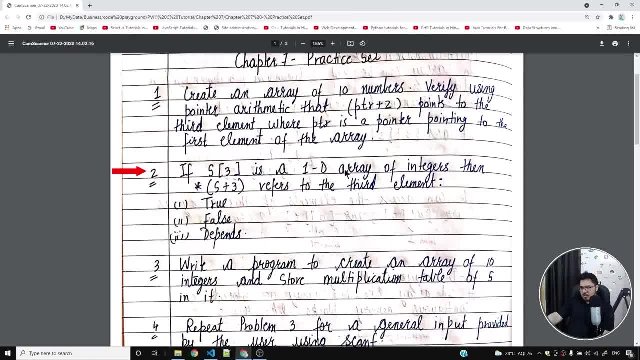 will now point to the third element. okay, this was pretty straightforward question. this was pretty straightforward question. this was pretty straightforward question. if s3 is a 1d array of integers, then if s3 is a 1d array of integers, then if s3 is a 1d array of integers, then star s plus 3 refers to the third. 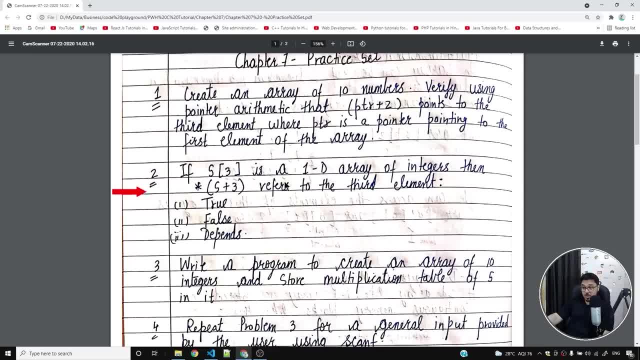 star s plus 3 refers to the third. star s plus 3 refers to the third element. is this true? is this true element? is this true? is this true element? is this true? is this true? tell me, is this true or not. i want you to tell me. is this true or not. i want you to. 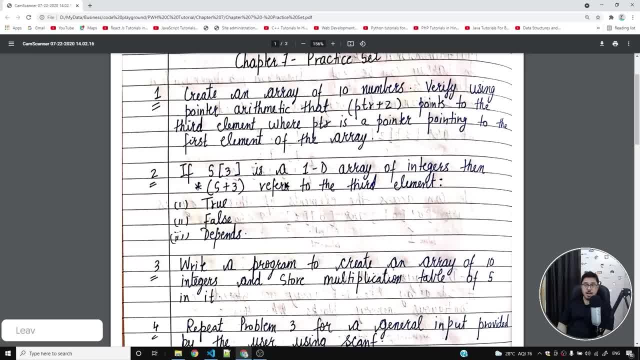 tell me: is this true or not? i want you to answer this question in the comments. answer this question in the comments. answer this question in the comments. write the timestamp and answer true. or write the timestamp and answer true. or write the timestamp and answer true or false. come on. 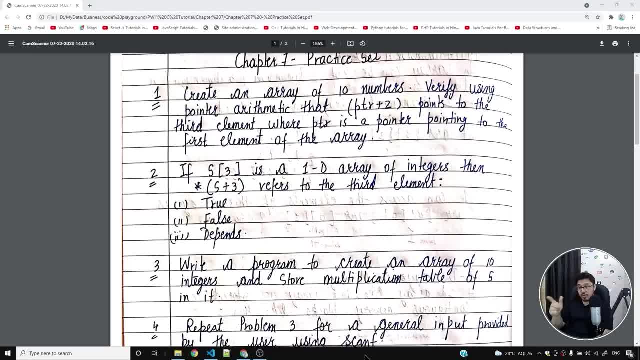 false, come on, false, come on. i'm waiting for your comment. okay, so if i'm waiting for your comment, okay, so, if i'm waiting for your comment, okay. so, if you have commented, i want you to. you have commented, i want you to. you have commented. i want you to understand that if s3 is a 1d array of 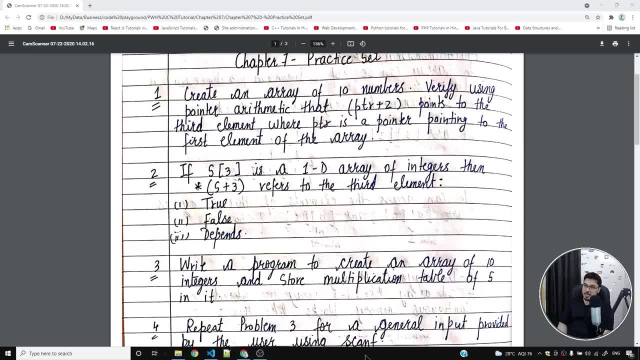 understand that if s3 is a 1d array of, understand that if s3 is a 1d array of integer s plus, one will point to the integer s plus one will point to the integer s plus one will point to the second element. if s is pointing to the 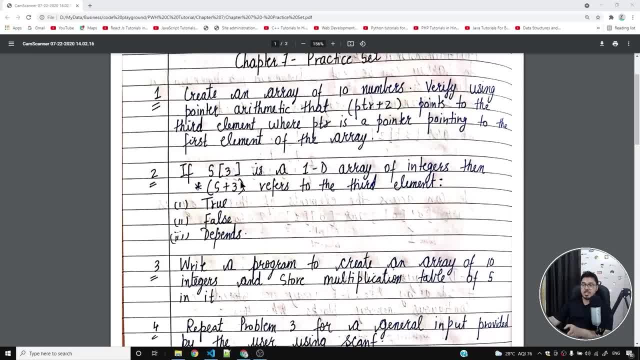 second element. if s is pointing to the second element. if s is pointing to the first element s plus one will point to first element s plus one will point to first element s plus one will point to the second element s plus two will point the second element s plus two will point. 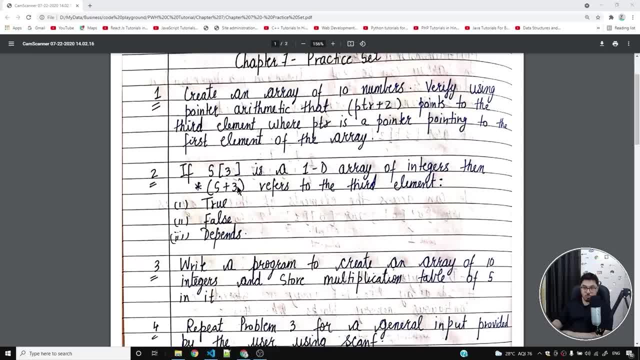 the second element s plus two will point to the third element s plus three will to the third element s plus three will to the third element s plus three will point to the fourth element, but there is point to the fourth element. but there is point to the fourth element, but there is no fourth element. there are only three. 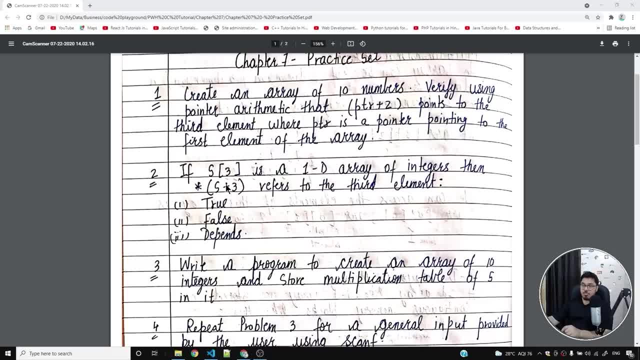 no fourth element, there are only three. no fourth element, there are only three elements. verify this using pointer elements. verify this using pointer elements. verify this using pointer arithmetic: you will find out. so let me arithmetic, you will find out. so let me arithmetic, you will find out. so let me let me google arrays. let me, uh, you know. 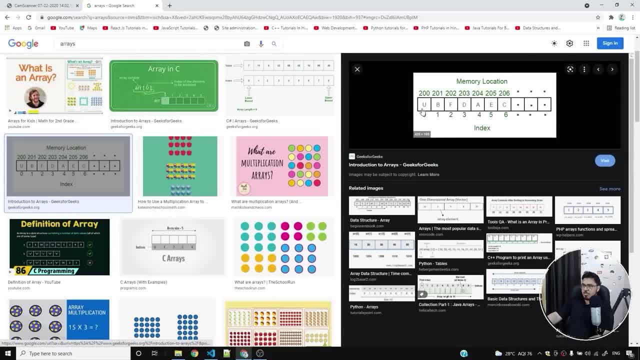 let me google arrays. let me- uh, you know, let me google arrays. let me- uh, you know- take some image and tell you so. let us take some image and tell you so. let us take some image and tell you so. let us say: this is the first element, this is ptr. 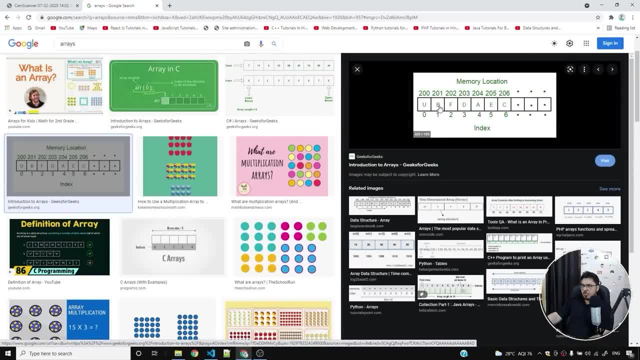 say this is the first element, this is ptr. say this is the first element, this is ptr. 200 is the ptr, so 200 is the ptr, so 200 is the ptr. so this particular value which is b, it is, this particular value which is b, it is. 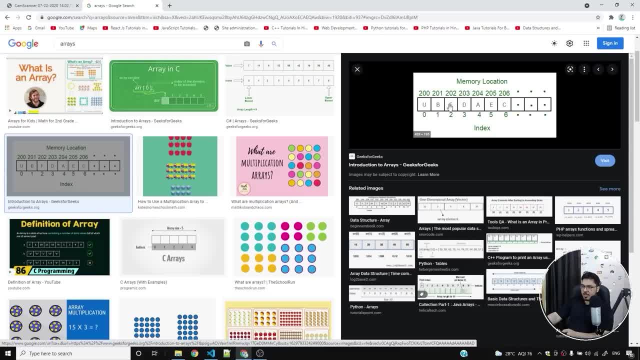 this particular value, which is b, it is ptr plus one, ptr plus two, ptr plus one, ptr plus two, ptr plus one, ptr plus two. so third element will be achieved after. so third element will be achieved after. so third element will be achieved after i uh increment my ptr by two. so if i 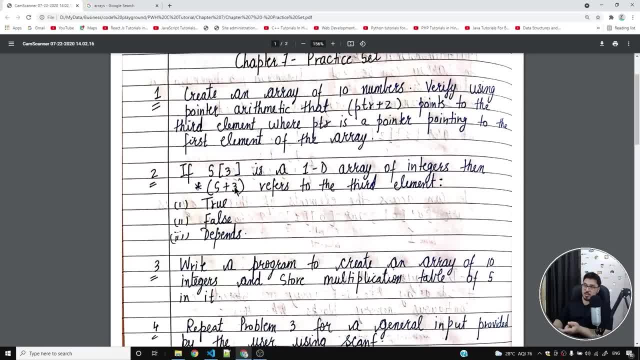 i uh increment my ptr by two. so if i i uh increment my ptr by two, so if i increment my ptr by three, increment my ptr by three, increment my ptr by three, that will point to the fourth element. that will point to the fourth element. that will point to the fourth element and not to the third element. so this is. 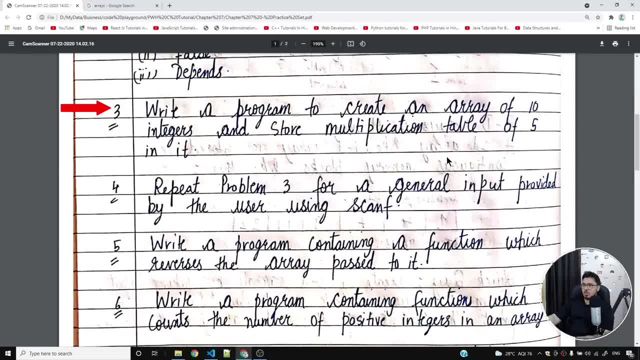 and not to the third element. so this is, and not to the third element. so this is false okay, false okay, false, okay. write a program to create an array of 10. write a program to create an array of 10. write a program to create an array of 10 integers. 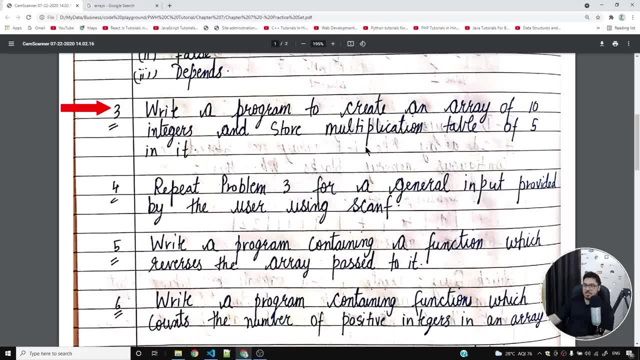 integers, integers, and store multiplication table of five. and store multiplication table of five. and store multiplication table of five in it. so you have to create an array of in it. so you have to create an array of 10 integers, 10 integers, 10 integers, and then you have to store multiplication. 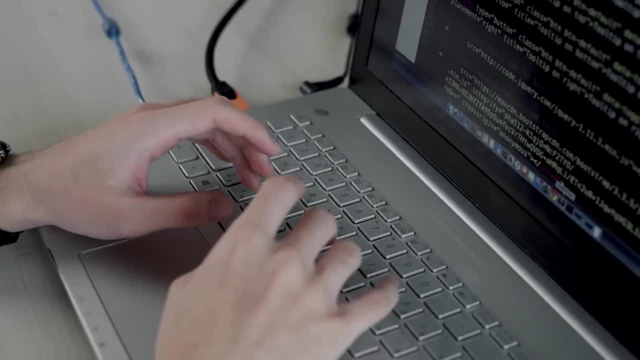 and then you have to store multiplication, and then you have to store multiplication- table of five in it, table of five in it, table of five in it. so this is a very simple problem once again. so this is a very simple problem once again. so this is a very simple problem once again. all you have to do is create an array. 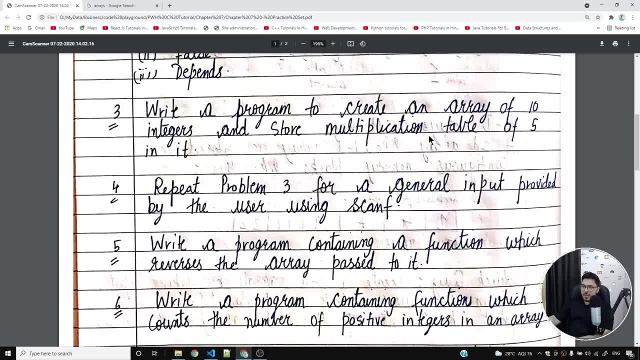 all you have to do is create an array. all you have to do is create an array of 10 integers, and then all you need to do of 10 integers, and then all you need to do of 10 integers, and then all you need to do is populate that array using a for loop. 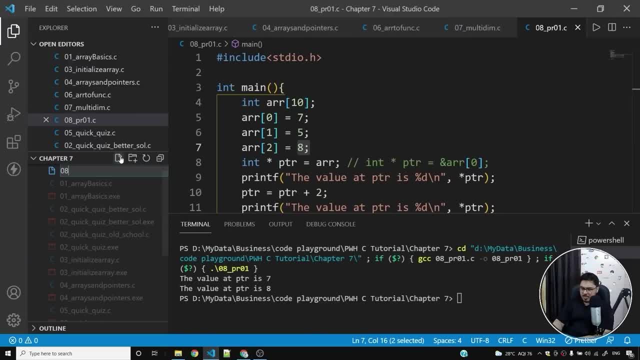 is: populate that array using a for loop is: populate that array using a for loop. let's see how this can be done. so let's see how this can be done. so let's see how this can be done. so i'll say 09, underscore pr02.c. 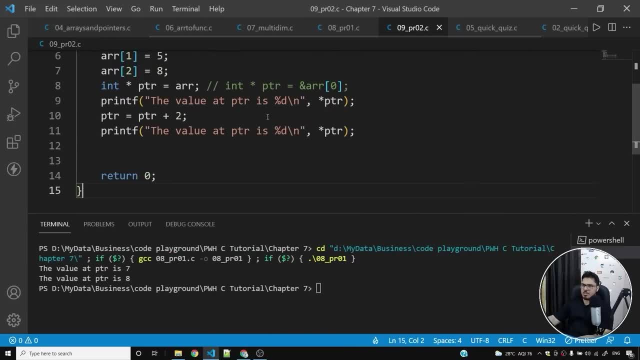 i'll say 09 underscore pr02.c. i'll say 09 underscore pr02.c, and what i will do is i'll copy paste. and what i will do is i'll copy paste. and what i will do is i'll copy paste the program that i've already written. 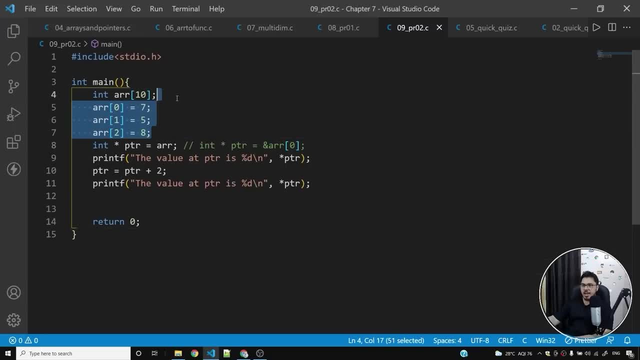 the program that i've already written, the program that i've already written. why did i do that? i did that. because why did i do that? i did that? because why did i do that? i did that? because already i've created an array of. already i've created an array of. 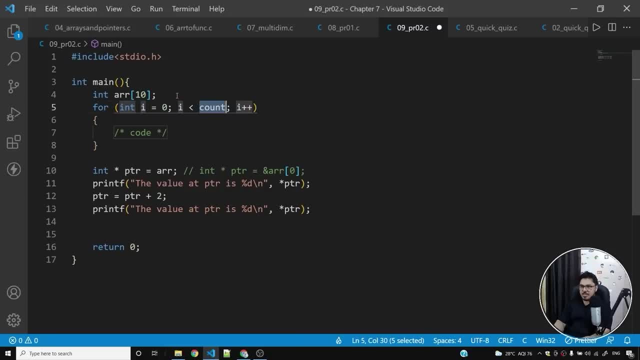 already i've created an array of 10 integers. now i'll use the for loop and 10 integers. now i'll use the for loop and 10 integers. now i'll use the for loop and i'll simply say: int i is equal to 10. 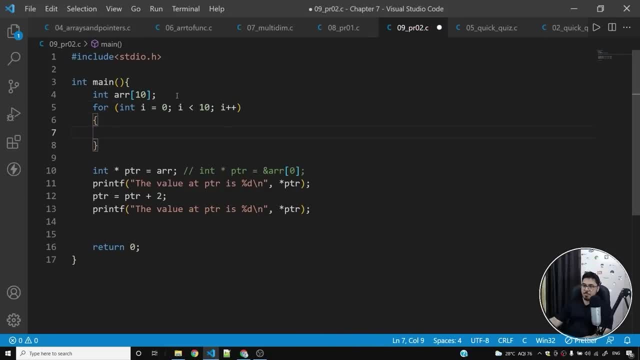 i'll simply say: int. i is equal to 10. i'll simply say int. i is equal to 10. sorry, i is equal to 0, i is less than 10. sorry, i is equal to 0, i is less than 10. sorry, i is equal to 0, i is less than 10. and uh, in place of this code, what i'll? 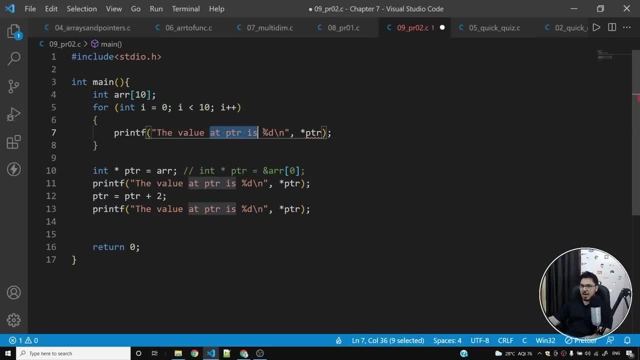 and uh in place of this code. what i'll and uh, in place of this code. what i'll do is i'll copy this printf. i'll say the do is i'll copy this printf. i'll say the do is i'll copy this printf. i'll say the value of 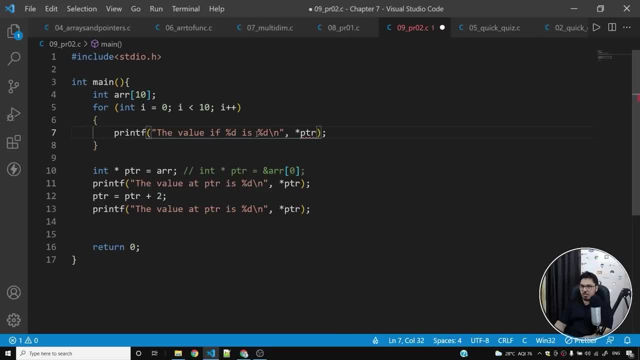 value of value of. i'll say the value of percentage d. i'll say the value of percentage d. i'll say the value of percentage d, or rather uh, or rather uh, or rather uh. five multiply by percentage d, five multiply by percentage d, five multiply by percentage d. percentage d is: 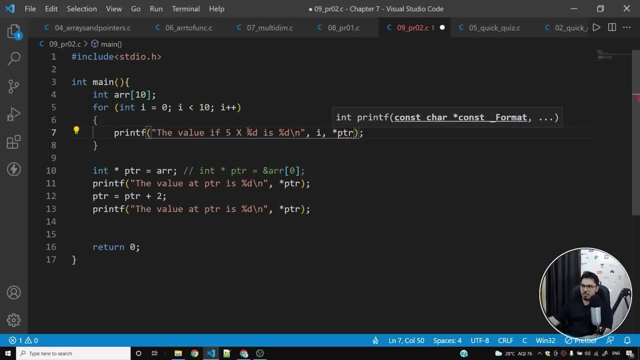 percentage d is. percentage d is. and also let me do one more thing. i'll say: i here. so, in place of this percentage d, this i will be printed, and in this place, uh, in place of this percentage d, i want a rri to be printed. so this is very simple and straightforward. so 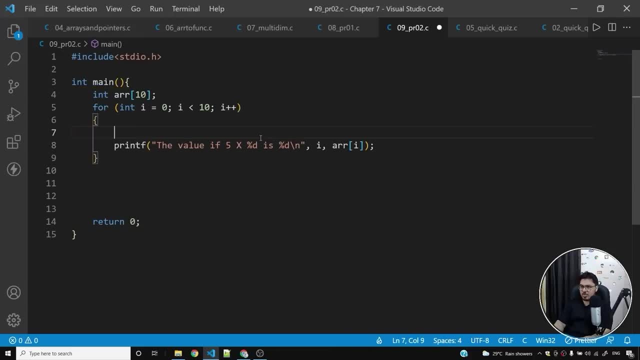 what i'm doing is, before i do this, what i'll do is, uh, i'll simply say: a rri is equal to 5 multiply by i. so what this will do is it will start printing uh values of 5 multiply by 0, all the way till 5 multiply by 9. so let me show this to you. so 5 multiply by 0 is equal to 0, 5 multiply. 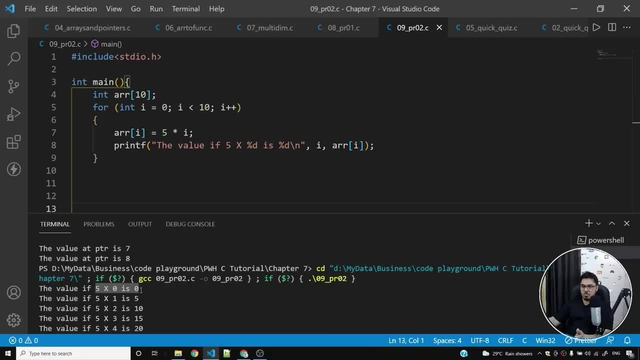 by 1 is equal to 5, so it's starting the multiplication table from 0 onwards, but i want to start my multiplication table from 1 onwards, so what i'll do is i'll replace this i with i plus 1, here as well as here. 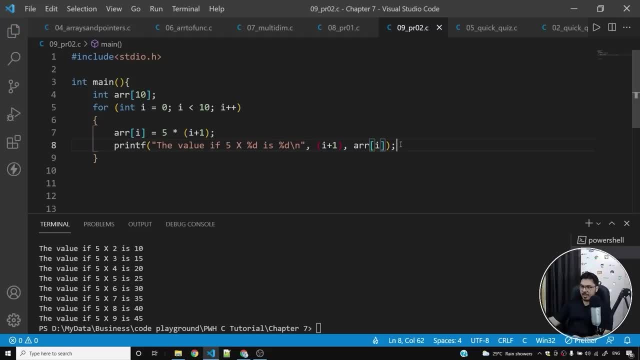 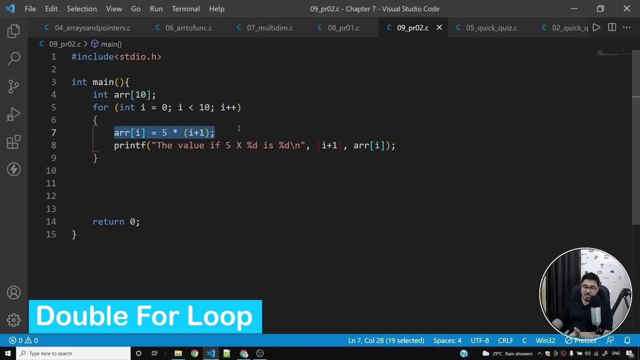 so i'll simply print i plus 1 instead of i. let's run this and you will find out that multiplication table of 5 has been printed. you might also want to use double for loop, but again, why would you do that? you can simply assign the value to the array as well as you can print the. 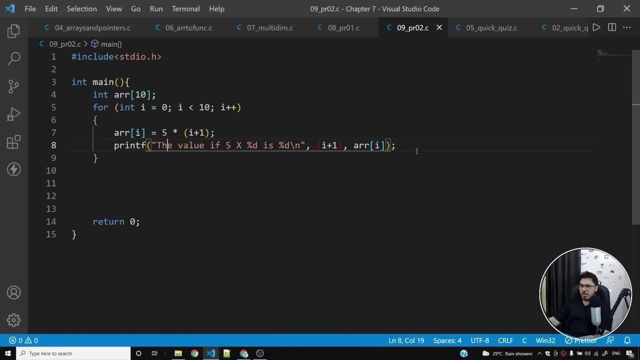 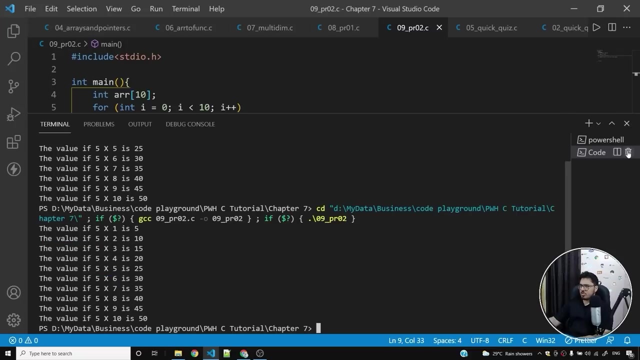 value inside the same for loop. if you want another for loop, you can do that as well. that also works. so all you will have to do is you will first initialize the entire array and then you will print. so that will also, you know, do the same thing. so, either way, it works. so i hope you were able to. 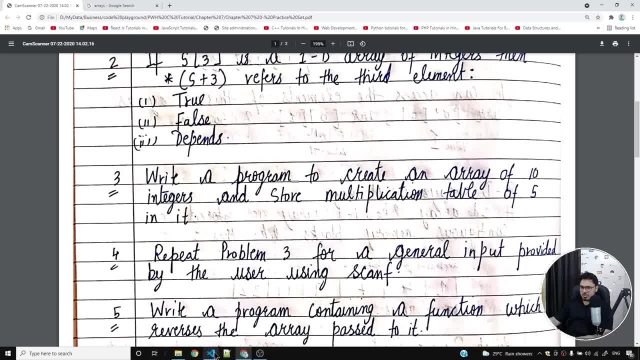 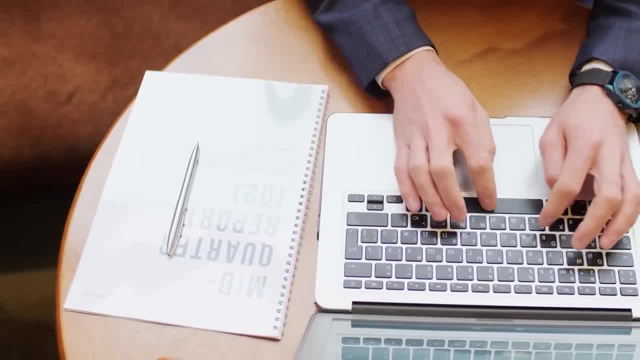 solve this problem and you understood this problem pretty clearly. this was problem number three. so i i would like to rename this program to pr03 because i want you to have all these codes for reference. i'll give you the notes, i'll zip all these source codes, notes and everything and i'll give it to you. 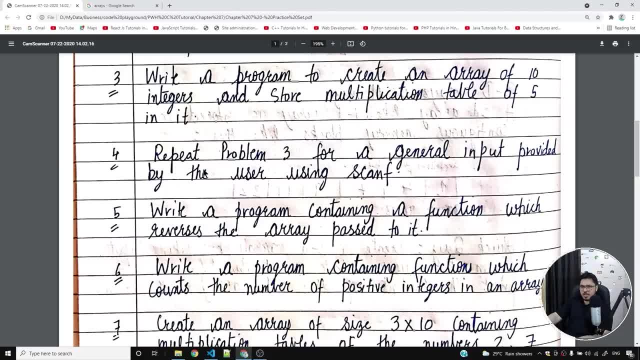 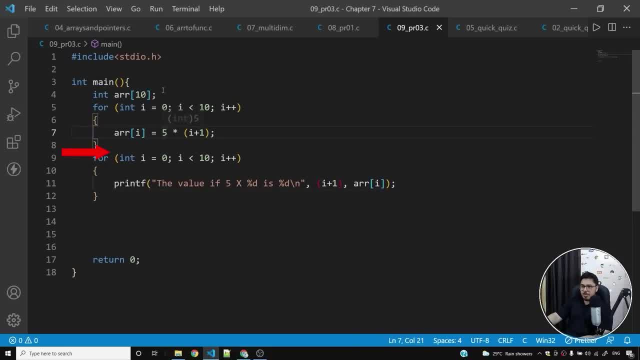 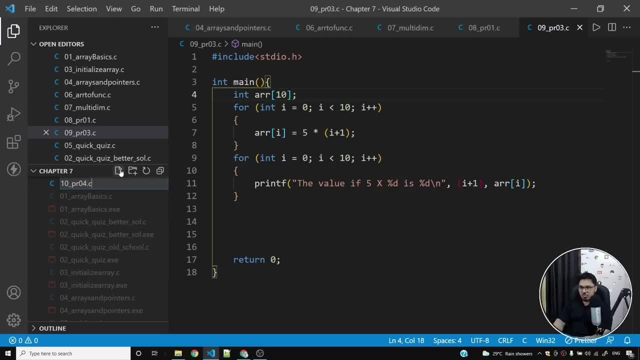 in the description. so, um, coming back to the practice set, repeat problem three for a journal input provided by the user using scanf. all you have to do is, instead of writing this five, you'll replace it with n. so let me solve this problem for you. this is very simple problem, so i'll say: is 10 underscore pr04.c. 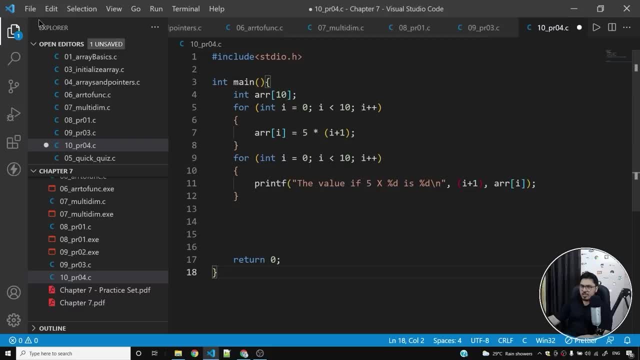 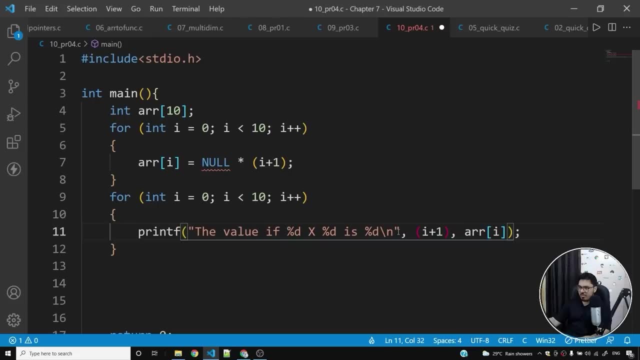 and what i'll do is i'll copy this code and, instead of writing five, i'll replace this five with n, and uh, you know, i'll have to use another percentage d when i'm printing n, and i'll do that. i'll do that and not null. i want to use n, so n is a very 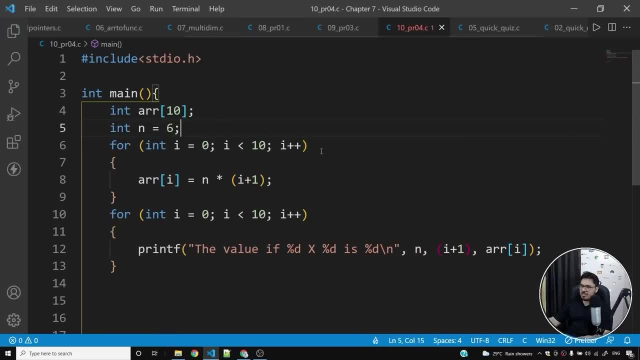 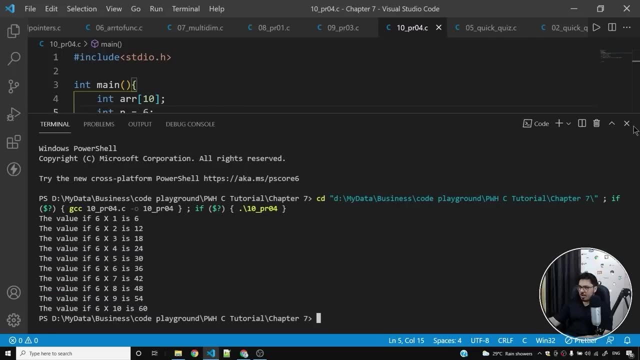 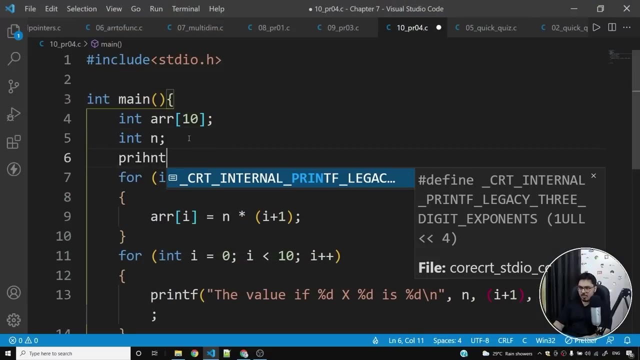 simple variable which will be, say, six, and let's see if we get the multiplication table of six. so if i run this program, oh yes, i'm getting the multiplication table of six. so this program works. it was pretty simple and straightforward. but the question asks for using a user defined. 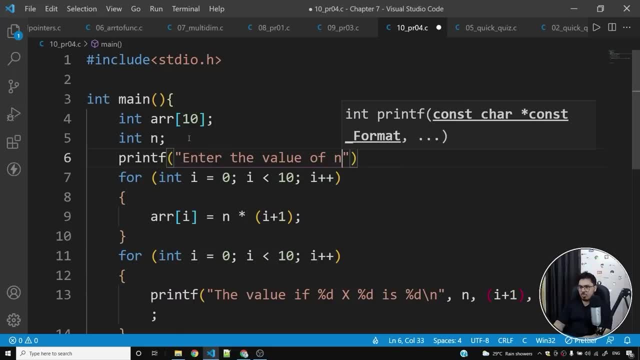 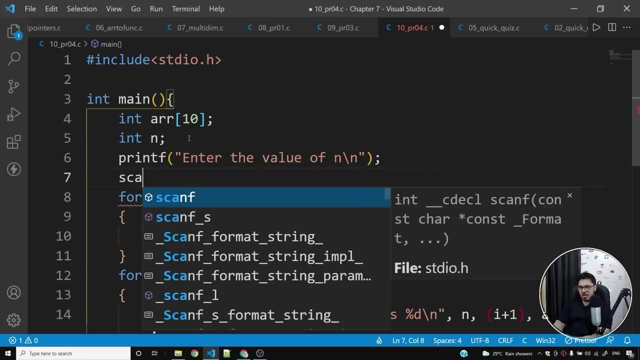 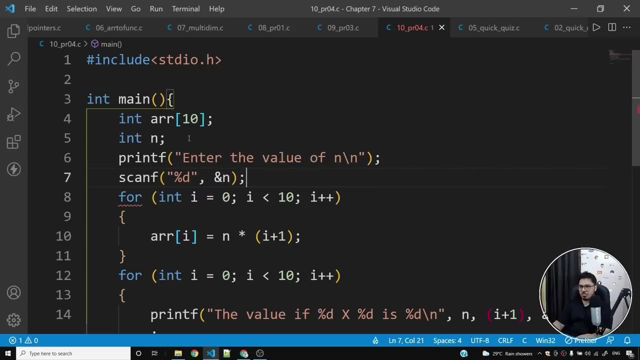 value. so i'll say: enter the value of n and i'll simply use backslash n and you can see i've gotten delivery of seven and we've got susceptibility. so we'll know what it's like. after taking threeyou can see if the interval is large. so if the interval is larger, 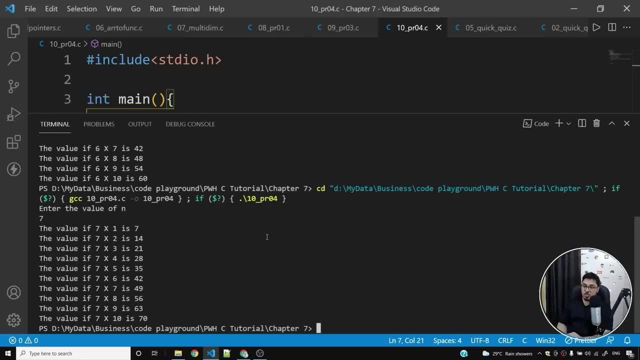 because the file has short record, or for smaller parts. you can also use double occupy. since you know special, we are道ing after the parameter. so if you want 미국 and you can even say you want something color, our code should be pick that nobody ever thinks about it. 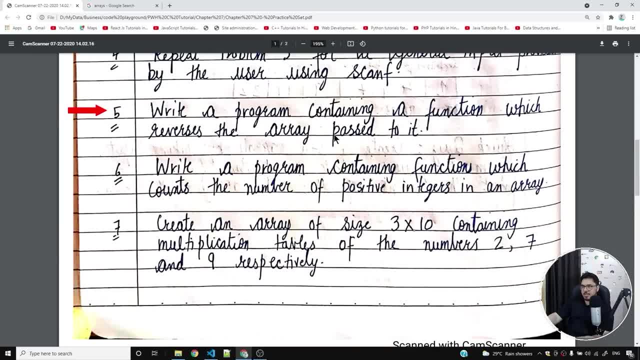 plus another parameter which for you, it's going toл be one of them. so just be careful. and if you don't use one of them and you feel like you can't write the percentile, so if you don't know what it is, just stay in that field for 10 or any type of question. 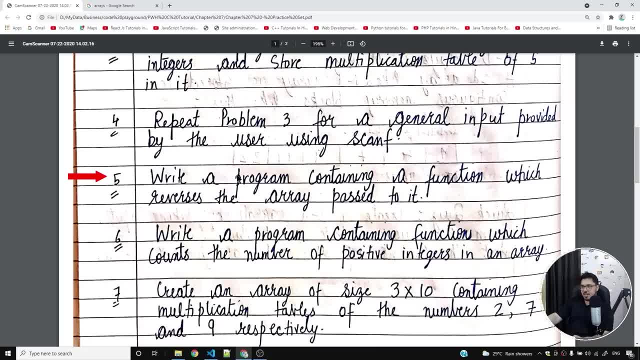 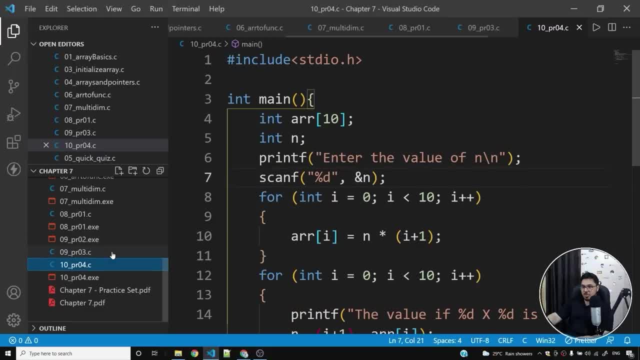 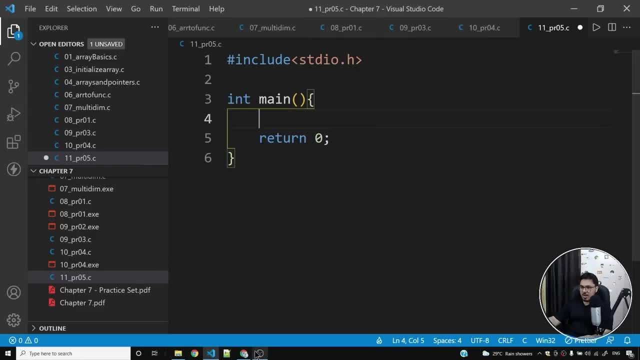 passed to it. so all you have to do is you have to reverse an array. so this is a very interesting problem. this is very interesting problem, so look at this problem very carefully. i'll solve this problem for you. so let me create another program: pr05.c. boilerplate code and problem number five. 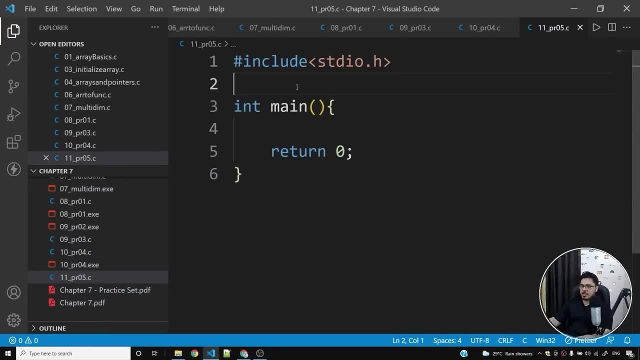 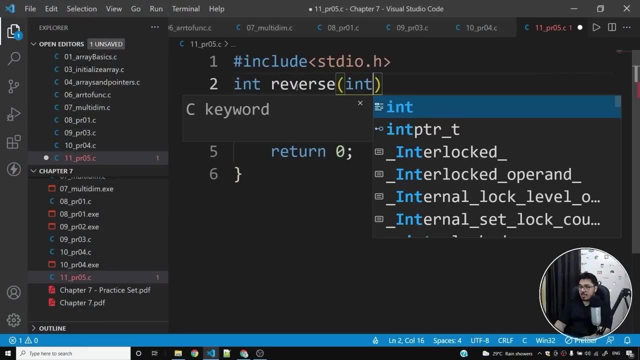 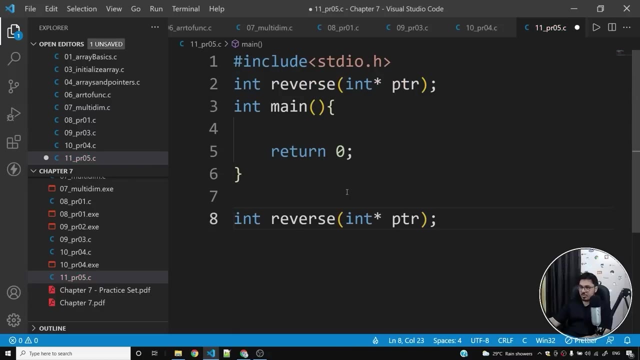 yes, so we have to reverse an array. so what i'll do is i'll say int, and- and this is a very famous interview question as well, look at this really very carefully, guys. so let me copy this and also let me write the function body. or let me tell you one more thing that you can directly write: the. 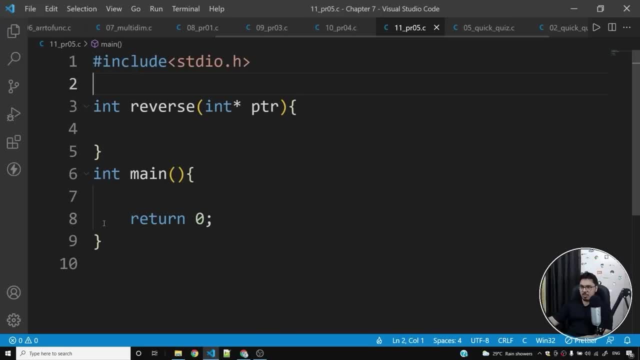 function, body, skipping the prototype. that also works okay. so i'll do that. if i say int reverse and star ptr, i'm taking the first elements address into ptr and then i can operate on the array. so what i'll do is i'll say int, ar is equal to let me have a one, two, three, four, five, six, seven, eight, nine and ten. let me have an array. 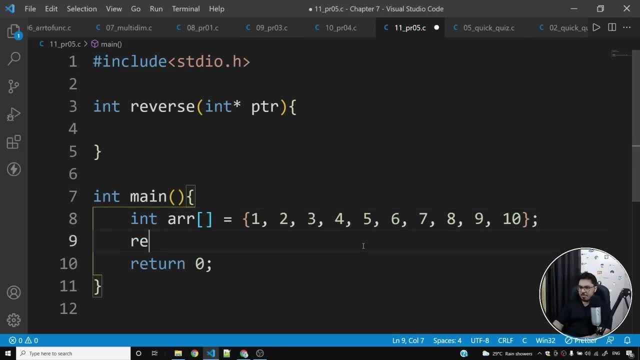 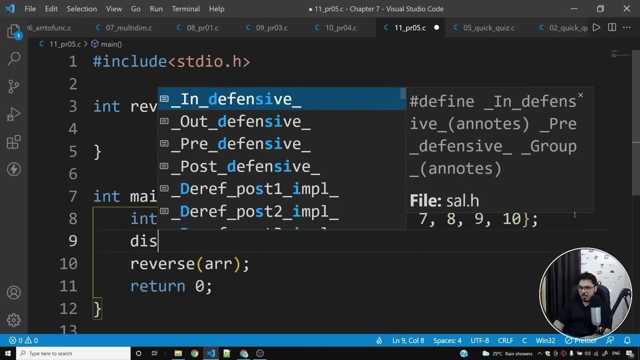 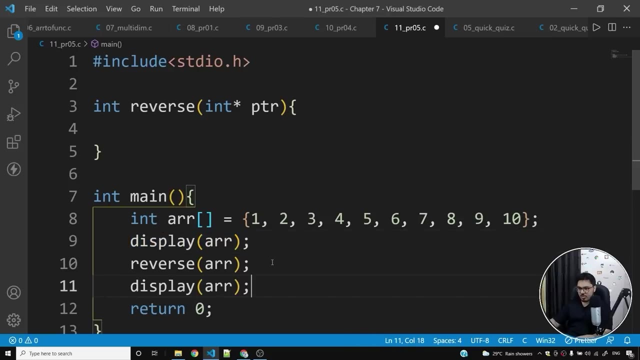 of one all the way till ten and let me reverse this array. but before i reverse this array, i also want to print this array, so i'll simply display this array and display something that i will write. it's a function. i'll write this function, so i'll say: 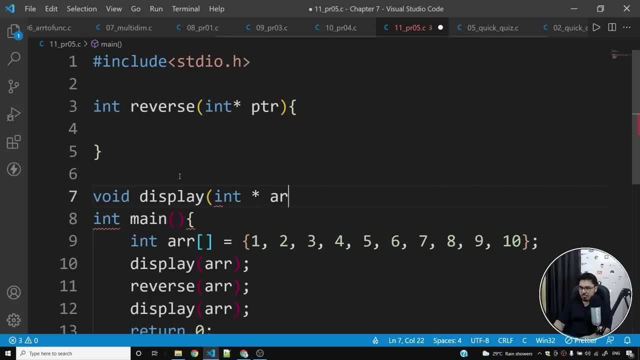 void display in star error, or let me call it ptr. because we have been calling it ptr, i'll use a for loop. i'll say int. i is equal to zero, i is less than i also need the size of this array, which is n. so i'll simply say int n, i'll say printf and then i'll say percentage d. 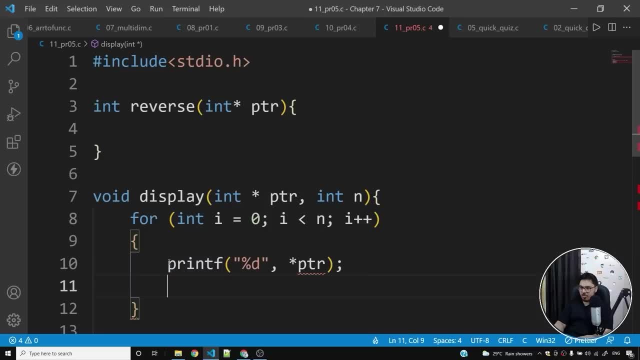 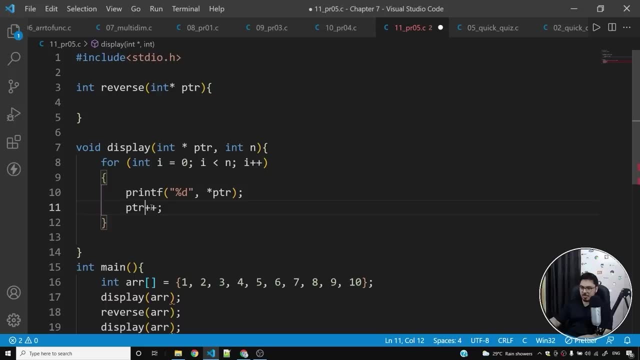 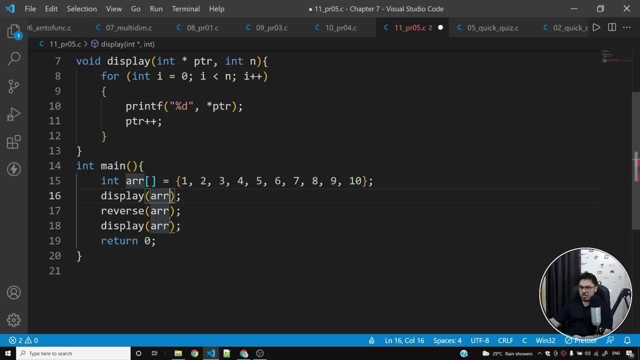 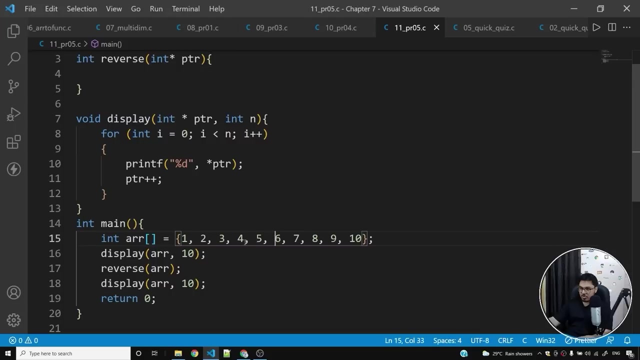 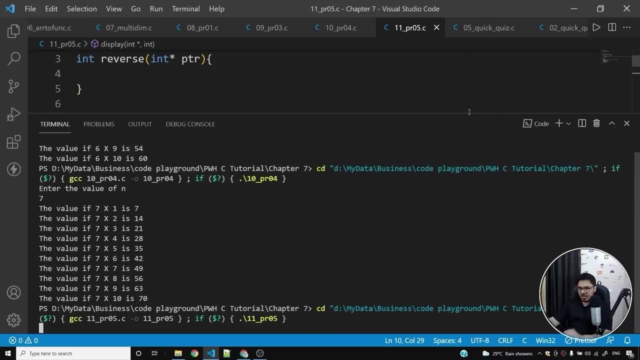 and i'll dereference ptr. and then what i'll do is i'll say ptr plus plus, that's it. so i'll dereference ptr initially, then i'll say ptr plus plus, which will increment ptr, and i'll get all the elements from this array. so let's see if this function works. so all i need to do is pass ten to it, because there are ten elements. let's see if this function works. but reverse does nothing so far. so you should get one, two, three, four, five, six, seven, eight, nine, and also add a space here so that we have space between the elements of our array and also before the ptr is. 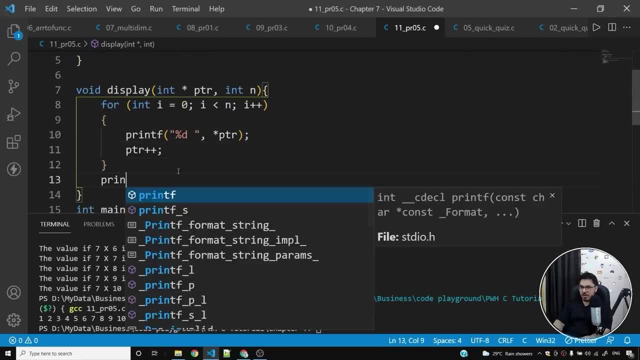 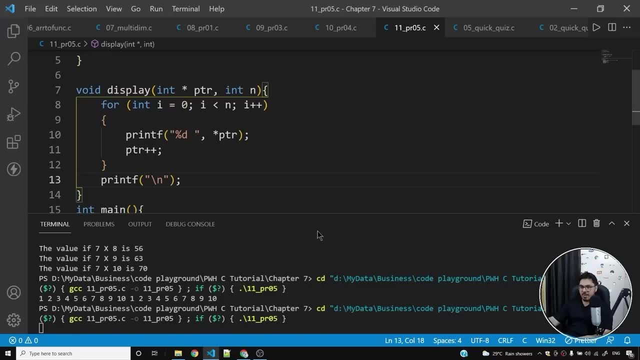 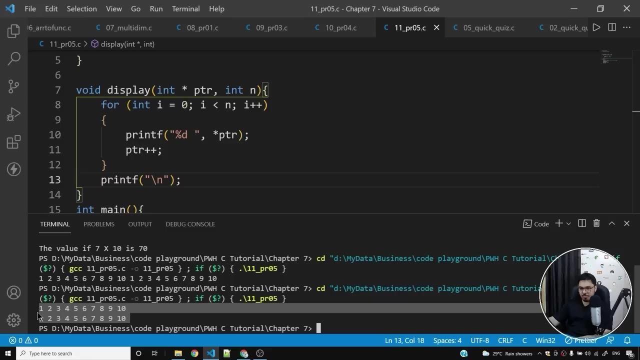 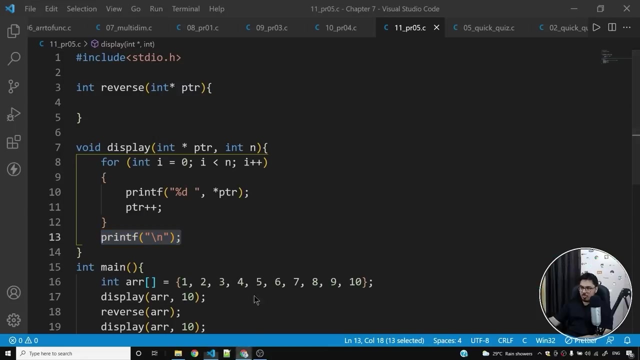 the function returns, i'll print a new line, because if we are printing something else after displaying the array, that should also get reflected. so you'll not see one, two, three, four, five, six, seven, eight, nine, ten and the same thing once again. you will see it in a new line this time. so that's why i have added this new line here. so one, two, ten. one, two, ten, because reverse does nothing. now listen to me very carefully. let me take an image. i'll use this image to explain you. 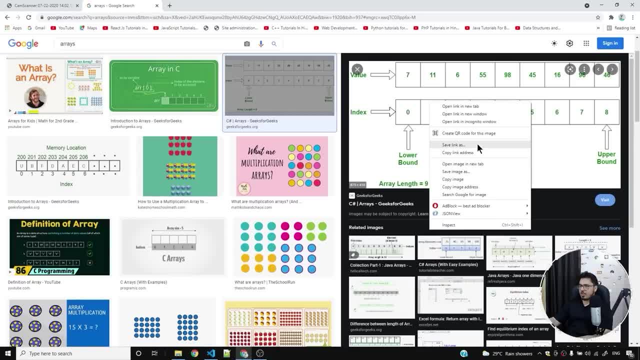 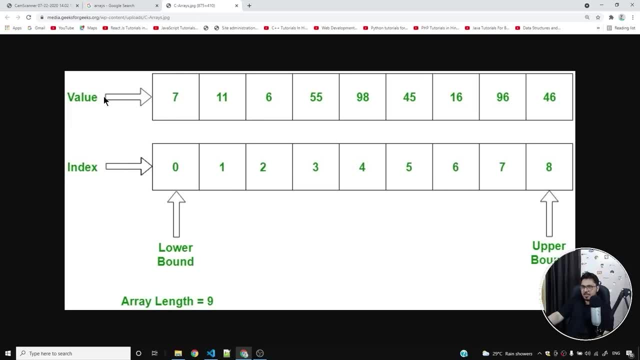 let me take some other image. okay, so this image even looks better. so let us say we have zero, one, two, three, four, five, six, seven, eight as the indices, and these are the values. okay, so we have an array of size nine, not eight. note that the size of this array is nine if you count the number of elements. they are nine because we are starting from zero, not from one. okay, now what will happen is, if i want to reverse this array, what i'll do is i'll replace seven with 46, i'll replace 11 with 96. 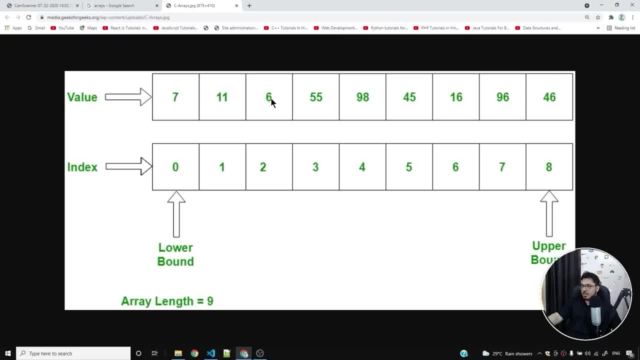 i'll replace 6 with, i'll replace 6 with 16, i'll replace 55 with 45 and at 98 i'll stop. now i'll not stop. i'll not go all the way till 46. i mean i'll not go all the way from this index to this index and keep swapping, because the moment i reach the midpoint, if i swap 7 by 46, 11 by 96, 6 by 16, 55 by 45, 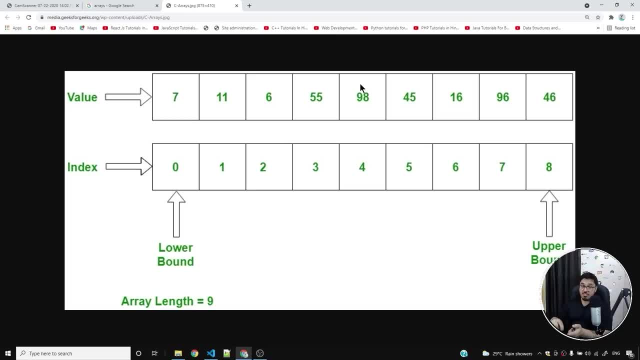 i will have to stop here if i want to reverse the array, because if i go even further, what will happen is i'll end up reversing the array two times. i don't want that. okay, if i reverse this array, if i start from index zero and go all the way till four, what will happen is i'll reverse the array the moment i reach four. but if i go beyond four, what will happen is i will 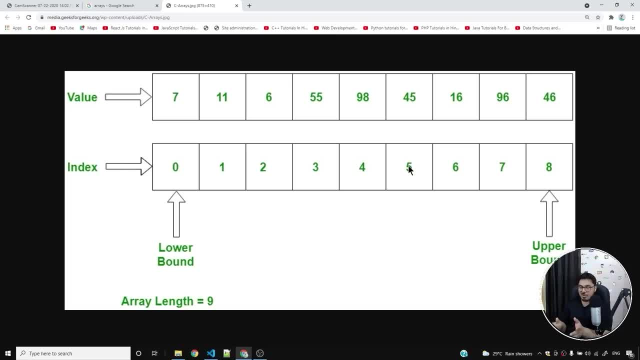 reverse the array once again, and what will happen is the array will not change. so let me code this for you. so how do we this? How do we code this? So this was the case when the number of elements in the array were odd. What if the number of items in the array is even? So, if we have eight elements, the index will go. 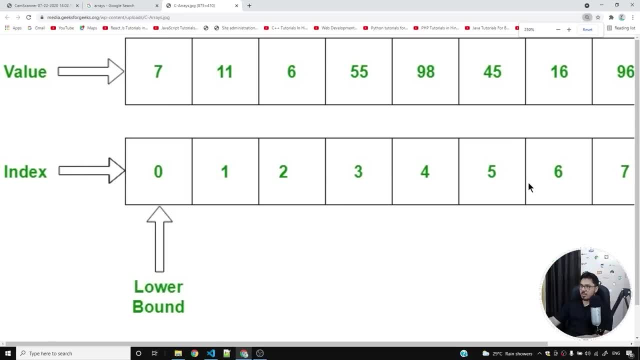 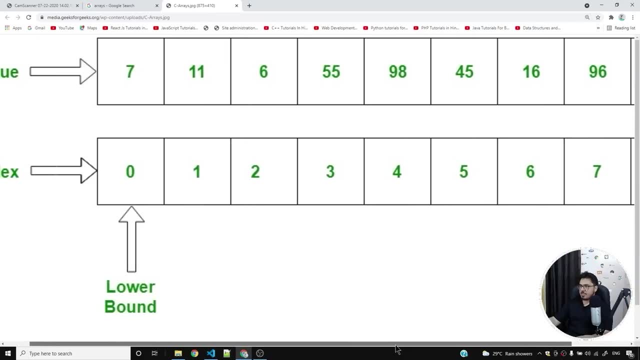 from zero to seven. let's assume that this 46 and eight is not there. Let's assume that we have this is this is all we have. let's assume this is all we have. let us say this array starts at index zero and ends at index seven. Let us assume this is the array. Now, if I want to swap the first, 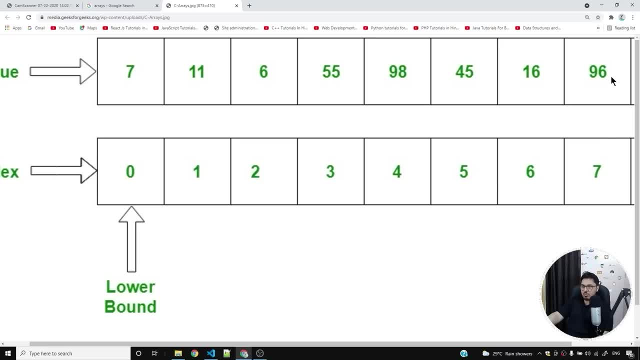 element with 96,. I will do that. I can swap. I'll swap 11 with 16,, I can swap six with 45, and I can swap 55 with 98. So I can keep swapping till the size of the array, which is eight divided. 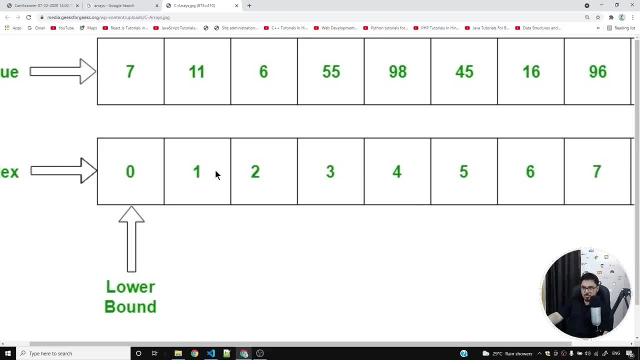 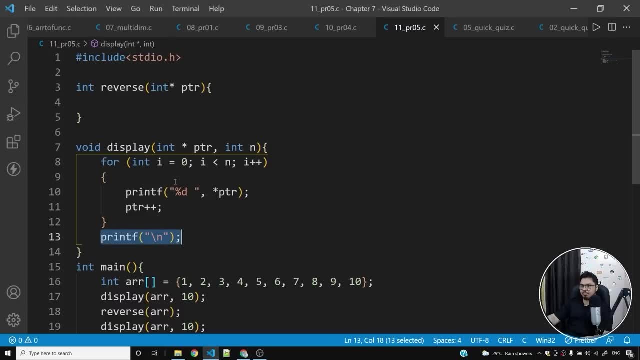 by two minus one, Starting from zero. I'll go till this index and I can keep swapping. Let me show you this in code. So what I'll do is I'll use the same array and let me use the same array, or, or. 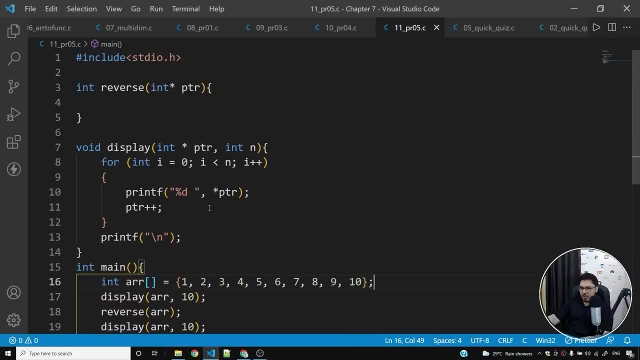 let me not use the same array. I'll use this array. What I will do is I have this PTR. What I'll do is I'll swap this element, which is index zero, with index n minus one. So I'm swapping zero with n minus one. Okay, so let me write this here. Let me. 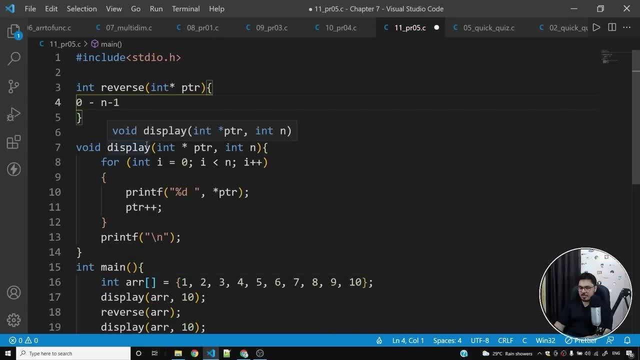 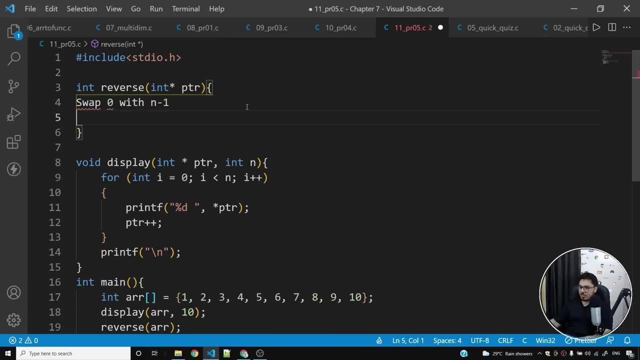 cut this from here. Let me write this here. I'll say: swap zero with n minus one And swap one with what? one with n minus two, And swap index two with n minus three, And so on. keep on doing till n by two. So you keep on doing till we'll find out till n by two. Okay, let's, let's. 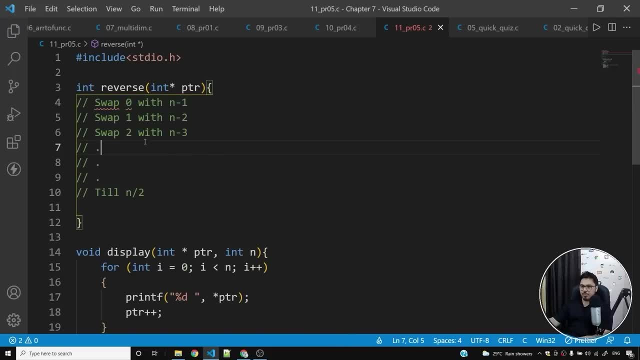 settle n by two. we are just assuming we might change this. So swap zero with n minus one, one with n minus two, two with n minus three. I can write a general swapping equation. you can call it I with n minus I minus one, or plus one. tell me minus one. Okay, so I can say n minus I minus one. 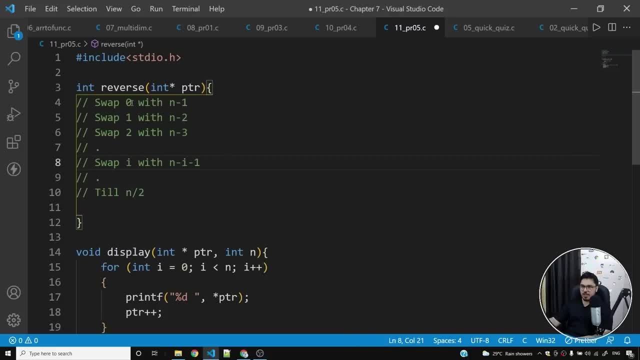 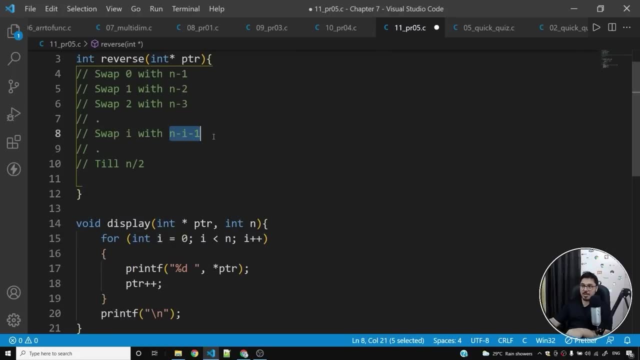 So if the value of i is two, it will be n minus three. the value of i is zero, it will be n minus one. So I'll swap I, the element at, and index i with element at index n minus i minus 1. let's do that. let's do that. so what i'll do is: 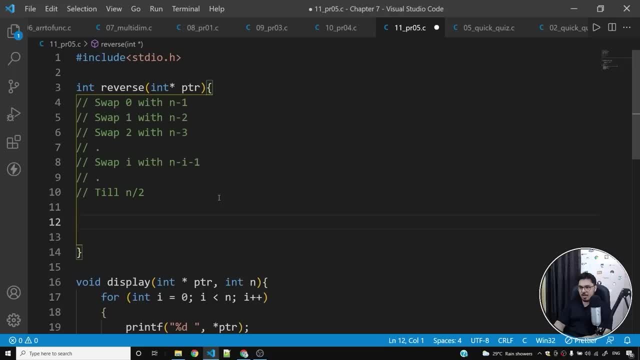 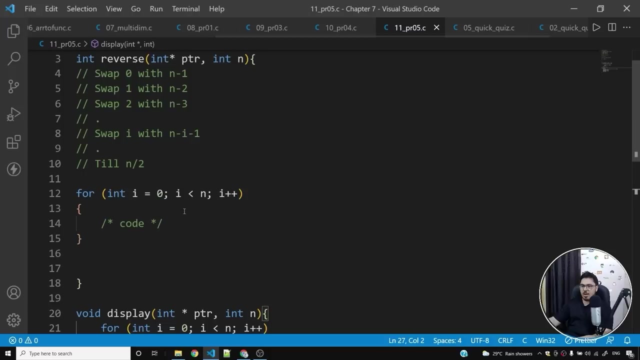 i'll write the swapping logic. i've already told you about the swapping logic, but before that, let me write the for loop. i'll say: i is equal to 0, i is less than n. let me also pass the size of the array, which is n, which is 10 in this case, and what i'll do is: i'll simply swap um. i'll do this inside. 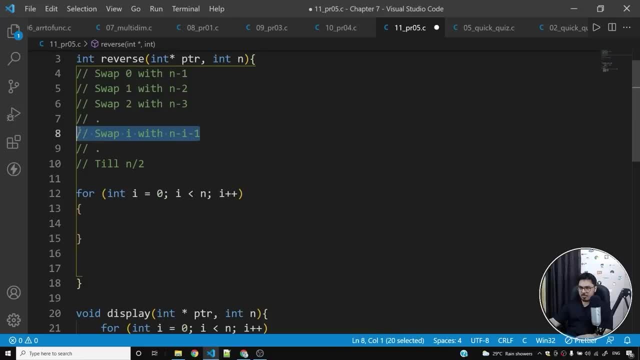 the for loop. so i'll say: swap i with n minus i minus 1. so what i'll do is i'll say: let me also create a variable called temp. i'll use this variable for swapping. i'll say: temp is equal to ptri. okay, i'll say: temp is equal to ptri. and also: let me do this instead of you know. 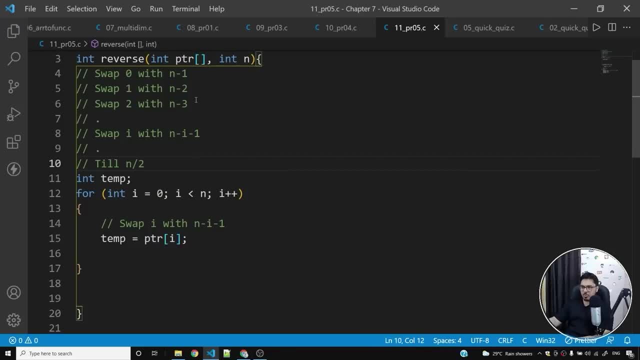 using the ptr as a pointer. what i'll do is i'll use arr, let me use ptri, or let me use a itself. if not arr, i'll say: temp is equal to ai. ai is equal to a n minus i minus 1, and a n minus i minus 1 is equal to what it will be equal to temp. 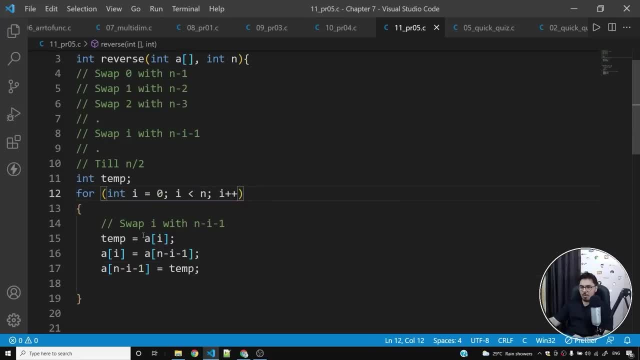 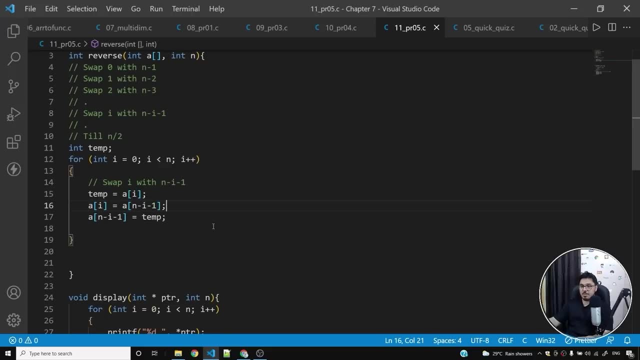 so this way, what will happen is i'll swap ai with a n minus i minus 1. i've already told you about swapping logic, so i've already discussed this in previous chapters, so i'll not discuss this again. so this will simply swap ai with a n minus i minus 1, and that's it. that should swap the array. 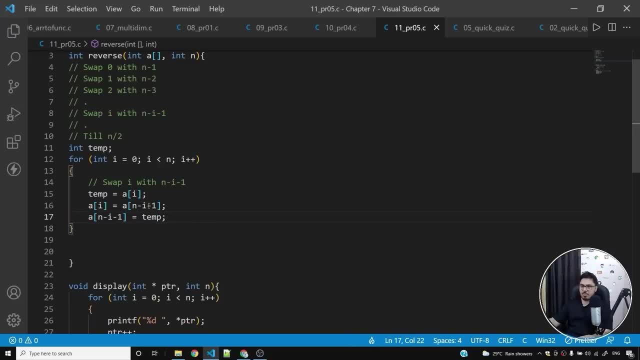 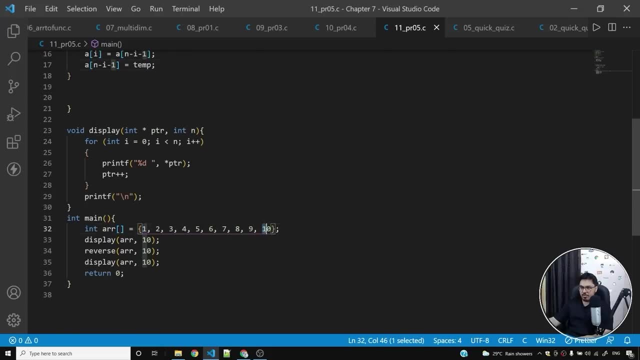 so let's see if we are able to swap this entire array. so let's start from. you know 1 and we are going all the way till 10. so if i run this program, what will happen is you will see that the array is not swapped, and the reason is that we started from 0 and we went all the way till. 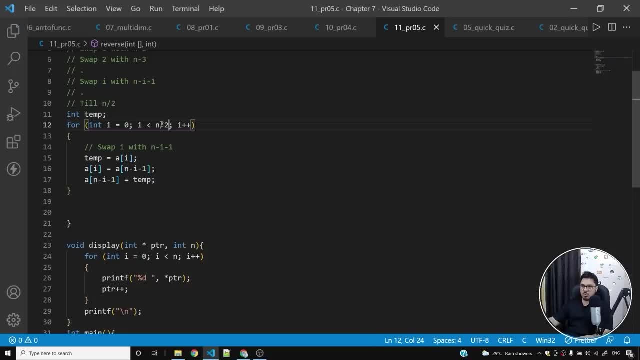 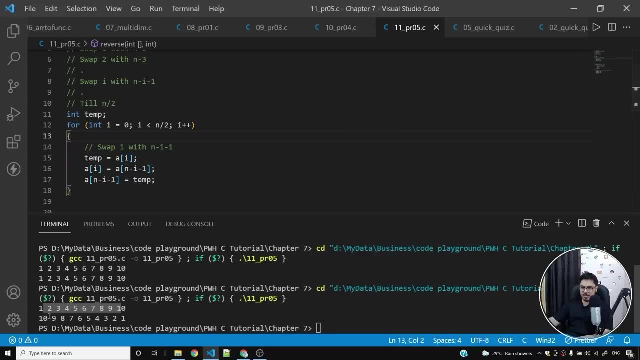 n. but what we want to do is we want to go from 0 to n by 2 minus 1. so i'll simply say i less than n by 2. um i'll run this program and you can see the array has been reversed. how does this program? 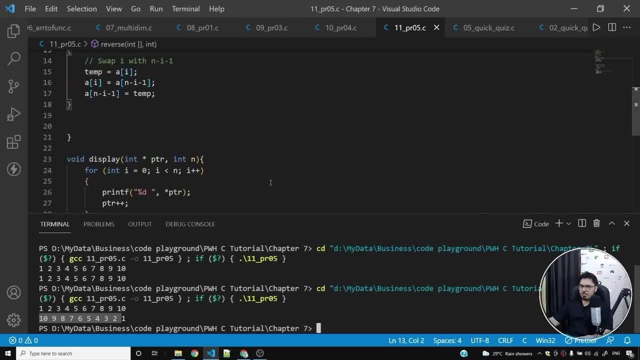 work. let me explain you. so if the number of- uh okay, let's check, does this program work? if the number of elements in the array is even, so, if we have- um sorry, if the number of elements in the array is odd, so we have nine elements here, let's see if this works. also, i'll say nine here. 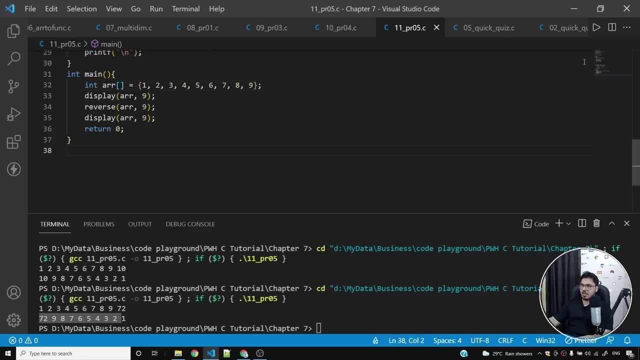 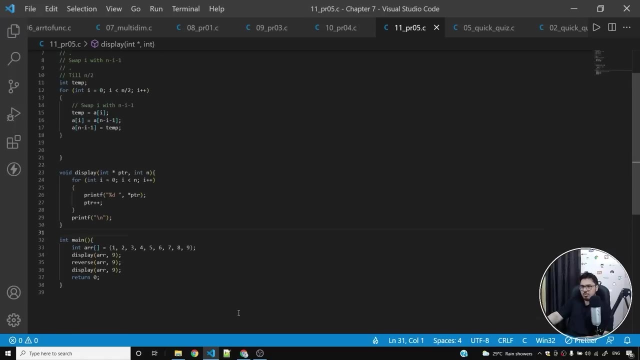 not ten. so let me also say nine and let me run this. so yeah, it works. it works for, uh, odd elements, odd number of elements as well. it works for even number of elements. we have already seen that it works for odd number of elements as well. so let's now try to understand how this works, how. 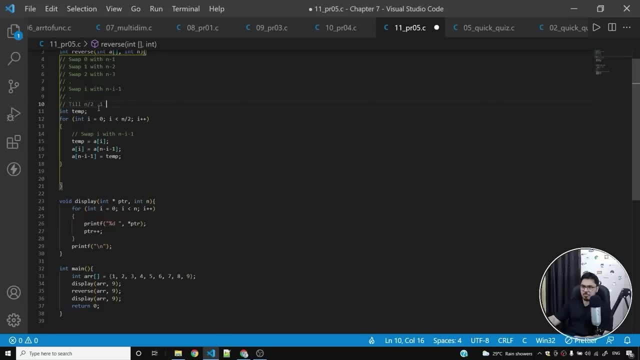 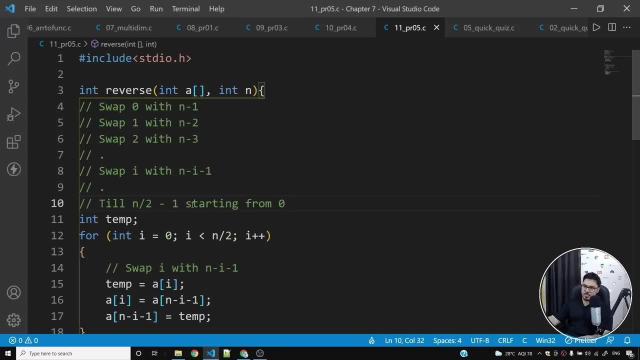 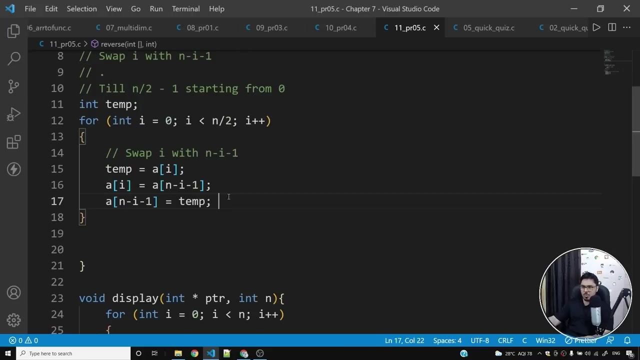 going from n by 2 minus 1. let me make it minus 1 because we are starting from 0 and we are going um starting from 0. so we'll say: i'm going till n by 2 minus 1, starting from 0. so i started from 0. i'll go till n by 2 minus 1. so this is how it. 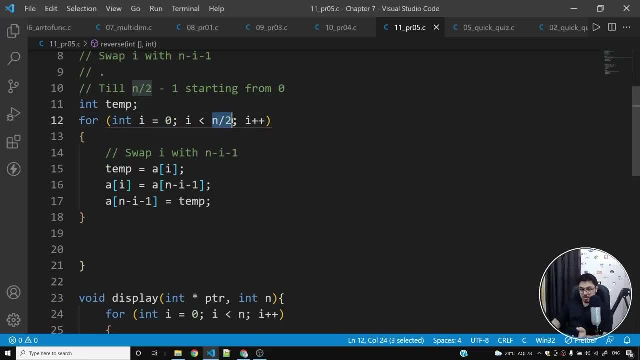 works. now, n by 2 for odd numbers will not be a floating point number, let me tell you so. if you have 9, 9 divided by 2 will not be 4.5, it will be 4, because uh, operation between an integer and. 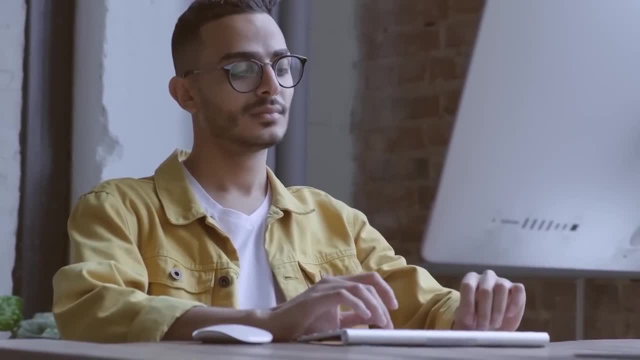 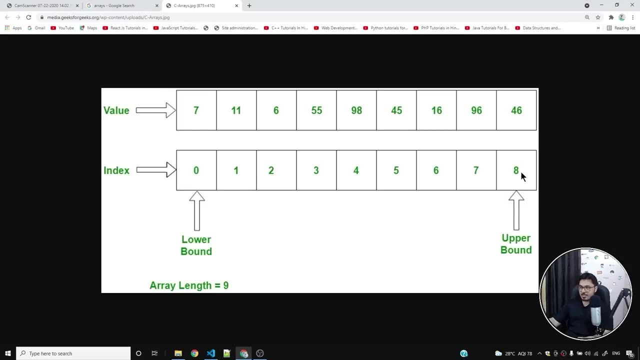 integer will result into an integer in c language. this is something that you need to understand. so, coming back to this figure, uh, the number of elements in this array is 9. okay, so the value of n is 9. so if i say 9 by 2, it will be 4, not 4.5. so what will happen is: 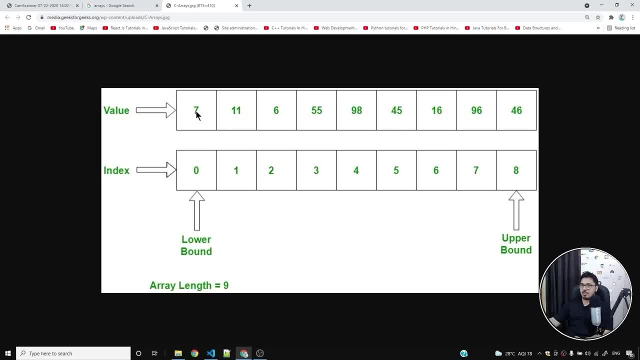 i'll start from here. i'll say, uh, 0, 1, 2, 3, 4. i'll start from 0 and i'll go all the way till 3. if i say, uh, i is less than 4, it will go from 0 to 3. okay, so if i go from 7 to 55, this: 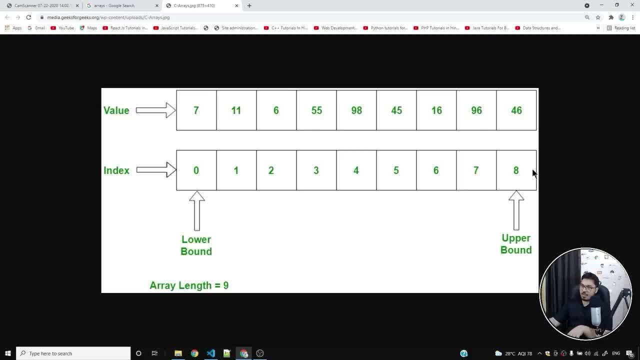 is the midpoint- i can swap the entire array. if, if there is an extra element in the array- or let us say, if there is, uh, if there are only eight elements in the array- what will happen is index will be from 0 to 7, and in that case, what will happen is that i can start. 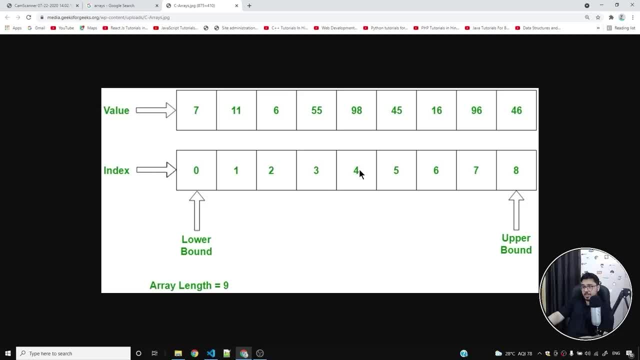 from um. i can start from 0 and go all the way till 3 once again, and i'll be able to swap the you can see. so 0 will be swapped with 7. 1 will be swapped with 6. 2 will be swapped with 5. 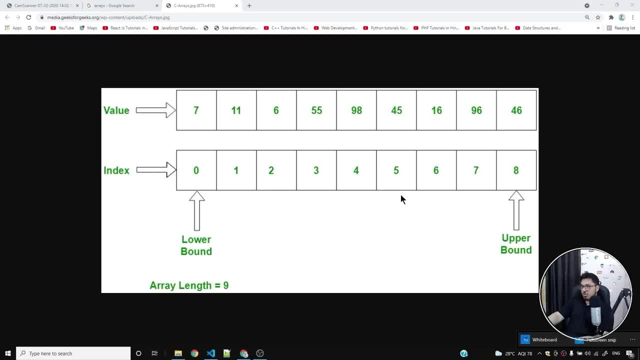 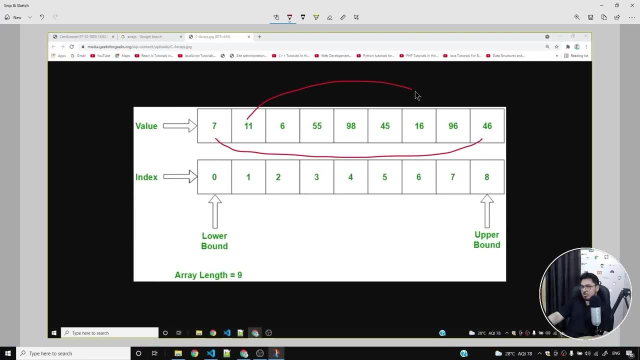 let me draw, let me you know, do a full screen, step and show you what will happen is: 7 will be swapped with what? 7 will be swapped with 46, 11 will be swapped with 96, 6 will be swapped with 16 and 55 will be swapped with 45. that's it, and then i'll have to stop here. 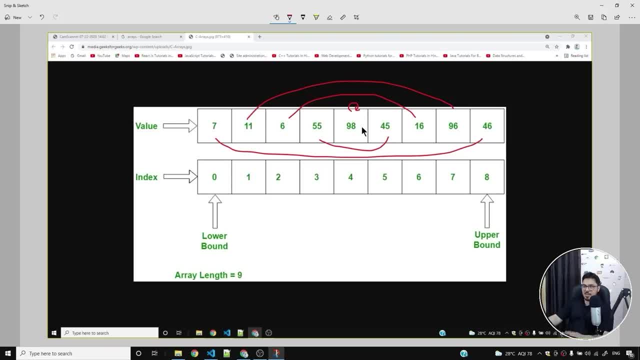 i can swap 98 with 98. that will not make any sense. i mean, you can do that, you might skip it. that will not add to add to anything, not even to the computational complexity, because this is just one element and that will not grow for larger inputs anyway. we are not talking about computation. 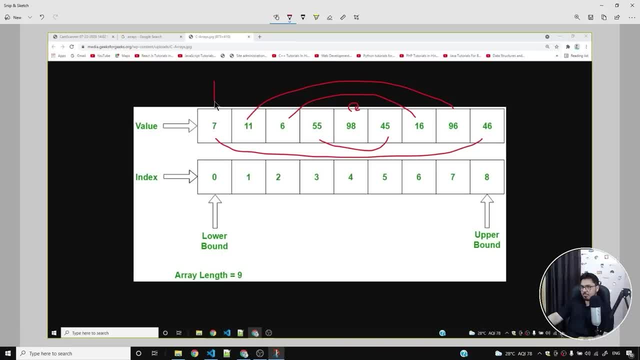 in this video. uh, so we can start from here and we can, you know, swap it till here. okay, so this was one case. now is there any way to clean the board? uh, i wish there was a way to clean the board so i can simply say, i can simply use this: let us say that this is not there. uh, let us say this is. 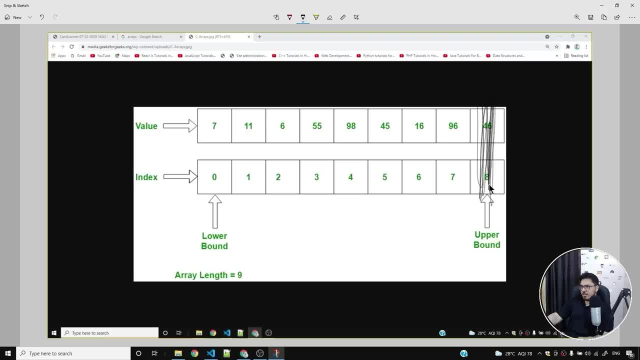 this is not there, so let's assume that these two- this last element is not there, so i'm just. i just scribbled it off. so let's say this element has, let's say, this array has, only eight elements. now, in this case, what will happen is i can swap 7, 96, 11, 16, 6, 45 and 55, 98, so all i need to do is 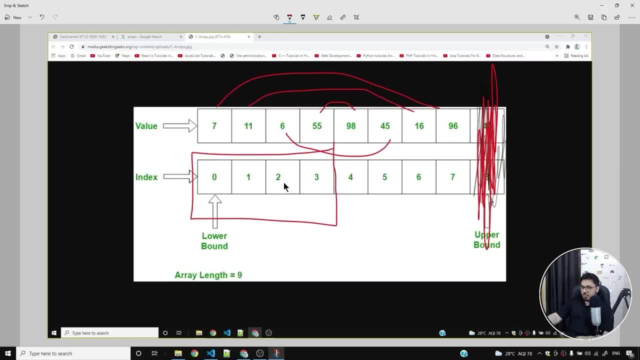 i need to start from 0 and go all the way till 3 for 8 elements as well as for 9 elements. so all i need to do is i need to go from. uh, i need to run my for loop from 0 to n by 2 minus 1, so 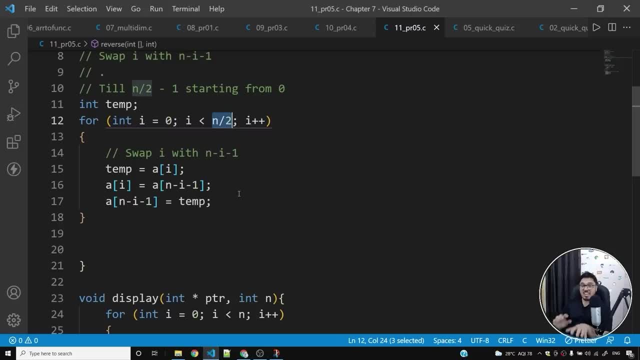 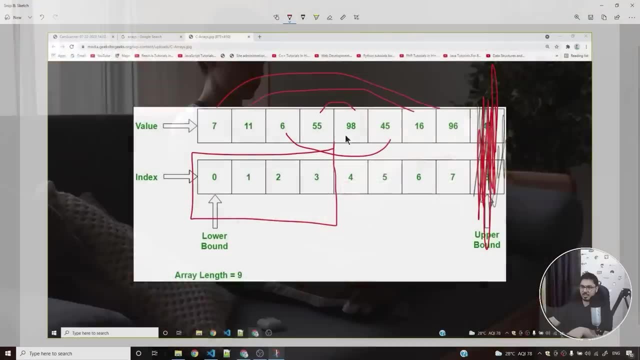 i'll simply write n by 2 here. this is something that you can, you know, get a feel of after doing some dry run. you can print the value of i. you can see how all these things are working by visualizing them, like i am doing here. but i hope that you understood and 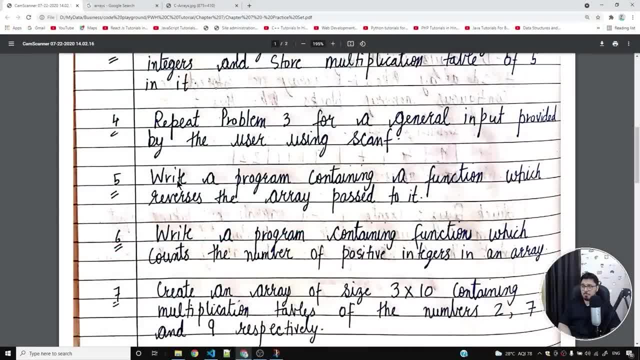 this might sound a bit intimidating if you are starting out, but this is a very common question and you will definitely encounter it. if you are working with c, if you are studying c in your college, you might get this question in your exams, believe me. moving on to the next question, which is: 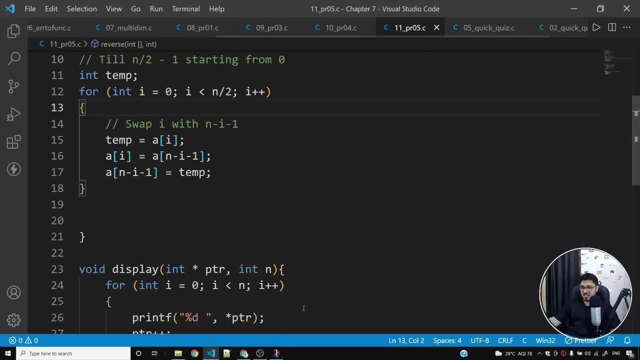 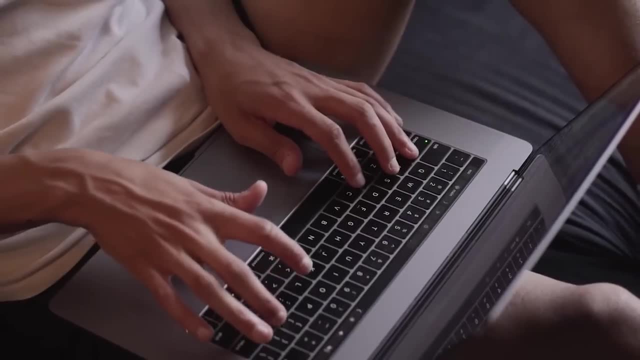 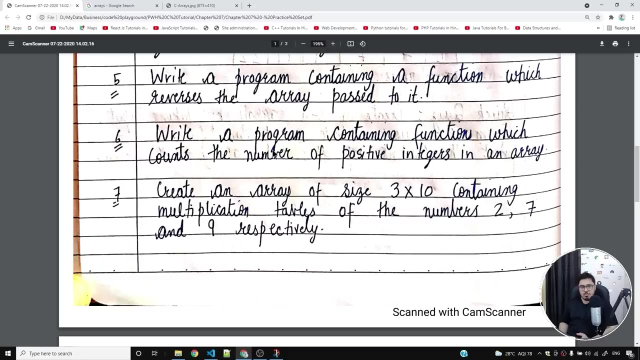 problem number six, if i'm not wrong, yes, write a program containing functions which counts the number of positive integers in an array. this is something that i want you to do. you need to write a function, you need to pass an array and you need to see whether 2 divides a number or not. so if 2 divides a number, it is even if 2 doesn't. 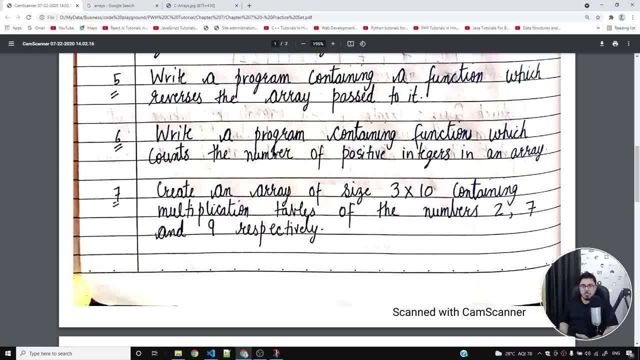 divide a number. it is odd, but we need to find number of positive integers, not positive even, or positive odd integers. so how do you find whether a number is positive or not? simply find out whether it is greater than zero or not. if it is greater than zero, 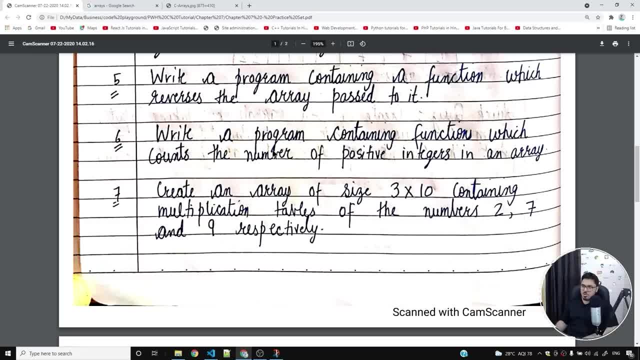 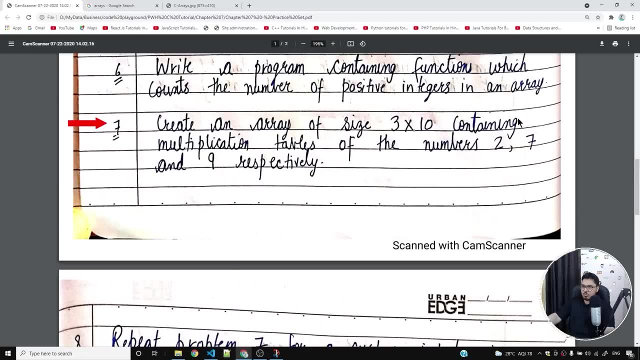 um, it is positive. if it is less than zero, it is negative. so please write your if else statements. write your function. this is very simple problem. i want you to do it yourself now. question number seven says: create an array of size three by ten containing multiplication tables of two, seven and. 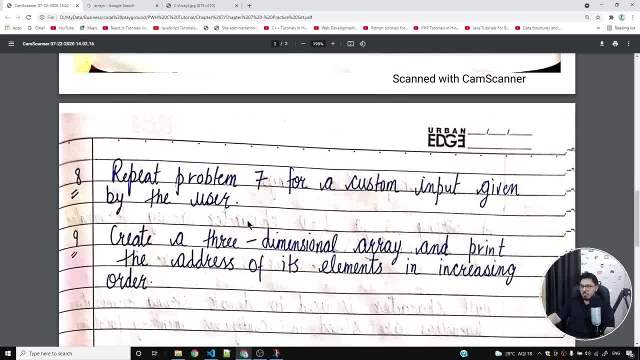 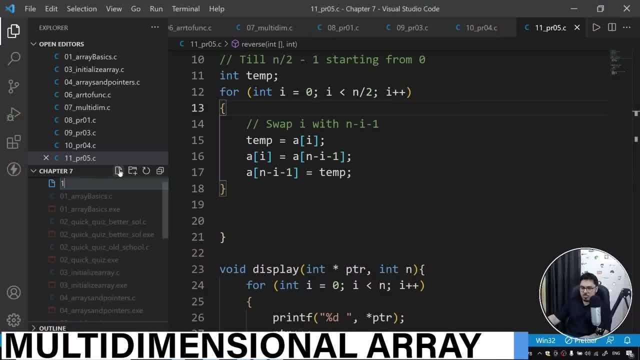 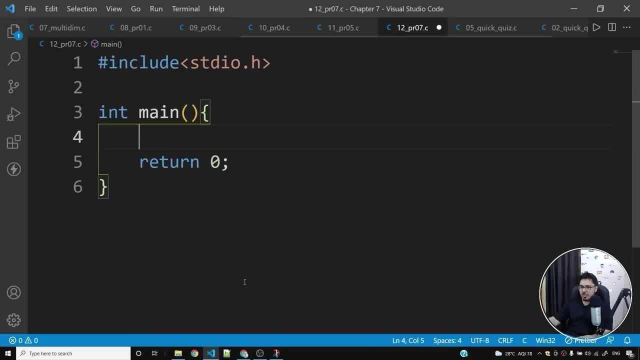 nine respectively. so this is something that i'll definitely solve for you. uh and uh, this will definitely give you some idea of multi-dimensional arrays, so let's solve this problem. so 12 underscore zero seven dot c- i'll put down the boiler plate code, and we need to store multiplication tables. 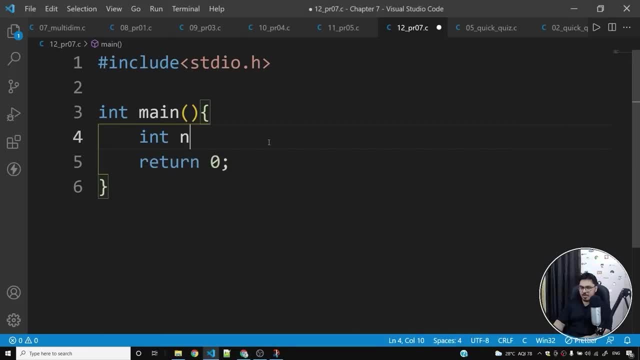 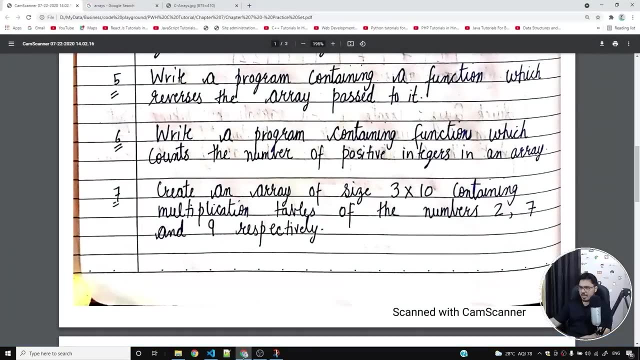 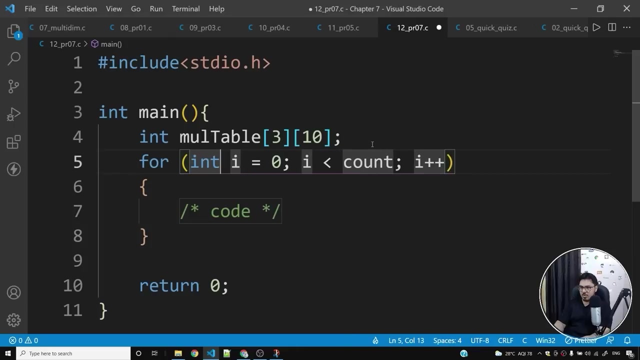 of two, seven and nine. so i'll say um, and i won't leave. what is the size? three by ten, three by ten. okay, now what i'll do is i'll simply write two for loops and simply write two follow-ups. one will run from zero to three. i mean zero or nine. 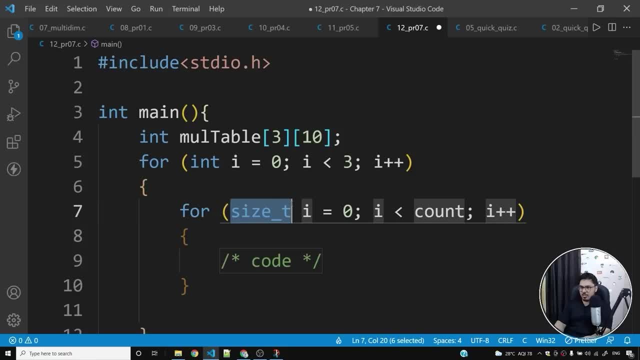 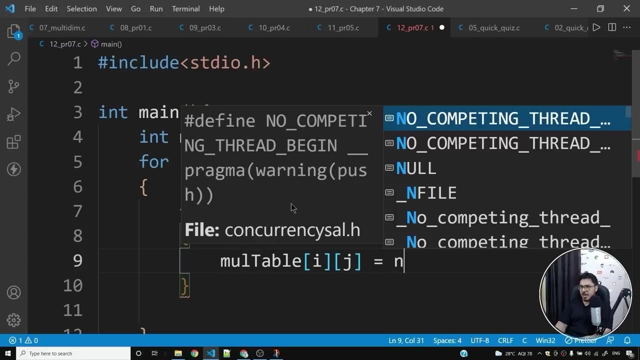 to 2 because i'm saying i less than 3 and the other for loop will start from. i'll change it to j because i already have i in my outer loop. i'll start it from 0 all the way till 9.. here i can use: multiple ij is equal to. i'll simply say multiple ij is equal to some value. let us say n. 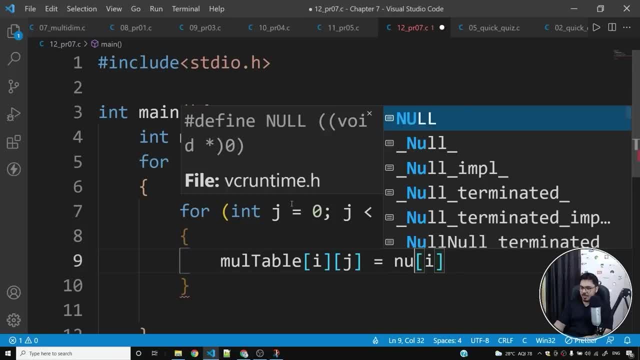 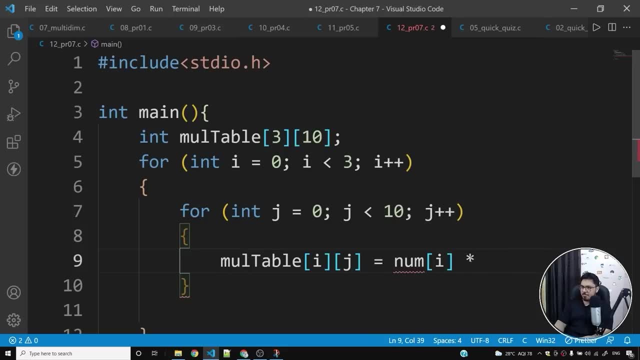 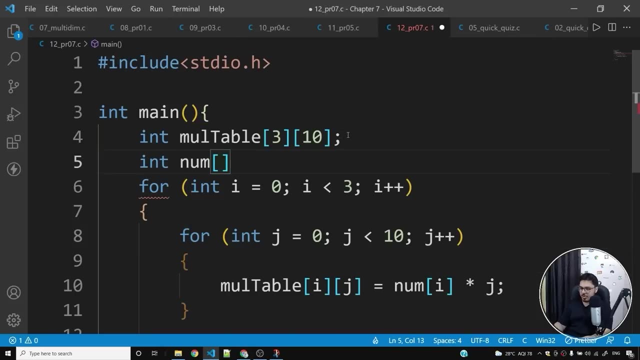 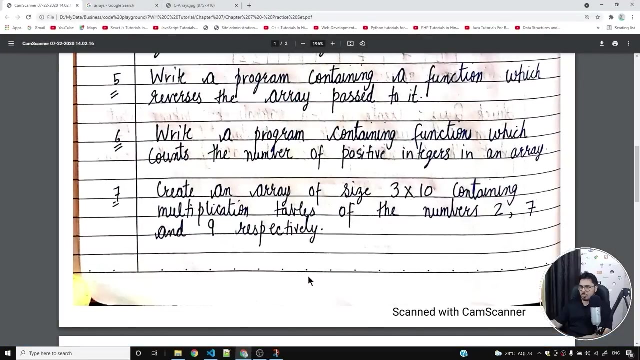 uh, num i. i'll tell you what num i is. multiply by, multiply by what? multiply by j. okay, so i'll simply say this and that's about it. but what is num? num is an array. i want to create an array num which will simply, which will simply tell me which number i am on. so 2, 7 and 9. so i'll simply. 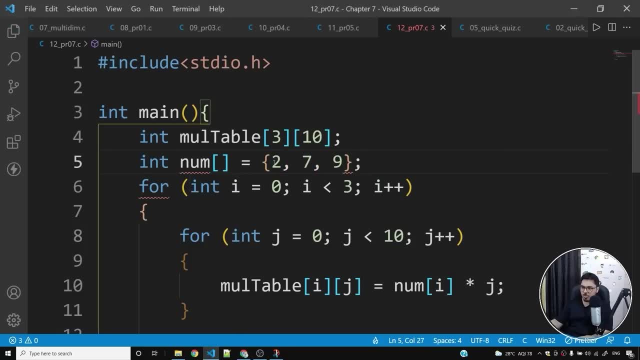 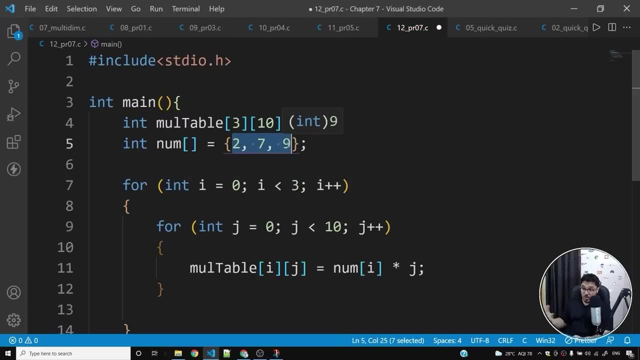 say 2, 7 and 9.. and i'll tell you how this is working, how this program is working. so num is a one dimensional array containing two, seven and nine. so num zero will be two, num one will be seven and num two will be nine. so whenever i need to seven or nine, i can use num i. so firstly, 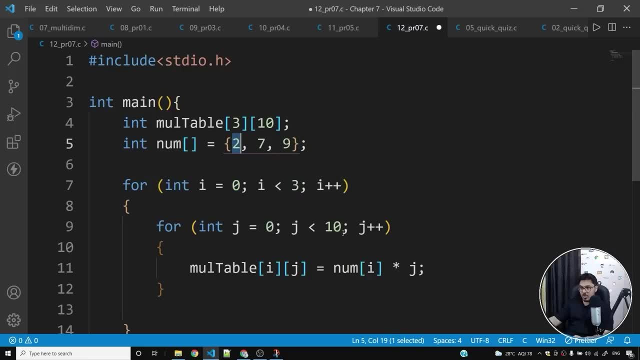 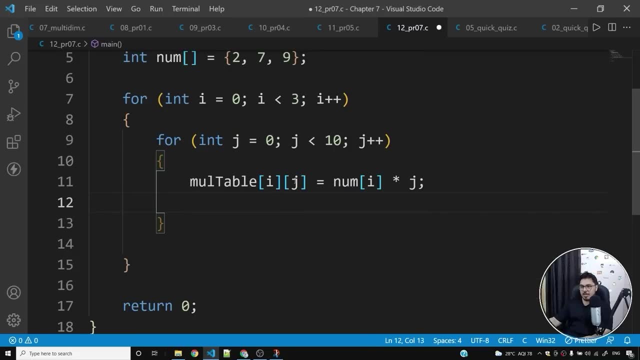 what i'll do is: i'll start from this number two. i'll write multiplication table of two. so, in order to write multiplication table of two, i'll simply say: multiple ij is equal to num i star j. and remember we have written a function to call it a function. 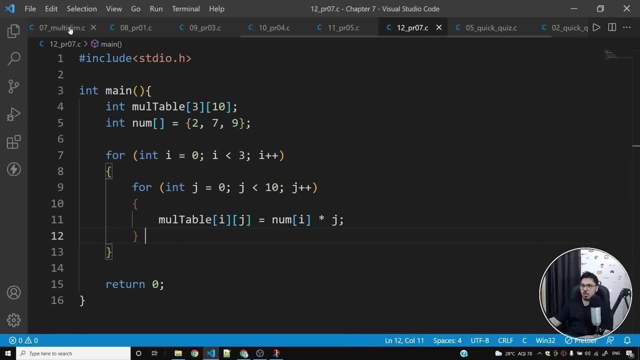 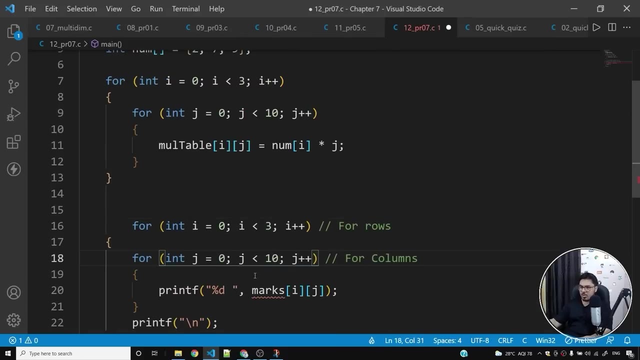 so i'm going to print a multi-dimensional array. if i'm not wrong, it was here, so this was the function. so i'll copy this function and i'll paste it here. so, after we are done, what i'll do is uh three and ten, so three and ten. what i'll do is i'll use uh, this function, to print all these. 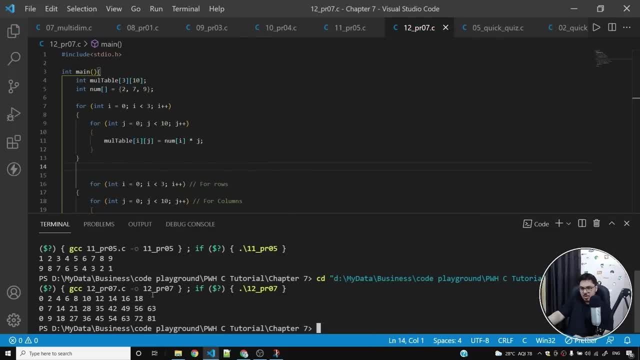 values. so let's, let's run this program and see if, if it works. so multiplication table of two is here and multiplication table of nine is here, but we are missing a number here, i don't know why. so i'm starting from zero, going all the way till nine. so nine multiplied by two is equal to 18.. 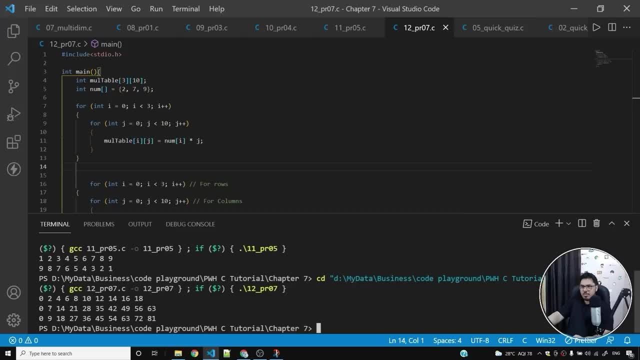 in case of seven, i'm starting from zero and i'm going all the way till zero: one, two, three, four, five, six, seven, eight, nine. so what this is doing is this is the multiplication table of two. this is for seven, this is for nine, so i'm going all the way till nine. so what this is doing is this is the. 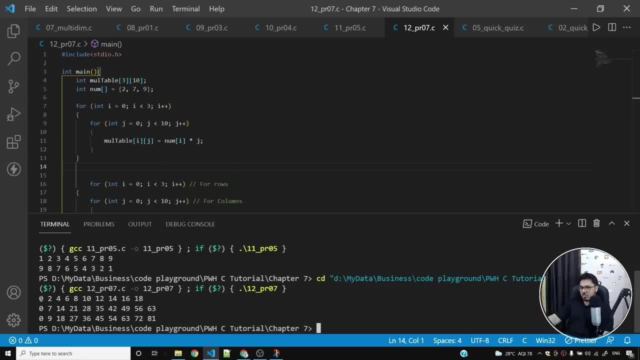 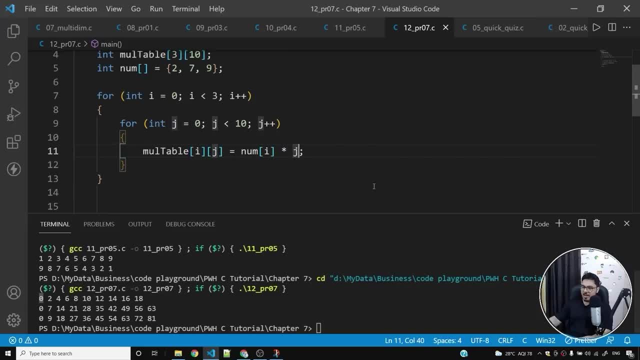 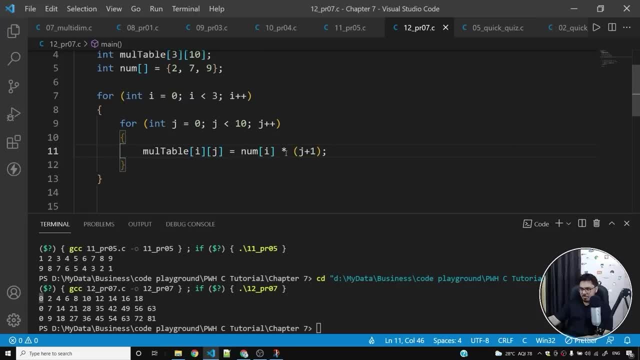 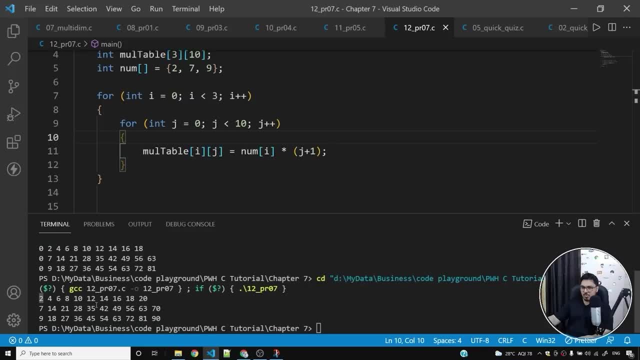 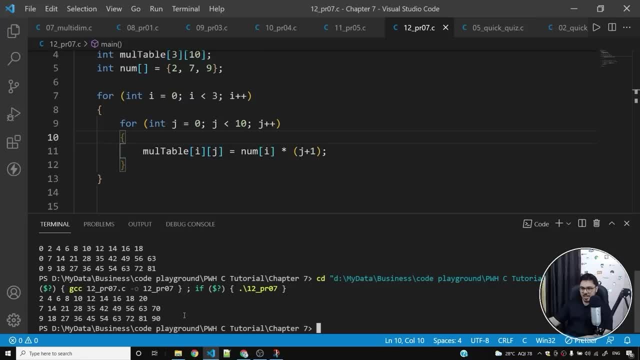 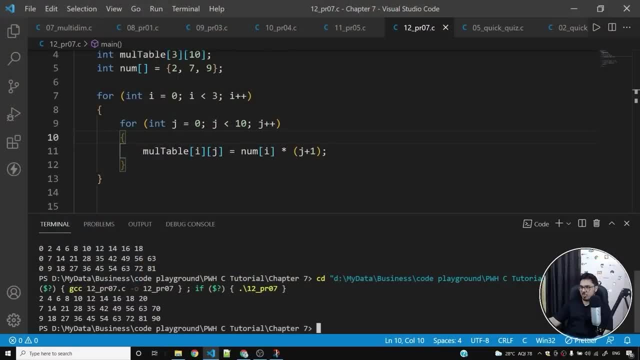 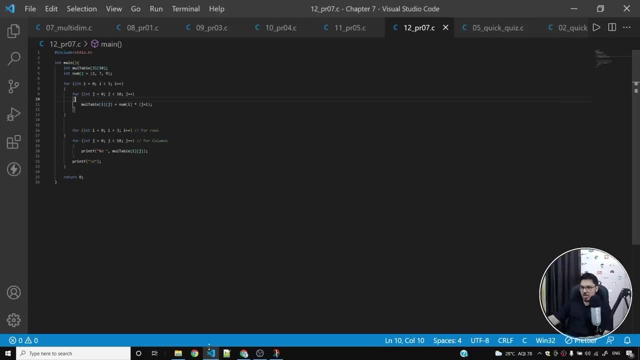 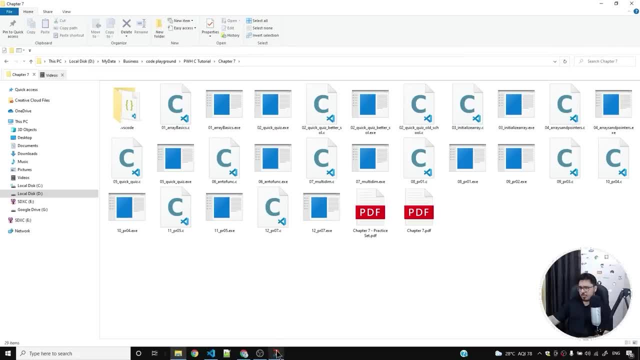 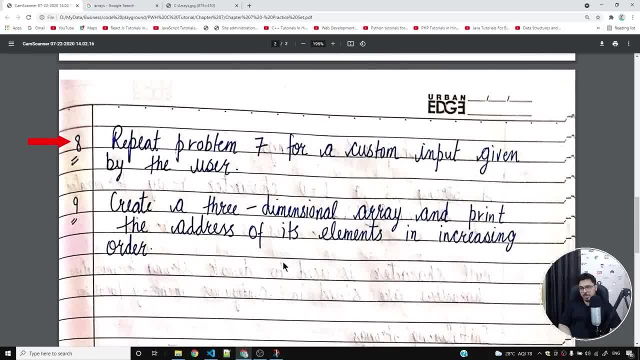 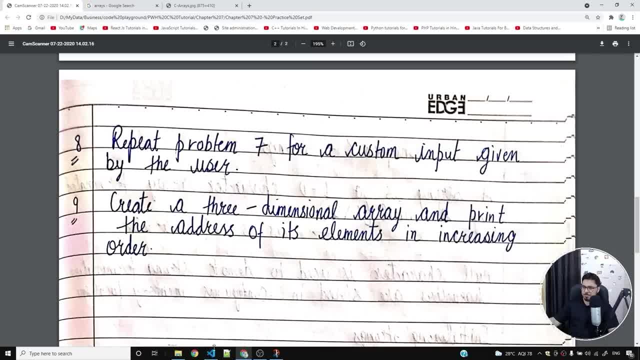 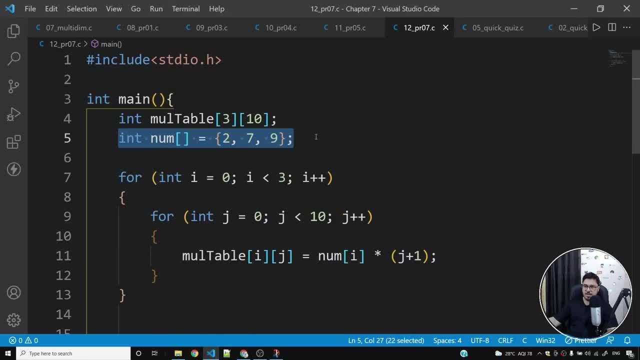 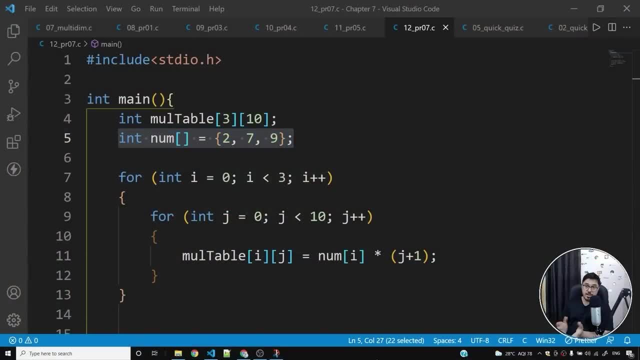 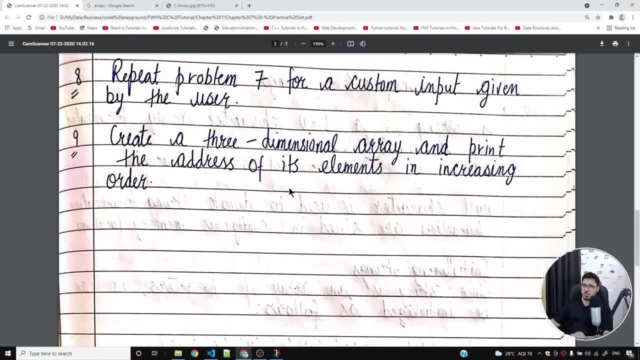 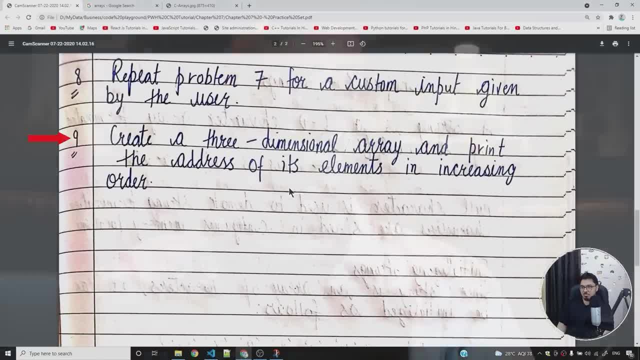 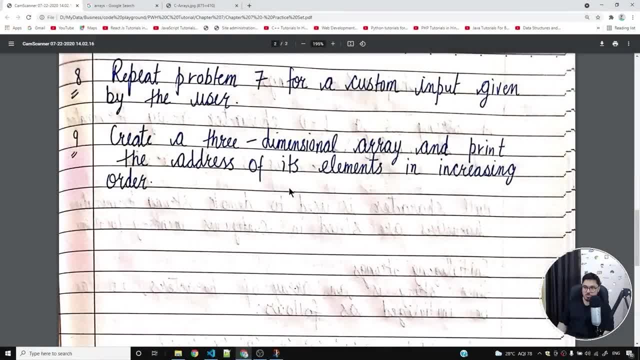 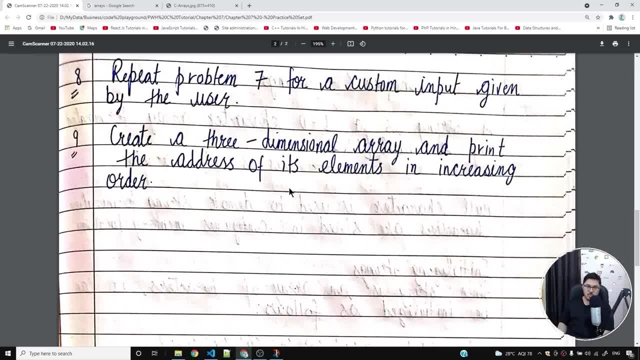 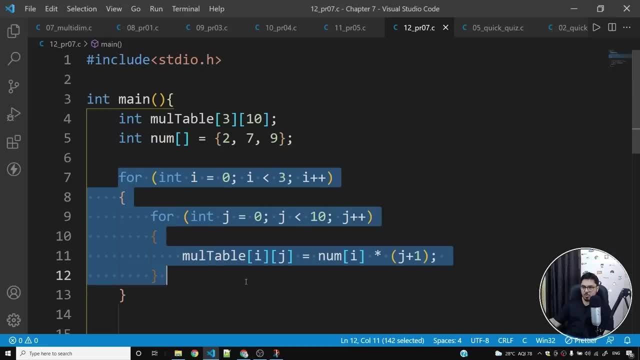 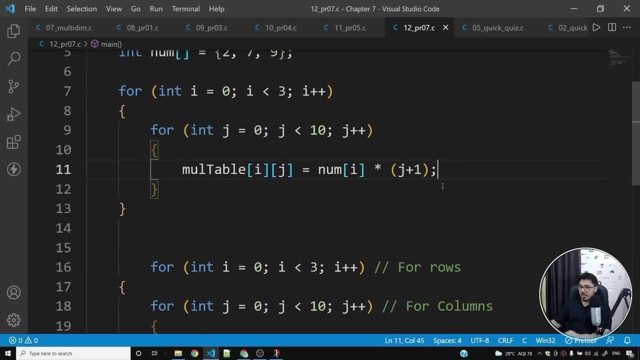 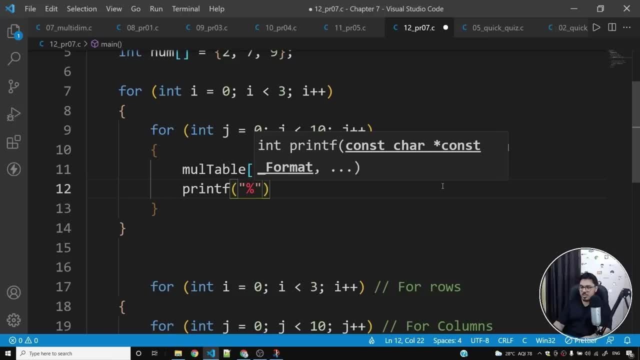 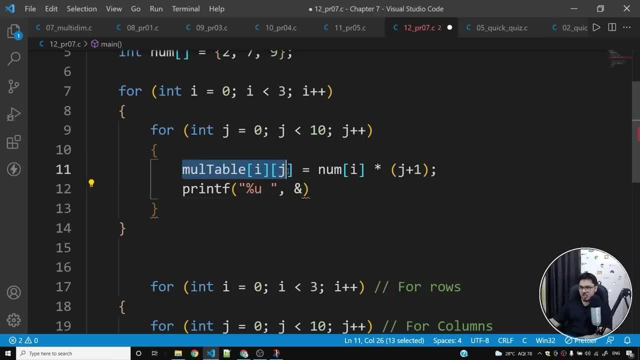 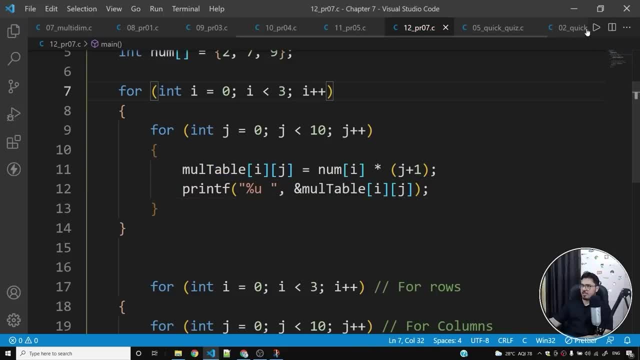 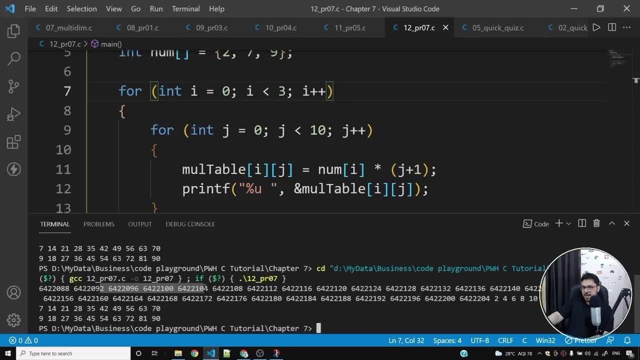 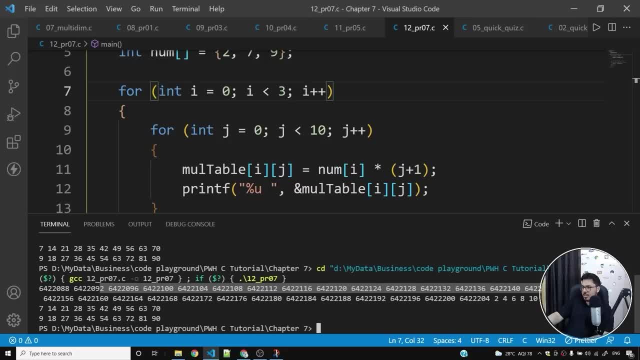 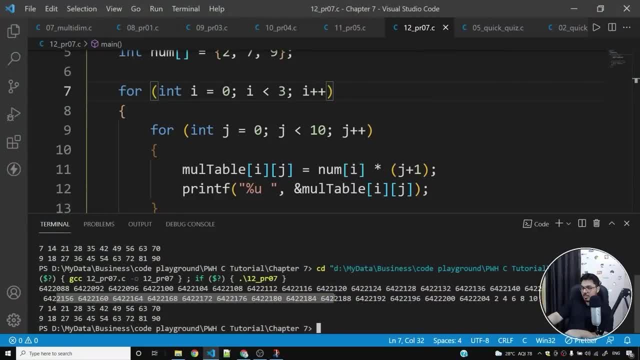 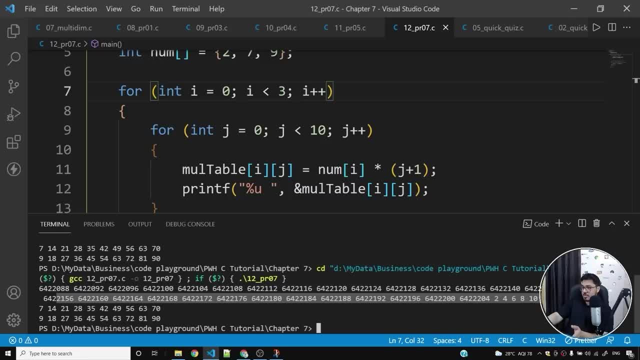 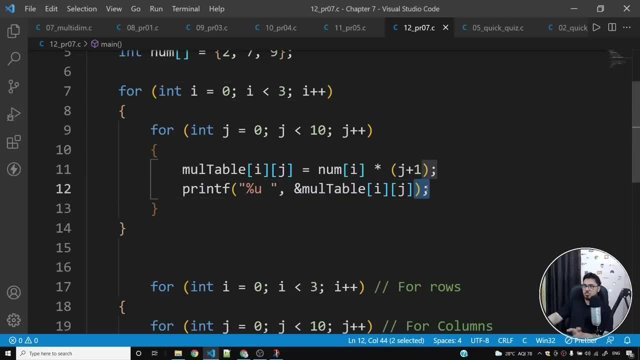 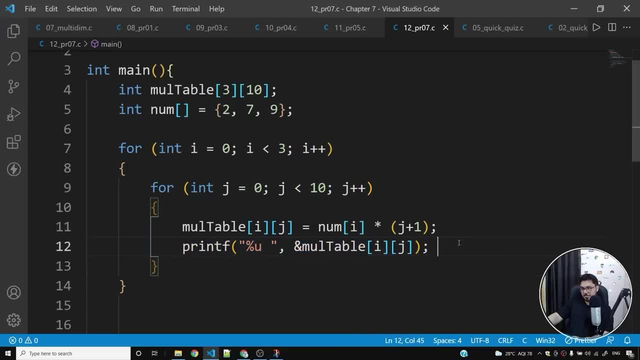 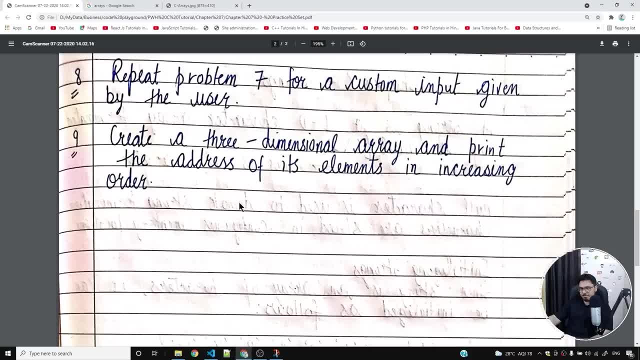 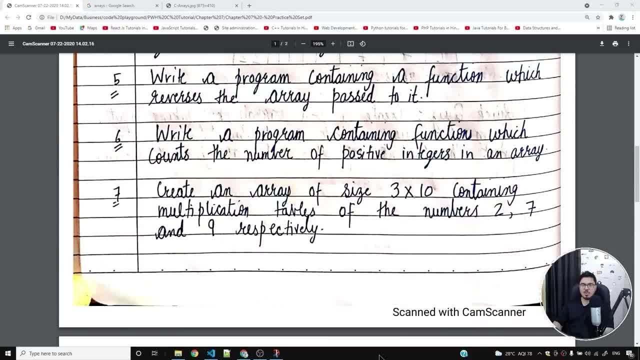 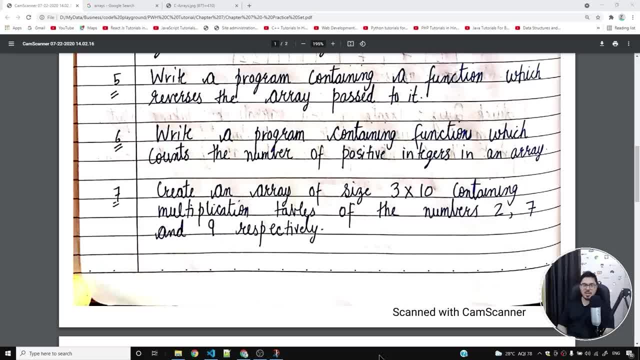 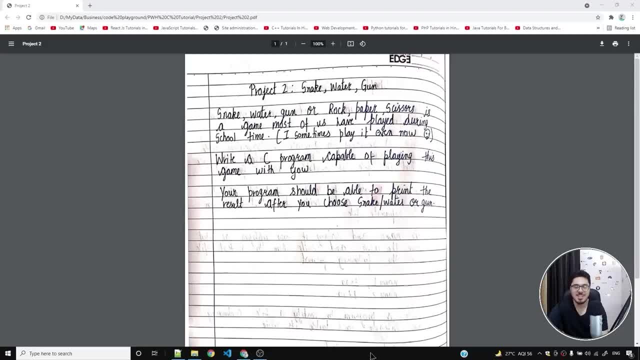 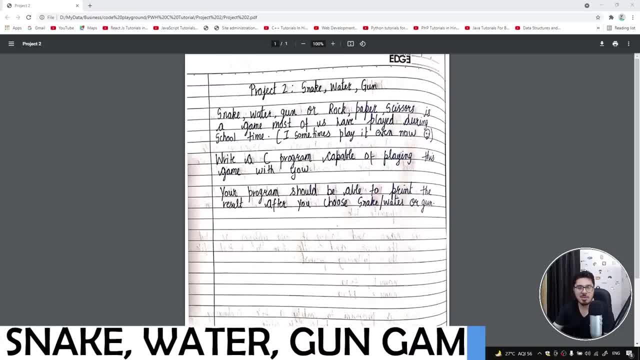 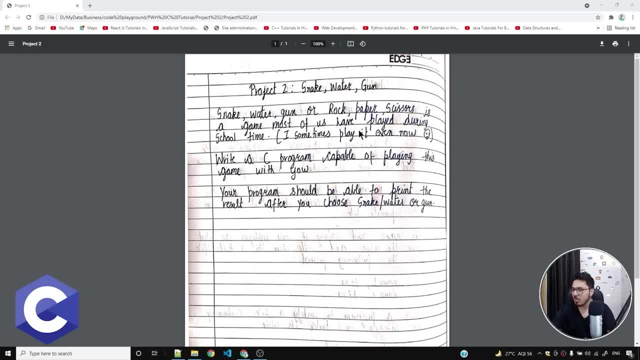 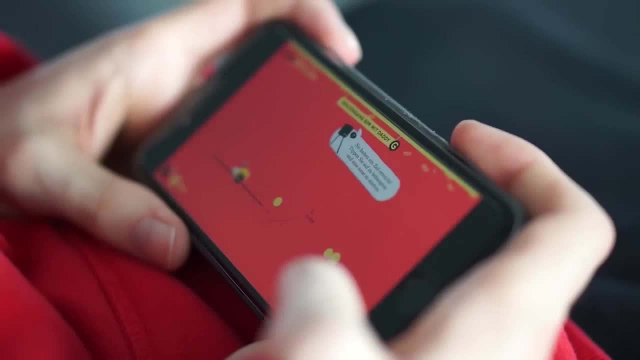 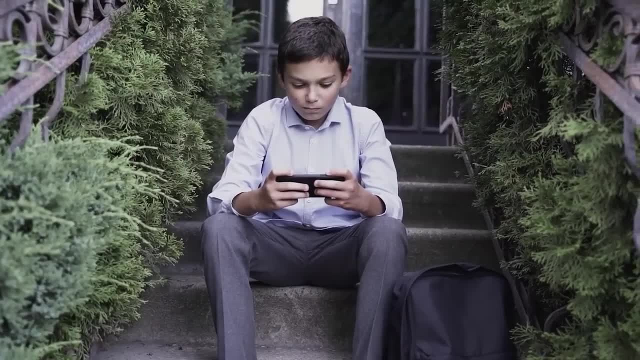 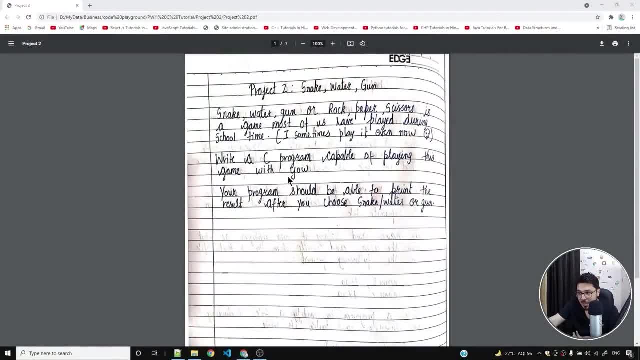 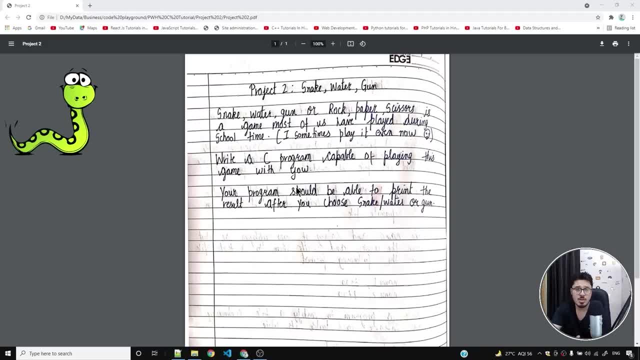 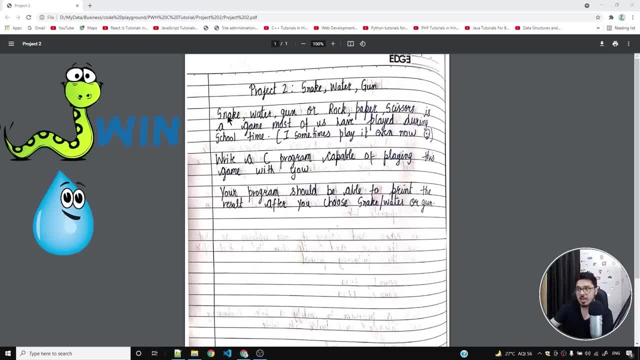 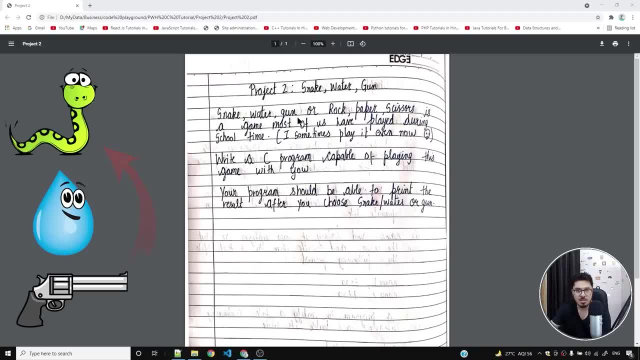 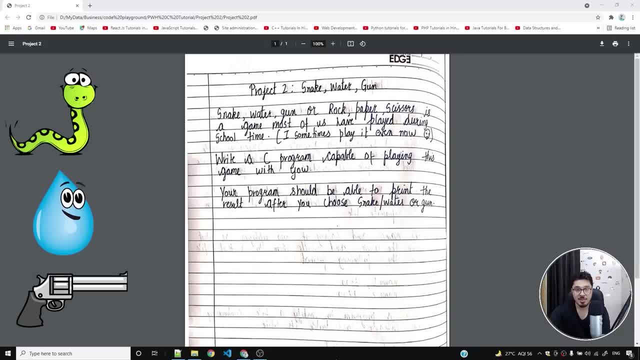 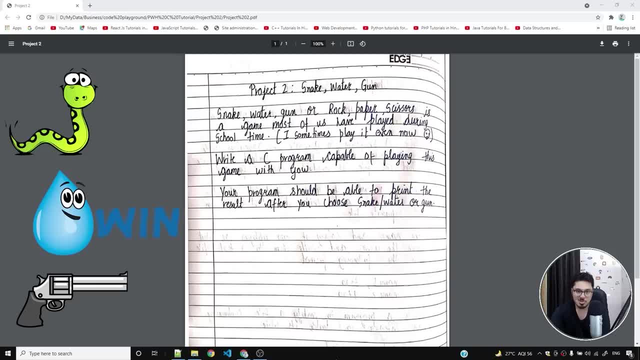 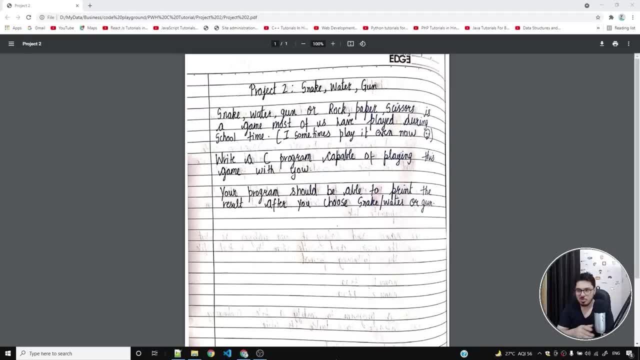 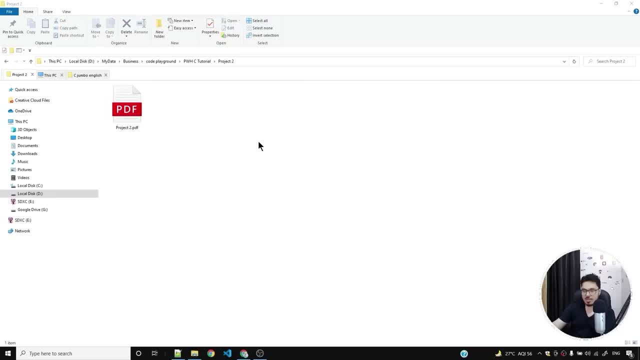 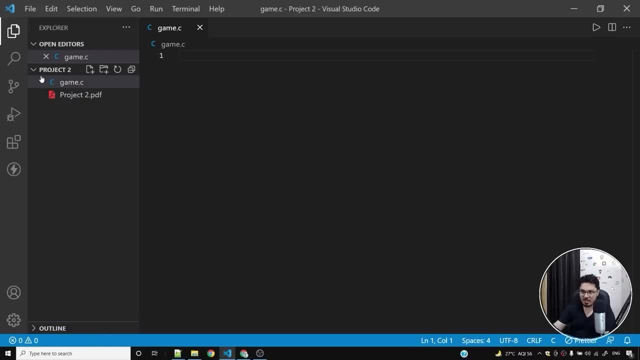 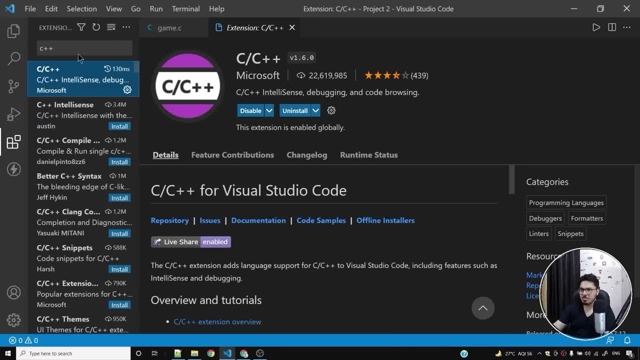 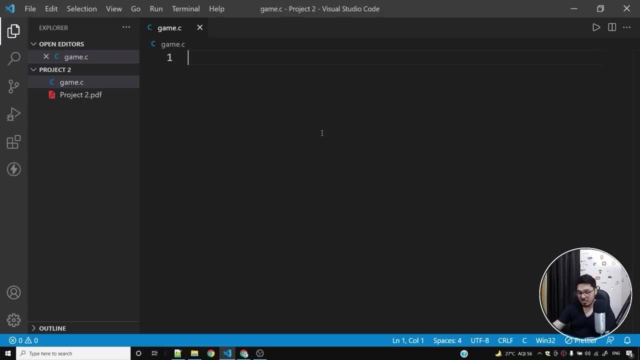 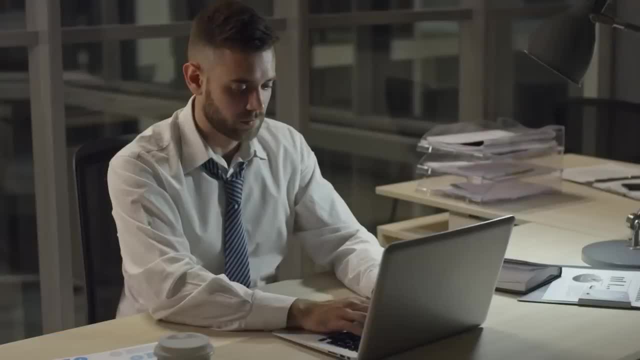 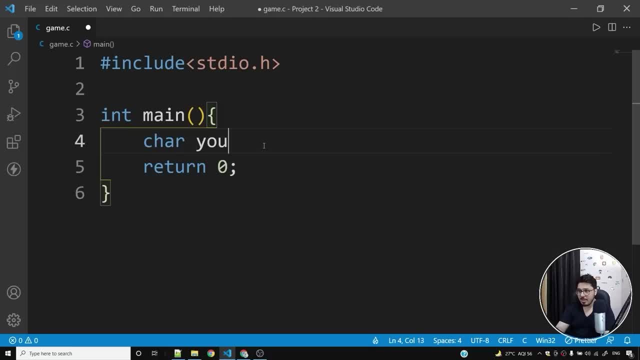 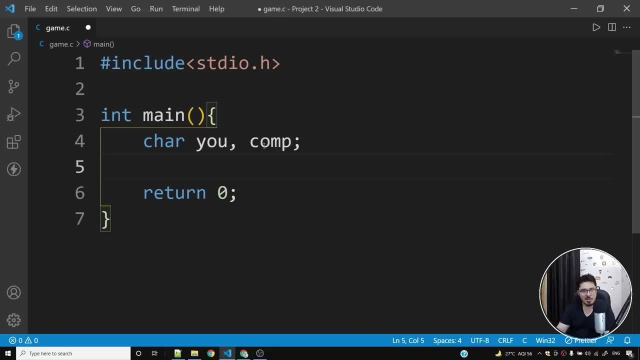 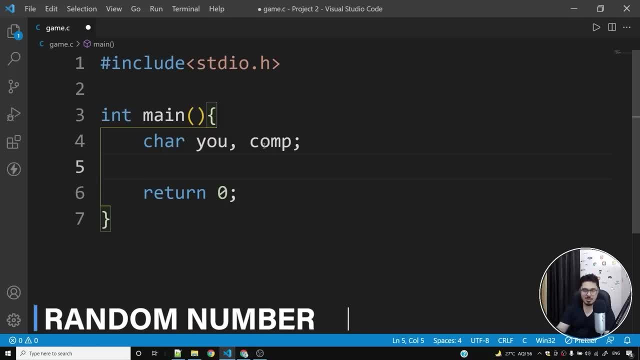 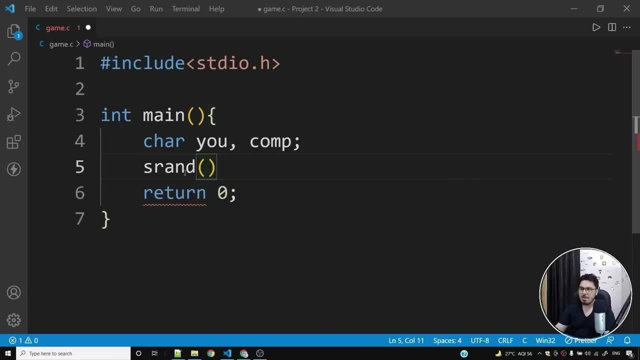 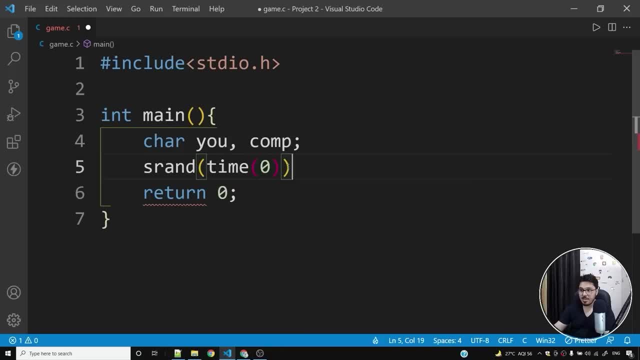 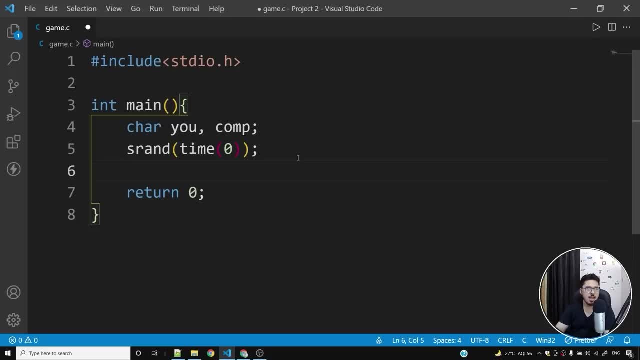 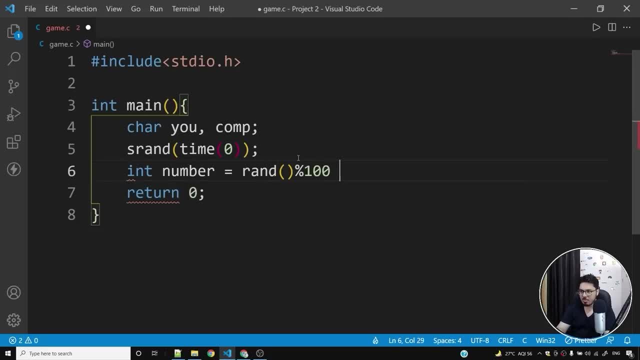 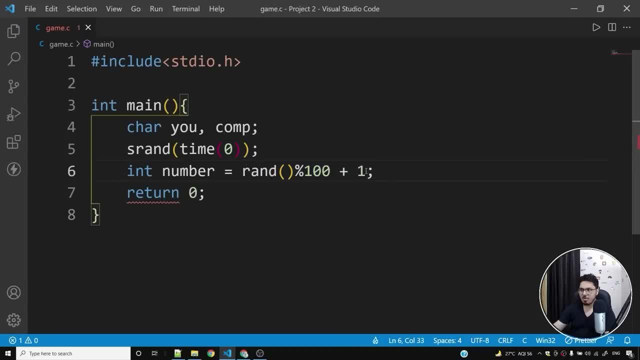 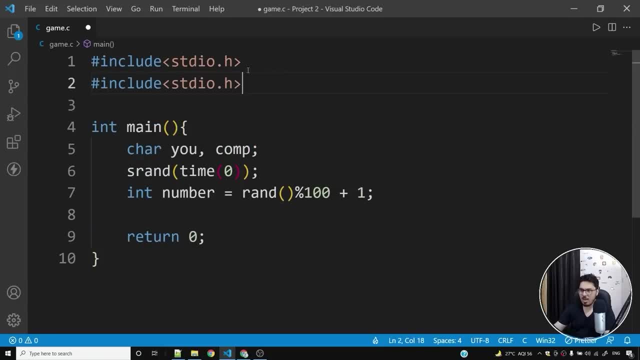 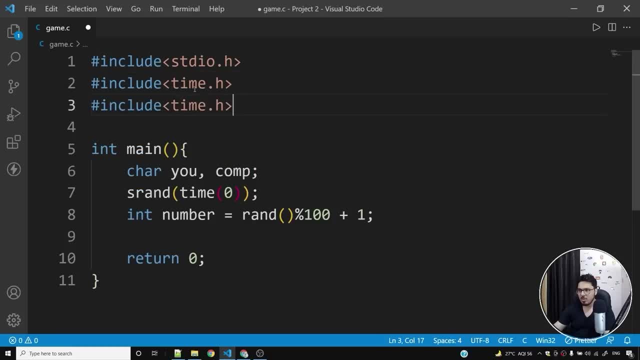 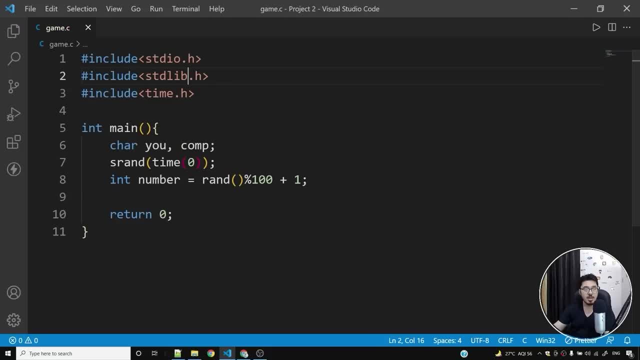 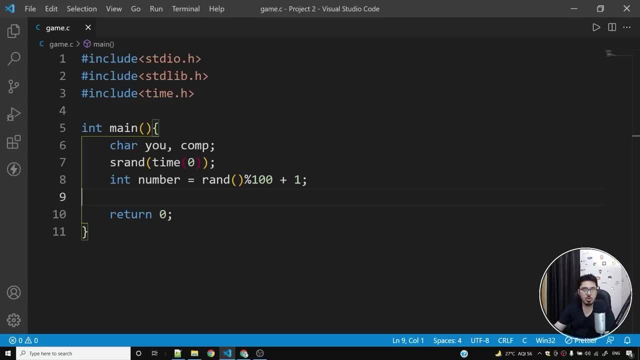 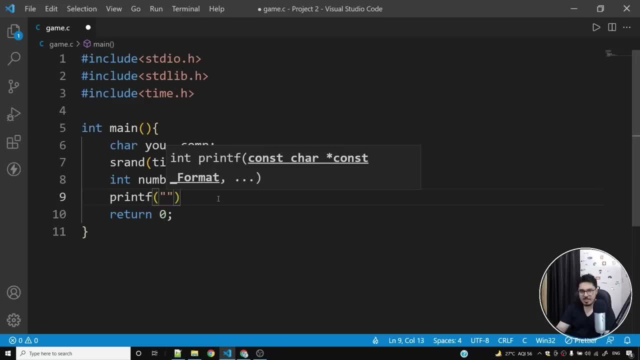 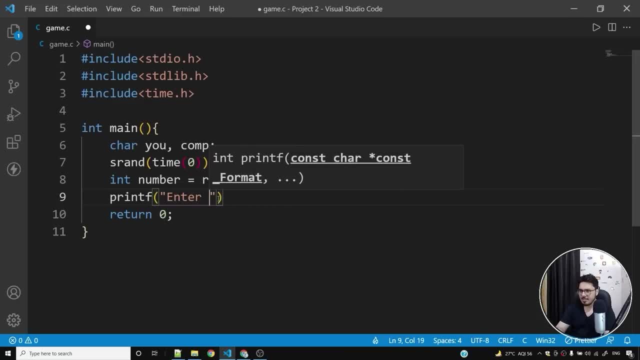 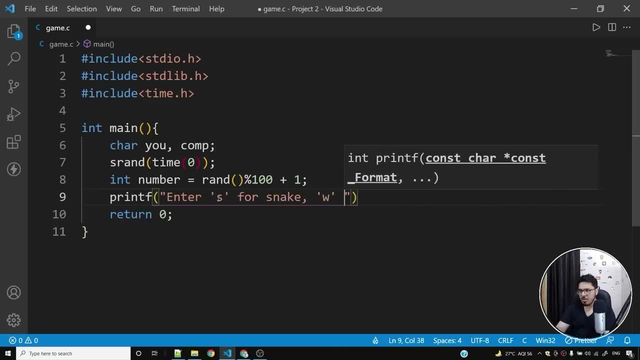 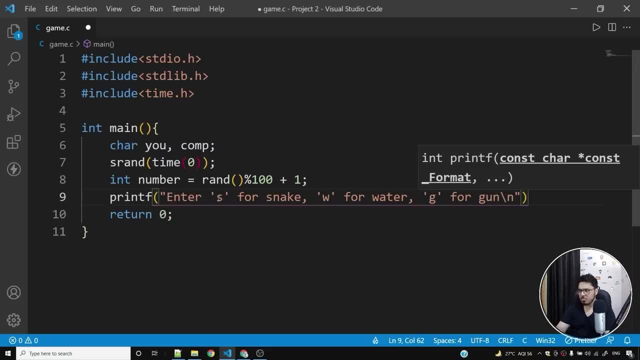 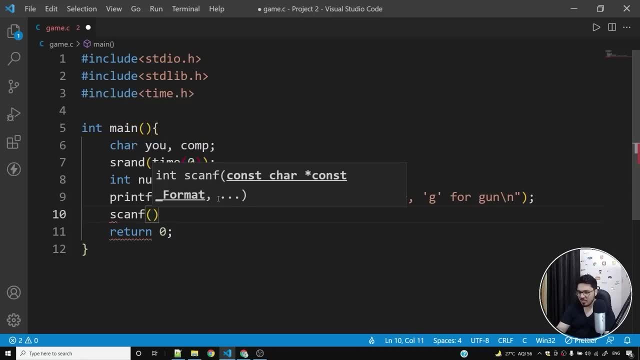 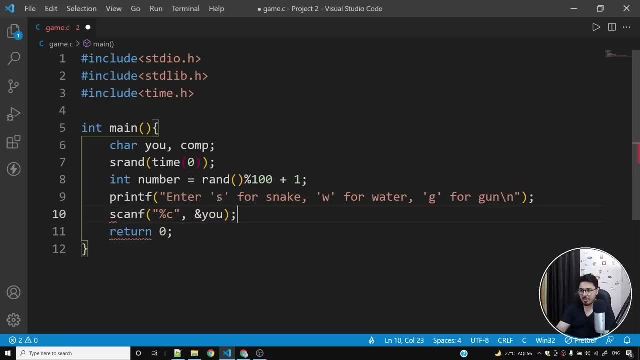 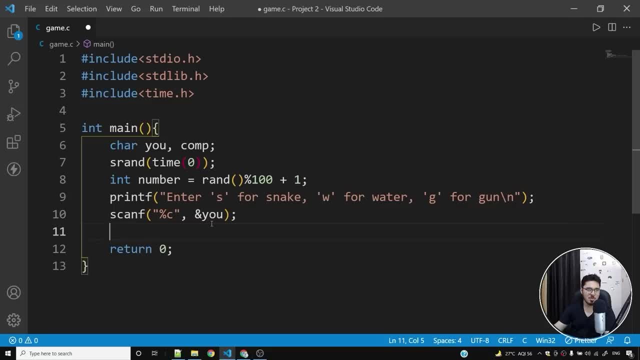 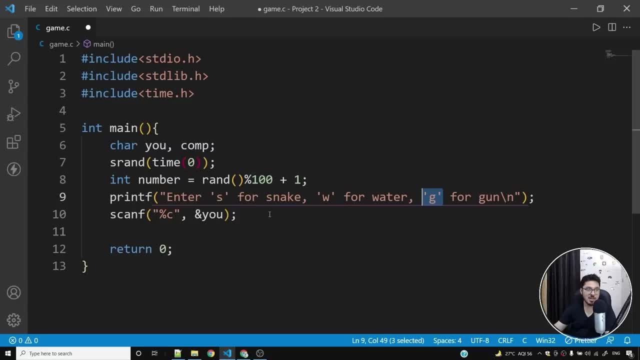 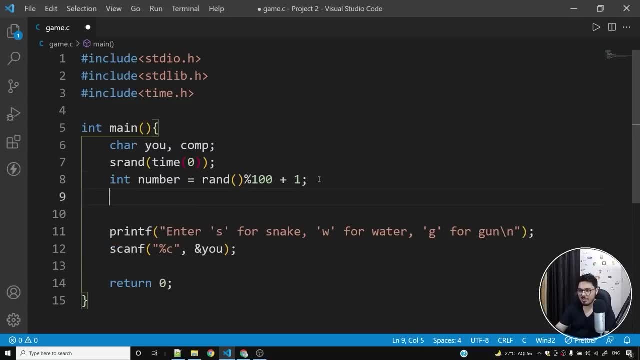 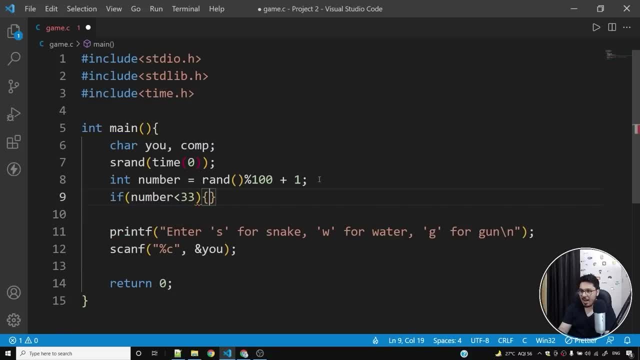 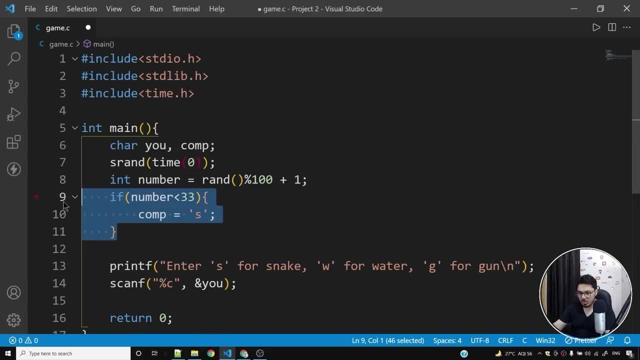 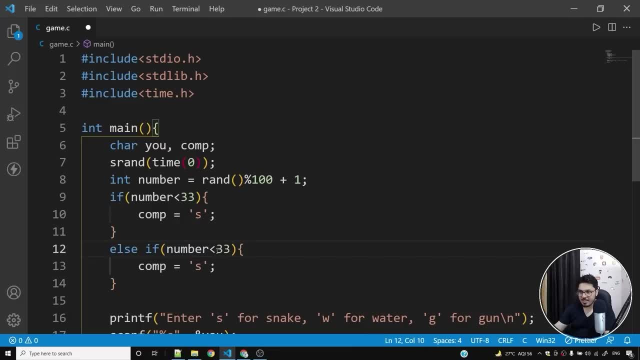 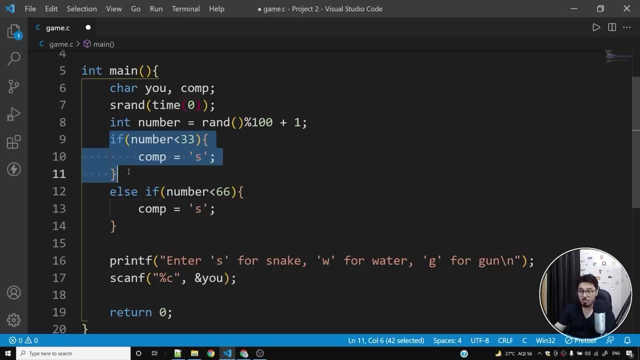 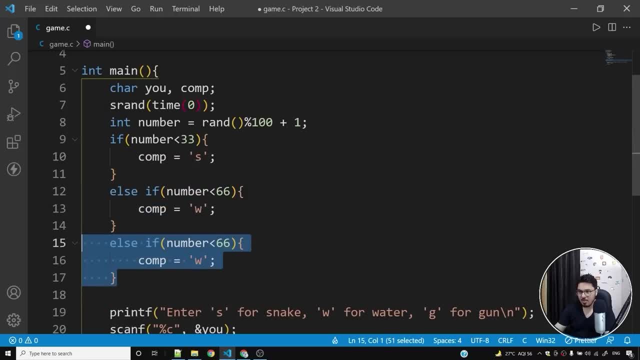 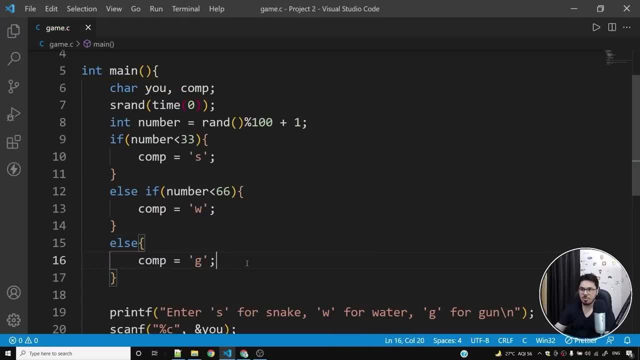 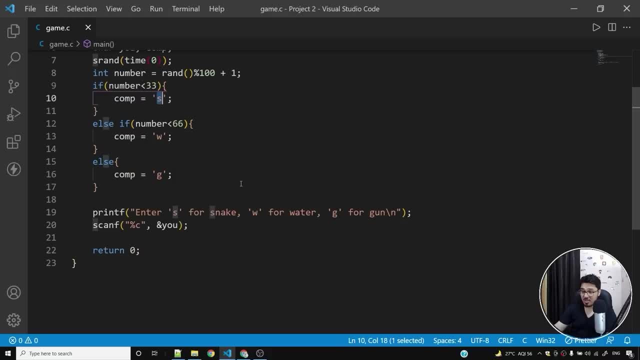 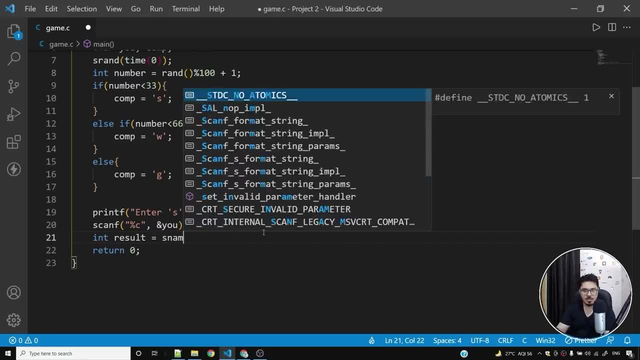 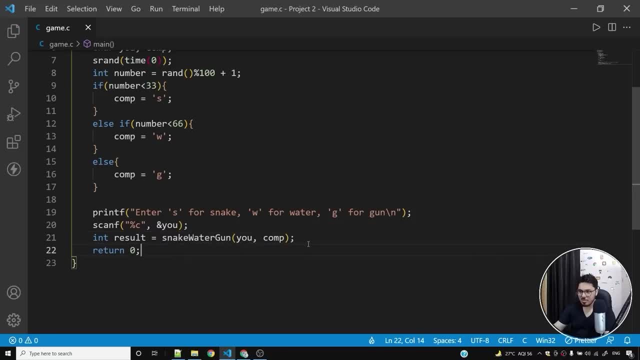 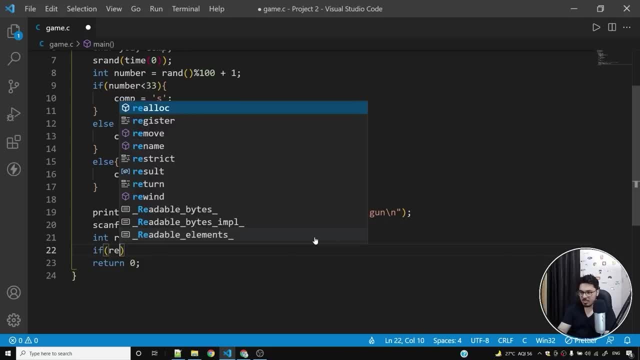 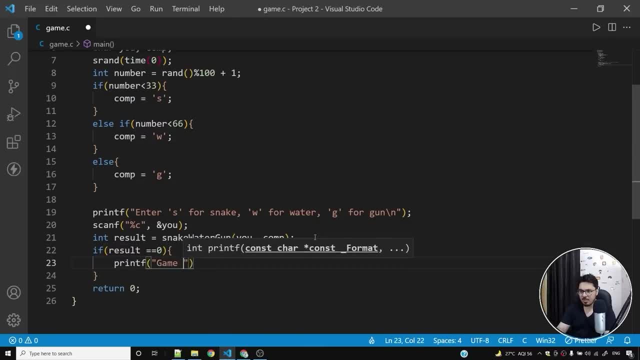 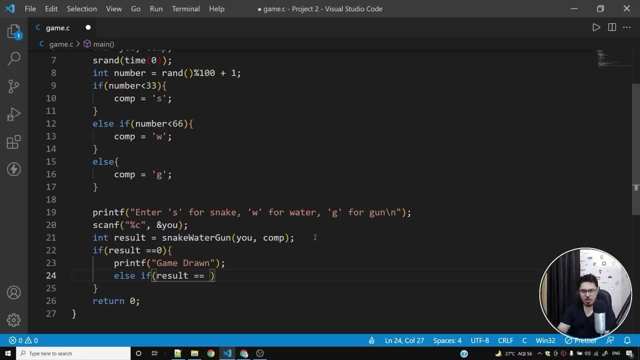 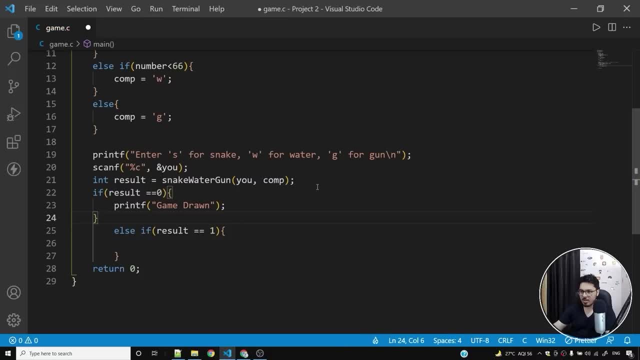 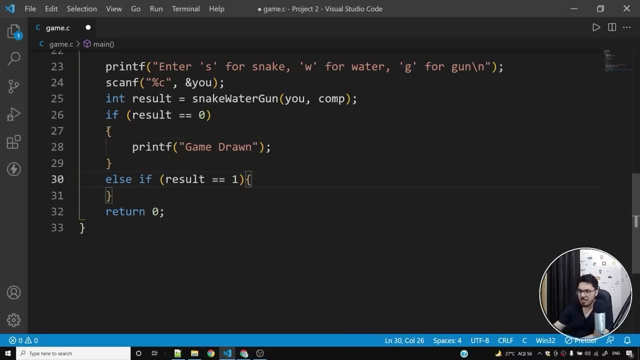 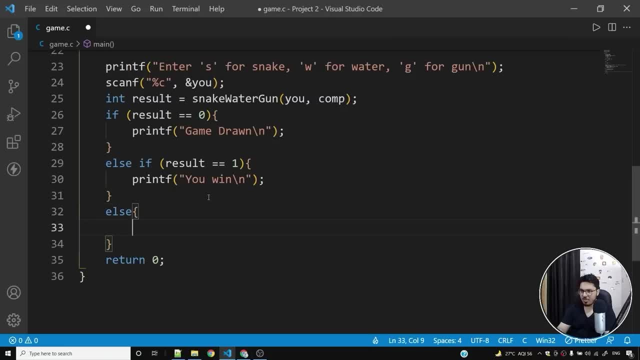 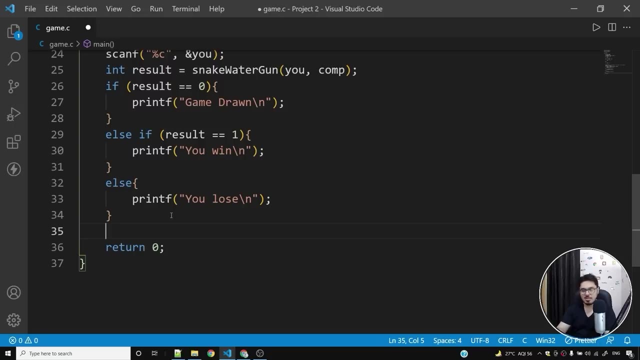 okay. otherwise definitely you lost okay. so i'll say you lost, you lost okay or you lose okay. now what i'll do is i'll simply show you at the end of the program what character did you choose and what computer chose. so i'll say printf, i'll say you chose percentage c and the computer chose 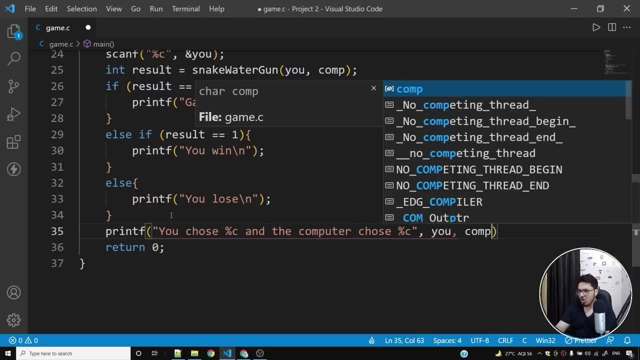 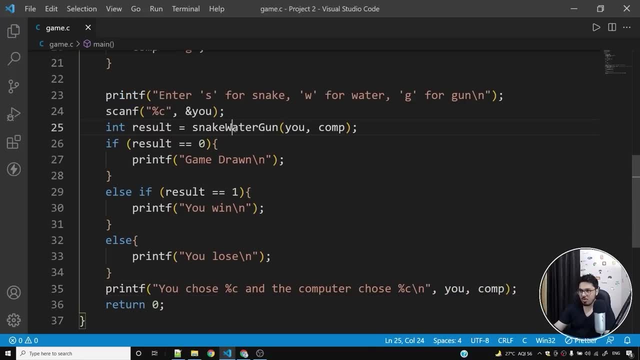 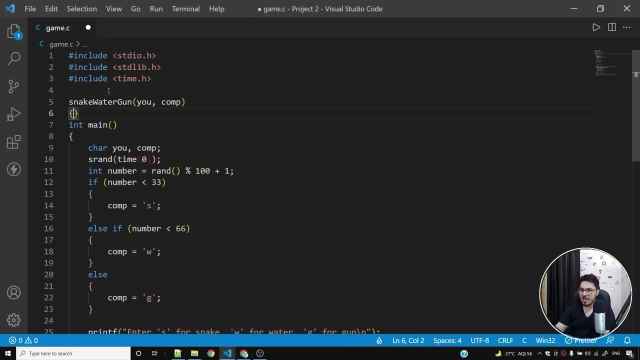 percentage c. okay, you comp, because at the end i'll definitely give you a good idea of why you won or why you lost. now our entire task, or the entire game, revolves around this function, which is a snake water gun game. it's going to return an integer and it will take two integers. 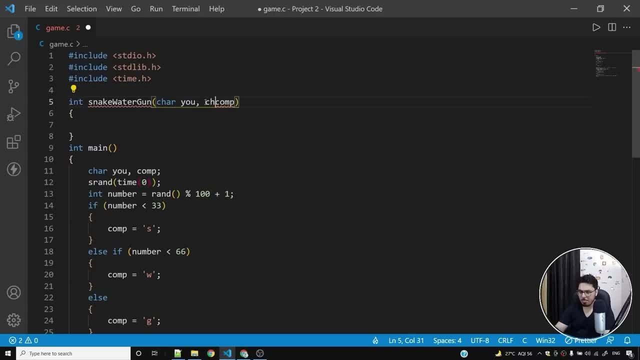 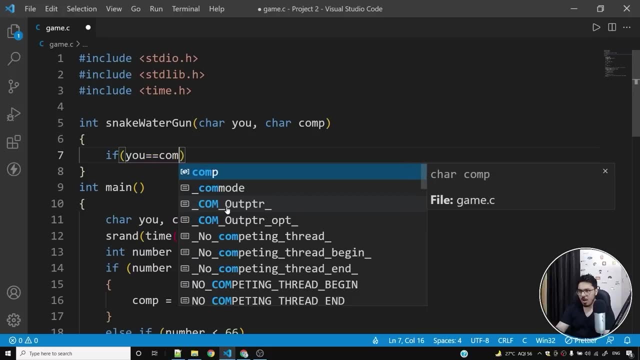 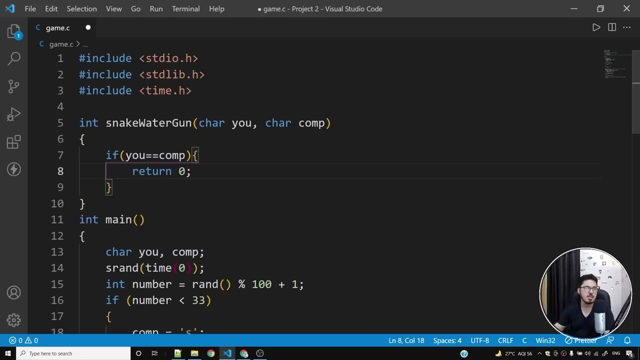 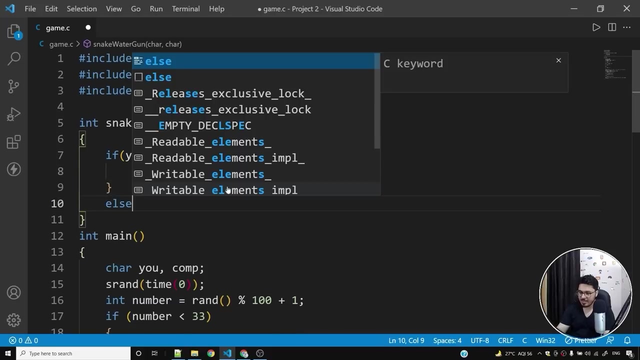 sorry characters, u and comp. now, definitely, if u and comp are equal, i'll immediately return zero, which means that game drawn, because if you both selected the same characters, the game needs to get drawn, okay, otherwise i'll say else. i'll say if else, if you are. 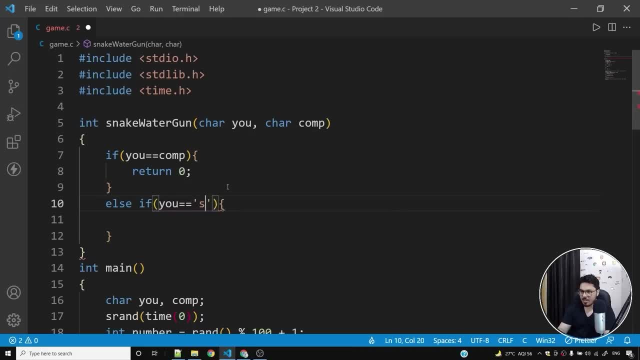 you are snake and let me add few more brackets. so what are the chances of you winning? what are the possibilities that you are going to win? what are the possibilities that i should return? one: if you are snake and computer is, say, computer needs to be water for you to win. 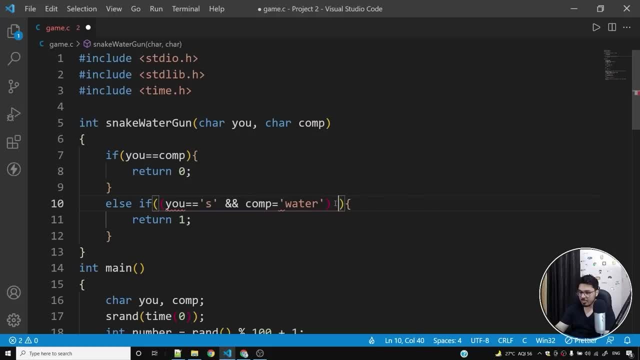 this is a win situation for you. i'll put in another win situation for you or another win situation for you, which is going to be. let me put in w here for water, and u is a variable. it says expression must be a modifiable l value. what's wrong here? okay, so this should be double equals two. this will work. 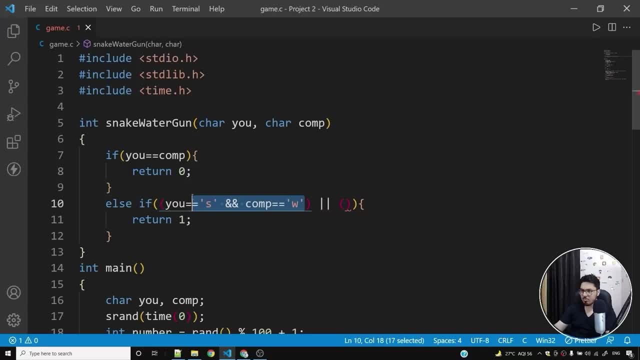 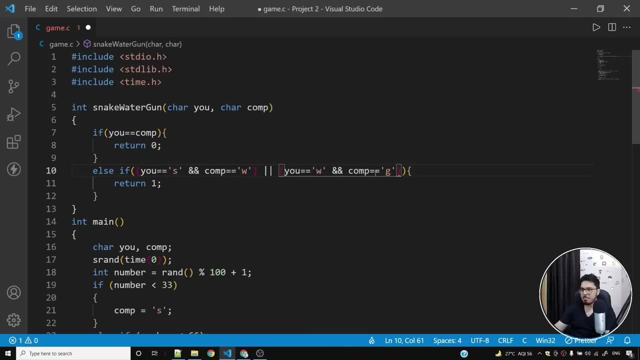 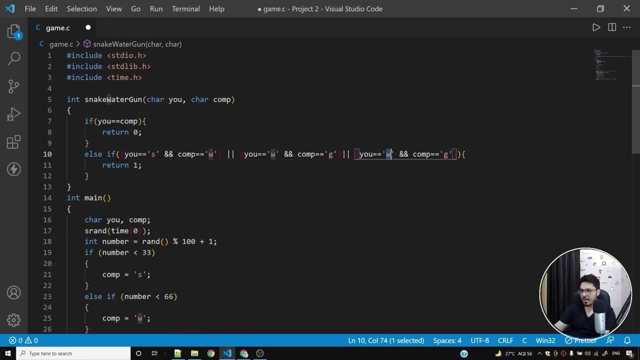 now. so this is a win situation for you. another win situation for you is to select water. to select water, and if computer selects gun by luck, you will once again win. another win situation for you is going to select gun, and in that case computers should select snake for you to win. in all these cases, you are going to win. 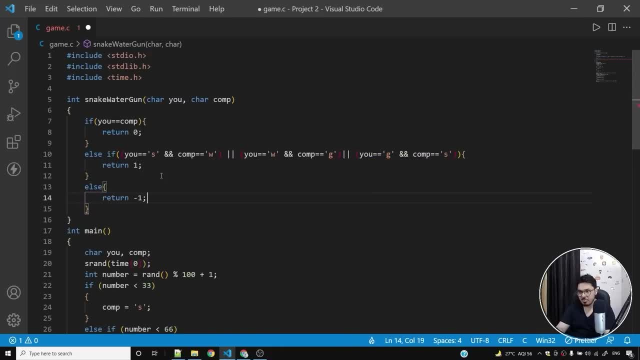 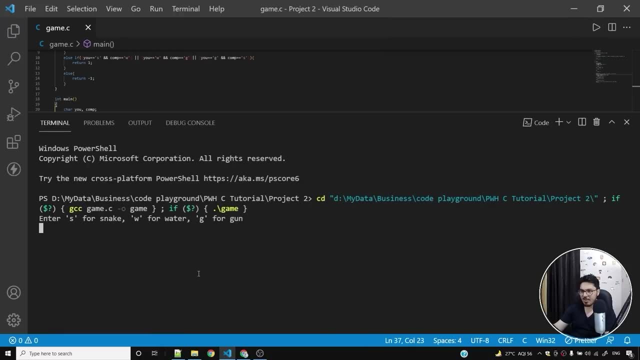 otherwise you are going to lose. so i'll say: return minus one, minus one for loss. okay, so let's run this program now and let's see if this program works. so if i run this program so it says interest for snake, let me choose snake. it says you lost because computer chose gun, my bad. 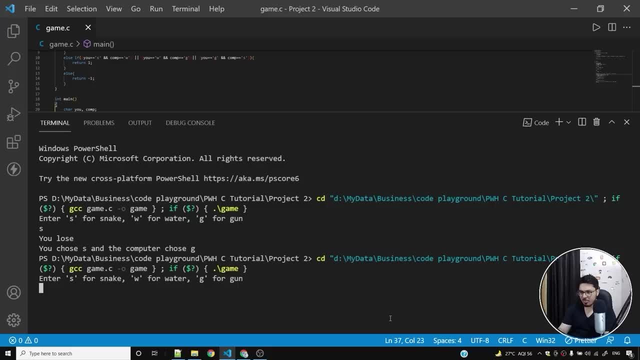 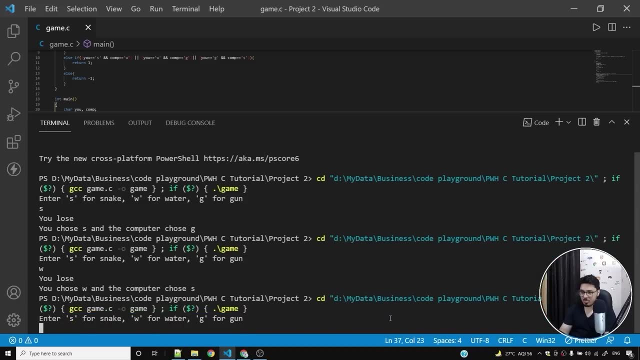 once again. i'll say water w. it says you lose because computer chose snake and it drank your water. my bad, why am i so unlucky? i'll choose snake and it says you win because computer chose water and you drank computer's water. now it's asking me for another thing: gun game drawn. 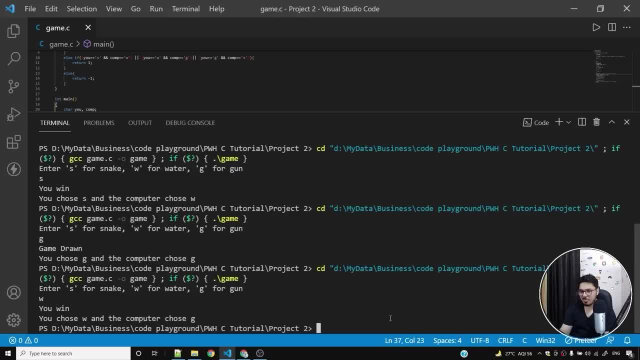 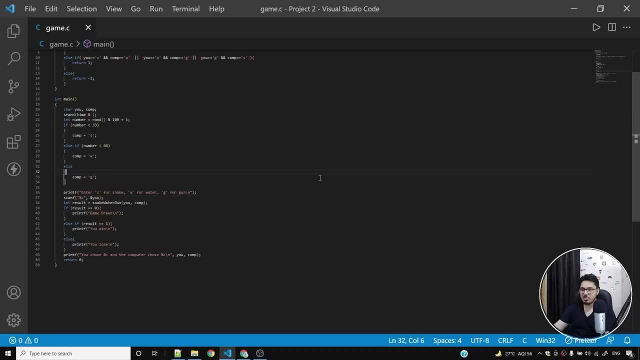 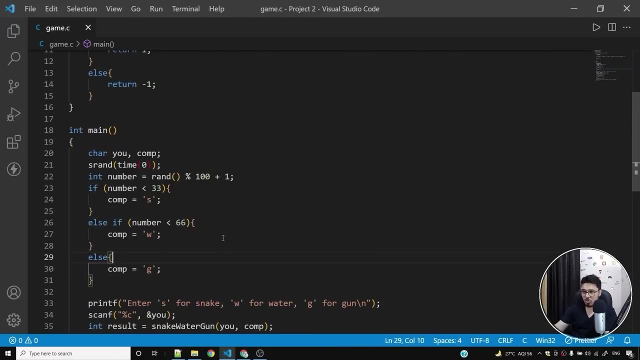 computer also chose gun. now, once again w you win because computer chose gun and you actually drown computer's gun. great, great, great. so this was the game. i hope you enjoyed it and you can format the you know code as you want. i want my code to be very clean like this. i don't want a 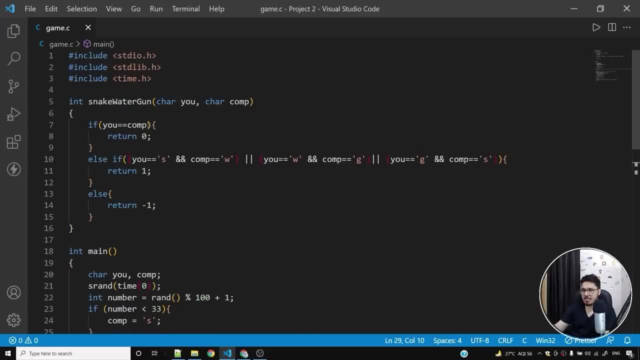 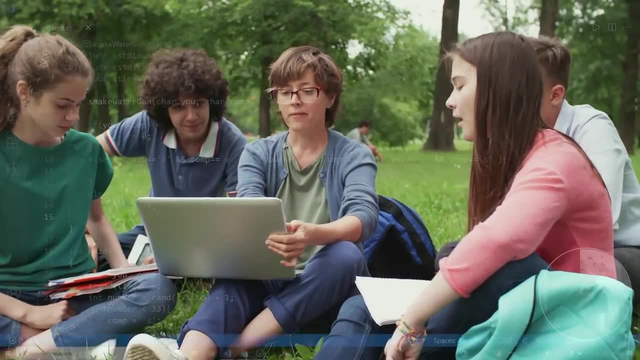 lot of new lines inside my code, which is why i'm formatting it like this. so i hope you like this game, enjoy playing this game and also play this game with your friends. they will also enjoy it. you can also refactor this game to play it with your friends so you can always, you know, do. 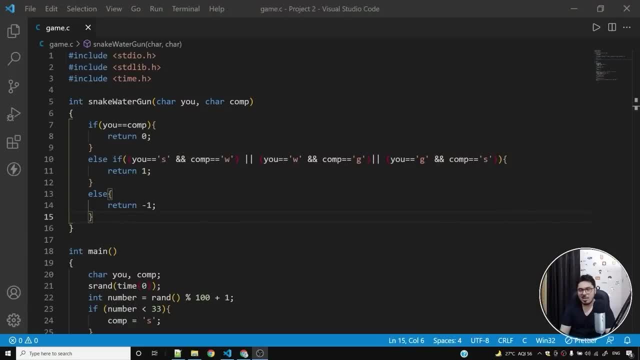 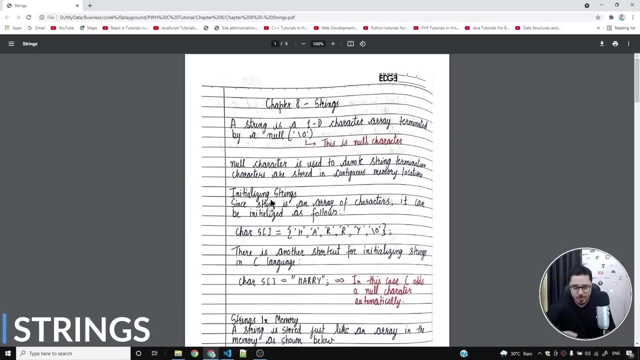 something so that you, you can play this game with your friends. so now what i'll do is i'll move on to the next chapter and we are going to explore some more concepts of c. so, topic of today's: string: in chapter 8 we are going to learn about strings, and strings is something that you are going to use, a. 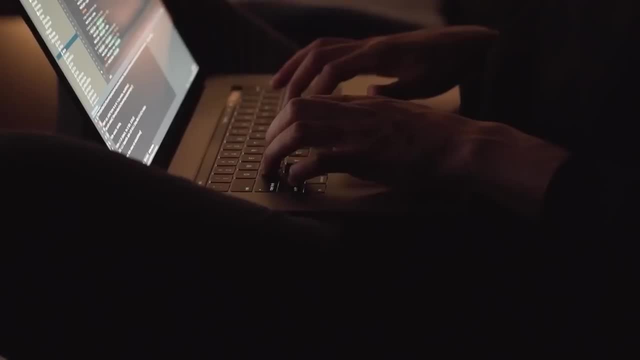 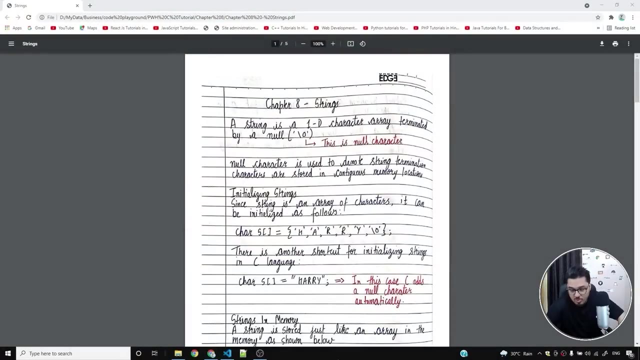 lot, not only in c programming language, but in programming in general. you are going to use a lot of strings, so let's talk about what a string is. it's a collection of characters. let's talk about string in layman terms. what exactly is a string? it's a collection of characters. 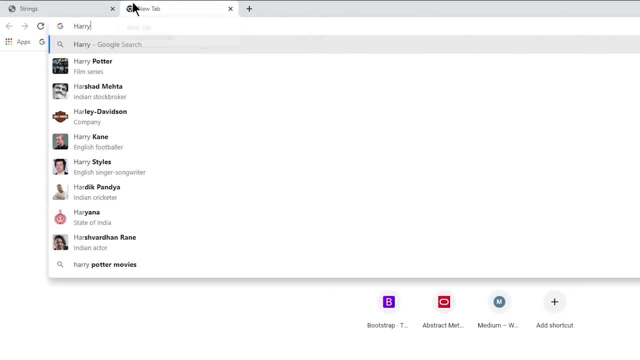 so if i write my name here, it will be a string. so if i say harry, it's a string. if i say, let us say john, it's a string. if i say kane, it's a string. okay, so you, you know what a string is. but let's. 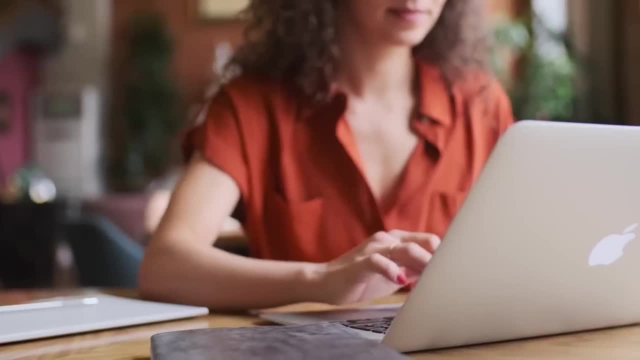 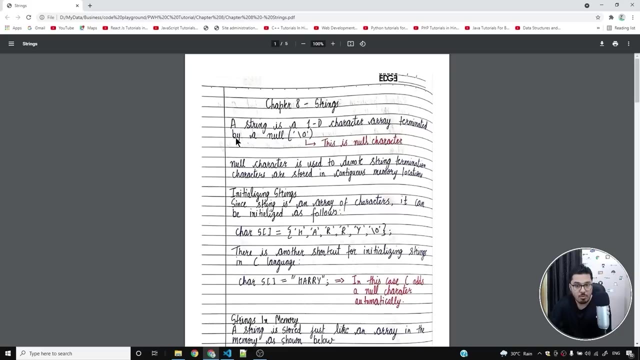 talk about what exactly and how exactly are strings represented in c programming language. so this topic is really very important. so when i talk about c programming language, when i talk about c programming language, let's say that a string is a 1d character array terminated by a null. 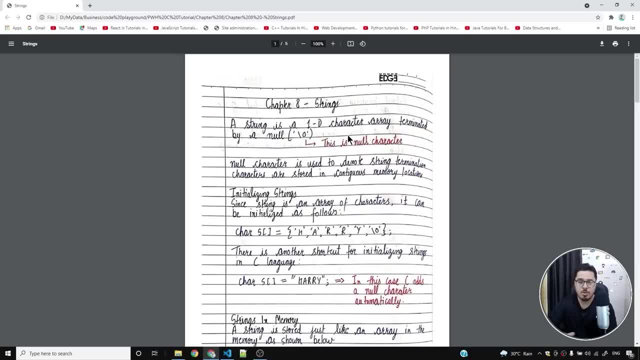 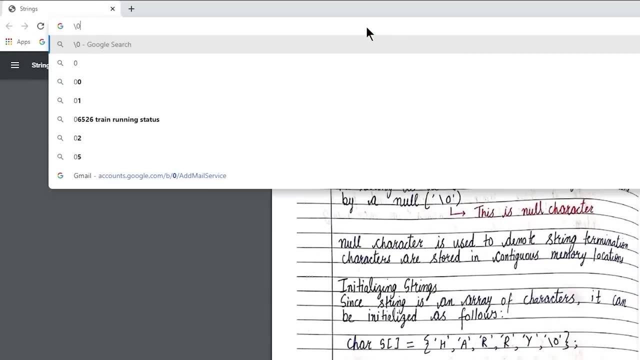 we know that the collection of items or others, collection of similar items, in c programming language is called string. so a string is a 1d character, or rather 1d character array terminated by a null character. okay, so what exactly is a null character? so backslash zero, it's a null character. 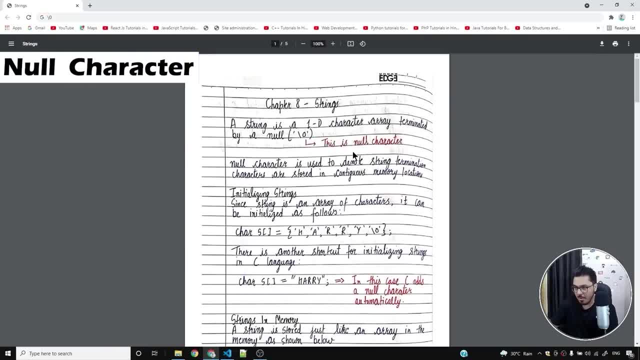 and we are going to talk about what exactly is this null character and how we can use it. but let's let's try to find out how we represent strings. in c, null character is used to denote string termination. characters are stored in continuous memory locations, so let us say this: 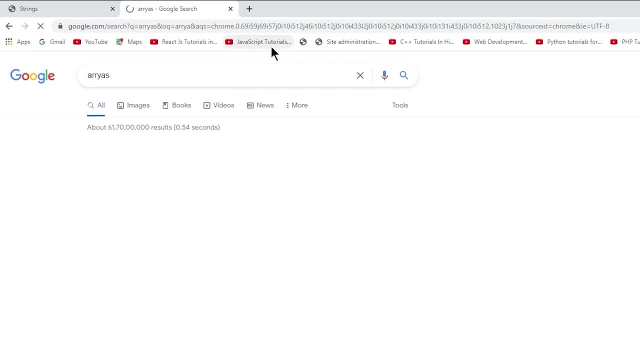 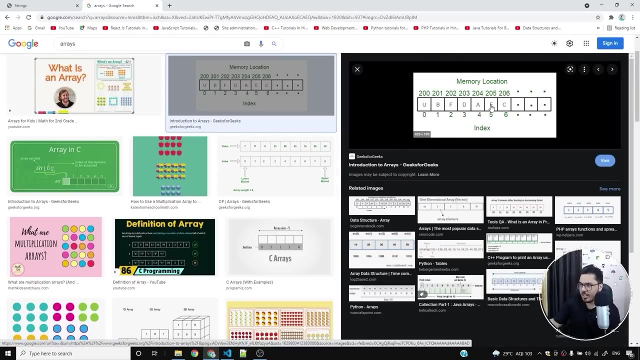 is my memory, so i'll simply google array, oops images, and let's talk about this image. let us say: this is a string: u, b, f, d, a, e, c. one byte is going to take one character and it is indeed taking one character. you can see that. 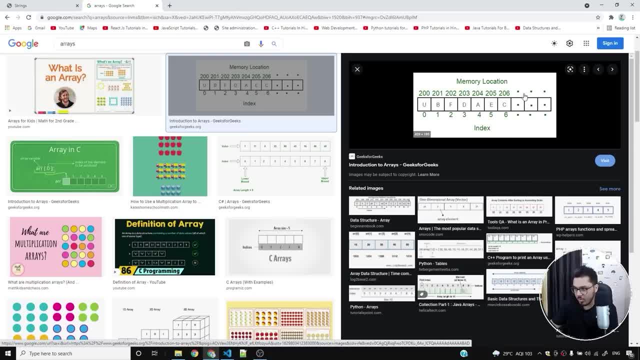 you can see that the string has been stored in continuous memory locations. so what exactly is the string? if i start reading from here, the string can be u in memory. it can be u b, it can be u b- f. where does this string end? i have no idea if i keep on adding character to this string. so in: 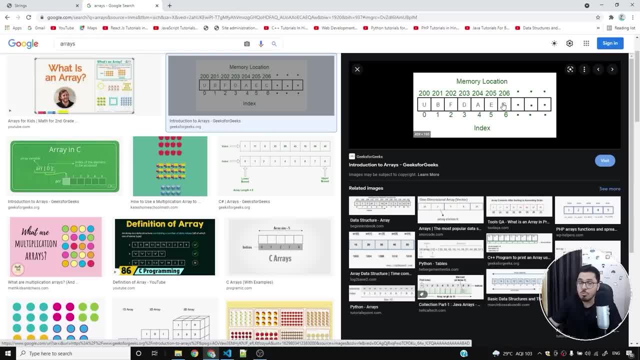 order to mark the ending point of the string. we say that wherever you encounter a null character which is backslash zero, the string ends there. so now we are going to see how to mark the ending point of the string. so let's say we are going to take a string that has a null character and we are 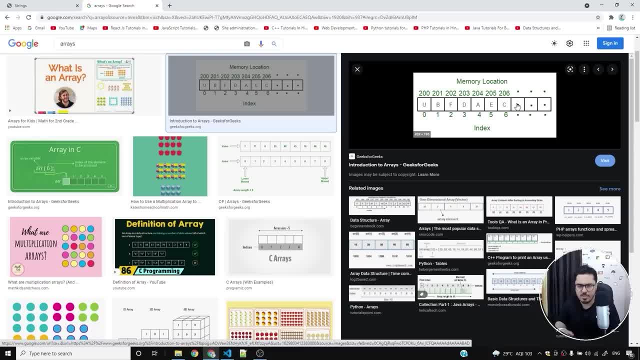 going to store it. so if, after c, i store a null character, which is nothing but a single character, backslash 0 is a single character. this is something that you need to remember. it is not two characters, it's a null character. okay. backslash 0 is one single character, uh, which is called a null. 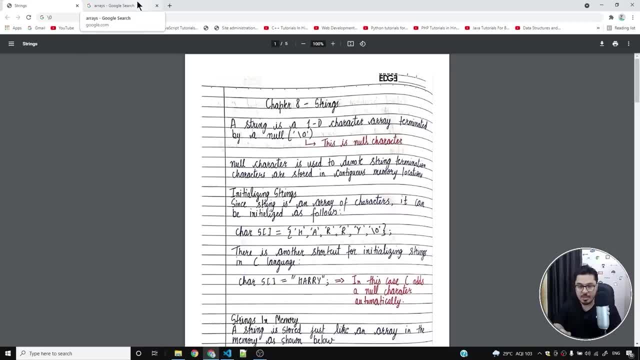 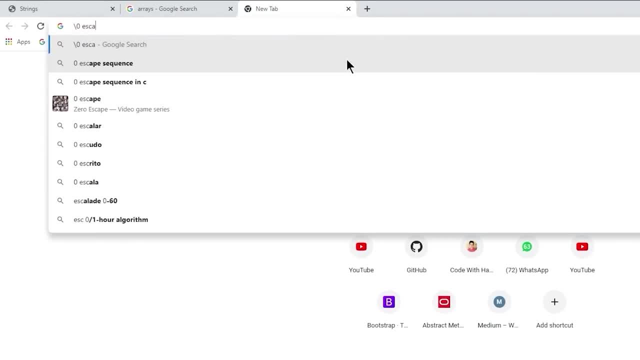 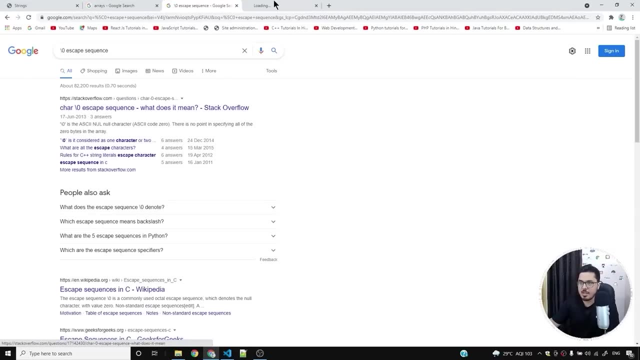 character. it's just that we need to type two characters in the keyboard to type this character. but it's actually an escape sequence character. uh, let me search this for you. uh, escape sequence. so what is backslash zero, escape sequence? let me also do this. so this escape sequence is a single character. it it is used to denote string. 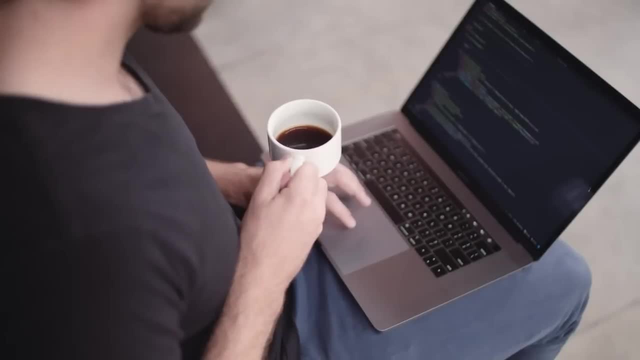 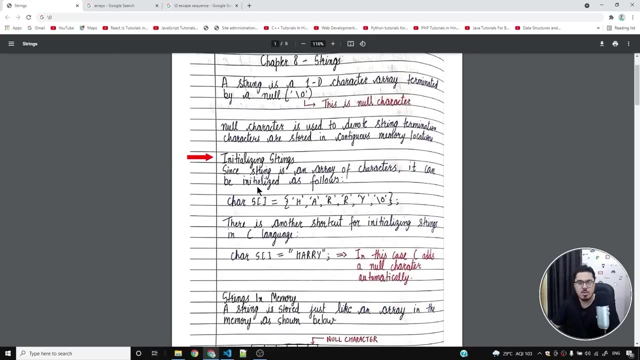 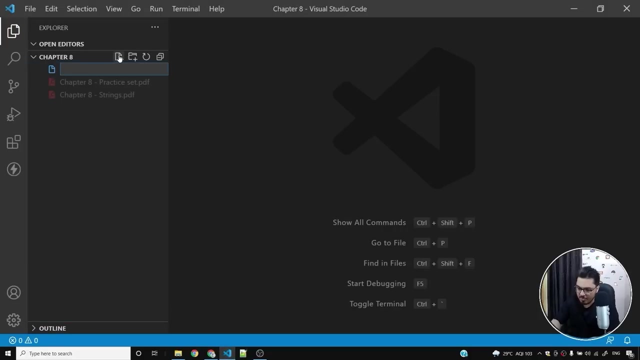 termination. okay, so i hope that you understood how this uh works. let's try to move further in the nodes and let's try to understand more on strings. since trick is an array of characters, it can be initialized as follows- and at this point i'll come to my visual studio code and 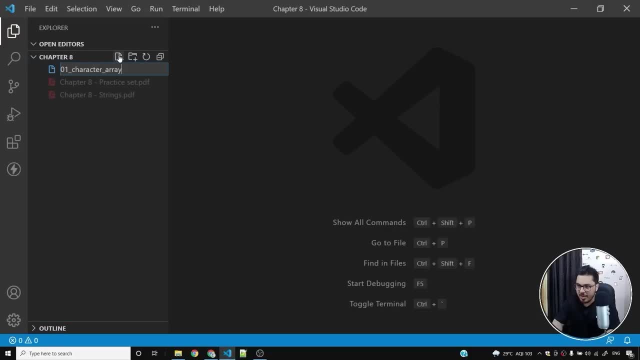 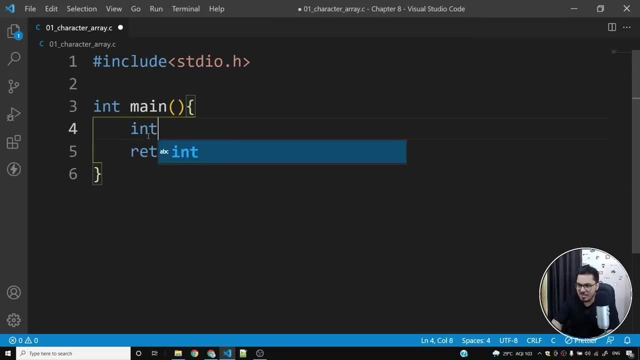 write the first program character underscore, array dot c. i'll put in the boilerplate code. i'll zoom in a bit and what i'll do is i'll simply say int, arr, or let me call it string, let me call it in str1. so let's say this is str1. so what i'm doing is: 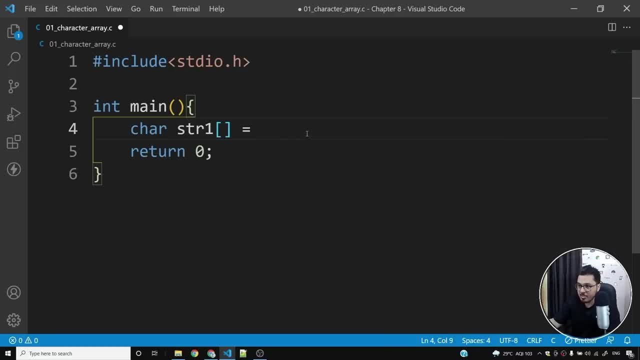 i'm saying: uh, sorry, i need to make it car, because string is collection of characters. so i'll simply say h, i'll simply say a, then i'll say r. make sure that you are using single quotes, because if you're not using single quotes, you're going to have to make sure that you're not using single quotes. 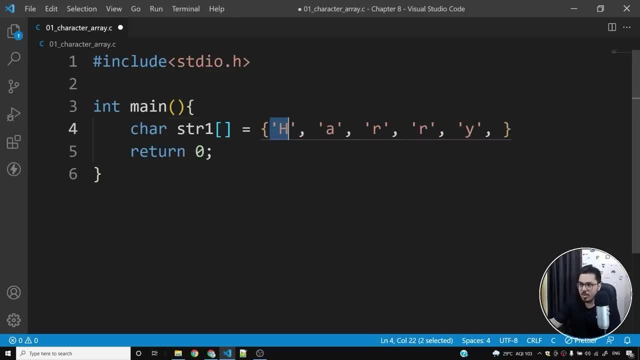 then, uh, it will not be a character. so in order to uh write a character literally in c, you need to use single quotes, do not use double quotes. if you're coming from a language like javascript, where single quotes and double quotes can be interchangeably used, do not get confused, right. 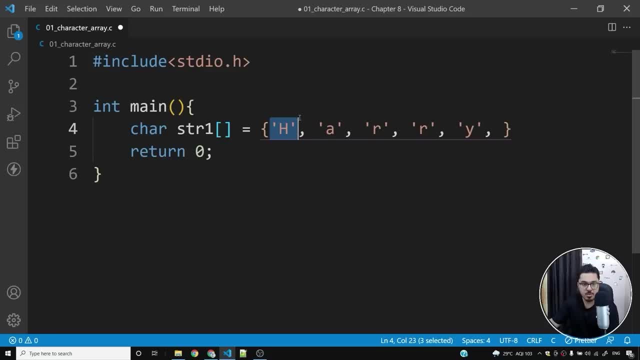 in c programming language you strictly use a single code for characters. okay, so h, a, r, r, y, and this is the last character. but no, this is not the last character. i need to write a backslash 0 to tell c compiler that my string has to be a double quote. 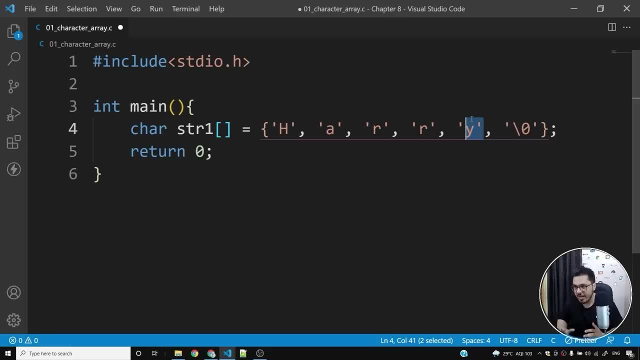 so the way we do that is, we free run mtls here printed string world to end foremult and then we have to read this: c would give us the background function for active backslash, to make sure that later we don't have to raise the number of characters come down and that we 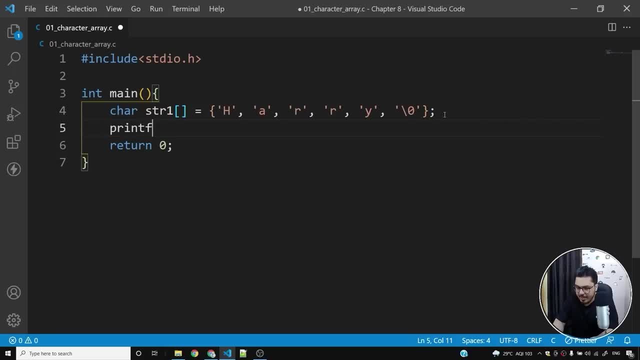 are finish mobile, etc. like that, if we don't want any chance for this to happen, like, let's say, we need 8 characters at our r1 and yes, i, i'll be able to print this string, so let me enable the extension. so i'll go to. 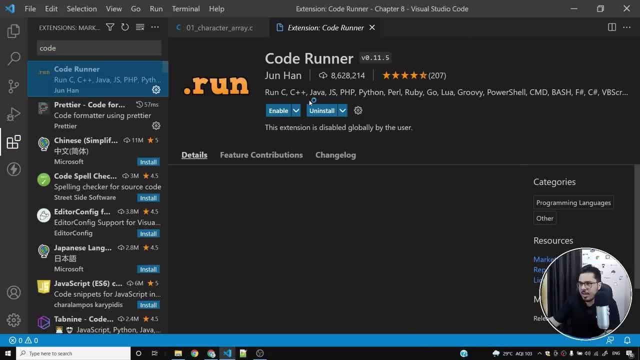 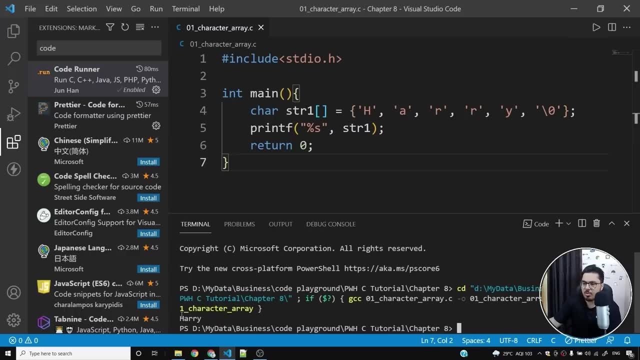 extension, i'll enable code runner by default. i have disabled code runner, so i'll simply enable it in workspace. if you can't see this run button, install this extension and enable it. you can see that harry has been printed on the screen. so this is how strings are represented in memory and this: 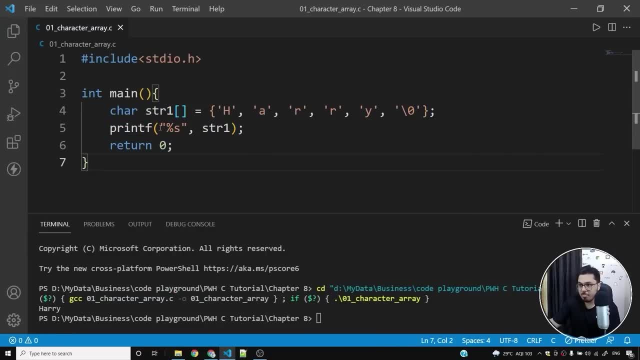 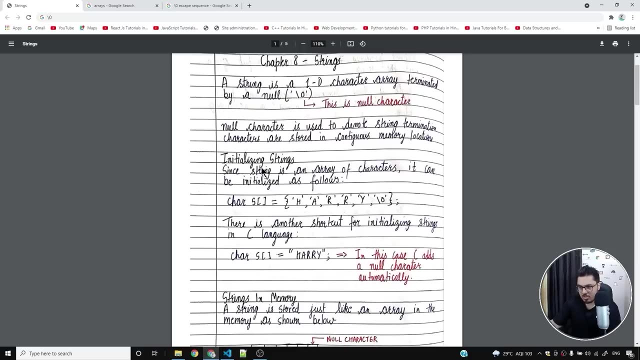 is how you can write a program to print a string. so percentage s is format specifier for strings. okay, let's move further in the notes. let's see what notes are saying. so, since string is, a is an array of characters can be initialized as follows. we just did that. there is another shortcut for. 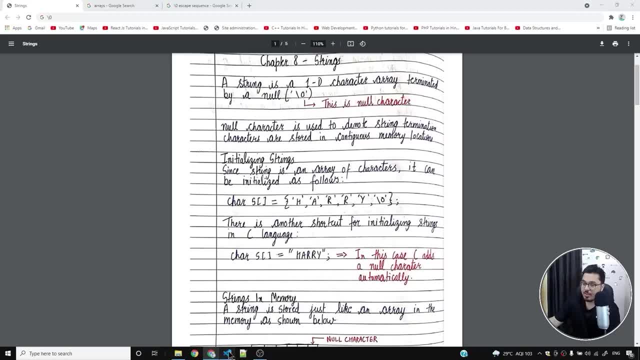 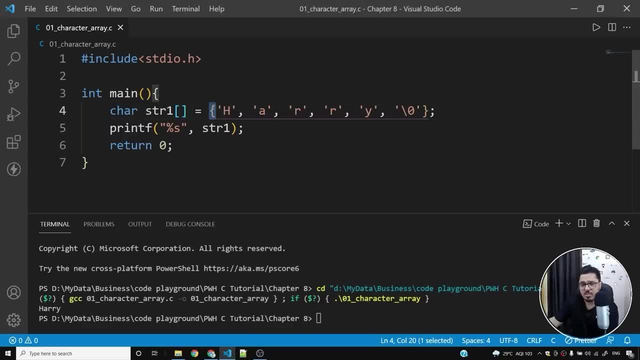 initializing strings in c language. okay, so this was a bit of a pain because we have to write single codes and then we have to write these curves brackets. yeah, this is a bit of a pain. so is there any shortcut to mark a string? can i not directly write harry? yes, there is a way. so in order to directly write harry, you can do something. 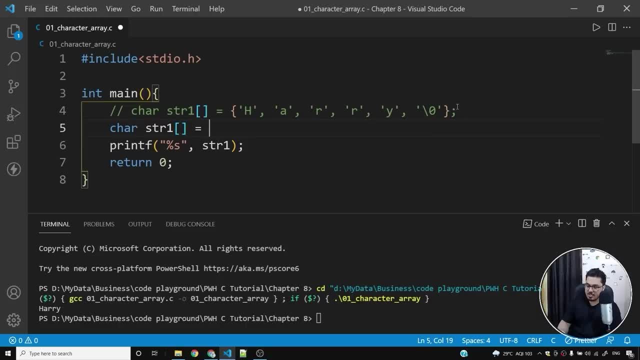 like this: you can say: int str1 is equal to double quotes, harry, and this will automatically add a backslash zero at the end, uh, or rather at the end of this character array. okay, not at the end of string, but at the end of this character array. so, uh, in the memory, this is: 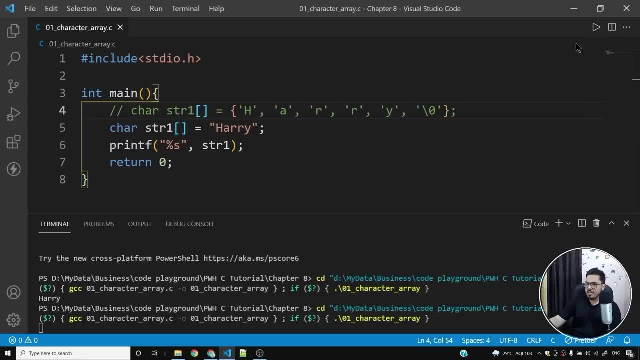 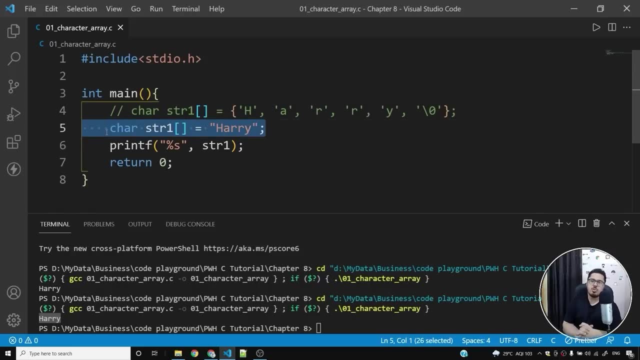 actually stored like this. so if i save this and run this program, i get the same thing which i got by running this. this is just a syntactic sugar. this is simply to make you love this programming language. uh, to make things easier for you, make sure that single quotes are used to mark a. 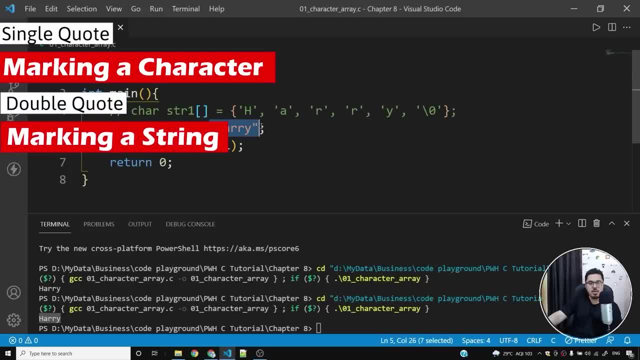 character and double quotes are used to mark a string. so this is how double quotes are used to create strings. so let me move further in the notes once again, basically what you we wrote: traditional MA2 strings and, whereas string, character, string- are used to create strings. so you should notice that character. 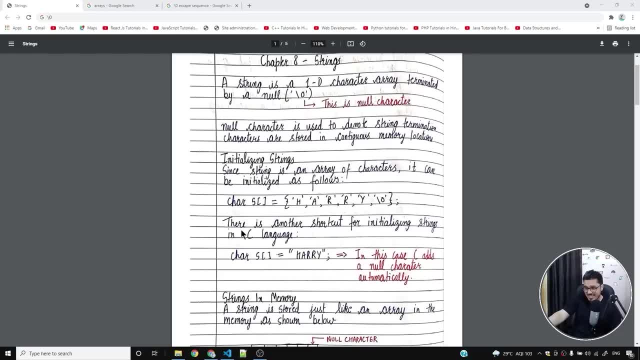 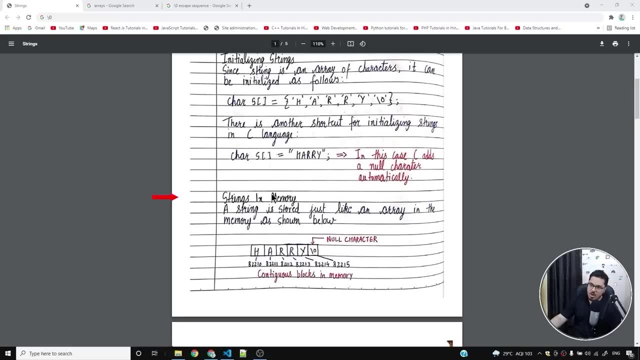 move further in the notes and let's see what else is there. so there is another shortcut. we just talked about this- and in this case c adds another character automatically. now let's see how strings are represented in memory. so one byte is one character. in fact, one character is one byte, and 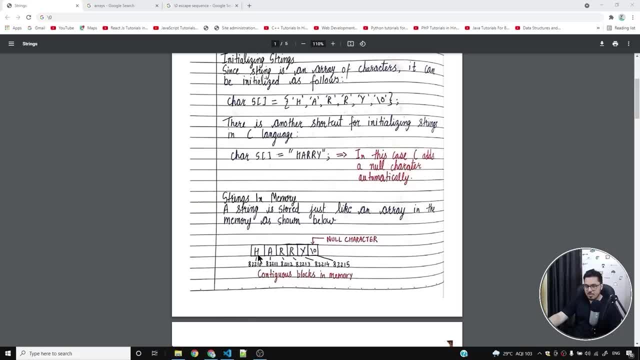 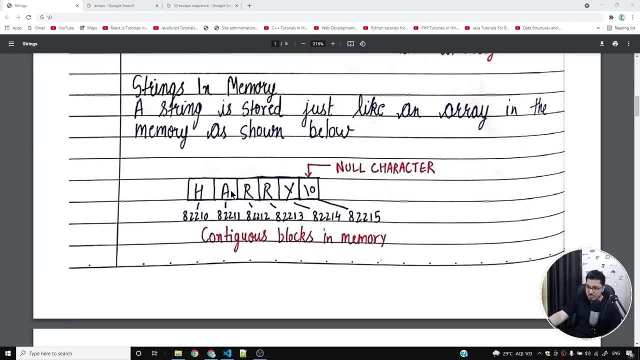 one character just needs a single byte in memory. so memory locations are contiguous blocks of memory when we talk about strings or character arrays. so what happens is, if i want to store harry, i will simply say h a r r? y and at the end will be a null character to mark the termination. 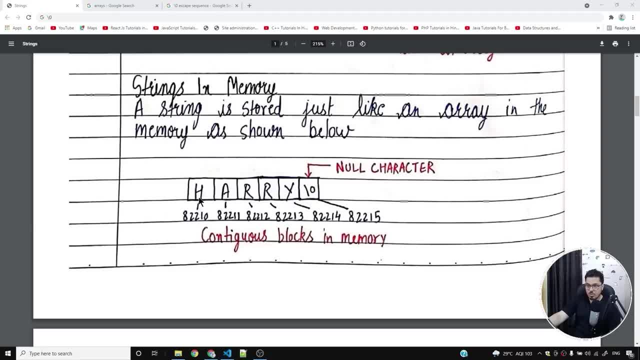 of this string. so if the memory location of h is 8, 2, 2, 1, 0, the memory location for a will be 8, 2, 2, 1, 1, and so on. so the next memory location is previous memory location plus one, because 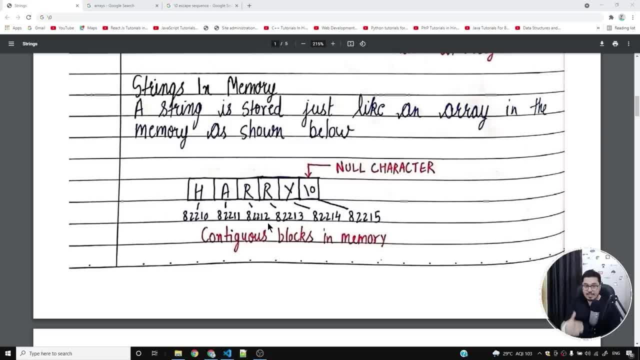 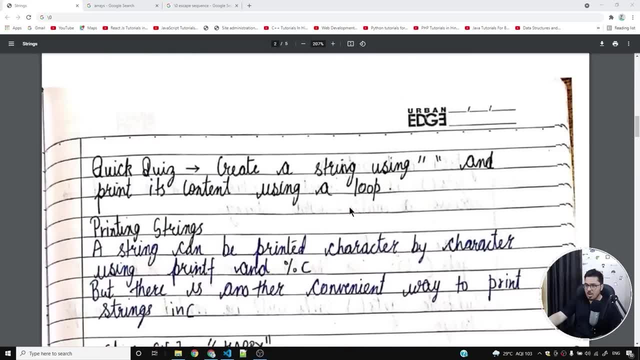 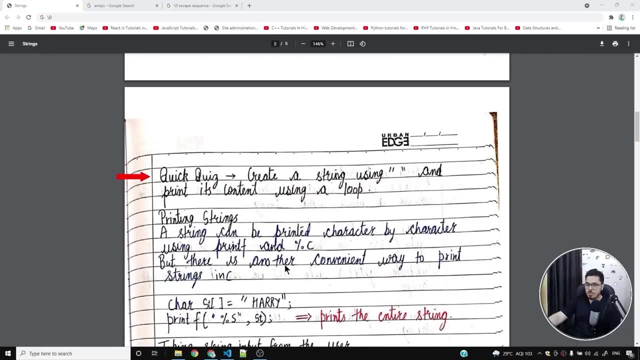 string contains characters, and character takes single byte of memory. so this is how strings are stored in memory. really straightforward, you? let's now talk about this quick quiz where we have to create a string using double quotes and print its content using a loop. so this quick quiz contains a bit of a catch. i mean, you don't have to. 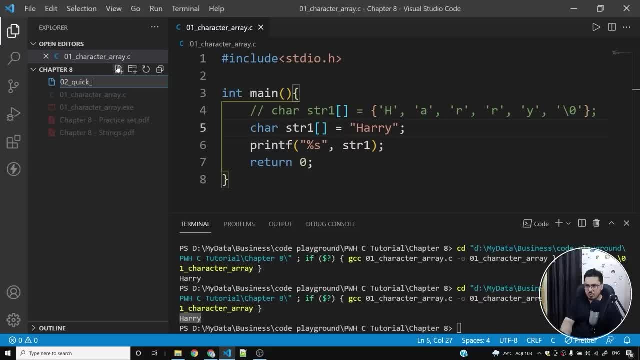 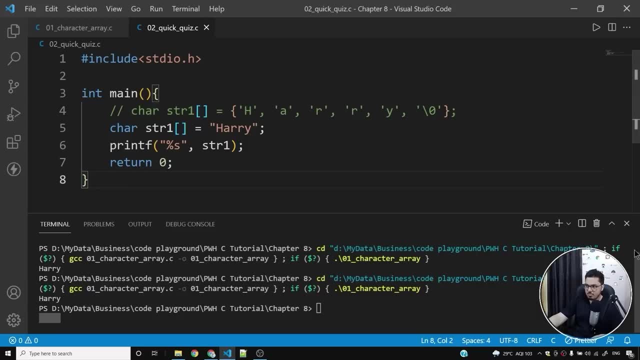 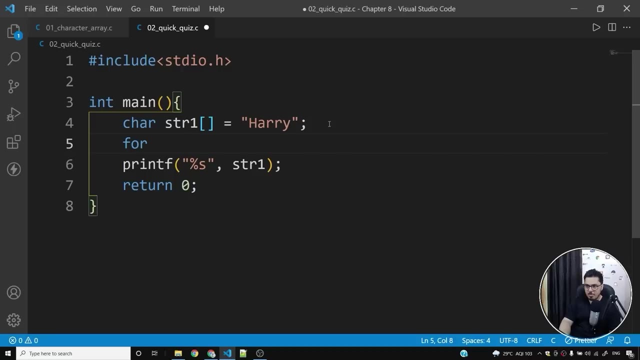 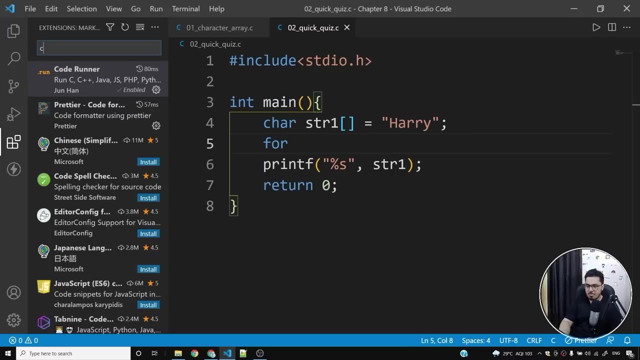 use percentages. uh, let me say quick, underscore quiz dot c, so you can easily print a string by using percentages. we just saw that. but this question demands you to print the same string using a for loop, because we know that deep within this particular, let me enable the extension c plus plus. 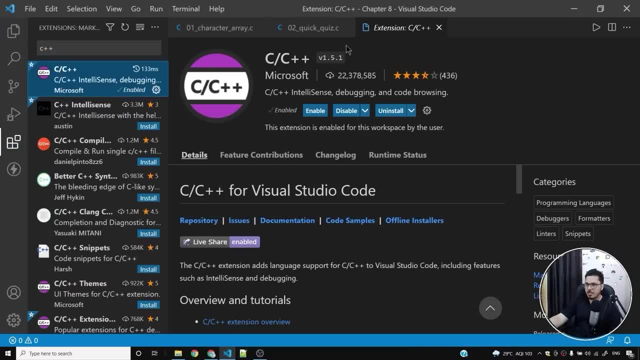 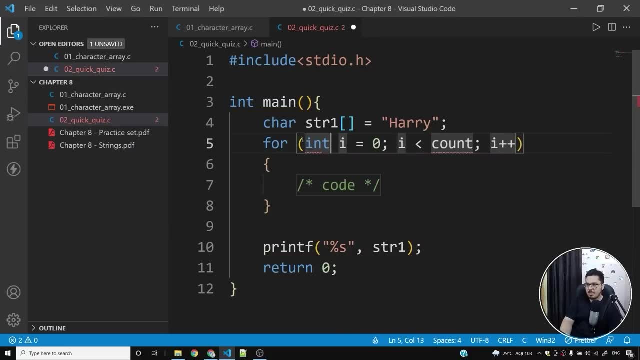 so c, c plus plus intellisense. this was not enabled. now it is enabled, so i can use the snippets. so what i'll do is i'll use this snippet for for loop and i'll say int i. int i is less than length of the string. what is the length of the string? i know that length of the string is six because um. 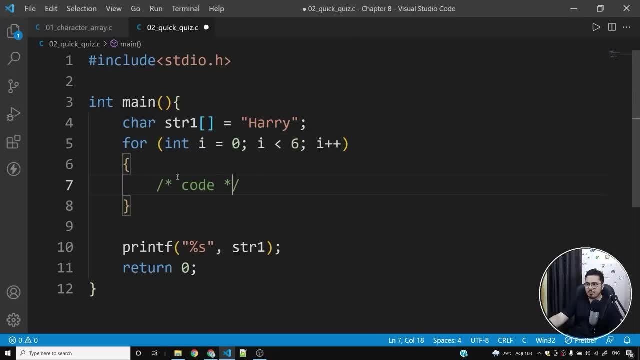 five for the characters, one for the null character and the index will go from 0 to 5. now what i can do is i can do something like this: printf, percentage c for character and i can say str1i. this will print the string, sorry, the character. so this: 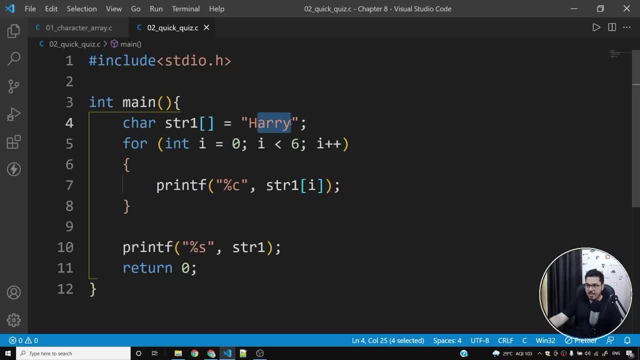 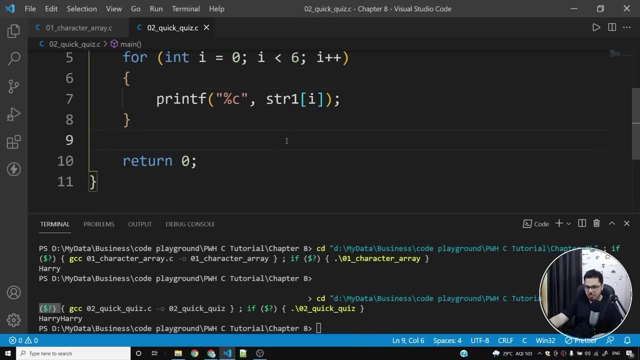 will first print h, then a, then r, then r, then y and then the null character. so let's see how this works. so, uh, oops, i i need to remove this. so if i run this, you can see h then a, then r, then r, then y. 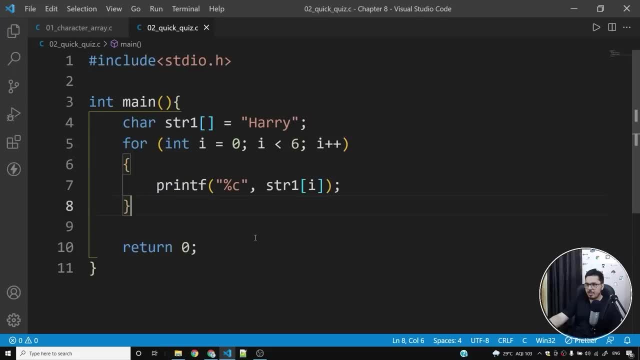 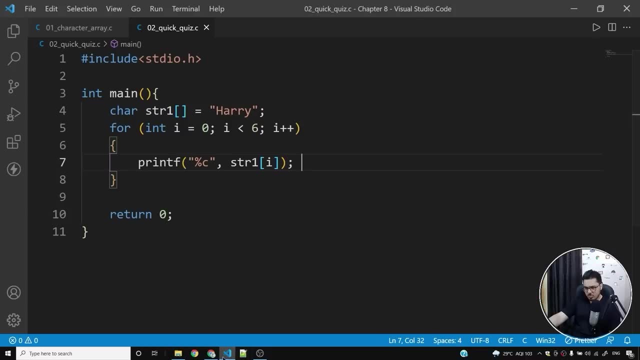 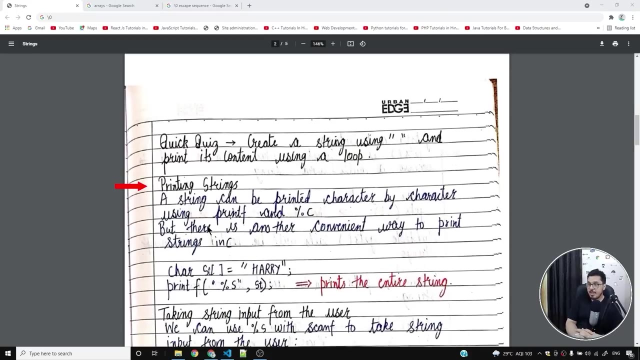 has been printed. so this is how the string is printed. so h a r r y has been printed and, finally, the null character is printed. so this is how you can, you know, solve this question. now let's see how strings are printed. i just told you how strings are printed. a string can be printed character by. 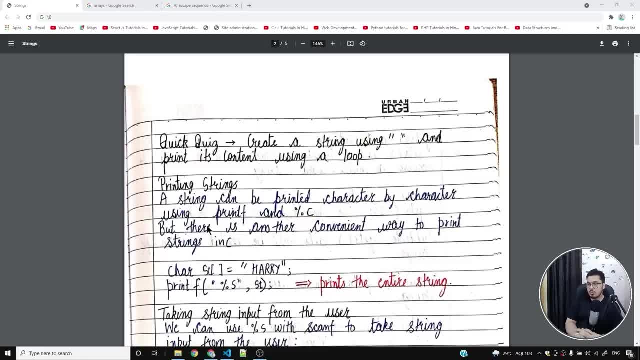 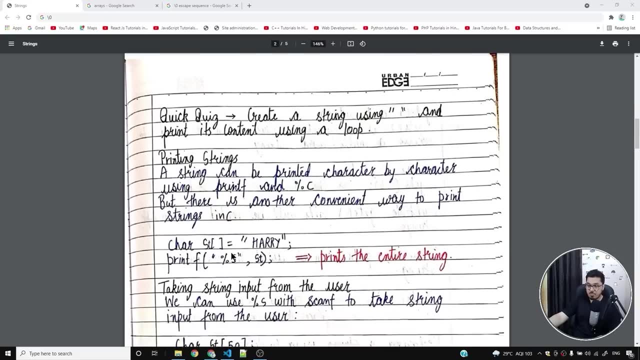 character using printf and percentagef: percentage c. so percentage c is the format specifier for printing a character. you can print it character by character using percentage c. so percentage c will print one single character. but there is another convenient way to print strings in c, which is percentages. we just saw. 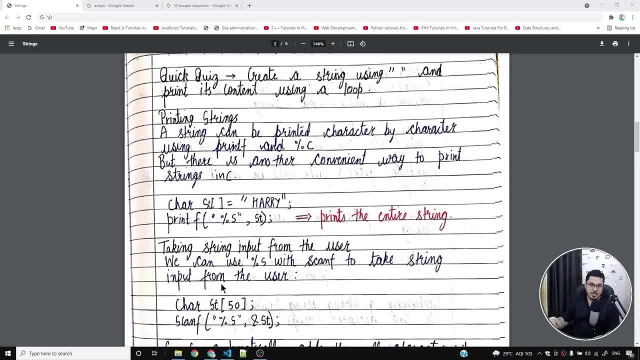 that okay. so you can either print a string character by character, by iterating this array. at the end of the day, string is an array and you can also use percentage s if you want to give the address s s s of first element of the array, which is st in this case. so this will print the entire string. 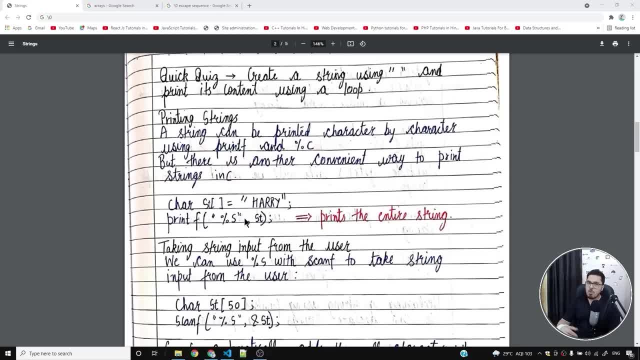 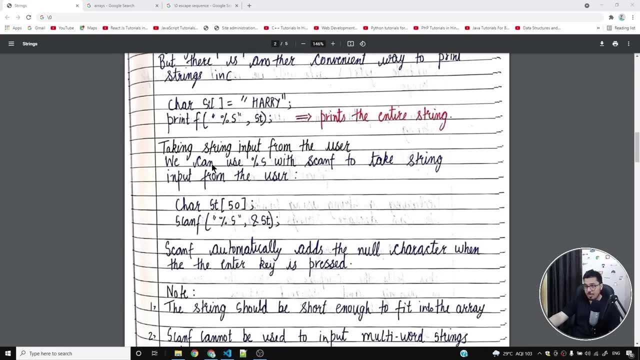 how this works behind the hood is this will simply keep on going to the next character, next character and so on, until it encounters a null character, which is backslash zero. so i hope that you understood how strings are stored in memory and how to print strings in your c program. now let's 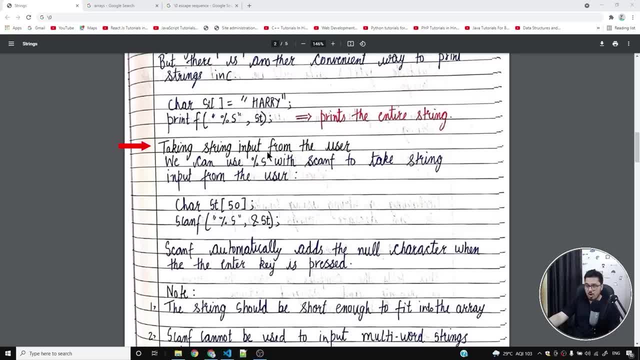 move to the next topic, which is taking string input from the user. how do you take string input from the user? taking string input from the user is really very easy. all you need to do is use percentage s as the format specifier and you can use scanf so this particular character array. can store 50 characters, but you can create a string of length 5, 6, 7, 34, 30. it will be working fine as long as the number of characters in your string are less than 50, because this particular array can hold a maximum of 50 characters. 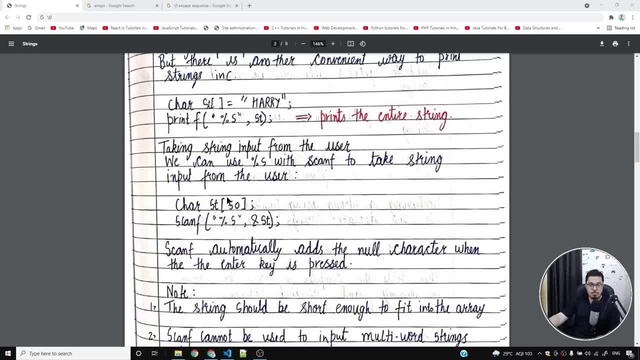 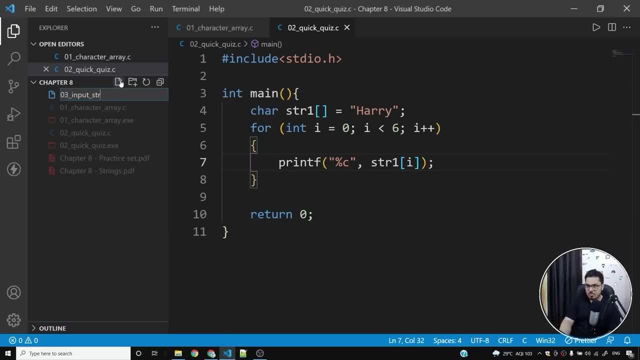 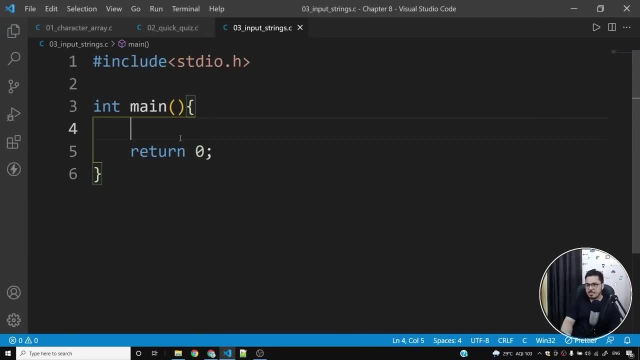 you including the null character, so this is something that you need to keep in mind. so let's take input from the user input strings dot c. i'll put down the boilerplate code and i will say char ch1 and let's say the max, the max limit of holding characters for this. 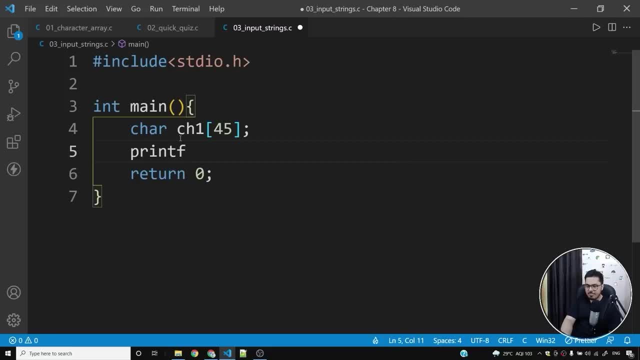 character array is 45. i'll write a printf here. i'll say: enter your name. okay, enter your name and see the magic. and also i will write backslash n. now what i'll do is i'll simply write scanf and percentage d- sorry, percentage s- and i'll say ch1. now i can print the string. 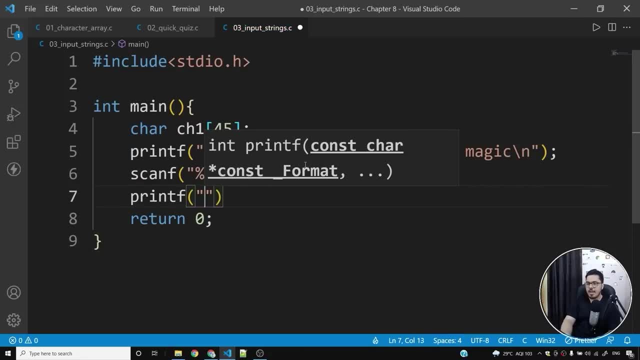 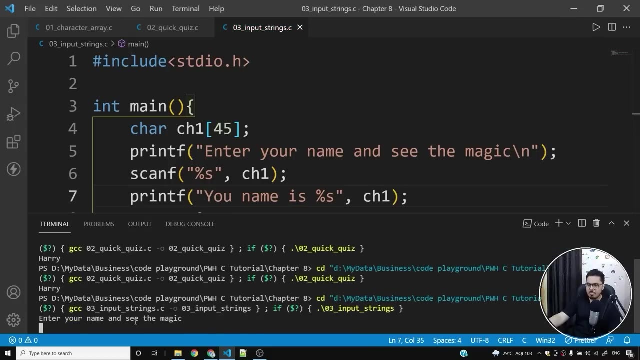 using printf once again and i can do something like this: your name is percentage- oops, your name is percentage s and ch1 and then if i save this program and show you, it is saying: enter your name and see the magic. it says your name is harry, so 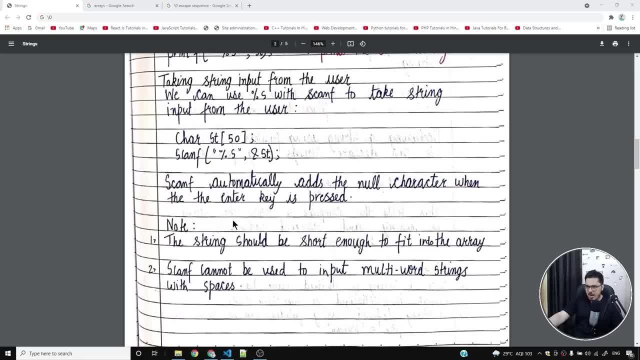 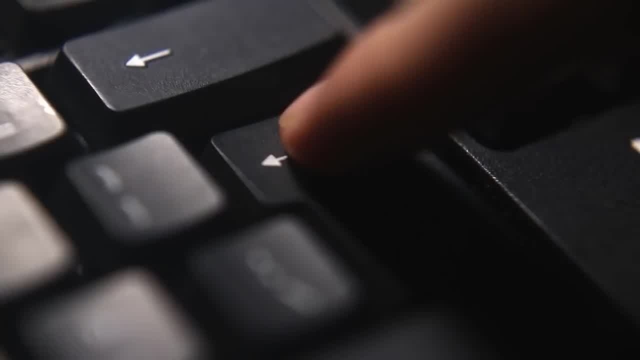 this is how this program works. let's now move back to notes and read more on it. scanf automatically scans uh, add signal character when the enter key is pressed. so the moment you press the enter key, scanf will automatically add the null character. now there are two notes that i've written here. 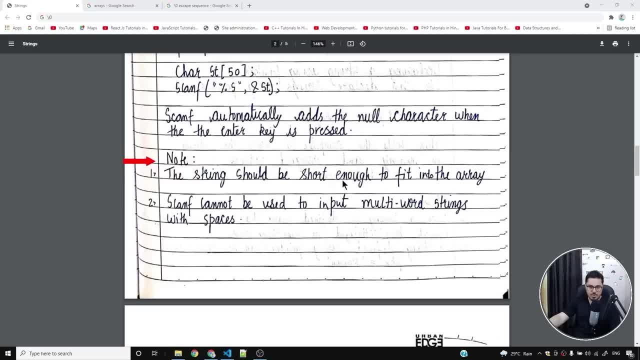 the string should be short enough to fit into the error. this is something that you need to make sure. sometimes he will not throw any error, but your program will not work as expected. so do not wait for the error. you might not get the error. you might have, you know, reached a memory location. 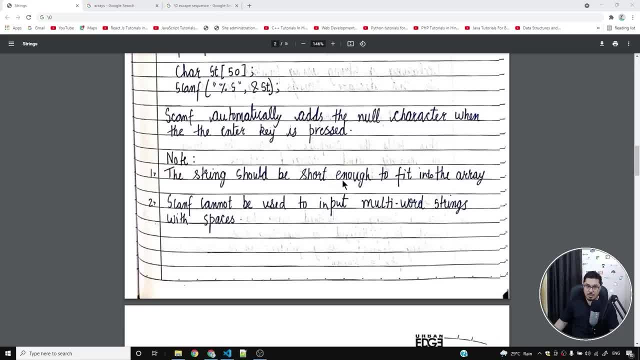 which you are not allowed to reach and maybe due to that, you might get some error. do not wait for that to happen. rather, make sure that you are able to hold the number of characters you intend to hold. okay, so scanf cannot be used to input multi-word strings with spaces. you cannot use scanf to input multi-word strings, and i'll show. 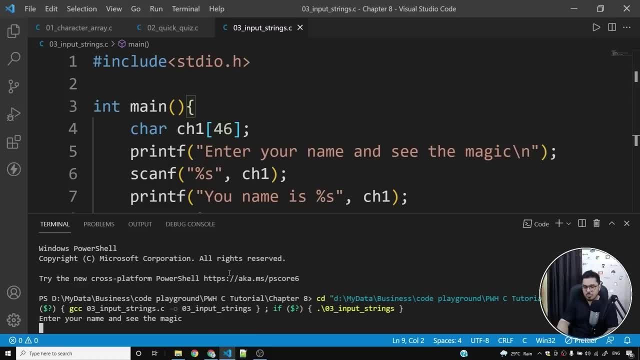 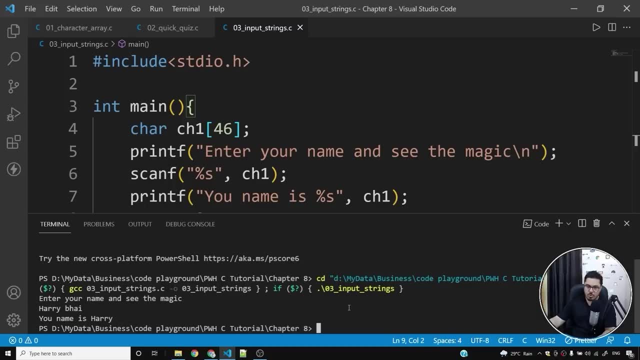 you an example. so if i run this program and let us say i try to say harry by, you can see that your name is harry is printed and not harry by. so what i want to do is i want to also make sure that the string is entered correctly. so the thing is the moment scanner sees a space, it will actually. 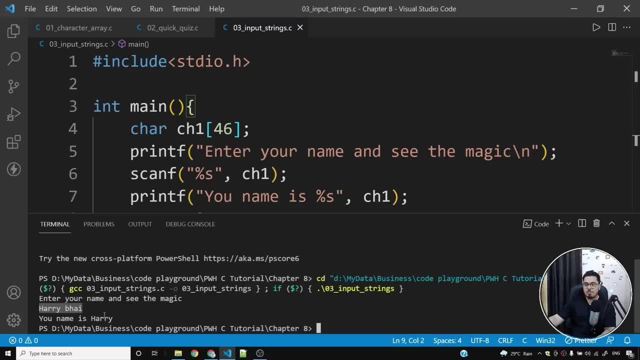 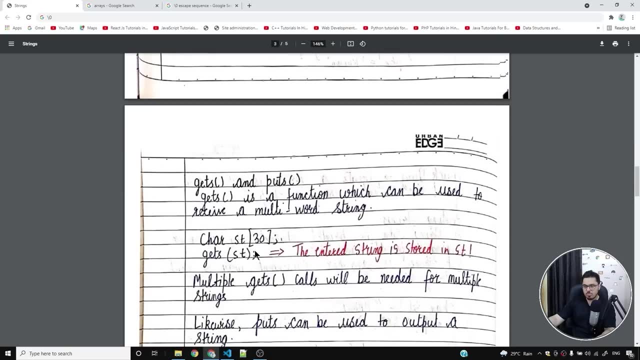 think that you are done entering the string and you will not be able to, uh, print your string or store the string. uh, as is okay. so what is the solution for that? we'll see the solution for that, and the solution for that is gets and puts. so gets is a function which can be used to receive a. 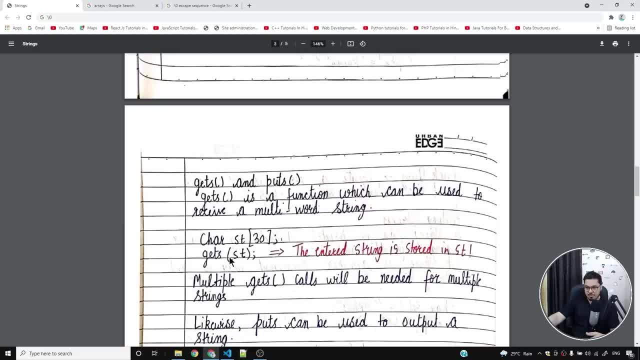 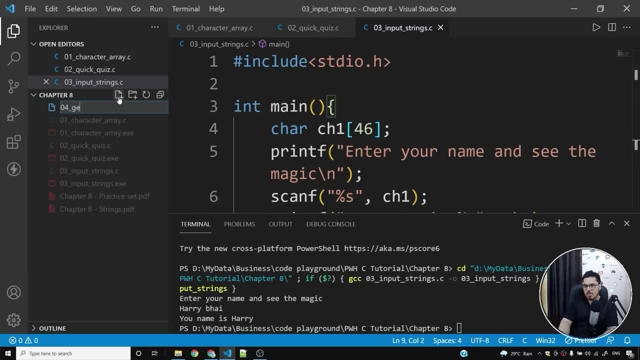 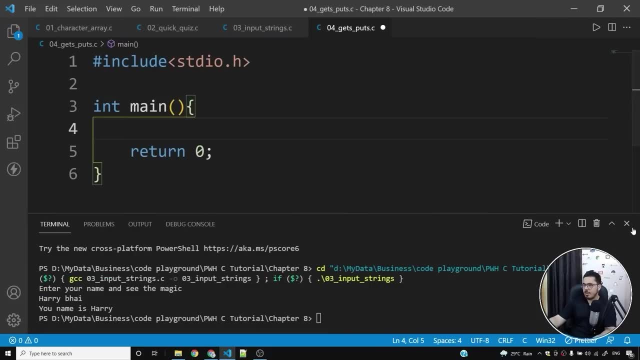 multi-word string. so if you want to receive a multi-word string, do not use scanner, rather use gets. so I'll name it 04. underscore: gets puts dot C. I'll put the boilerplate code here. I'll close this And also what I'll do is I'll simply copy this program. 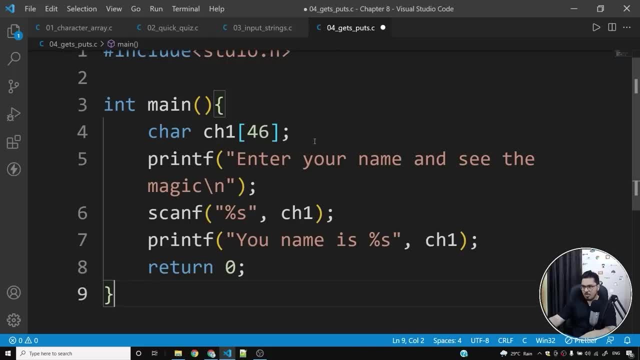 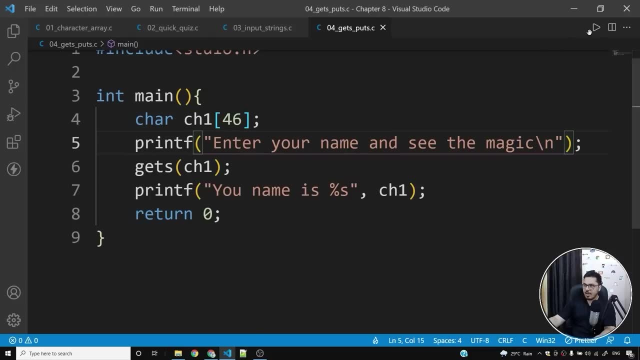 I'll copy this program as is And I'll change this canf call to gets call. Can I now add a multi-word string? I'll say multi-word string. yes, it works. So I can use gets in place of scanf if I know or if I suspect my string to contain one space. 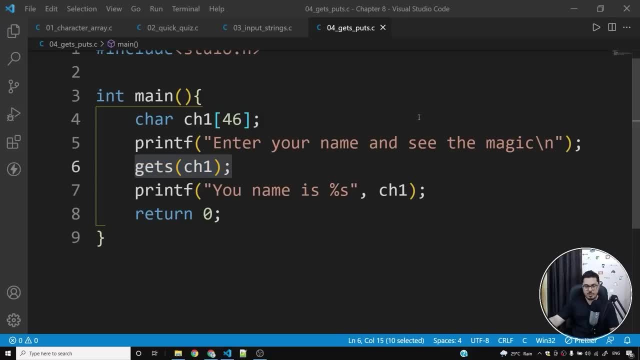 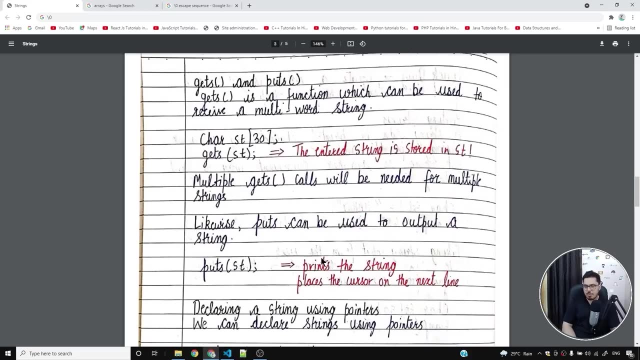 or more than one space. So if you think that your input string might have spaces in it, you might consider using gets. Coming back to the nodes, gets is a function which can be used to receive a multi-word string. So this is a very basic function. 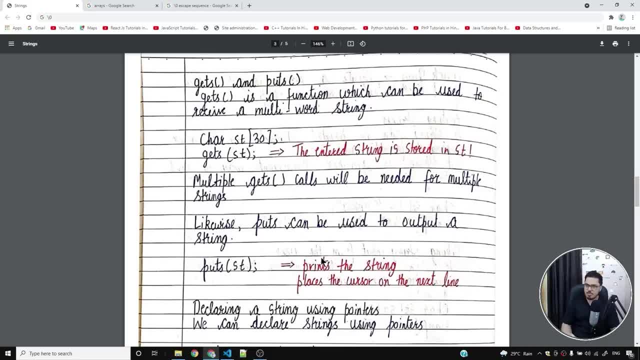 It can be used to receive multi-word string. There is an example here: The entered string is stored in st, So st is a character array, And gets will make sure that, even if your input contains a space, your string is stored in the appropriate place. 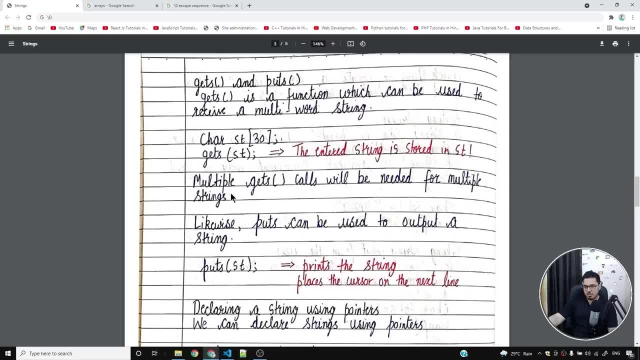 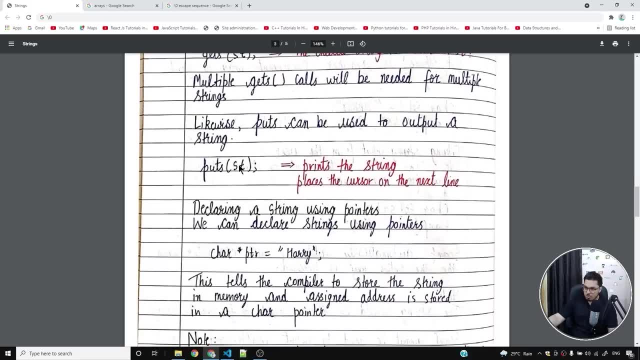 Multiple gets calls will be needed for multiple strings. So if you want to store multiple strings, you need multiple gets calls. Likewise, puts can be used to output a string. You can use puts as well to output a string. Prints the string places the cursor on the next line. 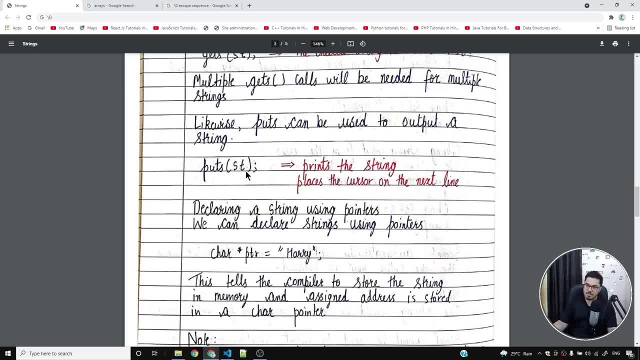 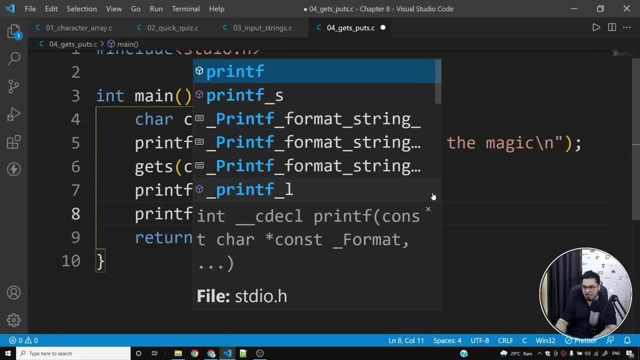 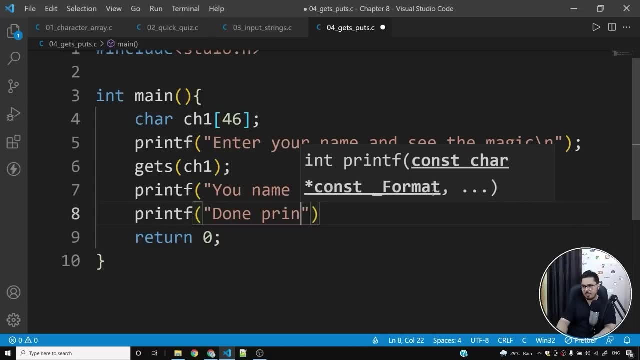 So puts will print the string first And then it will place the cursor on the next line. I'll show you. So there is a difference between printf and puts. So I'll show you This was using or, let me say, done, printing string. 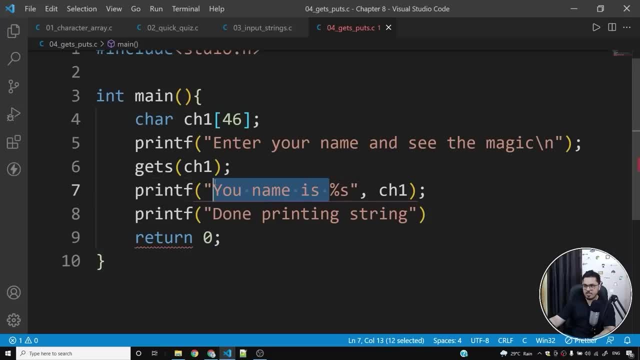 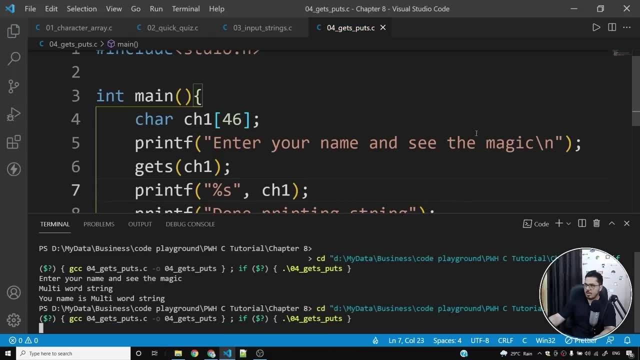 So if I'm using printf to print the string, let's just print the string and not print the name is So I'll save this program. I hope that this will work. I just placed a semi-colon. I'll say: hey, hi. 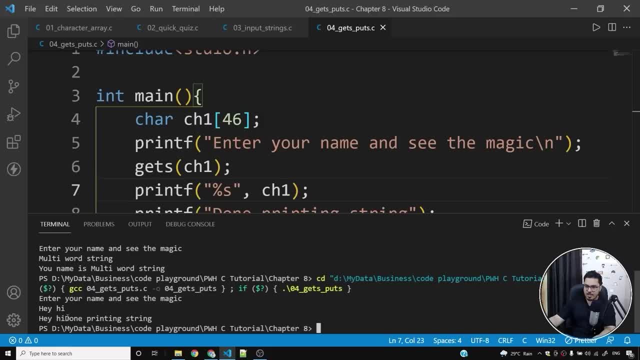 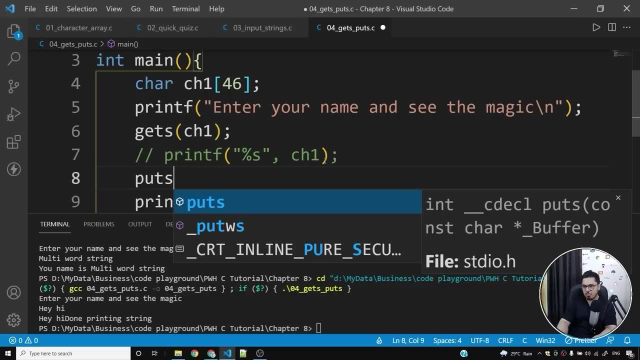 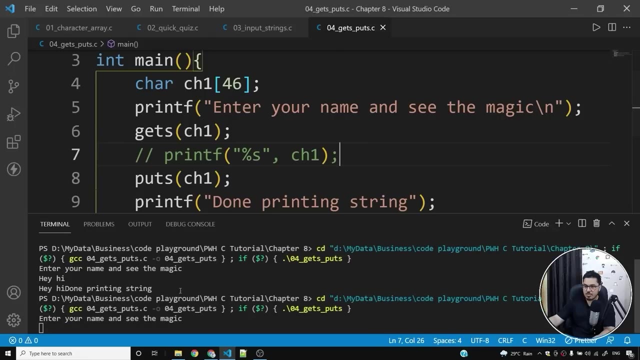 Hi. So you can see: hey, hi, done printing the string. There is no new line here. But if I use puts, let me show you how puts works. I'll simply say ch1.. If I use puts, the cursor will be placed on the next line. 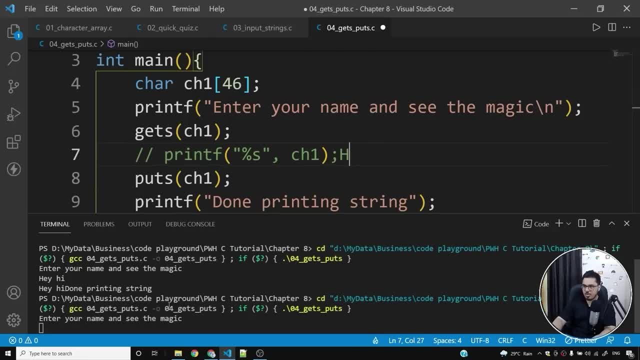 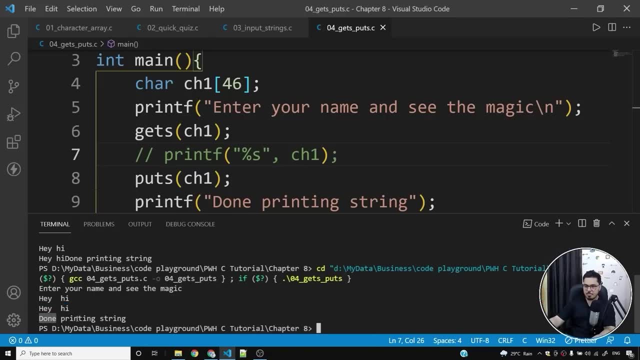 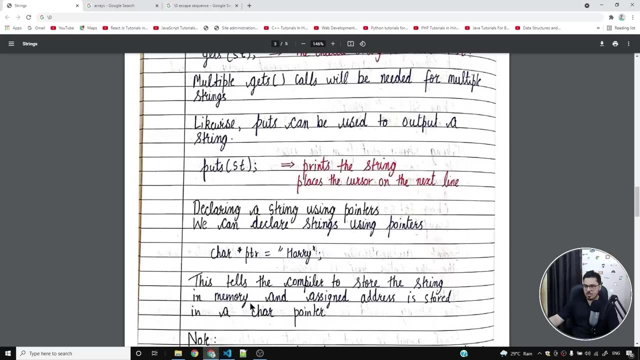 So if I say hey, hi, oops, you'll see that hey, hi, and then done printing string is placed on the next line. So this puts call will simply place the cursor on the next line. So I hope that you understood what is the difference between puts and printf. 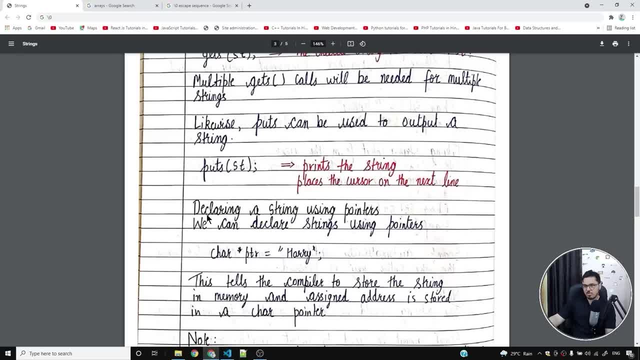 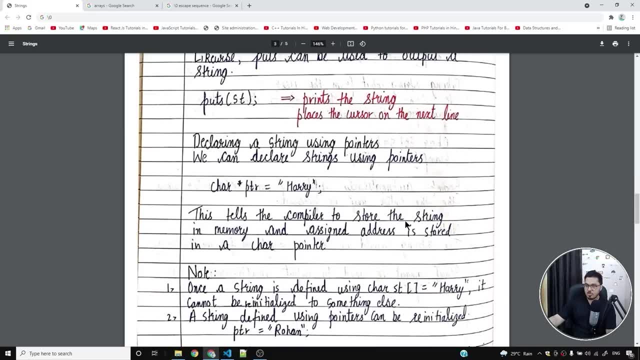 Now declaring a string using pointers. this is important So we can actually declare strings using pointers like this. we can say: char star, ptr is equal to Harry. This tells the compiler to store the string in memory and assigned addresses stored in a character pointer. 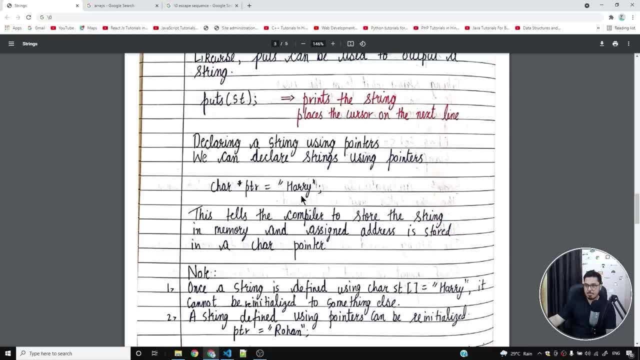 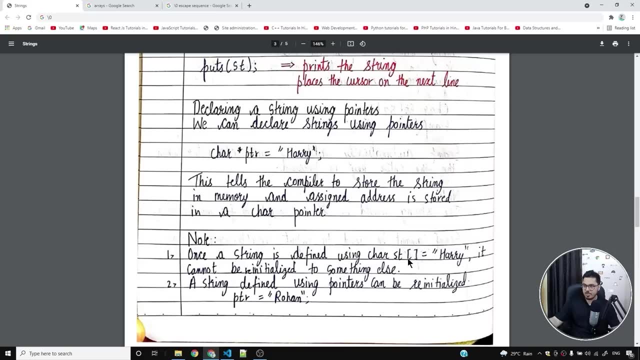 So this will actually find some space in the memory And it will the address of the first character to ptr. so ptr will hold the address of h. okay, i hope that you understood this syntax as well. now, once a string is defined using this, it cannot be re-initialized. 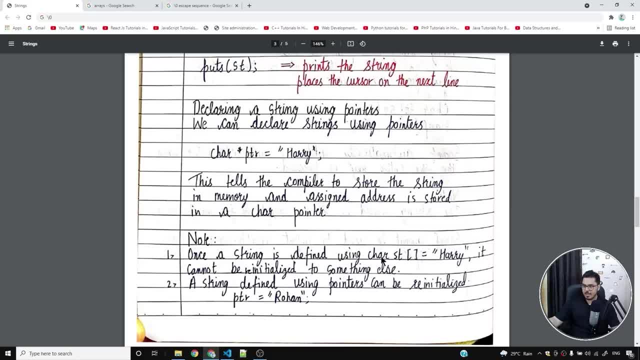 to something else. so if you do something like char st is equal to harry, you cannot change this string. but a string defined using pointers can be re-initialized. you can say ptr is equal to this, or you might want to change it to something else. so this is something that you need to keep in your 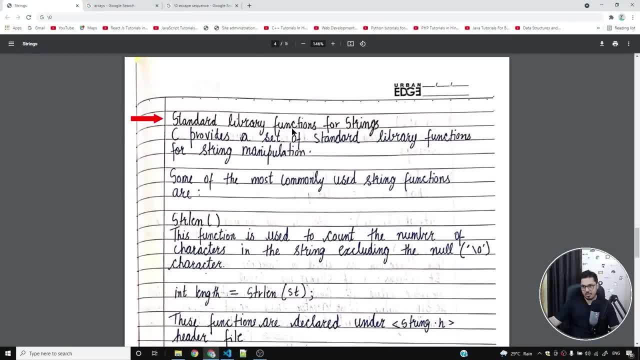 mind now standard library functions for strings. now c provides a set of standard library functions for string manipulation. you might write your own functions to manipulate your strings but sometimes that might get cumbersome. so there are some standard library functions for string manipulation. we'll look into all those standard library functions, some of the most commonly used. 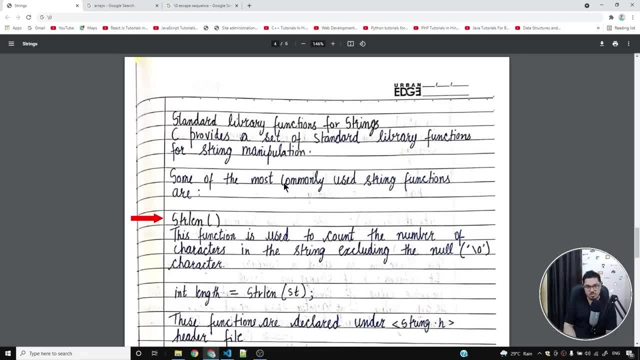 string functions are strlen, which will simply give you the length of the string. you might want to implement your own strlen, which will simply scan your character array and it will keep on counting the number of characters until a backslash zero is encountered. okay, so you can do that, but again, there is a built-in function, so this function is used to count the. 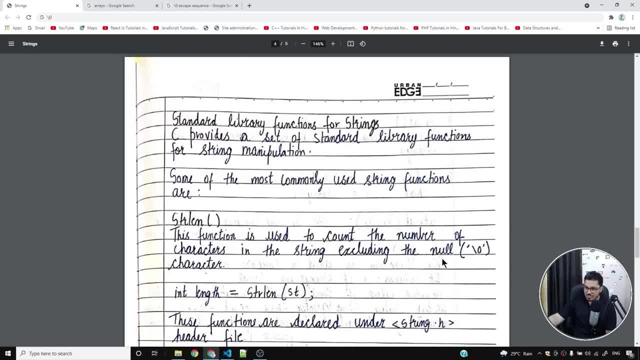 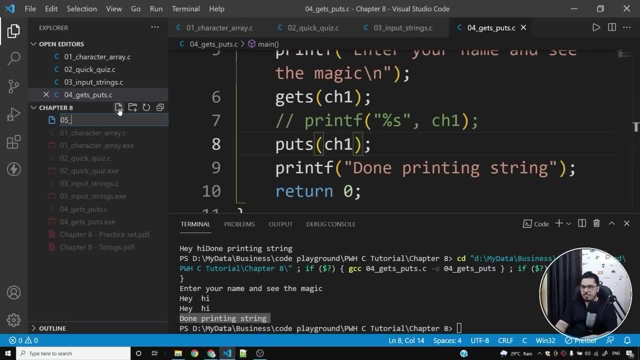 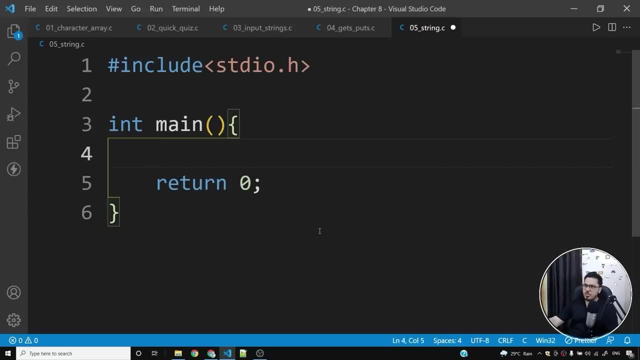 number of characters in the string, excluding the null character. so let me show you. so i will simply create a new file. i'll say zero, five underscore, string dot c, and what i'll do is i'll simply put down the boilerplate code and also i will. 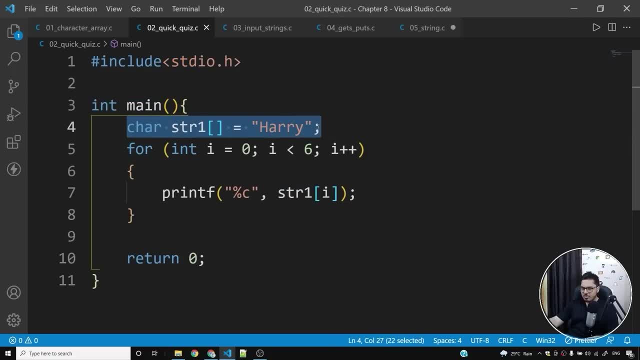 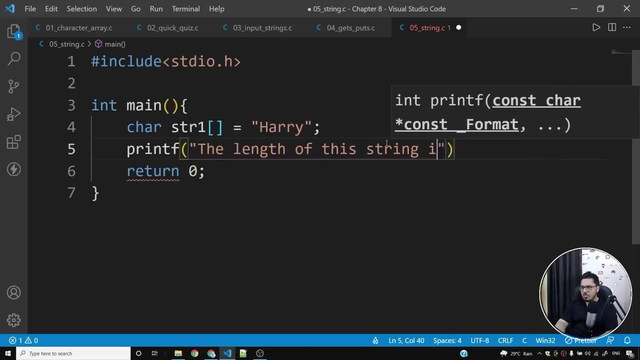 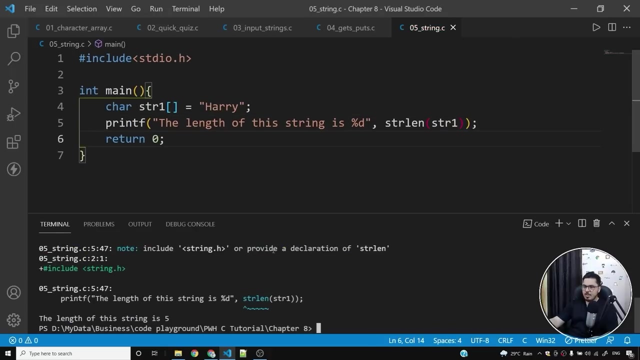 use this syntax to initialize my string. now what i'll do is i'll say printf- the length of this string is percentage d- and i'll say strlen- str1. so this should actually give me the length of the string. so if i run this program, i am getting a warning. it's telling me that please include this library. 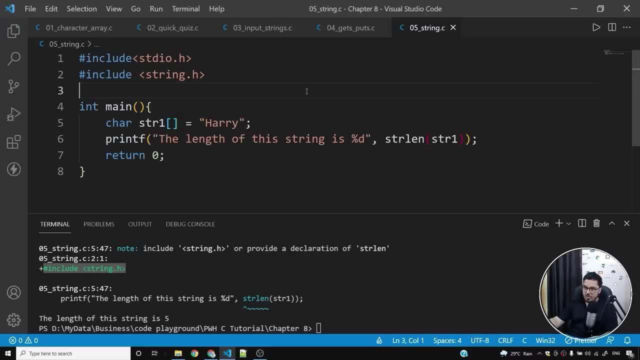 this header file. so i'll include this header file, which is stringh. in order to use string methods, you need to include this header file which i've just included. this is just a warning. your program still works. you can see. the length of the string is five, but again, it's a good practice to add. 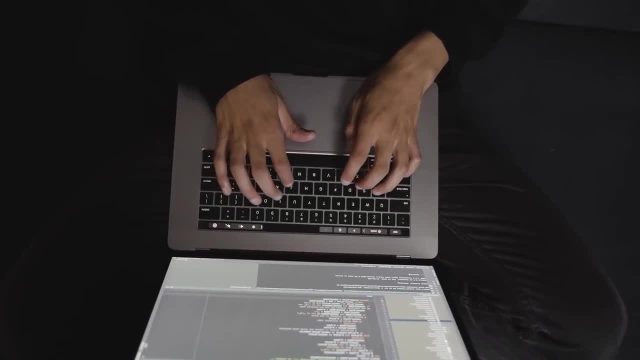 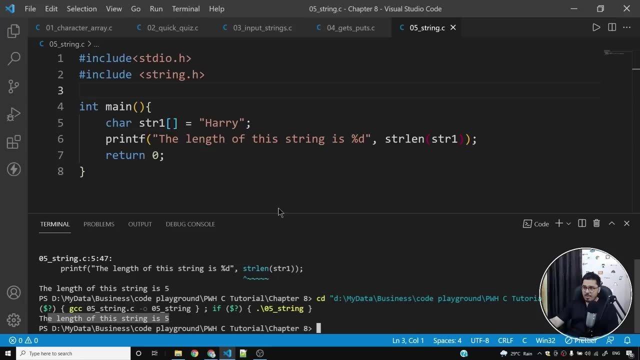 the header file when you are working with string functions. so the program compiles without any errors and warnings. you can see the length of this string is five. what if i change? change this to harry with with a double y, you will see the length of the string is six. so in this case, the length of 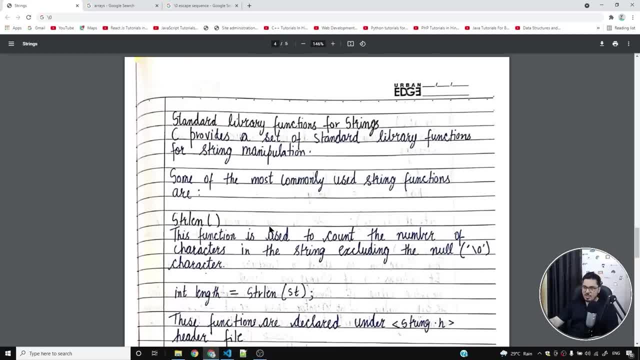 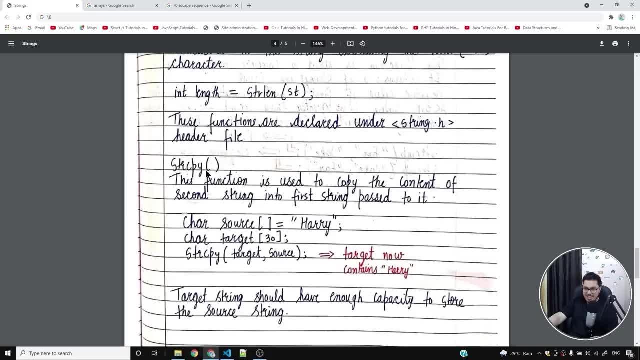 the string is six. i hope that you are able to understand how these things are working. now let's talk about the other function, which is str cpy. this function is used to copy the content of second string into the first string passed to it. so if i have, source is equal to harry and i click. 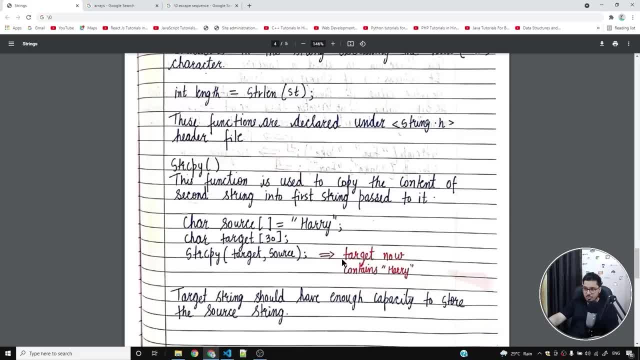 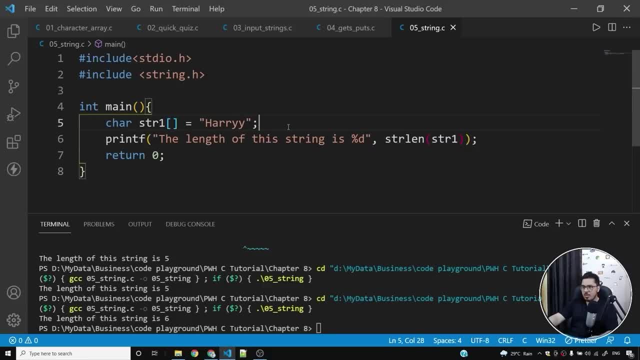 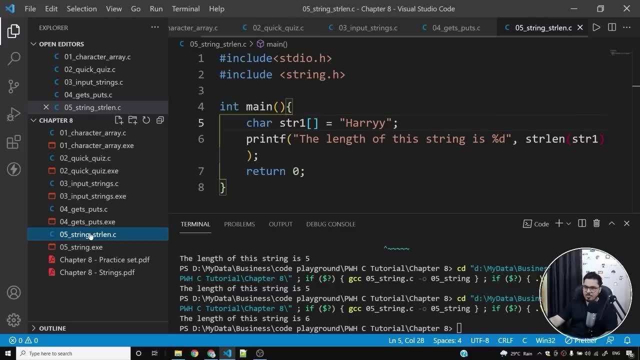 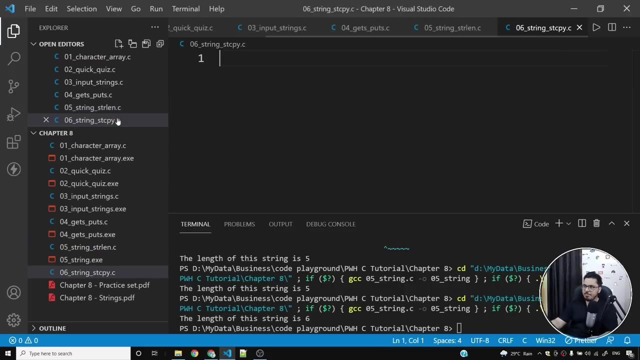 create a target. i can actually run strcpy target source to make target hold harry. let me show you. so i'll create another program. i'll say a string strlen. i'll create another program, 06 underscore, string strcpy, and i'm not going to type everything once. 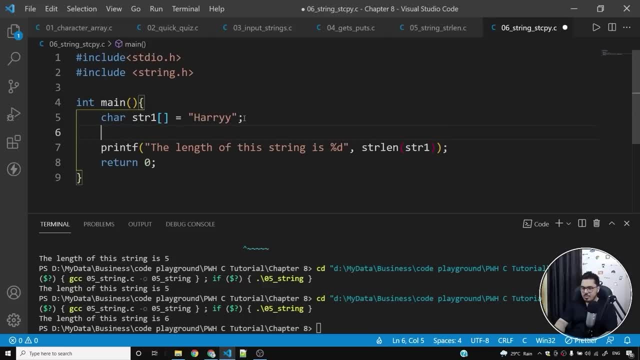 again. i'm going to copy this from here. so i'll now say char- target and let me create a target string with length 45. let me call this source and let me do something like this. what i'll do is i will say strcpy and i'll do target and source. did you notice that when we didn't add the header? 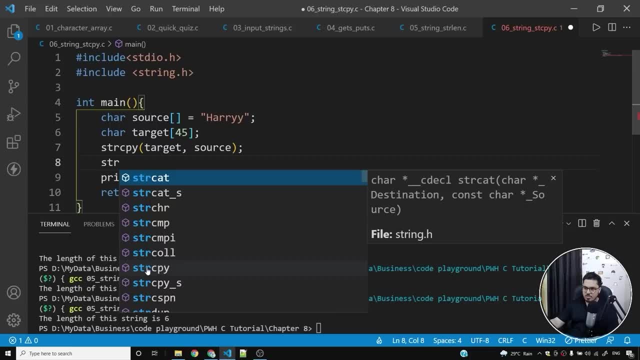 file. we were not getting the suggestion. now, if i write str, i'm getting all these functions, so i'm going to copy this from here and i'm going to create a target string with length functions in the suggestion. so this is also one of the reasons to include the header file. 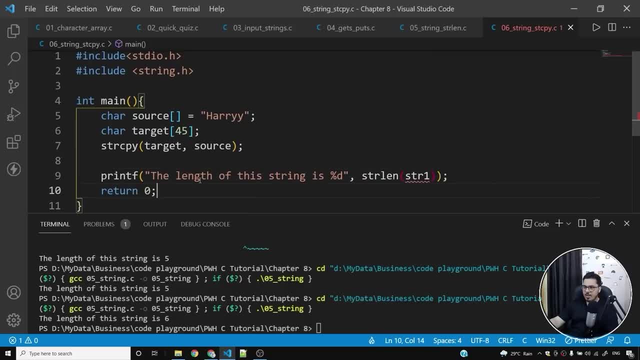 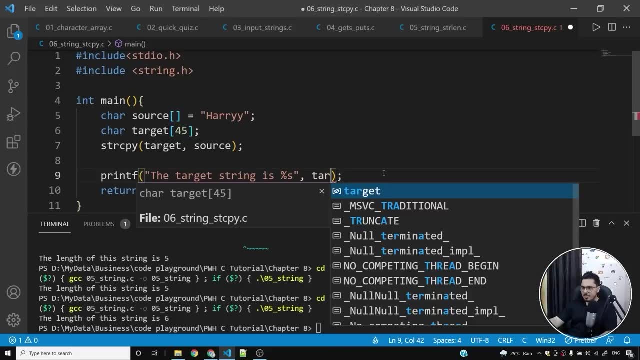 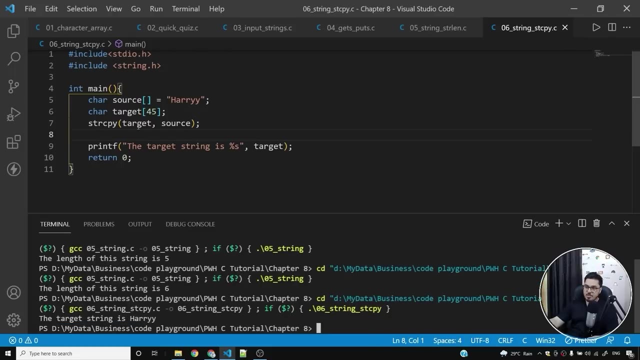 i'll save this program, i'll say the target string is percentage s and i'll try to print the target and you'll see that target now contains harry. so if i run this program, target string is harry. why? because this particular string was copied from source to the target. i hope that makes sense. 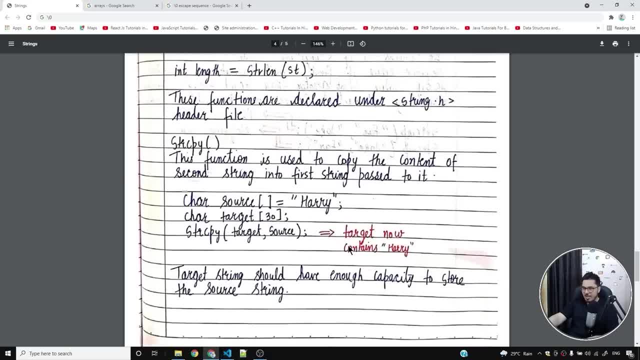 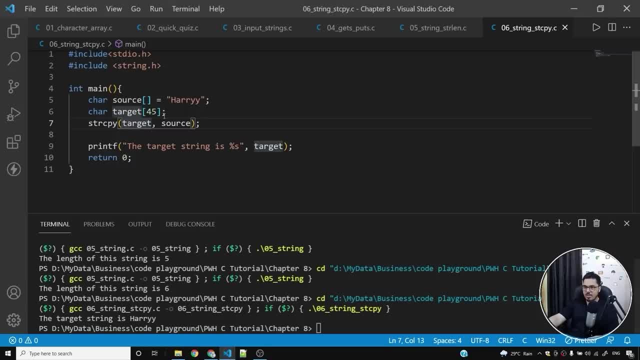 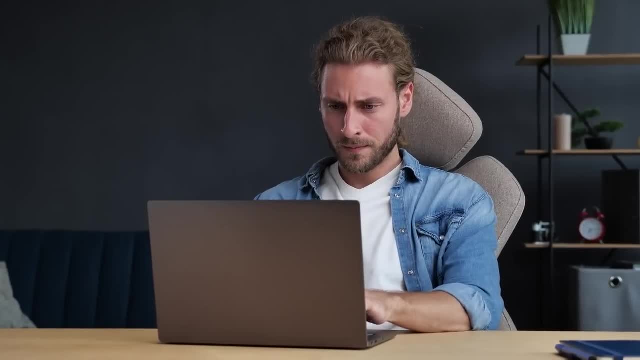 coming back back to the notes again, strcpy is something that we just saw. target string should have enough capacity to store the source string, obviously. so if i create a string with with four, i'll start seeing weird behaviors issue. you might not want your program to misbehave, so make sure the target 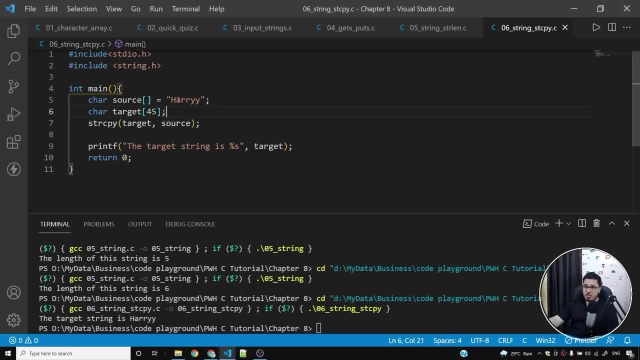 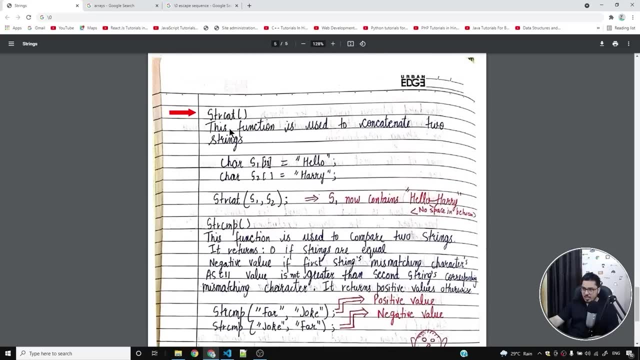 string has a sufficient character limit to hold the source string. okay, moving on to the next function, which is strcat, this function is used to store the source string. so if i create a string, i'm going to use strcat string and i'm going to use strcat string and i'm going to use strcat string. so if i want to join two strings, let us say i have s1 and i have s2- s1 contains hello, s2 contains harry, and i want to merge these two strings. so if i say strcat s1, s2, s1 will now contain hello, harry. 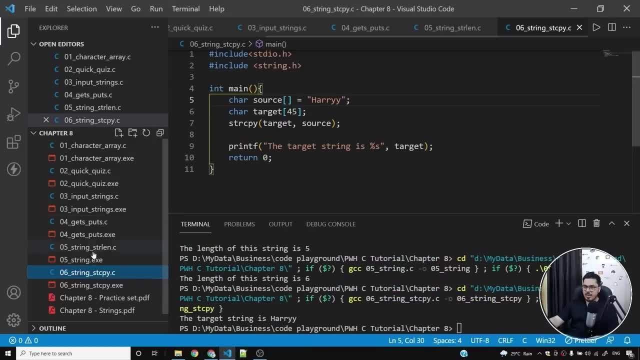 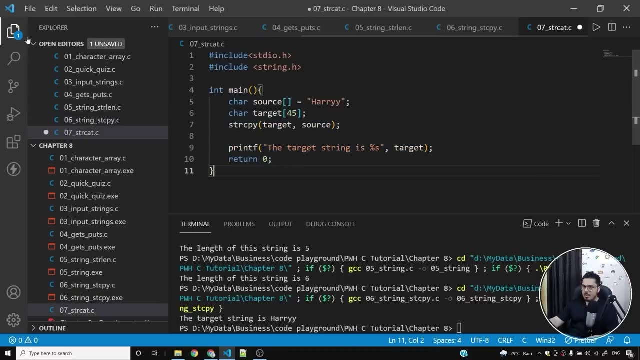 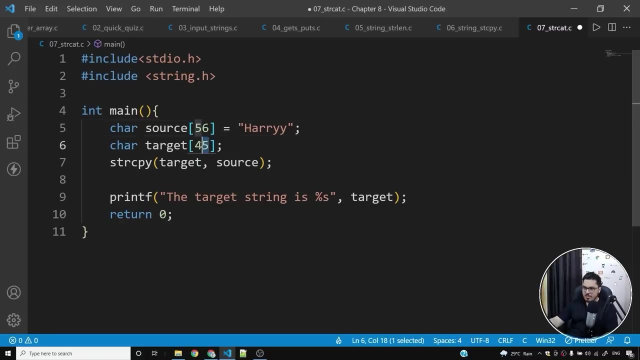 so let me show this to you: strcat string: concatenation zero seven, underscore: oops, s-t-r-c-a-t dot c. and let me copy this program. i'm starting from this program just to save some time. so let us say: source contains 56 characters and target contains this string. let us say it. 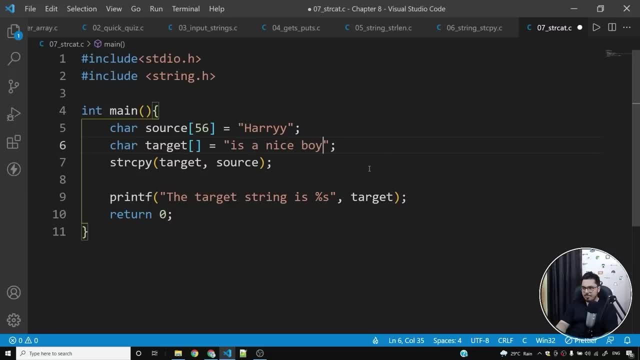 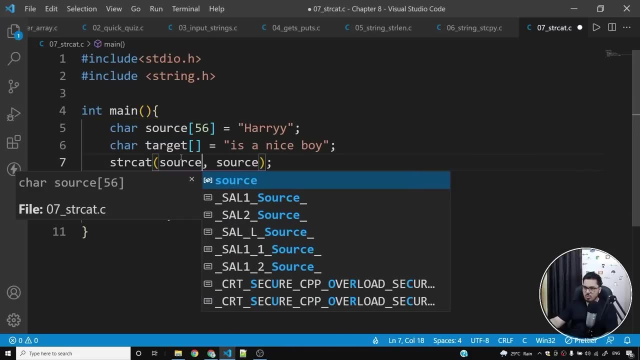 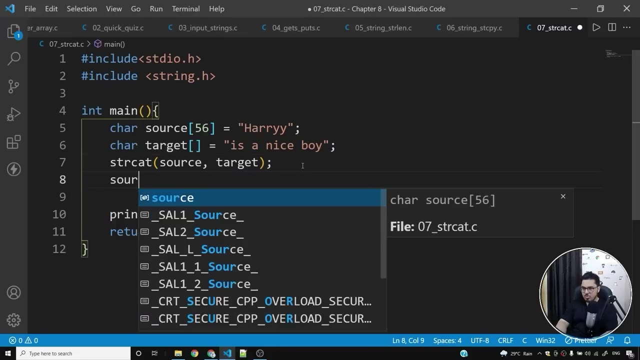 contains is a nice boy, and i say s-t-r-c-a-t. source target, so i want to copy everything to source. so source plus target will be assigned to source. so so if you want to, you know, get a rough idea of what is happening. this is something which is happening. do not take this literally. it's. 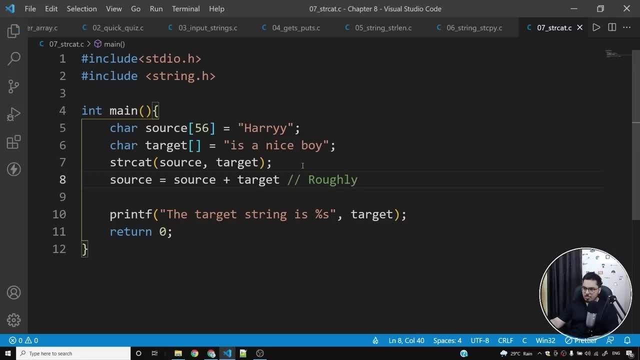 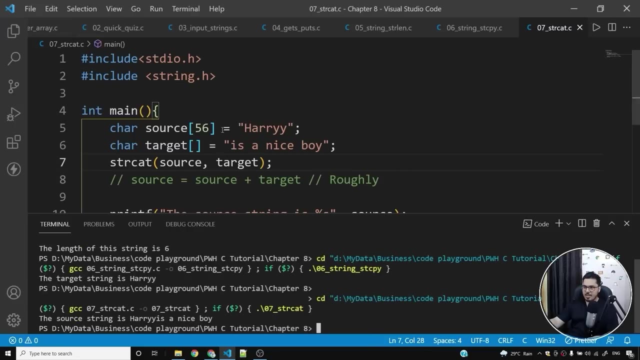 it's roughly which is happening, so i hope that you understood the gist of it. so if i now try to print the source string, i'll say source string is source. the source string will be changed and it will now contain: harry is a nice boy if i add a space here. 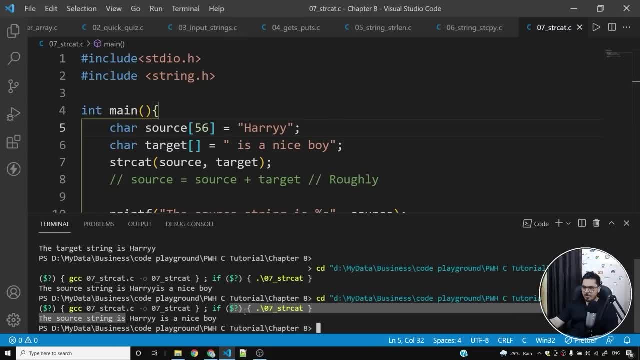 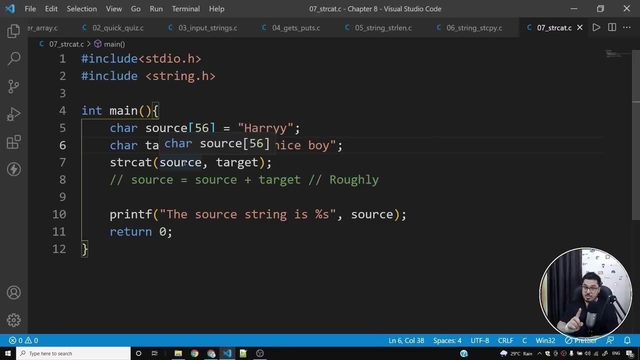 harry is a nice boy. so harry is a nice boy. okay, so these two strings are concatenated. this is the program to concatenate the string, and it will update source string, not the target string. this is something that you need to keep in your mind. now the last function that we'll discuss in. 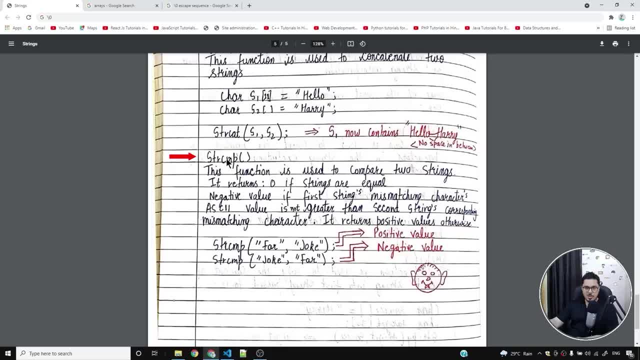 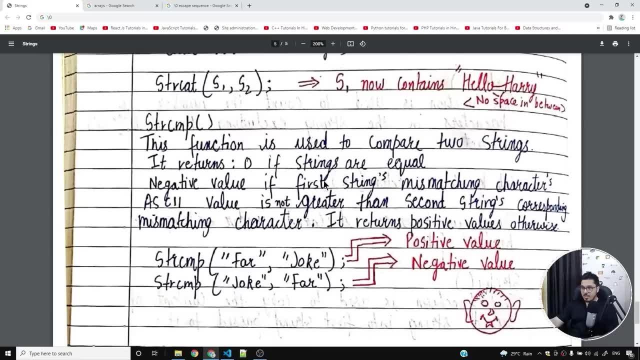 this chapter is strcmp, and this is last but not the least. you might google some other string functions. there are a lot of string functions, but these were some of the most important ones. now let's see. this function is used to compare two strings. it returns zero if strings are equal. so if you pass, 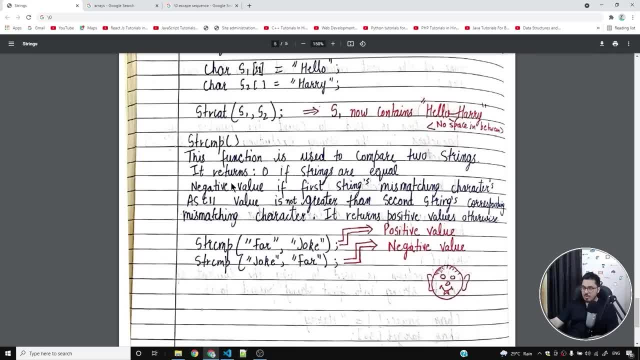 two strings and both of the strings are equal, this function will return zero negative value for strings mismatching characters. sky value is not greater than second strings corresponding mismatching character. so if far comes before joke in the dictionary we'll see a positive value. but if that is not the case, then we'll see a negative value. 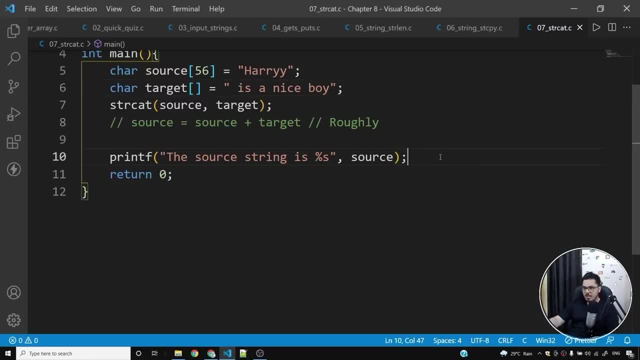 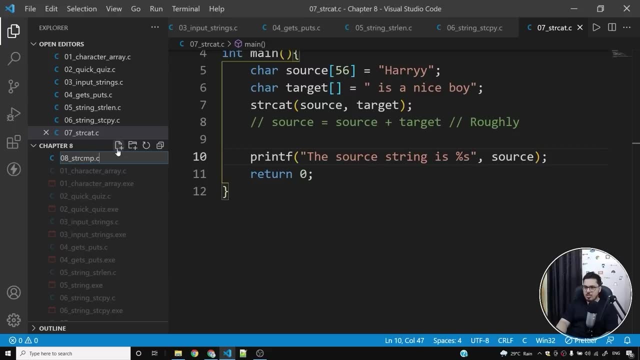 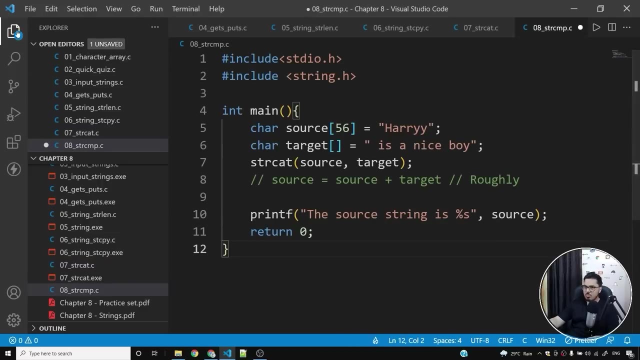 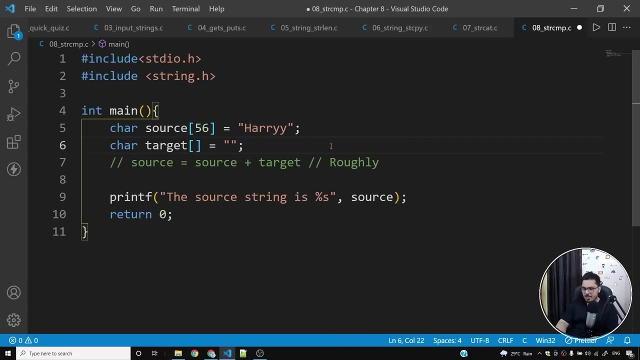 let me show you, so i'll use strcmp. let me show you strcmp, the new program. so i'll say 08, underscore strcmpc. i'll start with this. uh, oops, i'll start with this code: strcmp. let us say: source and target are two strings, and let me say: uh. 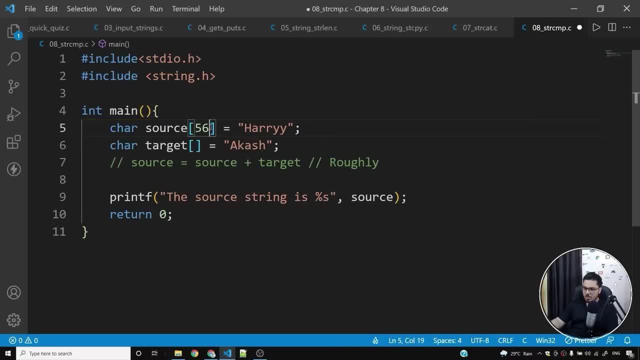 uh, akash, also. let me save this program and let me say source and target are two strings. um, let me remove this. and let me say the strcmp returns percentage d, this will return an integer. so strcmp will compare two strings. let me compare source and target, so 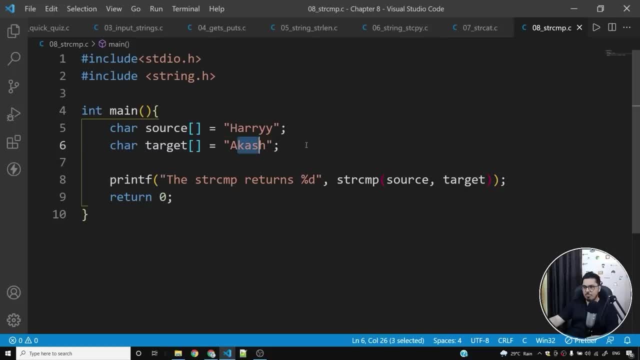 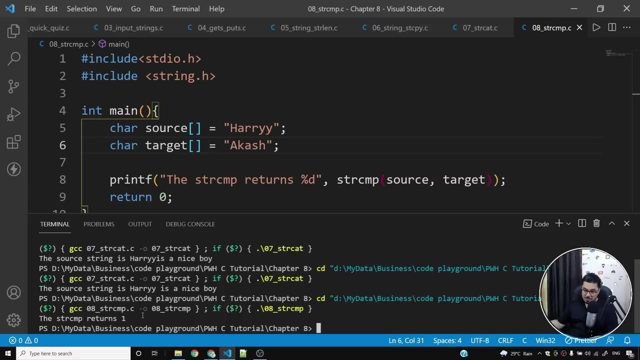 tell me which of these words will come in the dictionary before. akash will be the one that you'll encounter if you turn the pages of dictionary. you'll encounter this word before this. so what will happen is, if i run this program, one is returned, but in some of the compilers a positive value is returns. it might. 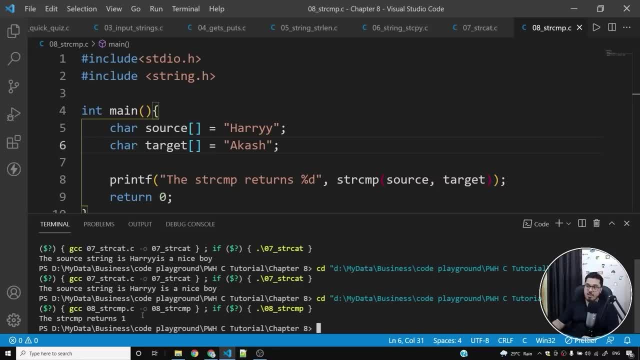 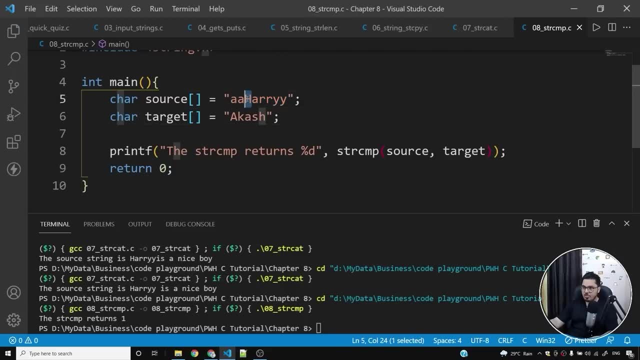 be one. it might be some other positive value, it might be a random positive value, but if i change this to aa harry, this word will come in the dictionary before akash. so let me change this to small case. let me run this for you. this still returns one, because the ascii value of 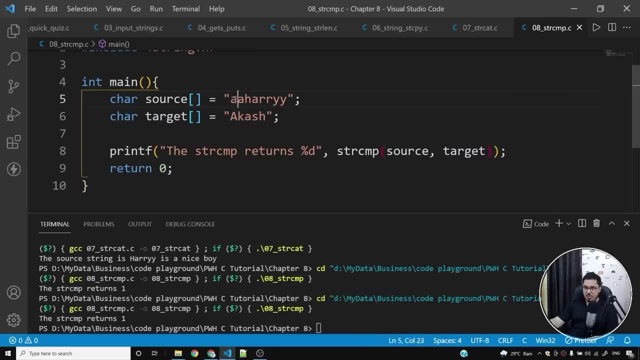 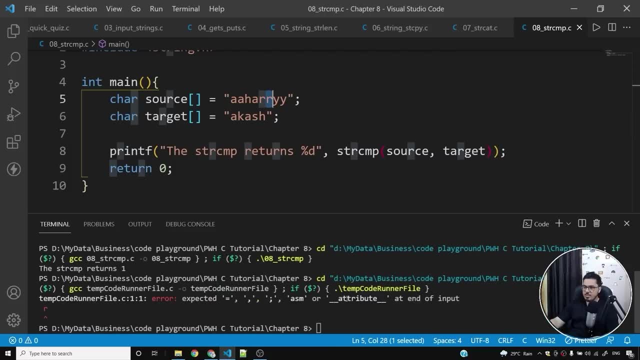 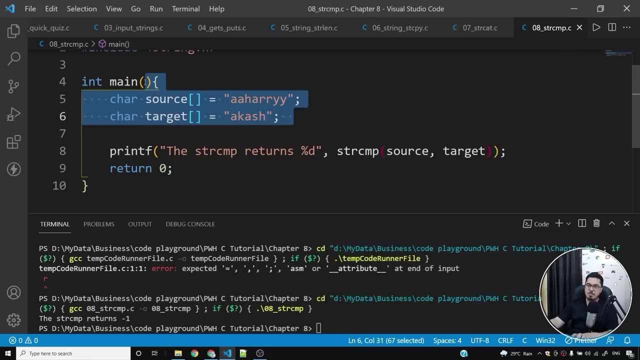 capital letters is smaller than the ascii value of small letters, which is why this is happening, if i change this to small letter u, and then i'll show you the case. oops, i selected something and ran. i need to. you know i should not select something and run, otherwise it will try to run that particular snippet and this is the. 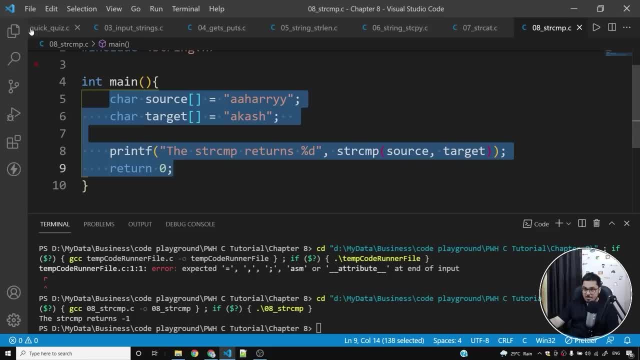 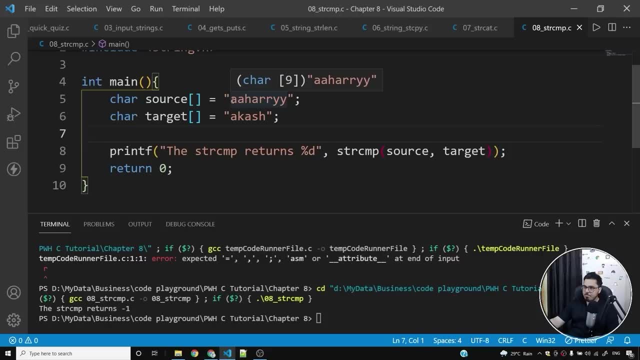 behavior of code runner. what it does is, when i'm selecting something, it will simply put that code inside temp code runner dot c file and it will try to run it. i don't want that. so if i make this aa, harry akash minus one is returned, because this particular word will now appear in the 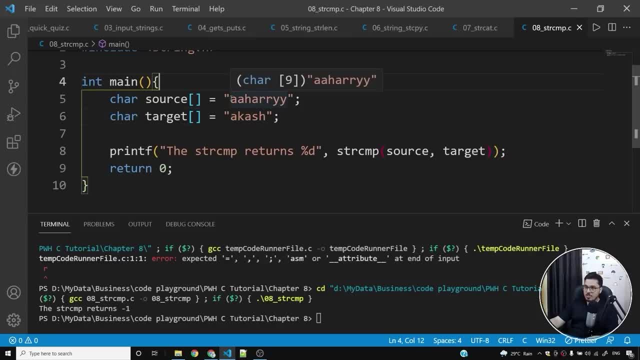 dictionary before this one. okay, so this is how this works, but let's not see it from the dictionary point of view. what we will see it from is we'll see it from the ascii value point of view. let us say, the s key value of this character and this character is the same, which is that it will check the s key value of this and 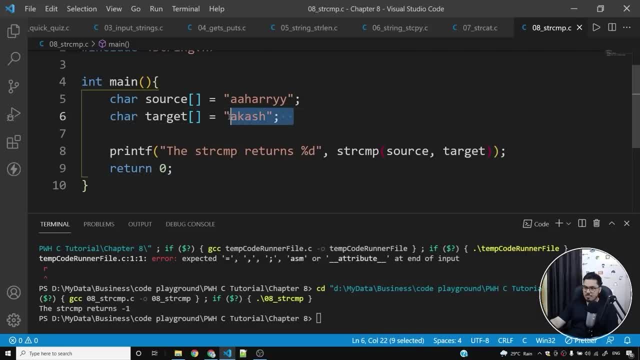 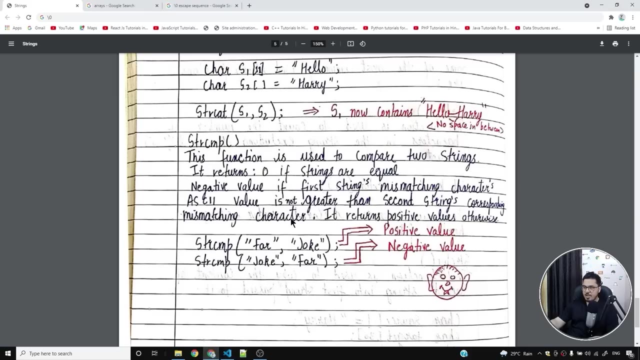 this. so which ascii value is greater? this s key value is greater, so it will return minus one. so i hope that you understood how this is working. what if i make both of these strings as the same? what if i make it a, a, a a zero will be returned. so let me show you. so zero is returned, and this is what i've written in the. 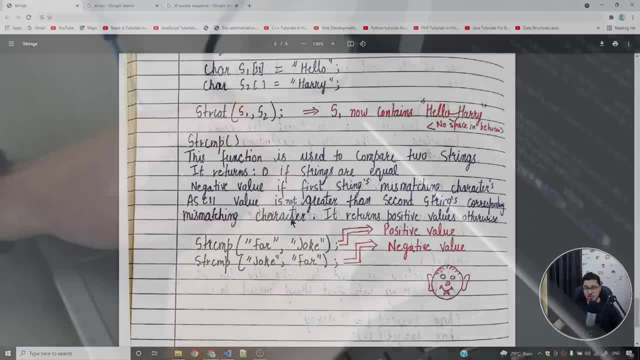 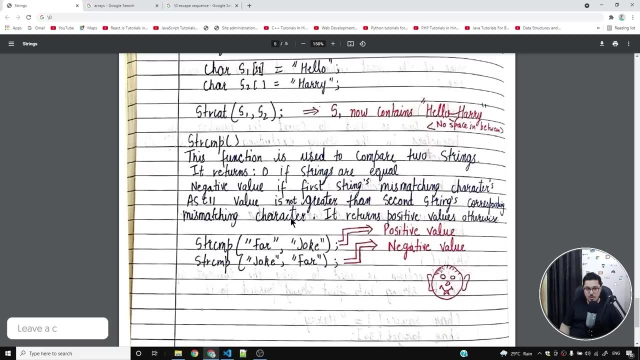 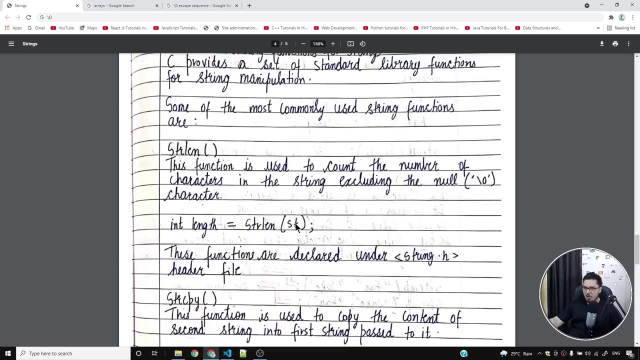 notes as well. i hope that you like this chapter and you can now use strings in your programs. if this course was enjoyable, make sure you leave a comment below and tell me that this course is something you are enjoying, so that i can bring more courses like this in the future. but for now, 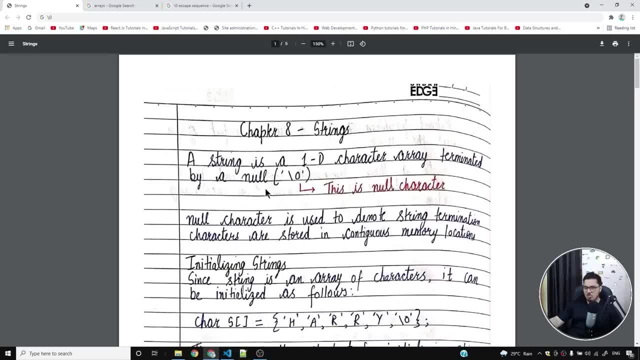 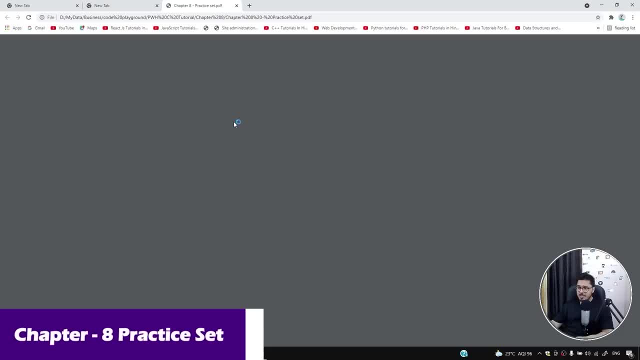 we'll move on to chapter 8, practice set, and we'll solve some problems on strings. let's move on to chapter 8, practice set now. so now what we'll do is we'll start with the practice set and we'll start discussing the problems in the practice set. so this is the practice set which i've created for 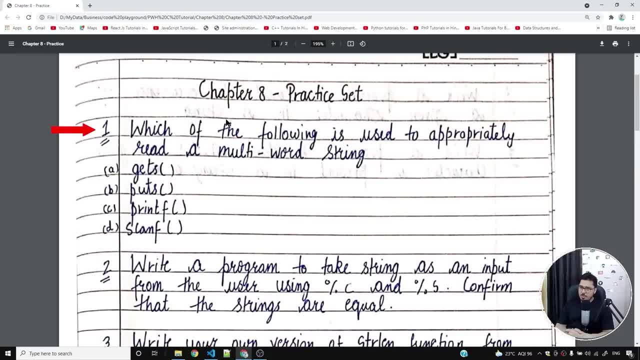 you- and the first question is an mcq, it seems- which of the following is used to appropriately read a multi-word string? and the answer is pretty simple. i want you to comment in the comment section. put the timestamp, please, and tell me which is the correct answer. so, if you, 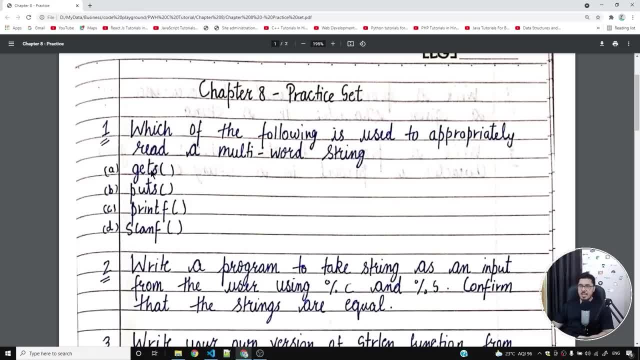 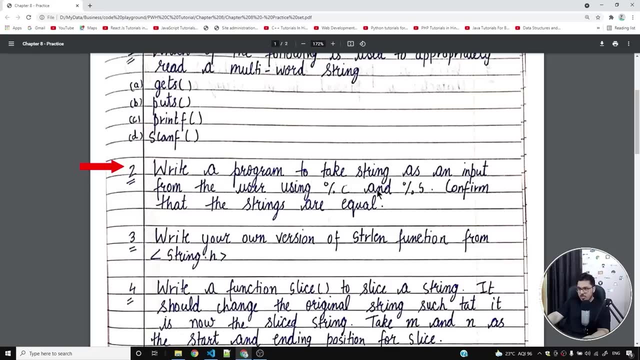 guessed it correctly. in fact, if you got it correctly, the answer is a gets. gets is the function which is used to appropriately read a multi-word string in c language. so let's move on to the next question. so the next question says that write a program to take string as an input from the user using percentage c. 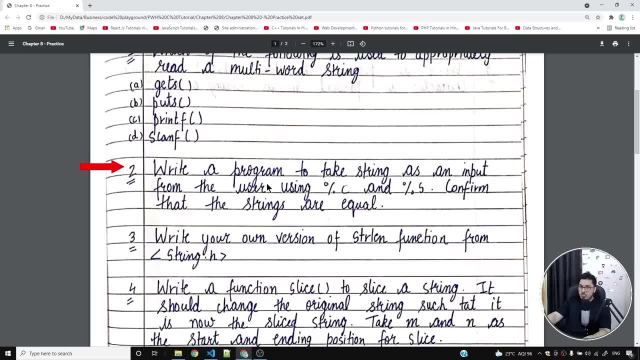 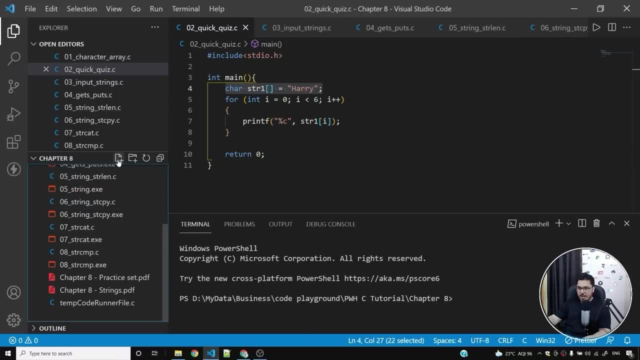 and percentages confirm that the strings are equal. so we need to write a program, firstly using percent c format specifier and then using percent s format specifier, and we need to confirm that the strings are equal. let's try to attempt this problem. so what i'll do is i'll create a program, number nine, which says: 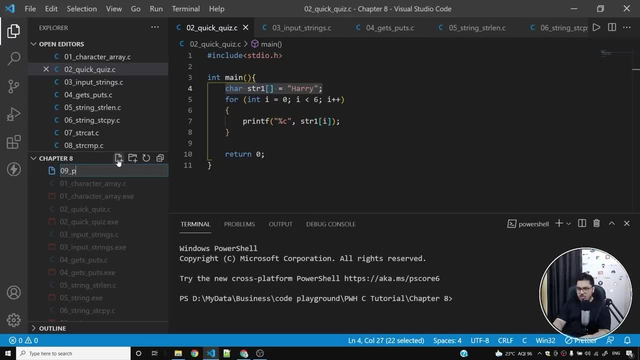 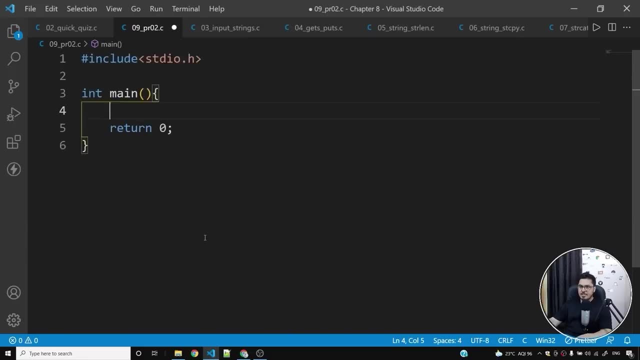 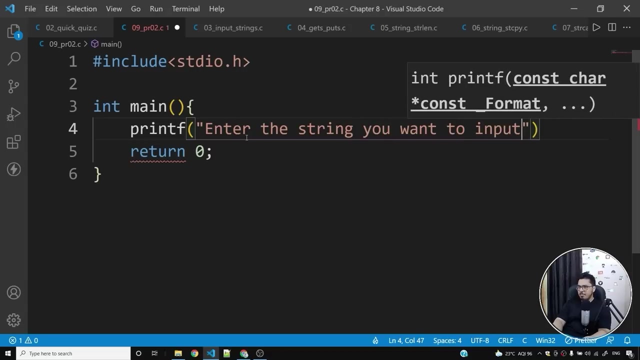 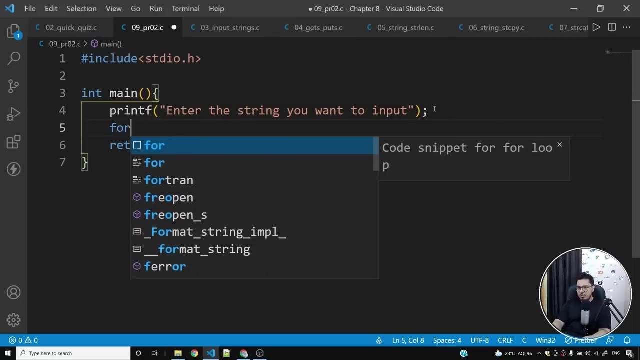 zero nine underscore p, r, zero two dot c, because this is problem number two. so i'll put in the boilerplate code and i'll simply say: let me start with a printf statement. what i'll do is i'll say: enter the string you want to input. okay, so this is a string that you want to input. so what i'll do is i'll simply use a for loop. 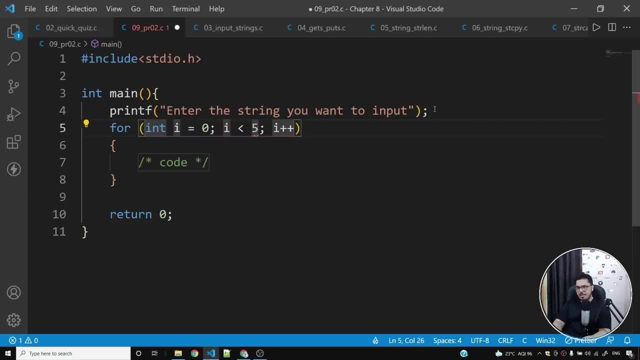 and i'll say int i is equal to zero and int i is less than five. let's assume that the length of the string is five and i'll also add using percent c, and i'll not write using percent c, using percent c, because i don't want to print anything here. 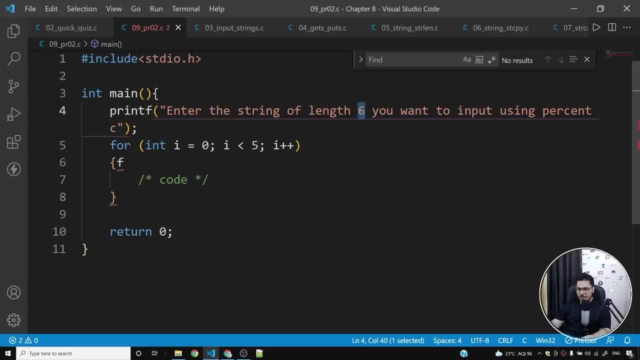 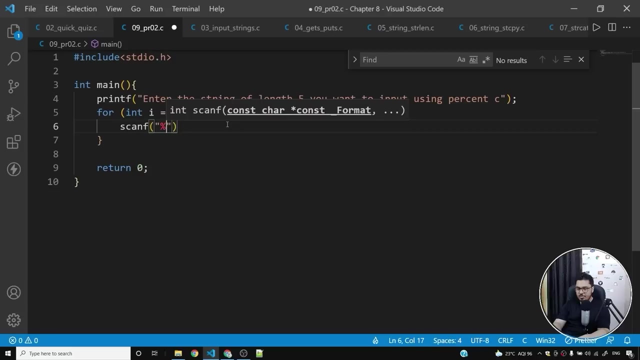 so what we'll do is we'll keep on pressing the enter key and also i'll say: enter the string of length five you want to input using percent c. now what i'll do is i'll simply use my for loop, let me use the for loop, and what i'll do is i'll say: scan f percent c. so we, in the first case, what we are, 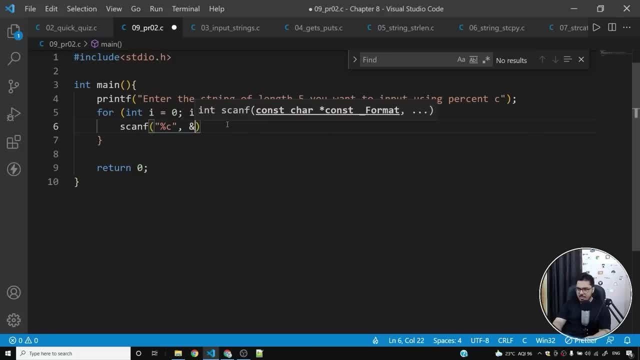 doing is we are taking the input character by character. so i'll say ampersand and let me say car i or sti, where st is a string, so let me also say car st5. this will declare a string with name st, of length five. in fact i'll have to make it six because length of the string is five. also, i need 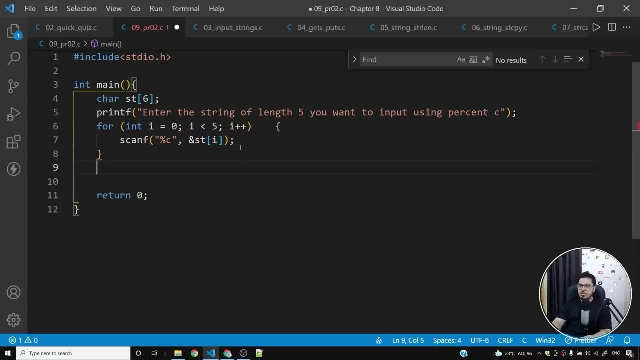 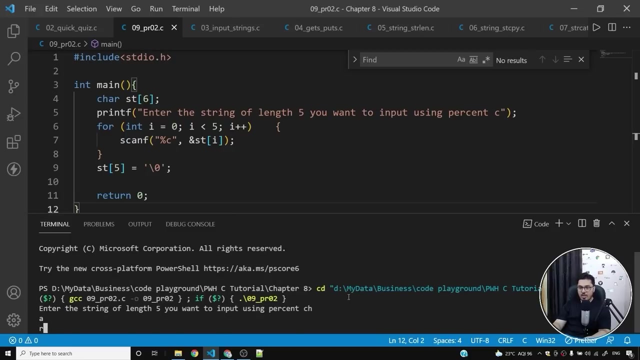 to add a null character to it. so i'll keep on doing this and at the end, what i'll do is i'll simply say: st5 is equal to. st5 is equal to a null character backslash zero. so let me run this program, and the moment i run this program and try to enter h a r, it stops me. 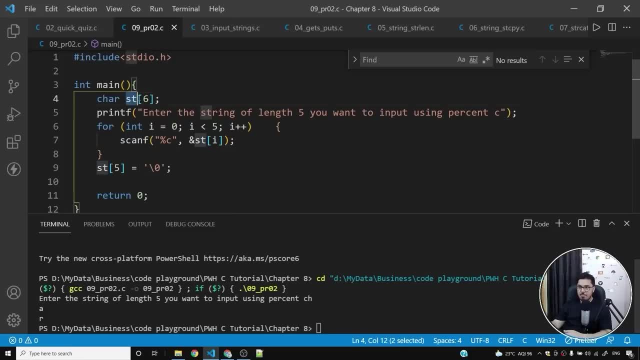 what is happening here? why is it not allowing me to enter my name? my name is of length five. the string can hold five characters. what's wrong that i'm doing in this program? let me explain you the moment. i try to run this scanf and i try to store h inside sti, which is st0 initially. 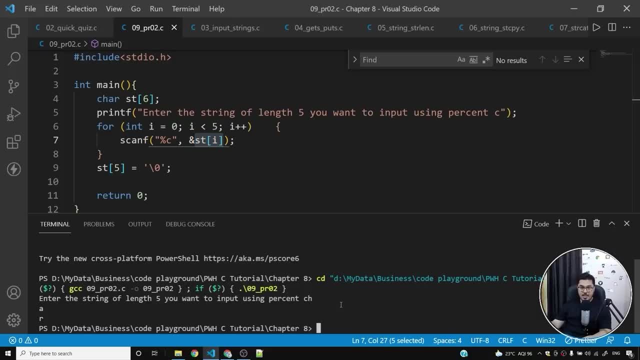 what will happen is i'll press c and i'll say car st5, an enter key, and that enter key will actually be taken by the next scanf, which means the next character will be the enter key. so what is happening here is so, when i say this, a for loop, 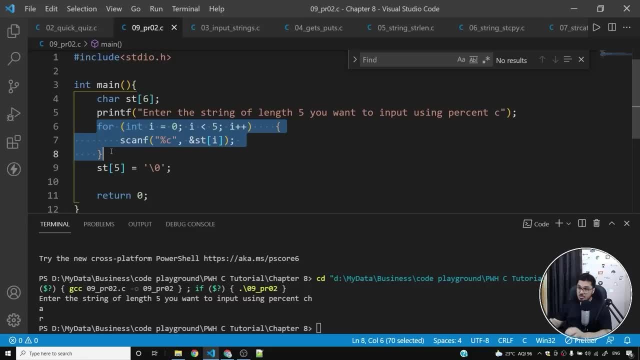 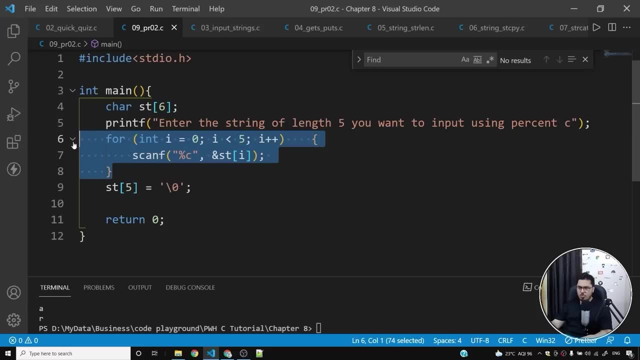 and a scanf inside for loop. listen to this very carefully because this is very important concept and if i have scanf inside a loop for loop while loop- or it can be any kind of loop do while loop- this scanf will actually take this character. whatever i'm typing using my keyboard will be. 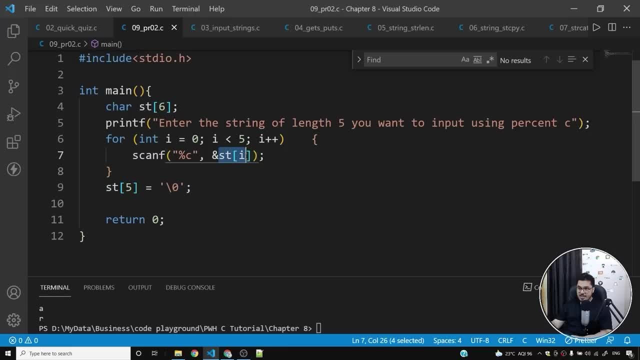 inside this. so initially i will be zero. so inside st0 this particular character, whatever is entered by me through the keyboard, will be stored. but after i press that character i'll definitely press enter key. that enter key will be cached by st1. i don't want st1 to catch that enter key. 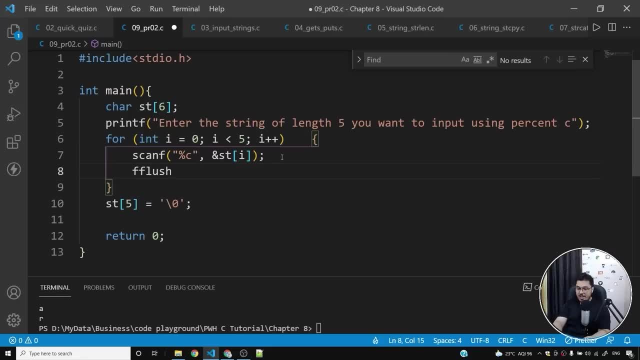 so what i'll do is i'll write a flush stdin. so what this will do is this will flush that enter key. So the moment I press enter key to finalize the character that I want to store in st0, that enter key will be removed from the stdin. 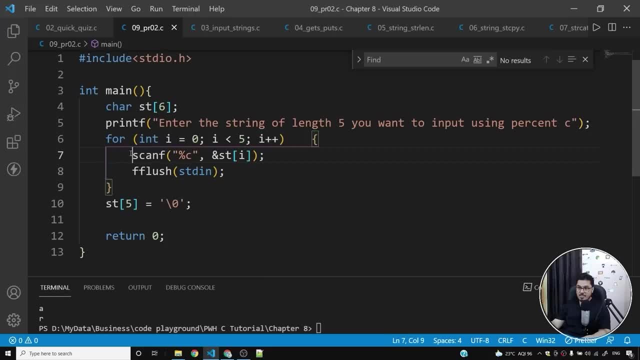 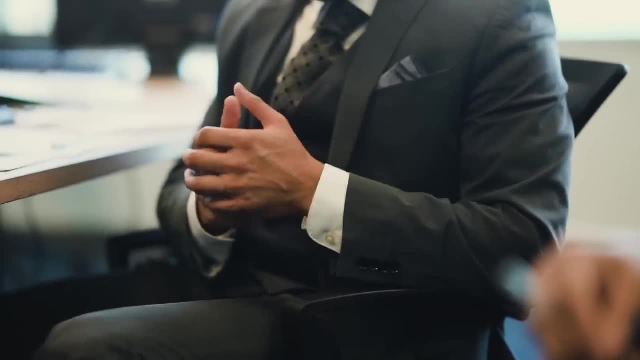 which means that next time when this runs, when the scanf runs, for i is equal to one, it will take the fresh character and not the enter key. I hope I was able to explain you this. So, basically, to flush the enter key that we have pressed, 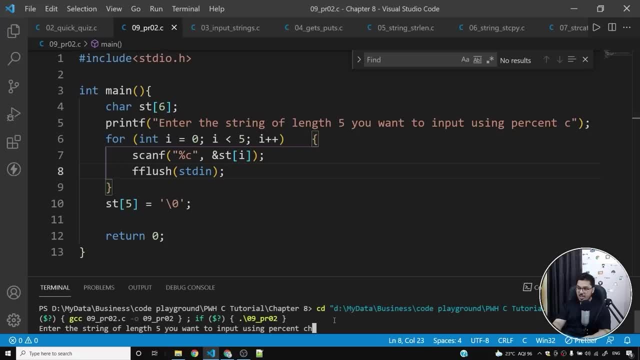 I have to write this. So now, if I run this program now I can say h a r r y and, yes, I can store harry inside st. Now what I'll do is I'll simply say: 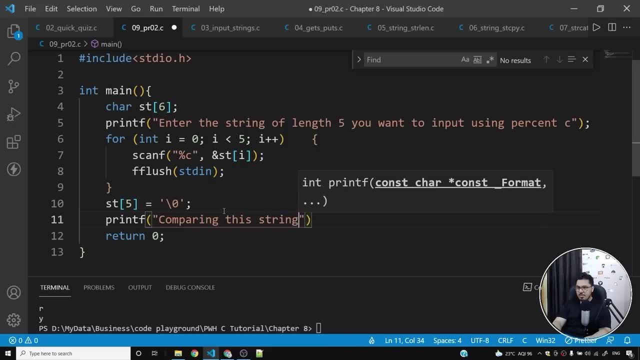 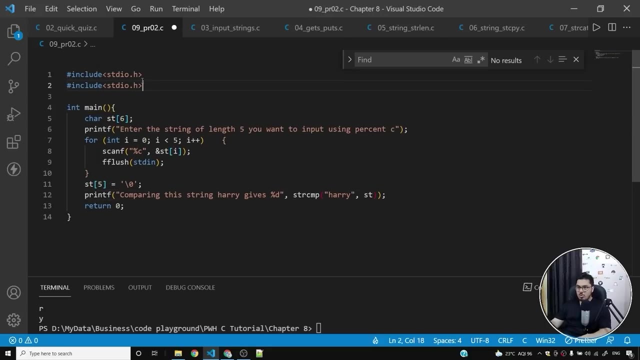 comparing this string with harry gives percentage d, and percentage d is nothing but the output of st or cmp. So I'll compare this st string with harry. Now let me also include stringh, because this is important. We discussed this in the last chapter. 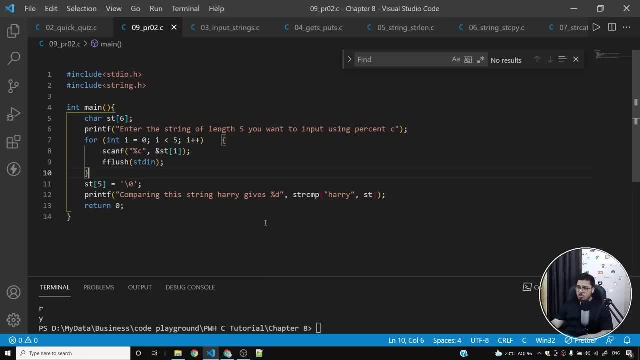 in fact in the same chapter, in chapter eight. Now, if I save this program and if I try to run this program and I enter harry h a r r y, So comparing this string with harry gives zero. 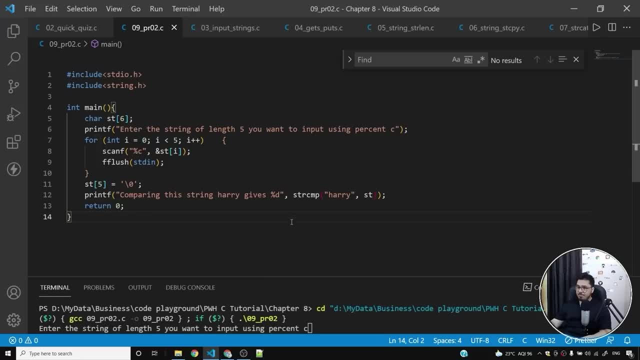 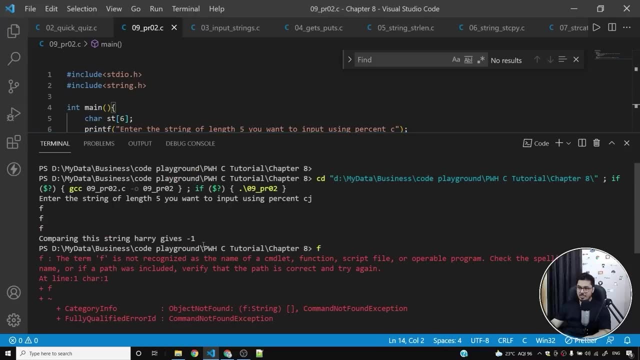 which means harry in this string is the same. So if I let us say type something else, you can see that comparing this string with harry gives minus one because the string was not the same. So this was a bit, you know, vague question. 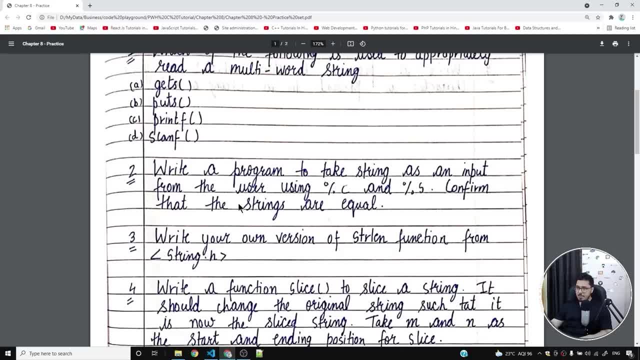 I hope that I was able to explain you the concepts. Maybe the statement might not lead you to the correct answer, but I hope that I was able to explain you some of the concepts. Write a program to take a string from the user using %c and then using %s. 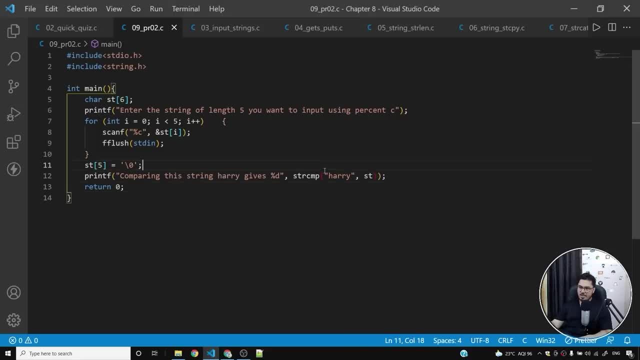 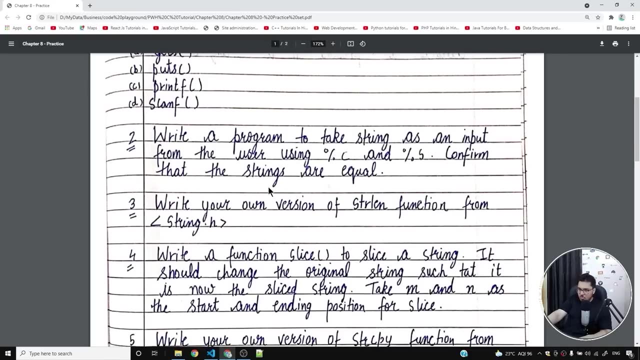 So I should have taken it using %s. but that's fine, You can. we can even use these double quotes. This works as well. You can refactor the program in the way you want. Now write your own version of stln function. 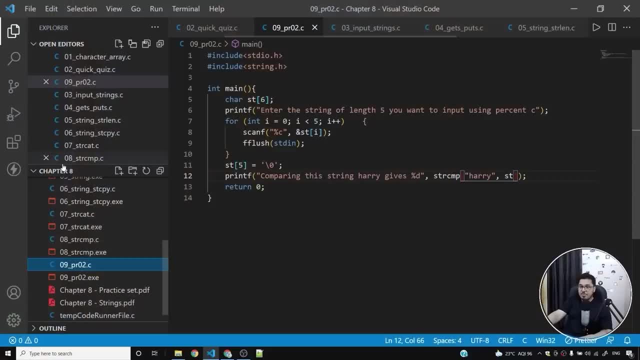 from stringh. This one is going to be interesting, let me tell you. So let's implement our own stln. So 10 underscore pr03.. So I'll say pr03.c. So what I'll do is I'll start with this program. 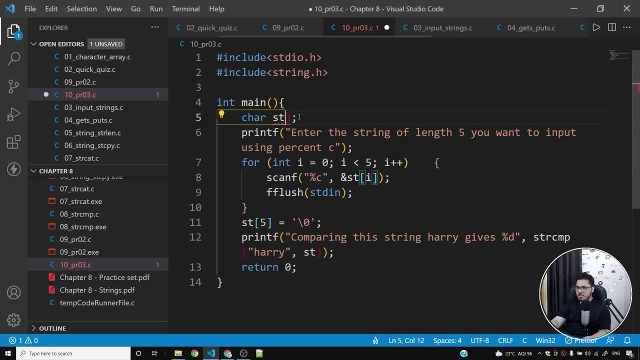 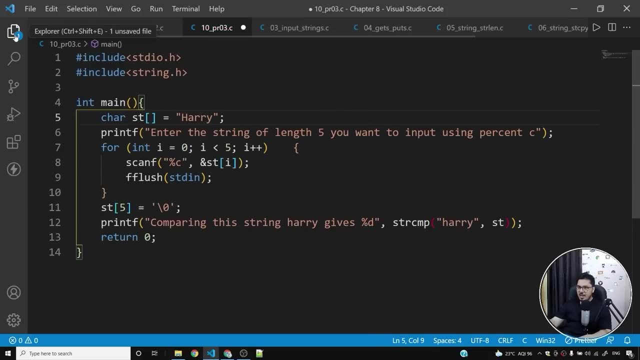 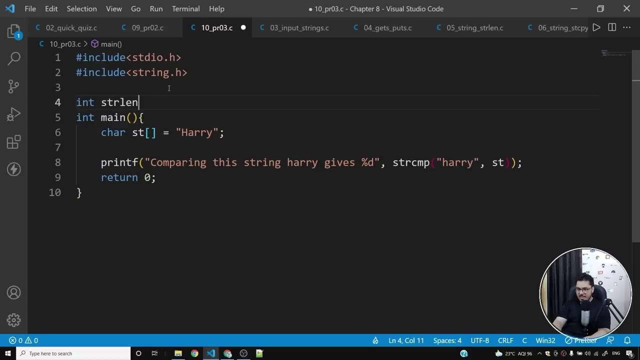 so that I have a string and I'll say char st is equal to char, st is equal to harry. Also, what I'll do is I'll write my version of stln. And what I'll do inside that stln is I'll return int stln. 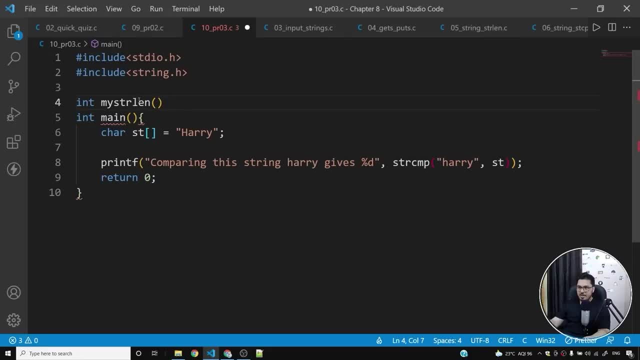 and I'll remove this my stln, let me call it my stln. And what I'll take is a character pointer and I'll keep on scanning this character pointer until I encounter a backslash n. So I'll say: char star, ptr. 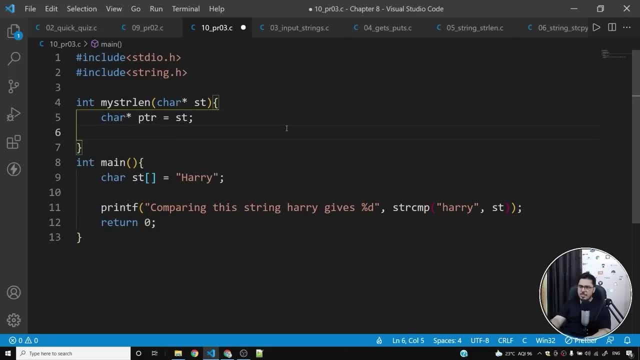 ptr is equal to st, and I'll keep on incrementing this pointer. I'll say: while this ptr is not equal to backslash zero, So the moment this ptr, you know, turns out to be backslash zero, what will happen is this while loop will stop working. 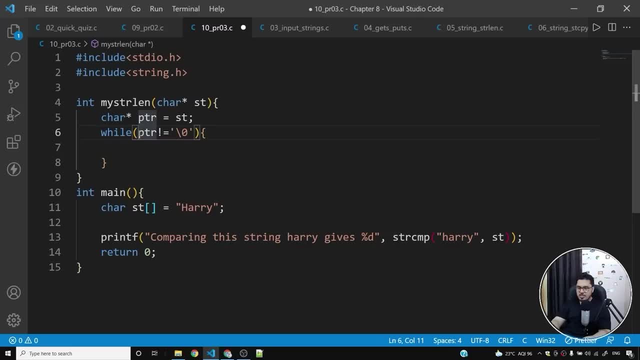 So this pointer is currently not equal to- or rather I should say star- ptr. the value of this pointer should not be equal to backslash zero. it should not be null character. I'll keep on incrementing, incrementing this pointer and also I'll keep on incrementing length. 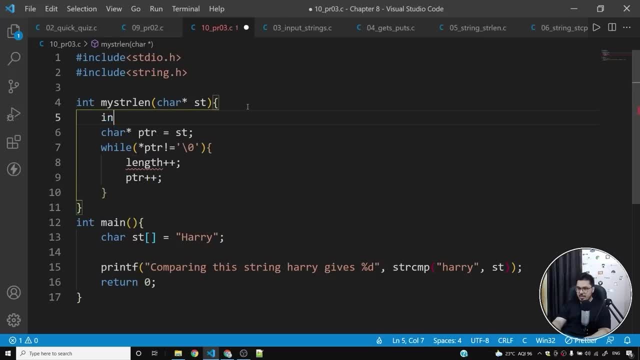 length plus plus. So initially the length will be zero. So I'll say length is equal to zero and I'll return length. The moment this, while loop exits, I'll return- sorry, not zero, I'll return length. Let's see if this works. 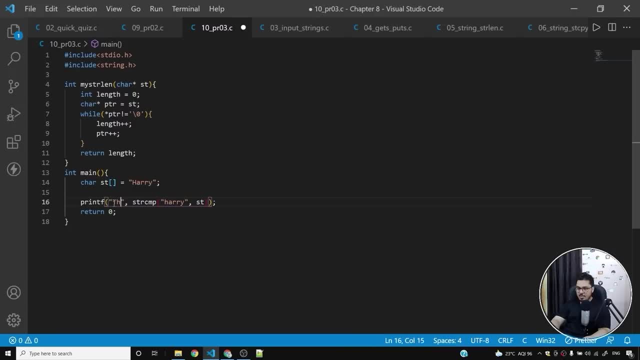 The length of the string is. I'll say the length of this string is percentage d, and what I'll do here is I'll simply write: the length of the string is percent d, and it will be my stln, and I'll give this particular pointer, which is st. 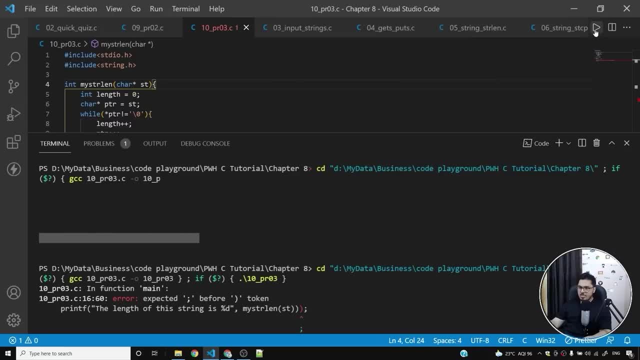 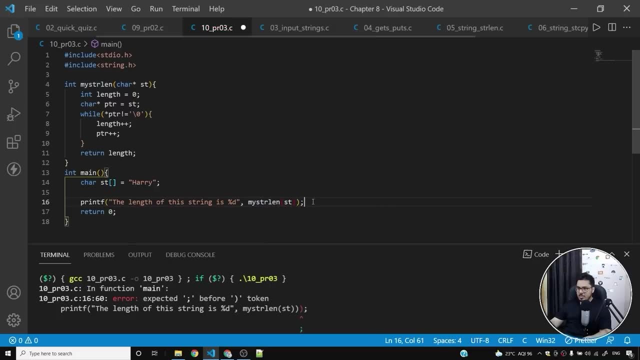 and let's see if it is able to find the length. So if I run this program, I'm getting some error. I think I forgot some brackets, So this is the bracket for this. Okay, I think this program should work And it says the length of the string is five. 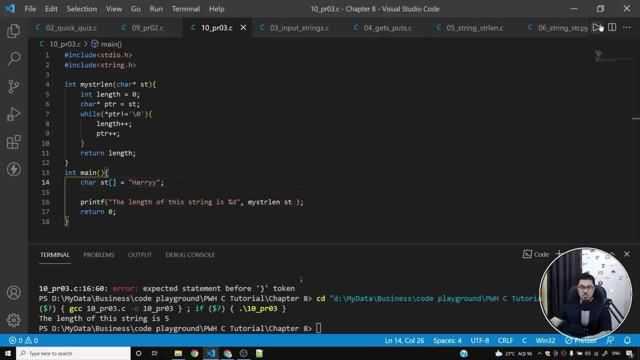 Let's see if it is able to return the correct answer. The length of the string is six. Yes, And if I even further increase my string, you'll find the length of the string is 15.. So this works. This, my stln, works pretty well. 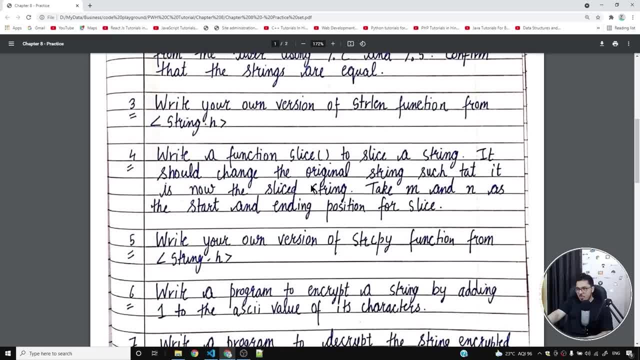 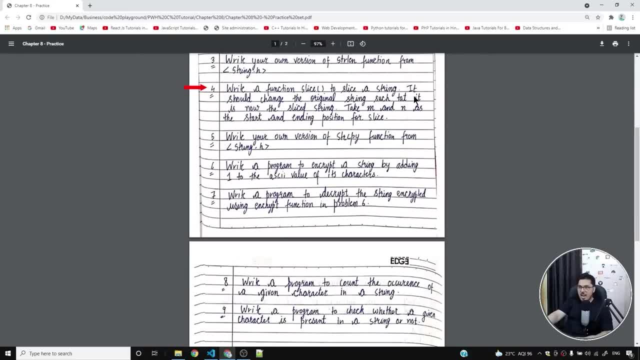 I hope you understood how I implemented this. Let's move on to the next question, which is question number four. It says: write a function slice- to slice a string. It should change the original string such that it is now the sliced string. 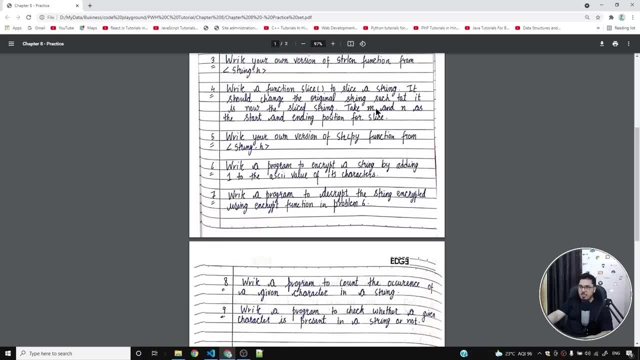 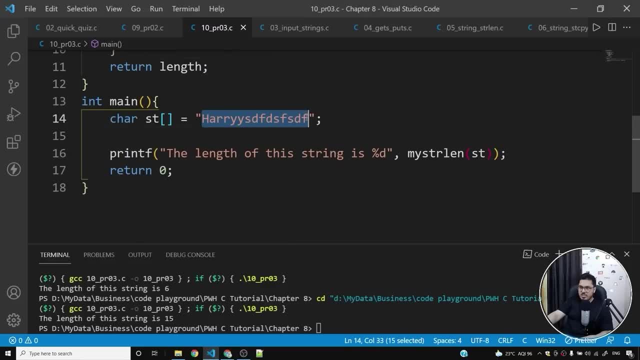 Take m and n as the start and ending point for slice. So this question simply says that if your string is this, you might want to change this to say this: a part of the string. So, in order to do this, what you'll do is you'll keep on copying st, f, d, s, f s. 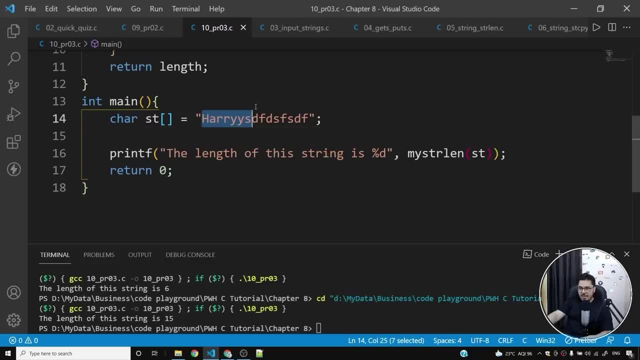 into these initial characters And, finally, what you'll do is you'll terminate the string with backslash zero. I want you to take this as a challenge and solve this problem, because we have already wrote a program on swapping two numbers and reversing an array. 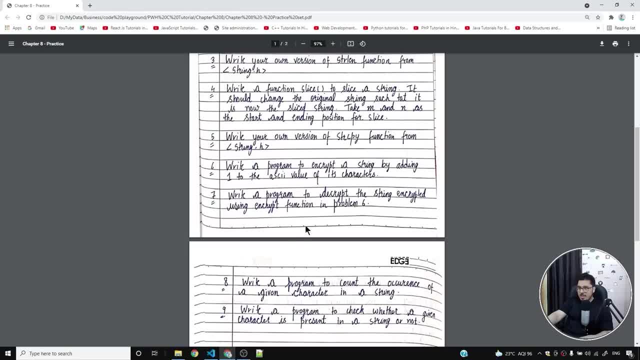 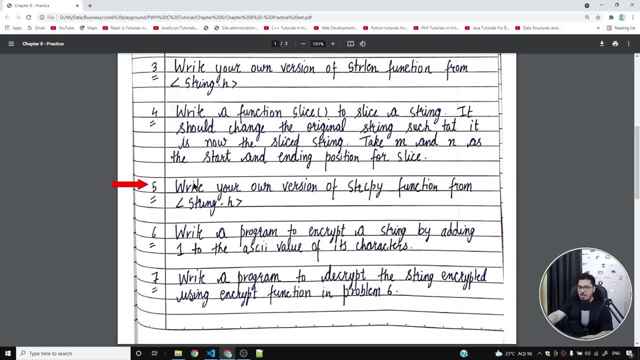 So this is exactly the same thing. I want you to try this on your own And also try to implement your own version of strcpy, because this is also very simple. This is also, you know, based on arrays. we have already solved a lot of problems already. 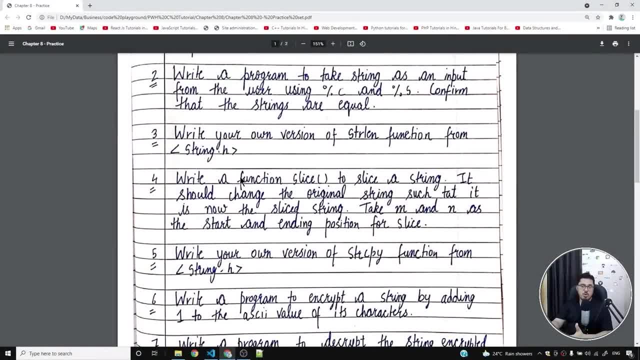 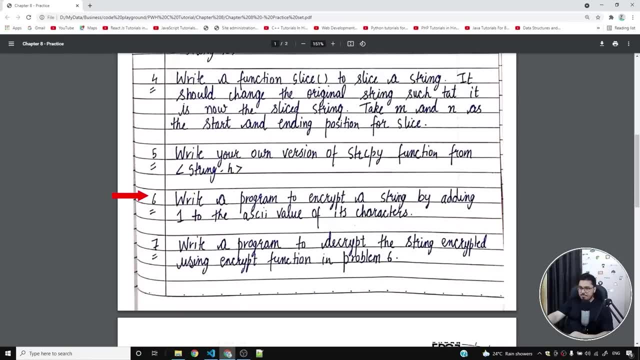 I don't want to repeat a lot of concepts that have been already discussed here. The next question says that write a program to encrypt a string by adding one to the ascii values of its character, And let me solve this for you. So this is problem number six. 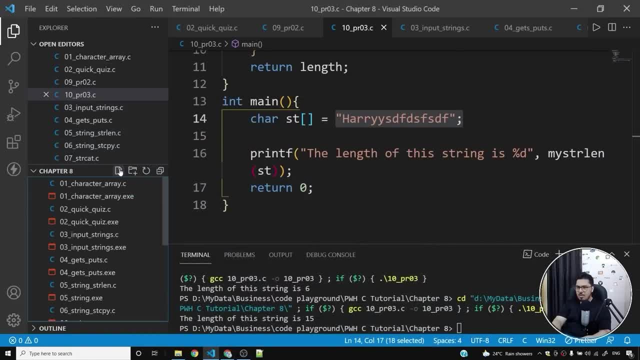 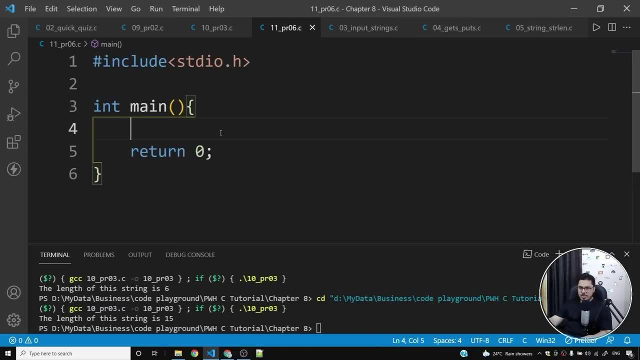 So 11 underscore, pr06, dot c, And what I want you to do is change a string such that it is encrypted. So I'll simply say char name is equal to. so the char name is equal to harry, And I want to change this string. 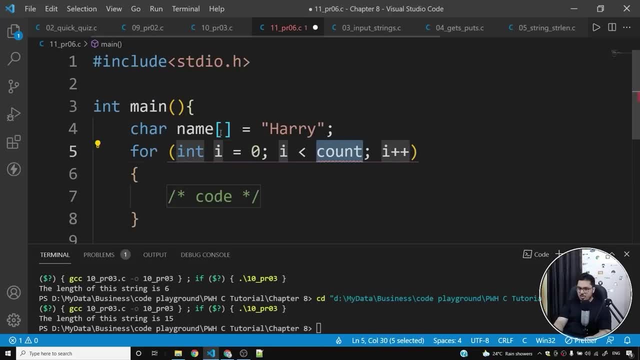 so that it is encrypted. So I'll use a for loop. I'll say int. i is equal to zero, i is less than six, because- or rather, let me make it five, Because there are five characters, I don't want to touch the null character. 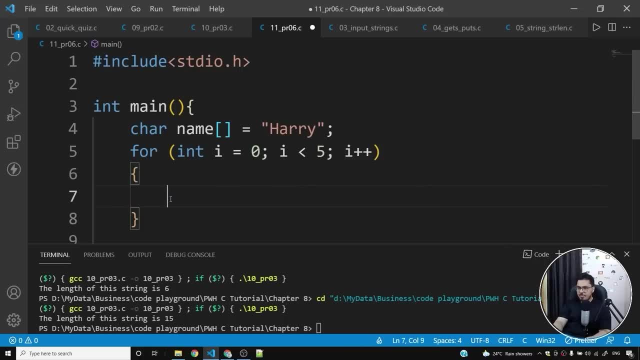 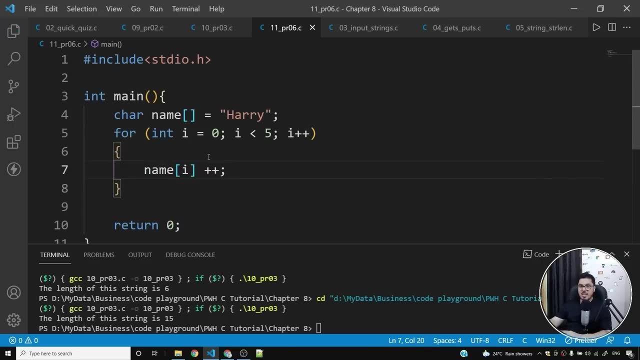 Now what I'll do is I'll say name i plus plus. What this will do is this will increment one to the ascii value of this character And if I try to print this string, I'll say: this string is percent s harry oops name. 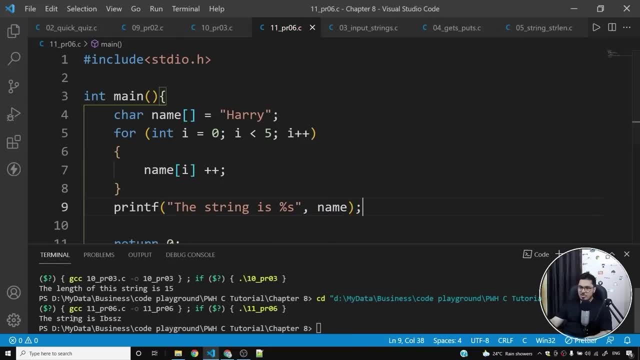 And that's about it. If I run this program, you will see the string is ibssz. Nobody can tell this is harry, but it's actually ghi. a, b comes after a, then s comes after r and z comes after y. 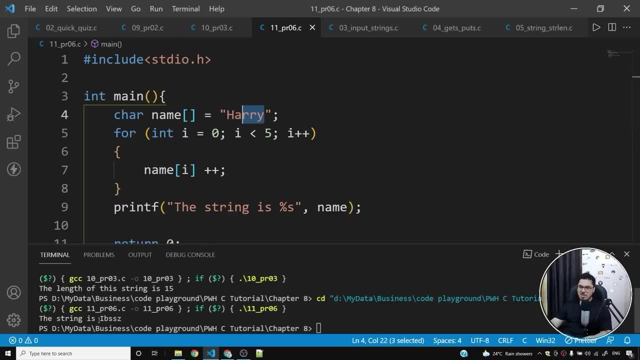 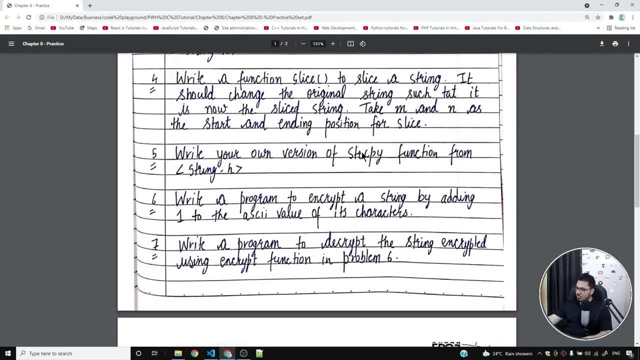 So we have, kind of, you know, encrypted this string, But this is not, you know, safe form of encryption in my opinion. But again, you can use it as some sort of encryption. okay, Now write a program to encrypt a string. 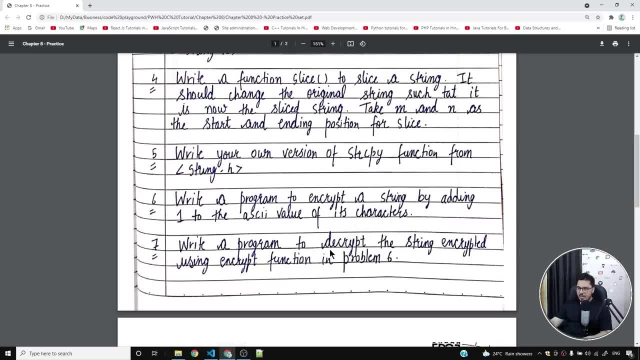 by adding one to the ascii value of its characters. Write a program to decrypt the string. encrypt, reducing this problem. So all you have to do is decrypt the string by reducing one from the ascii value. So this is exactly the same thing. All you need to do is you need to say: 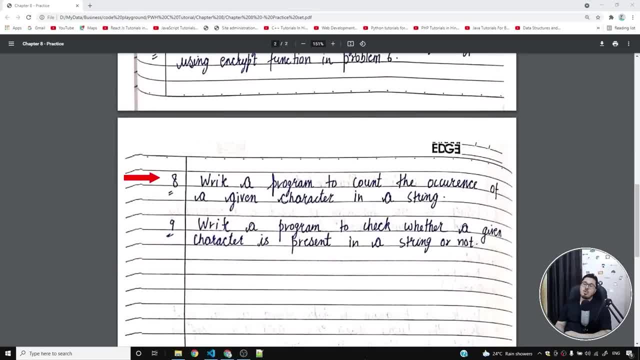 name. i minus minus and the problem is solved. Question number eight says that write a program to count the occurrence of a given character in a string. What you need to do in this question is you need to count the occurrence of a given character. 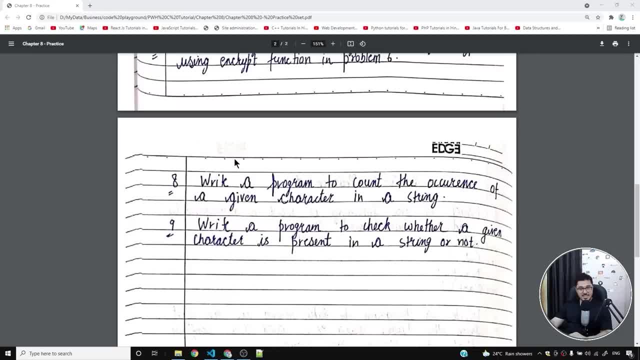 which is: let us say, I have a character. You can iterate the array and keep on checking whether that character is equal to the character of that particular iteration in the string, So you can count the number of characters in a given string. It's a very basic question. 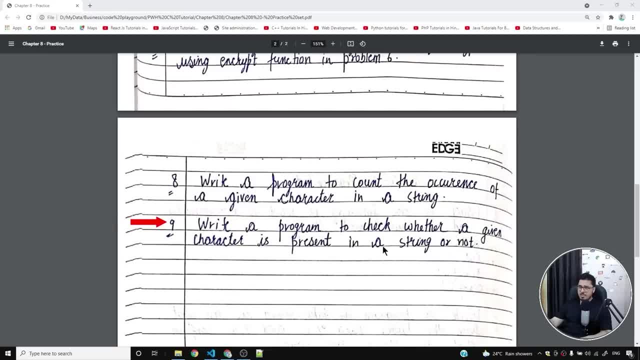 You should be able to solve it. Write a program to check whether a given character is present in a string or not. This is even more simple because all you need to do is All you need to do is iterate the array and, once you find that particular character, you 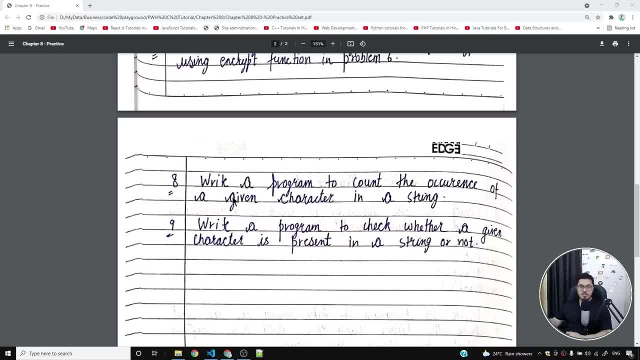 are looking for, you can break out of the loop. So, even if the length of the string is 17 and the third character in the string is the character that you are looking for, you can find that character and break out of the loop. 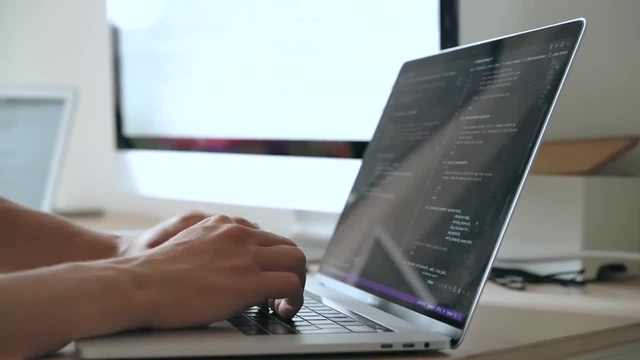 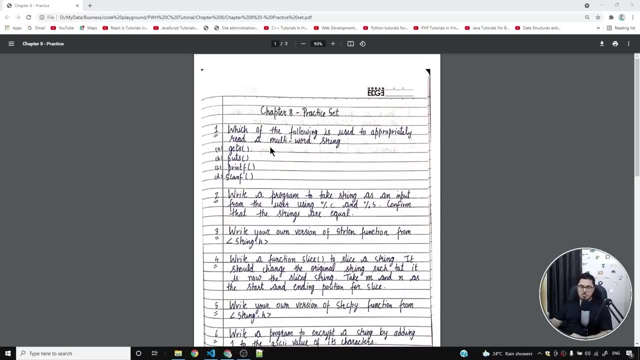 You don't have to check for the characters. I hope that this practice set was pretty simple and the concept of string was exactly the same as the concept of array, But once you understand where to put the null character and how all these things work, you 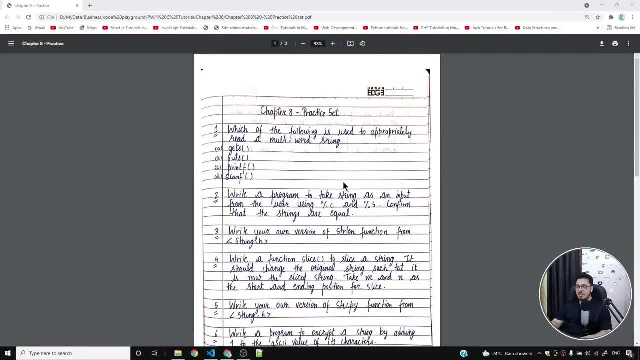 will be more comfortable in solving all these questions. So I hope that this practice set was useful to you. Now we'll move on to the next chapter and we'll further explore the concepts of C programming language. Let's move on to chapter 9 now. 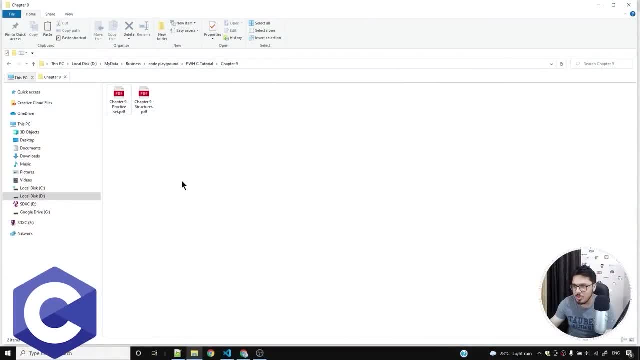 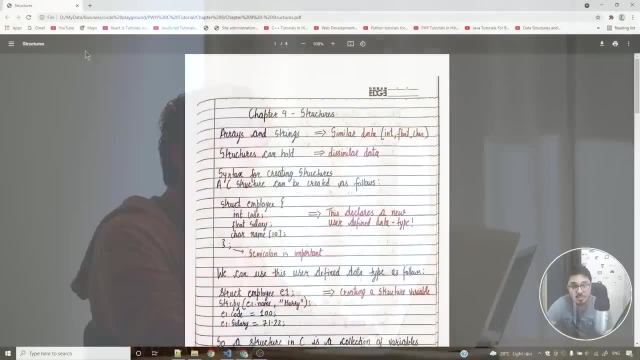 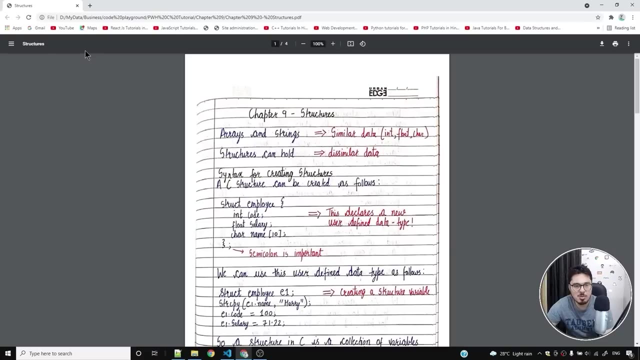 Now that we have done so many things in C programming language, let's look into structures, And this is something that people think is also a complicated topic after pointers. But let me tell you something: Structure is very beautiful. It's a beautiful concept when it comes to C programming language. 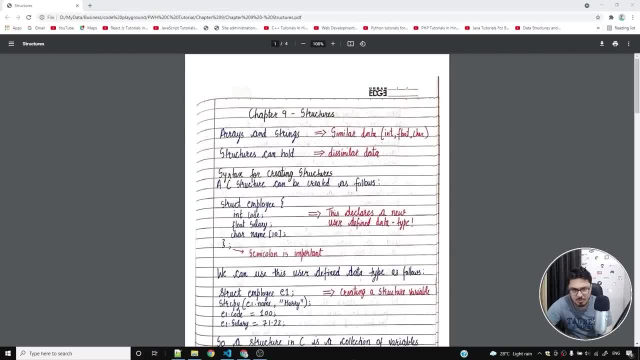 If you start understanding what a structure is, that will really, you know, build the foundation of programming concepts that you are going to hold in the future. So the concepts of object oriented programming and the concept of classes and objects that you are going to learn in maybe C C++ Java- not in C C++ Java- JavaScript and so on. 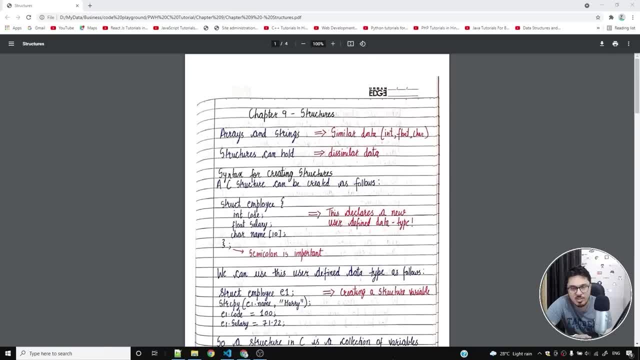 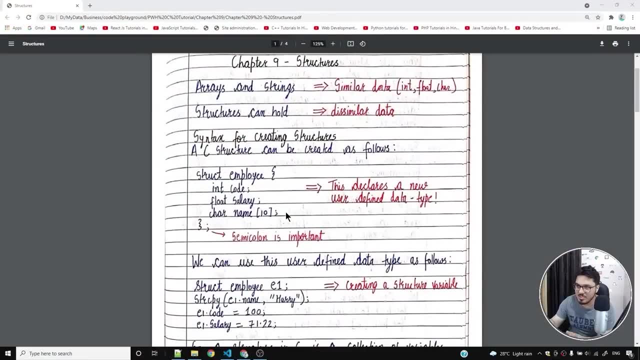 Those kinds of concepts will seem very easy to use. So structure is something that was introduced decades ago. It's been around for a long time, But still it's going to be a very important concept for you. So let's try to understand what a structure is. 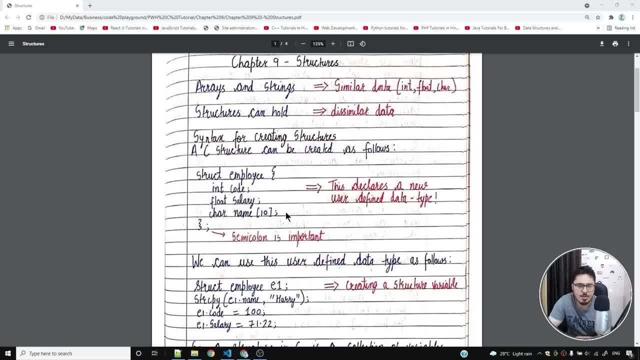 So let us say we have an array and we want to store two numbers inside that array. We can do that right. We can create an array and we can start storing all those numbers inside the array and that will work. But let us say I want to create a collection and inside that collection I want to put 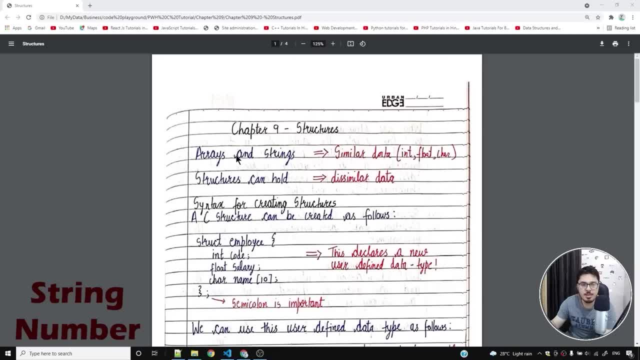 a number and a string. So if we talk about an array and if we talk about a string, what happens inside array is they hold similar data. Either you can create an array of integers, or you can create an array of strings, or you can create an array of characters. You can create an array of any kind of you know data type that exists in C programming language, But all those data types needs to be same. But what if I want to group together a collection That contains a dissimilar you know kind of data? 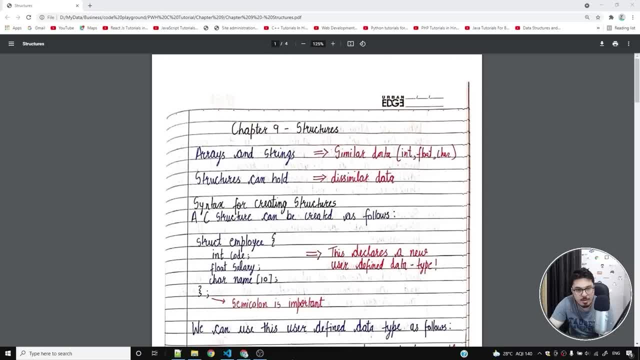 For example, let us say I want to hold a number, a name, let us say an address, a phone number. All these kinds of data are not of the same type. Some of these data types are integers. Some of these data types are going to be strings. 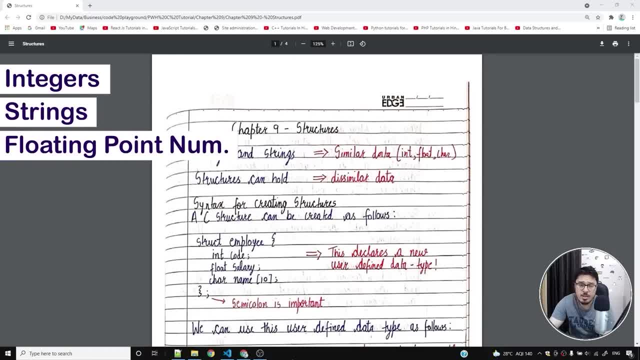 Some of these data types are going to be floating point numbers as well. So what we want to do is we want to group together dissimilar data. Okay, We want to create something that helps us do that. So structure is nothing but a way for us to hold dissimilar data in C programming language. 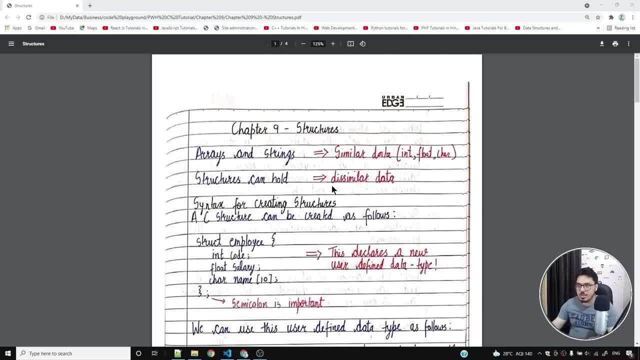 So this is something that we need to understand first. Now let's look into the syntax for creating structures in C programming language. So what I'll do is I'll simply start by writing a program, and I'm going to write a very basic program so that you can understand how structures work in C programming language. 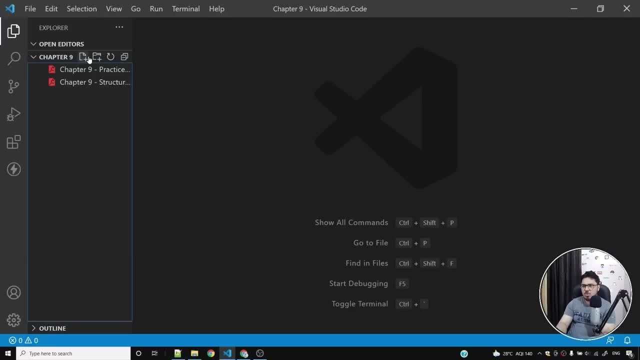 So let me create the very first program and I'll name it structure Or struct, And what I'll do is I'll simply say boilerplate code, so that I can put the boilerplate code inside my program. Now what I'll do is I'll use the syntax and start creating a structure. 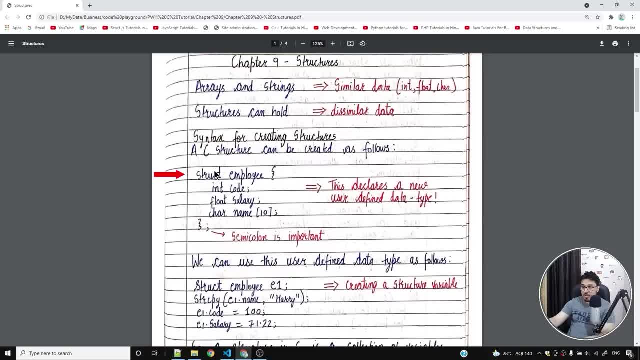 So a C structure can be created as follows. As you can see, I've written a struct keyword. Struct is a keyword that is used to create structures in C programming language, Then employee is a name chosen by me. It is just like a variable in C programming language, just like we created int. a is equal. 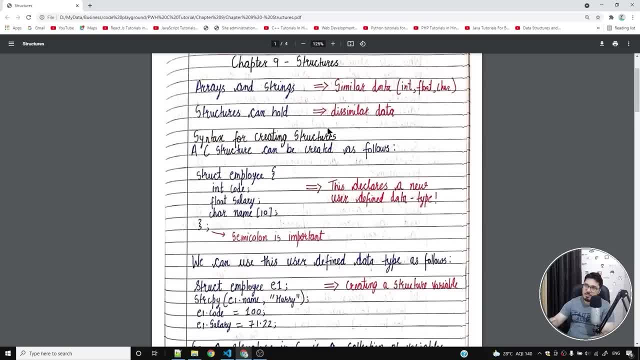 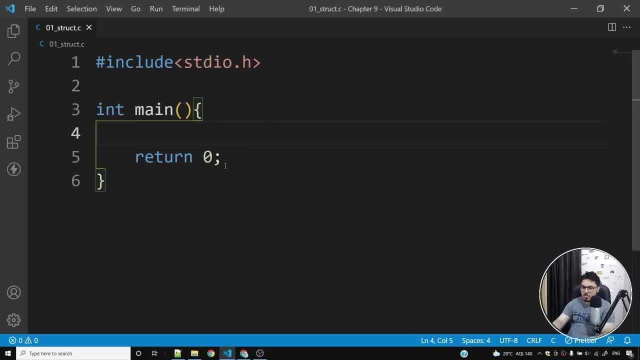 to seven, We can create: int employee is equal to 32.. Okay, So, in a very similar fashion, what we can do is we can say struct employee and we can start creating the structure. So let me show you something. What I can do is I can write something like this and I'll say: struct employee. 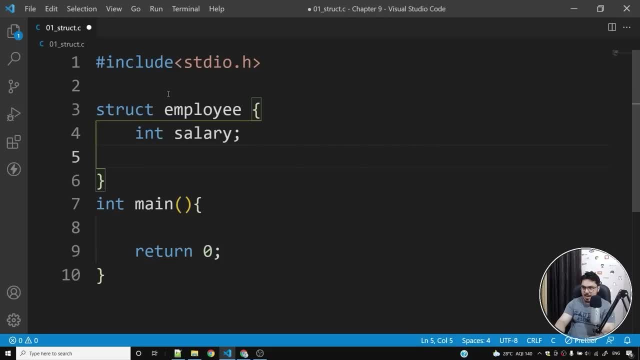 Now I can say int salary, let us say the salary is an integer. And what I can also do is I can say float hike. And these two are together are different data types: integer and floats Hike is a floating point number, salary is an integer. 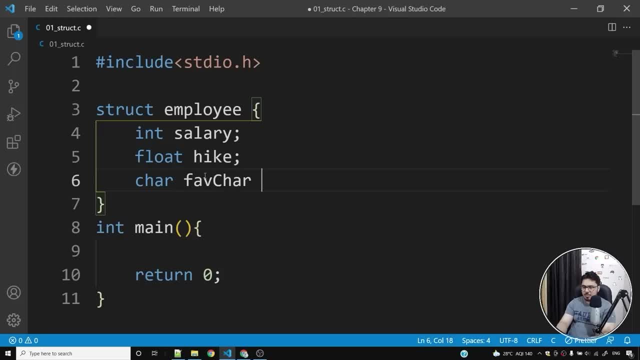 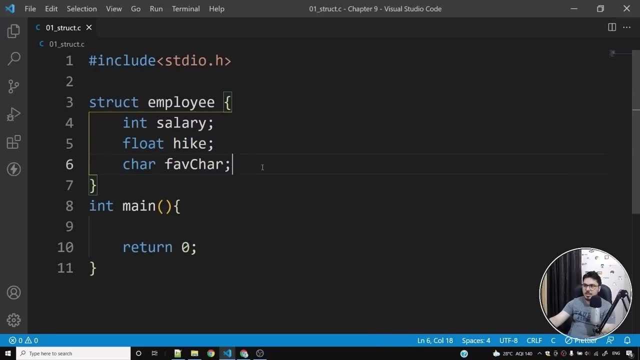 Let us say I also want to create a favorite character of that employee. for some weird reason, I want to store the favorite character of this employee. So all these three types of data types are different. Okay, In this example, what I've done is I've taken name his name as an array. 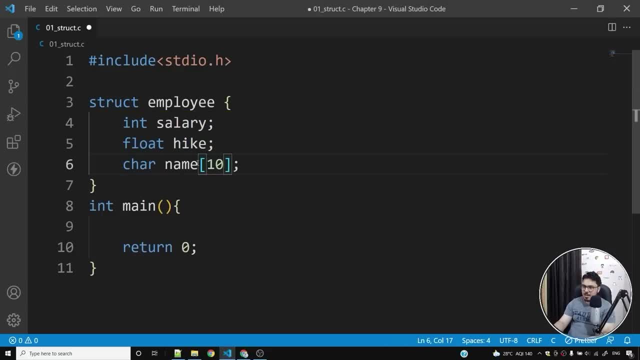 We can do that as well. So let me refactor this and let me say that the employee will have some name and that name will be stored inside this variable And it can contain 10.5.. Okay, Okay, 10 characters at most. 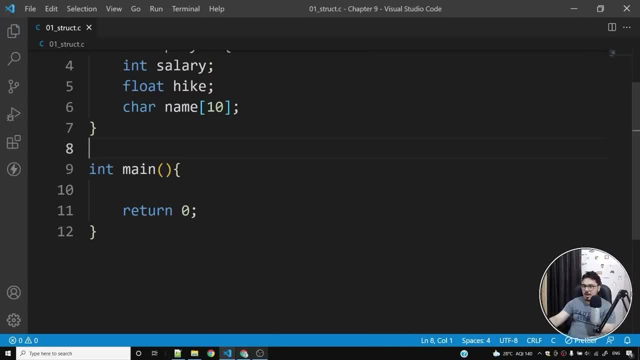 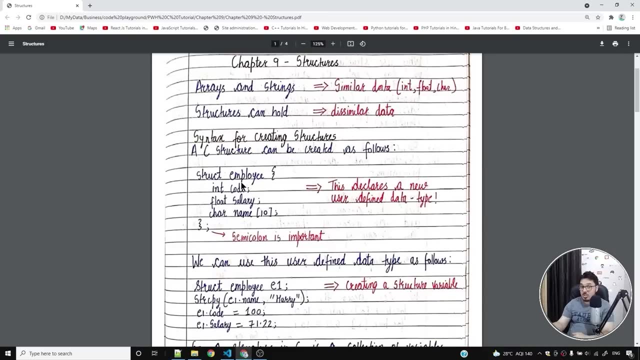 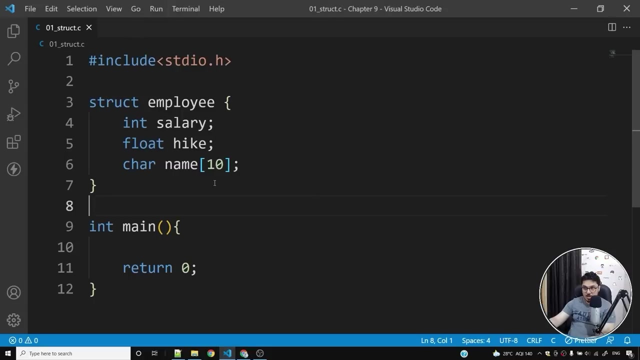 Okay, Now what I'll do is I'll save this program and you can see here that this declares a new user defined data type. So employee is just like an integer now, if that makes sense. So employee is a data type in C programming language for this program. 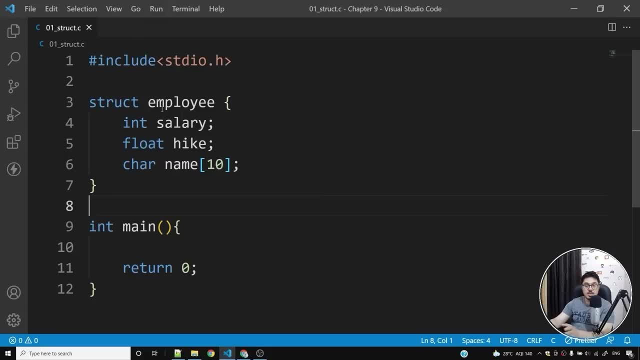 So I can say something like this: I can say employee E1, E2, just like I can say int A1, A2.. So something which is really very important here is a semicolon. I need to put a semicolon here. 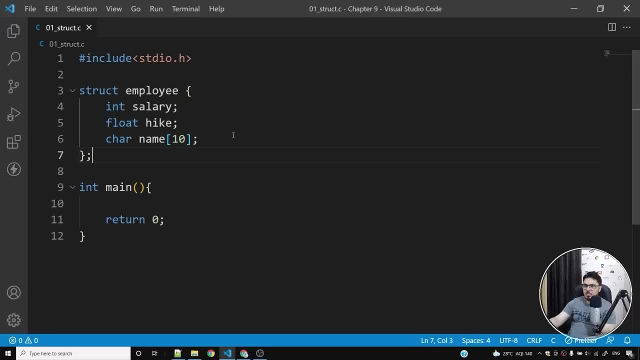 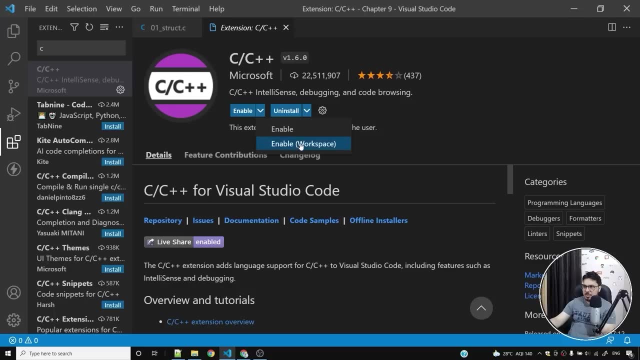 And if I run this program, let me show you something: where is my code runner? So I need to enable CC++ extension. I have disabled it by default because, you know, anytime I open some window, what happens is it loads all these extensions and my computer starts working slow. 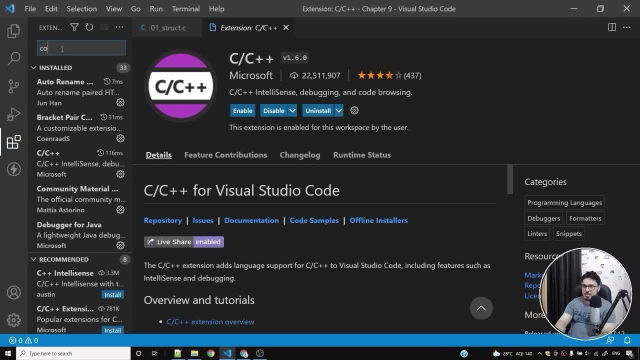 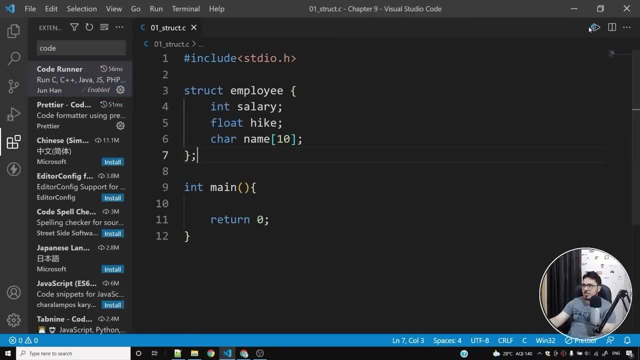 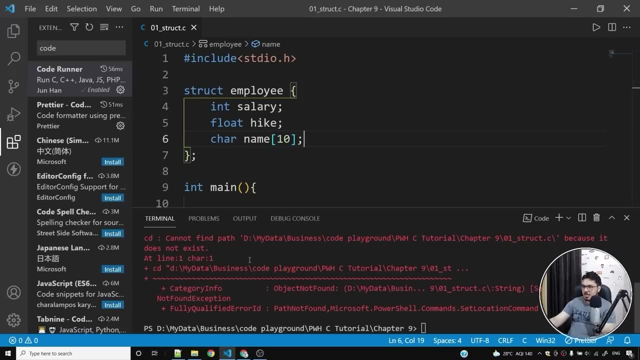 So what I do is I usually disable all these extensions by default. So I'm searching for code runner. I'll enable it for this particular window and I'll close it, And I'll close it, And then I should get this button. And once I get this button, what will happen is: so it is saying that cannot find the path. 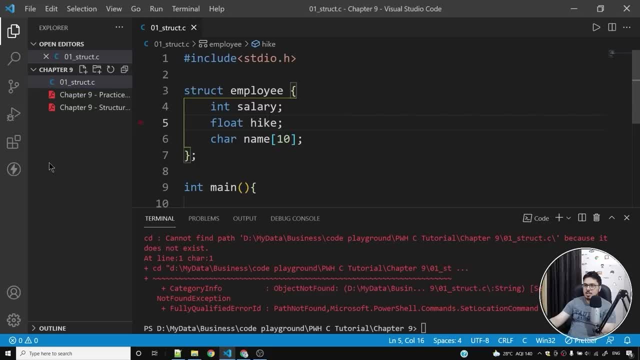 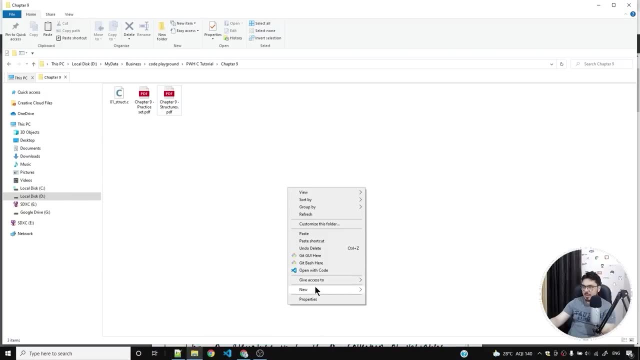 What's wrong with this structure? structc. Everything seems to be fine. If I run this, this is not working. Let me load the Visual Studio Code window once again. I don't know what the problem is, So I renamed my program and it worked. 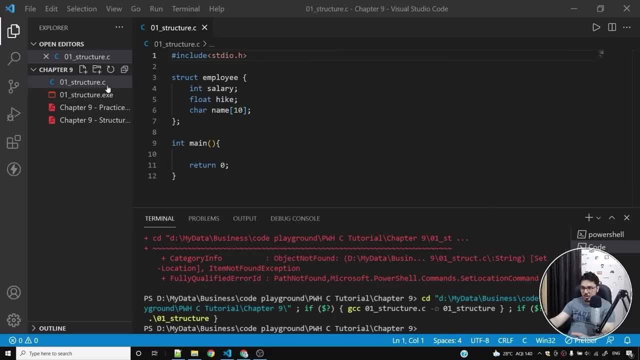 I think I accidentally added a backslash while I was naming the program, But anyways it works. So if I show you this program, it runs without any error. So I'm going to show you this program: It runs without any error. 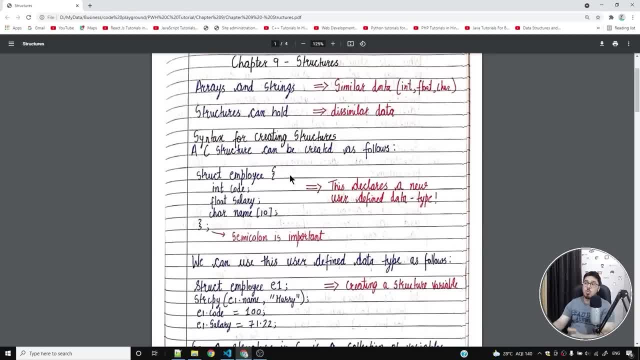 It runs without any errors and warnings, which means that this syntax works fine. So what I've done here is I've created a custom data type. Now, if I want to use this custom data type, I'll have to write something like this: 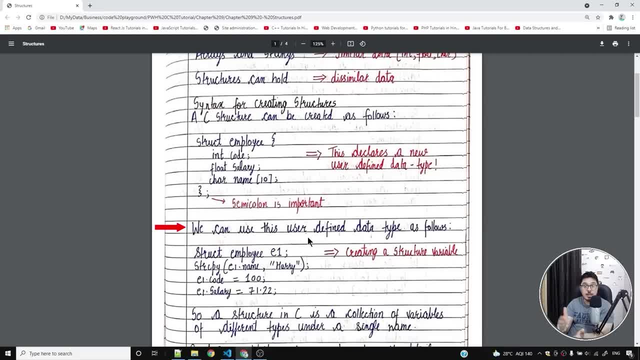 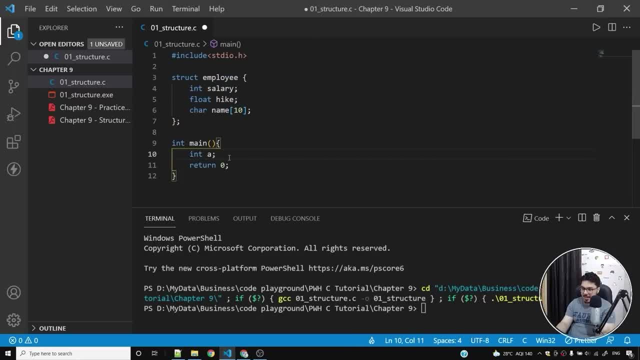 We can use this user defined data type as follows. I can say: struct employee- even Now even is an employee. So let me show you something. I can do something like this. I can say: int a is equal to 45.. And I can say: struct employee, employee harry. 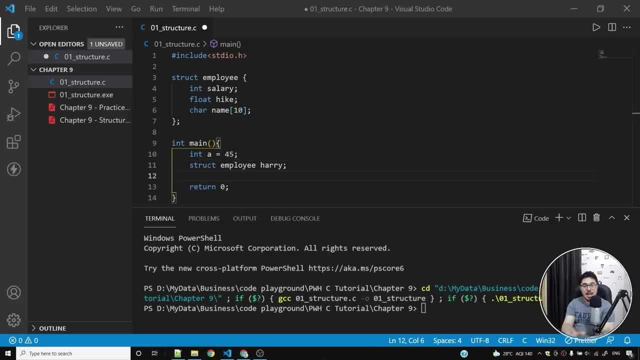 And I can say: int a is equal to 45.. And I can say: struct employee employee harry. And I can say struct employee employee harry, And harry is now a variable of type employee, So I'll have to write instruct employee completely. 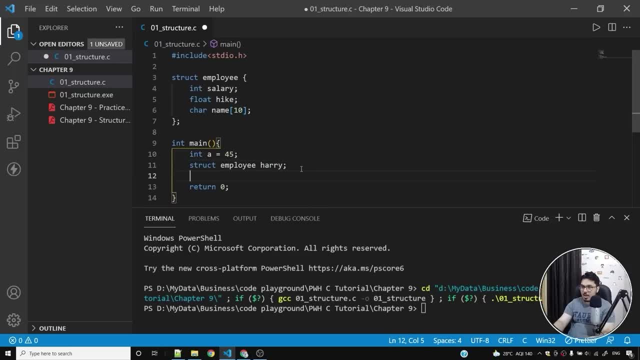 I cannot say employee harry. This is the rule. So I can now do something like this: I can say harryname is equal to harry And I can say harryhike is equal to 5.3.. I can say: let me write harry here. 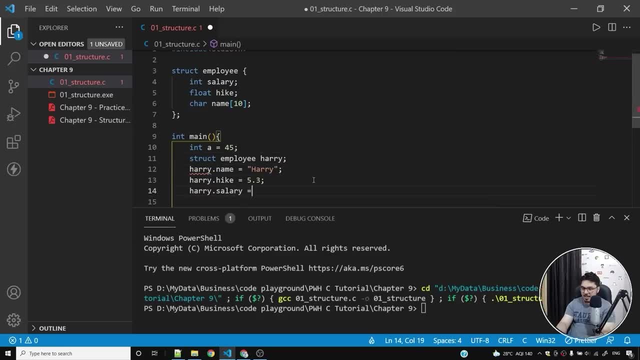 I can say: harrysalary is equal to 10.. Okay, so i can do something like this. okay, let me. let me add a couple of zeros here. okay, that sounds good. okay, so i can say: harryname is equal to harry. i can do all these things. what is it telling me? 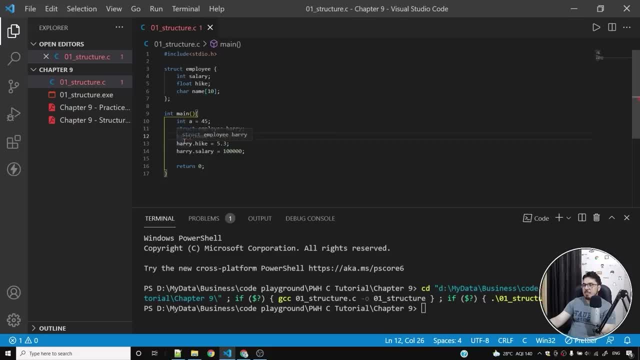 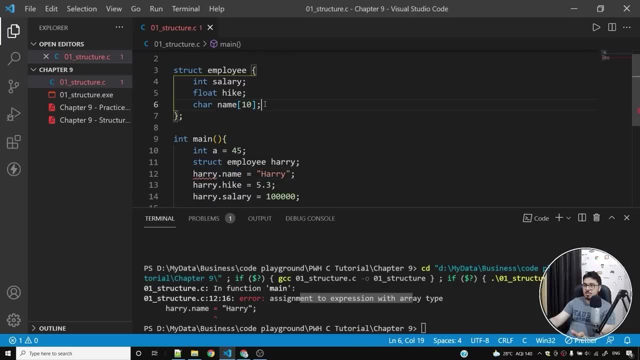 it is saying that expression must be a modifiable l value. so this is throwing me an error, because it is just telling me that harryname is simply the address of the first character of this array and you cannot assign it to harry. so what i'll have to do is i'll do something like this. i will. 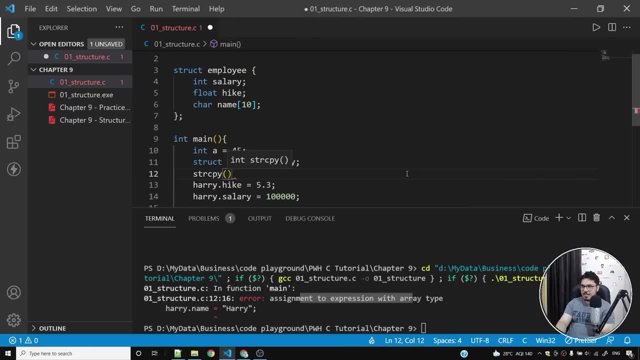 use str cpy and i'll simply say a name and i'll say harryname, and then what i'll do is i'll say harry, and this should work, and what i'll also do is i'll import stringh. now let me run this. 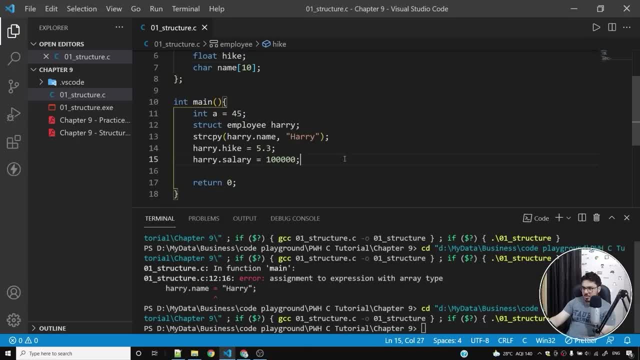 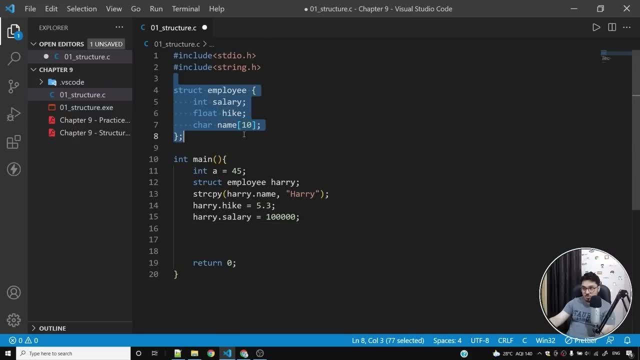 program and let me show you that this works. so i have not done anything so far, but let me tell you. what i'm going to do is i'm going to import stringh and i'm going to import stringh that i can use all these uh variables from employee structure and i can print them out. 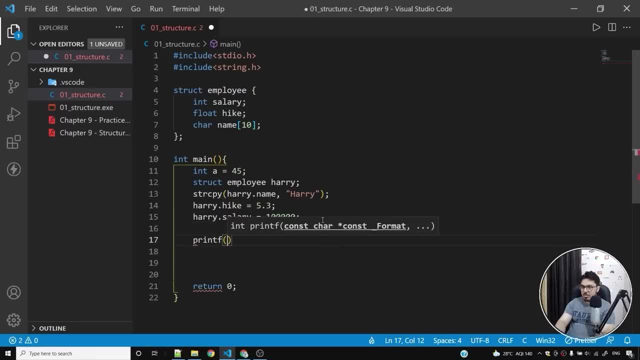 on the screen. let me show you what i mean by that. i can do something like this. i can say the name of the employee is, let me say percentage s and i'll say harryname. then i can also say that the salary of employee is percentage d. i can say harrysalary. then i can do percentage. 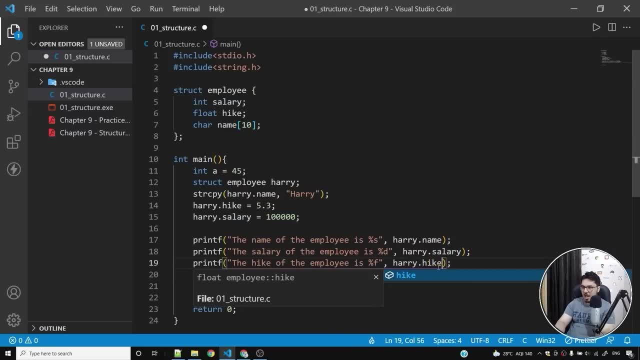 f, i can say hike of the employee is harryhike, because harry is the name of the employee variable. just look at this struct employee as a new data type, just like you are looking at integers, just you are looking at floats. look at this struct employee in a very similar manner. 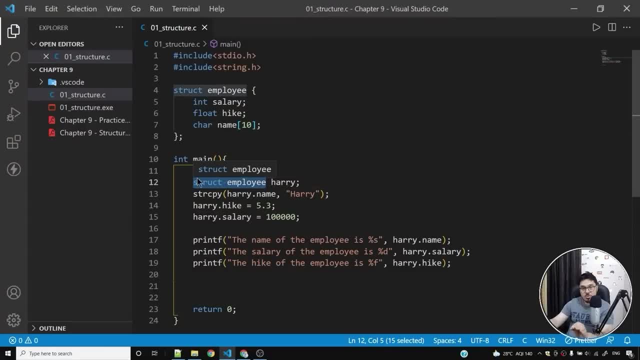 struct employee can now be used to declare structures or other structural variables of type employee. okay, so i. so harry is just like a variable. the only difference between the two is between this variable and the variables that we have seen so far- is that there are variables. 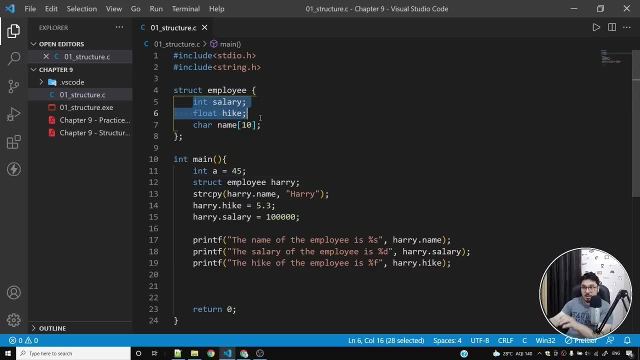 inside this variable. so harry has three variables. i can use these three values. so it's a collection of three different things: name, salary and hike. okay, i hope you understood that there is no other way in c programming language, using arrays, using string or using some other method to group all. 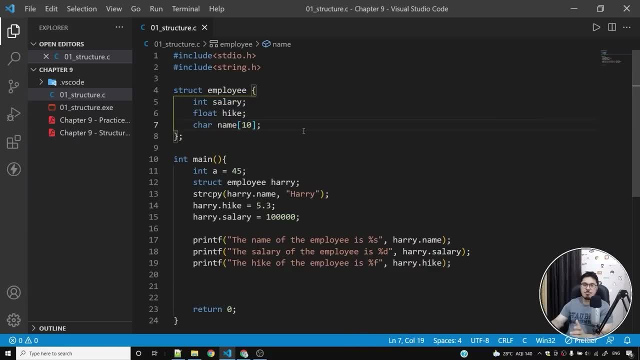 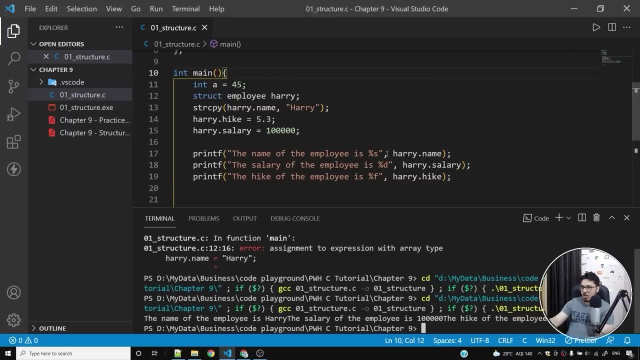 these things together. so this is something that was brought into the c programming language to solve this problem, problem, okay. now, if i run this program for you, you will see, uh, all these things printed on the screen. let me also say backslash n, so that you, you know, you can see the new line after this is: 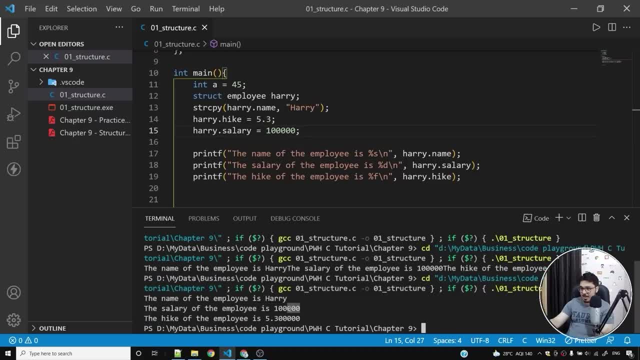 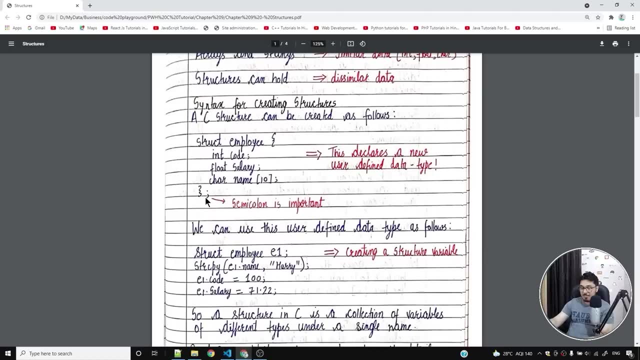 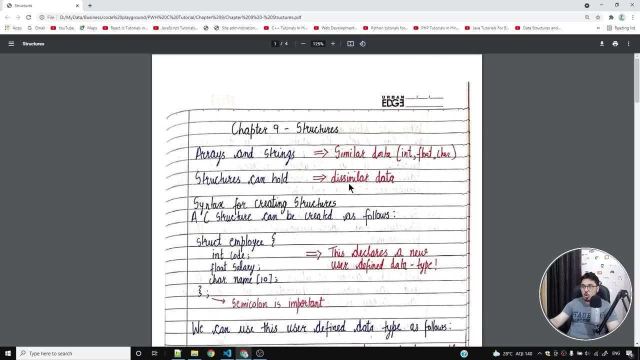 printed. so the name of the employee is harry, salary is uh, i don't know how many zeros i added. a hike of the employee is 5.3 and this is amazing. okay, because this solved a very big problem for us, which was grouping dissimilar types. so dissimilar types of data was not grouped by a. 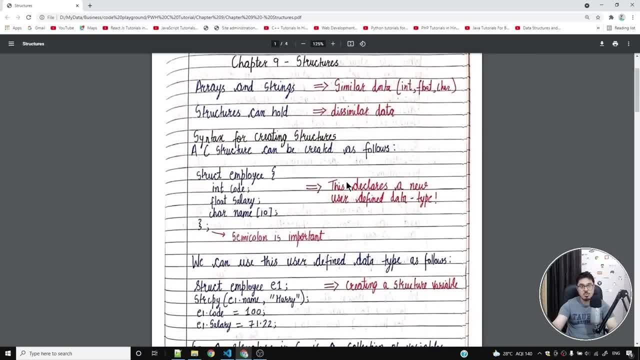 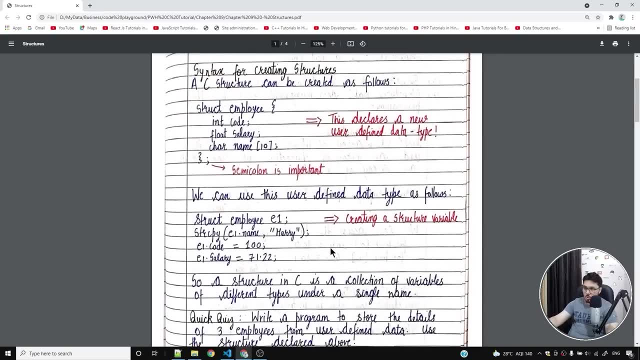 entity. now we can group this data types using structures. okay, so sammy colon is important. i have written these notes really very beautifully for you. make sure you download all these nodes. so a structure in c is a collection of variables of different types under a single name. 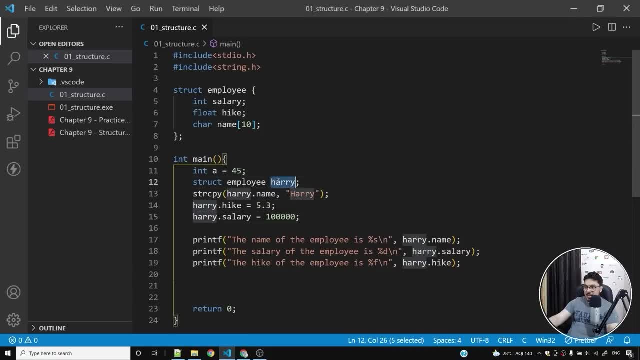 so what is that single name? single name is harry. harry is a structure, employee type structure which i have created. so this is just like a data type. this is just like a, like a float, or double for that matter- and harry is the name of the variable, just like a. now, i haven't used this. 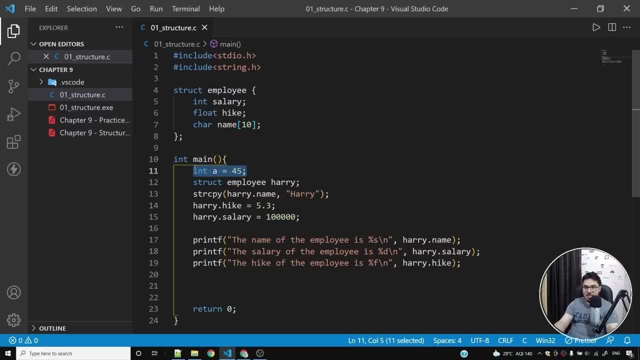 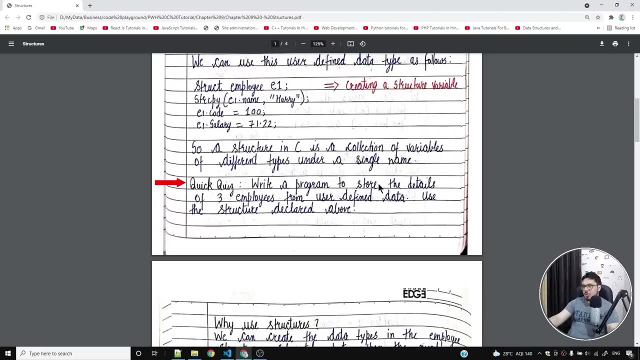 a, but i just wanted to tell you, just like we have a, we have harry. okay. so, coming back to the notes, let us see what this practice set is telling us. write a program to store the details of three employees from user defined data. use the structure declared above. so what we want to do is we want to 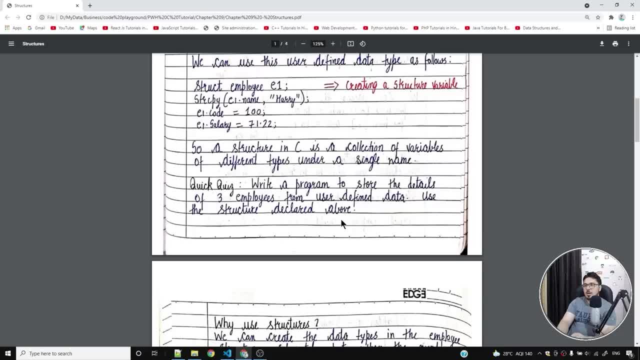 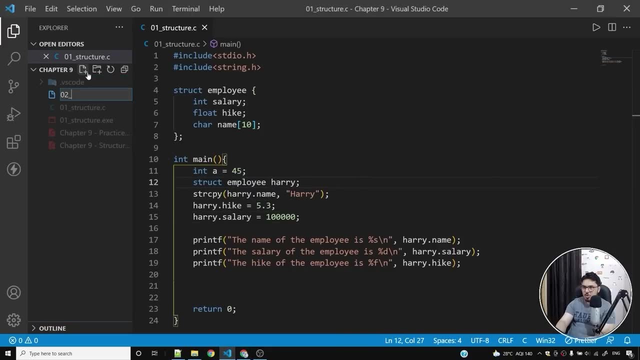 use a bunch of scan f's and a bunch of printf statements to take the user input and then display it on the screen. so let's do this. okay, let's, let's try to do this. what we are going to do is we are going to use the same program, but i'm going to create a new program. i'll say quick. 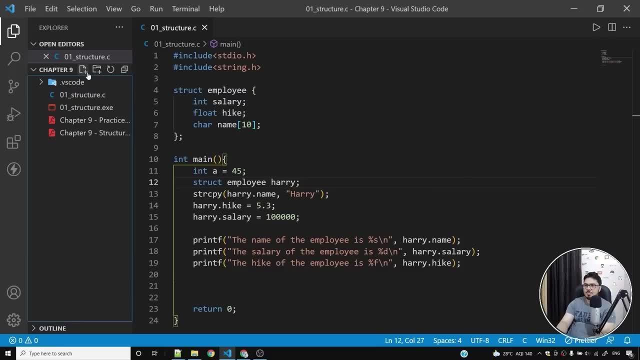 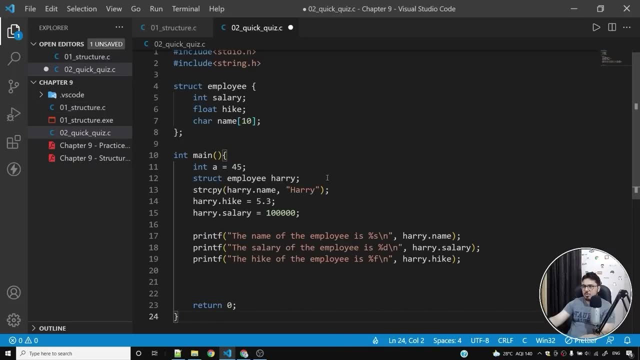 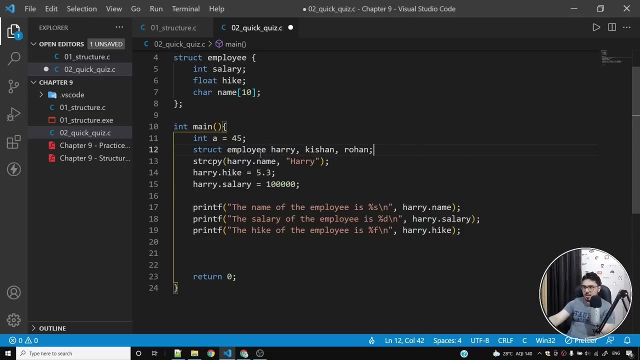 underscore: quiz dot c: i'll add the boilerplate code. but i'll not add the boilerplate code. i'll simply copy this program. what i'll do is i'll simply say harry, then i'll say kishan, then i'll say rohan, okay, so what i want to do here is i want to take the information from the user, so i'll say: 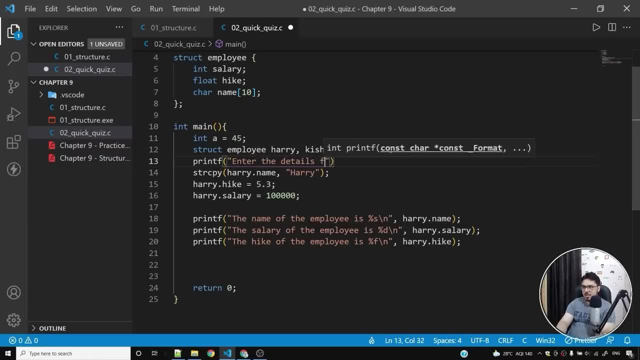 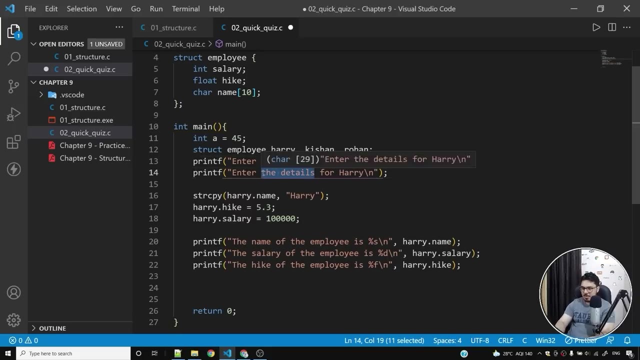 enter the details for harry. enter the details for harry. now i'll use backslash n and i'll also put a semicolon. now i'll simply say enter name. so let me use uh: enter name for harry. then i'll say: enter salary for harry, then i'll say enter hike for harry. and while i'm doing all 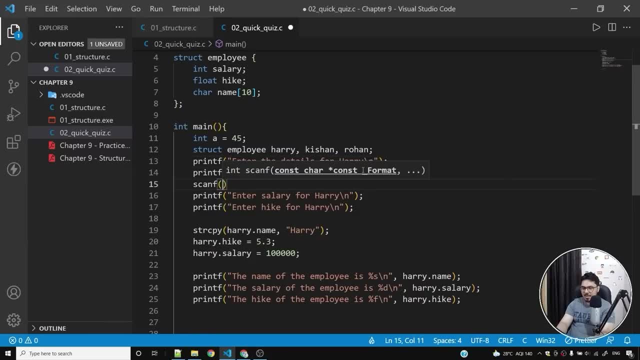 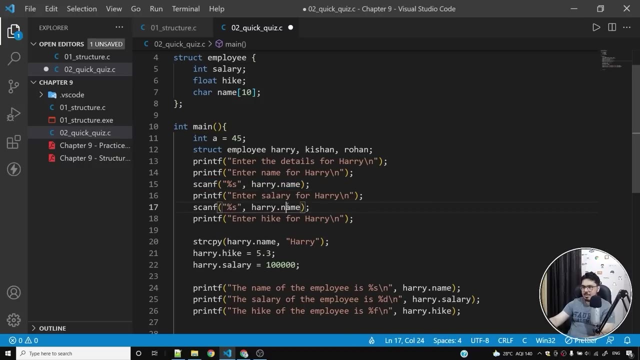 this. i'll use scanf function. i'll simply say scanf and i'll simply say percentage s for the name, and i'll say harry dot name. okay, now what i'll do is i'll simply copy this scanf. i'll do the same for salary. so salary is going to be an integer. i know i'm doing a lot of work here. 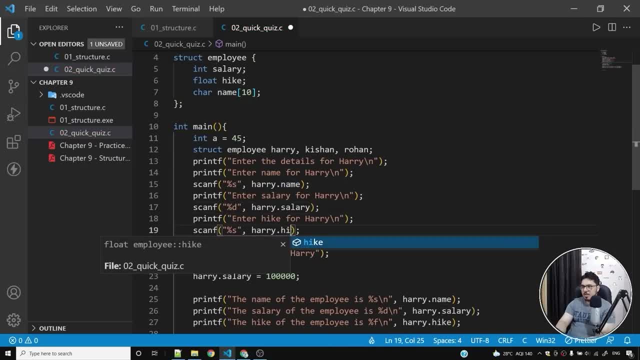 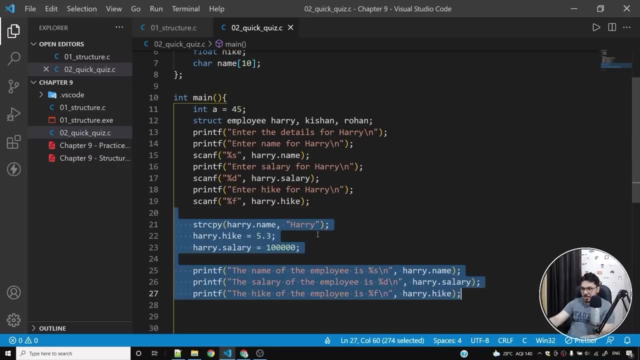 of typing, but that's because i want you to get this concept very clearly. so i'll say: percentage f. this will take the floating point number entered by the user and store it into harry dot hike. now let me get rid of all these things. now i have to do the same thing. i have to do the same thing. 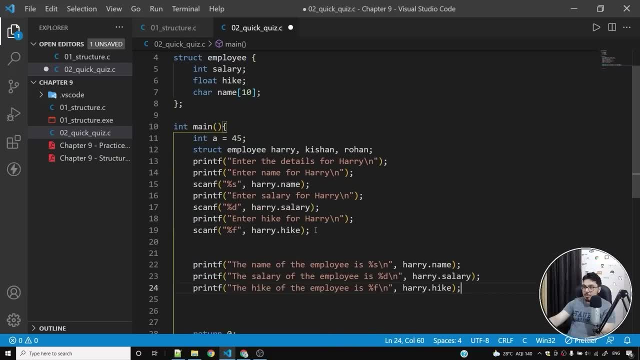 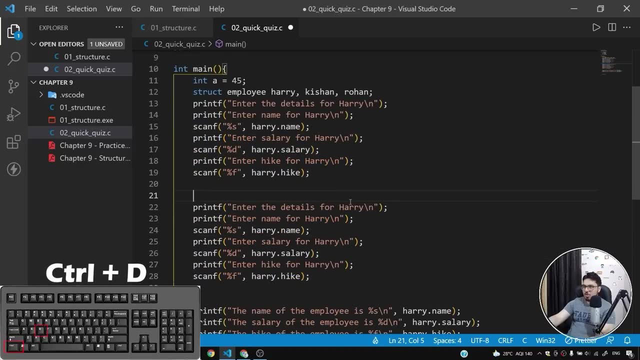 let me get rid of this one, because we'll need this one now. let me do the same thing for other three employees, so let me do control d now. i'm copying a lot of code which violates the dry principle, so we are not going to worry about that. dry principle is nothing. 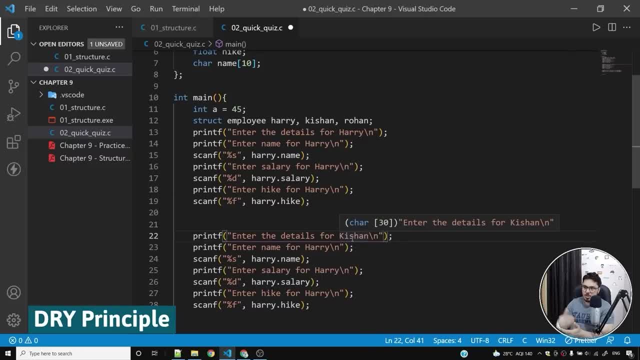 but do not repeat yourself. dry principle says that do not repeat yourself. something that you have already done should be kept by you, and it should be reusable in a way that you don't have to reinvent the wheel again and again. okay, so we are going to do the same thing for kishan. 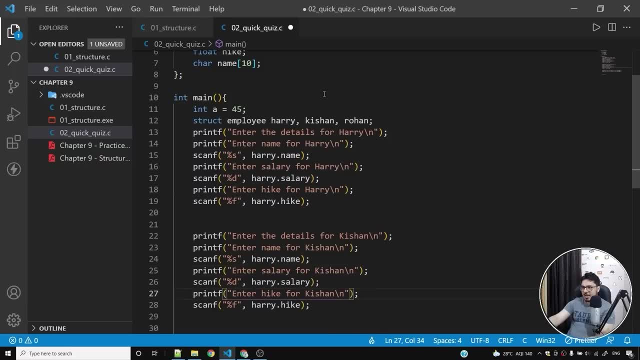 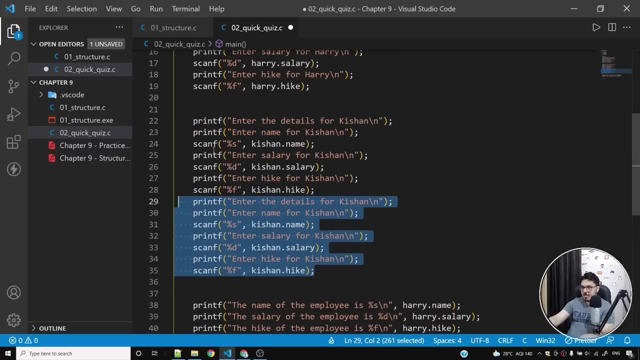 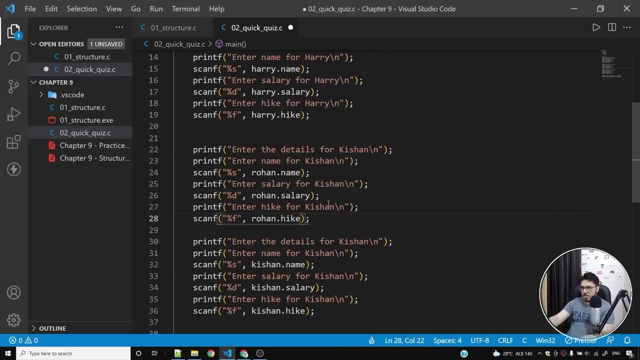 i'll replace harry with kishan and i'll also replace all these structure variable names. now i'll do the same thing for rohan. so let me do the same thing for rohan. i'll say rohan dot name, rohan dot salary, rohan dot hike, and we'll also replace all these values with rohan. 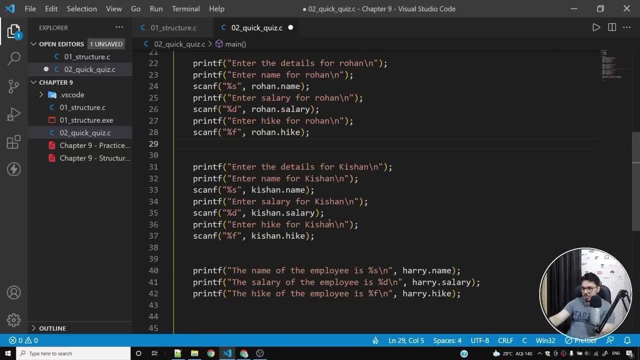 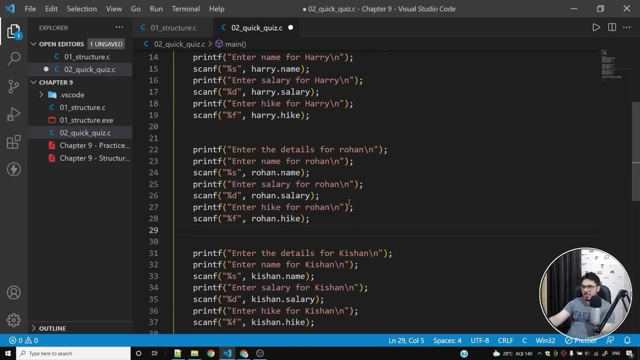 okay, let me use control s. so we have taken user input so far. now what we'll do is we'll print all these things. so harry, rohan and kishan- okay, so these are the three employees. okay, now what we'll do is we'll print the name of the employee and we'll print the name of the employee and we'll. 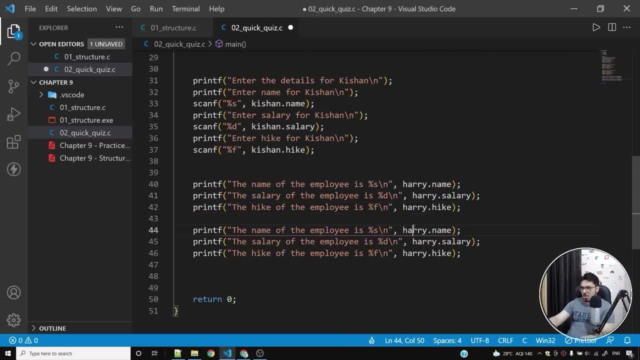 do the same thing for rohan and we'll do the same thing for kishan. so we'll say kishan, i'll copy, i'll paste, i'll paste. the salary of the employee of kishan is: so i'll have to replace this with kishan. 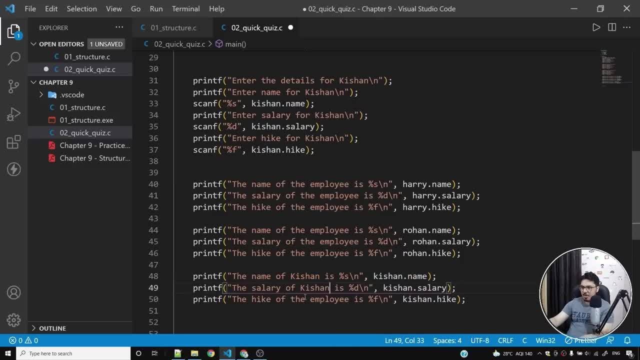 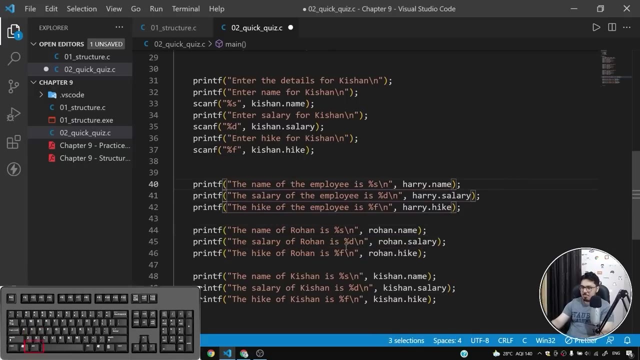 i know that's a lot of typing, but bear with me, i'll quickly do this and also i'll replace all these values with with rohan's. okay, so i've used multi cursor functionality of vs code which simply, you know can be done by pressing alt key and clicking wherever you want the cursor so you can press. 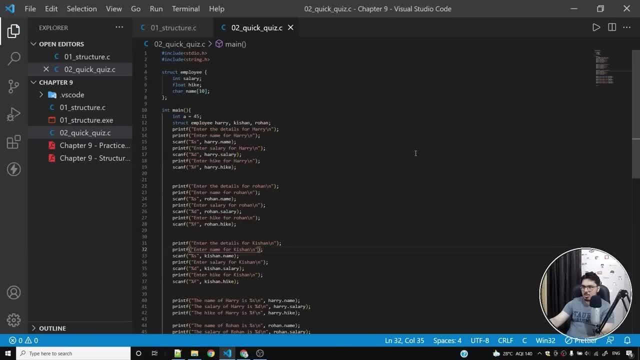 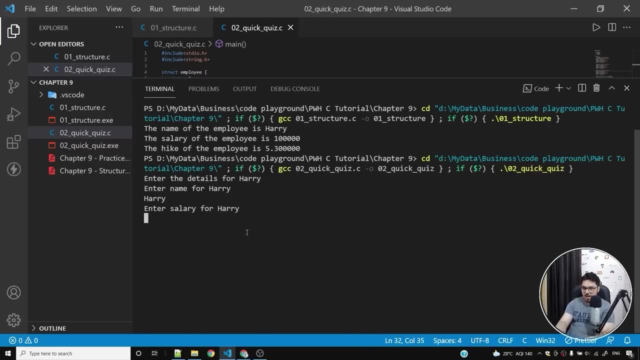 alt key and you can keep clicking and you'll see the magic of visual studio code. so let me run this program. so it says: enter details for harry. enter the name for harry. i want to enter harry. salary is 34 rupees and hike is 4.2. now the program ended. what went wrong? 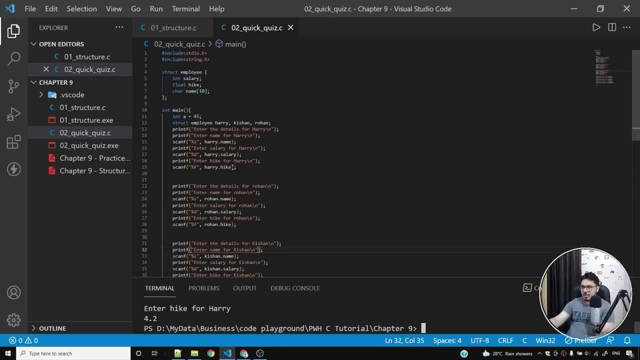 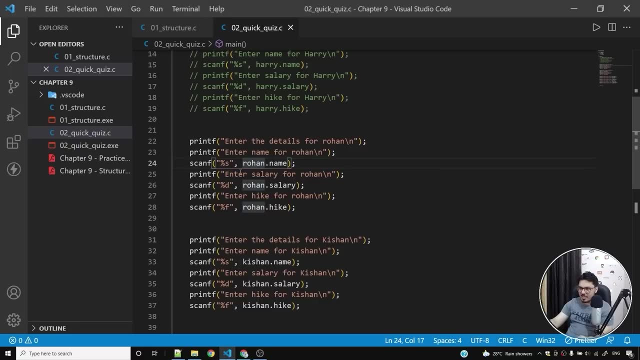 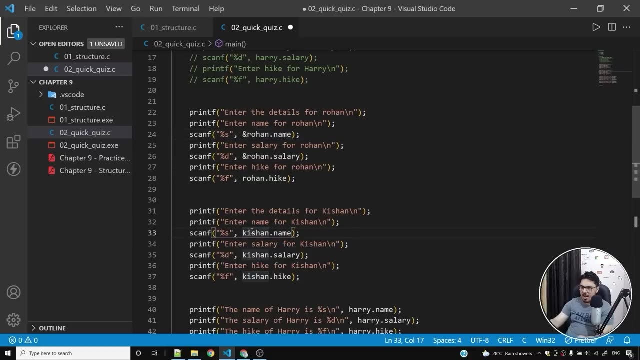 let me check. let me check what went wrong. so enter the hike for harry: uh, harryhike. so i have made a major mistake here. so what i'll do is i'll simply use ampersand here. i forgot to, you know, take the address of all these variables. i'll do the same thing here and i'll not do the same thing for. 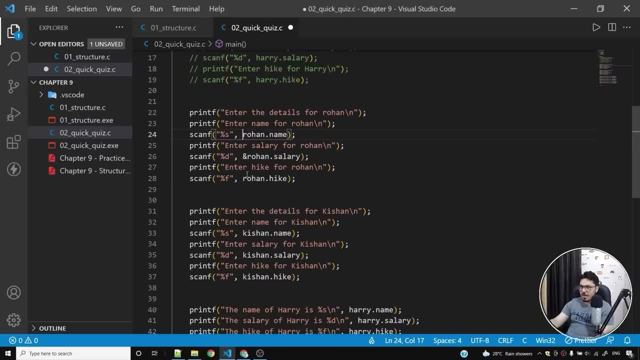 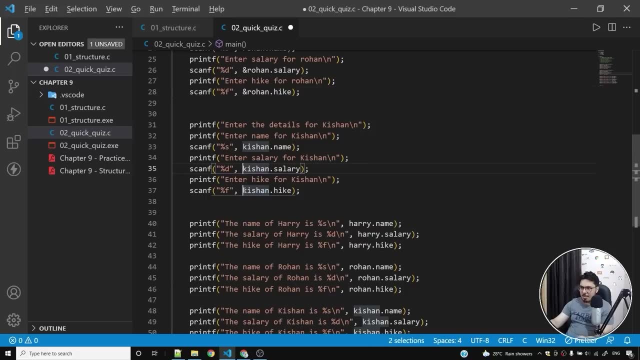 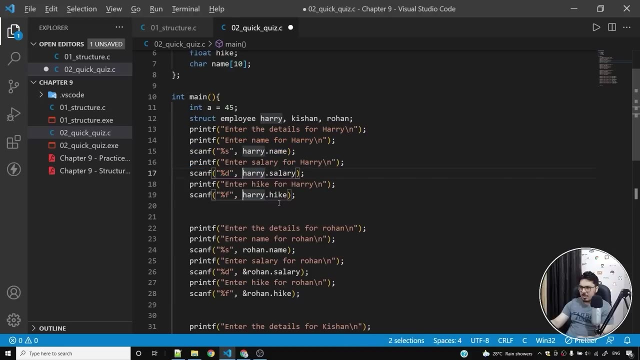 string because, um sorry, i don't want to put a ampersand here. i'll simply put an ampersand here and here, okay, so let me also put the ampersand for, uh, kishan's salary and harry's salary. so let me do the same thing for harry's. 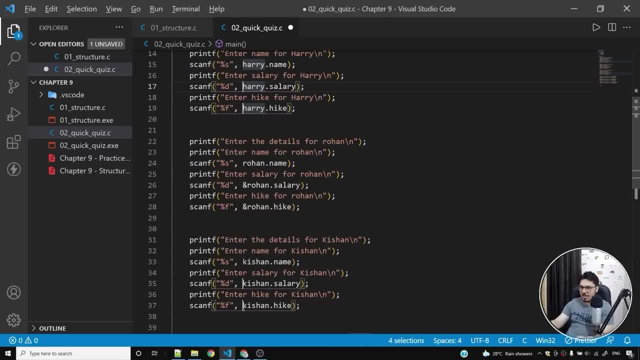 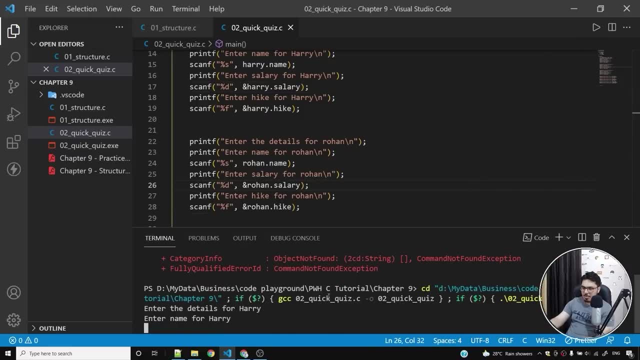 salary, and also for kishan's salary and hike. so i'll use ampersand here and now. this program should work. so let me run this program. uh, i accidentally selected the program, so i'll say: enter the name for harry, it's harry. let us say: 45 high can be 5.2. then again it asks the same thing for rohan salary. 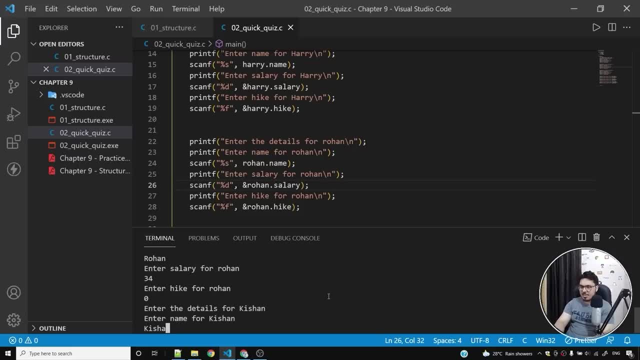 hike for rohan is going to be zero. i'm very sorry about that. uh, kishan, and then salary 477. he's the richest guy in this company. hike is 9.7 and you can see that all these values are printed on the screen. so the name of harry is harry, salary of harry is 45, hike of harry is 5.2 and all these. 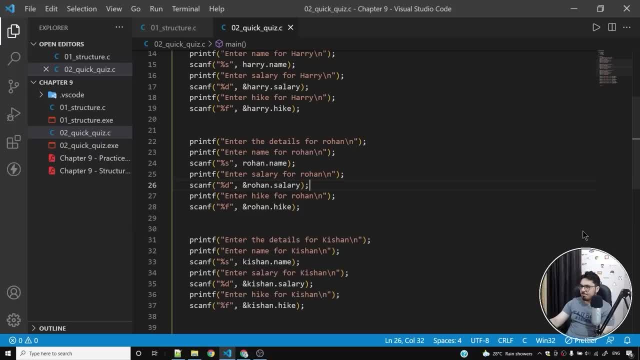 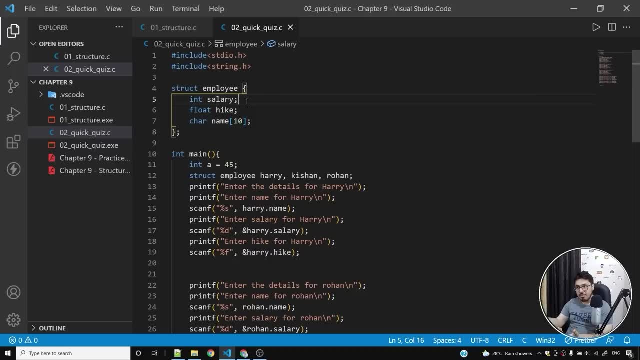 values were stored in a very compact way because we were using structure. we could have done the same thing by creating three different salary variables, three different hike variables, three different name character arrays, but we do not want to do that because we want to create an organized pattern to store our data. okay, so this was a quick quiz. now let's talk about why should 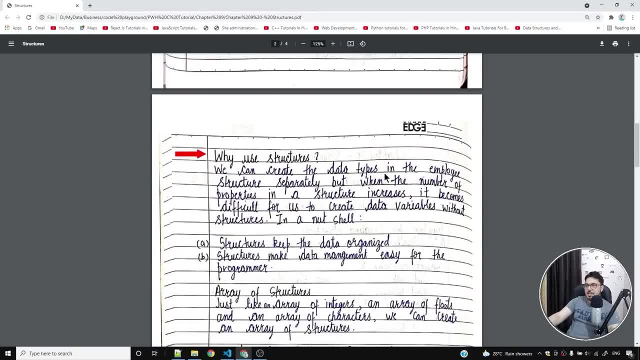 we use structures. why use structures? now we can create the data types in the employee structure separately, but when the number of properties in a structure increases, it becomes difficult for us to create data variables without structures. so what happens is, let us say we have three employees in. 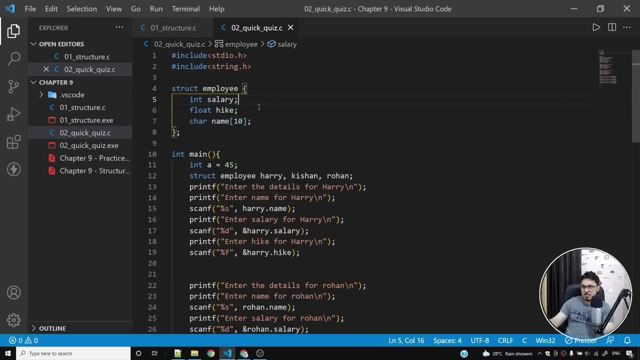 this case you might think that how about creating three different salary variables, three different like variables and three different name character, that is saying name underscore harry, name underscore kishan, name underscore rohan, and the same for hike- underscore harry, kishan and rohan. but we didn't do that. 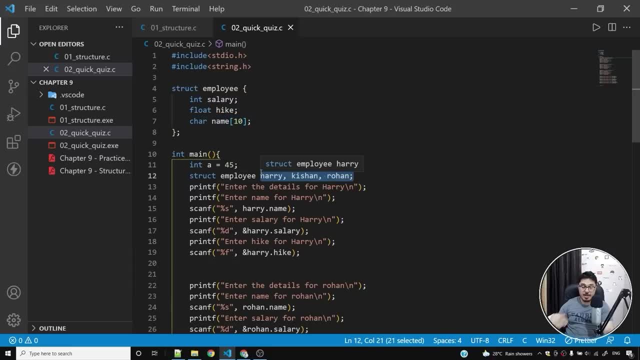 because in this case we had only three employees. but you might encounter a situation wherein you will have, say, seventy thousand employees, eighty thousand employees. in that case, it will not make sense for you to create eighty thousand, seventy thousand variables. okay, this was fun. now, the reason why we are using structure is: in this case there are only three data types. but what if the 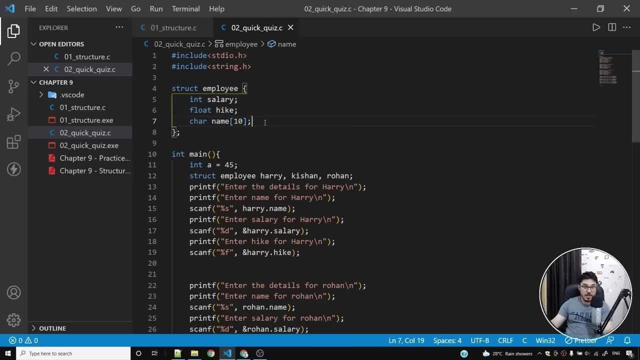 number of data types are, say, 20 or 40. now you might be wondering why would there be 40 different types inside a structure? but let me tell you something: when the complexity of a program increases, you will definitely encounter programs with this level of complexity. so 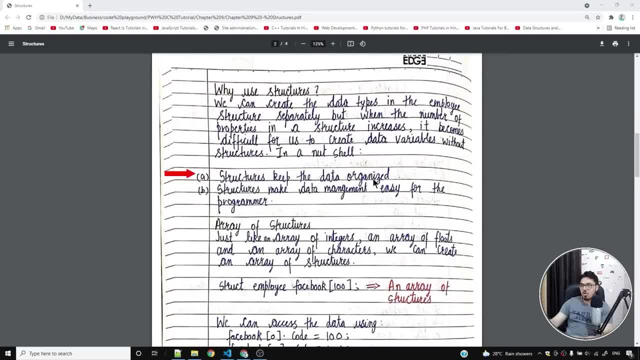 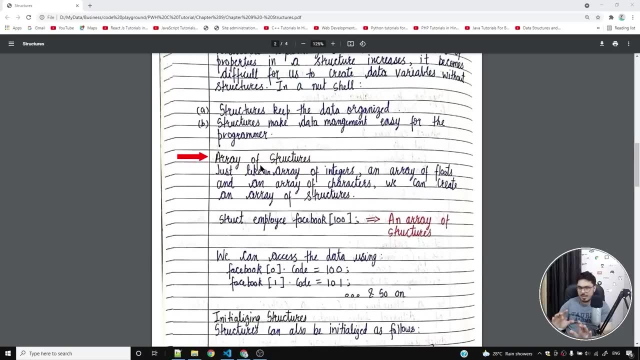 i've written it here in a nutshell: structures keep the data organized, so structures help you keep the organized structure, make data management easy for the programmer, just for the reasons i just told you. okay, now array of structures. so we'll talk about array of structures just like we create. 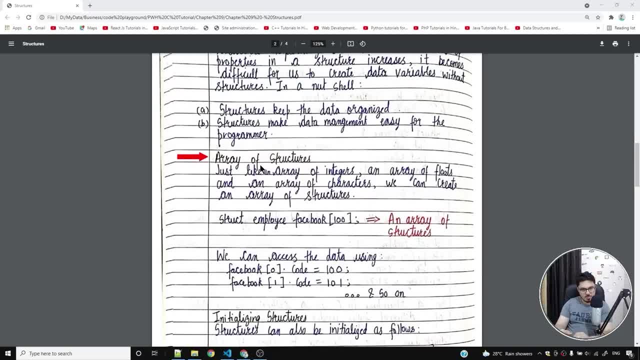 integer arrays. we can create array of structures. so what we can do is we can say: struct employee facebook 100 and this structure can hold 100 employees. okay, just like int a 100 can hold 100 integers. so this facebook variable is an array of structures. now this might sound really. 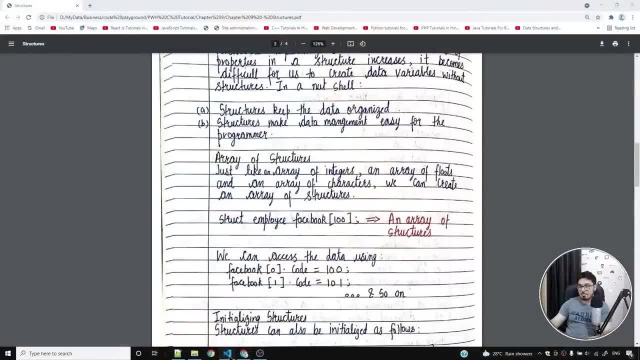 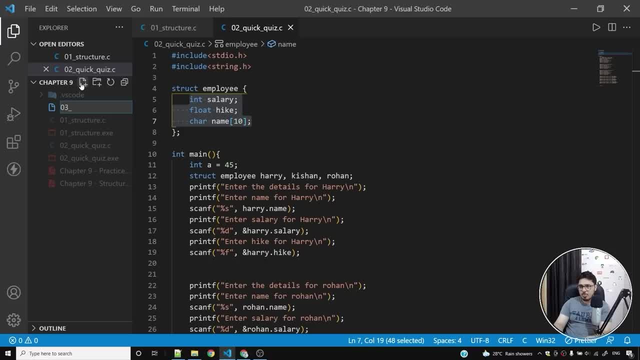 very confusing to you if you are a beginner. but bear with me, let me write a program for you so that this, this will become, you know, really easy for you. so what i'll do is i'll say: array of structs, dot c. i'll put in the boilerplate code. let me copy this structure because i'm not going. 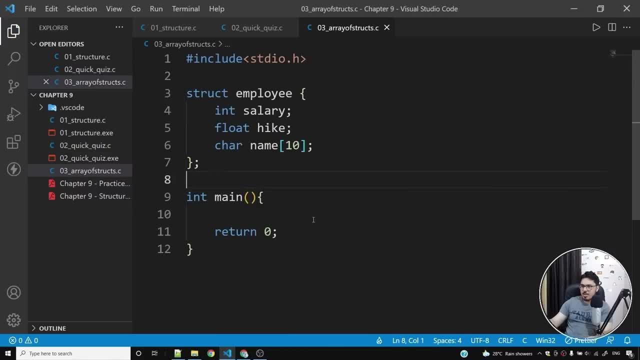 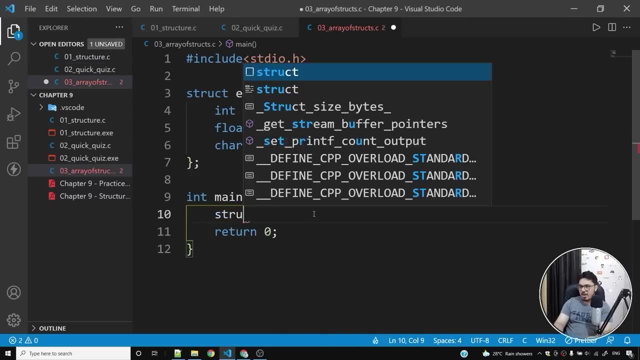 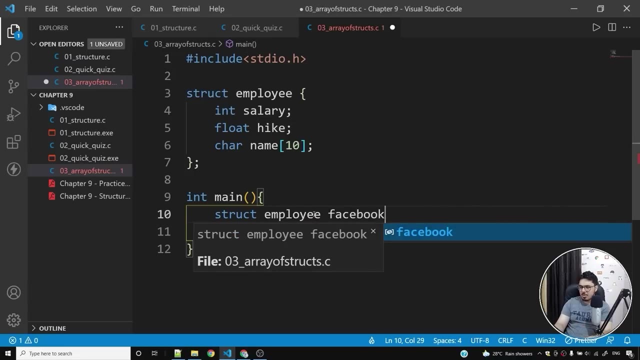 to type this again and again. i'll reuse it now. what i'll do is i'll say struct employee- i misspelled struct, and i don't want to use a snippet. i want to say struct employee and i can say something like this: i can say facebook and i can say 10. now, this array is actually capable of. 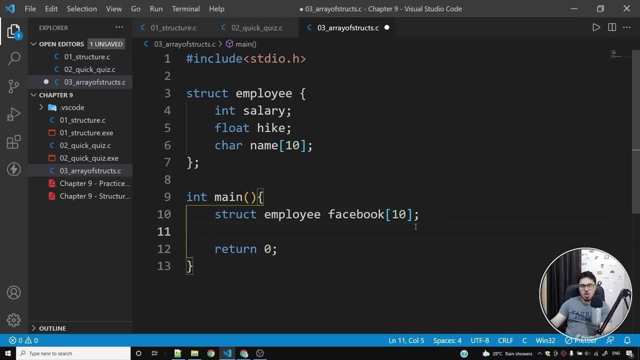 storing 10 different items or other 10 different employees from facebook company. okay, now it can be anything. i just wanted to, you know, present the data in a very meaningful way, so that you can see the data in a very meaningful way, so that you can see the data in a very meaningful way. 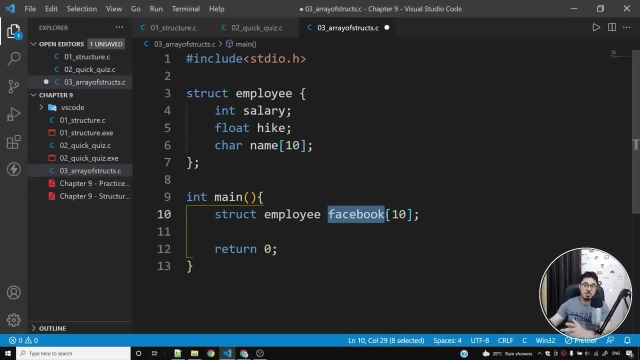 and understand that we are doing this for employees of facebook. but this can be anything. this can be a book, this can be, uh say uh, an electronic equipment wherein you will have the number of wires, the number of circuit connections. so it can be any complicated thing, but the basics. 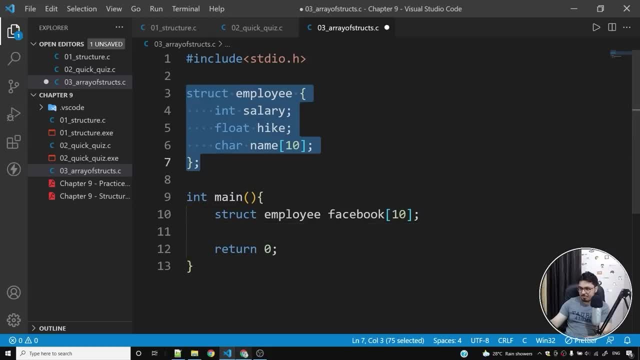 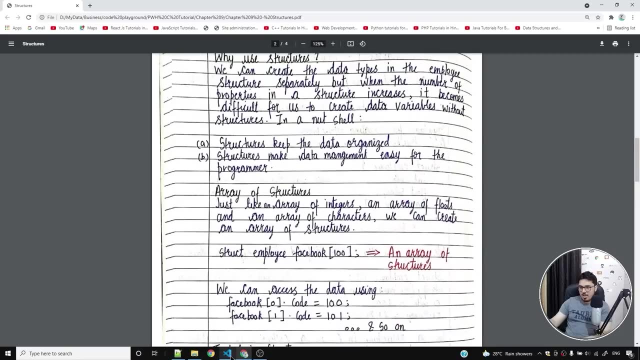 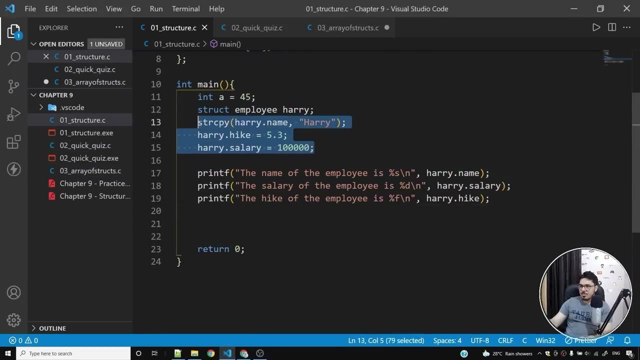 of c programming language and structures are going to be the same. okay, so what we can do now is we can access the data like this. we can say: facebook- zero dot code, facebook- one dot code. in this case, what i'll do is just like we have created our- uh, our struct employee, harry. what i'll do is i'll simply. 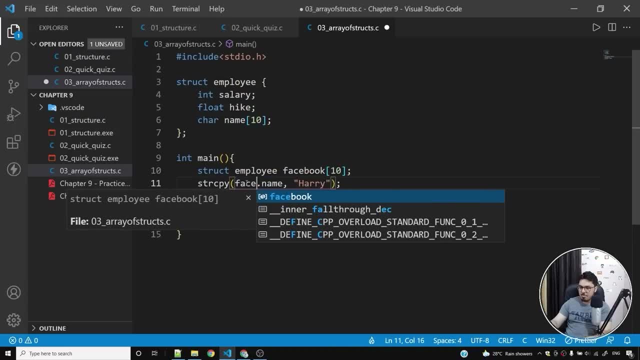 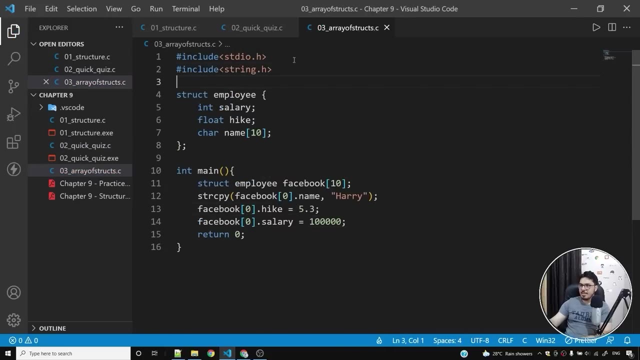 say, uh, facebook zero dot name. i can do something like this. so what i'll do is i'll replace all these harrys with facebook zeros. okay, let me also copy this and let me paste this. i'll save it now. what i'll do is: i will do the same thing. 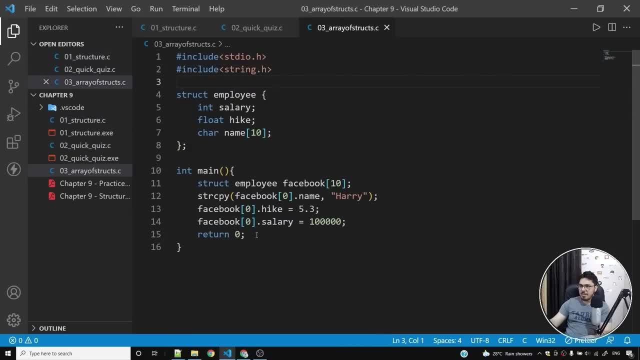 i did in the first program. i'll copy these printf statements and before i return i'm going to paste all these printf statement to print these values. so what i'll do is i will change all these harry variables to facebook zero so i can now run this program and show you that facebook zero was able. 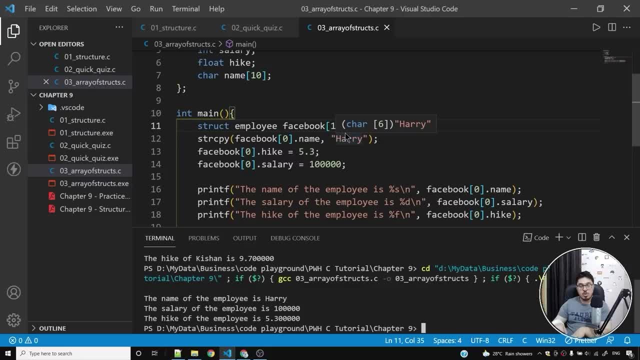 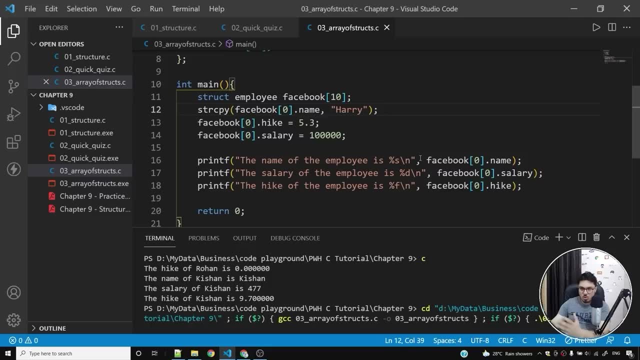 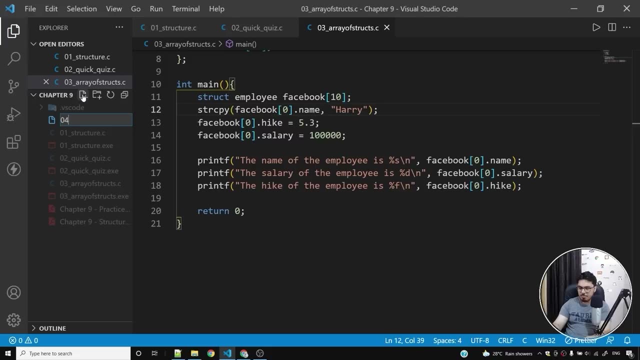 to store name employee- uh sorry, name, salary and hike of this employee. okay, so this is how it works and we can use facebook one, facebook two and facebook zero. one and two will store different structures. okay, let me also create a program which will tell you how we can refactor the 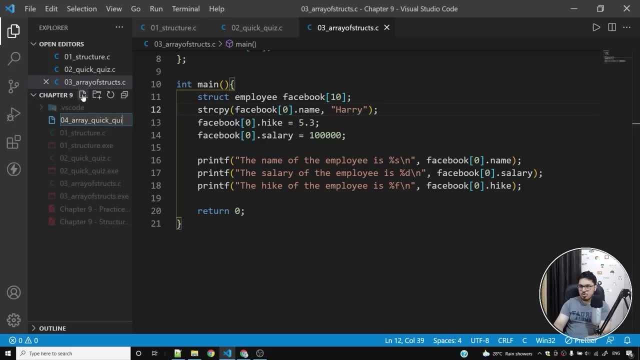 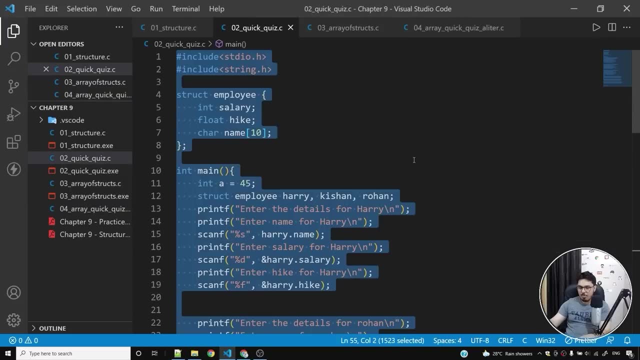 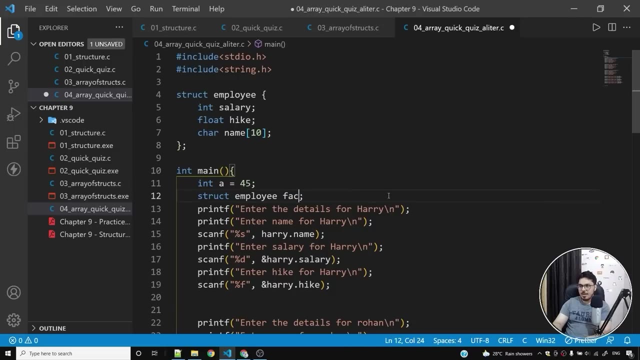 program from quick quiz. let me call it quick quiz alliteratec. what i want to, what i want to do, is i want to tell you that the program that we wrote can also be created by, say, creating an array of three different structures in the form of an array. 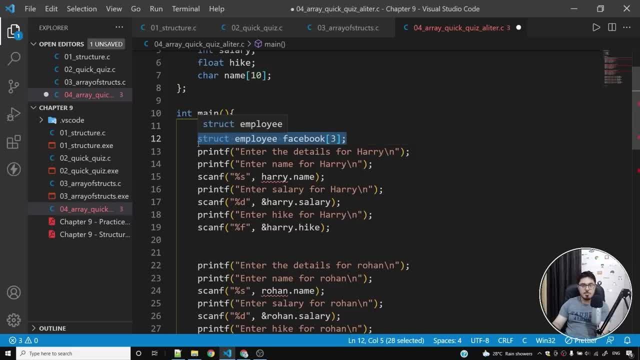 so this particular thing will look like one particular structure, but it is not a single structure. just like int a hundred is not one integer, it's hundred integers. this represents three different employees. okay, so now what i can do is i can replace harry with facebook zero. so 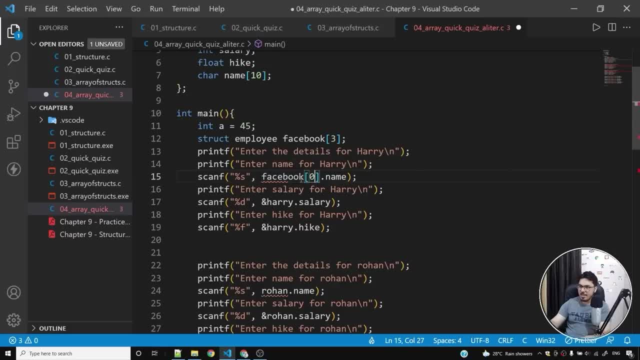 let me do that. so i'll say facebook zero. so whenever i've written harry dot, i'll replace it with facebook zero. so let me do that for you. so whenever i've written harry dot, i will replace it with facebook zero. so let me do replace all. but before that i want. 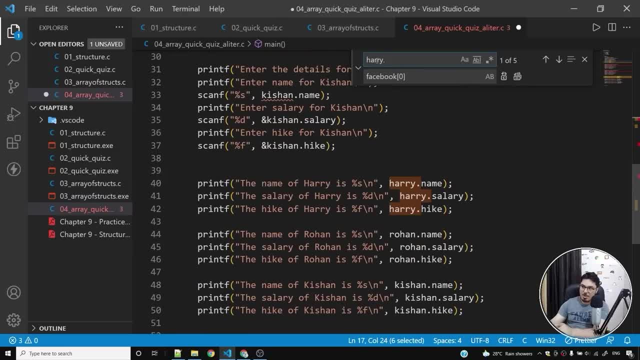 to make sure that i'm replacing the correct things. why am i not replacing harry and harry dot, and i'll replace it with facebook dot? i am replacing harry dot because if i replace harry, these things will also get replaced. i don't want that, so i'm replacing harry dot with facebook zero dot. 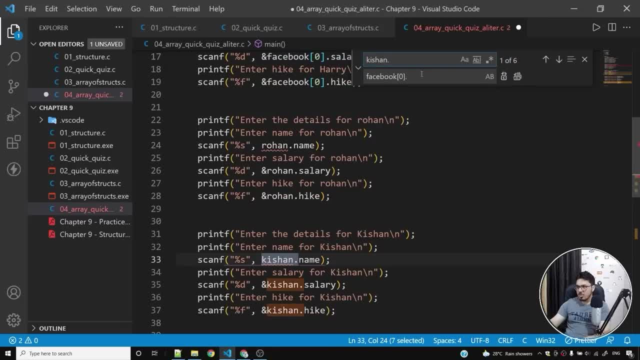 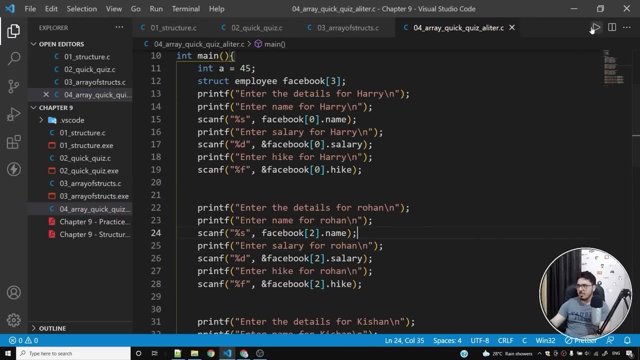 replace all. i'll do the same for kishan, i'll replace it for with facebook one, and then i'll do the same thing for rohan. i'll say facebook two, and this should work okay, but there is some error, it seems. no, there is no error in this program. let me run this program for you and i want to show you that. 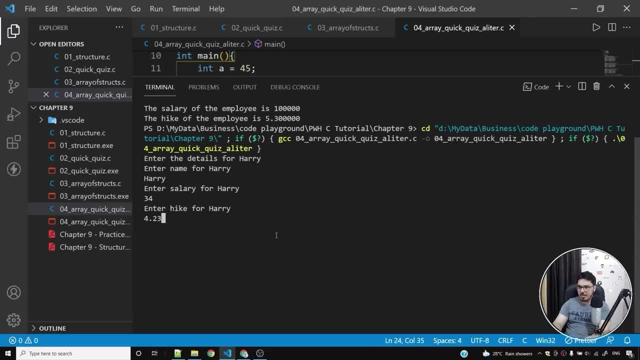 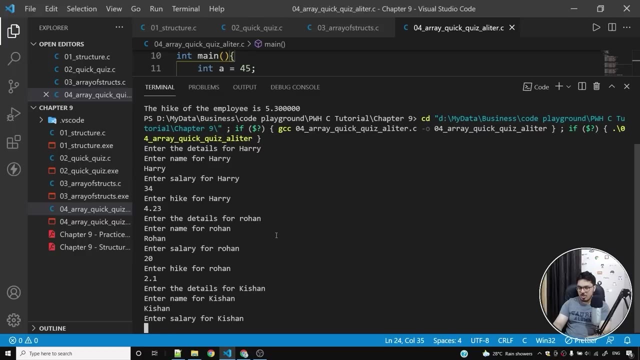 this will work okay. so let me quickly type few values and i will do the same thing for rohan. we'll remember that the rohan salary is 20 rupees. okay, and hike for rohan is 2.1 and for kishan name is kishan. four and one. okay, so you can. 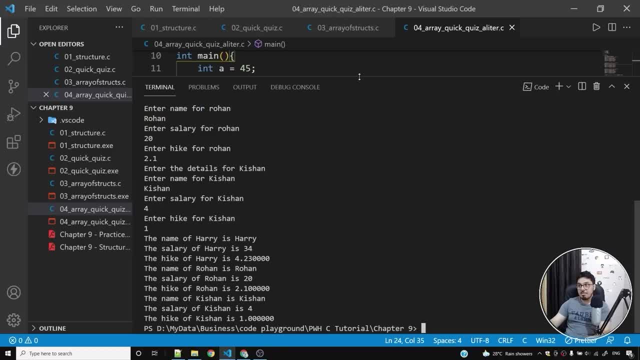 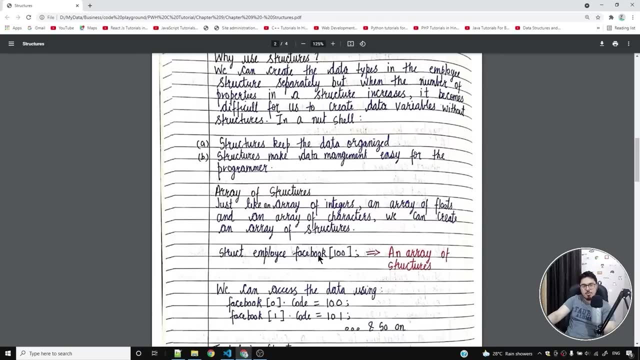 see that all these values are printed just like they were printed in program from our quick quiz. okay, so this is how you can use arrays, uh, arrays of structures. okay now, just like an array of integers, an array of loads and an array of characters, we can create array of structures. 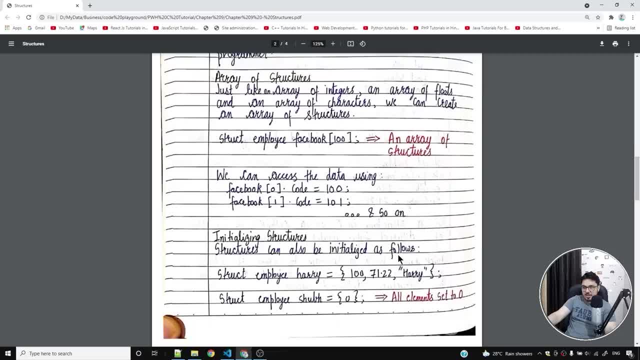 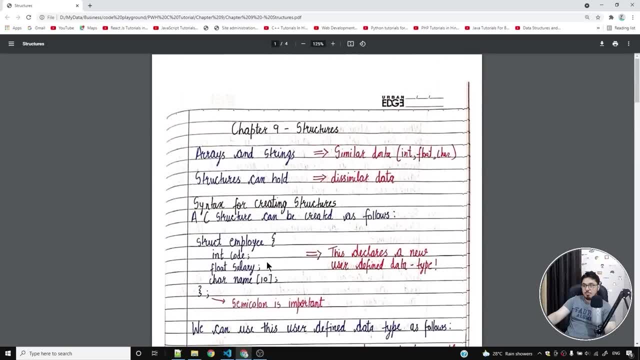 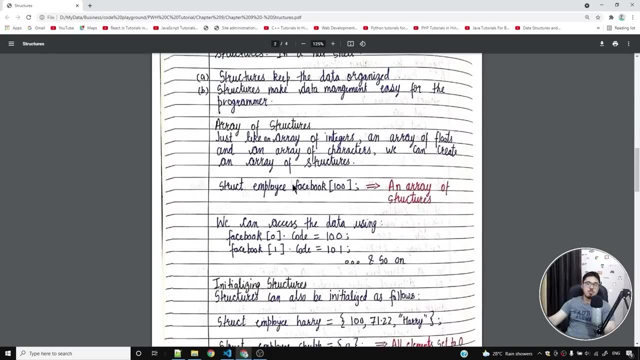 just like i showed you, struct employee facebook 100 will create an array of 100 employees, and what is an employee employee is the structure, so 100 such entities can be created just using this simple declaration: struct employee facebook 100. okay, now we can access the data using this, and i have written. 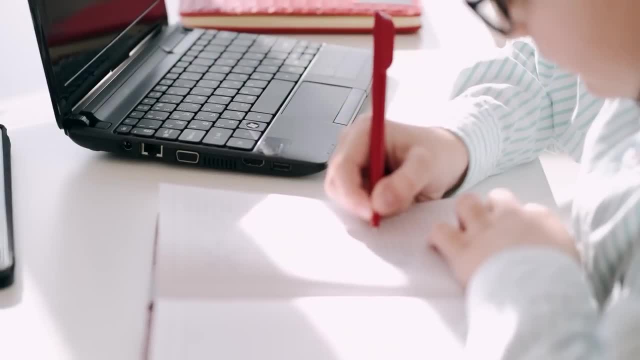 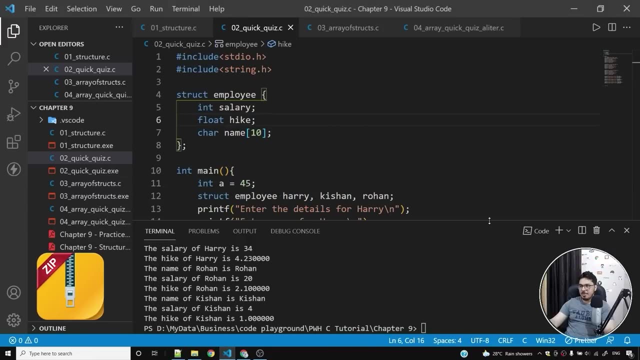 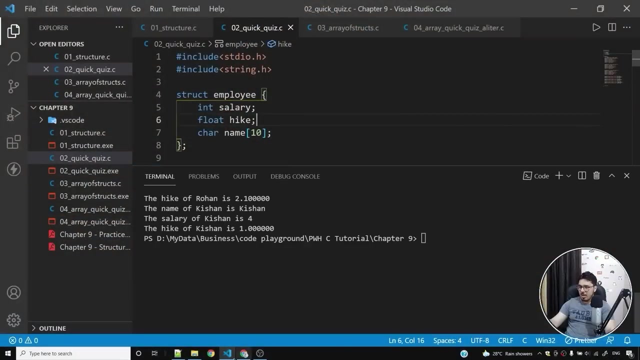 this in the notes so that you can always come back to the notes and you can access all this syntax. also, what i'll do is i'll zip all these code files for you and i'll give it to you so that you can run any program of your choice anytime you want. so we now 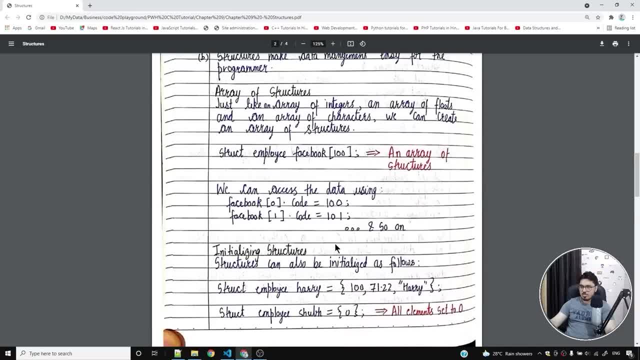 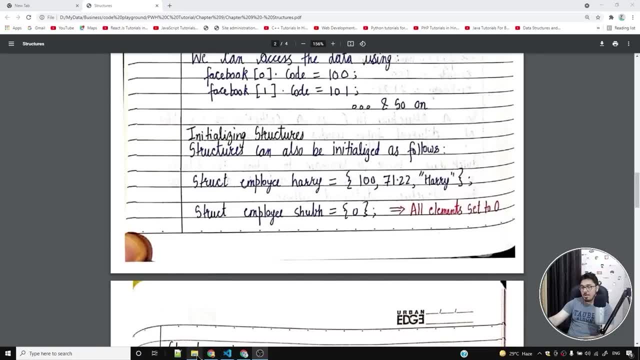 move into the next topic and we'll talk about initializing structures. so how do we initialize a structure? so structures can be initialized as follows. i've written syntax for you. we have already made the program and i have already opened this particular folder in vs code. i guess yes. 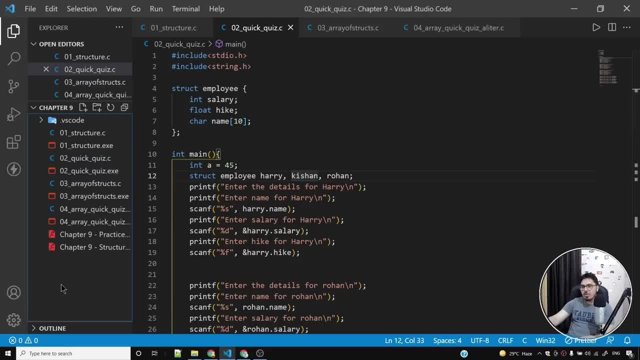 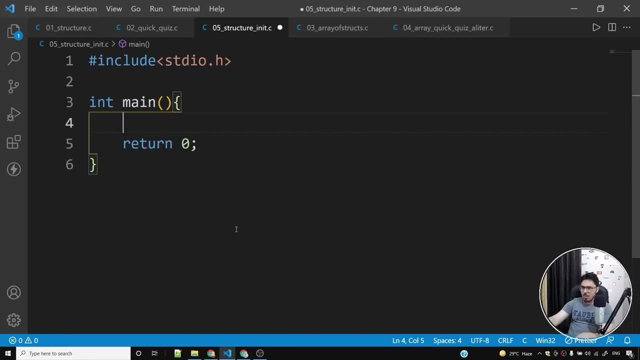 so what i'll do is i'll show you how to initialize structures using a program, and it will make it easier for you to understand structures. structure innate, dot c, and in this program, i'm going to tell you how to initialize a structure. okay, so what i'll do is i'll simply come to this particular page. 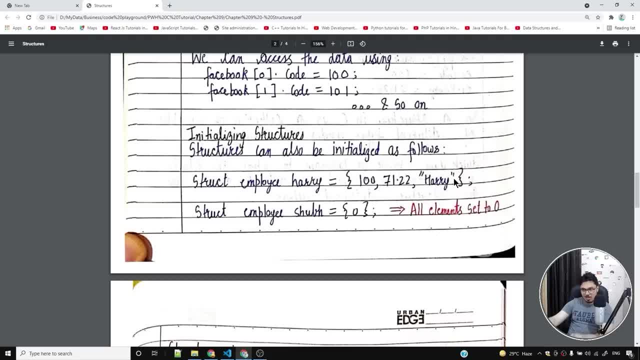 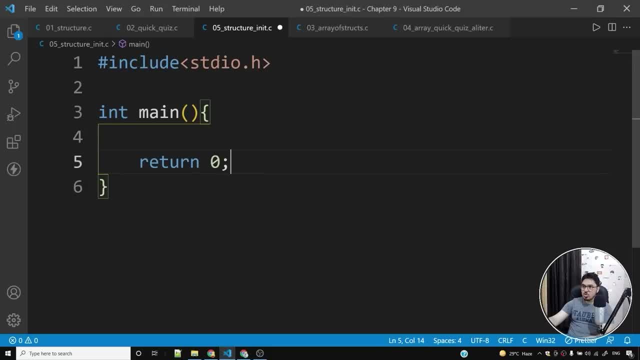 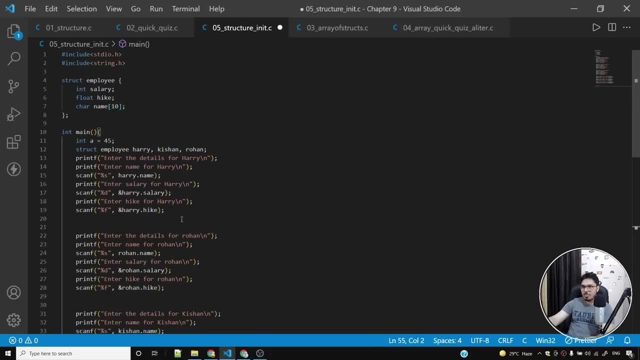 and i'll simply say: struct, employee harry is equal to this. and what this will do is this will initialize a structure. i can directly initialize the structure. i'll show you how. so what i can do is i can, you know, copy this program and i'll paste it here. and what i'll do now is i will simply get rid of all this. 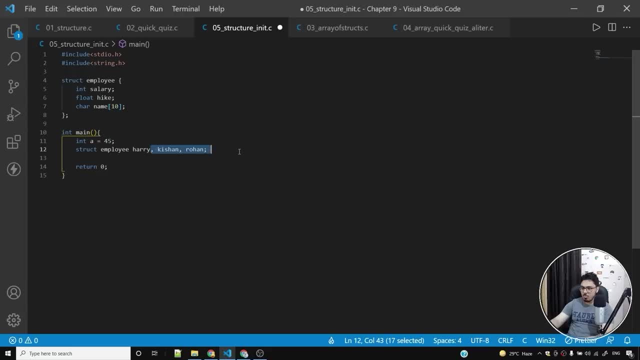 all the code which has been written by me in the main. but what i'll do is i'll simply say: struct, employee harry is equal to. i'll say salary is 34 and i'll say 5.2 is the hike and the name is harry. 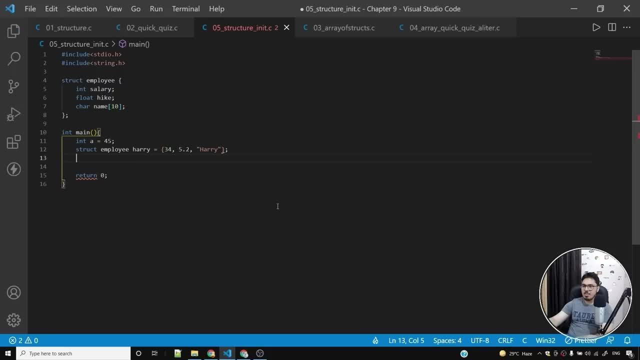 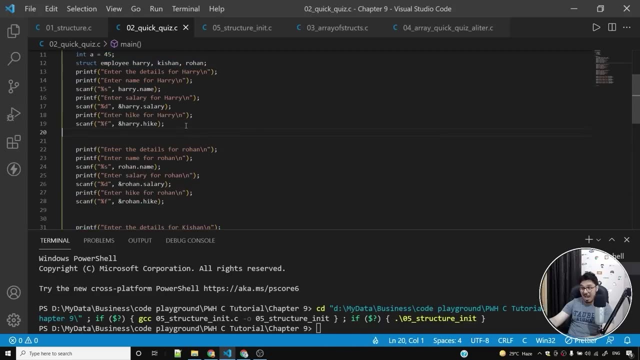 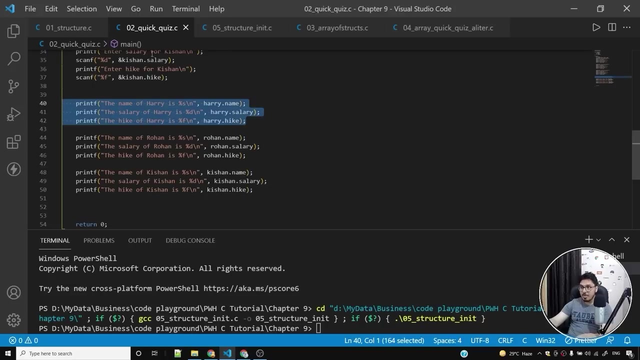 okay, now what i'll do is i'll save this particular program and if i run this program for you, you'll see that we are getting no errors whatsoever. but does this program actually initialize all these values is the question, and i'm going to answer this question for you. so here is the set of print. 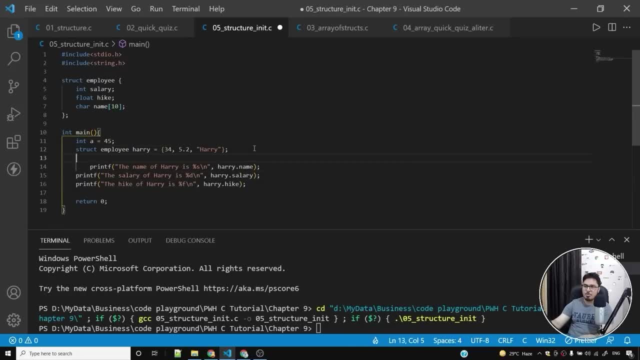 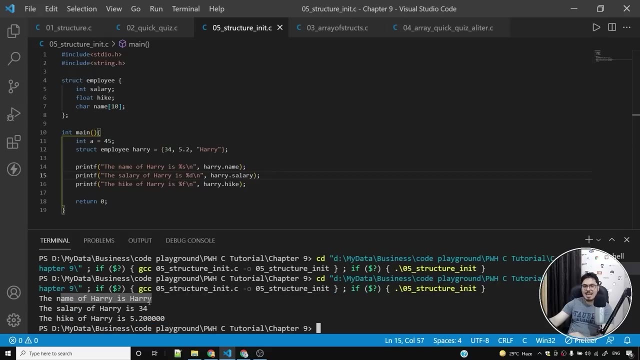 statements which were written by me in the previous program to print name, salary and hike of harry. let's see if these values are still working with this particular syntax. so i'll run this program and you can see that all these- uh, you know names, salary and hike variables. 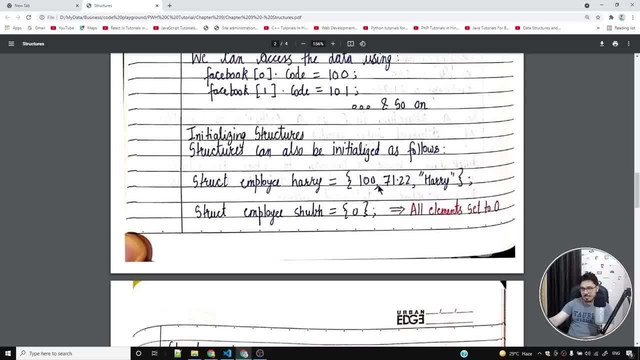 have been initialized properly, which means that the syntax works. you can also set all the elements to zero. so all the elements will be set to zero if you use this syntax. so in case you have a set of numbers or you want to initialize a couple of pointers to null, what you can do is if you 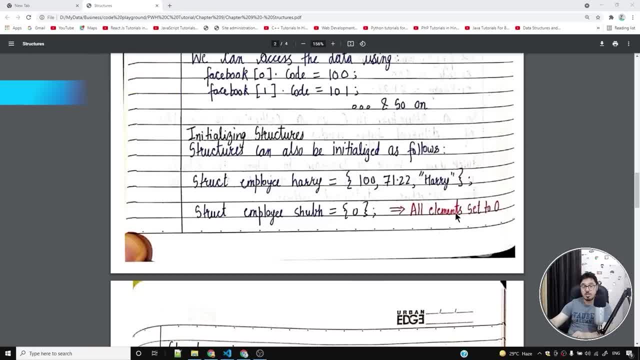 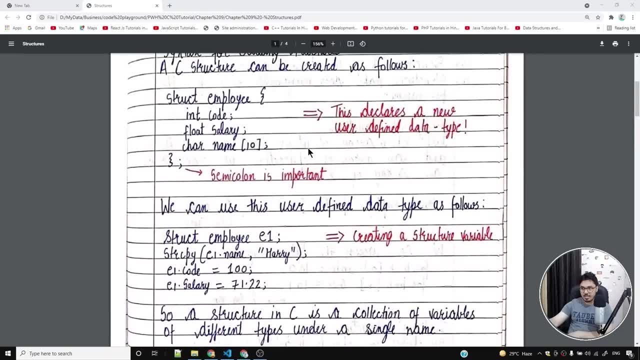 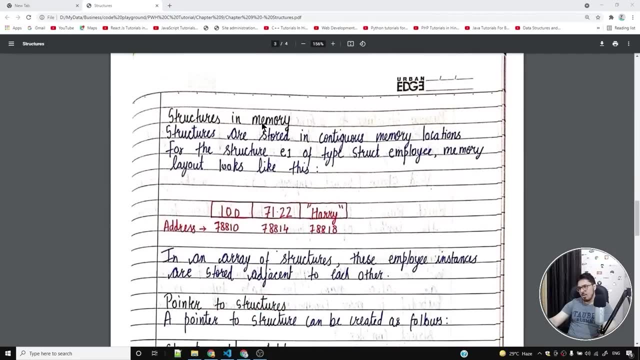 can always use the syntax and this will initialize all the elements to zero. so this was another way to initialize structures. we have already seen one of the ways to initialize structure here, where we set name, salary and hike manually using scanf and you know strcpy. now how does structure 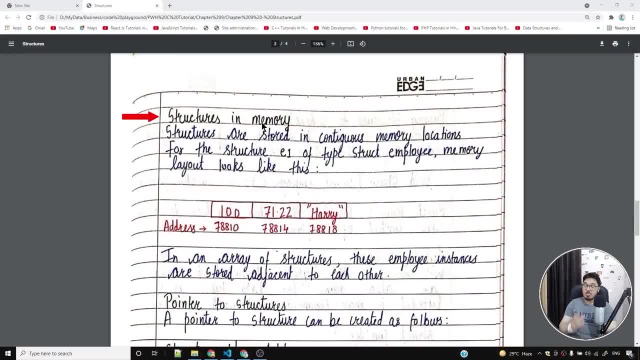 look in memory is something that you need to understand, because if you understand how programs are running in memory, you'll be able to easily decode what is happening in the program, and it will make you a better programmer, for sure. so let's see how structures look in memory. structures are stored. 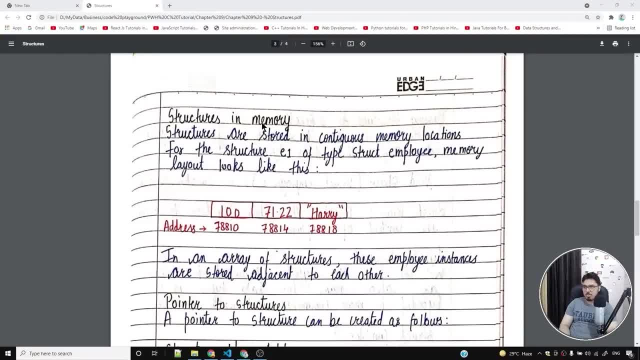 in contiguous memory locations for the structure, even of type struct employee memory layout looks something like this: so if the address of this particular block is seven, eight, uh, seventy eight thousand eight hundred ten, what will happen is this will take four bytes and the address for the next float will start from seventy eight, eight, one, four, and again it will take four bytes. the. 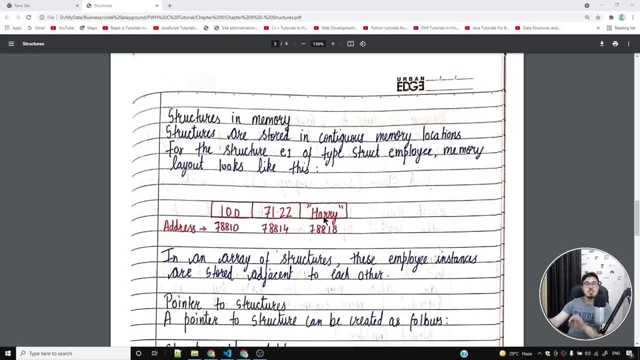 starting address of this particular block which is storing the string, uh, storing the name string, rather, is seventy eight thousand eight hundred and eighteen. so this particular block will have seventy eight thousand eight hundred and eighteen as the starting address. this will have this as a starting address and this integer will have this as a starting address. so 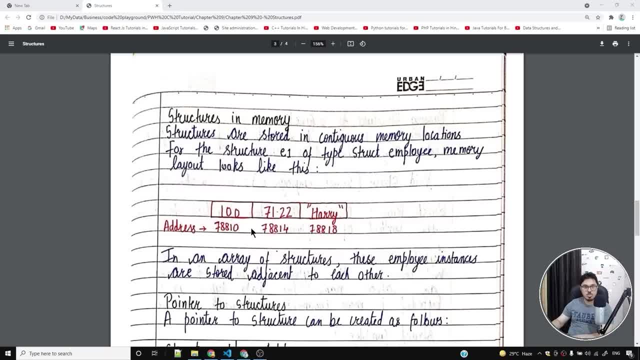 structures store the data in contiguous memory locations, so this is something that you need to keep in your mind. in an array of structures, these employee instances are stored adjacent to each other. so let us say we have us an array of 12 structures, or in a row of 12 structures. 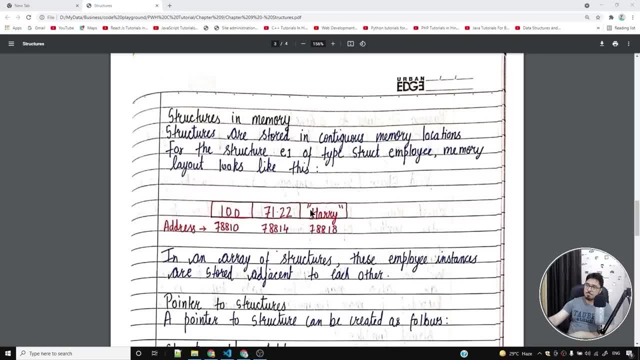 an array of three structures, for that matter. what will happen is three structures will be stored in further contiguous memory blocks. so what will happen is: let us say this is my memory. let us say this particular row is my memory. what will happen is the address will start from here for the first. 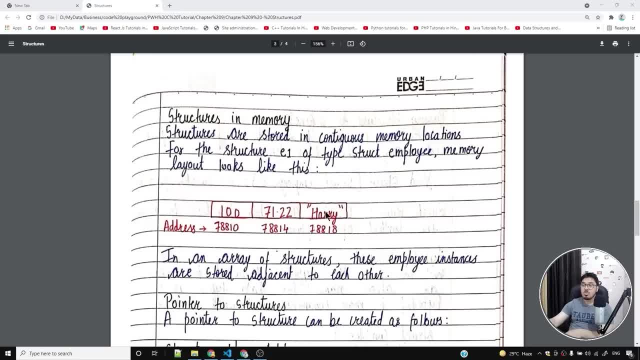 element of the structure. so after the ending address of the string will be the starting address of this particular uh, what is the salary of the next structure? so i hope you got the point. so, in contiguous memory, we'll have the first element of the structure here and the very next. 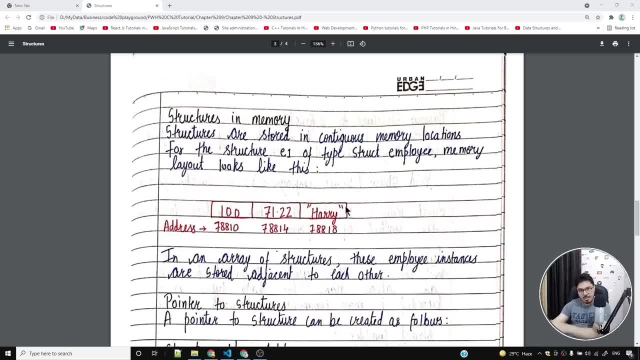 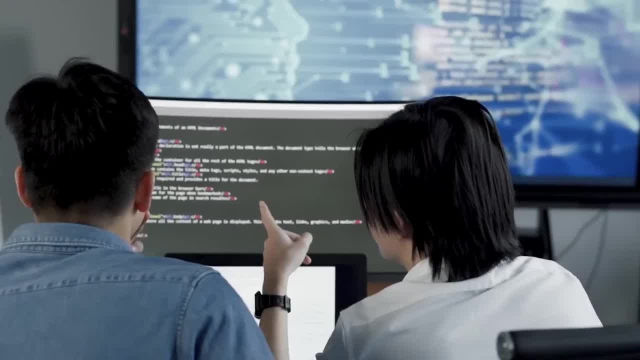 thing in the memory will be the second element of the structure array, then third element of the structure, and so on. so in an array of structures, these employee instances are stored adjacent to each other. i hope you got my point. so let's talk about pointers to structures. a pointer to structure. 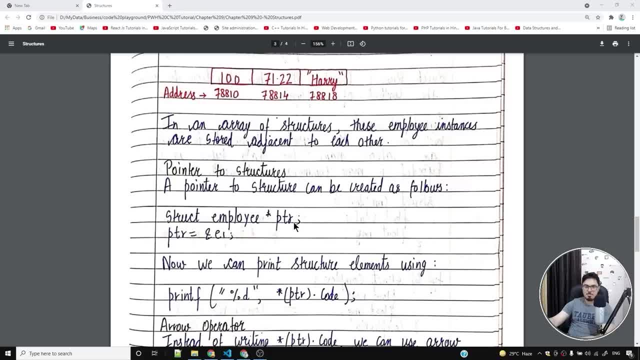 can be created as follows. so you can say: struct employee star ptr, and ptr is equal to ampersand e1. so this syntax can be used to create a pointer of type struct employee. remember i told you just like int is a data type, struct employee is also a data type and i can use this: struct employee data. 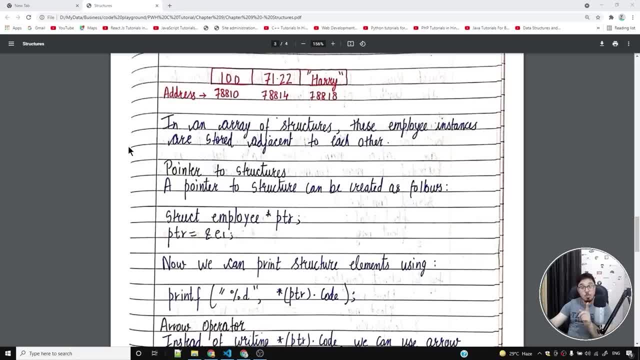 type to create a pointer of this type. so ptr is a pointer of type struct employee. ptr is not a pointer of type int or type float or type care for that matter. it's a pointer of type struct employee, which is a data type, a custom data type which is defined by me, just like we have int, float. 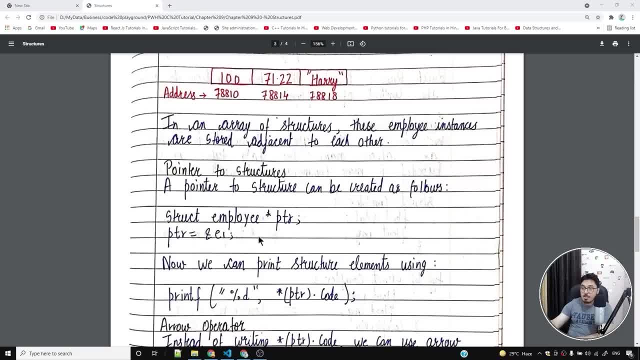 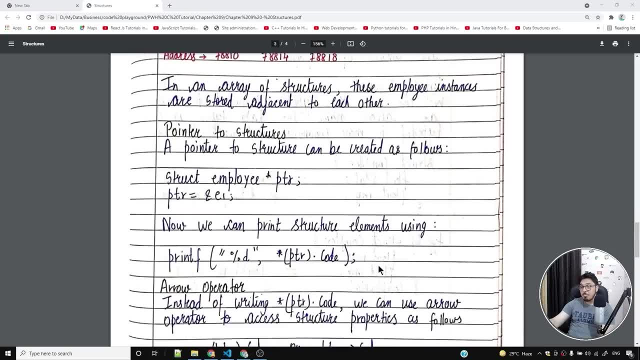 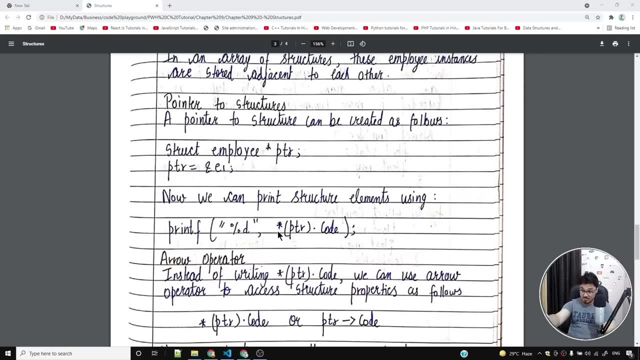 double all these data types available. this is something that we made available for us by writing the structure. i hope you got the point. now we can print structure elements using printf person d and, just like i was using this address of operator, this s2x operator, i can use it with the pointer to. 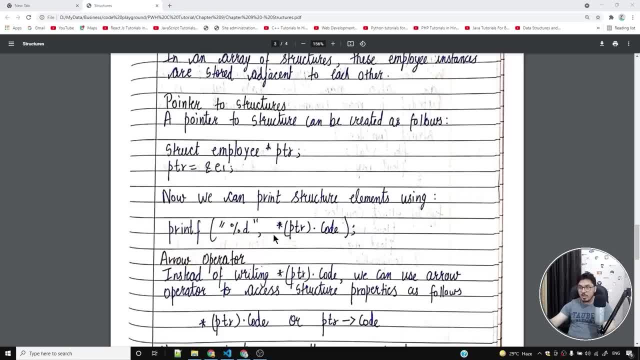 structure as well. i can say: tell me which structure variable is this pointer pointing to and i can decode this address address, i can get the structure. and once i get the structure variable, i can do dot code, dot name, dot salary. whatever is available in the structure can be, you know, used by me in this case i don't. 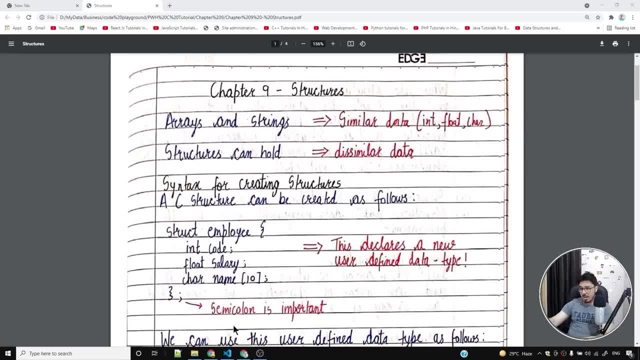 have anything such code but i have. okay, i have this code. i'm sorry i have not written the code in the program, but in this example i have the code. in my example i have salary, hike and name, so i can use dot salary, dot hike or dot name to get all these things. but in this example, since we have 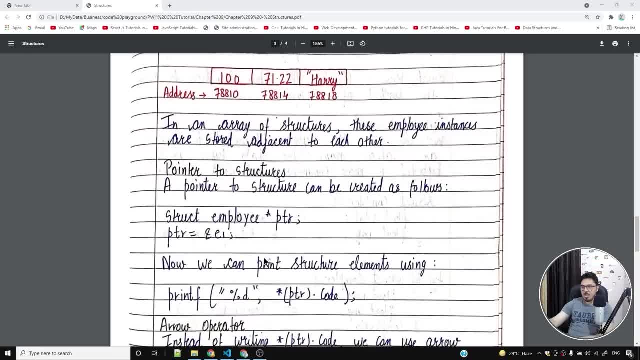 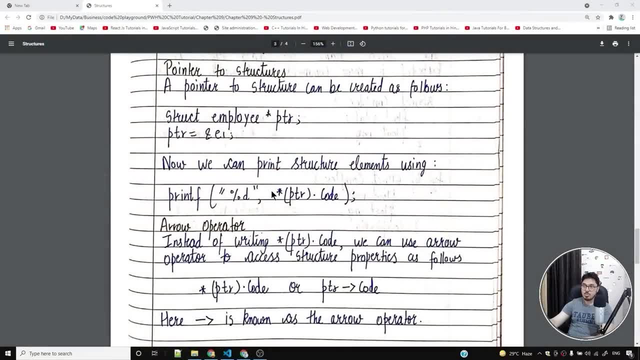 code here, so i'm using dot code. so this is how you can, you know, create pointers to structures and then further dereference them to get the value at those pointers using the star operator. now there is something called an arrow operator in c, which will make your life a whole lot easier if you are using pointers. 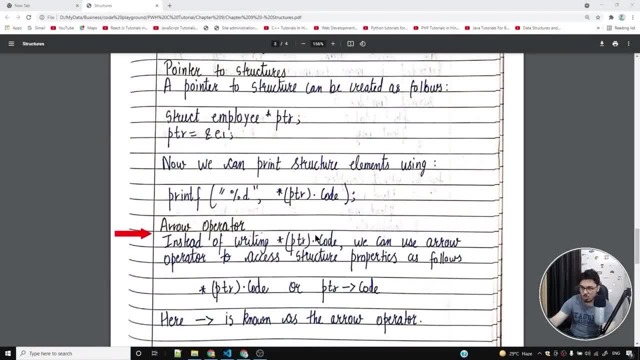 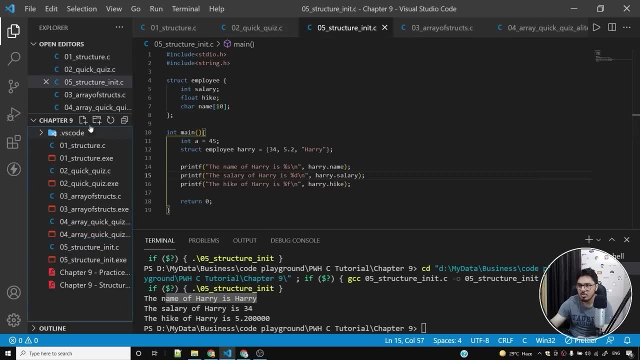 to structures. instead of writing star ptr dot code, what we can do is we can use arrow operators to access structure properties, as follows: but before that, let's write a program using pointers to structures. okay, so what i'll do is i'll simply create another program. 06 underscore. 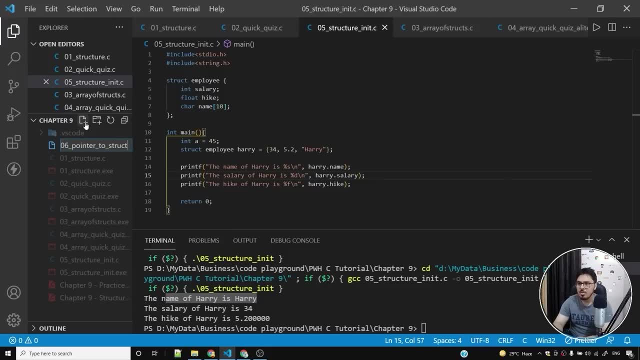 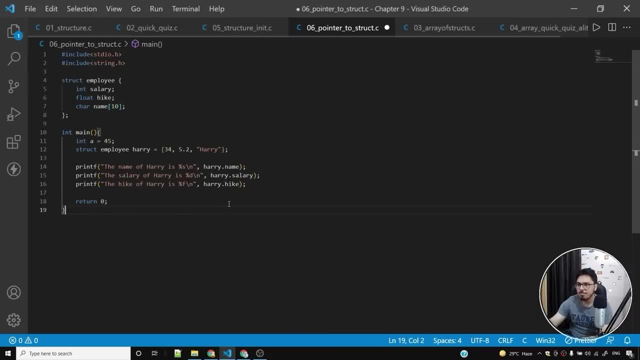 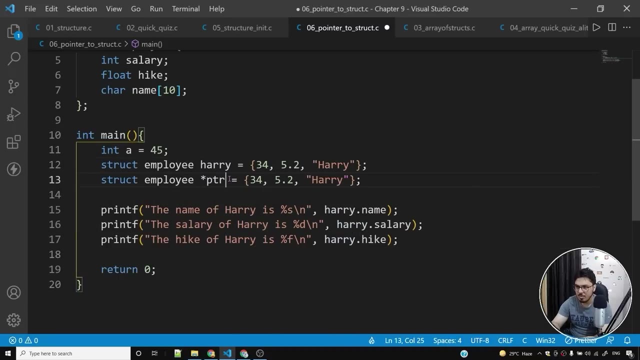 pointer to structure dot c, and what i'll do is i'll copy this code inside this particular file, and what i'll do is i'll simply create a pointer of type struct employee. and what i'll do is i'll set this to the address of harry. harry is what harry is: a structure of type employee. 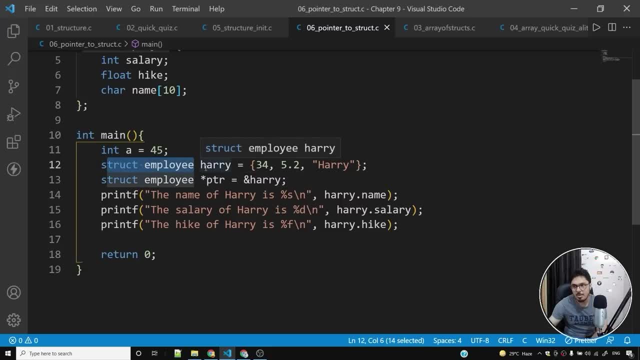 so it's a struct employee variable. so struct employee variable. harry now has a pointer ptr which is pointing to this structure. so how do i make a pointer point to a variable? i simply set it to the address of that variable and ptr will now point to harry. now, instead of doing harry dot name. 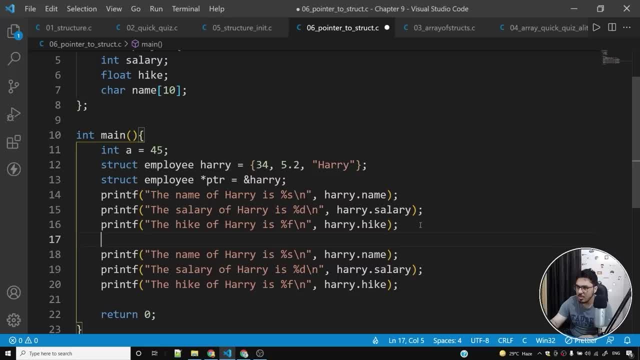 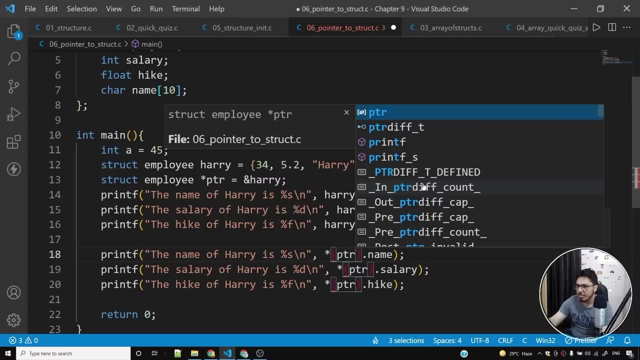 i can also do something like this. let me show you. so, instead of writing harry, what i can do is i can write. i can write star and i can do: uh sorry, ptr dot name. so i can do something like this: i can say star, ptr dot name. 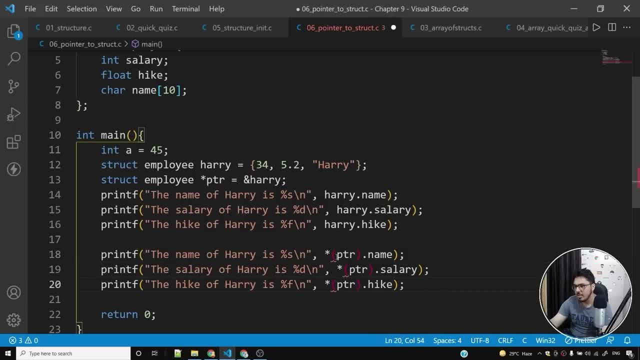 start ptr dot salary and star ptr dot hike. what this will do is this will dereference the pointer and finally, after dereferencing the pointer, what i'll get is: i'll get this particular structure. so this is something which is very important. i'll have to wrap it inside the brackets because 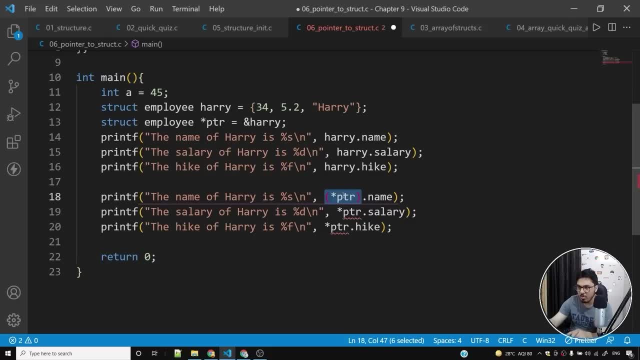 this will not work otherwise. so what we want to do is we want to get the structure first and then we want to do dot name on that structure. so what i'll do is i'll replace all this with the these brackets. so let me copy this, paste here, paste here: and all these red underlines which 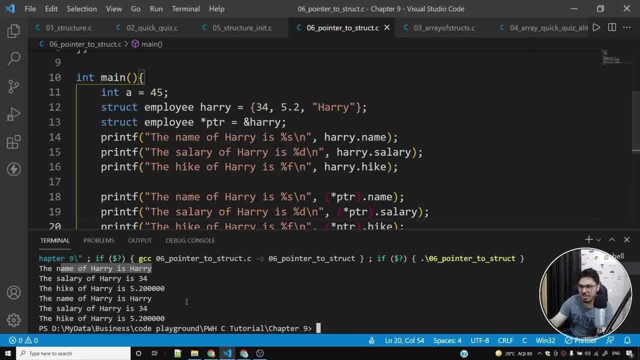 were indicating the error have now vanished. now, if i run this program, you can see the salary of area is 34 and this also prints the salary of area 34. name is also printed same and the hike is also printed same, the difference being this one is using the pointers and this one is using 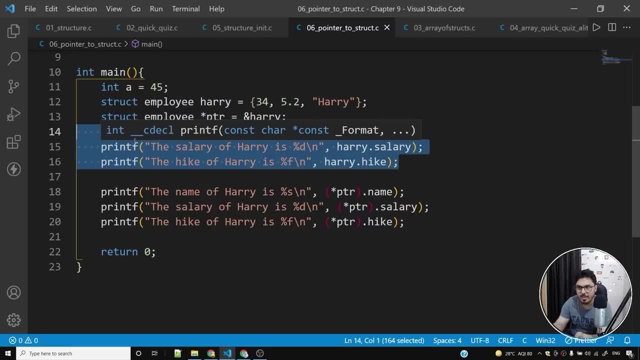 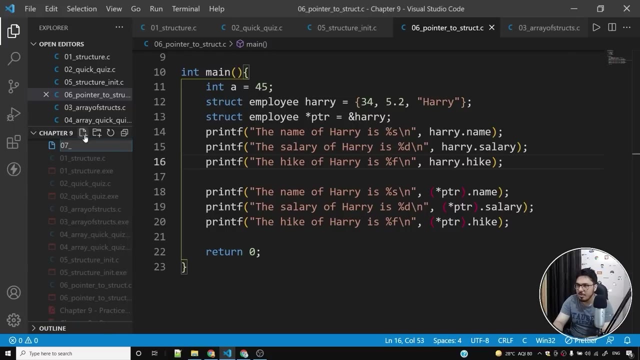 the direct structure, so i can either use a pointer and dereference it or i can directly use the variable, just like integers and floats. we have already seen all these things. okay, now what we'll do is: we'll create another program, and our next program is 07. underscore, arrow, operator and arrow. 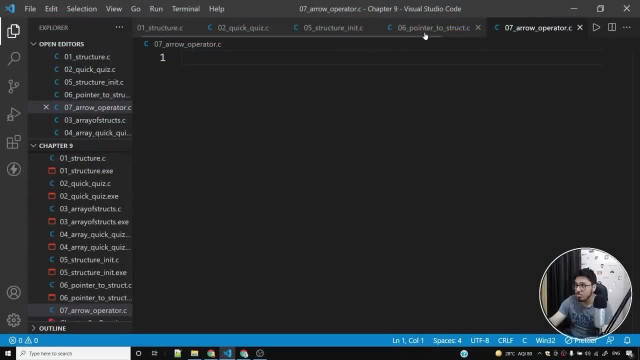 operator is really very important. if you want to go into data structures and you know work with structures, you'll definitely use all these things. so what i've done here is i've copied the code from the structure program, this particular program, and i've pasted it here, and now i'll tell you how arrow. 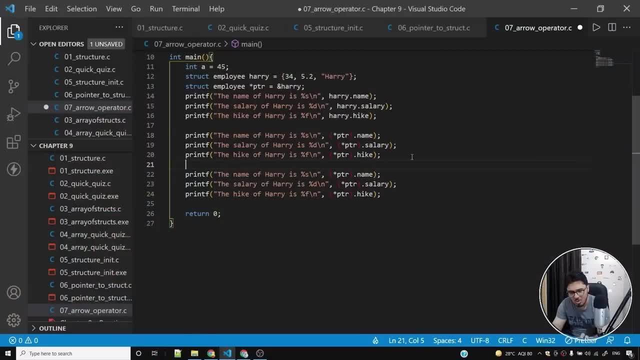 syntax works. so arrow syntax is really very easy. all you have to do is, instead of doing star, ptr, dot name, instead of dereferencing a pointer and then getting the value from that structure, what you can do is you can directly use the pointer and use the arrow operator, which will 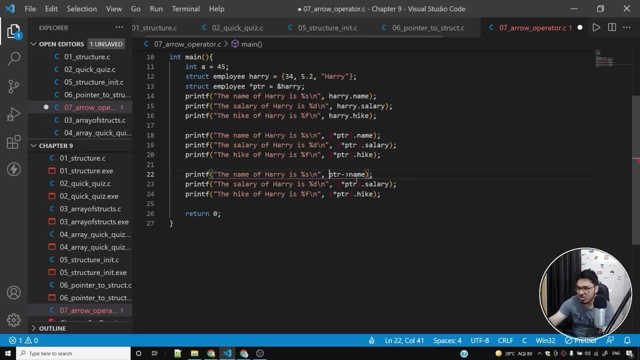 simply mean that what you want is you want to dereference this pointer and get name from it. so this syntax simply means that you want to dereference this pointer, get the structure and then get the name from that structure. okay, so this syntax is really very simple, so i'll use multiple. 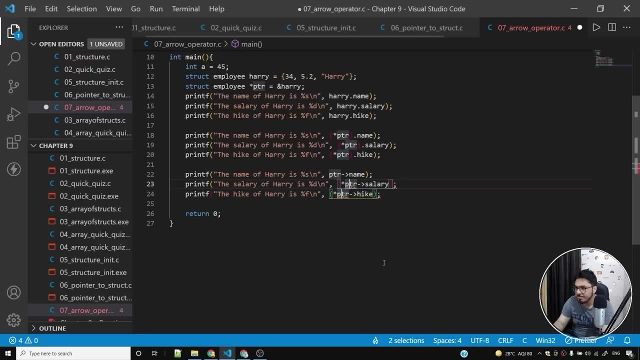 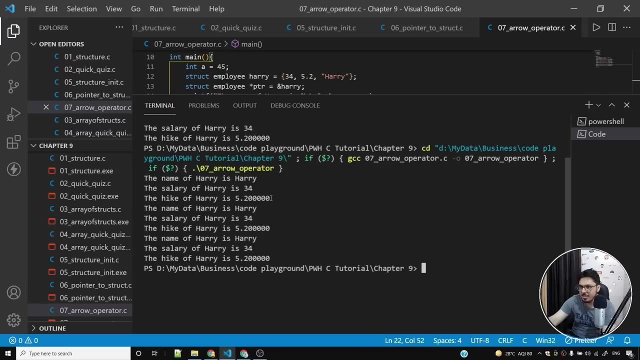 cursors here to create a arrow and i'll simply say ptr, salary, ptr, all these things, and this syntax will work. let me show you if i run this program. you'll see that the name and the salary and the hike have been printed. this is the output. 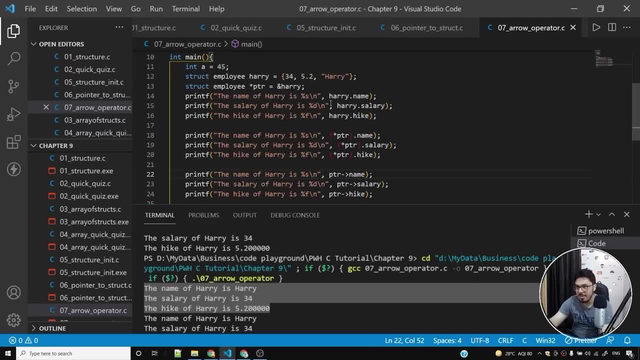 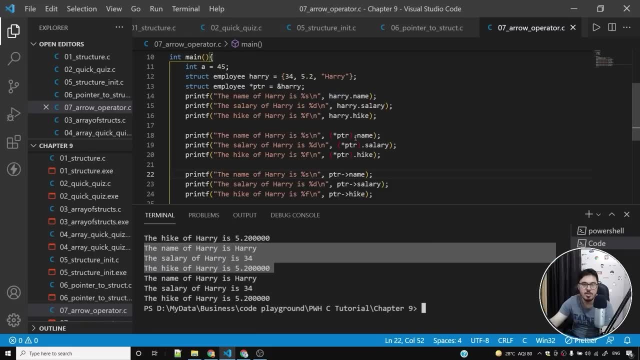 of this particular thing, where i've used directly the variable, the structure variable, and this is the output from using the pointers. i've dereferenced the pointer and then i've used a dot operator. dot operator can give me the name, salary and hike from the structure. 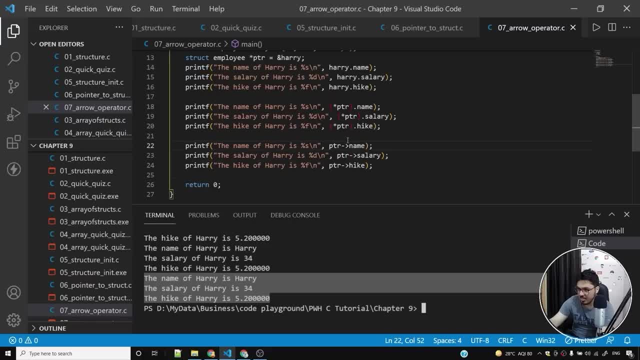 now, this is a special syntax that we learned, which is the arrow operator. so here the c programming language or the c compiler is smart enough to understand that. i want to dereference this pointer and get the name from it because i'm using this arrow syntax, so this arrow syntax. 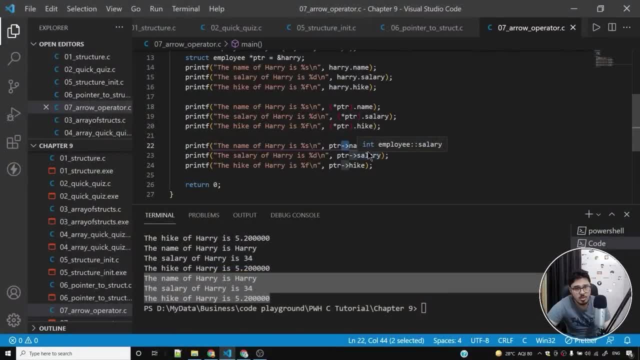 actually makes it really very convenient for users to you know dereference the pointer and get a value. if you use a lot of pointers in your program it will be a big headache to you know dereference those pointers and use dot operators. this is a clean syntax and 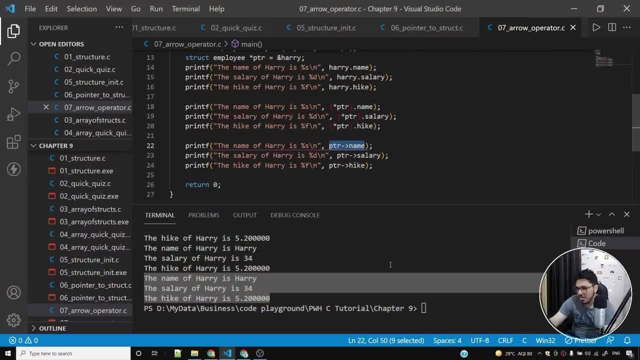 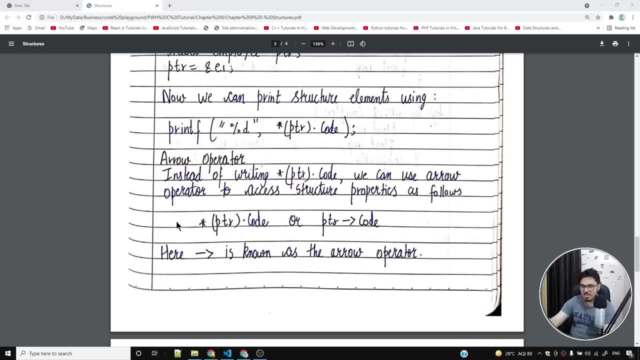 is easy to write, easy to read as well as easy to maintain. so this was the arrow operator. instead of writing star pdrcode, we can use this, so arrow operator to access structure property as follows: i can do star, ptr dot code or i can do something like this: okay, now here i think i have 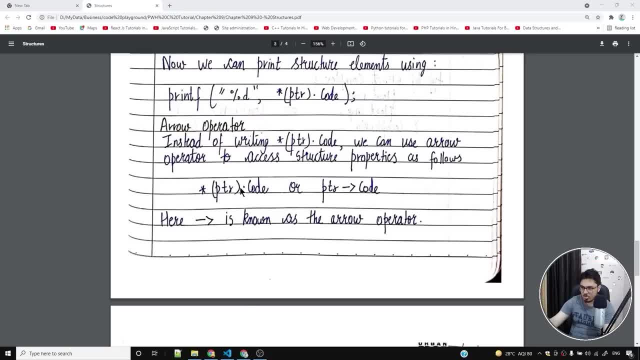 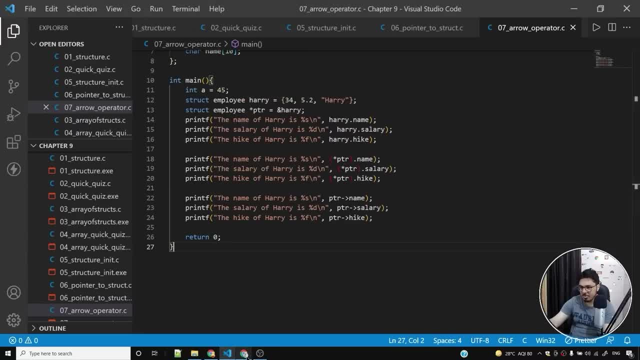 not written the bracket correctly. this bracket should come outside, so you need to make a note of this. this is the correct syntax. i accidentally wrote the star outside the bracket. this will create problems for you, so i want you to remove this bracket and put it here. so make sure that. 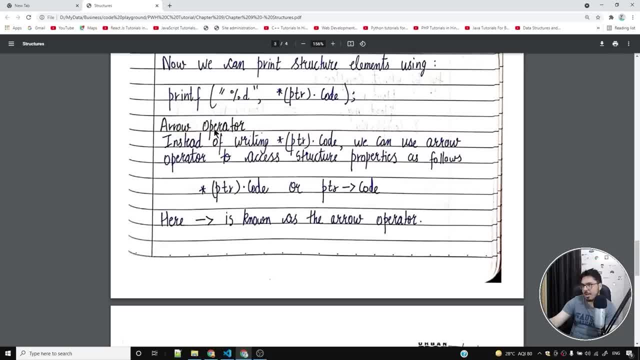 you do this. this is a minor mistake in the notes, but again, arrow operator is amazing. this is this is why we use arrow operators. we don't want to get into all these things- where to put the bracket, where to put the star, where to put the dot? simply use the pointer and say arrow code and this will. 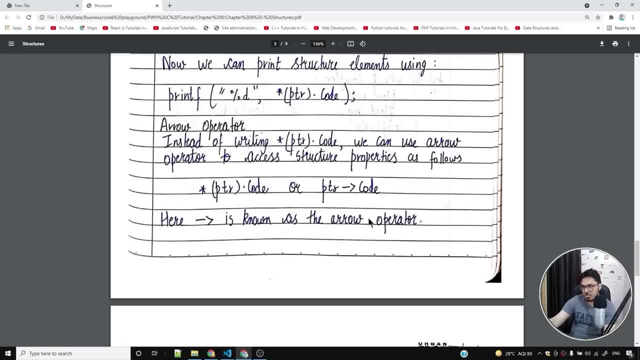 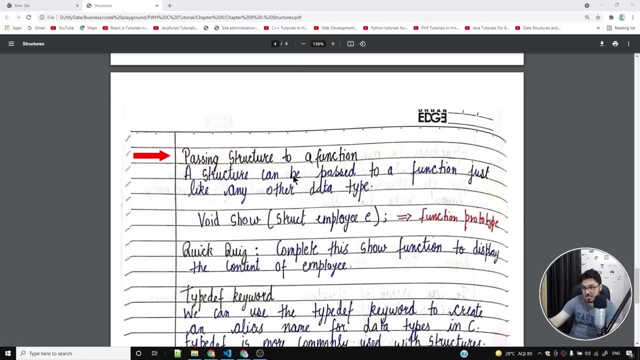 give you the code from this structure. okay, so here this is known as the arrow operator. you can use this operator to dereference a pointer and get. get the value from the dereferenced pointer or the structure. okay, passing structure to a function. can you pass a structure to a function? and if yes, 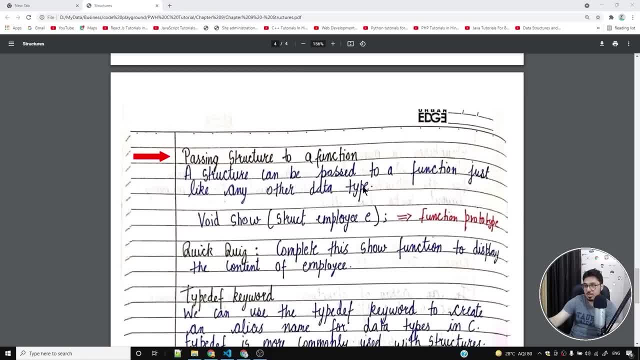 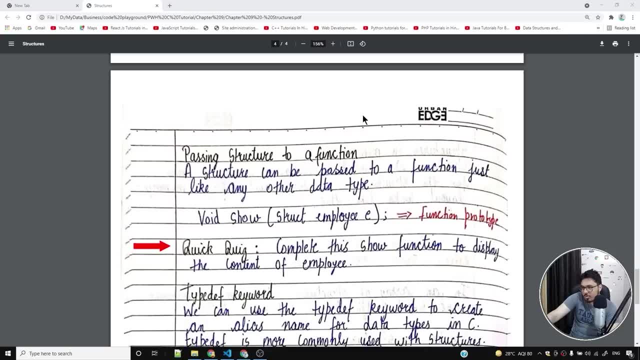 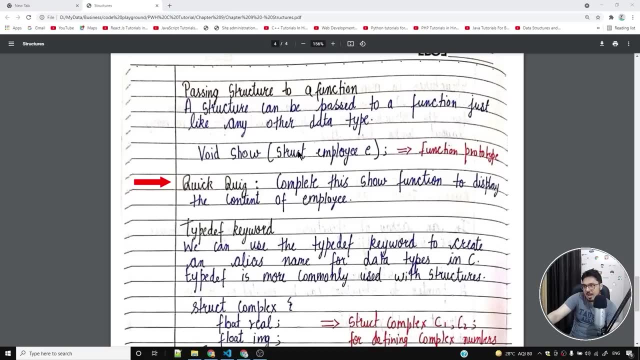 how? how does it look like? so a structure can be passed to a function, just like any other data type. you can pass a structure and this is the function prototype. so there is a quick quiz i have for you: complete this show function to display the content of employee. so you need to complete this function and you need to tell me 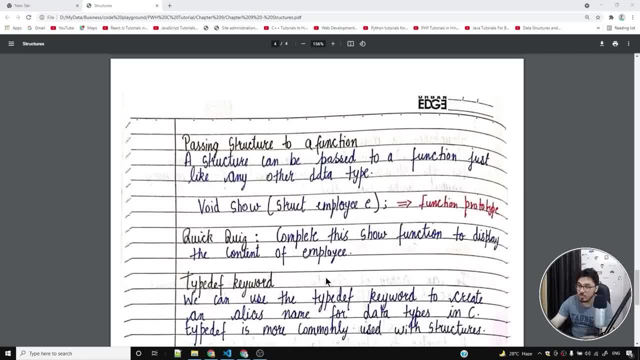 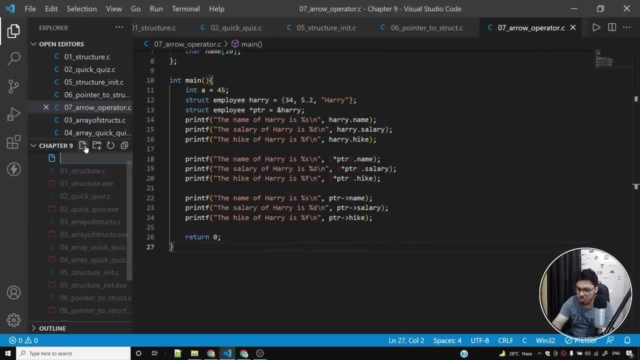 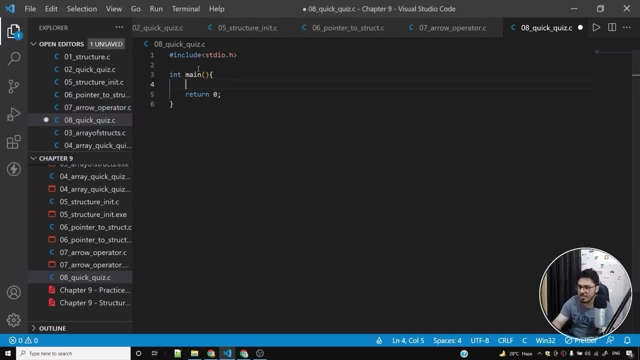 how to write this particular function. so what we'll do is we'll simply write this program, because this is a very important concept. so what i'll do is i'll write a program 08 underscore, quick quiz. so i'll say 08 underscore 08 underscore, quick underscore, quiz dot c, and inside this particular function, what i'll do is: 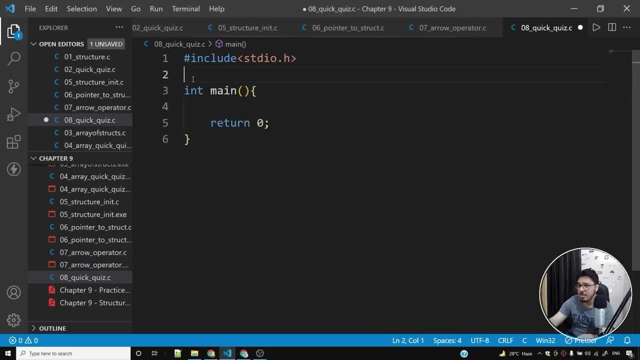 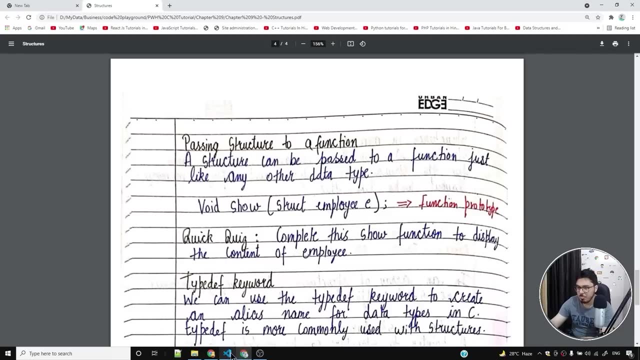 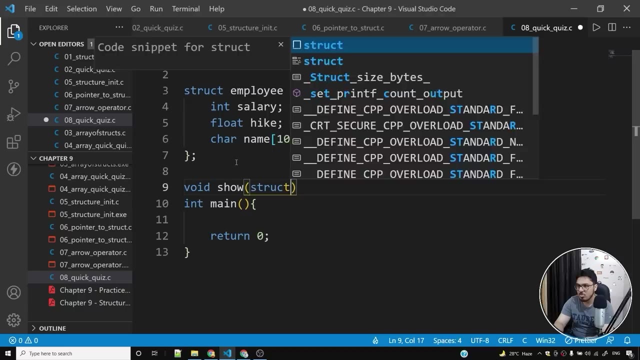 rather, inside this program, what i'll do is i will copy this structure first, and what i'll do is i'll copy this show function, so i'll say: void- show struct- employee. e. so let me write this function: void- show struct, struct- employee. e. now what will happen is, if i 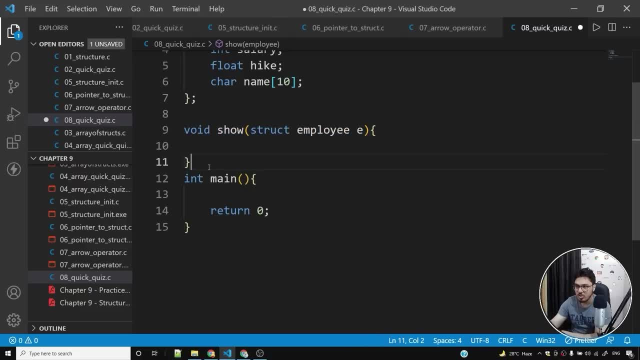 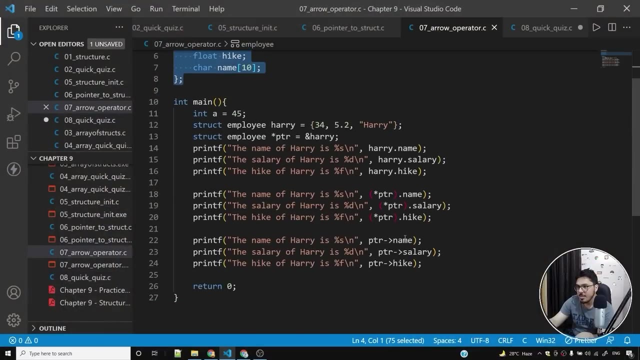 pass a structure to this particular function, that structure will be available inside this function. but the question is: will that structure be deeply copied or will that structure be passed as a reference? so this is something that we'll try to understand in this program. so what i'll do is i'll 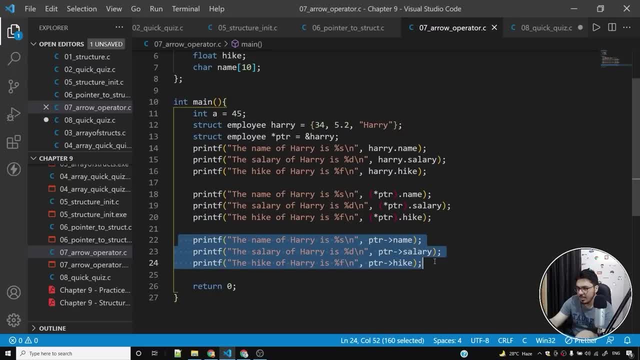 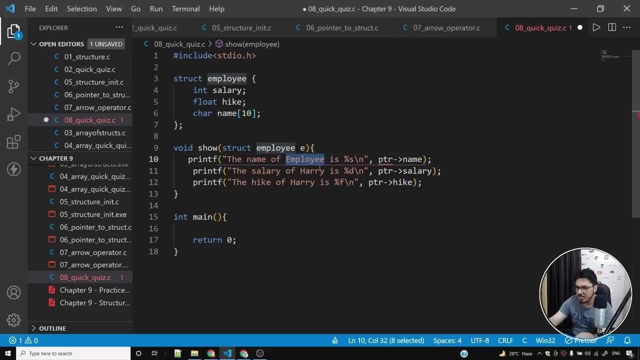 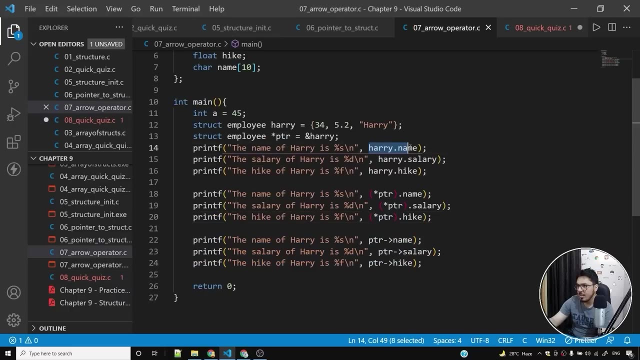 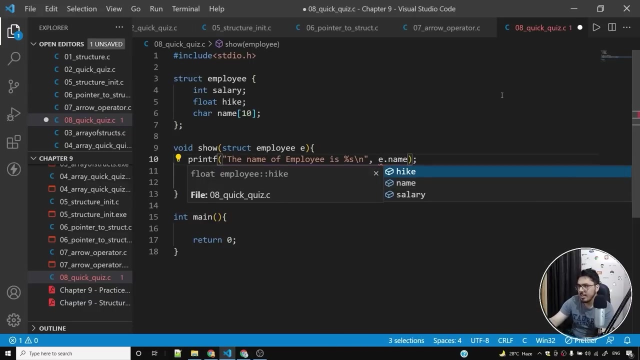 simply the name of employee is. i'll do something like this. so i'll say the name of employee is and here also i'll write employee and instead of saying ptr i will say harry dot name or e dot name. so i'll simply say: right click, change all occurrences. i'll make it e dot, so i'll say e dot name, e dot salary, e dot. 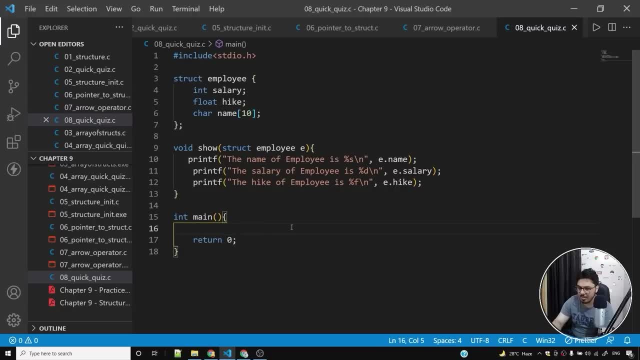 hike. okay, let me save this program. and if i create a structure, is there a program where i've created a structure? yes, here is a program where i've created a structure. i'm simply creating a harry structure here. now what i'll do is i'll simply pass this structure to show function and let's 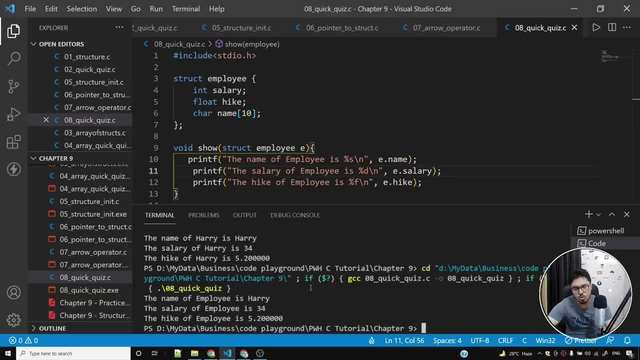 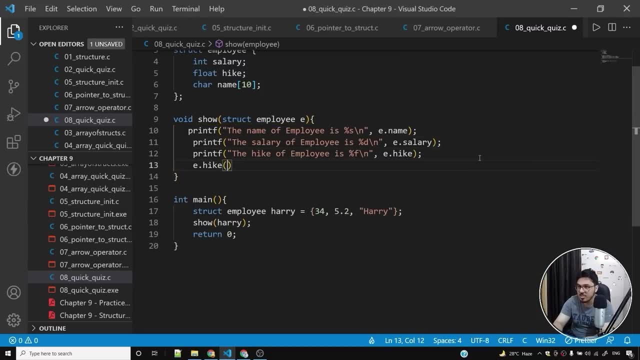 see if it is able to show all these variables. and indeed it is able to show. we know that. but what if i change a particular variable? let us say, what if i change the hike? but if i change the height of e, i'll say e dot hike is equal to 45 or 4.55. what if i change the? 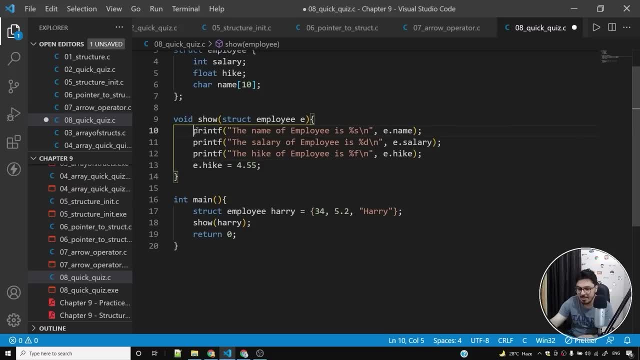 height to this. will this height change be reflected here as well? this is the question also: what if i change the name? will that change be reflected here? so all these questions are important. so this hike change will not be reflected here. let me show you. so what i'll do is. 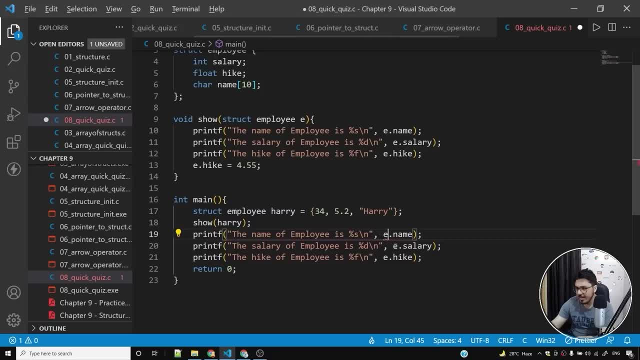 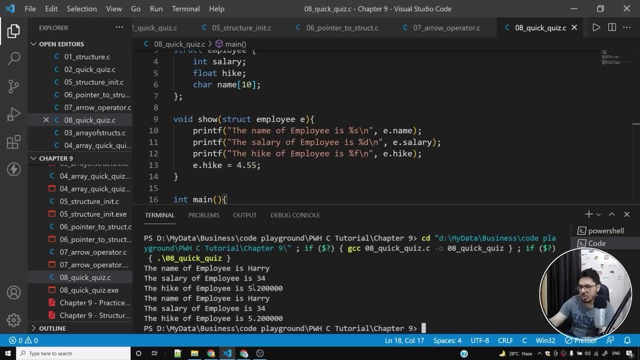 instead of doing this, i'll simply write harry dot name, harry dot salary and harry dot hike here and if i run this program you'll see that initially the hike was 5.2 inside the function. i tried to change it to 4.55, but it will not repeat. 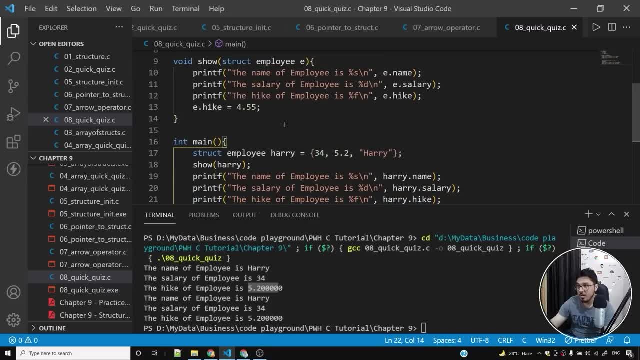 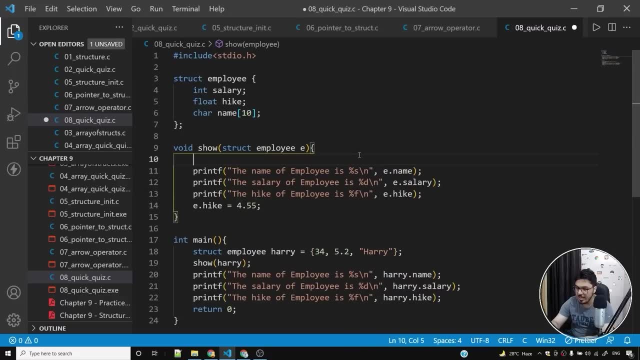 reflected here, because all these values are copied. what if i try to change e dot name? what will happen there? if i try to change e dot name? let us say i want to change the first character of e dot name and let me try to make it p. if i try to do something like this inside my function, i'll get. 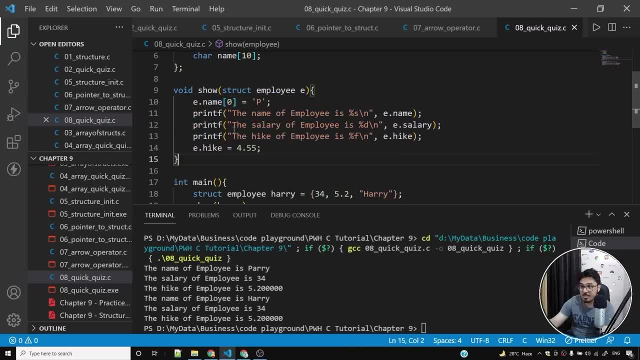 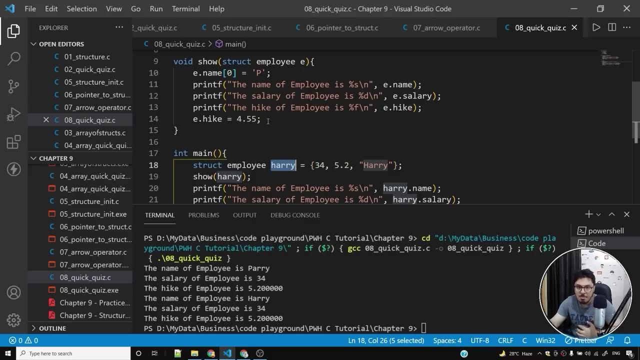 parry. but after this function returns, this change will no longer be reflected in my main function, which means that this function is making or receiving the copy of harry structure. it is not receiving it by reference. i can make it, you know, go by reference and in that case all these. 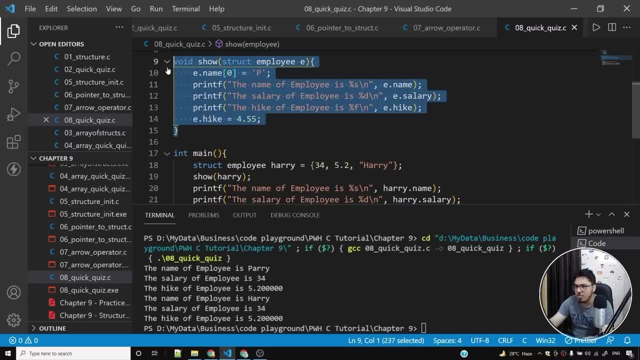 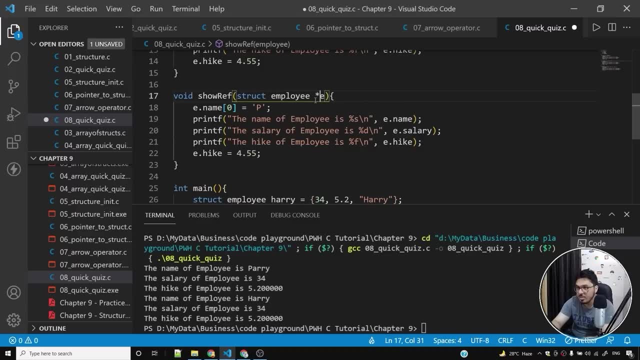 changes will be reflected. let me create another show function, and what i'll do is this time i'll name it show reference, sure f, and i'll receive a structure pointer and not a structure, and i'll change all these things to arrow operator, because we are dealing with structure pointers. 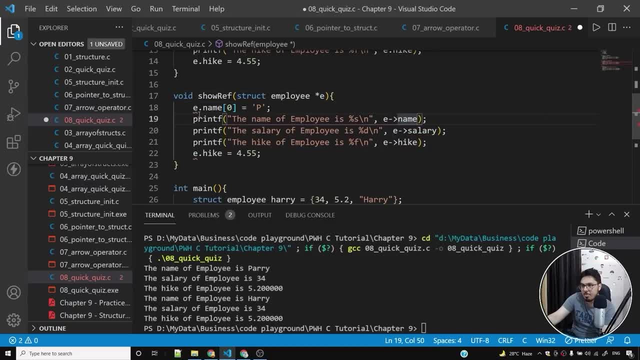 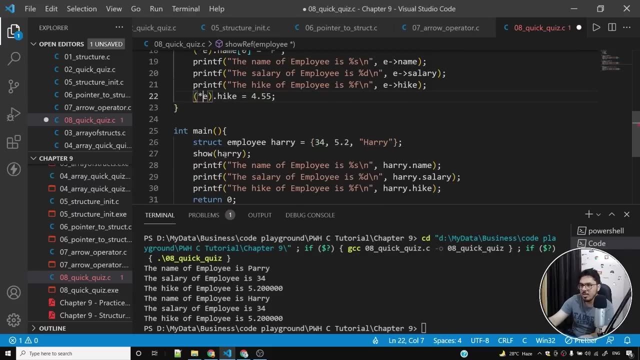 so i'll dereference this pointer and i'll get name, salary and hike from it. and also here. what i'll do is i'll simply say: star e dot name. zero is equal to p, so i can do something like this. and here as well, i can do something like this. okay, so star e dot hike is equal to this star e dot name. 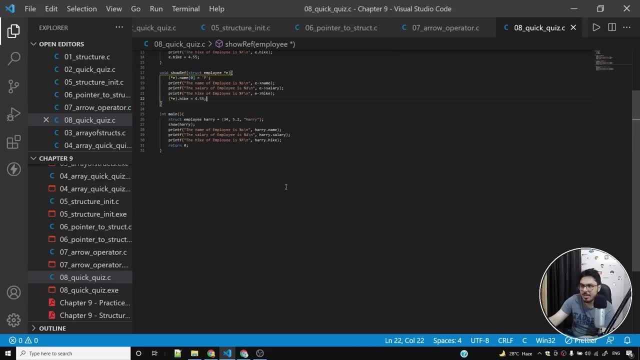 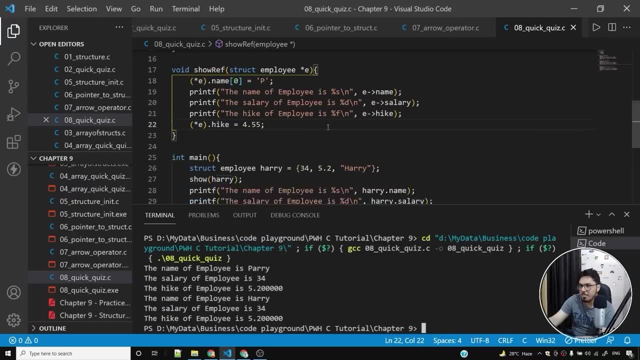 0 is equal to p. all these things can be written like this. okay, now, if i run this program, you'll see that here the change in the structure is going to be the same as the change in the structure is going to be the same as the change in the structure, but the change is not reflected. 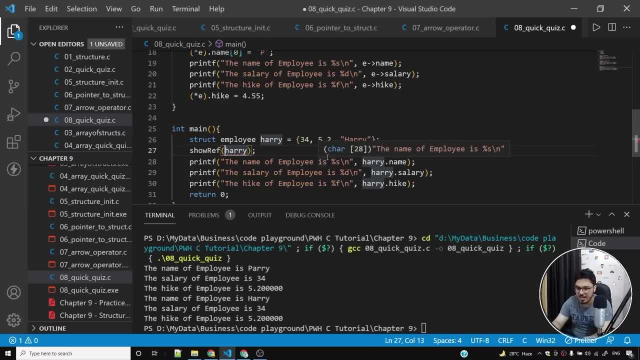 because i'm calling this show function. what if i call suref and i pass the address address of this structure? in this case, what will happen is if i try to run this program, this change is actually reflected here. also the hike change will be reflected. so initially the height change was 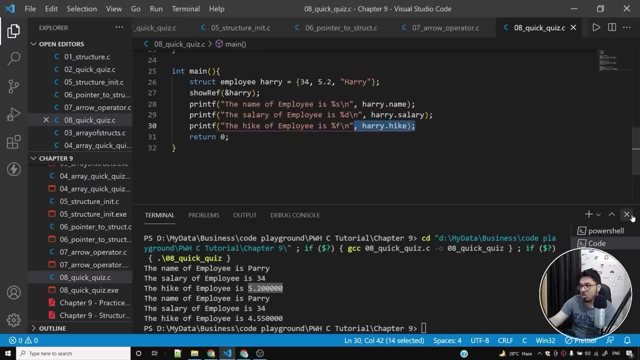 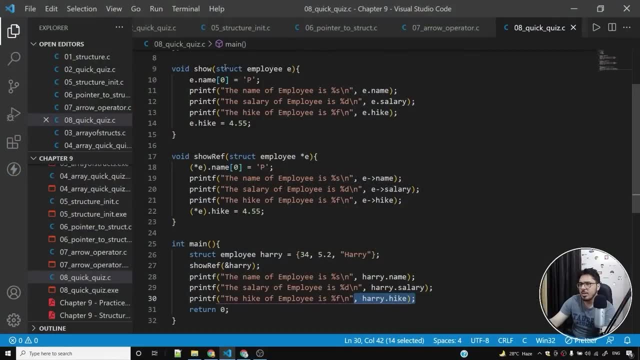 5.22, but after i changed it to 4.55, it will be reflected here. so all these things are something you need to understand. this is basic c logic. i would say this is something that you need to understand by now and i hope that all of you understood. 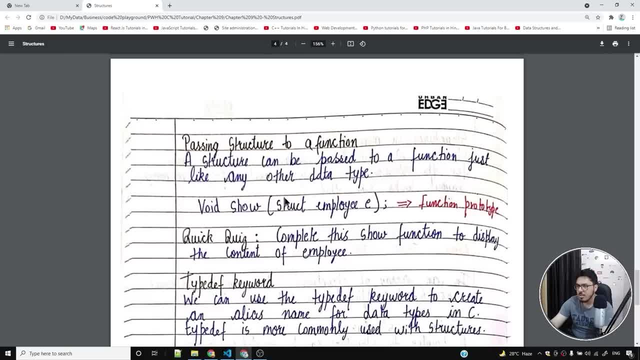 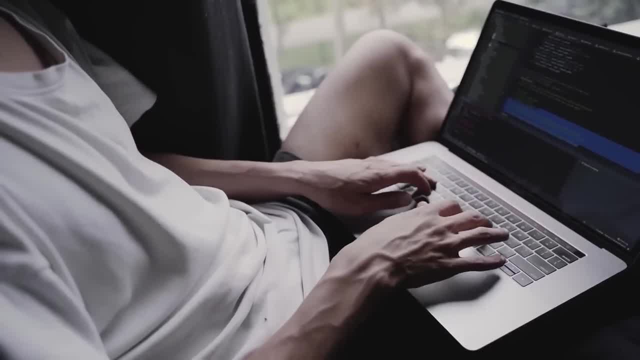 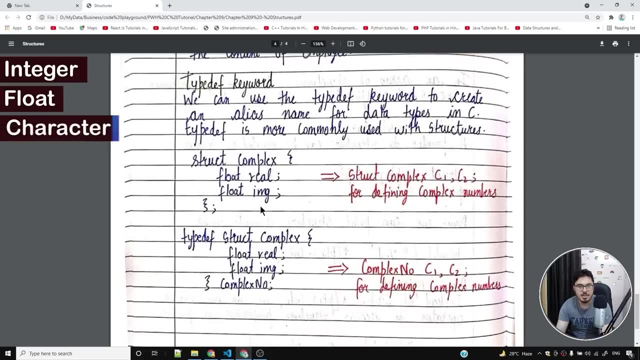 how these things are working by now. now, what we'll do is we'll talk about a keyword which is type def keyword, and this keyword is a syntactic sugar, but really comes very handy. now you, you all, must be thinking that when we have integer data type, float data type, character data. 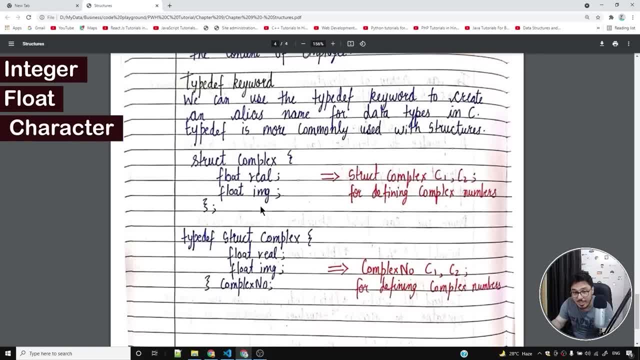 type. all these are single word data types. i can use int a, car b or i can say float c, but when we are using a structure we have to write the struct. we have to write struct complex. but there is a way where, instead of writing struct employee, you can replace all your struct employees with 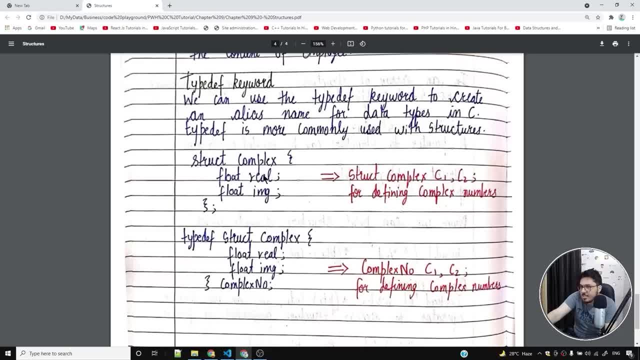 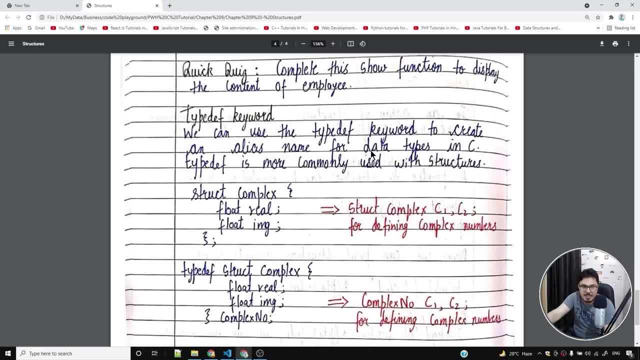 a single word, which is employee. how? how can we do that? in this case, you can use type def keyword. we can use the type def keyword to create an alias name for data types. in c, type def is more commonly used with structures. type def is used with structure. it simply renames the type it it will. 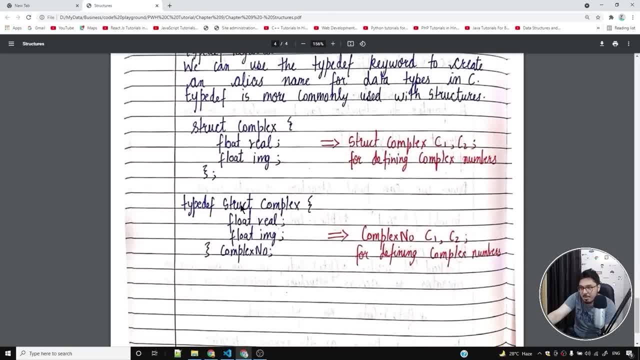 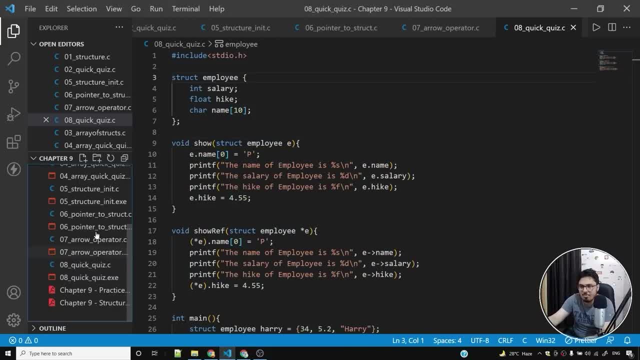 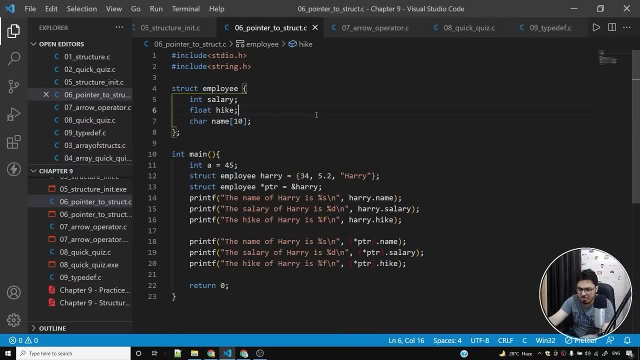 say struct, complex to complex number. so i can say type def, struct, complex, complex number. and in this case what i can do is i can say type def. let me create another program for type def. so i'll say 09 underscore, type def, dot c, and i'll use a very simple program which is here to demonstrate what 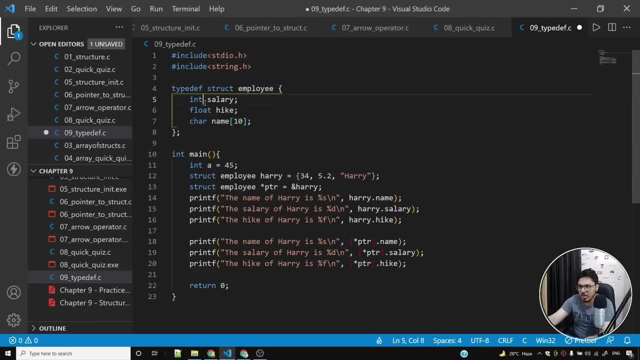 type def is and how it works. so i can say type of struct employee. i can do all these things. and instead of saying employee, i can say emp. I can call this EMP now. So instead of saying struct employee, I can say EMP- EMP here as well. 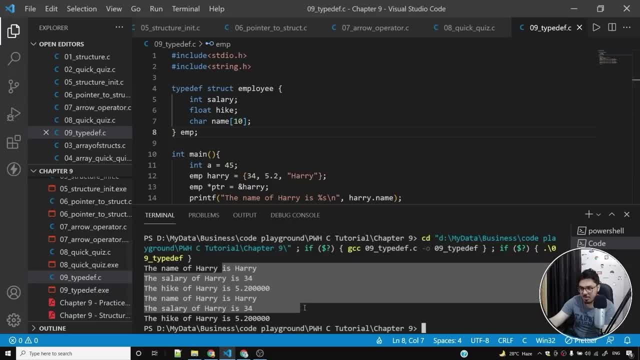 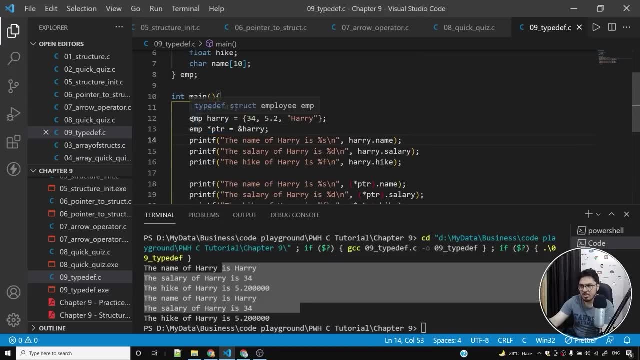 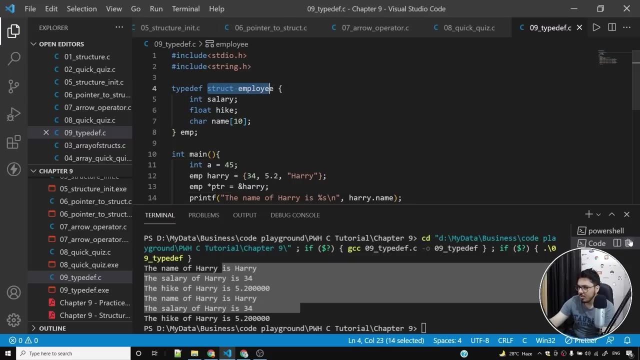 And no prizes for guessing. this will work. this works. So you'll see that we can use EMP to create a pointer as well as to create the structure. We no longer need to type struct employee every time. we want to create a structure of type employee. okay. 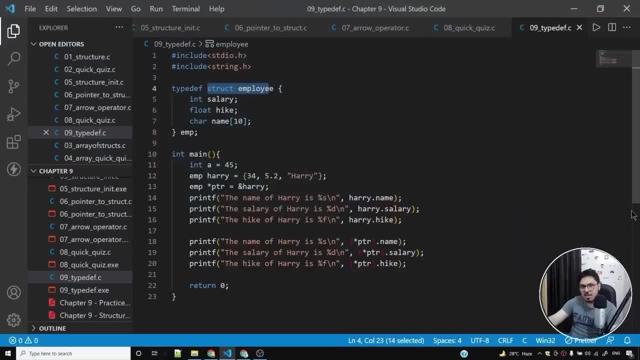 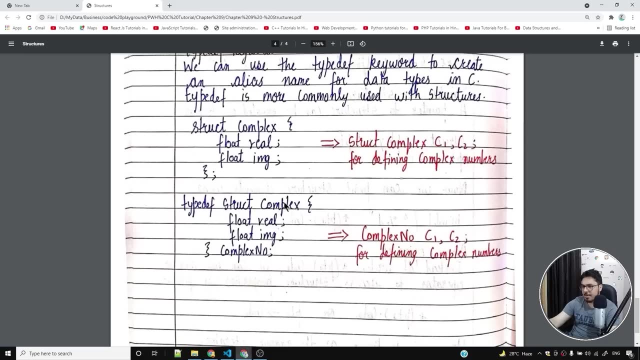 So this comes really very handy when you are dealing with complex programs and you are frustrated writing struct employee, struct employee- again and again. You no longer need to type struct employee again and again. okay, So this is something that you need to understand. 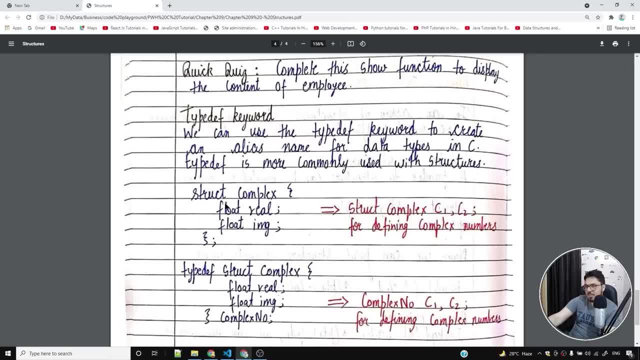 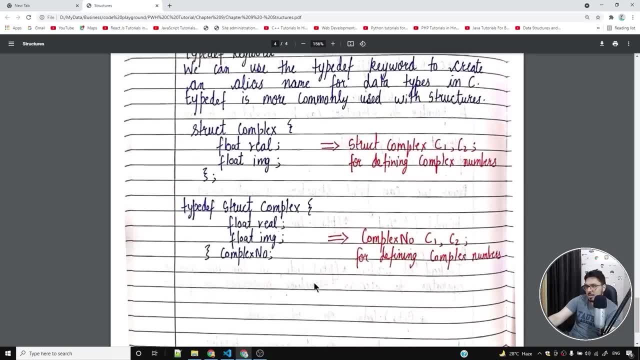 So in this case, what I've done is I've created a diagram for you, I've written the program for you. So, struct: complex C1, C2 for defining complex numbers. This is a structure for defining complex numbers. Now, here we are, using typedef keyword. 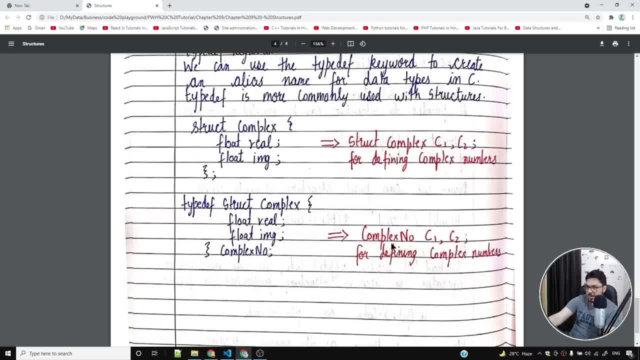 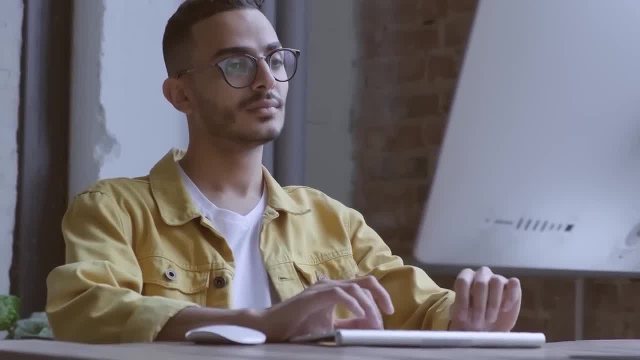 So instead of using struct complex C1, C2, I can write something like this complex number C1, C2. For defining the complex numbers. So I hope that you understood structures well enough and I hope that these notes will help you even further. 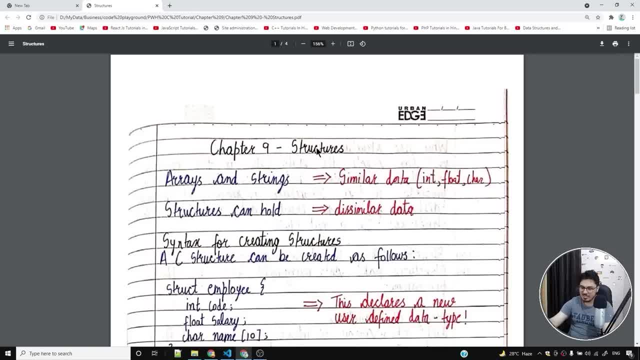 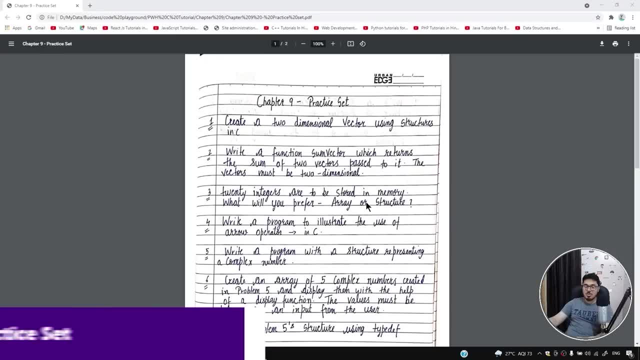 So we'll now move on to chapter nine, practice set, where we'll see all the questions pertaining to structures. Let's move on to chapter nine, practice set now. So let's now talk about chapter nine, practice set. Let's look into the questions in this practice set. 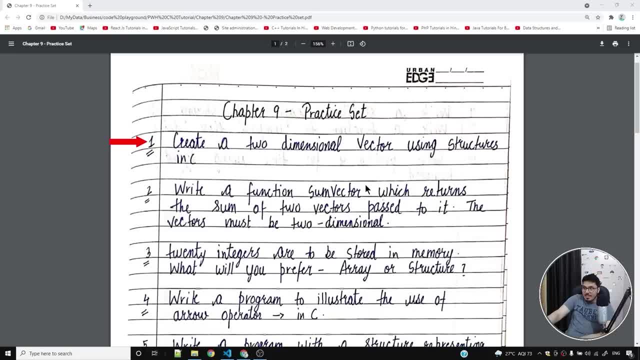 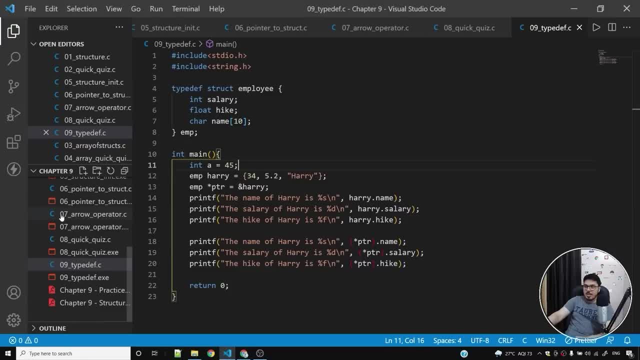 So the question number one says: create a two-dimensional vector using structures in C. So we just have to create a two-dimensional vector. You just have to create a two-dimensional vector Using structures in C. So what I'll do is I'll simply create a program. 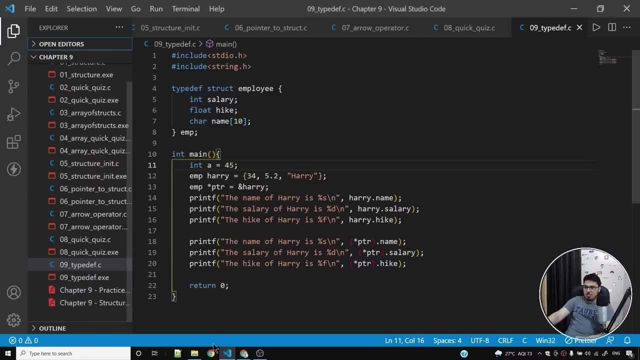 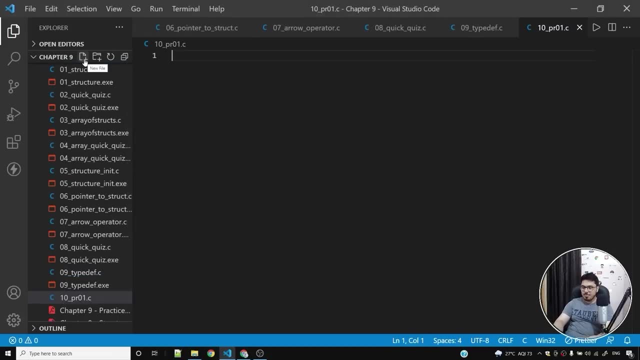 and let me minimize this one. I know I have made a lot of programs, So what I'll do is I'll simply create a new file and say, 10 underscore PR01.C, And I'll put a boilerplate code here. So now what I'll do is I'll simply write a structure. 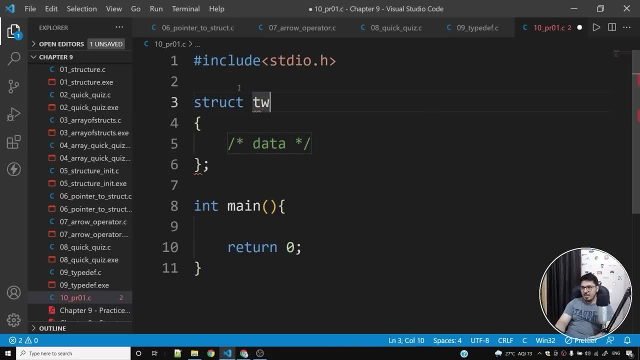 I'll use the snippet and I'll say TWO dim vector And I'll say struct to dim vector And what I'll do is I'll say int X, int Y and that's it. This is a two-dimensional vector. Now what I'll do is I'll simply create. 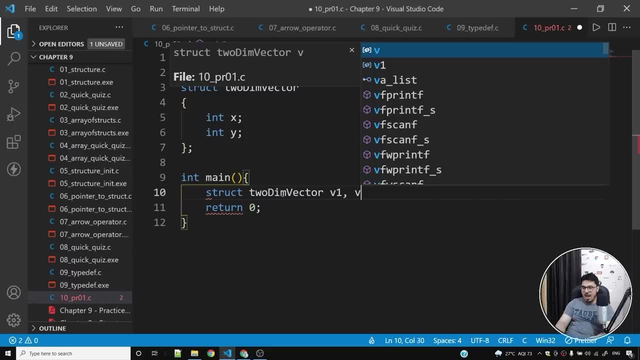 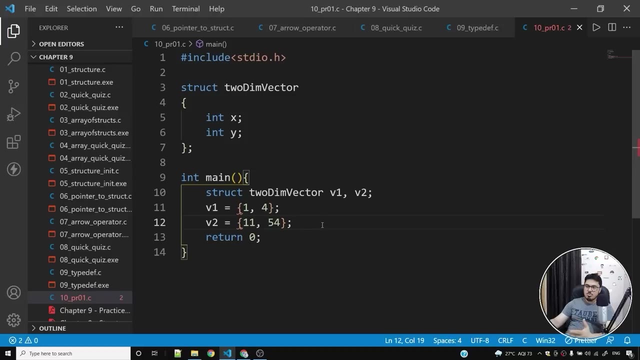 two dim vector, V1 and V2.. Now I can do something like this: I can say V1 is equal to 1, 4 and I can say V2 is equal to 11, 54, let us say, And also I can write a program to print these two vectors. 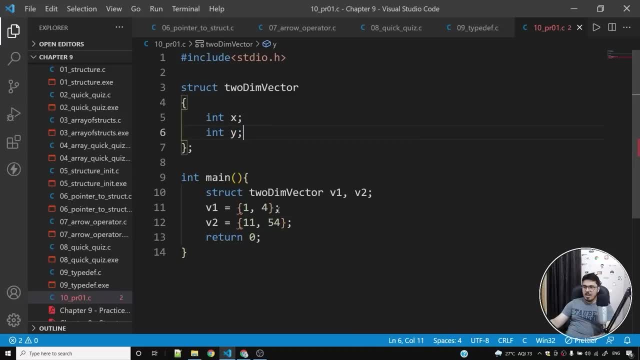 So, just like I have these two integers in text and y, I can simply assign v1 and v2 to 11,, 54 and 14.. Now, in order to initialize it, I will have to write this in a single line, and also the same thing for v2.. 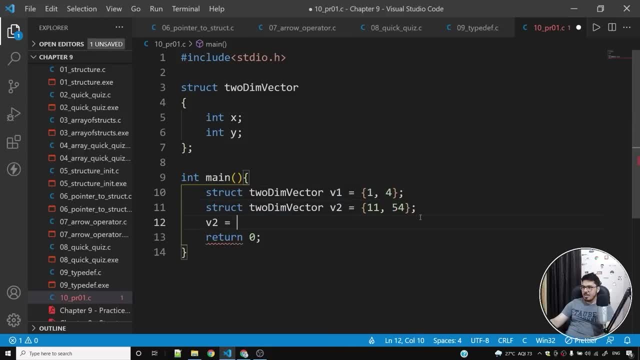 So what I'll do is I'll simply cut this and I'll paste it here. Now I can save it and run this program and it will work fine. But how do I know that it is going to work fine? I can simply print. I can do something like this: 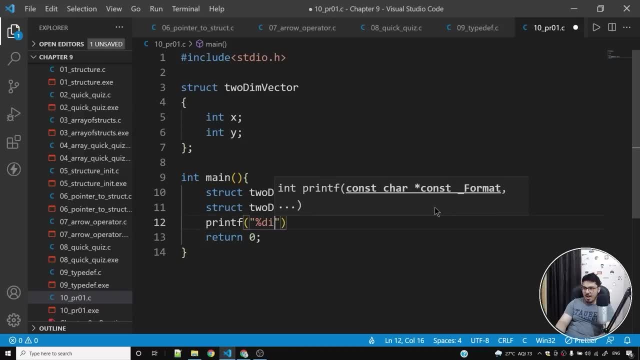 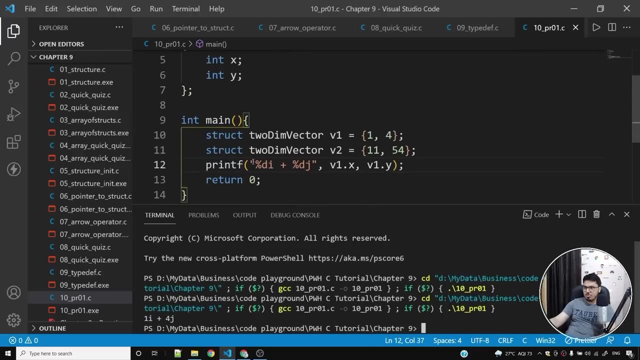 printf %d i plus %d j, and what I'll do is I'll say v1.x and v1.y, okay, And this should print v1.. So if I run this program, you can say one i plus four j. So this is printing a two-dimensional array. 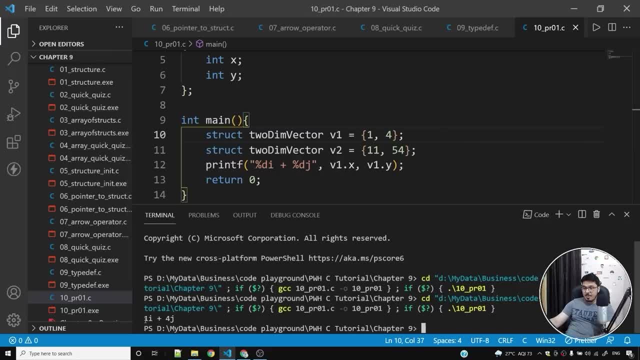 If you don't know what a two-dimensional array is, simply consider two-dimensional array to be an entity which contains two different integers: One is the x-axis, one is the y-axis. So let's move on to the next question now. The next question says that write a function: sum vector. 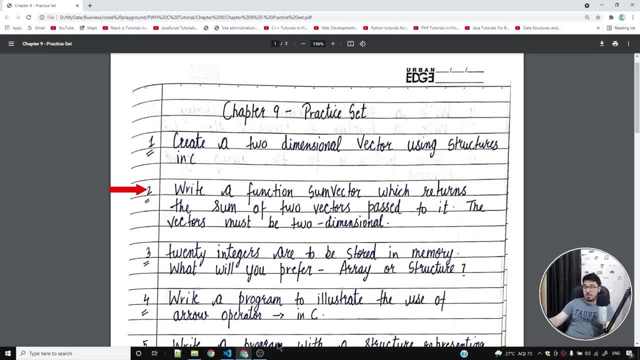 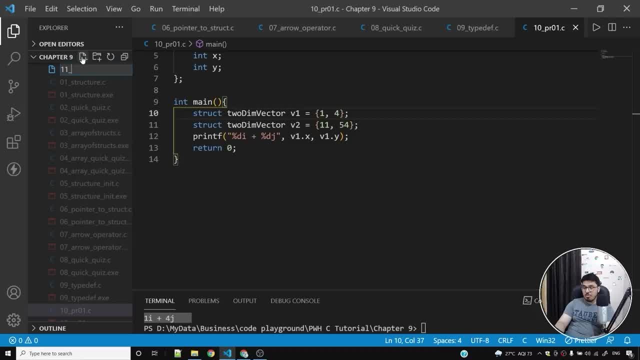 which returns the sum of two vectors passed to it. The vectors must be two-dimensional. So we have created a two-dimensional array. Now we want to create a function which can add such two-dimensional arrays. If you don't know how to add two two-dimensional vectors, 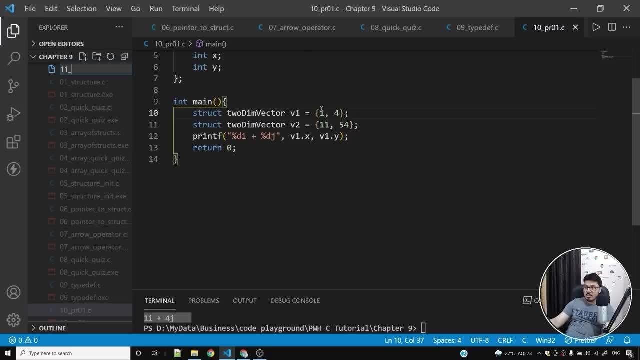 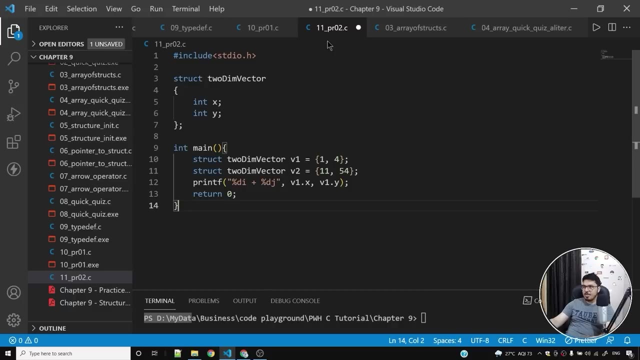 what we can do is we can add their x components and we can add their y components and the resulting vector will be the sum of these two vectors. So I'll say pr02.. pr02.c also, I'll copy this. I'll copy this program and I'll paste it here. 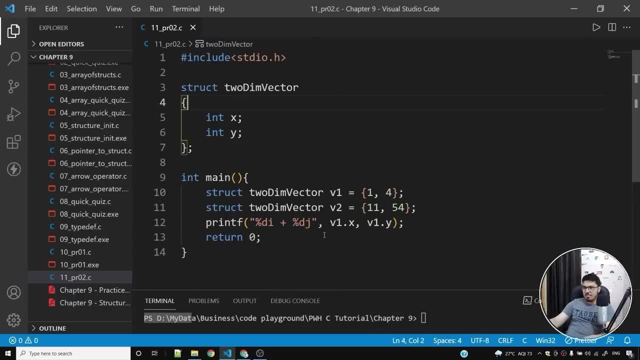 Also, I'll close other programs. I'll say: close others, I'll save this program. so v1 and v2 are two vectors. I'll do something. I'll say v3 is equal to, so we have to create a function: sum. 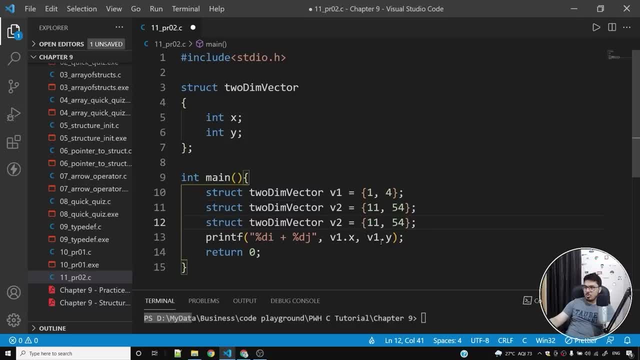 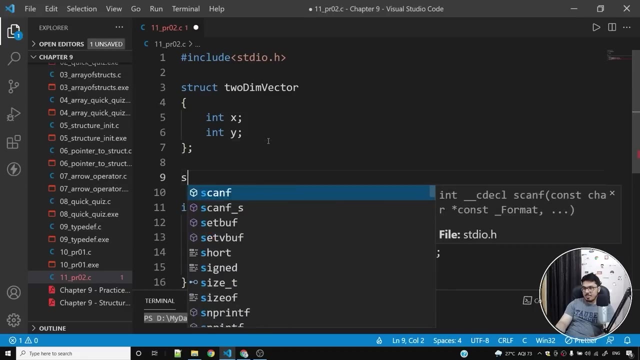 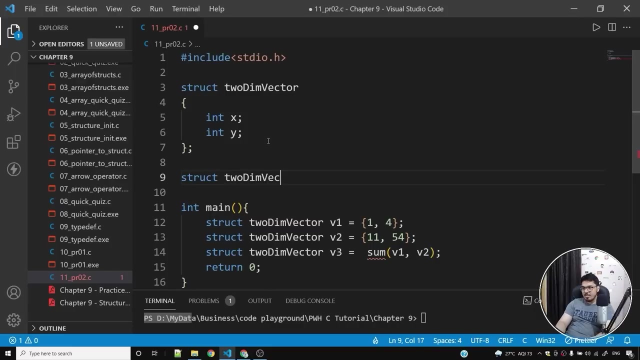 I'll say struct to dim. v3 is equal to sum of v1 and v2.. v1 and v2.. So sum is a function which will take two vectors which are two-dimensional vectors, and it will return a structure. So I'll say: struct to dim vector sum. 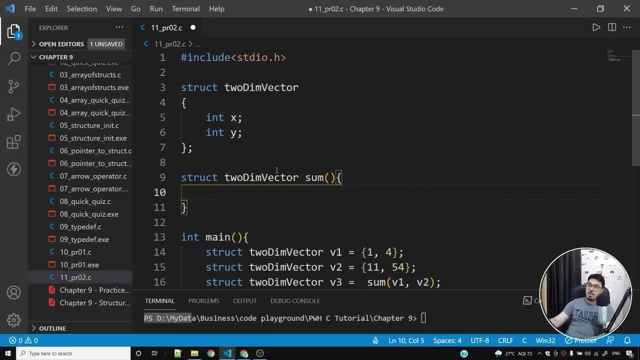 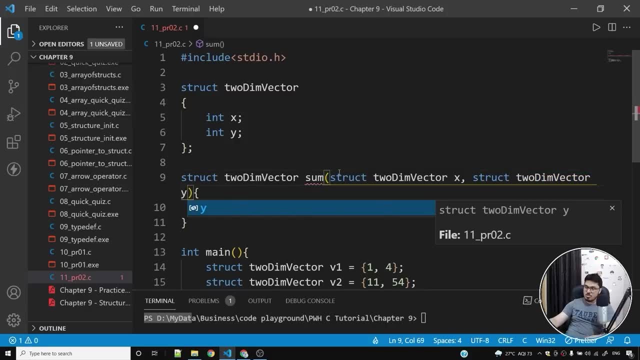 and this is a function. sum is a function, And this function is going to take two two-dimensional vectors. Let us call them x and y. So this will take two two-dimensional vectors. So this will take two two-dimensional vectors. So what I'll do is I'll create a third. 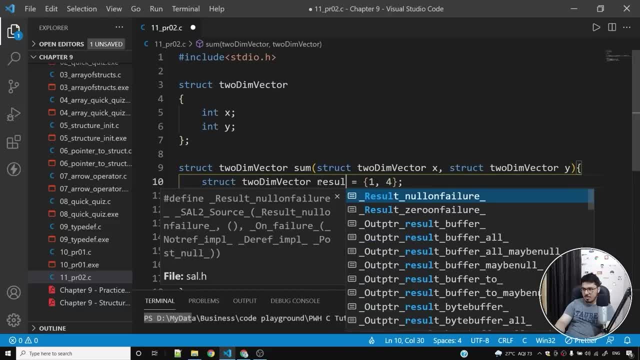 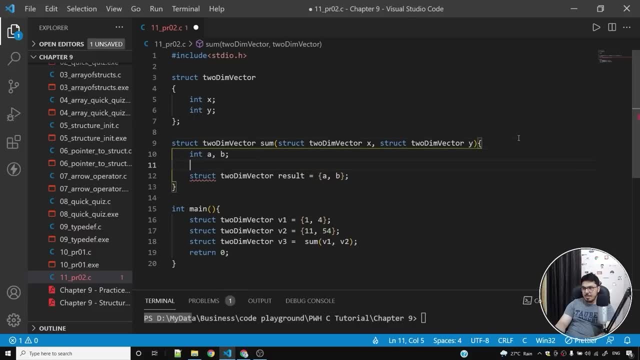 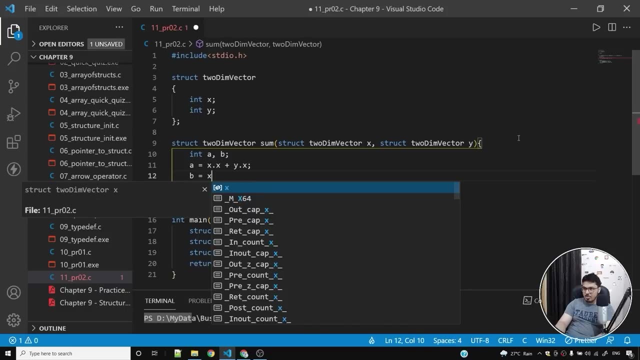 two-dimensional vector. here I'll say result, And result will contain a and b. Now, what is this? a and b? A and b are two integers, Int ab. a is equal to xx plus yx and b is equal to xy plus yy. okay, 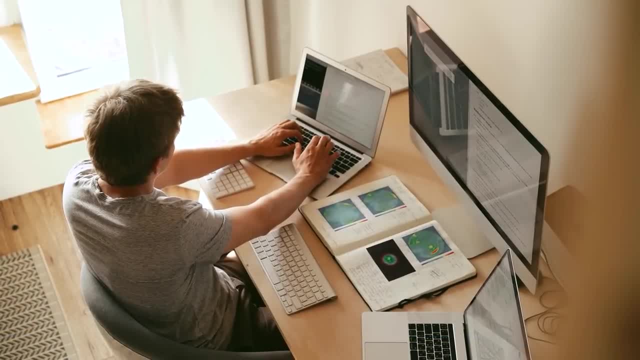 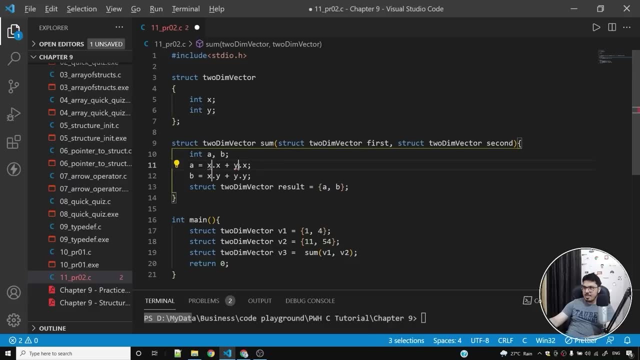 So what is this vector? To make it a bit less confusing, what I'll do is I'll call this first and I'll call this one second, And instead of writing x dot x and y dot y, I'll simply write first and second. 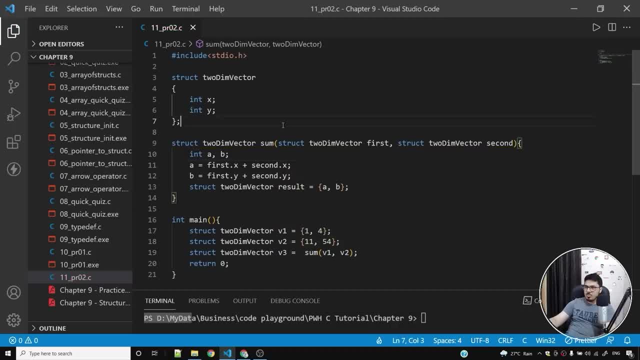 So I'll write first here and I'll write second here. So a is the sum of x components from first and the second vectors, And b is the sum of y components of first and second vectors. So a is equal to this thing, y is equal to this. 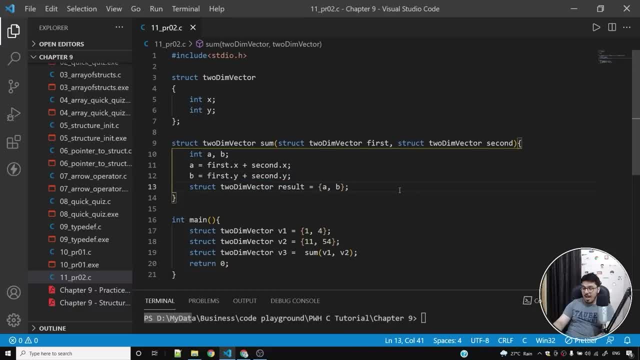 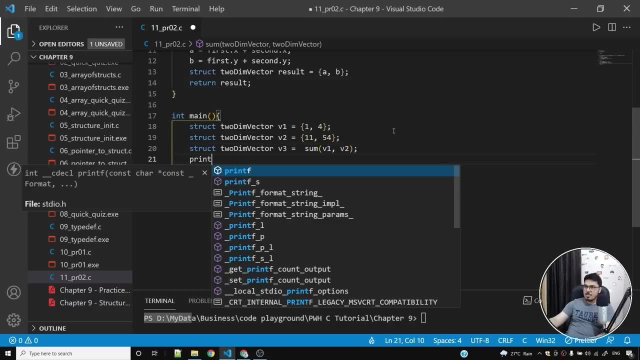 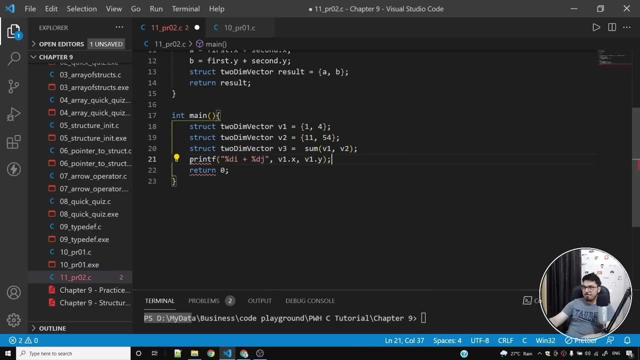 b is equal to this thing and the resulting vector is this: And I will return result. And I will return result. Okay, Now let's see if I'm able to print this vector, just like I was able to print this here. So, instead of printing this for v1, I'll print it for v3. 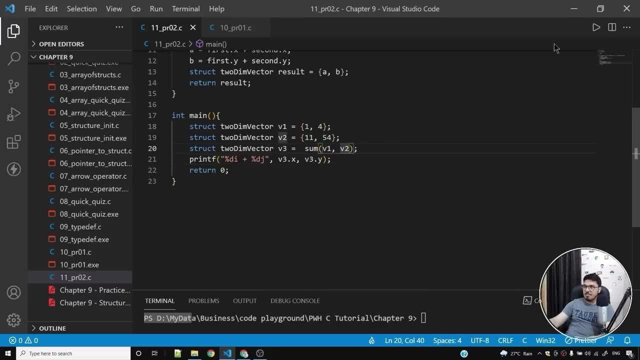 And I'll see if v3 is the sum of v1 and v2.. So I should get 12 and 58.. Am I getting 12 and 58?? Yes, I'm getting 12 and 58. Which means that I'm able to sum these two vectors. 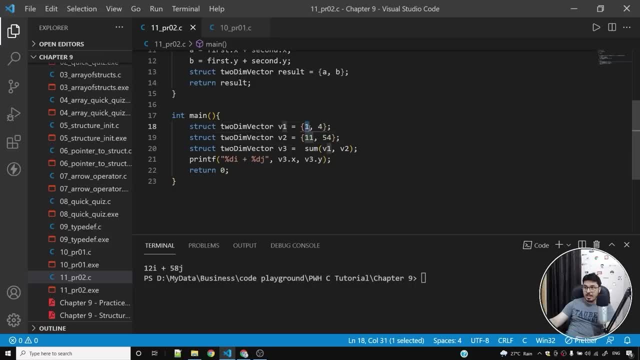 The sum of these two vectors is going to be 11 and one, one individually summed, and 54 and four individually summed, which is going to return us 12i plus 58j. Okay, I hope that makes sense. Let's now move on to the next question. 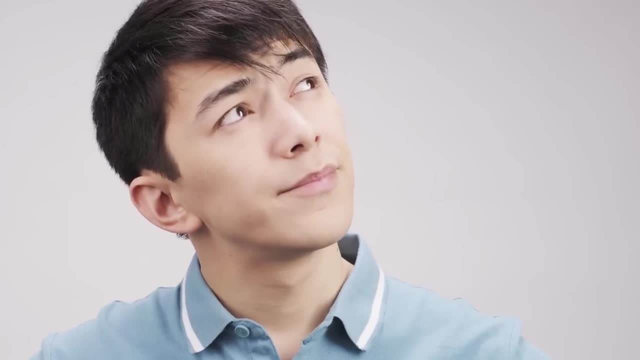 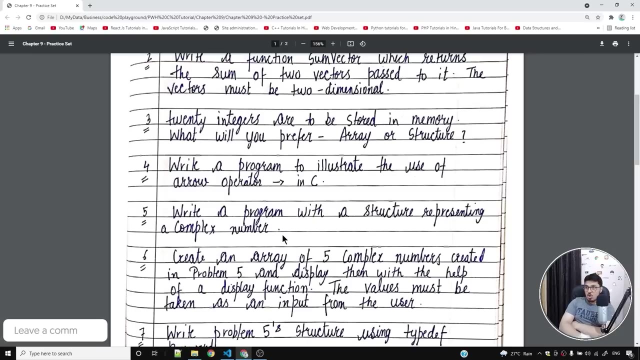 20 integers are to be stored in memory. What will you prefer? Will you prefer an array or structure? This is an important question and you need to think about it and tell me the answer in the comment sections. So, if you have 20 integers waiting, 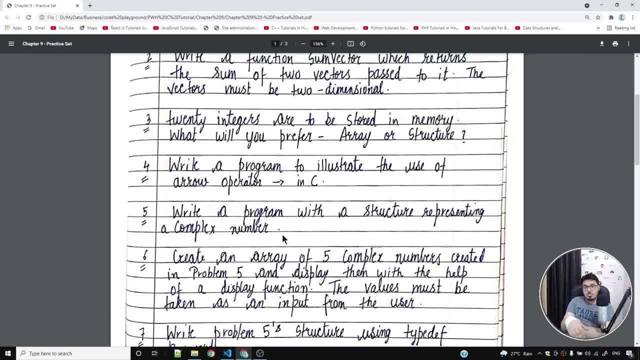 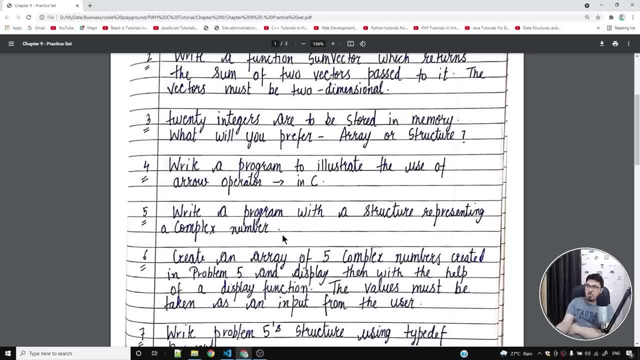 Are you going to create a structure with 20 integers? Are you going to create an array? Definitely, you are going to create an array, because we use structures when we have a collection of dissimilar data types and we use arrays when we have 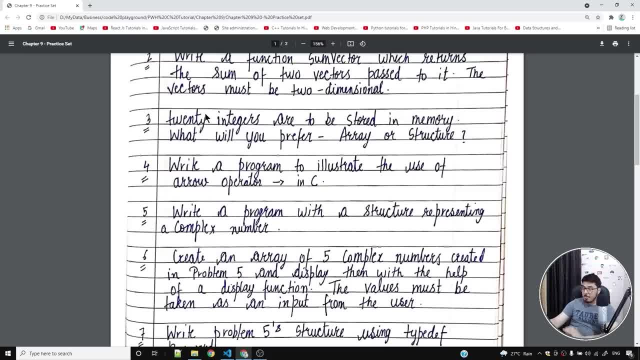 a collection of similar data types. 20 integers will be all of type integers and they are a collection of similar data types, which is why we will prefer arrays. Okay, We'll write a program to illustrate the use of arrow operator in C. 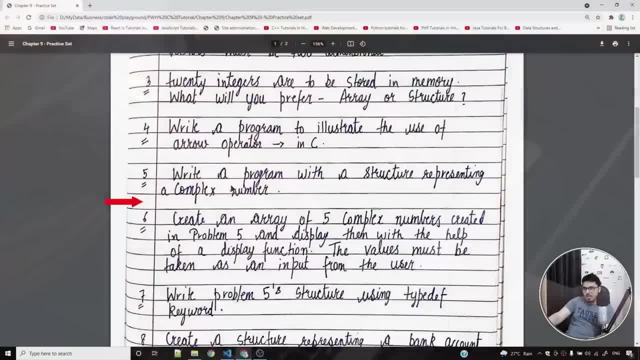 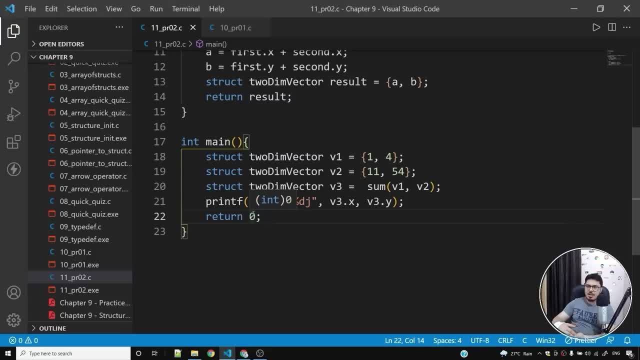 We have talked enough about it. I want you to attempt this program on your own. Let's move on to question number five. Let's move on to question number five. Write a program with a structure representing a complex number, and a complex number will have a real part. 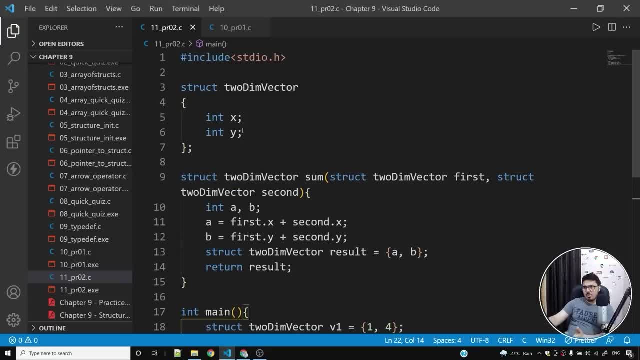 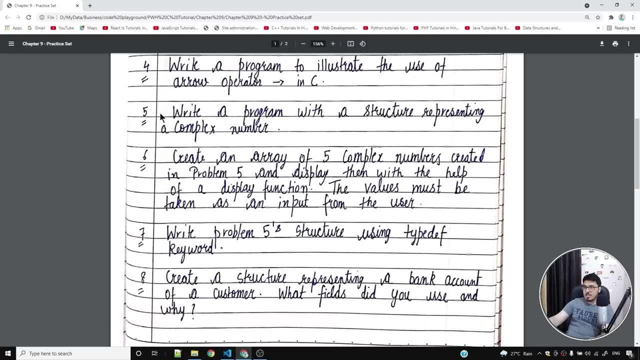 and a complex part. okay, Just like a two-dimensional array, we can use real part and complex part to store a complex number. So let's solve this problem. Which problem is this? This is problem number five. So what I'll do is I'll create a program. 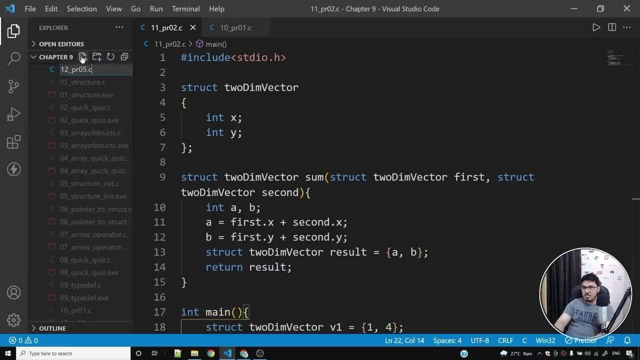 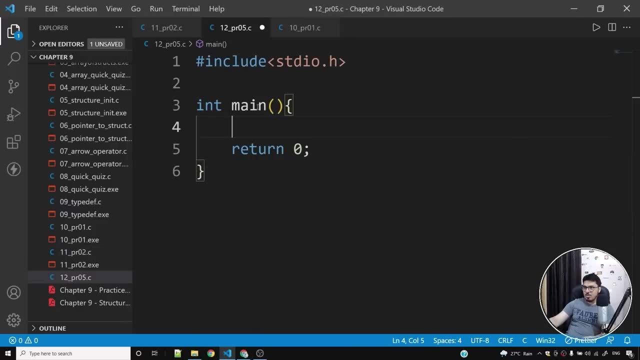 12 underscore: PR05 dot C. zero five dot C. I'll put in a boilerplate code and what I'll do is I'll copy this, this structure, and instead of making it in this time, I'll make it float. 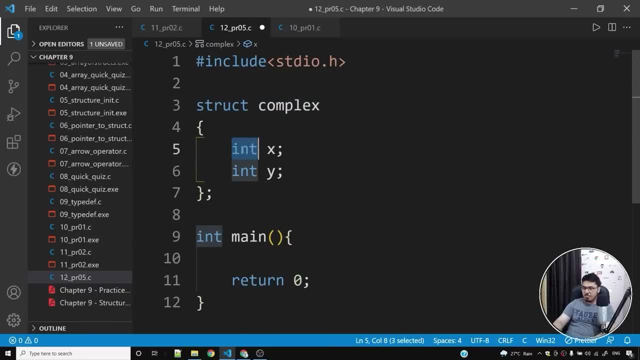 So I'll say complex. I'll make it float real- R for real and float C- C for complex. So it will have a real part and a complex part, and the rest of the things are going to be the same. 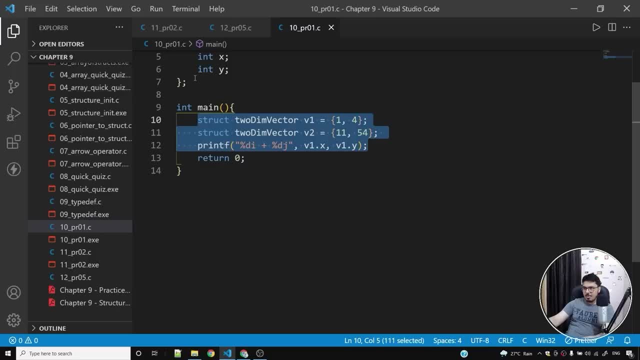 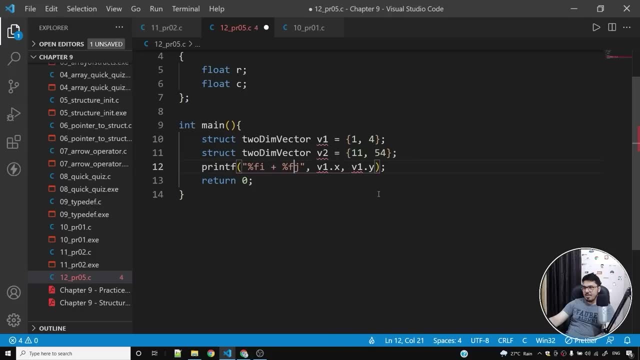 just like our 10th program. So it's going to be the same, except the fact that instead of taking integers, we'll use floats. So we'll say percentage F here. And instead of saying R- sorry, instead of saying X, we'll say R and C. 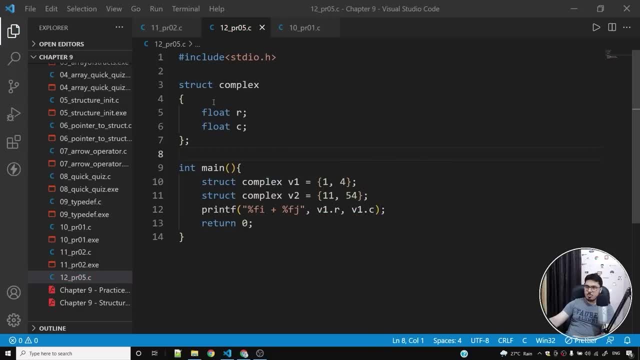 real and complex And instead of saying two-dim vector, I'm going to use complex, which is the name of our structure And this program should work. Instead of making it four, I'm going to make it 0.4,. 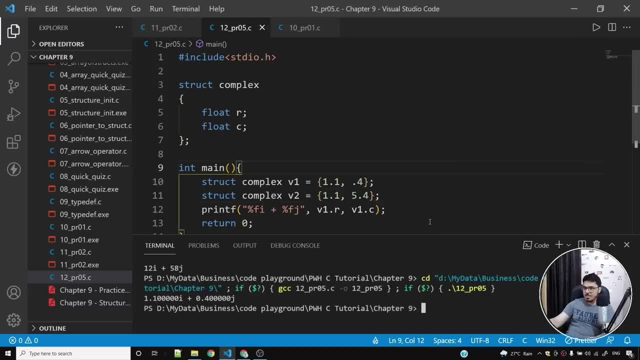 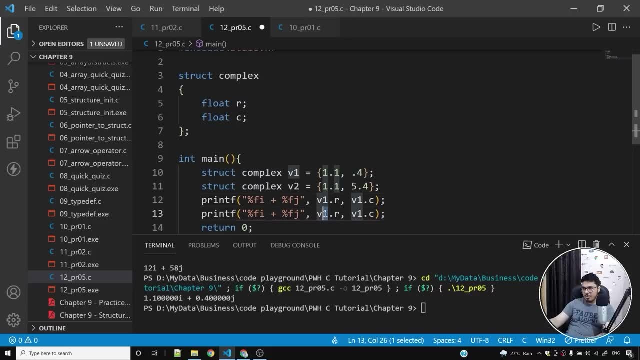 let us say 5.4,, 1.1, and let's see what it returns. So 1.1 I plus 0.4 J, which is true. I'm able to print V1.. In a very similar way, I can print V2 as well. 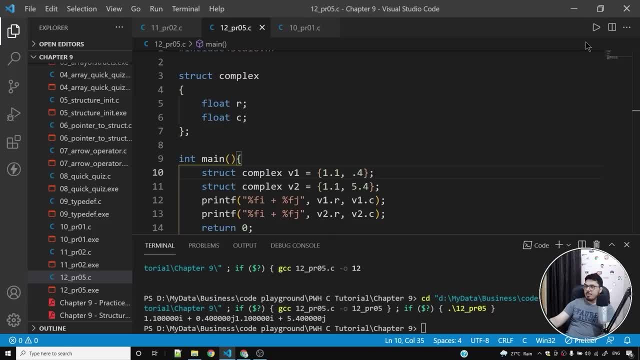 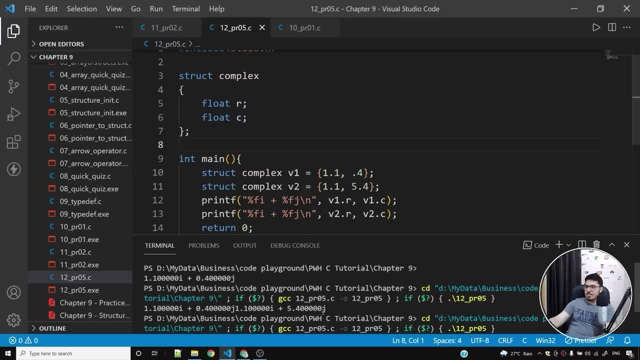 So I can print V2, something like this: Okay, so if I print V2, it is going to look something like this: I should use backslash N to better format it, And you can see that I have this 1.1 I plus 0.4 J. 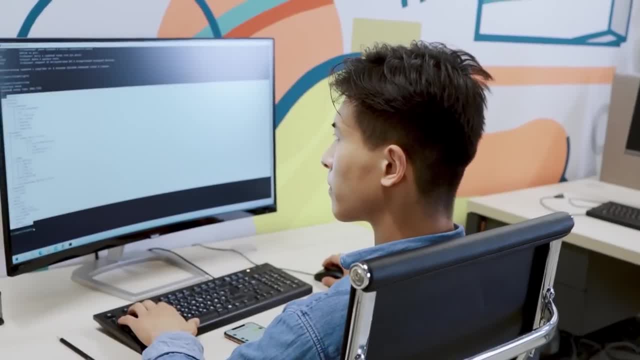 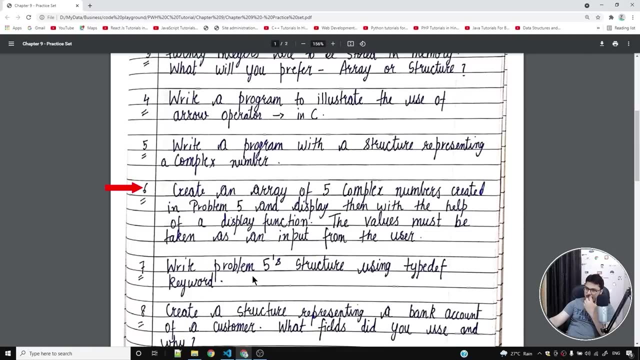 1.1 I plus 5.4 J. So I hope that you are able to understand how we solved this problem And let's move on to problem number six. Problem number six A is: create an array of five complex numbers created in problem five. 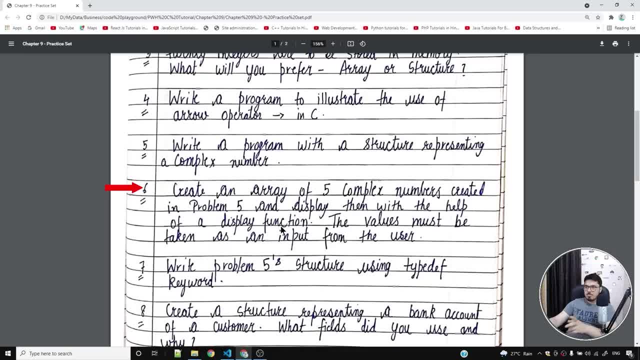 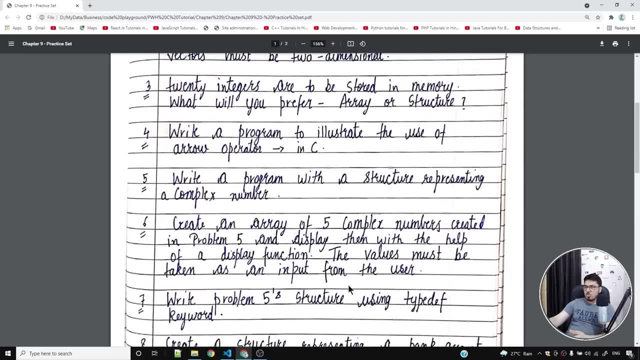 and display them with the help of a display function. The values must be taken as an input from the user. So you know how scanf works. We have already seen how to add two numbers. You can always create an array. We have already seen a program on array of structures. 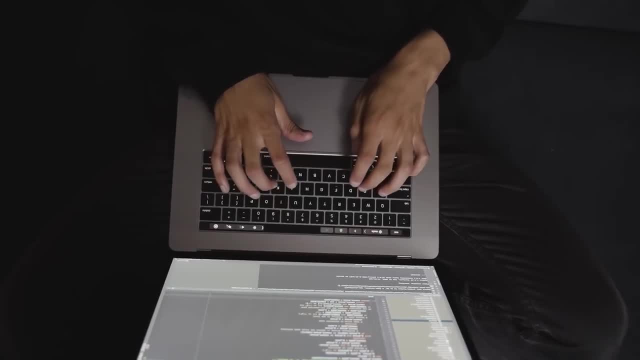 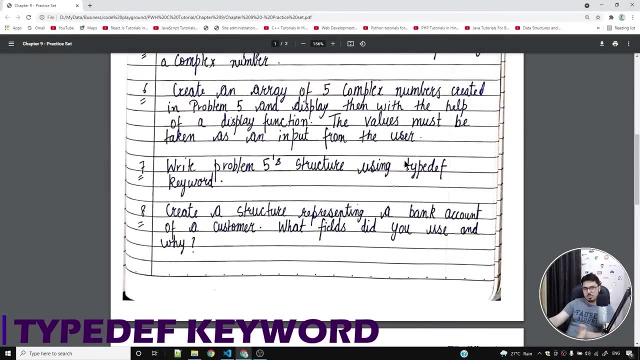 So I want you to use those learnings and solve this problem. And, in a very similar way, you can refactor the program to use the typedef keyword. We have talked about typedef keyword and how it works. okay, Question number eight says that 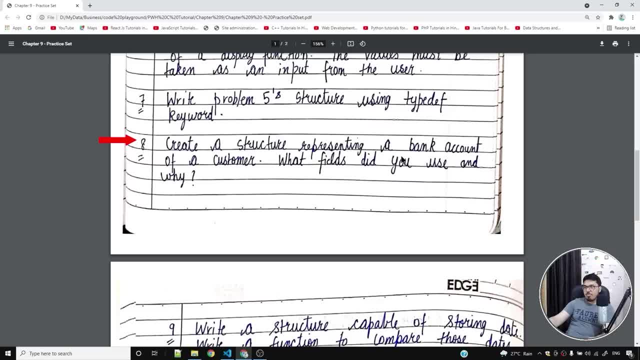 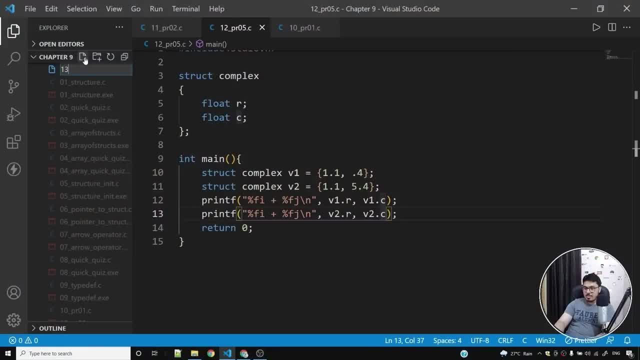 create a structure representing a bank account of a customer. What fields did you use, and why So? in order to create a structure for storing bank account of a customer? So I'll say PR. it's problem number eight, So I'll say PR08.c. 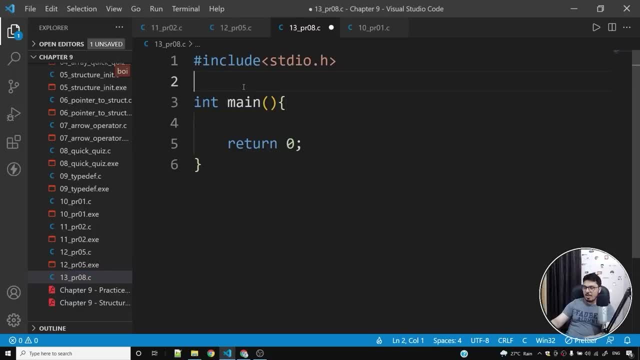 I'll put a boilerplate code here And I'll create a structure bank account. So I'll say struct bank and what will I put inside it? I'll say struct bank. I'll say int account number. Also, I'll create a name. 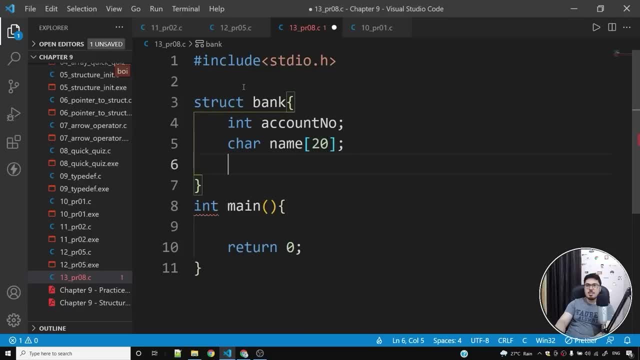 I'll say a name field for 20 characters, I'll say float, balance, And also I'll say: let us add a few more fields. What else can I add? So these are the three things that comes to my mind. 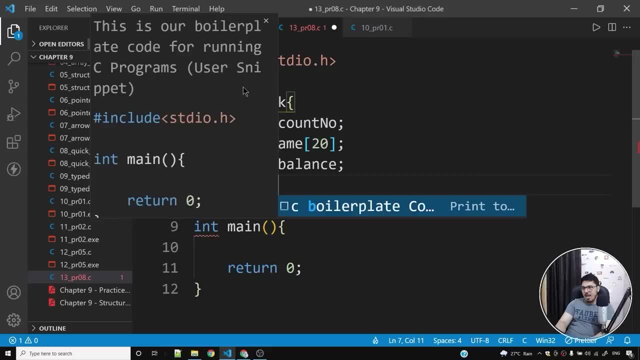 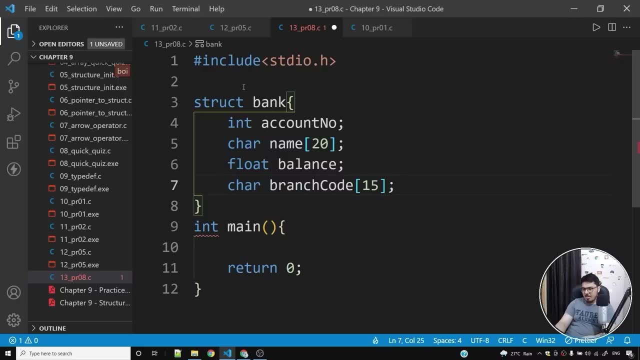 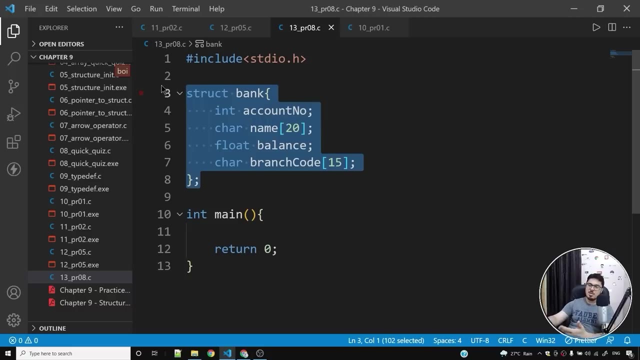 I can also say branch code. I can say char branch code and let's give it 15 characters, And also you can add some other fields. This answer need not be unique. You can come up with your innovative bank which will have some of the other fields for the customers. 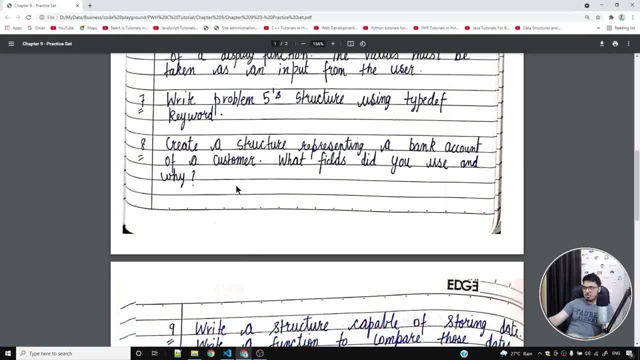 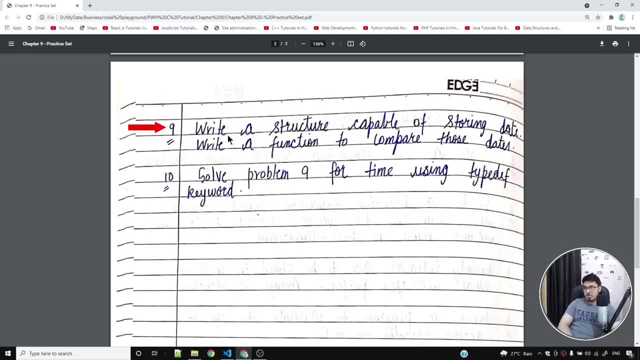 So this is what came to my mind, So I've added these fields. So question number eight is done. Let's solve question number nine now. Write a structure capable of storing date. Write a function to compare those dates. So this is something that I want you to solve. 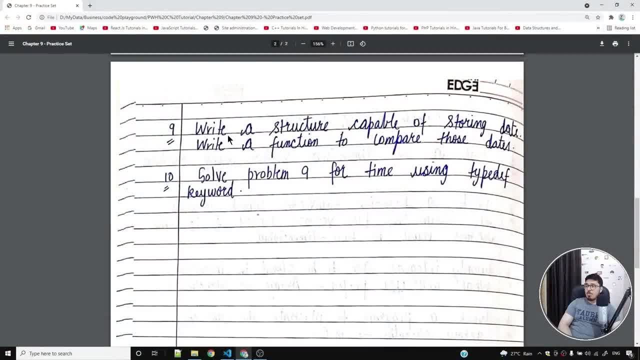 because we have already talked a lot about structures, Write a structure capable of storing date. So what, all fields, do you want to store inside a date? Maybe you want to store month. Maybe you want to store year. Also, you might want to store a day. 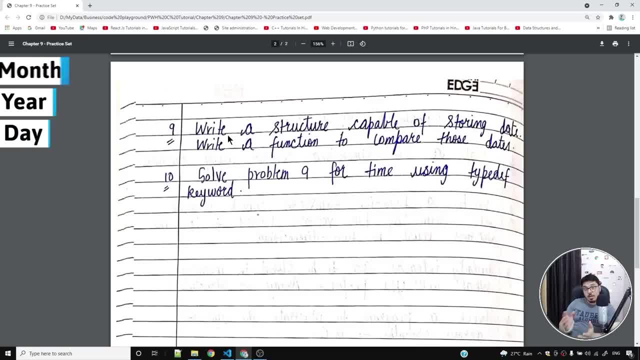 Okay, so day, month and year, And when you're comparing these dates, you can, one by one, compare these three things. Firstly, you will compare the year, Then you will compare the month. if the year is same, Then you will compare the dates. 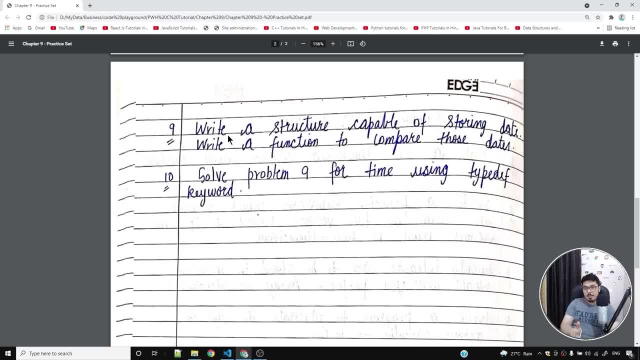 So you can easily tell which of the dates are occurring before, Let us say, the other date, So you can compare two dates And you can tell that which of these dates will appear first in the calendar. okay, So I want you to solve this problem. 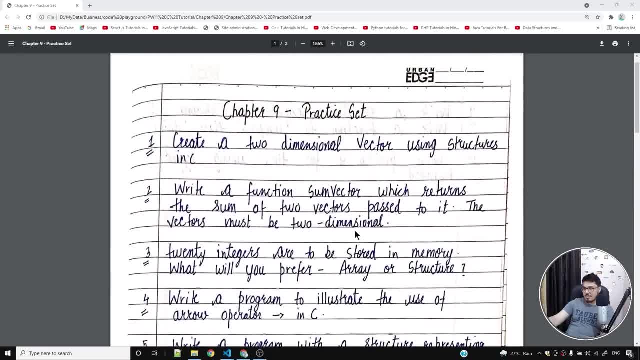 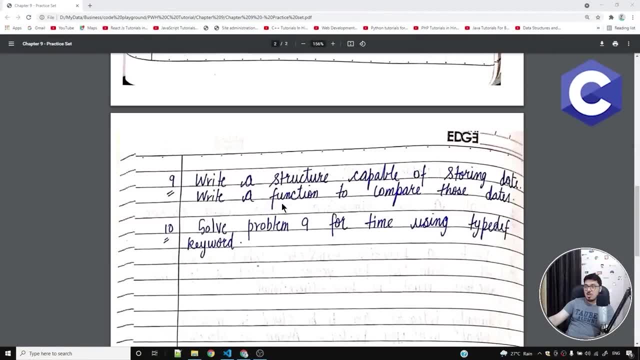 Now I'm aware of the fact that I've skipped most of the problems here, And the reason being: I want you to practice now because we have already completed nine chapters and we have learned a lot about C programming language. So problem number 10 is very easy. 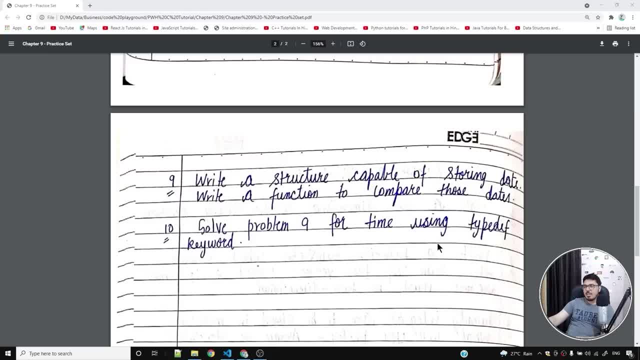 You have to refactor the program in problem number nine to type def keyword, and I know you can do that. So with this question we have finished chapter nine. practice it Now. what we are going to do is we are going to move. 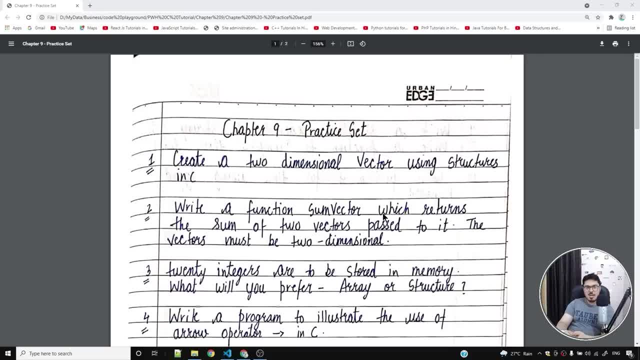 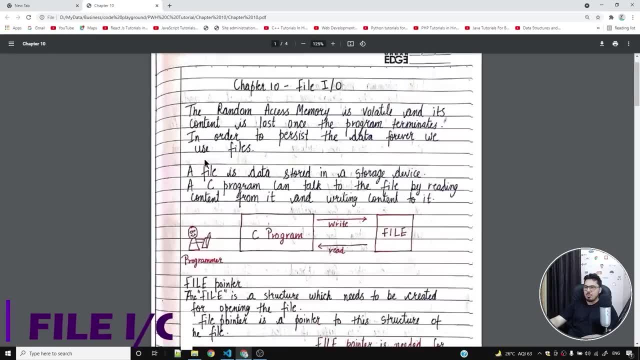 into chapter number 10 and learn more about the C concepts. Let's move on to chapter 10 now. So now we'll move on to chapter number 10 and we'll start discussing file IO. So the random access memory is volatile. 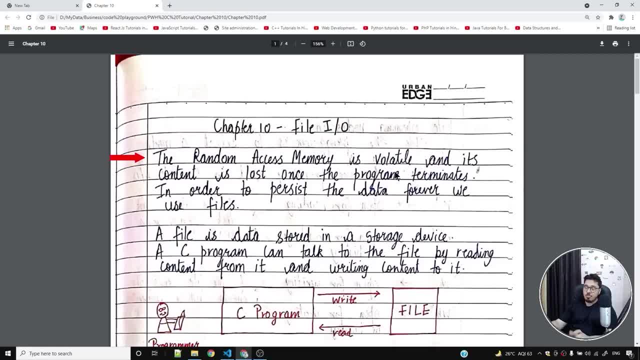 and its content is lost once the program terminates. So if you are aware of how programs work in a particular computer or in any particular device, what happens is the program is first loaded into the memory, and that memory is nothing but RAM, which is the random access memory. 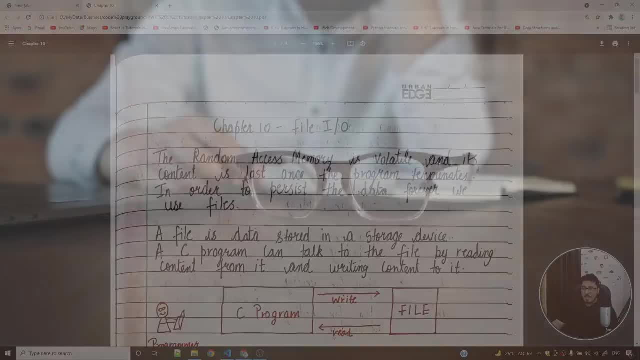 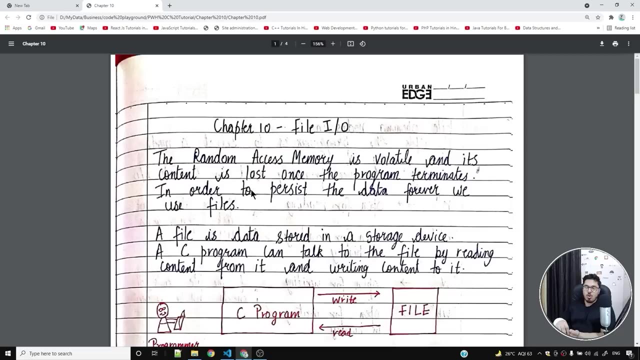 And all the content of that random access memory will get lost once the program terminates. In order to persist data forever, we use files. So in order to persist data, in order to make the data available later, even after the computer is turned off. 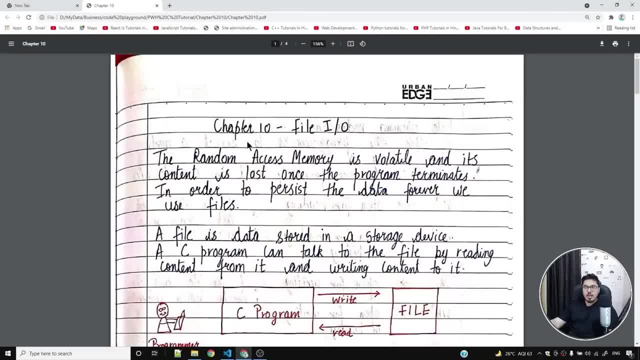 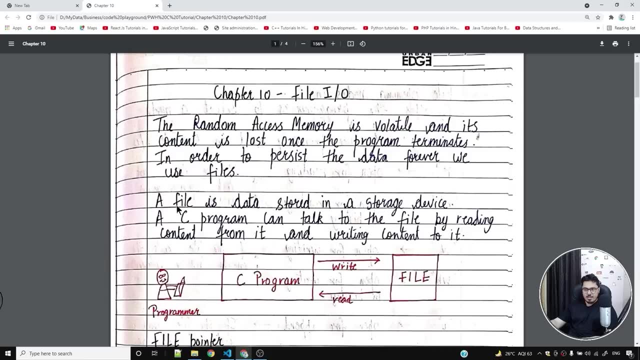 you need to store it in files inside your hard drives. You cannot store data in your RAM and expect it to be available all the time. In order to do that, you will have to store your data inside hard disk or some storage device, And we store our data in the form of files. 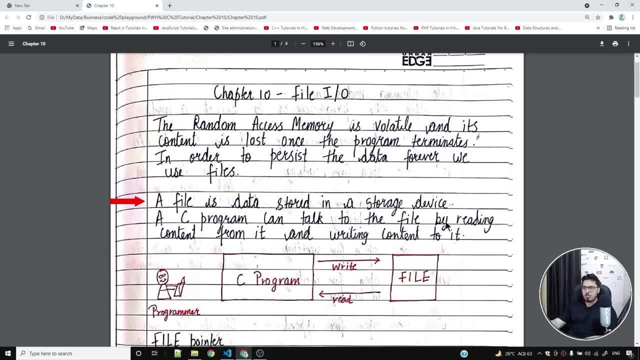 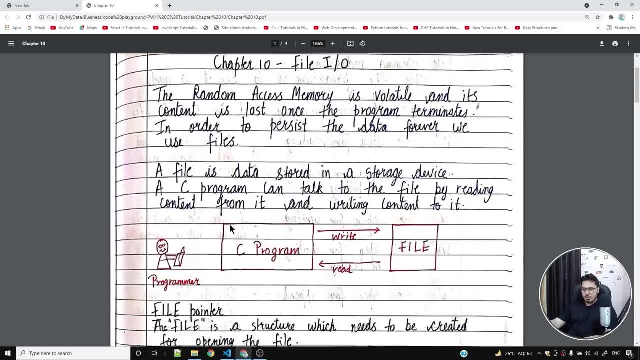 A file is the data stored in a storage device. A C program can talk to the file by reading content from it. So a C program can talk to the file by reading content from it and writing content to it. So here is a visual diagram. 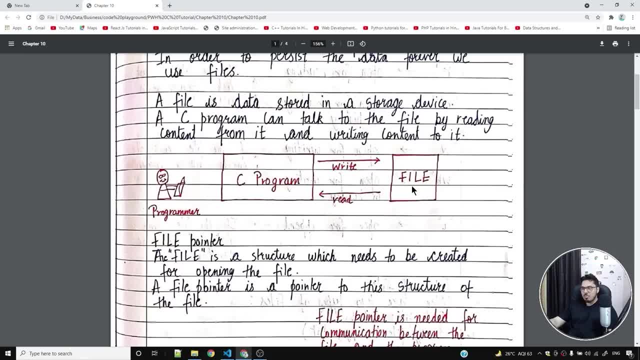 I hope you like this programmer. C program can write to a file and it can read from a file. So a C program can actually write data to a file inside a storage drive. It can be a hard drive, It can be a USB drive. 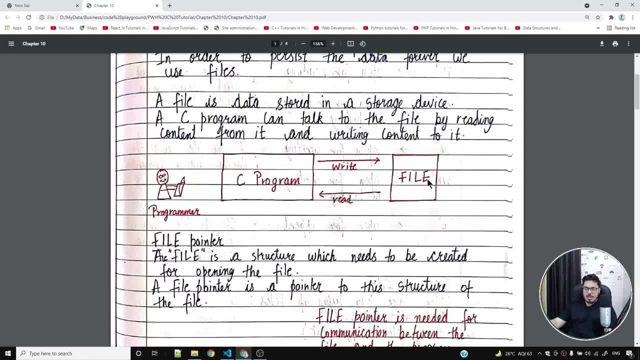 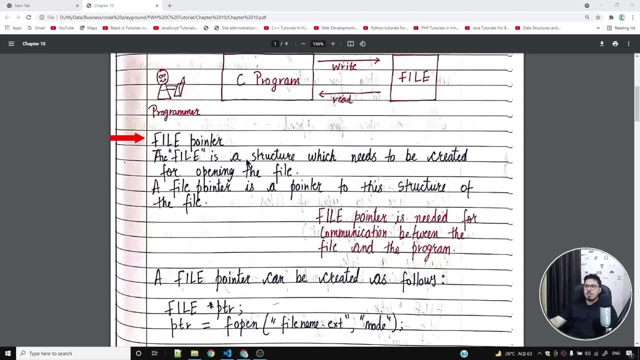 It can be anything. Your program can talk to this file and perform read and write operations. So let's now discuss what a file pointer is. A file is a structure which needs to be created for opening the file. okay, So this is a pointer which needs to be created. 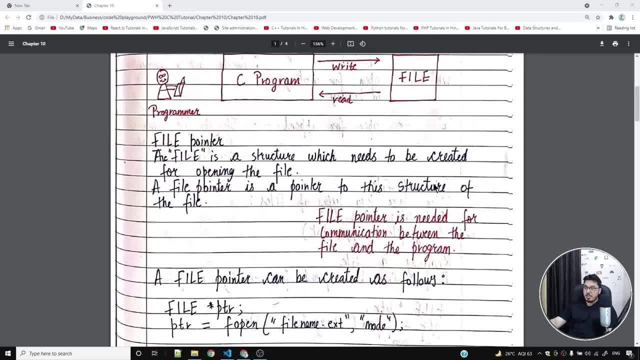 for opening the file, The file pointer. a file pointer is a pointer to the structure of the file. So a file is a structure and file pointer is a pointer to the structure. okay, File pointer is needed for communication between the file and the program. 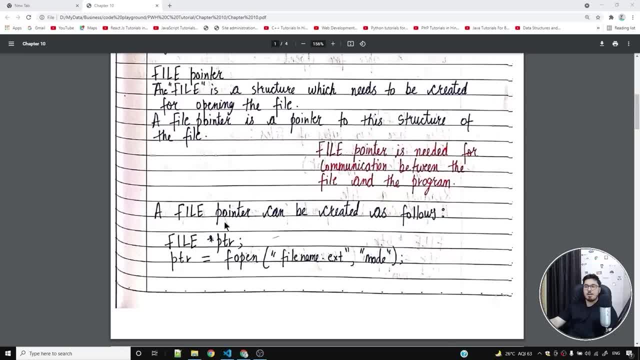 So if you need to talk to this file, you'll have to create a file pointer. A file pointer can be created as follows: All you need to do is you need to type file star, ptr, and all you need to do is you need to use this: have open function. 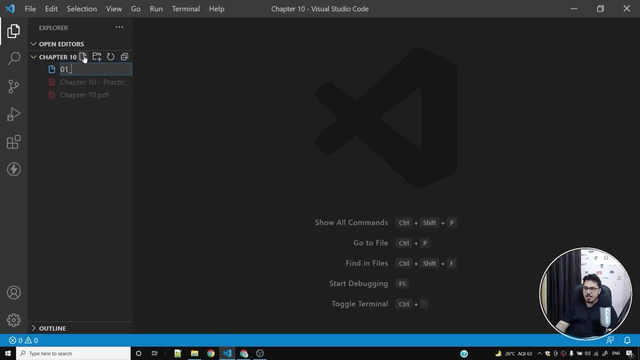 which is available. Let's create a program which can read a file. So I'll say: read filec. I'll put in the boilerplate code. I'll also, you know, write a sample filetxt and I'll say: this is a sample file. 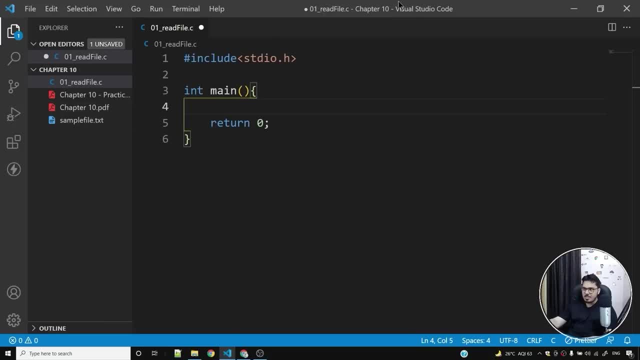 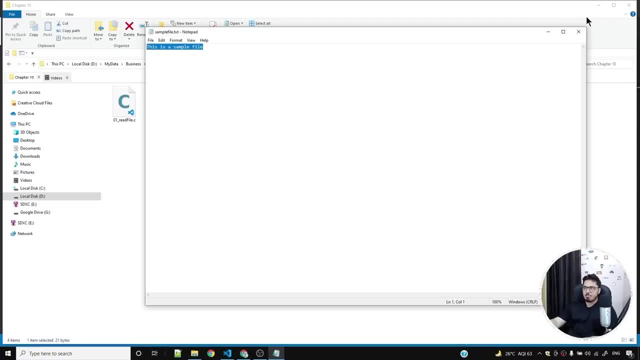 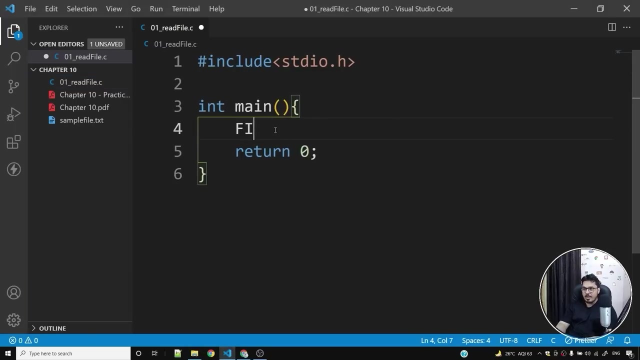 this file. so what i've done is inside my hard disk at this location, wherever this folder is open at this location, what i've done is i've created this sample filetxt and i've generated some content inside it. now what i'm doing is i'm trying to create a file pointer, so i need to keep it in. 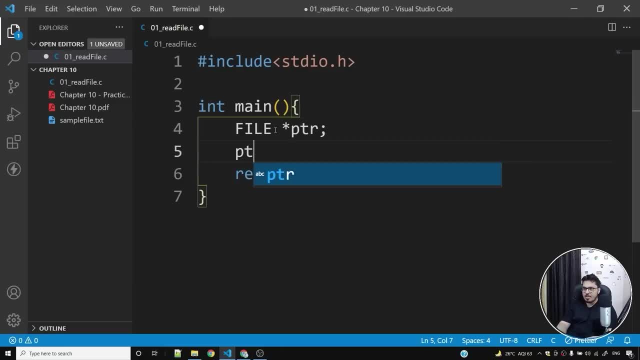 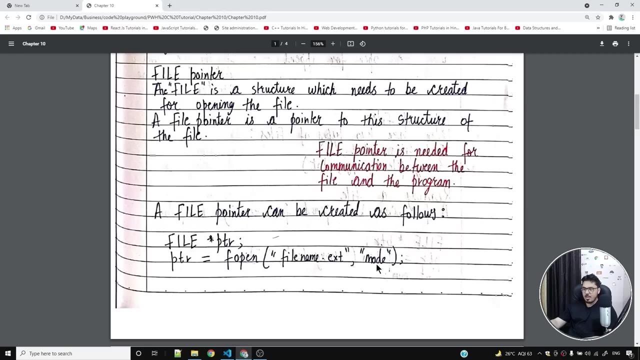 caps. i'm saying file star, ptr. now i'll say ptr is equal to f open. the first argument is the name of the file, which is sample filetxt, and the second argument is the mode. okay, so all i need to do is i need to give the mode here. so this is the mode, and mode is a string, so i'll use double quotes. 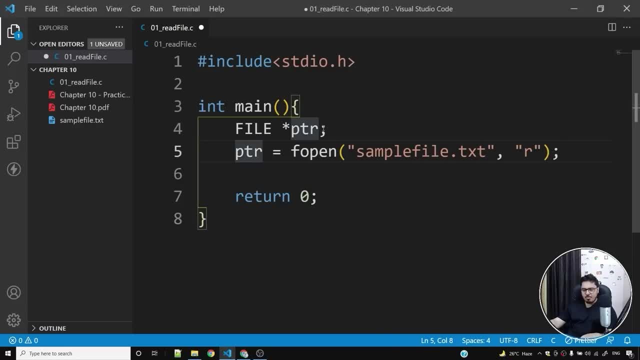 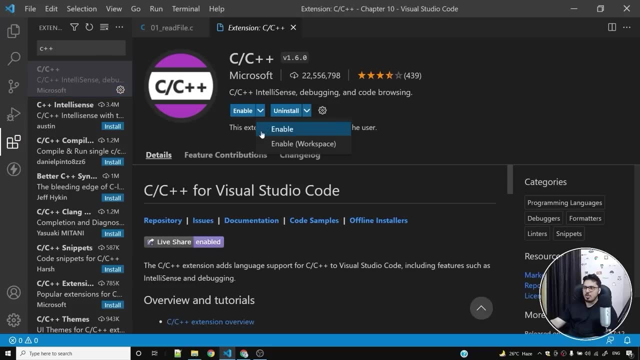 i'll give read mode. now let me show you that this program works. i'll save this program and i'll also have to enable c++ extension and also the code runner. so i'll enable these two things. i'll also enable code runner. so what i'll do. 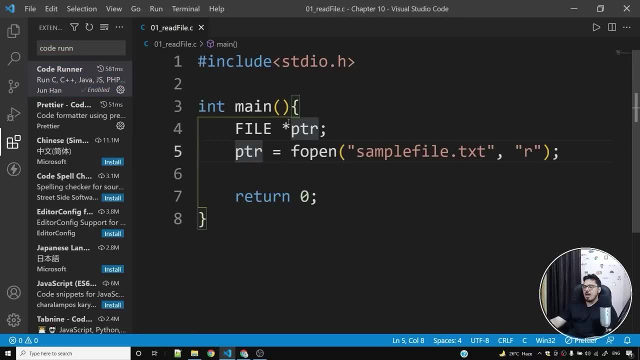 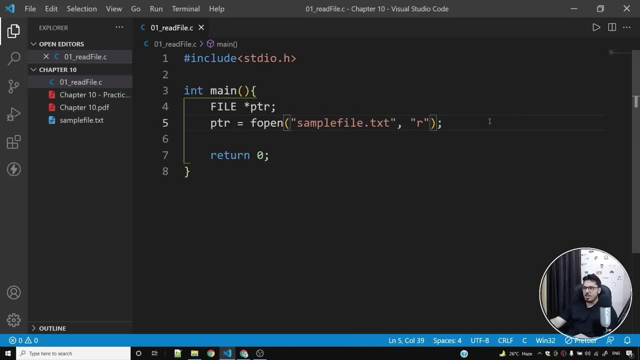 is, i'll enable it and what i'll do is i'll simply, you know, start with this. ptr is equal to f, open sample filetxt r. now let me show you that this program actually works. so i'll simply run this program and you can see that this program is not throwing any errors whatsoever, which means 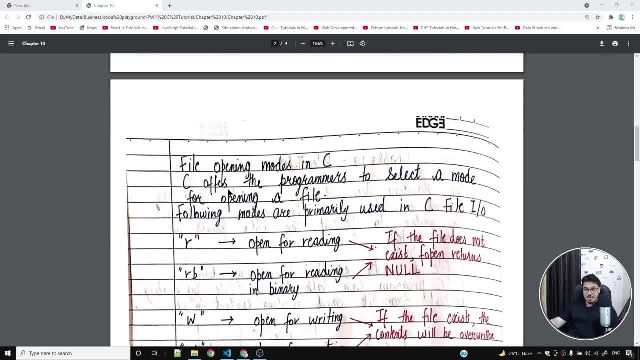 that this particular program works. now we'll see what are the file opening modes. in c we have already seen a read mode. i just showed you read mode. we can open our file in read mode. now let's see what are the other modes available, if you want to. 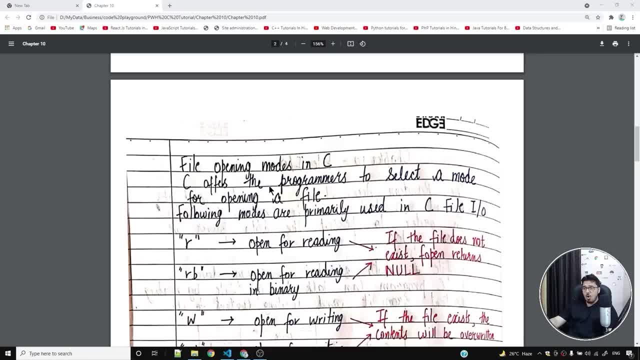 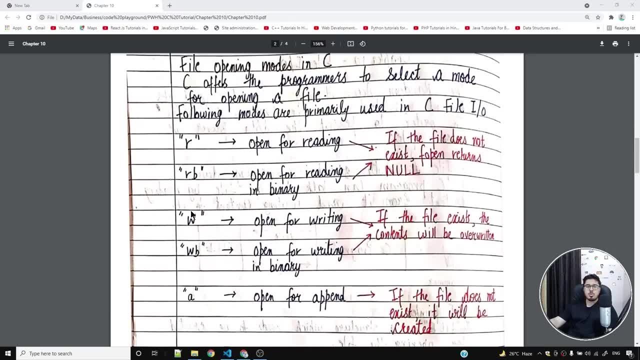 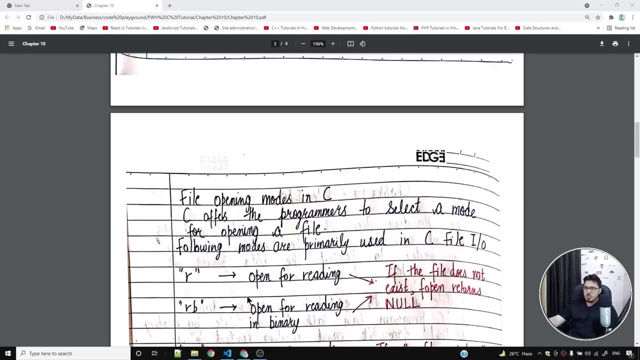 o, if you want to open a file in c. so c offers the programmers to select a mode for opening a file. so you can either open in read mode either. you can open and read binary mode. you can also open in write mode. you can also open in write binary mode. also, you can open an append mode. so let's see what. 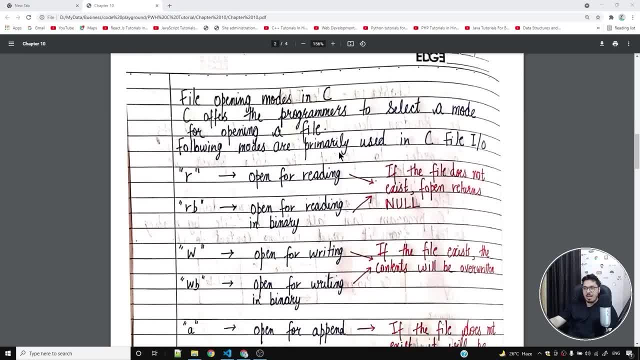 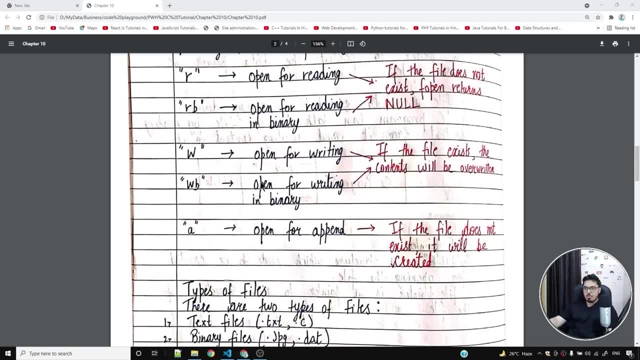 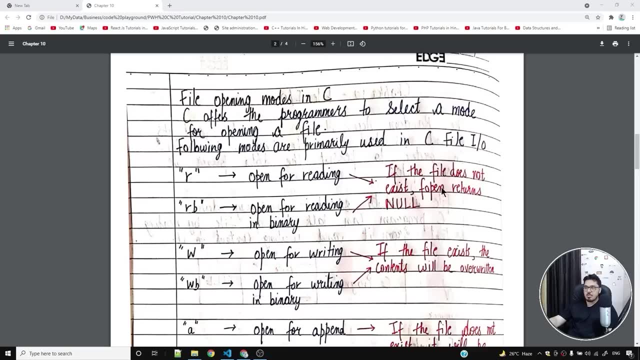 other modes available. following modes are primarily used in c file io. so r is open for reading. rb is for reading in binary. w is open for writing. wb is open for writing in binary a is open for append. now let me tell you something about read. if the file does not, does not exist. f open returns null. 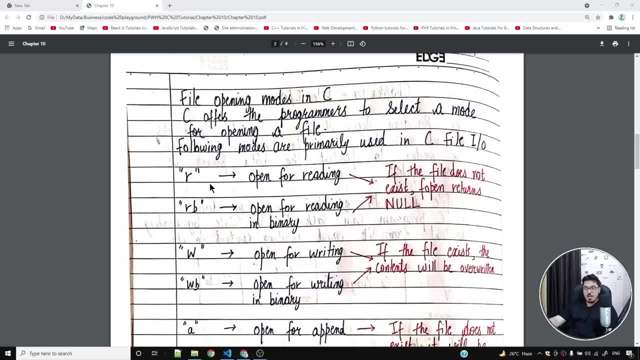 so if the file does not exist, you will get a null pointer, and you know what a null pointer is. null pointer means it is pointing to nothing, so null is a constant in c and if, if the pointer is null, it means that it is pointing to nothing. okay, so you can actually check if ptr is equal to equal. 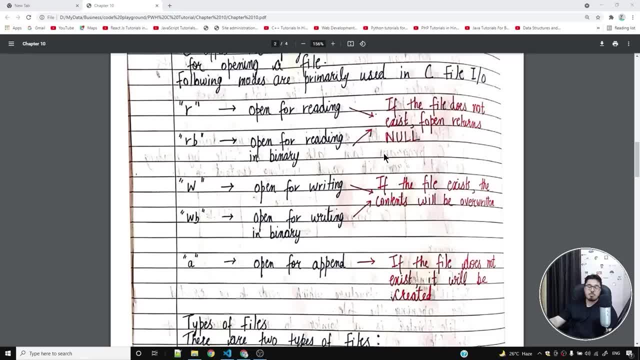 to null. you can perform these kind of checks to find whether a pointer is null or not. now let's talk about these open for writing, and open for writing in binary: if the file exists, the content will be overwritten. so this is something that you need to be very careful with. if you are 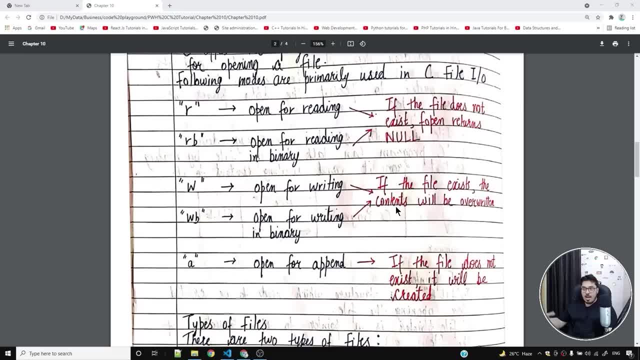 writing to a file and that file actually exists, that file will be overridden. so you should be very careful if you are dealing with files that you really care about. so let us say i write a program and i write a program to use write operation on sample file dot txt. 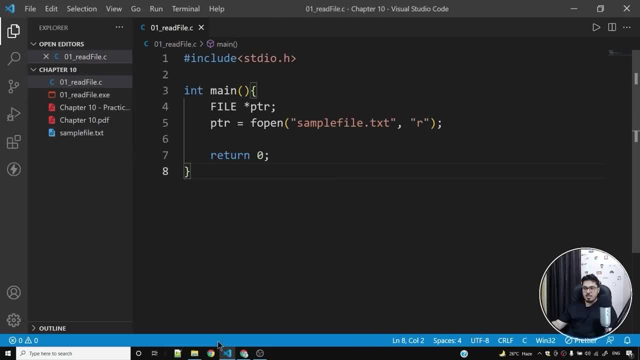 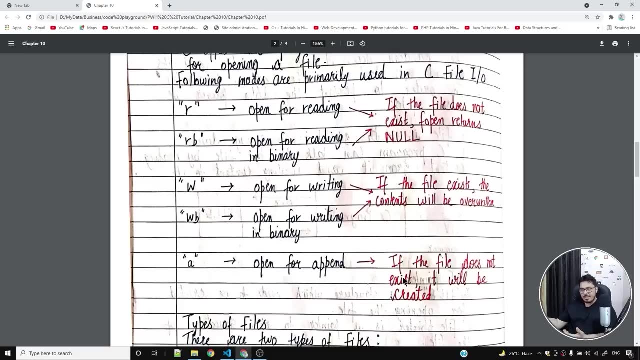 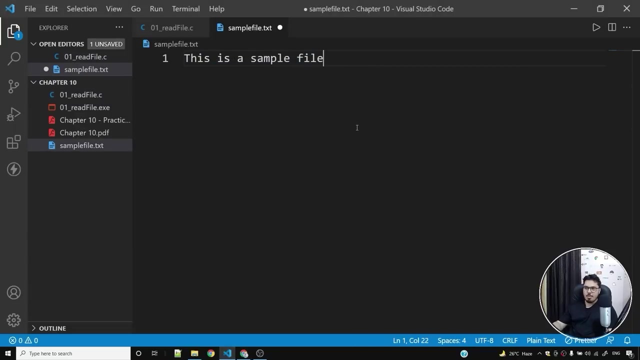 i might lose this content if i overwrite this file, so this is something that i need to keep in my mind. now let's talk about append. append simply means append characters at the end of the file. so let us say, i'm appending 3 to this particular file. i'll simply add 3 at the end. this is how. append. 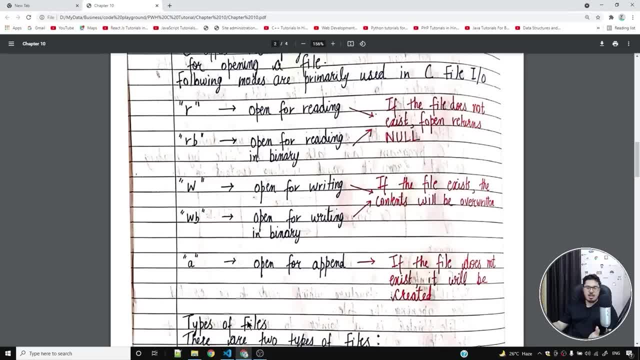 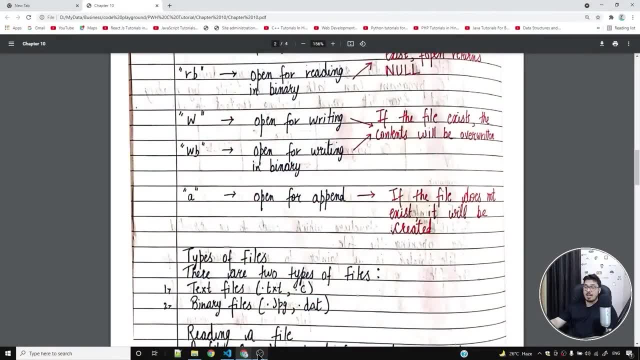 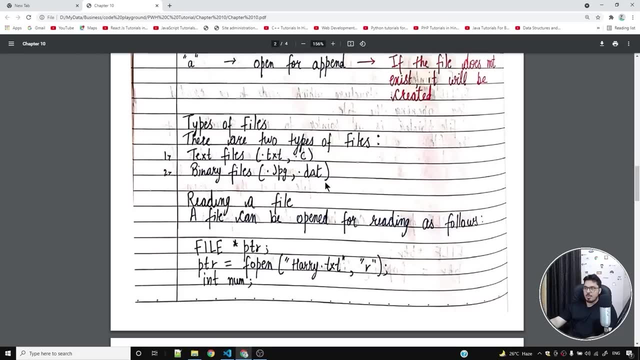 works okay, so append means adding content to the end of the file. if the file does not exist, it will be created. this is something that you need to keep in mind as well, because if the file does not exist in the append mode, the file will actually be created. okay, so i hope that this makes sense. 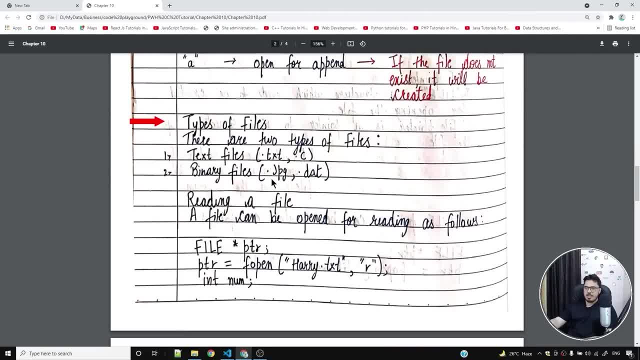 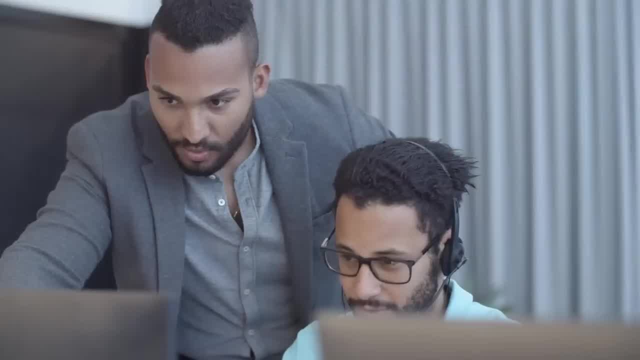 let's talk about types of files. primarily, there are two types of files: text files and binary files. text files are the ones which can be opened using notepad and the content of those files can be easily read by human. now binary file is a bit tricky. some examples of binary files: 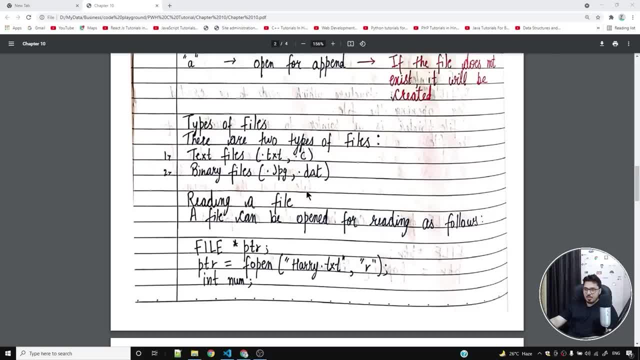 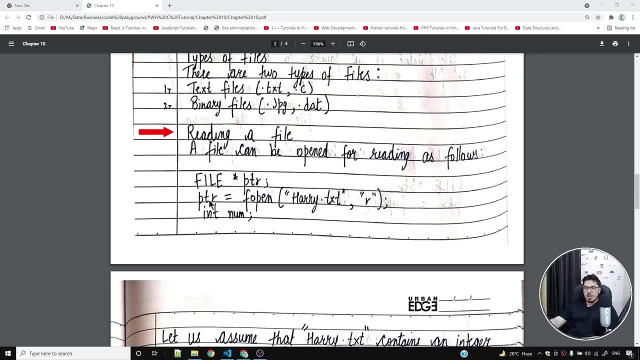 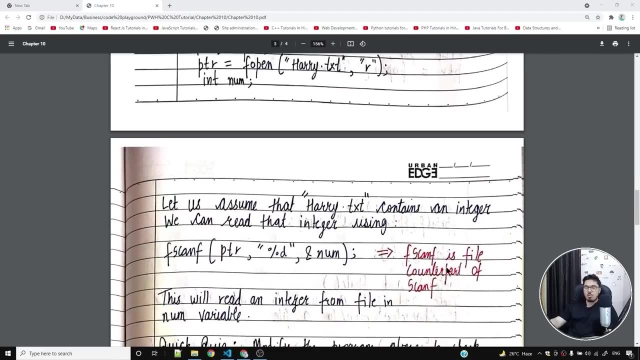 are dot, jpg, dot, dat. now let's talk about reading a file. how do we read a file? a file can be opened for reading as follows: you can create a pointer, you can say: ptr is equal to this thing, and you can actually use fscanf, which is a counterpart of scanf. you can use it to read. 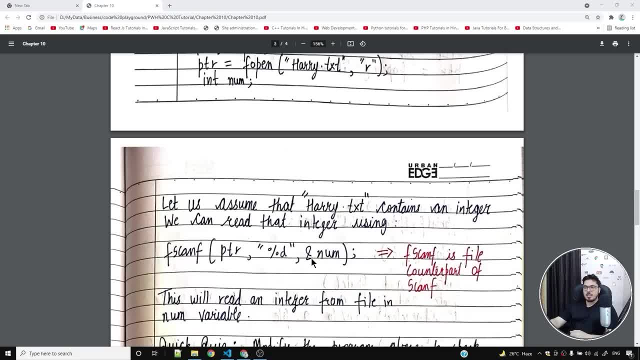 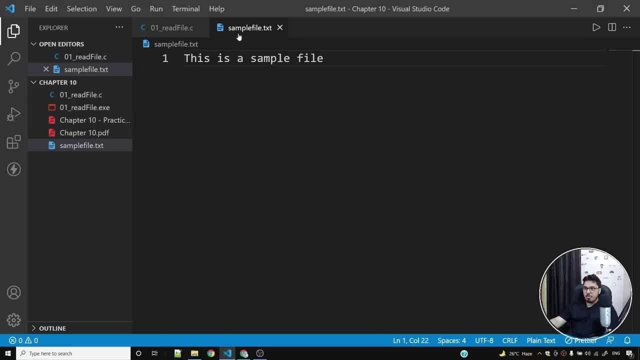 a character, or you can use it to read a, let us say, a floating point number, for that matter, or an integer, for that matter. let's read one character from this sample filetxt. so, in order to read a character, what i'll do is i'll create a character and i'll use fscanf. 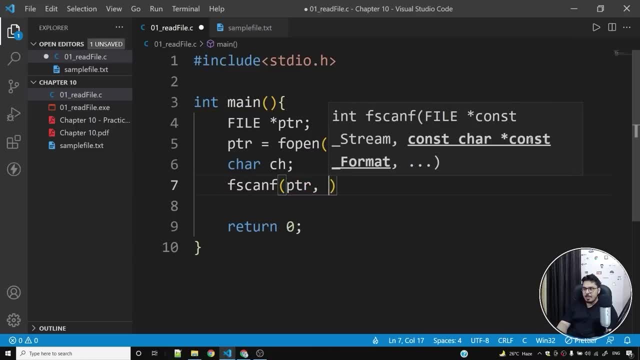 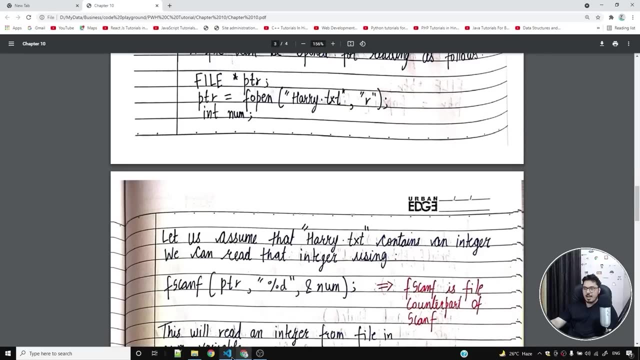 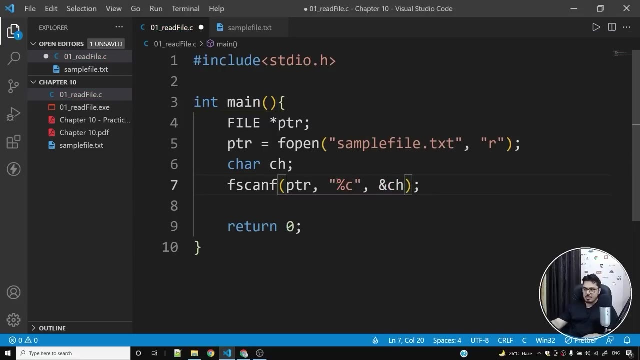 fscanf function. so what i'll do is i'll give this ptr. now, what i'll do is the first argument is the ptr, the second argument is the format specifier and third argument is the address of the character. so i'll say ampersand ch. now, what is the format specified? it's percentage c, because i'm dealing 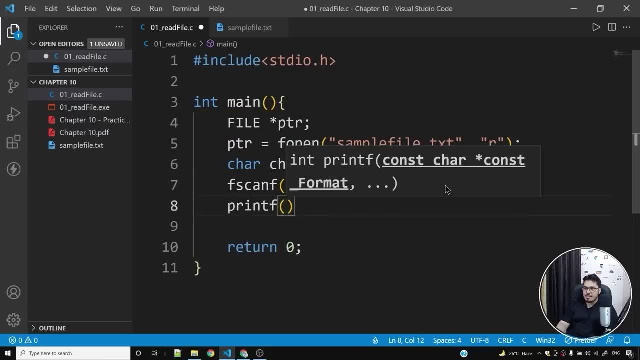 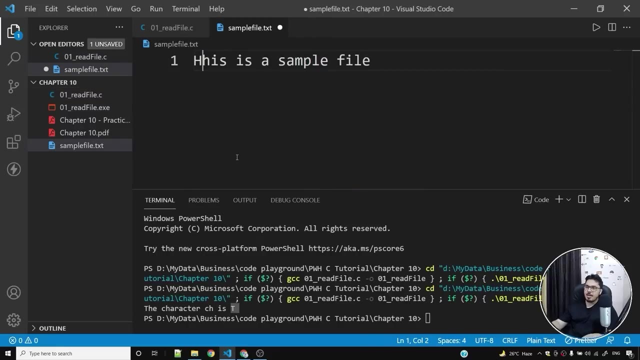 with characters. now what i'll do is, if i print this character ch, i'll say the character ch is percentage c, and if i try to print ch, you'll see that first character has been read from the file. so the first character was t. let us make it h. 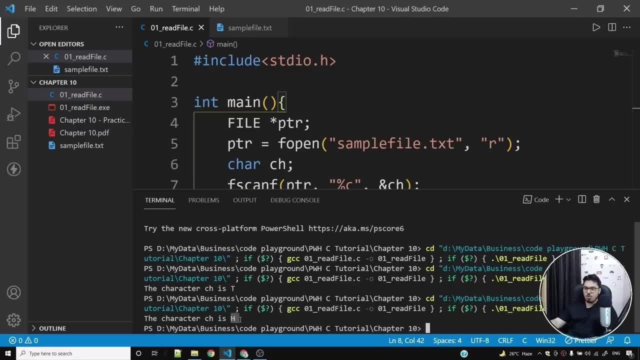 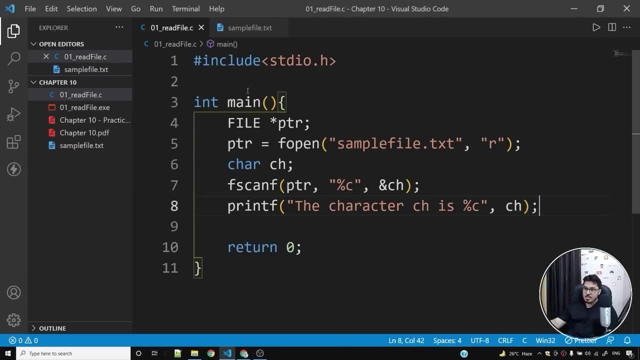 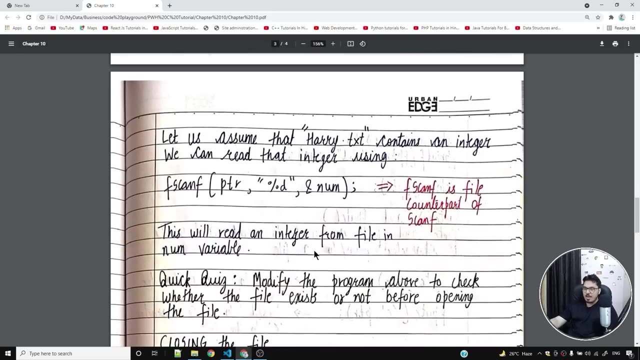 and let's see if the program is able to read h from this particular file. yes, this program is able to read one character from this file. i can actually loop through this and read all the characters, but we are going to talk about that later and now what i'll do is, at this point, i 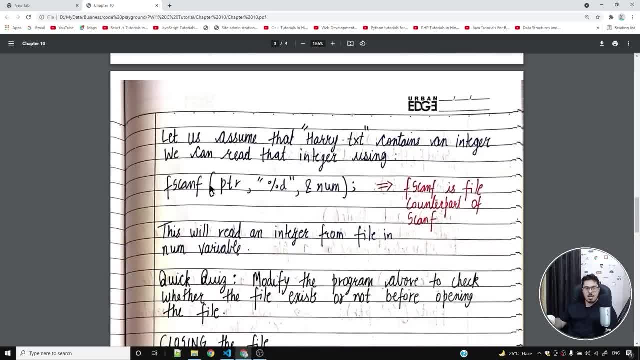 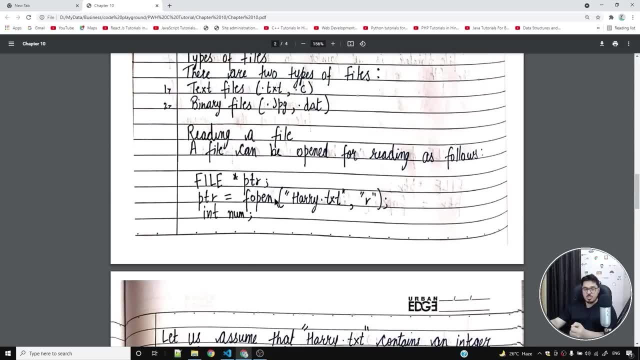 just want you to make sure that you understand how fscanf works. and let us assume that harrytxt contains an integer. you could have used int num and you could have read an integer as well, but in this case my file contained a character, so i read this character. now i can also read an integer. 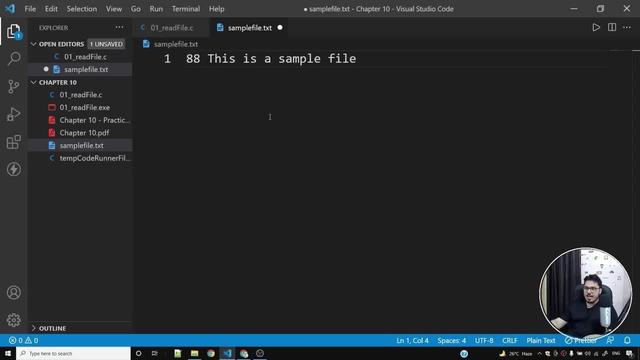 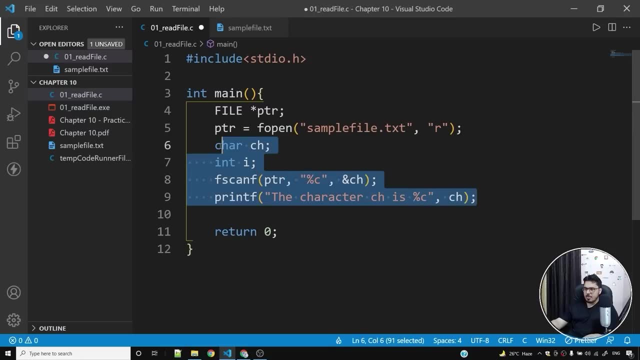 from here. so let us say i have an integer 88 and i'm adding a space. i can do something like this. i can say int i and instead of doing all this, instead of doing all this, what i'll do is i'll do int i and then i'll say fscanf, ptr, and instead of doing 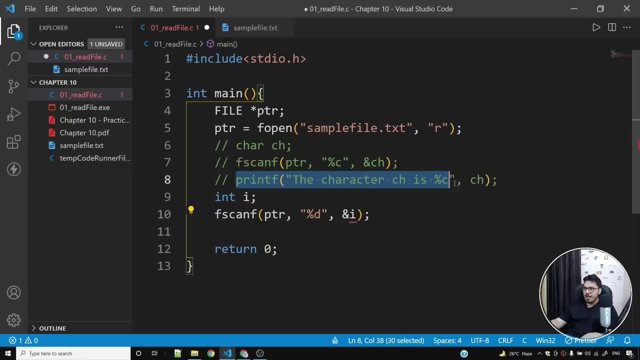 c, i'll do d and i'm percent i and i'll say: the value of i is. i'll say the value of i is what is the value of i, percentage d, i. so i'll say percentage d and i'll say i, and this will give me 88. so you can see that i can read an integer from a file as well. 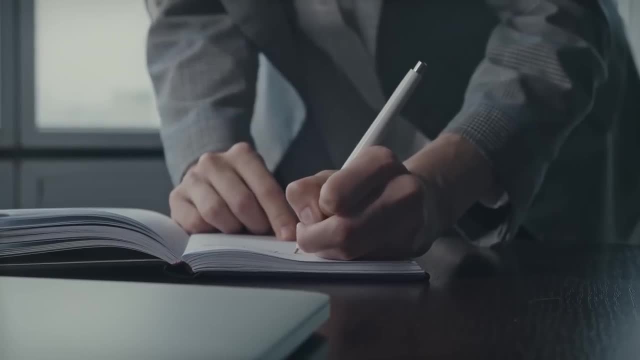 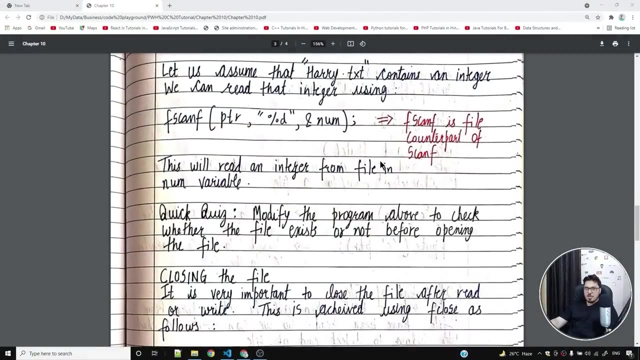 using this syntax now. i have made these notes very carefully so you can always download these notes for yourself. i've also made some comments about fscanf and other concepts that we are discussing in this chapter. now. this will read an integer from the file in num variable. in this case, it will read: 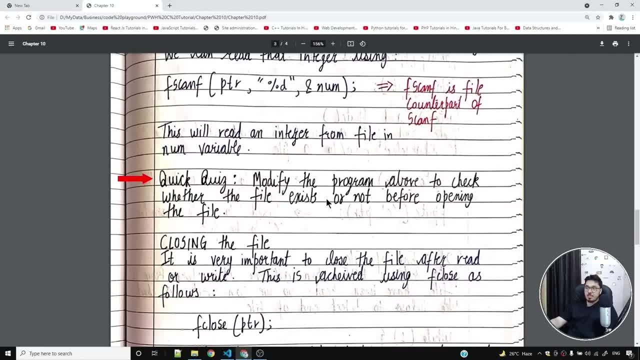 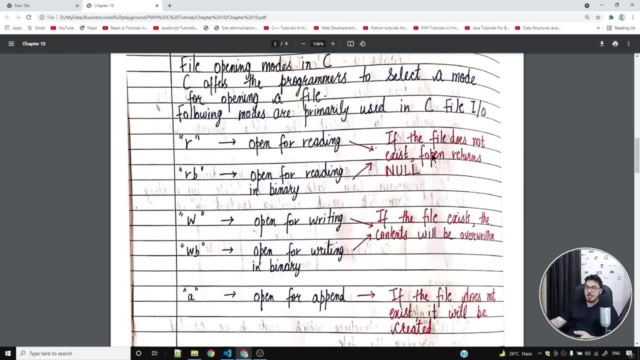 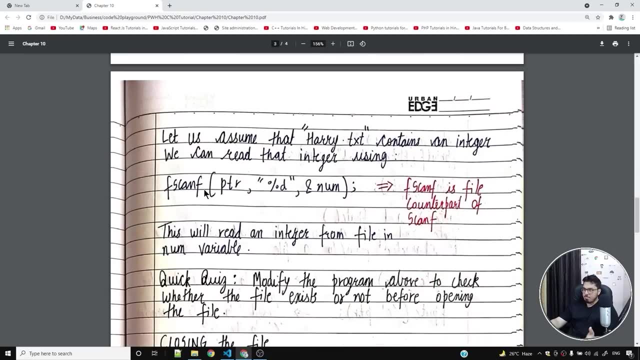 it in the i variable. okay, now, coming back to the nodes, quick quiz: modify the program above to check whether the file exists or not before opening the file. and how? how would you do that? you will simply check whether the pointer is null or not, because if the file does not exist, f open returns null. so 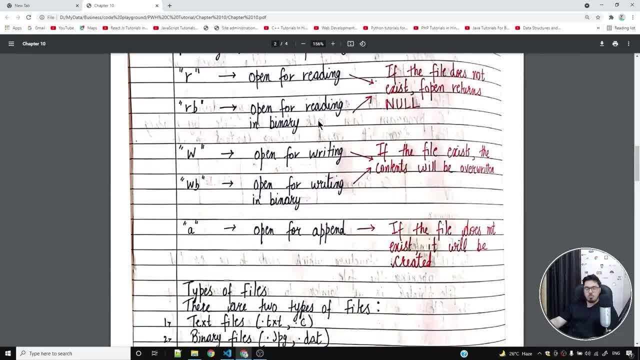 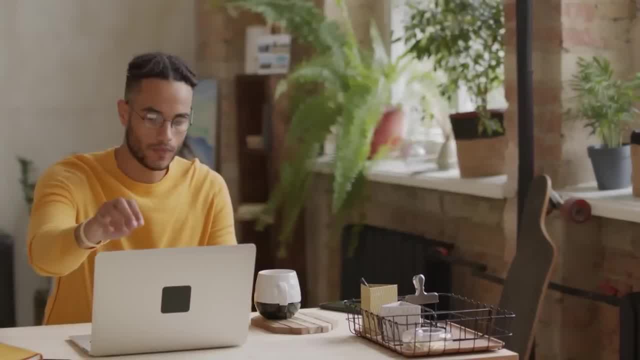 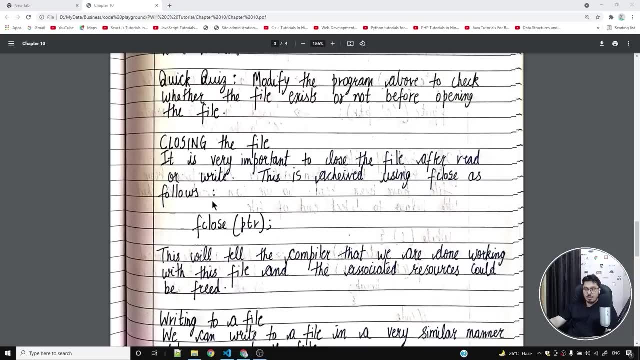 this thing is null or not. if your pointer is null, this means that the file does not exist. let's talk about closing the file. it's very important to close the file after read or write. this is achieved using app close as follows: so whenever you are reading a file and you're 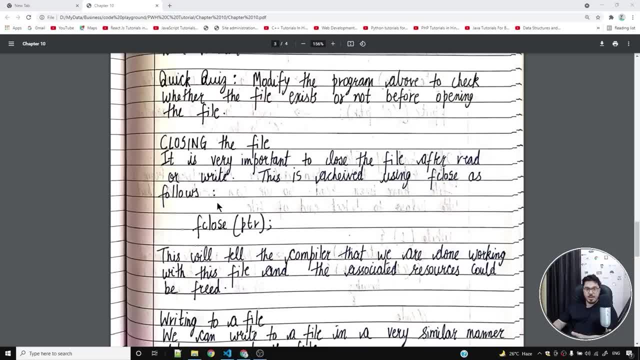 pointing a pointer to a file. after you are done reading or writing from the file, all you need to do is you need to run this app close, because you are actually holding that file resource and it is not a good idea to hold a file resource into a pointer forever. you need to free it as soon as. 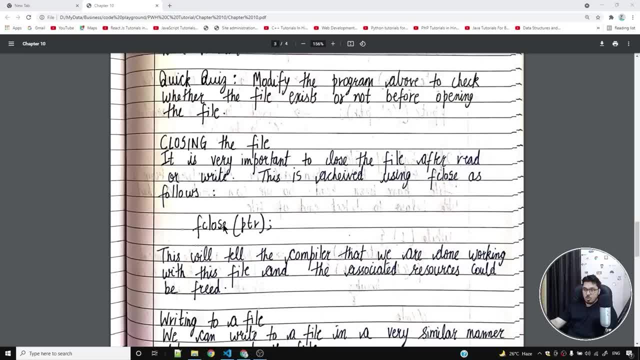 possible and we use app close ptr to tell the operating system that i am done with this file. i no longer need this file. this file is no longer opened in this program and this will actually make the file available for other programs. this will tell the compiler that we are done working. 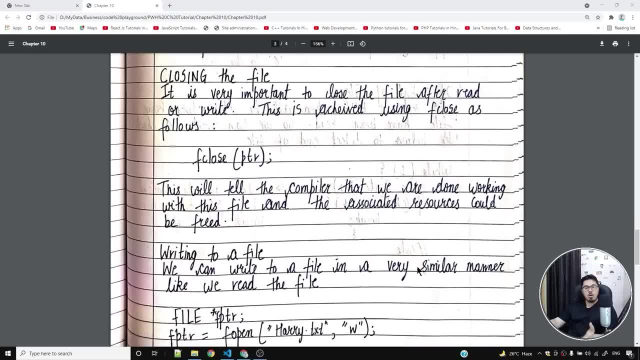 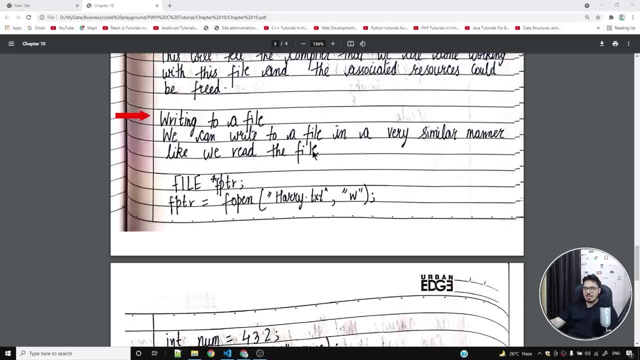 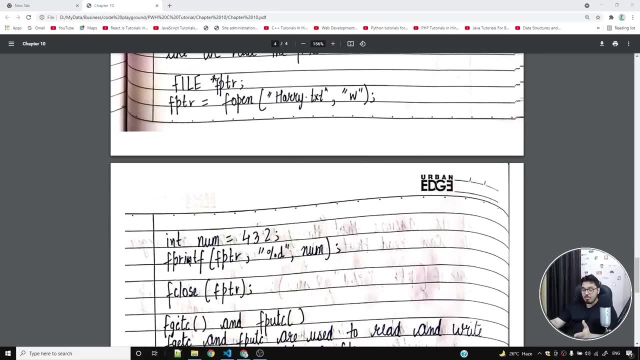 with the file and the associated resource, it could now be freed. okay, now let's talk about writing to a file. we can write to a file in a very similar manner like we read the file. you can do something like file star, f, ptr. you can write to a file and in order to write to a, 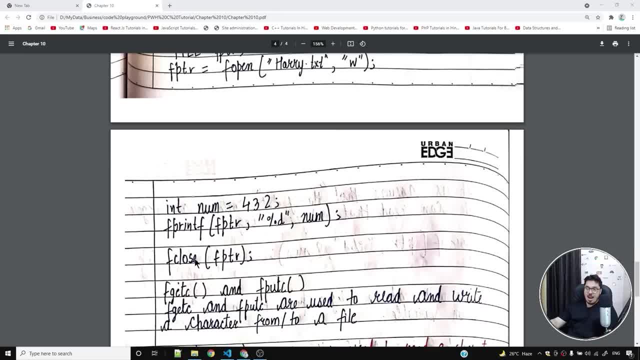 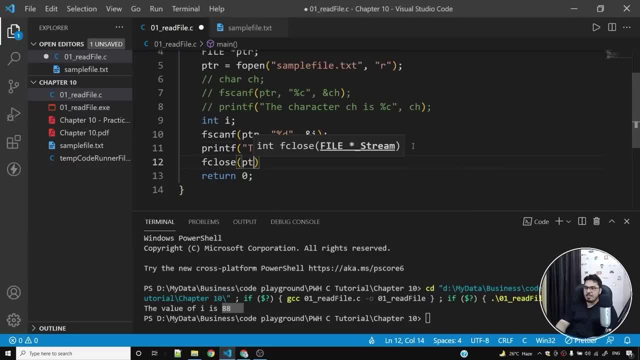 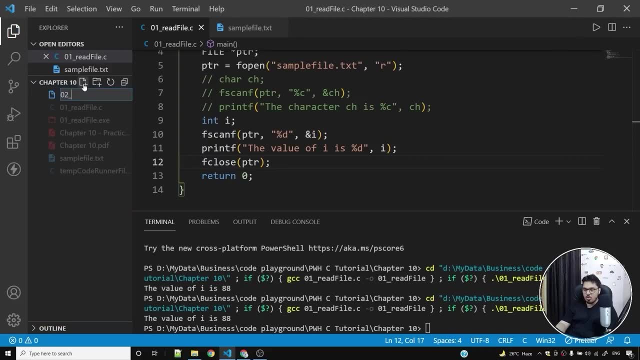 file. you can use f printf instead of f scanf and make sure that you use f close. in this case also, i'll use f close, so i'll say f close and then i'll give the ptr and this program will also work fine. but let's try to write to a file, so i'll say zero, two. 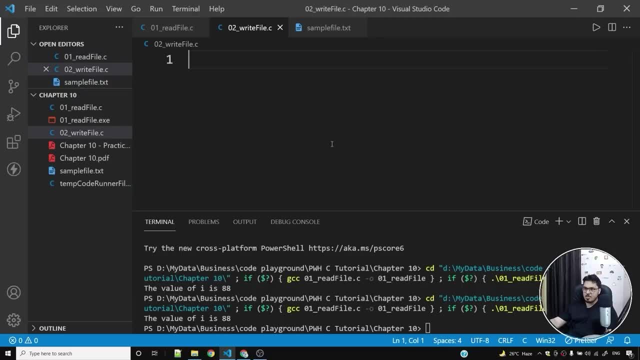 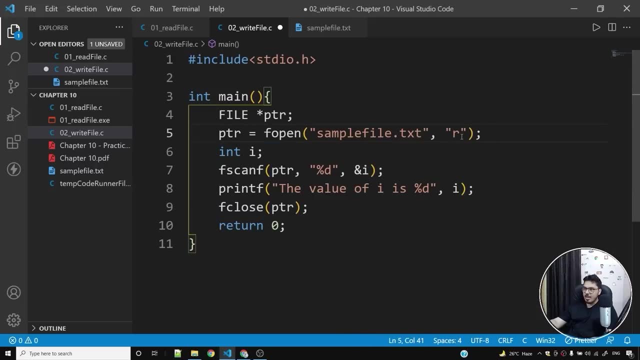 underscore: write file dot c. this program will actually write to a file. so what i'll do is i'll create a new file and what i'll do is i'll open it in the write mode. so i'll say: write file. okay, write file dot. txt is the name of my file, and i'll say int i is equal to 89 and i'll 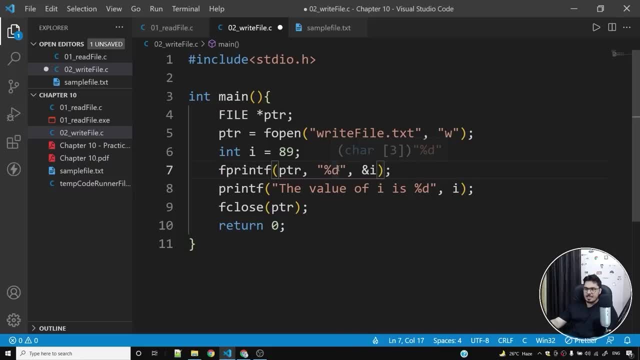 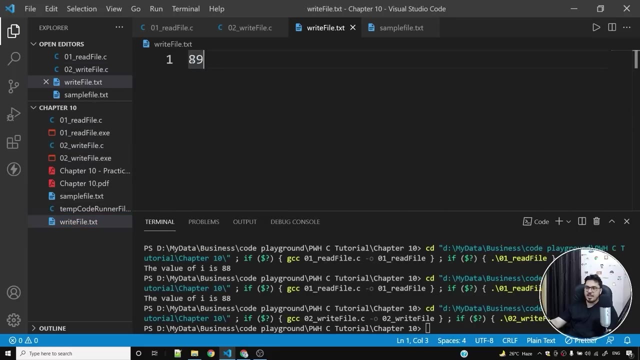 say f printf and i'll say ptr and i'll simply add i to this, to this file, and let me get rid of this. and we run this program and you can see that write file dot txt has been created in 89 is now part of this file, which means that we were able. 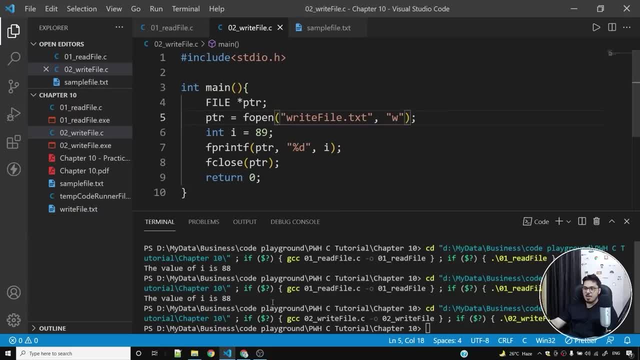 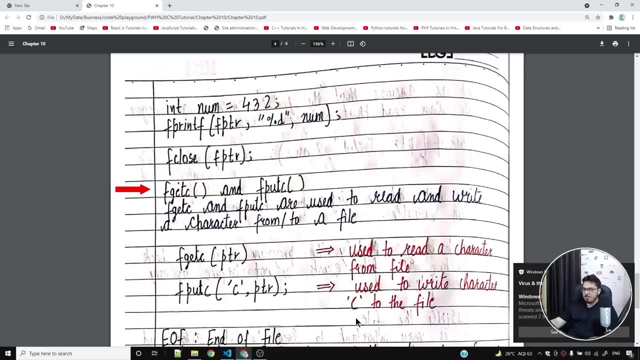 to successfully write to this file using f printf. so this is how you write to a file. now let's talk about two more functions, which are f get c and f put c. these two functions are very similar to f scanf and f printf: f get c and f put c. 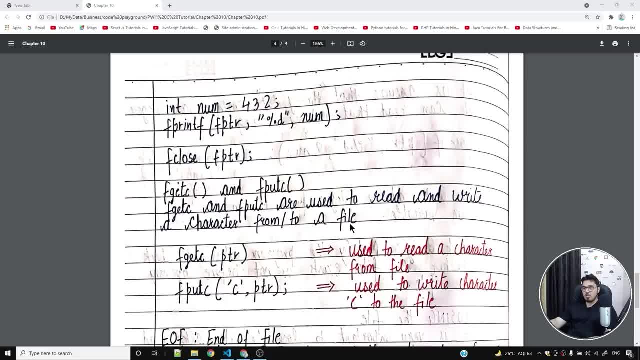 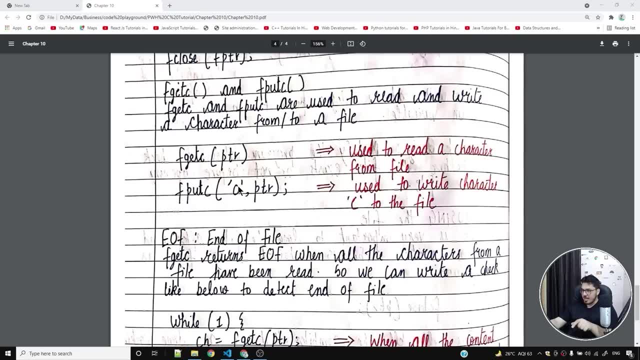 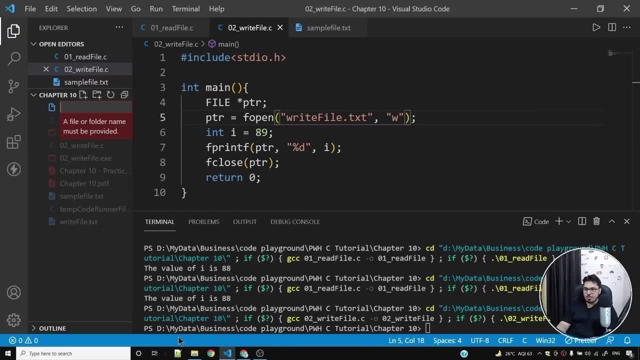 are used to read and write a character from or to a file. now if you do f get c, ptr, this can be used to read a character from file and if you do f put c, a character in ptr used to write character c to the file. let's see the demo of f get c and f put c. so this is program number three and i'll say: 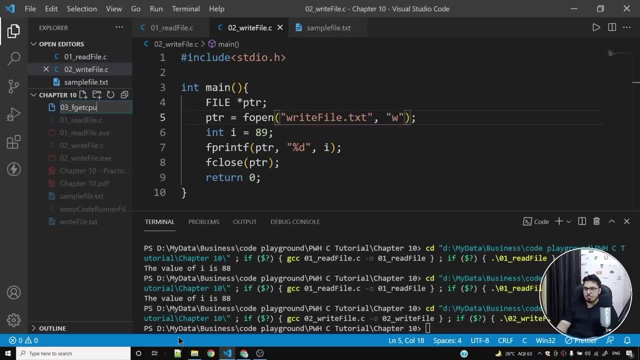 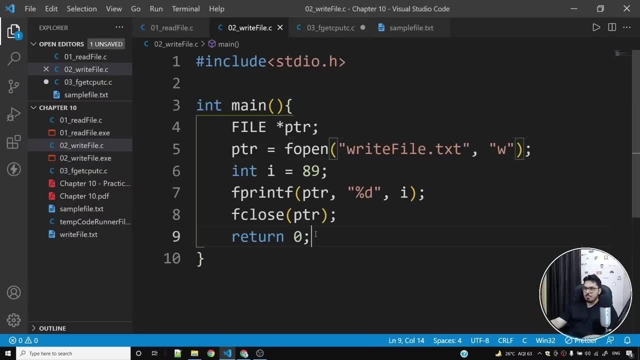 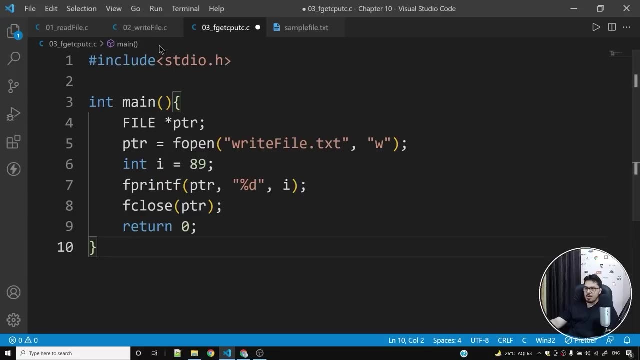 zero, three underscore: f get c, put c dot c. i'll put the boilerplate code if i want to add a character to this file and i'll add something else. let's say i'm going to use the, so it's gonna be f get c, but c dot dxt. i'm going to add this character and i'll do something. 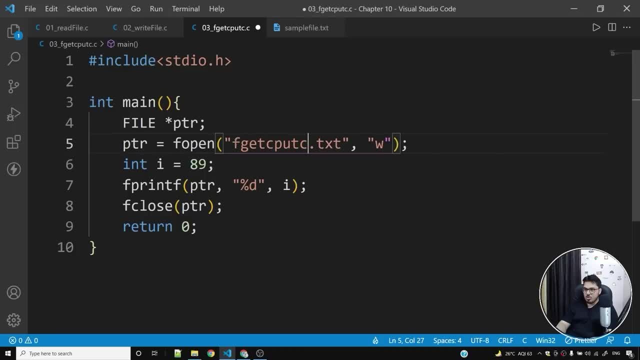 like this. so i'll get rid of this and what i'll do is i'll simply paste all the content of this particular file to to this file. i'll open: f get c. f get c, put c, dot txt. i'll open it in write mode and i'll demonstrate: f put c. so i'll say: 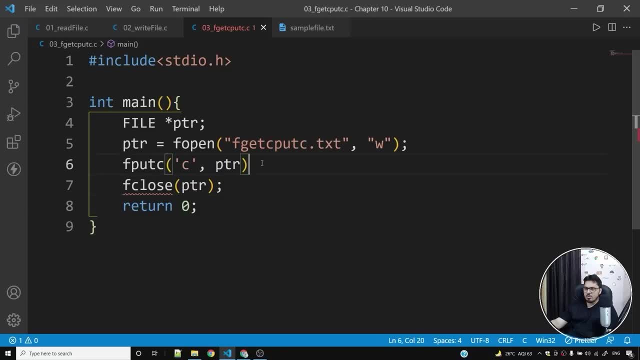 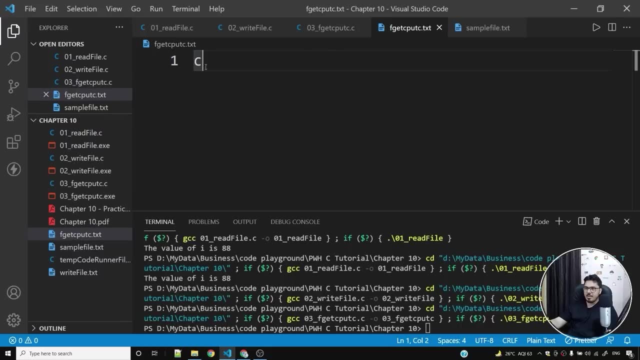 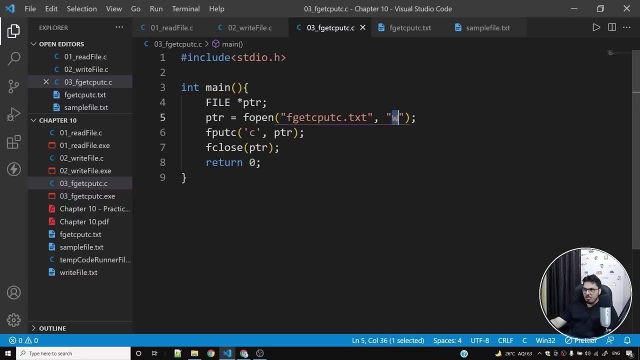 this int i is equal to this thing. i'll also put a semicolon here and save it. so if i run this program, you'll see that f put c dot txt has been created and this character has been written to this file. okay, you can do the same thing for f- get c as well. so now, if i want to read this file, 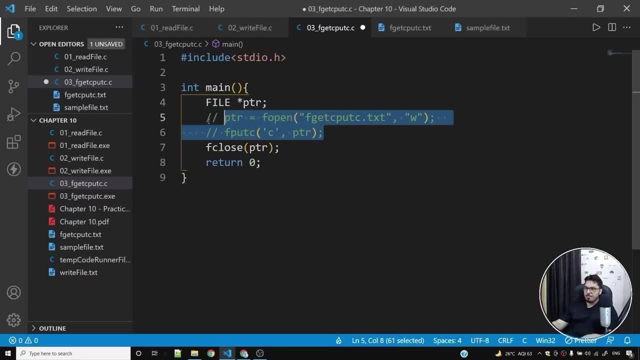 i can actually do something like this. let me get rid of this and let me replicate it. instead of opening it in the write mode, i'll this time open it in read mode and i'll say: f get c ptr, f get c ptr. and i'll do something like this and i can print this character. i can say printf. 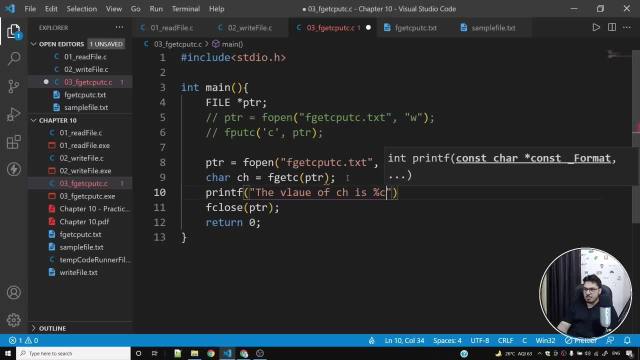 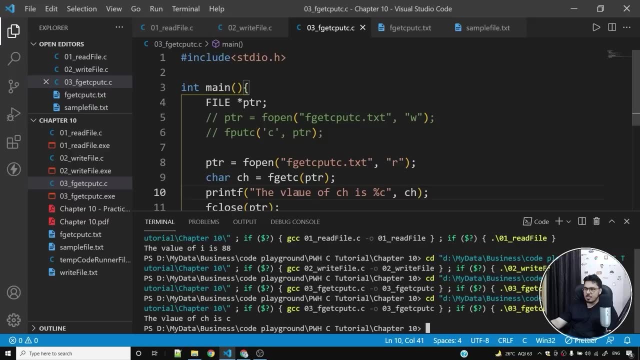 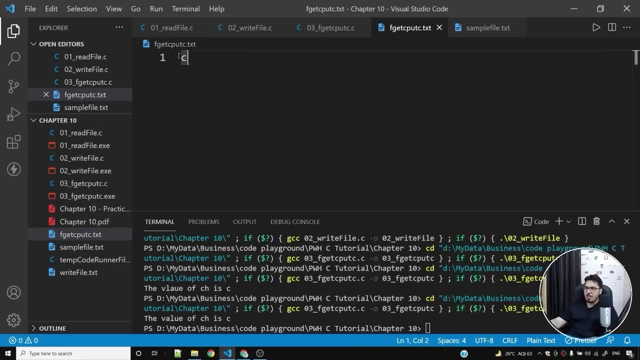 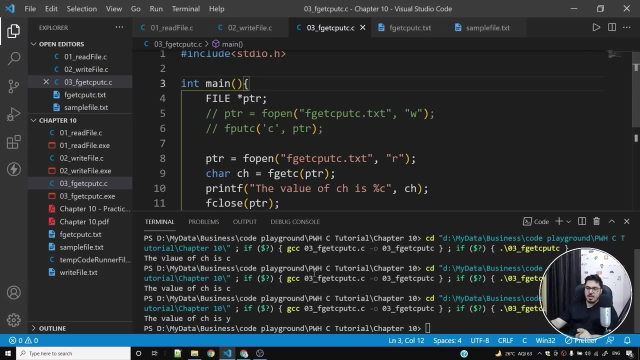 the value of chs, percentage c, ch. and this will, if i, if i run this, the value of c is- let me spell value correctly- the value of ch is c. now what if i make this character yyddlkm? this will show me why this will read one character. now, if i do this thing once again, 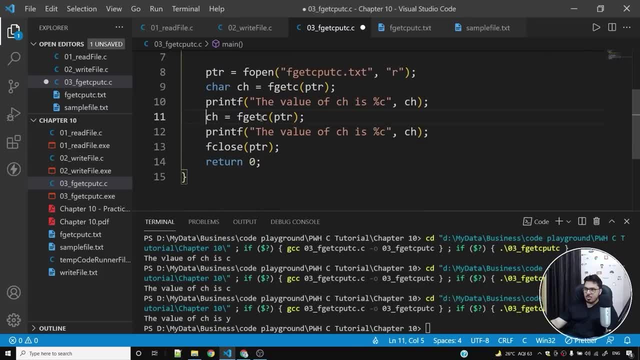 if i, if i do something like this: ch is equal to f, get c ptr and i run this again, what will happen is two characters will be read. so the value of ch is y, then again y. if i keep on repeating this, what will happen is it will keep on reading further characters from the file, so y. 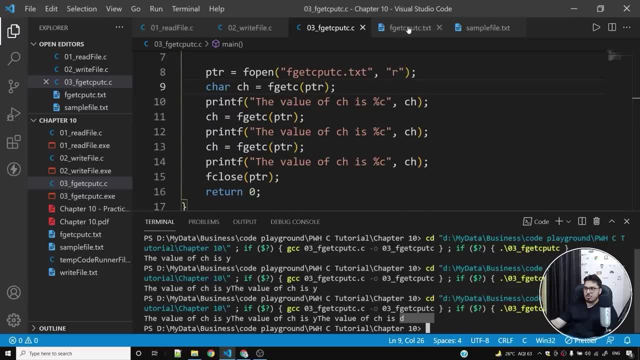 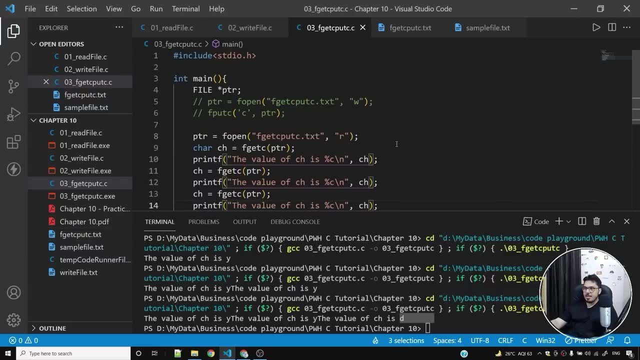 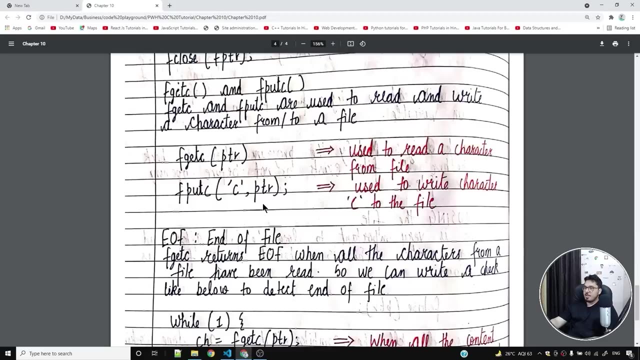 why. first one was y, the second one was y, third one was d. as you can see in this file now, it's always a good idea to put a backslash and for better readability. if i run this program now, it is a bit readable, a bit more readable than the previous one. so this is how f get c and f. 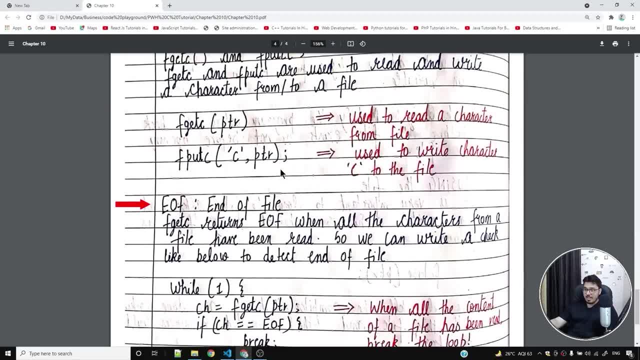 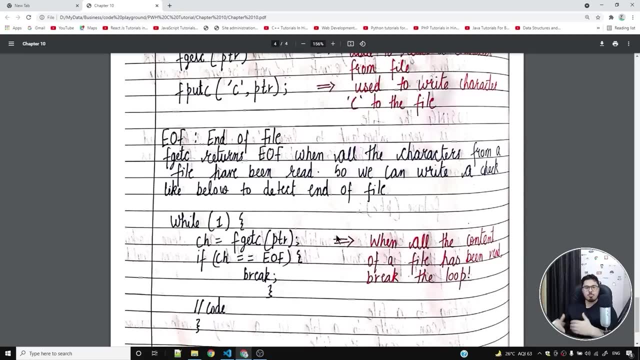 put c works. let's talk about end of file character. now f gets the return cof when all the characters from a file have been read, so we can write a check like below to detect end of the file. so what happens is when you are reading, using f, get c, you will keep on getting the character from the 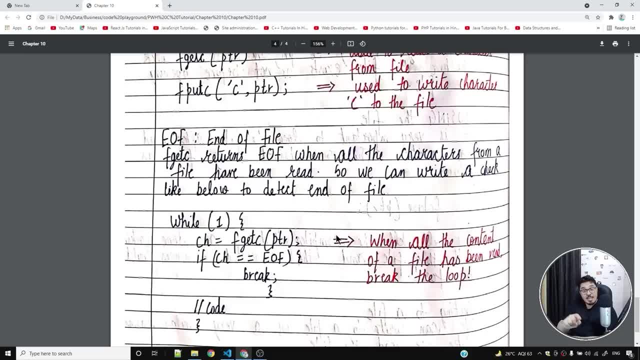 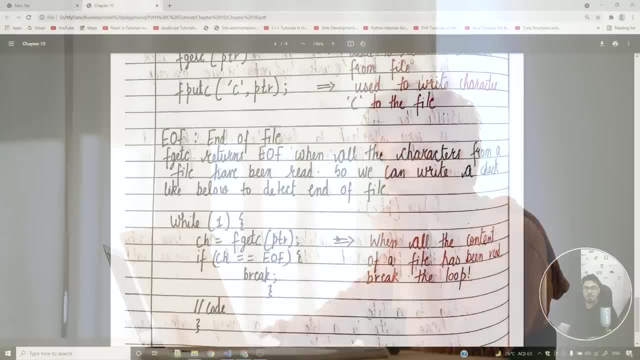 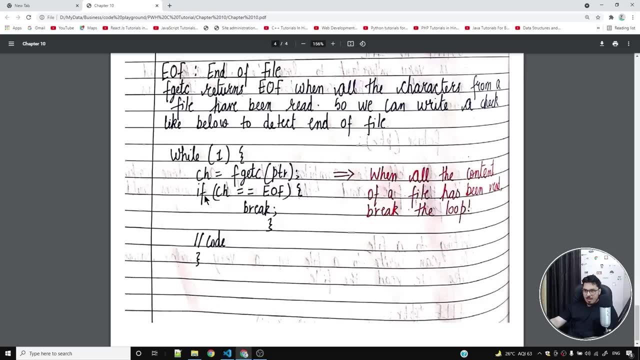 file until eof is encountered. and when eof is encountered, it means that there is no further content in the file and you can stop your program there. so what we can do is we can say while one and we can keep on reading from this file and we can put a check if ch is. 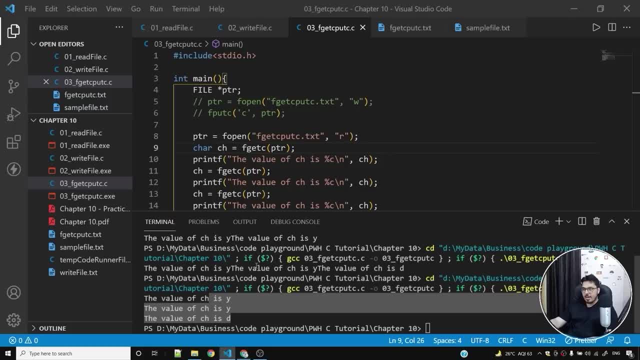 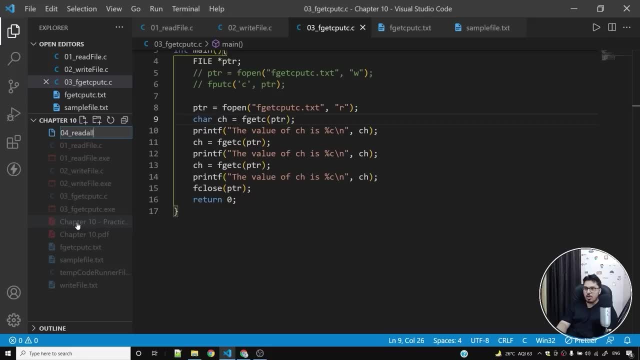 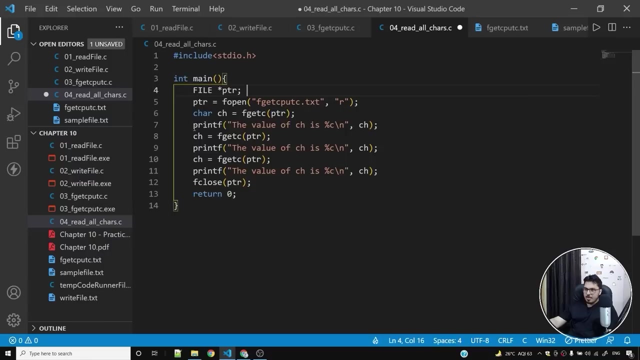 equal to eof, then break. okay, so so i can write a program like this. so let me let me read fourth program, zero, four underscore. read all characters, dot, c, and let me put some underscores here for better readability, and let me copy this program. so what i was doing here was i was repeatedly 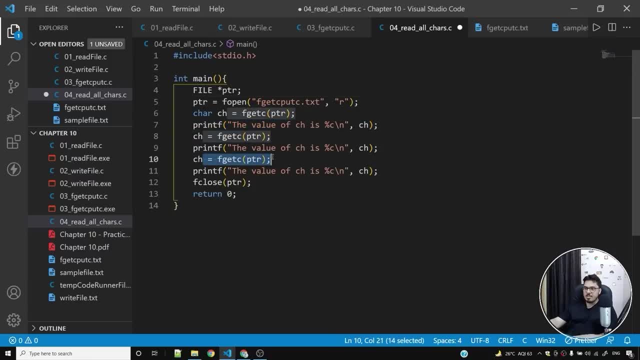 saying: ch is equal to f, get c pdr. ch is equal to f, get c pdr. instead of doing this repeatedly, what i'll do is: um, let me do something like this: care ch. and so what i'll do is: i'll create a loop for this one. so, instead of repeatedly doing this, i'll create a while loop. i'll say while. 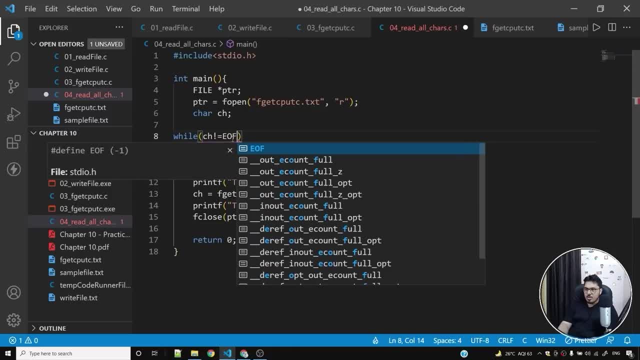 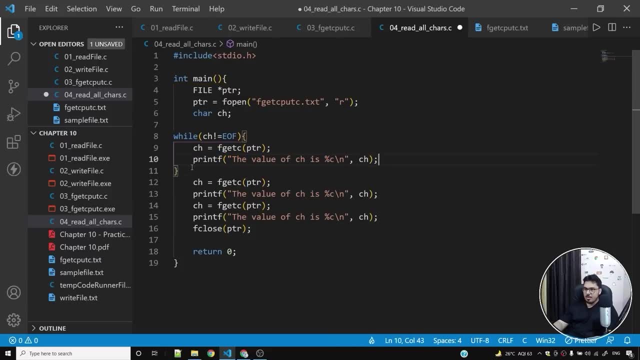 while ch is not equal to eof, so while end of file character is not in counter, do this and that's about it. the moment end of file character is encountered, what will happen is i will stop reading from the file. so let me run this program for you and you can see all the 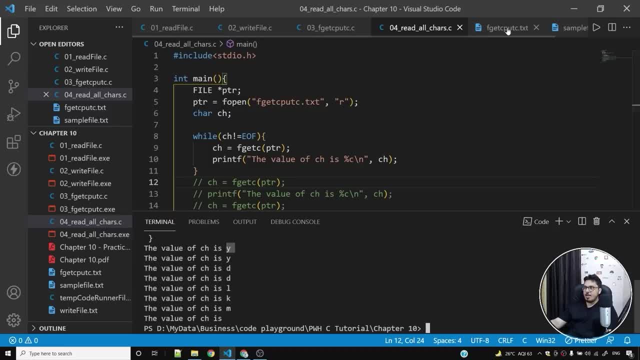 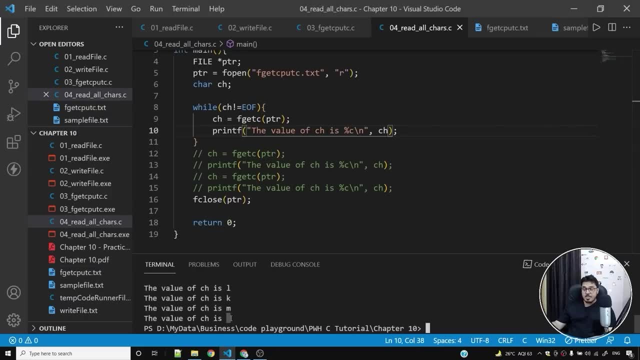 uh, you know, characters from the file have been read. so if i show you this file, the last character is m and this one is uf character. okay, now, this is printing this extra character because this extra character is eof. so if you want to get rid of this eof, all you all you need to do is 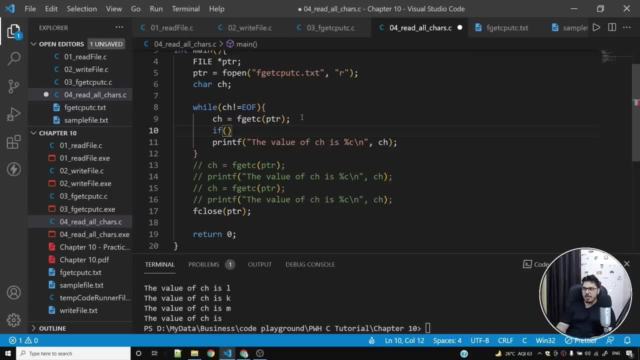 you need to print only when the character is not eos. so i can put a check here: if this ch is not equal to eof, all you need to do is you need to print this. okay, so i i no longer need curly braces, because this is just one line. so this is something that you can remember, but 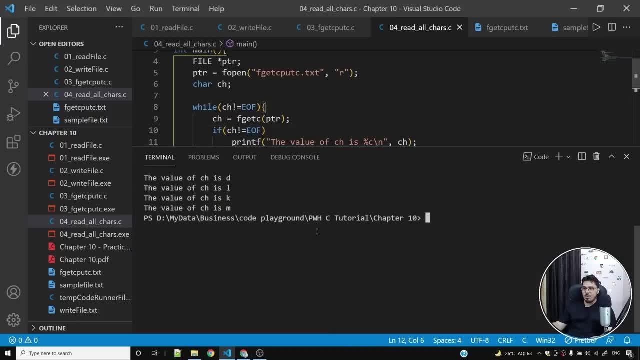 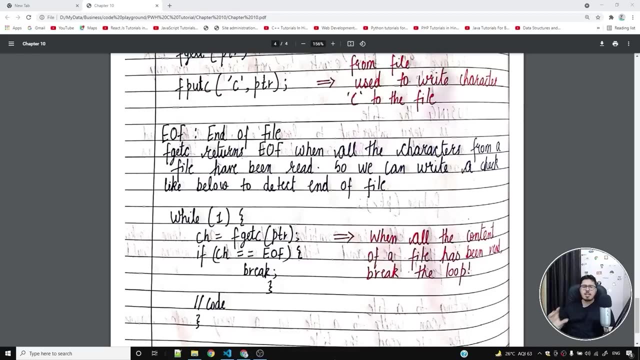 run this program, you can see it's sprinting, starting from, starting from y, all the way to them. okay, so all the characters from this file. so this is how you can read all the characters from a given file in c language. so when all the content of a file has been read, break the loop. so this is another implementation of the same thing. you can either use the z Aí dä Cstrá to call something else like this. you can either use this- that's an example of an example- ール to call a file using something else i don't remember. if you don't remember, the всехari. 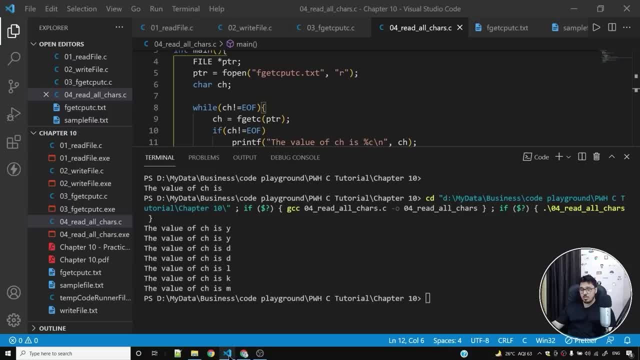 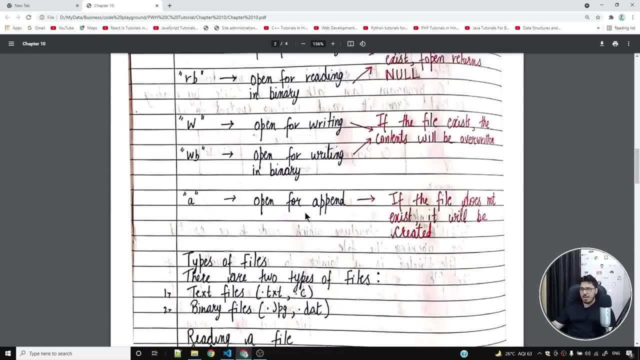 do another example of another file. so this is another. content of a file has been read. break the loop, so you can either use this implementation or you can go for this one. both of the things will get the job done for you. so with this we will conclude file io in c. i hope that these notes will be. 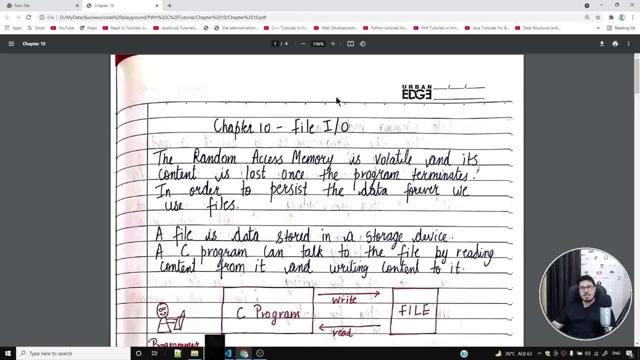 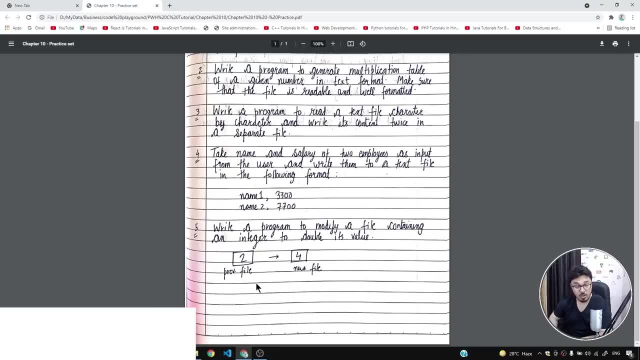 helpful for you also. let's move on to chapter 10 practice set to solve some more problems on file io. let's move on to chapter 10 practice set now. so, now that we have learned so much about file io, let's solve this practice set and let's see what this practice set has to offer. the question: 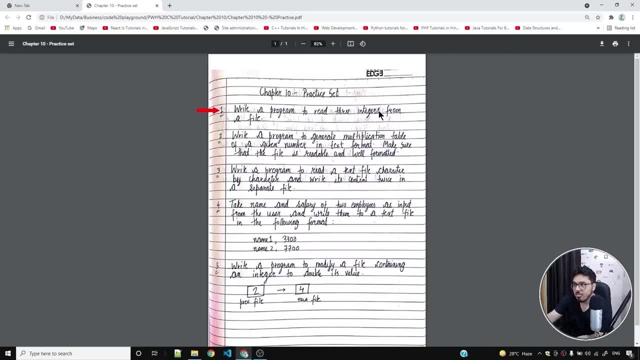 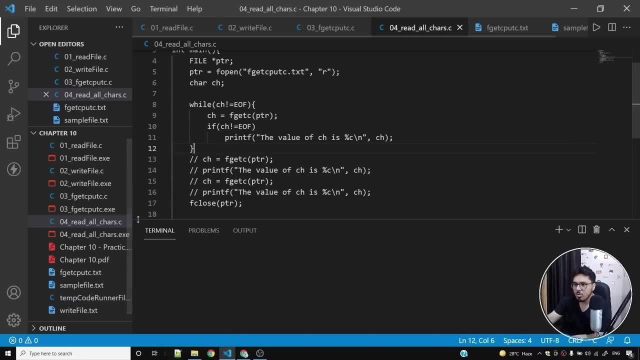 number one of this practice set says: write a program to read three integers from a file. so we have a file, we have three integers and we have to read those three integers from the file. so what i'll do is i'll open my visual studio code and i'll create a new file. i'll say 0- 5. 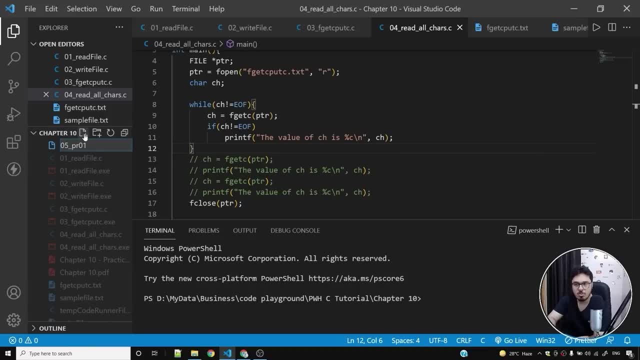 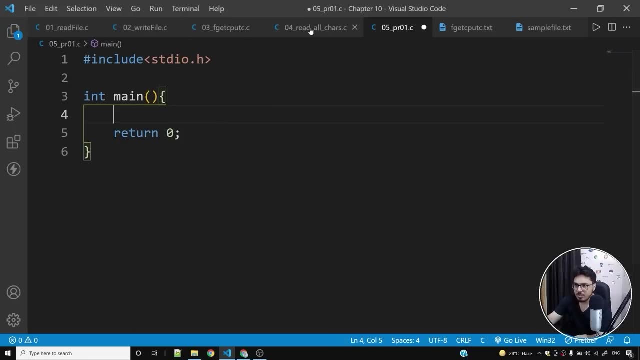 underscore: pr: 0: 1. since this is the first question of a practice set, i'll create this file as well as i'll put in the boilerplate code. i'll also use some of the other files which i've created here to read the integer, so i can use. 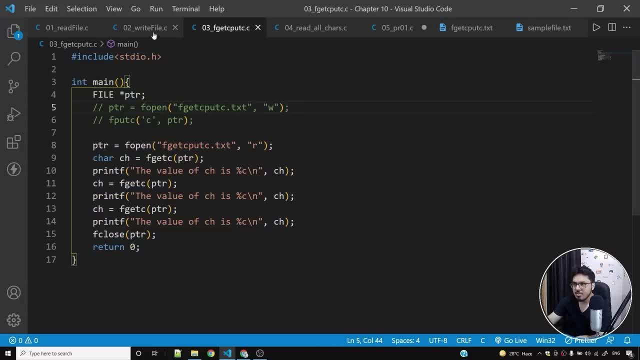 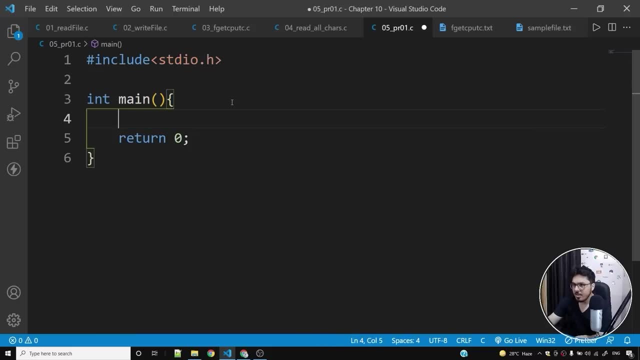 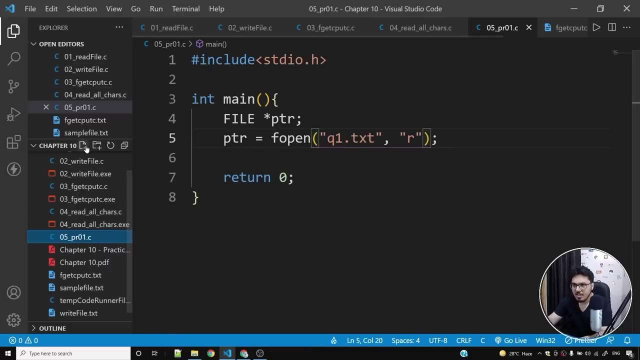 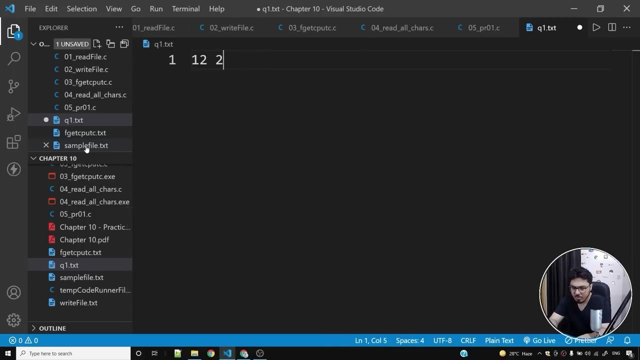 you fscanf, percentage d. and in order to use fscanf, i'll make use of this read file program. so i'll simply create a file pointer to read a string from a file. so let's say q1 is the name of the file. let me create this q1.txt so that we can have three integers inside this. so let me say 12, 24. 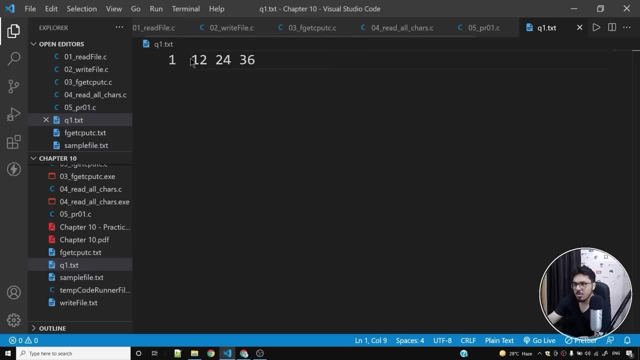 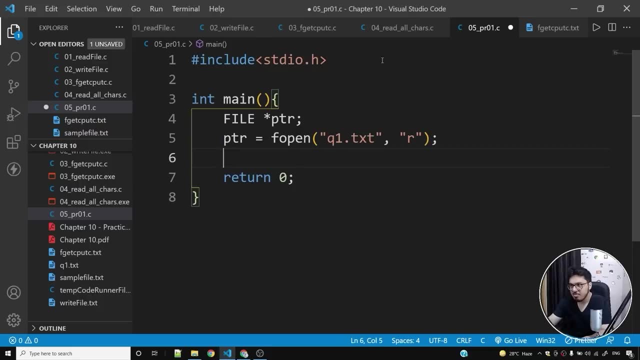 and 36, so we'll remember what integers are there now: 12, 24, 36. let me close this file and what i'll do is i'll keep on reading an integer using fscanf from this file. how do we do that? we have already seen that we can use fscanf like this and i can. 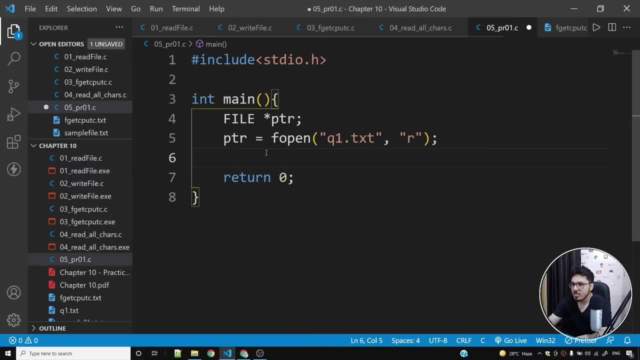 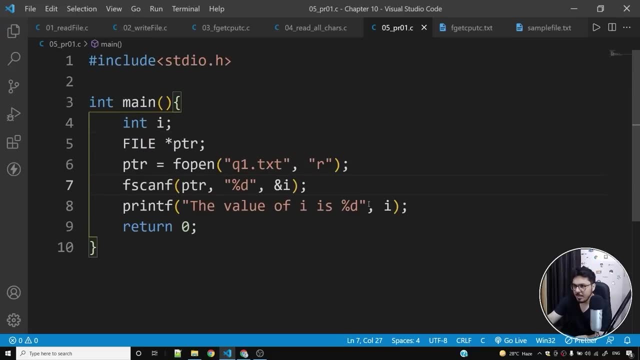 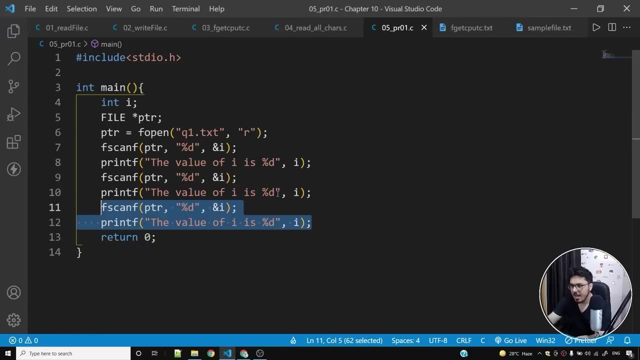 store this value inside i. so first what i'll do is i'll declare an integer variable, which is i, and then what i'll do is i'll simply print the first integer using this printf. i can do this on repeat, and let me show you that this will happen, so i'll simply print the first integer. 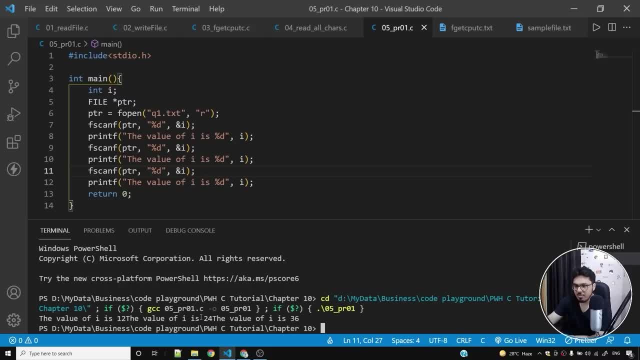 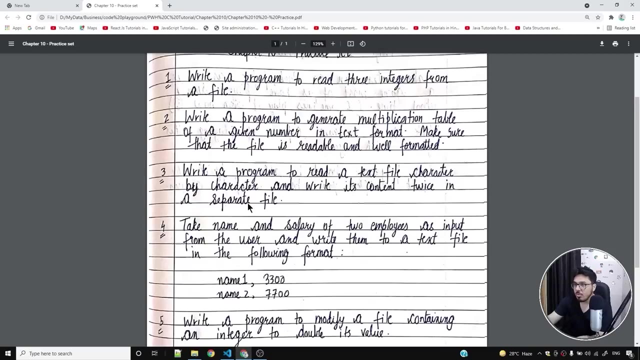 works. So if I run this program, you can see that the value of i is 12, then 24,, then 36.. So I can keep on reading from this particular file. let me write a backslash n just so that we can get a newline character and her output is shown in a formatted way. 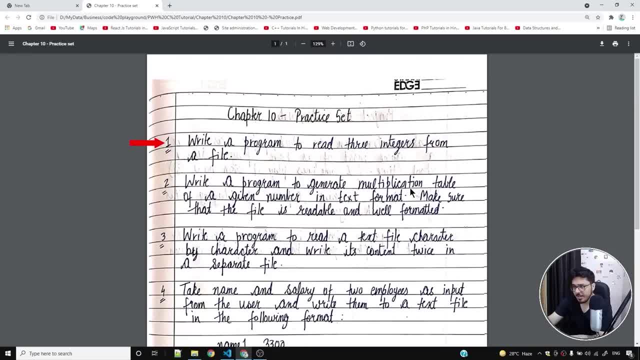 Now let's move on to the next question, which says: write a program to generate multiplication table of a given number in text format. Now, this is something that I want you to attempt, because this is very simple. you can attempt it using fprintf. simply use few fprintf calls. 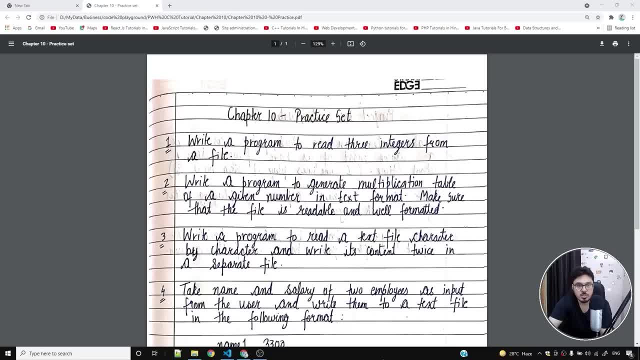 and you should be good to go. So please go ahead and attempt this question. all you need to do is you need to do the same thing that we have done in the initial chapters, but using fprintf instead of printf, So I hope you can do this. 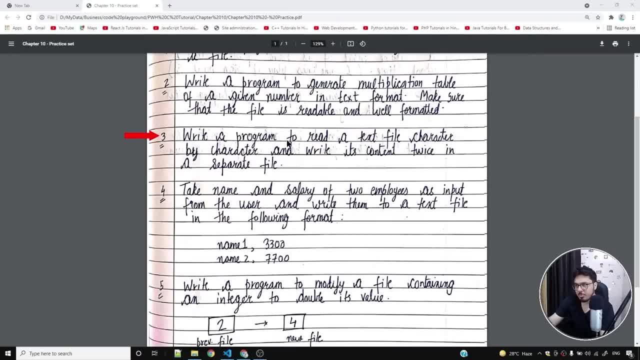 So let's move on to question number 3 now. It says: write a program to read a text file character by character and write its content twice in a separate file. We have already seen this. We have already seen how to read a text file. 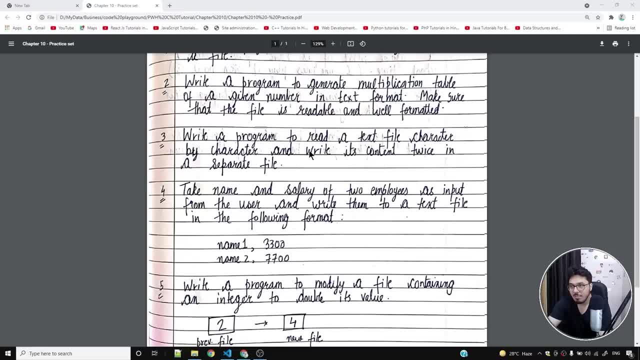 character by character. What you have to do is you have to print that particular thing twice, So you can read twice, or you can simply store it in a character array and you can write it. It's your choice, totally. you can do it however you want. All the methods will. 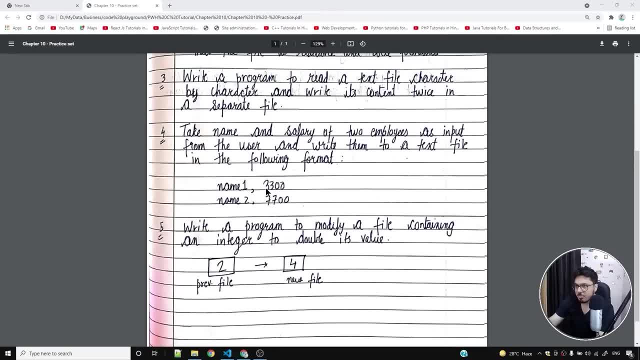 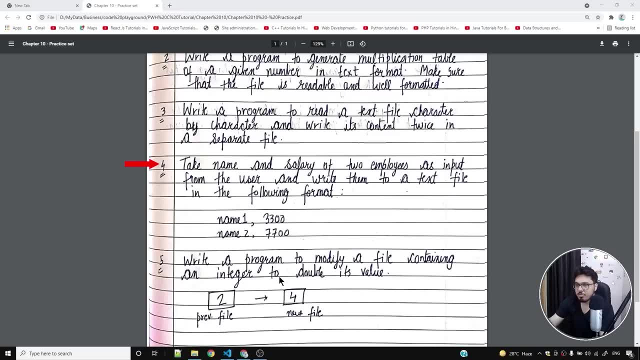 work. Let's move on to the next question, which is question number 4.. Take name and salary of two employees as input from the user and write them to a text file in the following format: So let me solve this problem for you. So what I'll do is I'll simply create: 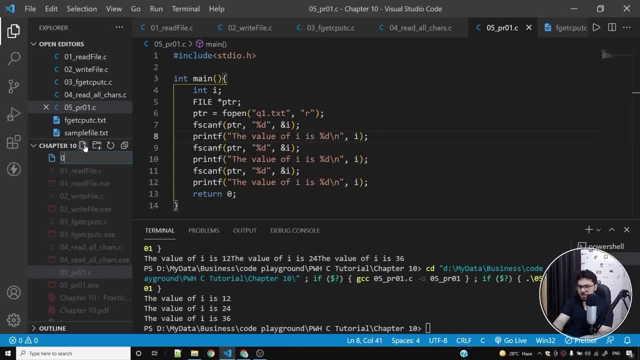 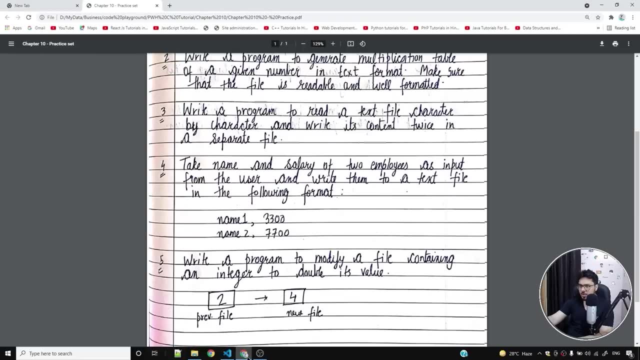 a new file. I'll say 06, underscore pr04 dot c. This is problem number 4, if I'm not wrong. Yes, it's problem number 4.. So what you have to do is you have to read name and salary of two employees. 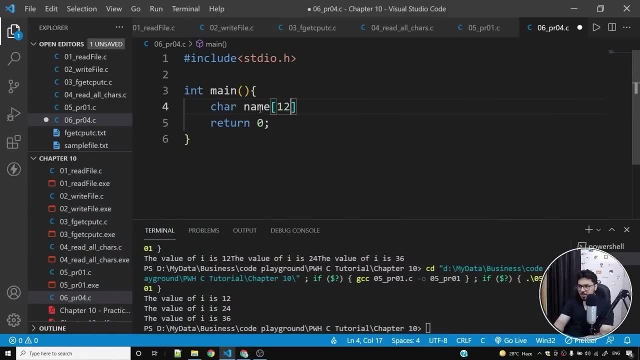 So how do we do that? I can simply create a character array and what I'll do is I'll use int to take the salary from the user. So I'll use printf, I'll say: enter the value of salary And, yes, I'll put a backslash. and to format the output correctly Now, I'll use scanf. 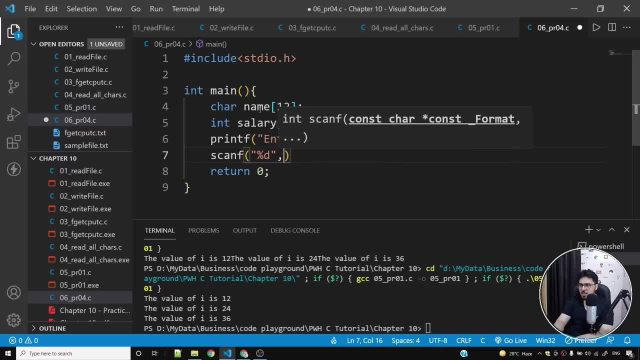 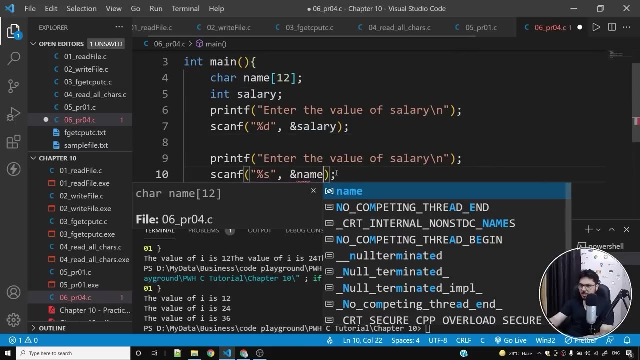 I'll say %d. So %d and ampersand salary. This will give me the value of salary And I'll do the same thing for my name. So I'll use %s this time And I'll use ampersand name. So let me do it name, because name is. 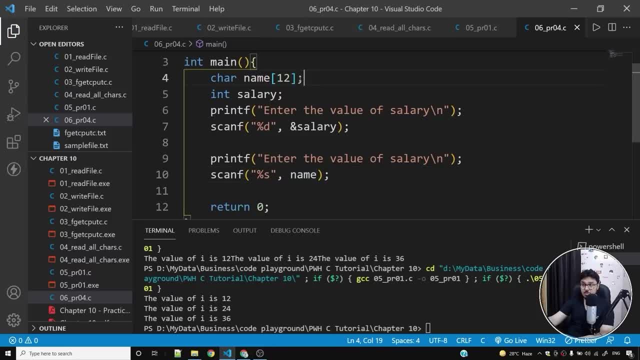 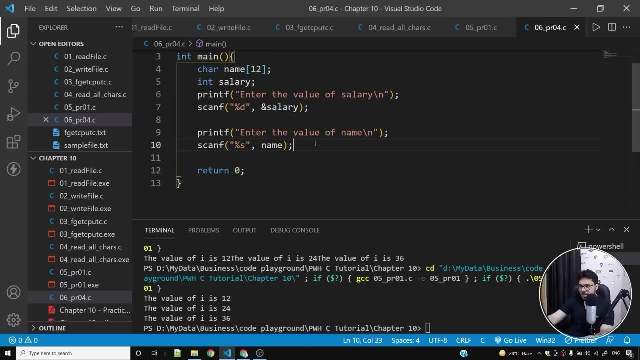 the address of this person, address of this, the first element of this character array- under the value of name, and I'll get name inside name and salary inside salary. so if I want to print the name and salary, I can do something like this. I can say salary. 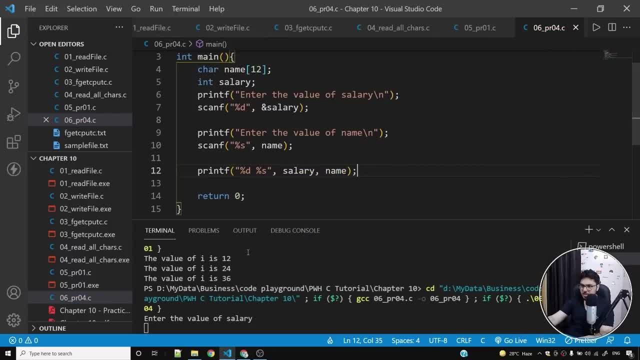 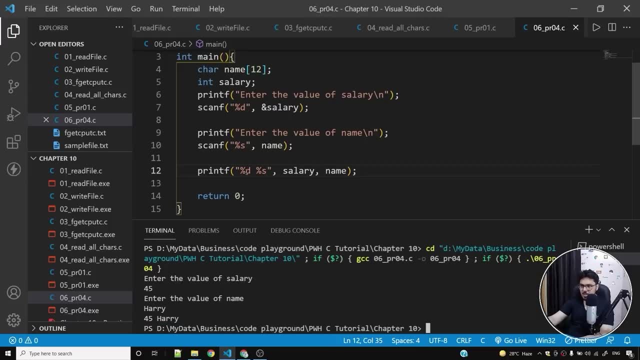 name and you'll see that name and salary will get printed in the output. so if I say 45 and I say Harry, so 45 and Harry are printed on the screen, which confirms that this particular variable now has salary, and this particular variable has Harry or the name entered by the user stored inside of it. so what I have to do 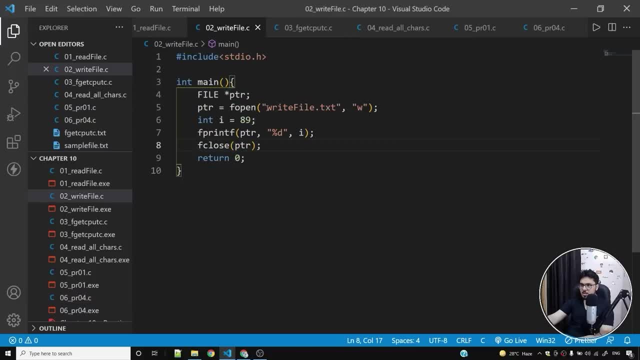 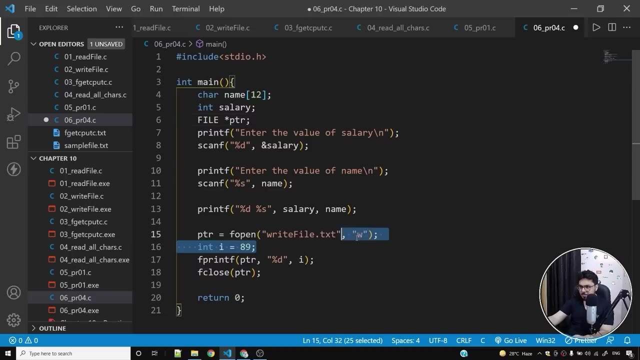 now is: I have to create a file pointer and I have to use this. I have to write to a file. so what I'll do is I'll copy this program and I'll use this file pointer, I'll declare the pointer at the top and I'll get rid of this integer. 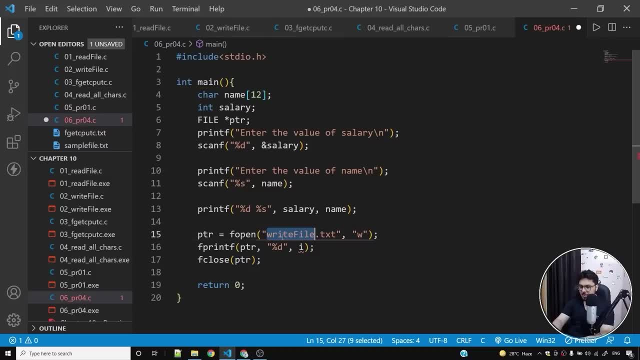 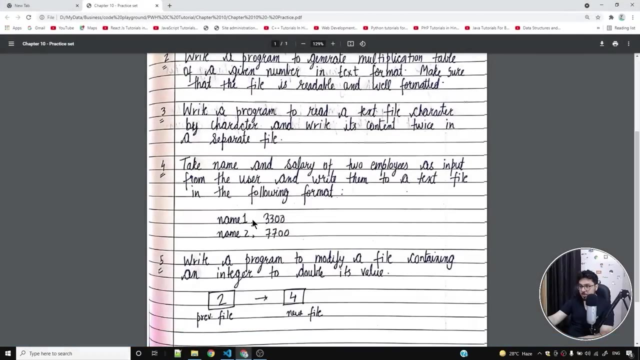 what I'll do is I'll say fprintf, and let me also call it q6.txt, so that you can figure out which question this file is referring to. I'll say salary, and and let me see in what fashion this particular thing demands to get printed. so we have to do it for two. 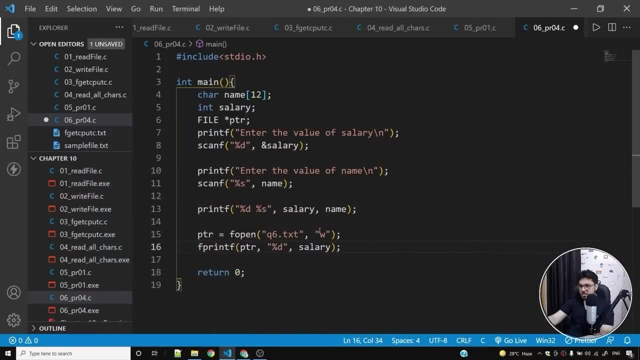 employees first of all. so name, one comma: salary. so let me format it in this way. so I'll say percentage s, and then I'll use a comma and then salary, so I'll say salary and salary. let me see if this works for one employee and name, let me. 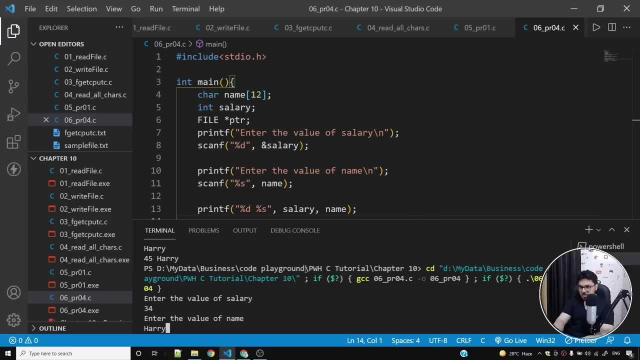 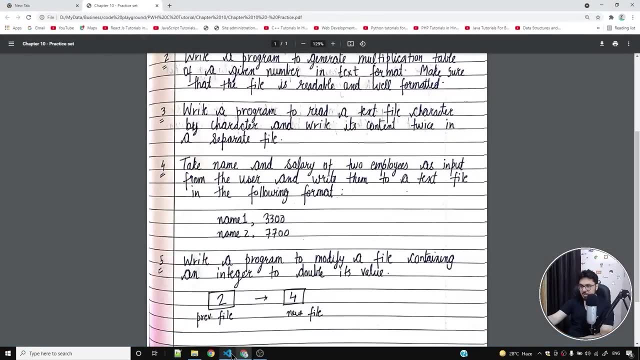 run this program. I'll say 34, Harry, and let's see if 34 and Harry are written to this file. yes, Harry, 34 are written to this file in this manner, but we have to do the same thing for two employees, not for one employee. so, instead of calling, 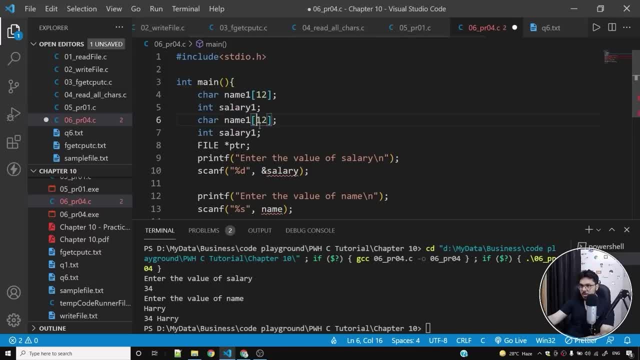 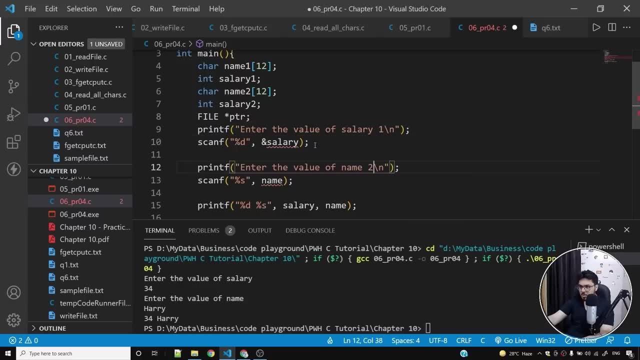 it name. I'll call it name one, and also I'll call it name two and salary two for the second employee and I'll say: enter the value of salary one, then salary two, and we are going to do the same thing for- sorry- name one, and then we are going. 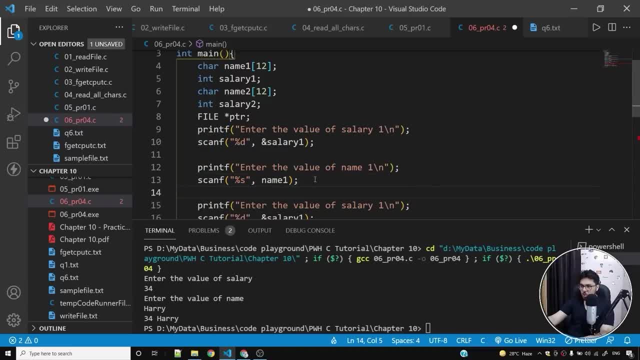 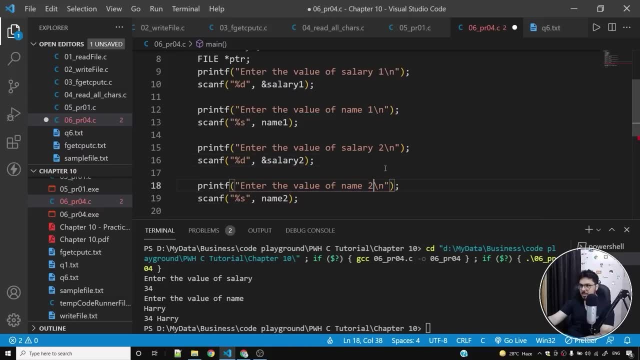 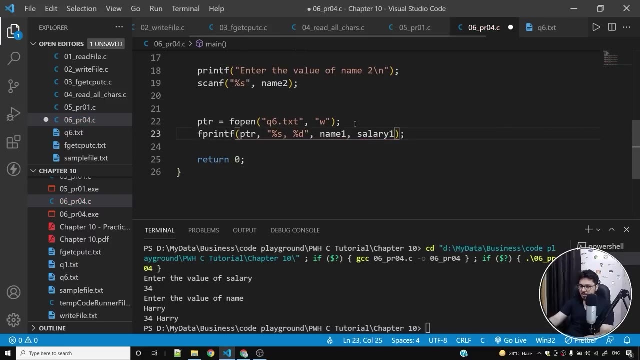 to do the same thing for name two and salary two. so let me call this two, two, two, once again, two here, two here as well, and instead of printing the salary, I'll directly write it to the file. so I'll say name one, salary one and also a back. 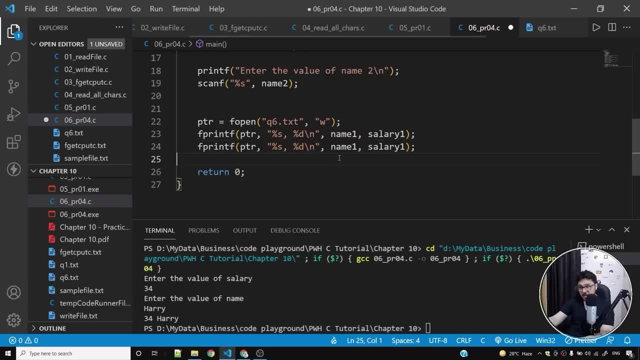 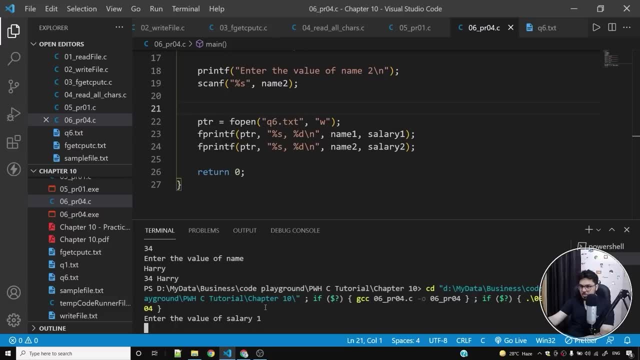 slash n, because I need to get a new line character as well. I'll say: name two, salary two. Let me save this program and let me run this program. Once I run this program, it is asking me for the salary. So if I enter this value and I say Harry, 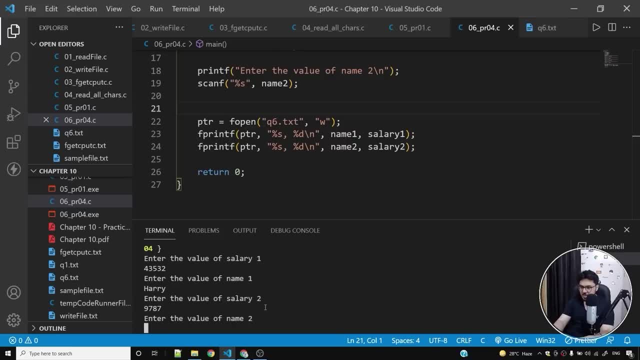 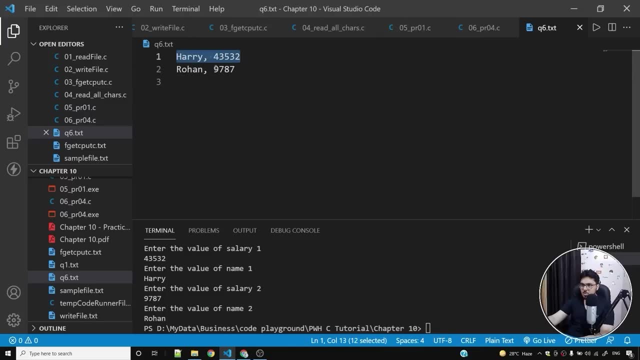 and then once again, the salary for employee two is this, and the name of the employee is Rohan, And if I look at this file, you'll see that Harry, this Rohan, this has been printed. If you want to get rid of this new line, 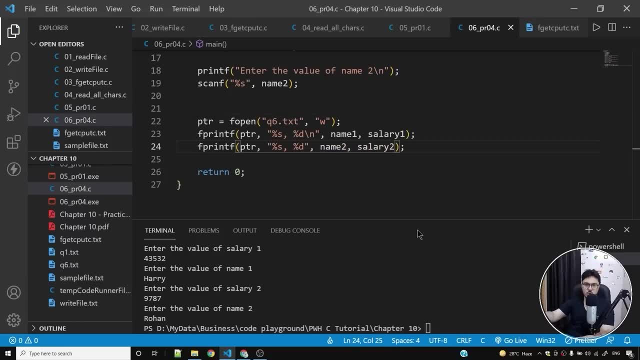 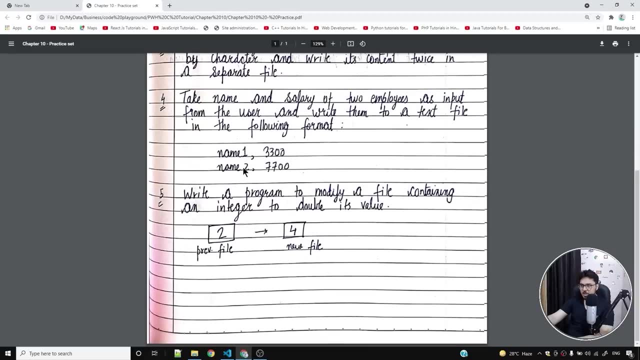 you can remove this new line character from here. You'll not get an additional new line at the end, But this is how you can write to a file in a specified format. Okay, in this case we wrote all the user input to q6.txt in this format. okay. 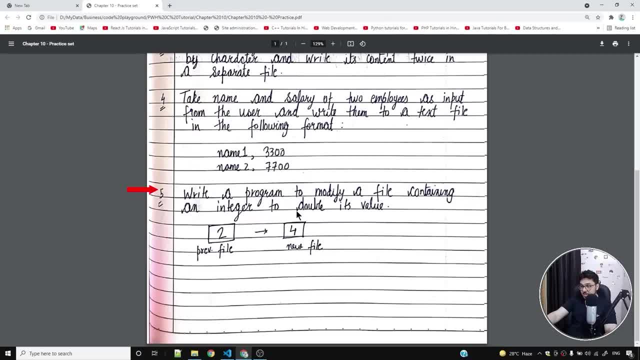 Question number five says that write a program to modify a file containing an integer to double its value. So in order to do this, what you have to do is you have to read the integer from that file and then you'll have to write to the same file. 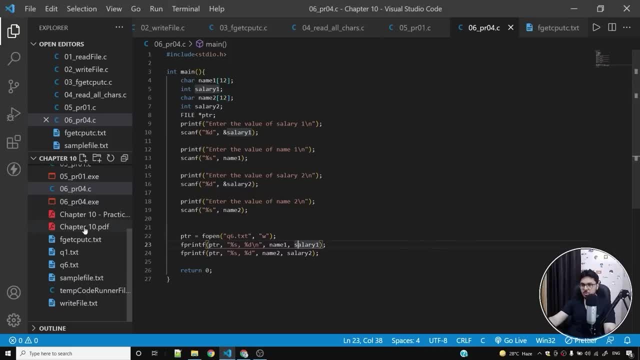 with integer multiplied by two. Let me show you how this is going to work. Let's write seven program, which is problem number q5.txt. sorry, not txt. we're going to get a txt file later, But for now I want to create a C file. 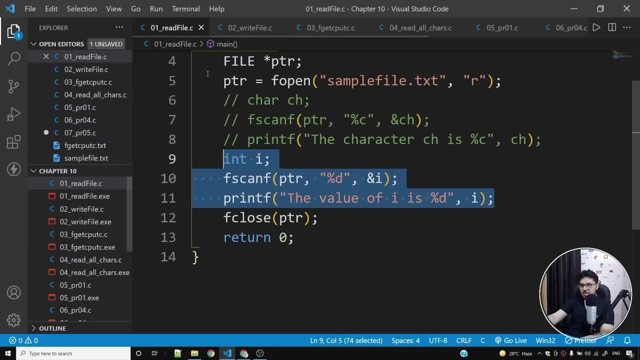 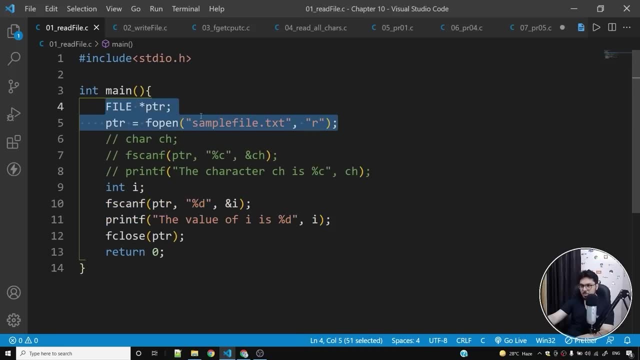 And also in this case we have to read the file as well as write the file. So these two programs are very handy. Sometimes you might forget the syntax. so you can use these programs. All you have to do is open the file in read mode first. 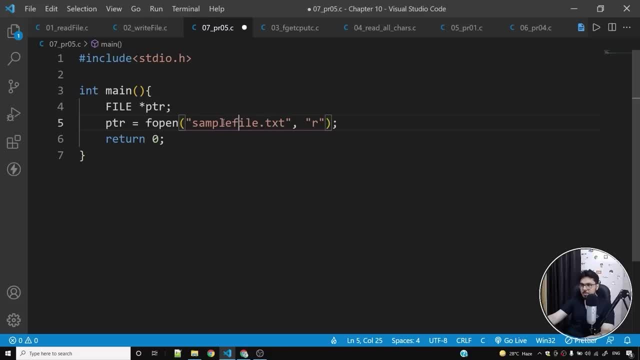 So I'll open the file in read mode and let me call this file q5.txt, just so that you know that this. this is a file from question number five And I'll read an integer from this. So I'll say int i. 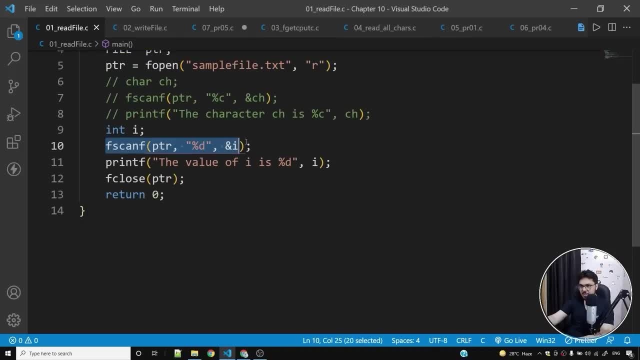 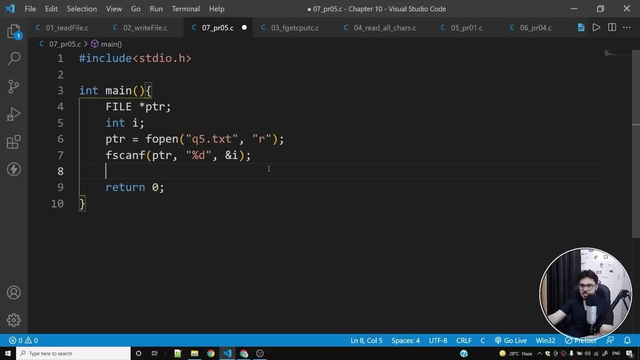 and in order to read an integer from this file, I'll use this fscanf and I'll use the syntax. So whatever integers q5.txt now contains has been stored inside of i, So i now contains the integer which was written inside q5.txt. 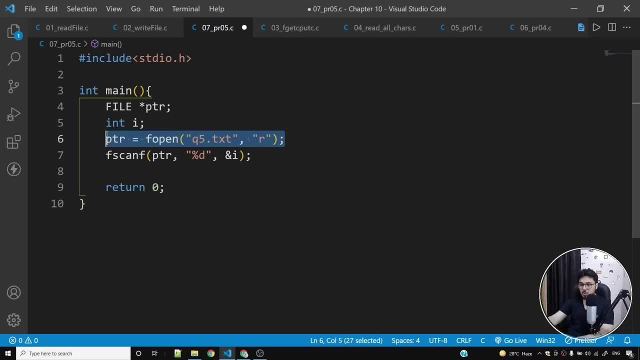 Now I have to open q5.txt in write mode. Now I have to open q5.txt in write mode. Now I have to open q5.txt in write mode, And what I'll do is I will simply write this particular integer to this file. 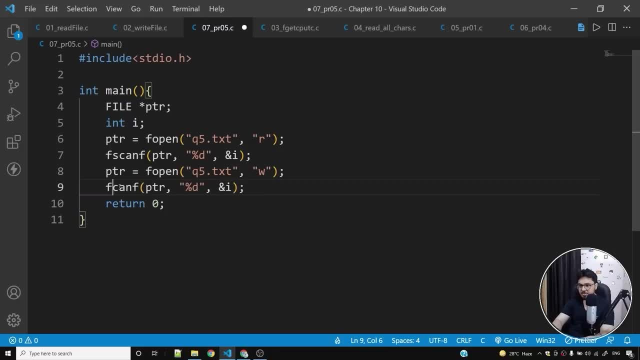 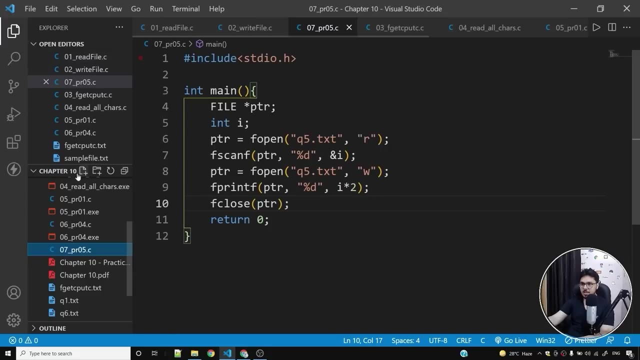 So I'll say fprintf instead of scanf. I'll write fprintf, ptr, %d and i, but not i. I'll write i x 2 to this file And also I'll fclose ptr. I'll save this file. Let me create a file q q5.txt. 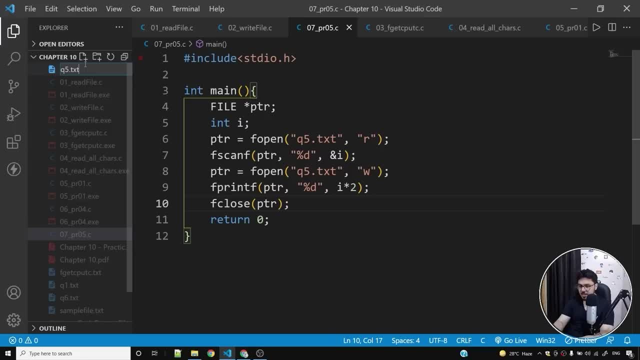 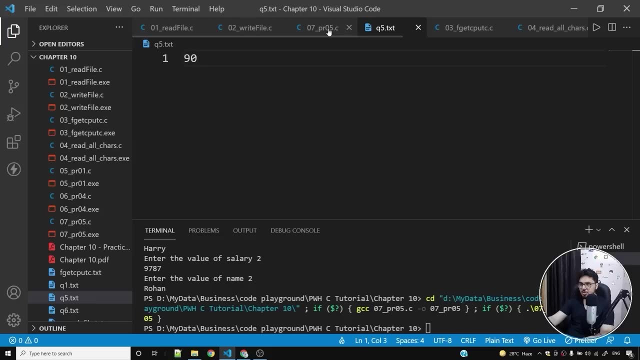 q5.txt. q5.txt. Let's write 45 to this. Let's run this program. if I run this program And if I check q5.txt, 90 is now there. So if I run this program once again, 180 should be present in the file. 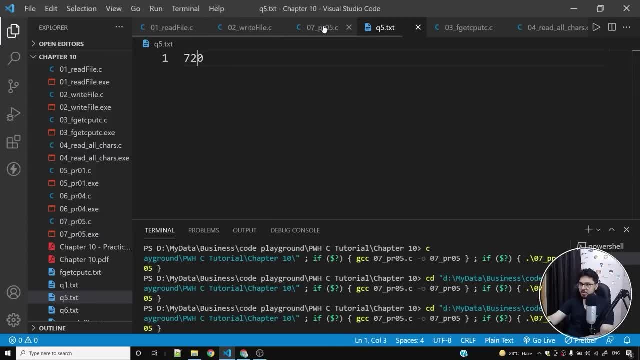 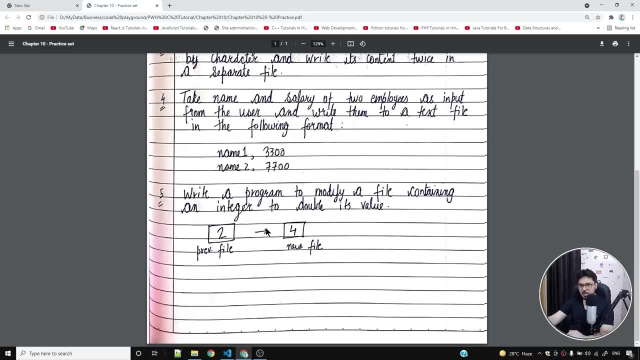 If I run this program been 360, 720, then 1440, 1440 and so on. Okay so this will print double the value inside the file. Okay so, this will print double the value inside the file. It will actually read the file. 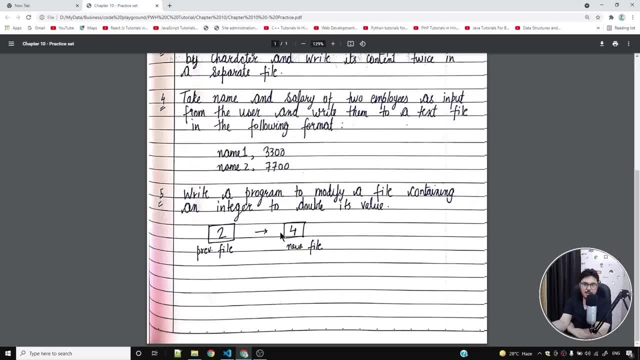 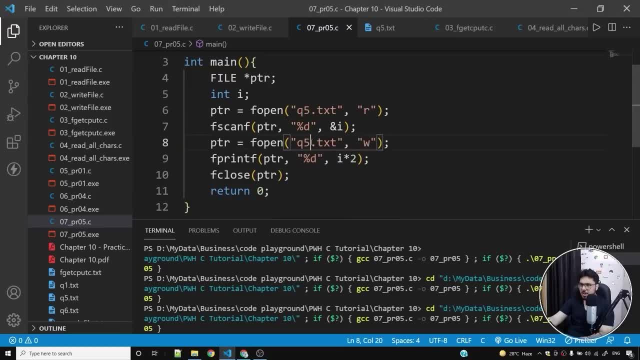 the file first and then it will write double the value to the same file. so i think we have to create a new file in this case. but you can always create a new file. you can always replace this q5 with q5, underscore new, and a new file will be created. so i hope that you understood how files work with c. 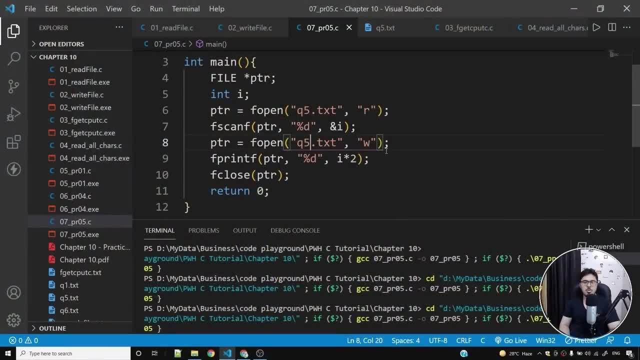 and how you can read and write files in c programming language. in the next chapter, we are going to cover a very important topic, which is dynamic memory allocation, and this topic is going to help you a lot when it comes to data structures and algorithms, so make sure that you. 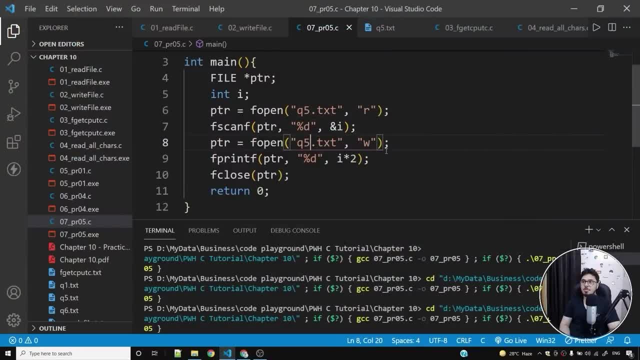 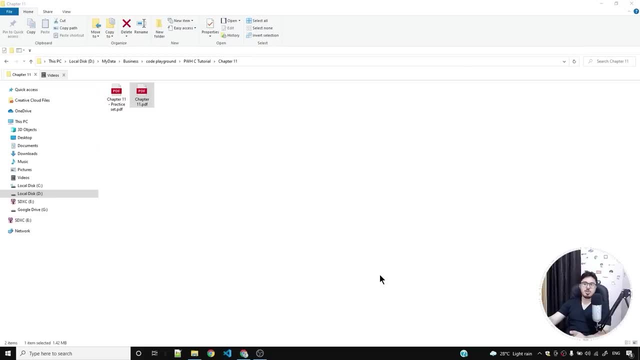 understand this topic really very well. we'll now move on to chapter number 11 and we'll look into dynamic memory allocation. let's move on to chapter 11 now. now, this is going to be the last chapter from this c programming course. i have opened this pdf and the name of the topic is dynamic. 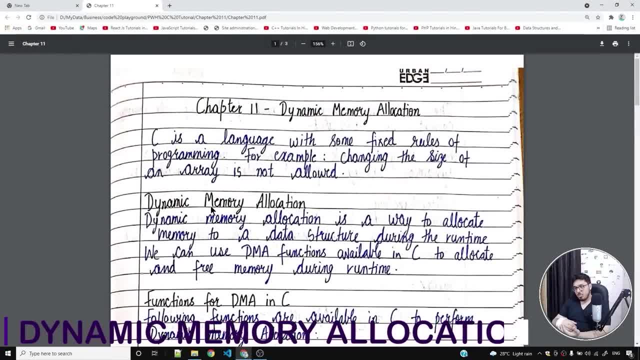 memory allocation really a very important topic if you are going to or if you are planning to go into data structures and algorithms- and for sure you will see it- you will see it for sure interviews and you are going to prepare for data structures and algorithms in the near future. so 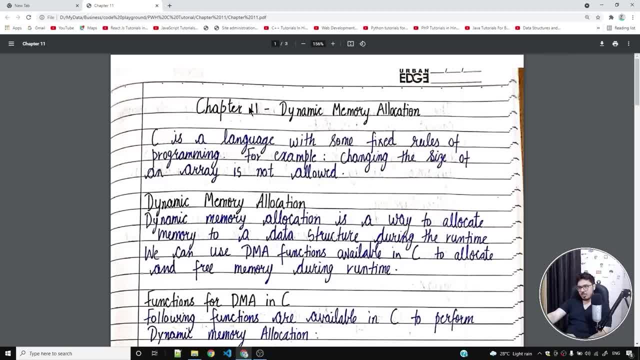 let's prepare for that. let's talk about dynamic memory allocation. so c is a language with some fixed rule of programming. for example, changing the size of an array is not allowed. there are a lot of other rules. you cannot use single codes for writing strings and so on. so we have some. 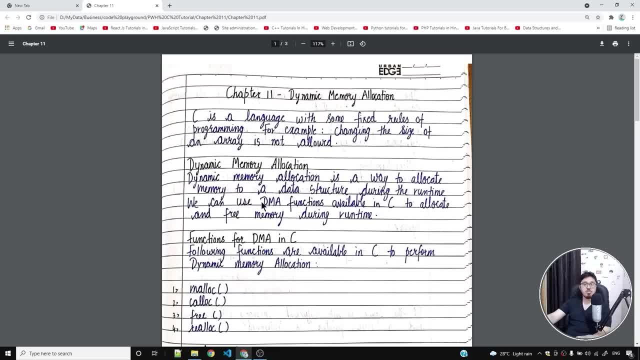 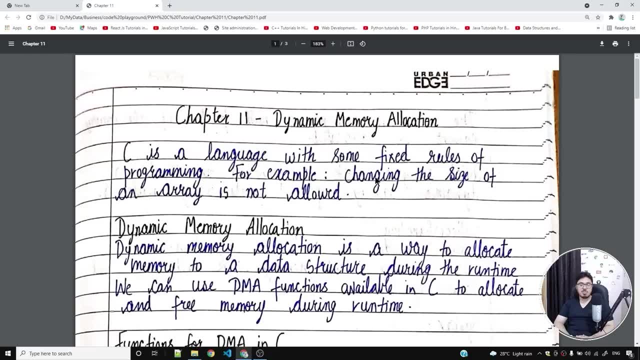 fixed rules. changing the size of an array is not allowed is one of the rules. now, why am i? why am? why have i mentioned this? changing the size of an array is not allowed as one of the fixed rules? because at times you might want to have a variable sized array. 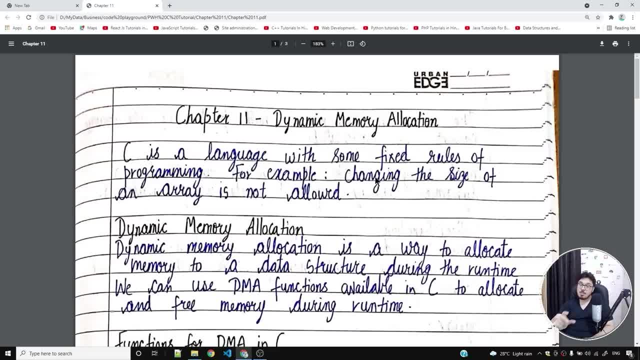 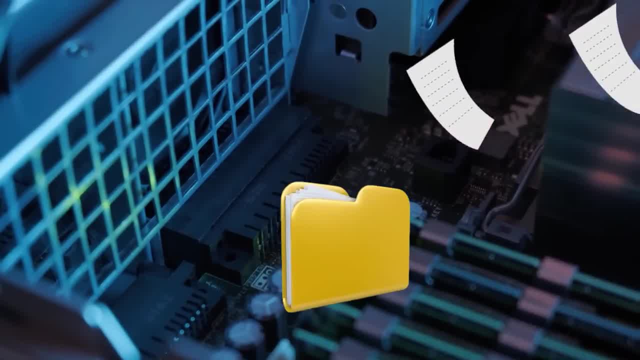 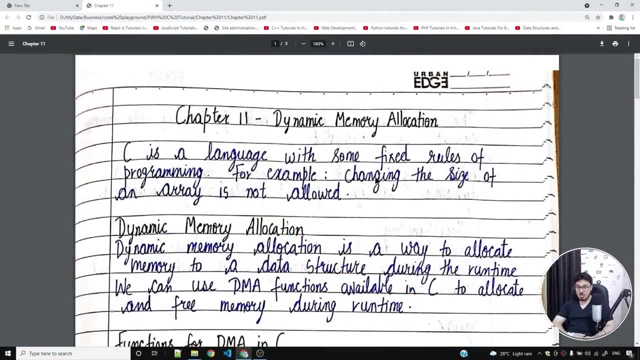 but what happens is memory allocation in a program happens before the runtime. so what happens is before the runtime your program reserves some space in the memory and your program operates on that memory, but at time what happens is we need dynamic memory. now let me explain you what. 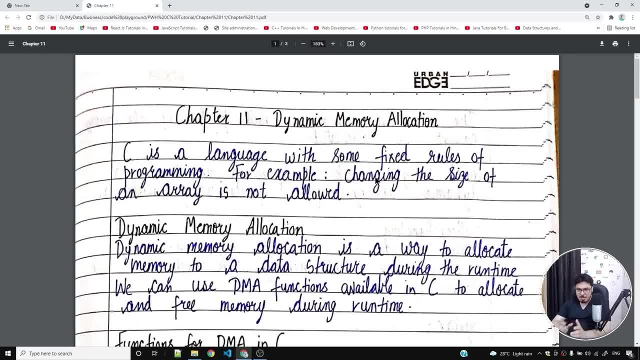 dynamic memory is. dynamic memory is the memory of a program that is operating on that memory that you don't know that you will need, but you might need while the program is executing. for example, you might ask the user for the size of an array now after user tells you the size of an array. 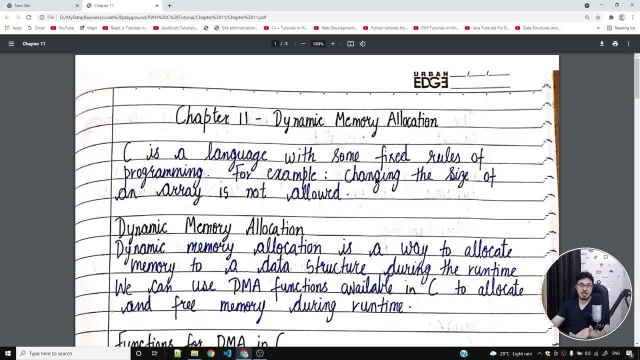 you want to create an array of that size for the user. now, user might enter 5, user might enter 10, user might enter 25, you don't know. so you will have to dynamically allocate the memory. dynamic memory allocation means that memory allocation will happen during runtime. so let's read about dynamic memory allocation from the notes now. dynamic memory. 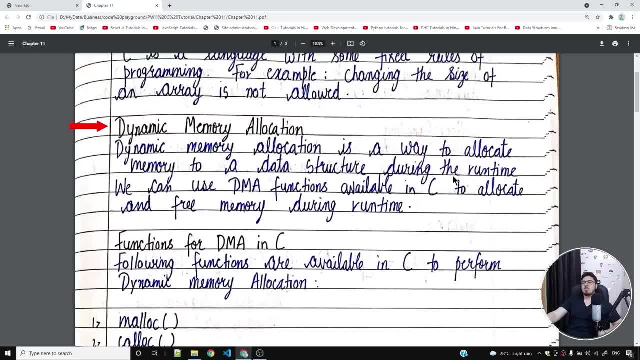 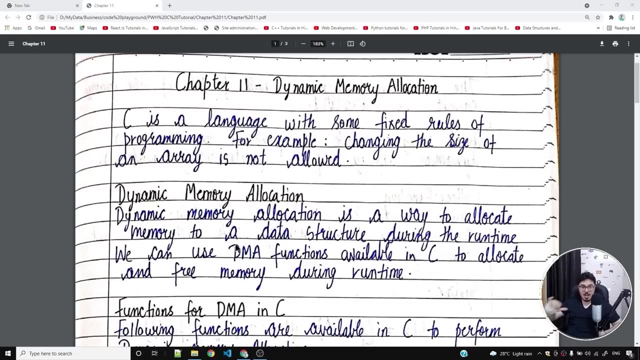 location is a way to allocate memory to a data structure during the runtime. we can use dynamic memory allocation functions available in c to allocate and free memory during runtime. so what happens is if you are using traditional arrays or integers, or character for that matter, what happens is memory is allocated in stack. now, what is a stack? whenever a function runs a stack for 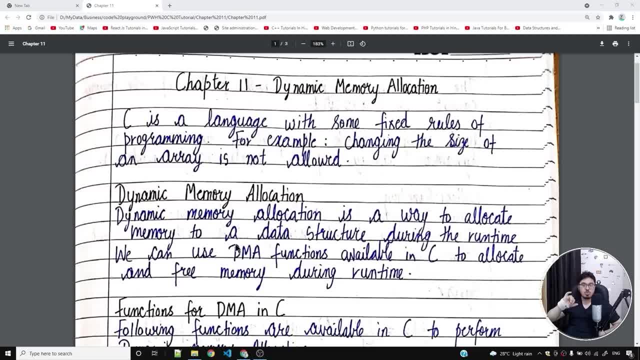 that function is maintained and all the variables are stored in that stack. now you cannot dynamically change the array which is stored inside the stack, but what we can do is we can request some memory from the heap, which is another area in the memory, and we can dynamically allocate memory from the 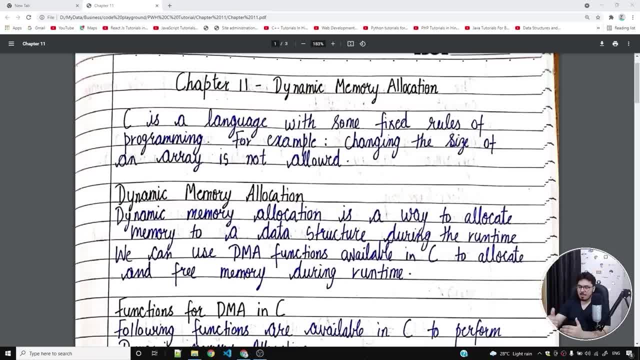 heap. so what we tell our c compiler is: hey, c compiler. i know we are between the program, we are in mid of the program execution, but please give me an array of size: 20, 25, 30, a variable size. it can be anything. the moment you request c compiler for that memory. 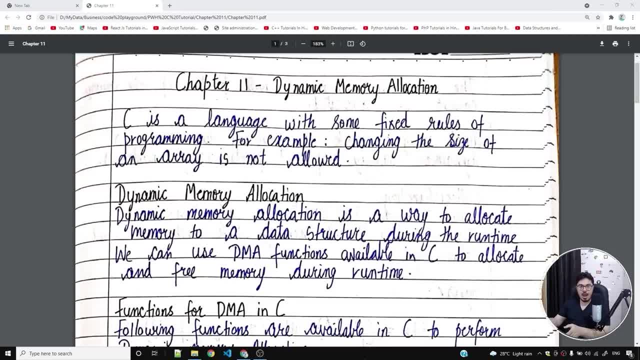 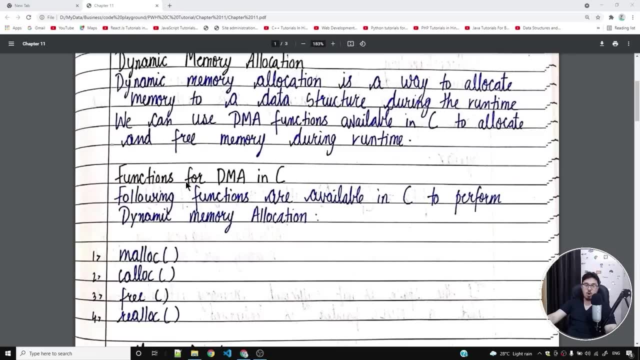 c compiler will go to the heap and allocate the memory in the heap and give you the pointer to that memory. now this might sound very strange to you, but let me show this to you. let me write some programs and we'll learn about some functions that c programming language offers to do the dynamic memory allocation in c. now following functions are available in c to perform dynamic memory allocation: the very first function which is available is malloc, then we have calloc, then we have free, then we have realloc. now, if i tell you in very short about all these functions, let me tell you malloc is for memory allocation. 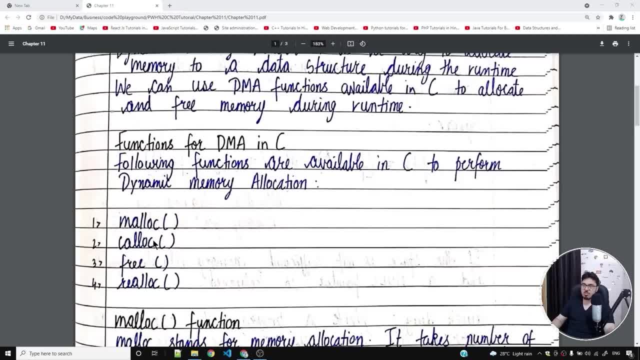 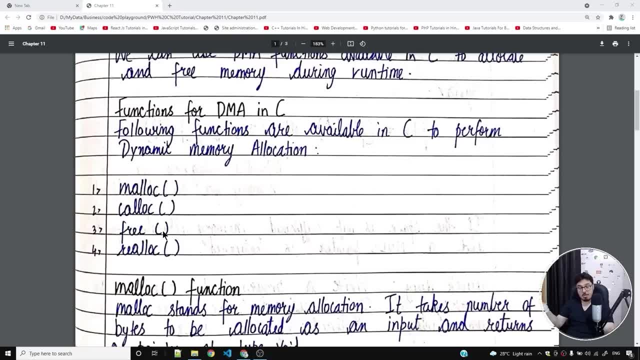 calloc is for contiguous memory allocation. we'll see how it is different from malloc. free is used to free the memory in the heap, because if you are requesting a memory from the heap and there is some memory which will be already in use because you have a pointer to that memory in the heap, now you want to free that memory. 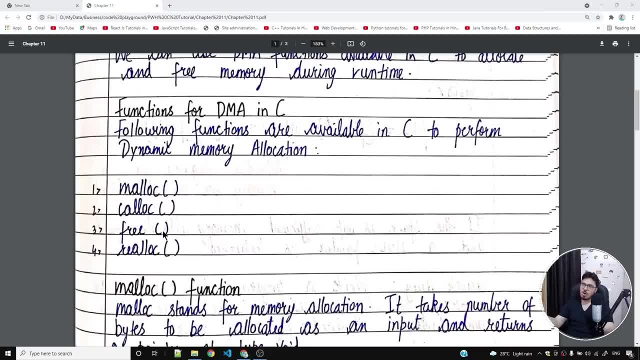 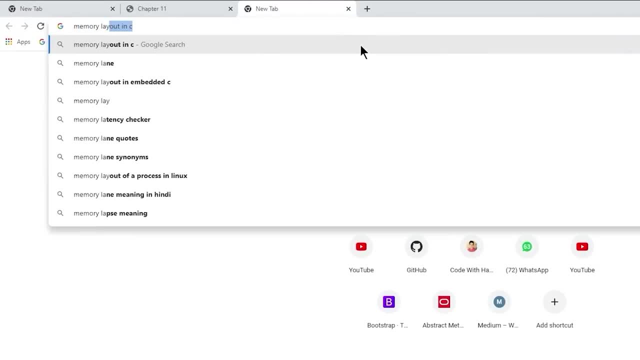 in order to tell compiler that i no longer need this memory. you are free to provide this memory for other tasks. now, realloc is used to reallocate memory in the heap using a pointer. now let me show you something. what i'll do is i will show you memory layout of in c. i want to show you how. 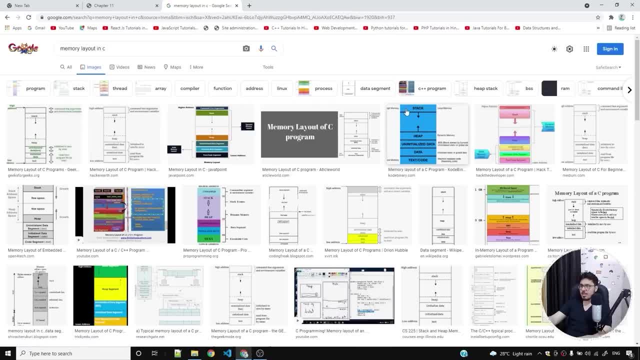 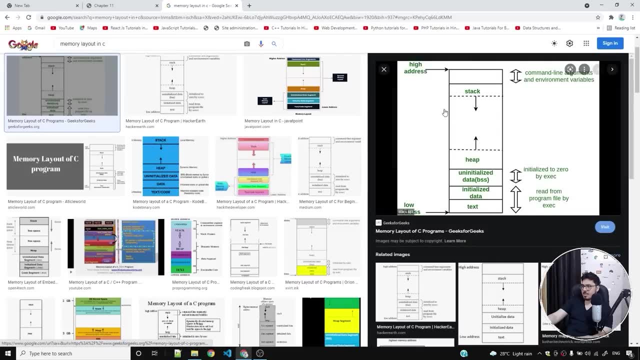 this thing is working, because if you don't understand how this thing is working, it will be really very difficult for you to understand dynamic memory allocation. so let me open an image here. you can see that this is your program in memory. so this is your ram now. this is. 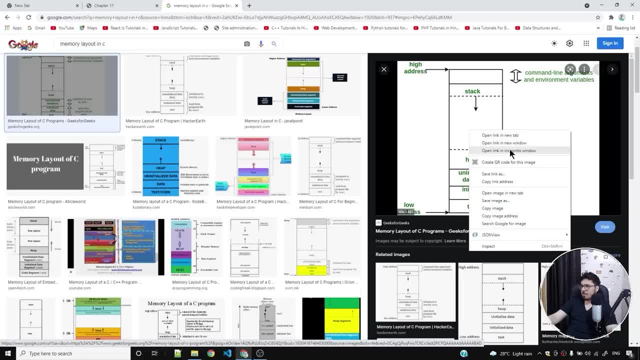 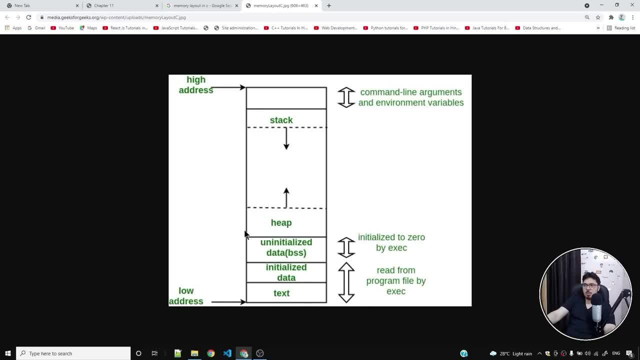 high address. this is low address. this is a nice diagram. let me open this diagram in a new tab. now what i'm going to do is i am going to explain how our program works. so what happens is: this is stack which starts filling from the top. this is heap which starts filling from the bottom. 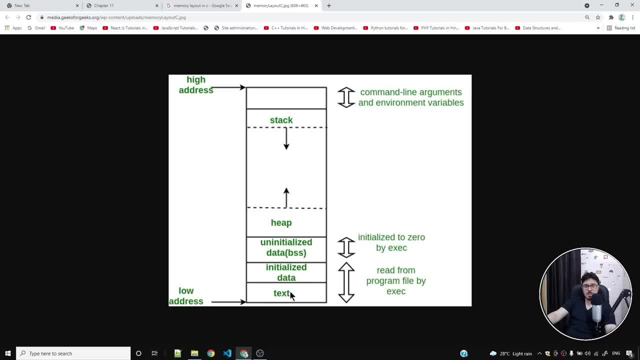 now the stack will hold all the variables from different functions in the program and heap will contain all the memory which is dynamically allocated. how will you allocate memory dynamically from heap? what you do is you allocate the memory in a heap and you request a pointer to that memory and you can now use it in your function from. you can store that pointer in. 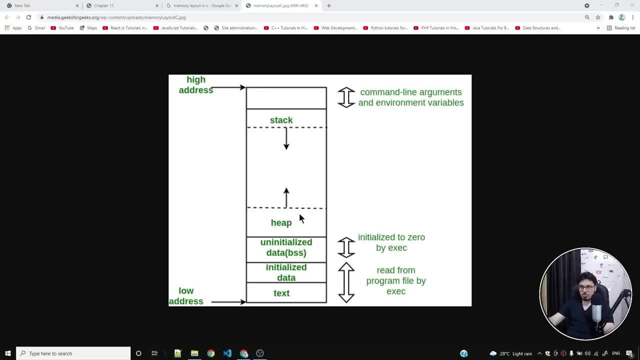 stack and use memory which is available in heap. so i hope that you understood how stack and heap are working. initially we were dealing only with stack, but now we realized that we might need some memory for some time during our execution of the program. we can request that memory from: 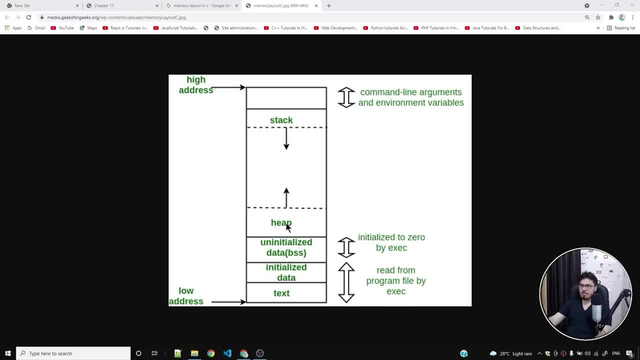 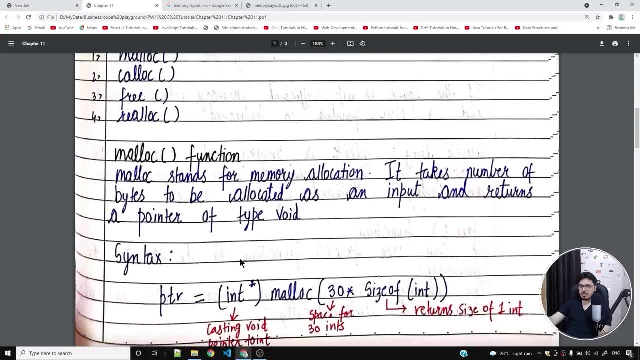 the heap dynamically. it can be any amount of memory as long as it is available. your operating system is ready to give it to you. your program will get it okay. so we'll come back to the nodes and we'll start with the malloc function. malloc stands for memory allocation. it takes number of 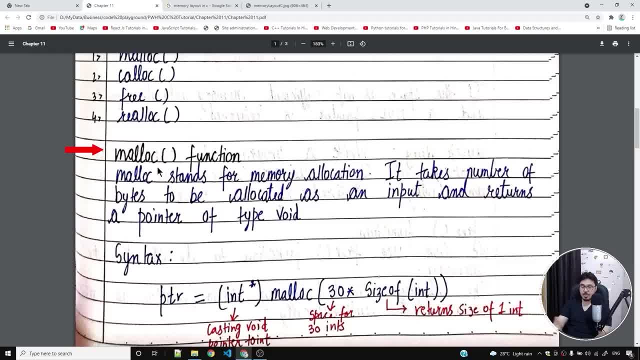 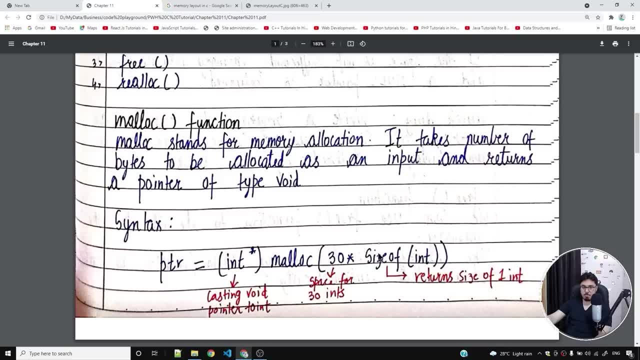 bytes to be allocated as an input and returns a pointer of type void. so what happens is you can use malloc and then you can use the amount of bytes you want, and once you give it this input, you will get a pointer. where will this memory be located inside your ram? it will be allocated in. 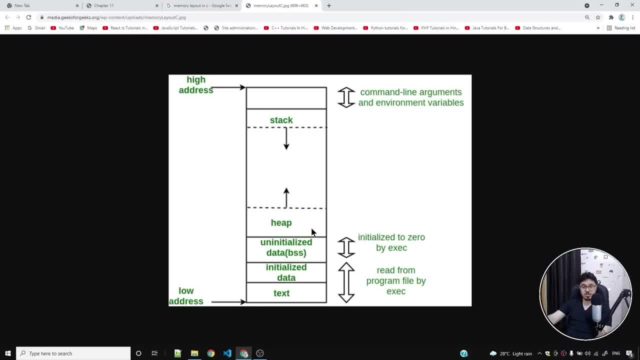 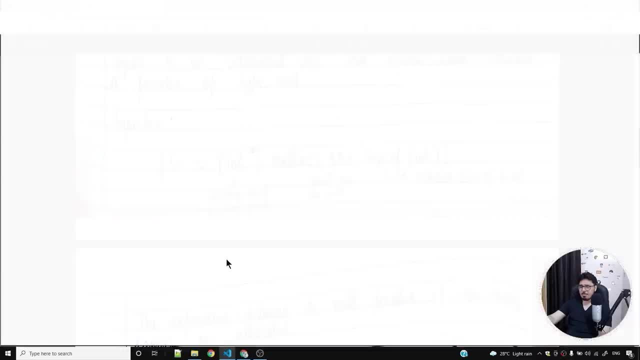 heap. make sure that will be available in heap. you need to understand this concept so that you understand how dynamic memory is working. okay, so let's try to use dynamic memory in our c programs. what i'll do is i'll close this one. i'll open this particular folder in vs code i. 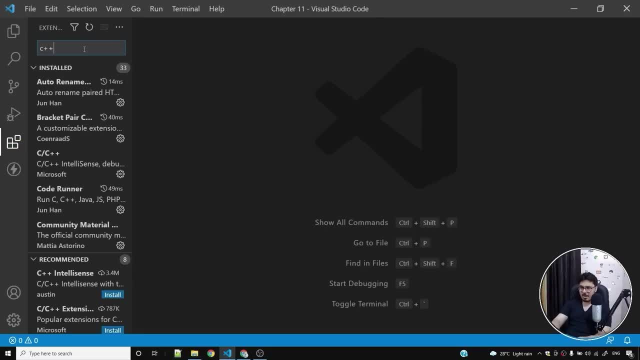 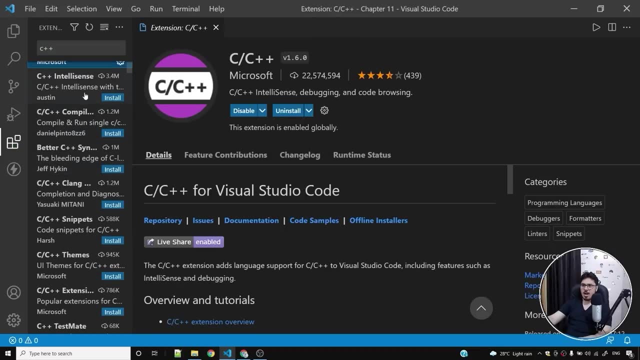 know i'll have to enable c c++ extension because by default, i have turned it off. i'll enable it. okay, it's enabled for now, which is good, and we have code runner as well. let me see if it is enabled as well. it is enabled as well, which is good. now, what i'm going to do is i'm going to 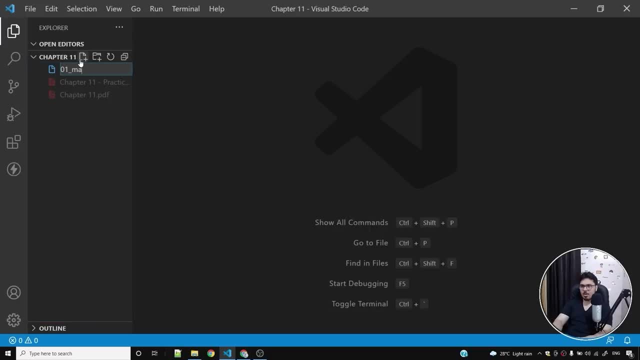 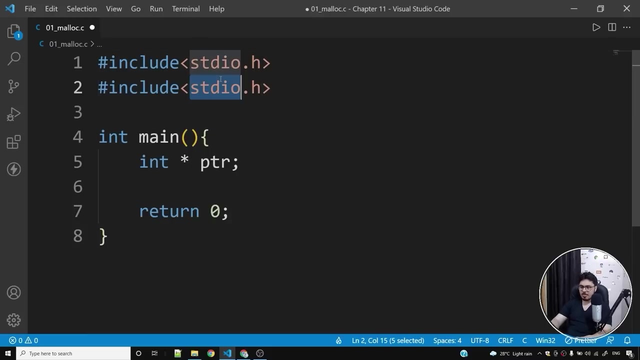 do is: i'll create my first program on malloc, i'll say mallocc and i'll put in the boilerplate code and i'll show you how you can use malloc to allocate memory from heap. now you'll have to use this header file, which is malloch. make sure you include this header file. 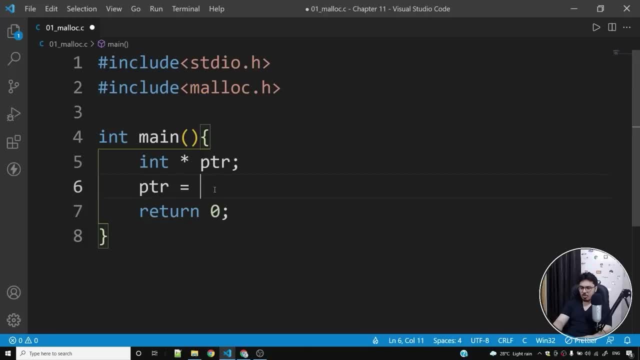 now what i'll do is i'll simply say ptr is equal to int star. we are typecasting the pointer here and i'll say int star and i'll copy that into this pointer type, and what the int star in the brackets does is it will convert the type whichever is supplied. here i'm going to use malloc function. 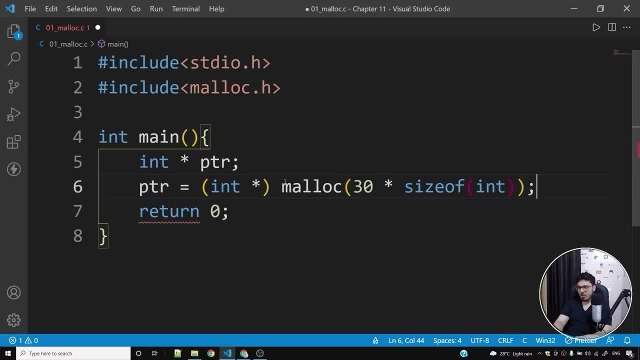 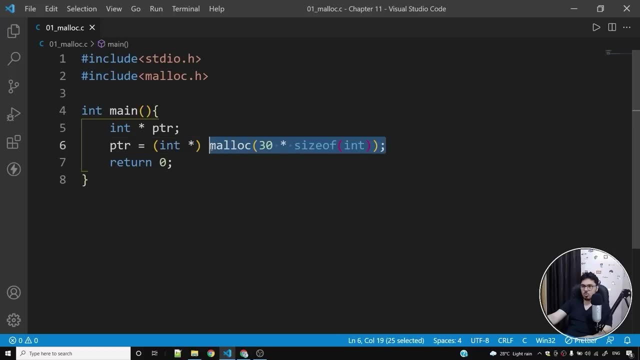 malloc will return a pointer of type void. let me use 30 multiply by size of it and i'll show you what this thing is doing. now, when i say int star, this is basically converting whatever is coming from this to an integer pointer type okay, and malloc, 30 multiplied by size of int will return. 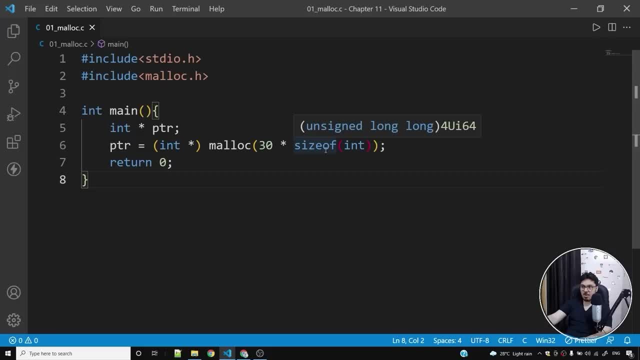 of bytes consumed by 30 integers. Now, size of is a function which will take a data type and tell you how many bytes that data type is going to take. Now, if you want to store 30 integers, you'll have to multiply the amount of bytes. 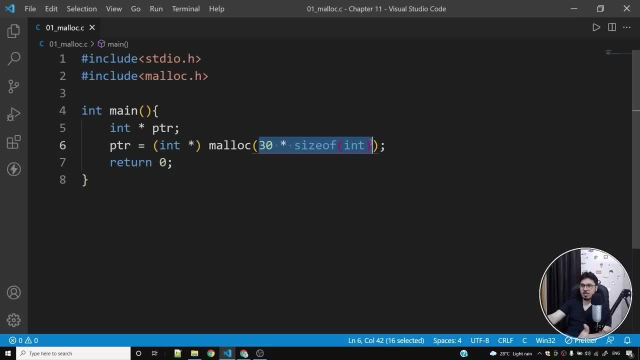 taken by one integer with 30, and you will get the amount of bytes taken by 30 integers. malloc will take the amount of bytes and it will supply you a pointer of type void which can be type casted using int star. If you use int star, malloc 30 into size of int. 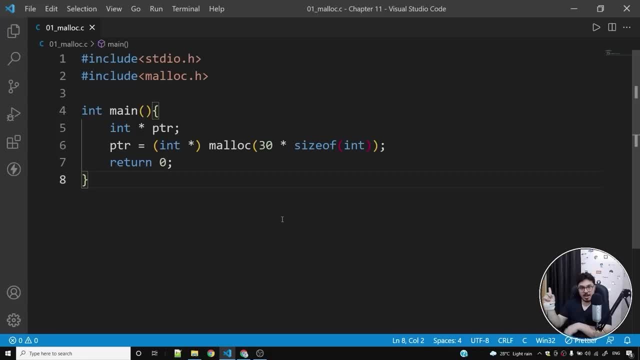 you will get a pointer to the address in heap which is holding your 30 integers in contiguous memory locations, if that makes sense. So I can now simply say ptr zero is equal to. I can use it as an array. I can say ptr zero is equal to 45,. 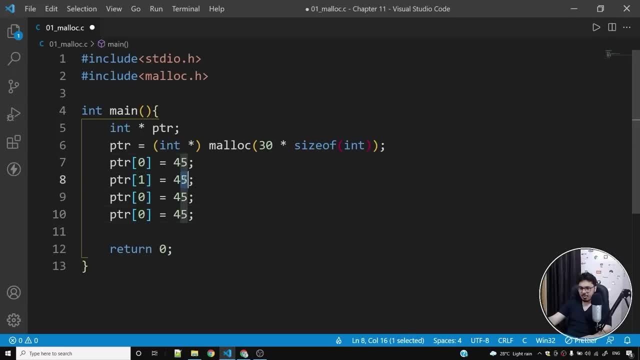 and I can keep on storing values inside this array. I can say 46,, then 47. I am free to store anything I want: Ptr two, ptr three, and I can go all the way around. I can go all the way till nine. 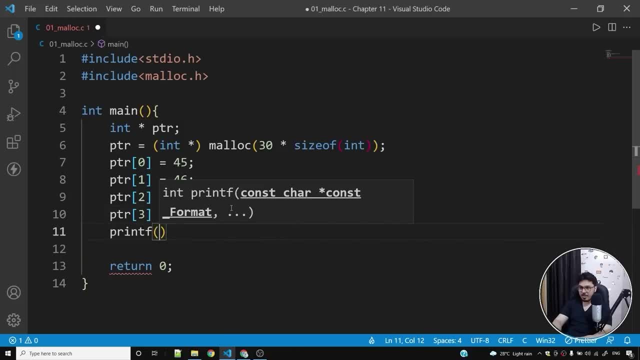 Sorry, 29,, because we have 30 integers. If I do printf %d and if I say ptr three or let me do ptr two, I'll use a semicolon. You can see 47 is printed because ptr two contains 47.. 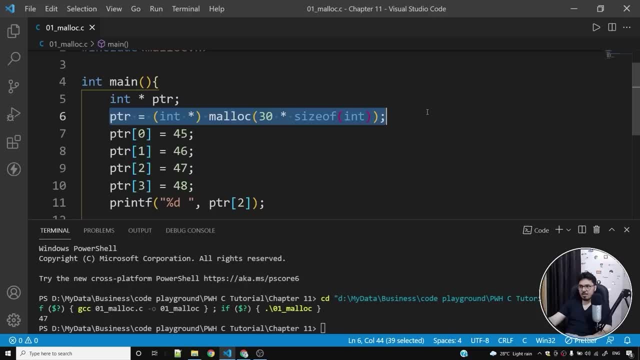 So you can use it as an array, okay, But the new thing about this particular type of array is that it is not inside stack, it is inside heap. It is requested dynamically. Even say int n is equal to five and I can say n into size of int, okay. 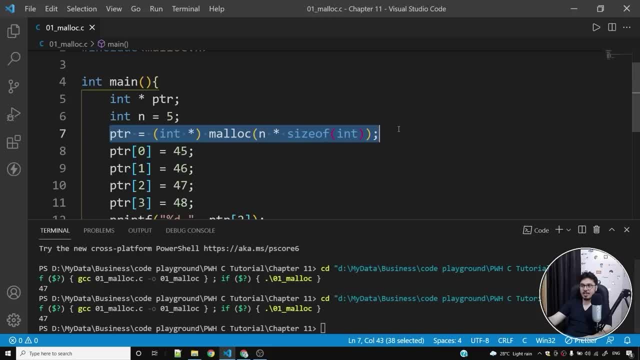 I can do something like this and I can create dynamic memory of size five integers inside my heap. Now this n can even come from a scanf. So if I do scanf %d and if I do something like this ampersand n. 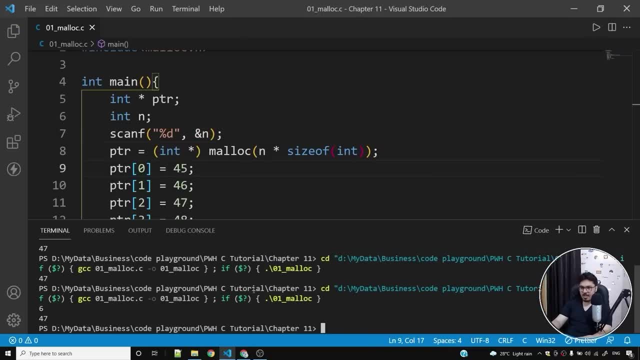 I can even supply six, seven, eight, whatever I want, from my keyboard and I can then use variable here. You cannot do this with arrays. You cannot do int i. or let me show you what I mean by int i. 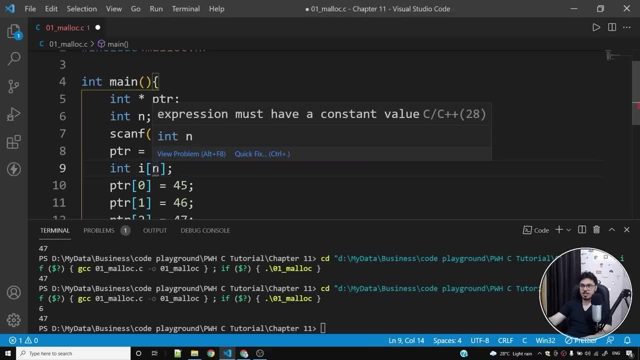 and you cannot do something like this. This is not valid. okay, You can see it's throwing an error. Expression must have a constant value. N is not a constant, so it is saying that it's a variable. You cannot use variable, okay. 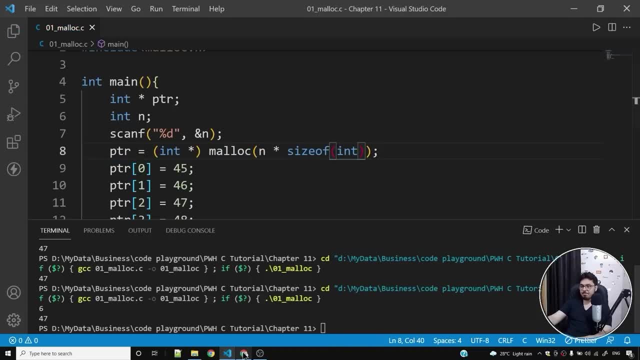 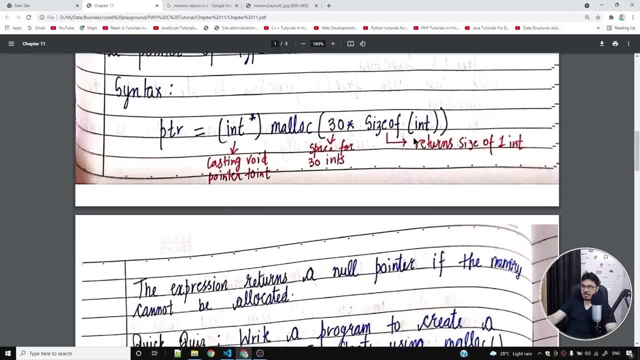 So you want to create an array dynamically. This is how you do it, okay, So I have also written this inside the nodes that we are casting void. pointer to int. This is space for 30 ints. This is size taken by one int. 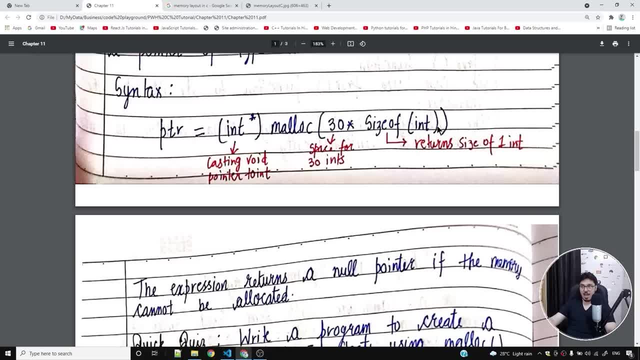 So if you want to create an array of characters, you can use size of char. Now, why do we use size of function? Why can't we simply hard code four here? You can hard code four here, but it's not a good idea to hard code a value here. 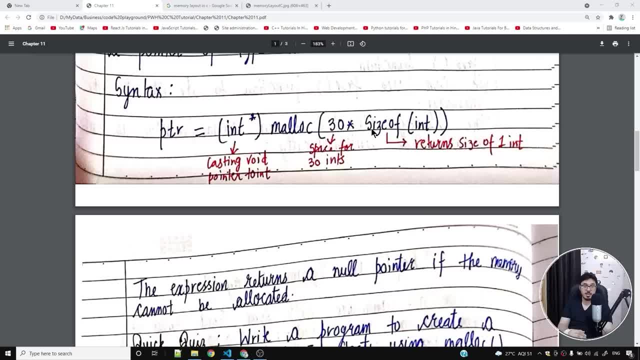 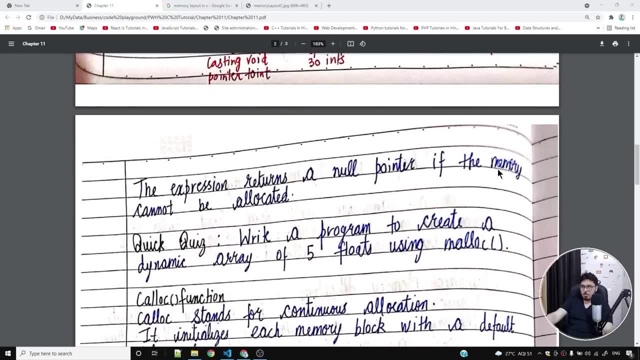 because in different architectures integer might take different bytes, So you don't want to hard code four, Four, two or eight for that matter. Now the expression returns a null pointer if the memory cannot be allocated. So if you request a memory size, 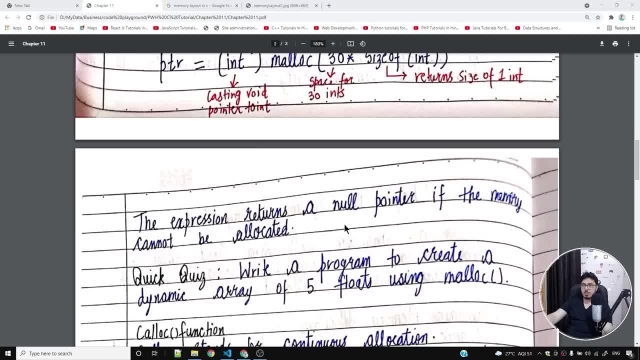 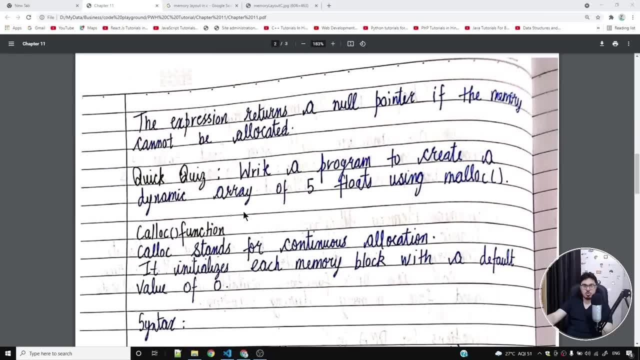 which your computer fails to allocate, you are going to get a null pointer. So if PTR is null, it means that your memory was not able to get allocated by the compiler. So here is a quick quiz: Write a program to create a dynamic array. 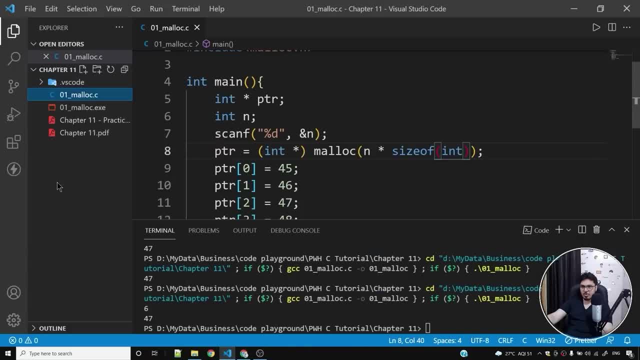 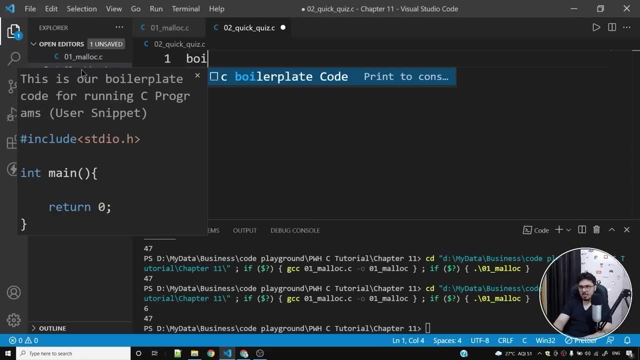 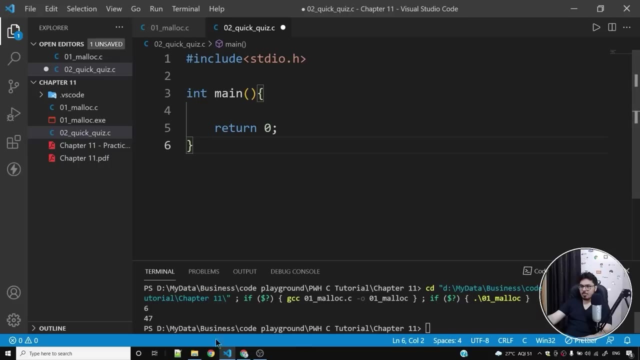 of five floats using malloc. So let's solve this quick quiz. So what I'll do is I'll say zero, two underscore, quick underscore, quiz dot C, I'll use the boilerplate code And what I'll do is let me write a program. 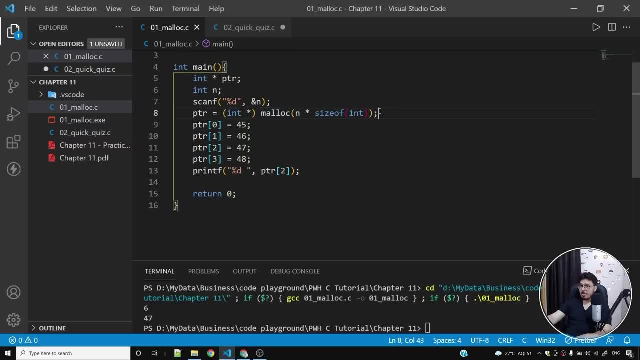 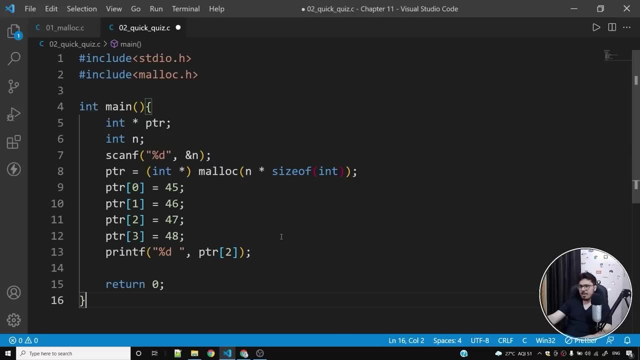 to create a dynamic array of size five floats. So let me use the same program and I'm going to refactor this. What I will do is I will simply say five n is equal to five and I'll say: malloc five into size of float. 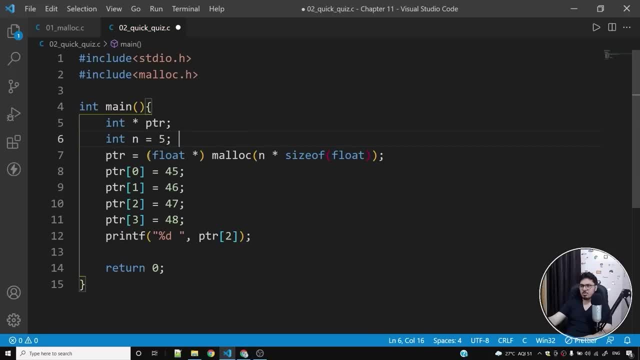 and I'll use float star malloc, because this is PTR, will be a pointer to float this time Float, and let me not use n, let me simply say five here, And I can use floating point numbers here. and since I'm using floating point numbers, 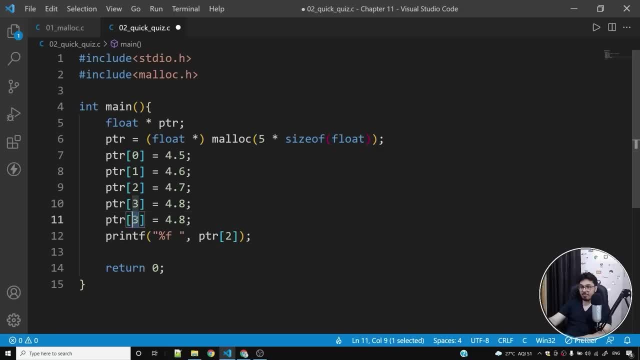 I'll use percentageF So I can store five floats. So I'll say one: four point one eight. let me run this program for you: four point seven, because PTR two contains four point seven. So this is how you can use malloc. 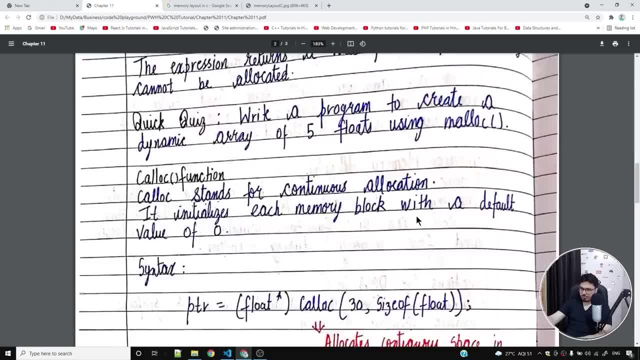 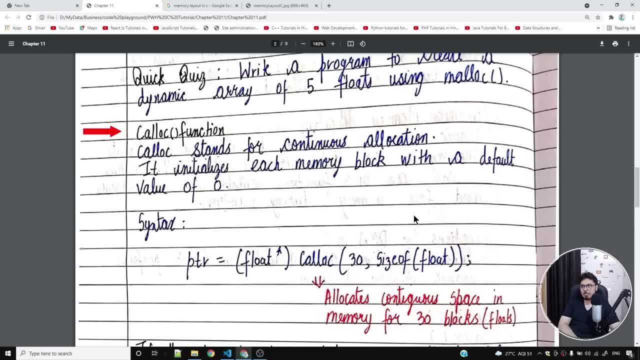 to create a dynamic array of five floats. okay, Let's talk about a Kellogg function. What is Kellogg? Kellogg stands for contiguous allocation. It initializes each memory block with a default value of zero. So in case of malloc, default allocation was not done. 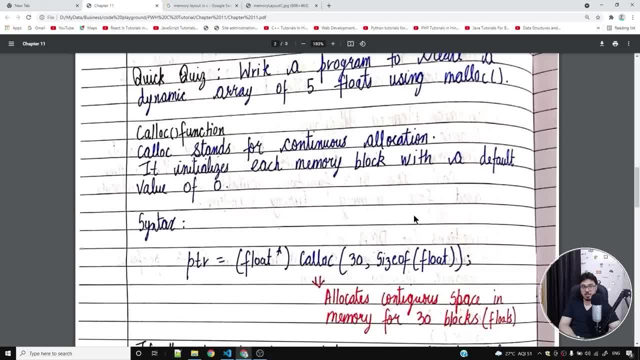 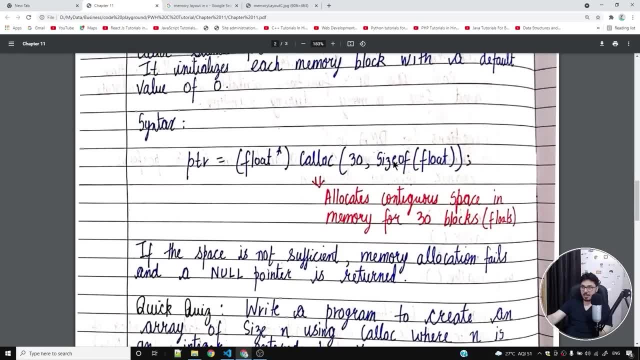 In this case, default value of zero will be initialized each memory block, so you can simply use kellogg. in this way you can say: ptr is equal to float star, kellogg 30 and comma size of float. so this allocates contiguous space in memory for 30 blocks. 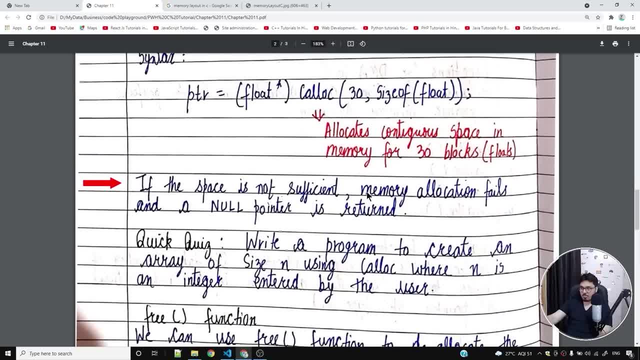 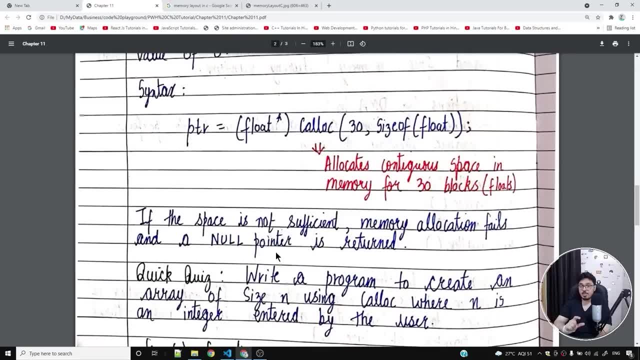 or for 30 floats. okay. if the space is not sufficient, memory allocation fails and a null pointer is returned, just like in the case of malloc. so if null pointer is returned, it means that your memory allocation failed. now another quick quiz says: write a program to create an. 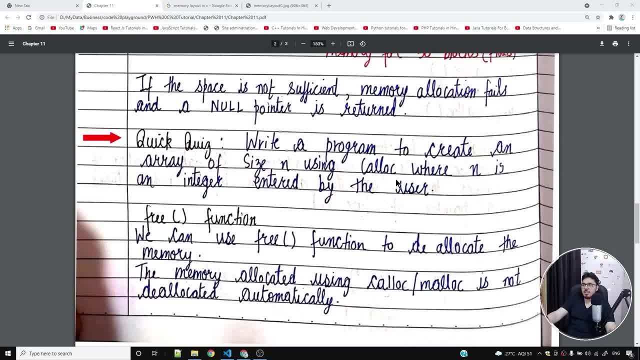 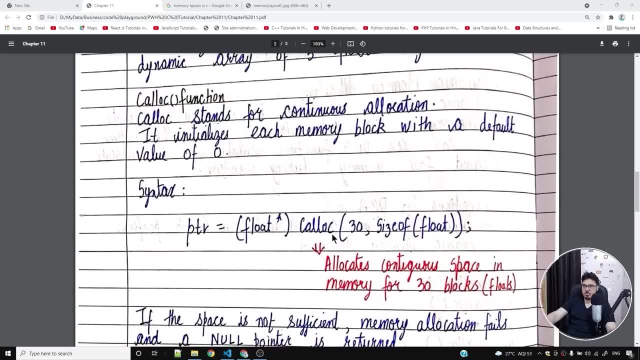 array of size n using kellogg, where n is an integer entered by the user. so n is an integer, which is which is going to be entered by the user. you will use canf and you can simply use this syntax to use kellogg. so kellogg is really very simple. let me show this to you. let me write this. 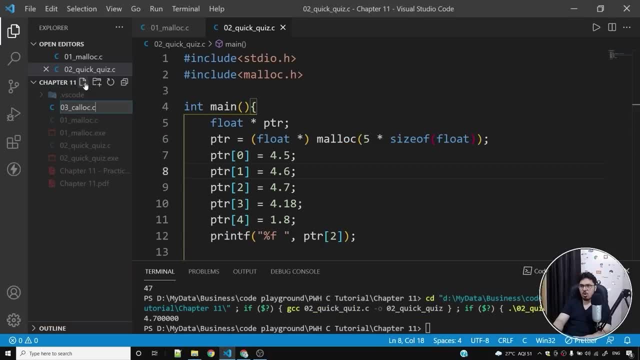 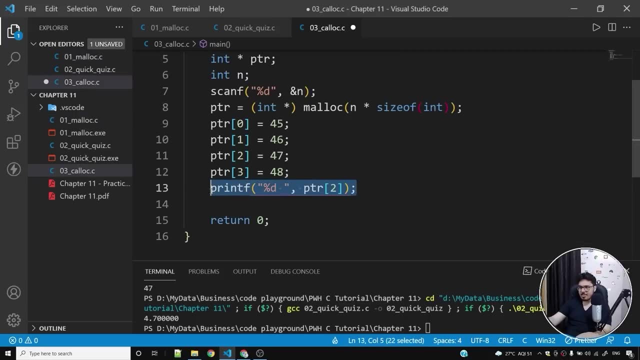 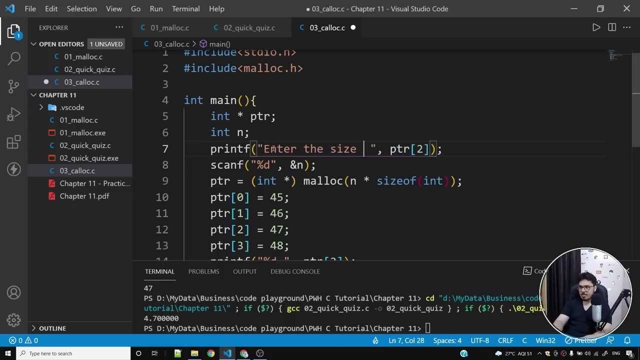 program for you. i'll say zero, three underscore, kellogg, dot c, and i'm going to use the same program that i used for malloc, except the fact that this time i'm going to use kellogg. so i'll say printf, enter the size of your array and i'll simply say ampersand. i'll say nothing because i've already. 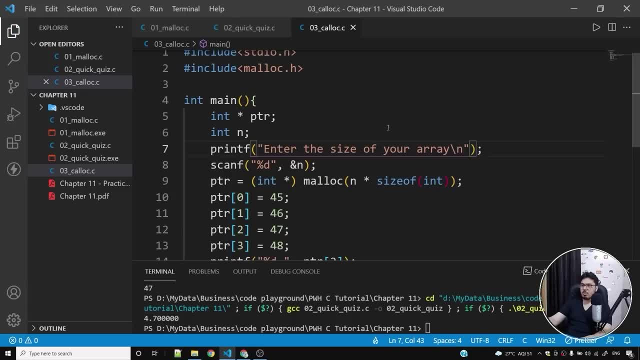 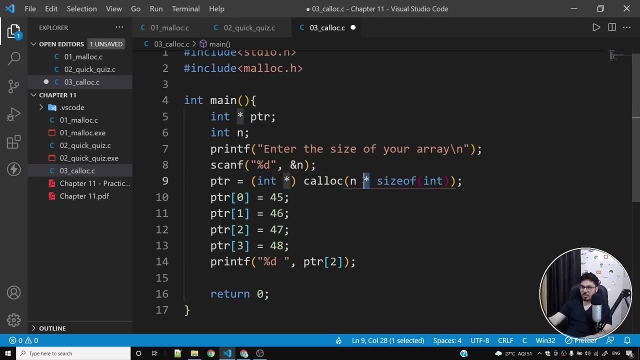 used this scanf in the new line. so what will happen is this is an integer pointer, this is an integer. now printf: enter the size of your array will be shown on the screen. then user will enter the size, and then what i'll do is i'll use kellogg, and kellogg takes two arguments. first is the, uh, the? 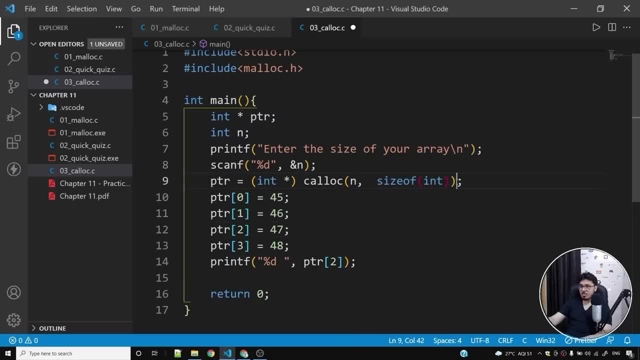 number of integers, loads or whatever you want, and then the size of one block, so it will allocate these many contiguous blocks of this size. so i want n blocks of size of int, which is four in this architecture. okay, so i can use this to create an array. let me come back to the question. so size n. 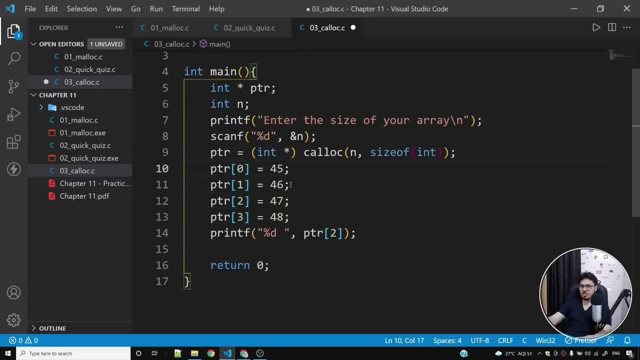 block where n is an integer, so i can enter as large n as possible and this will do the job for me. so if i save this program and run this program and if i say 4, 47 is printed, so i can allocate an array of size 4 by using this syntax as well, but by default what will happen is all the blocks will. 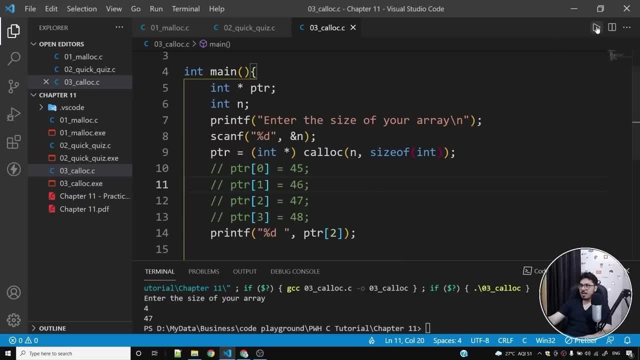 be initialized to zero. so if i don't do this, i will get zero as the output. so if i say 4, zero is the output. in case of malloc you might or might not be able to do this, so i'm going to do this in any case. in malloc you might not get zero as the output, but in kellogg you will always get zero. 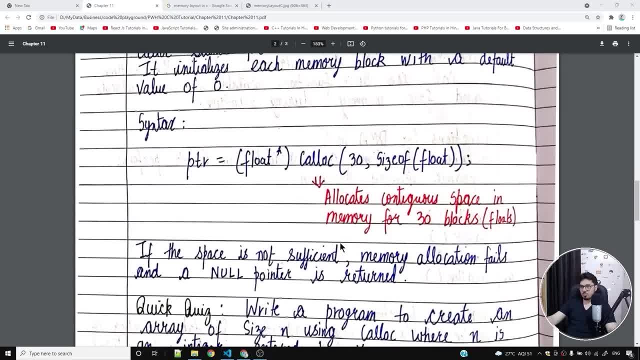 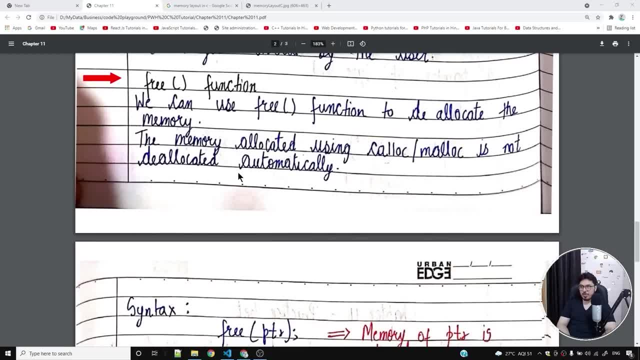 as the output, because all the blocks are initialized with the initial value zero. so i have already written it here. where is it written? it's written here. okay. now let's talk about free function. we can use free function to deallocate the memory. so if a pointer is holding some memory, 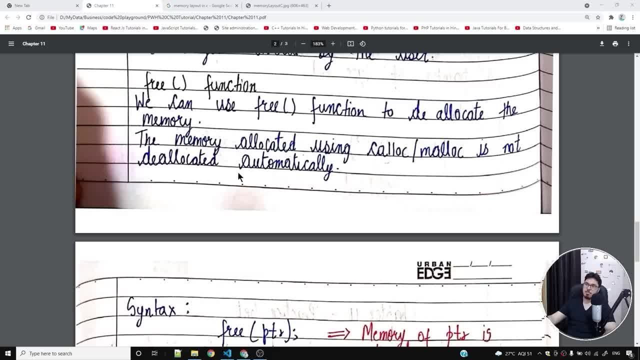 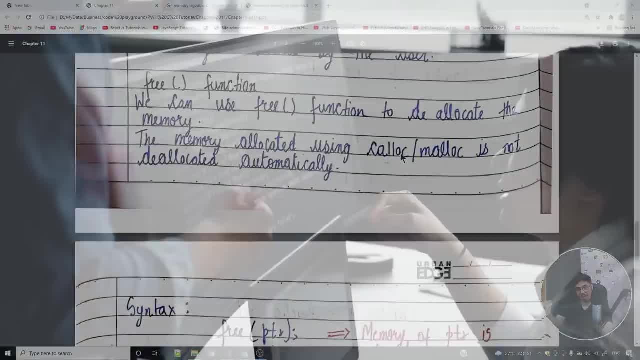 you can always use free and that pointer to free that memory in the heap. the memory allocated using kellogg malloc is not deallocated automatically. so the moment you use the function to free the allocate memory and use it and your program is still running, Kellogg or Melloc will keep. 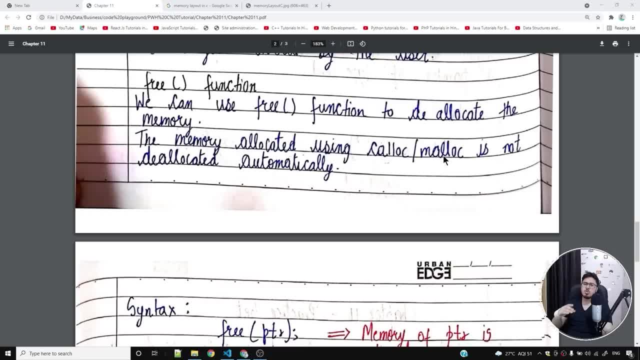 on holding that memory in heap. Now your compiler might do some sort of optimizations from its end, but we are talking about C program here and Kellogg Melloc will not deallocate the memory automatically. So in that case you'll have to use free function which will release the memory which PTR was. 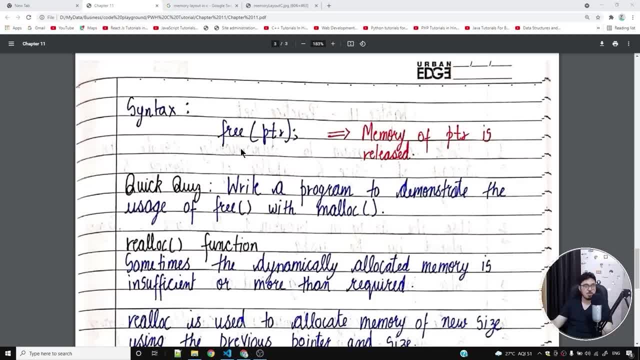 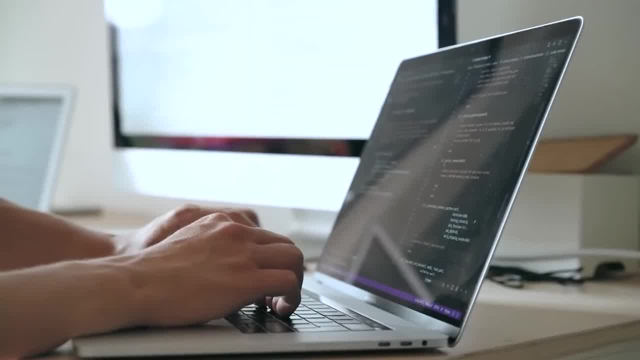 holding. So if you were holding, say, five ints, those memory blocks will be freed. So here's a quick quiz: write a program to demonstrate the usage of free with Melloc. So you are free to write the program. it's really very simple: simply use a free function. 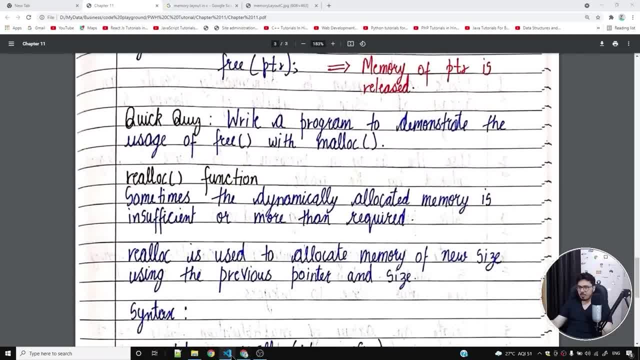 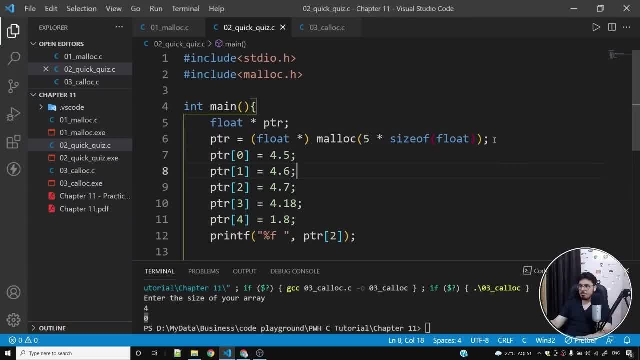 and it will deallocate the memory. Now let me show you this one thing quickly: If I allocate the memory, let me come back to this quick quiz. Let us say I use this free PTR here, So here itself I freed all the memory. 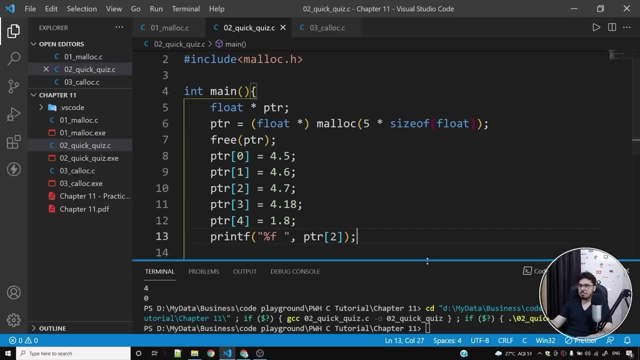 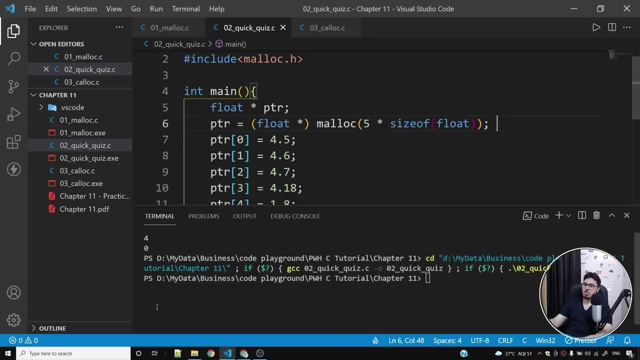 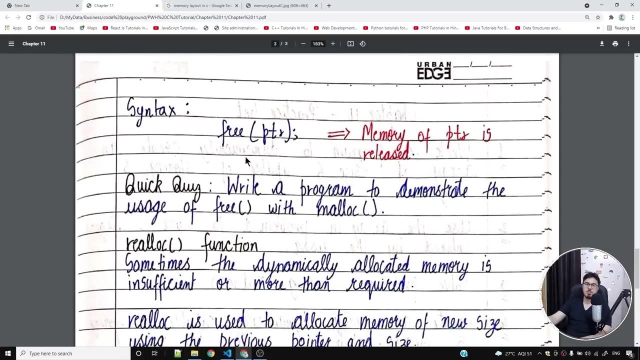 If I run this program, you'll see that nothing is printed. So this thing is free. This thing is not printing anything because I've already freed the memory which I was holding. So this was one weird usage of free. You might not want to use free in this way, but again, you can always use free to release. 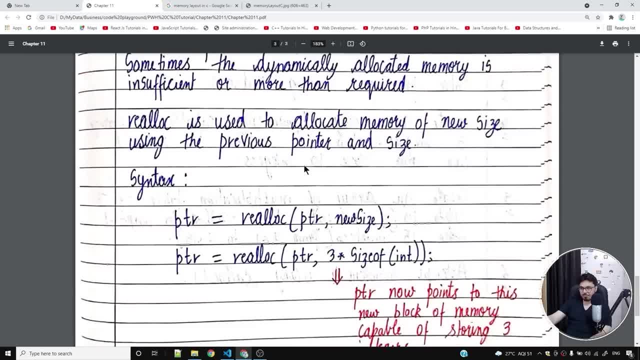 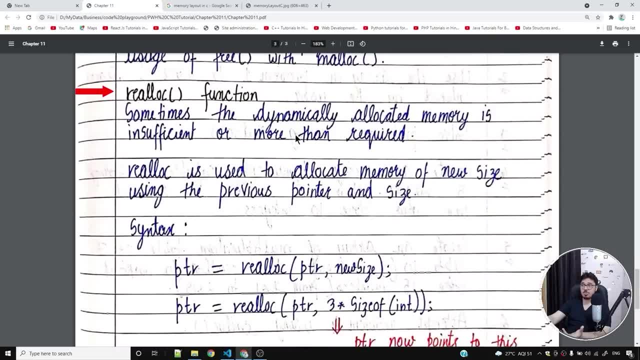 the memory which was held by PTR. Now, the last function is realloc, and it is also really very important because sometimes the dynamically allocated memory is insufficient or more than required. So you might want to reallocate using the realloc function. Realloc is used to allocate memory automatically. 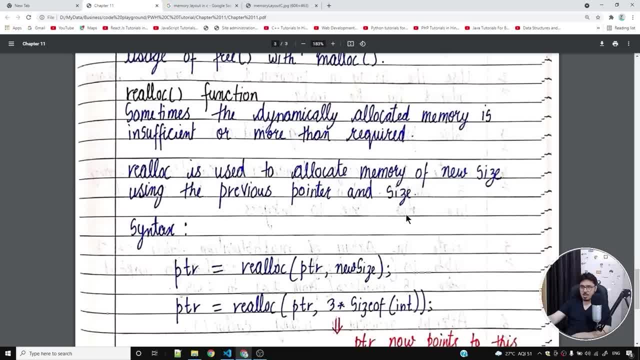 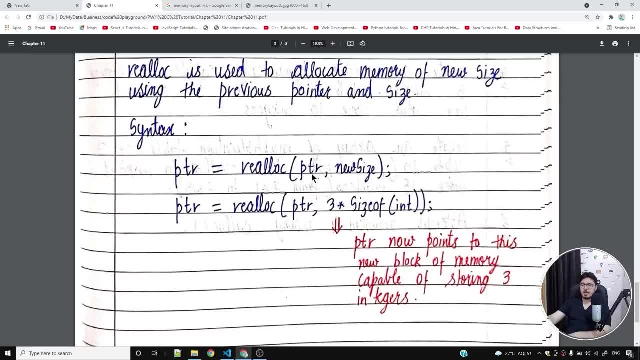 It is used to allocate memory of new size using the previous pointer, int size. So let us say you were having PTR and it was holding, say, four integers, and now you want PTR and you want 30 integers. You can always use realloc and realloc will give you new memory of your desired size. 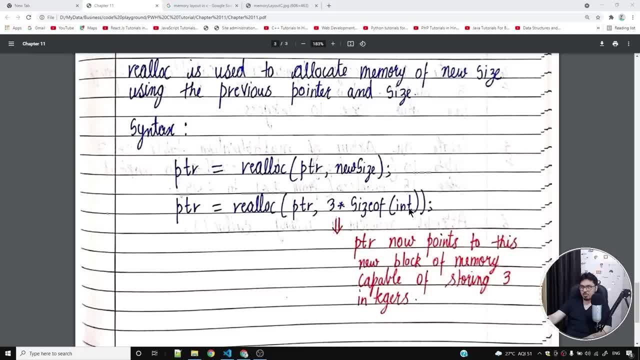 Okay, so PTR is equal to realloc. PTR, three into size of int, will give me a new pointer which is capable of holding three integers. So PTR now points to this new block of memory: It is capable of storing three integers. So this is how a realloc works. 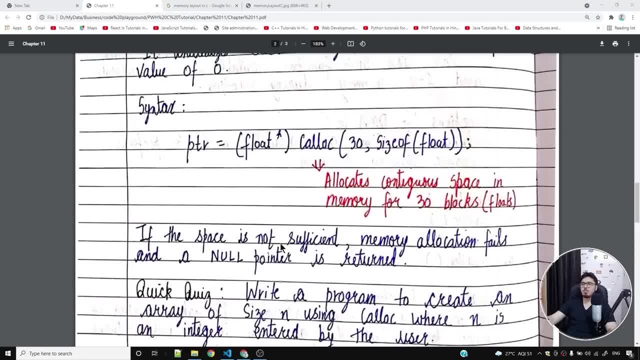 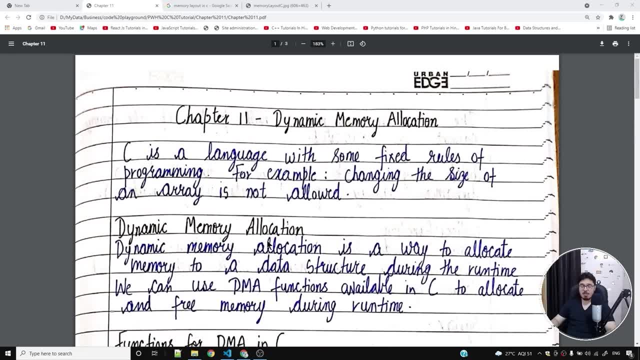 I have written all the syntax in the nodes. I hope that you like this dynamic memory allocation concept. Now you might want to dive deeper into dynamic memory allocation by writing programs on your own. So practice as much as possible and as hard as possible. 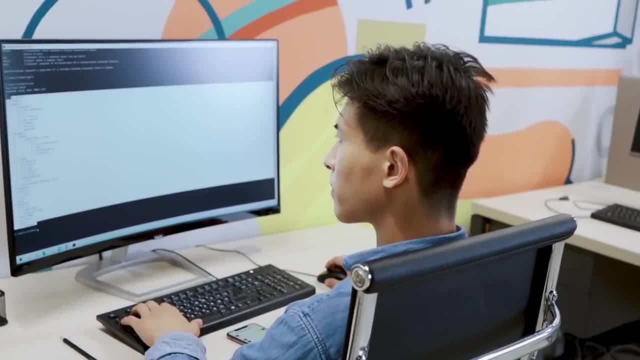 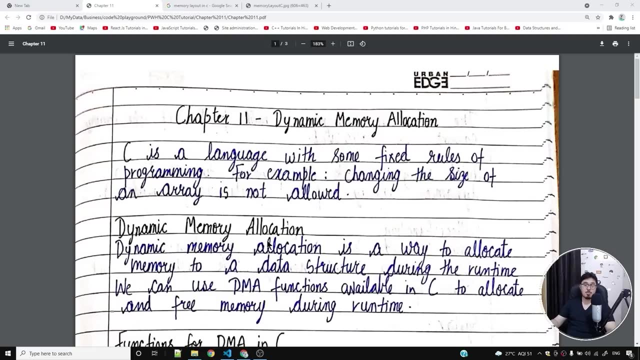 You will definitely get this concept. Sometimes it is really very hard to grasp for beginners the concept of stack, concept of heap And how a memory layout in a program in C looks like. Now we will see how this works, Thank you. so i want all of you to search on the internet about the memory layout of c programs, how memory 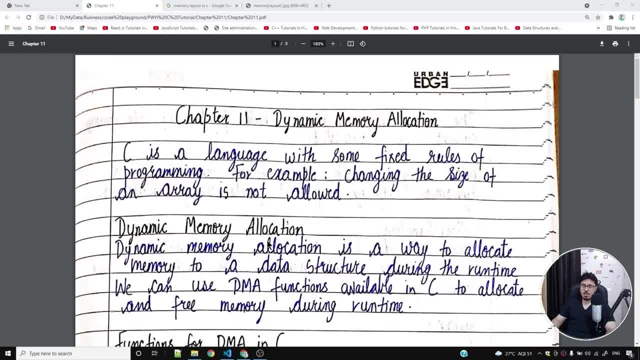 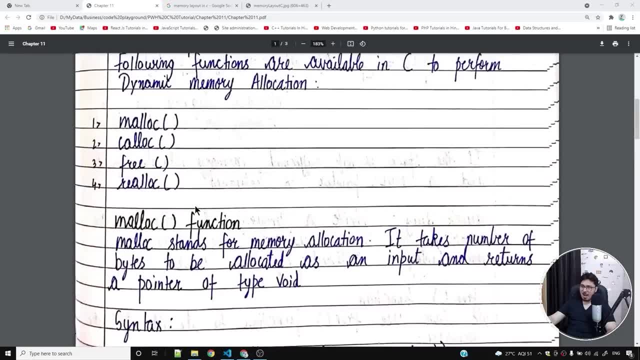 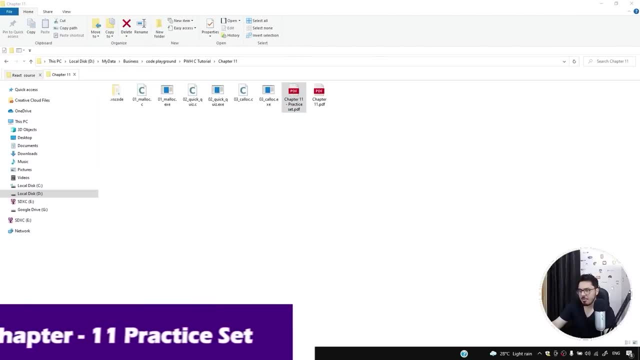 layout of c program looks like and then from there you can definitely understand how dynamic memory works. in order to add to our understanding, we will solve practice set from chapter 11. let's now move on to chapter 11, practice set, and solve some problems. so i'll open this chapter 11 practice. 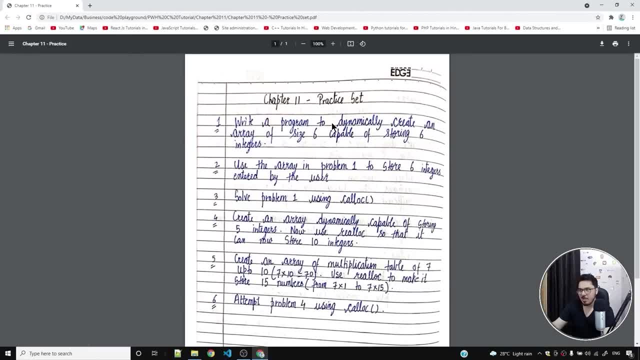 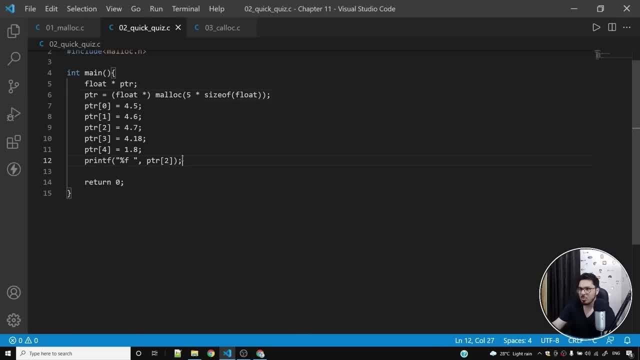 set for you and inside this chapter 11, we are going to solve few questions. so let me open this folder in vs code quickly. so i'll open this folder in code and also, what i'll do is i'll create program for the very first question, because i'm going to solve it no matter what. okay, so we are. 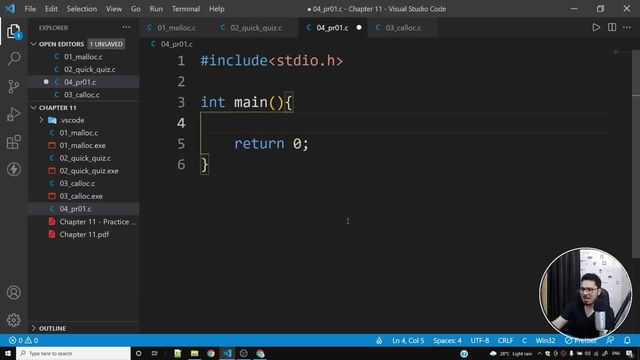 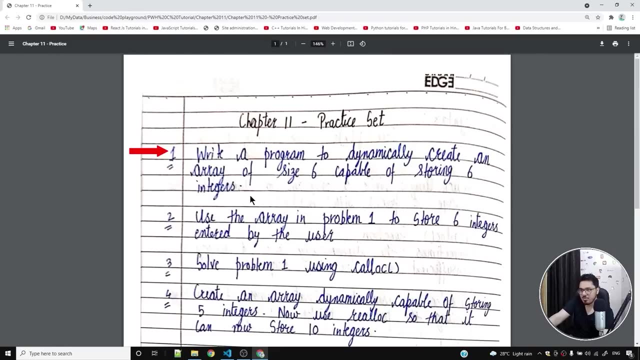 going to solve this problem. i don't even know what the problem is, but i'm going to solve it no matter what it is. so the problem says: write a program to dynamically create an array of size 6 capable of storing 16 teachers. i think i've already done this program. i'll simply use this particular syntax. 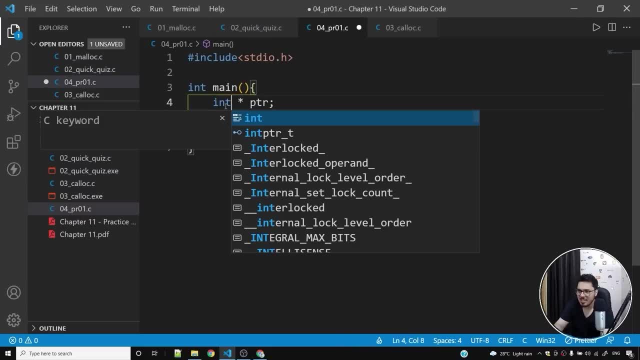 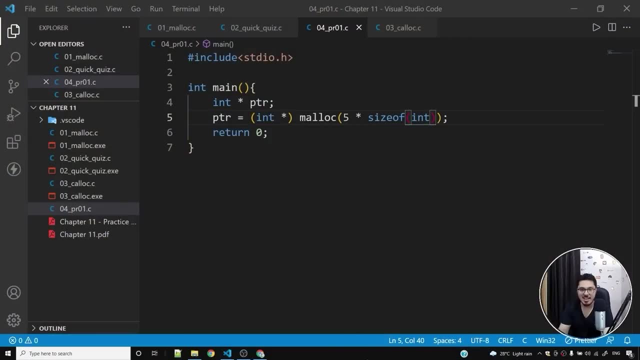 yeah, i am a big fan of copy paste, by the way, and you should be as well. it saves a lot of time. do not copy from others. do not copy with negative intentions, but again, if your intent is right and the code is yours and the code you are copying. 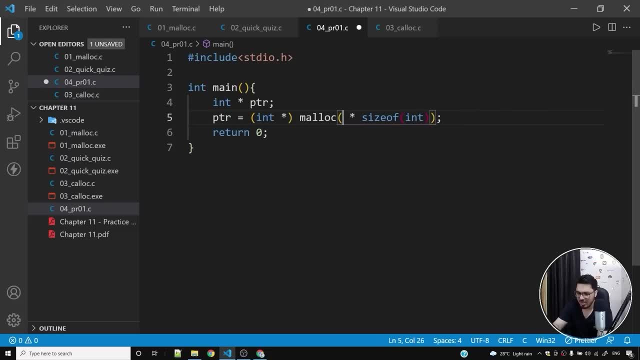 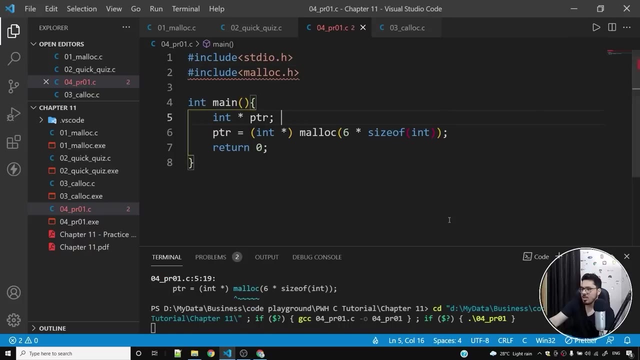 from is yours. you are free to, you are in fact more than free- to copy the code, so i'll simply write six here. i'll simply create this particular program and run it, and this program is capable of storing uh, six integers. i'll include my log dot h, and this time, if i run it, it's not going to run. 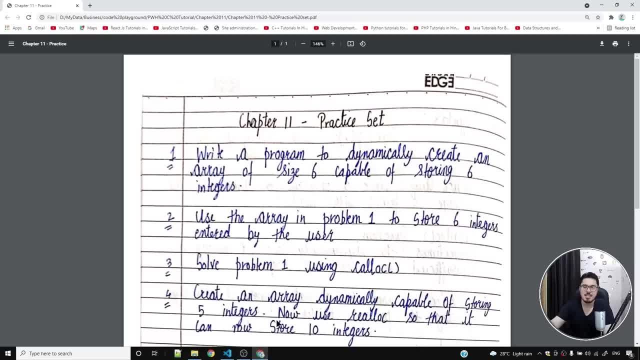 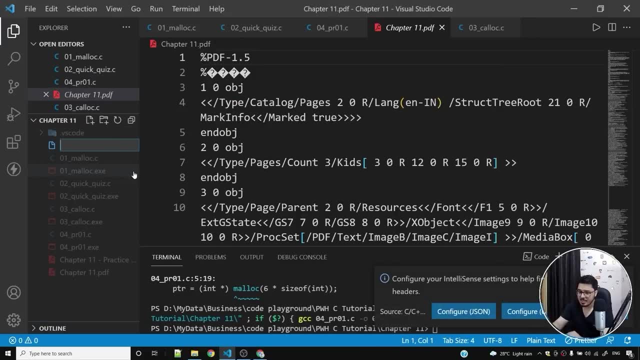 with any errors. i'm not going to get any errors and this is the official solution to this problem. okay, question number two: what does it say? it says: use the array in problem number one to store six integers entered by the user. let's do it. let's do it. so what i'll do is i'll simply write zero. 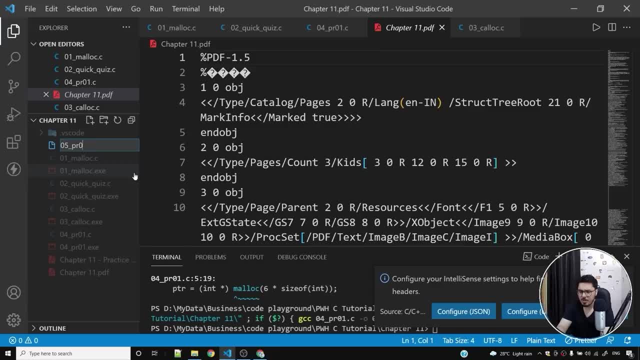 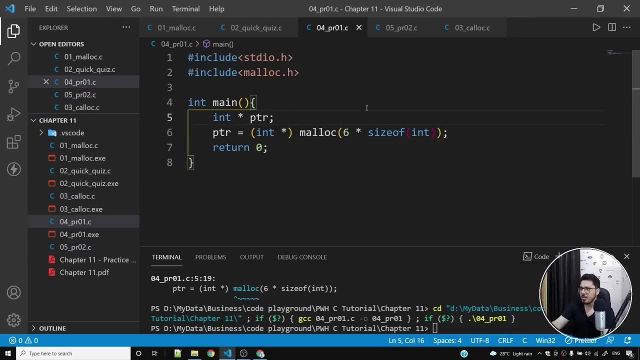 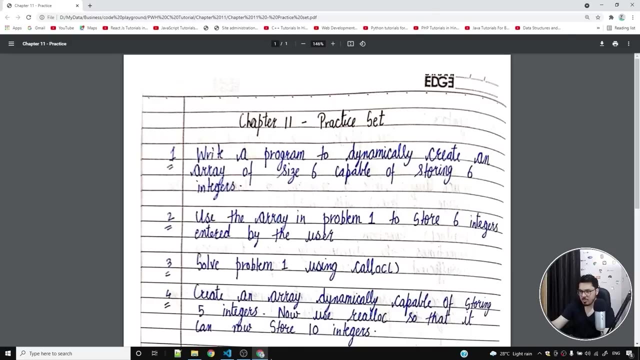 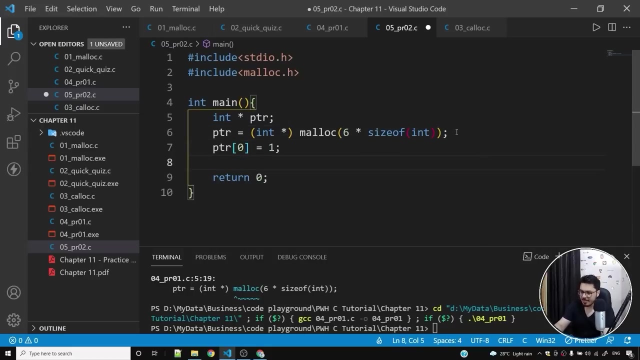 five underscore zero, five underscore ps02.c. and let me close this media file. i don't know why i opened it at the first place. i'll copy this particular code and i'll operate on this. this question says that use the array to store six integers. so how will i do that? i will simply say ptr. zero is equal to say one, and then um, i'll. 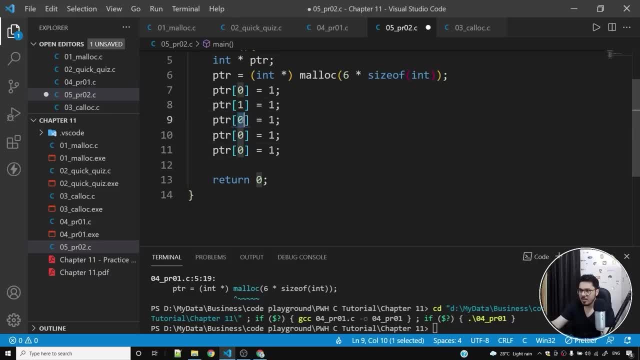 simply use one, two, three, four, five, six, seven, eight. so i'll say one, two, three, four. by the way, i can go only till five because i have to store six integers. and let me give some random numbers here, and i'll give it t8 this time. now let me simply print all these numbers, the value at index, percentage t. 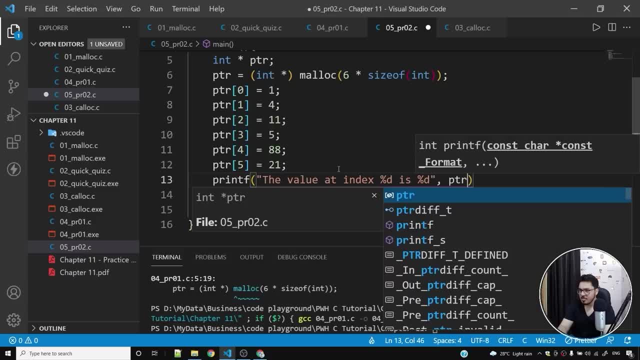 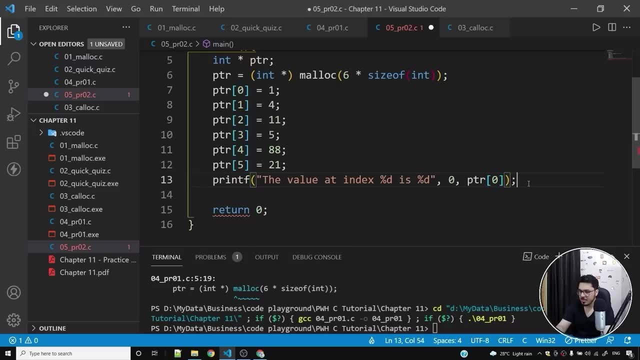 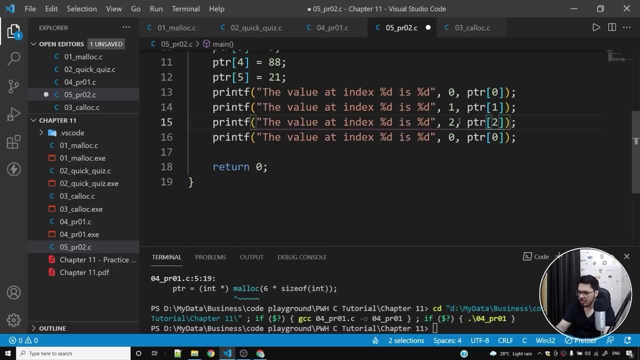 is percentage t. okay, so let's say ptr 0 and this is going to be at index 0. okay, so 0 ptr 0, and i'll do the same for one, two, three, four and so on. so let me do it for one, let me do it for two, then for. 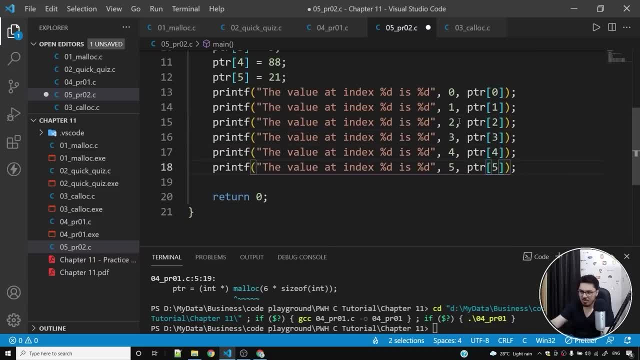 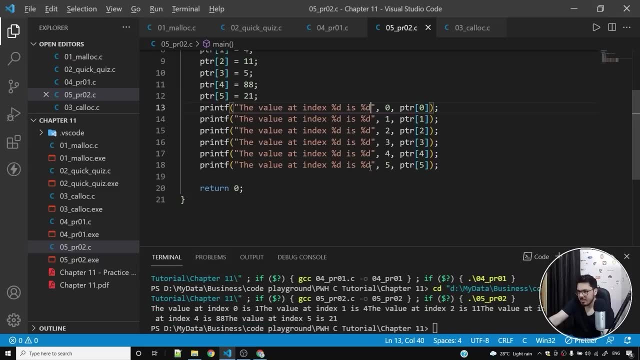 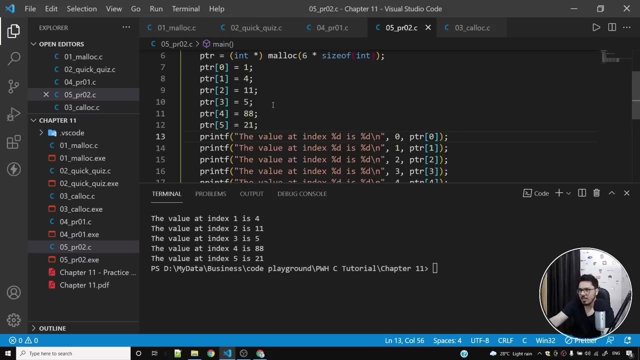 three, then for four, then for five. this is how you quickly edit: uh, anything you want in vs code. okay, oh, my god, i forgot to put these back selections and the output is horrible. so let me put a back selection for all the printf statements and you can see that all the integers i stored are now visible. so at index zero. 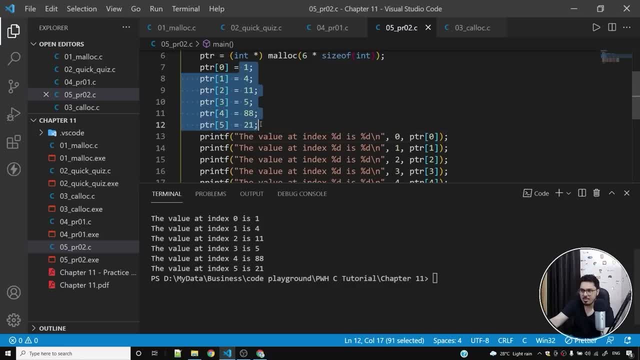 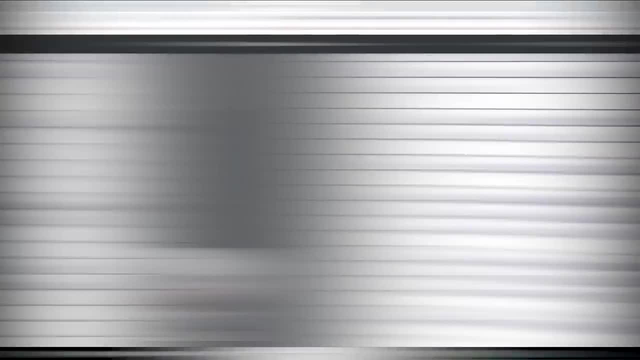 we have one, then four, eleven, five, eighty, eight, twenty one. these are the same numbers which we initially assigned our array with. okay, so i hope that you understood how this thing works. question number three says: solve problem one using kellogg. and yes, you can use kellogg, so kellogg is. 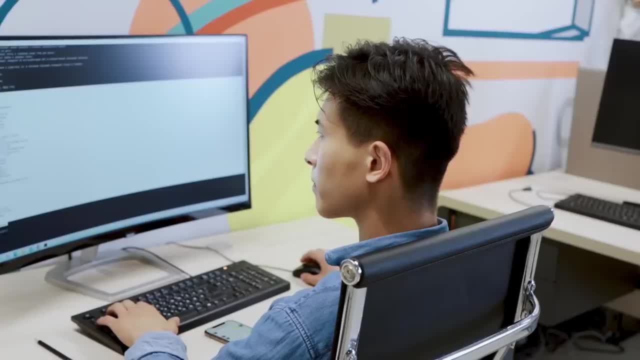 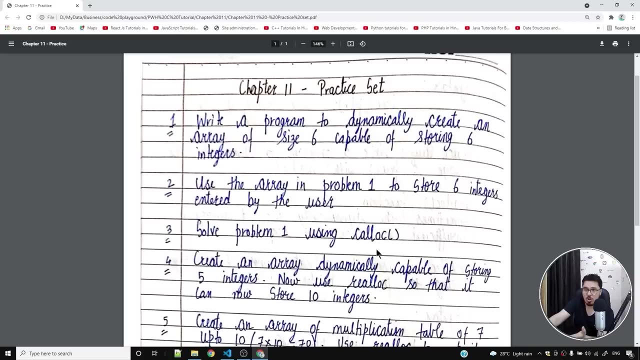 very similar to malloc and you need to. you need to solve it yourself. okay, this is very simple. you just have to change the malloc call to kellogg and just look at the syntax of kellogg from the chapter 11 pdf. it's pretty straightforward. question number four says that create an array. 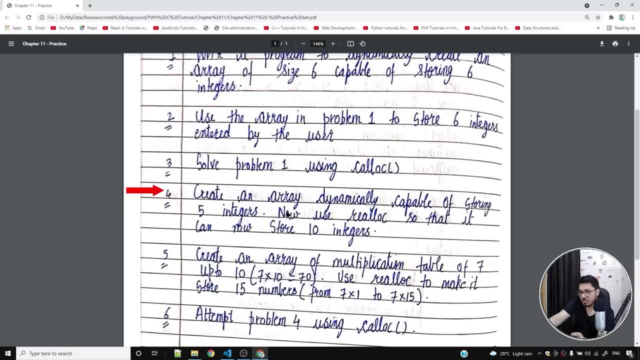 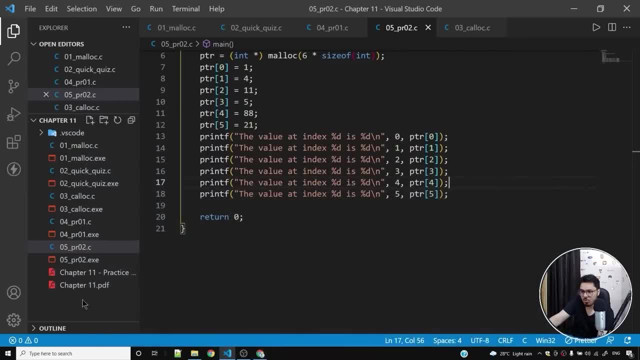 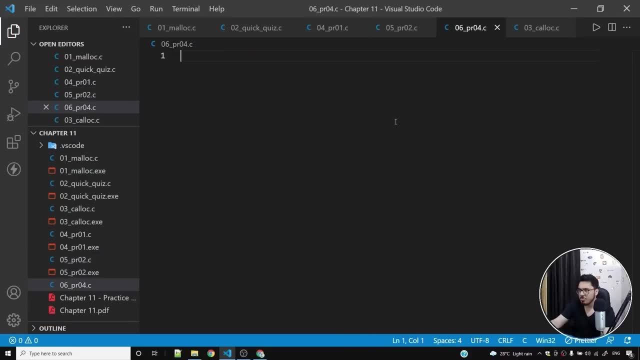 dynamically capable of storing five integers. now use realloc so that it can store 10 integers. we are going to solve this problem. this problem is interesting. this is question number four, so i'll simply say pr04.c, and let me start from this program itself. so initially, this program. 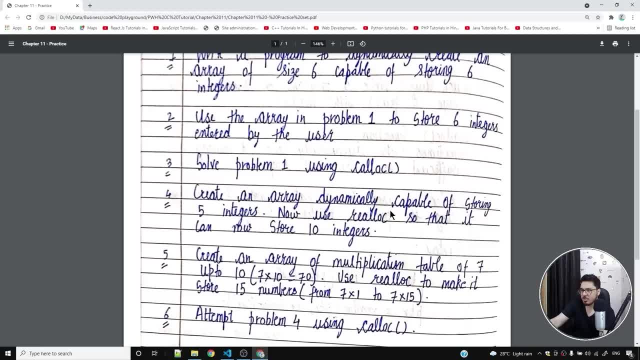 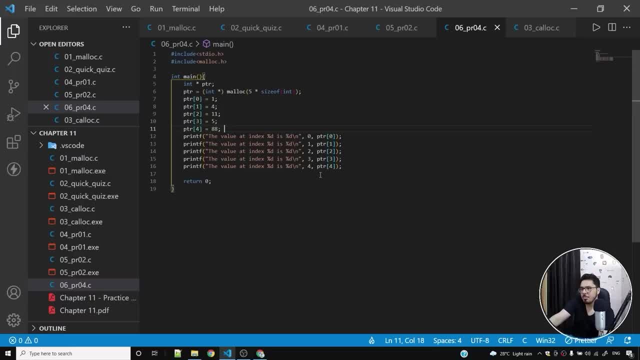 was capable of storing six integers, but my question says that create one which is capable of storing five integers. let me remove the last element from the array. so this is a program which is capable of storing with an array, with a dynamic array capable of storing five integers. now i need to change it to. 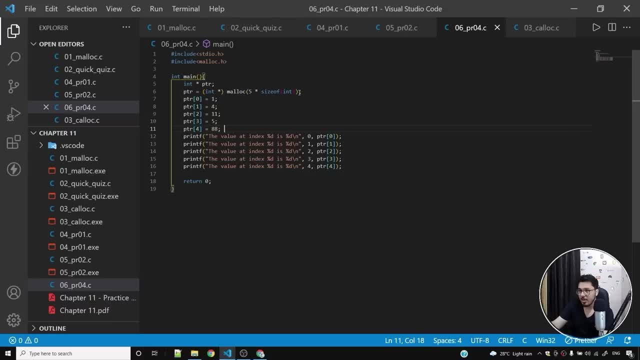 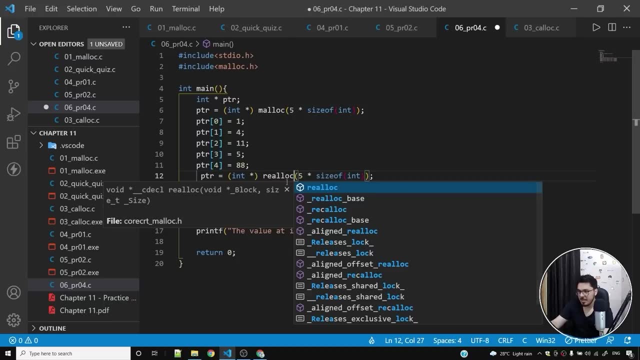 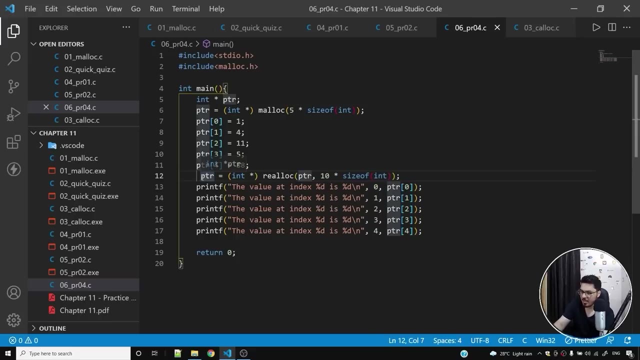 be, you know, able to hold 10 integers. so how will i do that? i'll simply say ptr is equal to, i'll use the realloc and i'll simply say realloc, and then i'll say ptr and new size. what is the new size? new size is 10 multiplied by size of end. now, this array is capable of storing 10 integers. 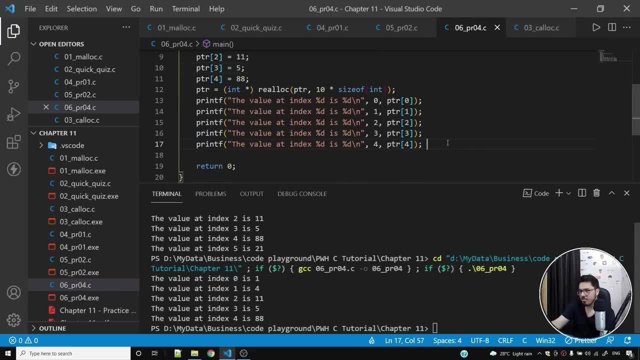 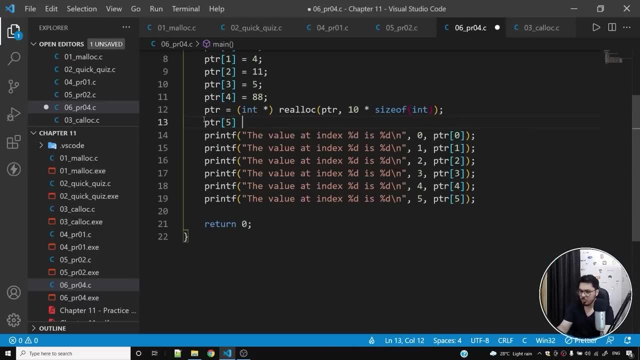 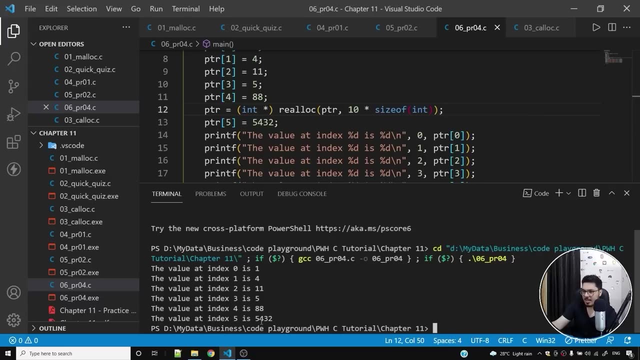 so if i run this program you can see that all these integers are visible. but now i can write ptr4 5 as well. now i'll say ptr5 is equal to, and i'll simply punch in some number and i can print ptr5 here, and if i run this code you'll see that index 5 is 5, 4, 3, 2, so i'm able to store one more integer. 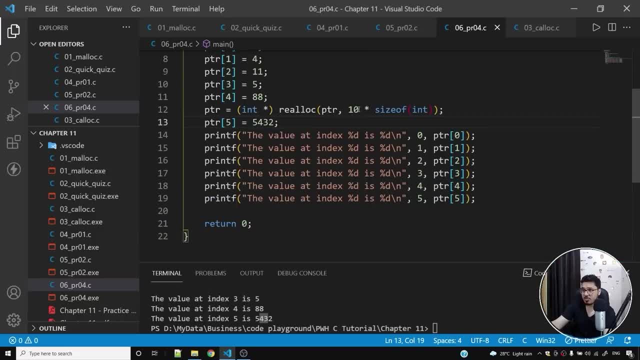 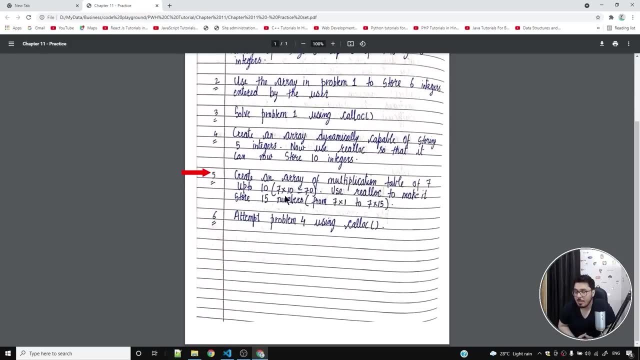 and i can store four more. yeah, this is an array of size 10, so i can store four more. okay, coming back to the practice set, the next question says that create an array of multiplication table of 7 from 10. so you need to start from 1 and you need to create a multiplication table of 7 from 7. 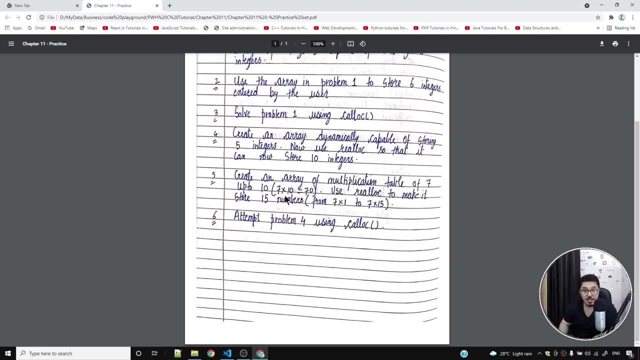 multiply by 1 all the way till 7, multiply by 10, and then you need to use realloc to make it store 15 numbers. so this is a very simple problem of using an array, a dynamic array, of size 10 and then changing its size to 15. we have already done that, so i want you to show some of your creativity. 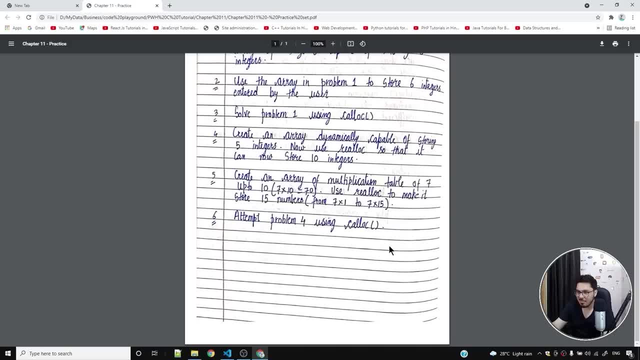 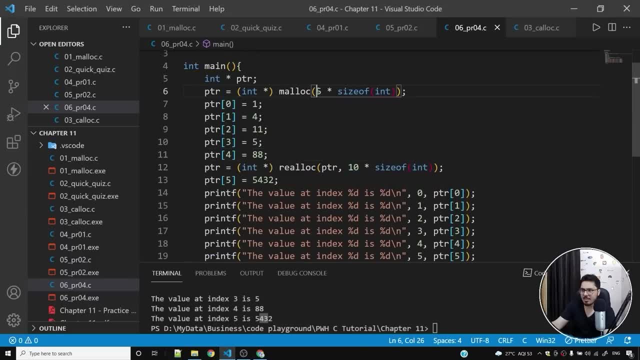 and start writing this code. this is very simple and then once again attempt. problem for using very simple. i just need to change this call to kellogg and when i say kellogg, i'll simply give the number of bytes- sorry, the number of blocks and size per block. okay, so this will. 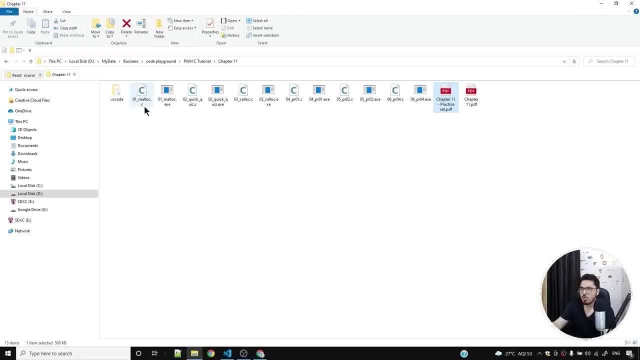 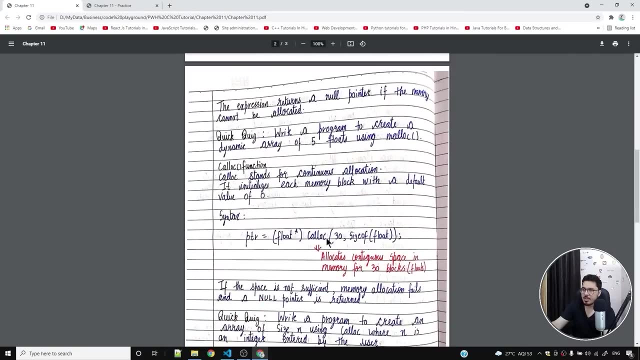 give me continuous memory allocation. i've already told you all this in chapter 11. so, in case you think that all these things are something that you are not able to remember, all the syntax is present inside chapter 11 nodes, so feel free to use chapter 11 nodes. so this ends this c tutorial. 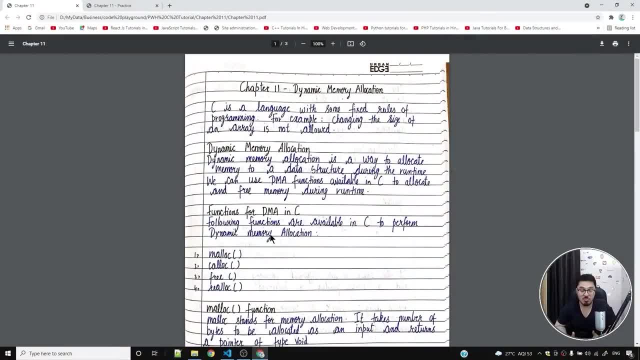 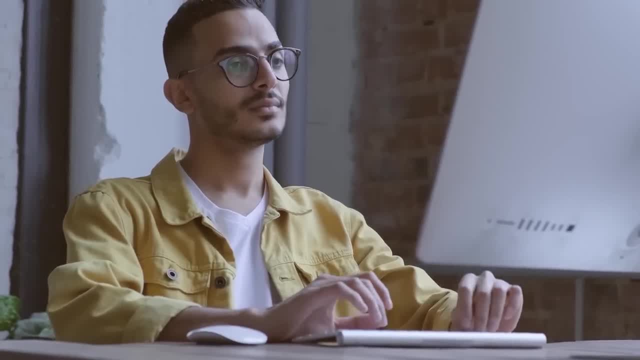 i hope you enjoyed this video. if you did share it with your friends as well, so that they can enjoy this video as well, and i hope that this will add some value to your lives. to your programming carrier, make sure you take the copy of these notes. i'll give all the links in the description, all the 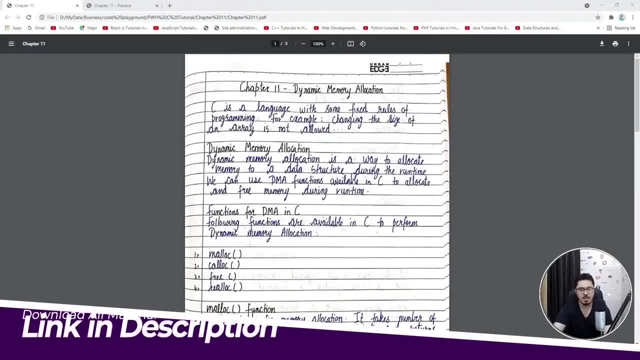 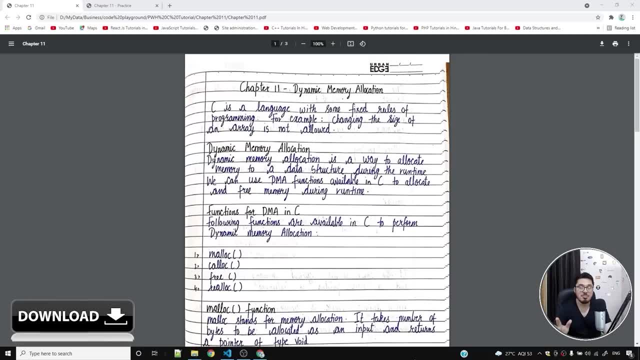 programs, all the source codes, anything that we have done here is completely free, available free. in the description you can get the link and download it. it is absolutely free, no conditions apply. also, if you think i should have done this in chapter 11, you should have done it in chapter 11.